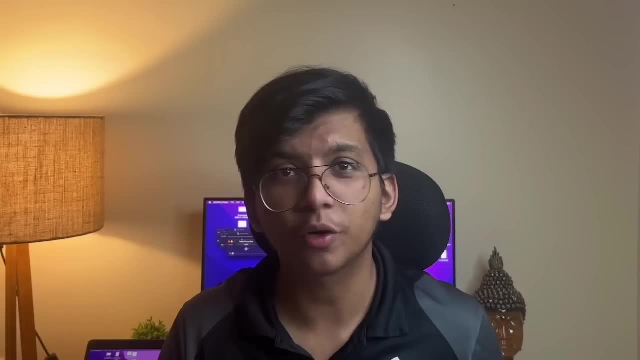 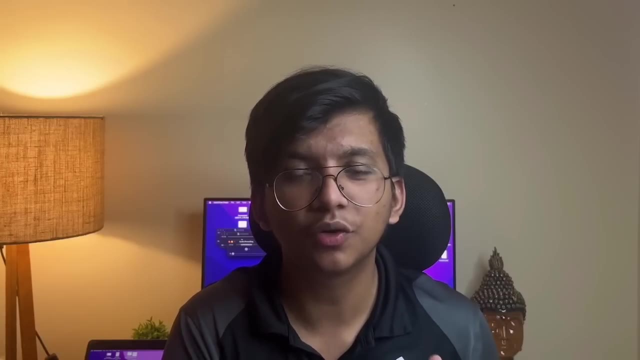 understand it. we talk about what is learning, we talk about generalization, we talk about inductive bias and a lot of things initially, and then we gradually move on regression analysis and we cover as much as we go in depth and to ensure that we are quite equipped with the practical. 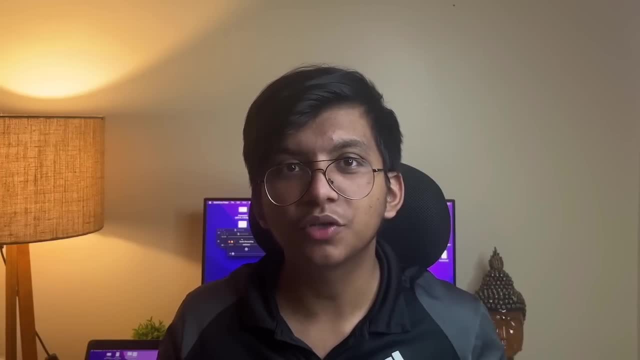 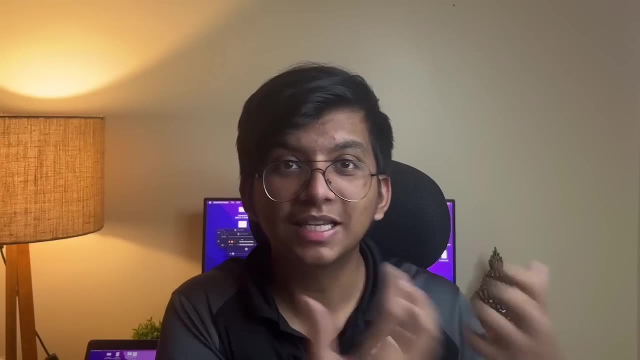 applications as well. i'm going to introduce two projects by the end of the course which you have never seen like that project before as well, because i have worked personally at several companies and i know how we deliver data science process to them, and the same way i'm going to do. 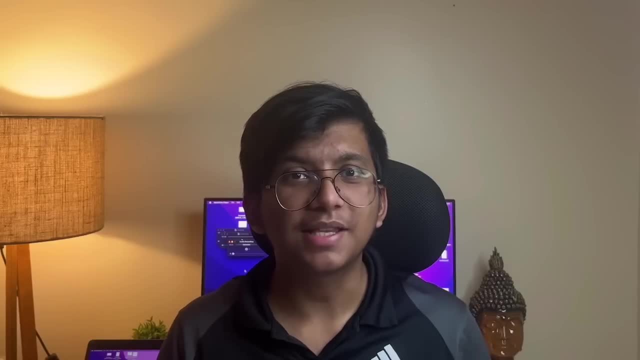 it in this course as well. but that's not all. if you want to maximize your learning opportunity from this course, then we are offering free updates to the course, regular assignments with personalized feedback to you and a tailored learning plan for you to complete this course in just one month. you. 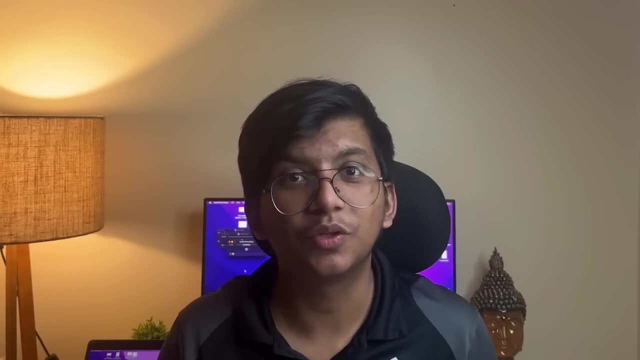 can simply go on a github page for the course and then get access to the elements directly from there, and all of this for absolutely free, one of the major issues which are not highlighted. you asking he was just for expression. most of the instructor takes around only one hour, you're. 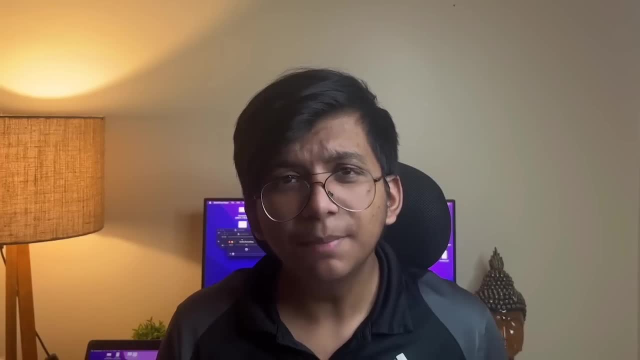 taking freaking so much of hours to teach it. i tell you that people forget the foundation, people forget the basics of it and they just just strictly go for advanced topics like people learning, and then they are not able to secure the job. and then they complain me that he is using data science. 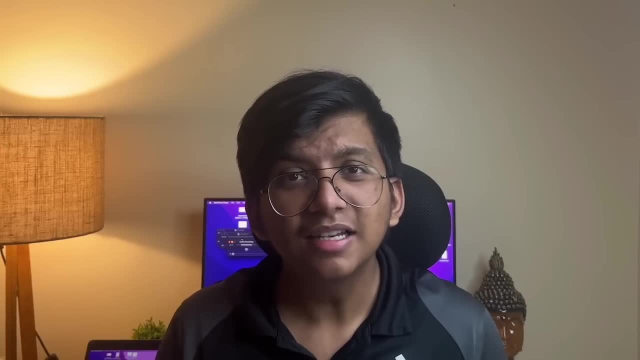 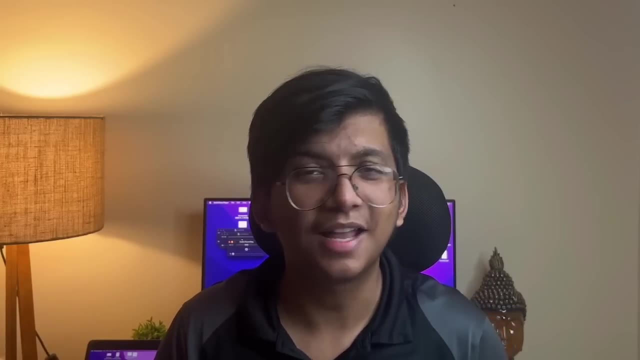 has no jobs. but actually if you think in a way that the talent is less than the actual jobs because they are not going to pay you thousands of dollars for just three lines of code which you write in secular, anyone can do it and crowd is increasing but the talent is decreasing. they're forgetting what's the base of machine. 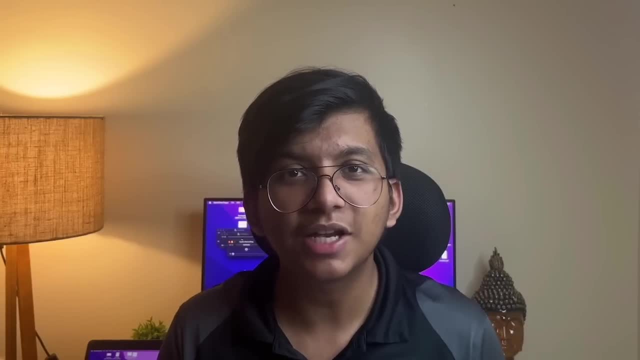 learning. what's the base of data science? they're forgetting the solid foundation which was used to be given in 90s and all. so that's what the course focuses on. we make sure that we emphasize the core concept of machine learning and regression analysis, so that you can even learn further. 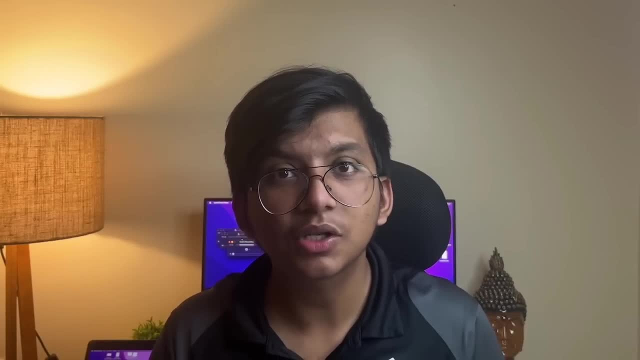 things on your own. our course is designed to put emphasis on core concept of machine learning and regression analysis so that you can tackle critical business problem and solve it the way real data scientists solve. so that's enough of it now let's get started with the course you can. 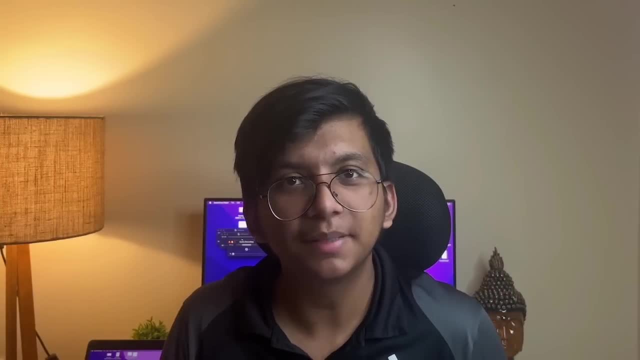 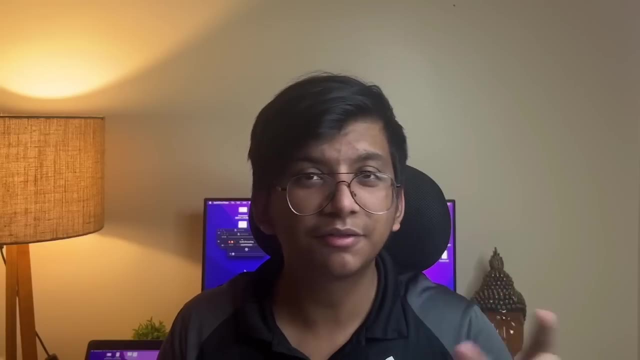 directly go to the lms and then start from there by seeing the tailored learning plan, or you can get started from here. let me know if you have any notes in the comment section and find any errors or errata in this course. please feel free to make an issue on the github page for the course. hey, 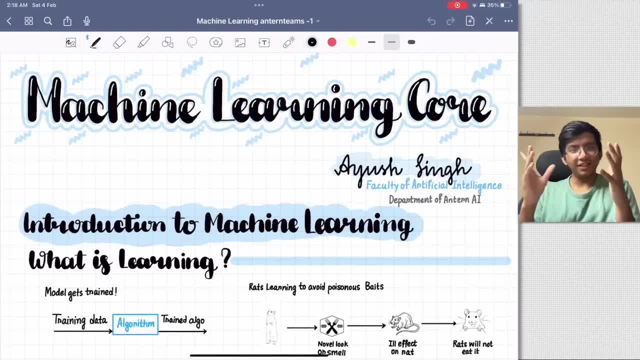 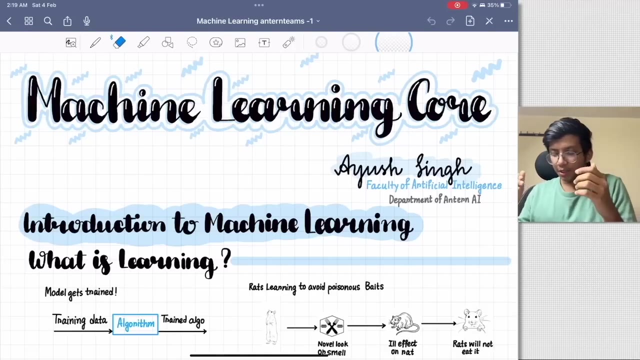 everyone. uh, so let's get started with our machine learning content and actually get started with a bit of discussion on learning the machines, learning intelligence, and give you some of the concepts which is required eventually to build up your ideas, right? so let's get started now. so i would suggest you to open up your notes if you have got it. 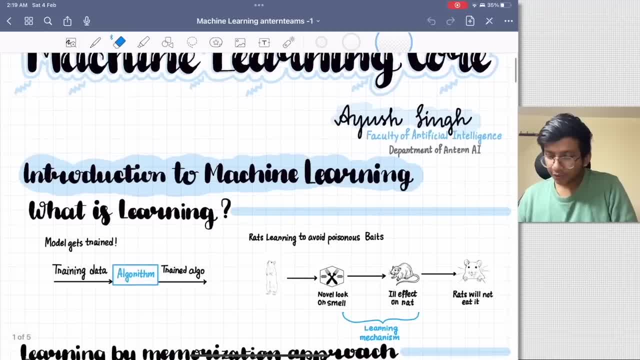 so, once you have the notes that you can see on the front of the screen. so we're going to start off with what is learning, right? so let's eventually talk about what is learning and slowly we'll get into the get on the concepts of you know. uh, very, very good examples. 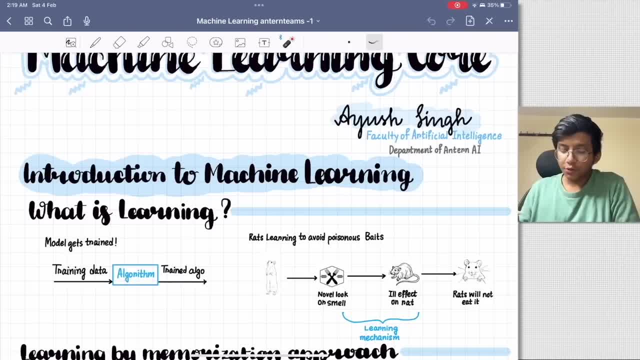 of learning and intelligence and etc. so the first one is that: what is learning? so i suggest you to write your answer in the comment box, if you know. so, according to what exactly, uh, what exactly you know about in terms of machine learning? we have the training data. we take some sort of you know. 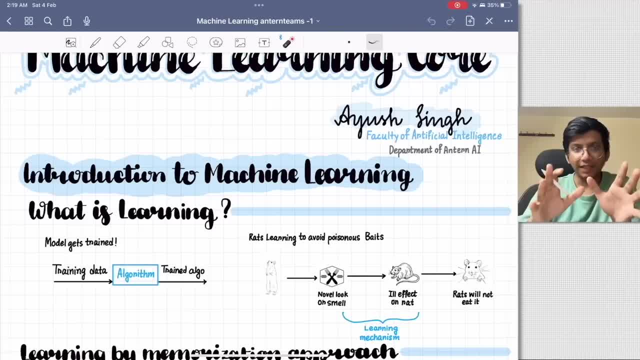 um, the data. don't worry what data looks like and everything, we'll cover that. so we have the data right and then we feed to a sort of a black box and then we get a trained algo that is trained on that data, for example. assume that you. 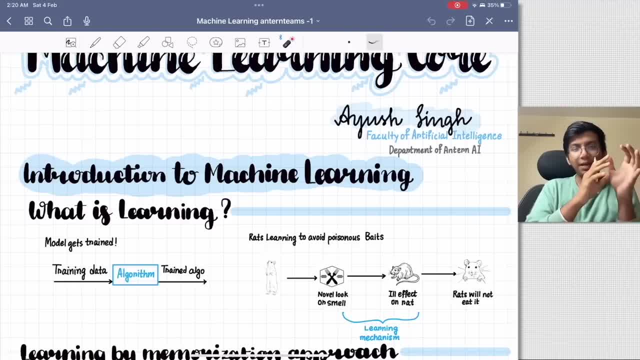 have a man right, you trained that man with that particular skill and then whatever output, after six or seven months you will be getting a trained man specialized in that skill right. so this is how your model mode model gets trained. your model gets the data, gets the training from the data and then 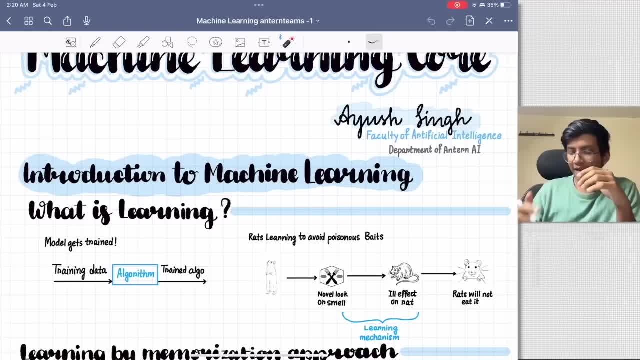 get it. it gets trained by some instructor, right? i'll assume that in this case, it's an algorithm. after, after, after some time, we get a trained algorithm right that, in terms of very simple or- and very you know- mind understanding behind any algorithm. but let's talk about a very nice. 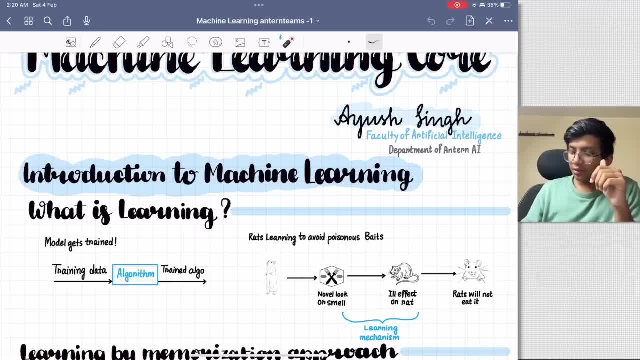 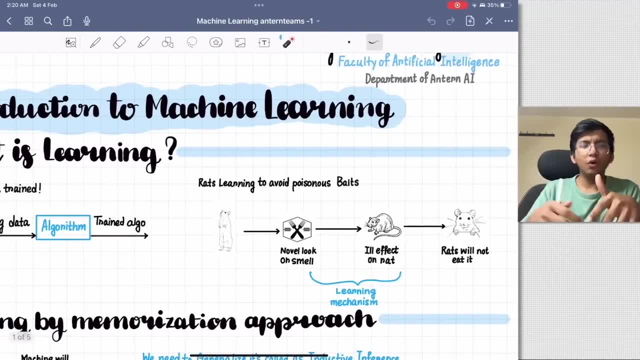 example, very nice example- which is called, which is known as rats learning to avoid poisonous baits. so what is baits? baits are some sort of- you know, food or etc. so the formal definition of baits is that it is. it is some sort of you know, it is a type of prey that is used to attract when 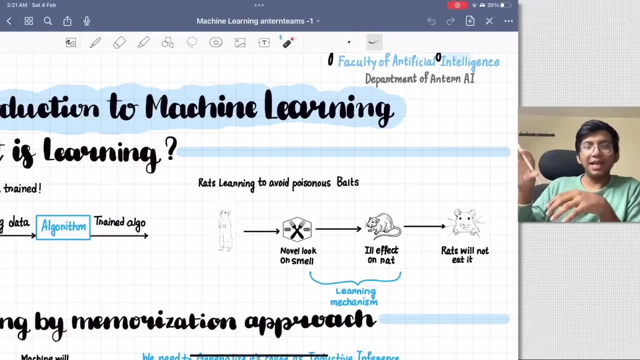 hunting. so sometimes you, we use that baits to attract you know poisonous thing. yeah, it is a poisonous thing that used to attract food, right, sorry, a mouse is, or any, any other things, whatever, for example fish. we also have the baits right. so in this way we have the bait. so basically the 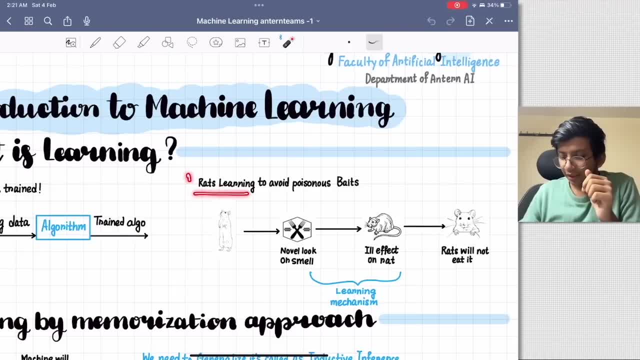 problem statement. the problem statement is that the rats are learning to avoid the poisonous baits. so how do lads rats learn to avoid that poisonous baits, right? so rats assume that rat came, and then assume that rat came, a rat came and that, and then they. 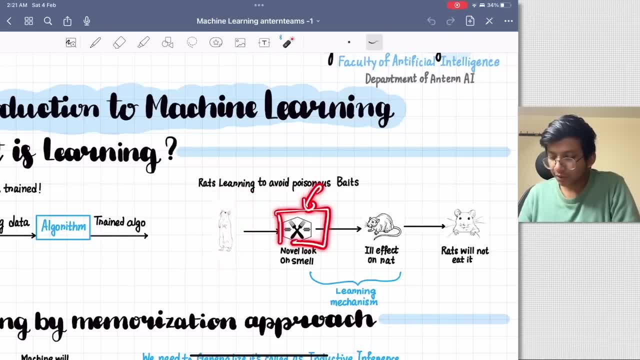 given a known they. there was a food available where this was a bait. this was a bait, right, so it gone, they gone, and then they- it was like smelling good and etc. rat ate, rat ate this food, rat ate this and there's an l effect on that game. right, there's an ill effect of that game. there's an effect of rat game when. 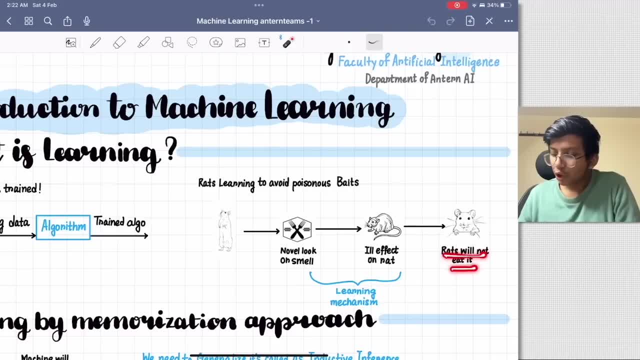 they eat this food and and then rats will not eat this food, because this is, this is the learning mechanism which happened right now, where where, according to the past experience, according to history or the mistakes in the in in the past, this rat did and he's not on, rats will no more. 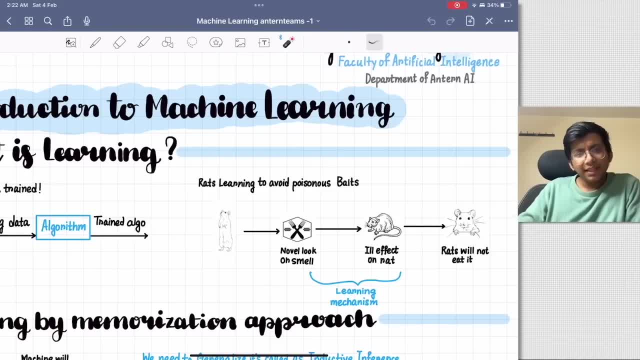 going to repeat this step again. this is one sort of a learning mechanism. another learning mechanism which you can think of is: assume that you, you have done some sort of mistake in your past. or a very simple example: assume that, uh, you go for someone for guidance, right, why? why they are capable of. 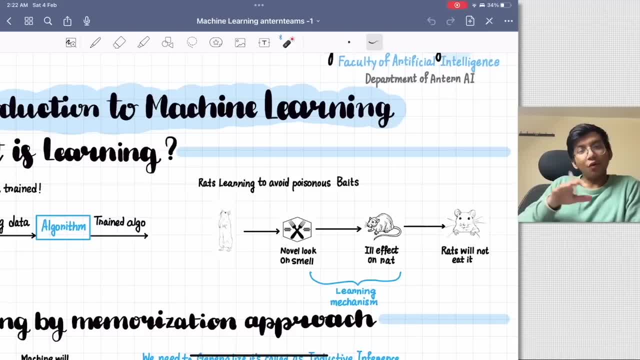 giving guidance because they have gone through the problems. they have already gone through the problems. so you go to them so that you get an easy path, so that you get an easy uh guidance from them so to achieve something in your career, right? so in that way i'm saying that they already have an experience of something. now they 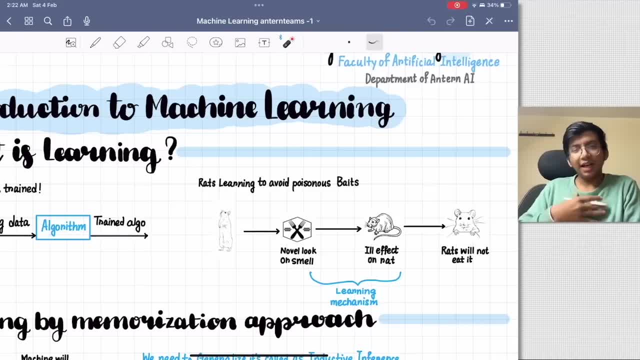 are capable of you to guide right, just like i do. i guide so many people right, so we, i guide so so many of folks right now. so i am capable because i've already gone through those problems. now i'm capable because of my past experiences. so whole point to take out right now i have learned what 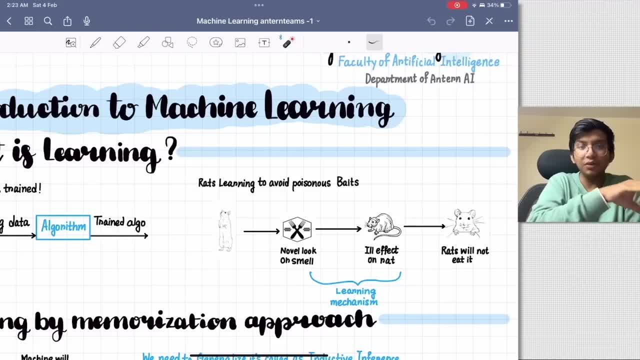 mistakes i, what mistakes and what things i did that leaded me to success and failure. right, that i've i've actually learned that. so, um, eventually learned that. so now that's a learning mechanism. for example, i'm you know more about this because i've you learned that, before you know you, you study some maths. 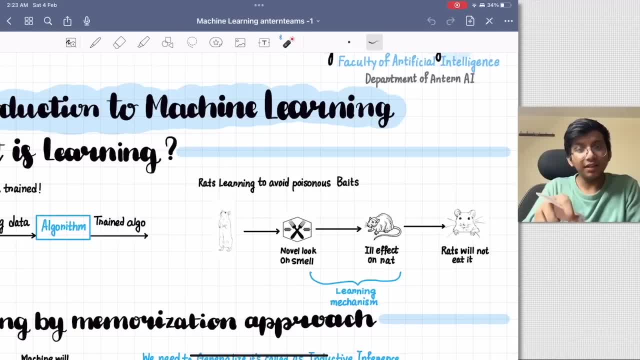 concept and not your computer equations or maybe some calculus concept. so when you study that, when you study that, um, what eventually happens is that, uh, you, you take a look at the particular concept. and once you take a look at the particular concept, now you understand with the help of examples, and then 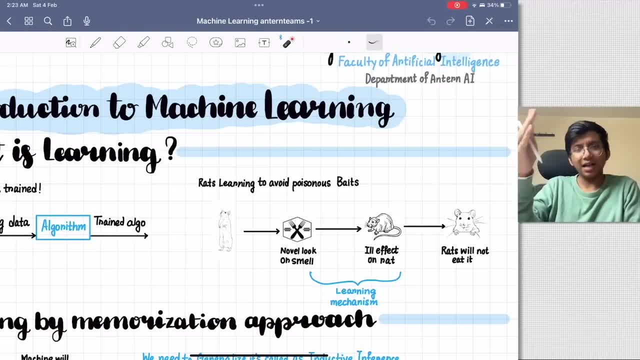 Then you solve the problems. so we said we handle also time, stad tickets rolling on and uh, uh, based on the ask, ask for help or see the solution. but when you uh but, but when you solve similar questions, you will be able, you, you will be able to answer that. why? because you have learned from the past. 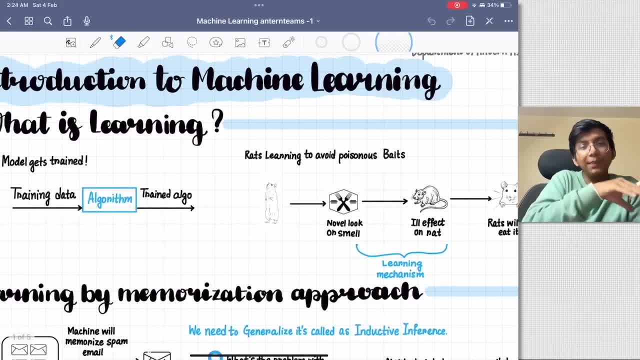 mistakes which you did right, because you are not going to repeat the mistakes which you did in the past, even while solving problems. sometimes it happens as well. sometimes it does not right, so you, you look, that's for the learning mechanism. that's why we say the failure is a part of success. 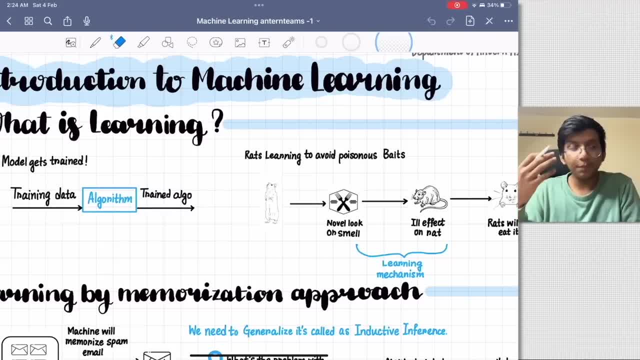 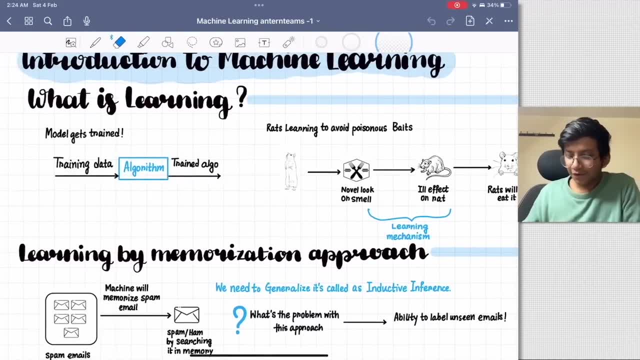 because it gives you the learning phases, the learning opportunities to actually go to grow forward. right, so there are several types of approaches which we go through. the first approach is learning by memorization approach. so this is something is very interesting, uh, where we we say, in in the language it's ratification and in ratification what? what we do, we memorize things. 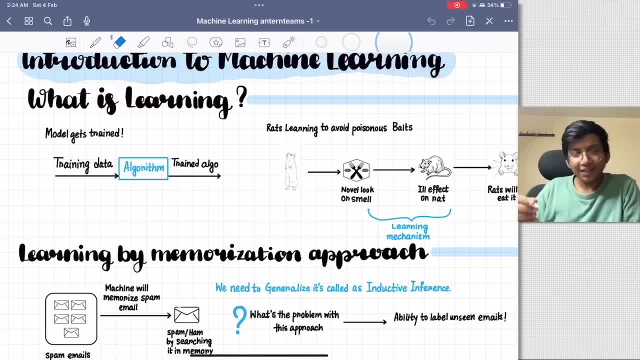 whatever we we, we, we want to study. so for example, i've seen students to literally memorize. you know science answers, sst answers, even computer science answers, because they literally memorize code and they just go and write in the sheet of paper in and then they they memorize literally like 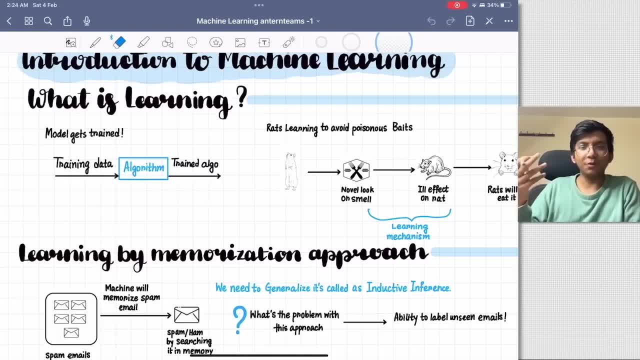 even mathematical questions. however, it's so obvious that they will not will perform well. but but but over here. assume that if you memorize each and every concern, each and every line of your answers, will you be able to perform good in examination. so even if one line you forget, 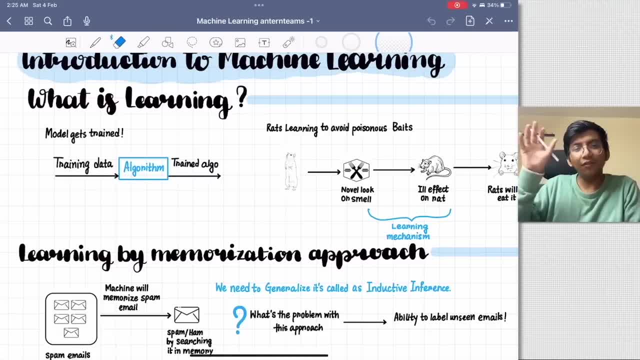 you'll mess up with all the answers. you'll start integrating first answer to second answer, answer to first right. so you have to apply so over here. memorization literally fails in your daily life. you cannot literally memorize everything and then go and sit in examination and you expect. 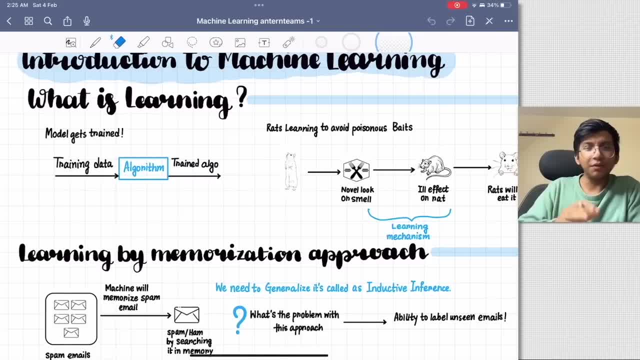 that you'll score good it. it works till class six or seven, but it does doesn't work when you actually grow right. so you can not, can't- literally memorize each and everything, whether it be answers, whether it be mathematical solutions or literally anything. so i hope that get that. 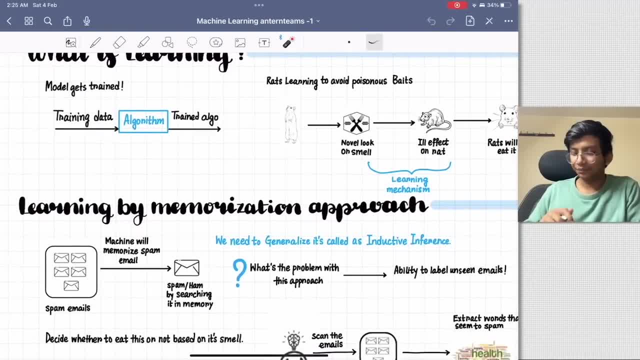 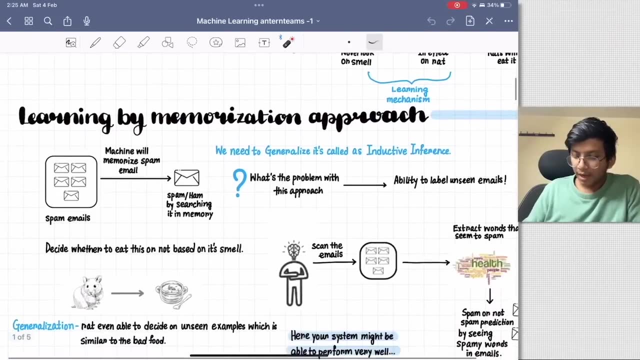 given a good sense about what exactly i want to talk on is, um learning by memorization approach. where we memorize, we learn some things by memorizing, uh, that sort of thing. right, so now. so, now, what i so, now what? what exactly i'm going to do is talk about some of the uh examples which 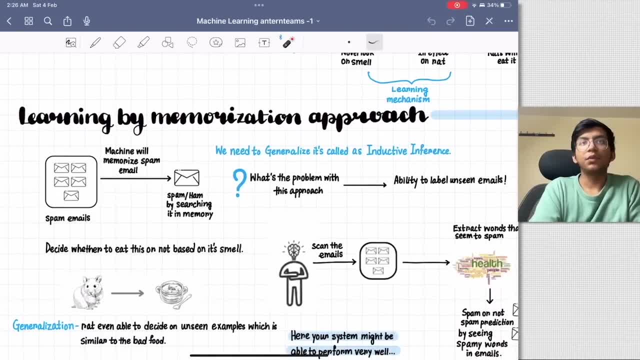 we have listed out here for you to better understand things. cool, so assume that you have you. you have a, you want to build a system. so you might have seen in your email, you know uh, gmail, where you, where you have several folders- promotions folder, social folder, spam folders- and it's an. 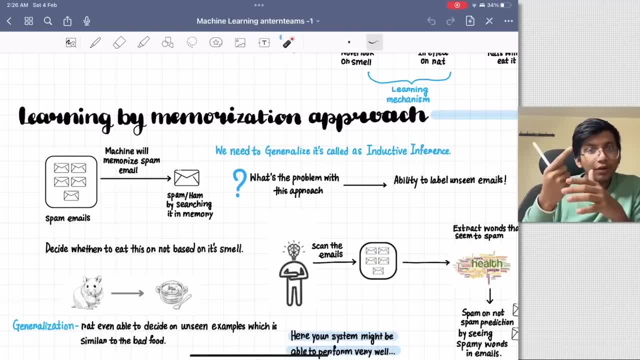 updates folder, etc. so you have these folders and there's one folder called spam, where all your spam goes in, right, where all the spam goes in. so what are, what are those spams? right, that's question. that's a question. so now, now we're gonna build a system, you're gonna build a system, you're gonna. 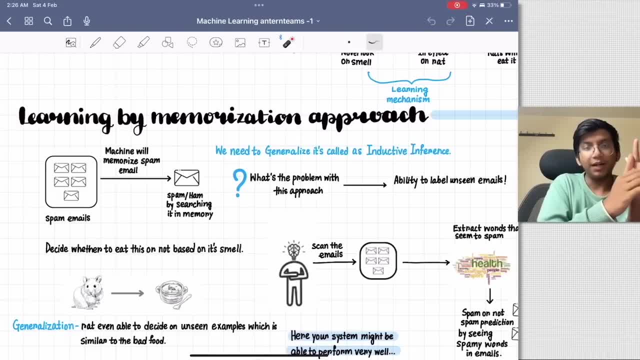 build a system that, given the past data right. first of all, if if you're learning something to identify your spam, you need to have the data. you need to have the amount of data you need to. you need to have the. you need to have some some sort of you know content to understand from right. 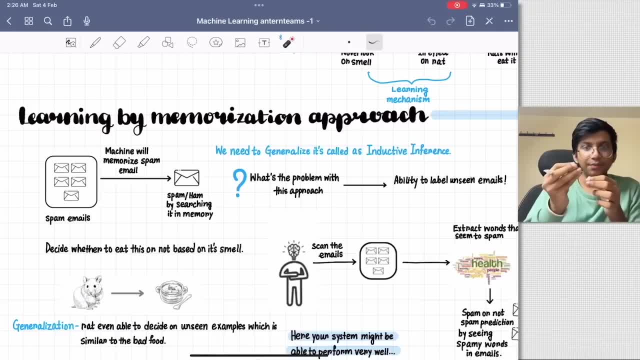 so, in this case, if you want to build a system, you'll build a system that, given an email, given an email, it classifies that email is a spam or not spam. okay, and given an email, it classifies whether that email is spam or not spam. right. so now that's a question, right, so you, you, so now. 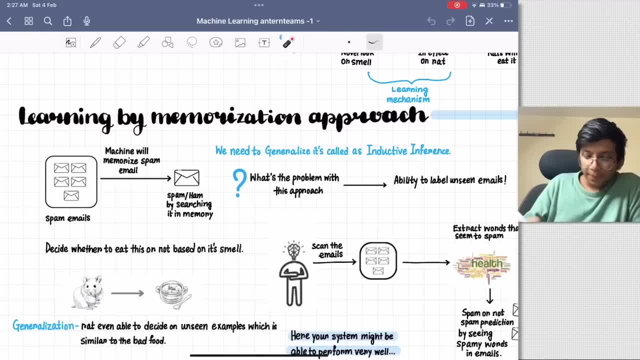 what you so now what you will do is that the first step is: for anything, for learning, literally anything- you need content for this, so we need the data for it, right? so we are. we are going to collect the, collect the email, collect, collect, collect the data. um, we want to collect the data which is. 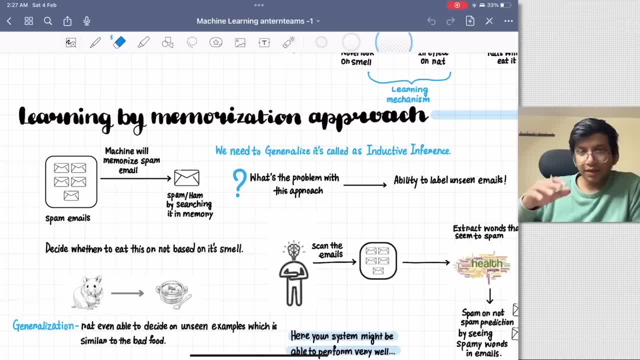 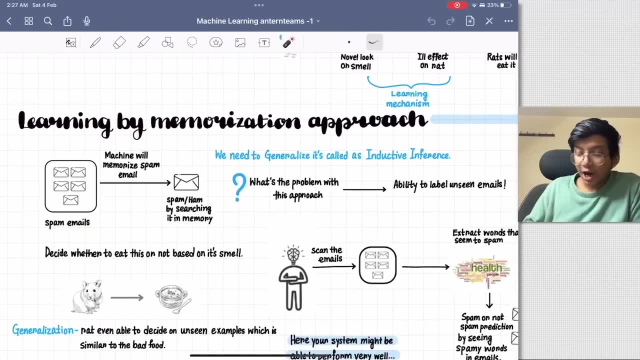 where, where we have the spam emails right. so we will collect the data which is spam emails out here. so we collected the data which is spam emails out here now, now we have the content, now we are. now we want our machine to learn from the data, so we are going to collect the data which is spam. 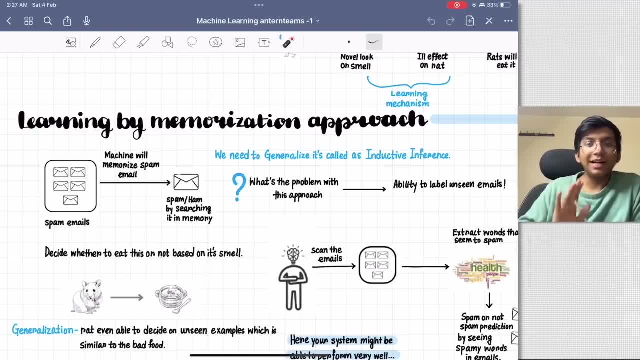 now we have the content. now we are. now we want our machine to learn from the data. so we are going to this content. so there will be two types of guys. first, who will memorize this, so the four. we'll talk with the first guy. the first guy will mem, who will memorize this, will memorize each and every. 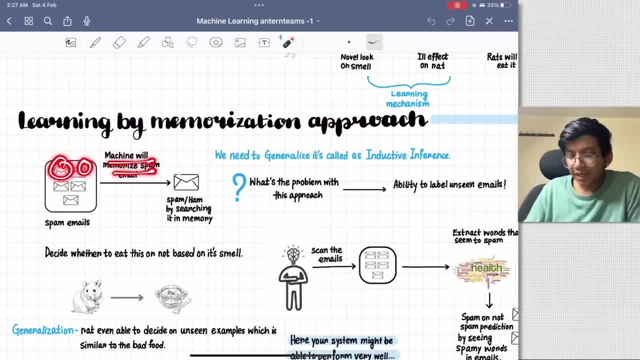 email, each and every email, so machine will memorize each and every spam email. right, and now, now your, now that machine is it capable? now, with that machine is, even if, if that is 100 correct, even if that memorized a very hundred percent correctly, right, so machine will be able to class, will be. 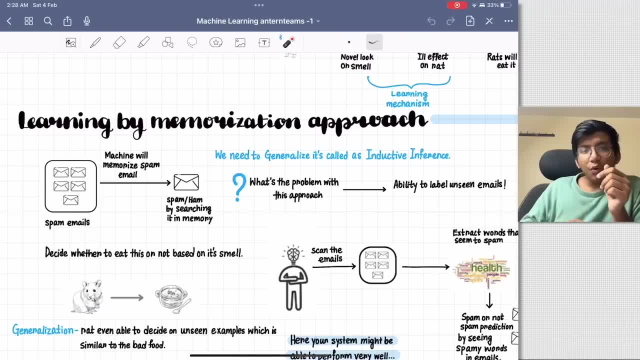 will be able to memorize each and everything. now, if our an email comes, a email comes to this machine, and now this a machine is stored to classify this email to be as a spam or to be as a not spam. right whether that email is a spam or not spam. so you got a new email and you classify it. so how? machine? 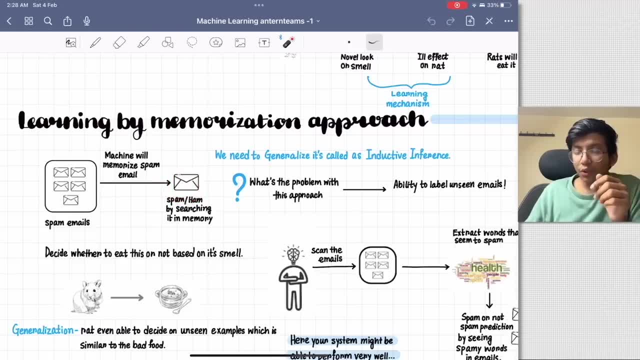 will classify machine, will search this email into its memory, whether this email is available into into its memory or not, right? whether the words of this email is available to in in my memory or not, right? but if not, then we say that it is non-spam. but because the data is, but because the the content. 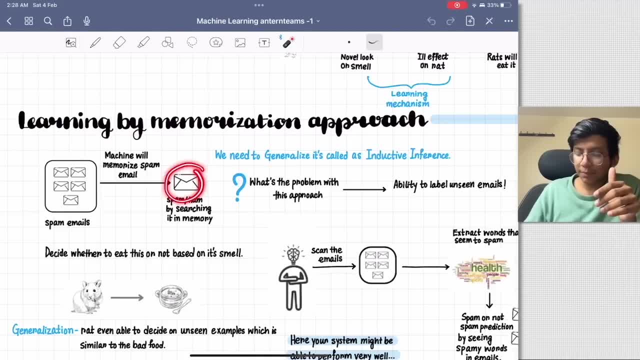 which we learned is about spam, right? so if the, if this is not available in that content, in his memory, what he, what the model has memorized from the data, then he, then the model, will be able to say that it is non-spam. but if that email is available, then it will be a spam. so what's the? 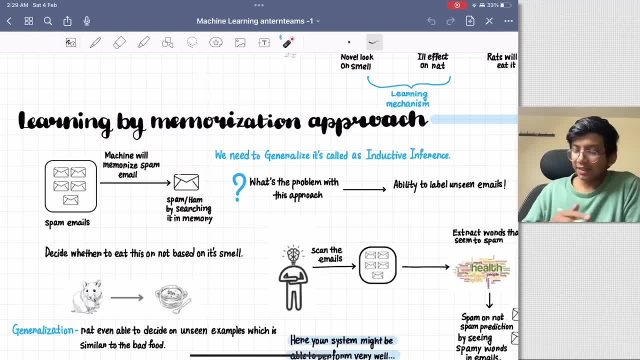 problem with this approach. what's the problem with this approach? right, that's a good question. what exactly the problem with this approach? that's a good question. to actually go forward to the problem with this approach. the problem with this approach? it is not generalizable. so why it? 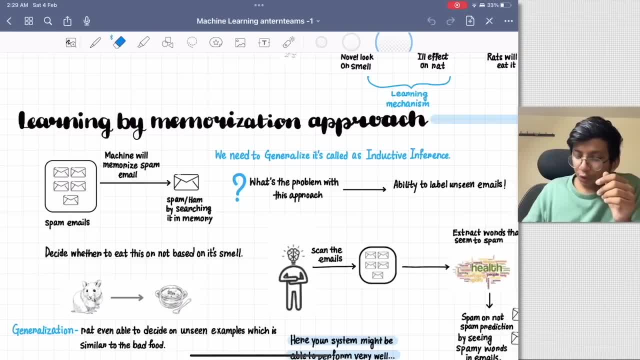 is not generalizable. so let's talk about a very instance. example: assume that you have got a new email, you, you've got a completely new email which, where your model has not, uh, you know, memorized- for example, you sat in your math, mathematics. uh, let's say science examination, you got your questions, which was in a textbook which you. 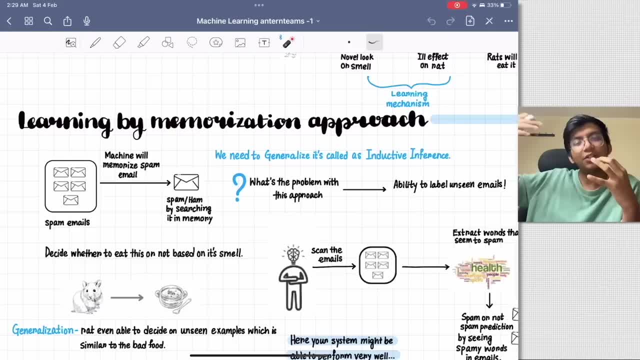 memorized, but you also got a tweaked question, but you also got a very different set set of questions. so where you have to apply logic and you know, apply several skills in that, so there you will fail right because you've memorized only the questions which came, but you're not able to. 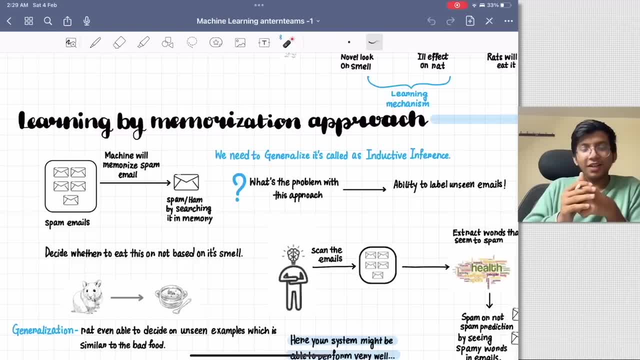 answer the questions which are new, which are unseen by you, right? so in this case as well, model will fail to gen to to, to predict for examples or predict for emails which are unseen by the model, which are not seen by the model, right? so that's, that's the problem with with the 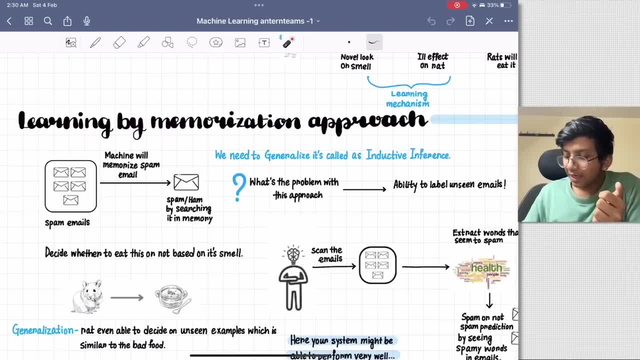 approach right now. right, so that's one of the approach. the problem is that the machine which we have does not have the ability to email any unseen emails to, to predict for any unseen email. so, for example, if any, any email comes and let's assume that it is a spam, but this is not available. 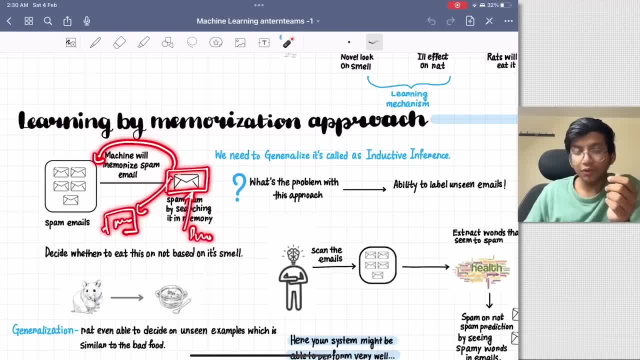 in this memory content so that will be flagged non-spam, but actually it was a spam, right? so this is one of one of the problem. so we need what we need to do. we need to figure out a solution to further generalize it further, make to, to, to. 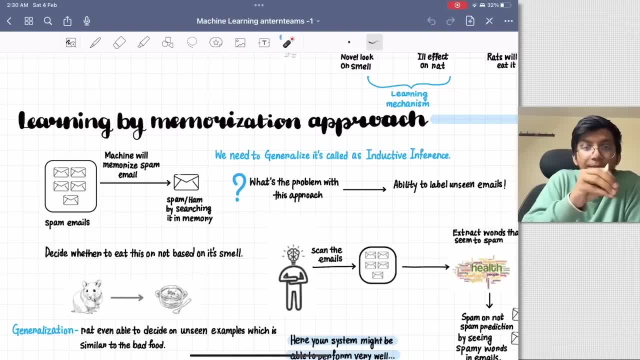 generalize means to have to give, to give this machine an ability, to give this machine an ability to further classify even unseen emails by logical thinking. so we're going to make this guy to the second number of guy, where it also understands, analyzes the data and applies logical thinking. 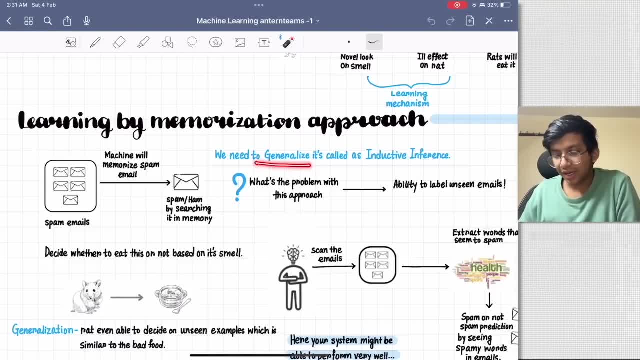 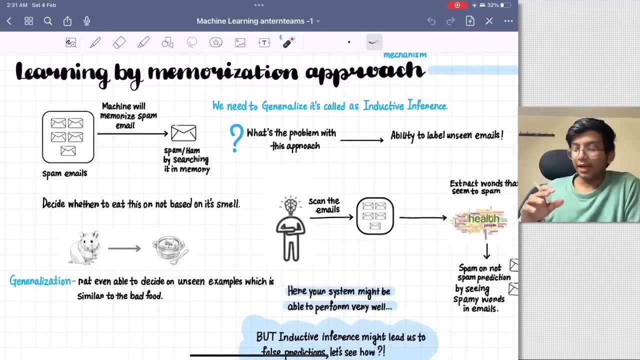 in further to predict emails. so that's, we had to generalize, and this is called something known as inductive inference. okay, this is nothing but called inductive inference. so we'll talk, we'll talk, let's. let's talk about inductive inference, uh, in the in detail in the next lecture. so now, 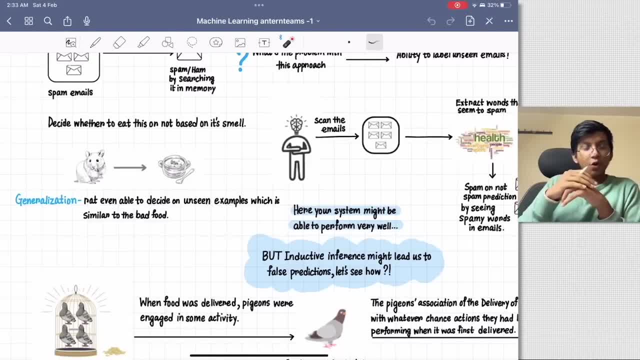 we'll talk about something known as a generalization, which we had had a talk, and we'll talk about the generalization of the generalization of the generalization of the, and then we'll talk about and what's the issue in this as well? right, so we'll talk about that. so 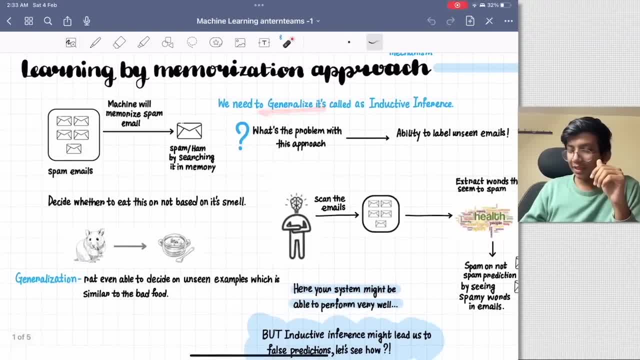 the. we call that generalizing. our model is known as inductive inference. right, um, please read the if you want to know more examples and all. i've linked the very nice book, the chapters, and every chapters is also included in the in in the lms, so please go over there. you will be able to see. 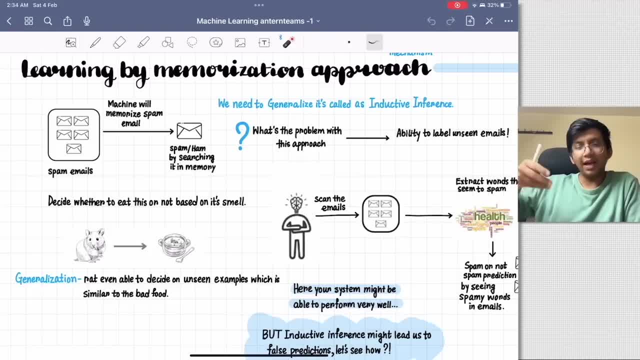 everything, uh, um, each and everything, with the resources and everything uh and the reading materials regarding, if you, if you want more examples, but that's it for today. thank you so much for watching and i'll see you in the next one. bye, bye, you can stay here if you have understood it. so, generalization, generalization is, it's an ability. 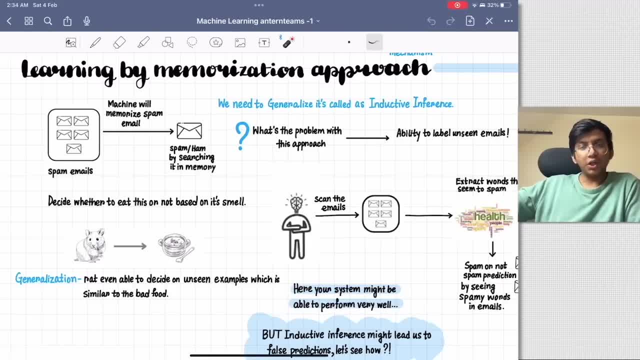 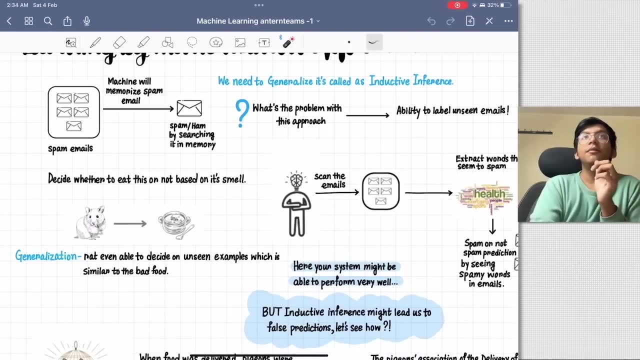 to um, to add the feature in your machine, to actually improve right to to actually uh, work on even unseen examples, but to apply logical thinking. so now let's take an example over here. is that the the problem, the problem which we had, the problem, the very basic problem which we had? 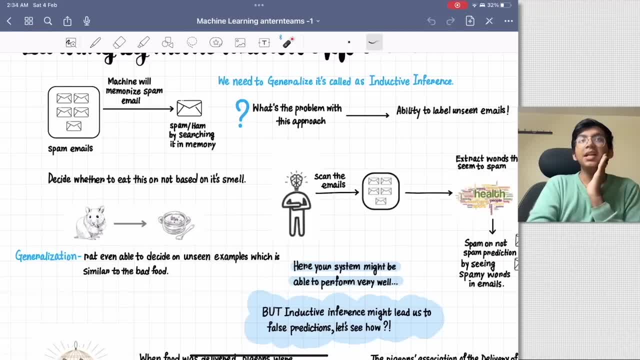 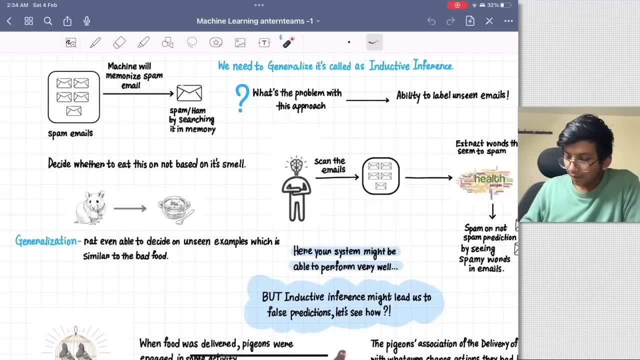 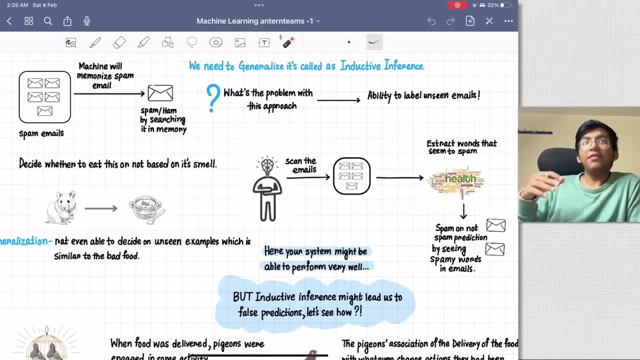 so i'm just going to take a very, very nice example right now. so now, now, over here, over here, this rat. so in the end, in this example, this rat, if we have the generalization available, if we have the generalization available, if we have the generalization, 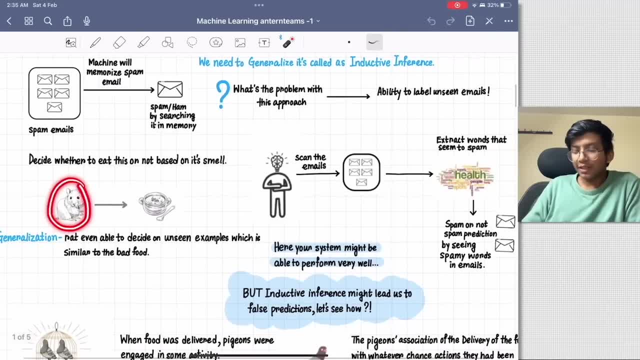 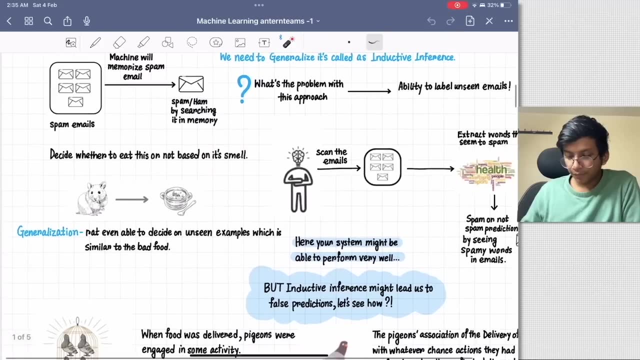 uh available, where your rat will be able to decide whether to eat this food or not, whether to eat this food or not, based on its smell right. so rat will be able to decide to to eat this food or not with the help of its smell, right. so, generalization, what? how does this help? how does this generalization help this? 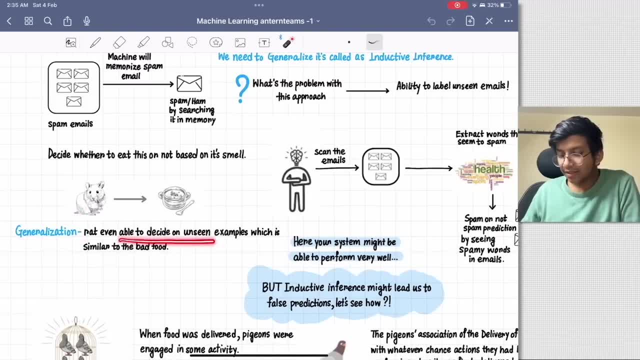 help this rat. it helps it to decide, and unseen examples, which is similar to the bad food. so what is this saying? that rat may have seen the similar existence, some similar food right, so that may have seen the similar food. so generalization is that that even that's even. 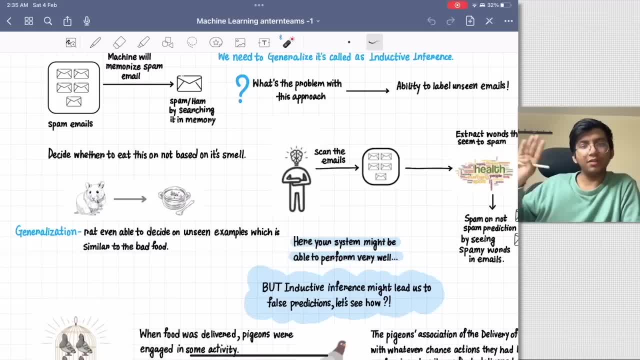 a similar something comes in that will be able to refuse. okay, this is a bad, for this is a good food, right, so that should. generalization gives an ability to even rat to decide on this particular food which he has never eaten before, based on the, based on the similar things which i've eaten, which he has. 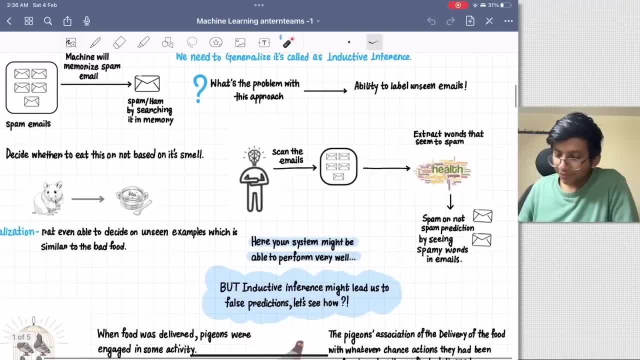 eaten in the past. another example which which we have seen that the that we have a machine which scans the emails we have. scans the emails, it extracts the words that appears to be spammy words, which is spammy words, and then it says spam or not by seeing the spammy words. so basically, 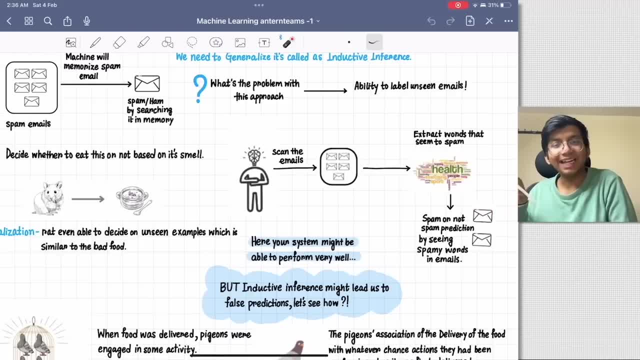 that email comes and then see what proportion of the spammy words is the amount of spam that words is in that email, and then classify it based on that. but there's an issue. so now, by this, if you have the, if you have the, if we have the words, that is the that is spammy, and then we check the. 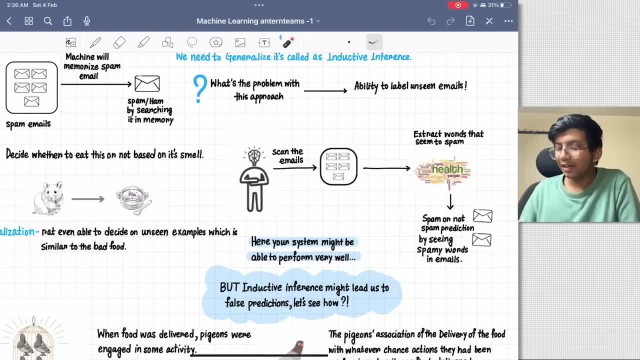 proportion in that. or we give the machine the ability to even classify: uh, based on the logical understanding of that, and or generalized understanding of: okay, this is this, this is how the spam email looks like, right? so, uh, your model will is able to generalize accordingly, according to the things. right, that's one of them. but here your system might be able to perform very well. 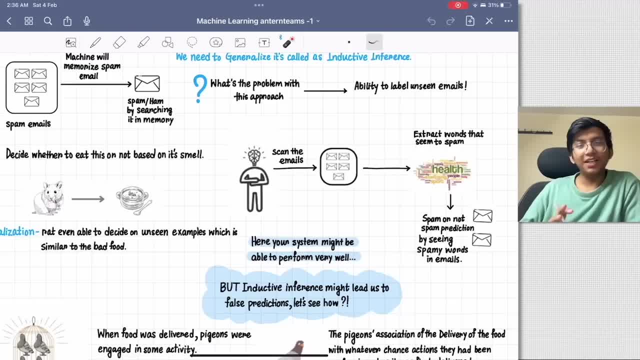 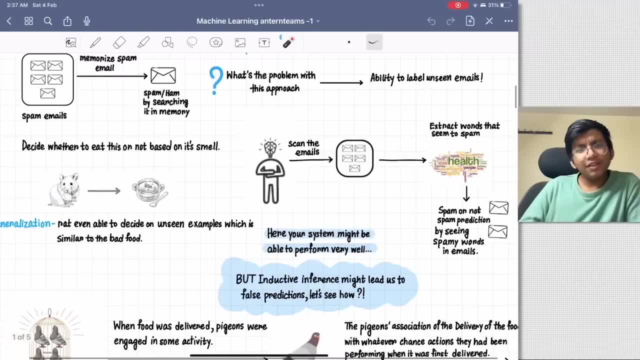 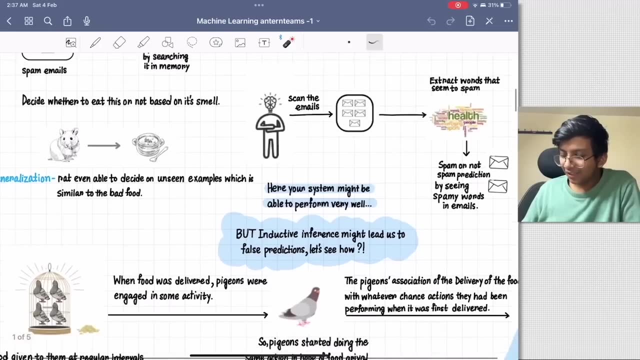 right. so in this case you might be thinking that you will be, your system will be able to perform omg right, but actually it's not true. uh, you have, you give the ability to the model that to identify even unseen examples, and then you think, okay, it's over right, it's not over. so inductive inference. 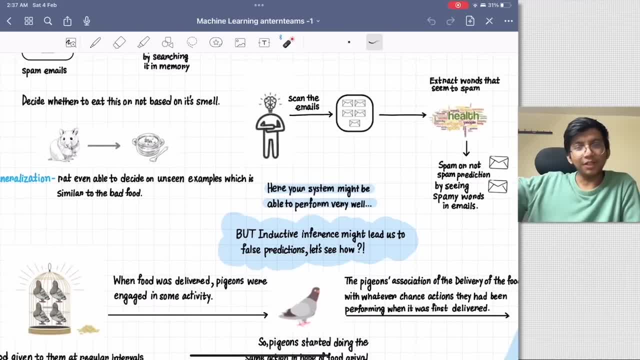 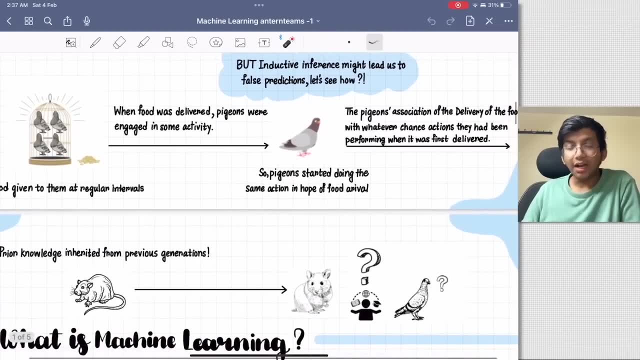 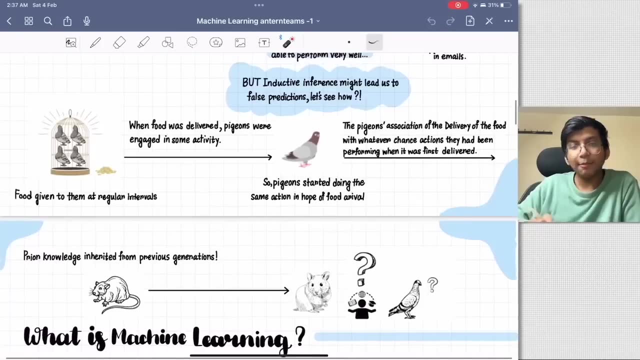 might lead us to false predictions, misleading predictions. let us see how. so this, uh, pigeon superstition is an example. pigeon superstition is an example- um, i will, which i have read in a machine learning theory book from algorithms theory, and also this is a very famous example on learning conducted by some sort of you know university which i don't remember. 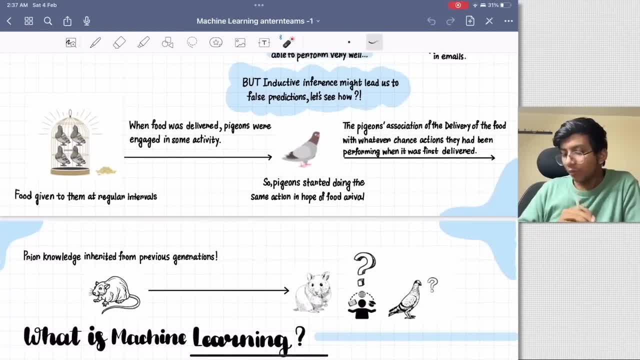 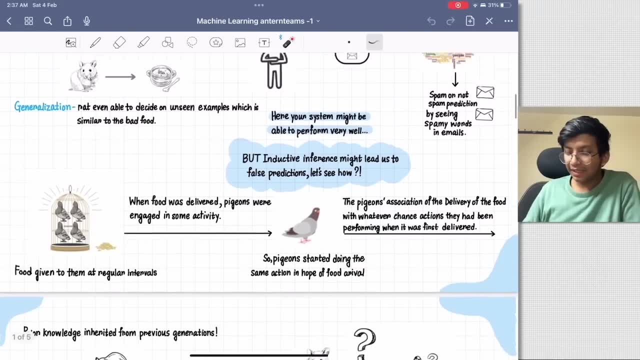 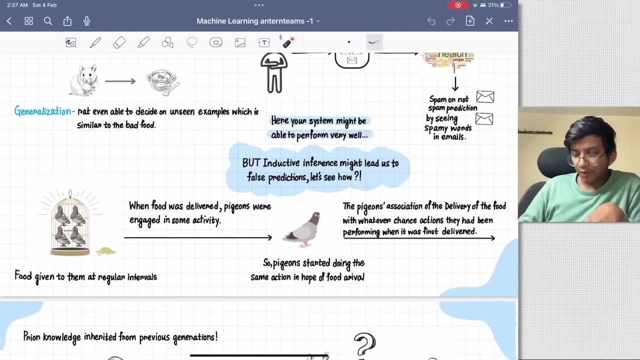 they have written it very nicely- is about how this inductive inference might lead us to bad inference, how this inductive inference might lead us to bad inference. so let's talk about the very nice stuff. as of now, is this this particular thing, pigeon superstition. so you will be seeing a way. uh, 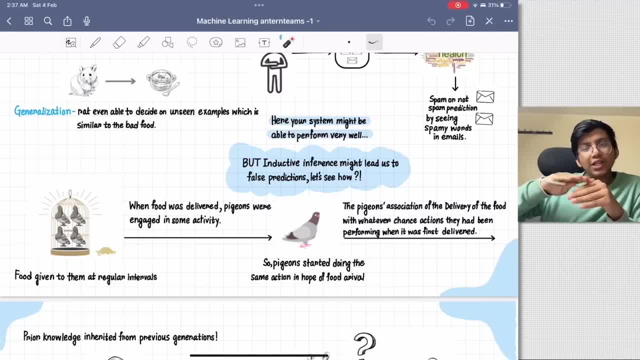 you'll be seeing a very nice, um, i'll be linking a very nice video which you, which i suggest you to go over there and watch that video first, right, so go over there, watch that video first, or i'll be giving a short, um short experience on what exactly is going on so you can actually pause. 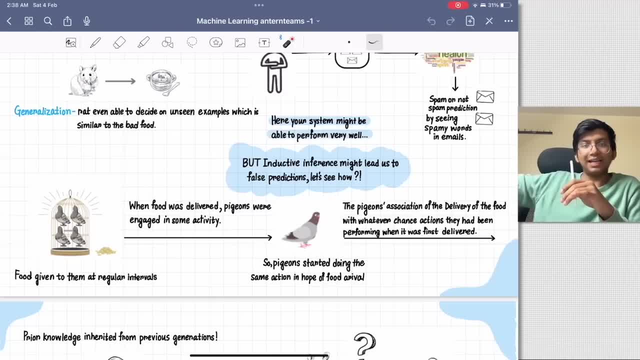 the video right now. go over there and understand what exactly is going in that particular video. that video. but i'll be explaining you in simple english terms so you can actually go over there and understand it by your own terms. but i'll be explaining in a very simple english terms. 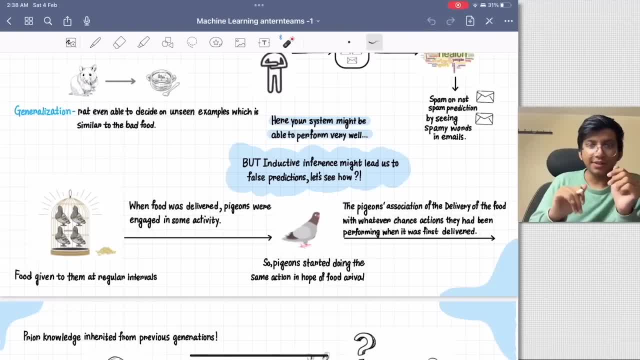 so you have, um, what, what? the what the experiment was, experiment was. now you have, you have set of, you know, you have set of pigeons, you have set of pigeons which was contained in a cage. so you have, you, you've taken a set of pigeons and what they did? they have, they have, they've kept it in a cage. 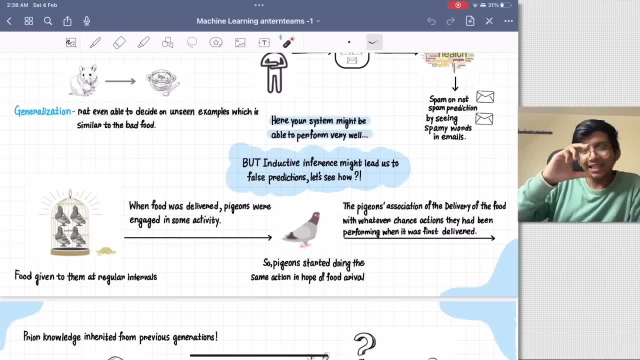 right, and that cage had a small hole, had had a small hole where the food was coming and going at a certain interval of a time. assume that every three seconds, four seconds, five seconds, 10 seconds, 12 seconds, 14 seconds, and all these pigeons are super hungry. okay, so so we have a cage and that 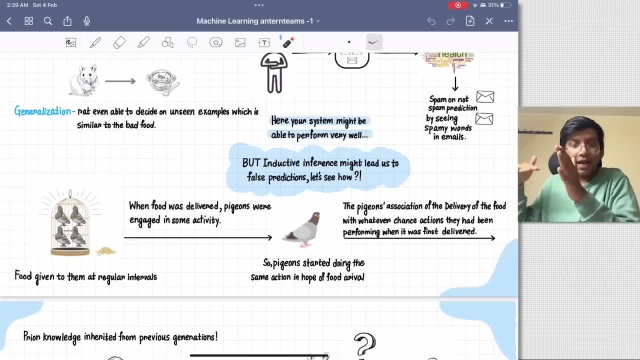 we have a pigeons which is super hungry, and then we, there's a hole where the food is coming at a certain interval of a time, okay, at a certain interval of a time. now, now, now when food is delivered, now they are angry, right. so sorry they, the pigeons are hungry, right? so if the 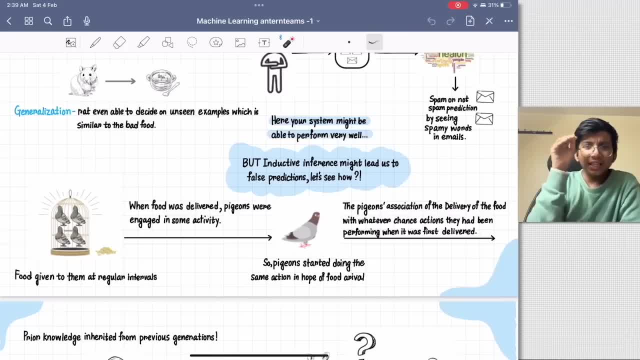 pigeons are hungry, they'll. they'll keep on doing some things. they'll try to peek. no, they'll. they'll try to peek and try to find you know some sort of um foods you know. so they try to peek, or they try to, you know wings as like, spread their feathers and then try to uh, go from here to the other, peak. 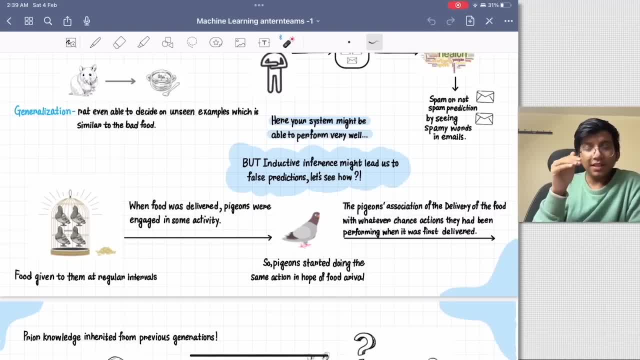 right. so in this case, as an experiment, i'm taking example: if the pigeons, if one of the pigeon, if two, two, three are peaking, right, so they're, they're searching for the food, they're, they're active. okay, they're active and they're peaking like this. 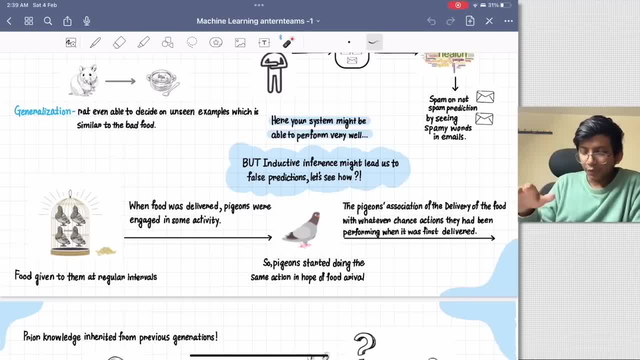 which is my like, searching for food. uh, they're peaking now. so when food is delivered, when food is delivered at every interval of a time, they are engaged in some sort of activity. that activity can be peaking or that can be feathering up, right, anything, literally anything. so if you see the 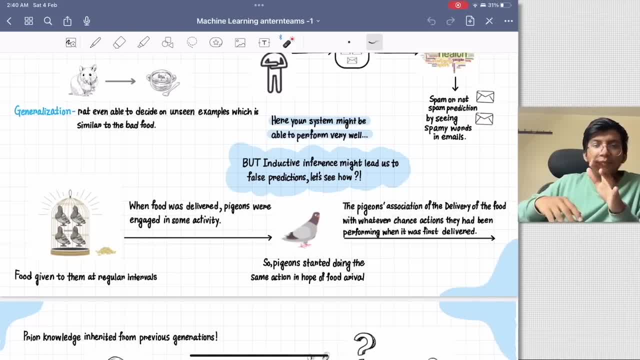 video you'll be seeing that some birds are peaking, some birds are- uh, there's only one bird which which the video which has some. the bird is speaking, or maybe the the pigeon is doing some sort of activity, right going from here to there and here to there. so this is some sort of 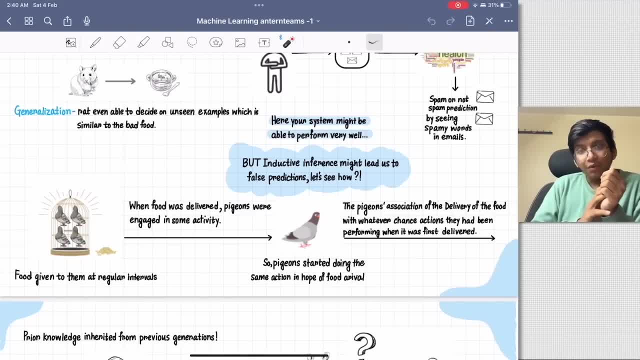 they're engaged in some activities. now, now, now when the food was delivered, they were engaged in some activity right. so when food is delivered, they go on and eat in that right. and then again started doing the same action, again started doing the same action in a hope that food will deliver. 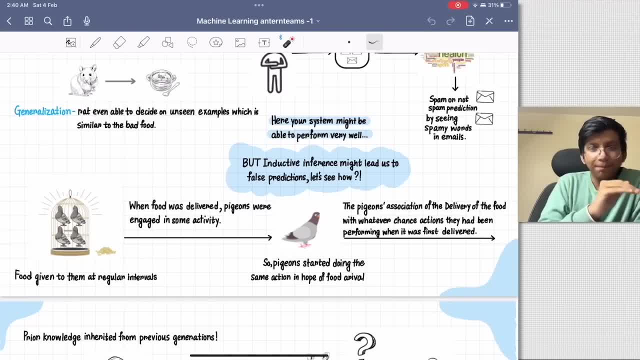 it once again, right so, if they would like, pigeon is doing some peaking and the food is delivered by doing that action. so you go on and eat and again started peaking. so he thought that if i peek i'll be getting uh food to me, right so? so basically pigeons started doing the same action. 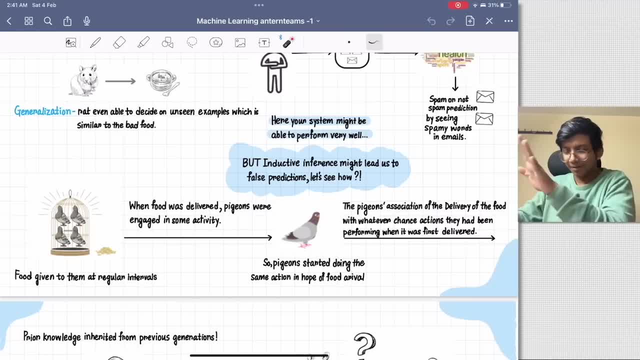 in a hope of food arrival. but i'll come to that, but later on. so the pigeon association of the delivery of the food with whatever actions they do- peaking, feathering, flying, literally anything it with whatever chance actions they had been performing when, when it was first delivered. so 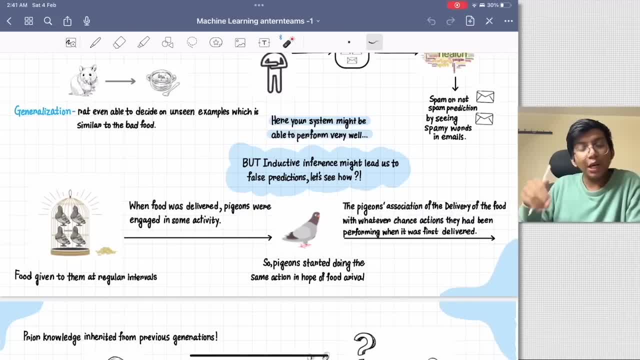 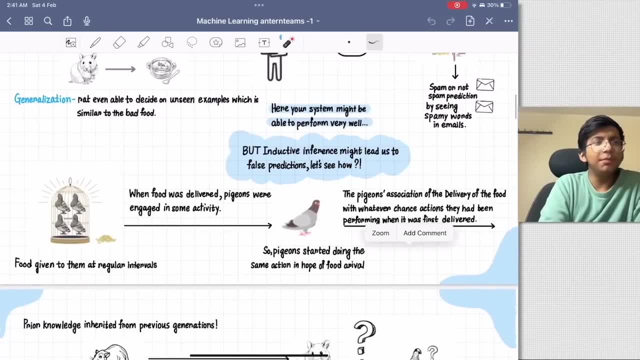 the first time it was delivered. so they were peaking, so they continued to peaking in order for the food arrival, because they hope for it, because they hope for it. so what's the problem in this right? what's the problem in this right? so let's talk about what exactly the 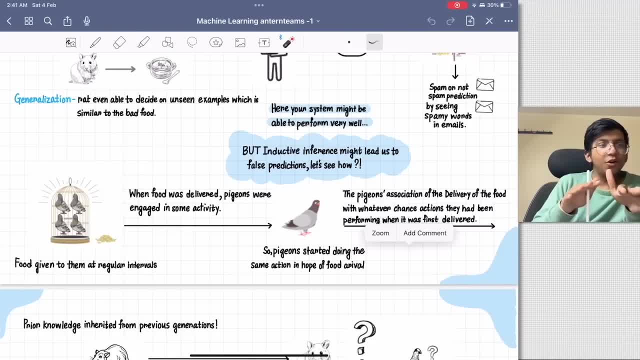 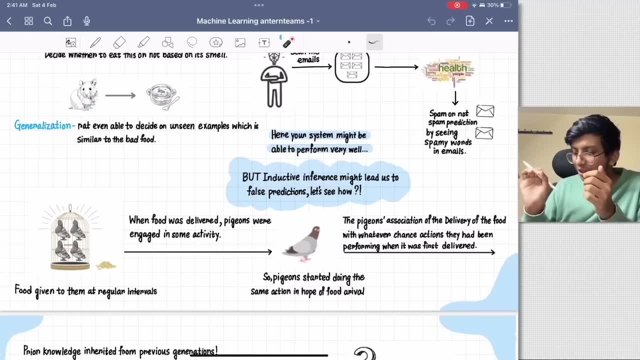 problem which which comes so basically, pigeon built an association, pigeon built an association with pigeon built an association of the delivery of the food, the delivery of the food with whatever chance or actions they had been performing right. so they built the association between delivery of food with the actions like peaking or flying they did. 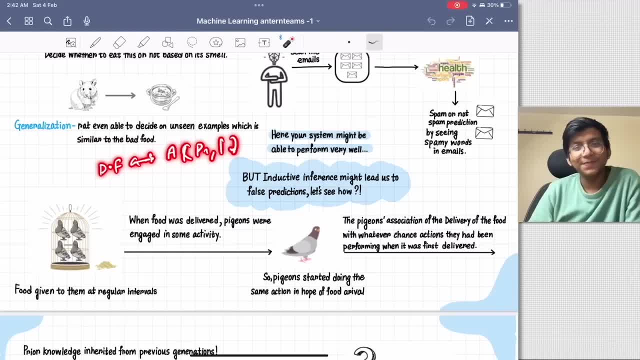 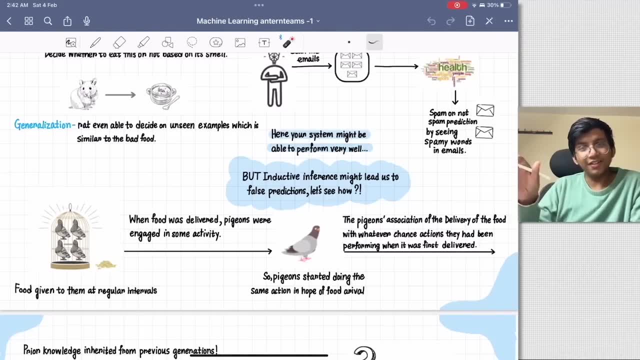 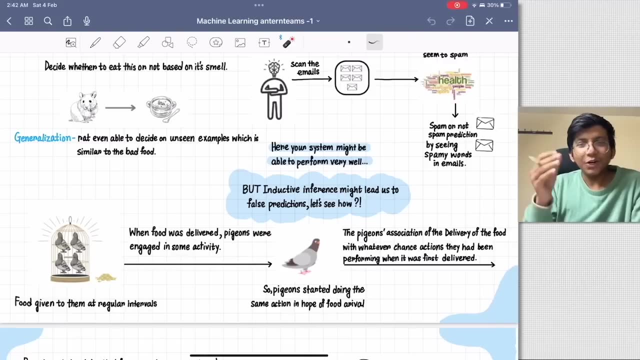 so they tend to do peaking in hope of food arrival, right? so very interesting. so your pigeon learned that, this, that they learned this, right, they learned it. but what exactly? but, but, but now, now this. now let's try to figure out what exactly the problem in this problem is: that human learners 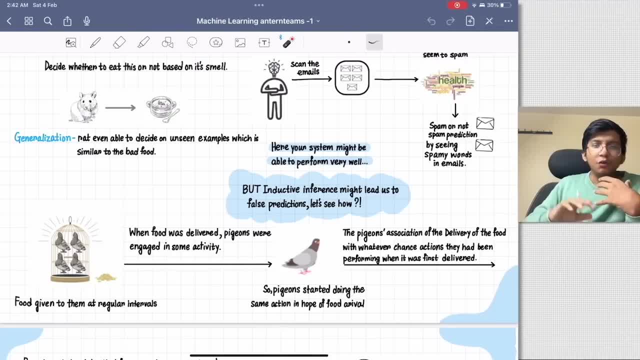 the we can rely on common sense, filter right to fit, to filter out meaningless sense, for example. for example, assume that, uh, every time i throw this pen over here, every, every time i throw throw this pen over here, right, every time i throw throw through this pen over here, my food will be. 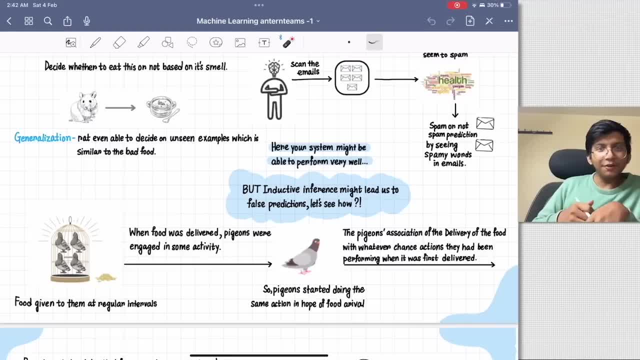 coming right like it is, at a certain, a certain interval of time in the morning, in the afternoon, in the night. it does not matter how much i do this, i'll be getting that interval of time in this case as well. it was delivered on the interval of a second. it was not dependent on what actions. 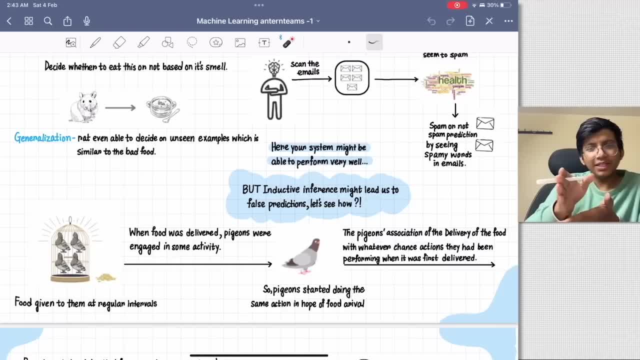 pigeons are doing. it was just lost. intervals: three seconds, four sec. three seconds, six seconds, eight nine seconds, 12 seconds, um, i mean 12 seconds, and then it is going on at a certain interval time. it is not associated with what actions patients are doing, it doesn't really matter. this is so. now we 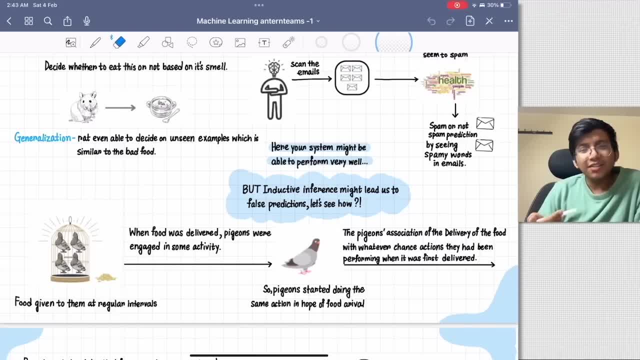 we can, even we can rely on. it is a meaningless right. whatever pigeon has understood, it is a meaningless right. this is a meaningless and this is something which is not so. human learners can filter out meaningless things. we can filter out. that's a coincidence or that's something that? 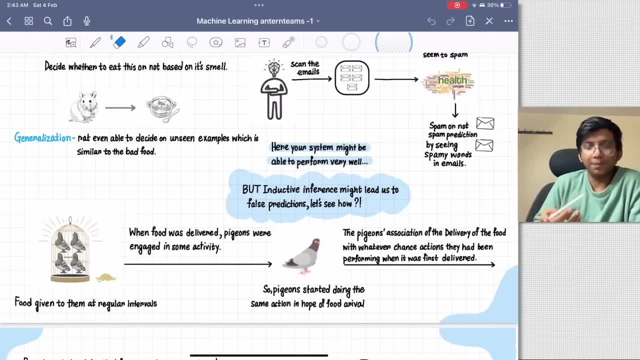 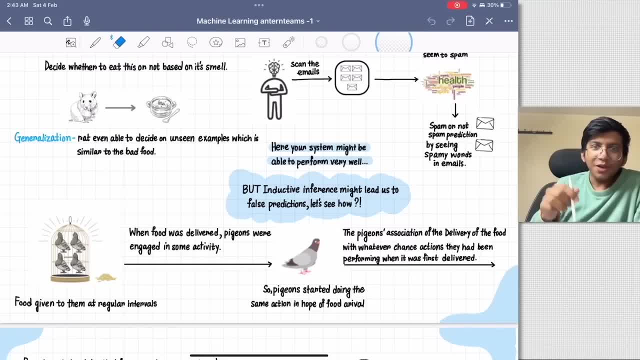 and you, yeah, and you got money on your bank. now you're not. cannot keep on doing this to get money in a hope of money arrival. money will come at a certain rate of time, right, um, so this is something which this is meaningless conclusion, but there are some humans who cannot apply the common sense. 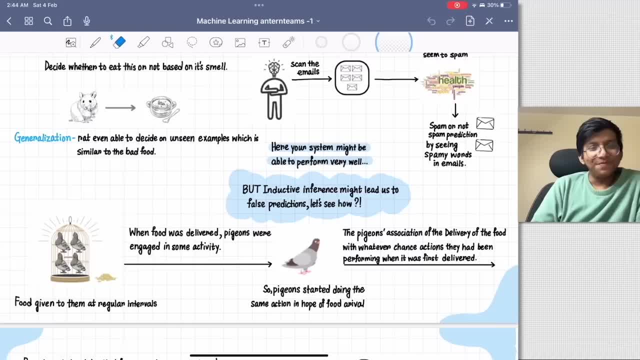 filters to not take out the uh meaningless. that's not the worst, but never mind so. and now now we now, uh, now. over here, pigeon also learned a very bad, meaningless conclusion: where is where it? he thought that peaking will get near food- right, that's a bad. so we also have to give this filter. 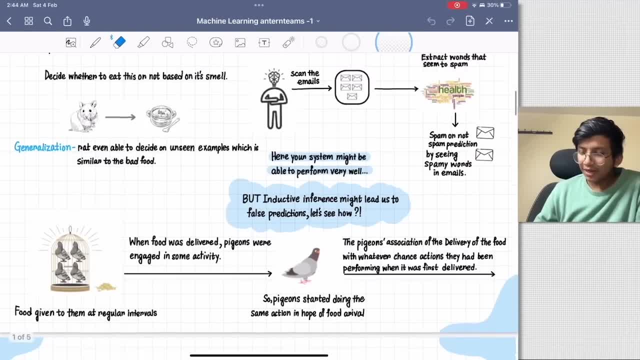 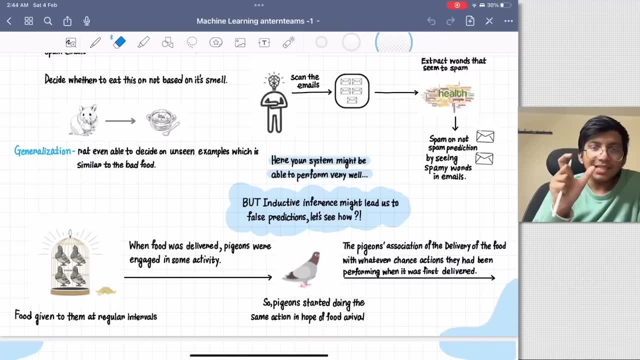 to our machines right. so in this generalization approach, the problem was that your model may end up learning a meaning, meaningless learning conclusions. so we must give the well defined crisp principles. again i'm waiting. we must give well defined crisp principles so that will protect our program, that, from reaching senseless, like what. 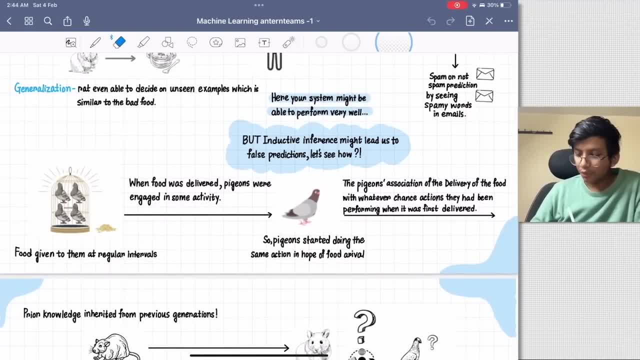 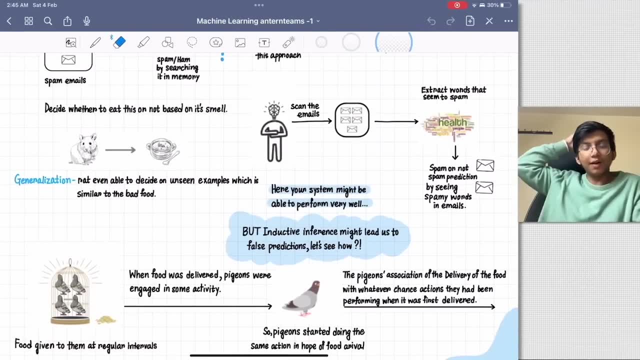 pigeon reached that will protect our machines. to reach that to to. to reach that conclusion. this except is taken from understanding ml, from theory to algorithm. this is very nice, that's why i've taken it from there. what exactly it tells? it tells that your that we need to give filters to a. 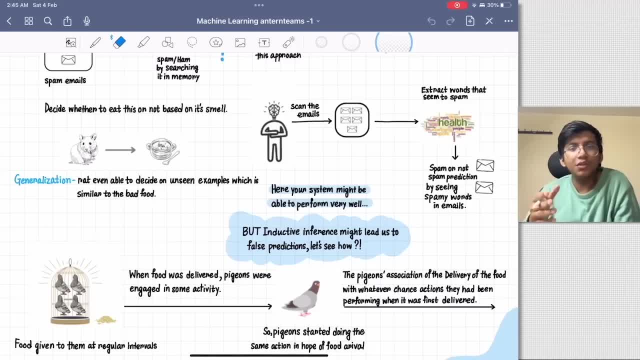 model, so that a model is able to identify the meaningless conclusions like this, right, meaningless conclusions. so we have to give the well defined meaningless- sorry, um, well defined- crisp principles, crisp principles to a model and those principles are only called, and those well defined crisp principles are called what that are called, nothing but. 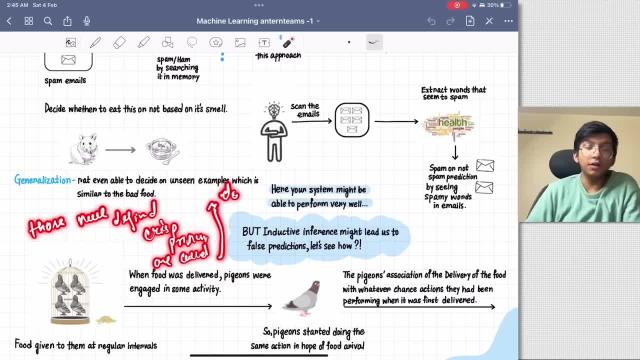 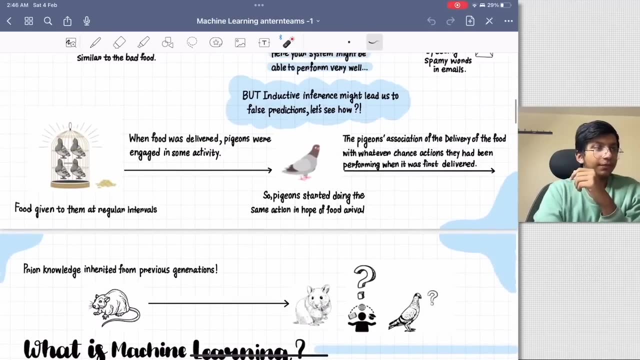 That's what we learn. that's where the theory of ML comes in, where we give the well-defined principles to our model. I hope that makes sense to you. that gives you a very nice understanding about whatever we want to have a talk on. 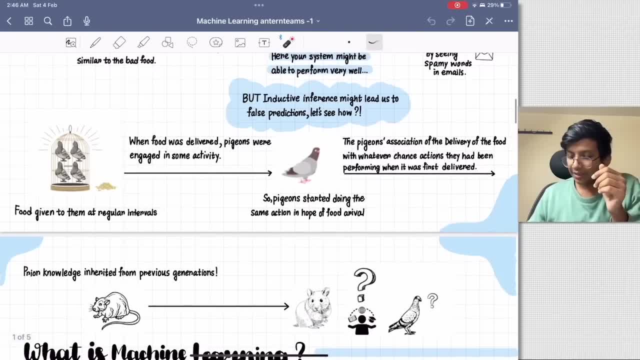 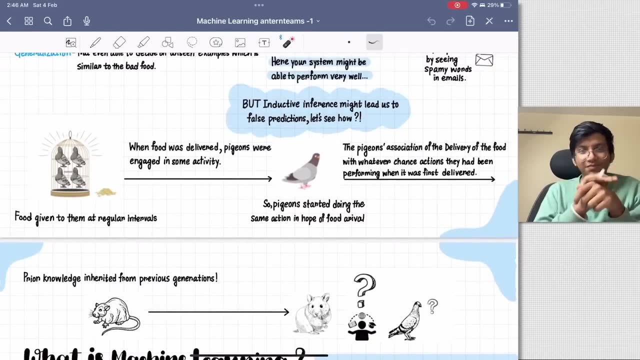 Now there is a very interesting concept which is known as inductive bias. So let's talk about that, and then we can end this video, and then we can go to the next step, which is exactly learning about what is machine learning? Now we know about learning, and then we can go over a bit of learnings. 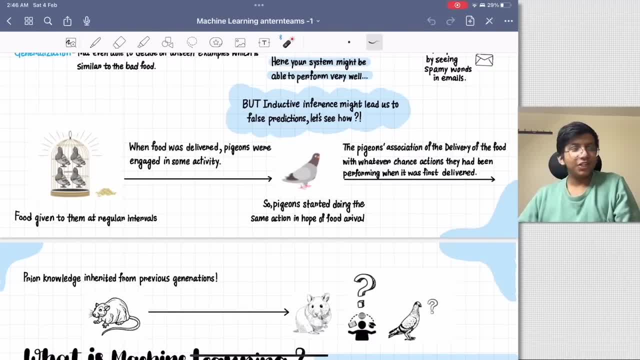 So assume that. so sometimes you might be noticing that a new cat, that a new cat, that a new cat- sorry, new rat. why am I saying cat? a new rat might refrain from eating a food Because they think that this food is poisonous. why? 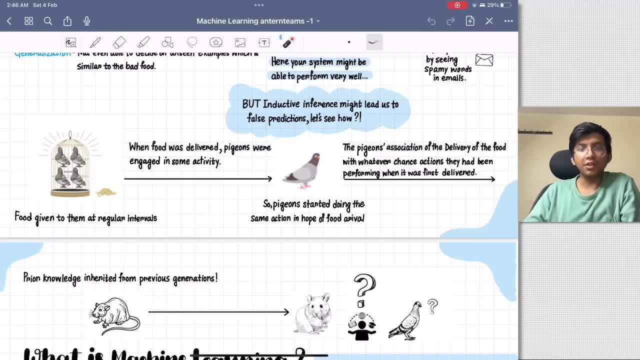 Because of the prior knowledge inherited from the previous generations. So they have some sort of genes that tells us: don't eat this food. this is poisonous because of the past generations, because of the habitual understanding. If you have studied biology, then you have studied that their evolution, or the evolution 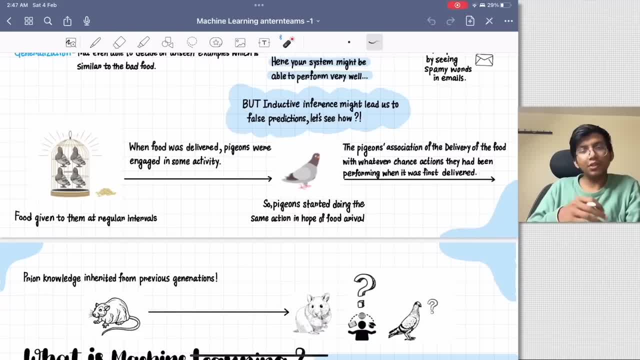 is necessary for human beings If there is no evolution, If there is no evolution, If there is no evolution, If there is no you know chain of you know whole food chain. So assume that you have lots of humans and they died from the disease. 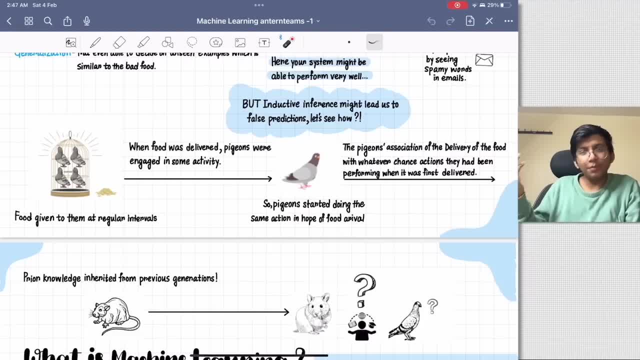 But there might be some newborn humans or babies, which later developed into humans, where they are capable of fighting with those diseases. They are capable of that, They've inherited. they have built a very nice combination of fighting with the diseases. So in this case, this rat has inherited from the previous generations, previous generations. 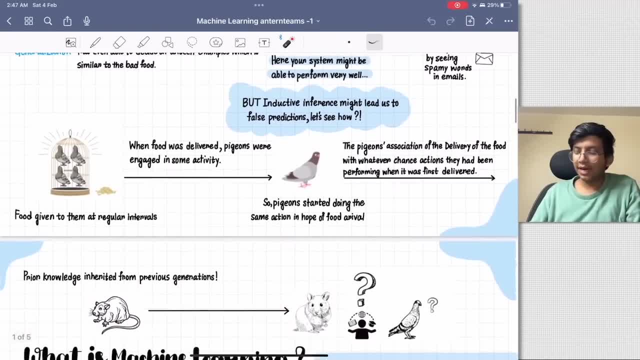 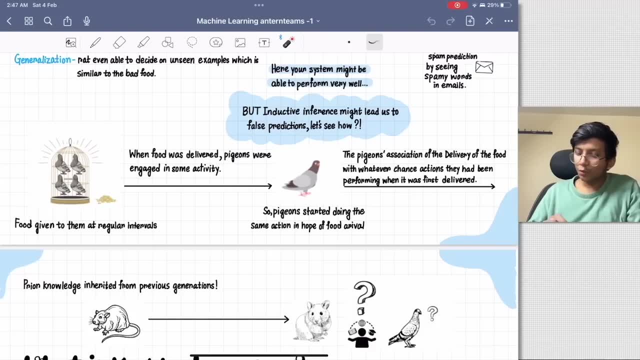 of the rats to further say that, okay, I'm not going to eat this food. I'm not going to eat this food because it gives some sort of sense. So you might be thinking: why rat so this? so why rat? why rat was able to successfully? 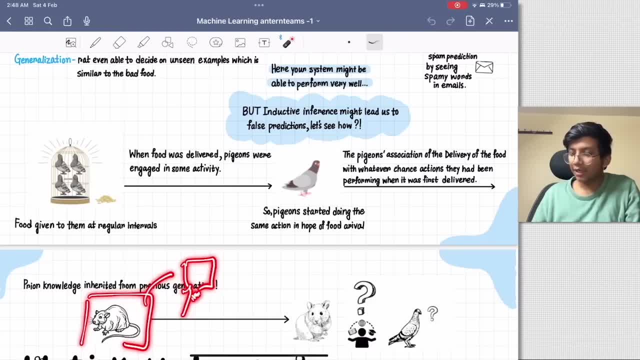 classify to not to not eat that food whether pigeons was not able to. pigeons was reaching to a meaningless conclusion. Okay, Because rats were having the prior knowledge and prior knowledge is super important where the rats were having the prior knowledge. 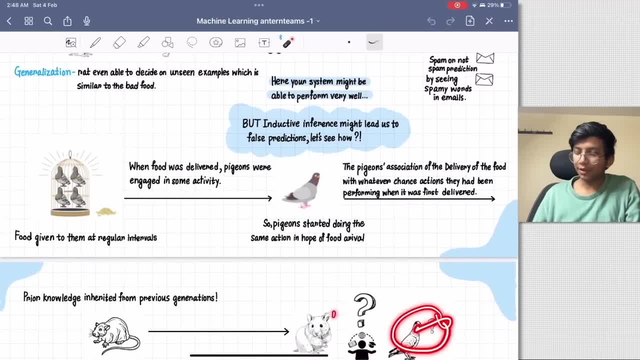 So pigeons learning was not more successful as compared to what rats did because of the prior knowledge, and prior knowledge is also called inductive bias. Prior knowledge is also called inductive bias. I hope that makes sense. Um, now, I hope that that given you a very nice introduction to learning in the next. 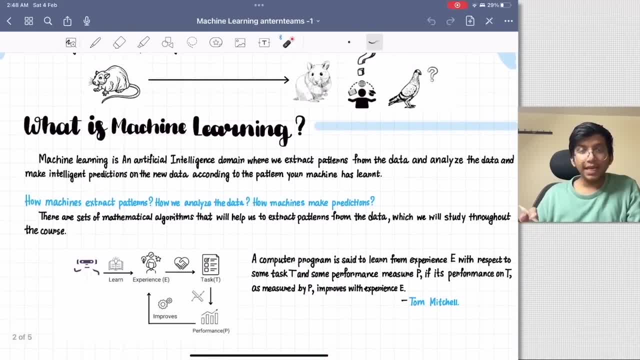 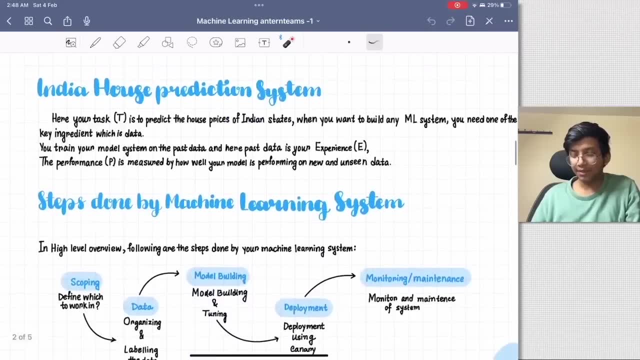 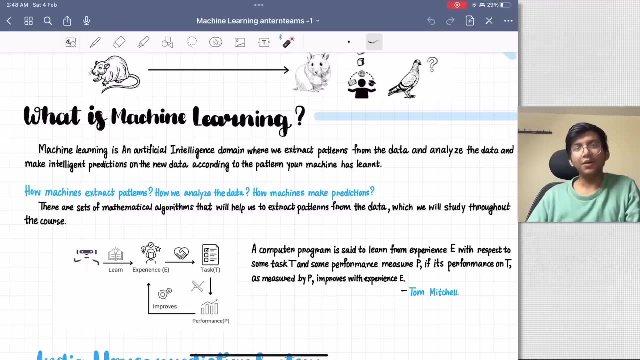 lecture. what I eventually going to try to achieve is talk about a very nice introduction to machine learning with applications, And we'll also do several examples as well. That's something um isn't necessary for you, right? So let's go to the next lecture and then try to understand machine learning with a very 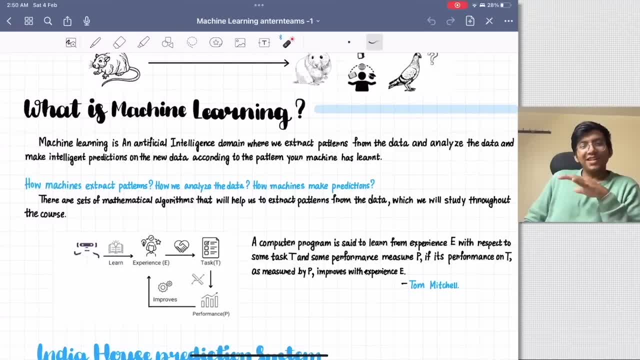 nice definition with a very nice set of examples, So, yeah, So now what I'm going to do is actually talk about- uh, start talking about, you know, machine learning stuff, And that's something which is super important. It's super important for you to actually go forward with it, right? 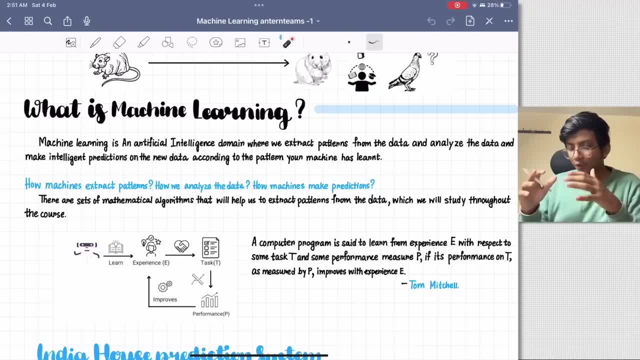 Let's talk about that. So now, what we're going to do, we're going to actually talk about what is machine learning and we're going to talk about some of the applications of it, And then we'll see some of the formal definition which comes in machine learning. 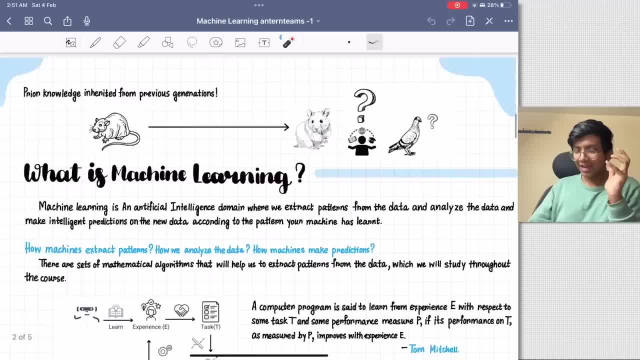 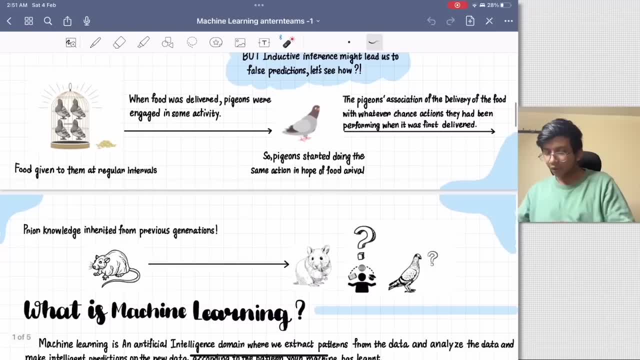 Now you know what exactly learning is right. Now you know exactly what learning is, And then you'll start referring that we have solved some of the problem. Now to dev, now just just to connect the dots, to connect the dots, the dots. how we're going. 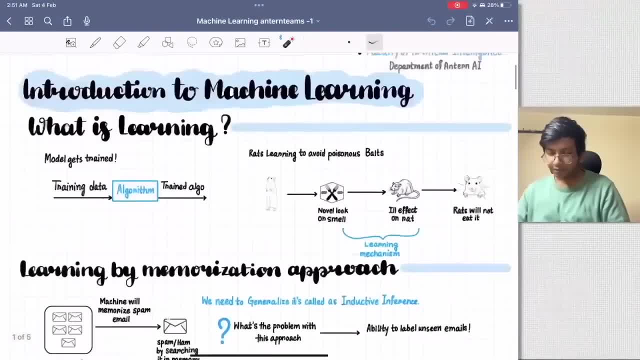 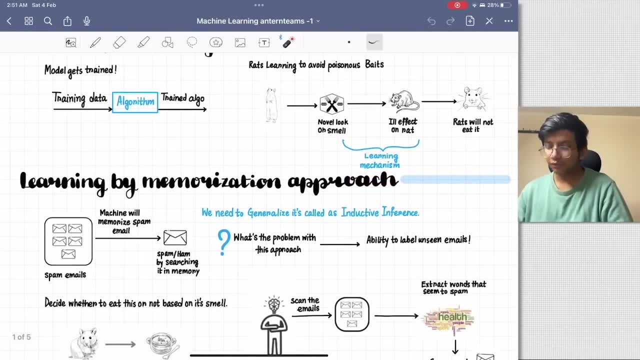 to connect it. The dot is first. It's there first. where? where are the? where we learned about learning mechanism? where are rats were learning to to to to, to further classify whether, whether whether to eat this food food or not. 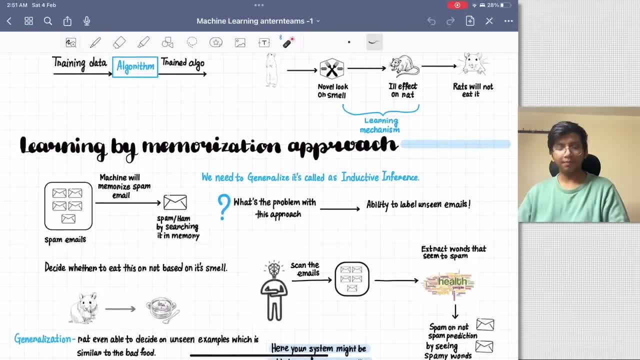 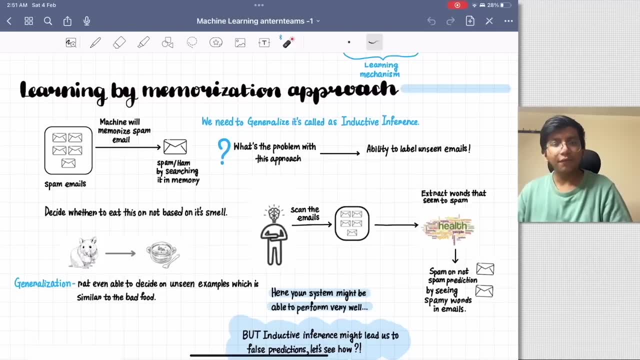 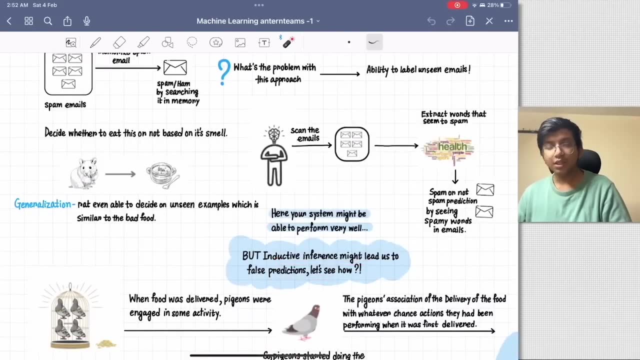 Right. So we've gone through memorization approach where, um, by taking a simple spammer ham examples and for memorization, we thought that generalization, that we have to generalize it, So that is inductive inference. So we've got another, another issue which we see in inductive inference, which is a 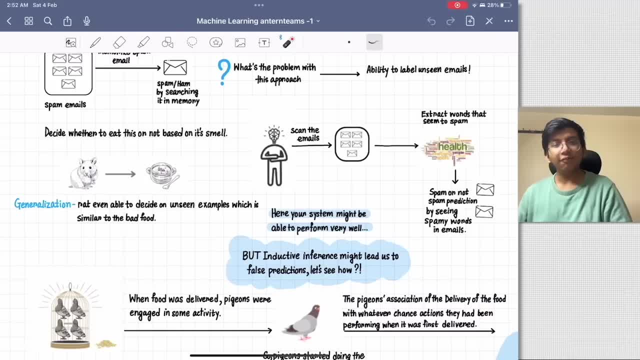 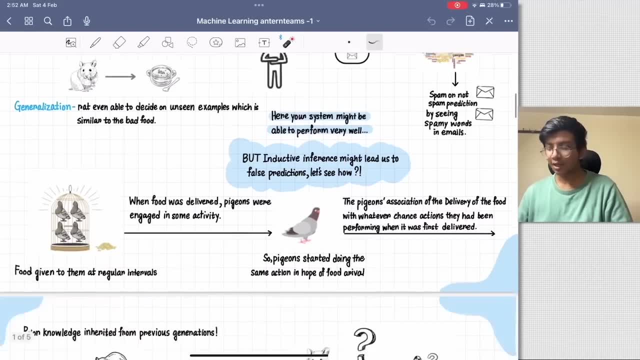 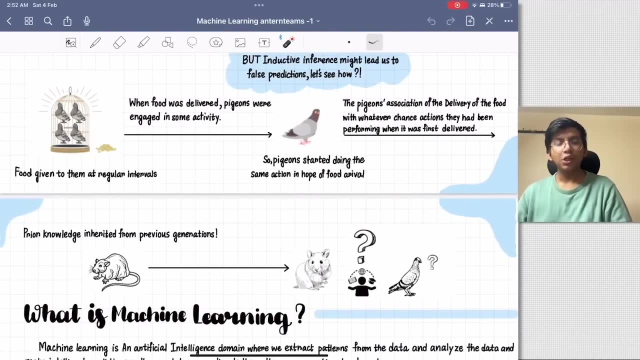 misleading 마idas And for defining that senseless and for for refraining or protecting our programs, for census conclusions or the principle conclusions. we have something known as machine learning, where, in this machine learning, we define our visits, define well defined crisps and 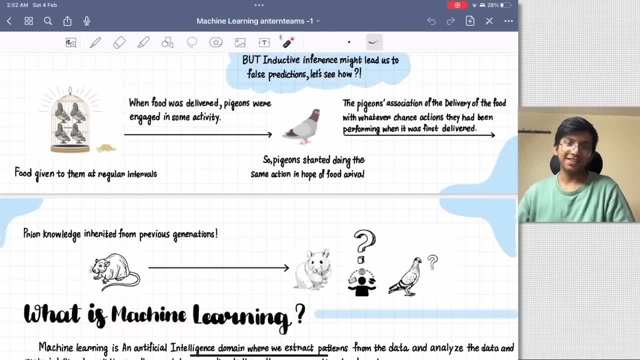 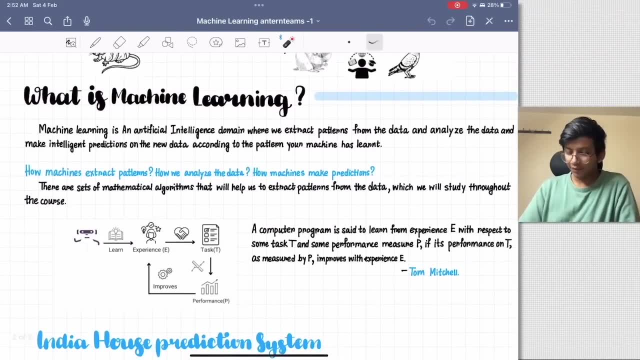 principles, so that our model or the model does not reach us to Cool. Uh, so let's get started. So I suggest you Maybe have a coffee with you, because that's something that's super important. But again, the defense that he's saying. it's one of the people who are usually called. 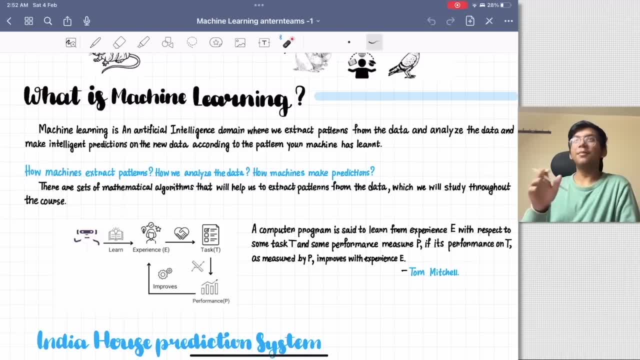 uh, essential lei, no brainsminds, no museums, arnamente parts of the story. If he had supp ant Minor Hm the different from so. correctly, I'm recording at 3 am because I have boats as well and I have to prepare, so I know how I'm managing this because I have a. 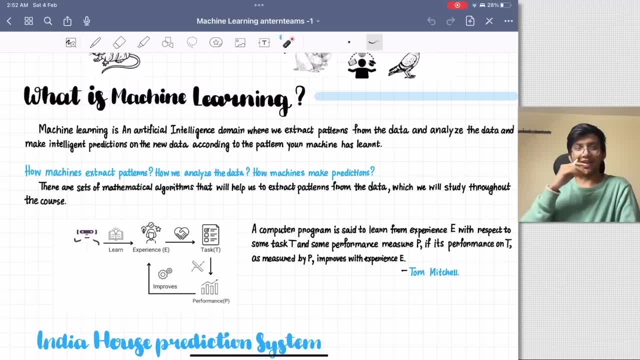 class 10 boats last an examination in 20, 24 days I guess, and I have to prepare a lot and I'm doing my day and night on that but eventually after to also do for community, and I'm doing it because I like it and not something when who's 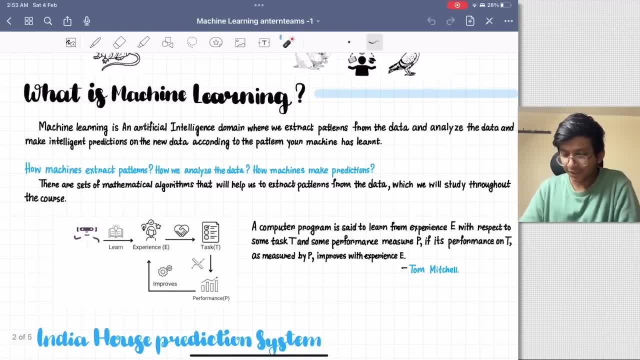 forcing me to do this. but coming back to what exactly I want to do, it is: what has machine learning question? so, whatever you know about machine learning, write that in a comment box, add a comment or whatever we can do, and just just write that in a comment box. what is machine learning right? so what has 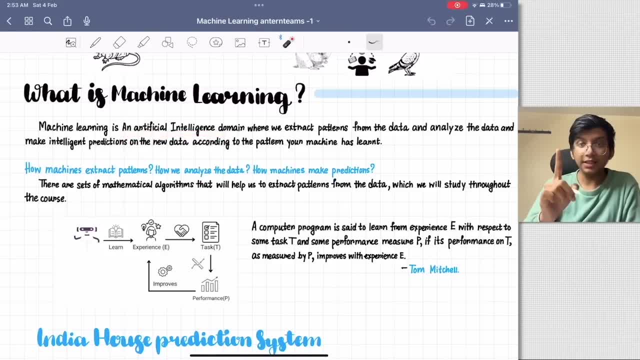 machine learning. it's an artificial intelligence domain. it an artificial intelligence domain where we extract patterns from the data and analyzes the data and make intelligence predictions on the new data according to the pattern. your machine has learned a very nice and influential statements, so let's try to talk about the very highlighted statement. 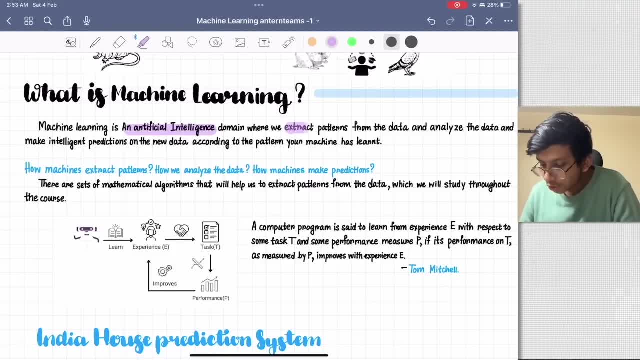 it's an artificial intelligence domain where we extract patterns from the data, analyze the data, make intelligent predictions on the new data- this new is very nice- keyword according to the pattern your machine has learned. so these are these. you know keywords. if you understand, you know machine learning. so let's try and understand each and every keyword first. 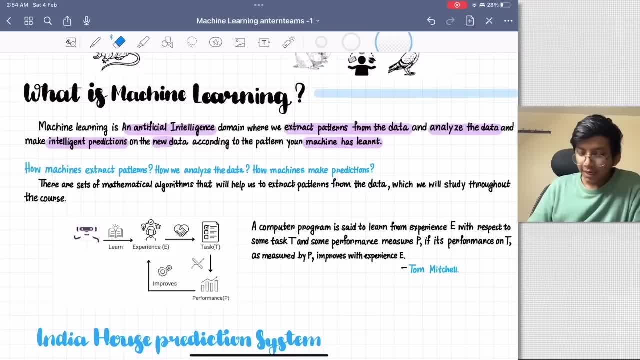 it's a domain of artificial intelligence. if anyone calls a, you know, uh, an mls ai, say mls ai, of course it is, but it is, but it is a domain of an ai, it is a subset of an ai domain, right, uh, where we extract patterns from the data, where we extract patterns from the data, so i 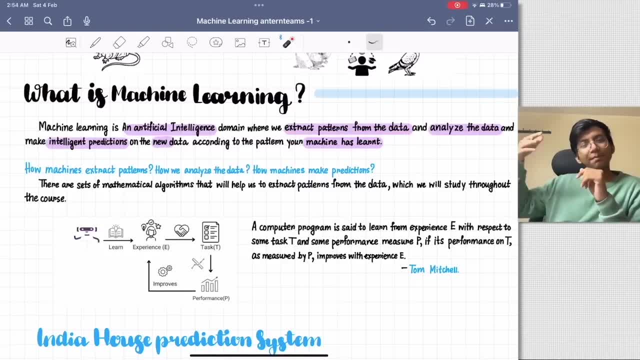 want to explain this to you with a very nice, you know practical example. let's forget, you know bookish examples. so assume that you- um, you want to, you are doing something like: um, yeah, so you're studying some sort of mathematical concepts. assume that you're studying quadratic equations. 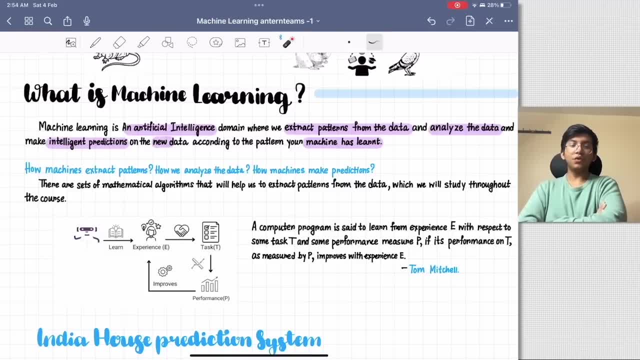 so you're studying about quadratic equations and in that quadratic equations you had something known as taking out the you know uh by. you have some sort of quadratic equation from. there's a formula for taking out using uh, like the concept, right? so there are so many word problems regarding ages, uh, distance and speed. 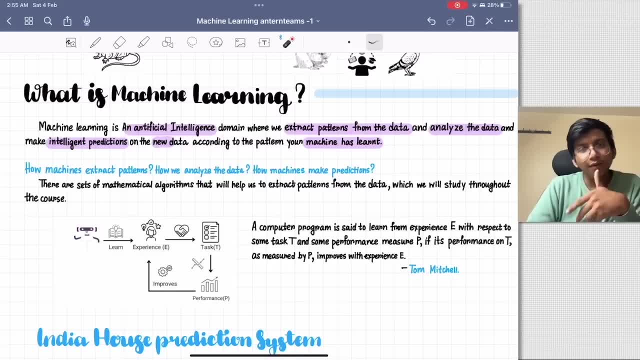 etc. so now, when you actually, when you actually solve those problems, when you actually solve those problems, you learn some sort of patterns that this is how i should solve it. when you learn those chapters, when you practice those chapters, when you actually understand those chapters, you learn how to what, what, what patterns are there, what patterns of questions are there? 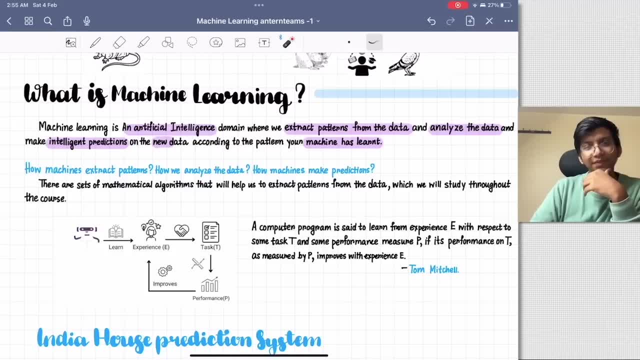 and how the solutions, how the solutions are framed right. so in this way, in this way we have to figure out. in this way you are learning patterns from the from, from the chapter, and by learning that you're able to reach to a conclusion right. so once you have the pattern, now, if the new question comes to, applies. 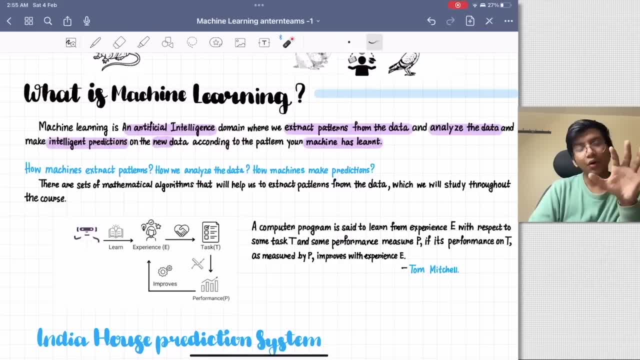 that whatever patterns which you have learned or analyzed, your, your, your content. now you use that analyzer whatever, whatever you learned to answer those or predict, predict the mcqs right. so answer those new questions right, and what? from whatever you have learned till now? so if you, if you, 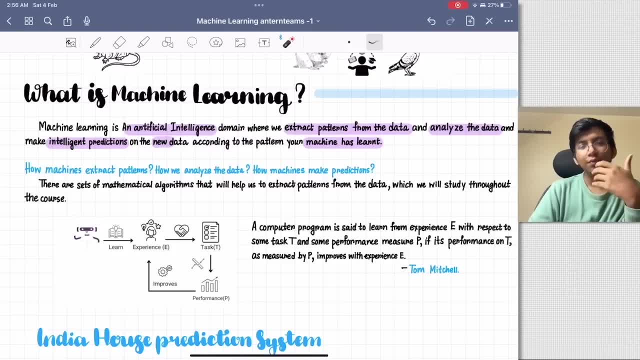 didn't find the pattern. well, you will be not able to, you will be not able to, you know, answer that well, but if you know what, you will be able to answer very well. right, cool, so that's exactly machine learning work. so we're going to understand in that way, so it extract patterns from the data. 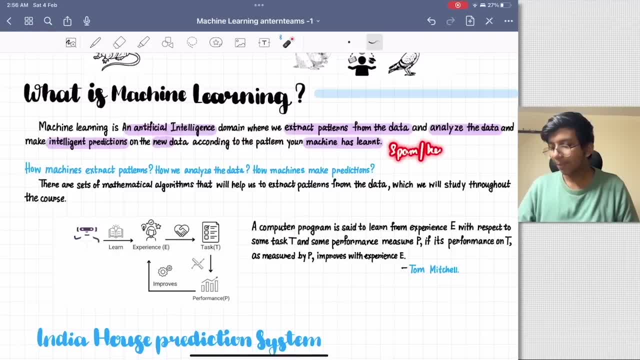 so, for example, if you take an example of a spam or ham example- spam or ham example- it extracts patterns from the data. it extracts patterns from the data where how spam email looks like, how ham email looks like. it learns, analyzes that whole data. data means the collection of information. in this case, you have a 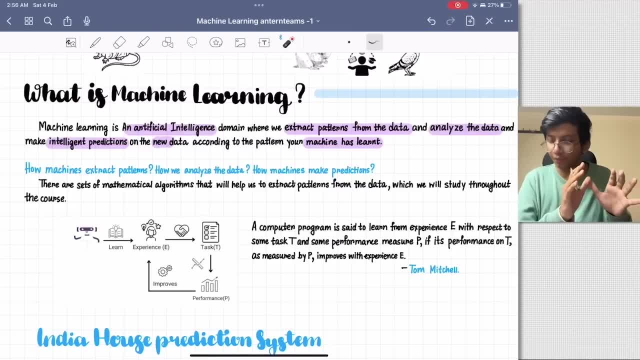 spam and spam and ham emails. that's the collection of information. you extract the patterns. you understand that- how spam looks like, how ham looks like. now, once you have that- i analyzed it now- now, when new spam email comes in, you use the model, uses that analyzed or patterns to make intelligent 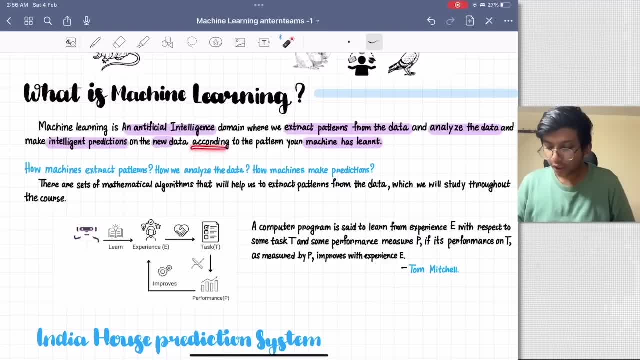 predictions on the data which you have right, according to the question, you're according to the pattern which your machine has learned. that's what exactly machine stores. so now you might have several questions by now. i know it first is again: how to extract patterns, how machine extract patterns from. 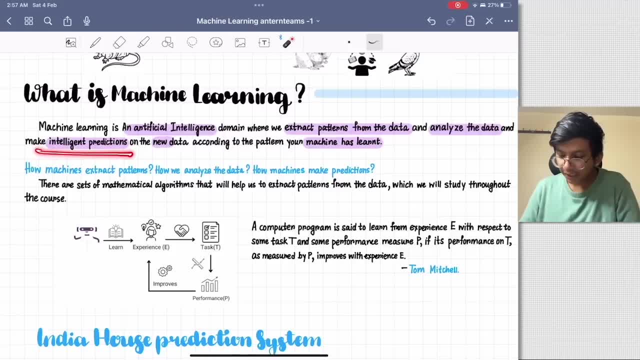 the data, how machines analyzes the data, how machines make intelligent predictions from the data, and etc. right, so these are questions and in the whole course we'll answer this. we'll answer this question, answer this: how machine extract patterns, how we analyze the data, how machines make predictions from your data, right so? 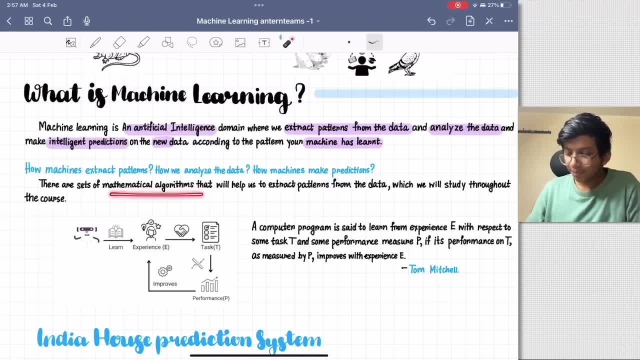 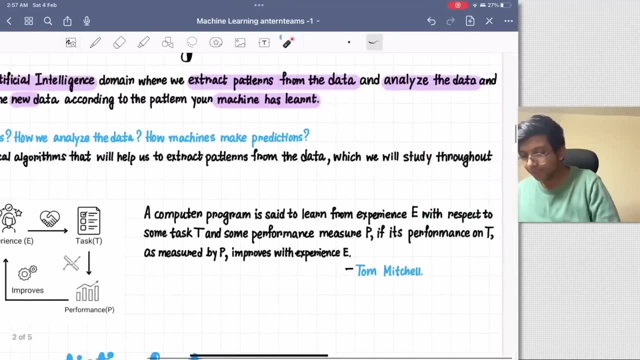 their set of mathematical. as of now, the answer is their set of mathematical algorithms. that helps us to extract patterns, mathematical or statistical algorithms, from the data which we'll study throughout the course. okay, uh, so that's an answer. so let's go to a more formal definition, which i 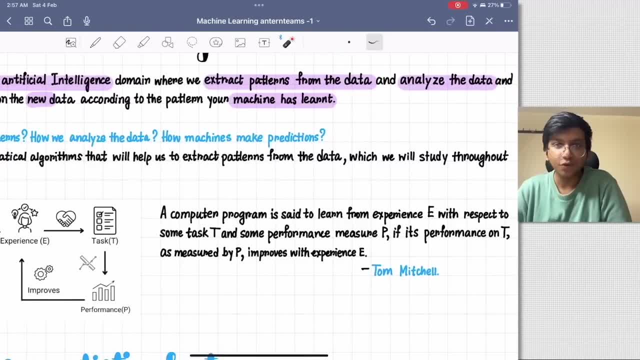 really like by tom michelle, and that's here's a nice book i recommend you read. that is a nice book, very nice book. um, if tom michelle is seeing this, i don't expect him to be seeing this, but hi to him, i'm just kidding. uh, he's my one of my big inspiration and machinery field. to get started, 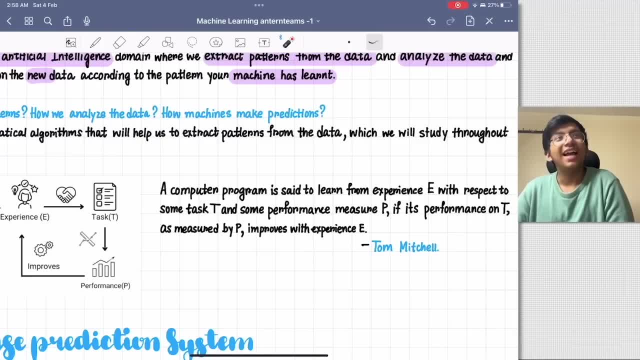 with his books on machining is really, really influential, and his lectures as well. so nice a computer program is, say, to learn from experience a with respect to some class of a task t and some performance p, if its performance p on on task t as measured by p improves with experience. 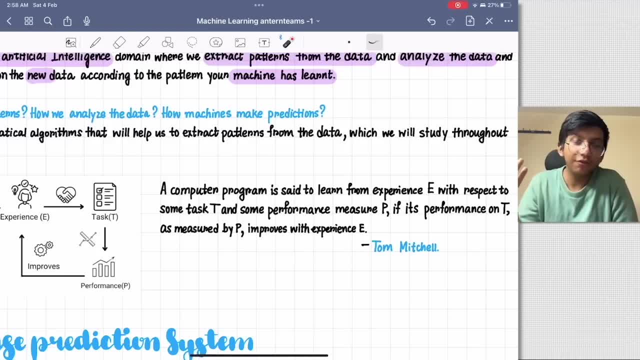 e, if you got this, very nice, if you know. if you don't, that's totally all right, because i was also the one, even in in my middle of the phases, i was not able to understand this uh definition. this is by tom michelle. okay, so let's understand this definition by this flow chart which i prepared. 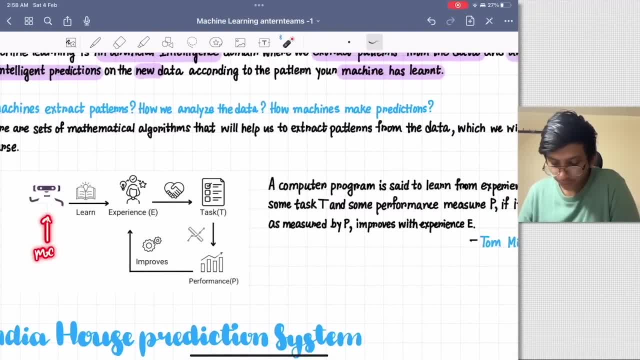 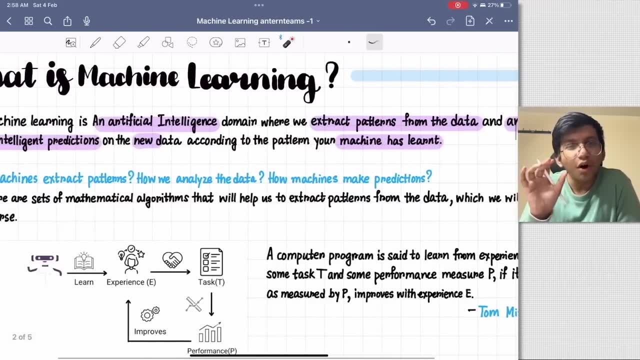 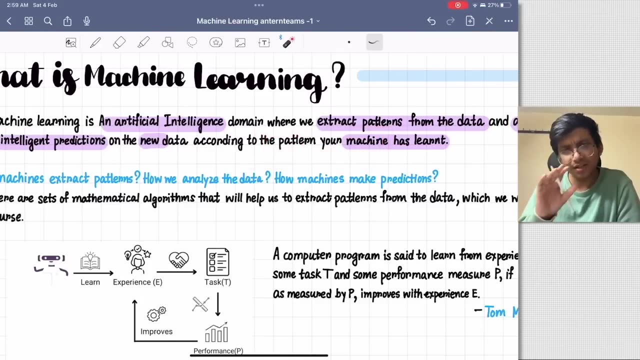 for you. so you have a computer program, assume that this is your machine learning. machine learning, uh, whatever you come to program, what is model? i've been taking model name right, so assume that model is a machines as of now. okay, machines, assume that as of now i'm just taking model. just assume that as. 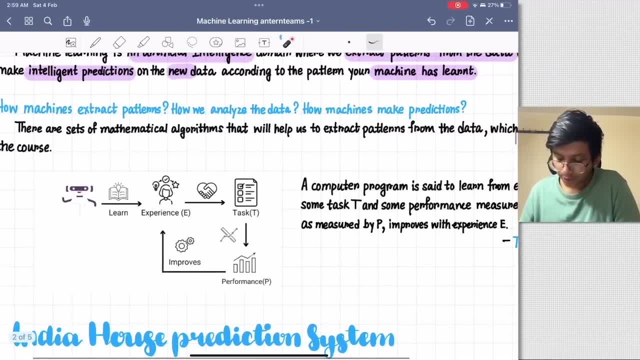 a machines. this is not having so much of jargons. so you have this computer program, you have this computer program. that computer program learns from the experience e and in this case, experience e is your data, your computer program. they learn or analyze, extract patterns from the data. 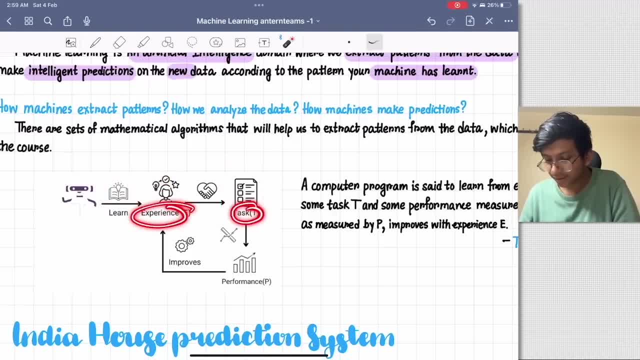 for some task. the data is for for some tasks, right? so, for example, if you have a spam or ham data, spam, which is a collection of information of the spam emails and ham emails. so that's the experience is available now. the task was to identify spam. so that's what for that task and that performance. on. 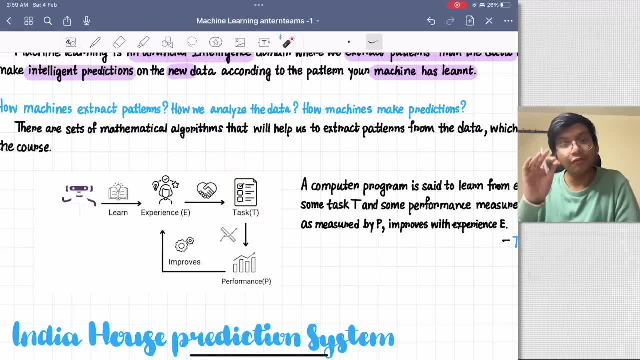 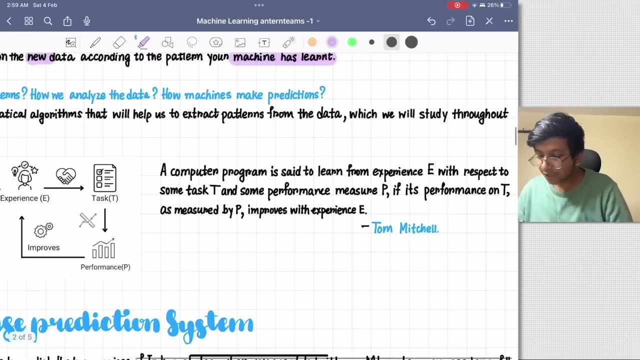 the task is measured by p, so we measure the performance and once we have the performance, we improve, and that performance is in being improved by adding more data or adding more experiences in that. so that's what exactly it says, highlighting the important terms it said to the. 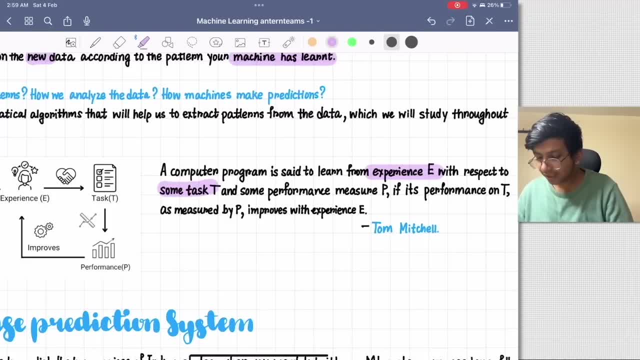 learn from the experience. e with respect to some task t and some performance measured p. if the performance on t- the tasks spam and ham- measured by performance, if they're measured by this, it improves the experience. if we, if we increase the experience experience, it will also be, it is going to be improved. so this is a definition. 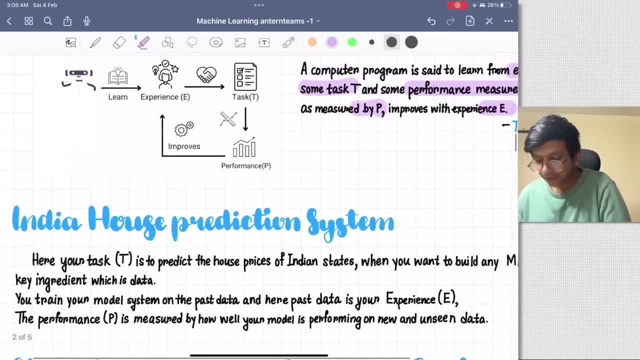 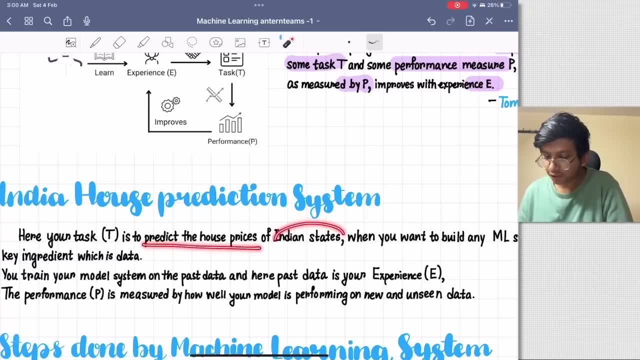 by tom mitchell. i hope that makes sense. another example is indian house price prediction: indian house price prediction system. so here your task is to predict the house prices of indian states. where you want to build any ml system, you need one of the key ingredients, which is data, which is 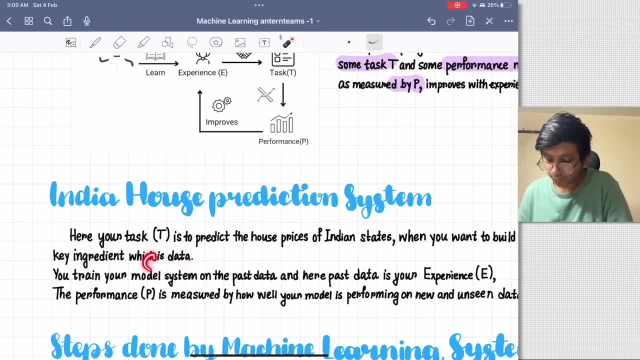 in this case you have experience. so your training model, which is your computer program on the experience, and this is the on the past data, which is experienced, because past is experience right and here past data is your experience. so the performance p is measured: how well your model. 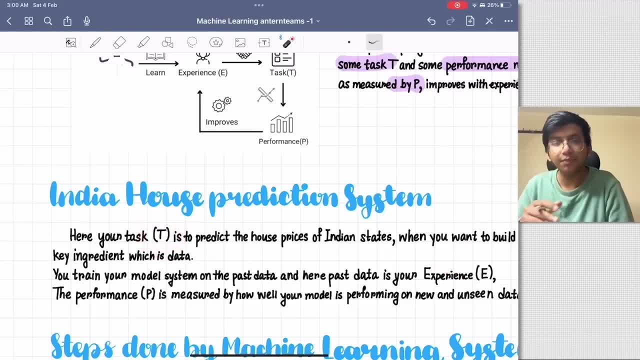 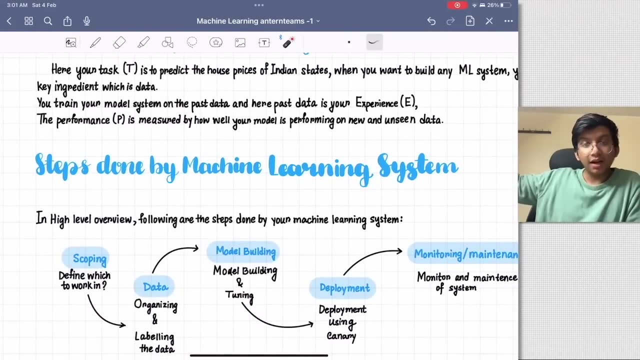 is performing on that particular task and if you add more experience, the performance will be improved. that's it. that's the definition, very easy now. i hope that you understood. do it for other applications. very, very, very nice practice. however, if you, if you want to do the practice all along, please enroll in our official ml course as well, as well as you can also. 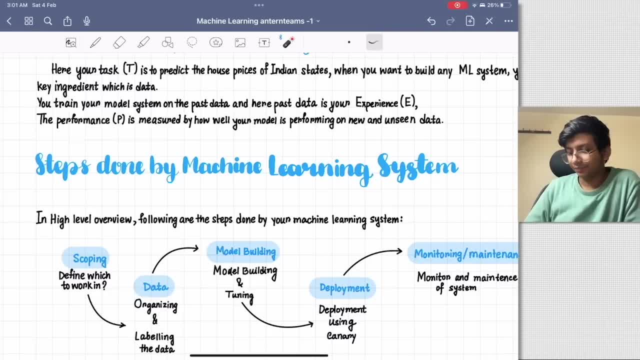 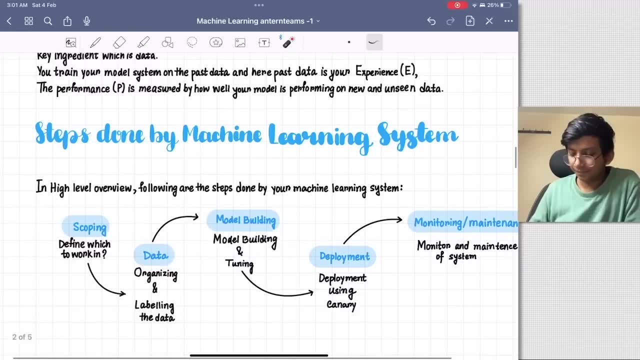 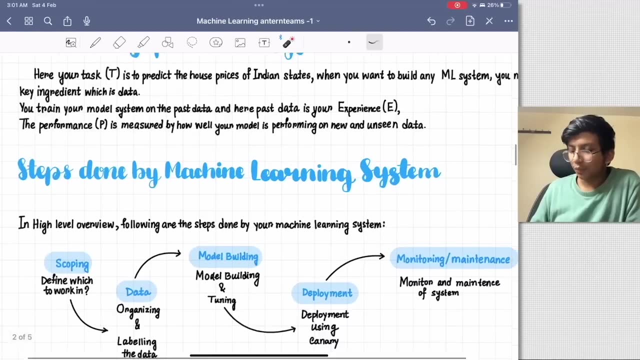 go um and review. some of you know, uh, our um courses available, or the, the free lms which we ask you to enroll in. good, so what are the steps done by your machine learning system? so that's something. what steps your machine learning follows to actually do this? i know this is early phase to talk about. 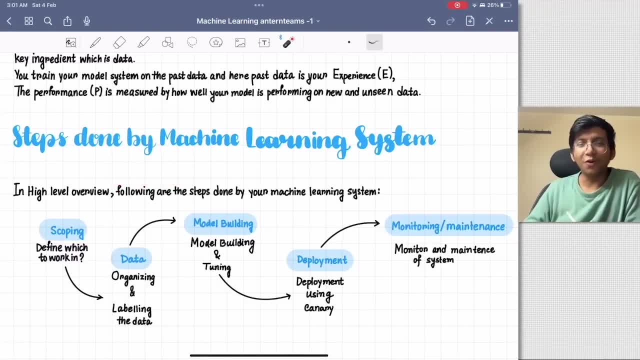 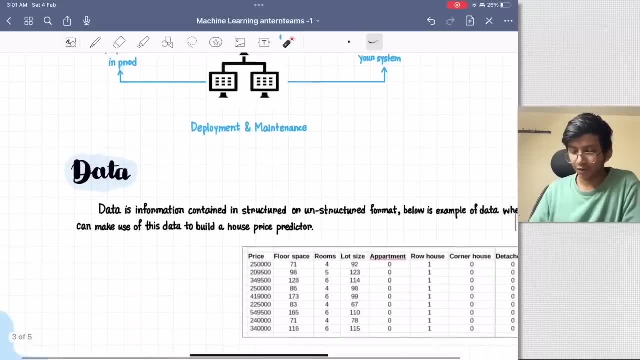 that that's something is super important, which i want to have a talk, heart to heart talk with my viewers on this. however, if it's okay, if you don't understand it, but i won't just want to have a heart to a talk with a very detailed explanation of everything, and then we'll talk about data. 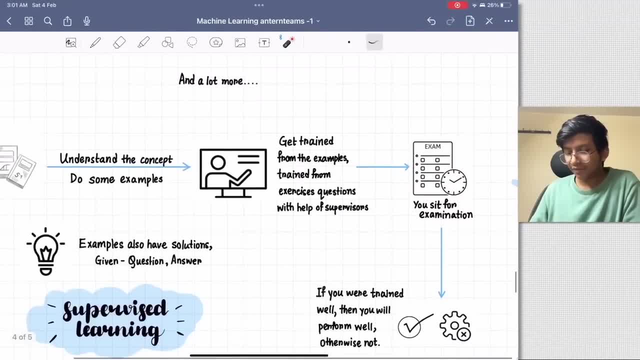 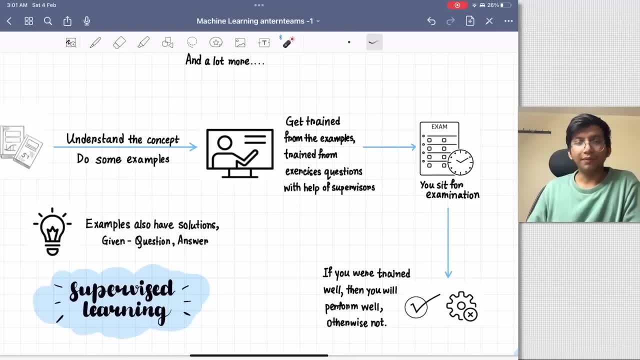 and then uh, and after that we'll talk about some of the applications and then we'll uh talk about a very nice uh application or the type of machine learning which is supervised learning. we'll talk about unsupervised later on, uh, but as of now i'll talk on supervised only. 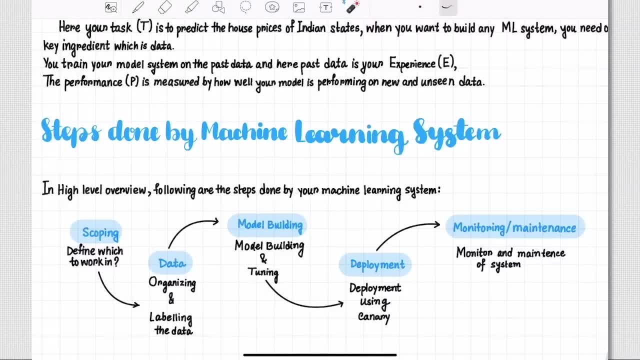 so, hey, folks, welcome to this video. in this video, what i'm going to do is to talk about some of the steps, uh, which is done by- usually done by- machine learning system. so what is the procedure, what is the process for going through, uh, for, for building a 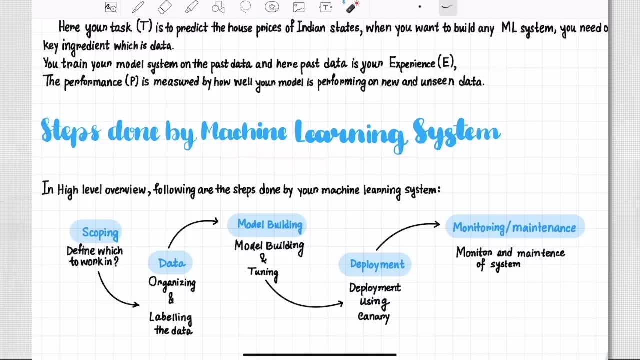 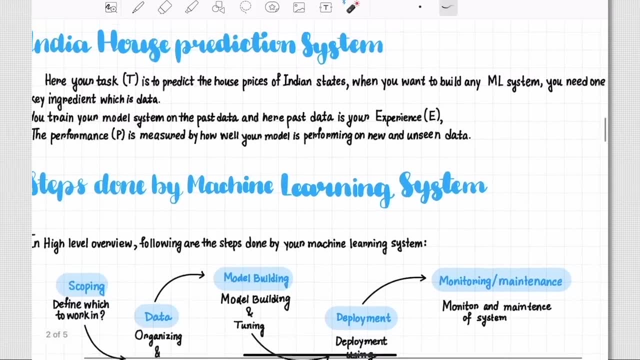 a good machine learning system. what is machine learning system? the system in which we give an ability. we give an ability to a, to, to, to, to a machine to be able to, to learn from the data, which which means to be able to learn from the data or extract patterns from the data. 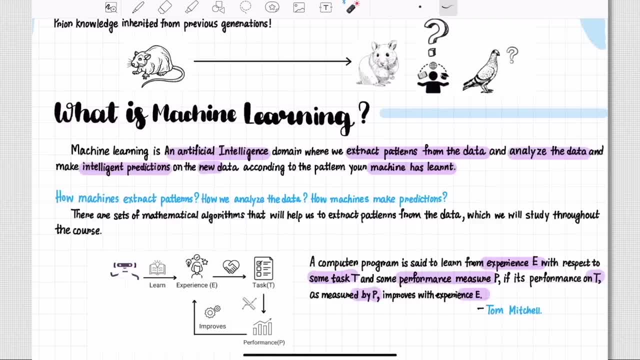 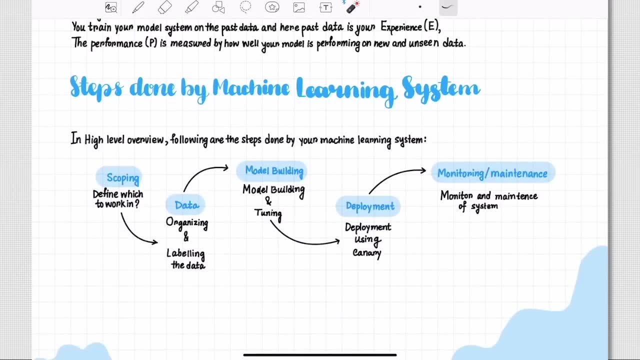 and make intelligent predictions. so, you know, make a machine, a system. what is the process of that system, where we extract the data, we analyze the data and make intelligent predictions according to what it has learned. so, um now, so what the like? everything, for example, like, while creation of, you know, maggies or any. 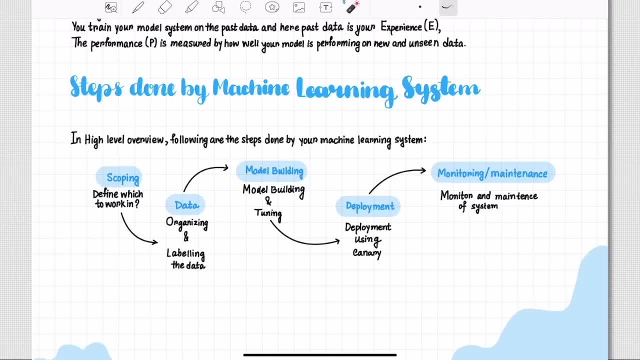 sort sort sort of foods. you have a processes, so just like that like while creation of machine learning system, there's a processes created or recommended processes, which i really want to talk to you guys. so let's get started actually with that. um, so it may happen, some of you may not. 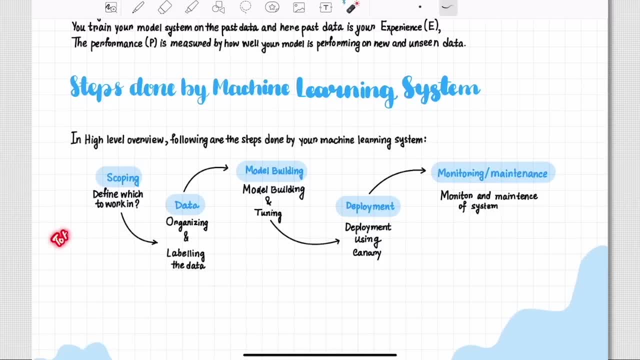 understand the fully thing, that's totally all right. totally all right if you don't. and if you don't understand it, because i feel like it's, it's something which you might focus on, things like um definitions and the understanding core and the crux of what exactly each step is doing. 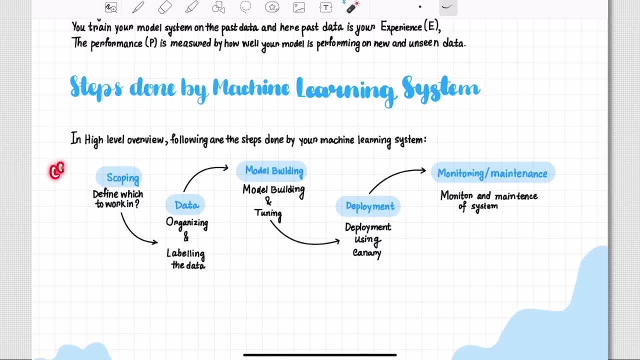 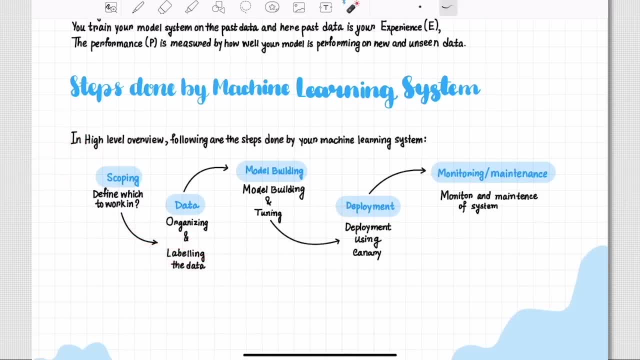 talking about several case studies and also, if you're interested in something you know, learning in depth and all, i recommend uh cs01 if you want to learn something fully. so now, coming back to this, you have something known as scoping. so you have something known as scoping and what. that's what. 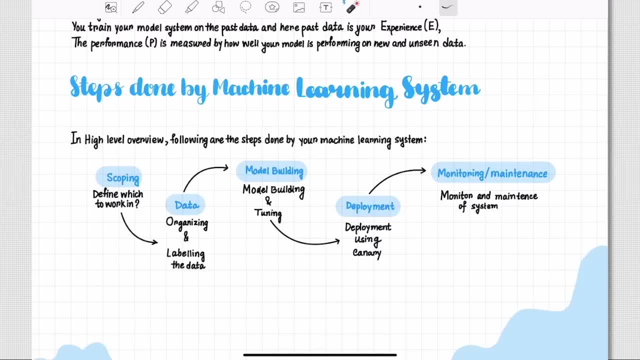 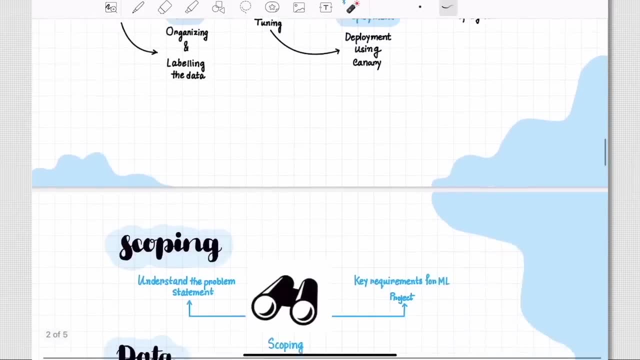 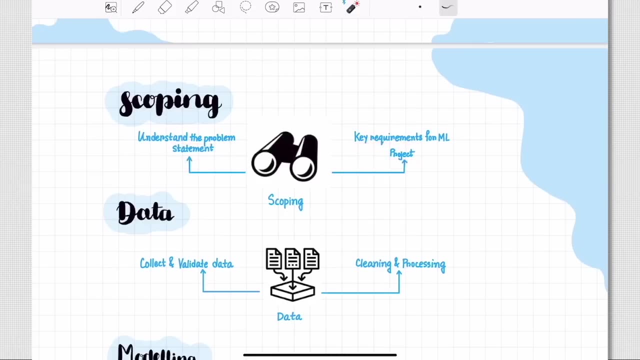 does this? scoping means scoping is something like: uh, the first step in your machine learning system is: scope out the problem you're trying to solve. scope out the problem you're trying to solve. the first step is scoping where you, where, what you do. you understand the problem statement and write down, or jot down, the key requirements for your 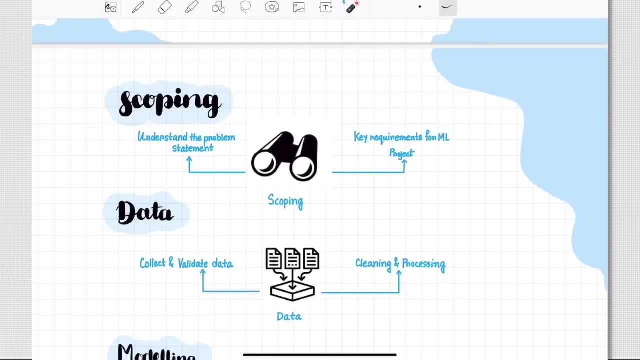 ml project. so, basically, whenever you start off with any sort of project or machine learning project, machine learning, any sort of machine learning project, so what you do over there, um, you simply first of all understand the problem statement, right? you? you understand the. for example, let's say you're building a spam or a ham classifier. so you have a system, they have a machine m, you're. 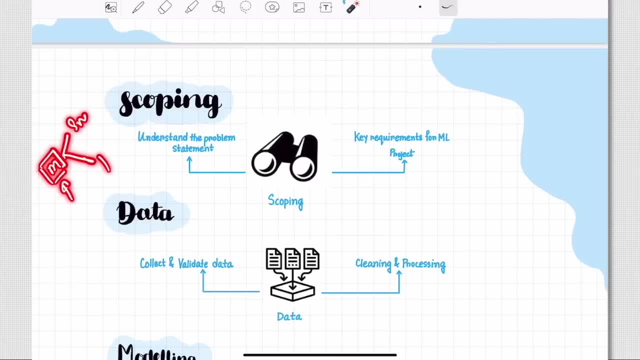 gonna build a machine m that that classifies with the whether that is a spam or ham, right? so the first step is scoping, where you understand what exactly this problem statement is. what, what sort of data which you have, right, what sort of data which you have? what are the key requirements? 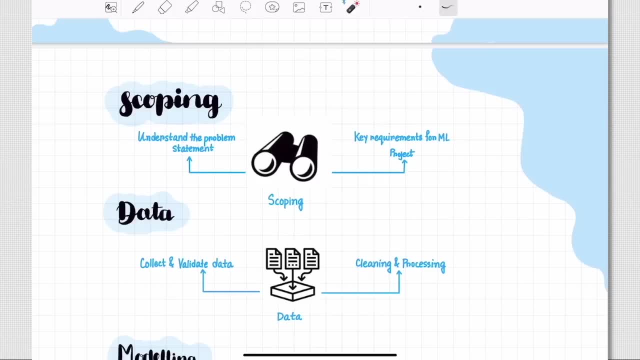 like key requirements, what is useful analysis, you understand the problem statement according to given by the stakeholders, and the second step is you understand key requirements like: do i require the? how many data scientists to work in this? what, what should be the compute power of this, what should the infrastructure required for this, etc. so scoping out means. 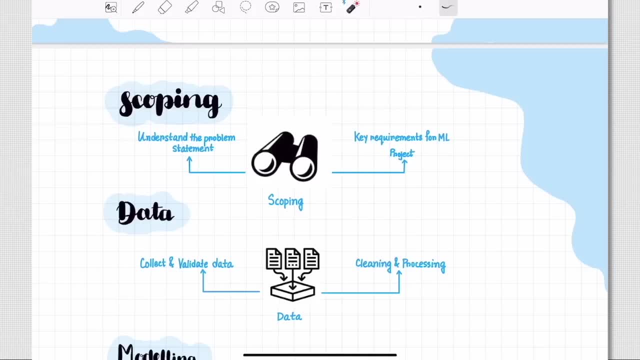 getting a brief understanding what this project will be about and creating a brief plan of go-to strategy for working on this project. then, after you have a brief plan and everything, now what you do- you simply go to the data part where you do, where the examples of the steps is now. 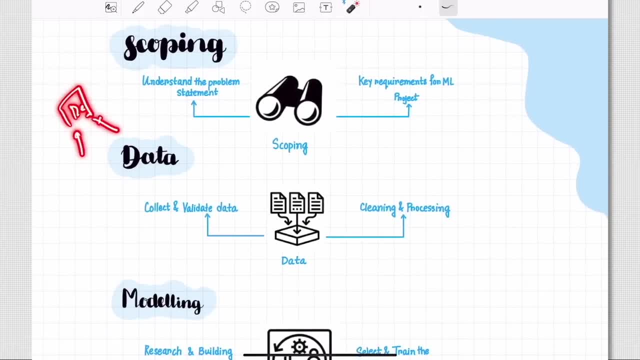 now, once you have the data, you have to eventually clean it. we'll talk about data cleaning and all in one of our project. so when you have the data, when you have the data, you have to clean this data. you have to clean the data, your processes, you have to process the data in a good 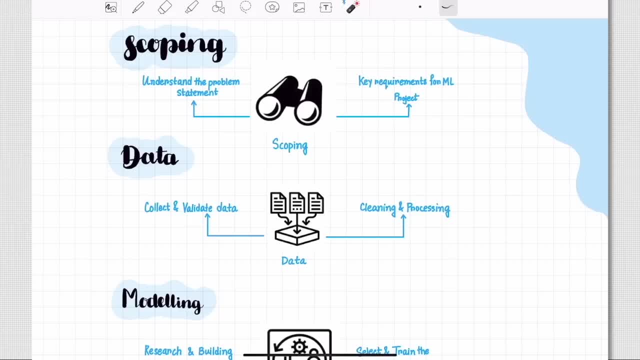 way and etc. so basically, what i'm trying to sell over here, what i'm trying to tell over here, that, given the data, you know you, you want to, you know uh understand it, you wanna to uh clean it, etc. so i think the and then you have the data, then you cross, collect and validate the data accordingly. 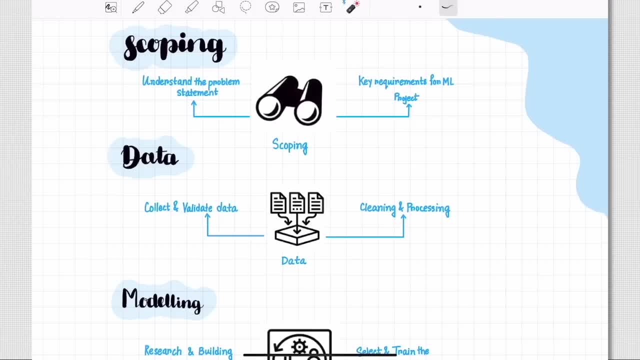 right. and then you clean the data where- uh, where- you have removing of missing values and etc. so i know that this, this will not make sense if you're a beginner. so it is something like you have the very bad data, you convert that to a good data by data cleaning and etc. 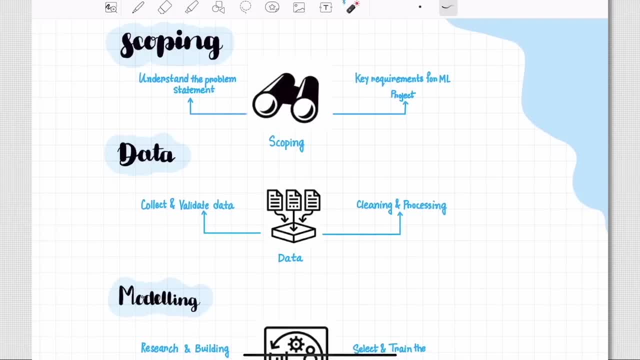 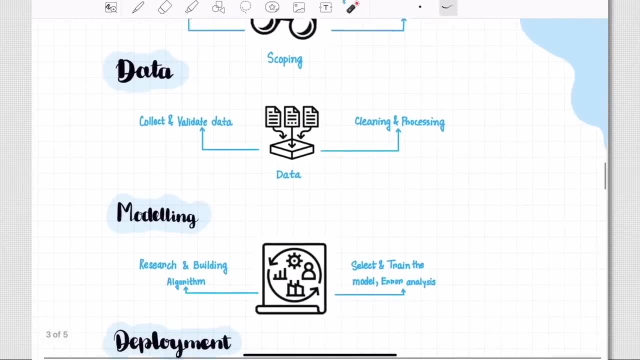 you validate the data, whether that data is from truthful resources or not, whether we can trust the data information or not. now we have the data now. now what? now what we need to do. we need to extract patterns from the data. and for extracting patterns from the data, we have something like: 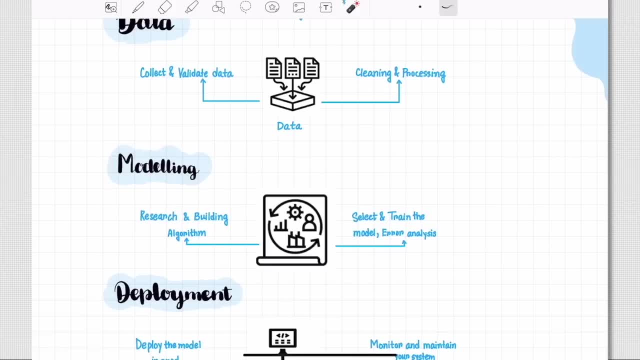 modeling, not something which actors do on a ramp work, but i think, on this, modeling requires something like you know, uh, some, something like your, your, your system tries to extract patterns from the cleaned data which you have right and then, once you have the once, once when, once you're done with modeling you have now you're gonna put this, you're gonna. 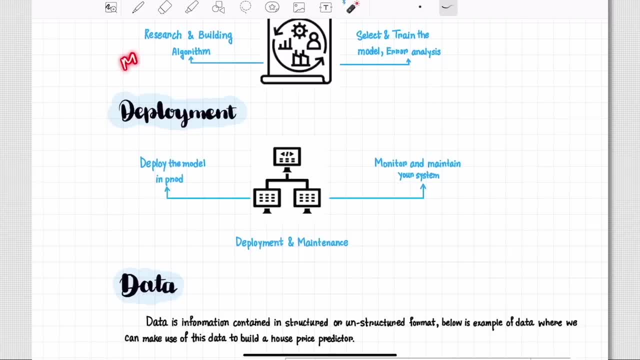 put this so that your users can make predictions from this model m. so once you have the trained model, get it low with learned extract pattern. so now we want to make predictions for it. for example, we're going to put this in production so that it is able to classify, so that every email can get. 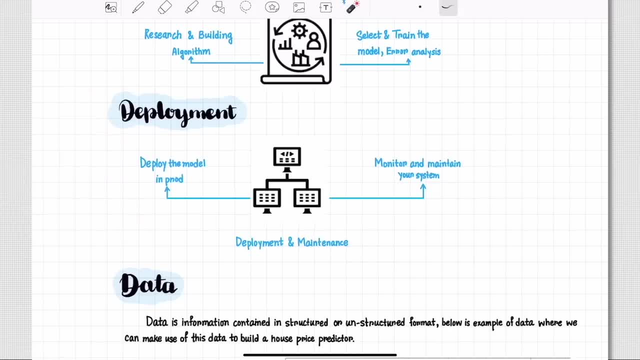 to this, and the model is able to classify a couple of stuffs, which is spam or ham. so we're going to put this in production so that it can be used by folks, um, in real time, and also we monitor and maintain our system. we see, uh like, how our system is performing. what is the like? whether a system 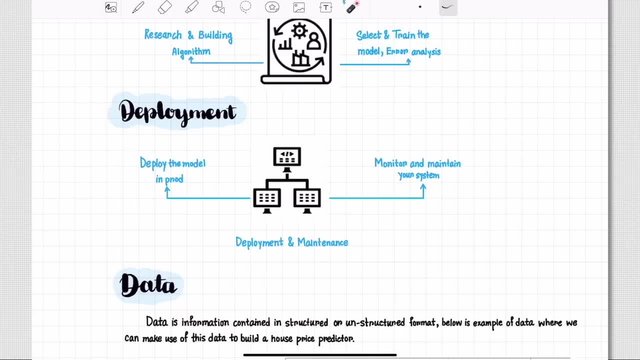 whether a performance of a system is degrading or what. what is the possible errors which are coming, what is the etc. etc. so what is the wrong predictions for which are coming, etc. so we have to monitor our system as well. there's four steps for any uh. 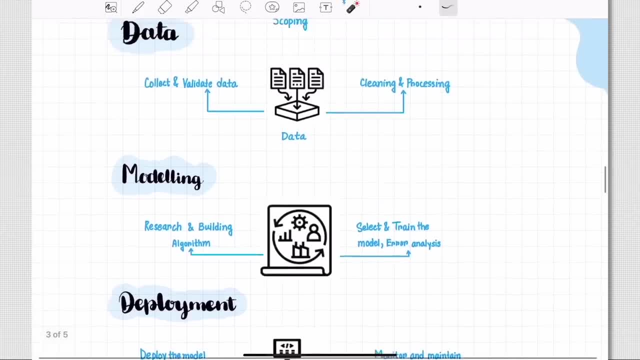 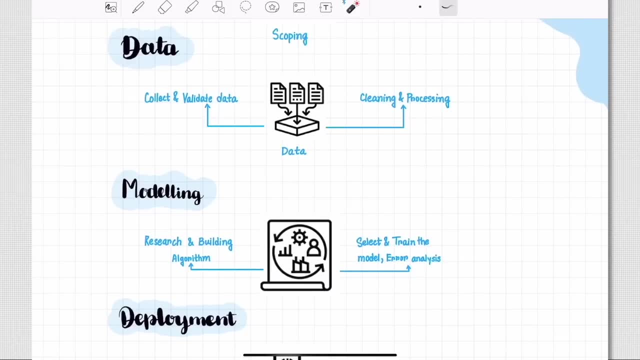 there's four to four to five steps of recipes of machine learning, where you first of all plan out what exactly you need to do by understanding the problem statement, and then you get the data, and while getting the data, you have to validate whether that data is from truthful resources. 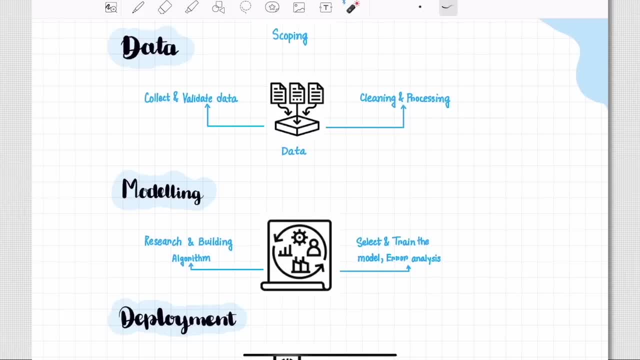 and clean the data in a good data. and once you have that good data, now you model it, which means that you extract, you learn to extract patterns from the data. and now you have the model which which has the patterns from the data. it should be able to successfully, you can use it in the production right and then and then. 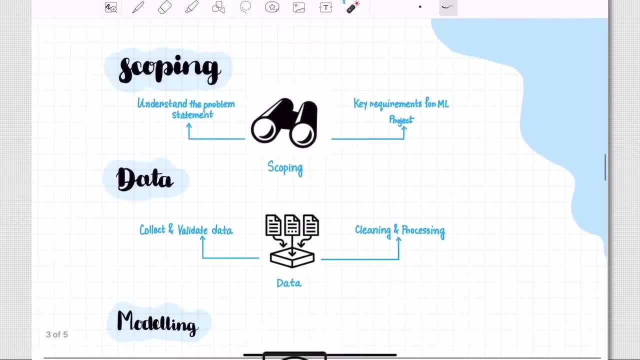 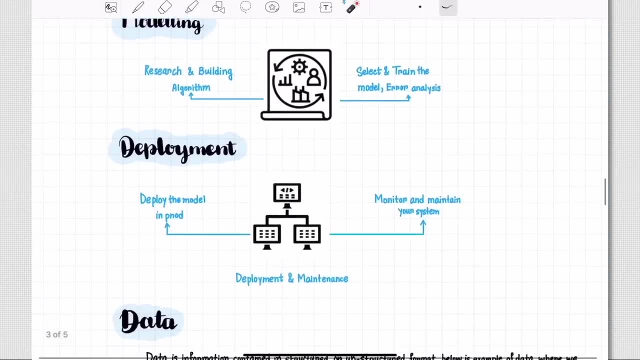 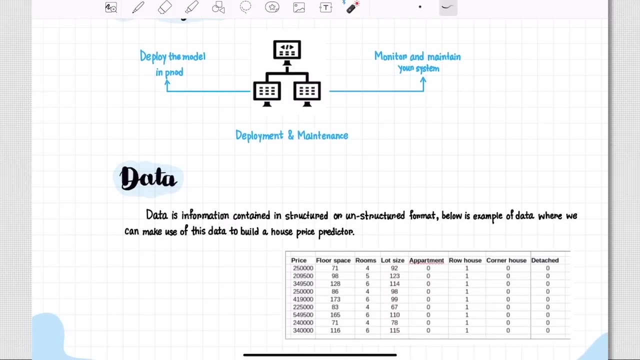 you have to continuously monitor it. so these are the steps for your machine learning uh applications. now, now let's talk about uh. i hope that this, this makes sense. but now, now let's talk about something known as data. so what is data? so data is info. it is in information contained in an 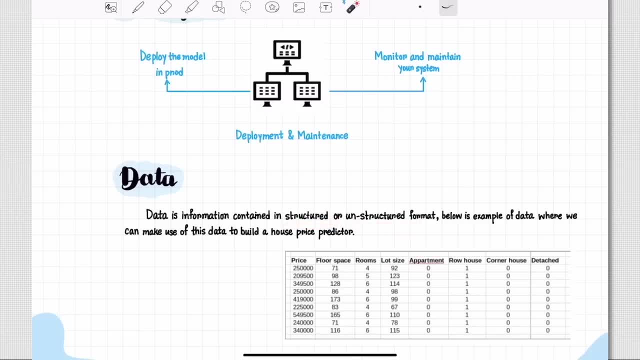 structured or unstructured format. so, um, so, data is set of records. so you, you might have seen in your, you know, machine learning lectures or, sorry, uh, in your class, eight or nine lectures of computer science where you might have gone through. uh, a data is a set of records, right, it's a records or set of information available for the particular uh. 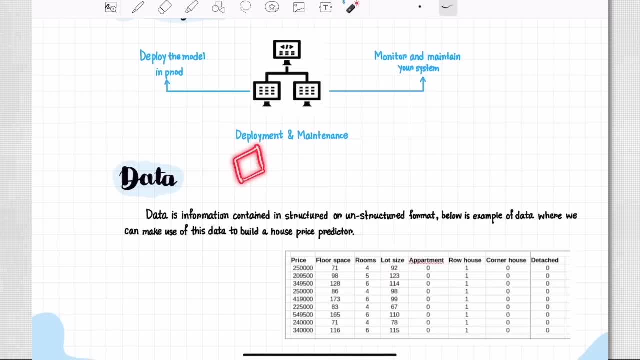 product. so, for example, you have amazon listing. you have amazon listing, let's say you have, you have mouse, right, you have mouse, so that mouse might have several, several data, right, several data like what is the description, what is the price. so these are the uh set of records for the particular day. 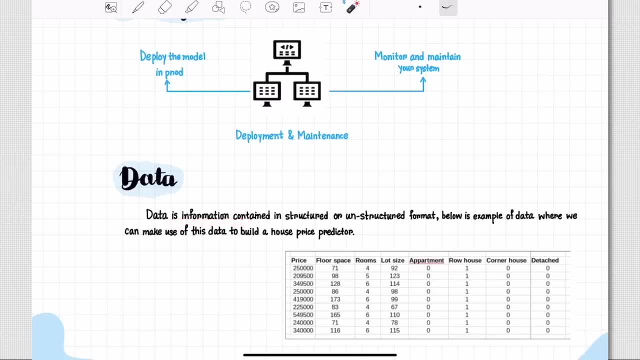 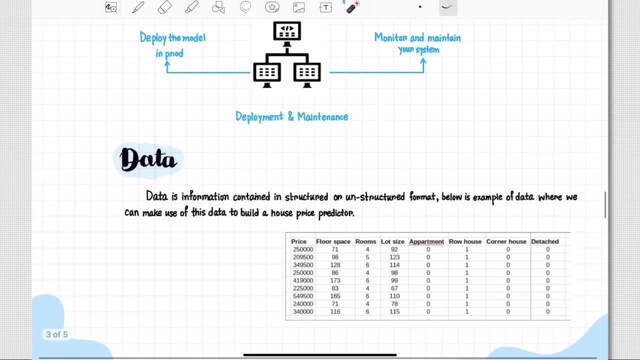 product. so, just just like that data is an informa in information which is in structured and unstructured format. okay and um, what we'll talk about what is structured and unstructured in a bit, but here's- here's an example of a data where this is an example of a structured data where 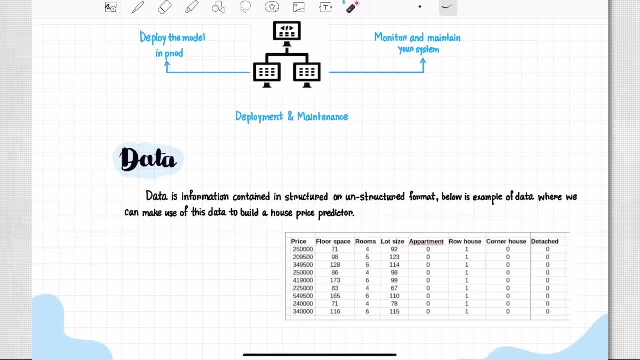 it is contained in a table where this data contains the, that it is the data of house price prediction, where we are given the some of the information about the house prices. uh, house housing price data, where we given the some of the information about house prices, which is first. one is the floor. what is the floor space? how many number of rooms in that apartment? how? 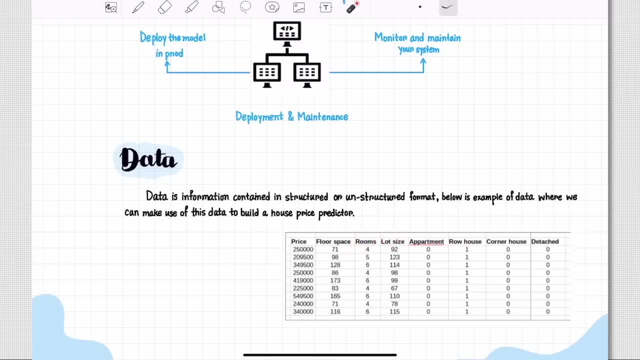 what is the lot size? is there any other apartment attached to it? right row house, corner house detached. so these are the information for a particular house, right? and this is the price in one thousand dollars, right? so this is a price for the for for this feature. but this feature, this is the price, uh, for that particular house. 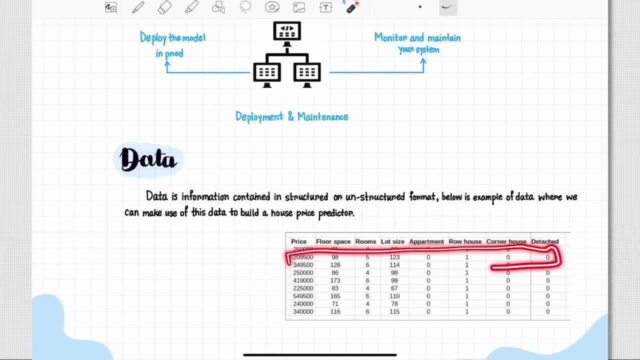 then, for we have the second data point. this is the. this is the. this is the record for the second house, this is the record for the third house, the record for this first house. second house, third house. four thousand five thousand six thousand seven hours, six, eight and nine out. so you have. 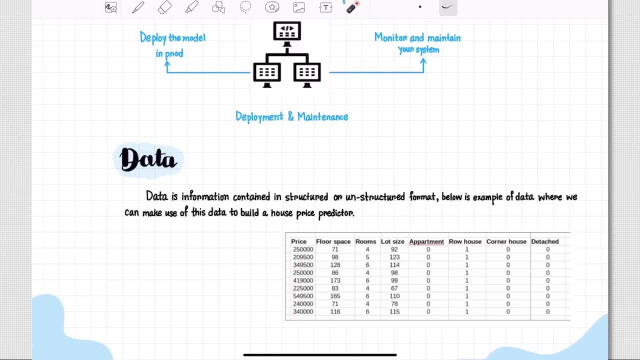 the nine, nine houses where, for every houses, you have your own infos using uh, including pricing, floor space rooms, etc. so these are nothing but uh, uh, these, uh, these are nothing but you know your data, where we actually have something, uh information contained. right, cool, so now what we do. 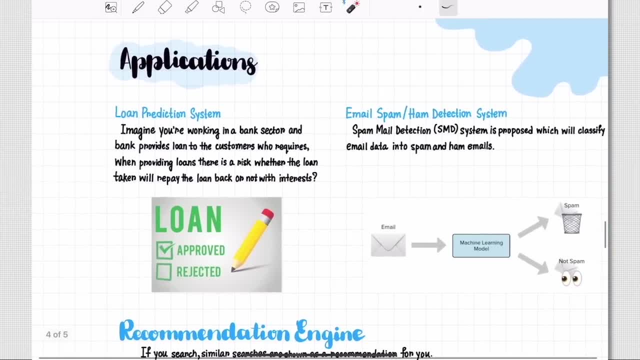 now what we know, what, what? what we're gonna do is talk about a bit of application, uh, in machine learning. right, the first application which we really want to talk on is a loan prediction system. it is an application. so loan prediction system is an application in which of machine learning. 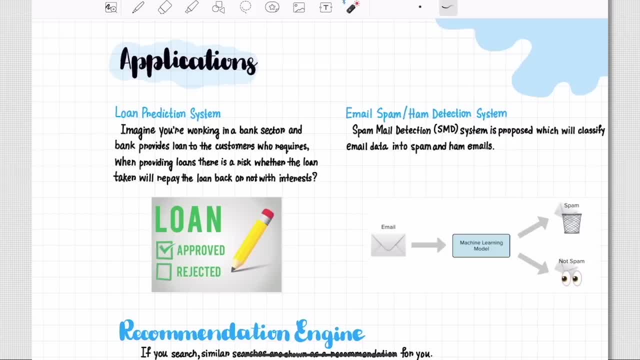 so assume that you are in a banking sector and you're in a banking sector and and bank provides loans to the customers, right? so you might have visited loans and also your bank man might provide loans and also the customers who require rates. so now, so now you assume that you're working in a 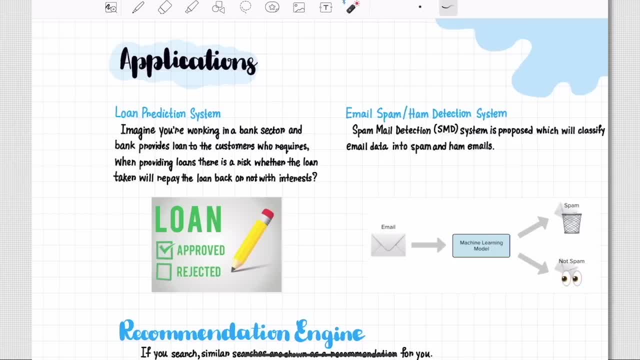 bank and then that that bank gives loans to the customers who requires the loans. so when providing loans there is a high risk that that that the person may or may not return the loan. so the risk is that the person will not return the loan back with interest right, it may return loan back, but 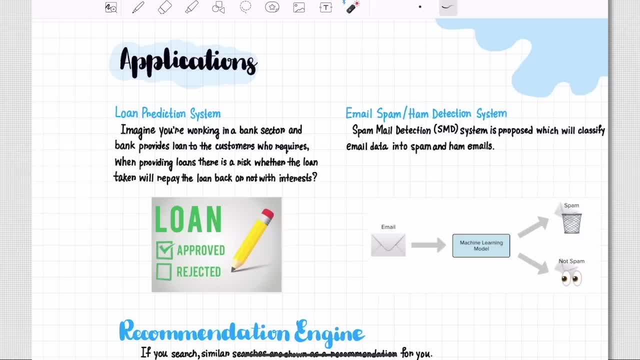 are they going to return back with interest or not? so, given the background information about the particular customer- what is the history of them, like salary, etc. etc. we've given those infos. we're going to predict. we're going to predict whether we should give loan to that person or not. 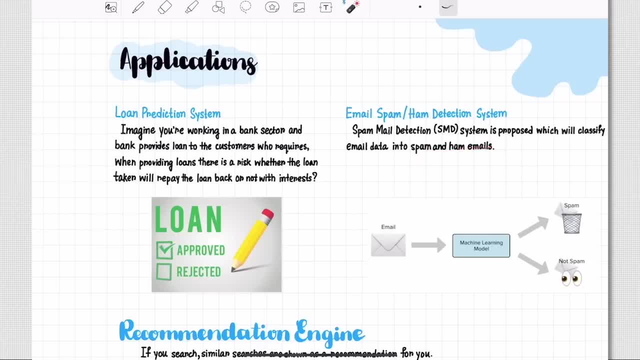 this is one example. another example is the spam ham detection system, where you prove it. another example is spam ham detection system: uh, where you have, where you've given an email, you know classify with the whether that email is a spam or have recommendation engine you might have. 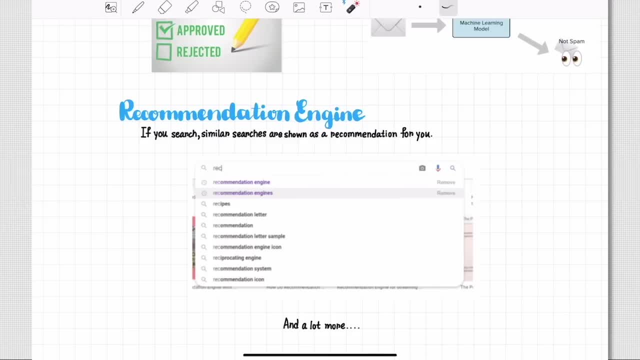 searches with something like this which you're seeing in front of you. so this is a recommendation engine, uh, in google searches, or maybe recommendation engine in your youtube. so these are a couple of applications which you might have already seen. i don't intend to, you know, just just. 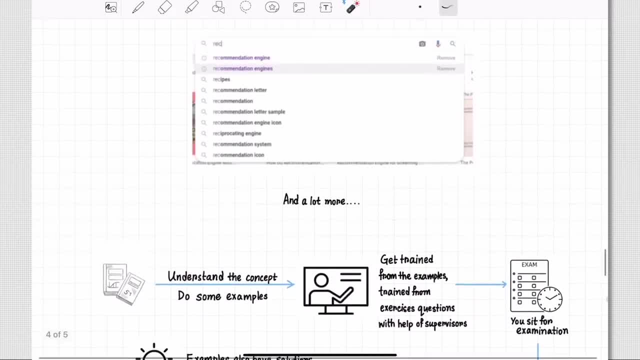 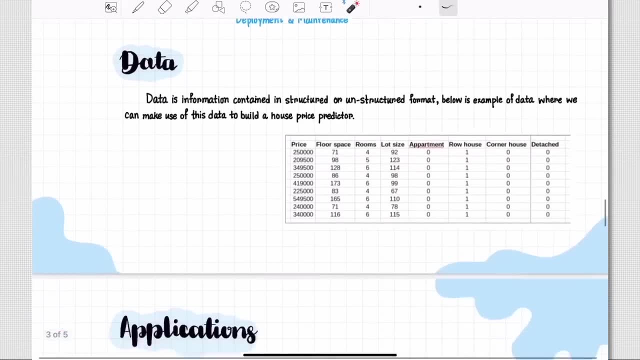 to give you a feel about it. so i hope that you understood uh in a nice way about a very good processes of machine learning. what i want to achieve in the next set of video is talk about the last thing of this uh to talk about. the last thing of this lecture is to talk about. 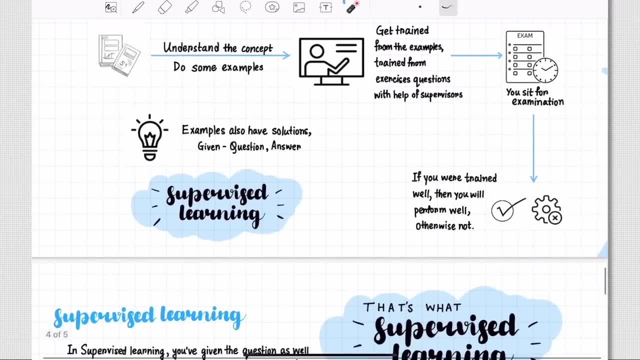 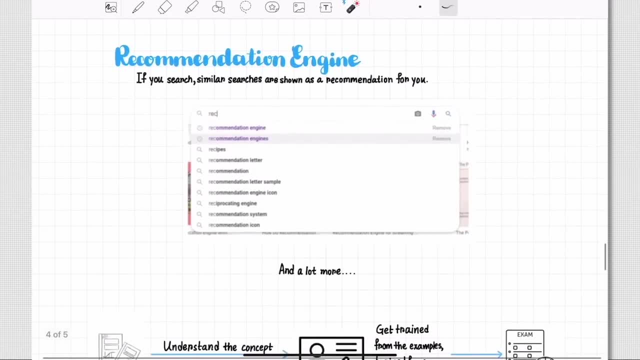 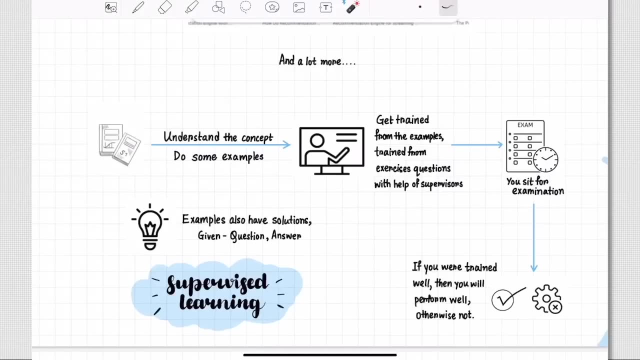 supervised learning, and we'll try to learn supervised learning with a very visual and very storyline of examples so that anyone, even if you're class five, you will be able to understand very easily. hello everyone, um, so now we'll talk about something known as supervised learning and hello everyone. hello everyone, we'll talk about supervised. so now we'll talk. 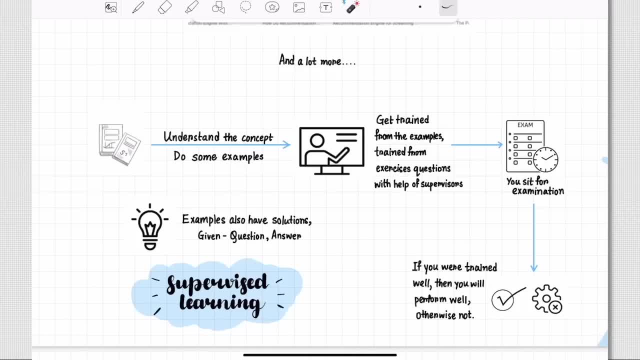 about supervised learning and, uh, we don't want to directly get started with. you know definitions at all. i want to tell you a very nice storyline or very nice example relating it to the practical stuff. so let's get started with that. the first is is to understand the concept. so now, so now, whatever you're seeing in front of me is to 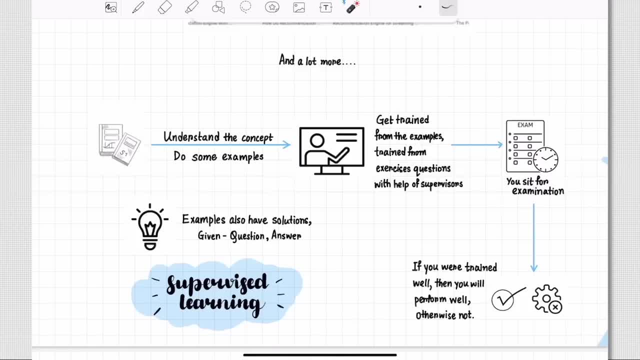 understand the concept, for example. for example, you have assumed that you are studying a mathematics book, right, so you're studying a mathematics book, and there you understand some concept. you understand some examples, right, so, you understand some. so, so. so you have a mathematics book, you understand, you know some concept, you. but you, for example, you have a quadratic equation as a chapter. 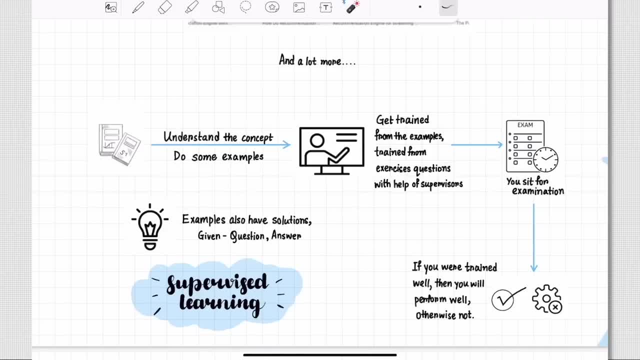 so you do some examples, you want to analyze some formulas, you want to analyze some patterns for solving a particular questions, and etc. so now you once have the questions, now what you do, you're trained with the text. you're trained, so now you understand the concepts. you're trained with the. 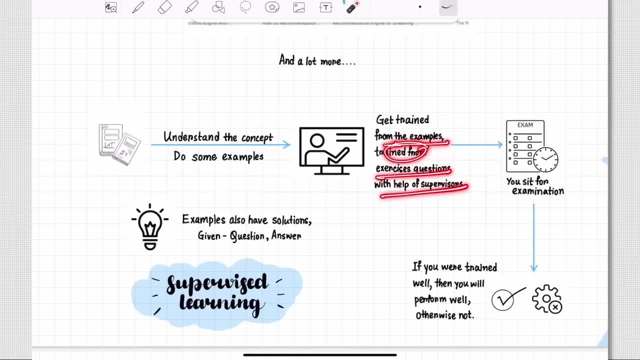 from the examples and trained for the exercise questions with the help of supervisors. so when doing exercise, you are doing examples, you're analyzing the patterns. so you're getting trained with the examples and exercise questions with the help of our supervisors. so of course you have a. you're also seeing the solution if you're not knowing, if you're up, if we're getting error in. 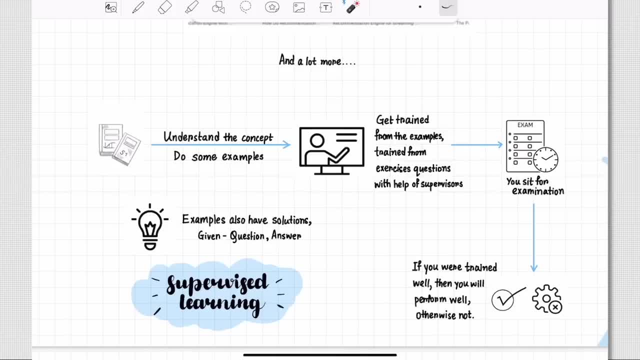 that question right. you're not able to solve that question, so you seek help from supervisors or whoever the instructor is out there. so by now that our storyline is that you understand some concept, you get trained from that examples. you do also do the back exercises, exercise questions with 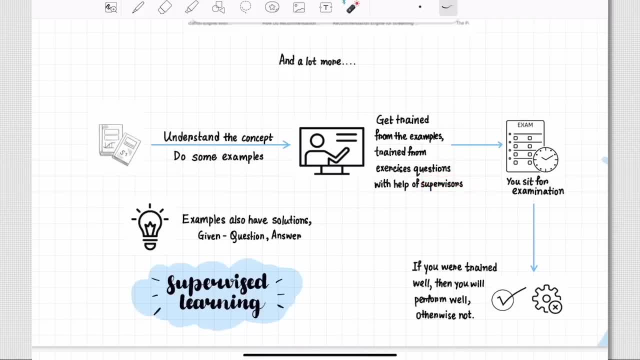 the help of your instructor and whoever. now, once you're trained with everything. now you sit for an examination, you sit for an examination and in that examination you're not, you don't you. you don't have any help of supervisors, you don't have any help of 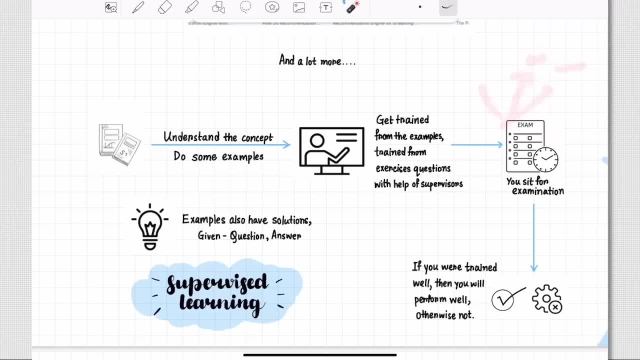 exercise solutions. you don't have any help of answer sheets, etc. right, so you sit for an examination and if you were trained well, then you will be performing well. otherwise, you'll be not performing well. okay, so this, this was your. uh, this, this will be condition after giving the. 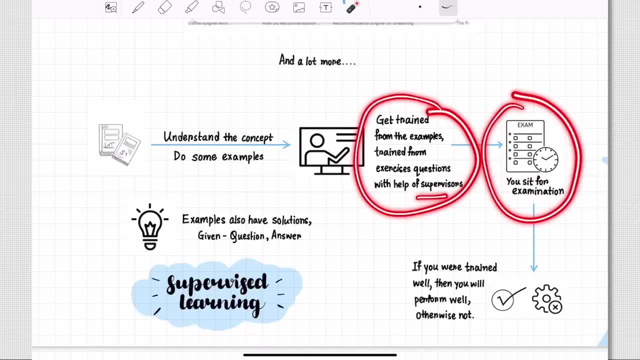 examination. so if you're, if you were trained well, with the help of your supervisors and everything, you will be able to answer it very well. so now, now you can see that how you were trained. you were trained with examples, questions where you're given question as well as the answer to it, so that you can understand the pattern right. 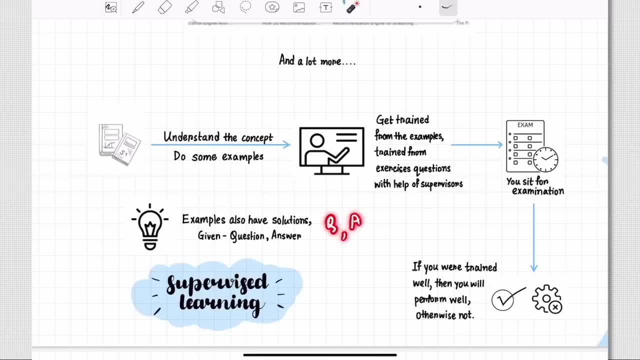 in exercise questions. you have a question as well the help of supervisors, which is question and answer. you have a possibility to see the answer right. so, just like this, you you're trained with examples and the questions. now you sit for an examination, you sit and give the examination. 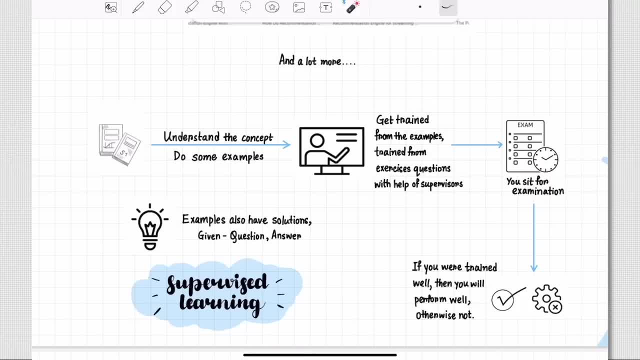 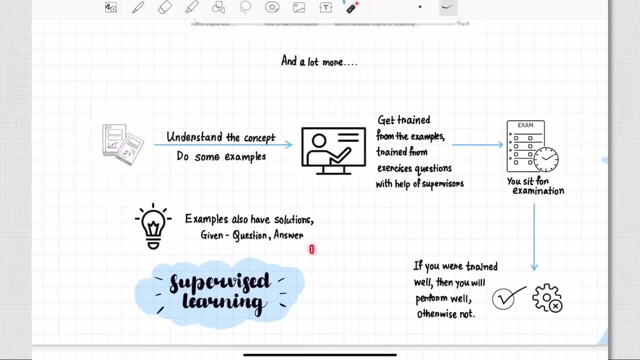 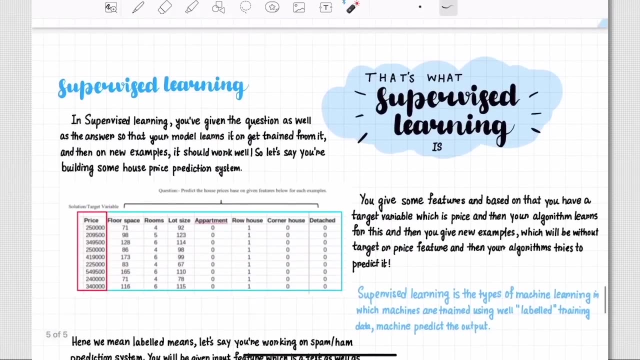 and then that will predict whether you're going to really um pass the examination or not. if you analyze the question well, you will be able to pass, and the whole concept is nothing but called supervised learning. so let's, let's talk about what exactly supervised learning is. so in supervised 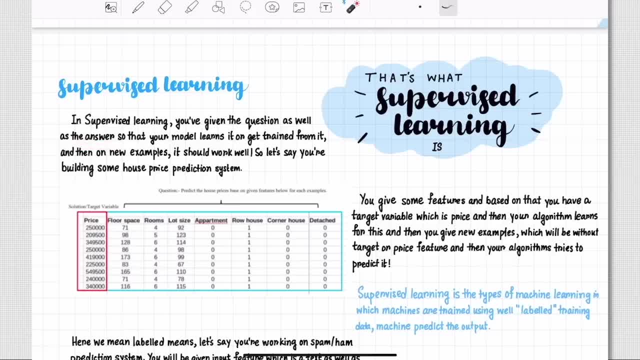 learning, you're given the question as well as the answer, so that your model learns from it and get trained from that right. so in supervised learning, you're given the question, just like this. just like in this case, you're in effort for for training for this particular question, you're given the question. 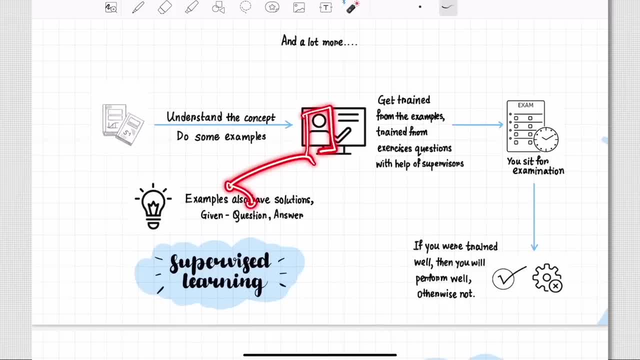 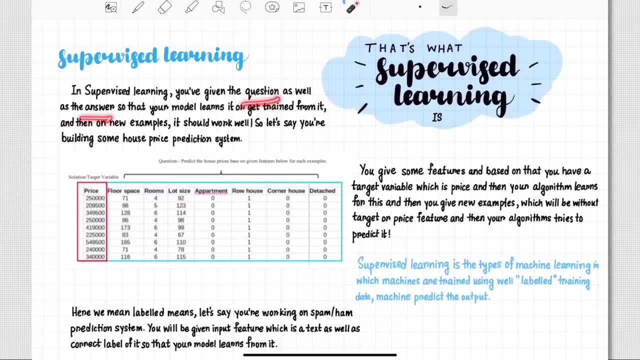 as well as the answer. so in supervised learning, you're given the question as well as the answer. so in supervised learning as well, you're given the question as well as the answer, so that your model learns to analyze pattern from it. and then, whenever you sit for an examination- which is the 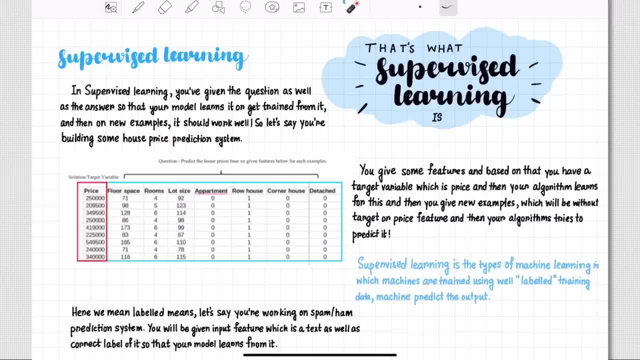 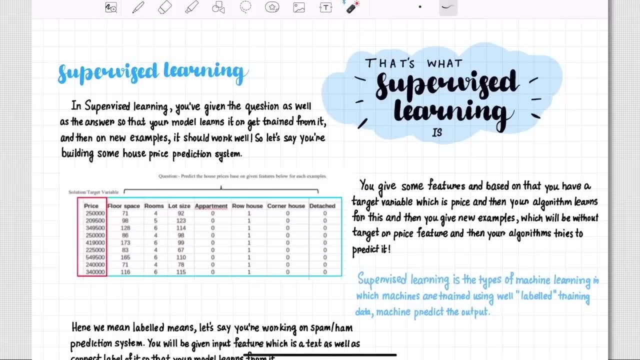 new examples. you, if you, if you were analyzed well, or if you're trained well, you'll be able to solve it right. but now, but now, what i want to do, but now, what i will really want to talk, is on something which is which you, which you might notice, is that, uh, assume that you have an example. 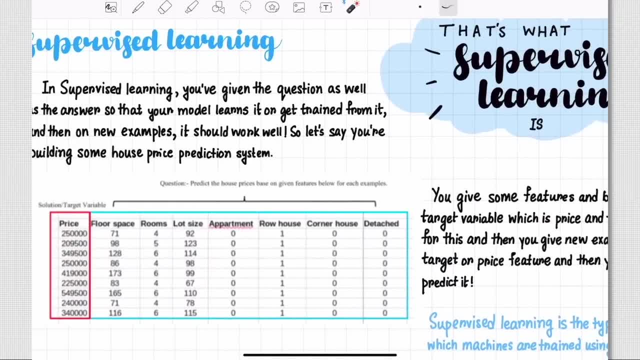 over here for house price prediction system. so you, so you have an example of housing price price prediction system where you want to predict the house prices based on the given feature. so you know, you know, you know you invest in real estate and you predict the house prices in the coming 10. 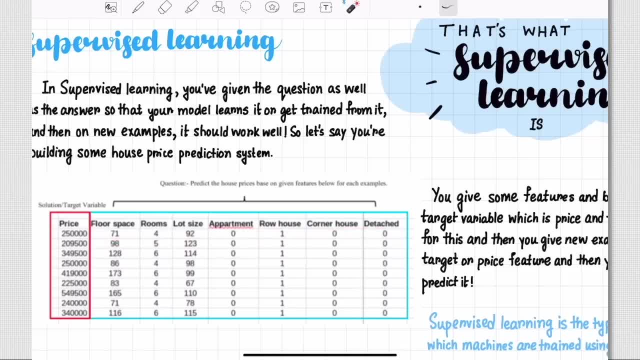 years by giving the following requirements for that uh reports for that particular house. so this house number one is the house number two, it's house number three. so, given this characteristics of the house we have, we want to predict the price of the house. right, given the characteristics of this house, we want to predict the price of the house. characteristics means what? 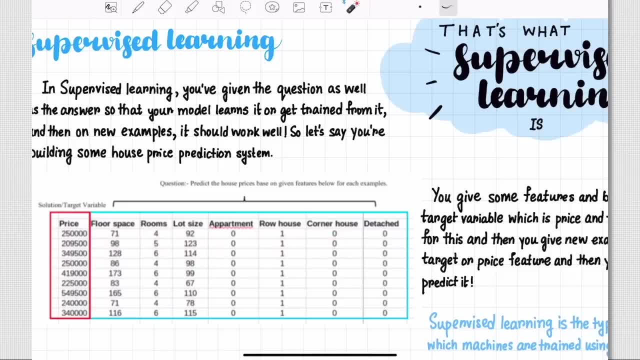 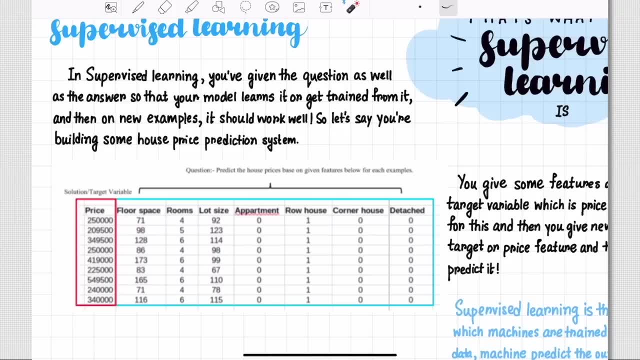 is the floor space, rooms and all. given all of this, we want to predict what is the possible price if we have this. so so now, first of all, we have to analyze it right. so any for every way, before sitting in an examination, you have to learn it right. so you're in supervised learning. we are 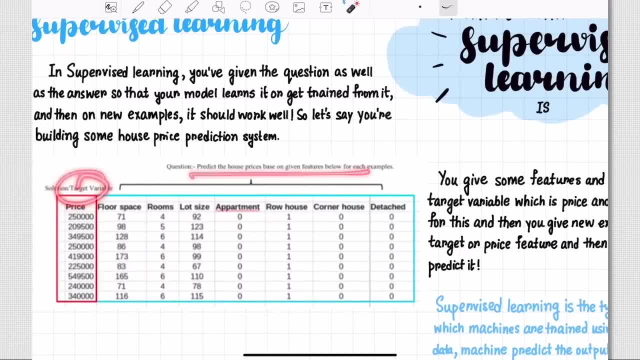 given the question, which is a predict, as well as the target, which is the solution, which from where to learn it? so your model sees the question. okay, this is, this is the question, this is the information given in a question. so any pro what problems has their own information? right, and they. 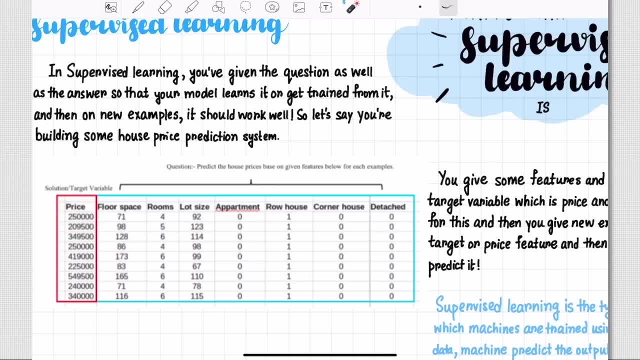 ask us to predict something, and also we are given the solutions as well. so your model will find the relationship between the price floors, pay relationship between solutions and problems and analyze patterns from the data, right, uh, and then, and then get trained, get, get trained. so over here this solution. this solution is acting as a supervisor for this model. 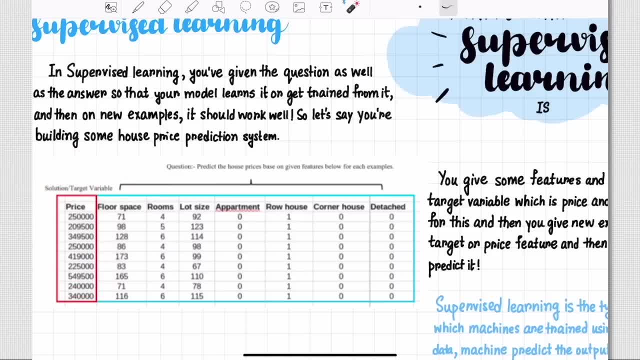 for this question. so basically, uh, this we, this is, this is, this is helping, this is helping your model to learn right if you don't have solutions. what example? you sit for a mathematical examination and you want to prepare for it. if you don't have the solutions, how will you understand the pattern? 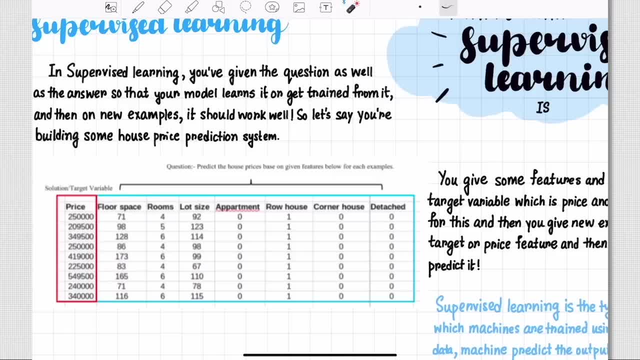 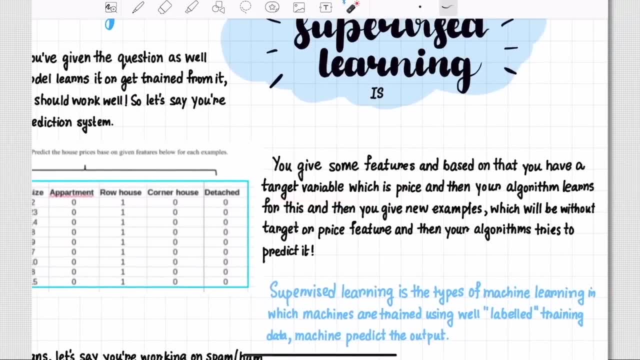 right. so over here you should have the solution. you should that that that that is called target variable, right? so you give some features based on that, the target, which is price, and then algorithms learns from this, and then you give new examples which will be without target. so 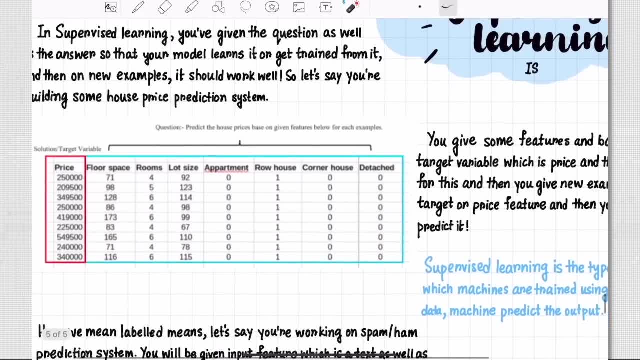 now. so now your model trained on this. now you, you want your model, set an examination where you only give this information, you only give this particular a question and then say, okay, predict the house prices based on the given info. say, for example this: now your model will predict this. 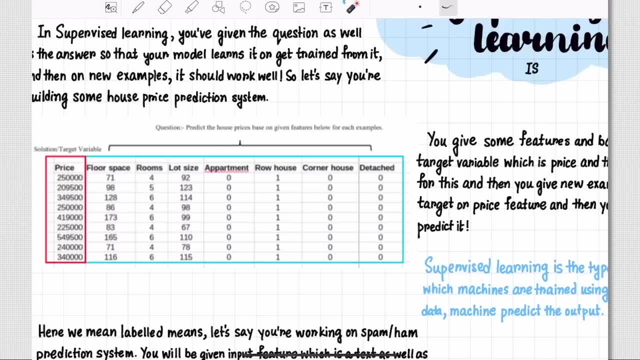 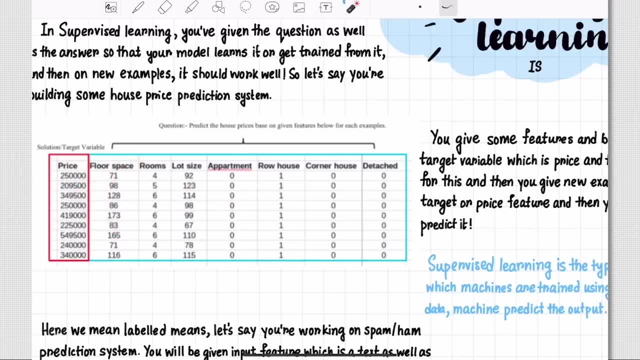 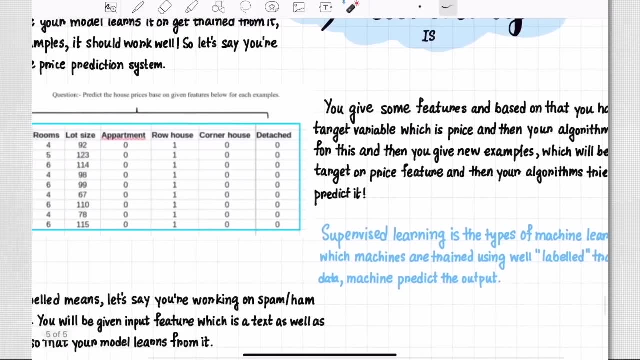 price you don't have to give this, because now, now, now it's our and now it's something will- will introduce to evaluation system, where it will check yes or wrong, right, which is, which is the which is the task of an examiner or a test checker. but as of now, once the model is trained, we can give only this question. 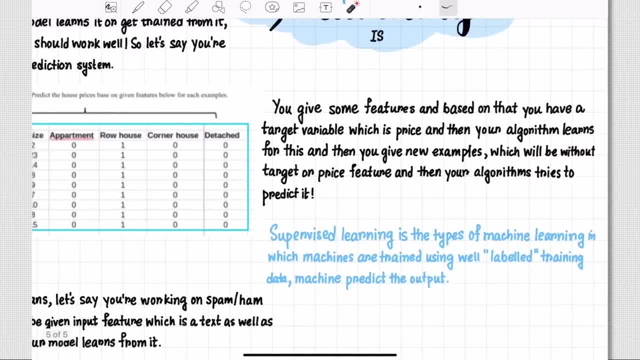 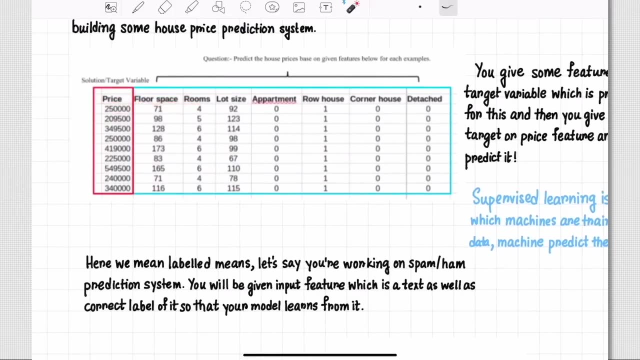 we'll have the answer later on- where the algorithm tries to predict the answer. so supervised learning is the type of machine learning in which models are trained using well labeled training data. so labeled means every data is labeled. well, right. so this, this, this particular information, is labeled. 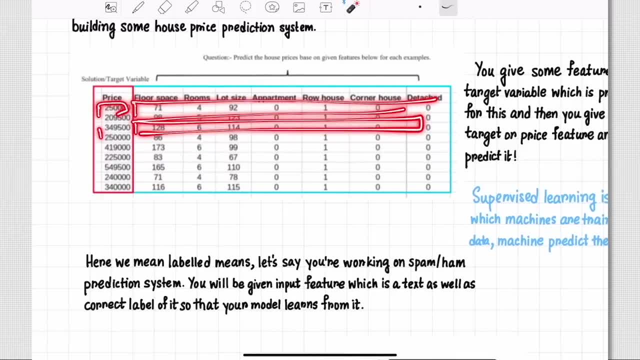 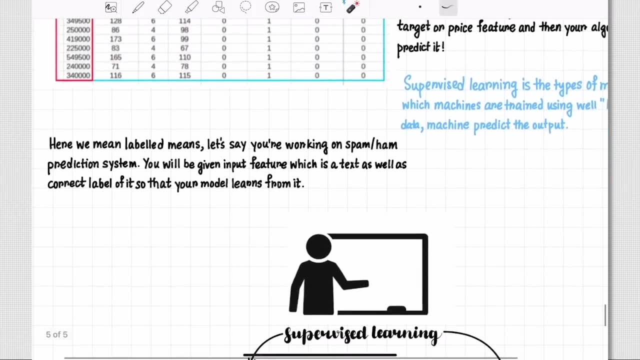 well out here. this particular information is labeled. well out here, right? so you have the question as well as the solution, and machine learning tries to predict the output. so here we mean labeled me. so here we mean labeled means what does. labeled means it means that, let's say, you're working on spam or ham prediction system. so for every email, every. 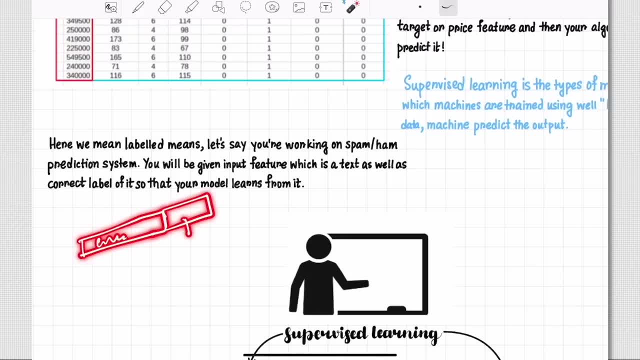 email, for example email number one, you have the label related so so that your model learns right. so you have the, you have the data, you have something like this data and for every email you have the weather with the wet for the foreign. sorry for, for the model to learn, first of all you have to make it learn by the historical data. so 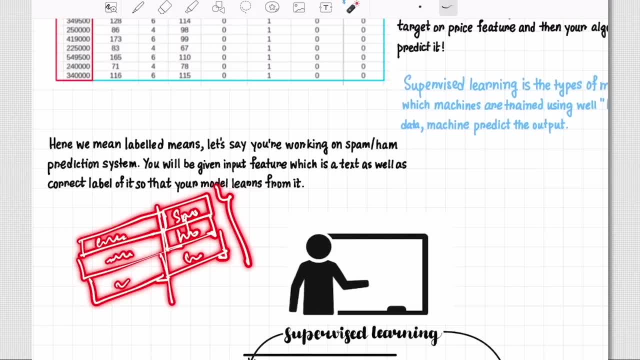 you have the email. number two: it is ham, even number three: it's spam. so the, the, the, the label, that label or the or the thing which are to predict is given over here. so this is what the label is: a machine learning where it is labeled means that for every given input feature, in this case email- 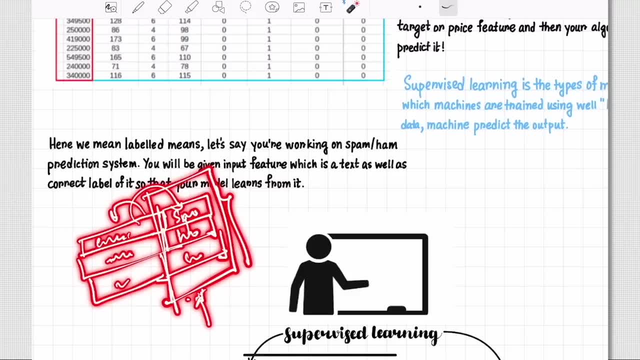 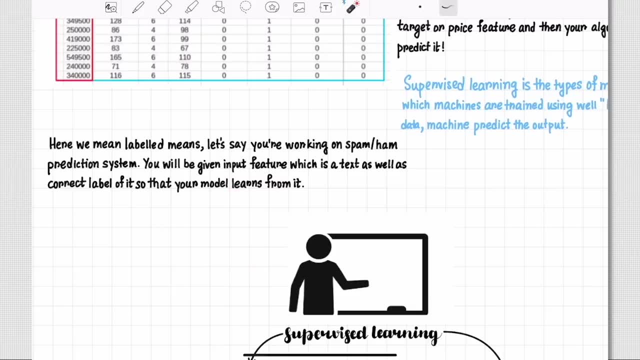 we have to, we have the correct, we have the correct uh label for that, whether the email was that. and then we ask our model to learn from this data, right, and then, and then after, after our model learned, we just say: we, we just only give emails. and then 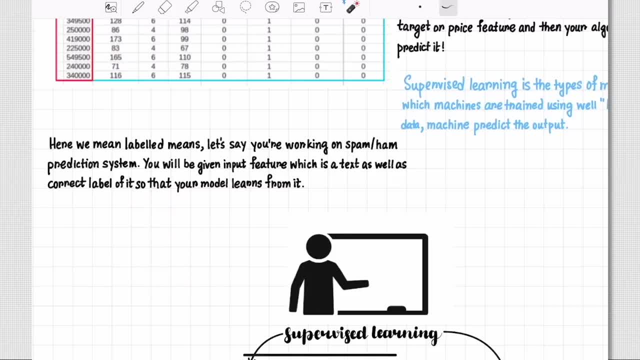 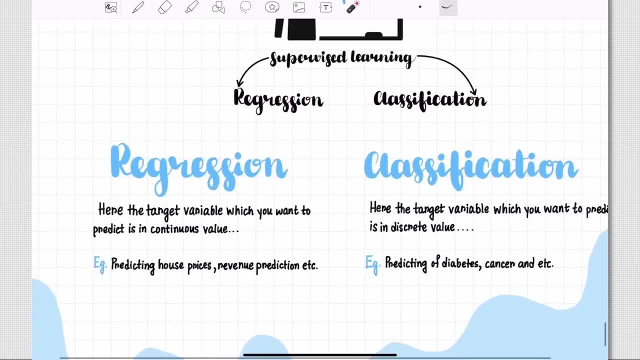 tries to predict what will the possible output from that? okay, so, uh, super supervised learning problems can be classified into two ways. so first ways is regression and second ways is classification. so we'll talk about classification, regression in detail. this course focuses on regression, but, uh, if you, if you want to learn more about you know, complete ML with earning. 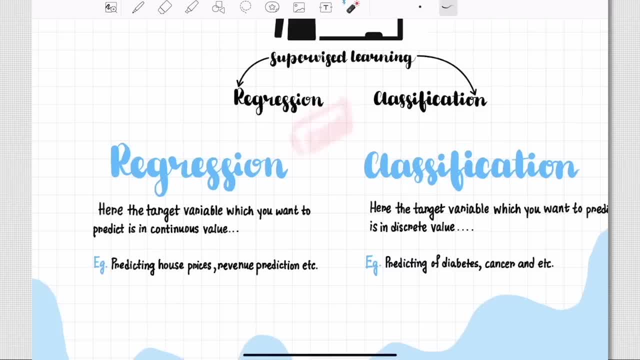 opportunities. I recommend CSO1. you can go and watch that. but uh, in regression, in regression here, here in in supervised learning, problems can be classified into two set of problems. the first problem is the first problem. the first problem is that your target variable, which you can predict, 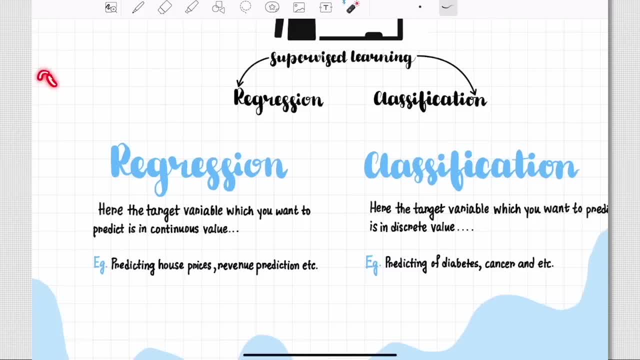 is continuous values. so assume that applications like in a predict prediction of house prices. so in this house prices you have your target variable, you have a target variable which are house prices, which are continuous, which are continuous value. so if you don't know what is continuous, discrete, etc. you can skip to the data fundamentals lecture where I'll be talking about. 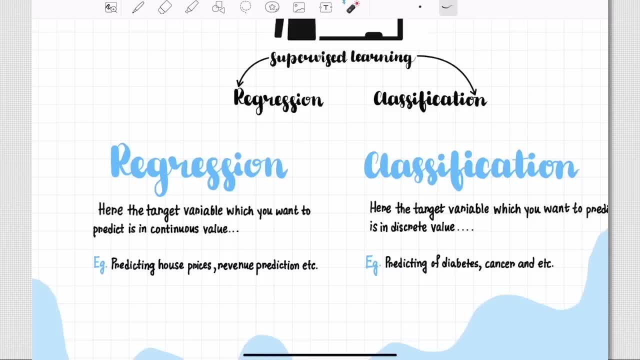 data fundamentals in detail. right. so over here, here, a target variable which you want to predict is continuous. so, for example, the house price, your pricing example, is continuous, right, a revenue prediction, sales prediction, Etc. so these are the examples of your regression values. right, there you're very the. the problems where we want to predict are the. 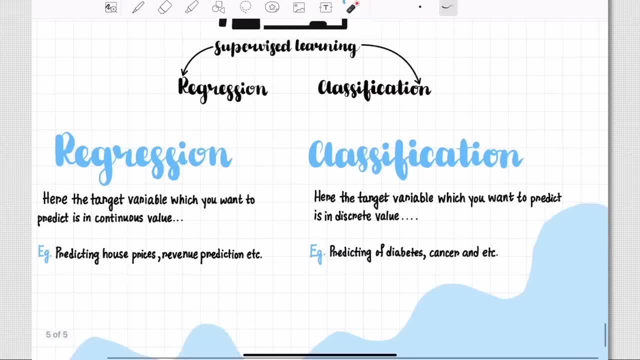 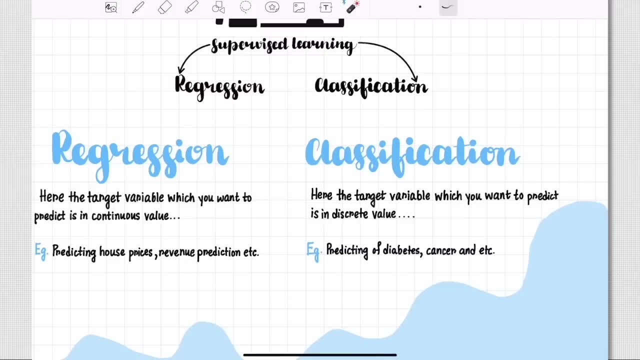 uh, when you predict where our target variable is of continuous value. but in classification, our target value is in discrete. whether the person has a cancer, yes or no, whether the person, whether the answer is correct or not, yes or no, whether this is this true or not, yes or no. so this is. 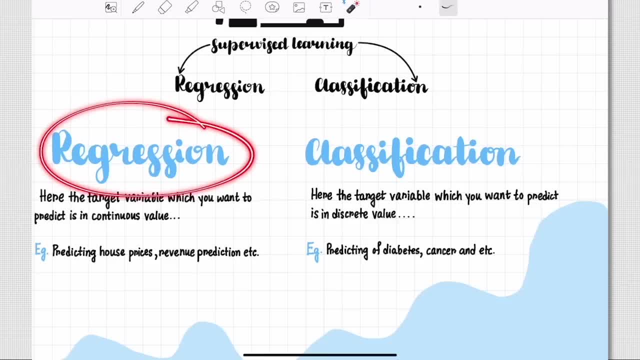 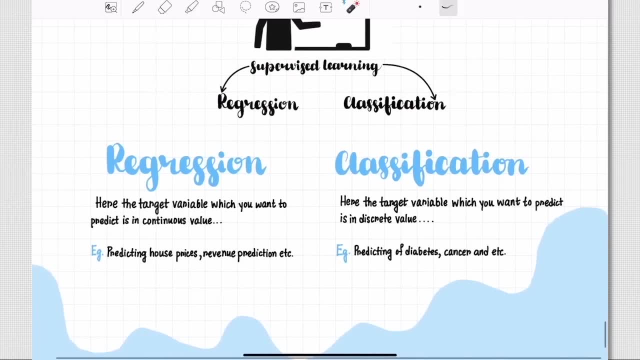 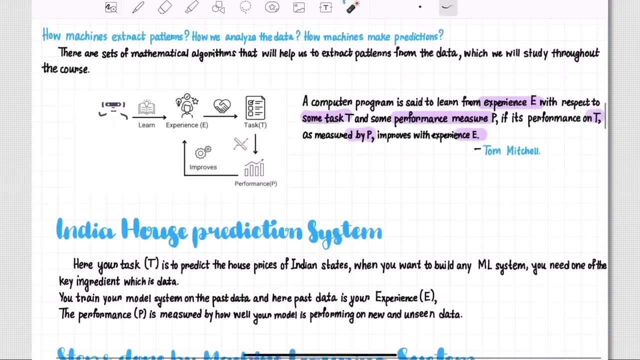 kind of sort of classification problems in this course will only deal with regression problems. if you want to know more about things in detail, you can go to classification problems. however, we'll talk about each things in detail as we go. now I think, uh, this is something which which we are done with, whole machine learning. now you may think here you 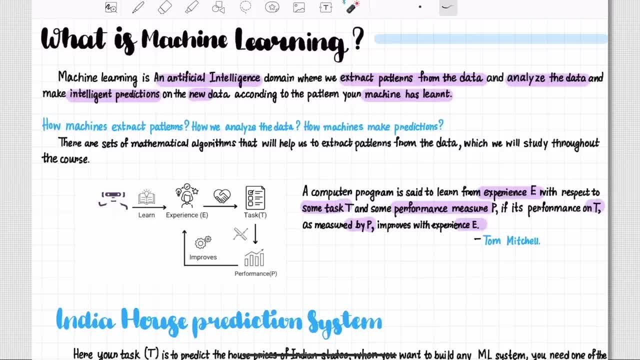 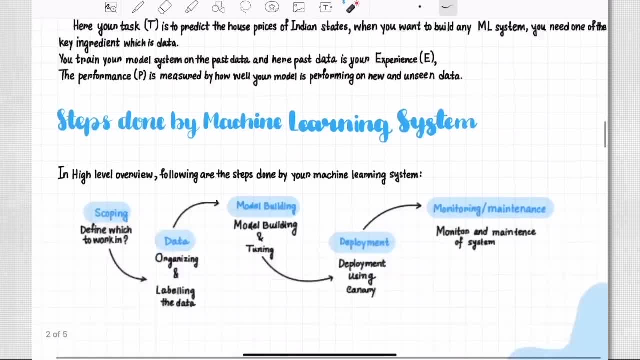 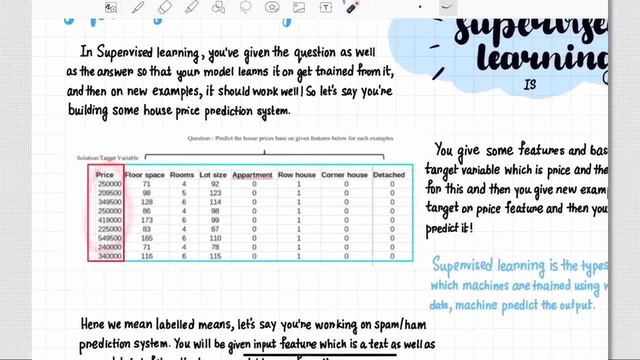 where is unsupervised learning? where is reinforcement learning? this course is intended to make you inclined towards the learning, the core stuff of it, so I'll just give you the idea. what is unsupervised learning is unsupervised learning in which you don't have the solution, you only have. 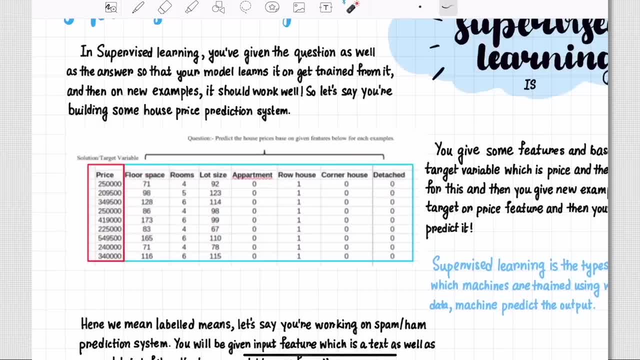 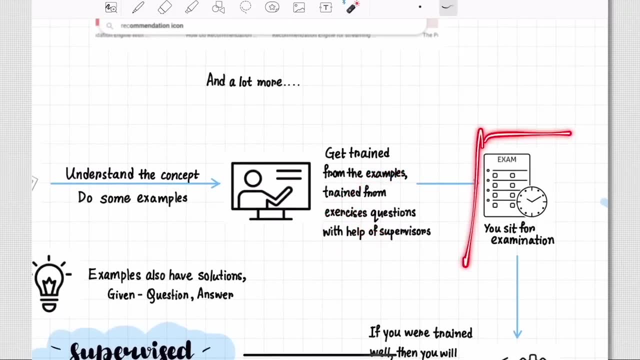 to. you have only have to make this loss any sort of sense of logic from out of the data, and then you don't have any sort of supervisor. in this case, in this case, in this case, you don't get any examples, you don't get any questions, you just don't get any help of supervisors, you just strictly. 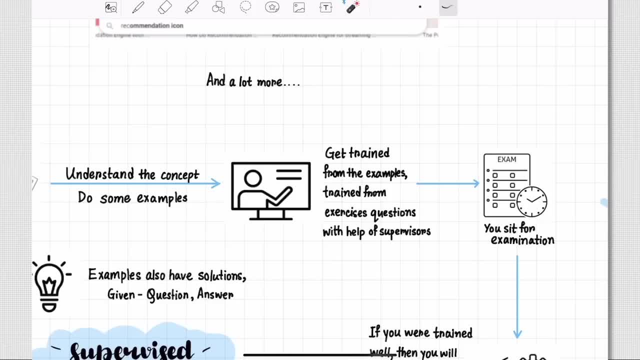 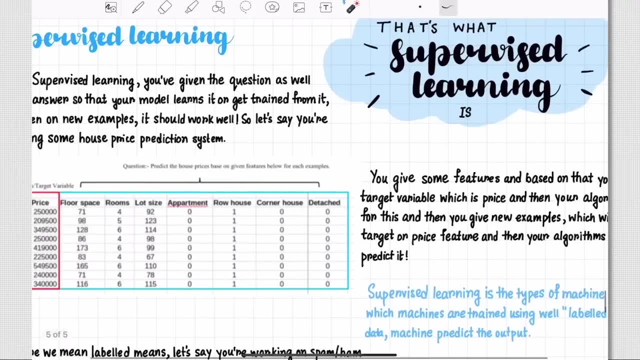 sit in examination and then you have to learn from it. you have to analyze the questions and then make a pattern, sort of it, right. so that's what- unsupervised, which is the most challenging today, and most of the work is being done in super supervised learning, but, uh, but unsupervised. 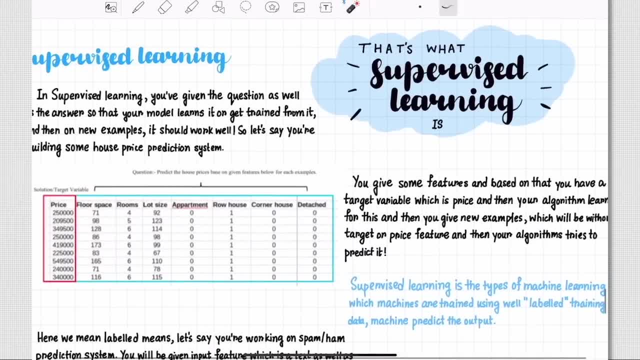 learning is very challenging, but, uh, that's something we'll take a look at later on, right? uh, that's something which we'll take a look at later on, at the end of this course, but I want you to stick with as of now is with supervised learning, and let's try. 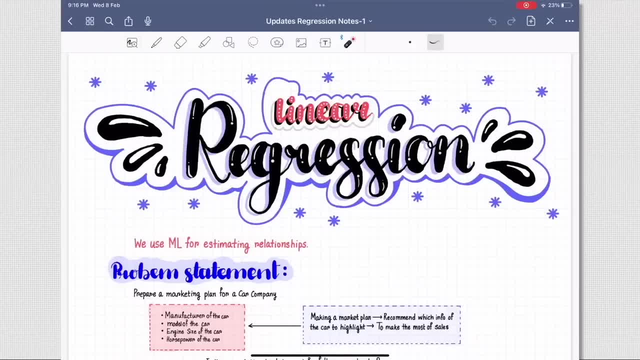 to learn- the core of supervised learning- and master it. hey everyone, welcome to the another module, which is linear regression. so what we'll try to achieve in this module is we'll try to learn in depth about a linear regression. we'll try to understand each and every concept. so the 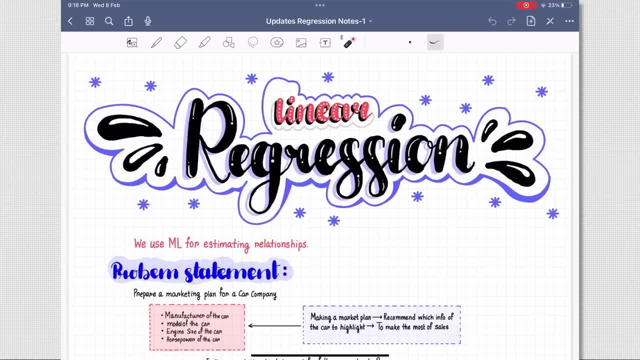 table of contents and everything is already introduced to you, so I hope that you know what you're going to learn. so, before starting this video, I would like to a bit talk about the two terms. right now is to talk about linear and then talk about regression, as this course is only based out of. you know, machine learning, code and 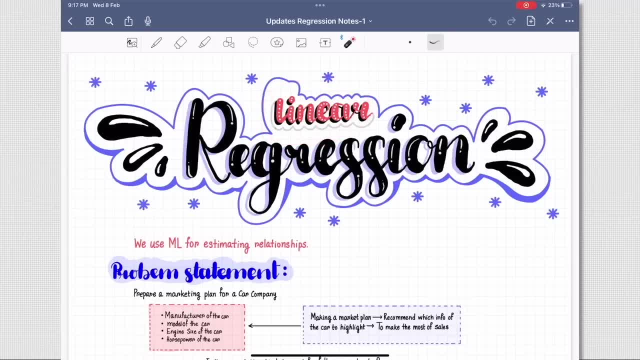 linear, regression. so we'll talk about only these two terms: which is linear and regression separately. so what is linear? linear is something which, which is, which, which is like a straight line, like you define right. and then what is regression? regression is a sub problem of your machine learning, you know. 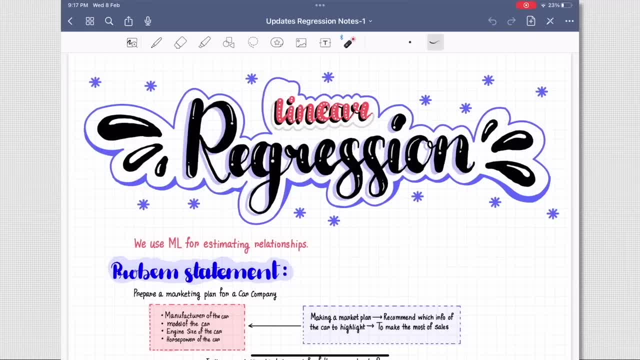 it's, it's, it's, it's a sub problem of your supervised machine learning, uh, machine learning task where your output variable is mine output variable, output variable of your. so the output variable or the target variable which you want to predict is continuous. what is continuous, we have already seen. 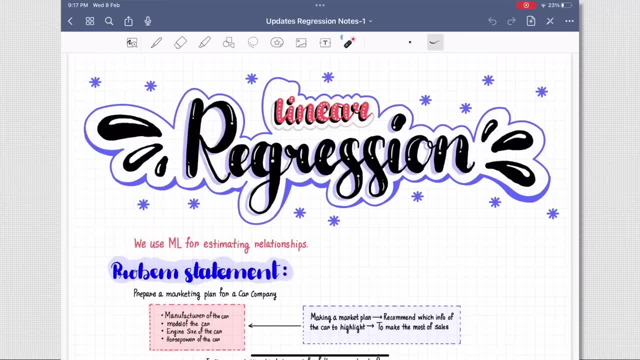 the height of the person, if you predict the height of a person to predict the stock or stock of stock of the particular company, or if you want to predict anything which is, which is which is uncountable or, I would say, non-finite, or something which is continuous, like height, a height, age, Etc. but 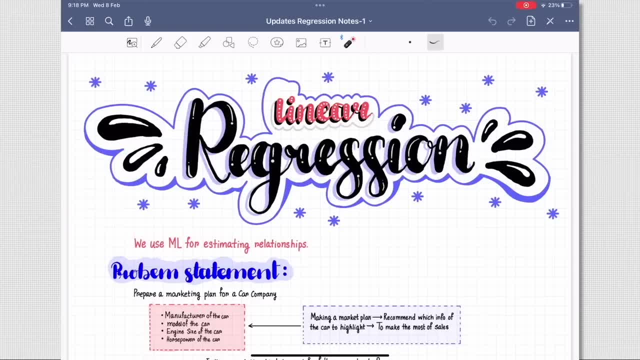 there's discrete, where if you're a target variable, discrete where you have a finite number of possible outcomes over there, then that's a classification problem. so we are going to approach, approach a regression problem out here using one of the one of the algorithms called a linear expression. so 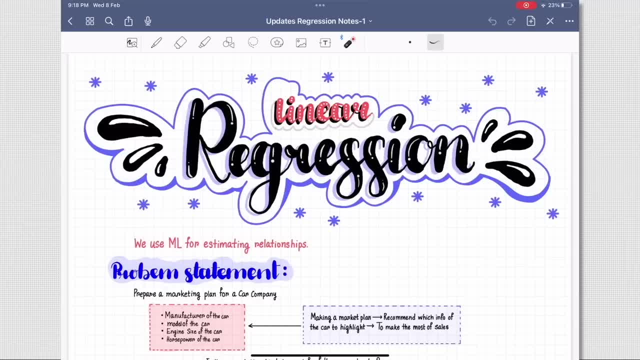 now one of the now. you might have seen in our definition of machine learning that we use um, that that we, how we, how we extract patterns from the data. so this is one of the ways we are going to study, one of the ways for extracting patterns from our data, and then this sets a very nice base. 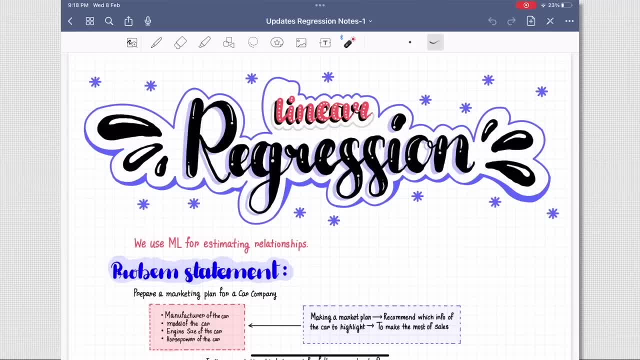 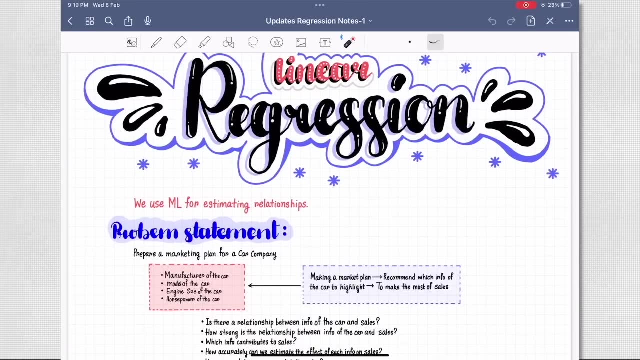 so once you have this, you will. you'll be easily able to learn logistic, regression and other things. but if you fully want to learn, I suggest the CSO one course for you, which is the best for you, maybe, yes, so let's get started eventually and let's try to talk about what are the things which is needed out here. cool, so over here you're seeing. 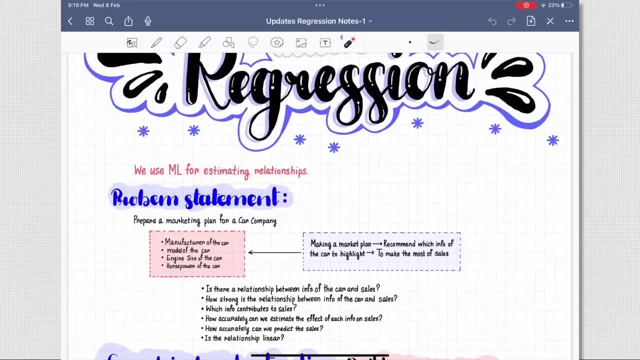 something known as um. we use ml for estimating or establishing relationships between two variables. so that's something is very confusing, so I would like to take a time to make you understand what exactly I mean by that. so over here, over here, what I, what I exactly mean by that is. 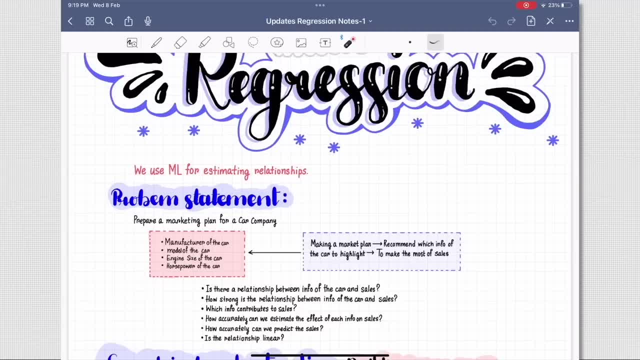 that. assume that you have- um, you have, that you're working on something like- let's, let's take an example- that you are working on cancer Europe. you know, you know predict where. you know predict whether the person has a cancer or not. you know right. so you know predict whether the person has. 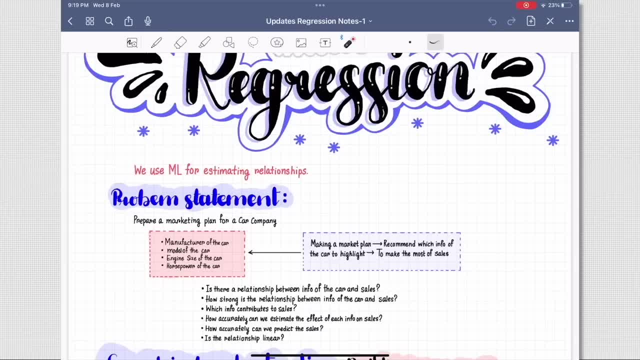 a cancer or not. so you're given the. you're given some of the information about the person, so you're given out the, the B, BMI of a person, which is blood, which is BMI, and then you're given the weight of the person, you're given the height of the person, so you're given these three features. 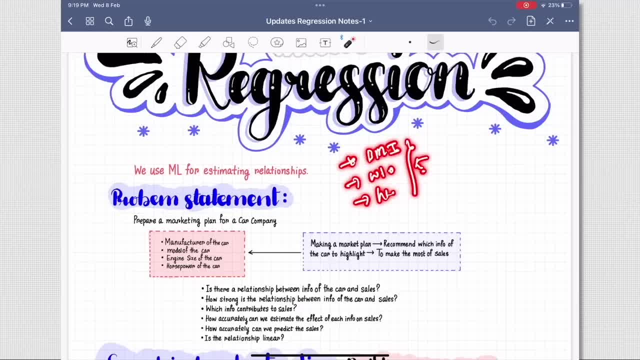 these three features, you know, predict. you want to predict whether the person has a cancer. I know this, these features are not enough, but base assume that, based on this hypothetical situation, based on these given features you know, predict whether that person has a cancer or not. okay, so how we're going? 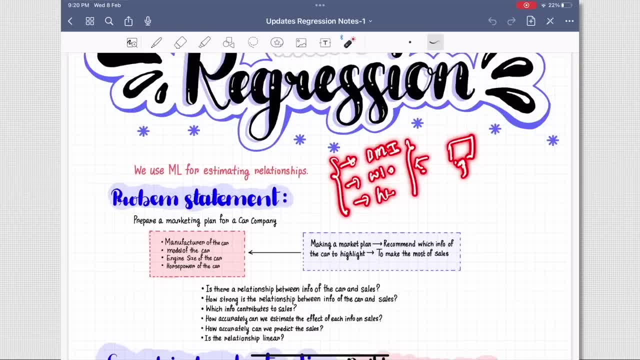 to approach this and how exactly we are going to uh, take up now from here. so one thing which I just want to tell you is how, how we are going to approach this. like, why, how can we relate this to a relationship? so you have these feature, you know, predict whether the person has a cancer or not. so 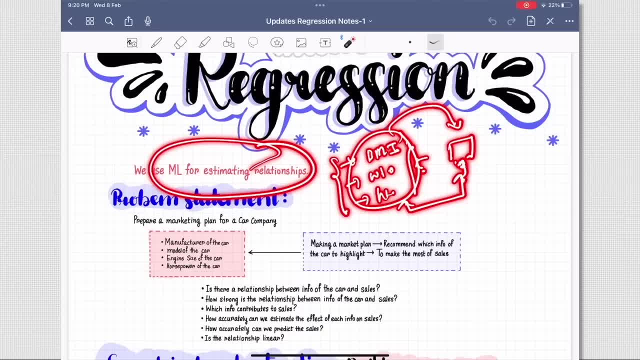 over here. you want to establish a relationship between every feature you have. so you know, you know, establish a relationship between these, these two things. whether there is any relationship between BMI and cancer, whether BMI has any effect on the person is having cancer. so if BMI is high, 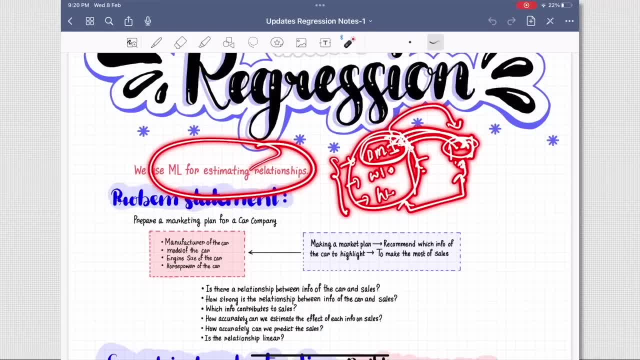 whether the person is having cancer. BMI is low, the person is having a cancer. so we want to, we want to have the relationships, or something like: identify any sort of you know, and any sort of um, uh, you know the, any sort of relationship between uh over there out there. so, you know, establish the relationships. 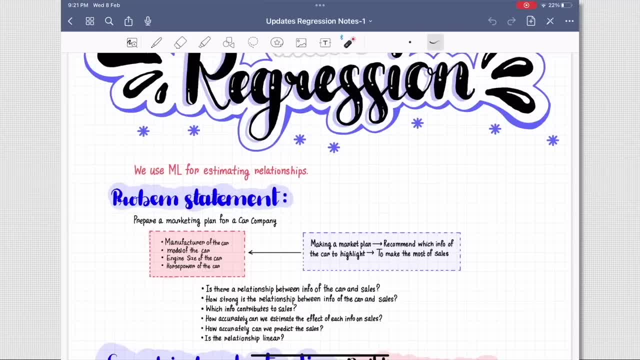 in um, in variables, like you know, the BMI, and the cancer, or maybe establish a relation between feature number two, which is weight of the person, and the cancer. so, does weight of the person affect or not? does does this particular info affect whether the person is going to have a cancer? so 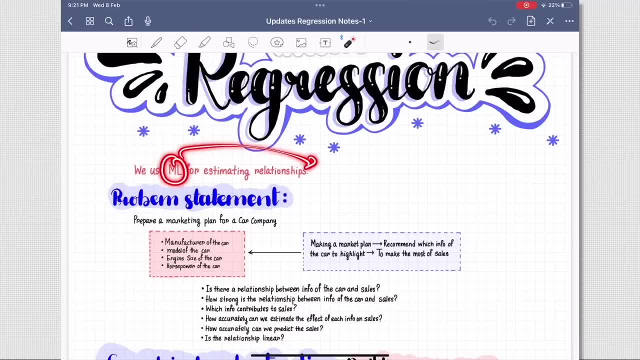 over here. what exactly we we use ml for exactly? I'm identifying that exactly the same thing you use ml for establishing the relationship whether this particular feature is going to affect my output variable, in this case, where my age or weight or BMI will affect whether I have a cancer or not. 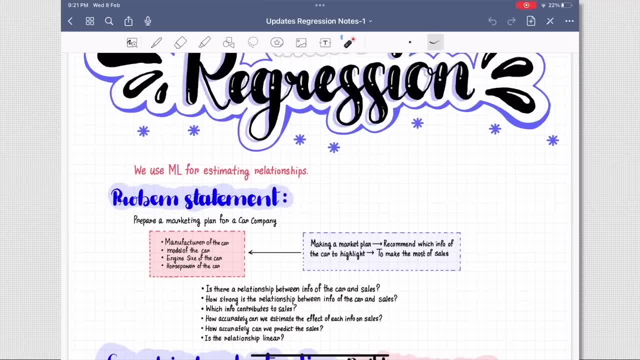 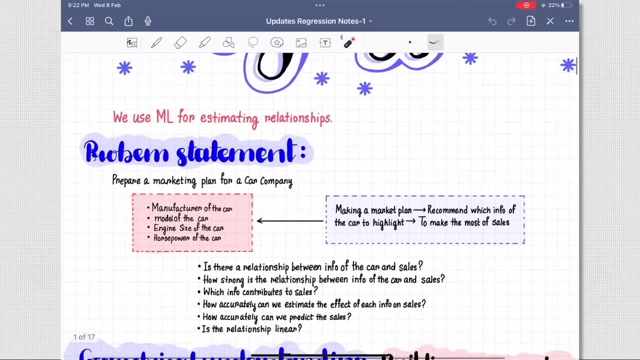 okay, individually, like this feature. effects or not this feature? if it's, if yes, then how? right? by by what units, Etc. so these, uh, these questions are answered. so we'll take a very nice problem statement to make you understand this particular statement, which would be easy for. 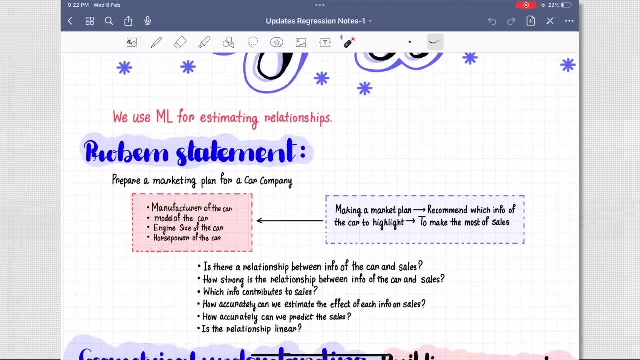 you. so let's take an example: your marketing strategist to data scientists for a company and basically this is what the data scientists do eventually have the marketing team, or have the decision team to take certain decisions, or marketing team to take some certain marketing steps. so you prepare a marketing plan for a car company. so you have 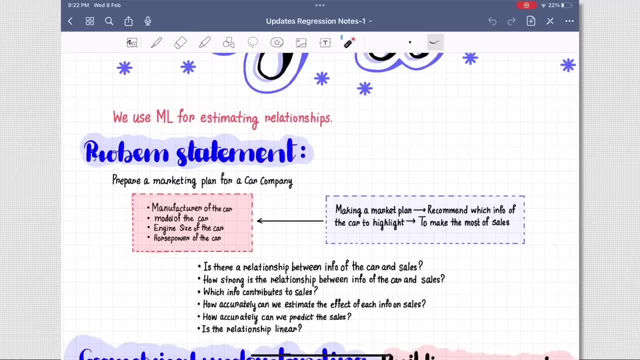 a car company and then you know, prepare the marketing plan, how the marketing plan should be there for car company. you have to help the marketing strategies out there with your data driven decisions so manifest. the first is a manufacturer of the car. so so you're given these particular infos about the car, the features about the car, right? so you're so you're given these. 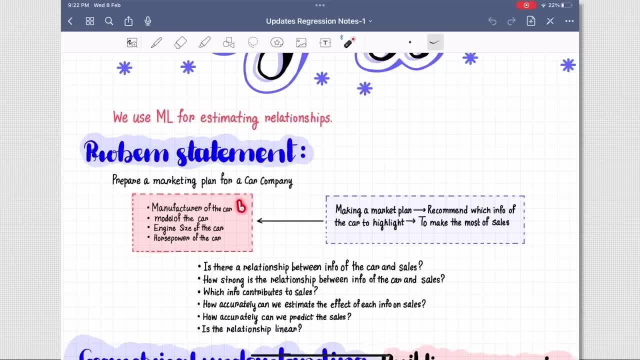 one, two, three, four, four information about the car, four features of the cars and based on this, you have to make a marketing plan. okay, so you have to make a marketing plan. so in what way? the marketing strategist asked you, as a data scientist, asked you, that tell me which info we should highlight out of all these infos in our 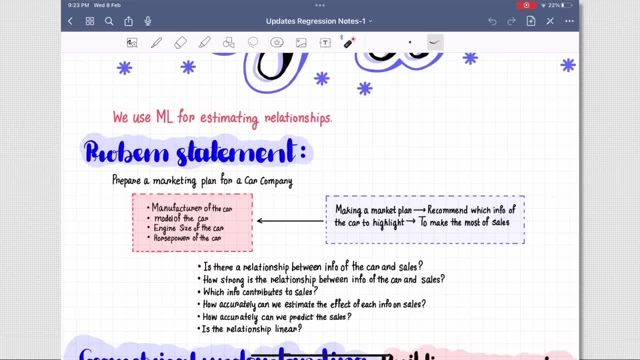 main ad. so in a maker, when we make our main ad, which info out of all of this we should highlight so that we make maximum of sales for that car. understanding what I'm trying to say? what I'm trying to say? that there is a marketing team sitting out there. you're a data scientist out. 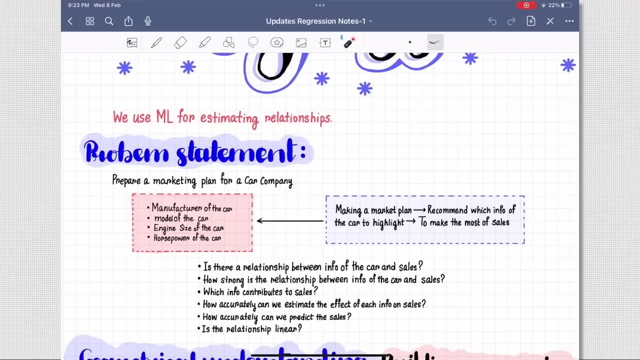 of all these features. can you recommend me which info, which info I should I should take and show it in ad so that I have a most of the market, uh, most of the sales? okay, and just, I don't want the prediction. I also want to know the following questions: so marketing's team is setting and? 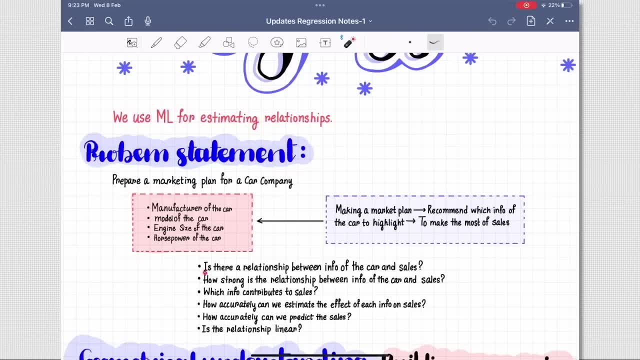 asking, asking these questions. so what are those questions? questions is: is there any relationship between in for that particular information in the car? so is there any relationship between the manufacturer of the cars and the sales? so of course, as everything that let's assume that manufacturer is BMW brand is high right, but but it may have like there might be a very nice in. 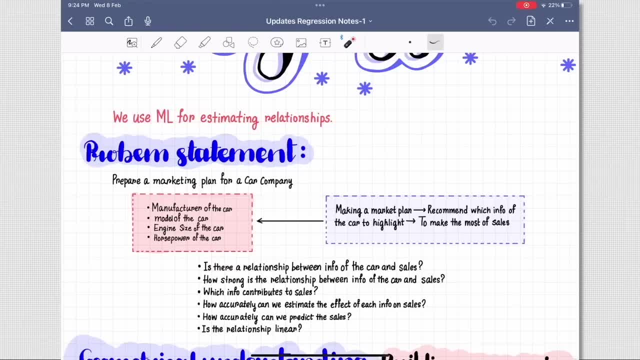 relation some. it may happen that the of brand manufacturer of the car is high but the sales might be low because the brand is super high and expensive, right. but if you have something Wagoner or you know low budget, the brand is Tata. you know Tata Motors and all. so they produce less. 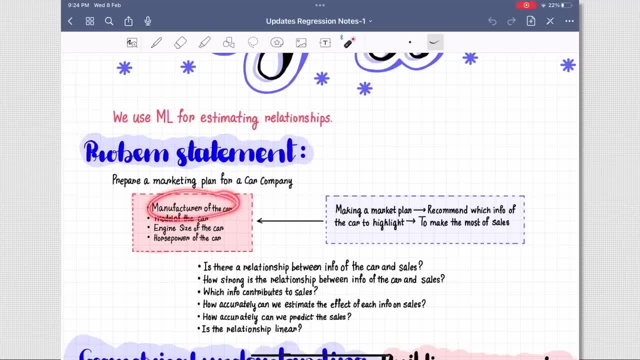 expensive, so the sales will be also very high. so the manufacturer of the- so you have to understand- is the relationship. if yes, then what relationship is available between both of them? and that answer is: how strong is your relationship between that particular manufacturer and the sales you do for every model of the car? 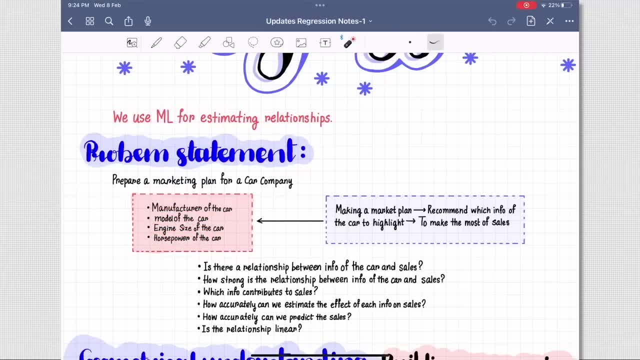 engine size, horsepower, right. so what is the relationship between a horsepower and the sales? so it force powers high. what is the sales if horsepower is low? what is the sales, right if? if engine size is highs, uh, size is highs. what is the sales if the engine size is low? what? 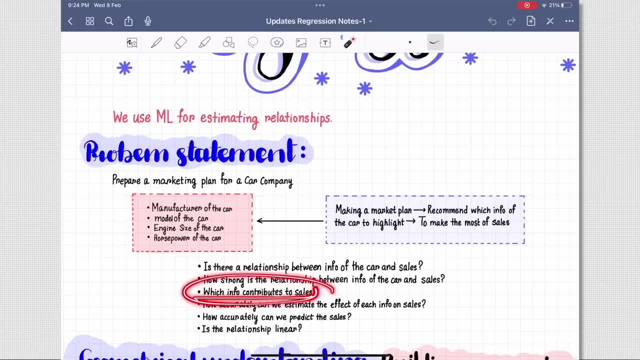 is the sales, etc. which info contributes to the sale, so which information? sometimes it may happen that this, that that any particular information may not contribute to, may, may not have any effect. that does not really make sense, just like in pigeon pigeon example, which is senseless, right. 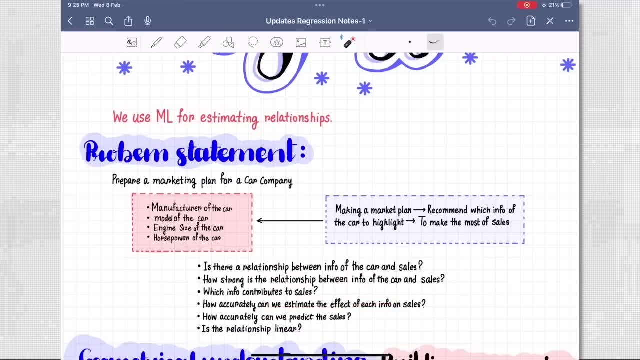 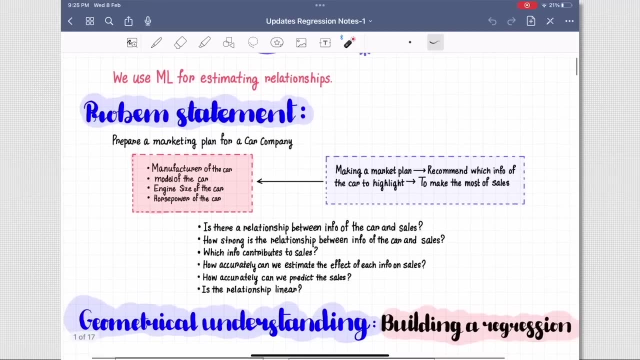 how accurately can we estimate the effect, how accurate we are in estimating the effect of each individual features, each individual features, on our output variable Y, and is the relationship linear between both of them? and what exactly? we say that the relationship is linear, which means: do they follow the linearity or do they follow the the straight line convention? so what is linear things? 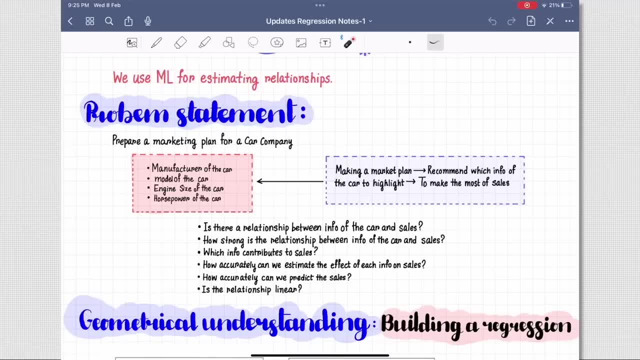 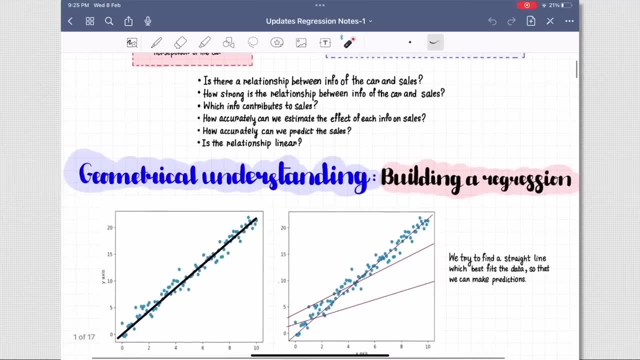 which are, you know, in straight line or something in any in any straight line, it should be linear. it should not be like this, right, it should be, uh, linear. so you might have studied new lower classes about that. so I hope that this gives you a very nice sense about you know, uh, we use ML for. 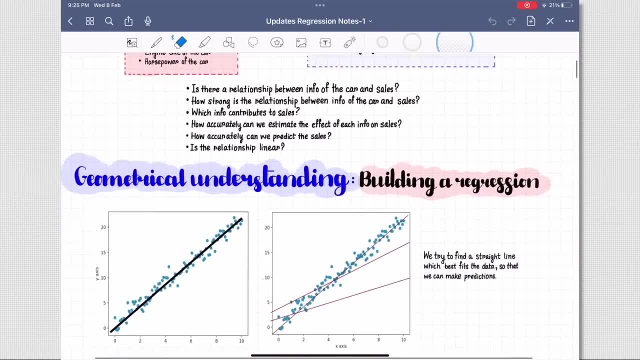 estimating the relationships in the next video and what I'll try to achieve in the next video. what I'll try to achieve is- I don't know what I want to do is to work about geometrical understanding. is to work about geometrical understanding, geometrical understanding, right. so to work about geometrical understanding of our 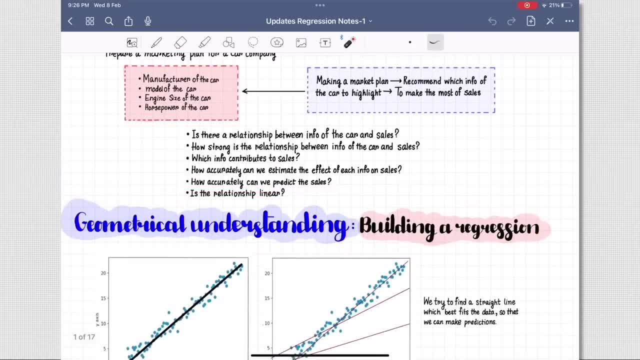 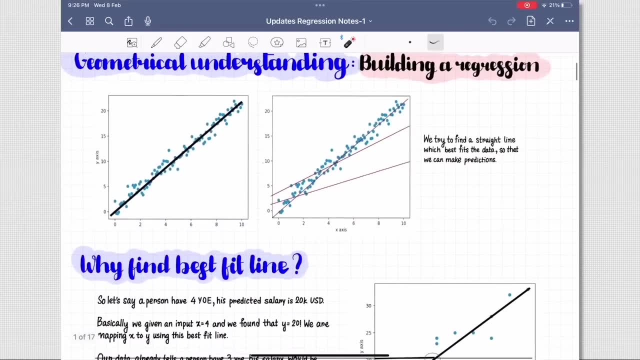 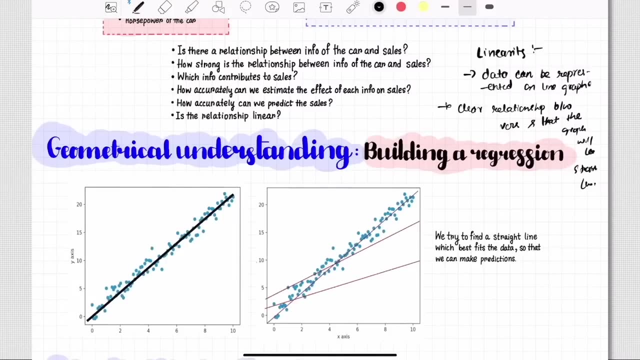 regression. so we'll actually go ahead and then talk about how we can estimate the relationship between features and the outcome variables in easy way. so let's go ahead and talk about that. so now we'll talk about something which is now now once we, and now we have studied about, you know he, this is how. 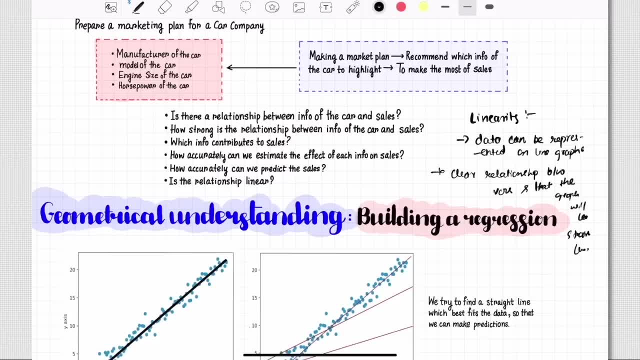 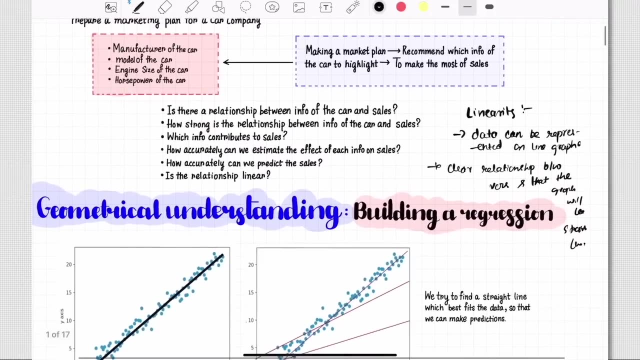 we asked. this is what we have to do. this is what ML is about: estimating relationships. so let's start talking about how we estimate relationships between variables, right? so let's, let's get started and actually talk about that, right? um, so, over here, what uh? so now, uh, before going on that, let's talk. 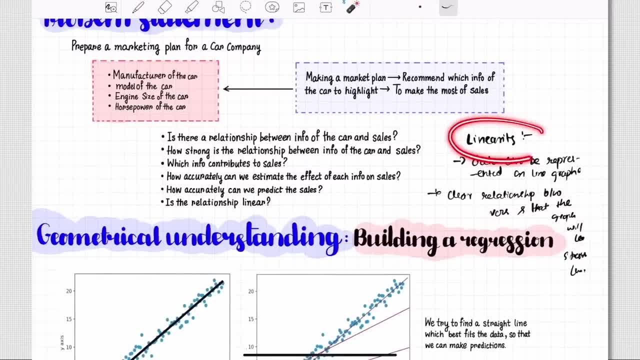 about what? what it? what does it means to say that data is linear? right, data is linear. what is it? what does it mean? so, data that can be represented on a live line graph: right, it's a data which can be represented on a line graph and there's a clear 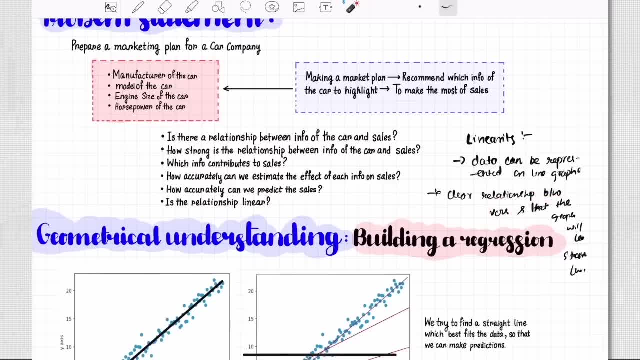 relationship between two variables. between two variables is a clear relationship between two variables that the that, that the graph can be shown on a straight line. so there's a clear relationship which, which you're seeing, and one unit in it, one unit increase in X is giving a constant increase in Y. right, that's what the data is safe to be linear, you might have. 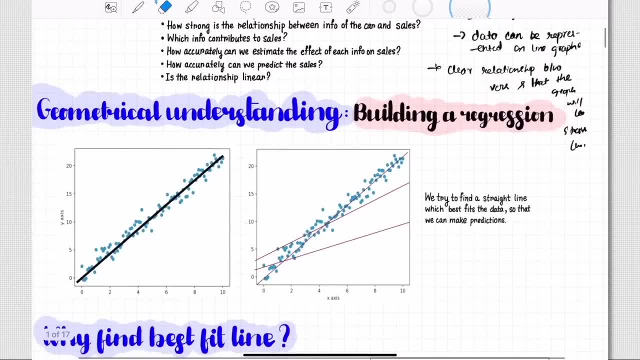 studied in lower classes. just for those who would know who, who just want to recap: I just told about that this is an example of a linear data. this is an example of a linear data. this is an example of a linear. ignore the lines as of now. okay, ignore the lines as of now, just go. just go about the just. 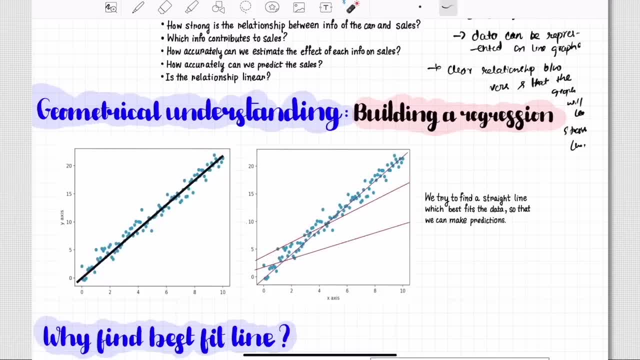 go about the data which you have out here. just just go about the data so you see that the data is linear. if the data would have something like this, you know, very, uh, very random. you know there's not showing any clear relationship, there's not showing any. 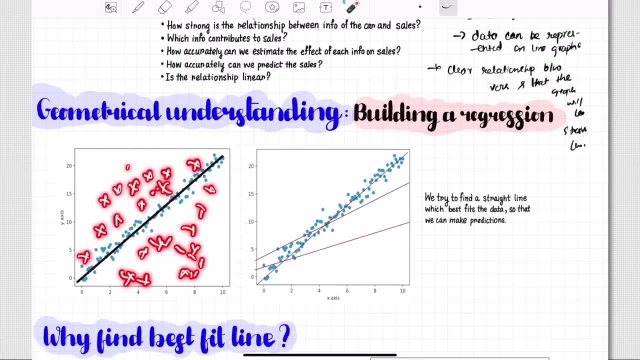 clear relationships between between variables, then it might have not been. this is called a non-linear data, so data is linear over here and over here, over here. assume that this is your data. assume that this is your data. so now assume that this is your data. where on? 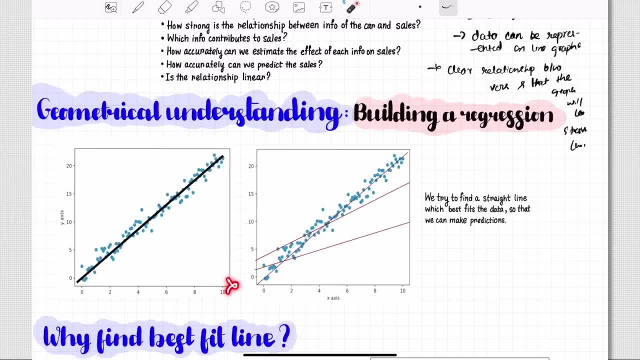 x-axis, where on x-axis you have something like the number of years of experience. so you're gonna build a system. so, uh, let's, let's formulate a problem right now. you're gonna build a system. you're gonna build a system that predicts the salary of a person, given the, given the um. 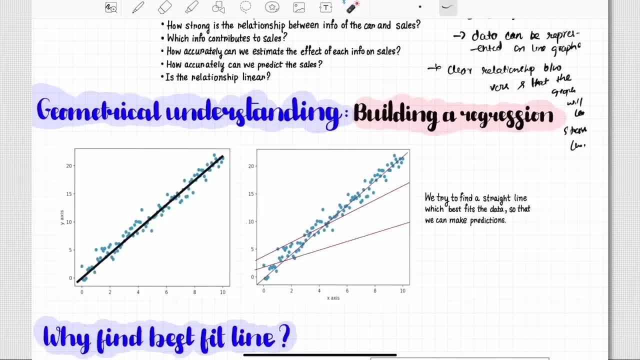 years of experience of a person. so given the the- the years of experience of a person, you're gonna predict what to what, to leave the possible salary. so if the person is a two years experience, you have such such number of salary. so you are given a data in a csv, in a csv file, or you give 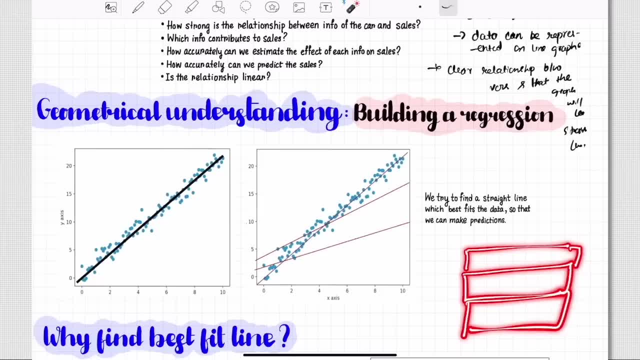 that data and in that data you have something like this uh record and your. you have one information available which is the years of experience and assume three, and there is the label, a target variable which will predict the salary, which is in, let's say, five right, which is in 5k dollars, 5k. 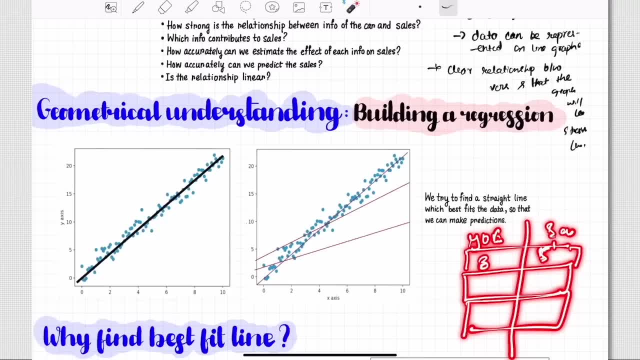 five thousand dollars to ten thousand dollars, whatever, per year, according to Indian market. um, so over here you have years experience and the salary of that person, right, and this is in five k, okay, so if there's five over here, that means five thousand, okay. so, uh, and then you have. 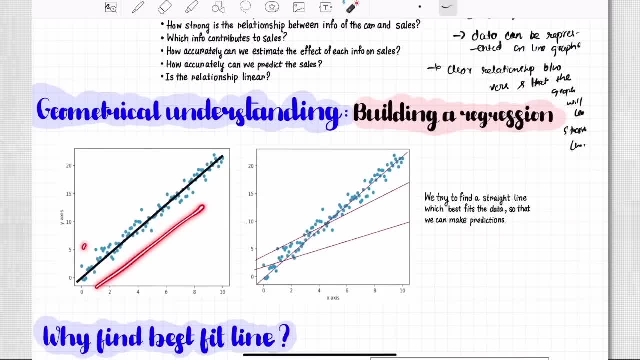 the data and then you plot this data over here. now you plot this particular data over here because you have only x variable. you have only x variable and then you have y. so you know, you're given x, you're gonna predict y out here, right, you're given x, you're gonna give an x, you're gonna predict y. 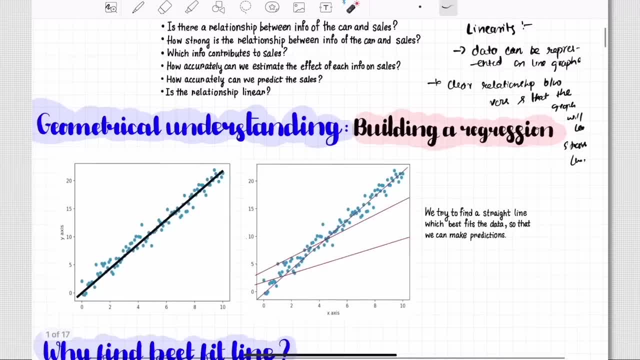 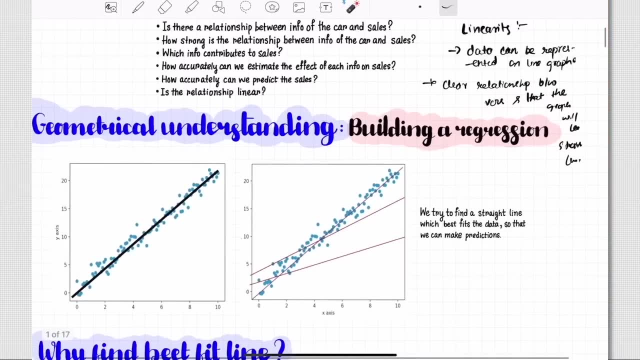 right. so I just want to talk about one of the thing which is super important right now is: is this something known as functions, concept of functions? so in functions, what we do in functions, what what we do in functions, what what we do. say, for example, that this is a function which x squares the number. 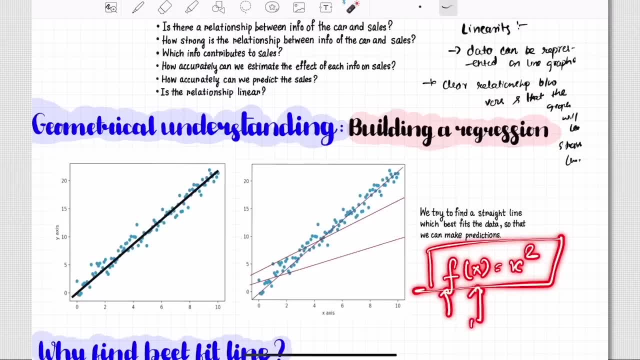 which squares the number. so this function takes the input value of x, takes the input value of x and outputs y and outputs y, which is a square of x, right? so when you plot this function, when you plot this function, this looks like a parabola. this, this, this looks like a para. this, this is a parabola. 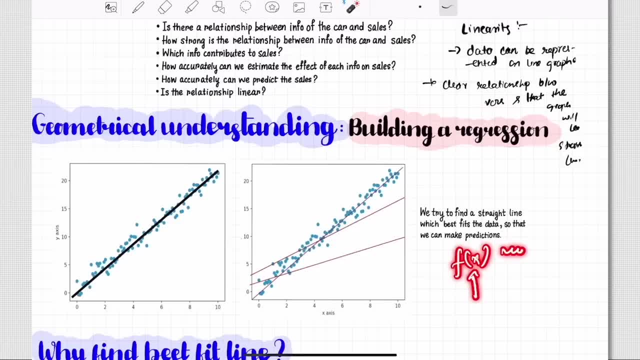 so that f of x. then it takes the, it takes the input value, does some processing and returns the square of it that runs the square of it, which is a square right. so in this case we want to tell, we want to, we want to build a function f. so we're going to build a function f, you're going to build. 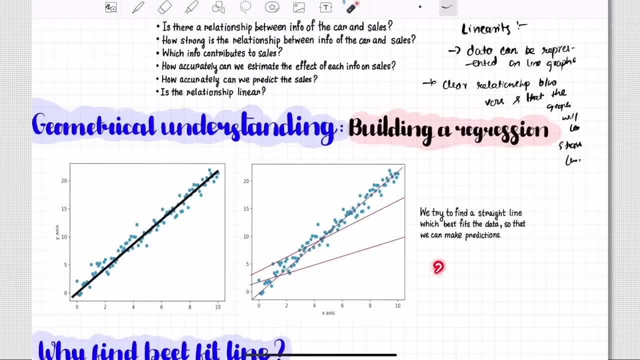 a function f. we're going to build a function f that takes up your build a function f that takes a year's experience of a person, that takes up years of experience of a person, and map this, which we call this, x- in this case, the input value, the, the thing which you're going to input to the. 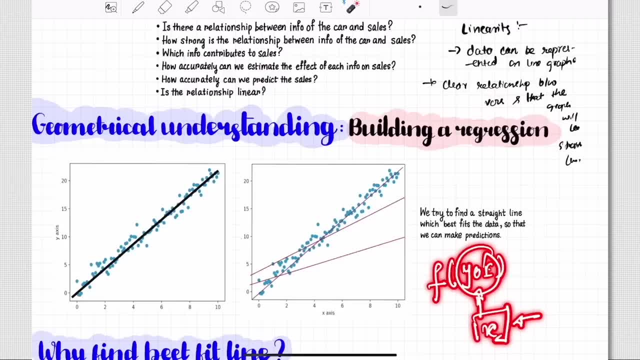 output. give this input. for example, in cancer prediction, we're going to give the input, like BMI weight agent to give input and then, as output we're going to, we're going to predict what will the salary of the person. that's the output out there. that's the output out there, which is the 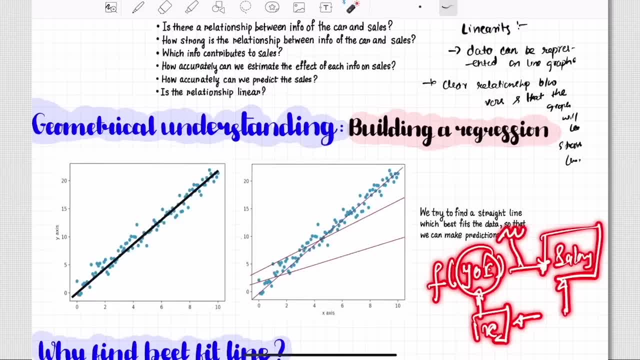 salary of a person. so you know this, this does something. so this does something with this input value and then returns you the salary. so now, so now we're going to build a function, now we're going to build this black box thing, this, this, this, this thing out here, this particular 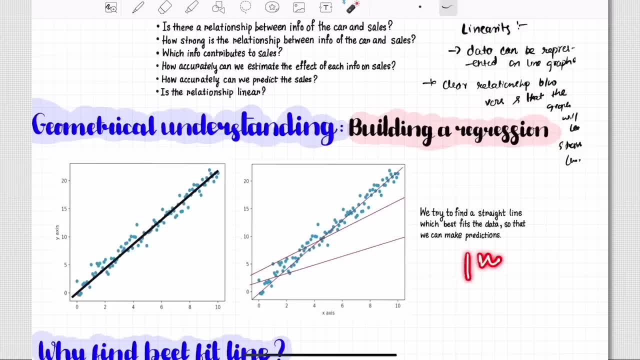 whatever processing that does with the years experience. so we're going to build that you know for. for for building that we wanted to learn up, it's the algorithm called linear regression, where it helps us to building that particular processing that takes up your input, feature X, and does some. 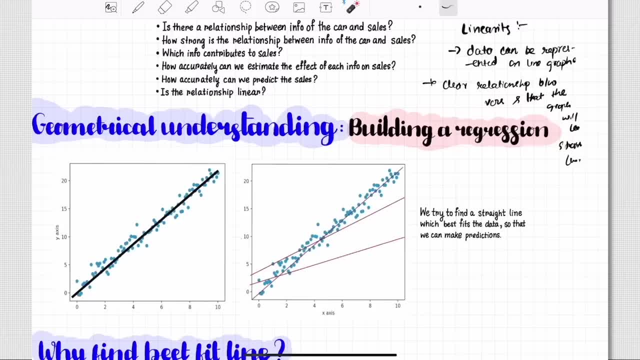 processing and returns some values Y. okay, so so how do we learn that function F that takes the value Y- years experience- and returns the Y? so let's start off with a geometrical understanding. so assume that you have the data plotted over here on x-axis. you have. 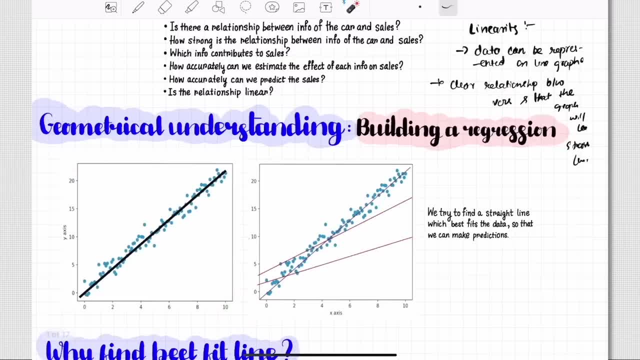 the years experience. and on y-axis you have uh salary of the person. so this is the data which you plotted. this is the data which you plotted, I hope, so that you know data plotting at least, given the tables, given the tables out there, you should, you should be able to uh plot data out here very. 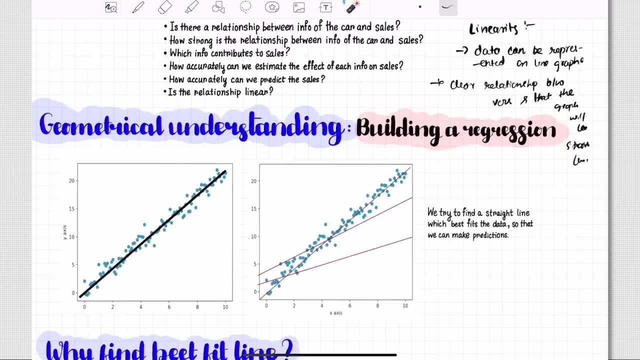 easily, right? so when you plot this data out here, when you, when you plot this data out here, you plot this data out here, now you look that ignore the black line. as of now you plot this data now. now you're a you- what? what you do? find a straight line. you find a straight line that best fits the data. that best fits the data. 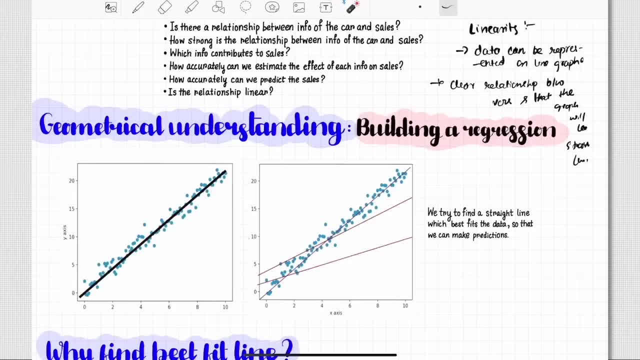 you try to try to find the line that best fits the data. so why do we find the line that best fits the data, right? that's a good question, right? so assume that. assume that you wanna. you have um four years experience. you have four years experience. so what? what will be the possible uh salary of yours? so if 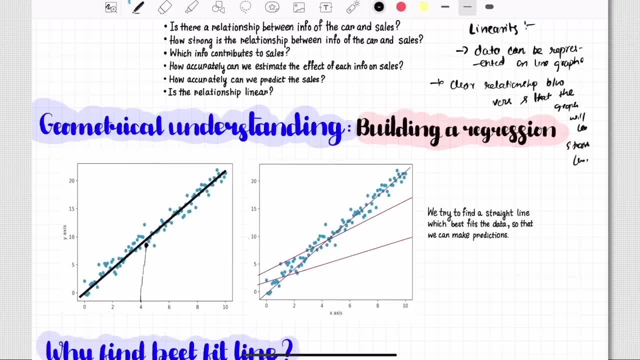 the actual value states that the actual value states that you will be having somewhat, like you know, um, i think, uh, eight, eight thousand dollars for a new right, but your model, so. so basically the intersection from x and the in the intersection point. so basically the intersection point is: this, is this point. so this is the intersection point and this intersection point. 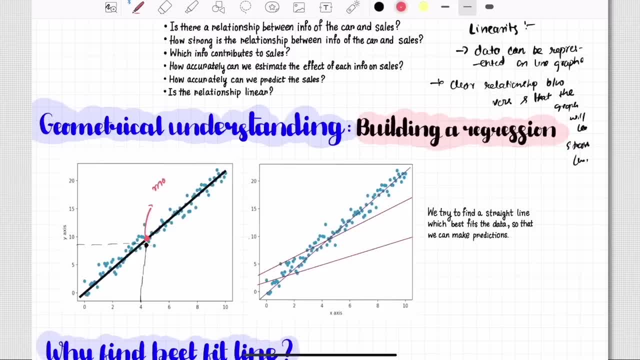 is your, is your, is your model approximation, model approximation. so let's talk about what exactly this model approximation mean. model approximation is something like your model approximated. so this is there, is a there, as as we say. for example, assume that you have, you have, you have your examination and it's the examination. similar questions comes, or exactly same questions. 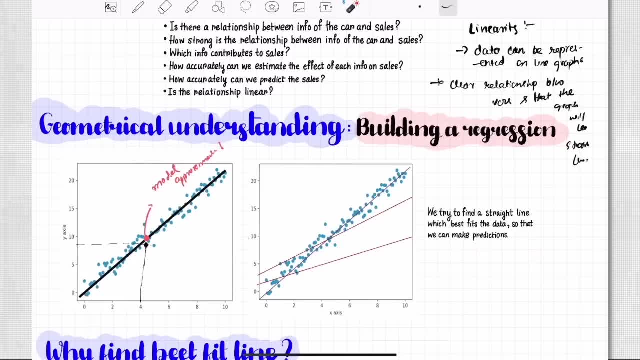 comes right. so it might happen that your approach might be different from the book's approach. you- it may be similar question, it may be similar question, so you answer differently, right? so you over here don't exactly answer the same thing. you written differently, for example in science exam. 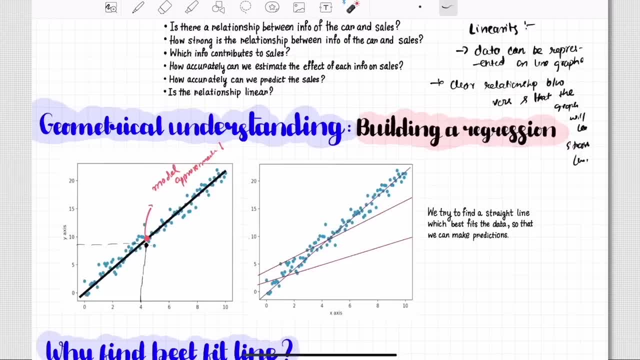 in science exam you don't write exact, exact the same question, it's exactly the same answer. there is some, of course, the you have approximate answer right, not exactly similar to the original answer, not exactly similar to the bookish answer, but similar to that. so someone asked what is. 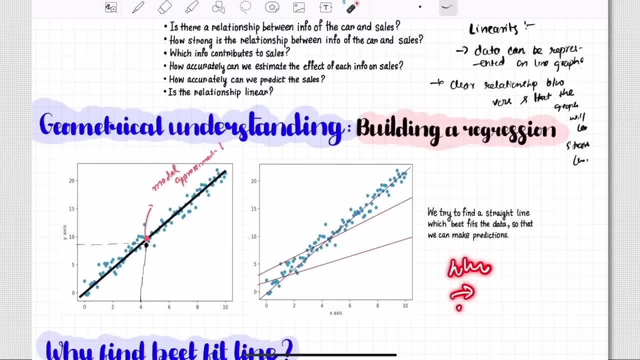 photosynthesis. you might ask you. you might write your answer in different language, but the original may be different. so there is, there should be some difference between both of the answers. so, in the same way, if someone says that someone asks a question, what is the? what is the salary? 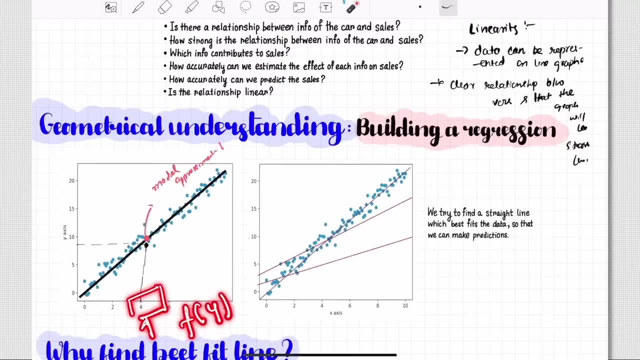 of person with the years experience. for where they ask, they give the years of four. we have some processing done and then it results in some values. okay, and as of now, you are trying to understand the geometrically how it should work. if someone asks what is the, what is the salary? 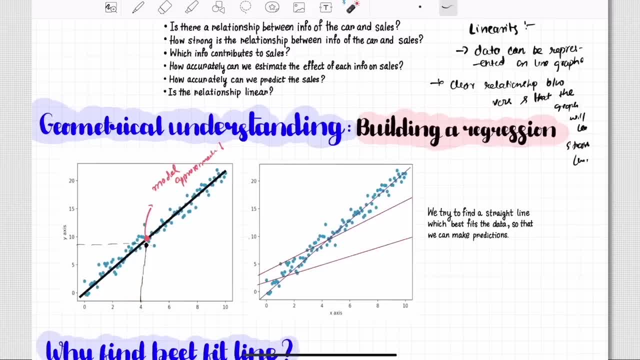 if the person has the four years of experience, that says that it's. if I asked: what is the years experience when, when? then when the years experience is four, it says that the actual answer is this: the when actual answer. is this actual answer is this with the original? but is of course the difference? but there's of course the there, but 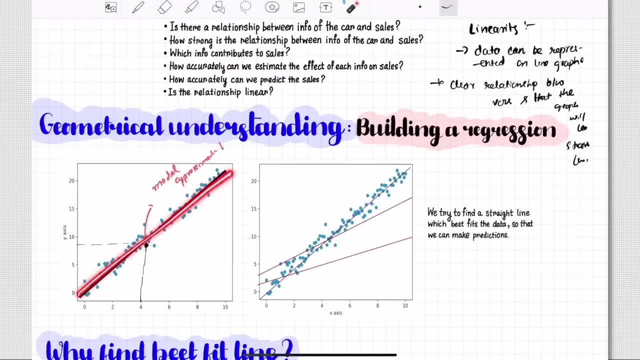 the actual model approximated this, this straight line. as of now, this is straight line to us, this is straight line. so we found the straight line that best fits the data. okay, so we found this a straight line. and then we go gone and see, okay, this is the point of intersection and this is your. 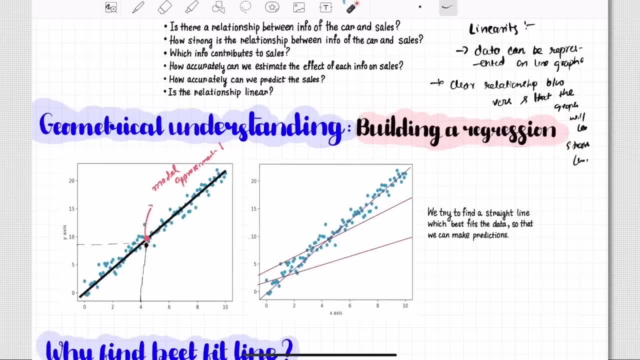 model prediction. this is your function: approximated value- not exactly same, but similar to that. there's small difference between both. both of them right, right. so now you may- may- have several questions. please don't worry, we'll tackle each and every question in detail. okay, so let's start tackling each and every question in detail now. over here, what you're seeing is that 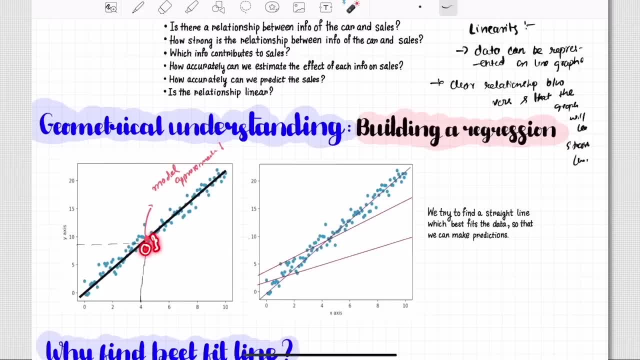 assume that this particular information and this particular information. so there is of course the difference, this model approximation, and your actual, actual value. so what is the difference between model approximation, actual value? as i again told, in science examination for a particular question there might be different answer, but concept is same but different answer right in. 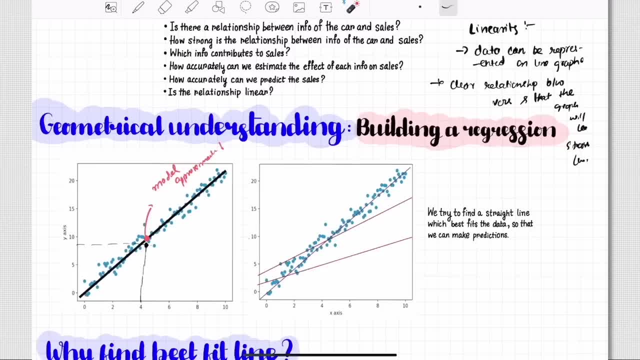 their own words in bookish language, but you might have different answer in your own language. so so there's of course a difference. so if the difference is high, that means the concept is not same. so it will. so your, your examiner will match your answer with the original answer, and if the difference is similar, then that's good. but if the difference is, 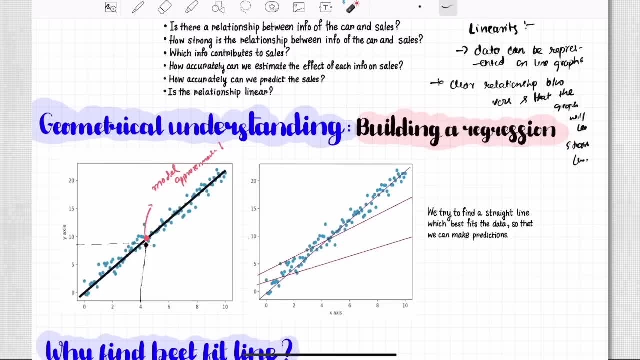 high. this, this, the, the dissimilarity is high, then the answer is wrong, because you might have written in when you, when you, when you were told to write the photosynthesis, you, you, you came and write, written something like: um, respiration, right, so that's that. that will be wrong, right? so i think 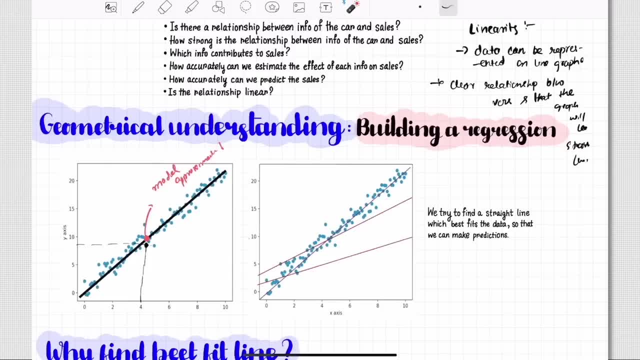 that's. that's a very, very good example to state over here. so now you're the. the actual answer someone asked about photosynthesis is the bookish answer which is so correct, which is 100 correct. we call that thing as a ground truth. and then you you written that is a student approximated answer that that student might. 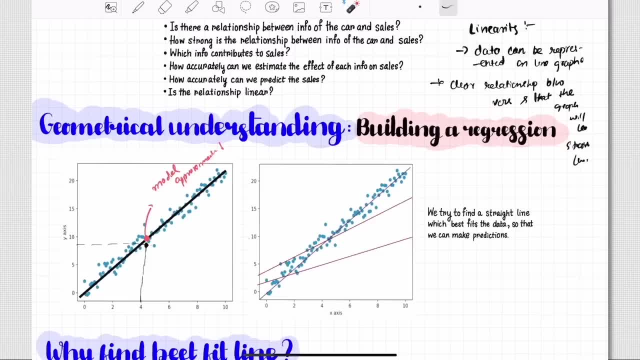 have written some answer, so we we match both of them, but take out the difference. how, how, how, how similar they are. if the similarity is if the same, if, if, if the similarity is if the same, if the similarity is less, that means that, uh, that the answer is correct. but if the similarity is high, 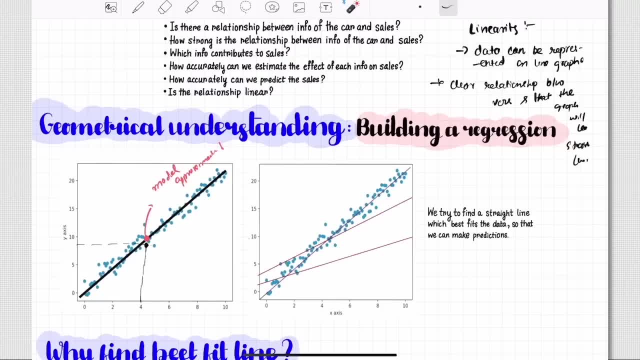 that means, oh, that something is uh away right, that something is wrong, that they have written respiration instead of photosynthesis chemistry, is that something? never mind? so this is what the difference between model approximation, so in this case, only your model says that. for this much, for this much of experience. 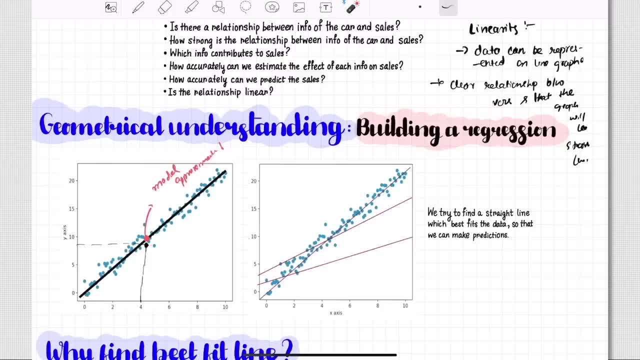 this is the particular uh value of this particular salary, but your actual value states that this is. but there is a difference, so higher the difference bad, bad, your straight bad. your line is for. but why did i say that best fit line? but why did i say this best fit line? so why? 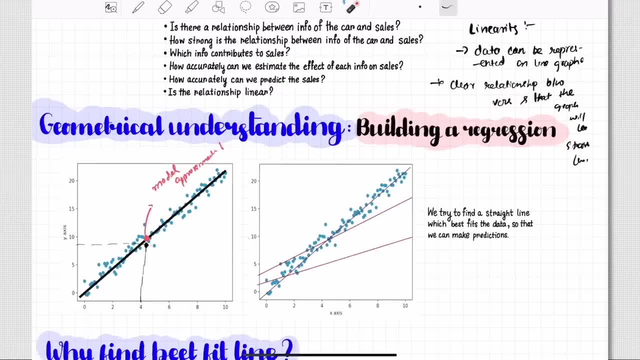 did i say this best fit line because, for example, assume that your line is like this: which does not best fits the data, which does not fits the data? well, so now, if you have four years of experience, if you have four years of experience, you have four years of experience. the model approximate. 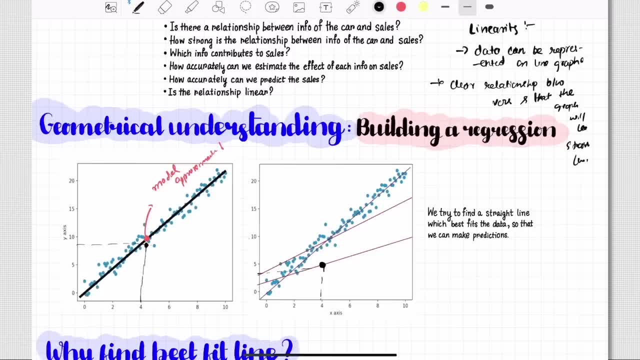 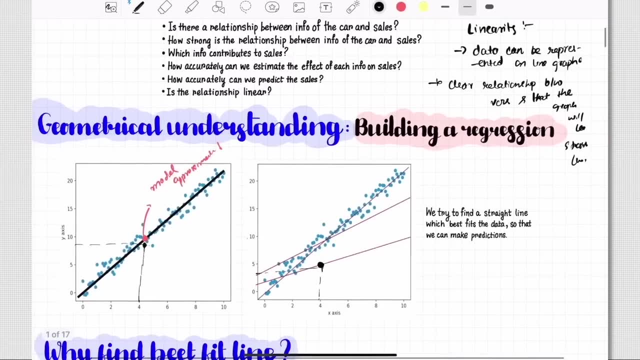 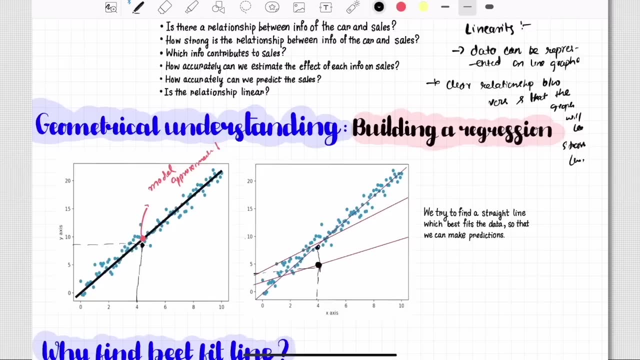 is that intersection point, which is nothing but, which is nothing but four, four thousand dollar, but actually, but actually it was six, right, so the difference is high, so the difference is super high, right, but but actually, if you see that this is your actual value, so this is your actual value. 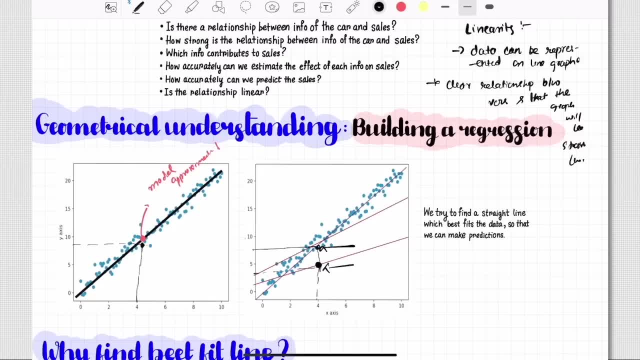 right, this is your. this is your correct answer, but this is your model approximated value. this is a model approximated value, right, so more there's a difference between. so over here there is a small difference, but over here it is a bit large difference. so that's why we want to find the 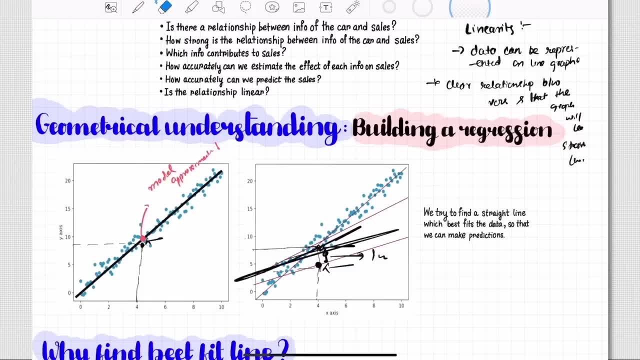 line which best fits the data. so now, for example, so now for. so now, for example, assume that you go to this line, or or the remember And this is the best fit line which is out there, which isn't over here, But assume this line. 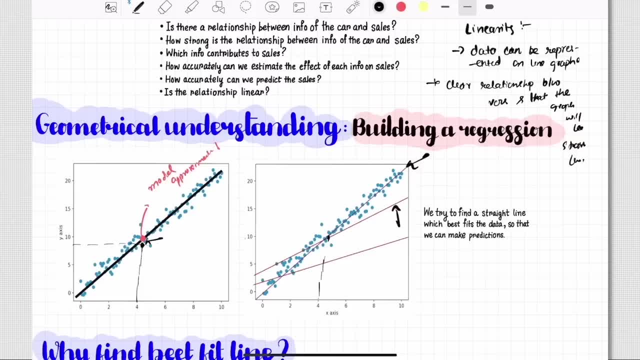 We have four years experience. We have four years experience, This is, But actually the correct is this one? So of course there's difference, But this particular line which best fits the data. we are using that to make prediction. 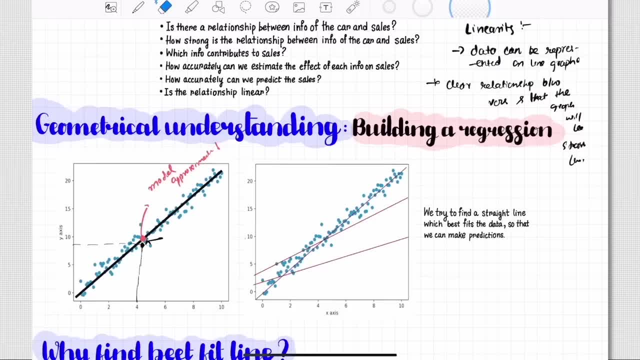 So now I think you got a way to approximate your values. You got a way to approximate your values. Now let's worry about, let's talk about in detail. okay, Let's talk about in detail what exactly I'm trying to tell. 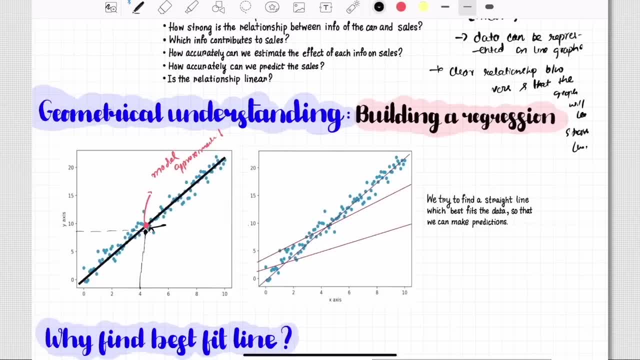 Is why, exactly how exactly we got to our answer. So what our problem was? Our problem was that we wanted to extract patterns from the data. Basically, we want to learn from the data and make intelligent predictions, So we want to find the best fit line. 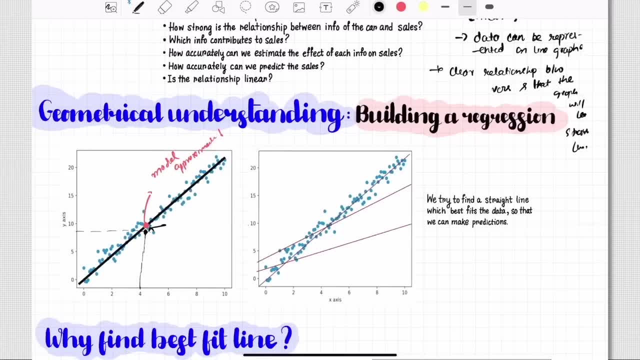 That means learning that best fits the data. For example. you want to learn, You want to Train your mind that best fits the concept, The best fits the concept, And around that concept you utilize that concept And that's called hypothesis. 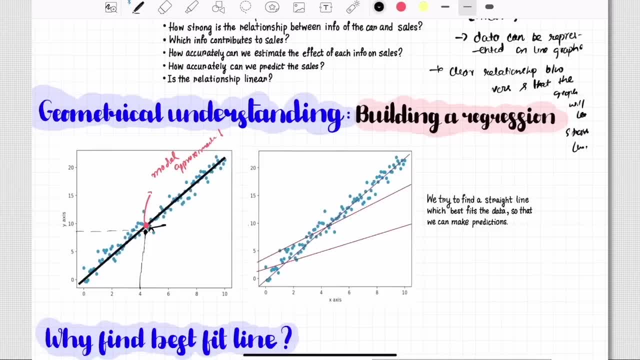 You utilize that step to further make prediction, To further make predictions Or to further solve the question. So in this way only, it first of all makes the best fits the data. Best fits the data by a straight line, It should be linear, right. 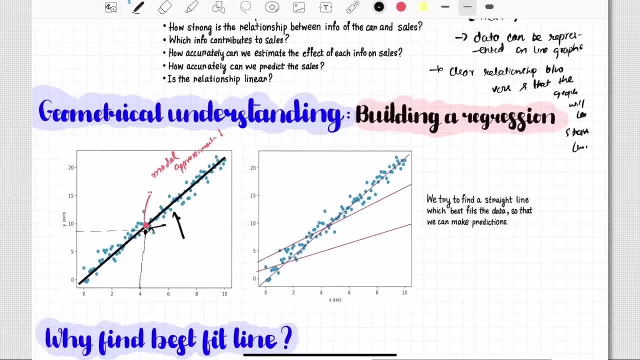 It should be linear, In a straight line, And then it best fits the data, And then we can use this best fit to see. okay, if you have, Currently we have only one input value. If there's more, then there's several things. 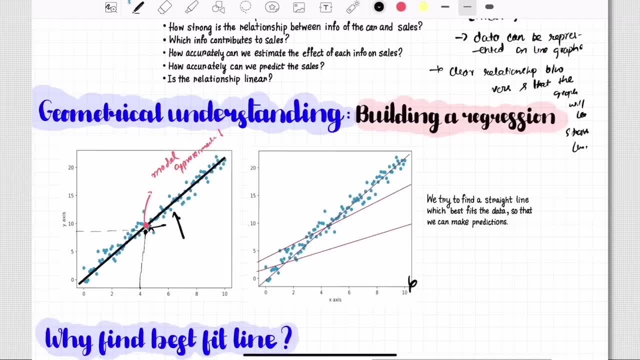 But you have only years experience on a predict Given, years experience on a predict salary. So, given that you can just go, And then this is a point of intersection, So this is your y value, Which is, in this case, the y values on y axis. 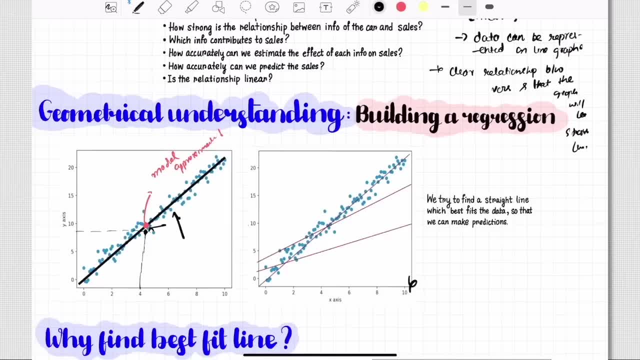 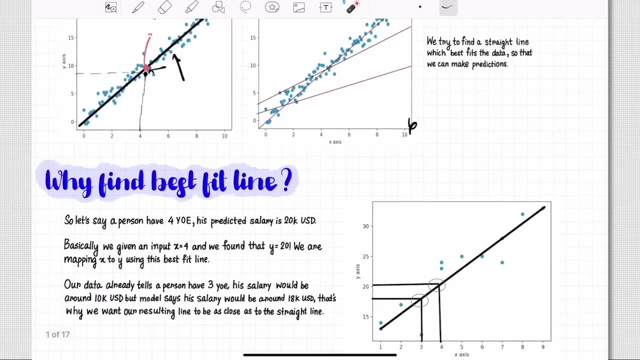 We simply predict that. I hope that it makes sense. If it does not, please review the lecture again and again, And if you still don't, please go and review the concepts of class 8 and 9.. Okay, why? to find the best fit line. 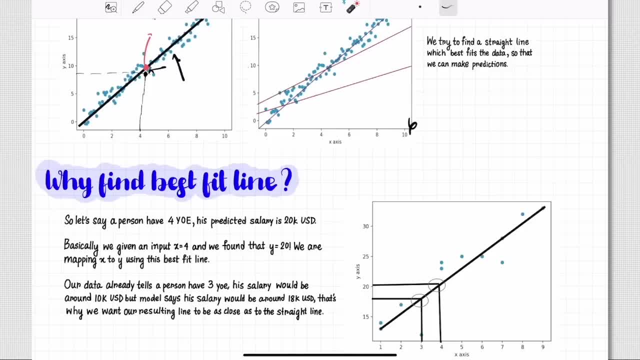 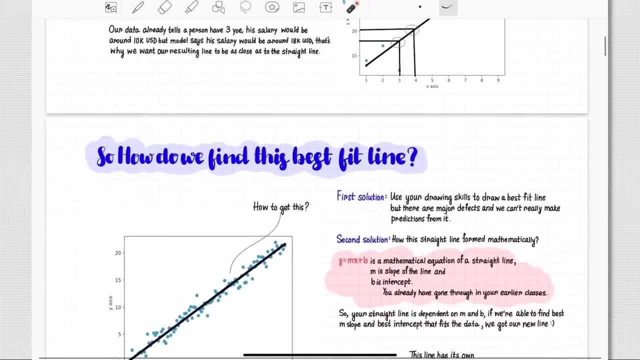 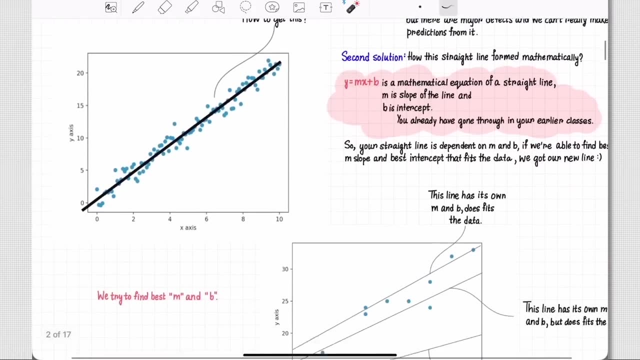 That's a good question about why exactly we want to find the best fit line. So I have given a very nice example out here Which I have just described to you. So now you might have question on how do we find this best fit line? 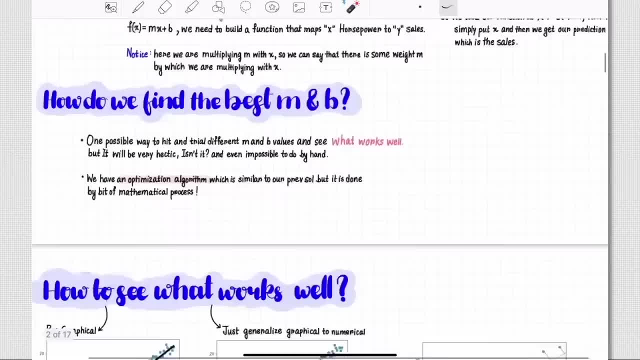 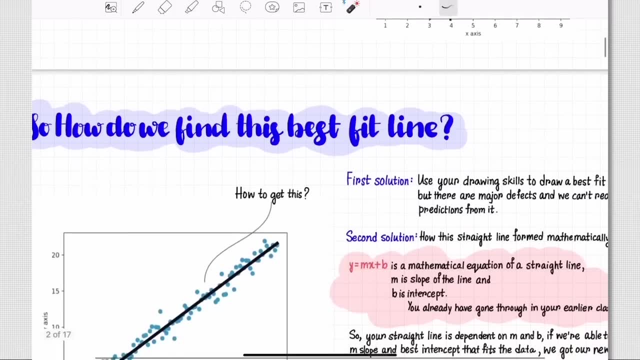 How do we find this best fit line? So let's go ahead and let's try to find this: How exactly We go ahead and find the best fit line. So now you might have question. Okay, now we have the data. 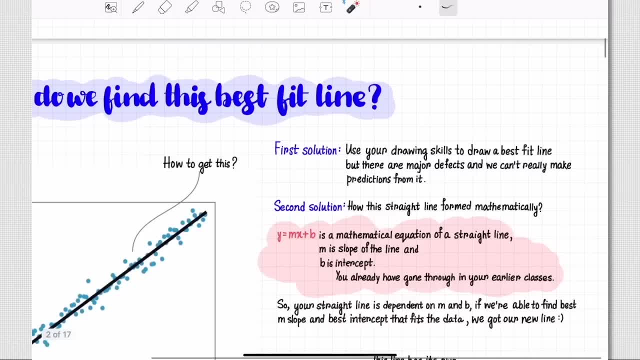 Like: how can we find the best fit line? The first solution in your mind might come that we can plot our data on x and y axis And then use our drawing skills to draw best fit line. So you can simply say and draw like this: 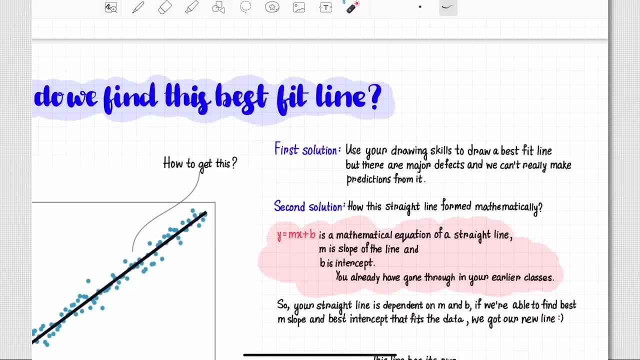 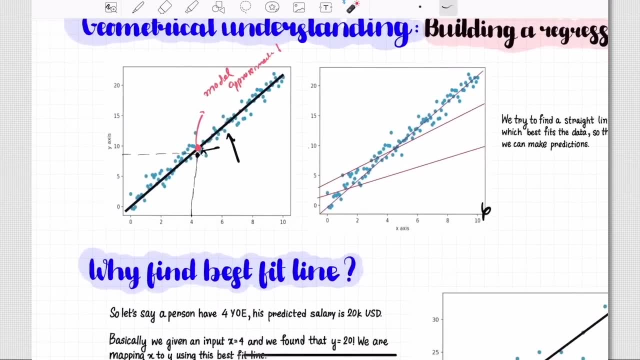 And then draw best fit line. But the major defect is, we cannot really make predictions from that. So how can you make exact predictions from it? Tell me This one defect: How can you tell and give me the exact prediction? You cannot give me the first prediction. 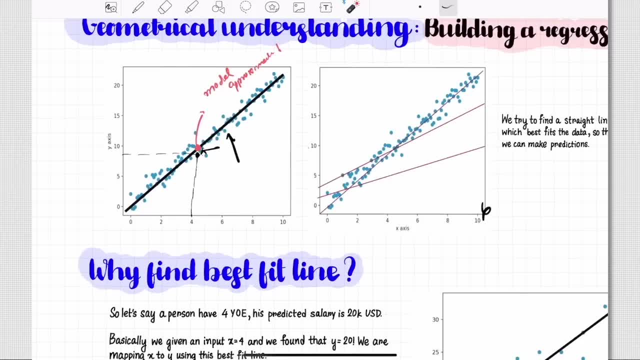 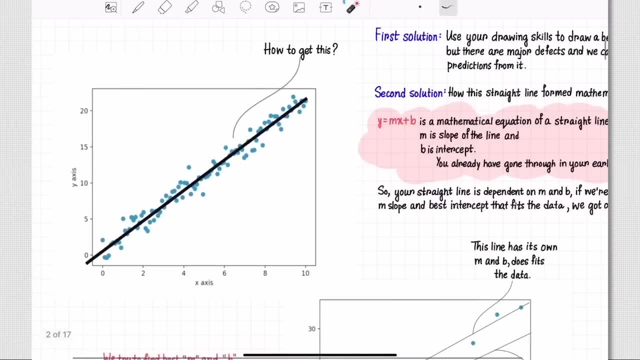 You cannot give me the multiple exact prediction I've just told over here. approximate it, right? Not exactly the same what model. approximate, Just approximate I use, approximate it. That's the first defect. And the second defect is what if you have more than one feature in information? 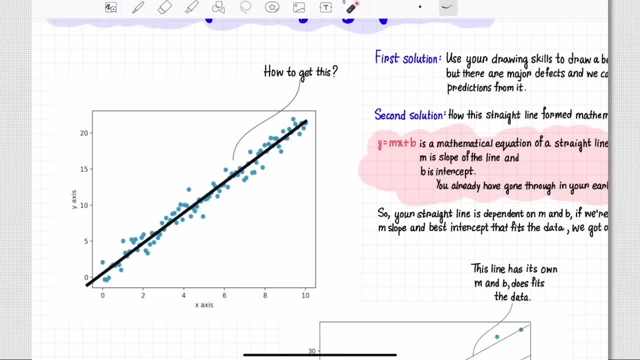 For example, currently it's x and y. only Whether you have years of experience you're going to predict the salary. But what if you have years of experience, the designation, the skills, the readings, etc. So four x's, four input values, you're going to predict one salary. 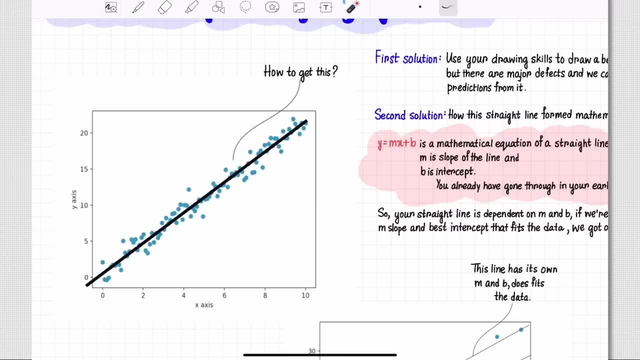 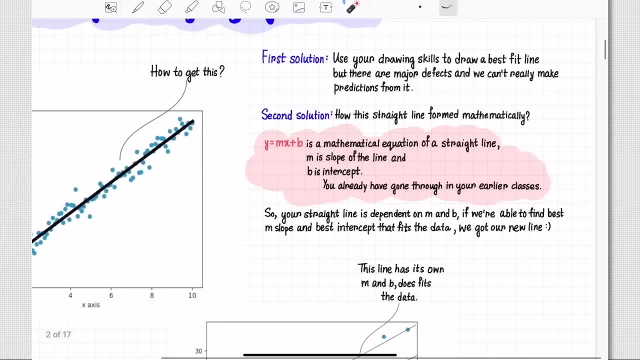 So this is a multidimensional thing. You cannot really plot a straight line. That's the first solution cut Where you cannot use the drawing skills to draw a straight line which the best fits the data. So how can we get this straight line? 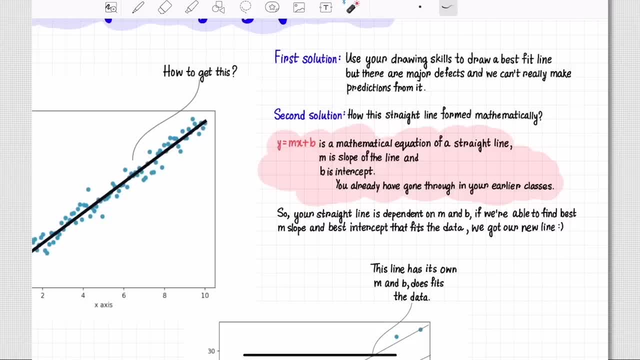 So the second solution is that, as of now, let's go ahead and talk about only one thing, which is you're only given only one information, which is x, which is the years of experience You're going to predict the salary. 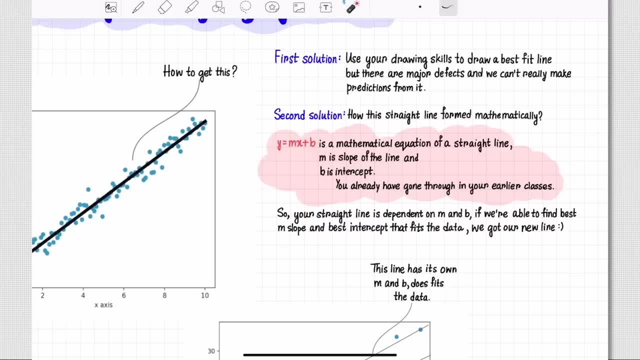 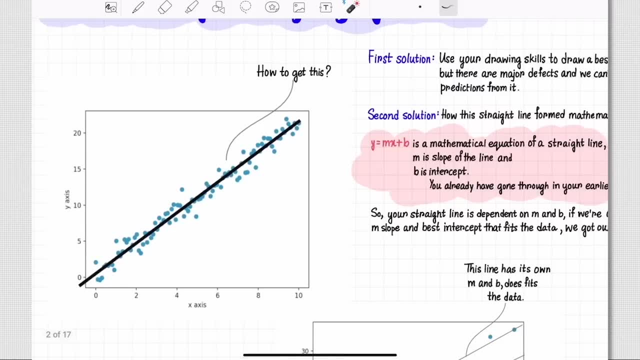 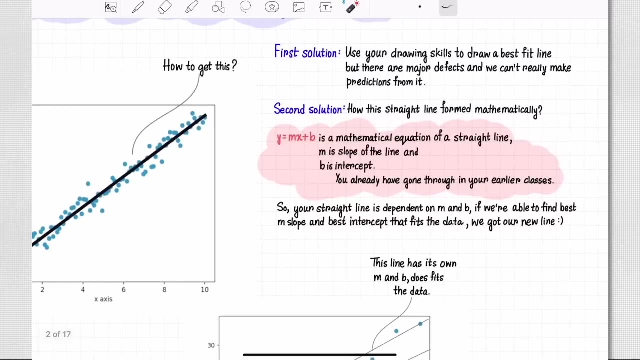 That is only one. So how can we do this? So second solution might arise, that you might have seen this in your early classes: y is equals to mx plus b, yz. This is an equation for any straight line. So y equals to mx plus b is the mathematical equation for a straight line, where m indicates the slope of the line and b indicates the intercept of that line. 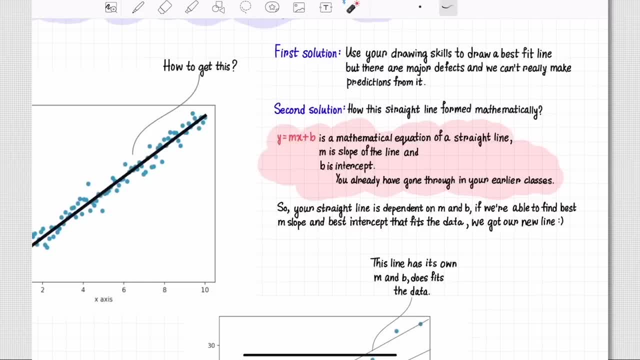 Slope means how much y changes when x changes. and intercept b, which is the y intercept, which is the y intercept where your line cuts at y right. If you don't know about the concept, don't worry, I'll just recap. I'll just recapitulate a little, a little, a little bit on this. 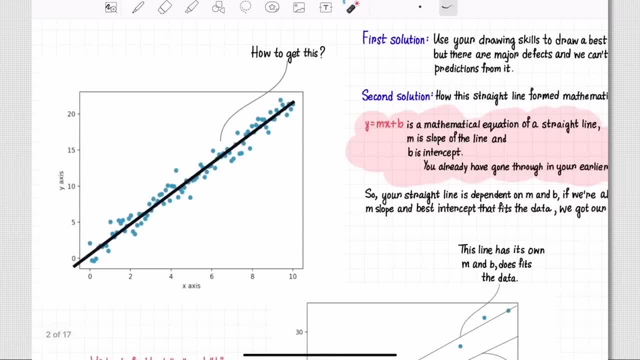 So what exactly slope in this example? So slope in this example states that how much my salary will change, how much my salary will change if my years of experience will change. That's the slope. that's the slope which says how much your y changes. the salary changes when x changes. that's the slope. 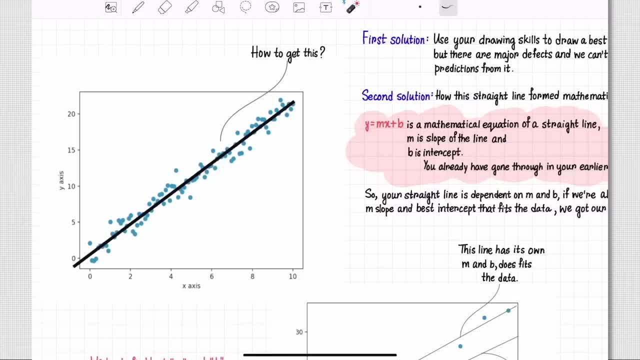 So m over here is your slope, and m is also the coefficient of your x and x, in this case is your years of experience, plus the y intercept. where at exactly your y intersects And y? y intercept is one of the major thing, because we'll talk about y as term later on, but over here, if you have this y intercept over here, if you've, then y intercept also plays a very nice role. 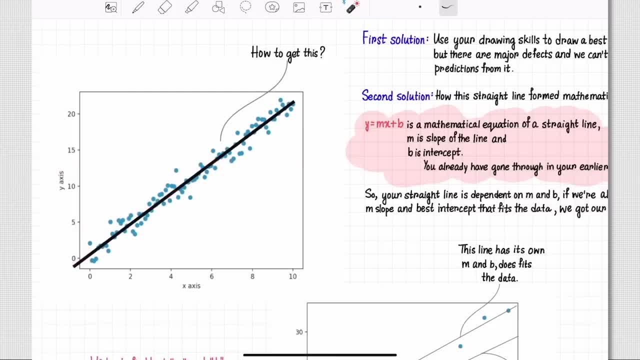 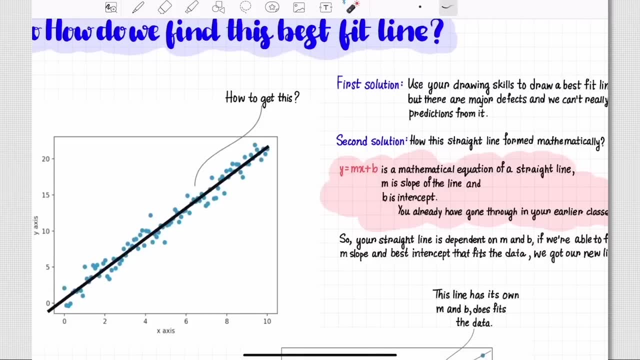 So over here, this is the y intercept. where did y cuts on the y axis? So now there's one, There's one interpretation which we can get from this, that, if we are able, so this particular line is fully dependent on this in these two parameters. 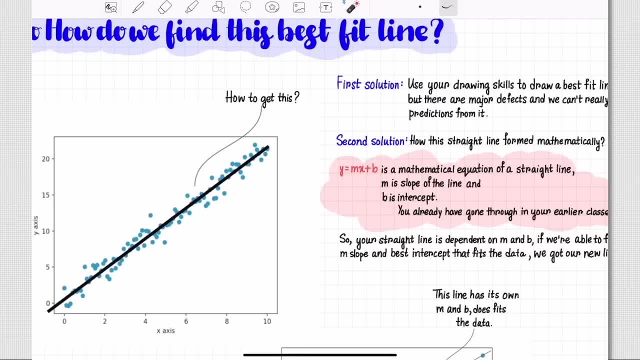 Only these two parameters can change this line right. Only slope, because x will be anything right. But but m and b determines how this line should be. So slope and the y intercept. So if y- y intercept is different, it should be like this, it should be like this and slope is different, it should be like different, different shapes. 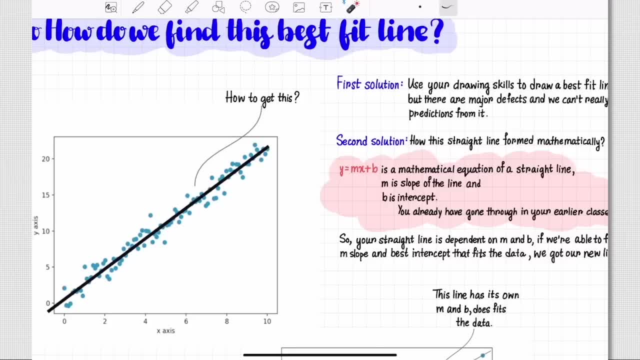 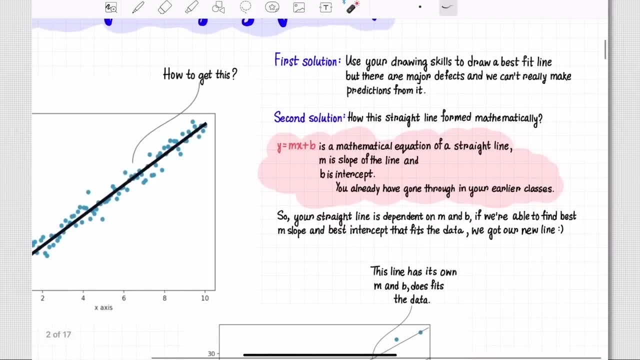 So that your, your straight line, your best fit line, depends on the slope and the b, which is the bias term. so a straight line is dependent upon slope and the y intercept. so if you are able to find, if you are able to find the slope and the best interface and intercept that best fits the data, you got a new. 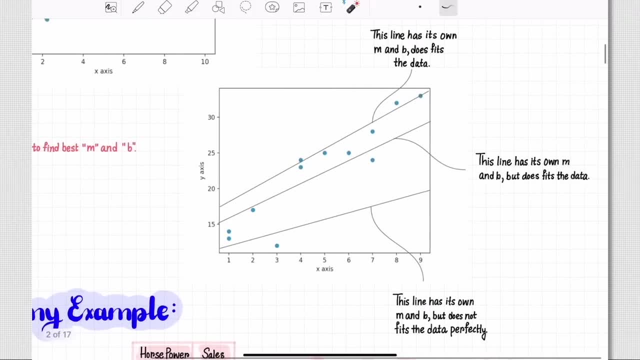 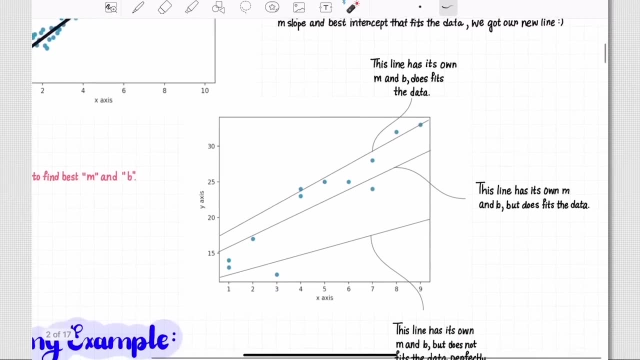 line. so very interesting, very interesting. uh, an analogy is why i'm saying that they are dependent, why i'm saying that we are depend, that our straight line is dependent, for example. so you have, you have, you have this data where i plotted the very smaller, small amount of data. 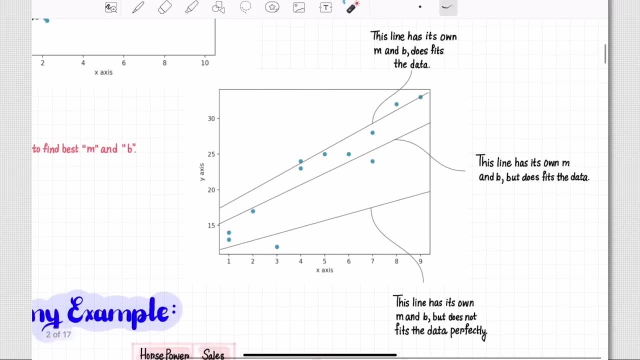 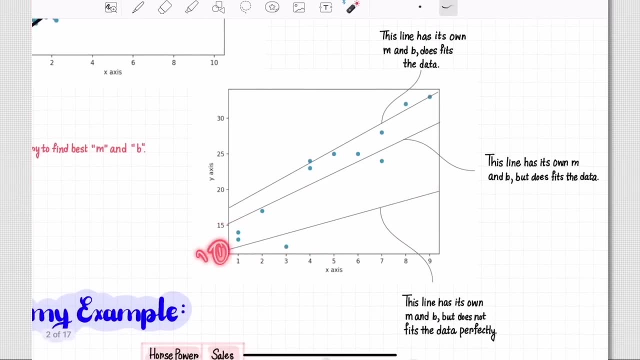 and in this example, uh, and in this example, assume that we have this, this particular, assume that we have three, three different best fits lines. let's go with the first one. let's go the first one. this over here, our slope is different and y intercept is different. that's why our it is not perfectly. 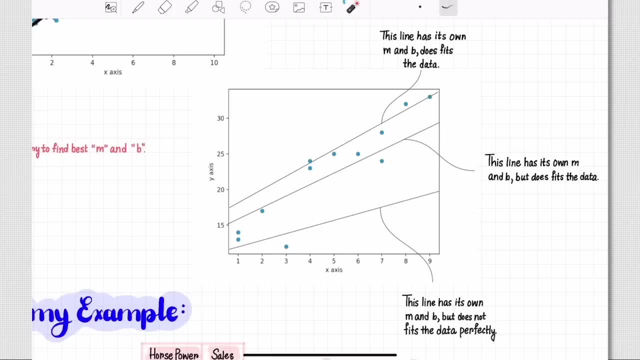 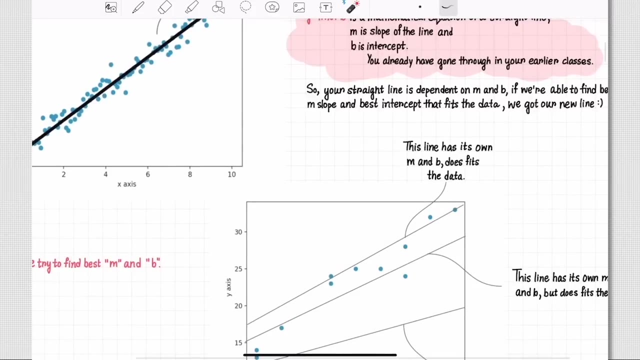 fitting our data. so now we tweaked in a way that we changed. we changed the slope and the intercept. we go to this: it okay, fits the data. but over here, which again changed, and seen that it it is also, it fits the data very well, right, so so so you're, all is a straight line is dependent upon m and b, so if you're. 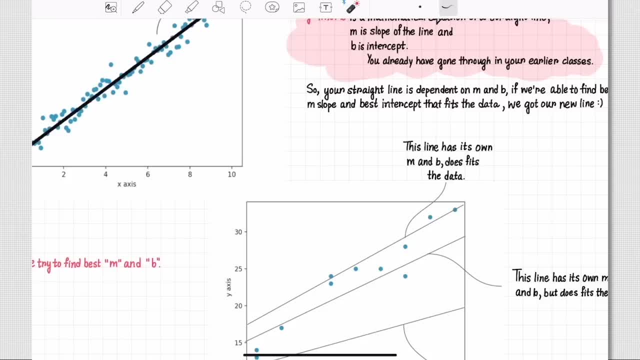 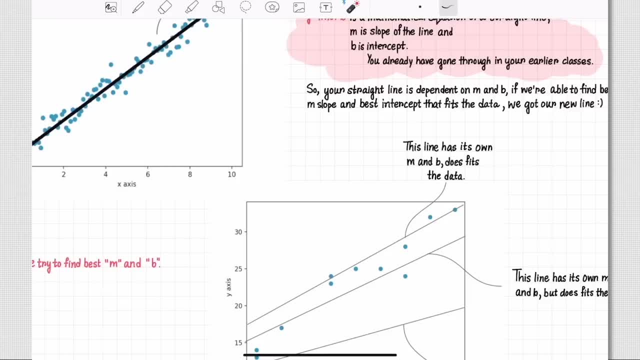 that's a nice analogy. i hope so that you're getting what. what? what i'm trying to tell is: i'm just trying to tell you that you want to get the best m, which is the slope, and the best b, because it determines your values. it determines your x values. 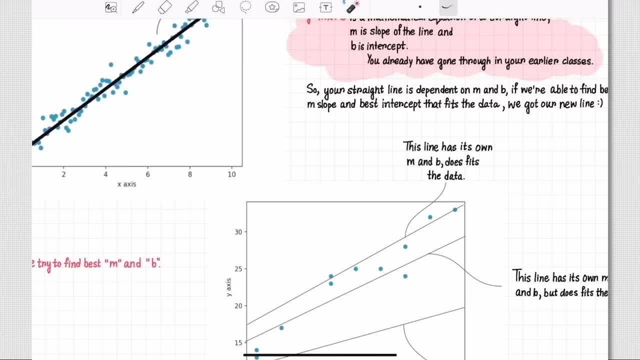 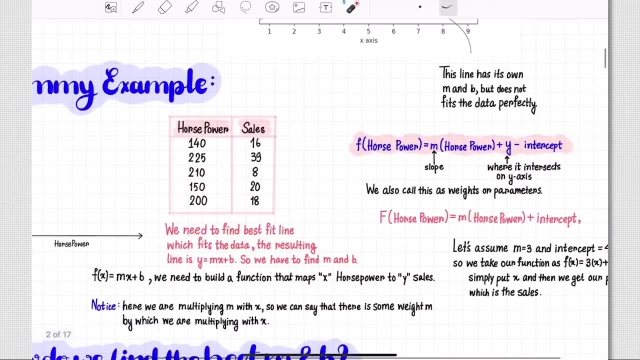 right. so i hope that this could. this gives you sense that are. so if you're able to find m and b, we'll be easily able to get the best fit line. i hope that this makes sense. okay, i don't need to again repeat it again and again. so this is a very dumb example which which. 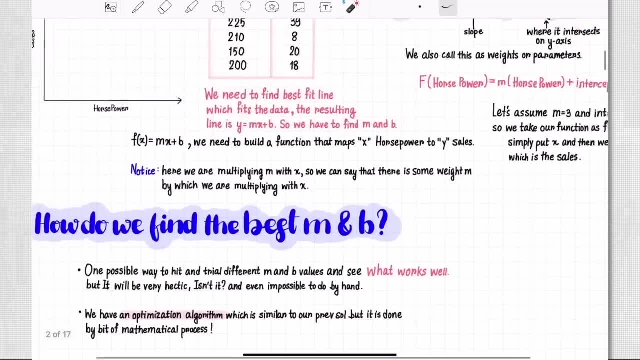 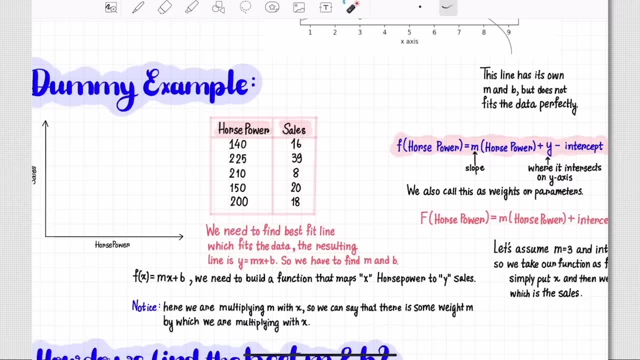 which, which you're seeing in front of me, uh, is about is is about horsepower and sales. so so you're, you're given the horsepower of a car. you're given only one information. as of now, as i said, we'll only go with one information. uh, so you're given the horsepower of the car, your rfi, based on horse. 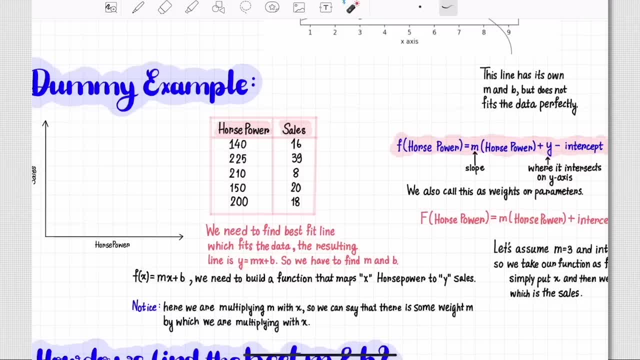 power. what is the sales for the car? right, you know you identify that. so to find the best fit line, that. so if you plot this data it should look something like this: so if you plot the data, you have to best fit data. so sometimes you don't need to really draw, make your graphs. you know, you know draw. 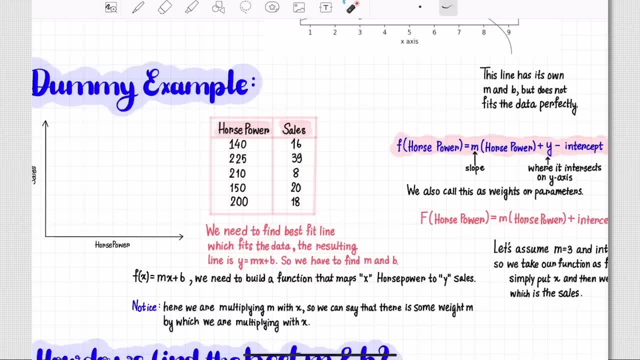 you know, find the equation, you'll find a straight line or linear equation. um, not linear equation? yeah, so the the straight is straight line equation that best fits the data. okay, so you build this function f. you're gonna build this function app that takes in horsepower, and then, and then uh, 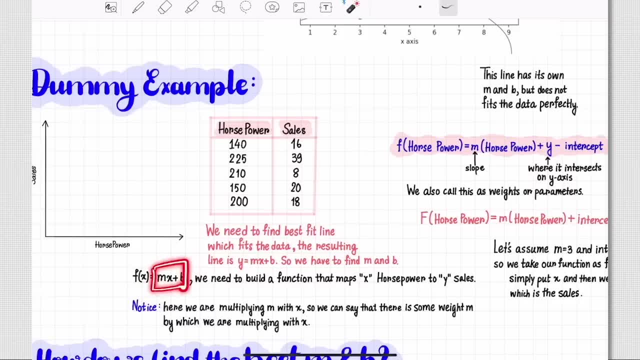 does, and then multiply, and then you have multi, and then you have the straight line equation which is used for use, which is used for making uh predictions. so we need to build a function f that maps your x, which is the horsepower, to the sales. establish a relationship. 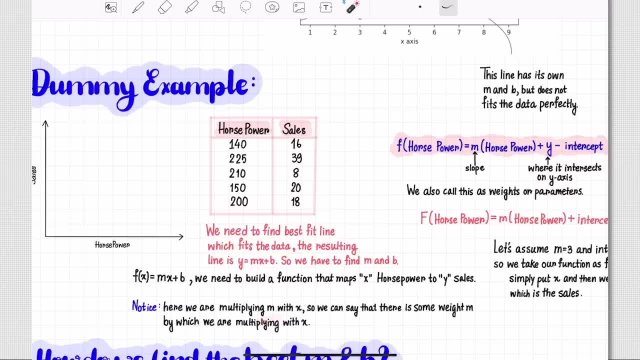 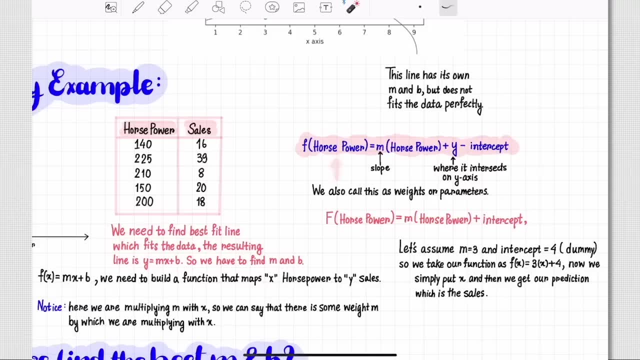 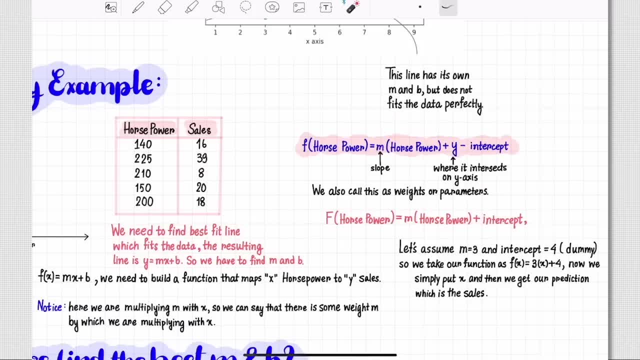 why? how much? how's horsepower, how much sales? will sales changes when horsepower changes, plus y, which is your y intercept, which is y intercept where it intersects on y-axis. so now you might have question that: how the why we multiply and how does this affect the output. so when we multiply, what effects does it? goes on output. 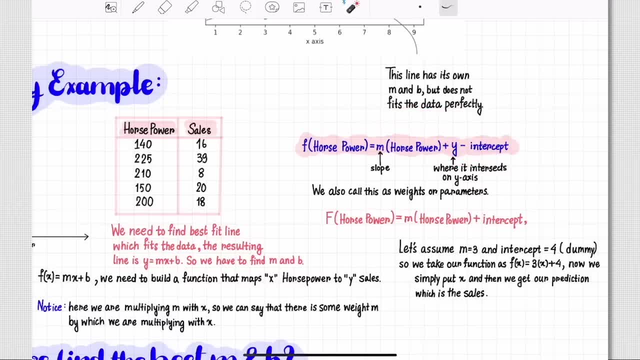 variable what effect this y intercept gives through the output variable. that's something we should talk about in interpretation of our coefficients later on. but as of now you can get that. then this is the equation: where you put in the values of x, you'll get the particular value. 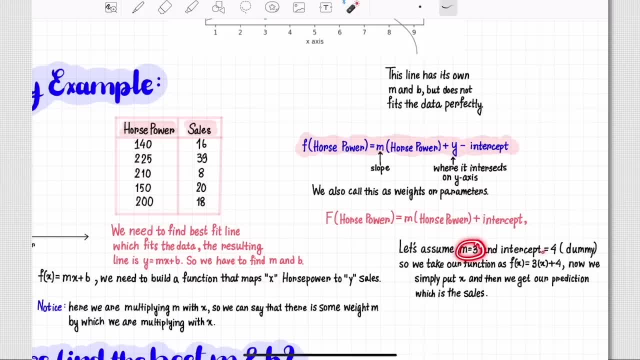 you can see over here. let's let us assume your slope is three and intercept is four, which is dummy as of now. so we take our function. so now, this is a function like this. now you have built your function and built your function. you built your function, built your function, so you simply 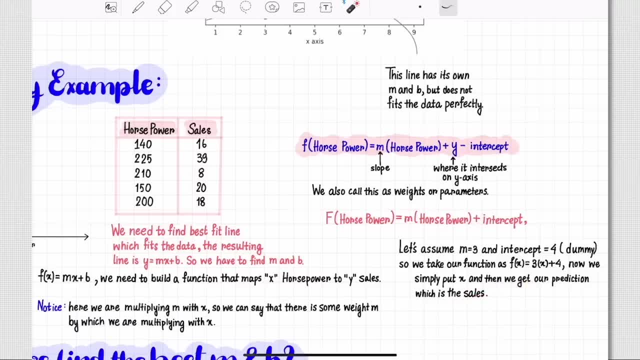 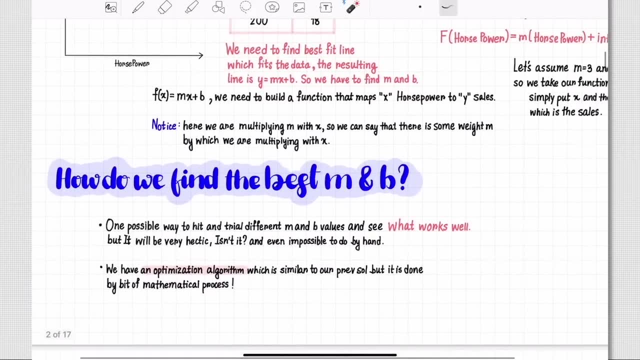 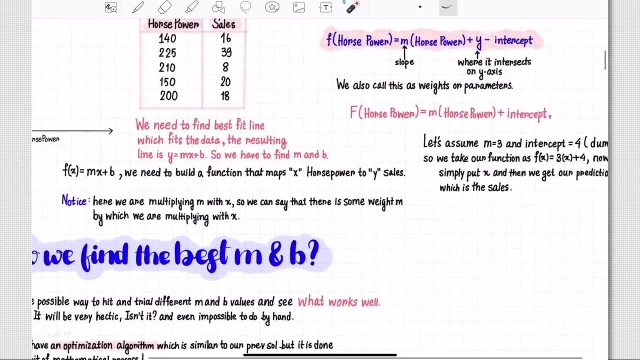 give the value of x and then get your answer, and then you get a prediction which is number of sales which you'll get. okay, so, um, now you might have service. now, now you know you might have, uh, several questions right now, like how can we find our best mnb? like currently we have just taken a dumb example, so how can we find best mnb? 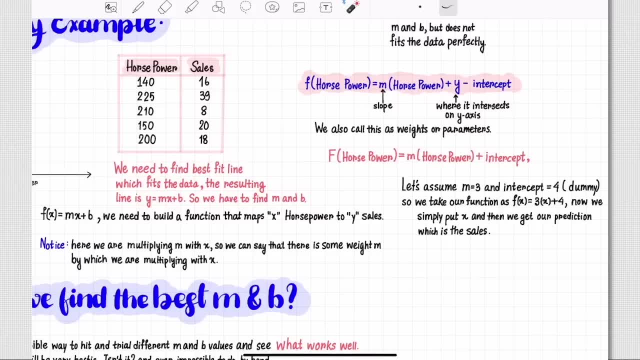 what exactly this mnb contributes to the sales, what, why exactly we use it first of all at first place, why exactly we use it, etc. that that can be will. that will be answered in later phases as you go, but as of now, what i just want to tell you: you have got to know that very nice geometrical 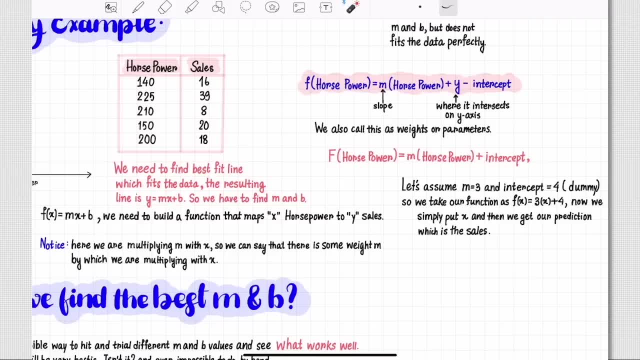 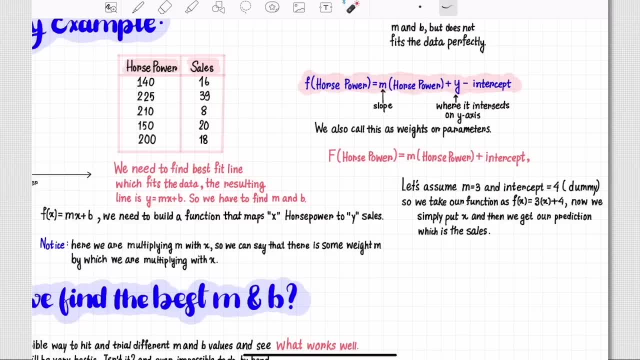 from my website. you can also uh enroll in the course which i'm teaching in fully ml pro, which is from teaching from baby basics to earning opportunities, etc. so i hope that you will enroll in that. let's catch up in the next video, typically. so, folks, we are going to continue our. 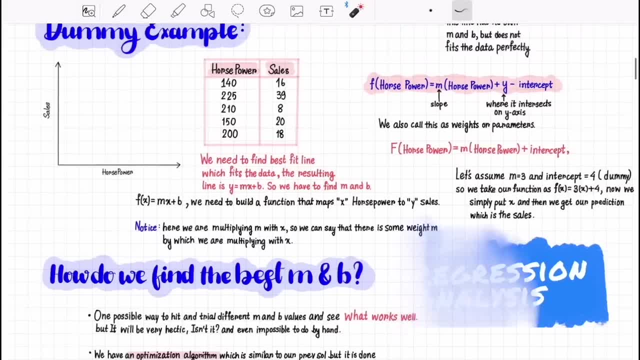 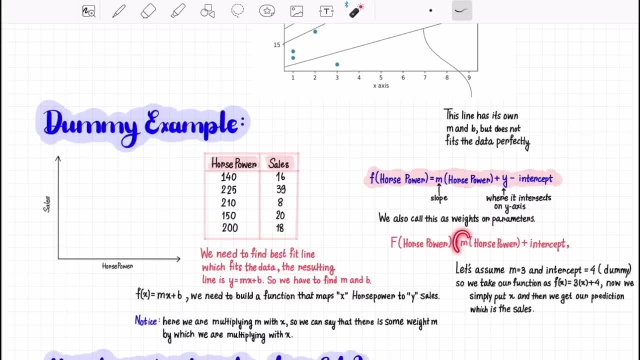 journey on regression analysis. so in the previous lecture we had a talk on this, some example and we have shown that, how each uh, like we have m and b, and how this m, how horsepower, has its own weight, and then we have an intercept. we have talked about this. if you haven't seen my previous 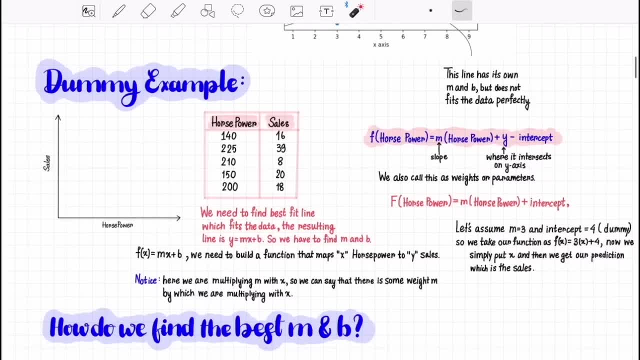 video. please go and see about that. so our main idea was: how can we find this main m and this intercept, which we usually call as b? okay, so my question was: how can we find how to find these two terms, because your best fit line depends on this m and b. only right. so basically that that was. 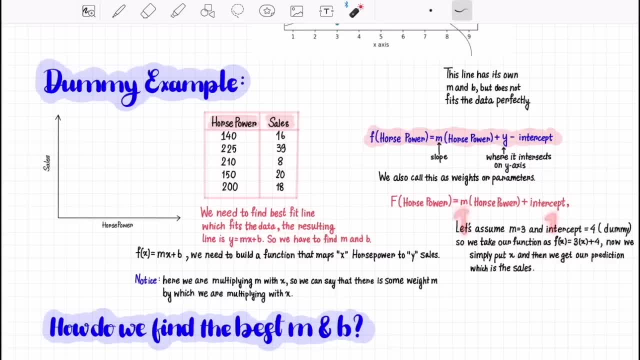 the basic question that your best fit line depends on this. so for, if you want to get the good fit line, then you need to find this m and intercept, which is a slope of the particular variable- how horsepower- and the intercept of that particular variable. so i hope that that makes sense. now, what, what? 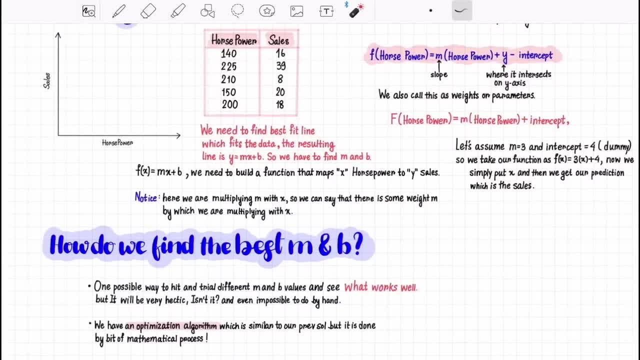 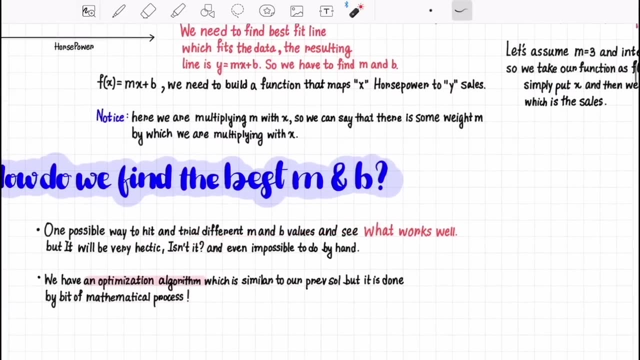 we're exactly going to do. we're going to study about how can we find best m and b for your data, which is eventually, in other words, best straight, best fit straight line in your data, right? so what was the pause? what is the sum of the possible way which we can think of so over here? what is one of? 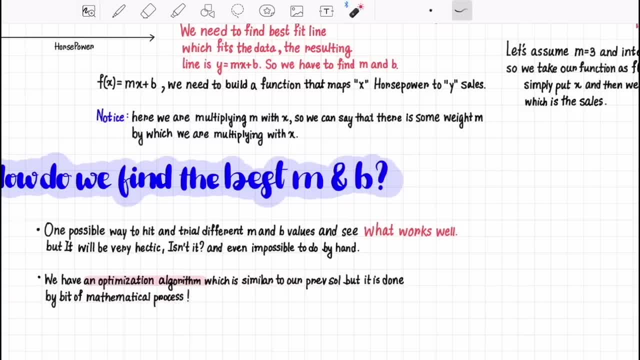 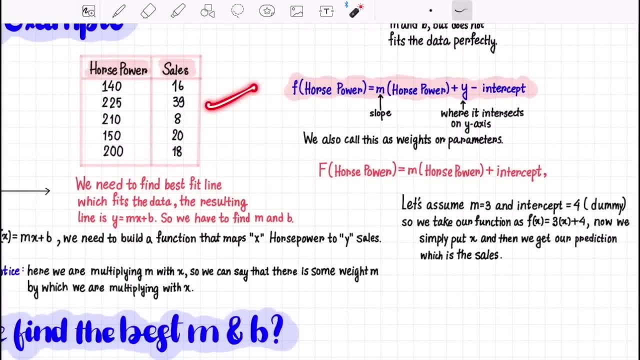 the possible way is to hit and trial different, different values of m and b and see what works. well, right. so, for example, for example, in the, in the, in this example, you know you're gonna use the, you know builder function f that takes the horsepower as an input that takes the horsepower. 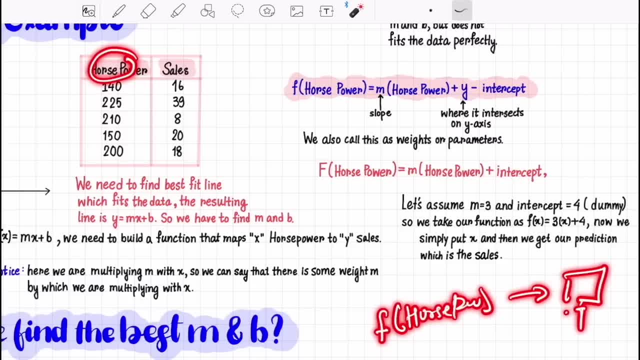 as an input and predicts the number of a sale. so if you want to promote your car with that horsepower, what is the possible number of essays we have you're going to get? right so you know. build a function f that establishes the relationship between your horsepower of a car and the sales. right, so you know. predict how how much sales would be done if. if we actually 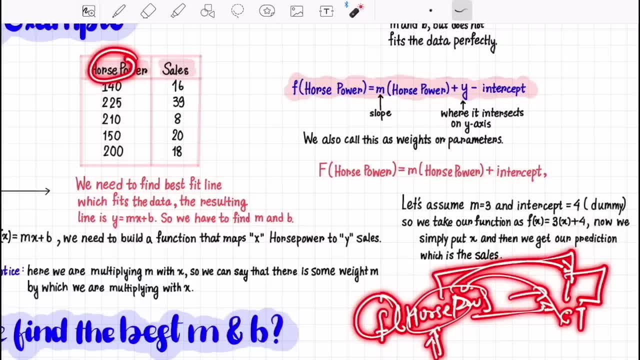 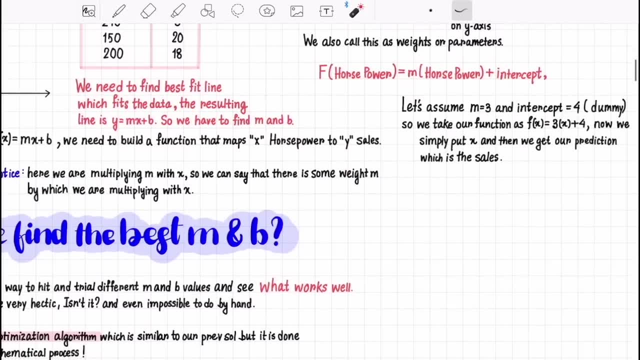 use the horsepower as an, or how much sales are based on horsepower? what is the relationship between them? right, that is the one question out there. but what i want to convey is that over here, for for building, let's assume that x is a horsepower. you have mx plus b and m. for for 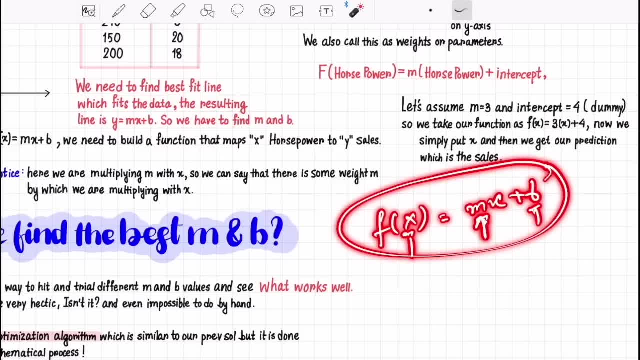 finding the relationship right. so here, over here, m and b, we need, we need to find out. so over here, you, you cannot just plug anything like. we have seen that if you plug anything we are going to we're not going to get a best fit line. so what can we do? we can, we can try out several values of 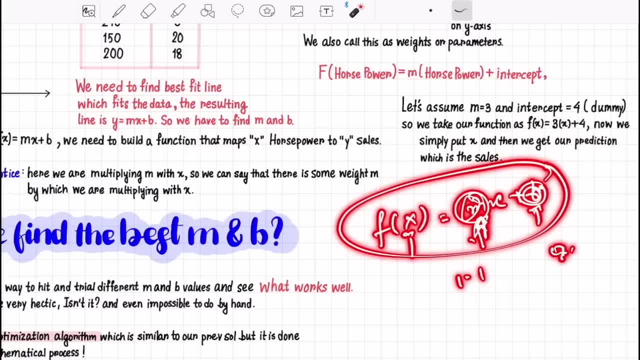 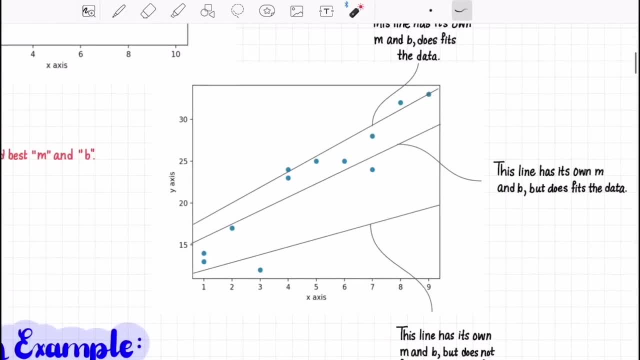 m and b. so we can try it: 1.1 or the, and then some 1.2, and then, with these values, given the x value, we can test how well these values are by plotting it on a straight line like this. so um, we plot on. 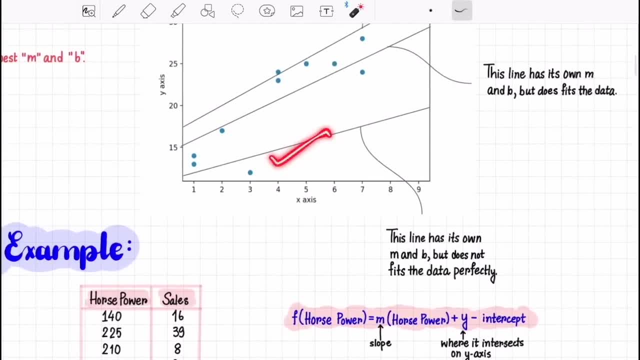 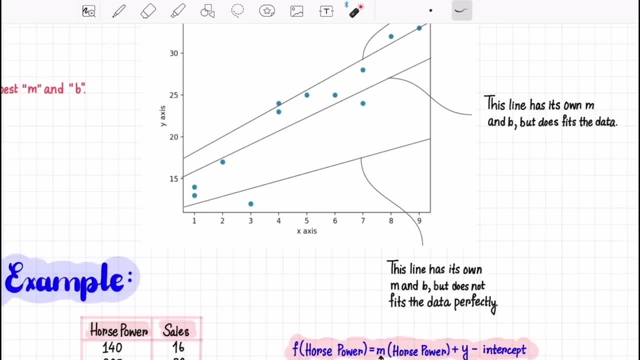 a straight line and see how it performs by hit and trial. right, we first of all perform like this and then the next. what we do is we conduct another, we try another value and see if you're getting the best fit line. so you, what, what eventually you will do. 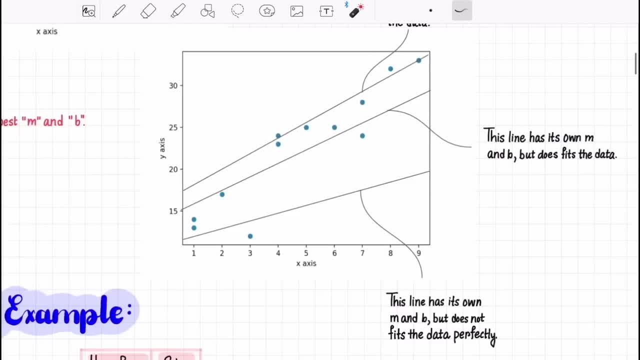 you will try this several set of m and b, right, and then you will try to plot the best fit line or the plot that equation, and once you plot it you will be able to see: okay, this is the best fit. i know this is not so. you'll plot and see: how is it the best fit line, right, so hit and. 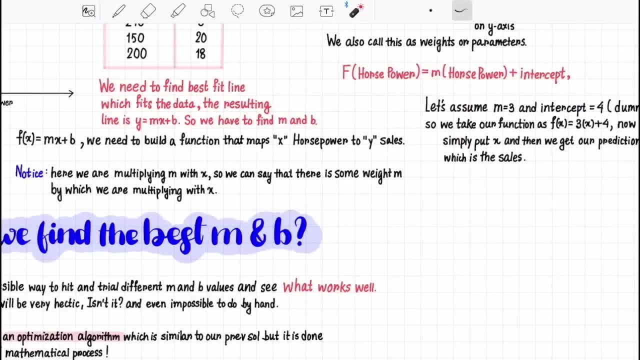 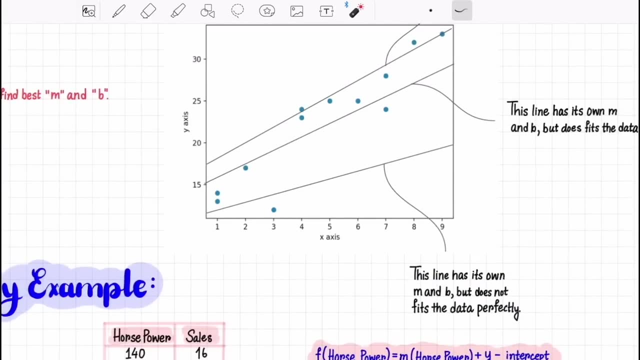 try different values and see what works well. but it has several problems. the first problem is it will be very hectic. it will be very hectic and time consuming and time consuming, okay, first thing. second is what if, if you have a 3d or 4d um in higher dimension of data, right, you might have 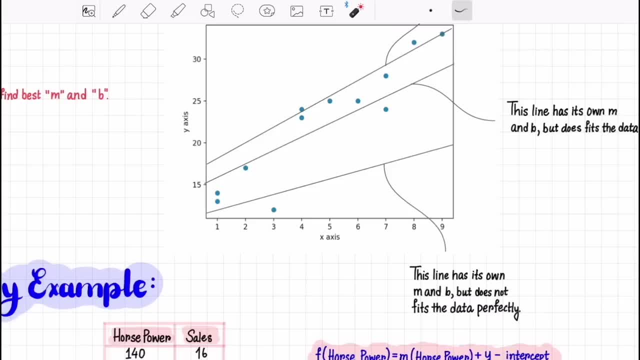 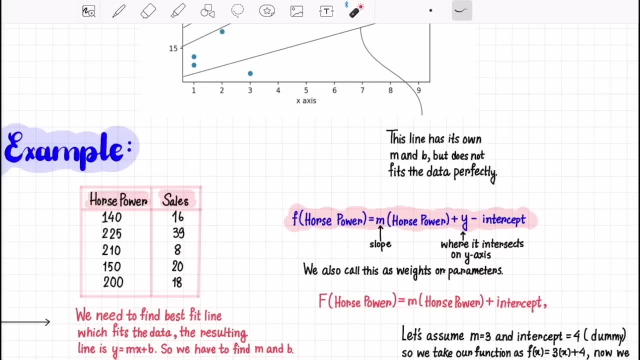 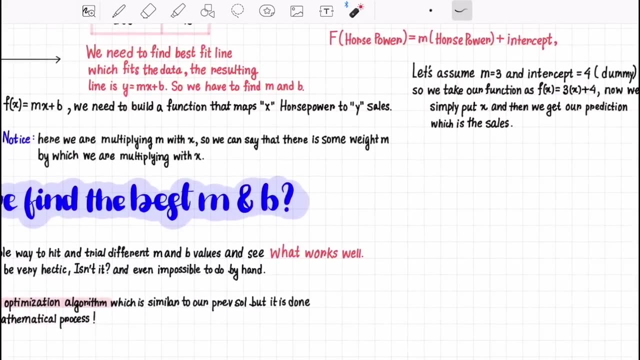 you might have higher dimension of data and you may not be able to plot every time and then see: right, so in that, in that real world, data will not look like this. it will have a millions of examples, millions of input features, right? so, uh, we exactly want to talk on, uh, that, so we cannot really plot. 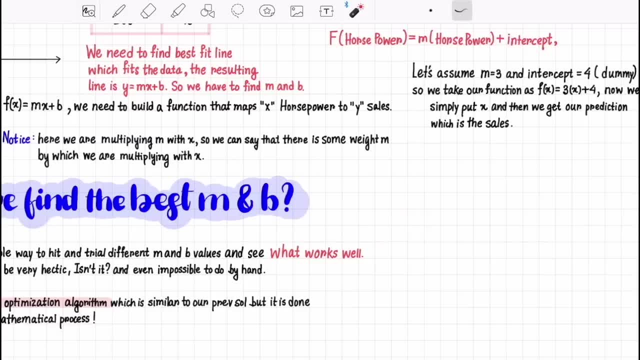 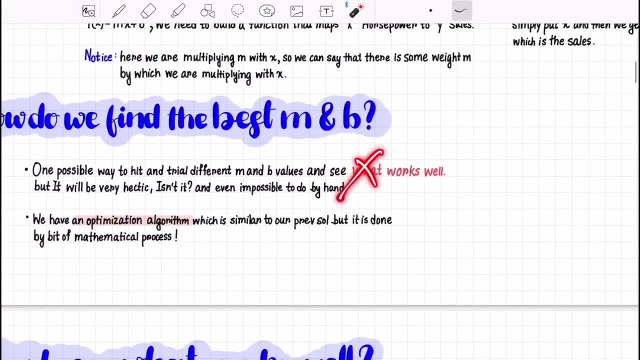 and then see against right. so that second one is: it will be very hard for us to eventually plot the data and see every time, so eventually hectic and time consuming, so we need to cut that approach out. what's the next approach? we have an optimization algorithm which is based 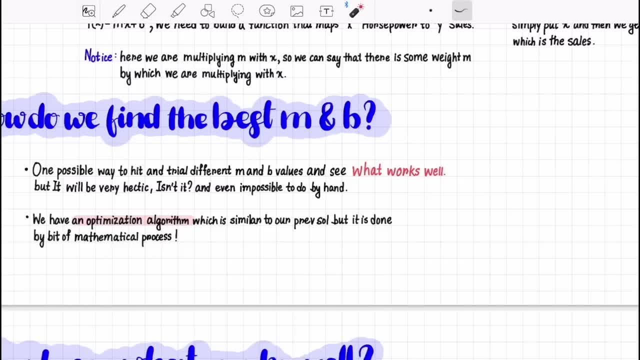 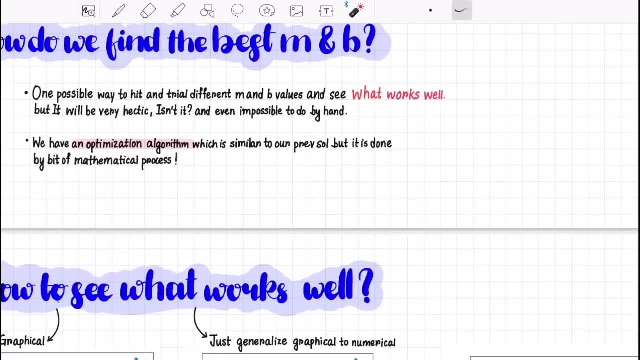 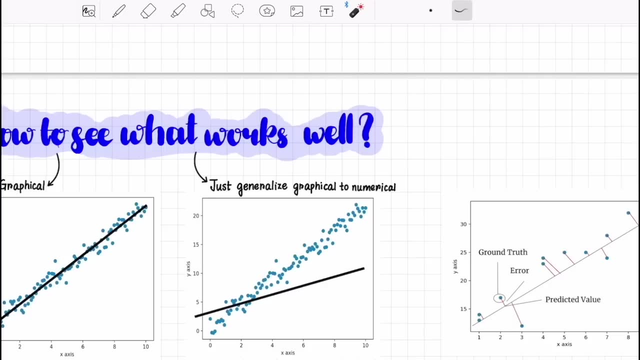 on this hidden trial only, which is based on this hidden trial only, but we do it very strategically. you learn how we do it very strategically using mathematical process, right? so i hope that will make more sense when i actually go into this now. um so, let's, let's see. let's see how to see what. 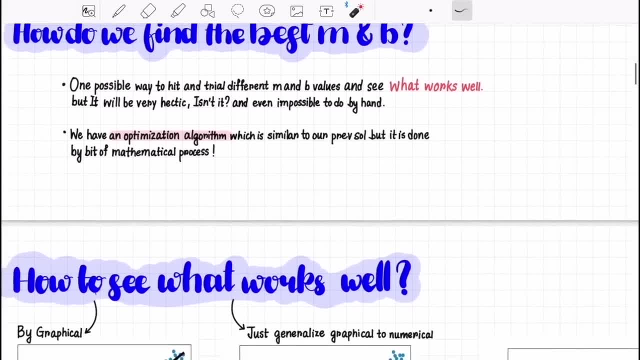 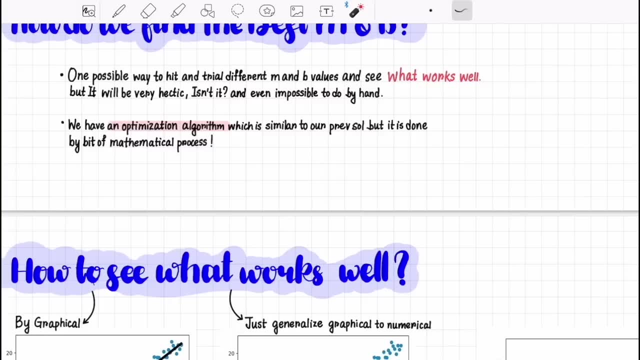 works well, right, so how to see what works really well? so over here, as of now, we have seen that we can use optimal optimization algorithm to come up with that. so, uh, but before that we need to see how what works well and what not. then we can come to this optimization problem. so if we want to see 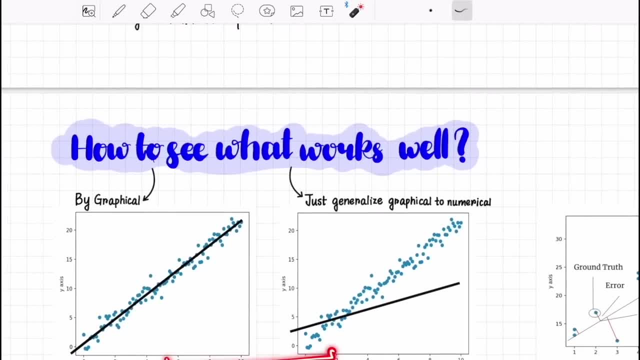 the graphical problem. like over here, we have two sets of data, so the first set of data has this, this, this data, and then you plot the best fit line and this is the best fit line available for your data. and over here, you, you, you don't have the best fit line, so this: 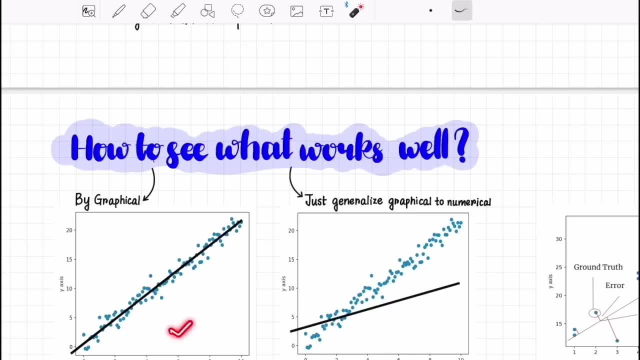 particular this: this particular equation is wrong, but this particular equation is correct, right? why? because this particular equation has a best fit line, or this particular line fits the data best, and this particular line does not fit the data well, right? so that is one of them now over here. 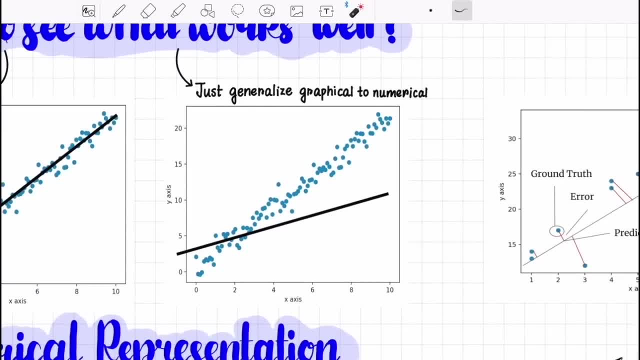 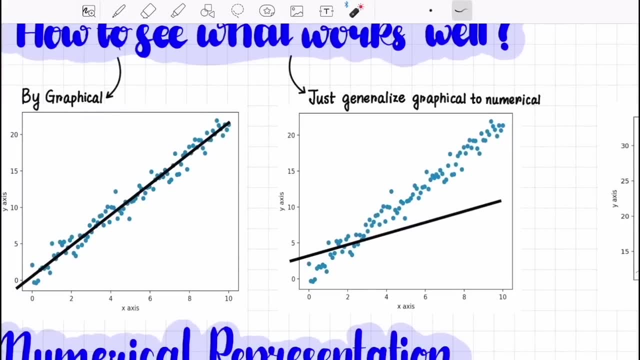 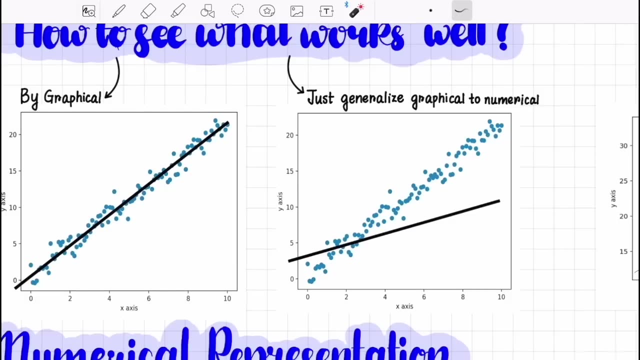 you can see that over here, you can see that it is not fitting the best fit line. so what is the? what is the conclusion which i make is: if you want to see the best fit line, which i've already seen is will, will be this. but by now we are only seeing, or we are only telling by seeing the data. we are only seeing. 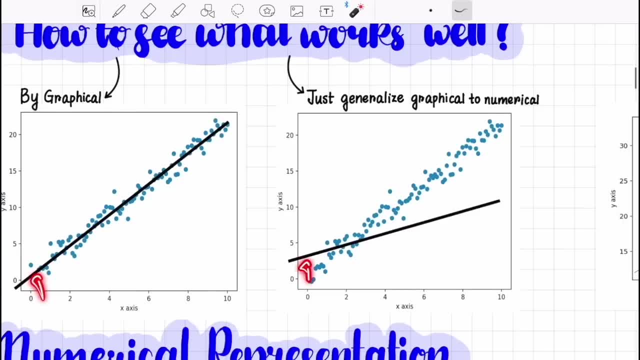 uh, we are only telling: how is this the best fit line? is the best fit line by only seeing the data. but data will be. you know, you have only the horsepower. as of now, there will be a lot, of, a lot of uh input variables. for example, you may want to establish relationships. 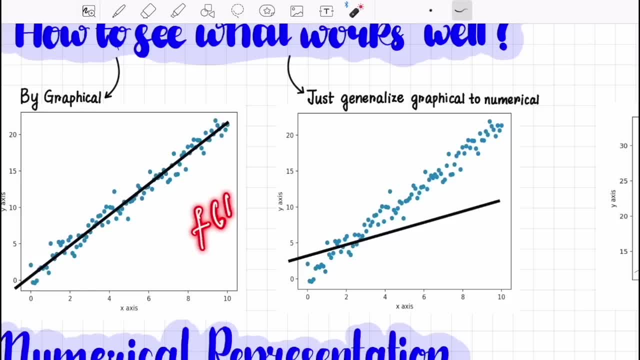 you know you may want to establish a relationship between, maybe horsepower, and then you know another one which is the brand of the car. you know the, so social media, you know engagement of the car and blah, blah, blah. i mean to find the relationship where all of these three to a particular variable sales. so we have to find you will be getting 3d. 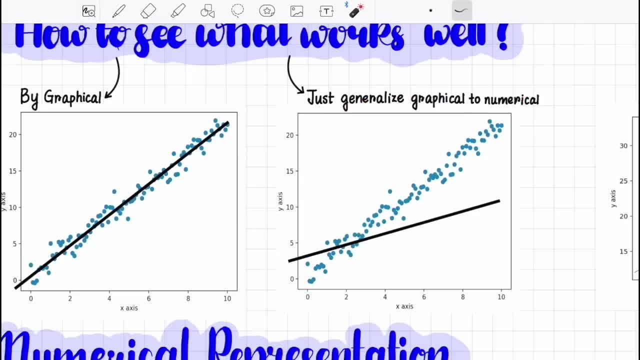 we'll learn about this. uh, multiple, uh, multiple linear regression. we are soon, but you will see that we will have three dimension of data, even four dimension of five dimension of data. right, but it's not always possible to plot. it will always not get only some 100, 200, 300, or you'll get 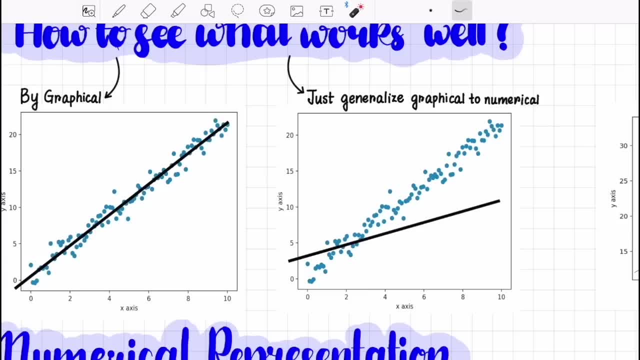 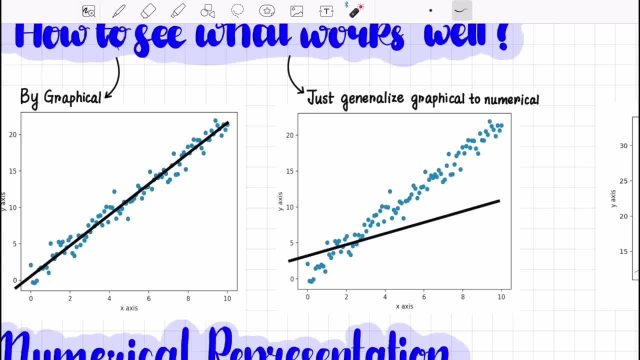 you can see that how it's performing. you can see that how it's performing. it's not for something which you have to do in real world, but sometimes it also comes in handy if you have a small amount of data. but eventually you'll have to deal with numerical way. 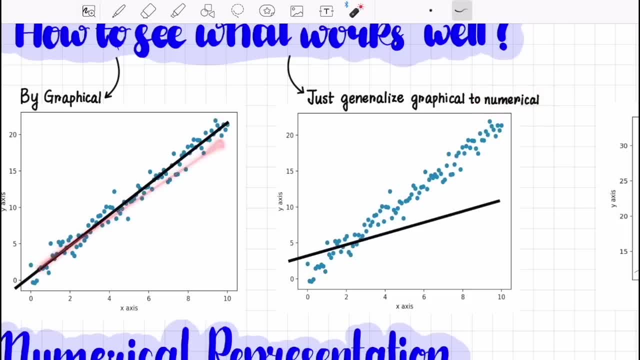 right. so, for example, when you plot the, when you, when you plot the line, you can, for example, assume that you have a equation: x, f, f of x is equals to x squared. so the, the, the graphical, will look like this: the graphical is parabola, the graphical is parabola, but you cannot eventually use this. 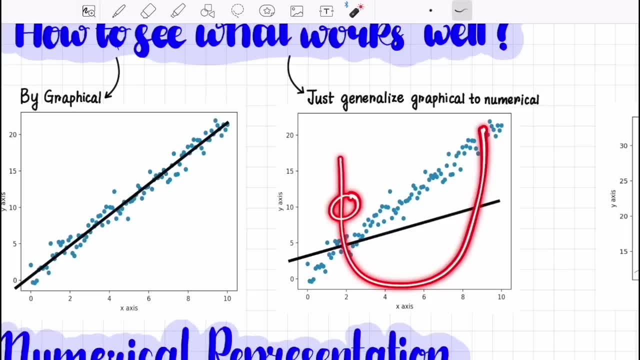 to get your answers. for larger values, you know, for larger way for subset, you can do. for two or three you can do. but what if one, two, five, nine, nine, nine, so you cannot even do that. you cannot even try to use this parabola to do that. you can eventually do that, but it's very hectic and very not possible. 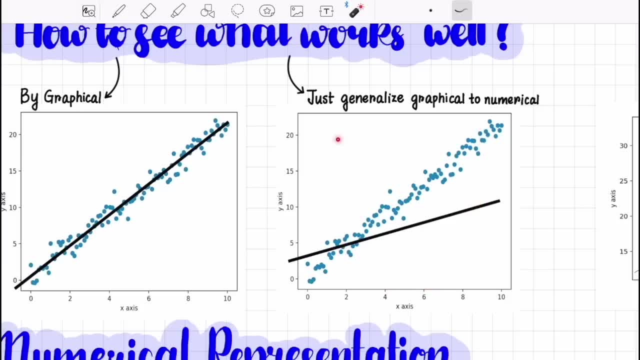 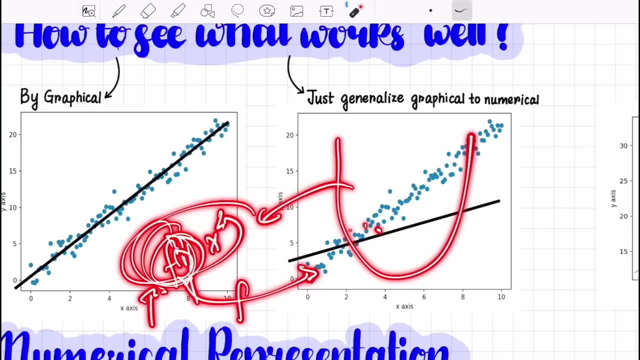 sometimes it's also not possible, right? so in that case, what you will do? you'll utilize this numerical way: x squared f of x is equals to the function numerical. this is the function, this is the numerical way, right? so you'll go with the numerical way. your plugins go one, two, five, nine. 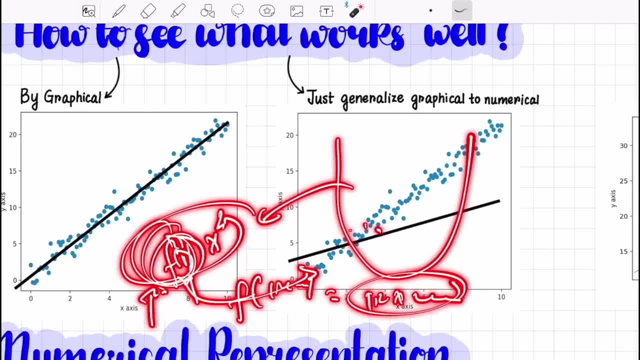 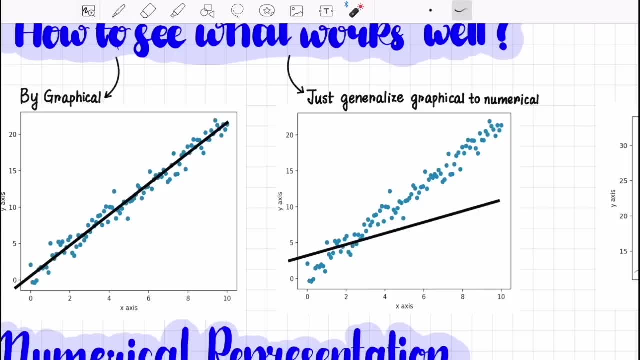 nine. and then you just one two five nine, nine times one two five nine. you just squared this and then you get it exact value. and then you'll get it exact value right. so just in the case of linear regression, okay, we have the graphical uh best fit line to from at our data, but this: 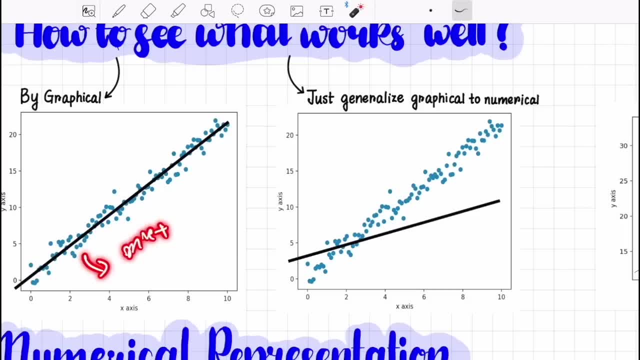 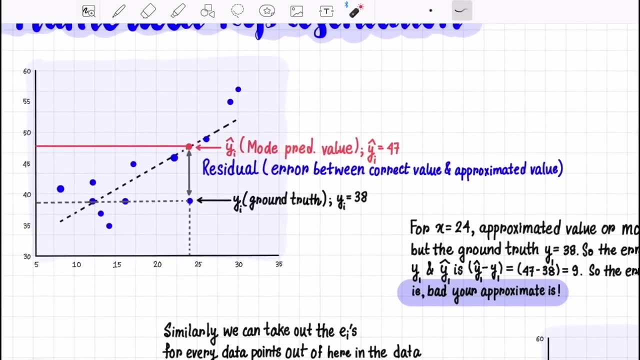 graphical line is represented by a numerical value, which is mx plus b. we need to utilize the numerical as well. i hope that you understood why the importance of numerical is getting given over graphical- graphical for understanding as well. so now let's come to numerical representation that works really really well over here, which, which you're seeing in front of me, is that you 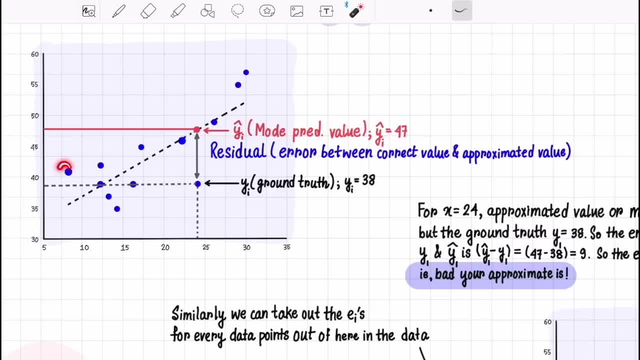 have some data points out here, so assume that this is your one data point, this is another, this is another, this another, this another. so you have some data points out here, some data points out here. right, you have this. blue points are data points in the labeled example, so this data point has. 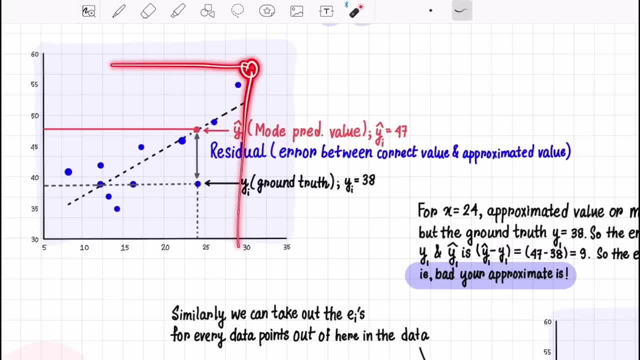 x value this and y value this. this is the point. so it has the label of the value of the data point, and then we have the label of the data point, and then we have the label example y as well, y as well. please note that we're dealing with supervised learning algorithm and we should know. 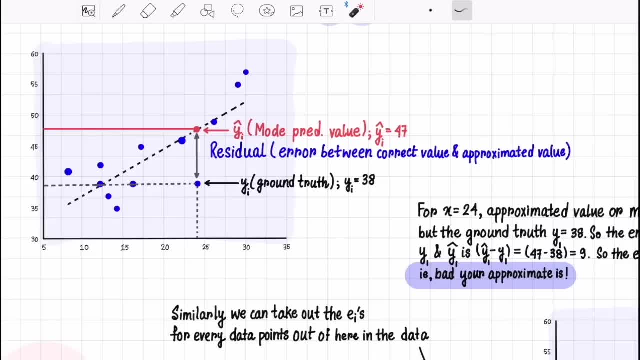 that this is the y, this has y, right, cool, so over here, assume that. assume that your x is equal to 24. okay, your x is equal to 24.. your predicted would be: assume that this is a straight line. you plotted the best fit line. you plotted the best fit line, so this is the best fit line which you have in your 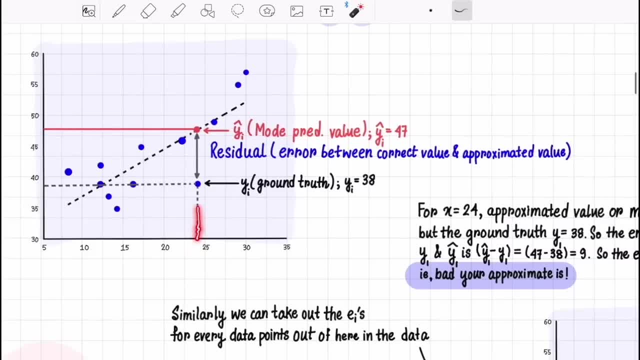 data right and then x is equal to 24.. this x is equal to 24.. if you just see, if you go over, it will. this is actually the. this is actually the ground truth. this is actually your level value. but over here, this is what your model predicted, because model will predict at the point of. 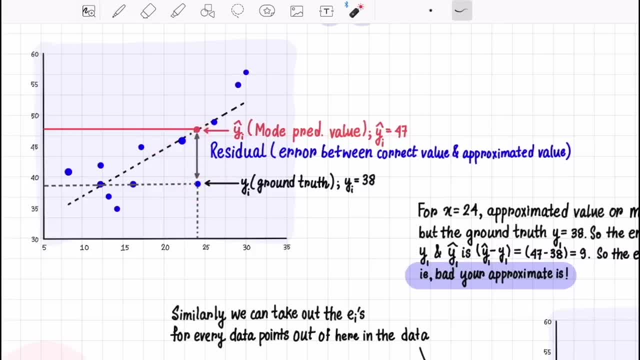 intersection. the point of intersection is your model prediction right. for example, if we, if we say x equals to 20, x equal 20 would be gone, gone, gone, gone, gone. and here it intersects right, because we don't have any example, we don't have any x equals to 20 label in there, or data point. 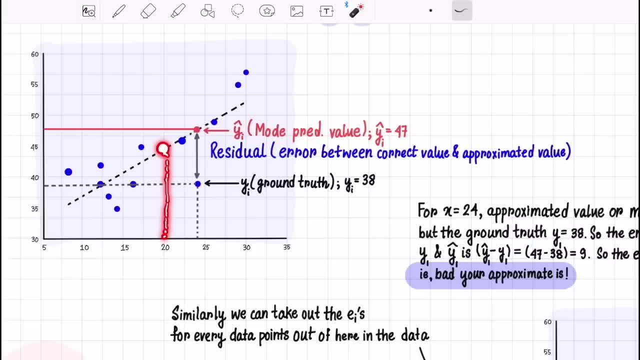 in your data. but over here, the reason why you better know this is because this is where you, so that we can predict like this. and then if we, if we see the y value, we have 45 as the prediction. right, this is how we make sense. but over here for something. but let us assume that this value 24. 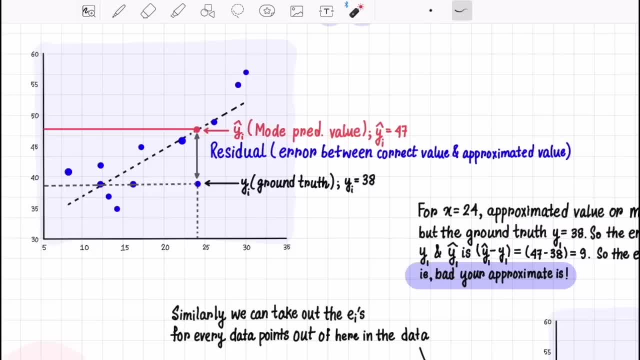 for 24. your true value, your ground truth. ground truth means true value. for example, what is ground truth? you have a scored. you have scored 45 out of 15 years test scores. this is a 45, which is the correct value, which is the truth, but your model predicts that you have scored 57 out of 50. so 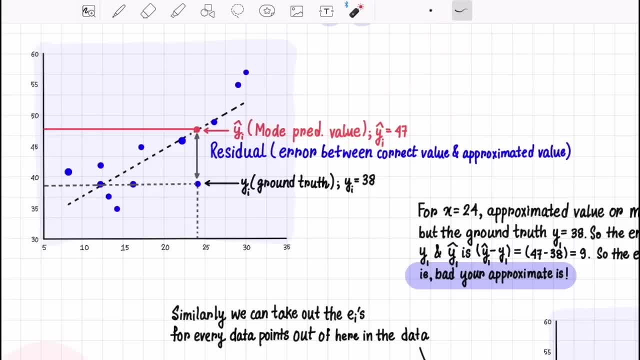 this is a, this is a predicted value or approximated value, and that was your. 45 out of 50 is your ground truth. 45 is a ground truth. so over here as well, for this particular problem, x1 for this particular data point, x equals to 24, x is equals to 24, so x is equals to 20. for x, x is equals to. 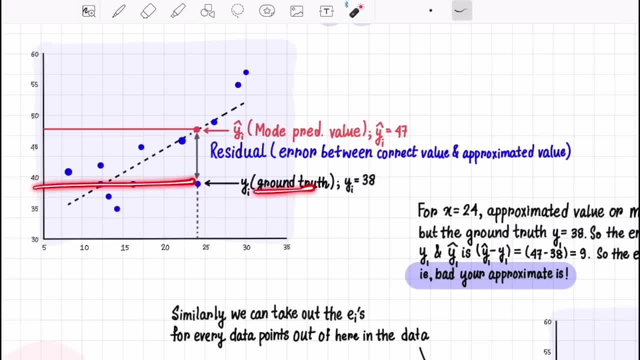 24, your predicted value, your ground truth, is 38. right for the for x equals to 24, but the model prediction lies over here at the point of intersection. so when you just go above, go above, you see the point of an intersection over here and the model. 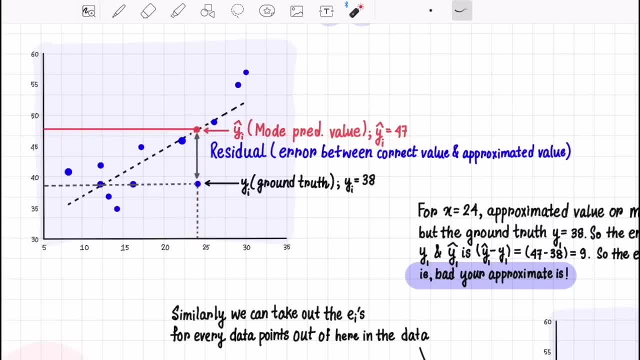 predicted value is nothing but 47, right? so actually the correct value for x is equals to 24, is 38, but your model approximated or predicted 47. so of course there's there's some sort of errors, you know. for example, you might have noticed that when you're actually were that in class 10 dna. 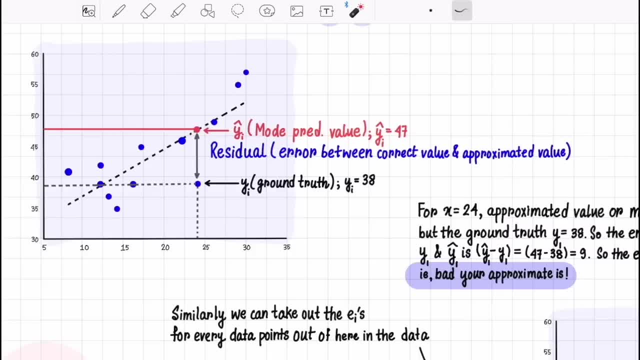 you know when actually dna copying is done? there are variations, right, there's some, there are some errors. so when model approximates, it comes with errors as well, right? so those errors between approximated and correct value: 38 is the correct value and there is, and 37 is the approximated, or 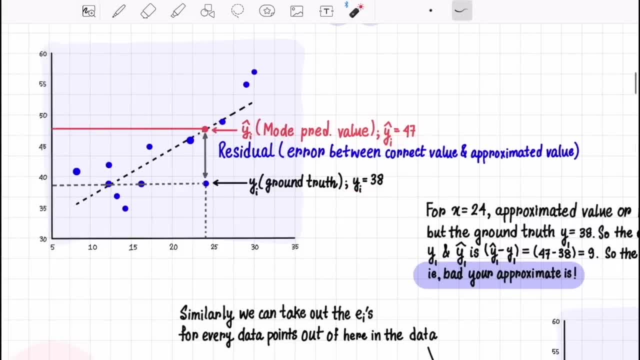 the model predicted value, the model what? what model thinks? what model thinks x equals to 24 and what model? things decided by the straight line, right, uh? so that's why we see that best fit line really works. for best fit line we need to have for a line. we need to have a best fit in the data. then 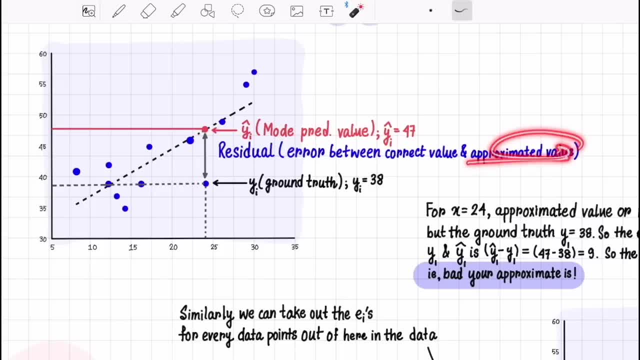 we need to have a very good data point, right, so the difference between the predicted, which is approximated, and the actual value, the correct value, which you call is a ground truth, is called nothing but residual or difference of errors. right, so it's called residual or difference of errors. 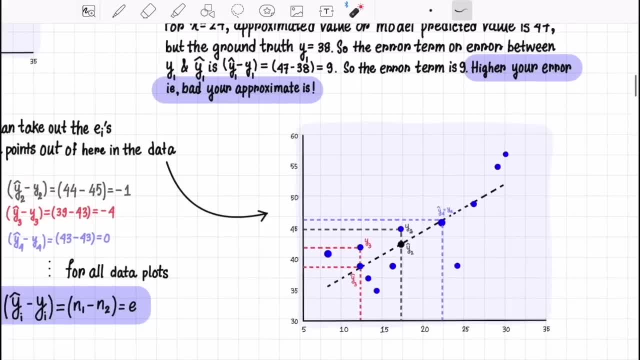 let's take a look at another example by taking a look over here. so assume that, assume that you have this particular data point, you have this particular data point, assume that this one, this one- so over here you have x is equals to maybe 12, and when x is equals to 12, your, your, your. 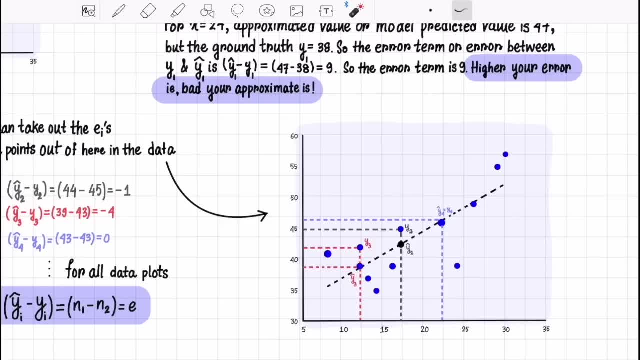 correct value, your correct value as well as your correct value. the blue point is ground truth- as well as your model prediction lie on the same point, which means why I, which is a ground truth, which is down through 4x, equals to 12, and why hat I, which is your, which is your model, predicted? 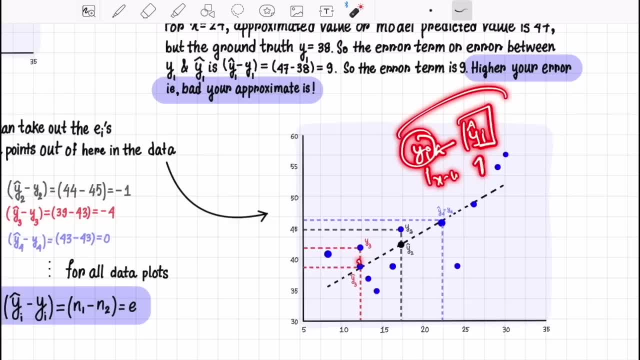 value are on the same point, which means that they both are equal, and assume that the model says that you will have 200 samples, 200 sales. your model predict predicted 200 and actually 200 sales was done, which means that the model was perfectly accurate. your model is. 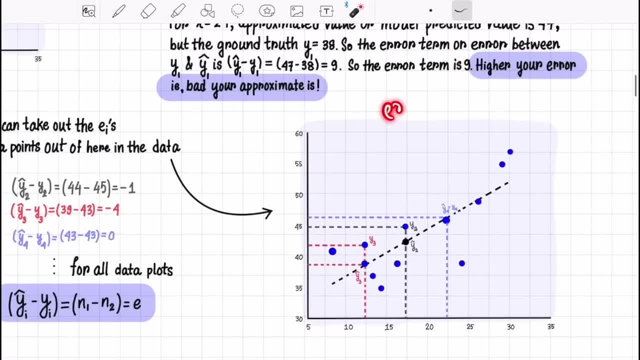 perfectly accurate right. so in this case, the error will be equals to zero. error will be equals to zero, right. so i'll take one example to make you understand. assume that you're working on your, you're working in a date as a data scientist in ice cream shop and over there you want to. 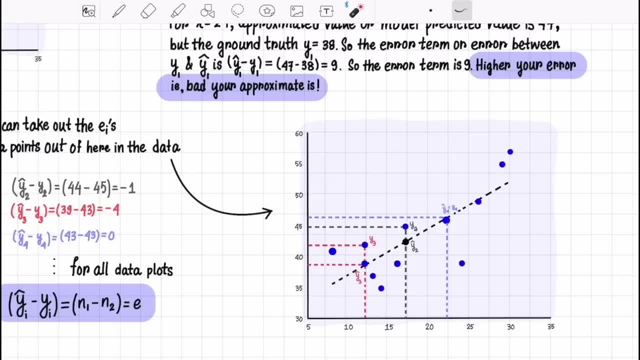 predict. you know, predict based on past data. you want to predict what will be the number of sales in the next day. so your model says that there will be 200 sales next day. right, but actually 200 sales was done, which means they are on the same point. so over here, with x equals to 12, then a y, 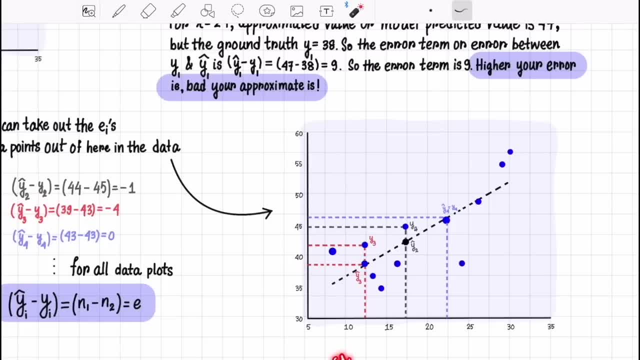 hat is equal to 37, and when y i is with 37 and y hat i also is for 37, which means both are equal and the residual between them is equal to 0.. let's take a look at another example. when your x is equal to 24, when your x is equal to 24, over here your the actual the. 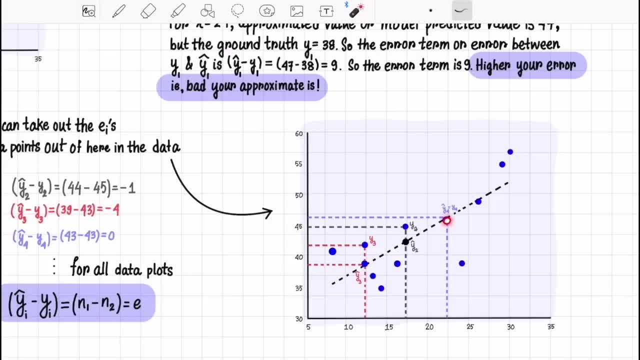 blue point as well as the, as is the predicted value is on the same point, which means that your predicted as well as approximated is r equal. let's take a look at another example. when your x is equals to, let's say, 29, you have, you have this as the predicted value. sorry, this has a correct value. 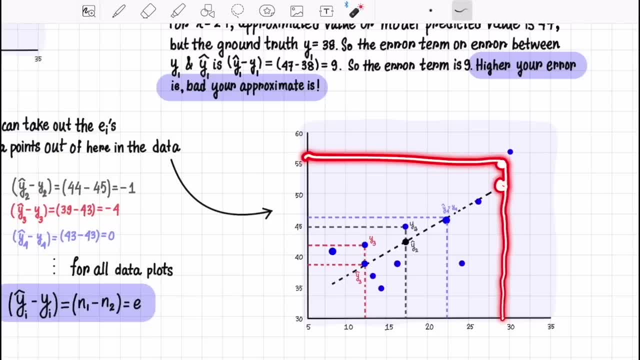 which is a ground truth, and this as your approximated value. this, this has an approximated value, this has a correct value, and so the this, the difference between both of them is a jewel. so your correct value is little bit more than the actual predicted value. so what predicted? 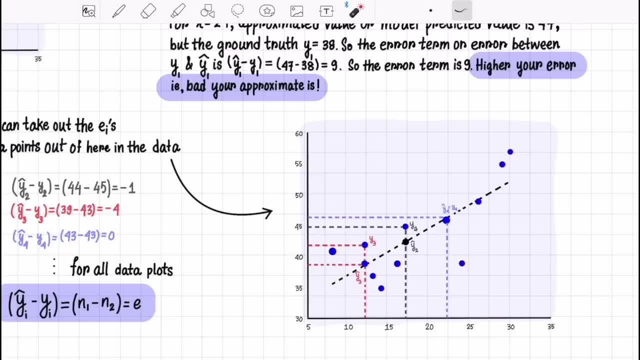 value is nothing but the point of intersection when we draw from the x-axis. i hope you are getting what i'm trying to say. i'm just trying to justify that, that the difference between the ground truth as well as the approximated value. nothing else i'm doing. i'm just trying to justify. 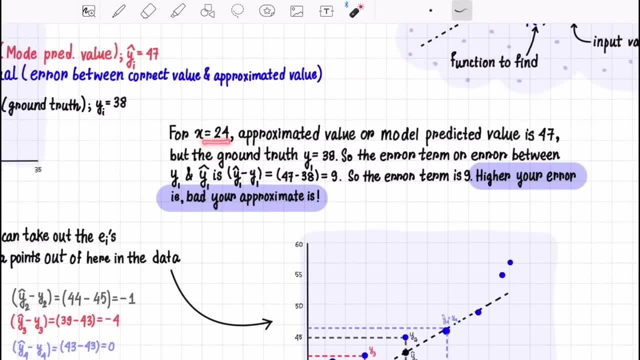 that. okay, let's read something for: x equals to 24. approximated moral predictive is 47. but the ground term on error between y and y hat, which is y hat means which is approximated, and ground truth is nothing but nine. so the error term is nine higher. your error is bad, your approximation is. 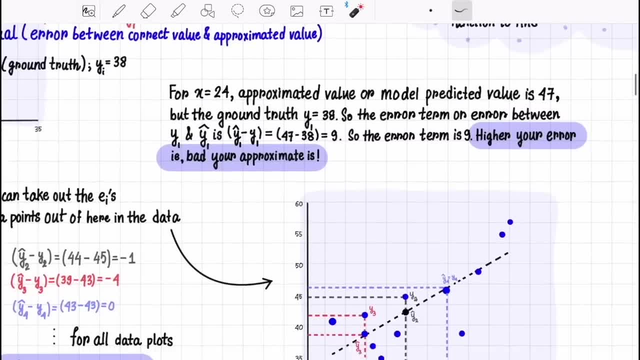 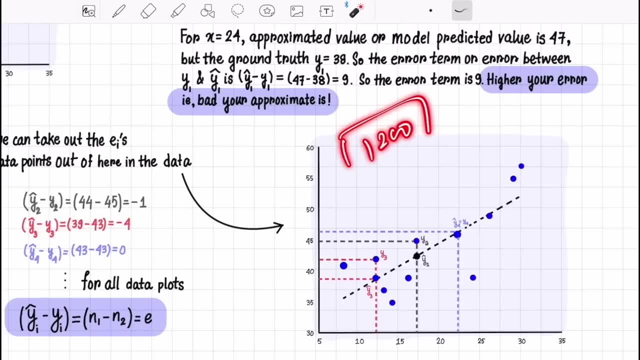 what does this mean? higher error is in bad approximation is, for example, assume that you are an ice cream shop and then you play the end. your model predicted 200 sales. which will? which? which will happen in the next day, says that 200 sales will happen, but actually only 400 sales. 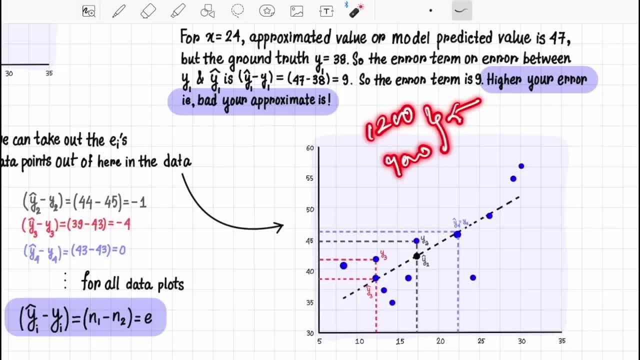 happen. so the difference between- okay, you know, for example, you're giving a maths test, right, you write a very different steps, write a different, different answer, very different answer, rather than the actual answer. so you're absolutely wrong. right, you should be at least close to it when you're giving a science examination. 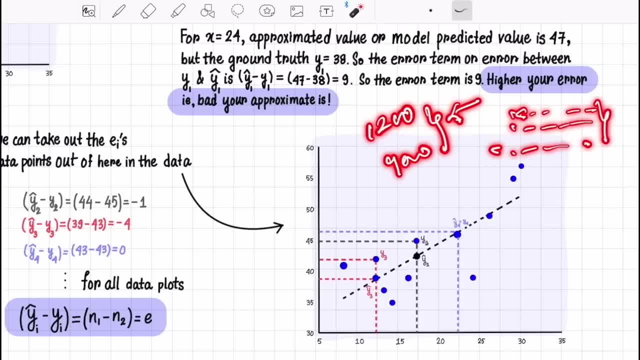 you've written something, you've written some text which is the actual, which is the your answer, which you think is answer, and there is a correct answer in a marking scheme. right, there's a correct answer. so your, your, what you, what your teacher will do. your teacher will match with this if the error. 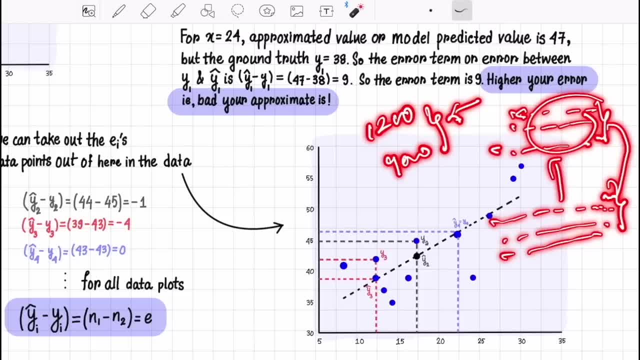 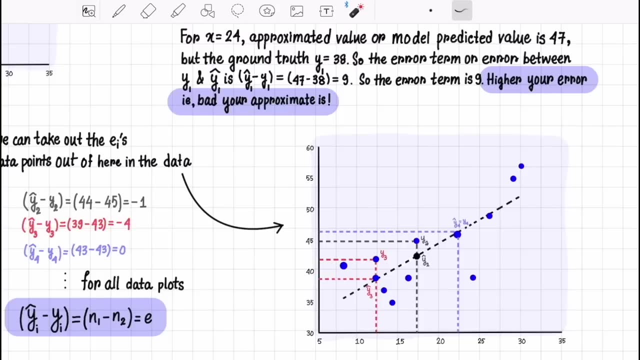 is so much in this is so much the, the difference between so much, then the error is bad. so the the difference between the y, y i and y hat- oh sorry, y hat i and y i, which is the model, which is the actual value, and there's a moral value. if the error between them is high, then bad, your approximation is. 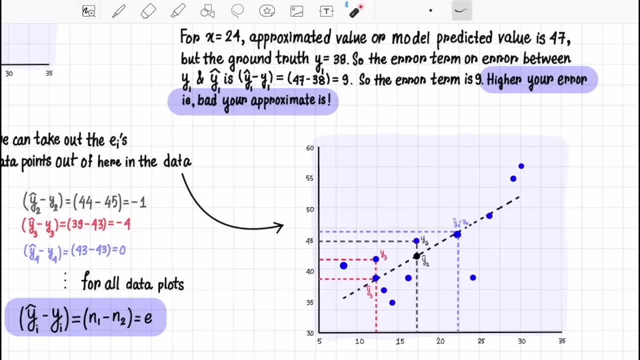 why i have given you a very simple example. one example was ice cream shop, which is 1300 and 400. so error between them is very, very high, right, and that's why we don't. that's why the higher the error will be, that your approximation will be right. so i hope that makes sense about this higher. 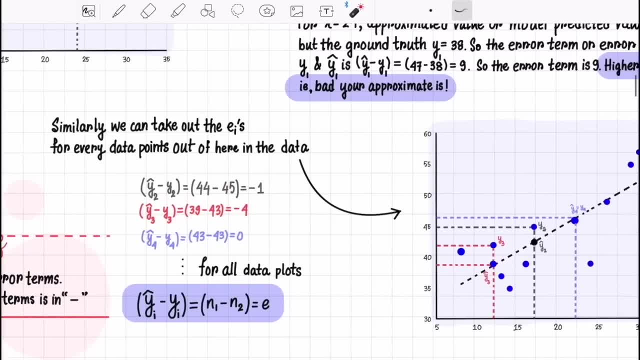 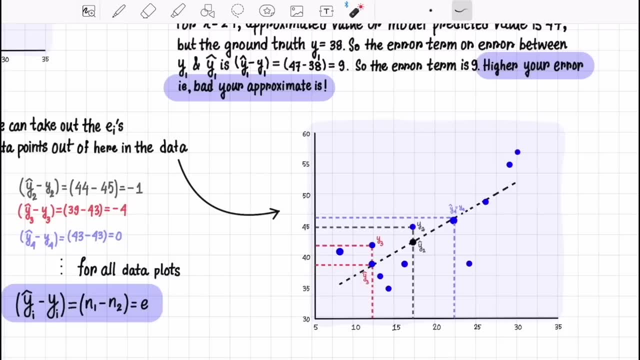 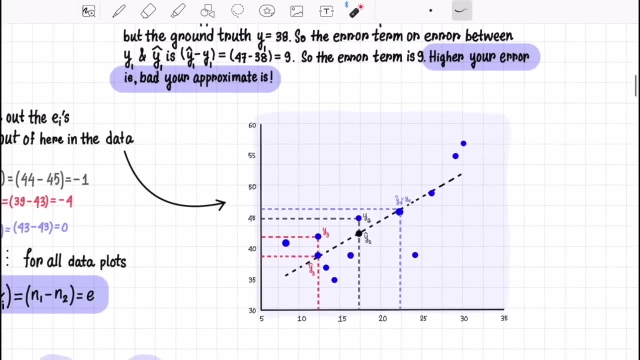 error and that approximation is but what we can do. we can for evaluating how well our line so. but why are we learning all of these things? the reason why we are learning, you know, identify how well this line is for based on numerical representation. by seeing we can tell: okay, this is good, but 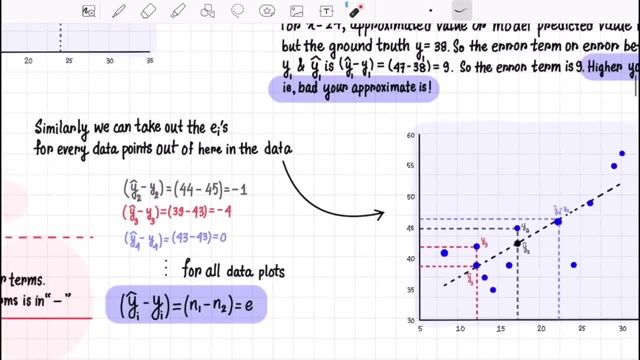 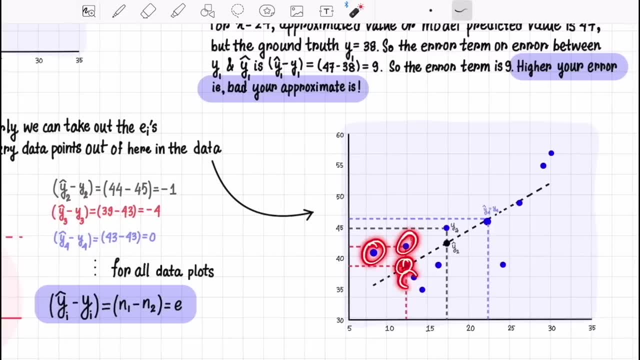 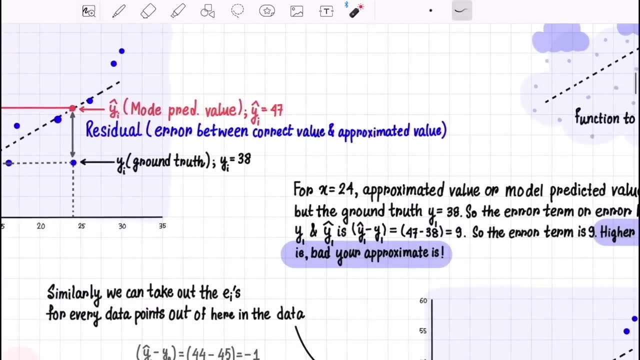 numerically, we should we also be verified, right. so what we do? we do for every sample, which which right. so what you do for all these blue points? you take out the difference of errors for all these data points. for example, for example, y1, which is this: y1, my y hat my one minus y1, which. 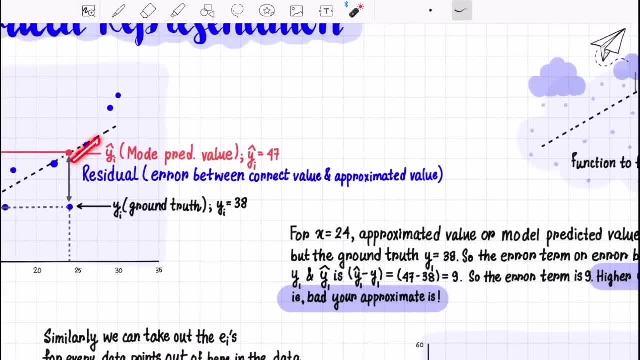 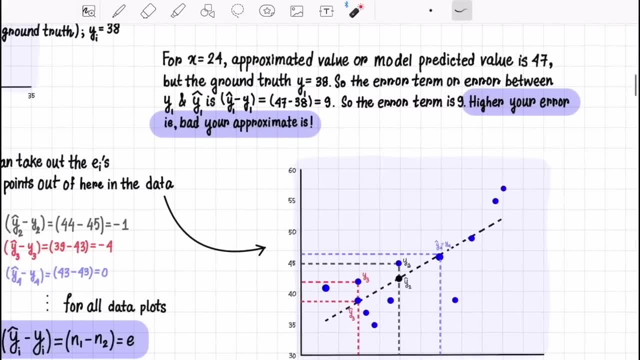 is equals to nine, right, which is equals to nine. so you're taken out for the first, for the first one, and then you do for the second one: y2, y2. so if you see over here, y2, where is y2? yeah, this is y2. 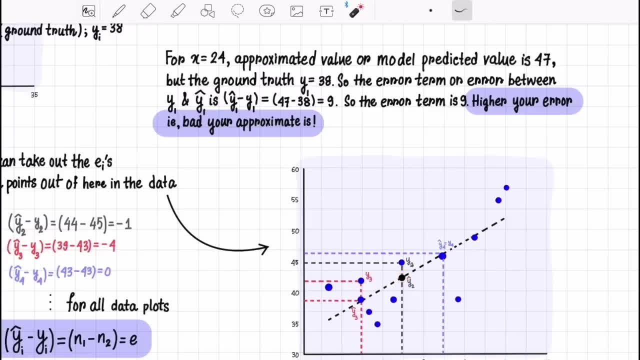 so this is your predicted value. this is your predicted value and this is your ground truth. so the difference between them is 44, which is the predicted value, minus 45. you get minus one right. so this is the. this is the difference between predicted and the actual value. 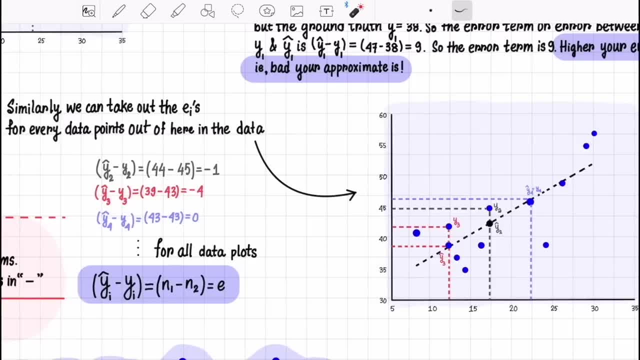 right. and then you have for y3, for y3, your difference of errors, where you have y3, which is the actual value, and the predicted value, which is minus four, and then you have y4 and where the all predicted actual value are on the same point, you have zero, and you do for all the data points. 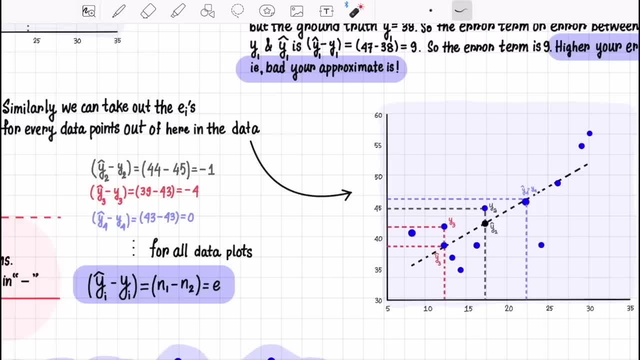 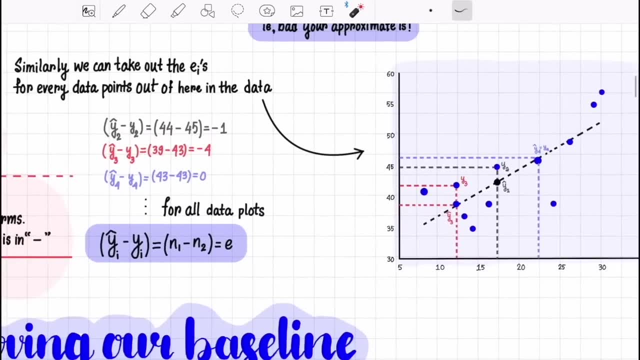 and blue points are nothing but the data points. these blue points are nothing but the data points, right? so you do? for you to calculate the, for example, what you do eventually. so let's take a scenario to make it a little bit more easy to understand, right, when you actually? let us assume. 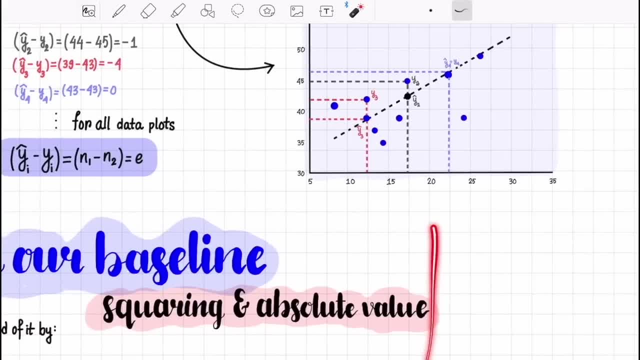 you have 10 problems in an exercise, 10 problems. you have the problems one, two, three, four, five, six, as well as you have the solutions. so what do you do? what do you do? you make your own 10 solutions. you make your own 10 solutions based on the questions, what you have learned. you're going to. 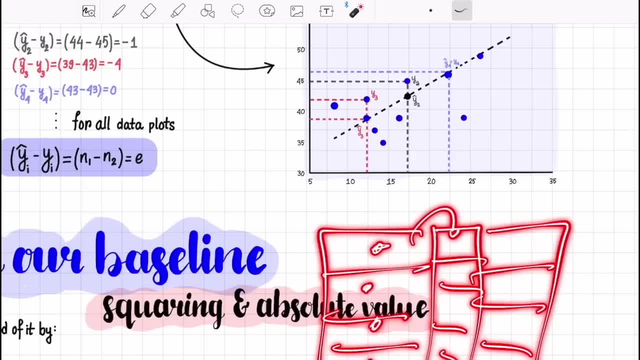 make your own 10 solutions right and these solutions- let us assume that this is your name- is model and you approximated this or predicted these solutions. now, what you do? you match it with this. you match with the correct solutions given in your book, right? so higher the difference is. 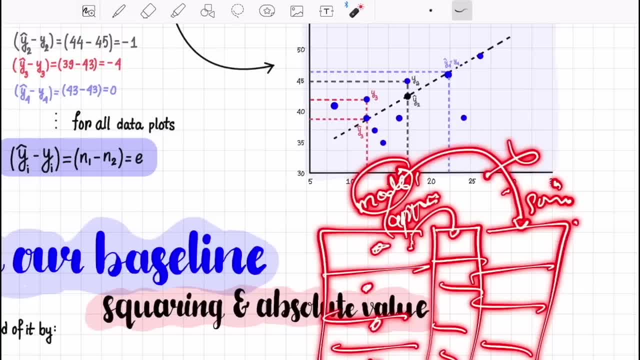 bad. your answer is right. that's what we are doing over here to evaluate how well our paper gone is. we match each and every predicted value with that respective correct value. for example, question before. we match the question before with question number four, the correct answer as well as the. 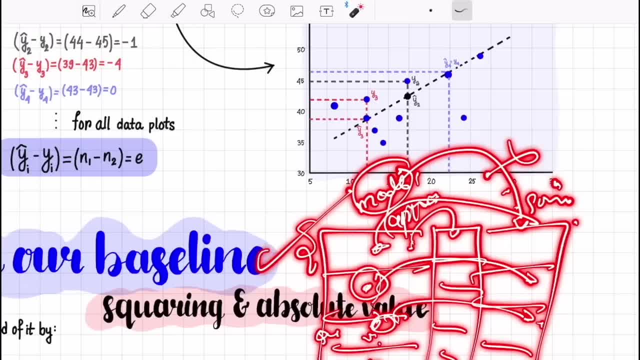 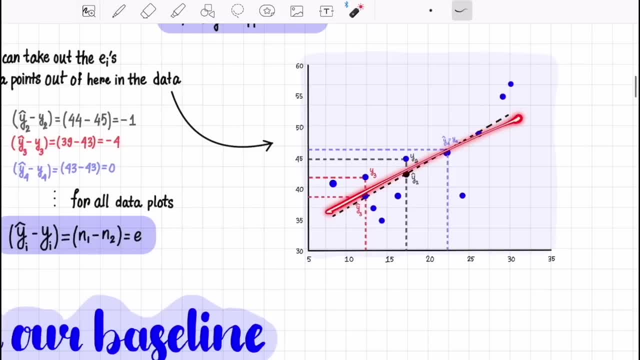 proof. so we just match and check how, where it is, and we give our mark space on that. so just like this, for evaluating how well best deadline our r, we just have the straight line and given that straight line employee, we evaluate more operations minus the correct value for all data points. 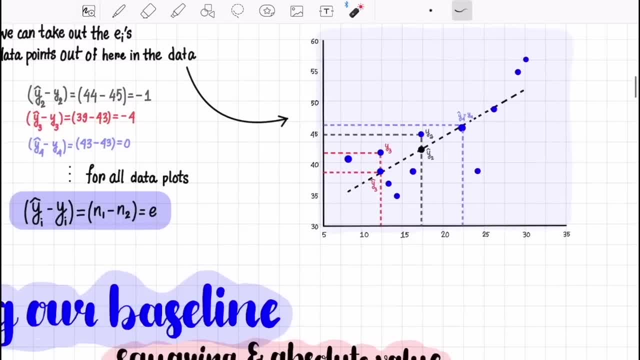 available in your data, right? we do not do for data points, for data points which we don't have any label for that, for example, we cannot do for uh. assume that, uh, we cannot do for let's say two. we cannot do. do, do for let's say two. right, we cannot, because we do. 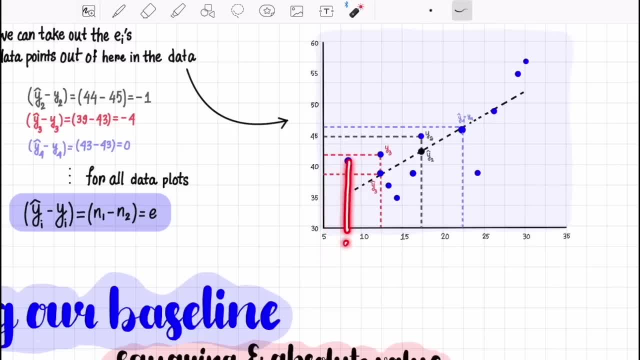 not have data point for that, but we can do for there maybe a seven, right, we can do this because we have the prediction over here and then we have the model practice correct value over here. okay, i hope that makes sense, and then you then. then you take out for and then you have a. 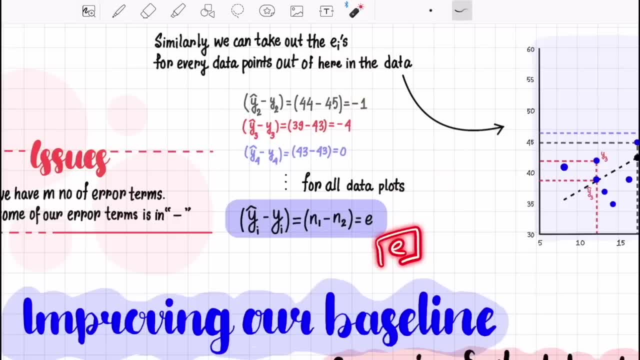 n number of errors, or we can say e number of errors e i's, so you have e number of errors. e will be equals to the number of data points which you have in your data right, so it will have the e number of errors, how n1 minus n2, and the one denotes y hat i and. 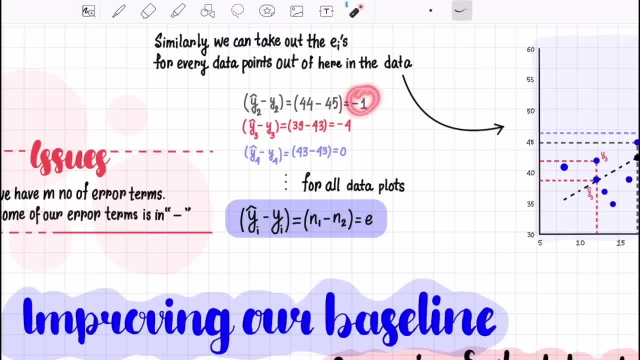 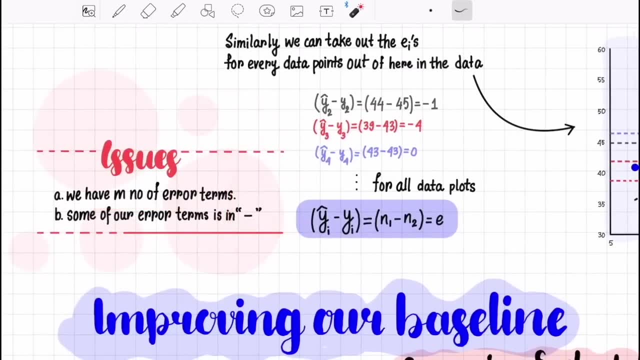 n2 denotes y, i, and then you have negative values as well somewhere. so there are two issues which we come. we have m, we have several number of errors. how can we combine all of this into one single number to better describe our model? and then second one is some of our error terms are negative. 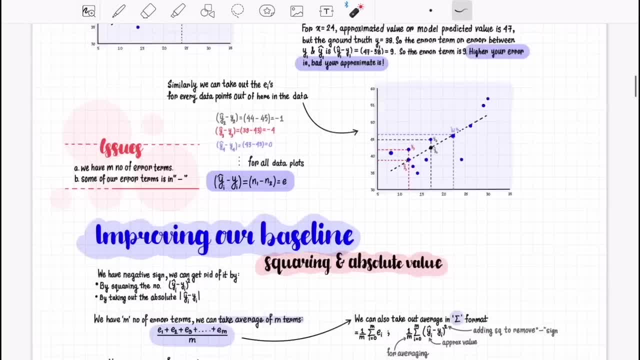 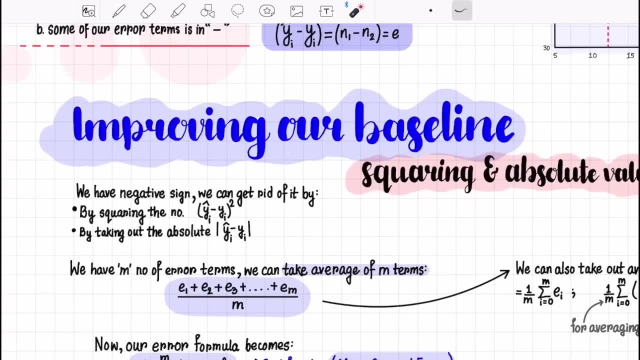 so you can see that they some are negative, right? so what we do to take care of this, so we can solve the problem? we have the negative sign we can get rid of by two processes: by squaring the number or by taking out the absolute of absolute of that, absolute of that number, absolute of that. 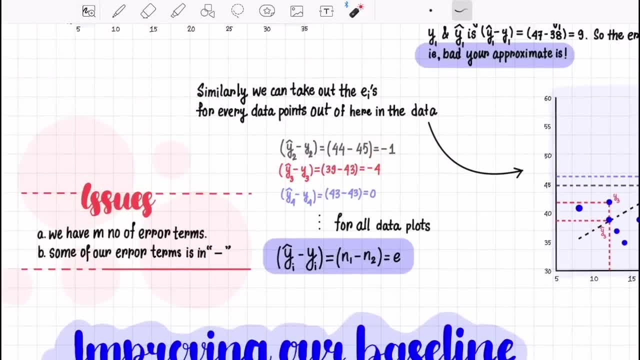 so, for example, you can, we could simply take out the absolute of this. whatever the answer which can take out, the absolute or the square, absolute or the square, so square will just cancel out as well as absolute we will just cancel out. so we can. we have two approaches: either square, the 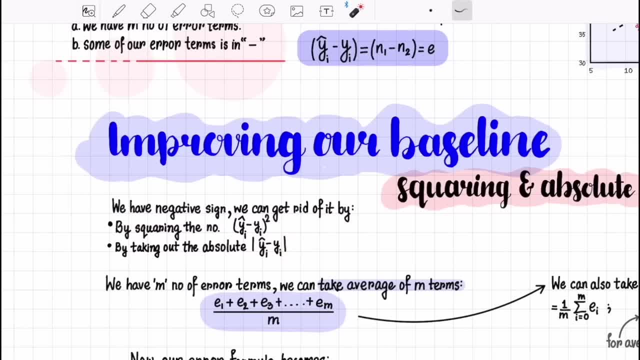 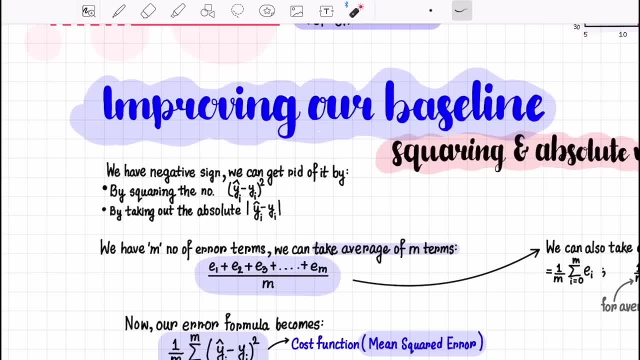 differences or absolute the differences. so what we usually we, what, what we will usually do is we are going to use the square of the number. i'll talk about why we are not using absolute, but there is an app. we also use absolute as well, but i'll tell you later on. we'll just wait for my confirmation for some, for some, maybe next set. 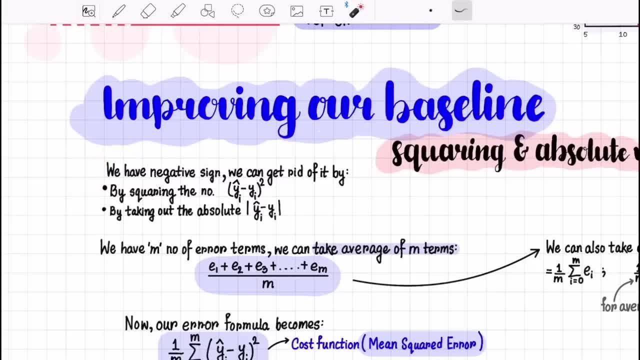 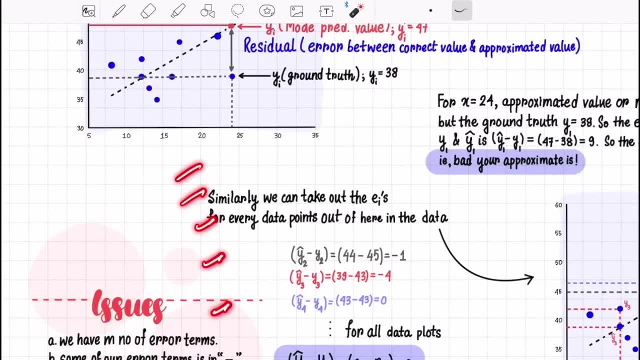 of sections. and then the first problem is all negative. we can either use any any of the approach to fix the negative sign, but but even after fix it we have several number of m number of errors. m. m is nothing but equals to the number of data points and 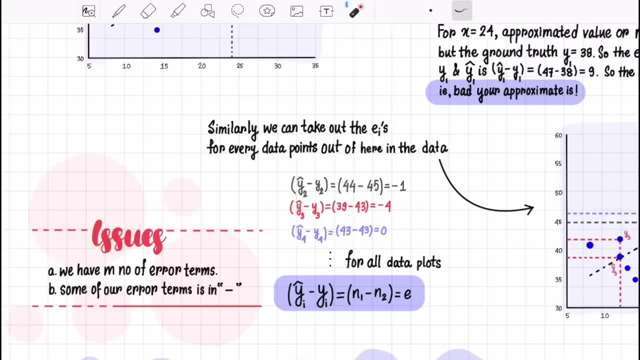 as i said, your error should be equals to number of data points, because the difference is where, because you will be only to your only, ask your model to take out the answer. you do ask your model to take out the answer as uh for the questions which we already have the correct. 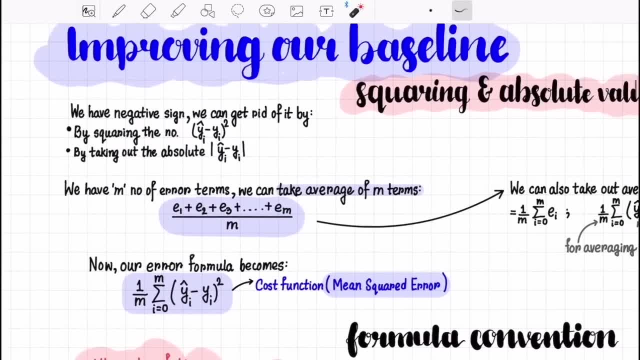 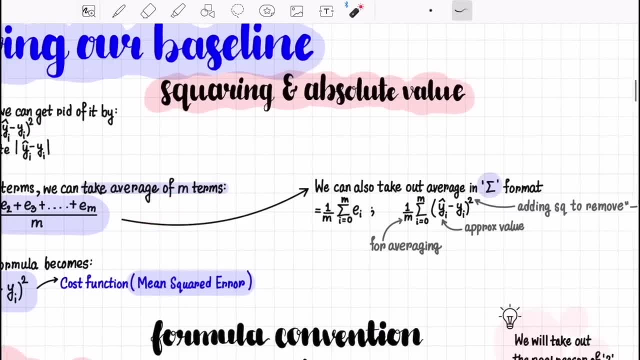 answers so that we can match and test how model performs. so what we can do: we can take out the average of m terms we can have. take out the average of all the errors: e1, e2, all around em. then what we can do, we can put that in a summation format so that we come up with the formula. 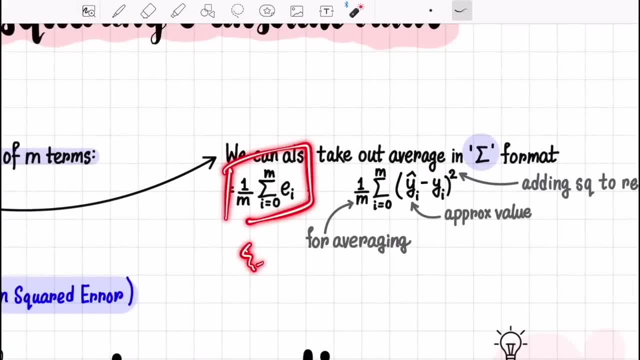 so formula is this: one by m summation i equals to zero all the way out of the m for every e i. so we take out the every a errors. here's the expanded formula: one by m i is equals to zero all the way out of the m. so you do. 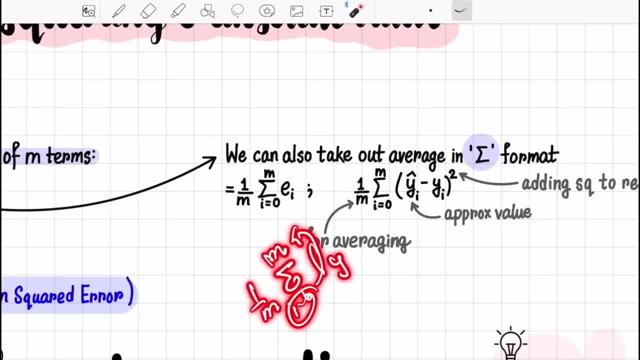 so you go from i equals to all the way out of the m right y i y hat i minus y i squared. so over here you're taking the differences and differences, you're squaring that up and adding the another: i equals to one, then i equals to two and then i equals to three. so please note that you have. 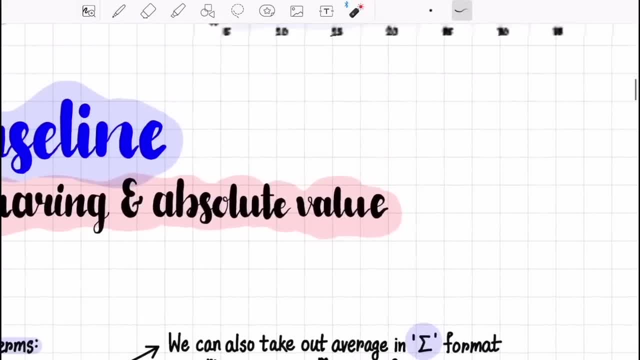 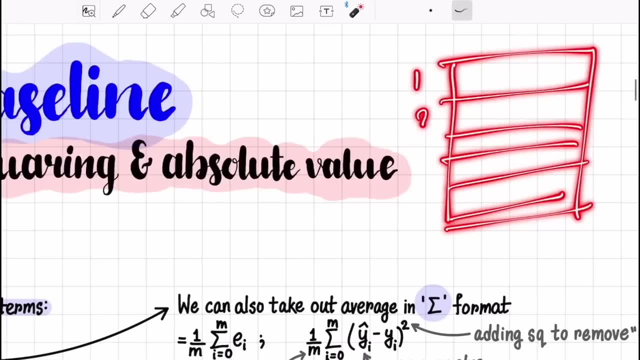 already studied the summation format, right. so how would you get an answer? by doing that you're doing will perform spot. example: assume that you have a date. you have a data point. you have a data point something like this, where you have 1, 2, 3, 4, 5, right, you have 1, 2, 3, 4, 5, so i equals to, 1 is equals to. 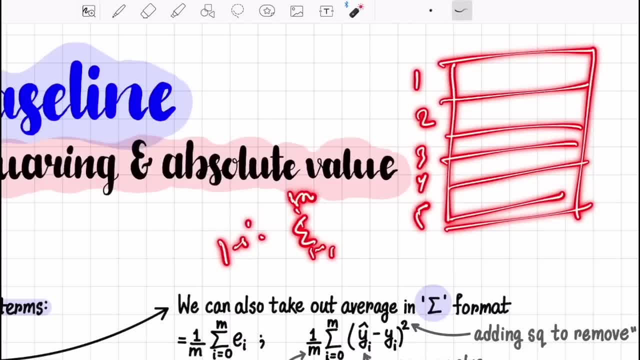 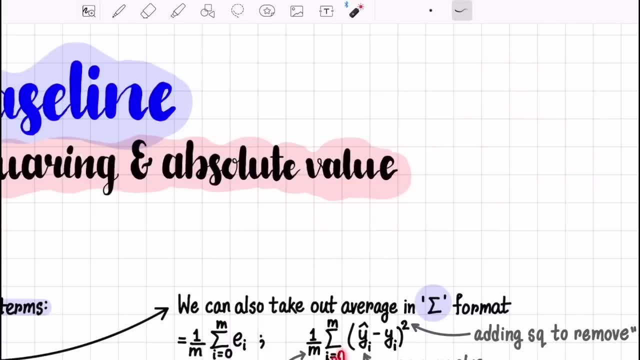 i equals to. i equals to 0. i equals to 1 other other m right. so you have y 1 y 1 minus y. y 1 is quick, right. so you do for: y equals to one, i is equals to 2. i is equals to 3, i is. 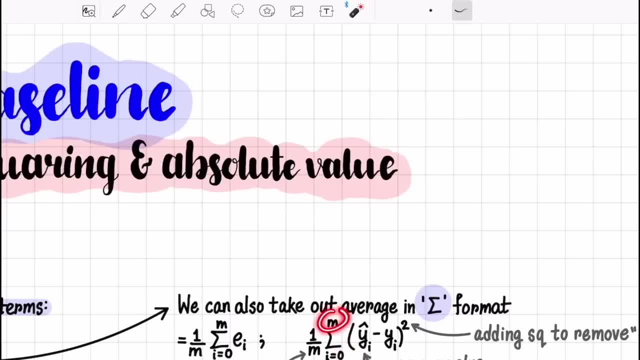 equals to four as well, so five. so you do for every data point, for all the and for all the data points in your data, you add a square to remove the negative sign and then you up, and then you have the approximation value by your sorry at the. 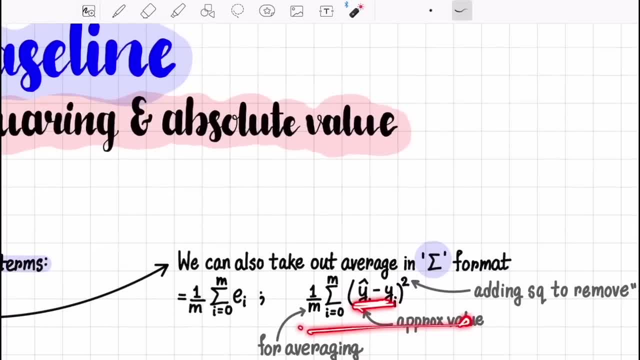 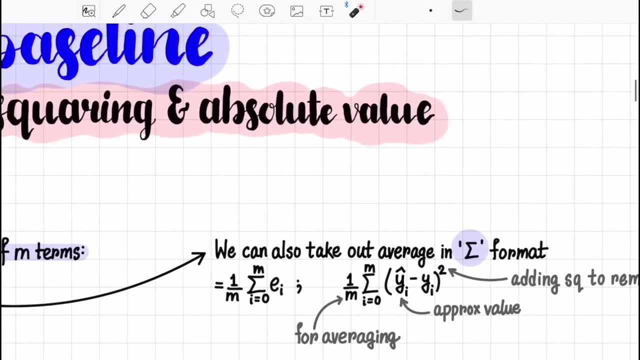 difference of errors. this is called the residuals which you will get, and we divide the of the value by sub, by all the summation, or all the sum, by M. right, I hope that this makes sense. this, this formula makes sense. so this formula should make sense to you. you know, people usually learn these type of formulas, but 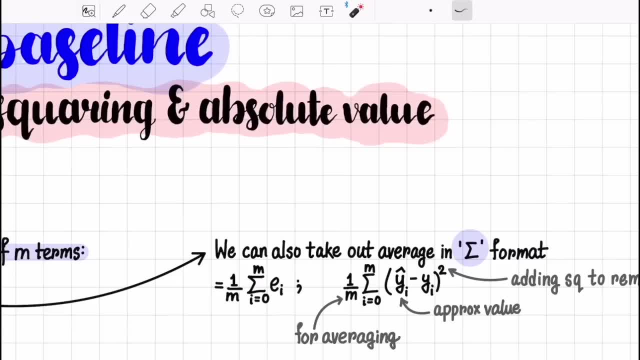 it's eventually what you're doing. you're just taking on the differences of the modulated value and the actual value is querying it up to remove the negative sign, and then you're taking, and then you're taking the average of all of them, you're taking the average of all of them, and this comes up with the name of cost. 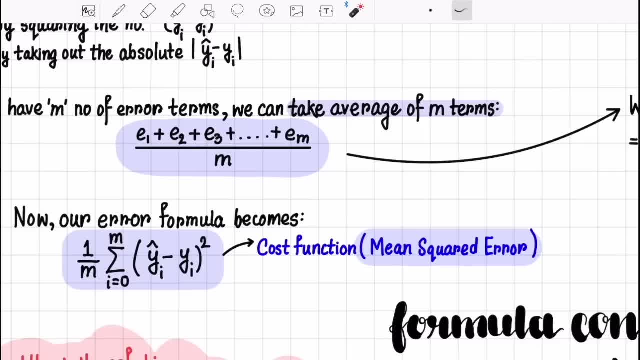 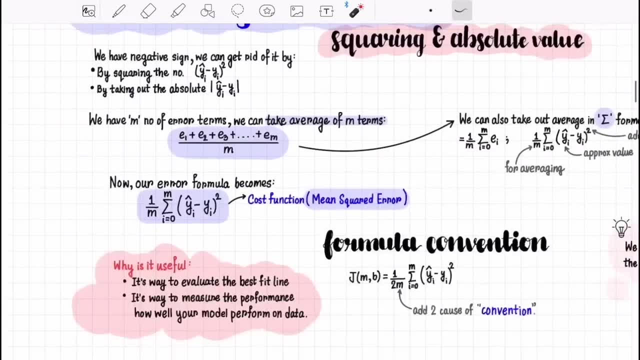 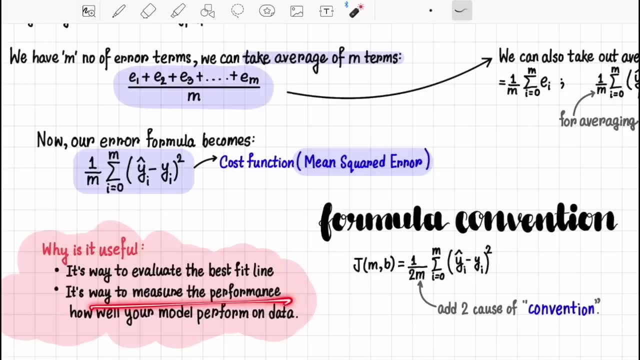 function- or we can say, mean a squared error- for evaluating how well our best fit line is, how well our best fit line you this, we will work on a world example. so why is it useful? first, it is way to evaluate the best fit line. it measures the performance of our model, so higher. 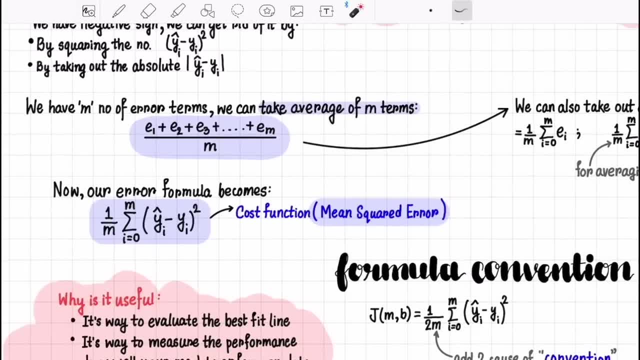 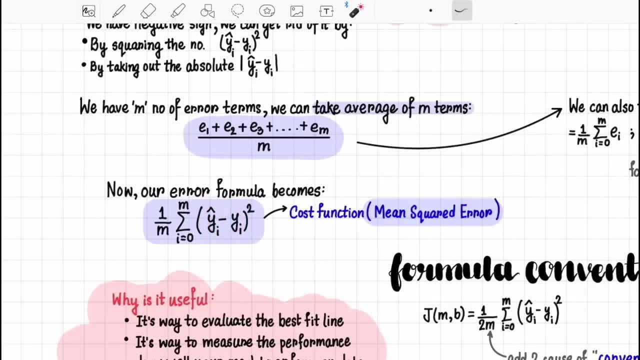 the MSC is bad. your model is why? because higher the MSC will indicate the differences are also higher. as I said that if the differences are had, if the differences are higher, then it's not a good model, right? we had a talk on that, right, so this is one of them. this is one of the key criteria which you should know. 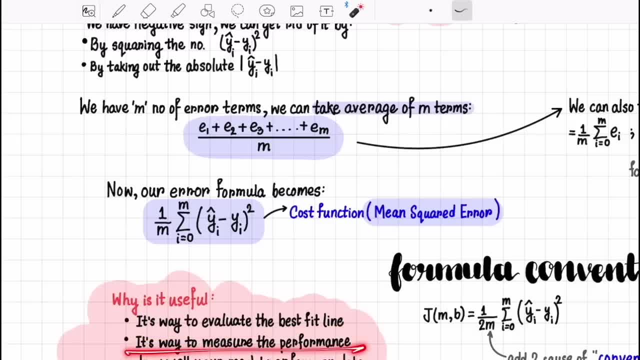 so it is very important that you know what is the best fit line, what is the way to evaluate the best fit line, and this is way to measure the performance. how well, so higher the edit is better. so you have to make sure that your cos function is approximately, or is, or around, 0. so now we come up with: the more 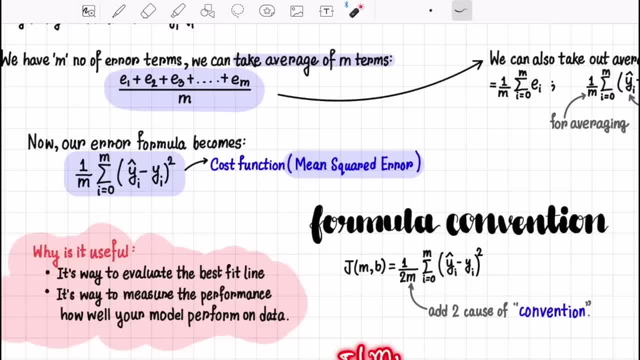 conventional formula, which is J of M and B. so basically, evaluating our M and B is equals to 1 by 2 M I is equal to 0, all the 1 out of the em, why I had minus Y I, which is the difference of errors. we square it up, we take the average, but what is 2 over half? what is 2 over here? what is 2 over here, or whatever thing is, but what is 2 over here? what is 1 over here? what is 2 over here? what is number 10? how do you calculate your cost function? so you can quite simply do it by clicking. 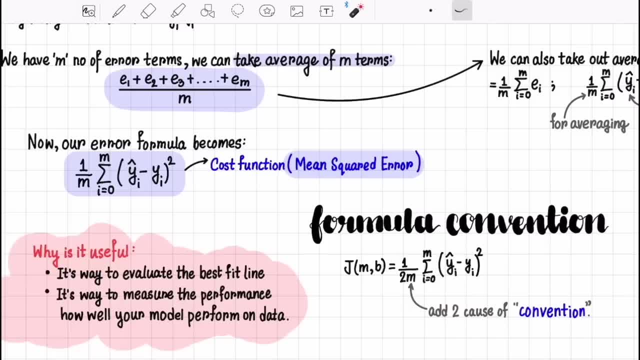 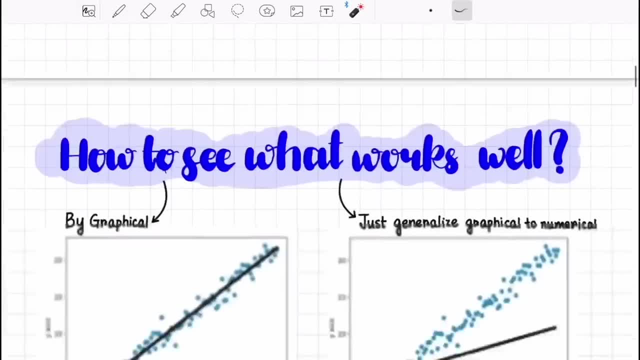 the measure and we know the value of divided by two and you're contributing that difference and what is two over here? it's because of the convention, but usually people say because of convention. but eventually when you learn about this optimization algorithm which i was talking about, which i was talking about this two, really helps in getting it in when you actually do the 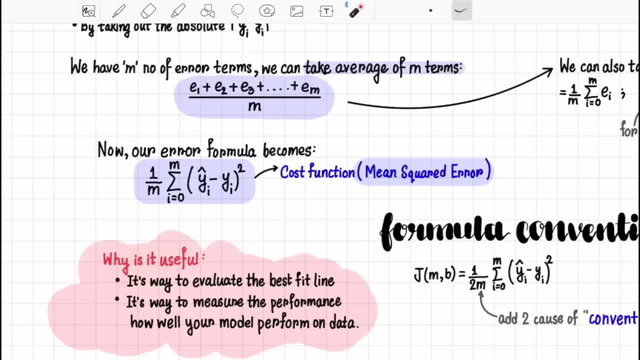 calculation stuff. you know, sometimes researchers find out easy method, too easy to calculations, and these two really helps in that optimization algorithm. we'll see how this helps when you actually derive the formula, but as of now you can just remember it. okay, now to recapitulate what. 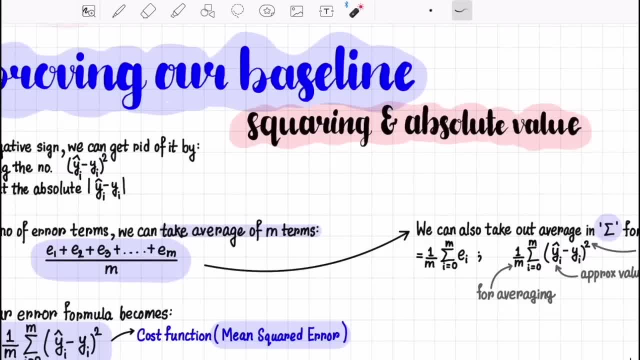 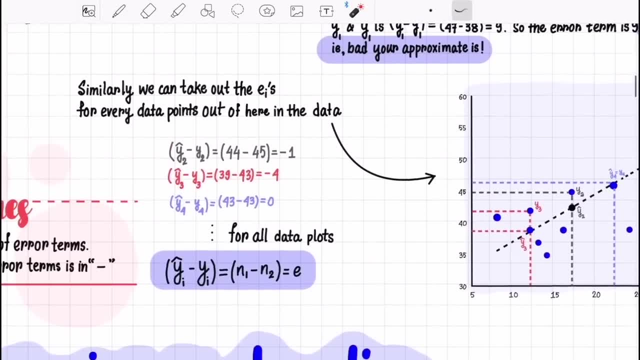 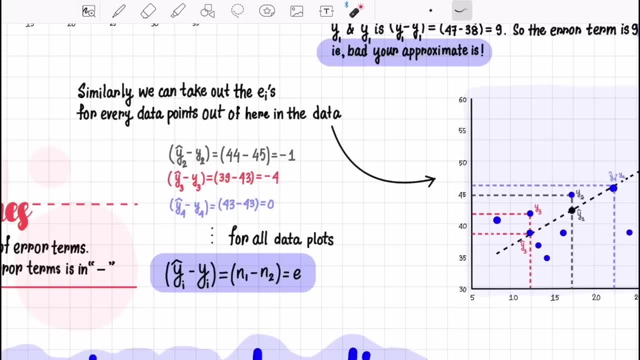 what we have studied. to recapitulate, what we have studied is what we can eventually do is that we can take out the differences between moral predicted and actual value, moral predicted and actual value, and then square it up to get rid of negative sign. and we have several values now. now, 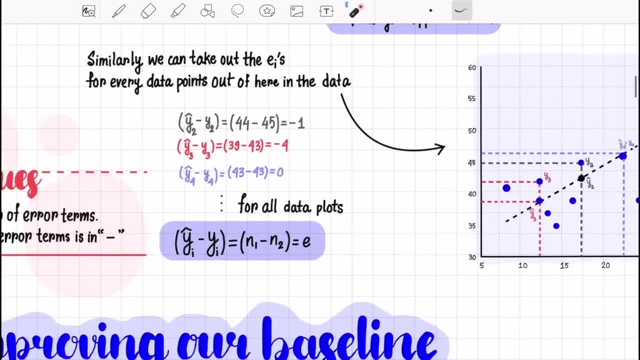 we have to simply divide the term by the number of values in your data set, which is take out the average of them. how you? the error is that your model is because the higher the different it will showcase, the higher the differences is right, but there are two questions now: why we don't use absolute and what? 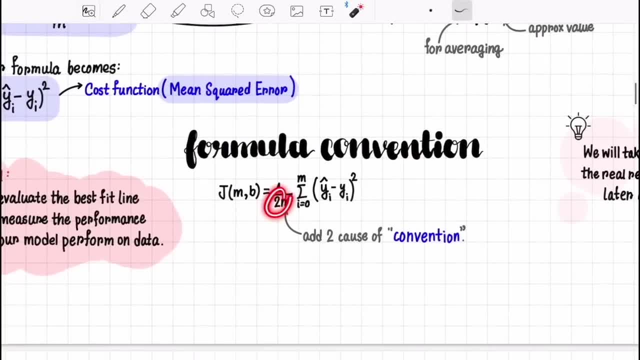 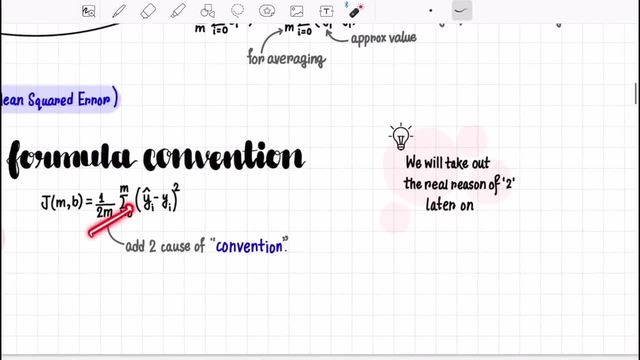 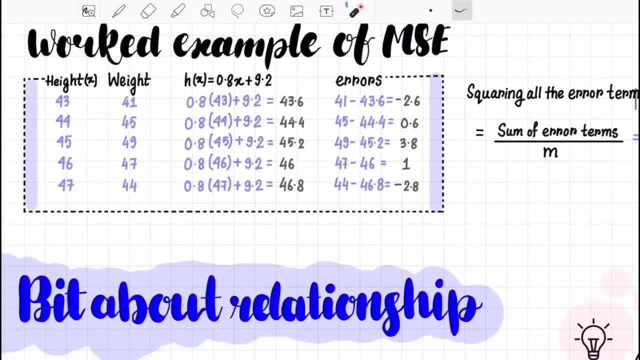 is two. what is the two over here, or what is the use of two over here? and we will talk about the real reason of why we don't take out absolute and why we don't use two over here, right, why? why we are not using in gradient, descent or optimization section. cool, so let's quickly work on a worked. 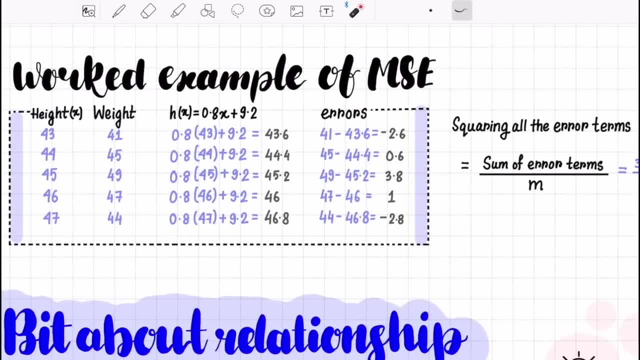 example of mean square error, an error that will make more sense. so you have your height over your, you have a height of a yaw and then you have your weight over here. so basically, given height of a soверson you wanna predicting, establish a function F that takes the height of person and then predicts what's the weight. 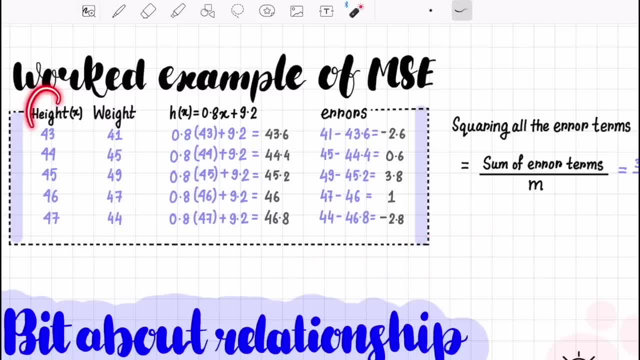 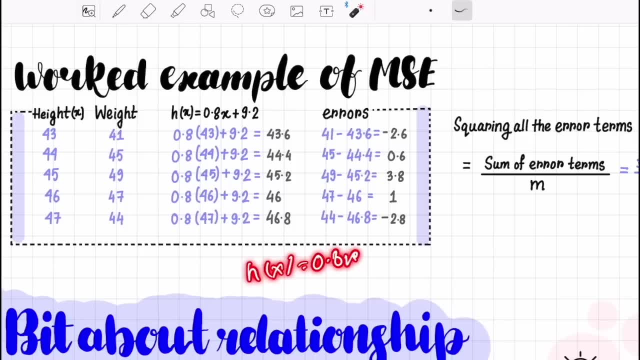 of that person. what's the late of that person? right? so, given this height and and predict the weight, right so now, over here, we came up with this. you came up with 0.8, X, which is M, plus 9.2, which is b. so you came up with these with this formula. so, as i told, as i told that you have your uh, now what? 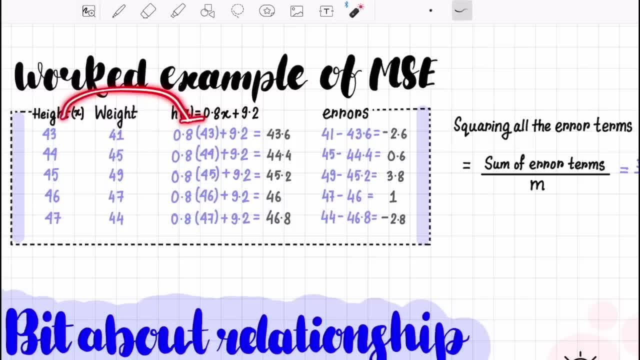 you do, you will put in the values of x for the known value, for the only x's for which you have the known labels, right, or the data points only, and you may figure how we came up. this: 0.8 is 9.2. it's because i just randomly written it, because i want to show you not how we get this, but how we. 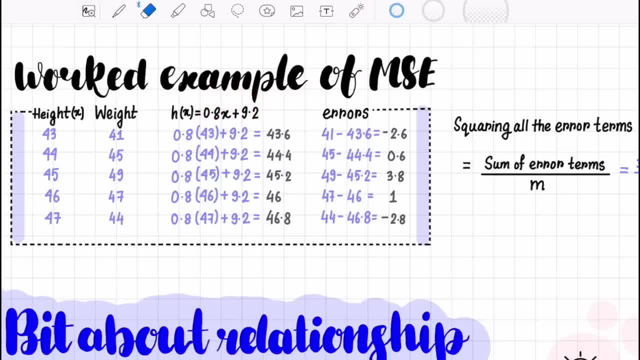 evaluate its performance. okay, so what we do? we have 0.8 here. we have 0, 0, 0.8, which is over here, multiplied by this 43 plus 9.2, which is you just exchange the value of x every time: 43.6, 44.5 for every values, for every x's values. now, now what we do? we compare the correct value. 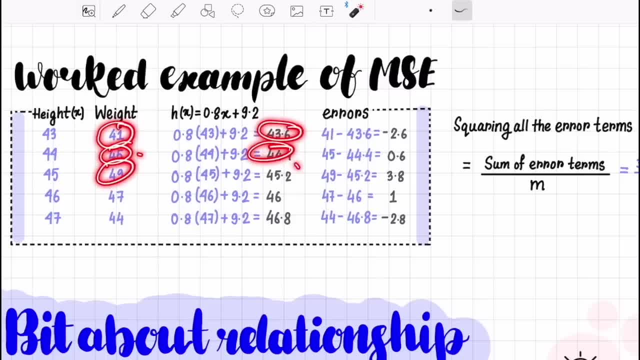 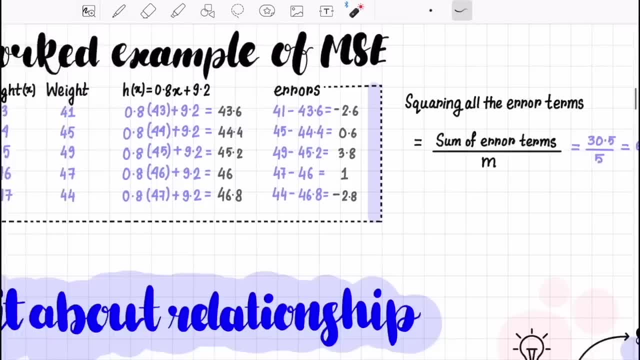 and the model: approximated value, correct value. in the model: approximated value, correct value and model like rocks- correct model, direct model. we take out the differences, errors. okay, we have these errors out here. Now what we do? first of all, we square all the terms and then we sum it all up and then 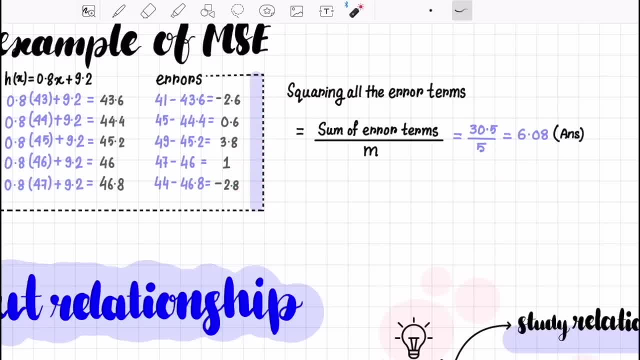 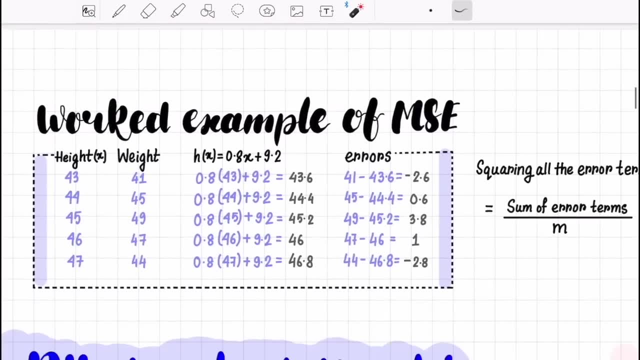 Divide by M, which is 1, 2, 3, 4, 5, 5, and then 6.08 is your square error. So when you apply this formula, you will get that Okay. so, basically, what we are doing over here is Nothing but taking out the answer for every axis and then comparing with actual answer. 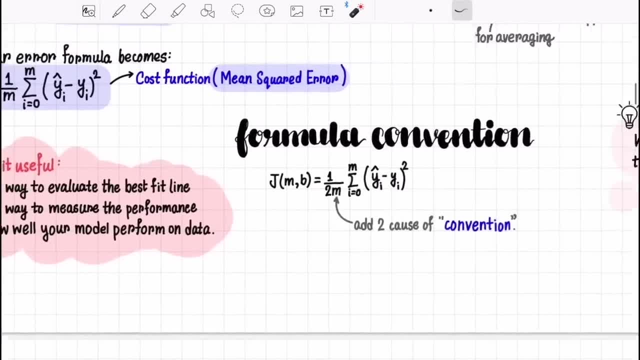 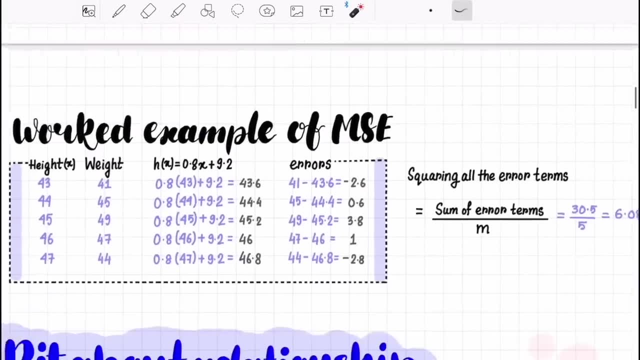 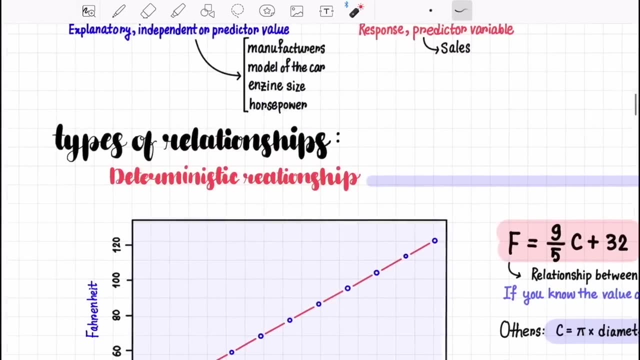 Okay, cool. I hope that this worked. example of MSA really helped and everything is pretty much crystal clear. Let me know if you have any questions in the district community or in the comment box. I try to answer each and every question. Now, what you're eventually gonna do is talk about the relationships. talk about relationships in terms of mathematics. 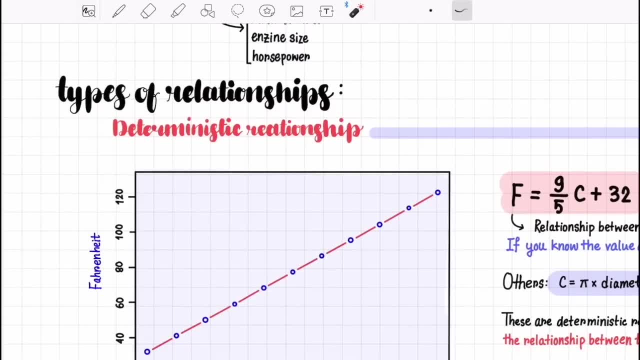 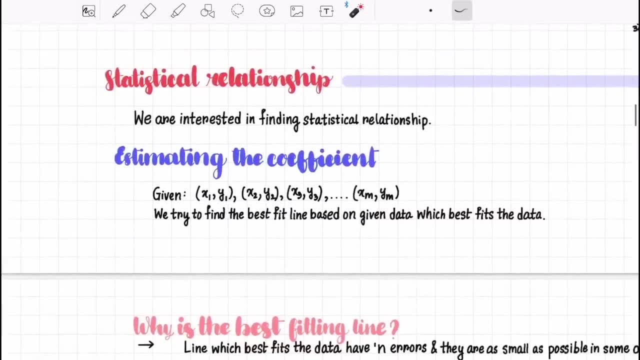 not in terms of life, because I'm pretty much dashed up in relationships and life, So please ignore, I'm not good advisor on relationship in life, But I'm good advisor on how can we establish relationships. Okay, we'll talk about the definition of relationships. 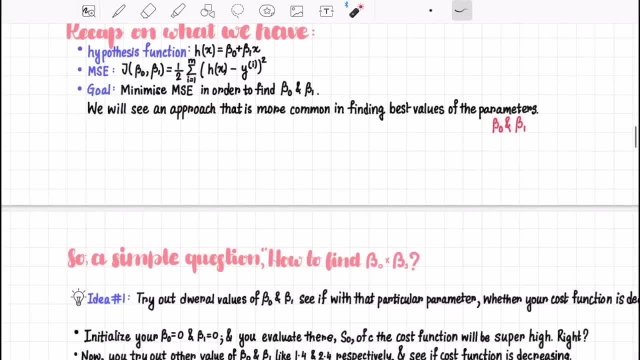 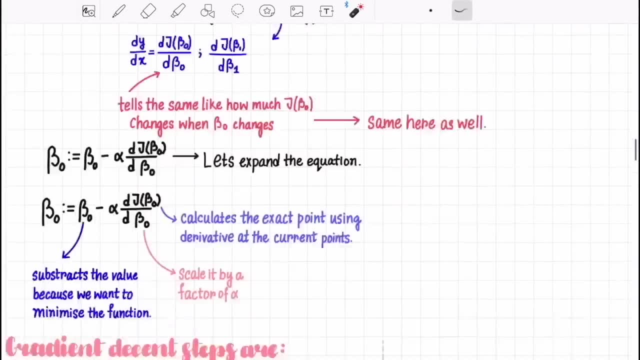 We'll talk about some notational changes, and then we talked about How to find that beta 0 and beta 1, which have been meaning for a long time. We have several ideas, a bill from a plain English language, and then we go to a level. 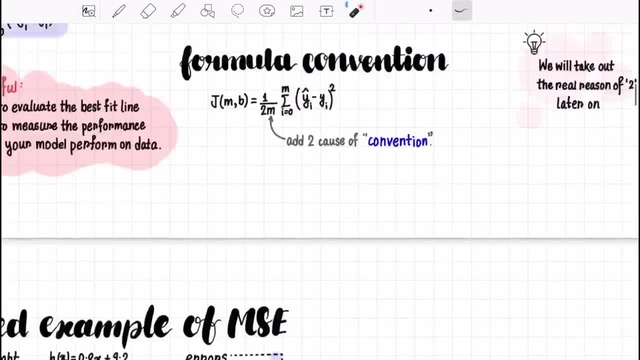 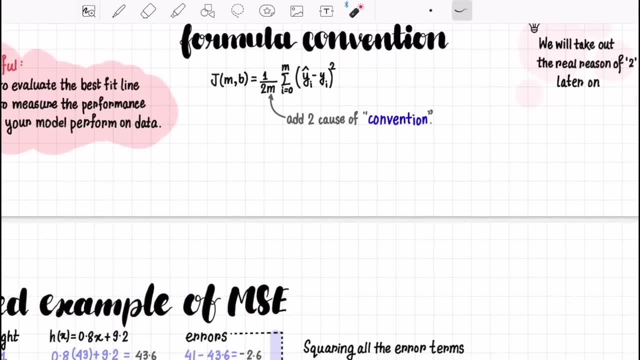 But before, prior to this, I would suggest that you're pretty much comfortable with derivatives, the geometrical understanding of derivatives, as well as pair of. You know formula and rules of derivatives. It will really, really cool. so now what we need to do is get started with a bit of next sections about relationships and 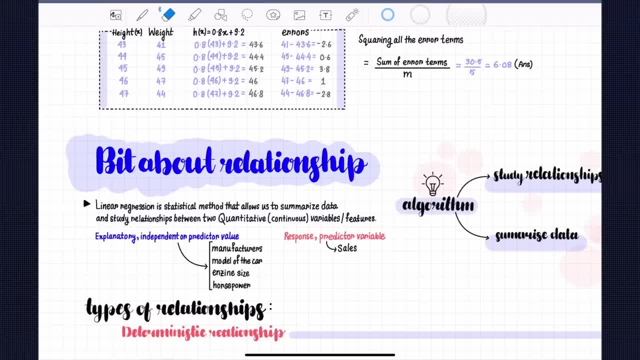 till. then i'll talk later. so now what you're going to do is talk a bit about relationships. relationship is one of the most, uh, important thing to talk about, because usually people tell: you know, establish a relationship, you'll establish a relationship, and blah, blah, blah, and eventually you, you get confused what exactly this term relationships means. so we have even just 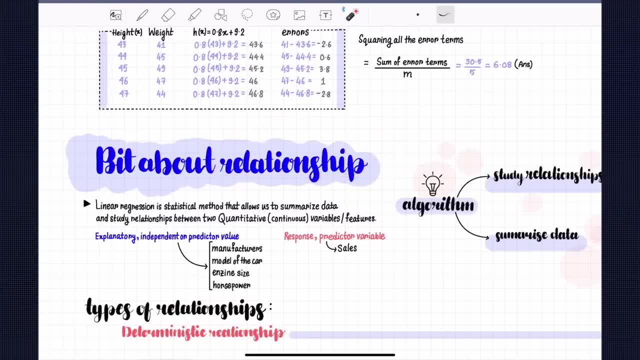 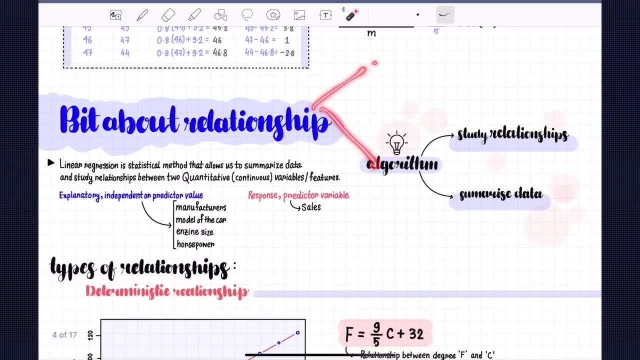 clear about that, what exactly this relationship means, so that it makes much more sense out of it, right? so, over here, what i, what i'll try to do, is tell you what exactly the relationships are, tell you what exactly relationships are, and then i'll tell about two types of relationships. 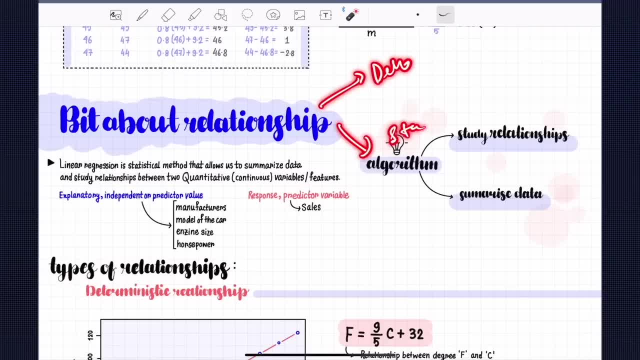 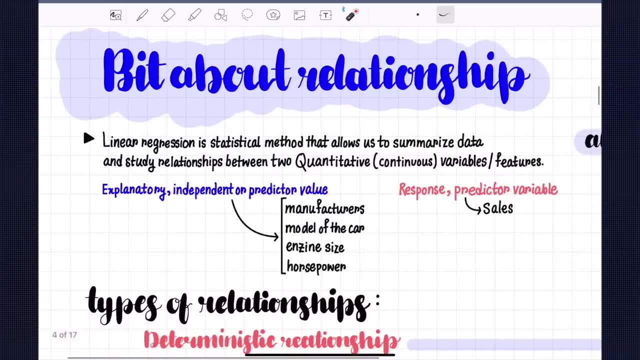 which is the terministic relationship, and second is a statistical relationship, and why we're going to focus only on statistical relationship over the course. right, so let's talk about what exactly. the current thing which is studying right now, the current thing which is starting right now, is a linear regression, which is a statistical method. 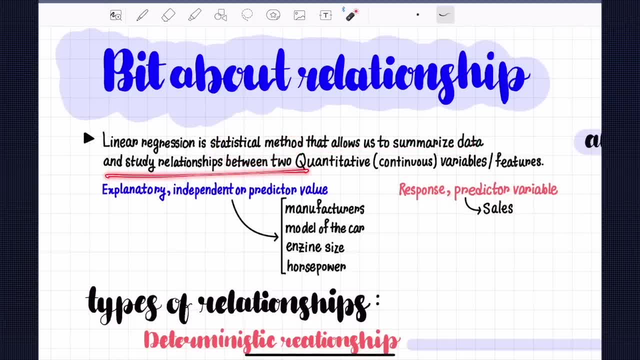 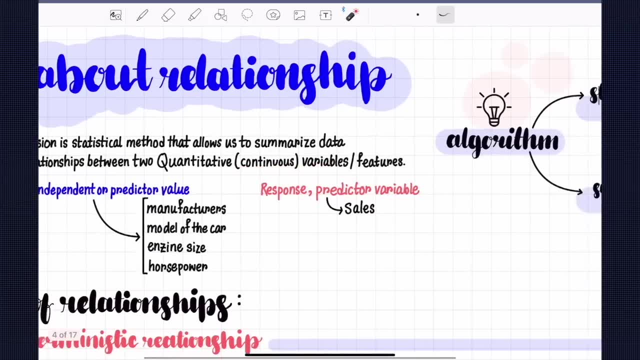 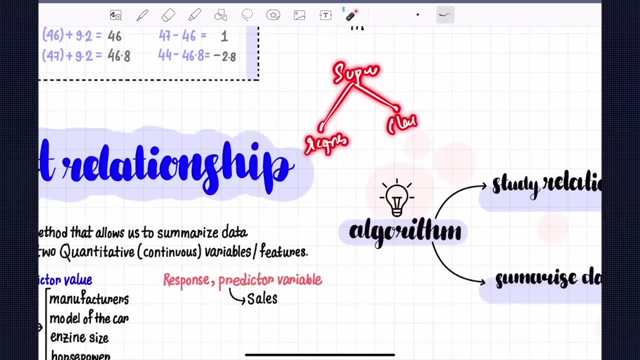 that allows us to summarize data and study relationships between two quantitative uh, which is the quantitative variables, which is that type of continuous variables. so we have seen that supervised learning. supervised learning has two types of problems. one is regression problems and another one is classification problem. so we have two types of 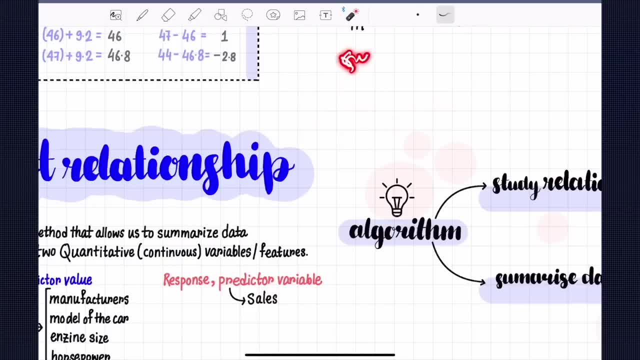 problem: classification and regression problem. in terms of regression problem, how can we identify a problem? is regression problem if the target variable or the thing which you want to predict, the thing which you want to predict, the thing which you want to predict, is continuous, continuous data? or is continuous data or some sort of a? no, a non-countable or non-finite, or something which is 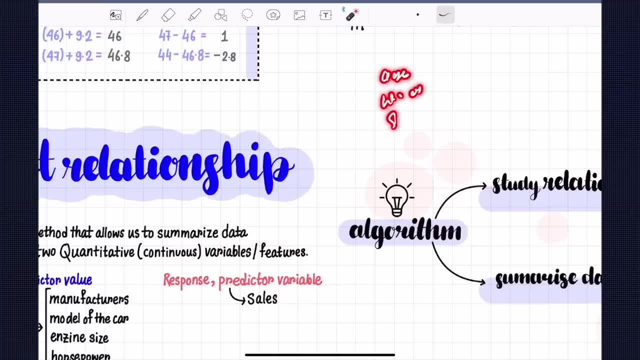 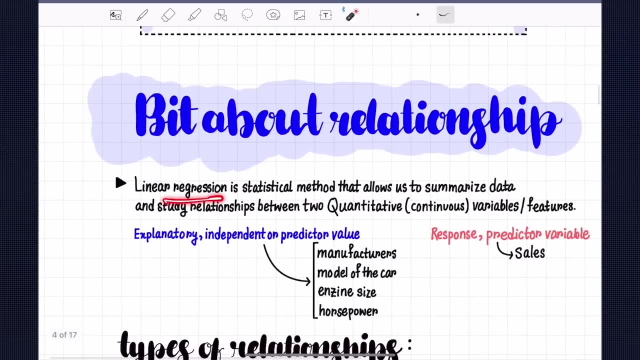 continuous, like the age of a person, the height of person, the salary of a person. they are the, their example for continuous value. so if the target variable is of, is, is, is of, is of continuous data, then then the, then it, then we know, then it's known as the regression problems, then it's known as the 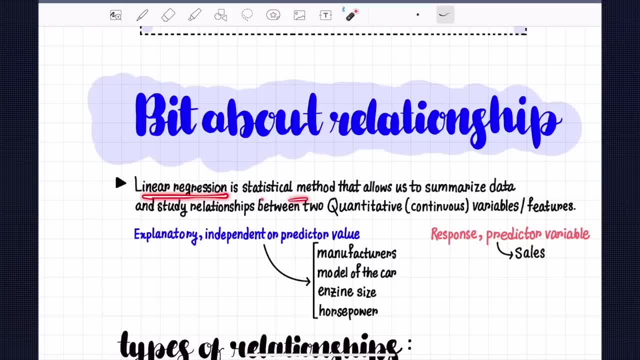 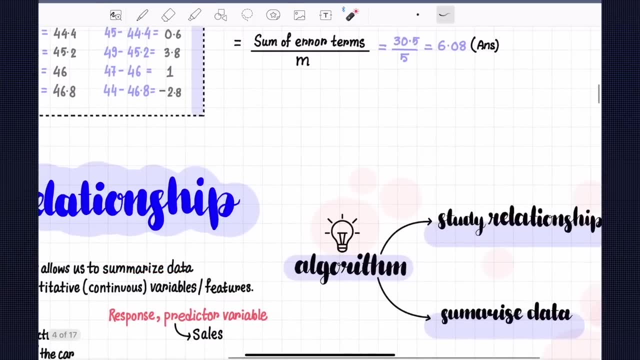 right, cool. so linear regression is a statistical method. we'll talk about what exactly this statistical method means. that helps to summarize data and study relationship between two variables. now you you may ask: hey, ayush, what do you mean by study relationships and summarize data? so you'll study, you'll. you'll understand more practically later on, but assume that you have. 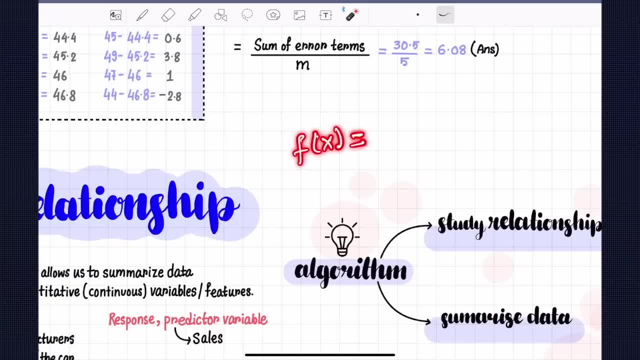 a function, your function f of x, your function f of x, that tells you, that tells you about the the price of a house in a certain area, given its size, right. so you're given the size of the house, so you're given the size of the house, it will make you, it will make you it, it will predict. 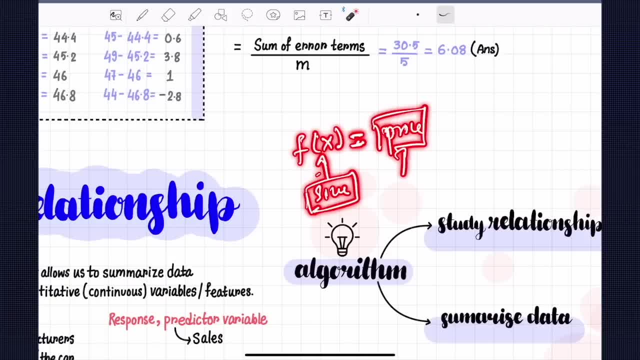 it will predict the price of the house. this is the output variable which which you're gonna get right. so, given the size you know, predict the price of the house, right? so what does this? f tells? f will tell you. f will establish the relationship, as f will tell you about what is the relationship. 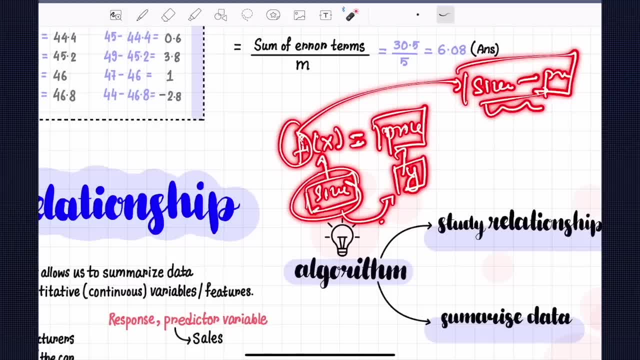 between these two, right, it will tell you what is the relationship between these two right, that's, that's the first thing which the linear regression tries to answer, this. and second, it will summarize by how, if we increase size by this much, by some unit, then what will be increase in price. so, if we make price, if, if, if we 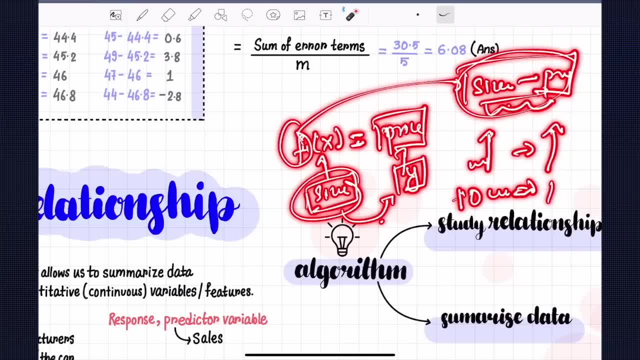 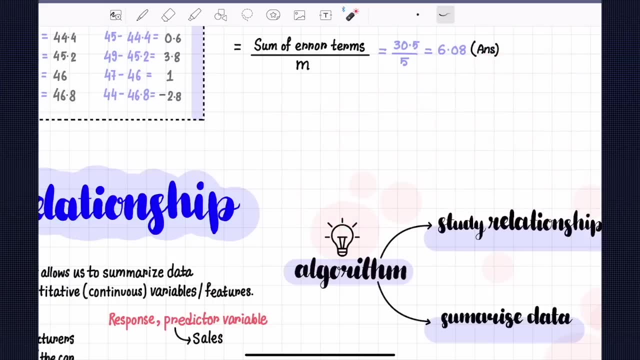 increase size by 10 units, what will be the increase in price? right, that's what it tells it's it tells you about the relationship it tells you about if one increases, what will happen to another? right, we'll study about interpreting the coefficients- uh, soon, interpreting the coefficient soon. but 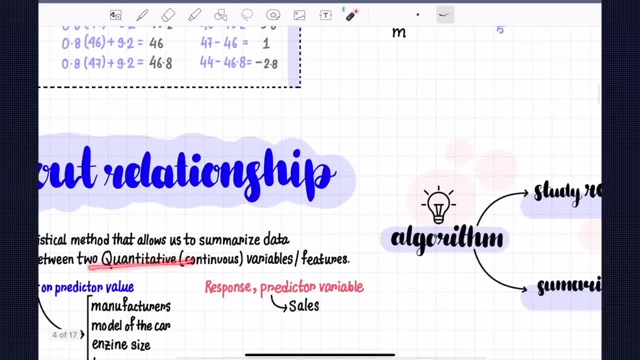 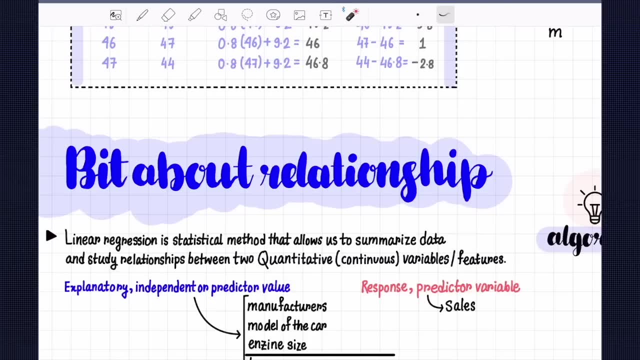 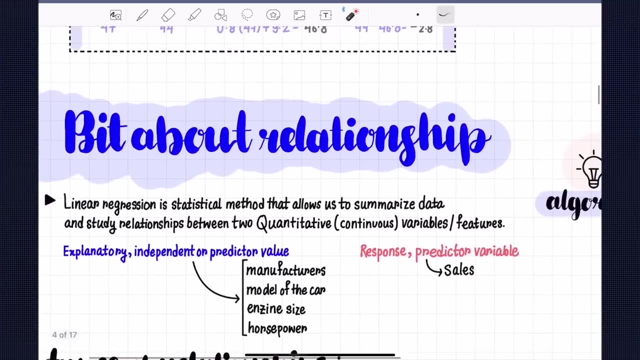 that's what the that's, that's that's what it uh conveys, that you have, um, uh relationship between two quantitative variables, where you have a particular over here, which is it tells you about the two quantitative continuous variable sort of features. okay, so assume that, assume that you. 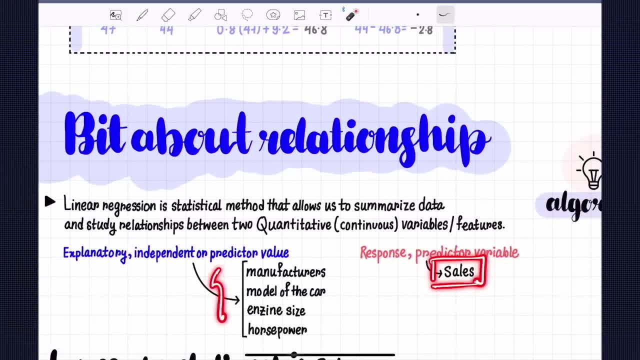 want to predict the sales of a particular car given these particular features. so you know, build a function f that takes the manufacturer, that takes the model, that takes the engine size and that takes the horsepower, that takes all these poor fiend input features and predicts the sales of a particular gap. it predicts the sales of a particular gap, so 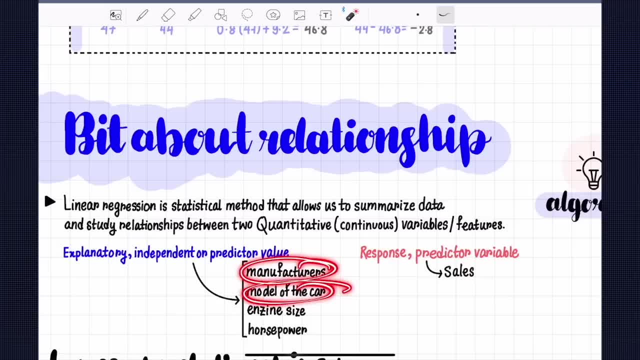 basically, we, we, we tell: okay, this is a manufacturer, this is more of the guy, this is the engine size, is the horsepower and predicts the sales. so how, this function f, which will eventually help us, the function f will tell, that is, if, if we, how this manufacturer is affecting the sales, how this model car is affecting the 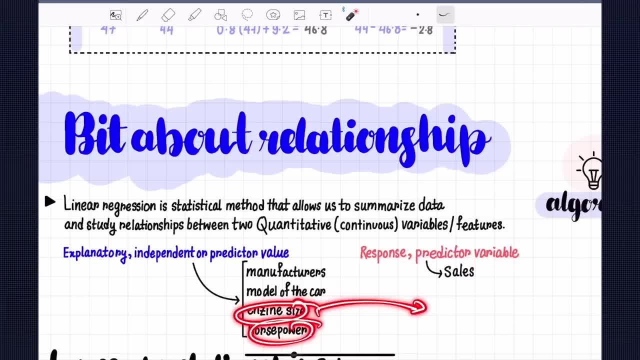 sales. how does engine size is affecting the sales and horsepower is affecting the sales. so we can figure out which of the following is affecting more of the sales, like if we focus more on manufacturer. then, for example, assume that model of the car affects the sales the most. so we can 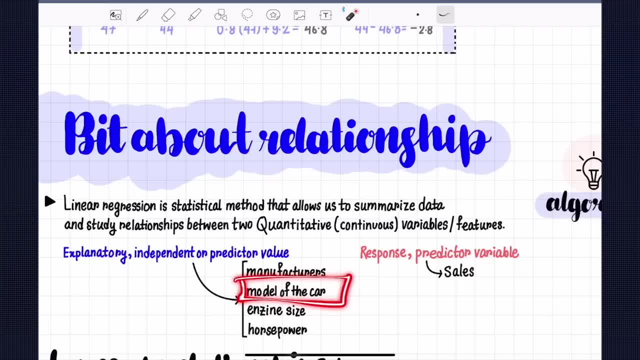 focus on model of the car, a model of the car to brand it up, to get more sales right, because this is generating most of the sales for us. or if this is generating, then we can focus on showcasing engine size or we can show us so, focus on showcasing horsepower, or we can focus on showcasing 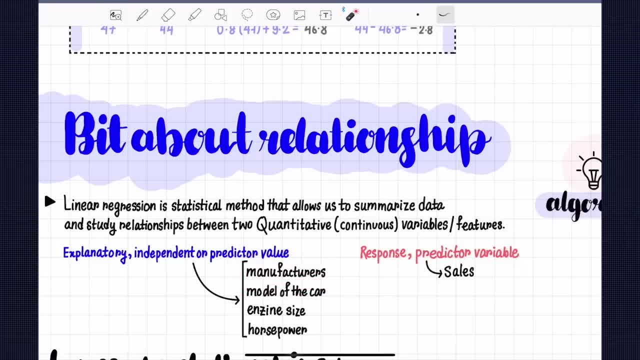 manufacturer, according to our analysis. that's why I say it helps us to summarize and study relations between these variable and output variable Y- okay. so these variable which we give as an input are called explanatory variable, or independent, or predictor variable- okay, or value. so why we call? 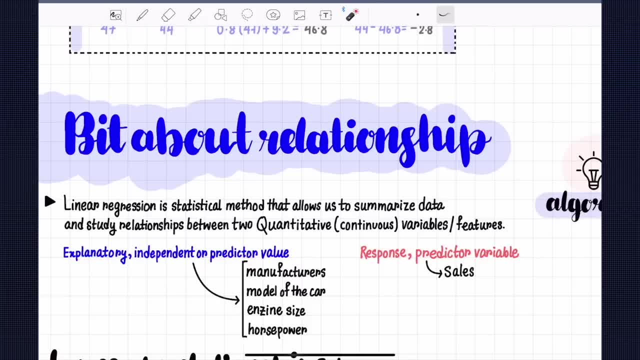 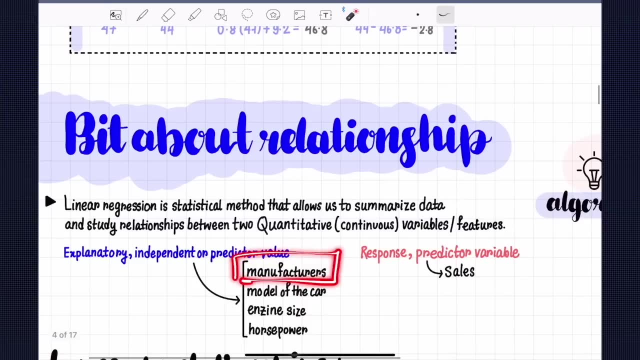 them independent. independent or predictor or explanatory. first of all, every, each individual feature, each into each individual feature or variable are independent of each other. for example, this particular variable is not dependent on this manufacturer's is not dependent on this for its own existence. model of the car is not dependent on the engine size for its existence. 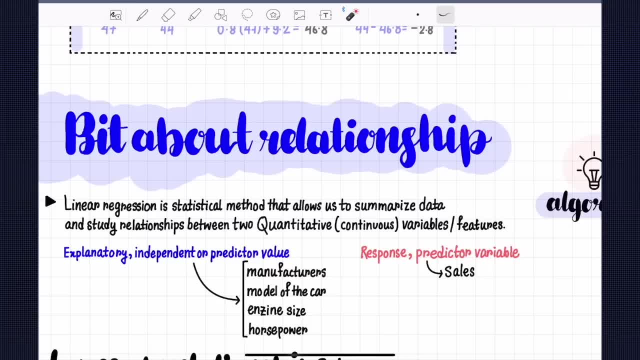 horsepower is not dependent on the engine size for this, because that's why you call independent. but this particular sales variable is called the dependent because this is something which you're trying to predict. we cannot predict sales if any of these variables are not here, right? so sales is dependent on manufacturers. 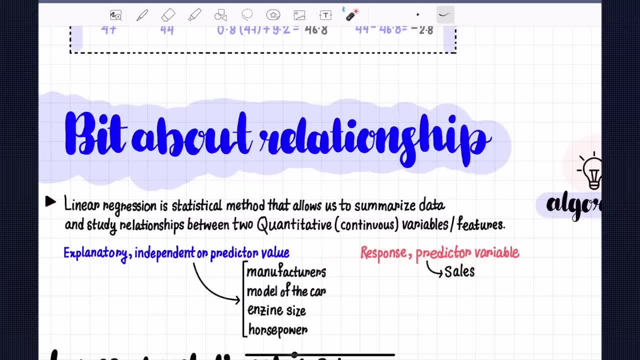 sales is dependent on more of the car for its own existence, right? I hope so that that is clear. there's something to be removed over here, that this is not the predictor. let me just remove this, maybe it makes more sense. yeah, so now this is: this is a response or dependent variable. this is a response or dependent. 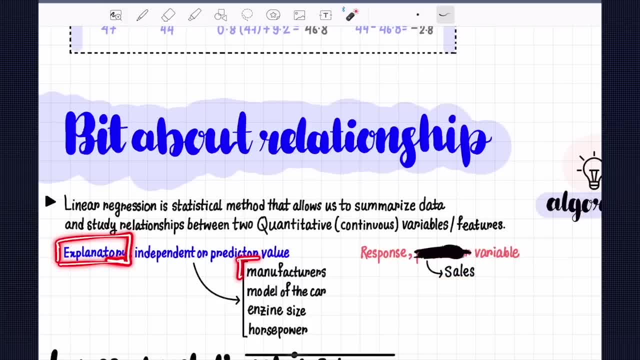 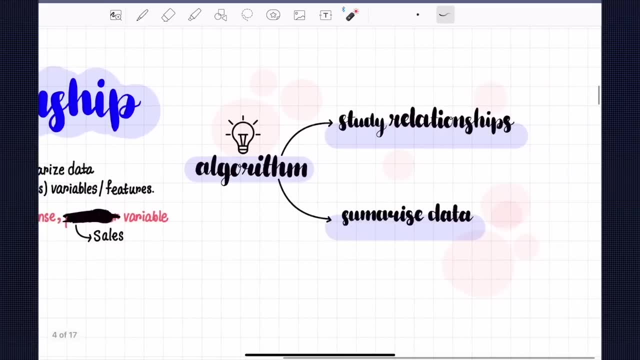 variable. explanatory variable means it is self, explains it like it. it is explanatory by itself. manufacturers, we know that more of the card. that's why it was a stimulatory variable, right or independent, I hope. so that it makes there. you can see our data fundamentals lecture for more info. cool, so the 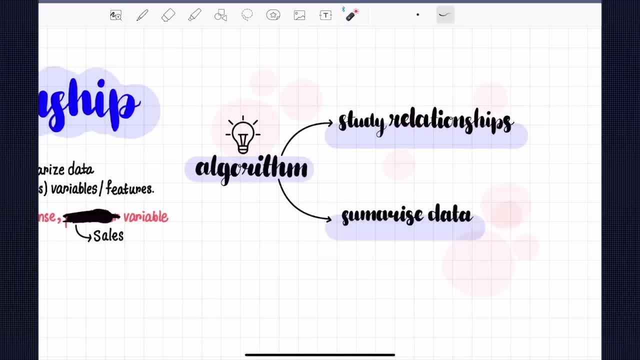 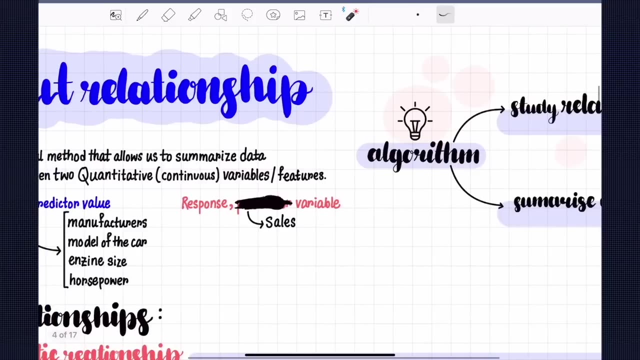 algorithm. let's first talk about what is an algorithm. algorithm: it's in step-by-step procedure, is in step-by-step procedure to solve a particular problem, and we have and we have an algorithm in machine learning to study relationships and summarize data. so I hope that this gives you good sense of what this various 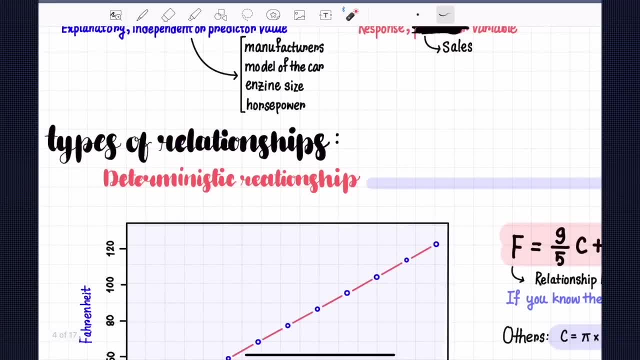 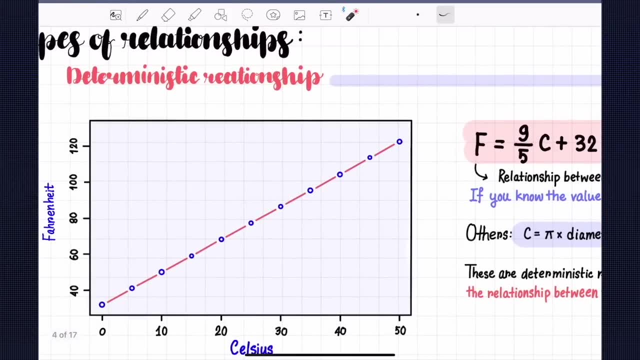 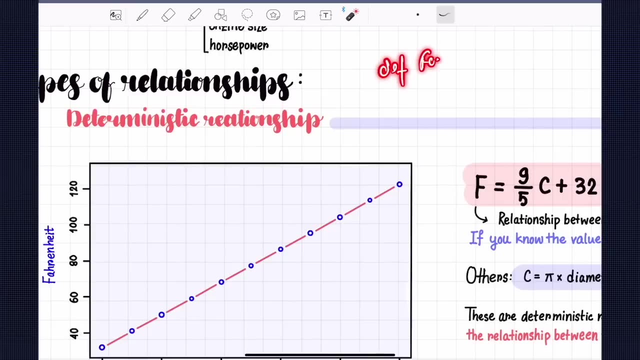 examples: we have a dog, okay. so there are several types of relationships which you come up, come across. first type is deterministic relationship. deterministic relationship: so you might have coded in Python that you have for boarded a function in Python that converts Fahrenheit in. so you have de abhorrent fungal that converts Fahrenheit to. 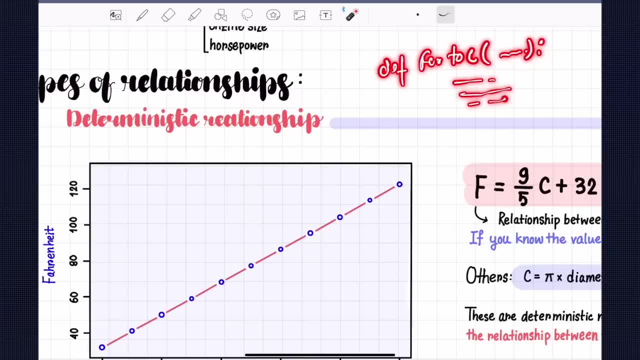 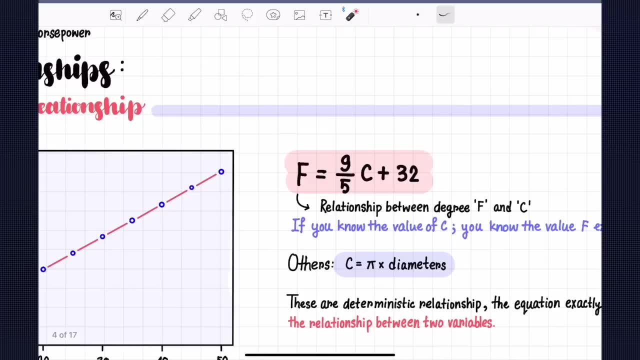 Celsius, right. so you have code in Python that converts Fahrenheit to Celsius, right? so that is the deterministic religion y, I'm saying that is a determinist religion. the formula for converting your Celsius to Fahrenheit. so we can build a function F that takes in the value of and that of that death. 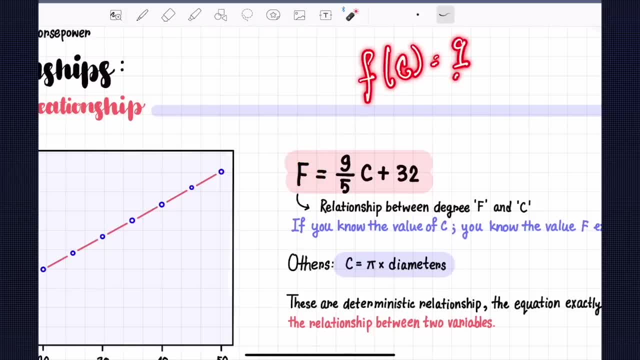 function F is a Fahrenheit that takes in the value of C, 9 by 5, C plus 32. so this is so. this is an example of a deterministic. why it is deterministic? because you can simply plug any value of C. you will get exact, for example, just you. it will just be converted into Fahrenheit. so then there. 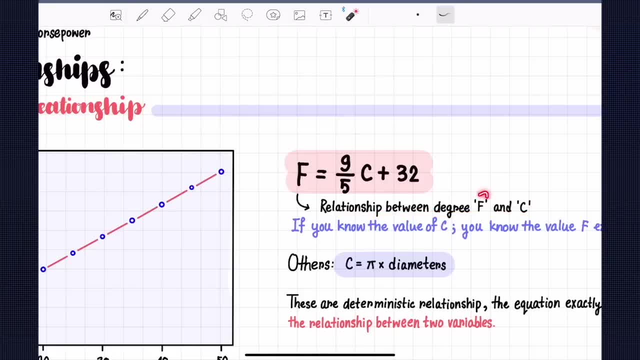 is a defined relationship already there for F and C. so if Celsius is this much, then it will just calculate things up and get you the firm F. if you know the value of C, if you get the value of C, you can easily get the value of F exactly. 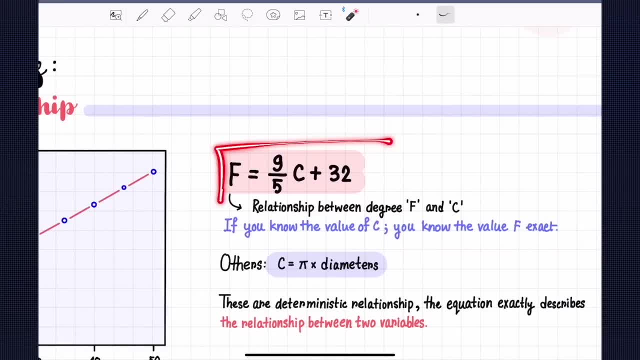 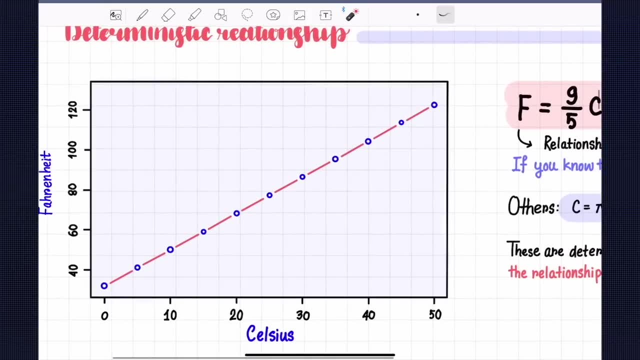 okay, because this is already defined, the formula which we have, this is already defined, the relations of which which we already have, and it is linear sort of thing. for example, if, if your cells is 0, then you, Fahrenheit will. well, when will be this? if your Celsius is 10, then your, then your value will be also on y-axis. 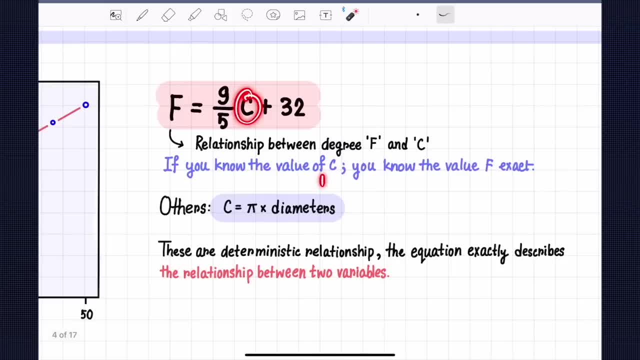 which is the Fahrenheit. so you, if you know the value of C, you plug in the value of C and then you get exact F. you Other examples are: if you want to calculate the area of a circle which is pi r squared or pi d, 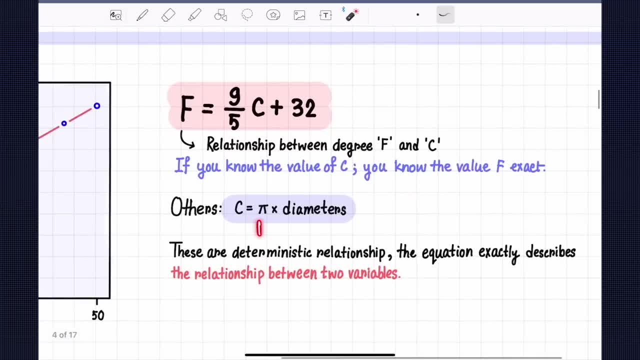 so this is the area. this is defined. you plug in the value of pi and diameter, you get the area. 1 by 2 times bh, defined relationship. you plug in the value of b and h, you get the value. 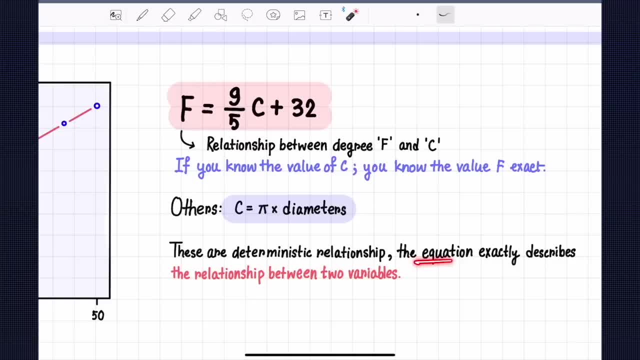 So these are defined relationships. This equation exactly describes these equations, exactly describes the relationships. Plug in the value, it will multiply with some factor and then it will multiply that c with some factor, 9 by 5, and then add 32 to it. 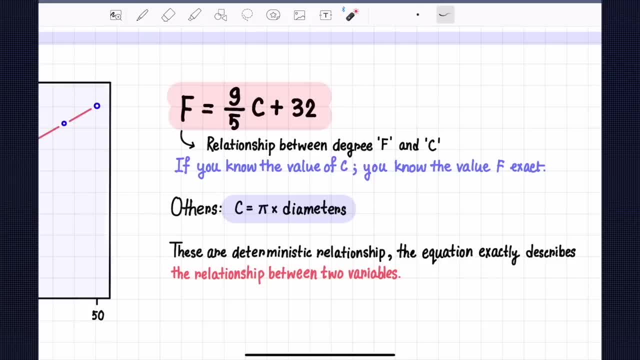 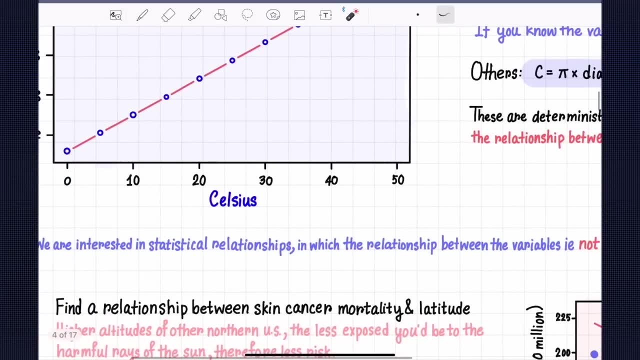 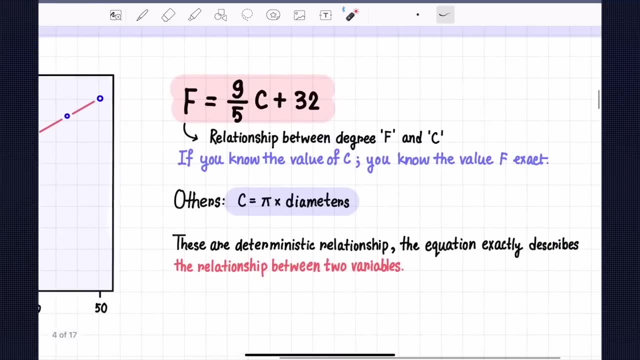 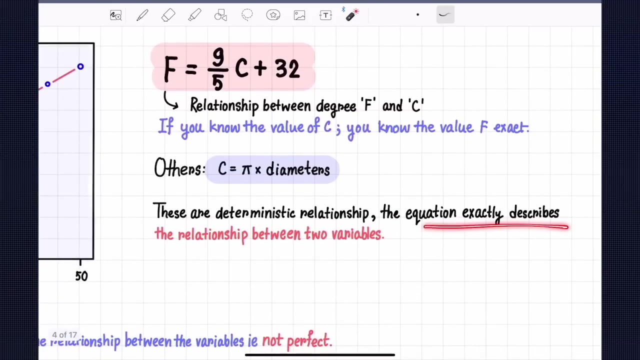 And it's the exact or defined relationship between the two variables And it's also defined relationship between the two variables. But in machine learning we are interested in statistical relationship. In statistical relationship the relationship between two variables are not perfect. Please note that in deterministic and statistical. in deterministic your relationships perfectly defines the particular variable between two variables. 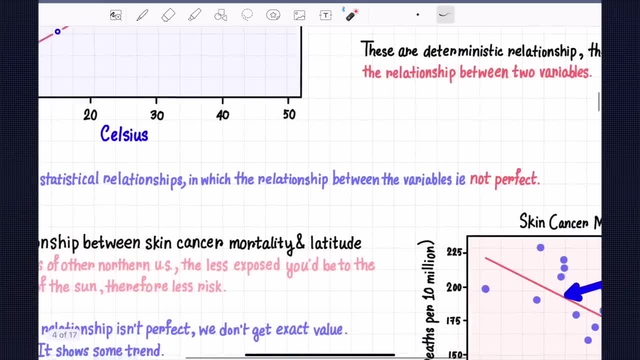 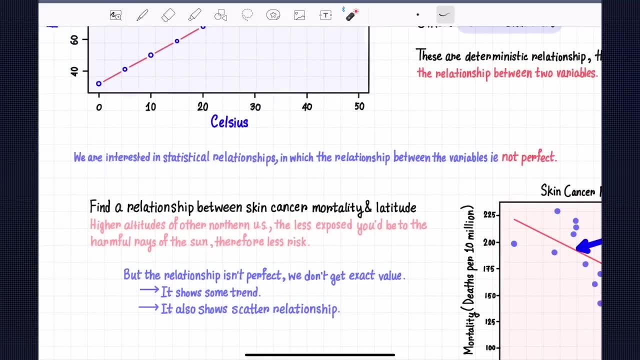 But in statistical it does not perfectly defines it. I hope that is much more clear. So one such example is: If you want to find a relationship between skin cancer mortality and latitudes, So you want to find what is the relationship between the latitudes of a particular country and skin cancer mortality. 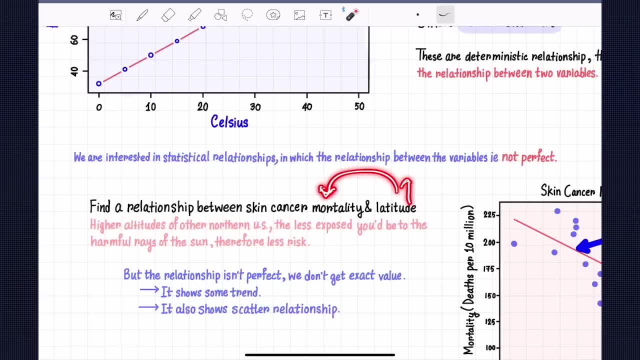 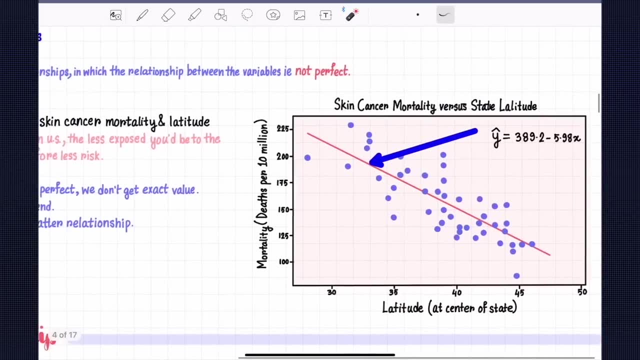 So if the latitudes increases, whether the skin cancer decreases or increases, This is a question. right, This is a question. So this is the data which we have. this is the data which we have. on x-axis, we have the latitudes at the center of the state. 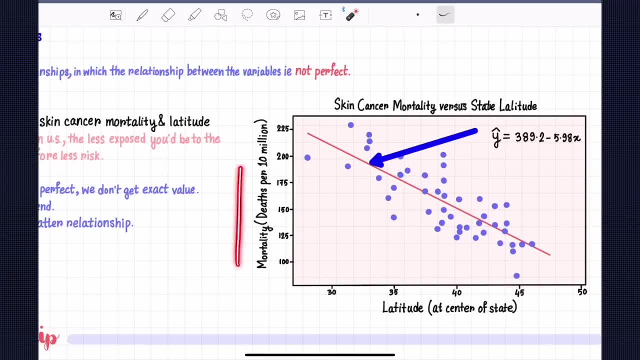 On y-axis. on y-axis, we have mortality that's per, that's per 10 million. this is the mortality rate. this is the mortality rate and this is your latitude, And all the blue points are the data points. 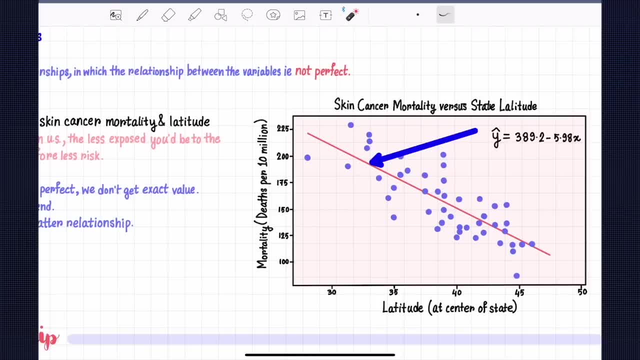 Now what you did, you, you, you, you modeled the you straight line on this which best fits the data, and that straight line is of this, where your intercept is 389.2, minus. I think, yeah, yeah, that this, this, this, this particular thing, is bit wrong. 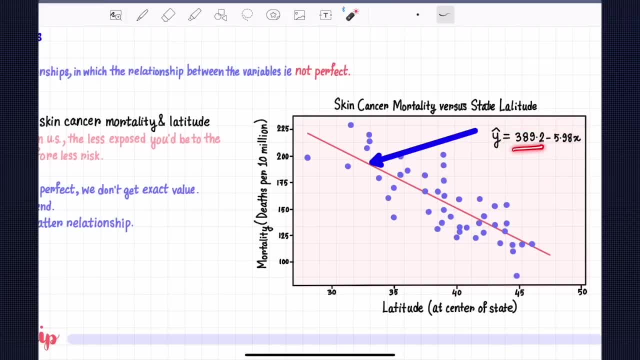 Yeah, over here this, this should be yeah, so which is 3, 3.389.2 minus 5.98x, where this is, assume that this is your straight line. this is your straight line, okay. 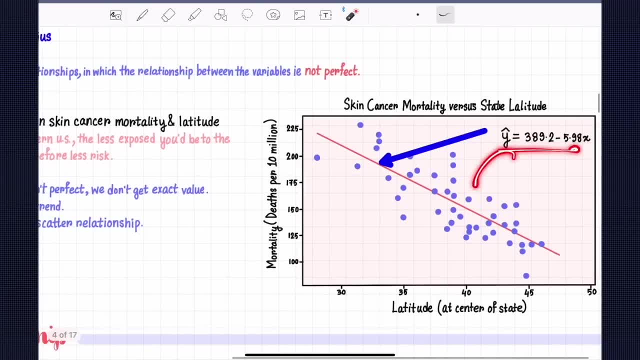 This is your straight line out there. this is your equation for this straight line. this equation for this straight line. I hope that it makes sense. And this is the negative relationship. this is the negative relationship. first of all, we'll talk about the positive negative relationship and further on, later on. 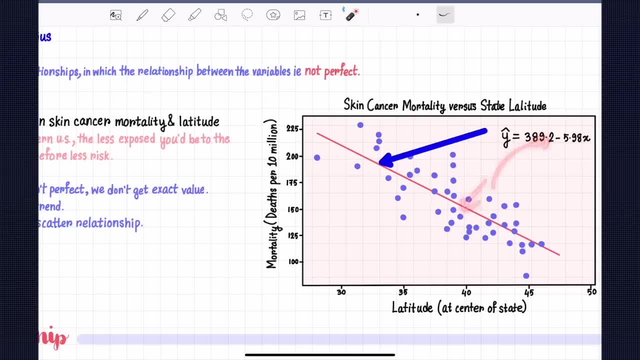 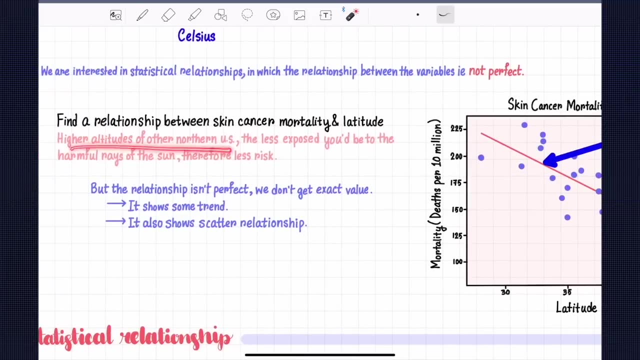 But, but as of now, you can see that this, this equation, is defined by this, this- to stay straight line- defined by this particular equation. now, how can we interpret what is going on over here? well, how can we interpret what is what is going on over here? so assume that you can see the higher lat altitudes of northern us, the less 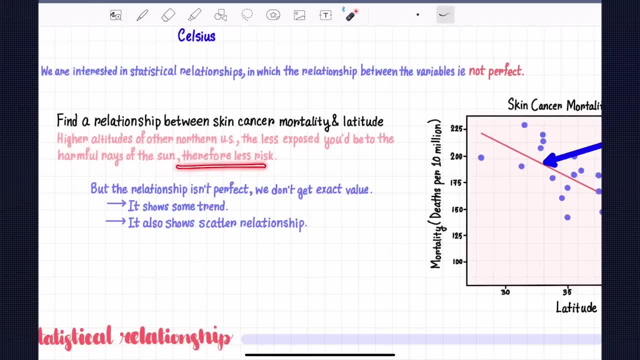 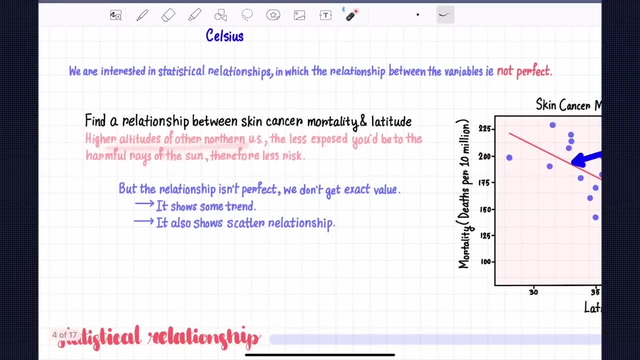 exposed you did due to the harmful rays of the sun. therefore, the less risk, therefore, the less risk. so let's, uh, let's, figure out. it is saying the higher latitudes of the modern northern us. higher latitude means over here, high, higher latitude, which, which, which are going to the right of the 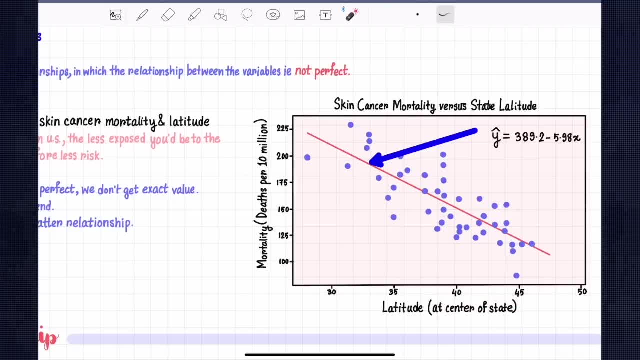 side. then you then this 45 uh 45 to 50. so higher latitudes. higher latitudes means you are less exposed to the harmful rays of the sun. so when you go over, when you, when you go this side in the higher light. so if you see, there is no data which suggests, which suggests that any, any uh values of 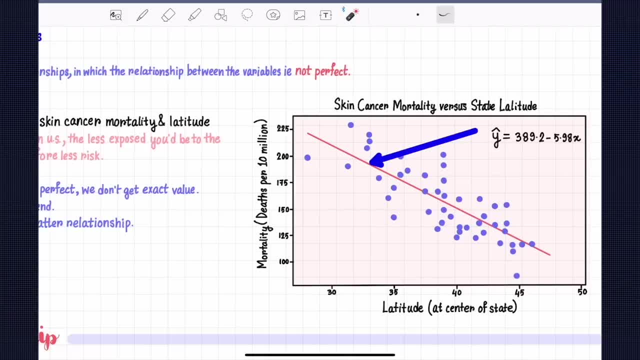 cancer mortality. right, cancer mortality, is it? there is a less. or even for on whatever, there is a less, not too much, not too much. on 50, there is nothing but on. so if you go to the right side or the, or, the more, the higher the altitude is. 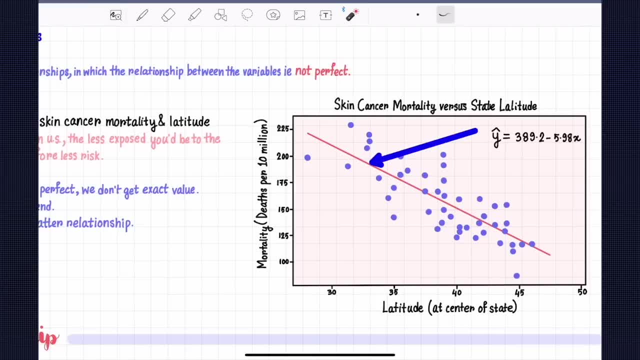 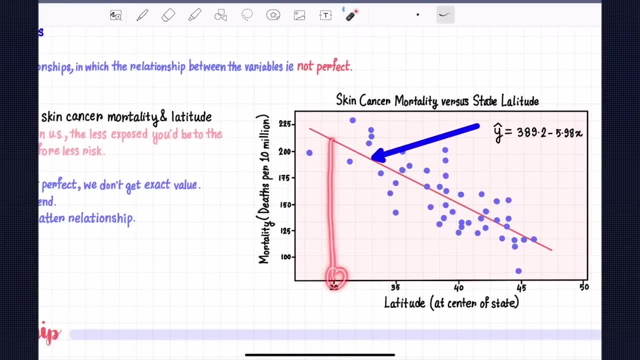 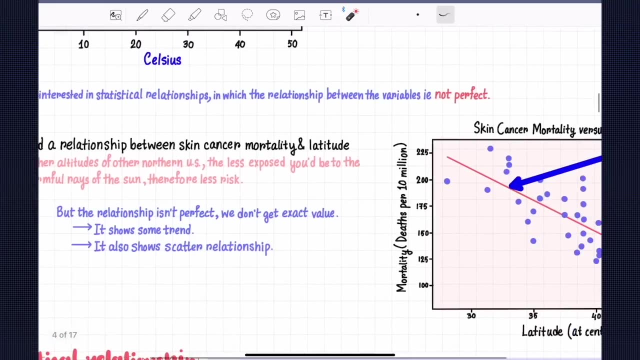 less. the more mortality, therefore less the risk. okay, but if you go over here on 35, there is lot, you know, there's a whole chunk of uh information out there or the mortality rate out here, okay, so i hope that this gives a good sense about it. so, but over here you can see the 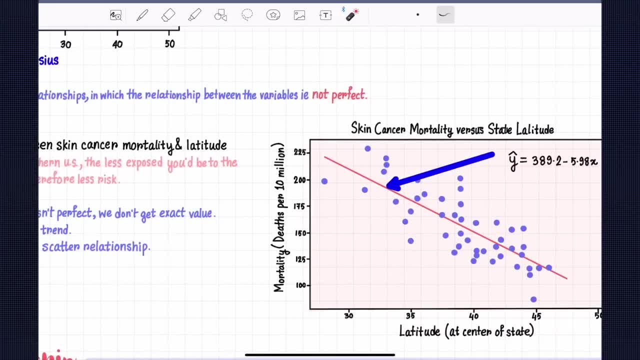 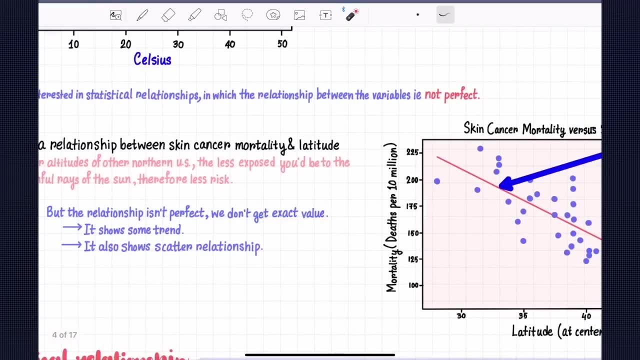 relationships are not perfect. sometimes over here there is this much right, but the relationships are not perfect, because we don't get exact value. we get approximated value, but we'll not get exact value. so if you, if, if, if you have seen over here, if you have seen over here that we have that, that 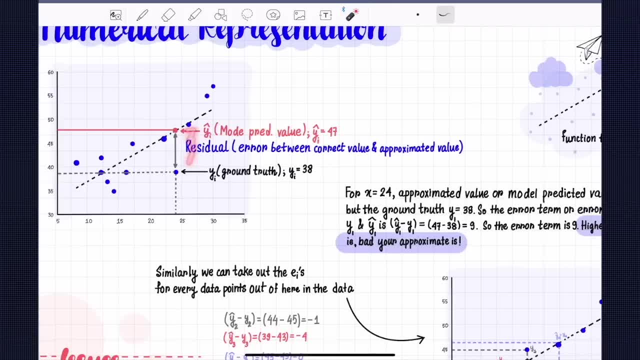 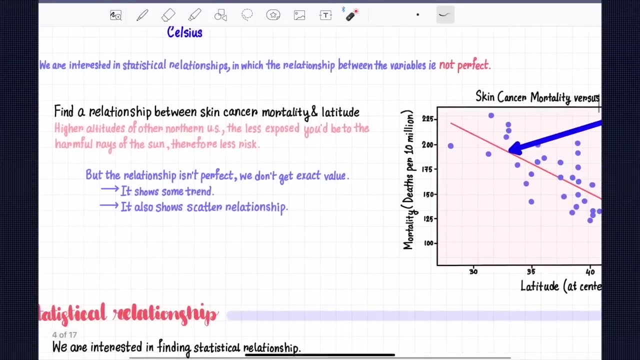 we were getting some sort of residuals, that that we were getting some sort of residuals, right. so your model has approximated but didn't got the exact file. this is called exact value. but your model is approximated and the model has approximated it, okay. so i hope that this gives a good sense about what is why exactly it's not perfect. 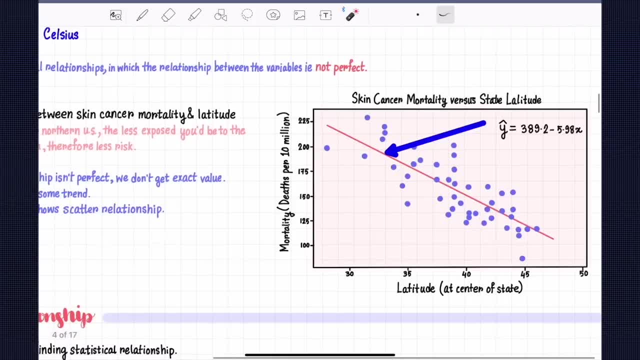 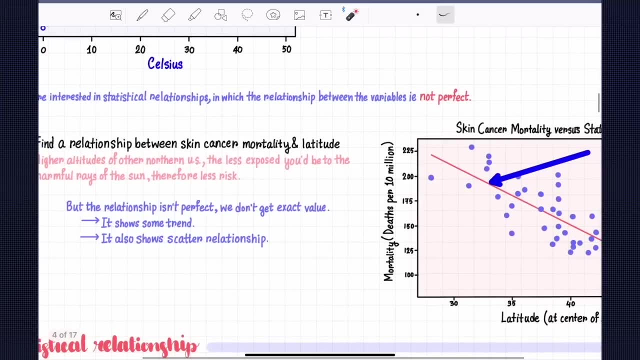 it shows some trend. it is showing some trend as we go to the, as we increase the latitude your cancer mortality rate is in decreasing. okay, and it also shows the scattering relationships. you can see that already there is a scatter and it's the scattered relationships. so, as you can 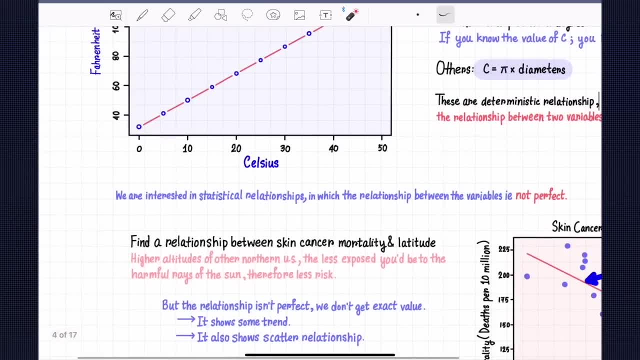 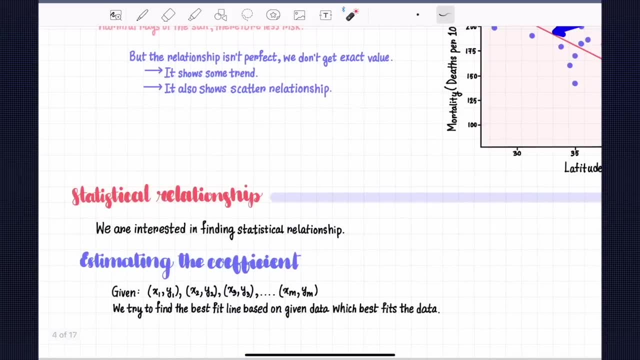 see that this is, this is what the statistical and over here over the course, we are going to talk about studying, modeling, the statistical relationships. okay, cool, so we are interested in finding the statistical relationships. so now, now, uh, we'll summarize what exactly we started after changing some rotational changes, so that it makes sense in the next lecture what 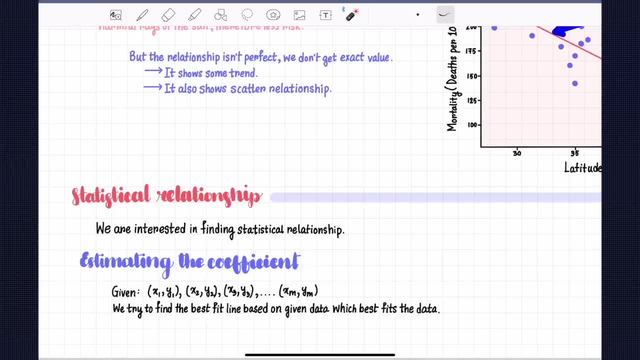 exactly we are going to do, if we are going to talk about: how can we estimate the coefficient? how can we estimate that m and b in that equation? so you have, i guess y equals to mx plus b. how can we estimate mx plus b? mx plus b? 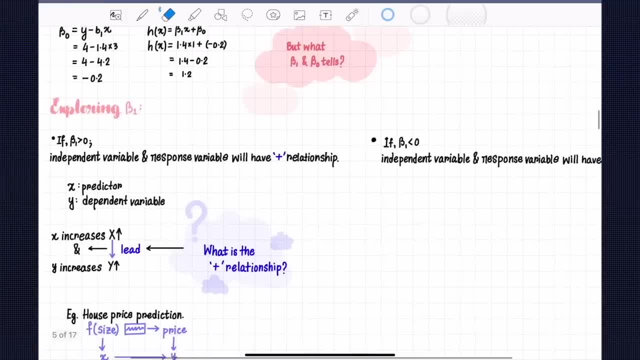 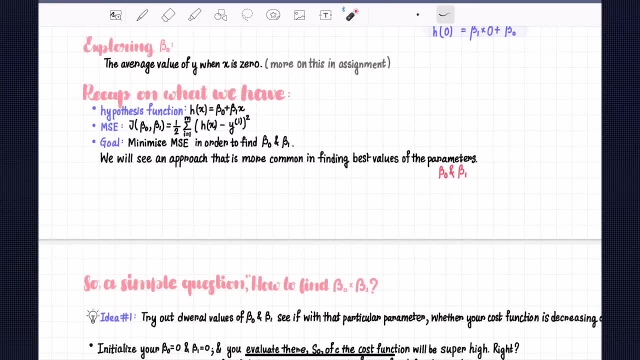 m and b by giving you some notational changes, and then we'll talk about how, what is the interpretation of that m and b in different terms, and then we just, and then we'll just recapitulate whatever we have studied so that it makes much more sense, and then we finally go on. 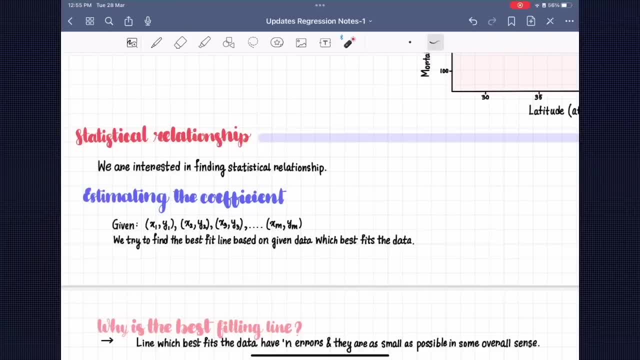 understanding how we can get that in simplest terms. so, everyone, now what you're going to do is and talk about a bit about. how can we estimate m and b, what are its interpretation? what is this interpretation? what is this interpretation like, what exactly it means, and etc. after some notational 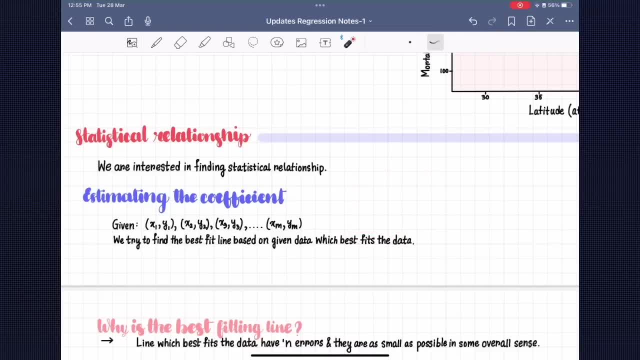 changes. so yeah, so first of all, what are we given with? so you, so you're given the data, so you're given the data x1, then you have y1. so basically it is a supervised learning problem. so you have input value as well as its label y1. 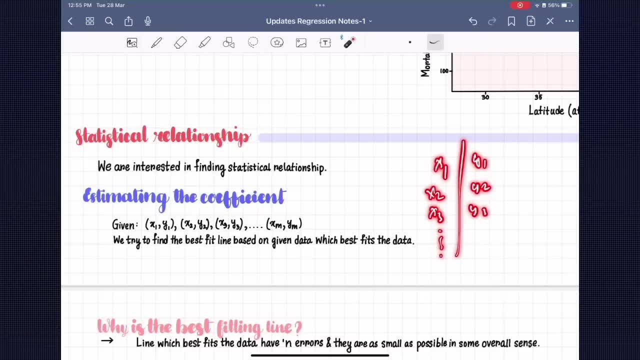 x2, y2, x3, y3, all the way down to the xm, yn. so you have particular input value according with, with, with with these labels: x2 with this label, x3 with this label. so you, so you're given the data and we try to find the best fit line, based on the given data which we have, that best fits the data. 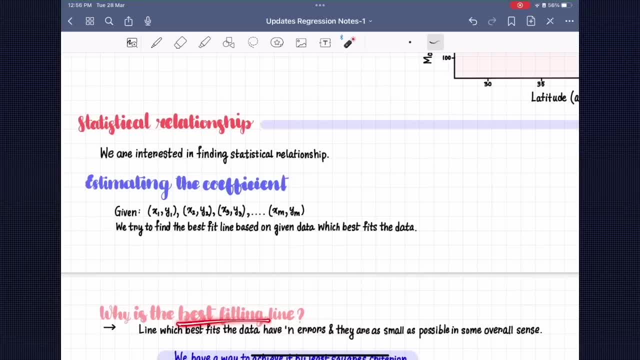 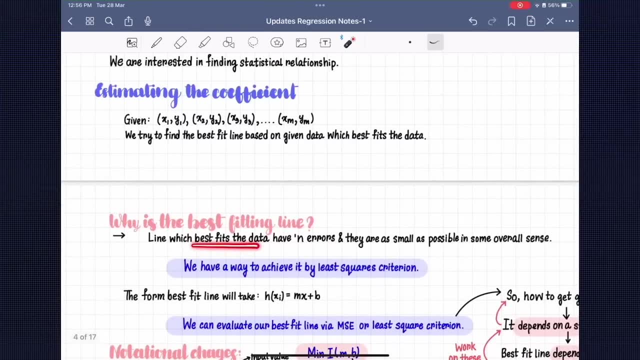 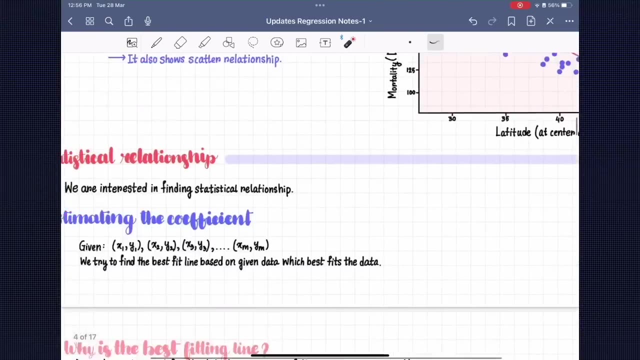 that's our end goal. so why best fit line? a very nice question to tackle. why do we want the best fit line, right? so line, line, line, the line which best fits the data. have n errors and they're small as possible in overall sense. okay, so we want to find, so we want to find a line which have n number of errors, which are 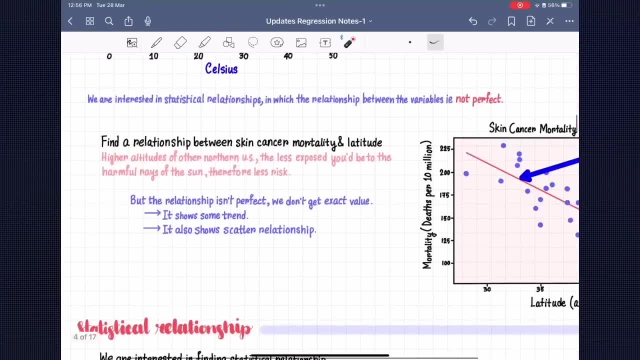 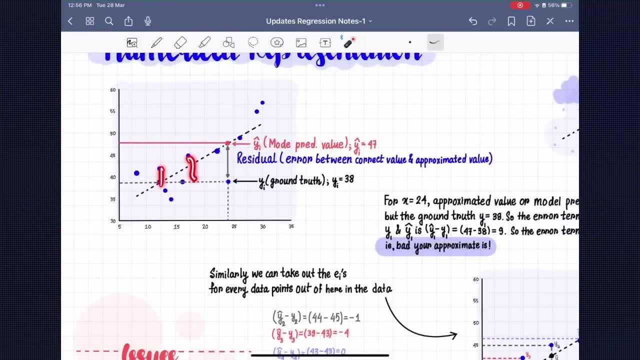 n number of errors and they're small, as much as possible, overall sense. so what does this mean? overall sense? in overall sense means that we have n number of errors: n1, n2, n3, n4, n5, n6, n7, n8, n9, right. 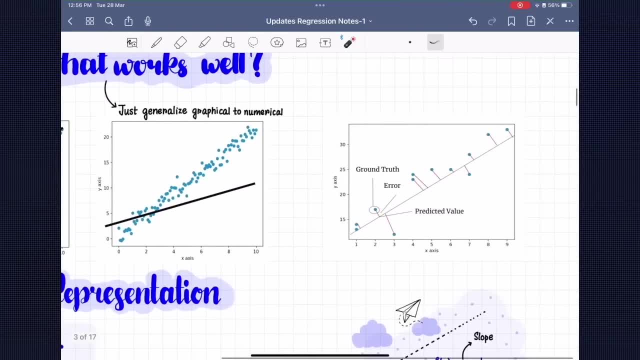 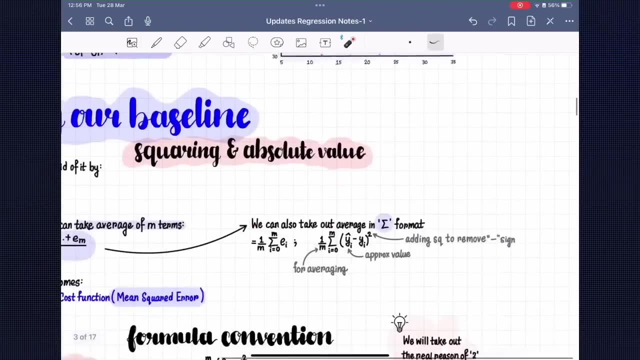 so this is the, this is the so over. you can see that we have 1, 2, 3, 4, 5, 6, 7, 8, 9, 10, 11, 12. so we have a 12 number of 12 errors. so 12 means when we take an average, it should be very small. so overall means average. 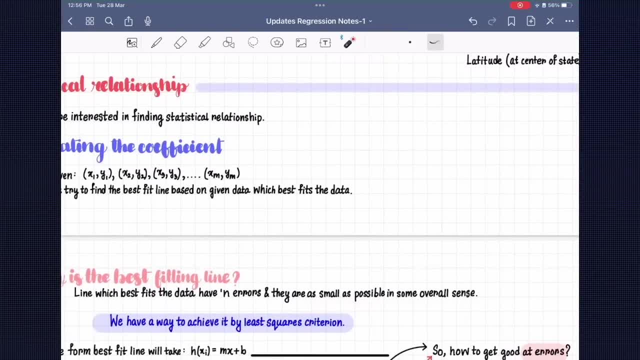 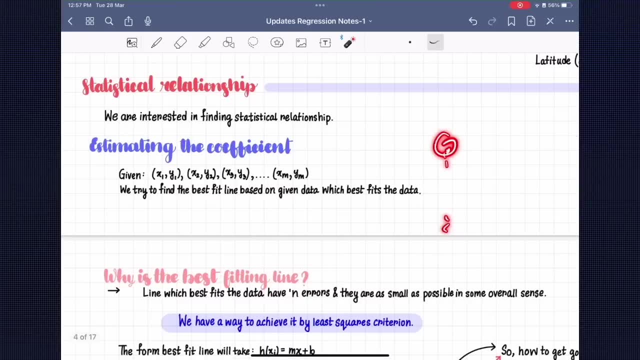 so it should be as small as possible. and then, and then we can simply, and then we can simply approximate by going off from the x axis at the point of intersection, that is the y, that is the, that is the coordinate which contains y as well, and then we get a prediction: y, okay, so we have a. 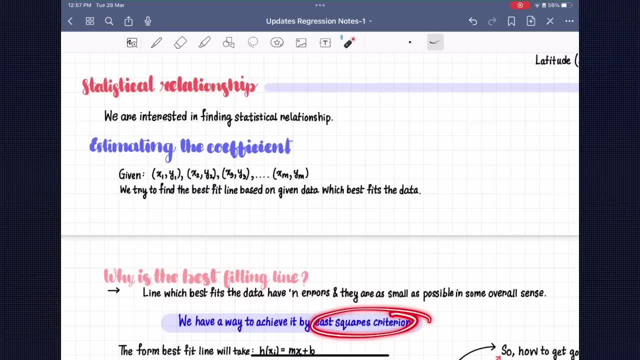 way to achieve it by least squares criteria. so least least squares criteria is something which which will study as well later on. but we have a way to achieve it, which will study later on, but but you can ignore this as of now. so this forms the best fit line. so our equation for best fit. 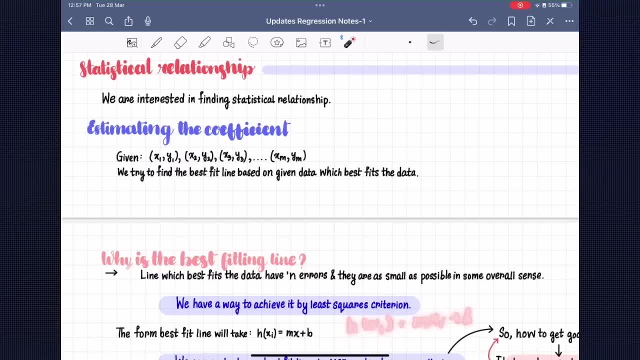 line x1 is m x i plus b. so let me just make sure that this is something. this is something which we should ignore. yeah, so which is h of x is equals to m x plus b, m x plus b. this is the. this is an equation you plug. 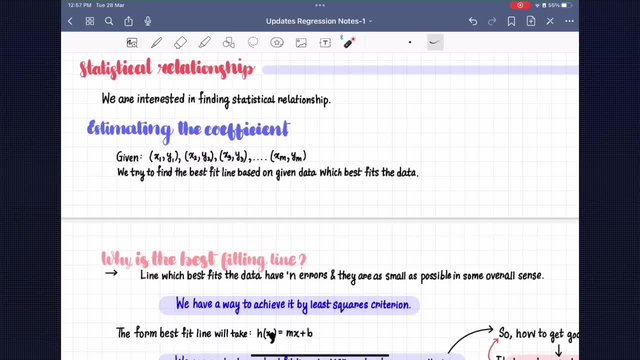 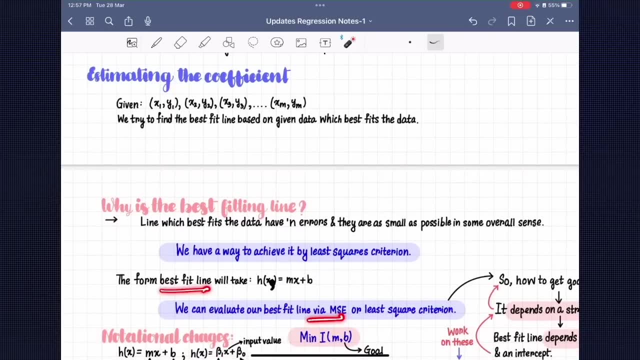 in the value of x and then you get a prediction, and then you can get a prediction for the straight line. so our goal is to find that m and b right right, so we can evaluate our best fit line using our msc or least square criteria. so we can simply evaluate, evaluate our best fit line 1 by 2 m. 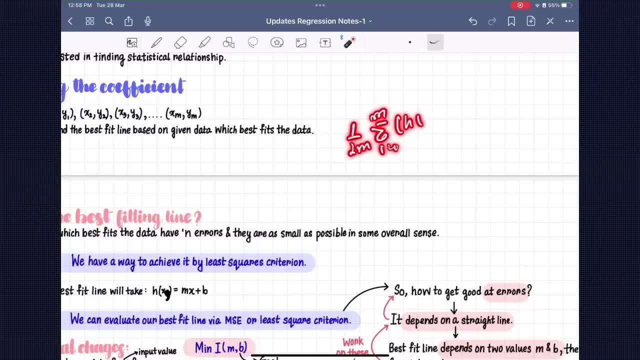 i equals to 0 all the way out of the m h of x minus y minus y squared. why are we squaring? because to, to, to avoid the negative, as we are taking the average and adding two as a convention. but we'll, we'll, but we'll see why this two really helps. 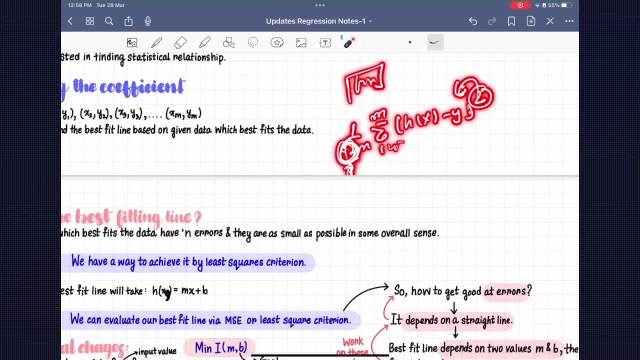 while, uh, in later spaces, of gradient descent, we'll talk about that, but you can assume that as a convention. but we'll talk about- really we will talk about that. why is that too? because i think this is important to talk um, so you can use, simply use this equation to take out some errors and 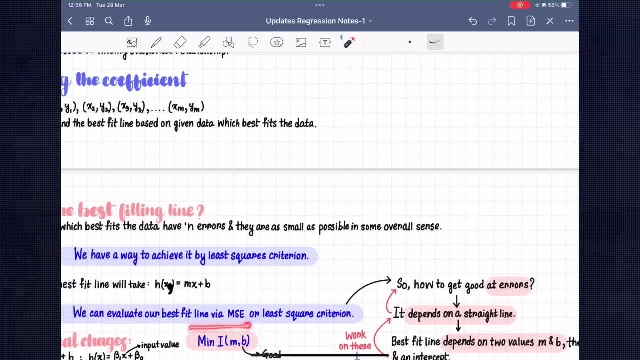 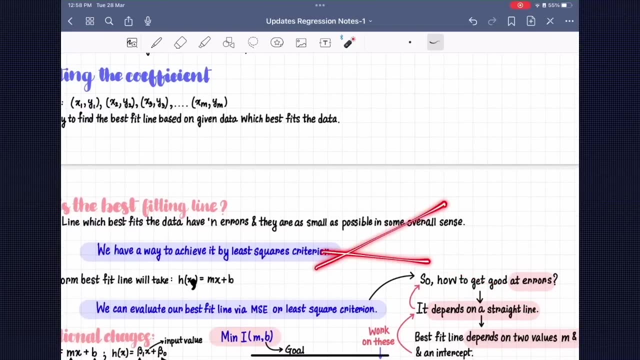 higher the error is bad. your model is. so you use msc to calculate how you're, how you perform, so how you're good at errors. if error is small, so errors depends on the straight line. so if the straight line is bad, like this is like, this is a, this is something straight. 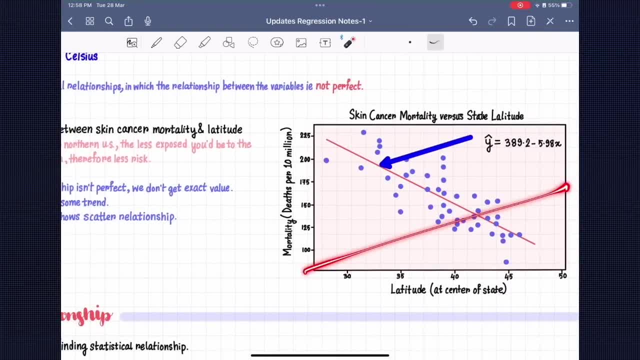 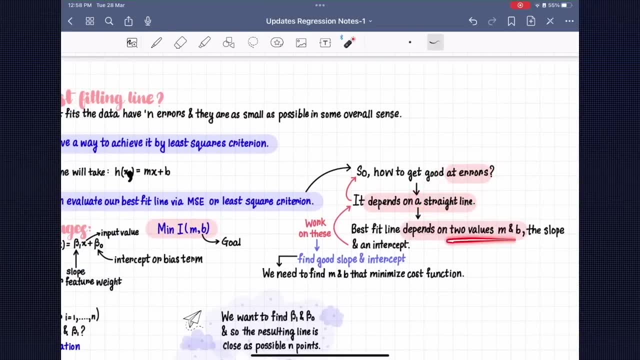 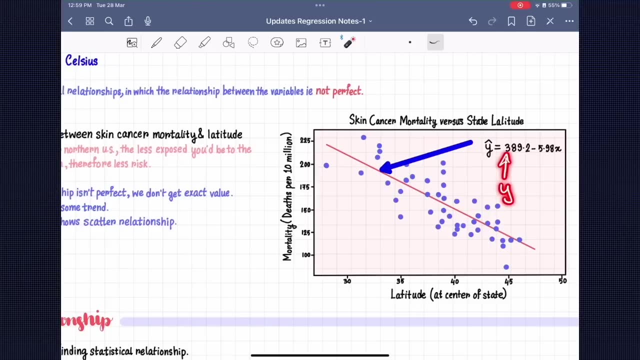 line, this is your, assume that this is your data and this is your straight line. so this is, this straight line is bad, right? so your errors depends on straight line and your straight line depends on two values: m and b. right, because this particular, this particular value has its own y intercept and has its own m. so b and m right, it has own, so it is dependent on. 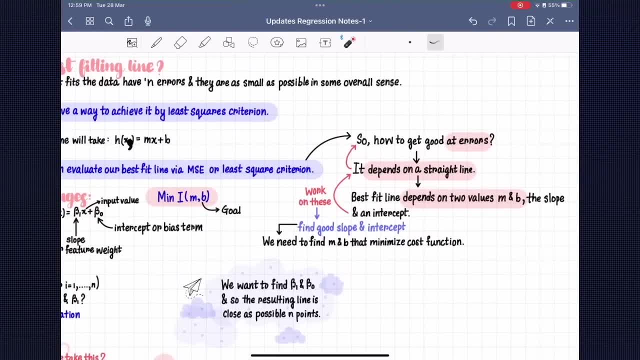 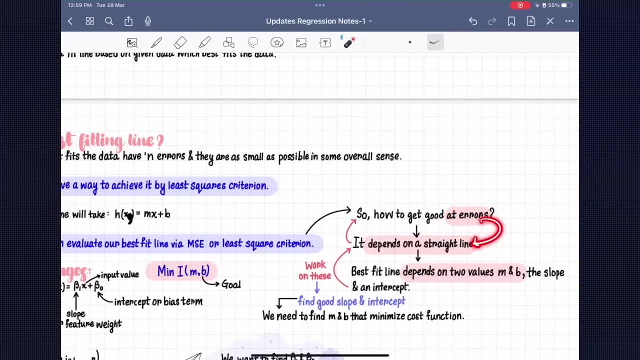 m, which is the slope, and the y- intercept. b, the slope and intercept. so what we want to do we are now. we want to reduce our errors, right. so if you want to reduce our errors, what we should work on, we should work on straight line, we should work on getting a good straight line, and if you want to, 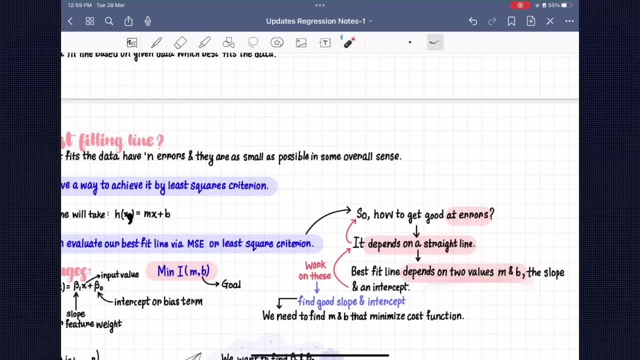 get a good straight line. we should work on what we should work on in getting the good values of m and b. we should, we should find good slope and intercept in order to get the good values of m and b, in order to minimize m and b. that with you, in order to minimize the cost function to find m and. 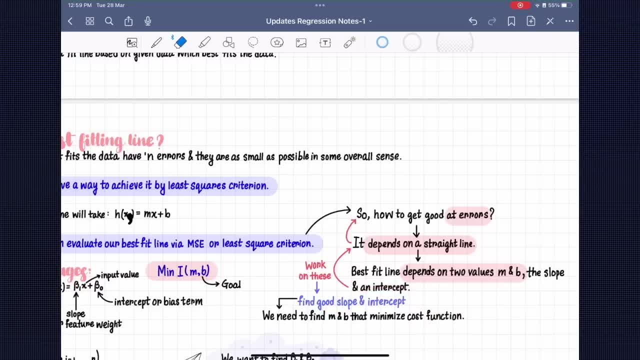 b. so you'll find m and b. that minimizes your cost function, which is you. you have a cost function, j of m comma b, which is equals to 1 by 2 m. i equals to 0, all the way around. so j of m comma b, uh, 1 by 2 m. 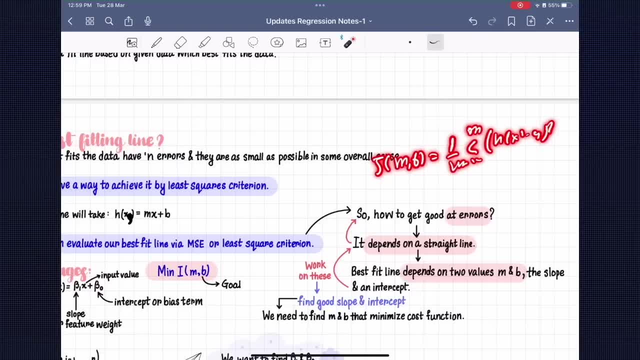 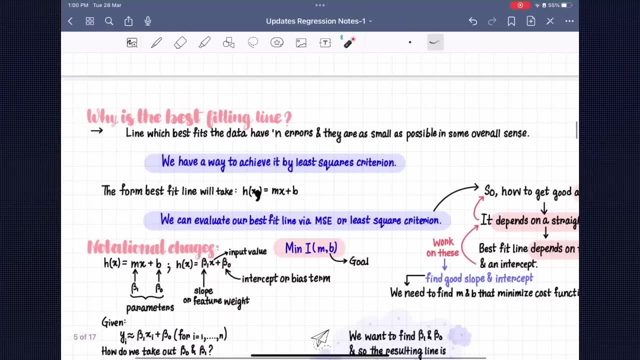 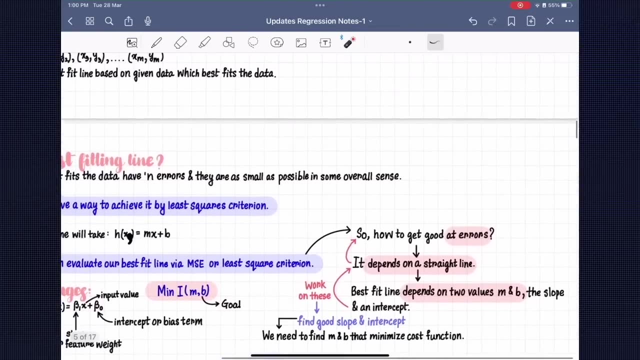 i equals 0 all the way around to the m h of x minus y squared. so squared for negative sign average is out and 2 for as a convention. so now find m and b. that minimizes the cost function. so what are its notational changes? so what are its notational changes? so again to, to, to repeat. 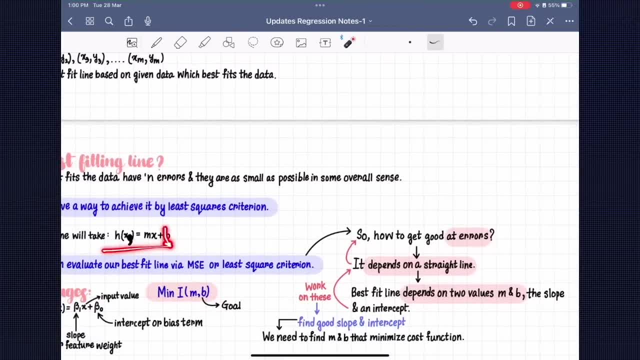 your summary: we, we have an hypothesis, hypothesis give some error, like to now here. now we said how, how the hypothesis is, we get some error, and then we, and then the error depends on straight line. the straight line depends on m and b. so to find a good slope, m and b, to get this good straight line. 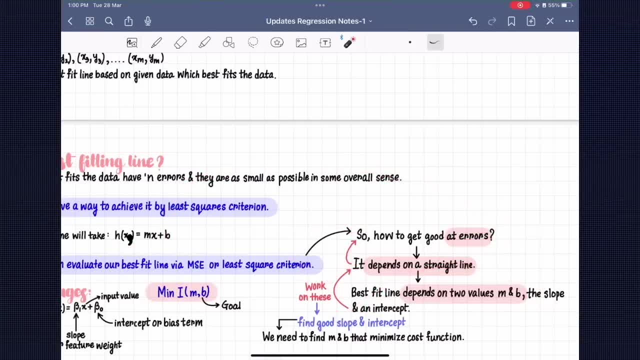 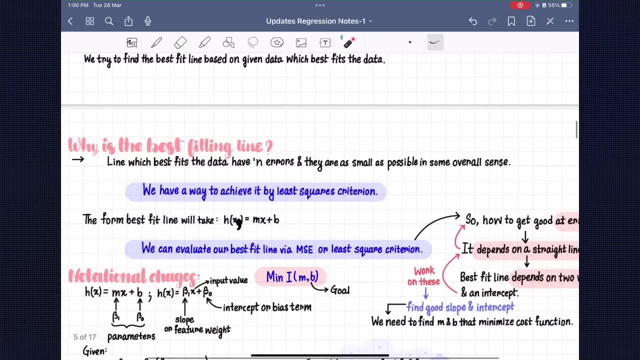 if we get the good straight line, it will automatically reduce the error. a whole story represented on your screen. i hope that this gives a good sense about whatever i'm talking about. so let's do. our goal is to minimize this particular thing which is j. it should be j. i'm so sorry, i'm very sorry, some of the um i'm, i'm, i'm. 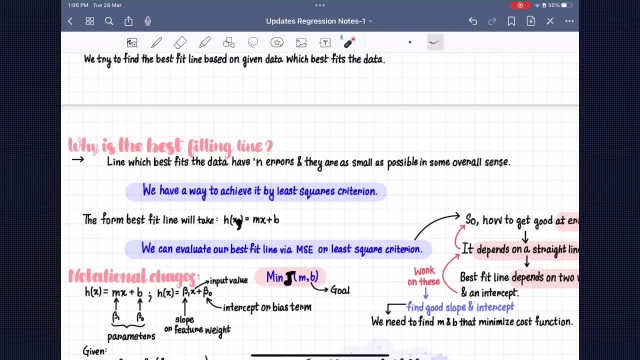 very sorry about this, about. sometimes you get you, you have a bit of you know on errors and all you can definitely report in our errata page. we can fix this up right. it will be much more helpful if you help us to complete it, okay. so what are some of the notational changes? so over here, right? 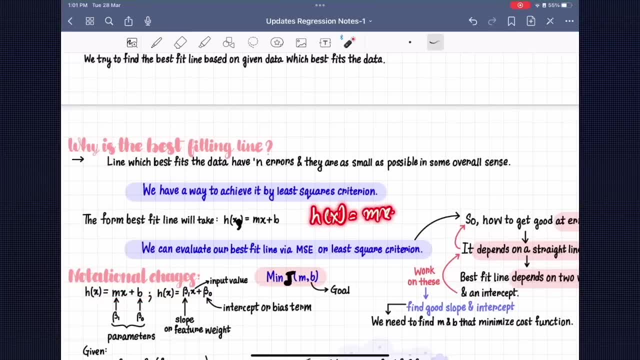 you'll see some of the changes that are there, but so far you need to know as of now if we- you might know this, if you know how to do, um, uh, we call is we'll go to the beta as and now. if you're done with, the beta becomes beta 0. you'll notice again now in our SOJO Jupiter. 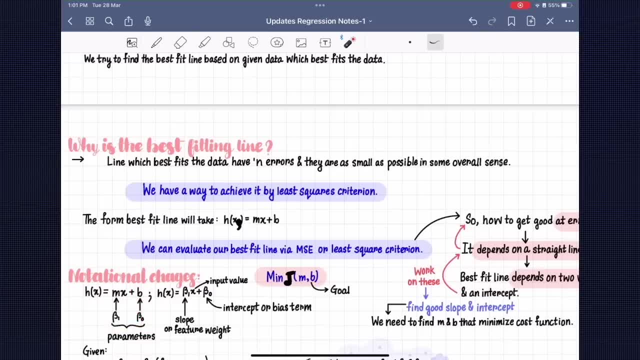 theta. okay, so in this meta then when we edit here in this meta, we'll see what are the pairs that we'll do. so what are the pairs that we Hgeito bit, uh, beta Jones, if it, if we're done in that way and also in the other, you'll see the Baumann, you'll see the putels in addition. 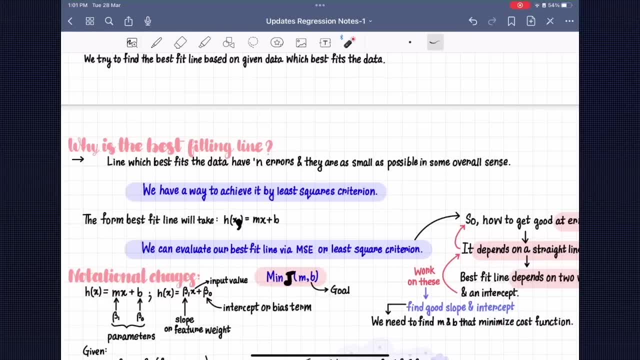 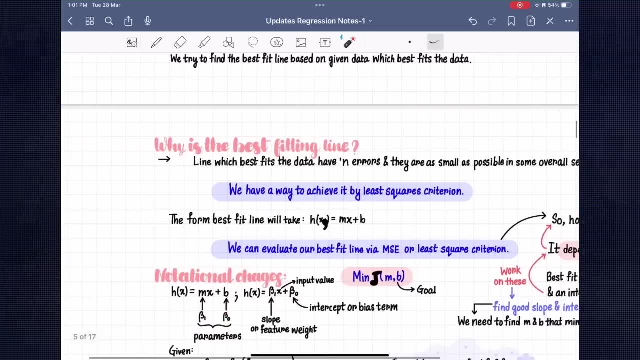 to that right here seated bar right. So when you go to online article, you make sure that you are comfortable with the beta 1 and beta 0. Sometimes, instead of beta 1, theta 1 and theta 0, or sometimes you have some other notation, but we will use this beta 1 and beta 0. 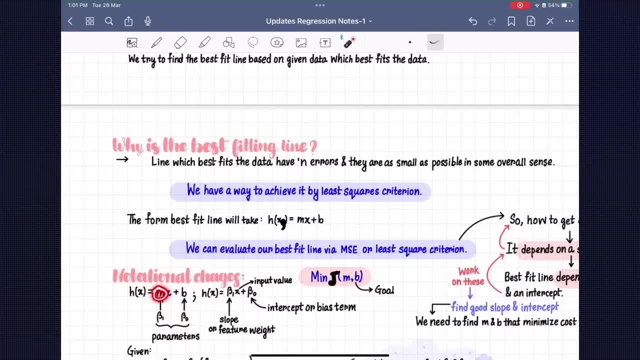 So over here you might assume why are not we taking M as beta 1, M as beta 0, beta 0. But as a convention we always start off with our bias term B, which is B plus MX. So B assume beta 0 plus beta 1 times X. 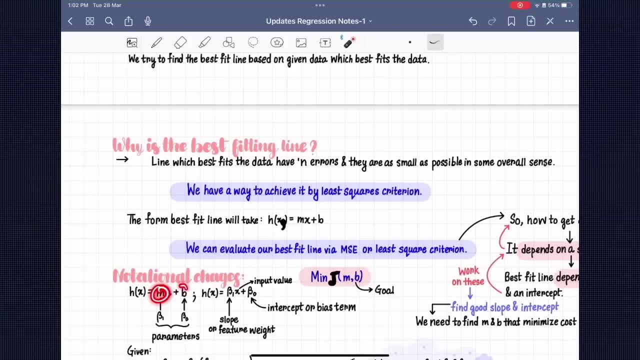 I'll just make sure about this. So your M becomes beta 1 and B becomes beta 0. So you can write beta 0 plus beta 1, X. that is also. that is equivalent to B plus MX. B is equals to beta 0 and M equals to beta 1.. 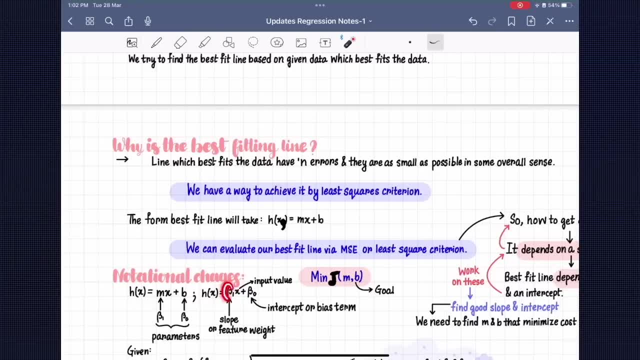 These are the parameters, but the meaning stays the same: Beta 1 is nothing but the slope, and beta 0 is nothing but your intercept. So now there are other names as well. So over here. when you multiply 2X, 2 is 2. over here. 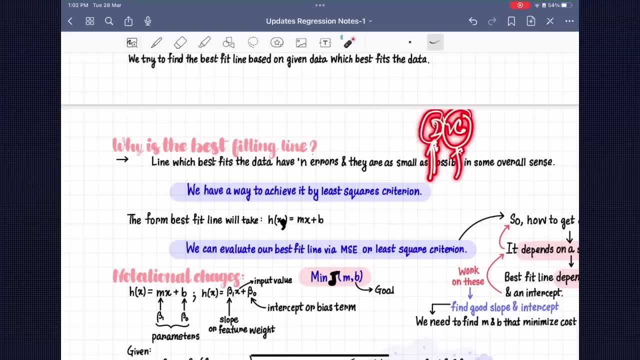 It scales your X, So 2 over here is a weight given to this X, Just like that X has a weight. We have a feature which is X, For example, the horsepower. Horsepower has gotten weight, Horsepower has gotten beta 1. or we can say, even in this case, horsepower X has gotten weight M. 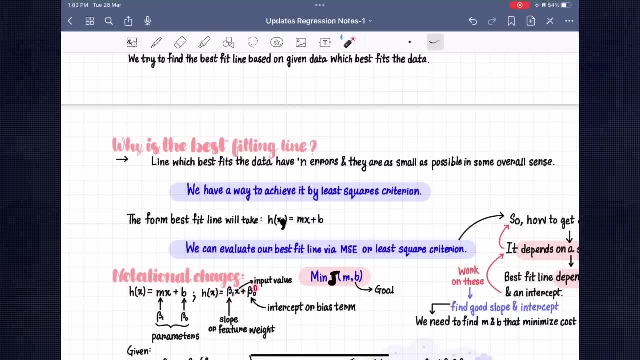 So in this case The horsepower has gotten a weight. beta 1 and beta 0 is intercept or biased term. We'll talk about what is this biased term means later on. but this is a Y intercept, Okay, from where it should intersect at Y axis. 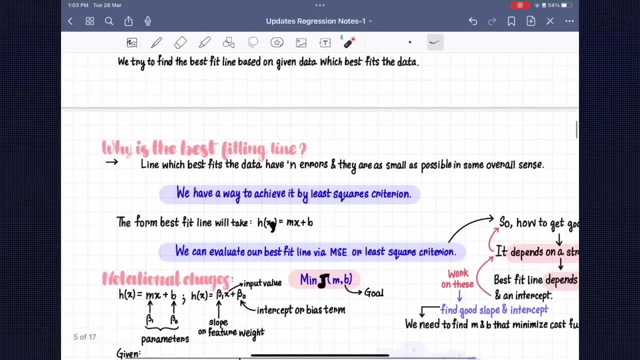 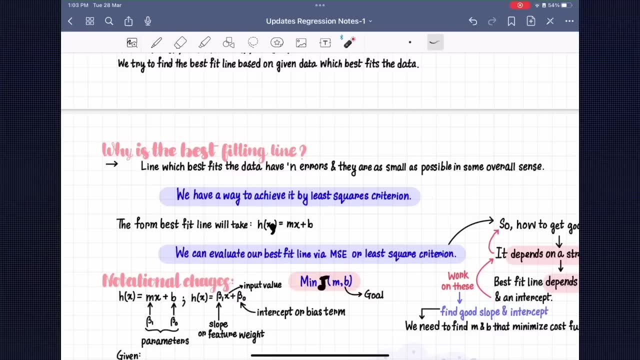 I hope it gives you a good sense about it. Cool, So I just want to talk a bit more about these things, a bit more on your hypothesis. So your H of X is equals to beta 0 plus beta 1 X, right? 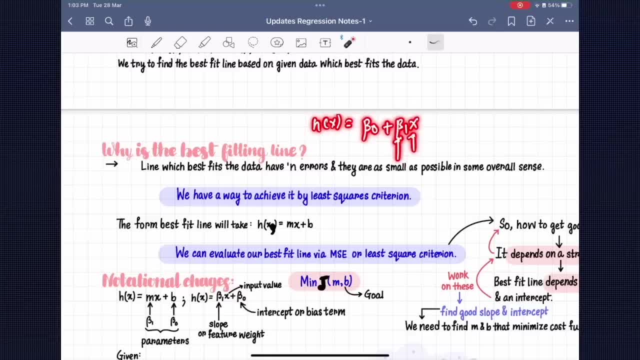 And beta. beta 1 is a feature weight and X is a nothing but your but your but but beta 1 is nothing but a coefficient of your feature or a feature weight or a parameter. Beta 0 is also intercept. We call by convention. 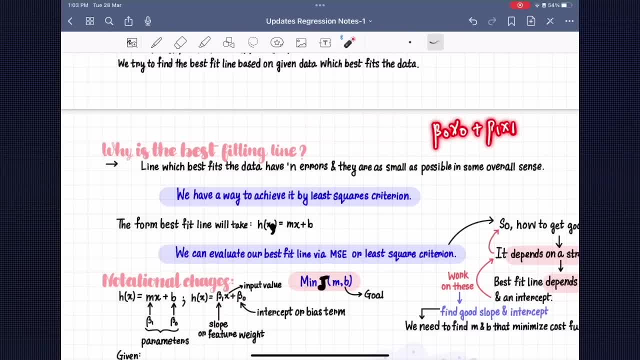 We are beta 0 X 0 plus beta 1 X 1, or we can say beta B times X 0 plus M times X 1.. Okay, So what does this mean? They both are equivalent, but? but we are going to use a new notation. 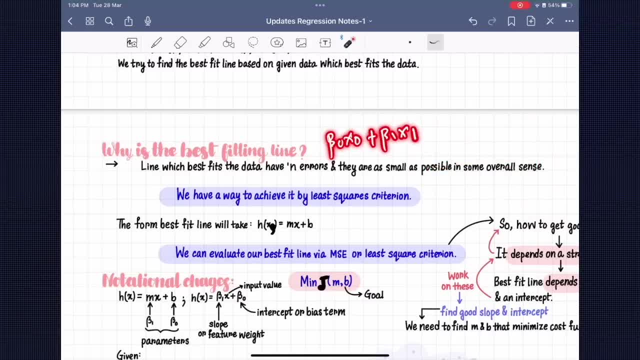 It is beta, So we have beta 0 X 0 plus beta 1 X 1.. Okay, or you can say B X 0 plus M A M X 1, both means the same. So going with the beta 0 X 0 plus beta 1 X 1 by convention X 0 is nothing but equals to 1.. 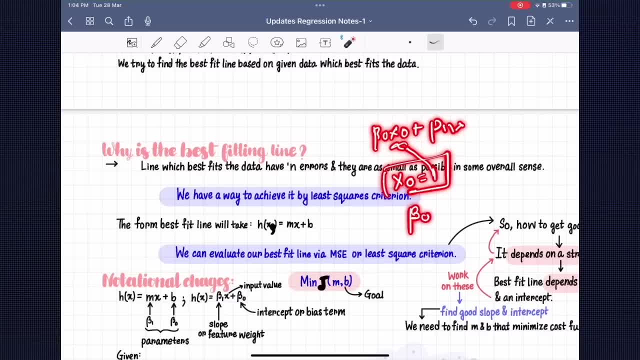 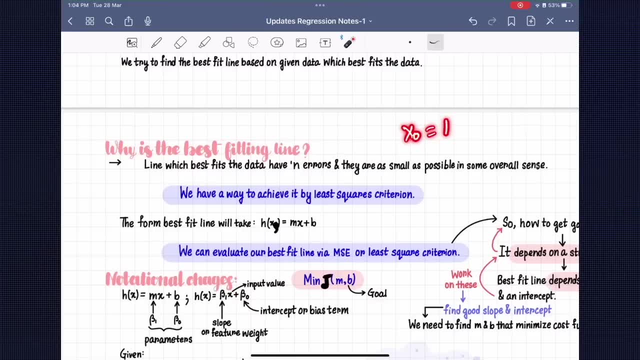 So whenever you multiply anything with 1, it just remains that number, So beta 0.. So that's why we write beta 0 alone, plus beta 1, X 1.. Okay, so we have. so we have X 0 to be equals to 1, right. 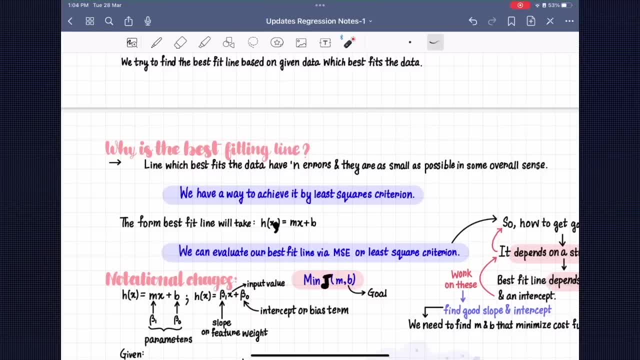 So that's why we don't usually write X- 0.. Okay, So I hope that you understood. Well, it will be more handy when we talk about multiple linear regression. We will finally understand it, But as of now, just keep in mind that we have did the bit of notational change. 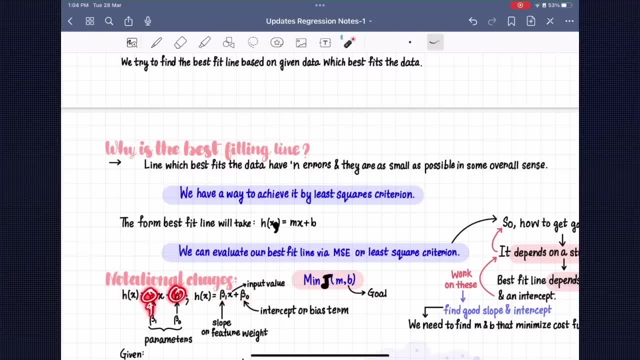 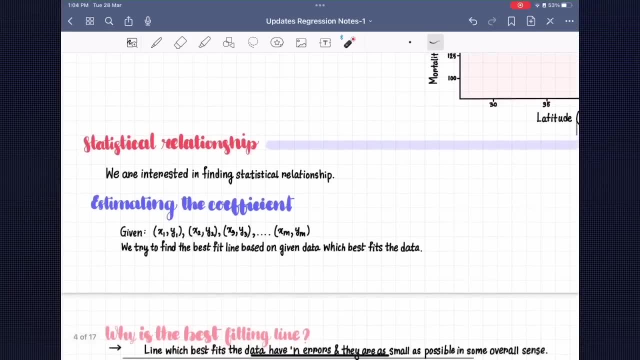 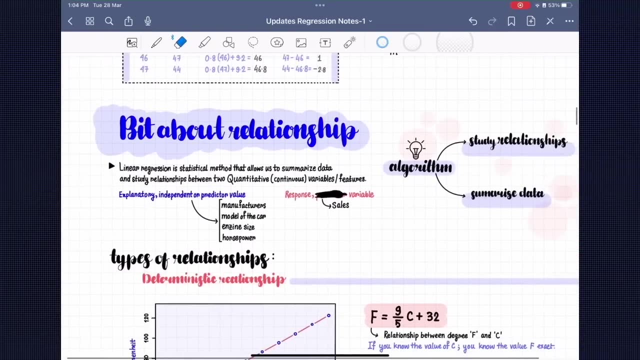 Everything remains the same, Just our notational changes. introduce beta 1 instead of M and beta 0 instead of B. Whole story makes sense. I hope so that you, that that you understood about relationships in detail And now you can. you can easily ignore. there's a direct formula, but I just want you to ignore it. 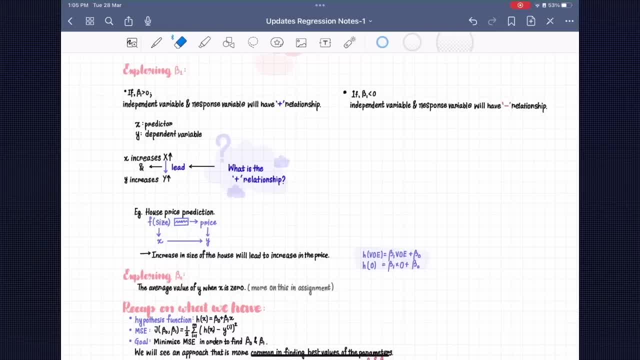 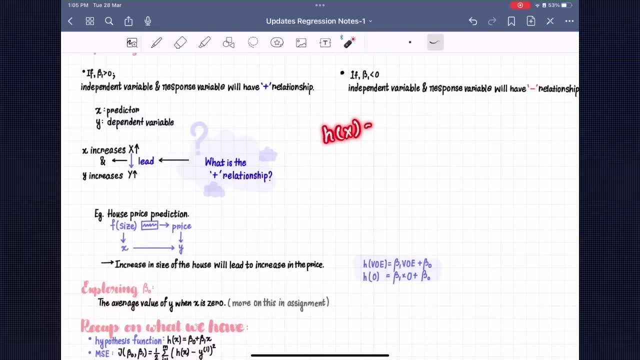 Because I don't want you to focus on that. I hope so that you'll not focus on that. Now, what we'll do, we'll talk about. we'll talk about. So we have an hypothesis: H of X. H of X equals to beta 1 times X, 1 plus beta 0.. 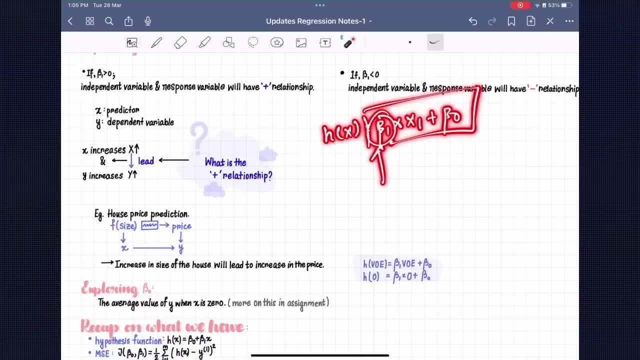 So this is your hypothesis. So what does this beta 1 represents? What does this beta 0 represents In terms of, you know, predict the price of a house given the size. So you're given the size of the house. 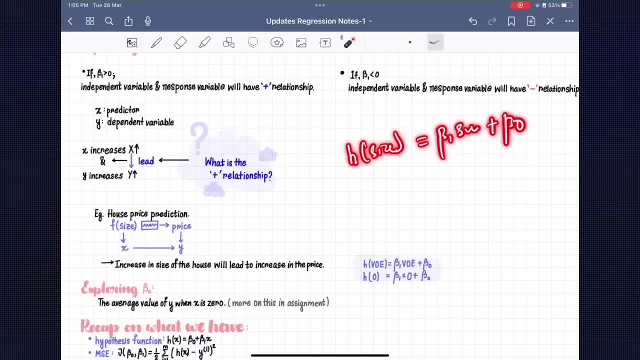 So size as beta: 1 times the size of the house plus beta 0. So what this beta 1 represents. How does this beta 1 affects your output variable? If we introduce beta 1, how does it affect on your output variable? 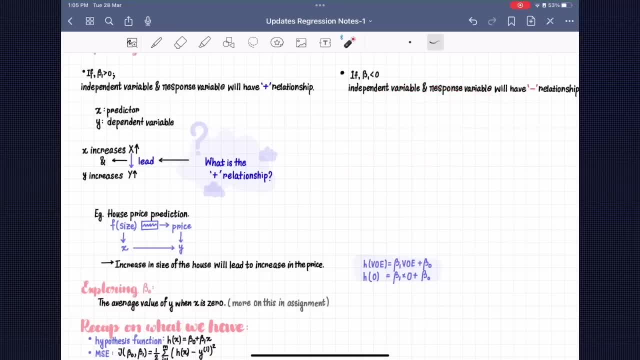 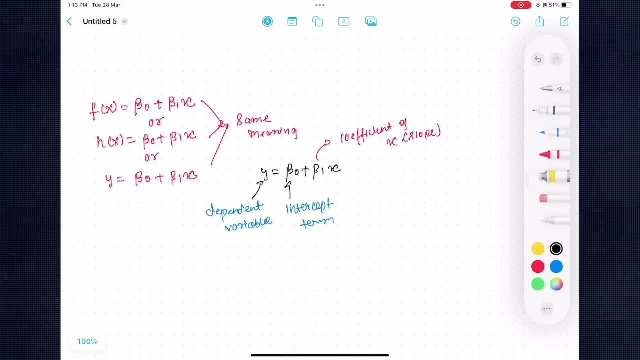 And what is beta 0 effect on your output variable? We'll talk about that later on. So, everyone, we come back to our next section of our video, which is talking about, which is talking about interpretation: interpretation of coefficients, of coefficients parameters. 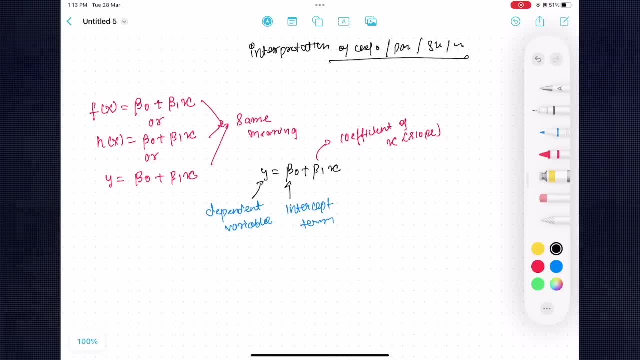 or slope and intercept, Both all mean the same. So usually, just just to make a remark, just to make a remark over here, your F- I sometimes use F of X- is equals to beta 0 plus beta 1.. So, function of, we want to build a function of F that that maps your X to your output variable. 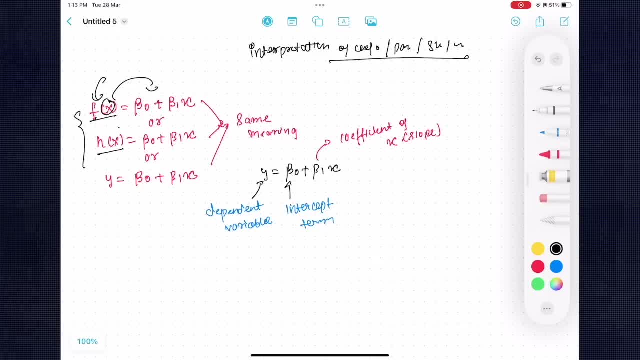 H of X means the same and Y, So they all mean the same. Eventually, at the end you're taking out just an output variable, Y, Right. You're taking on the dependent variable- Right. So all mean the same. 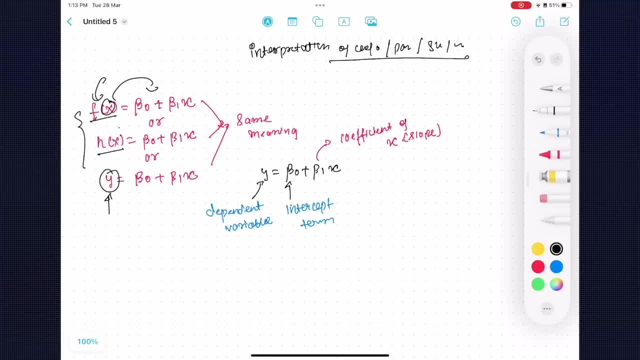 They're used interchangeably, Just to make sure that you're on the same piece. So we are going to use this, this, this particular formula, eventual equation, where we're going to take out Y, which is a dependent, which is a dependent variable. 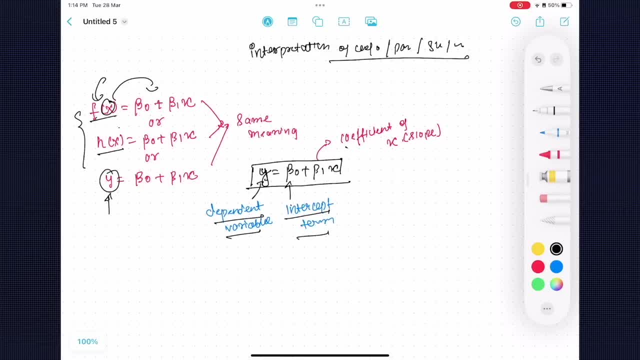 And beta 0 is intercept term, And you have a beta 1 is a coefficient of X, or feature rate of X, or we can say slope, OK, so now, so, now, so, now let's start talking about. so now let's start talking about, about what is. 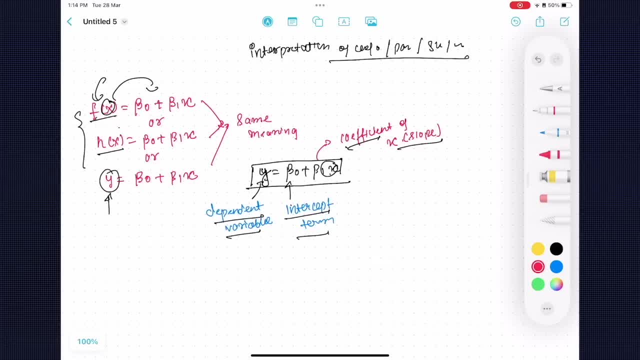 the significance of your beta 0 and beta 1 in terms of problem statements, That that that could make much more sense, that that will make much more sense. So let's get started now. So assume that. so assume that let's start talking about beta 0.. 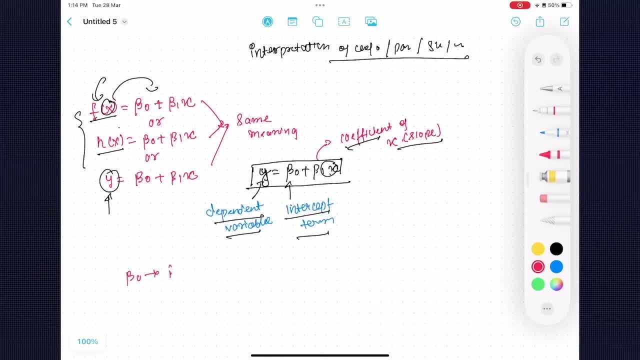 So beta 0 is nothing but called the intercept, the Y intercept, the Y intercept term, the Y intercept term or bias term, Y intercept term and the bias term. So this is what we're going to do. This is what the beta 0 is. 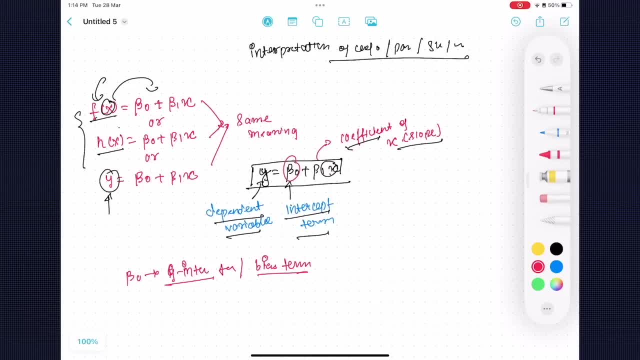 So what does this beta 0 represents? What does this beta 0 affect the output variable? How does it affect the output variable? So beta 0 represents the value of Y when X is equals to 0, when X1 is equals to 0. 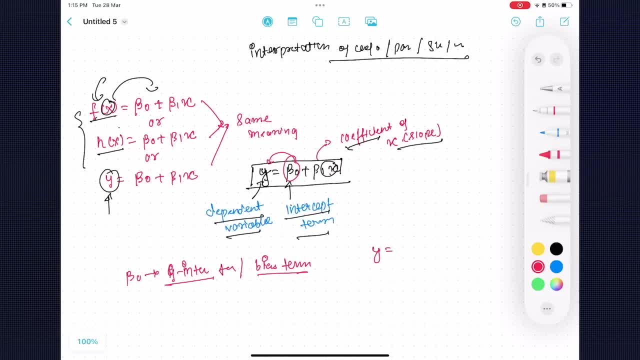 So your beta 0 comes into play when represents the value of Y. Beta 0 represents the value of Y when X is equals to 0. So when 0 multiplied with beta 1, that will be nothing but equal to beta 0 plus 0.. 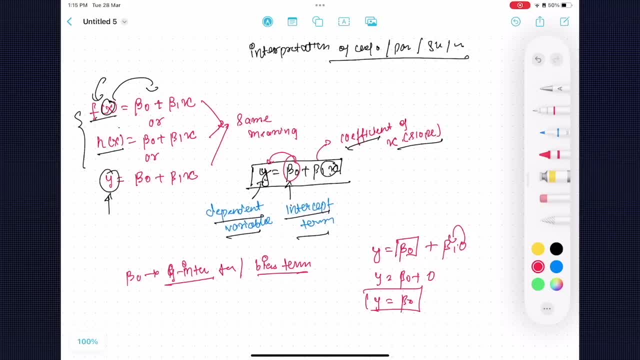 So Y is nothing but equal to beta 0. That's the first scenario. when beta 0 really helps is when X is by chance. when X is not there, when you don't have the information, we just go with the baseline. 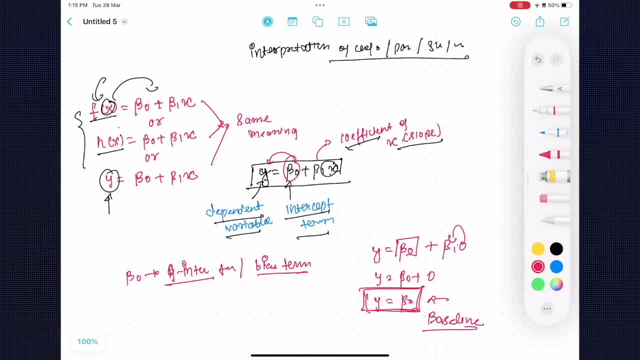 This is what called. this is known as a baseline. This is known as baseline. So when X is equals to 0,, when X is equals to 0, then when X is equals to 0, then your Y is equals to beta 0. 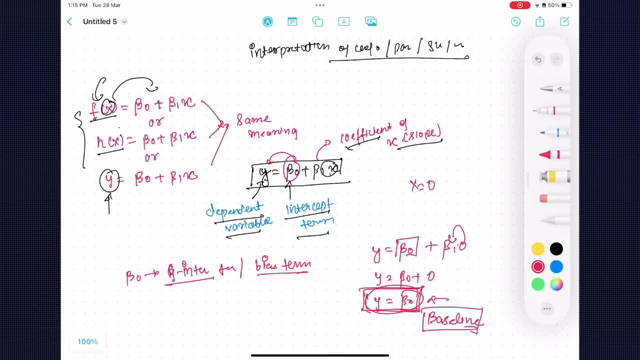 So that, in other words, the intercept of the regression line line with the Y axis, which means this comes into play when X is equals to 0. And it's also the intercept, It's also the intercept, It's also the intercept of the regression line on Y axis. 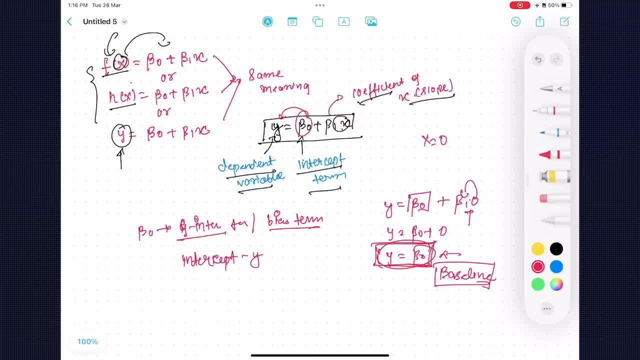 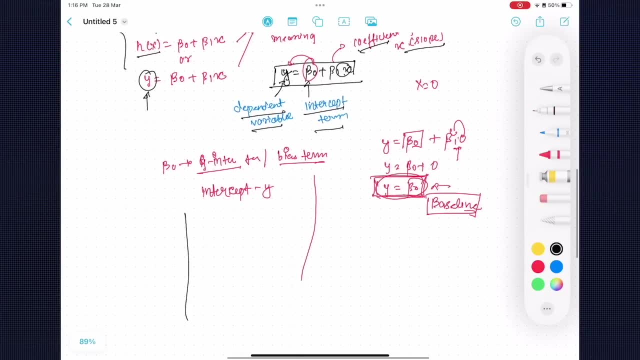 So it's a Y intercept. So if beta 0 is positive, if beta 0 is positive. So let me just make it clear. So if beta 0 is positive, is beta 0 is positive. If beta 0 is positive. 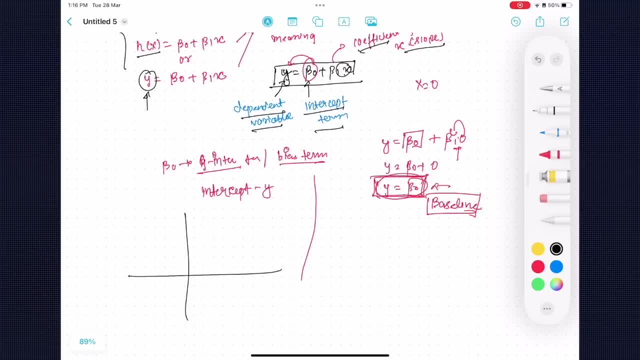 It means that it's. it means that the regression line starts above the Y axis, above the Y axis, which means it's it's above the Y axis, or something like that, But but if it is negative, then it's below the Y axis. 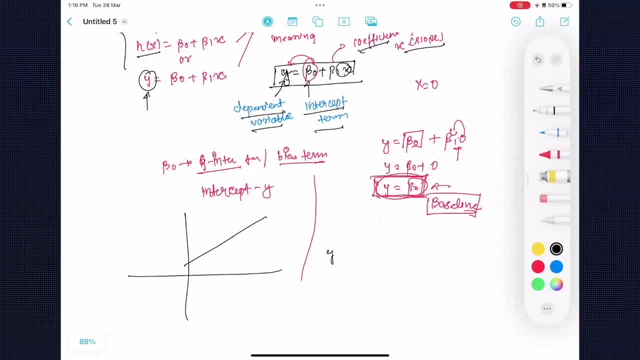 So you know it's. it's like if, if, if, if your intercept is positive, if your intercept is positive, it will stay somewhere over here, But if it's negative, then it will stay somewhere over here, Right? So that's one of the, that's one. 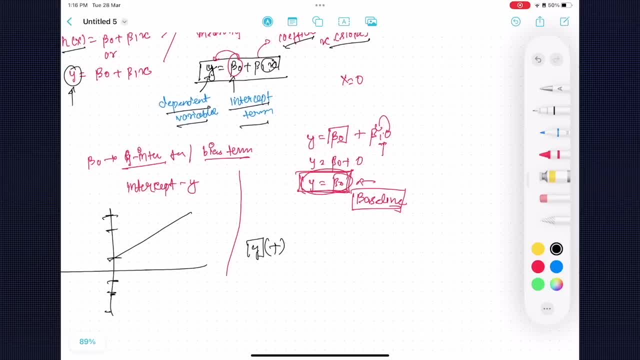 of the property. So let's take an example to make sure that we better understand this. like to what exactly when X equals 0 and all? So suppose, suppose you know. build a simple linear regression model where Y represents the price of a house and X represents the size of the house. 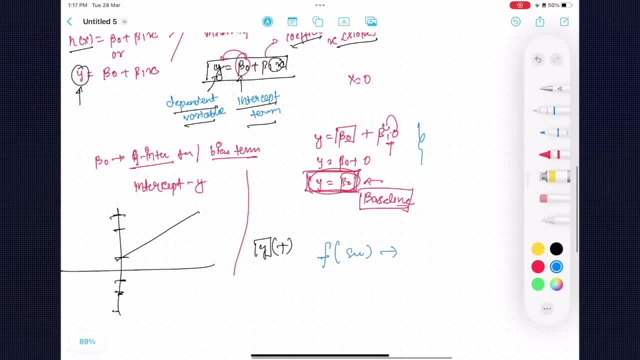 So you know, build a function F that takes the size of the house and and predicts the price of the house. So you know, build a function F right. You know, build a function F that takes the sign and predicts the price. 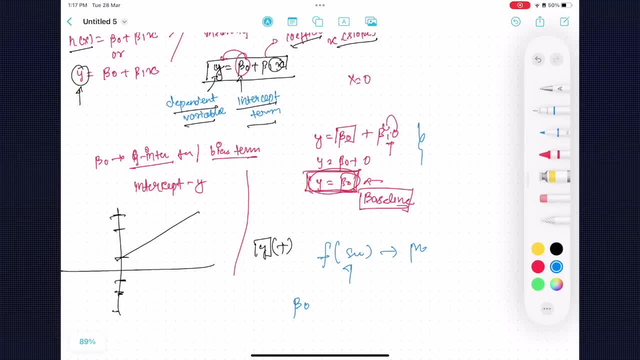 So beta 0, beta 0 would be the price of the house. So this equation will be more or less Beta 0 plus beta 1 X 1.. So beta 0 would be the price of the house. will be the price of the house when X is X is equal to 0. 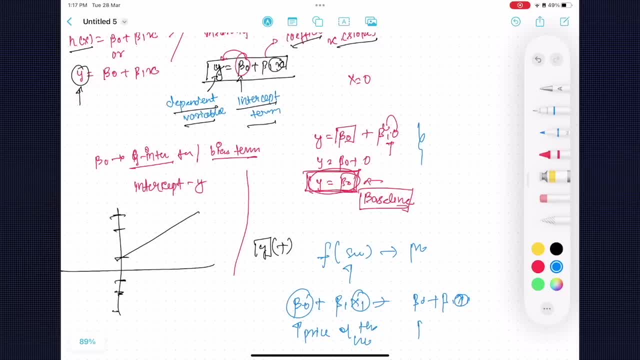 So beta 0 plus beta 1 X 0, which is this is beta 0, is 0 multiplies The beta 1 is also, of course, 0. So beta 0 would be the price of a particular house. 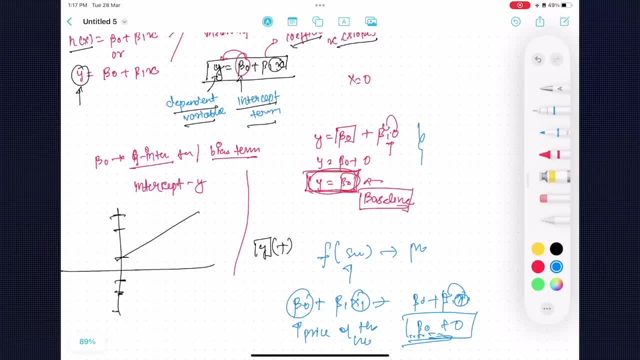 When price a particular house, when, when, when the size of, when the size of the house is 0 and the size of the house is 0 or nothing, OK, That's when the beta 0 comes into play. That's when the beta 0 comes into play. 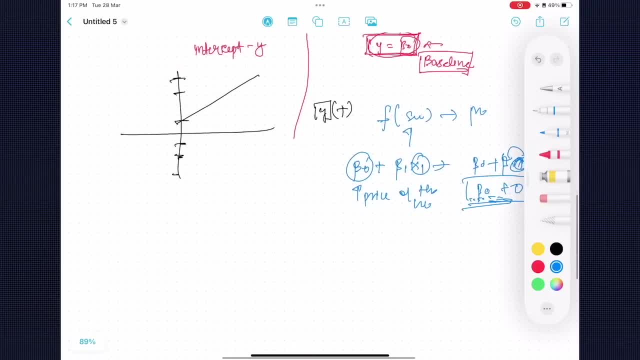 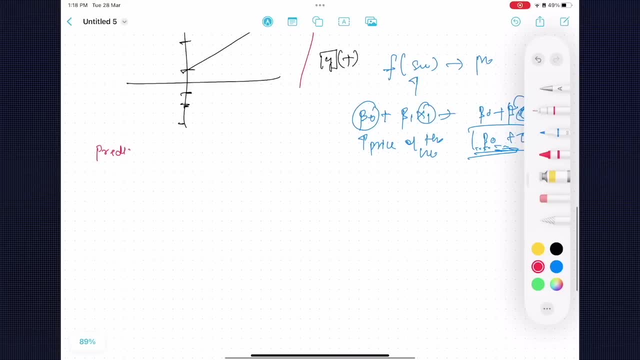 So let's take a very simple example. Let's take a very simple example to make you understand one more thing. So assume that they that that that you know, predict. the application is predicting Exam scores, exam scores, predicting exam scores. So to build a function F that takes in the number of hours you study, 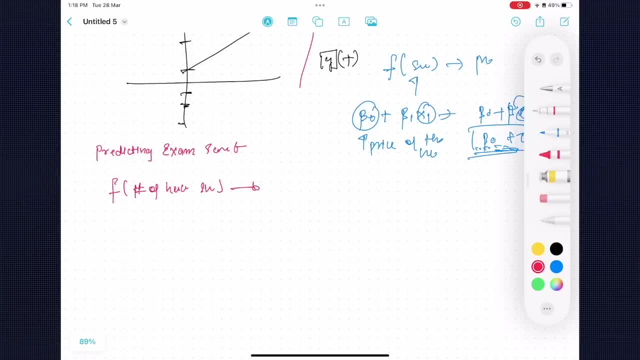 number of hours to study, number of hours to study and predicts the exam, predicts the exam scores of that particular child. So that's that's the basic. that's the basic function And you and you build, and you build a function. We'll talk about how we come up with this M and B later on. 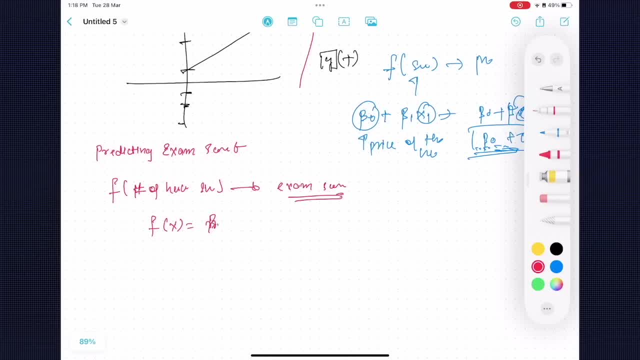 But you build the function F of X, which is nothing but equals to beta 0 plus beta 1 X. So F of X- number of hours study- which is equals to assume that your beta 0 is 60 plus plus beta 1 is 5 and X. 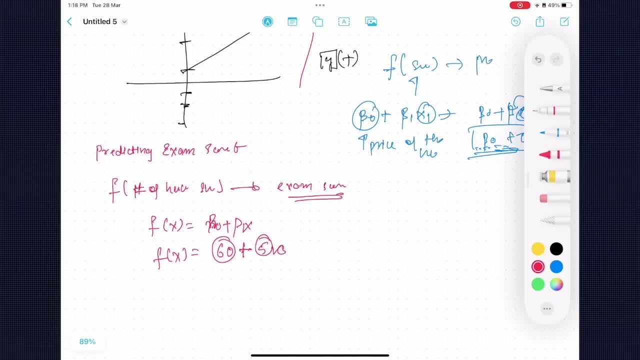 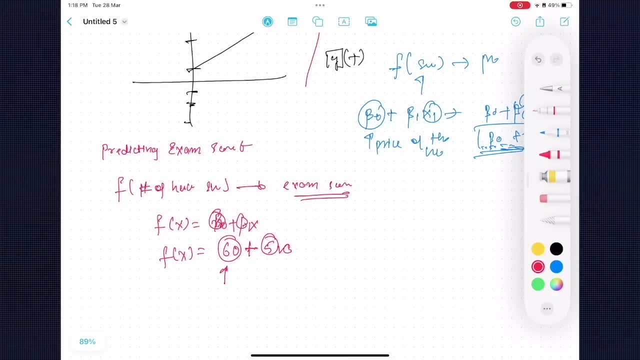 So you have just taken that number. You're just taking that number. for example, we'll talk about how can we take out this beta 0, beta 1 later on, but just assume that you're taking the random one. So over here, over here, your intercept term. 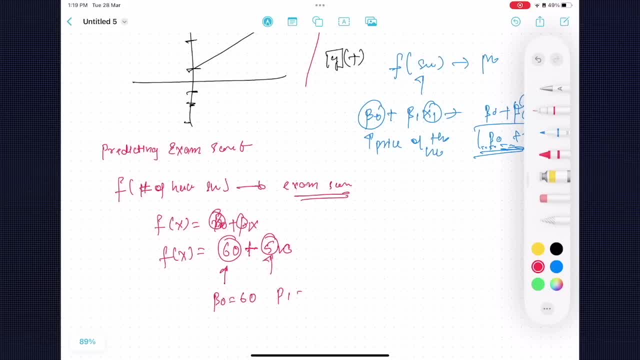 your intercept term is nothing but 60, and your and your coefficient is nothing but the 5, as is this 5.. So so your beta 0 is 60. This means that if, if this, truly if the, if the student haven't studied anything. 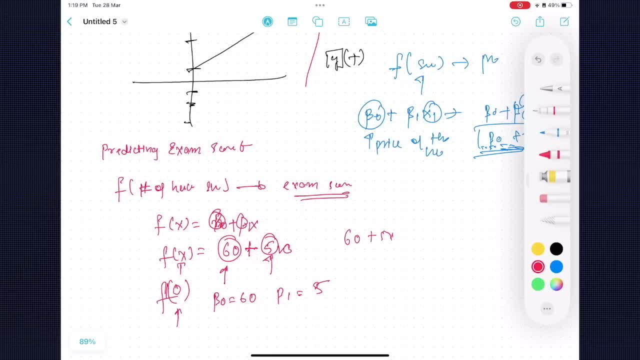 if the student haven't studied anything, which means because 0, 60 plus 5 times 0 is nothing but 60. So if student has not studied anything at all, which is that is equals to 0, the predicted exam score would be nothing but 60, would be nothing but 60,. 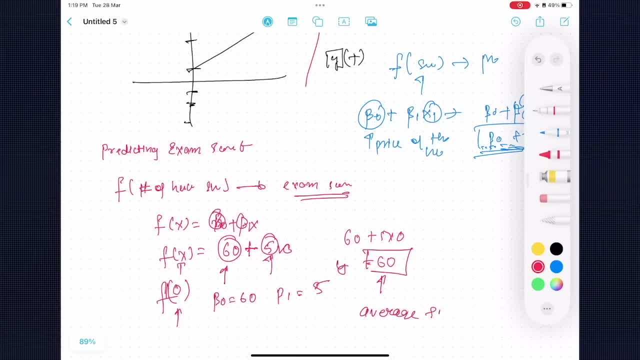 which represents the average, which which is nothing but the average score, which is nothing but average scores of students who do not study, who don't don't study. So 60 is nothing but the average score of the students who don't say that it's a bit. 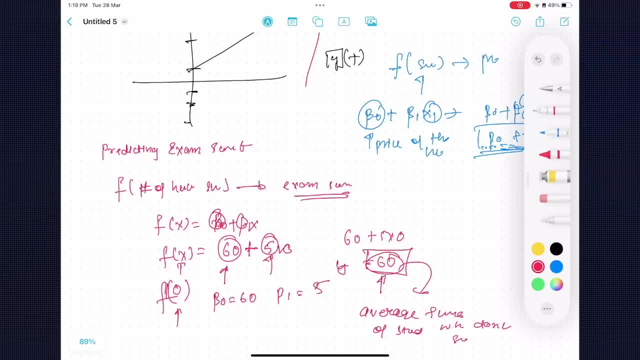 higher, but that's what the beta 0 represent. So that's the situation when your X0 is nothing but equals to X, X1 is nothing but equals to 0, which means that that in this example, the person has not studied at all. or in the previous example, 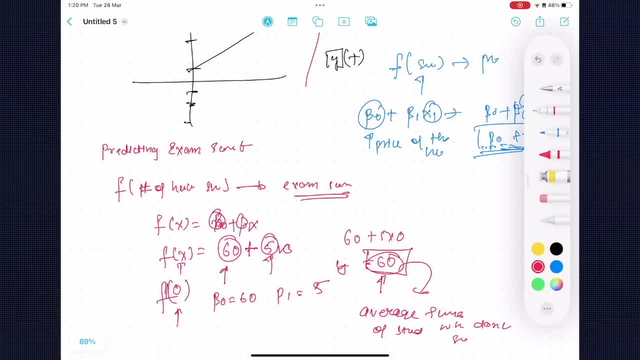 the size of the house is zero, which was the average of the size. average a house of the price, when size of the house is zero. OK, I hope that you understood what exactly this beta 0 means. If this beta 0 means, and it. 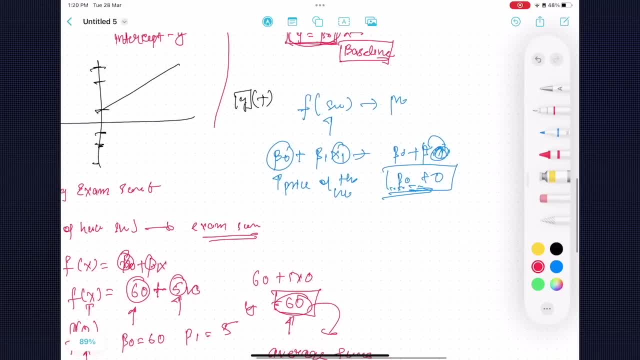 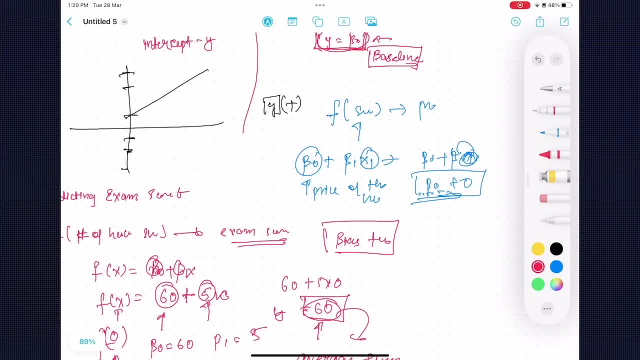 yeah it, it makes sense. OK, so sometimes beta 0 really does not make sense, but it acts as a biased term. but it acts as a biased term, the average term. That's why we call this as a bias as well. 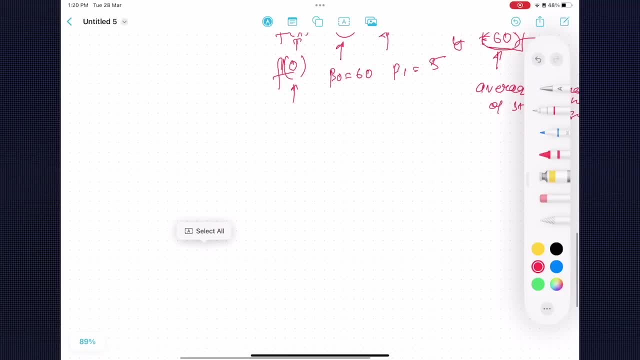 OK, cool, So we have studied about beta 0. Now let's talk about beta 1.. Now, now let's talk about beta 1.. Let's talk about beta 1 in very detail. So beta 1.. So beta 0 represents the when X is 0, but beta 1 is the coefficient of X, right? 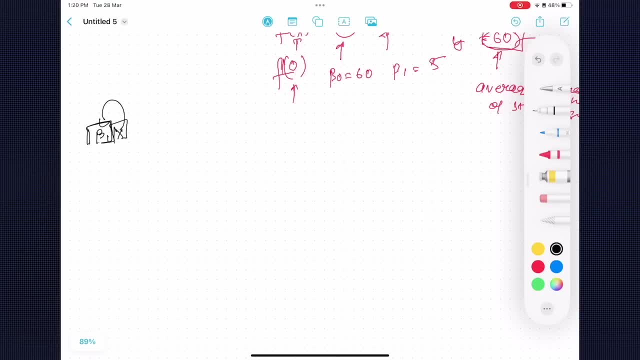 The coefficient of X. So we are multiplying X with something, beta 1.. That means it represents that how this beta 1 will affect this output variable, Y. So it says that it is the beta 1 represents the change in Y for one unit increase in X. 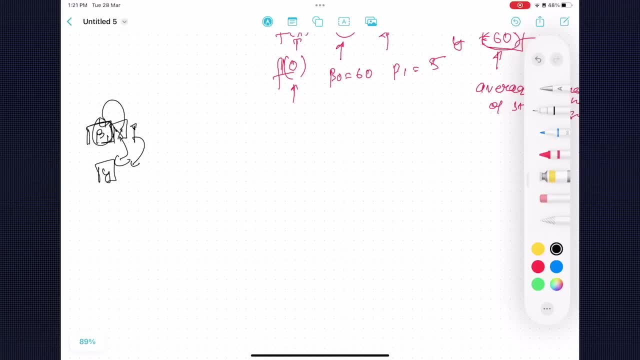 So if X increases by one unit, what will be the change in Y? That's what the beta 1 represents. That's what the beta 1 represents. Beta 1 represents what? The change in X, The change in X, The change in X. 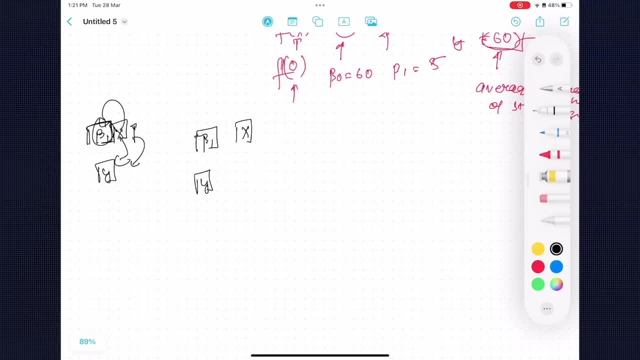 The change in Y. How much Y will change if we increase X by one unit? Let's take a very simple example. Let's take a very simple example to make you understand about this. For example, if we have a simple linear regression model where Y represents 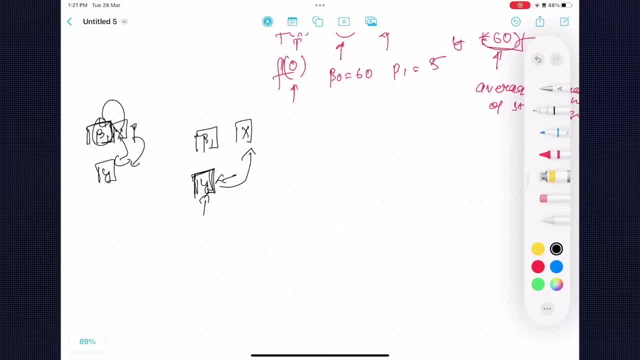 where your particular Y represents the number of hours of sleep a person gets. OK, the number of hours. So you're going to build a function F. you're going to build a function F, that you're going to build a function F, you're going to build a function F. 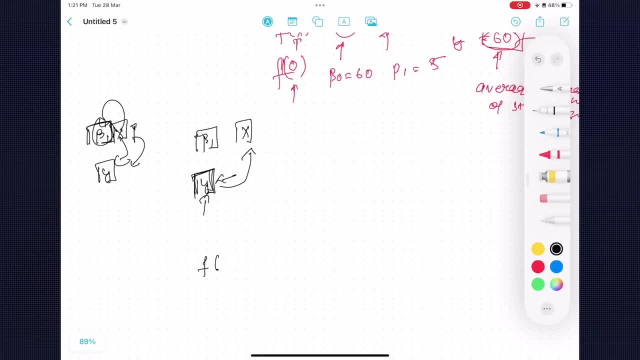 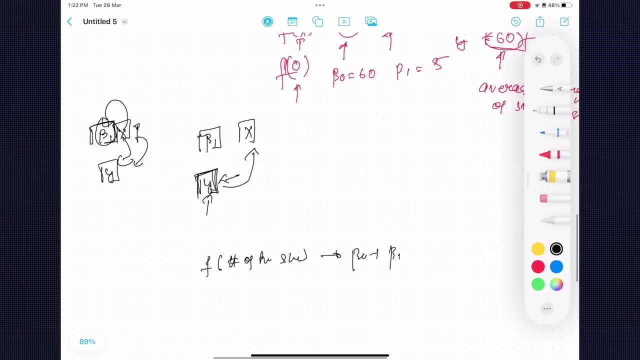 So let me just clear this. So over here we build a linear regression where you're going to predict the number of hours a person will sleep, the number of hours a person will sleep, the number of hours the person given, given that, then, given beta 0 plus beta 1, the number of coffee cups. 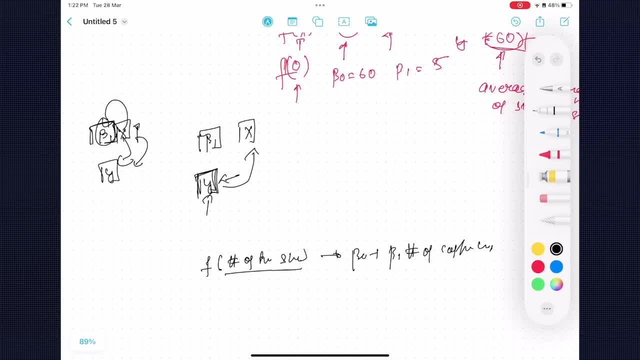 the number of coffee cups, right? The problem statement is: you're going to predict the number of hours the person will sleep, given how many number of coffee cups he has drank. OK, that's the function which you know me. So, if you have a simple linear regression model where Y represents the number, 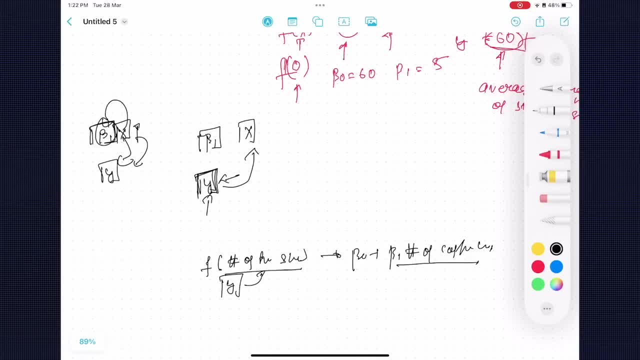 of hours. Y represents the number of hours a particular man sleep, where Y represents the number of hours sleep a person gets and X represents your. X is nothing but the number of coffee cups a person had. right, Then the beta 1 represents. 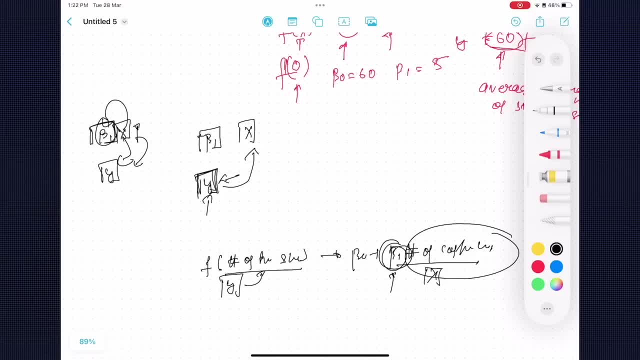 what this beta 1 tells. beta 1 represents the change in hours of sleep for one cup increase in a coffee consumption. So if we increase the coffee consumption by one hour, what will be the change in number of hours of sleep of a particular person? 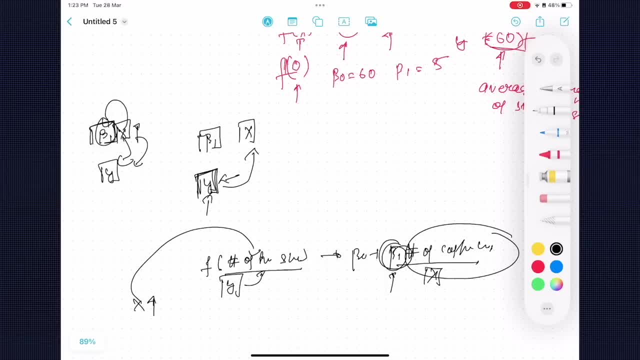 OK, I hope that you're understanding Over here. the number of coffee cups. assume that number of. if we increased, if we drank one more coffee, what will be the effect on this output variable? That's what beta 1 says about it. 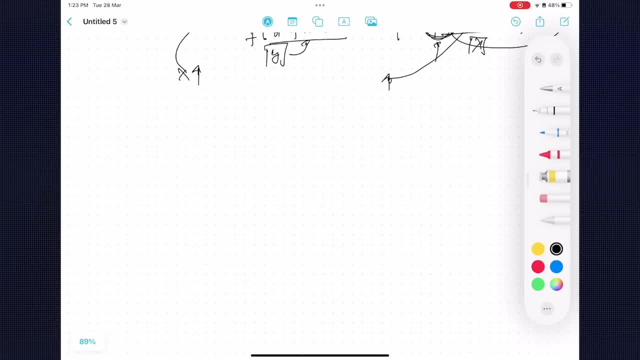 That's what beta 1 says. It's about it. Let's take a look at the previous example, which which we had. So the example was the predicting salvage exam scores. we had to build a function, F, that dates in the number of study hours a particular person predicts. 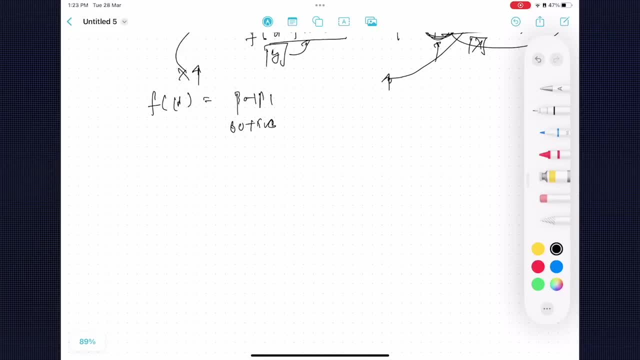 So beta 0 plus beta 1 X, 60 plus 5 X. So now we have now- now we don't have- X equals to 0.. Now we don't have that. that, that This is for the beta 0.. 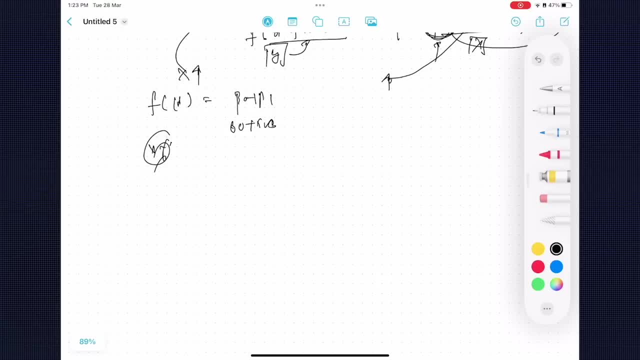 But now assume that. assume that what this is beta 1 tells over here. beta 1 tells that for every additional hour of a study, if we increase an X by one, or which is one unit, which is every additional hour of study- X increases by one. 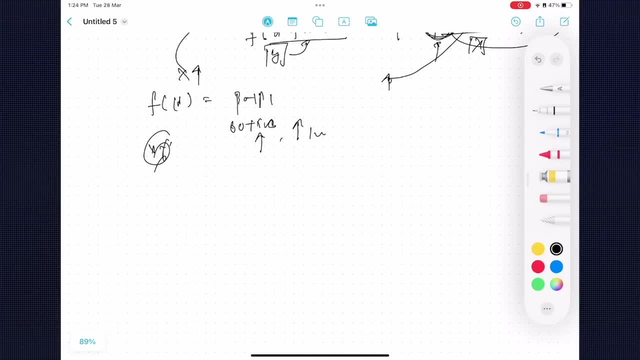 the predicted exam score also increases by five, increases by five. So this, this five, represents the rate of change in Y, which is the exam score. the rate of change in exam score. what will the change in exam score, given the, given this, one unit increase in X? one unit, one unit increase, one additional hour of study. 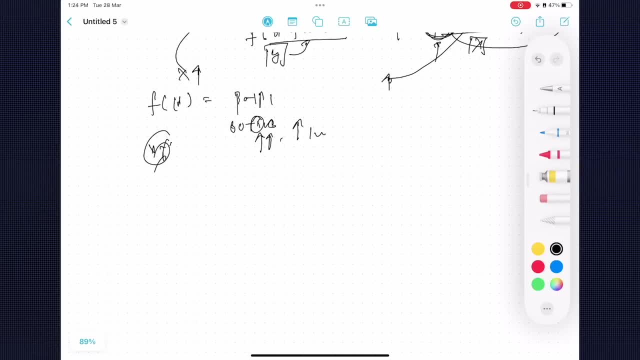 So, in this case, for every additional hour of study, which is X increases by one, the predicted exam score increases by five. increases by five. This is the rate of change in Y. change in Y with respect to change in X By one unit. increase in X with respect to X. 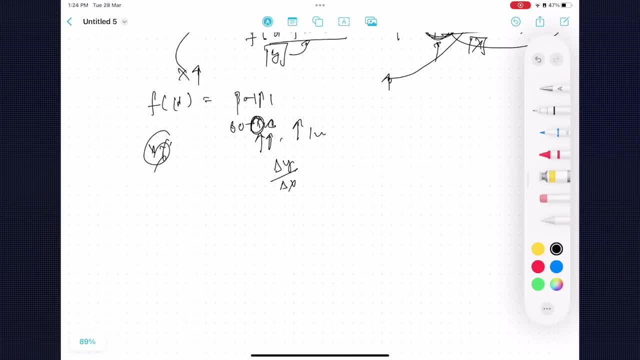 Okay, So assume that if a student studied, if a student studied three hours, so now F of three, which is nothing but 60 plus 5 times 3,, which is 60 plus 5 times 3,, which is 15.. 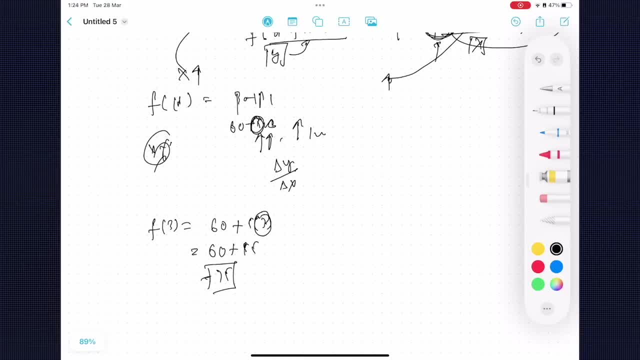 Which is 75,, which is 75. So a student has studied three units, three. three hours extra, three hours additional hours, so three times five. so it will increase by 15 times. The baseline will be increased by 15 times. 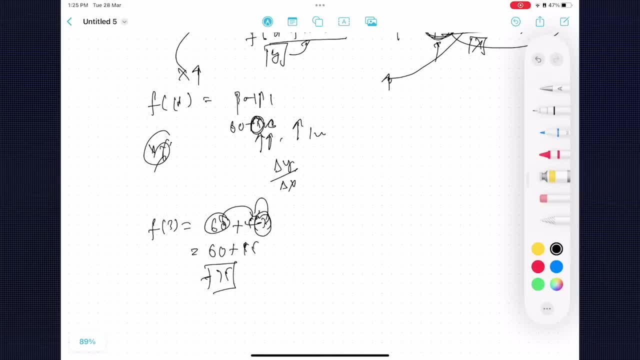 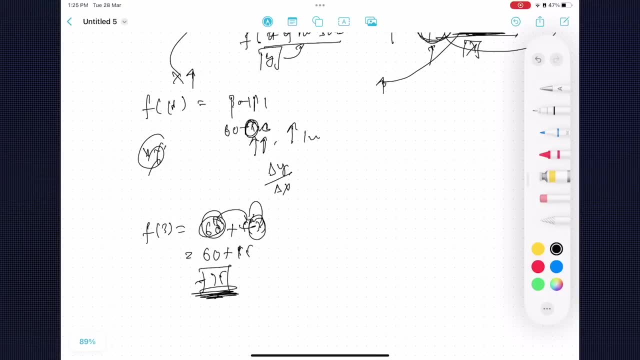 So we can study. if a student has studied for three hours, the predicted exam score will be 75, which is 15 points higher than the baseline if the student has not studied at all, Which means that the that does the. if your X is was three, then there is, then there is an increase in X. 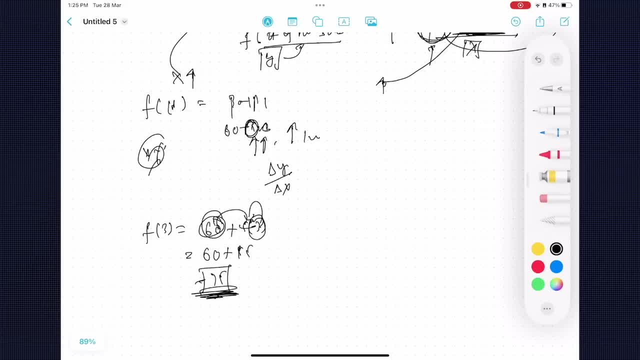 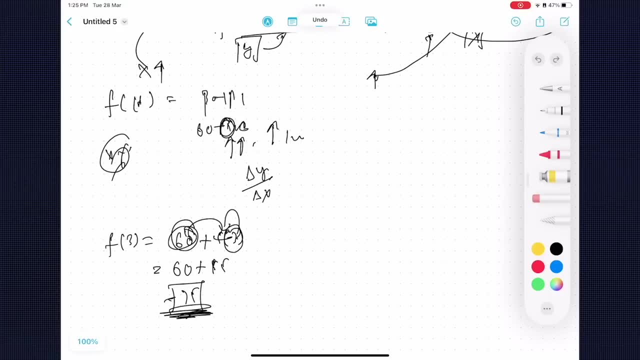 Okay, Then then, if, for every additional hour, every additional hour, the his or her score increases by five, You can see clearly that, how this, how this five, is affecting your output variable, how this five is affecting your output, how this five is affecting your output. 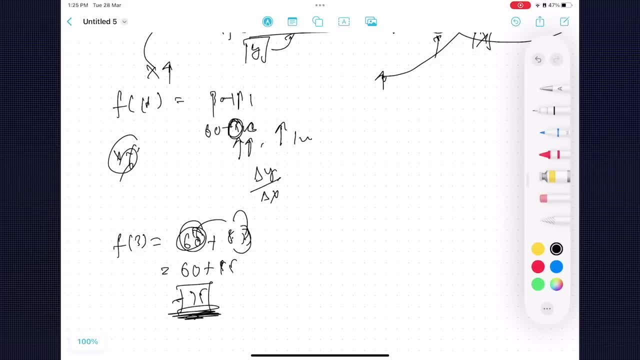 variable, how this five is affecting your output variable. oops, Five, five is affecting the output variable out there. I hope that it makes sense to you as well. Okay, cool, Sometimes- currently it was positive, but sometimes you have negative as well. 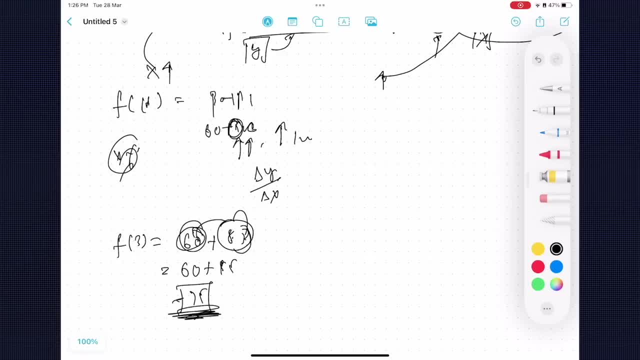 Sometimes you have negative as well. Okay, sometimes you'll get negative scores as well. So let's talk about negativity as well, which will make much more sense, And I'll give you a sheet where we have much more examples of interpretation. that will make much more sense as well. 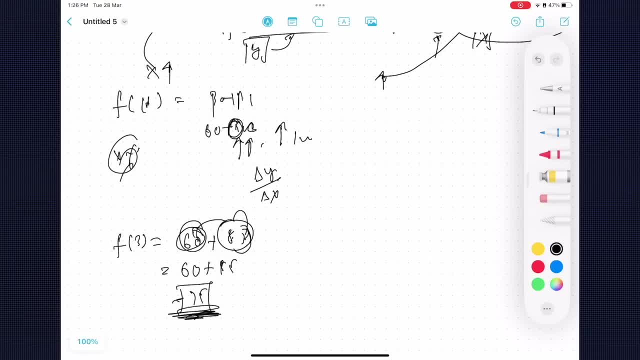 Right, so assume that if you have a linear regression model where y represents the number of R study and x represents the age of a student, okay, So you're going to predict the number of hours a particular student will study, given the age of a student. 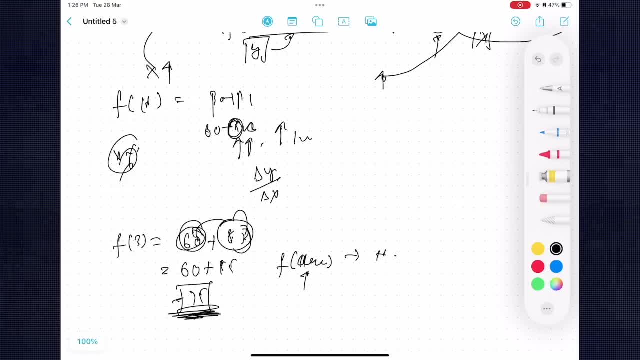 So you're going to give the age of a person and predict the number of hours a student will study. You're going to give it like higher the age, higher the study, and the coefficient for x is minus 2.. So you have got beta 0 plus beta 1 x. 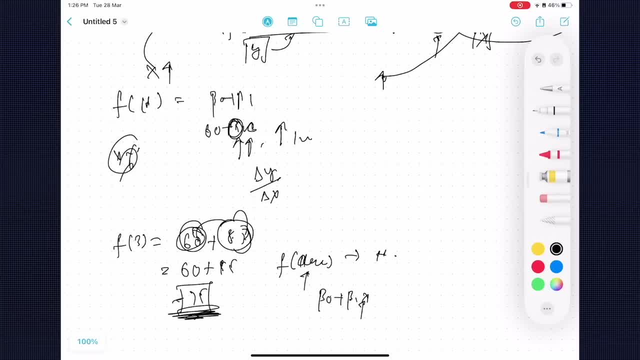 and x over here is the age of a person, right? So if your beta 1 is nothing but minus 2, which means it's different. So what does this indicate? This means that every one year increase in x, so x is nothing but age, right. 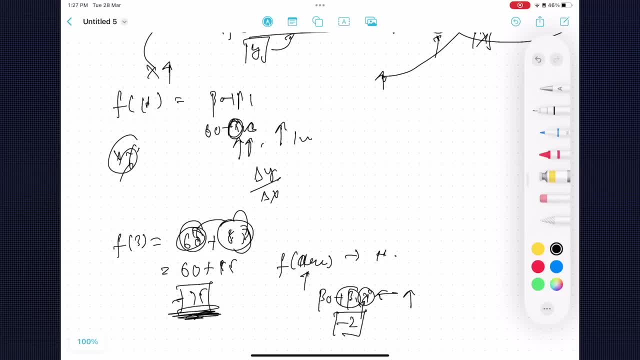 So every one year increase in x. the predicted number of hours of a study decreases by 2.. You can see our misconception was that higher the age, higher the study hours. But over here it decreases. So minus 2 represents. so if your beta is positive, 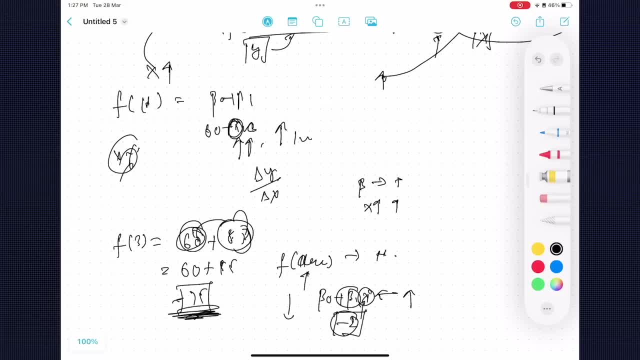 this means if x increases, then beta also increases. In this case of predicting exam scores, if the study hours increases, then the exam was positive because the beta was positive. But in this case, if beta is negative, my beta 1 is negative. 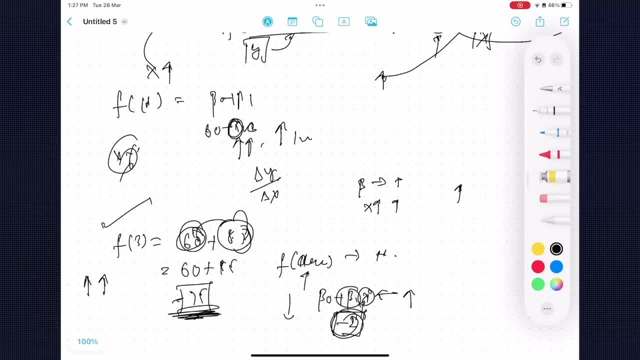 which is minus 2, which means for every additional hour. if x increases- sorry, if beta 1, sorry. if x increases- your output value decreases. Okay, If x increases, output value increases, But in this case, if x increases. 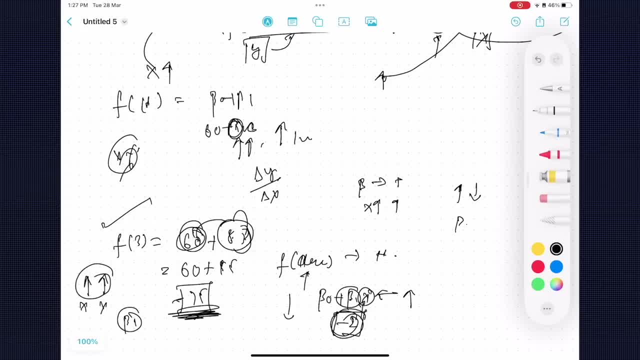 output value also increases When beta 1 is positive, But in this case, when beta 1 is negative, when x increases, output decreases. One such example was that in this case, beta 1 is minus 2, which means for every one year increase in age. 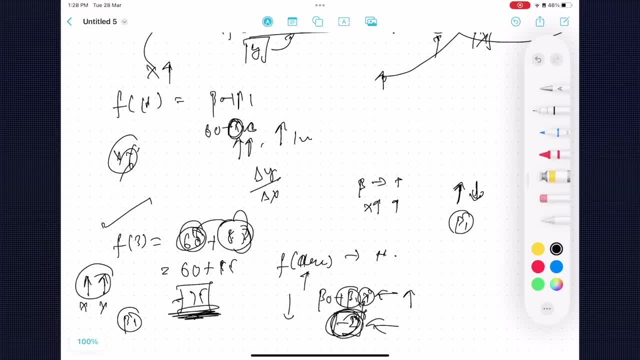 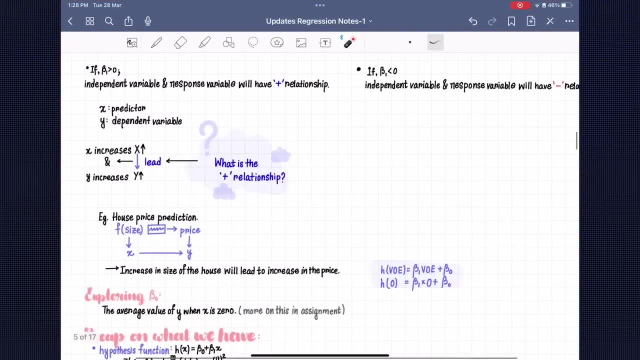 the predicted number of the study will decrease by this factor, which is minus 2.. Okay, I hope that this makes sense. So we have studied, we have written over there here as well, here as well, that if there is a 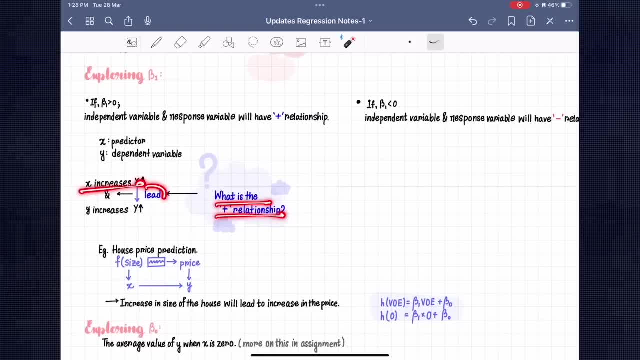 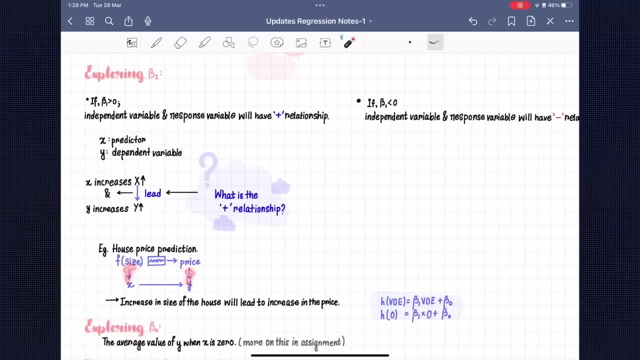 if there is a positive relationship. if there is a positive relationship, if x increases leads to y increase as well, As well. Okay, So you can see increase in size also also increase in price. So I hope that this gives a good sense. 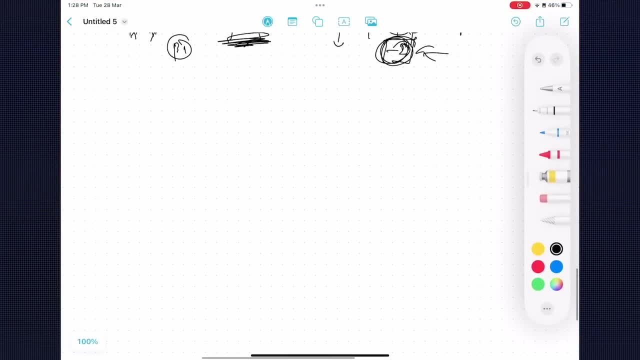 about. whatever we are talking about. I'll take one more example, maybe to make you understand in much more detail, so that we are on a good page. Okay, So what exactly? what I want to do is take an example of predicting sales. 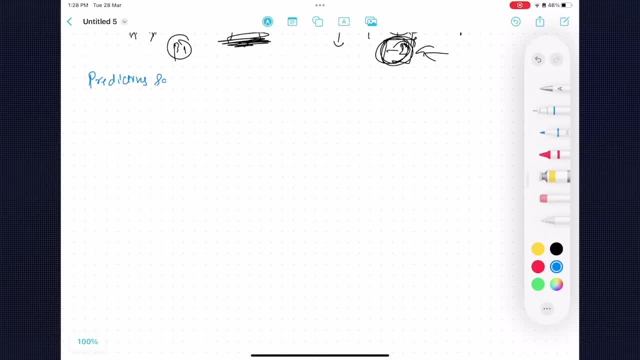 You know, take an example of predicting, take an example of predicting sales, And this is this is a nice example to start talking on. So suppose you have a data set that contains information on advertising expenses and the sales of a company. So 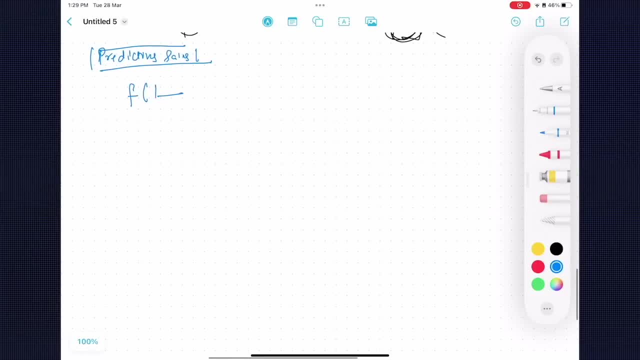 so you're going to make a function f, you're going to make a function f that you're going to predict the advertising expenses. you know predict the revenue. you know predict the revenue, the sales of a person, based on the like. 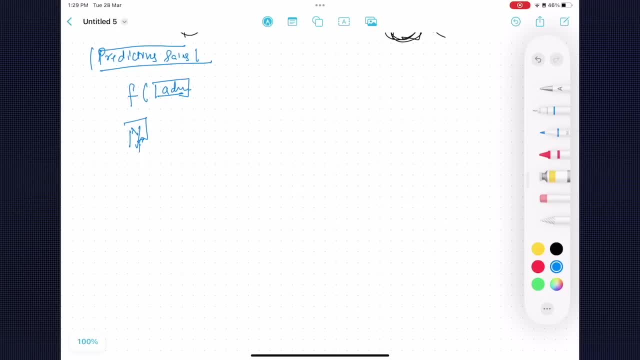 you know, give the advertising expenses, like how much you spend, how much you spend on advertising and predict what. And you're going to predict y, which is the sales. You know, establish a relationship between advertising expenses and the sales. Advertising expenses means: 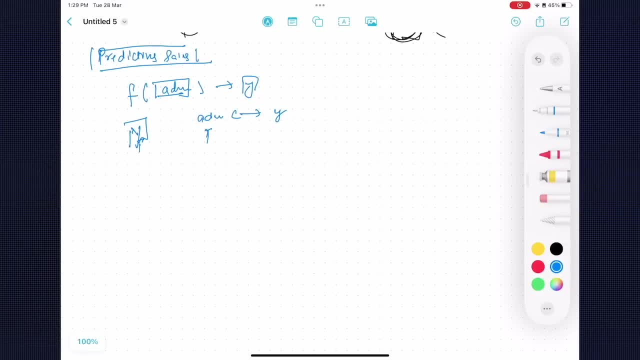 the money you spent on advertising of a company. Okay, So you have only one feature, x, and you're going to predict y. You're going to predict y, So your f of x will be nothing, but x is because of advertising expenses, which is equal to beta 0 plus beta 1, x. 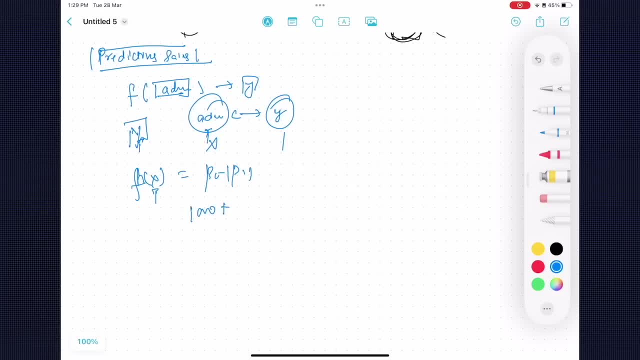 So assume that your beta 0 is nothing but 1000, plus beta 1, which is 0.8 x, 0.8 x. So what does this mean? What does this signify? So this signify that your beta 0 is 1000.. 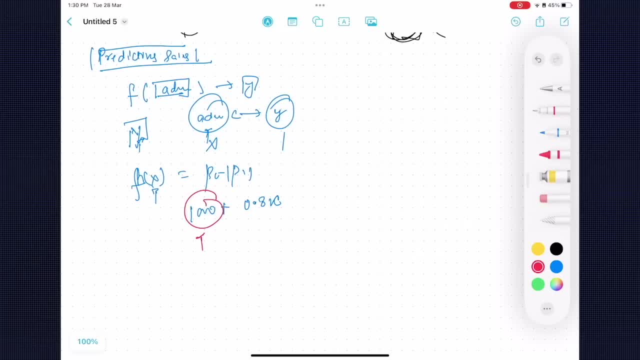 Beta 0 is 1000.. What does this mean? Beta 0 is 1000.. If the company does not spend any money on sales. if the company does not spend any money on sales, which means x equals to 0,. 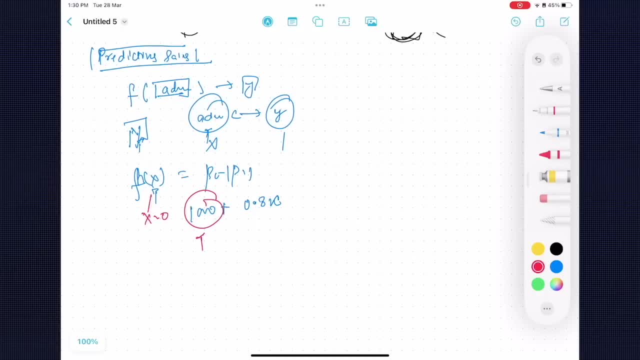 your sales with the revenue, the revenue, the sales revenue would be 1000.. Which is the average, which is the baseline, when your baseline of y, which represents the average revenue of company when they do not spend without any advertising. Okay, 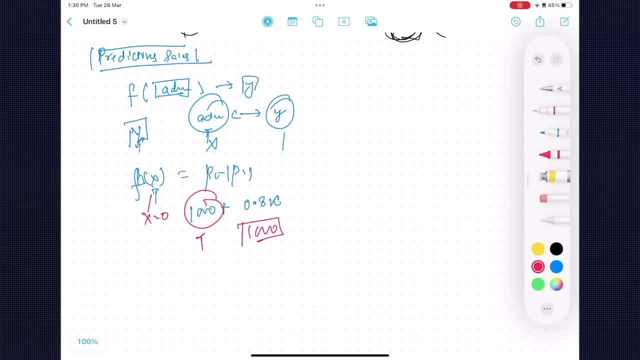 let's be touch the rope. But what about beta 1?? But what about beta 1?? Beta 1 over here is 0.8.. So this says that for every additional dollar we spend, for every additional dollar dollar ways we spend, 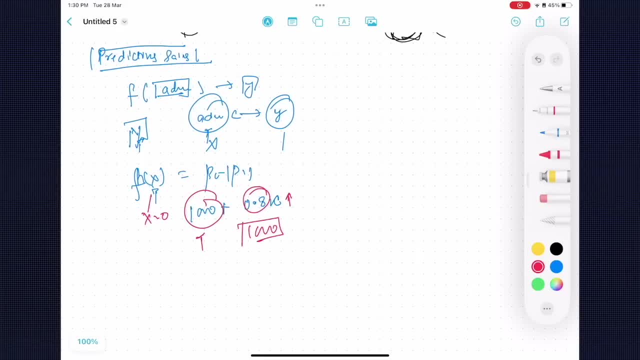 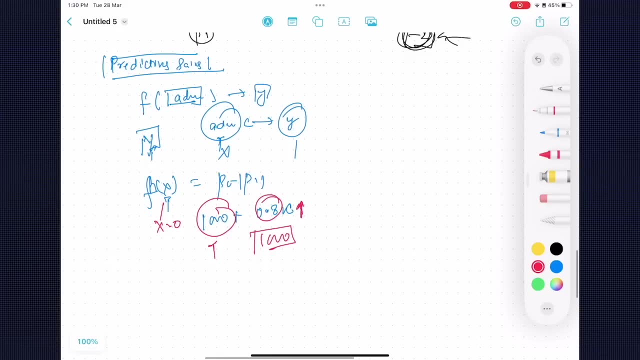 which is a one inch increase in x will lead to increase the door, will lead to the sales Revenue increased by $0.8.. So if increase $1 on revenue, then 0.8, then we'll all will get a raise of $0.8 in revenue. 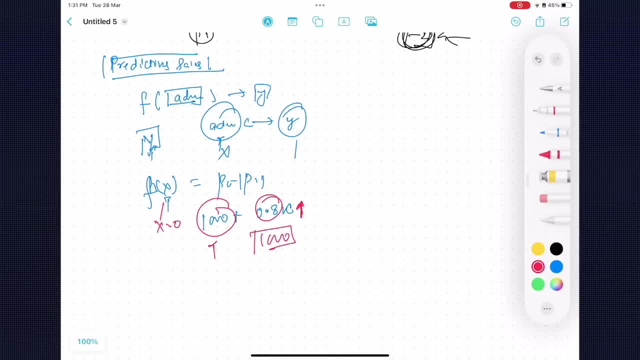 So this is a rate of change. So this is a positive relationship. So it's based the, the, the, the, the advertising. uh, revenues increases, Uh, then the sales also increases. Okay, So assume that your company spends $5,000 on advertising. 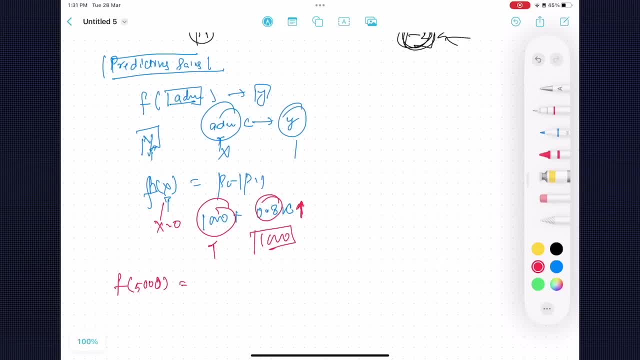 So you're F, F, 5,000.. Okay, This is goes to beta zero: 1,000, less 0.8, 5,000.. So this is nothing but your, your, your total answer would be your total. 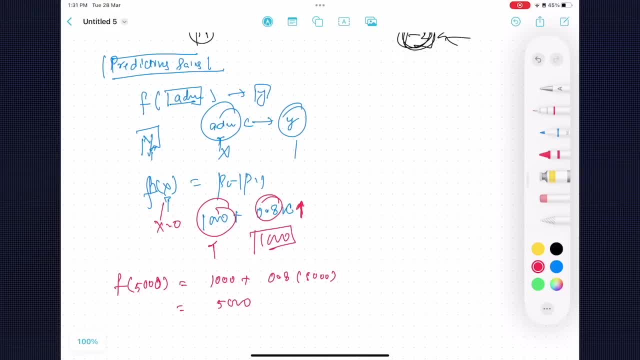 So your total answer would be 5,000, which is 5,000.. So your total, uh, your, your, your. your answer would be- let me just calculate it So it will much worse: 1,000 plus 0.8 times 5,000, 5,000,. 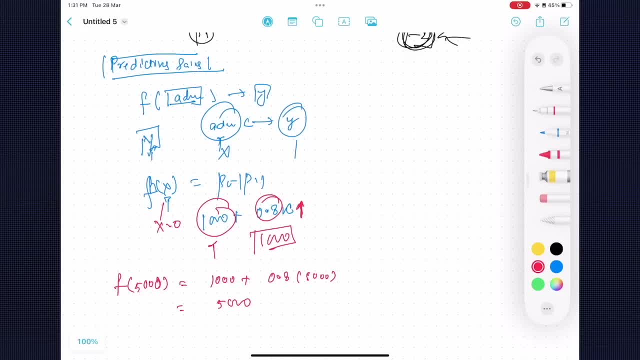 which is nothing but 5,000, thousand dollar, is the five, five, five thousand which would would be the sales. so, basically, if your company has spent five thousand dollar on advertising, the predicted, the predicted sales or the revenue would be five thousand, which is four thousand higher, with the five thousand would be. 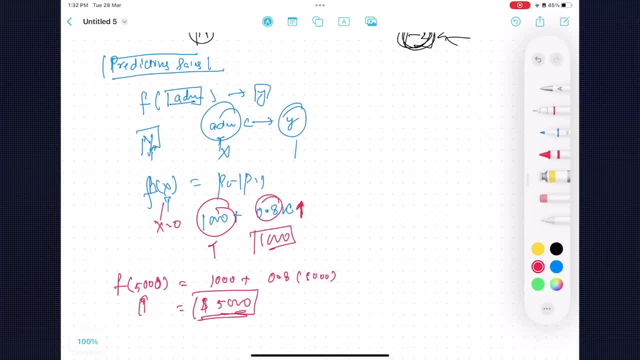 the final sales, if you, if you spend five, five thousand dollar, the five, five thousand on advertising, which means that there's a four thousand higher, four thousand higher than the baseline revenue. so this is four thousand higher than the baseline revenue, right? so this is a positive, positive guy. so it says that for every increase in, for every, for every one of increase, 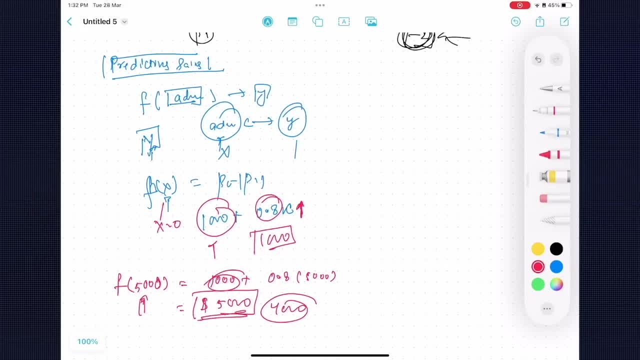 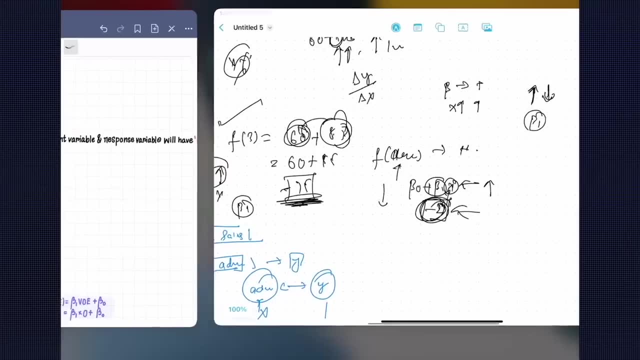 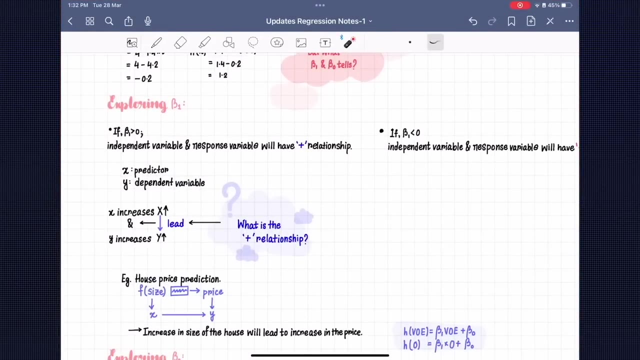 in the advertise. for every one dollar increase in the advertising, your revenue will increase by 0.8 dollars. i hope that this makes sense. now i'm not going to talk more in that. uh. well, you, i've given you an enough example for you to explore by your own. uh, i hope that this really helped. i'll be catching up in the. 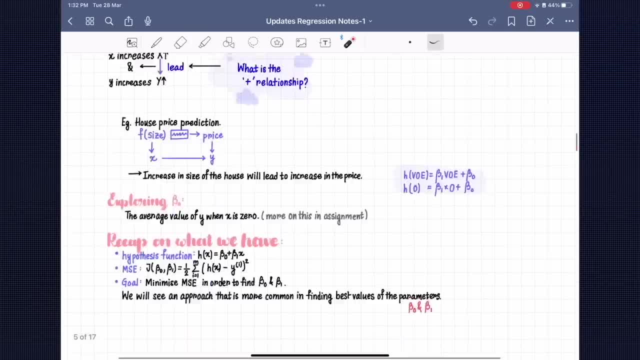 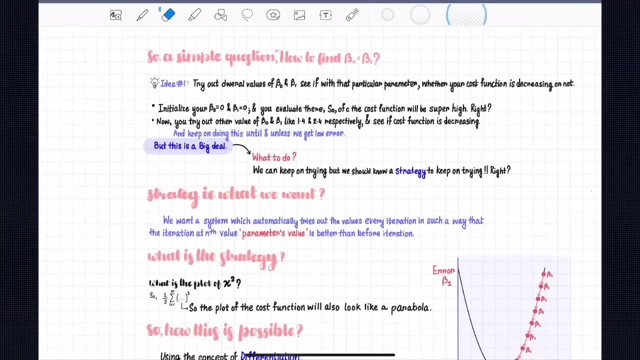 next lecture. then we'll talk about how can we estimate our x, how can we estimate our beta zero and beta one in 3d. let's get started in the next lecture. hey, everyone, welcome back to this lecture. in this particular lecture, what exactly we are going to cover is- uh, we'll just recapitulate. 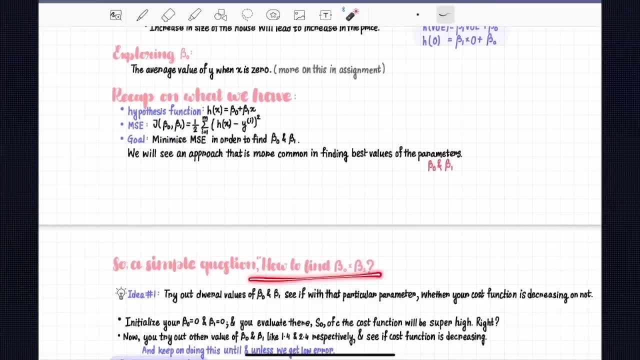 whatever we have learned, and then we'll talk about how can we find beta zero and beta one in the in. like our whole, you know, discussion is: uh, if we don't have better beta, beta zero and beta one will be not getting our best fit line. eventually we'll be failing to get the good predictions. so that was one of our, one of our. 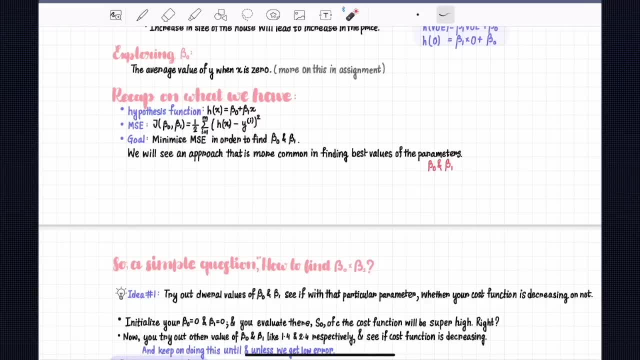 goal. so let's recapitulate: whatever uh we have uh done. so we have an our hypothesis function or a prediction function- our hypothesis function or prediction function- and over here the hypothesis or prediction function states that you have h of x in a builder function, or maybe you have f of x. 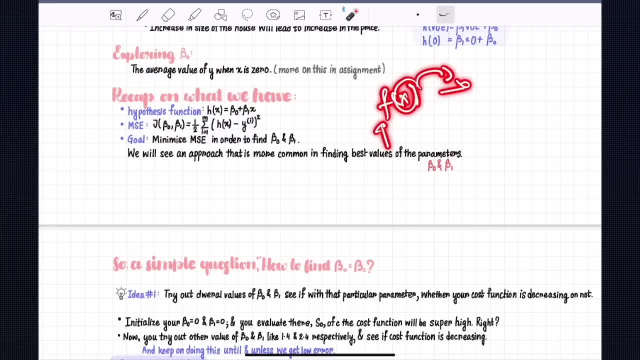 that did that. you have a bit of function f that takes in the value of x and then, and then uh takes in value of x and map it to y and y can be any any problem. for example, you want to predict the sales given uh, given the advertising expenses or, you know, predict the exam scores given the 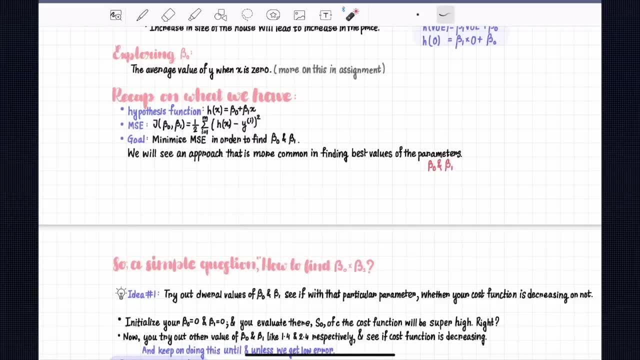 number of our study. so you have input value only one, one input feature. as of now. you have only one input feature x. you have only one input feature x and given uh, and and using this one input feature x, you're predicting what is the uh y right, but it may happen that you have several input features. 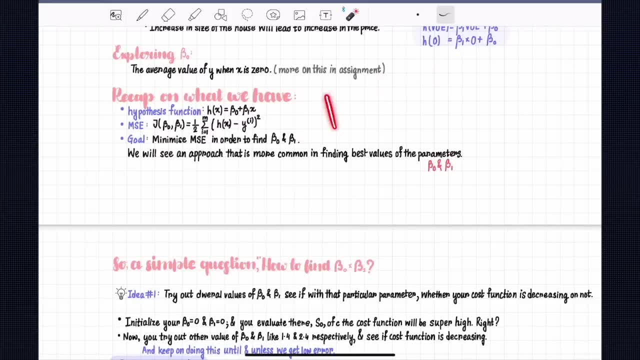 x2, x3, all the way out of the x, and you have several input features and based on these several input features in a predict the y. but we'll take a look at that several one later on. but first of all let's build our baseline. so whenever you work on any type of problem, the first you should think: 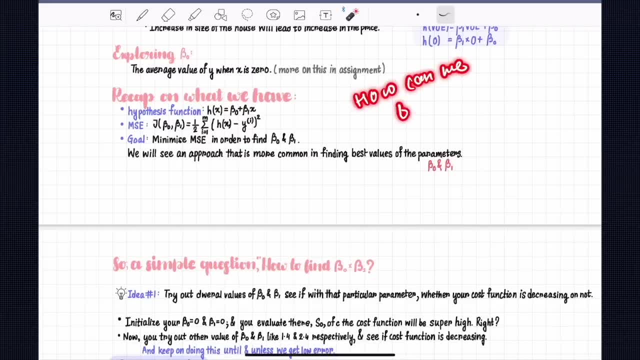 about how can we, how can we build the baseline? build the baseline and a working solution. then, after building a baseline, we can extend it. okay, usually i have seen a lot of people you know: initially they started focusing on advanced things and eventually they they end up losing time. 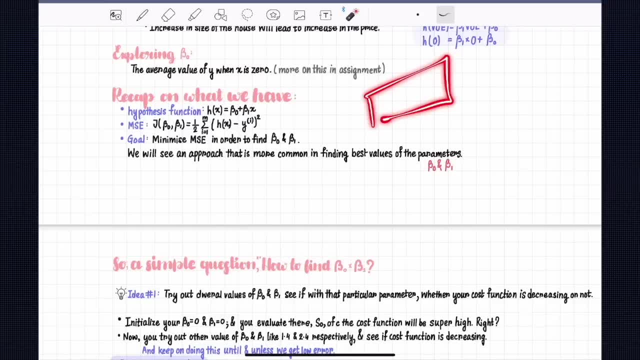 money and etc. so what i recommend is start with the very basic or sim baseline and then build upon that. so, just like this we are doing over here, we are currently taking only one feature as of now only one feature, and then we are trying to predict and then, and then you will see. 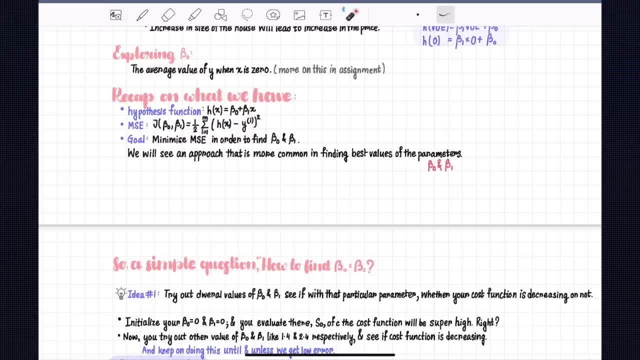 that how we'll extend it, streamlining it very nicely, to other features as well, to several features, several input features as well. okay, cool. so, um, let's get started. so, over here, which you, which, which you're seeing over here, which is the hypothesis function, which is the prediction, 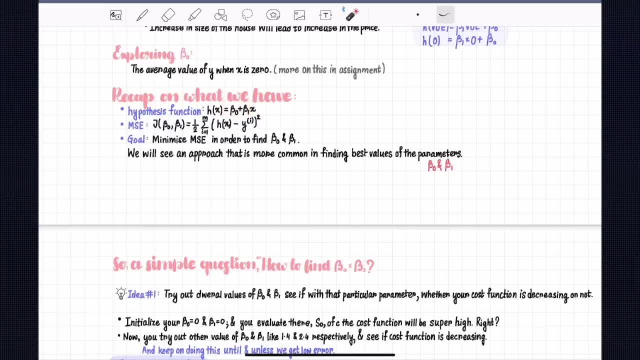 function. you put in the value of x and you get a prediction. and you have to learn your beta 0 and beta 1.. you have to find the value of x and you have to learn your beta 0 and beta 1. you have to. 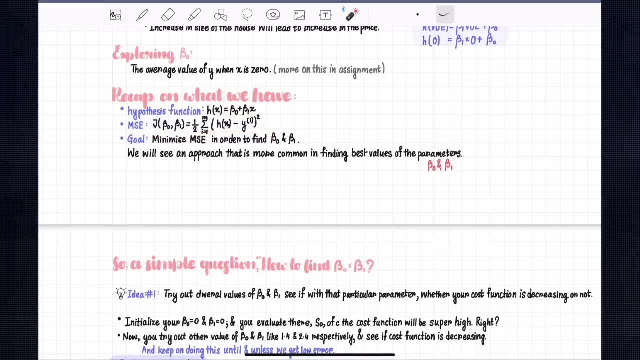 find your beta 0 and beta 1, and then you have your mse, which is which is used to calculate, which is used to calculate your uh, how well your best fit line is. how well your best fit line is, which is 1 over 2 m or i, equals to all the amount of the m h of xi minus y i, where we are taking the. 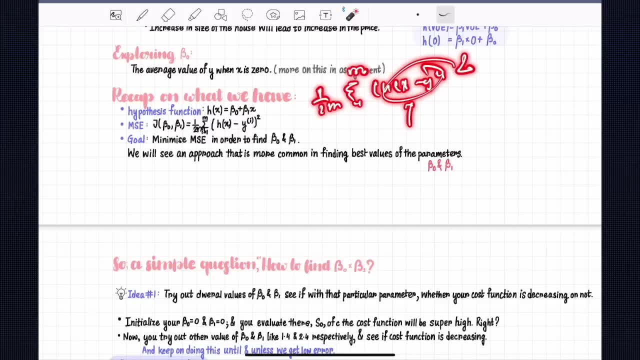 difference of residuals and the squaring to remove the negative sign. and then we are averaging it up so that we we get an overall sense and we're adding two as a convention, or you will see that how this two will help us later on, but as a 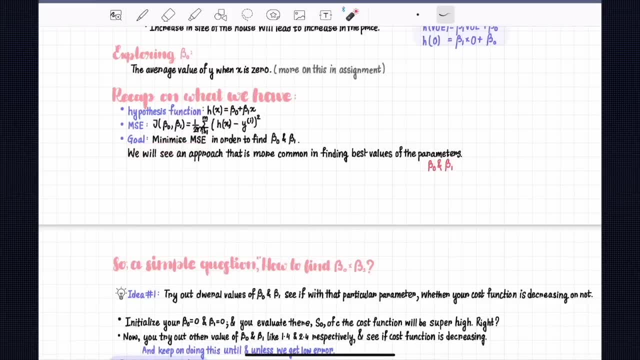 now assume that this is a convention. so what's what's our goal is? our goal is to minimize a mean squared error, which is mean squared. why divide this called mean squared error? because it's we are taking mean of the squares of the error. because we are taking the squares of the error. 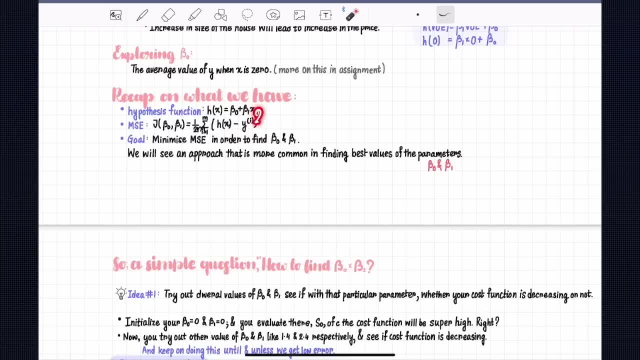 because these are called errors, because these are residual, the differences are errors and the squaring this up, and then we are taking the mean. that's, that's that's why it's called the mean squared error, and our end goal is to minimize this mean squared error. minimize this mean squared. 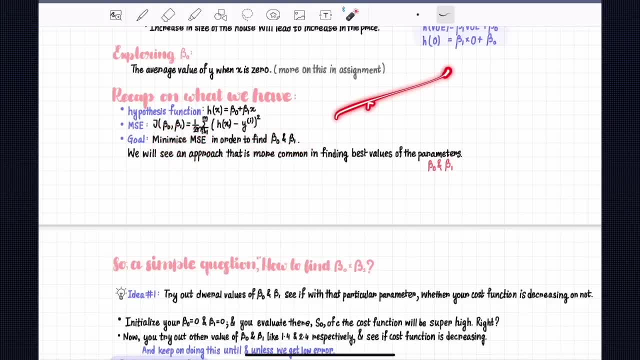 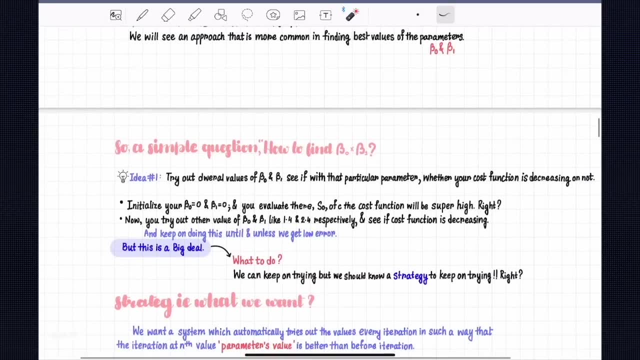 error in order to find your beta 0 and beta 1, because our best fit line depends on this beta, beta 0 and beta 1.. so we'll see approach that is common in finding these. so we have to find this beta 0 and beta 1.. so what are, what are your initial ideas? right? so let's talk about what. 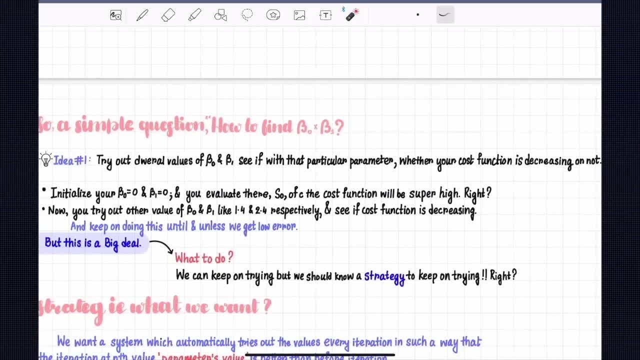 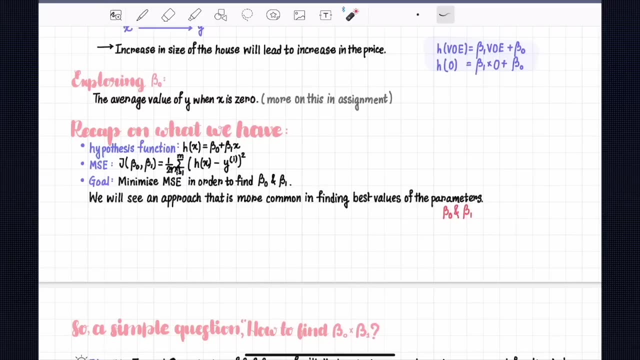 are initial ideas. i would like to give you some seconds, five seconds from now on, to think about what, what ideas, what idea you can come up with, what idea you can come up with to actually to actually get this beta 0 and beta 1.. so you can take five seconds from now on to think about what. 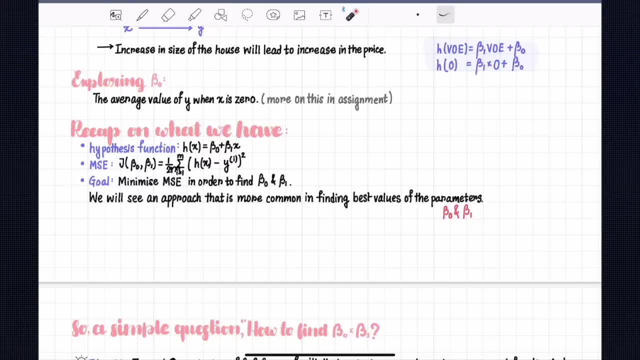 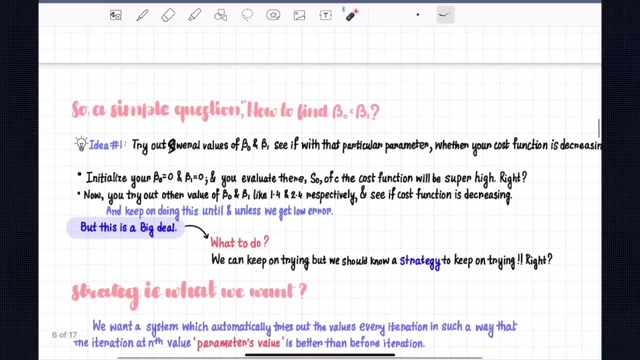 way you want to achieve, and you can actually take a break as well if you are just feeling overwhelmed. but i'm trying to make it explanation so easier, so i hope that you have understood now over here in i. what is the idea number one? the idea number one is to try out several values of beta 0 and beta 1. 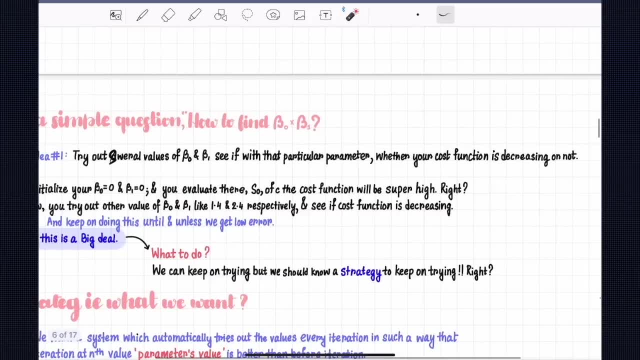 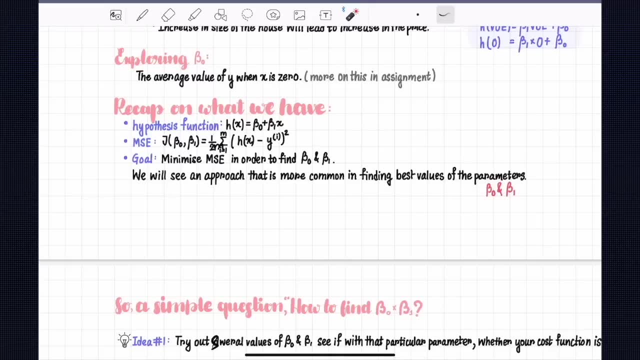 and see if, with that particular parameter, whether your cost function is decreasing or not. so what i'm trying to say that you can try out several first. first what you what, what the idea is that you can try your random, say for the, for example, you guess, beta 0. oops, what happened to me? 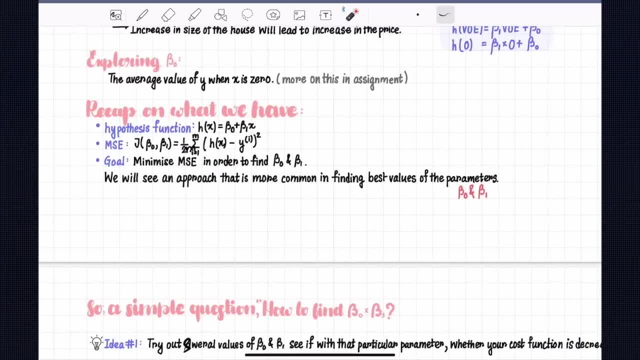 omg, okay, wait, uh. yeah, so you can try your several values. let's let us assume beta 0 to be 1 and beta 1 to be 0. you take in these values and then you plug in the value of over your beta 0 and beta 1. 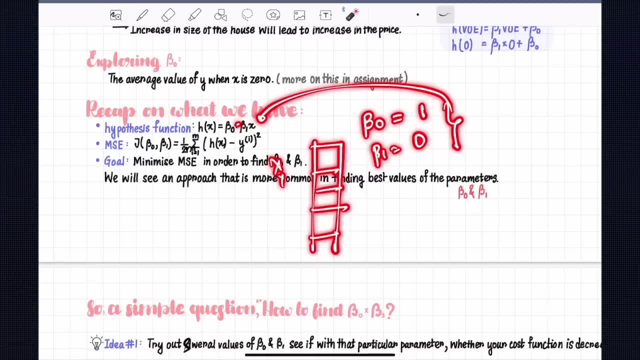 and then you evaluate, and then you take in the predictions for every x's x is out here, for every predictions, and then you take in out the mse and then we have taken. we have done this. please don't don't. please see my past lectures. okay, so we have. we will take out the msc now. we'll take out the msc. 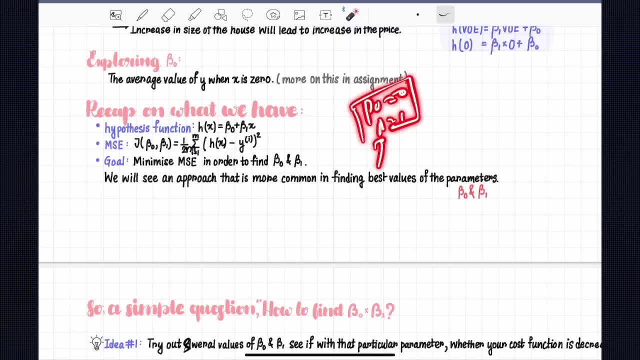 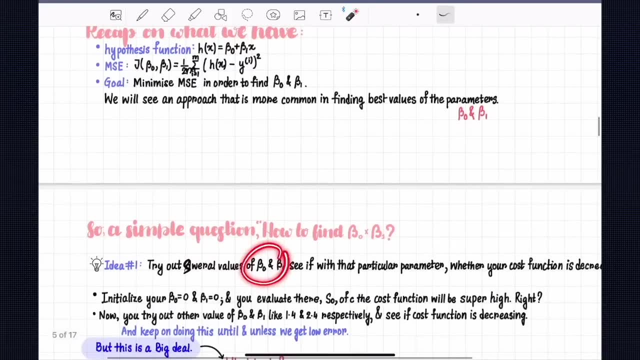 so if, with these zero and one, if our msc is decreasing, first of all, if, if our msc is decreasing, if our cost is decreasing, if our error is decreasing, then what we did then, then we'll update our values of beta 0 from, for example, assume that the first in the when, when you get, 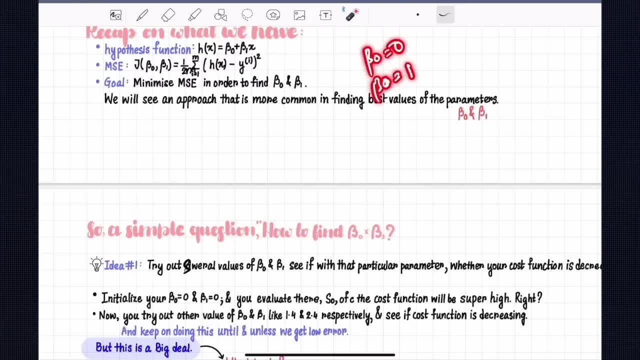 started. you say every to be zero and zero. you initialize beta 1 and beta 0 to be random values. initialize the 0 and beta 1 is 1.. so first of all initialize and then you try a different value, okay, and then you take out the cost function with this m mean square error. the error from this uh. 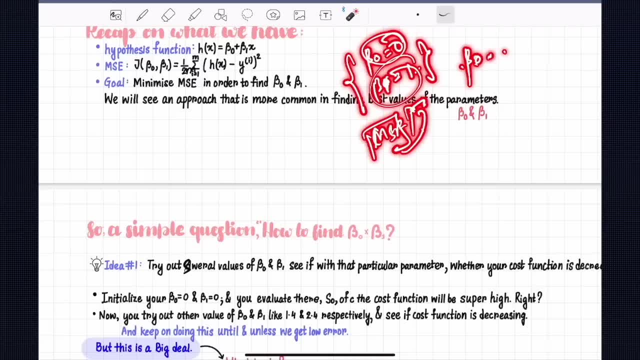 particular, uh, betas. and then what you do, you, you, you randomly take another value, you just you, you just take out the value like 0.25 or beta 1, 0, 1.75, you take the value and then you check msc and then 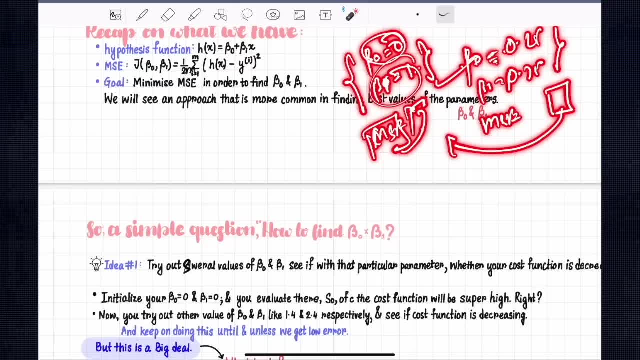 you check your msc. if the msc is less than the previous one, then you update the beta value. okay, then you update the beta value. right, so you update the beta value. if with this, if with this new value, if your ms is dick, is is less than the 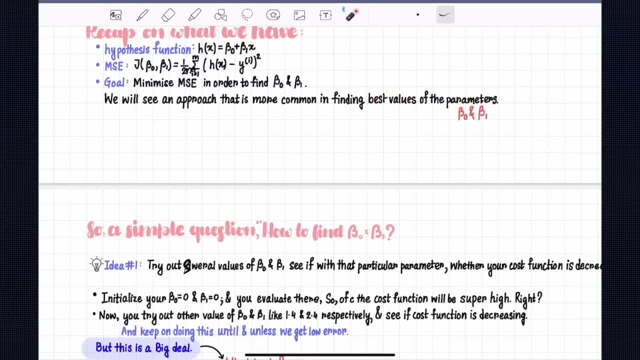 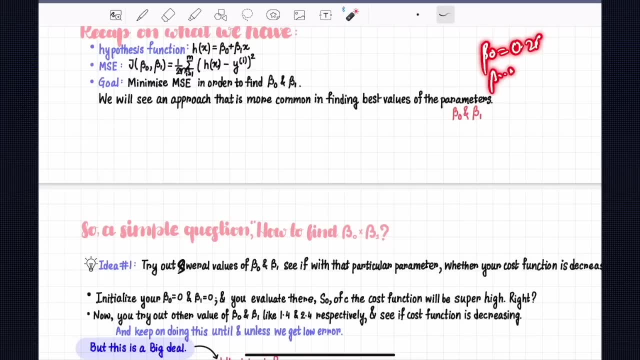 previous one. if your error is less than the previous one, right, and then you update your beta value to be a new one whose error was less than the previous one, okay, and then, after this, you have beta 0 to be 0.25. beta 1 is 1.75. now, this updated one right where msc something, mscc. 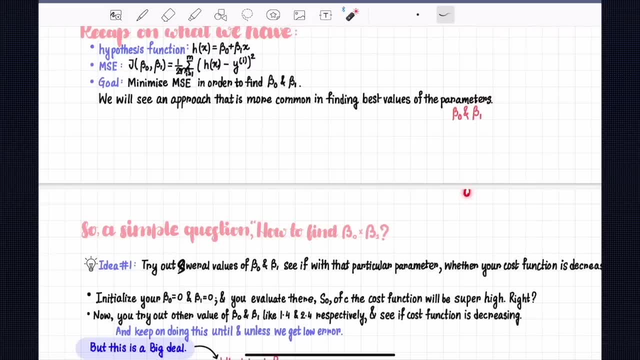 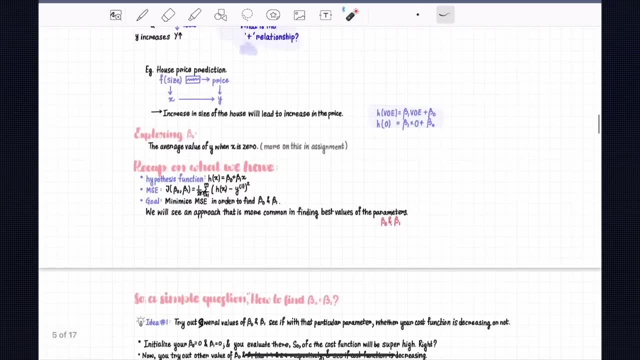 okay, now you update. now you again update 0. maybe 95, and beta 1 to be zero. now beta 0 is 0.95 and then you check. okay, now, if i check, our msc is less than previous one. if yes, then we have the, then we. 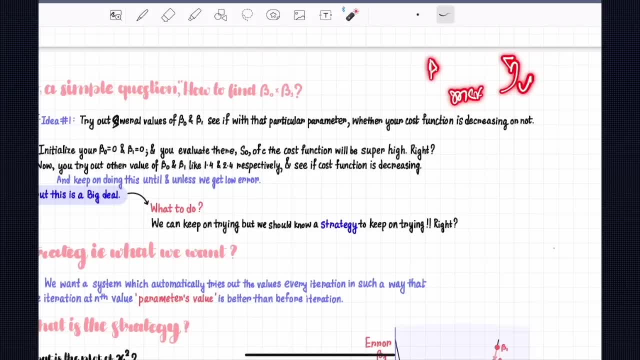 again update the value, then we use the, not previous the, but the current, which is 1.95, and beta beta 1 equals 1.995, beta 0 is equal to 0.95. okay, so we use the updated one. so what exactly we are doing? we are trying out several values of beta 0 and beta 1 and see if, with that particular, 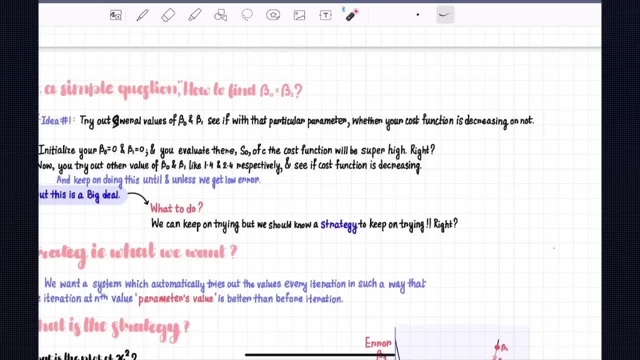 value of the parameter, our cost function decreasing as compared to previous one or not. so we are trying out several values of beta 0 and beta 1 and see if, with that particular value of the parameter not, if it is, then we update, and if it is not, we just stick to the previous one. okay, so our first 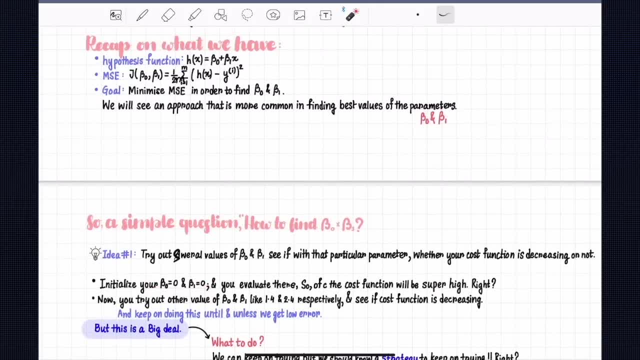 step in this idea would be to initialize your beta 0 and beta 1 and the evaluate with these. uh, how do we evaluate using this cost function where you predict on every samples of xi and then you compare with the y i and y hat i and then you simply predict it. so the cost function will be 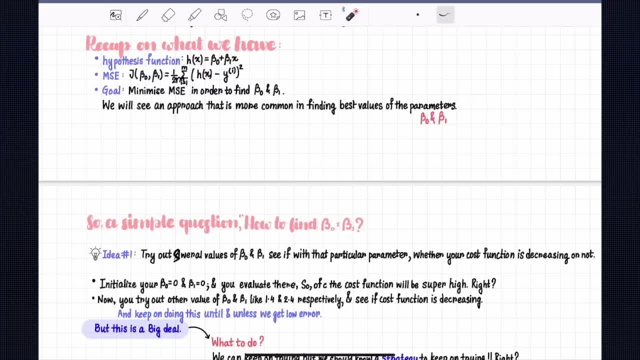 super duper high, right? so the of course, the cost function will be super duper high, because when you have beta 0 to be 0 and beta 1, because so it's, the cost function will be super, super high. now you want to try and very low, right? so we have to try, for example, the cost function to be 0 and beta that. 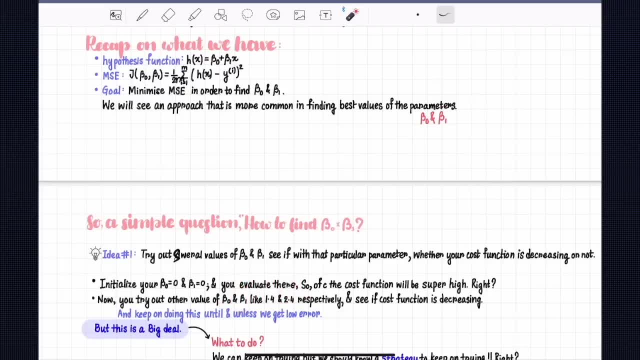 is the cost function for beta 1 to be 0, because you can see the different values of beta 0 and beta 1, like 1.4 into 1.5 respectively, which is beta 0 for 1.5, beta 1 through to 2.4, and see if. 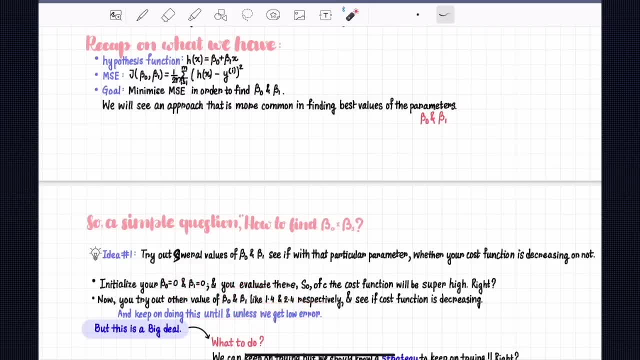 the cost function decreasing. so if the cost function is decreasing as compared to previous one, you update the beta value from 0 to these values and keep on doing this until and unless you get low error. you get low error right. so you have to try out several values of beta and beta b, beta 1. 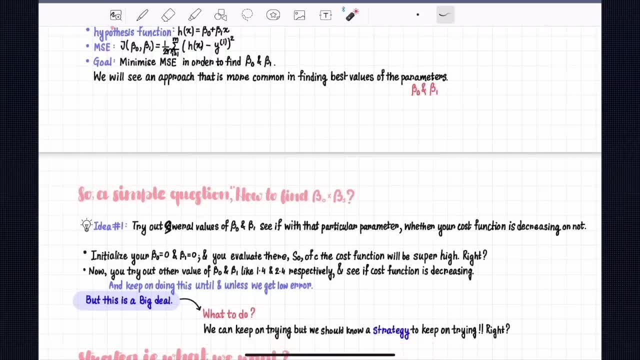 deal in this is that we can keep on trying. so what to do? like this is something which you have to think of, right, so we need a strategy, right so we can keep on trying. but we should know a strategy to keep on trying. we cannot just think about any, any value, and then just go with it. right, it will. 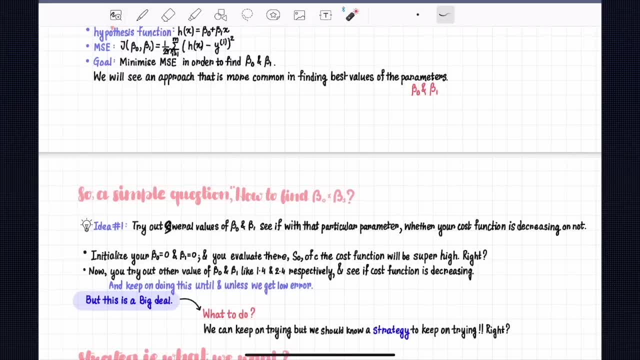 definitely not make sense, right? so what exactly we want? we want to think about in terms of: we want a strategy for us or we want an algorithm to try for us. this is a good, a good good, uh, this is a good strategy, but we have an algorithm to try this strategy for us. to try this strategy for us. 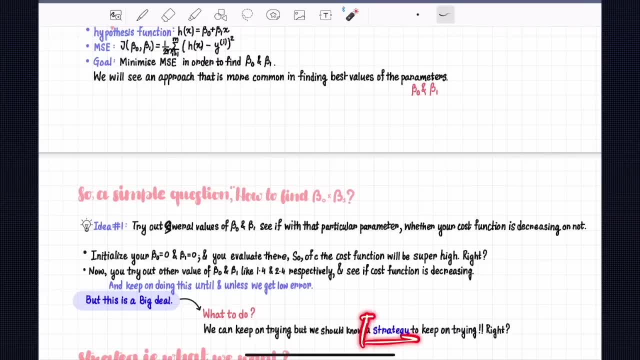 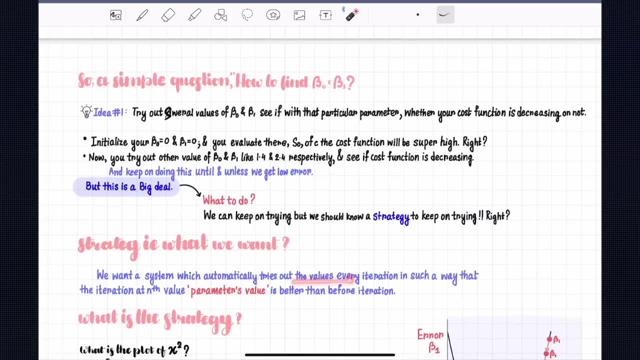 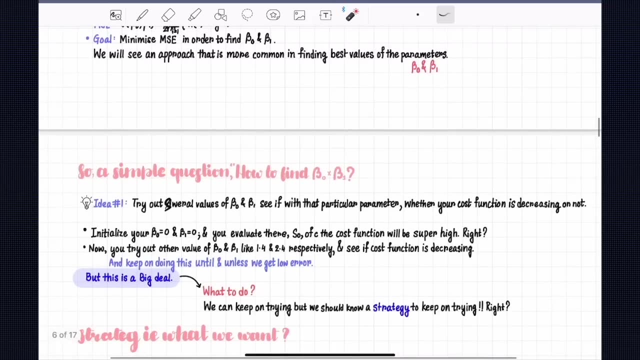 in an efficient and timely manner within a strategy. so what's that strategy? the strategy is we want, we want a system which automatically tries out several values without any human intervention. tries out every of values, every, in every iteration. so what is iteration in this case? you might be confused in this. so when you are, beta 1 is equals to 0 and beta 0 is. 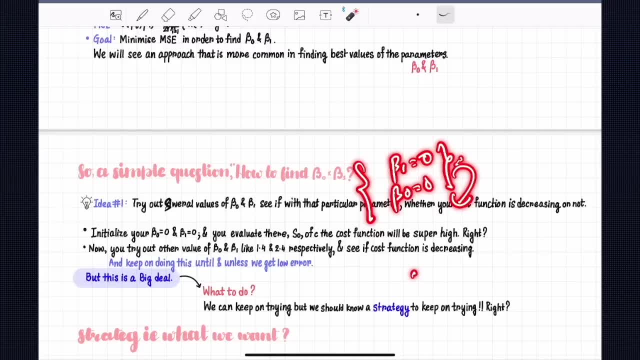 equals to 0. so you have these betas right. this is now when you update. now you are. now you update the value. so the first iteration would be: now you update the value and then check the msc. then a second iteration: you update the value as compared to the previous one and then check mscs less than 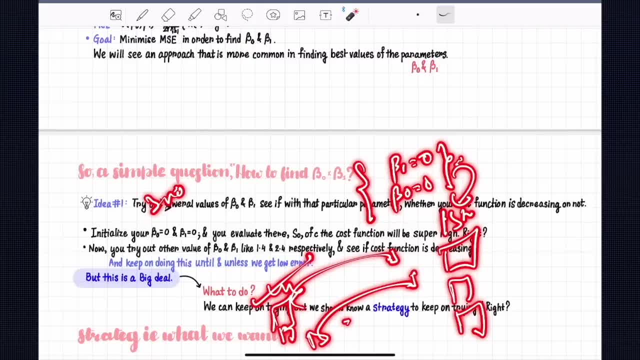 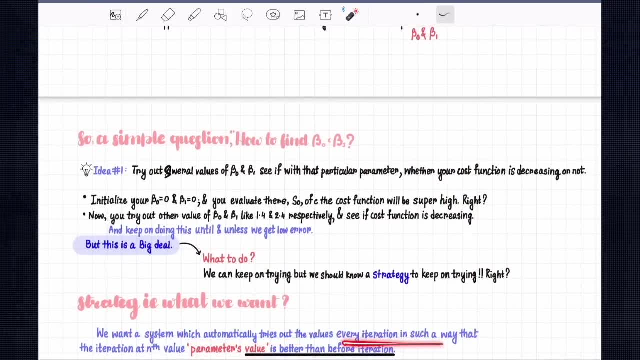 if it is, then you. this is second iteration. the third iteration means the third time you're changing the value and seeing if the mscs, so that's iteration, okay. so we want a system which automatically tries out the values every iteration, in such a way that your iteration at nth value, iteration at the last parameter. 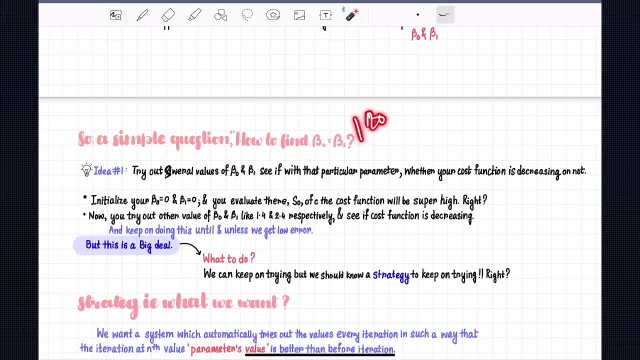 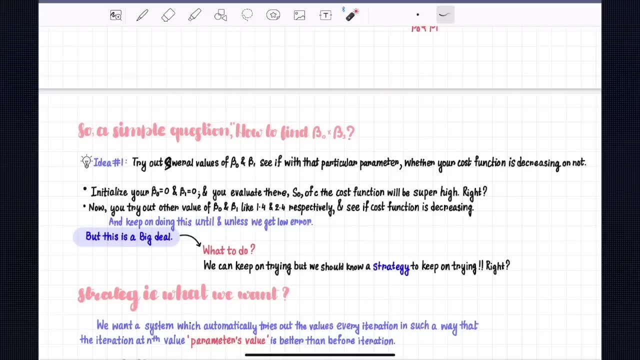 value, which is the last iteration or something like that, would assume that you want to make a 20 iteration, so a 20th iteration is better. or maybe this your second iteration? at the the the. the error at the second iteration, where you have updated beta 1 and beta 0 should be less than the. 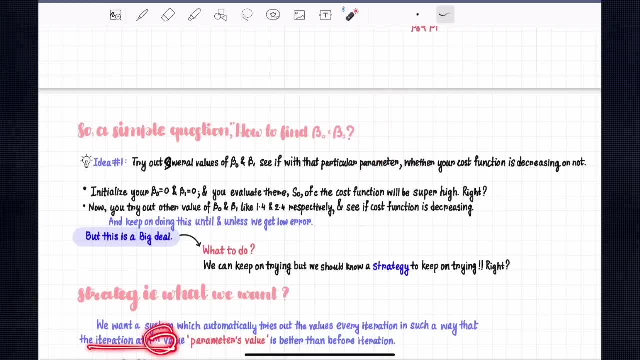 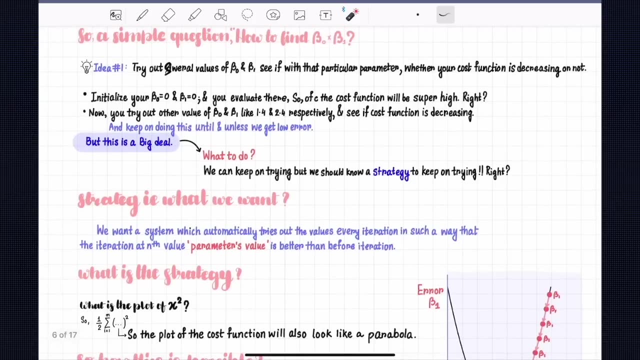 previous one. okay, it is what is telling the iteration at the nth value, for example, third iteration, the parameters value of the third iteration should be better than the second iteration, and how to check betterness by msc is better than the before iteration. hope so that you got it this. 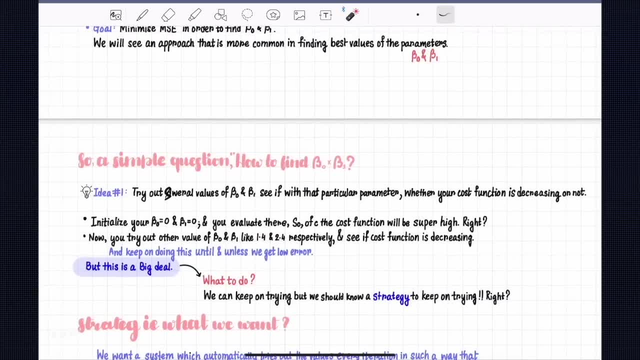 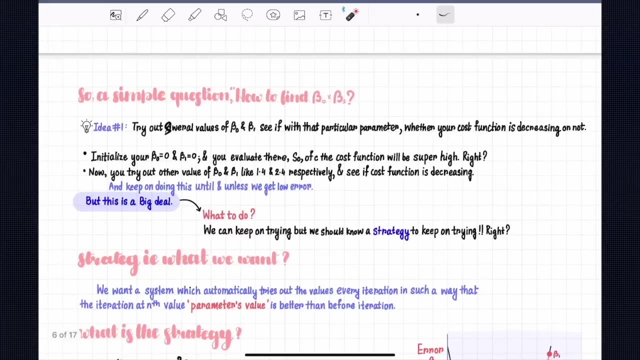 is a strategy one. now, how can we come up with this strategy? this is something you know, this, this is something which you should be able to uh confront by yourself. so how, what is the exact strategy for this to occur? so the strategy is, the strategy is: uh, the strategy is we can make use of something. 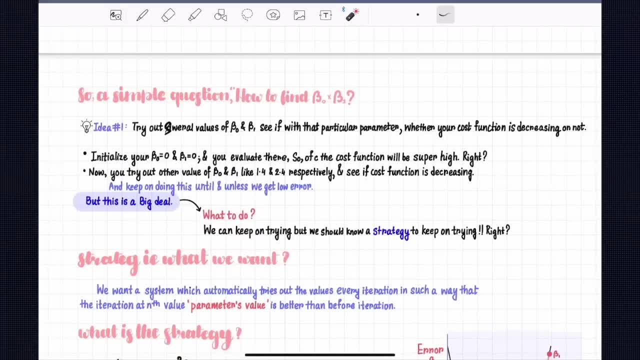 known as not go to what exactly. I have a very different mind to teach you are. so assume that. assume that we, we want to know. so what exactly we we want to know. so how can we check, how can we check we want to check that, that, that, whether my 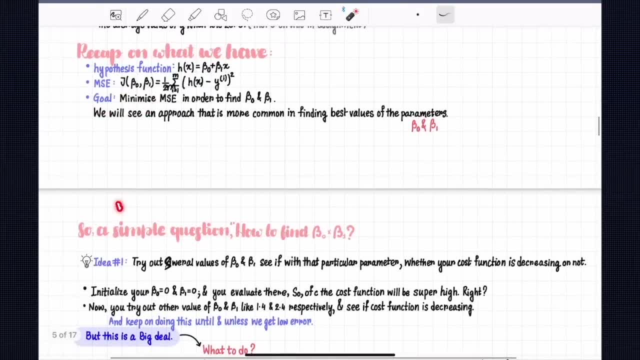 cost function or whether my mean square error is decreasing if I change beta 0. awesome, if, if I change the bit beta, beta 0. so what exactly? you want to know whether, whether my cost function, cost function, is decreasing if I change my. what if I change my beta 0 or and beta 1? so I want to check this right. I want to. 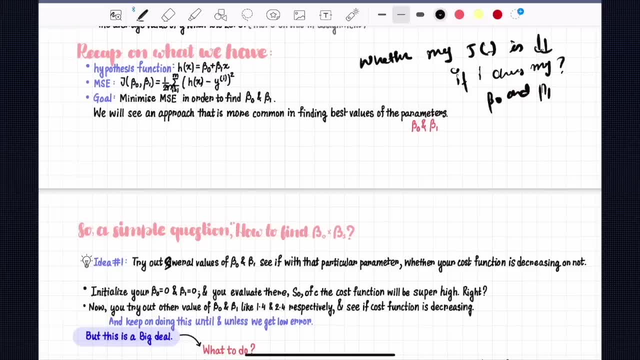 check this. so you might have heard about let's, let's, let's not gonna get a mathematical dump, so we wanna, we wanna check this, right, so what is the we can? we can check this. so you might have heard about slope okay, slope okay. so let's talk about change in Y over. 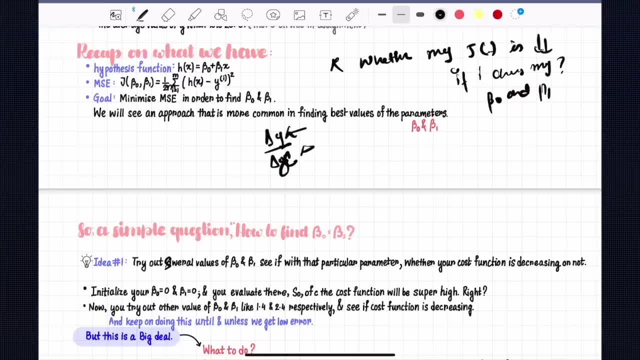 so let's talk about change in Y over. so let's talk about change in Y over. change in X: how much Y changes. how much change in X, how much Y changes. how much change in X, how much Y changes. how much Y changes when X changes. that's, that's. 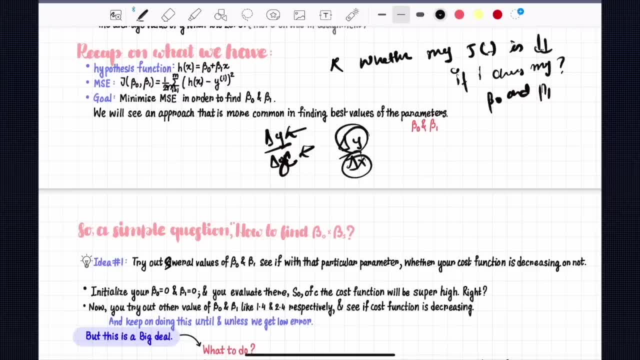 Y changes when X changes. that's that's Y changes when X changes. that's that's what is change in Y over change in X. so what is change in Y over change in X? so what is change in Y over change in X? so how much Y changes when X changes. so 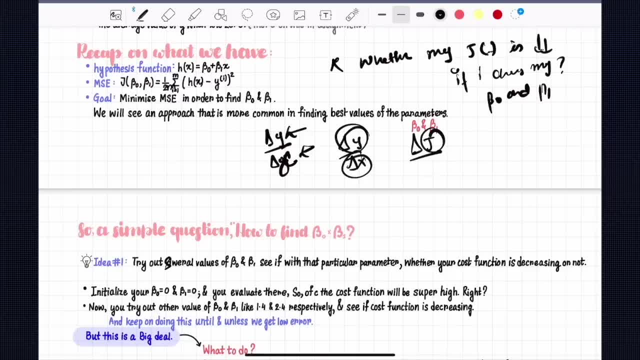 how much Y changes when X changes. so how much Y changes when X changes. so what if I can write how much J changes? what if I can write how much J changes? what if I can write how much J changes? how much your cost function changes when? how much your cost function changes when. 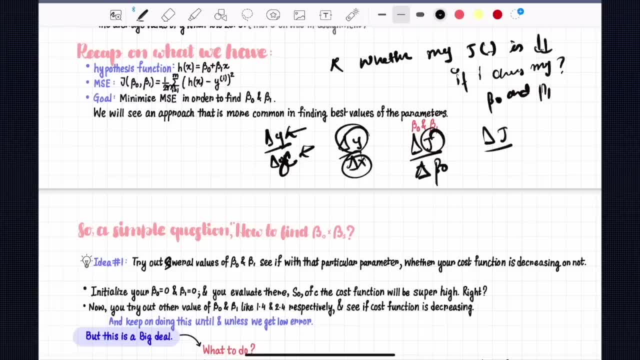 how much your cost function changes when you change, when you change your beta 0. you change when you change your beta 0. you change when you change your beta 0 and how much your cost function changes. and how much your cost function changes and how much your cost function changes when you change your beta 1. so can we? 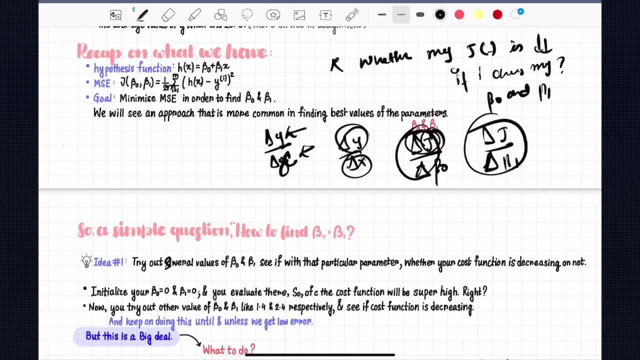 when you change your beta 1, so can we. when you change your beta 1, so can we. get our change the rate of change right. get our change the rate of change right. get our change the rate of change right. so if my cost function decreasing as 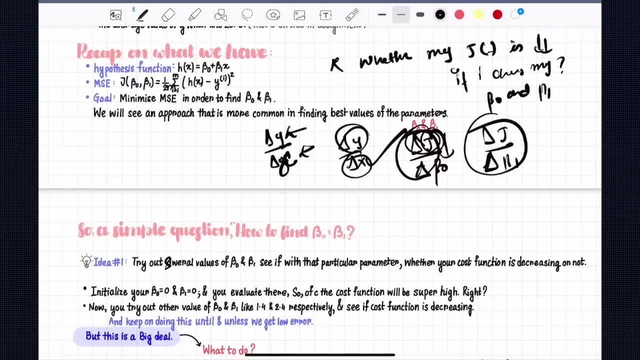 so if my cost function decreasing as so if my cost function decreasing as compared to brief as guest come to. compared to brief as guest come to. compared to brief as guest come to. previous one: this is good, we can check. previous one: this is good, we can check. 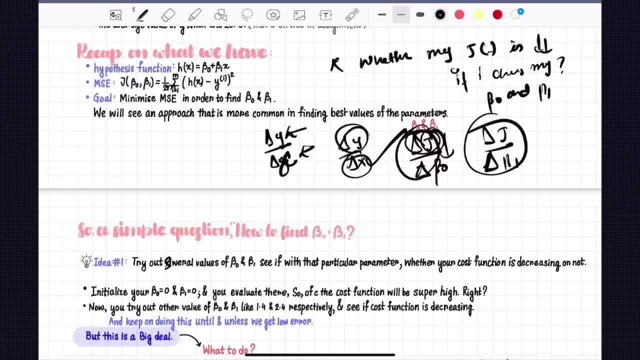 previous one. this is good. we can check the rate of change by nothing but the, the rate of change by nothing but the, the rate of change by nothing but the slope, my nothing but the slope. oh you slope my nothing but the slope. oh you slope my nothing but the slope. oh you, which, which, which you have heard, now, now. 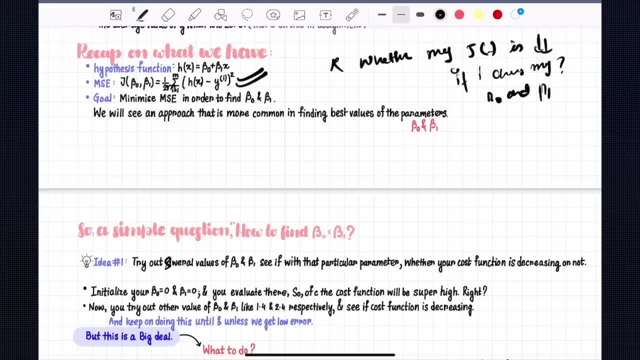 which, which which you have heard now, now, which which which you have heard now. now, here comes an interesting part. now, over here comes an interesting part now over here comes an interesting part now, over here. how can we take out the slope of here? how can we take out the slope of? 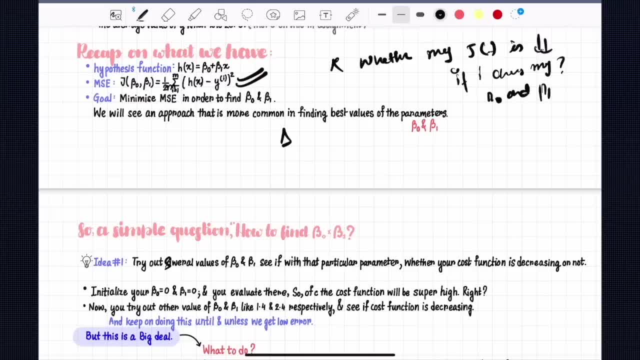 here. how can we take out the slope of this? because we eventually want to take this, because we eventually want to take this, because we eventually want to take out the slope of this particular function, out the slope of this particular function, out the slope of this particular function, how can we take out this? a very 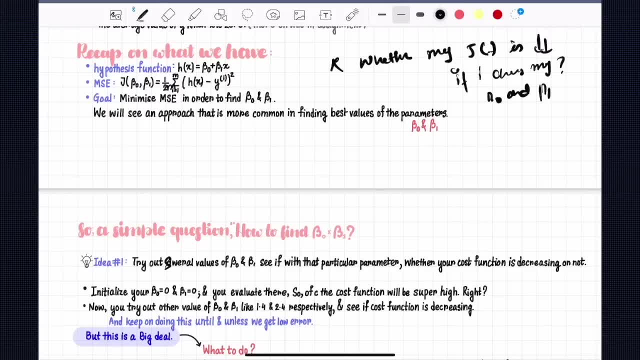 how can we take out this? a very how can we take out this? a very interesting question. so the though let's interesting question. so the though let's interesting question. so the though let's let's let's worry about first of all tell let's let's worry about first of all tell. 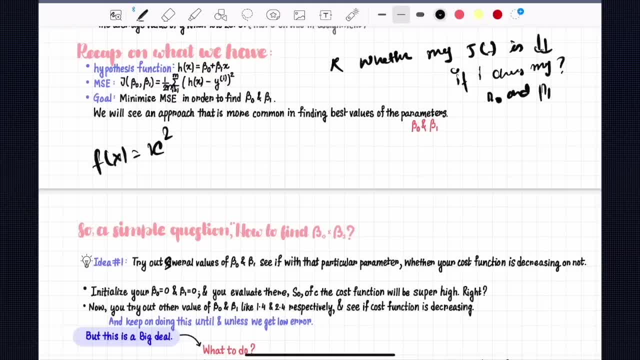 let's, let's worry about. first of all, tell me what is the if he, if he can applaud me? what is the if he, if he can applaud me? what is the if he if he can applaud this function f of X, how? what is the? this function f of X, how? what is the? 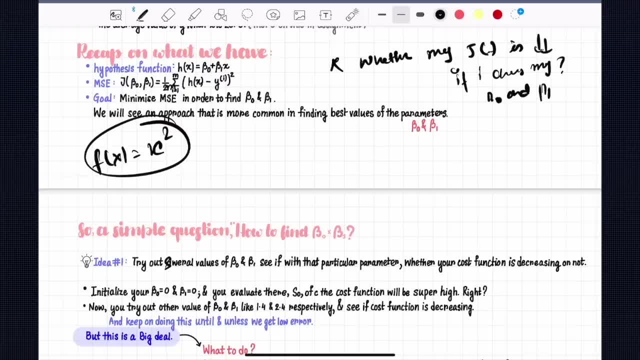 this function f of X, how? what is the what? what will the plot looks like so what? what will the plot looks like so what? what will the plot looks like so well? I would recommend you to plot this well. I would recommend you to plot this well. I would recommend you to plot this function on a graph right now, where you 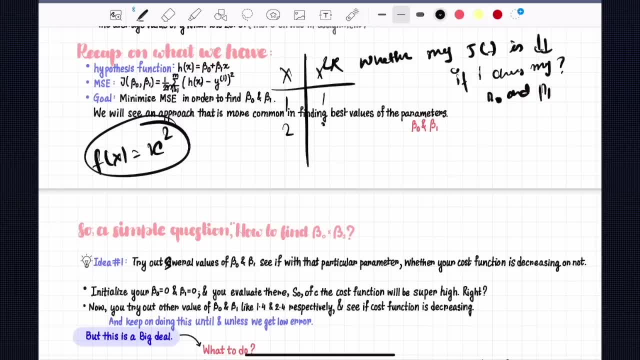 function on a graph right now. where you function on a graph right now where you plug in the values of X and x squared. plug in the values of X and x squared. plug in the values of X and x squared. plug in the values 1, 1, 2, 4, 3, 9. plug in. 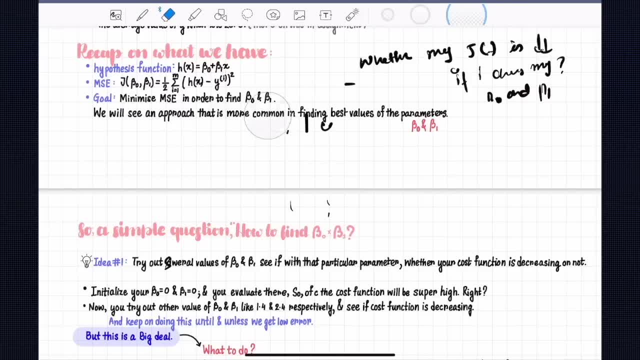 plug in the values 1, 1, 2, 4, 3, 9, plug in the several values and then plot it, the the several values, and then plot it the the several values and then plot it the plot which you're going to get the plot. 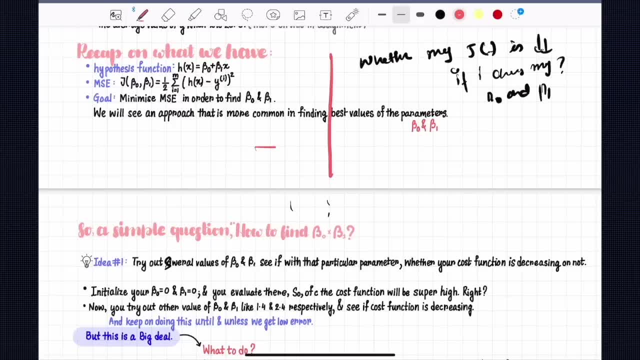 plot which you're going to get, the plot, plot which you're going to get, the plot which you're going to get. it's a nothing which you're going to get. it's a nothing which you're going to get. it's a nothing, it's nothing, but something like this, but. 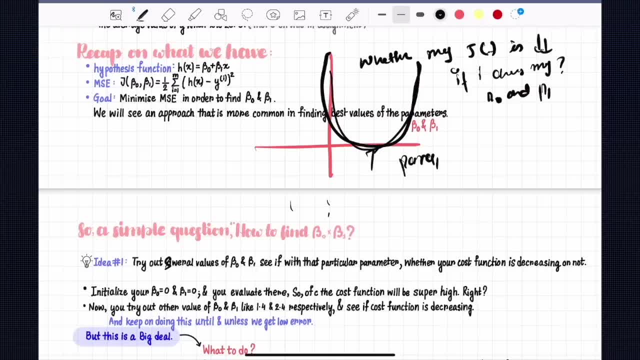 it's nothing but something like this. but it's nothing but something like this, but something like this: okay, a parabola, a something like this. okay, a parabola, a something like this. okay, a parabola, a parabola, okay, or something like the some. 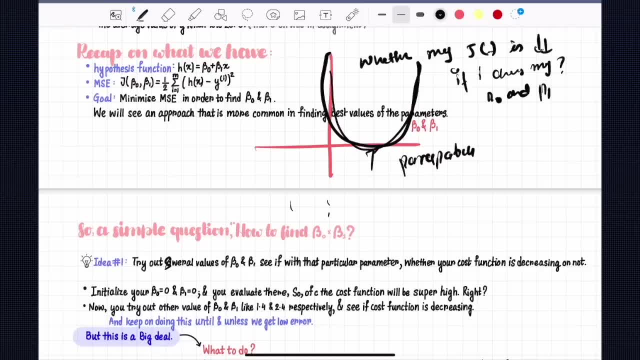 parabola okay, or something like the some parabola okay, or something like the some, the. so if not not exactly parabola but the. so if not not exactly parabola but the. so if not not exactly parabola. but you, if you plot this on, if I just 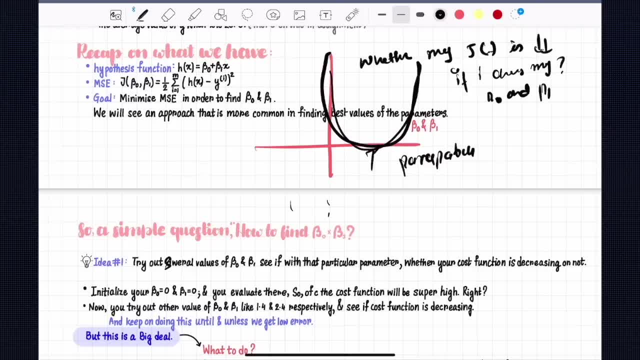 you if you plot this on, if I just you, if you plot this on, if I just plotted it on terms of you know positive, plotted it on terms of you know positive, plotted it on terms of you know positive one, but if you plot this on, but the but. 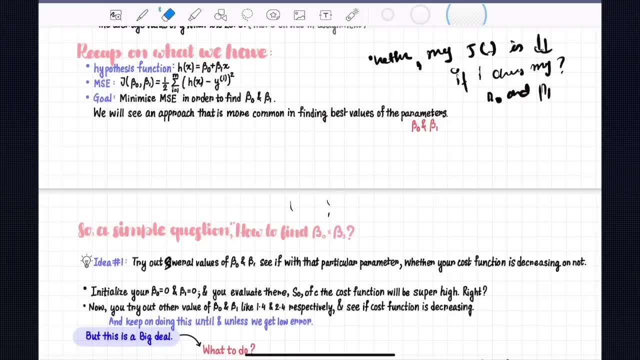 one, but if you plot this on but the but one, but if you plot this on but the but the parabola, if you eventually plot this, the parabola, if you eventually plot this, the parabola, if you eventually plot this up, if eventually plot this up. so let me. 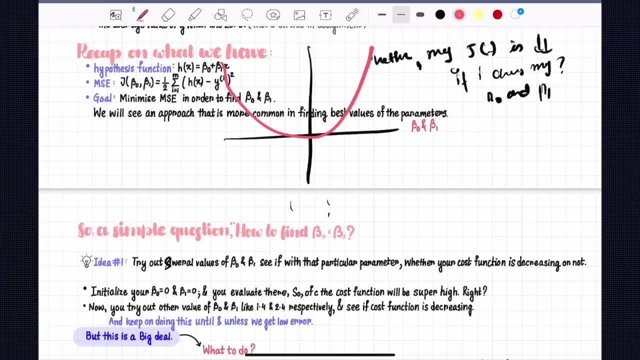 up. if eventually plot this up, so let me up, if eventually plot this up. so let me, let me, let me just plot this up. so the let me, let me, let me just plot this up. so the let me, let me, let me just plot this up. so the plotting would look like this: which? 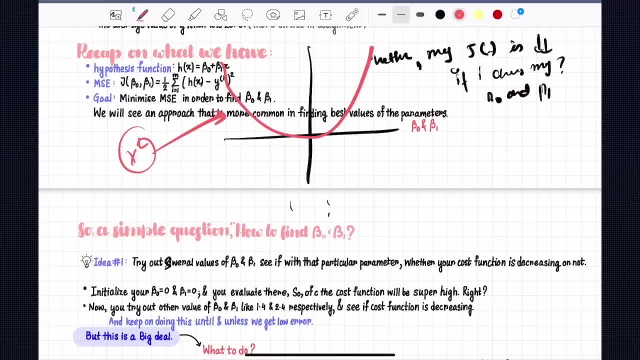 plotting would look like this. which plotting would look like this: which is the function x squared. this is a. this is the function x squared. this is a. this is the function x squared. this is a. this is a for. this is a function. this is a is a for. this is a function. this is a. 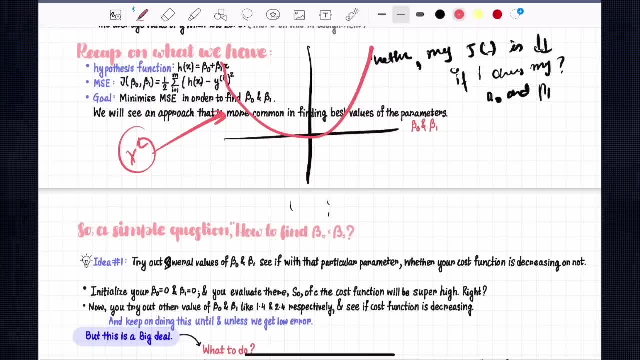 is a for. this is a function. this is a graph of your x squared. this is a graph graph of your x squared. this is a graph graph of your x squared. this is a graph of your x squared now. this is a graph of of your x squared now. this is a graph of. 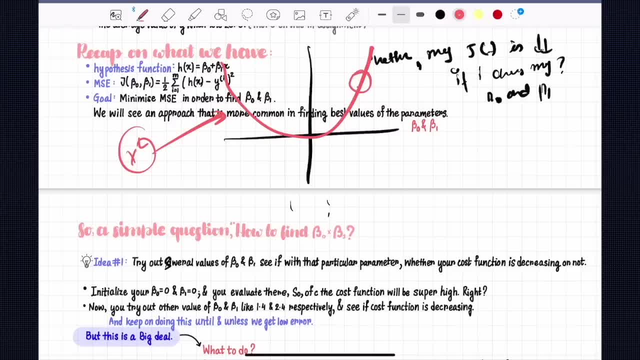 of your x squared. now this is a graph of us xx weight. so you can you tell me how us xx weight. so you can you tell me how us xx weight. so you can you tell me how can you take out slope in this? because can you take out slope in this? because 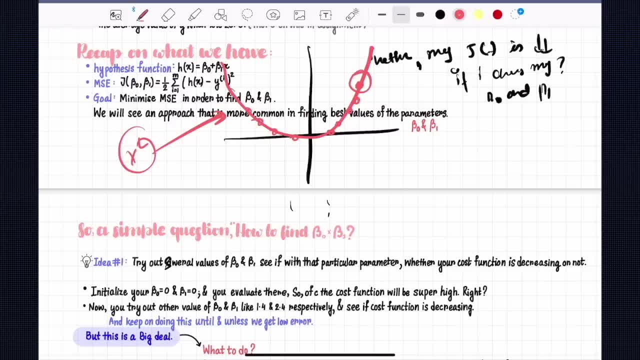 can you take out slope in this? because at every point, every point, your slope, at every point, every point, your slope, at every point your slope changes. so there is not a constant slope changes. so there is not a constant slope changes. so there is not a constant slope. right? so assume that you want to take a. 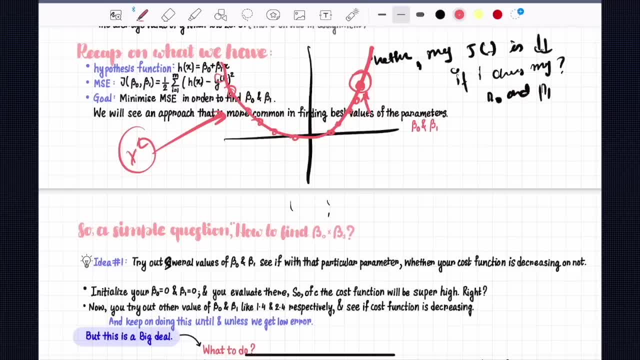 right. so assume that you want to take a right. so assume that you want to take a slope at this particular point. so at slope at this particular point, so at slope at this particular point. so at this particular point. what does it tell? this particular point? what does it tell? 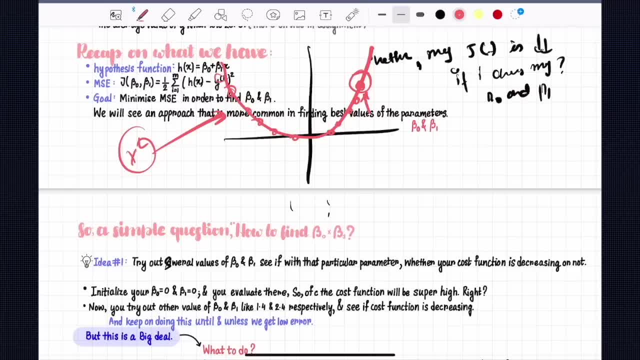 this particular point. what does it tell what? what does the slope will tell how, what? what does the slope will tell how, what? what does the slope will tell how much that, how much it will be, how, what much that, how much it will be, how, what much that, how much it will be, how, what? what is at this particular point will? 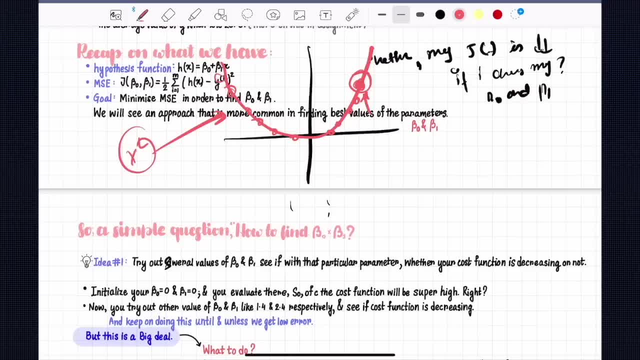 what. what is at this particular point, will what? what is at this particular point, will will tell how much your x square will tell how much your x square. will tell how much your x square will change when you change this a little bit. will change when you change this a little bit. 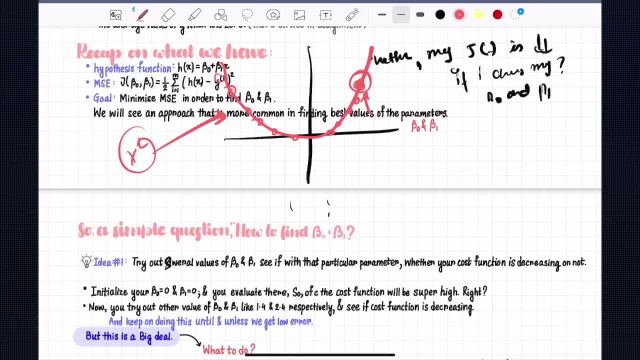 will change when you change this a little bit. let's forget it, you can. let's forget it, you can. let's forget it, you can. let's say you wanna to take a slope at. let's say you wanna to take a slope at. let's say you wanna to take a slope at this particular point you want to take a. 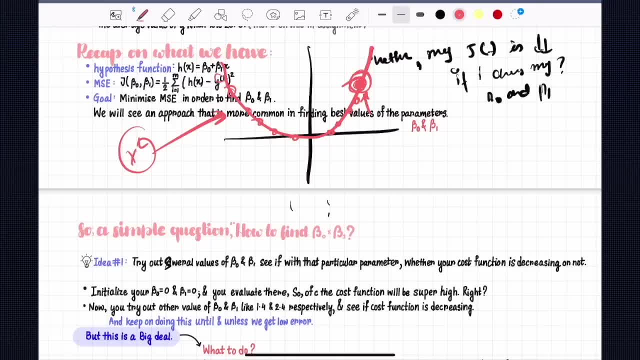 this particular point. you want to take a this particular point. you want to take a slope at this particular point. because slope at this particular point? because slope at this particular point? because slope at is not is not constant. slope at is not is not constant. slope at is not is not constant. right, it's not same all over the graph. 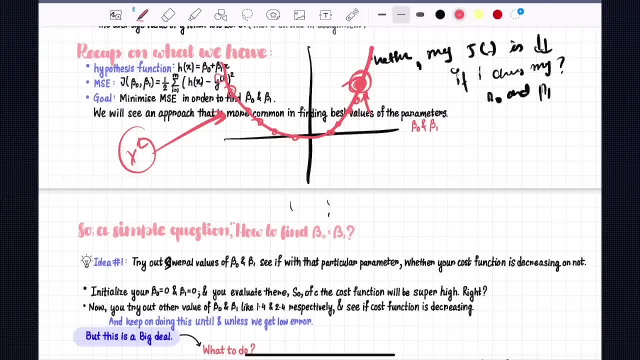 right, it's not same all over the graph. right, it's not same all over the graph. it keeps on changing right, it keeps on, it keeps on changing right, it keeps on, it keeps on changing right, it keeps on changing. so, now, now, it is not possible changing so now, now, it is not possible. 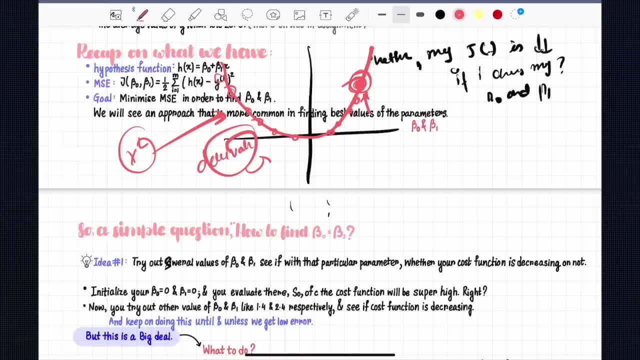 changing. so now, now it is not possible. so what we do? there's a concept of, so what we do. there's a concept of, so what we do. there's a concept of derivatives which takes out slope of a derivatives, which takes out slope of a derivatives which takes out slope of a curved line. 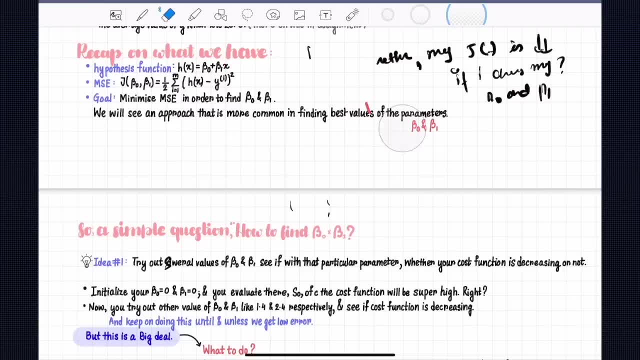 curved line. curved line okay of a curved line. i hope that this okay of a curved line. i hope that this okay of a curved line. i hope that this gives a good sense. now this parabola gives a good sense. now this parabola gives a good sense. now, this parabola. why does i introduce this parabola? to? 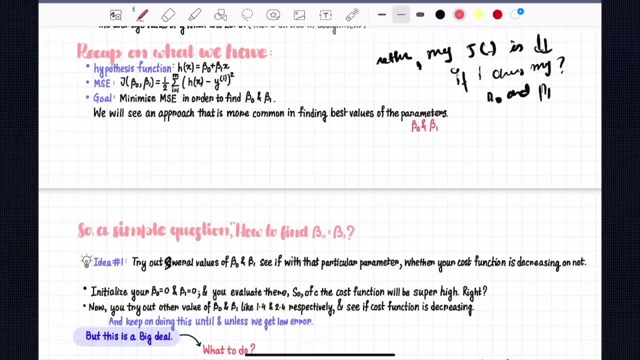 why does i introduce this parabola to? why does i introduce this parabola to you? interesting question, right you? interesting question, right you? interesting question, right, observe carefully, observe carefully, can observe carefully, observe carefully, can observe carefully, observe carefully. can you see this? you see this. 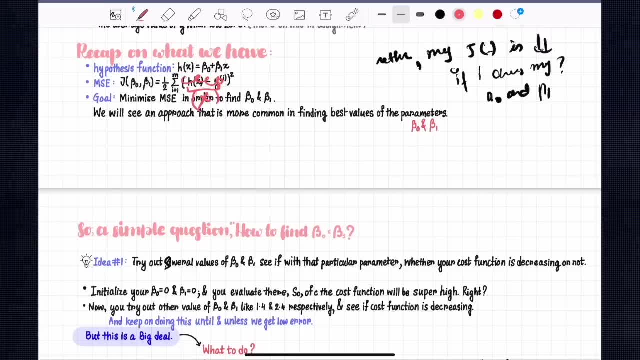 you see this, this is something. assume that this is this is something. assume that this is this is something. assume that this is something, something, something x. and then you're squaring this up, isn't x? and then you're squaring this up, isn't x? and then you're squaring this up, isn't your cos function will look. 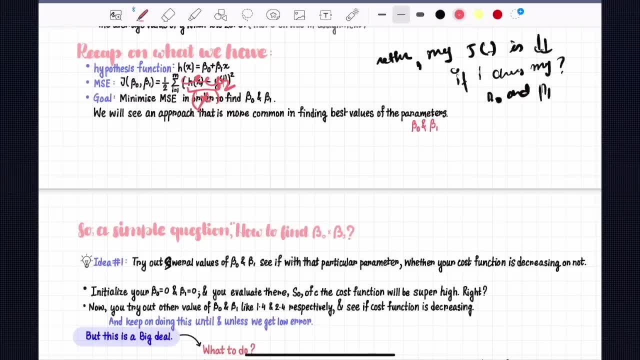 your cos function will look. your cos function will look something like parabola. right because something like parabola, right, because something like parabola. right, because we're squaring directly, squaring this up. we're squaring directly, squaring this up, we're squaring directly, squaring this up. right. it will look like something like: 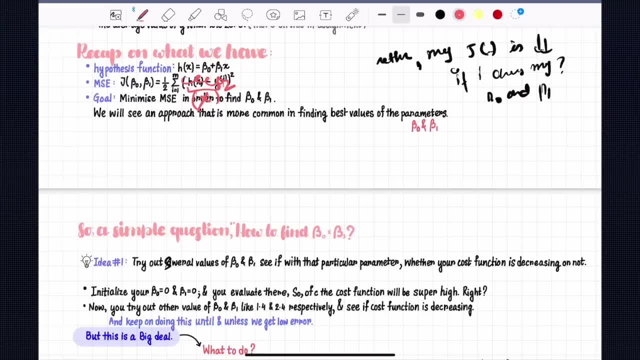 right, it will look like something like right, it will look like something like parabola. so when you plot this equation parabola, so when you plot this equation parabola, so when you plot this equation up, and you plot this equation up, you will get. you will get something like: 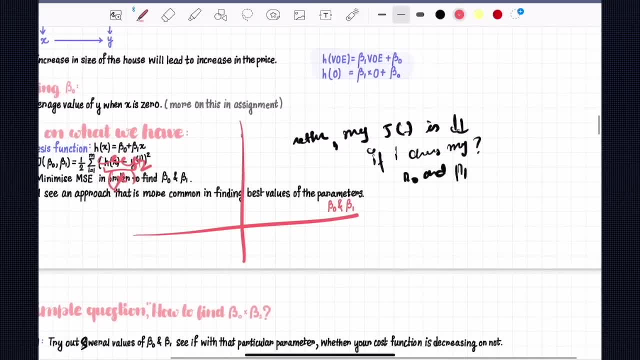 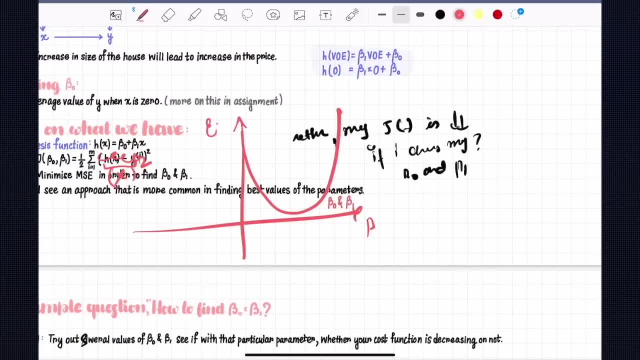 you will get something like that: now, on x-axis, you will have your betas on y. on x-axis, you will have your betas on y. on x-axis, you will have your betas. on y axis, you have your errors axis. you have your errors axis, you have your errors. so now again it might can can confuse. 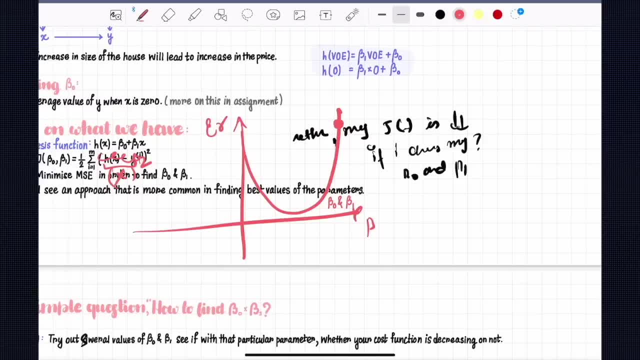 so now again, it might, can, can, can confuse. so now again it might, can, can, can confuse you, you, you, for every point of the betas, for example, for every point of the betas, for example, for every point of the betas, for example, let let us assume this is a beta zero. 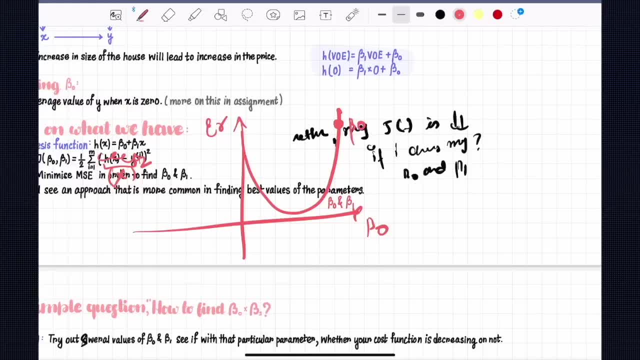 let let us assume this is a beta zero. let let us assume this is a beta zero. okay, so, in beta zero, beta zero over here. okay, so, in beta zero, beta zero over here. okay, so, in beta zero, beta zero over here. if beta zero is, uh, if beta zero, point is: 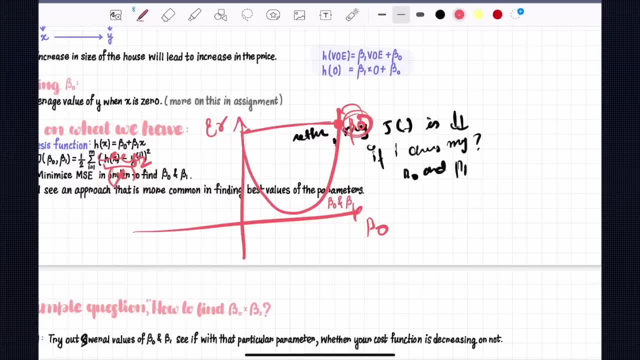 if beta zero is uh, if beta zero point is if beta zero is uh, if beta zero point is over here. so your error at this point over here, so your error at this point over here. so your error at this point where error with this beta zero is very. 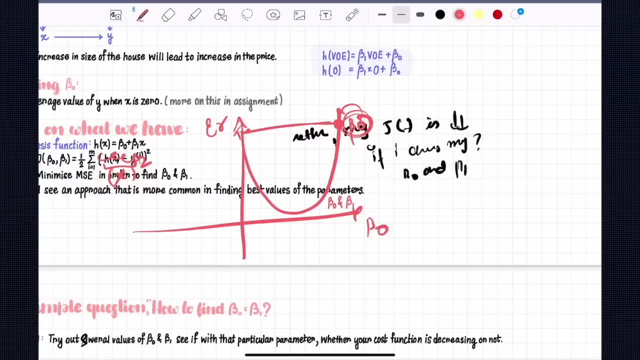 where error with this beta zero is very, where error with this beta zero is very high, high, high. error with that particular beta zero is error with that particular beta zero, is error with that particular beta zero is very, very high, very, very high, very, very high. if beta zero is over here, if beta zero is. 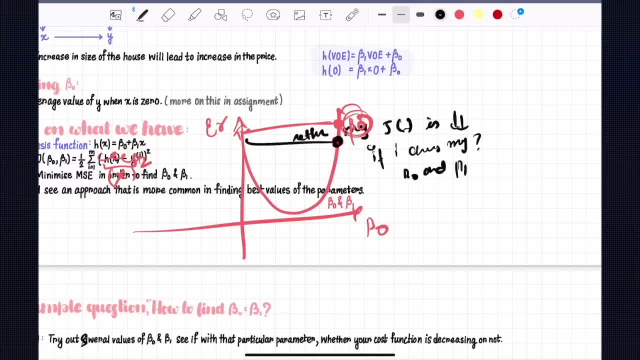 if beta zero is over here, if beta zero is. if beta zero is over here, if beta zero is over here. over here, over here. error is bit low. the previous one. if error is bit low, the previous one. if error is bit low the previous one. if beta zero is over here, error is bit low. 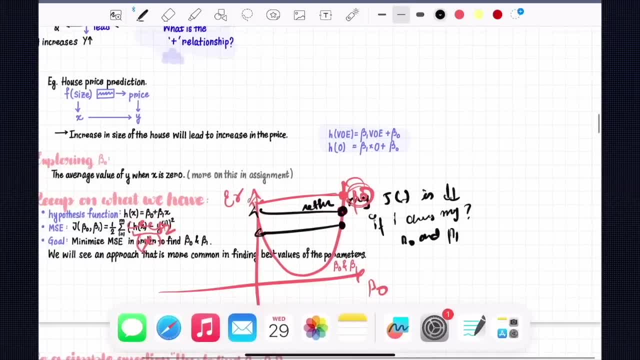 beta zero is over here. error is bit low. beta zero is over here. error is bit low then. so this represents this. uh, the x then. so this represents this. uh, the x then. so this represents this. uh, the x. axis represents the beta, the values of axis represents the beta, the values of. 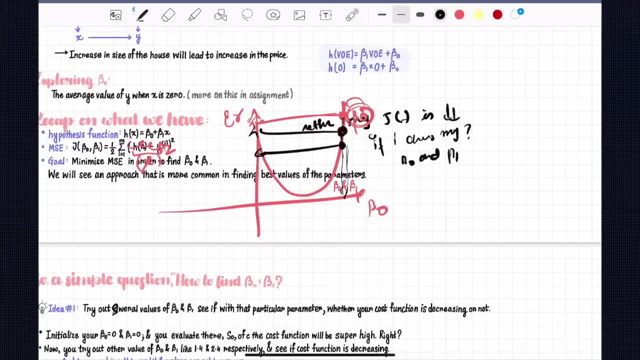 axis represents the beta, the values of beta: 1 beta- sorry beta 0. and y- beta 1 beta- sorry beta 0. and y beta 1 beta- sorry beta 0. and y represents the error. y represents the represents the error. y represents the represents the error. y represents the error. okay, so over here what our goal. 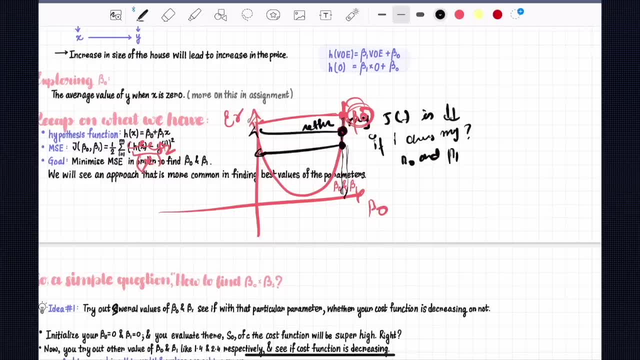 error. okay, so over here what our goal error. okay, so over here what our goal should be. our goal should be to to get. should be. our goal should be to to get. should be. our goal should be to to get the beta, to get that beta. value to get. 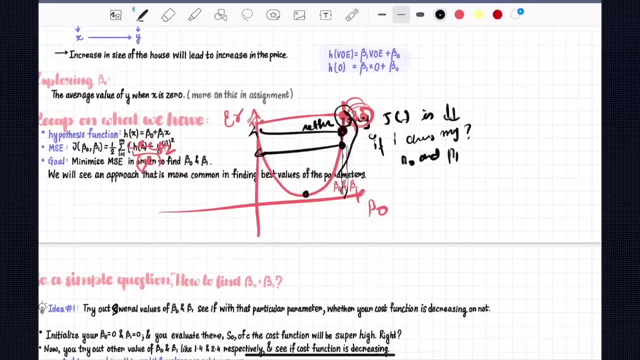 the beta to get that beta value, to get the beta to get that beta value, to get that beta value over. we, we want to get that beta value over. we, we want to get that beta value over. we, we want to get that beta from here to here, so that our 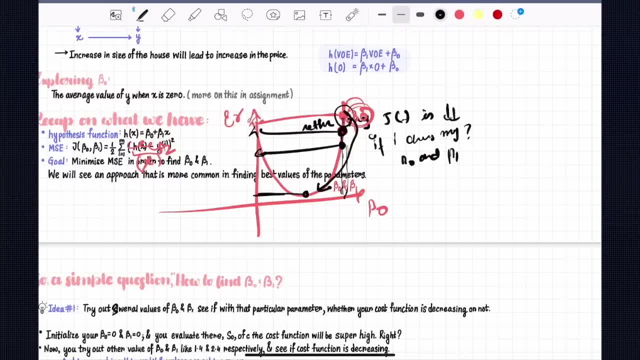 that beta from here to here, so that our that beta from here to here, so that our error is very, very less approximately. error is very, very less approximately. error is very, very less approximately. equals to zero, equals to zero, equals to zero. so eventually we want to get. so assume. 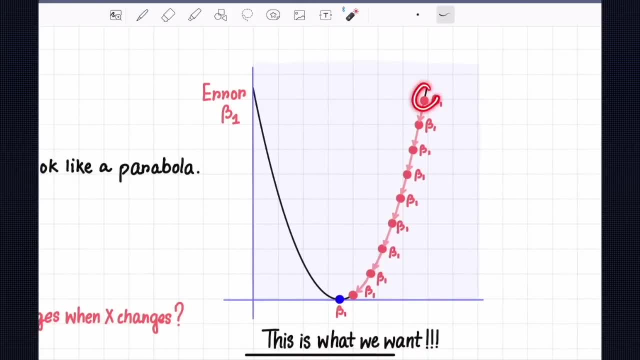 so eventually we want to get. so assume so, eventually we want to get. so assume that this is a beta one, that this is a beta one, that this is a beta one, this is a beta one, and then over when, when the, and then over when, when the. 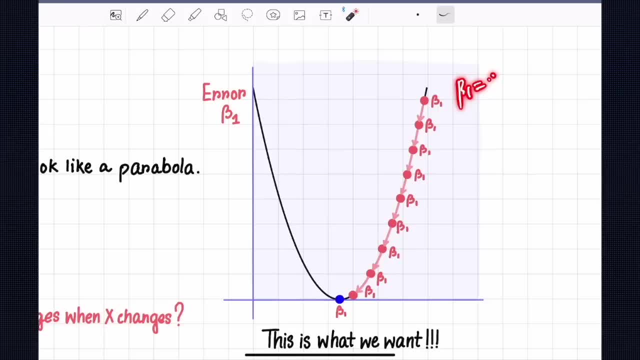 and then over when, when the beta one is over. let us assume beta one is. beta one is over. let us assume beta one is beta one is over. let us assume beta one is something like something like something like um four. beta one is something like four um four. beta one is something like four. 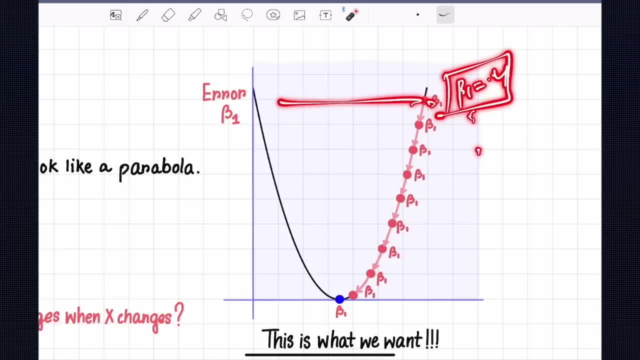 um, four beta one is something like four. okay, beta one is something like four. okay, beta one is something like four. okay, beta one is something like four. so what will be the error? error will be, so what will be the error? error will be, so what will be the error? error will be super duper high. 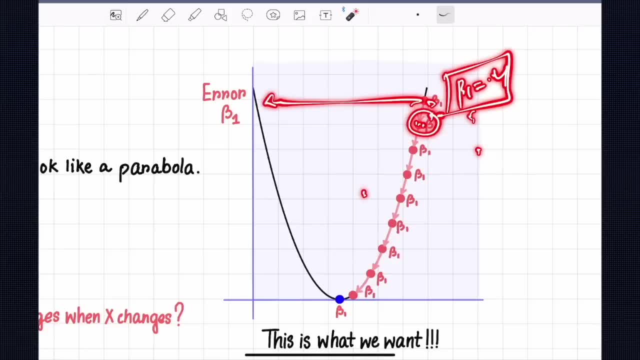 super duper high, super duper, high, beta one. so now you have beta one as beta one. so now you have beta one as beta one. so now you have beta one as a little bit less than, or maybe uh, a little bit less than, or maybe uh. 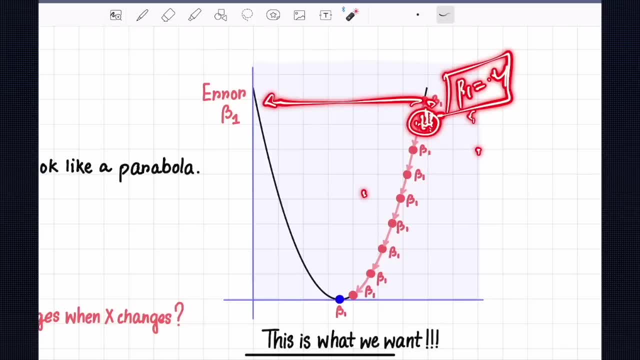 a little bit less than, or maybe uh, something like that. so bb beta one is something like that. so bb, beta one is something like that. so bb, beta one is oh. in this case, beta one is oh. in this case, beta one is oh. in this case, beta one is less than the previous one. the error is: 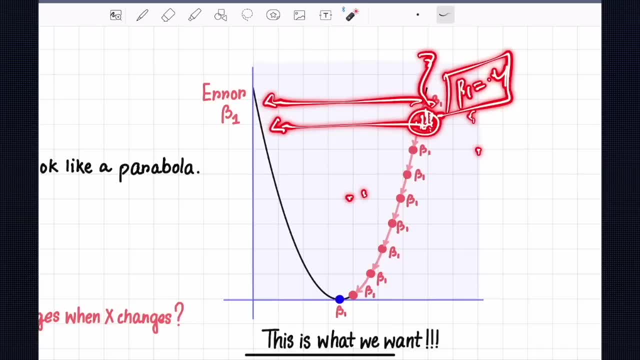 less than the previous one. the error is less than the previous one. the error is also less, also less, also less. i'm just taking an example. it can be. i'm just taking an example. it can be. i'm just taking an example. it can be more as well. 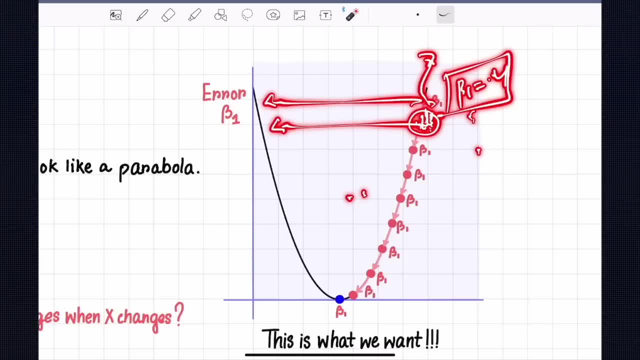 more as well, more as well. it can be more as well. don't worry, don't it can be more as well, don't worry, don't, it can be more as well, don't worry. don't worry about anything. worry about anything, worry about anything. currently, it's a very simplest example. 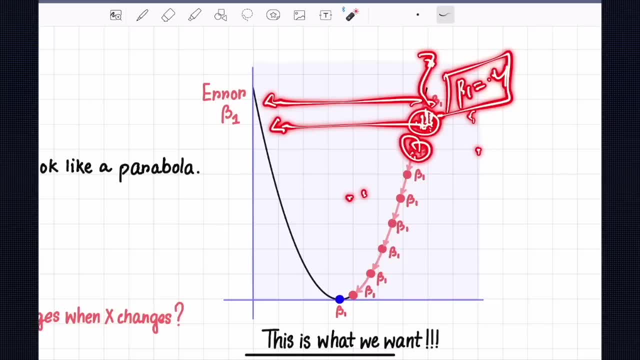 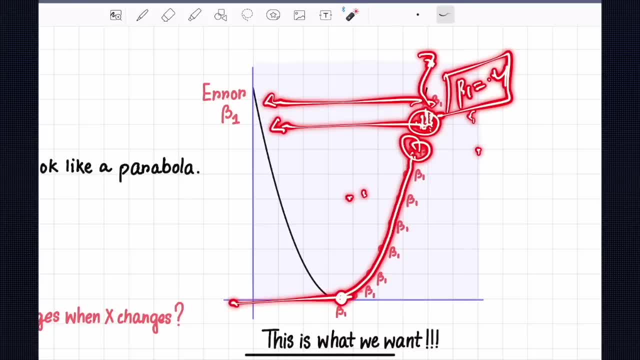 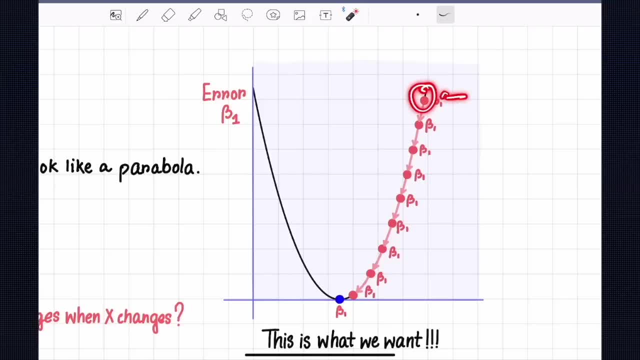 global minima where your error is very global minima where your error is very, very less. where is negligible? so you very less. where is negligible? so you very less. where is negligible. so you know, start with the beta value whose. know, start with the beta value whose. 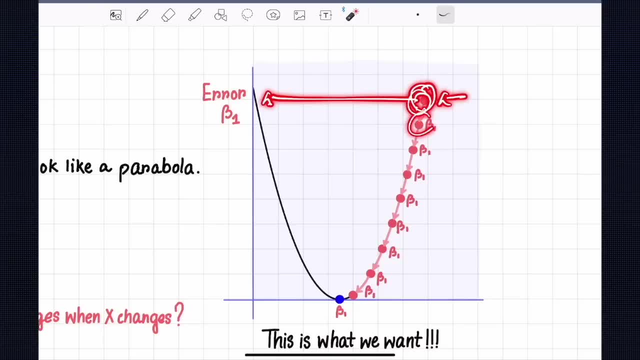 know, start with the beta value whose error is very, very high, and then you error is very, very high, and then you error is very, very high, and then you have to learn the beta value on a chain. have to learn the beta value on a chain. have to learn the beta value on a chain. keep on changing the beta value so you're. 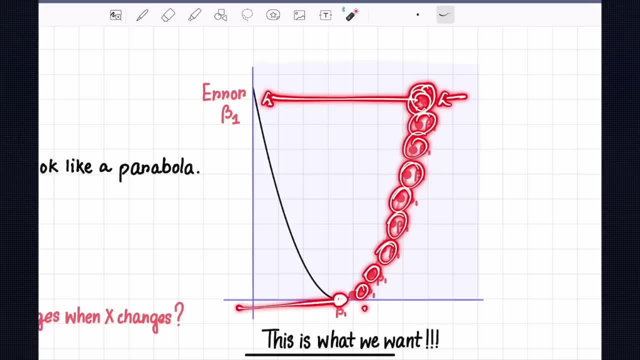 keep on changing the beta value. so you're keep on changing the beta value. so you're seeing that we are changing this, seeing that we are changing this, seeing that we are changing this: definitely with the beta values, until definitely with the beta values, until definitely with the beta values, until, unless our error is nothing but equals. 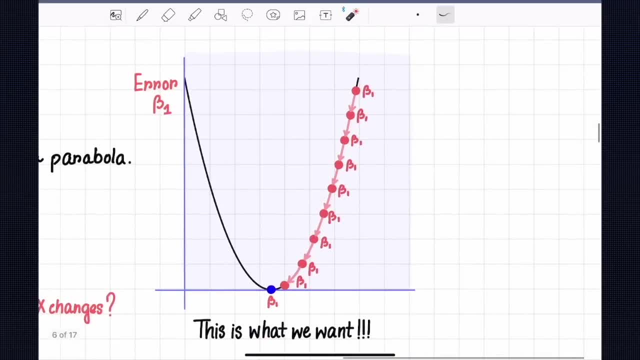 unless our error is nothing but equals, unless our error is nothing but equals to zero to zero to zero. okay, i hope that you're getting what i'm okay. i hope that you're getting what i'm okay. i hope that you're getting what i'm trying to convey. i'm just trying to convey. 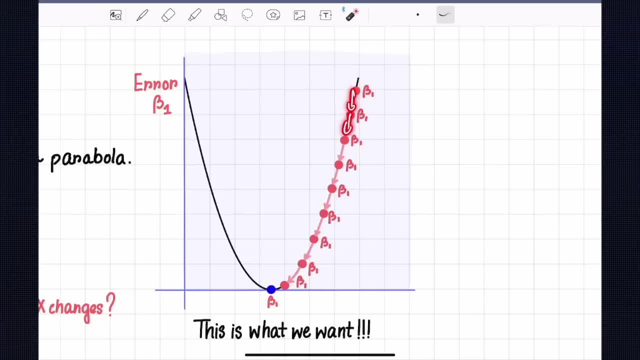 trying to convey. i'm just trying to convey. trying to convey that you know, keep on changing beta value. that you know. keep on changing beta value. that you know, keep on changing beta value. you keep on changing the middle value, you keep on changing the middle value. you keep on changing the middle value. that will help us. that will help us to. 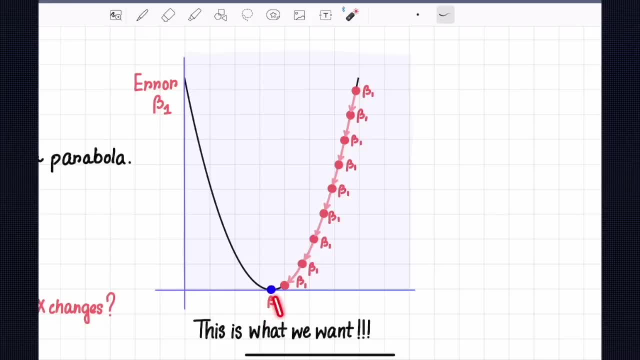 that will help us. that will help us to. that will help us. that will help us to get your beta. that that will help you get your beta. that that will help you get your beta. that that will help you. that that that will help you to get beta. 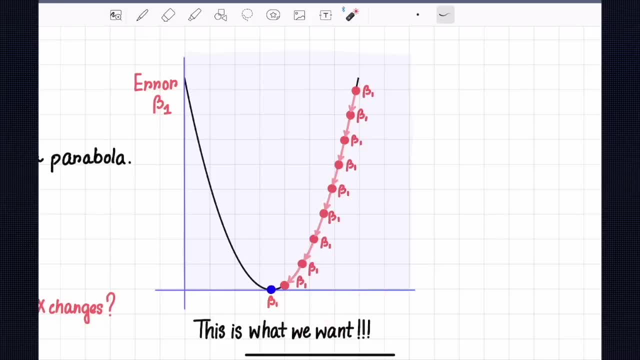 that that that will help you to get beta. that that that will help you to get beta. one equals two. so, uh, beta one. the one equals two. so, uh, beta one. the one equals two. so uh, beta one. the error of beta one is equals to zero. error of beta one is equals to zero. 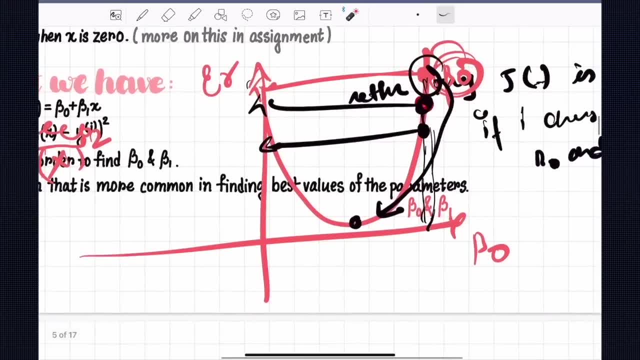 error of beta one is equals to zero. okay, i hope that you, that, that you are okay. i hope that you, that you are okay, i hope that you, that you are getting. so how can we take out the rate getting? so how can we take out the rate? 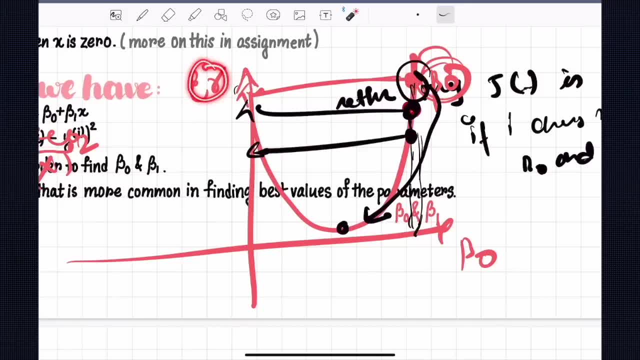 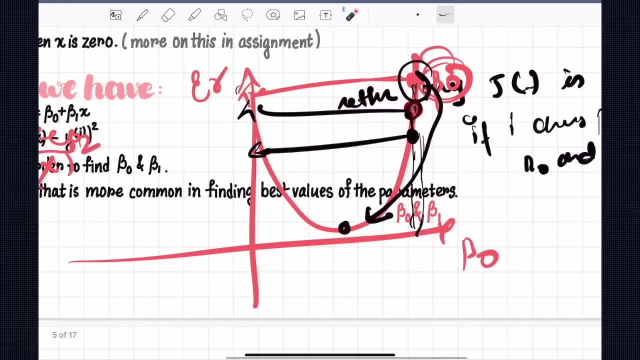 of change. so how much your error changes. so when, when your beta beta beta zero. so when when your beta beta beta zero. so when when your beta beta beta zero changes, how much you're at how much your changes? how much you're at how much your changes, how much you're at how much your error changes when beta 0 at this, 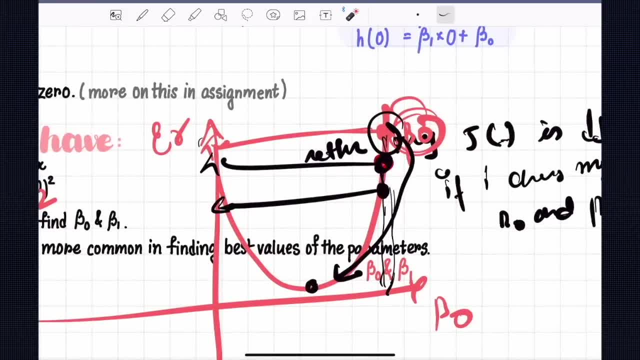 error changes. when beta 0 at this error changes, when beta 0 at this particular point changes, beta 0 will be particular point changes. beta 0 will be particular point changes. beta 0 will be same. will will be not same, it will be same. will will be not same, it will be. 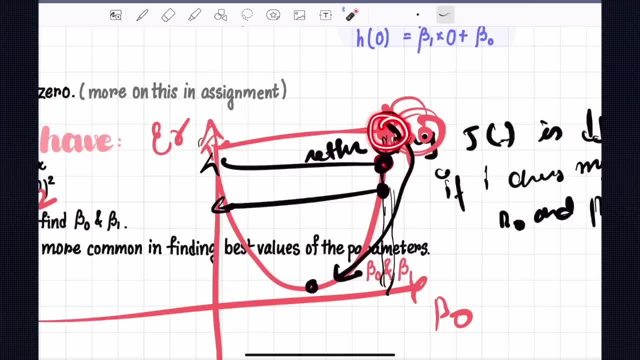 same will will be not same, it will be changing right. so what will the what changing right? so what will the what changing right? so what will the what will they change in error? when at this will they change in error when at this will they change in error when at this particular point? so what is, what is the? 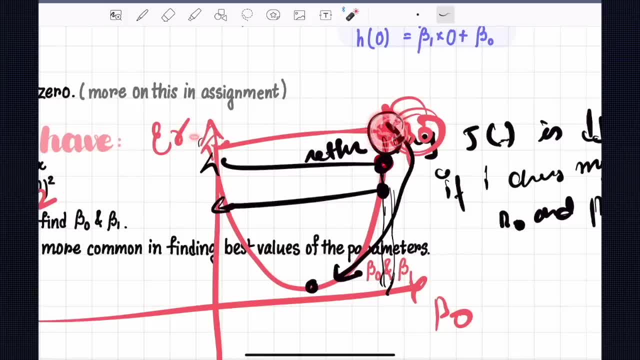 particular point. so what is what is the particular point? so what is what is the derivative of your error with respect to derivative of your error, with respect to derivative of your error with respect to this beta zero at this particular point, this beta zero at this particular point? 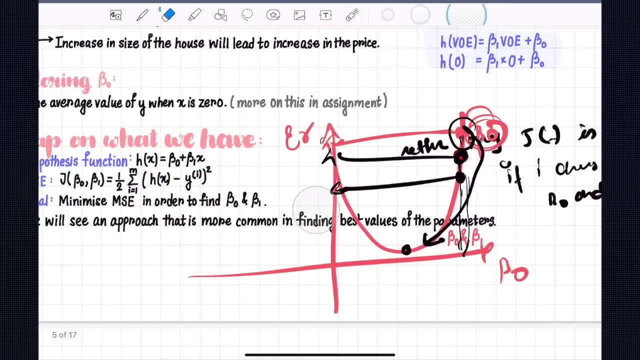 this beta zero at this particular point. okay, okay, okay. so let's uh uh so it. it will be more so. let's uh uh so it. it will be more so. let's uh uh so it. it will be more clear once we uh. so let's uh uh so it will be more clear once we uh. 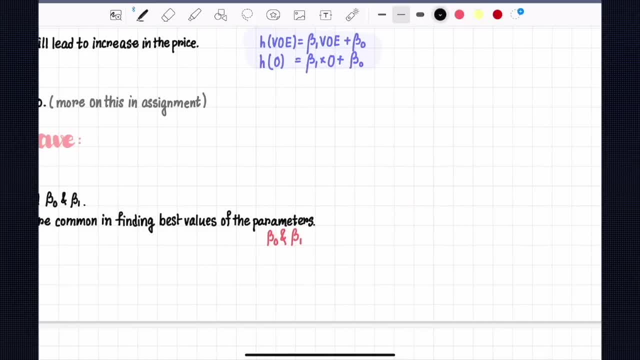 so let's uh, uh, so it will be more clear once we uh understand more in mathematical, understand more in mathematical, understand more in mathematical perspective, but eventually what our perspective, but eventually what our perspective, but eventually what our derivative is telling. it is telling that derivative is telling. it is telling that. 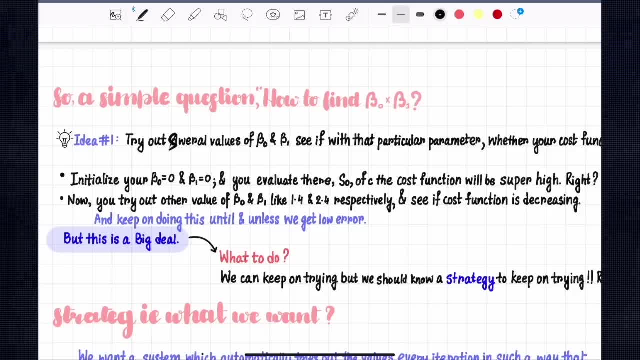 derivative is telling. it is telling that how much your dairy, how much your, how much your dairy, how much your, how much your dairy, how much your cost, function or error will change if you cost. function or error will change if you cost. function or error will change if you change your beta a little bit. 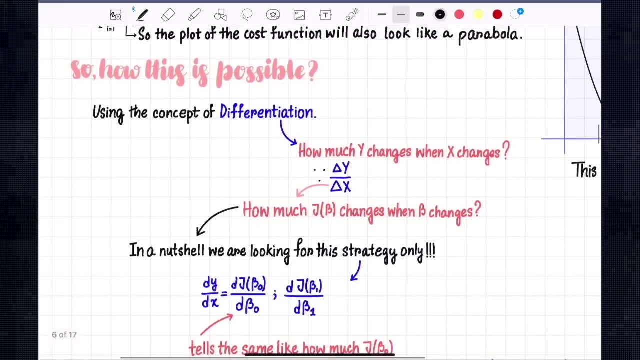 change your beta a little bit. change your beta a little bit, okay, okay, okay, can you change your beta a little bit? can you change your beta a little bit? can you change your beta a little bit? so we use the concept of differentiation. so we use the concept of differentiation. 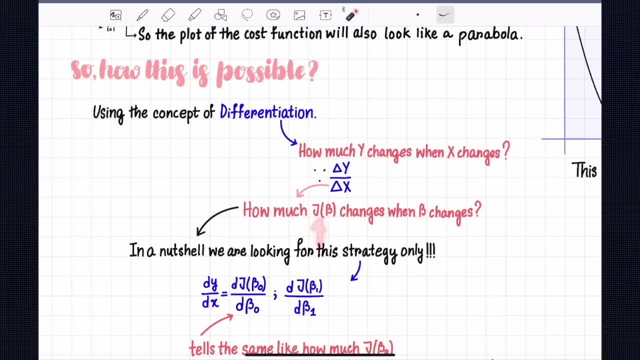 so we use the concept of differentiation, which is how much y changes when x. which is how much y changes when x. which is how much y changes when x changes with the key. how much your error changes with the key. how much your error changes with the key. how much your error will change when your beta changes. 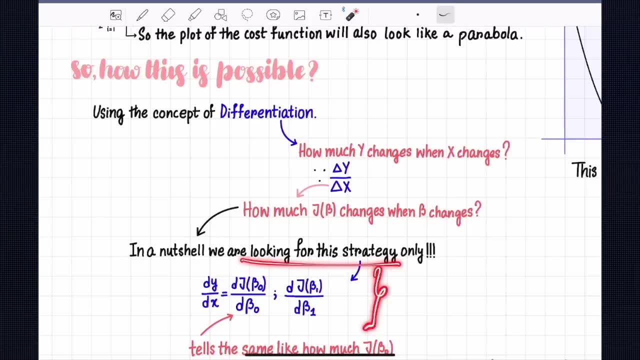 will change when your beta changes, will change when your beta changes. so, in a nutshell, we are looking for this. so, in a nutshell, we are looking for this. so, in a nutshell, we are looking for this strategy only. we are just looking for strategy only. we are just looking for. 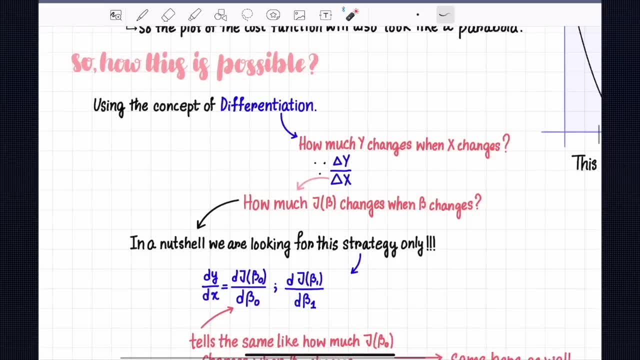 strategy only. we are just looking for the strategy where we can take a look, if the strategy where we can take a look, if the strategy where we can take a look, if this something increases or decreases, this something increases or decreases, this something increases or decreases, we're just looking for that strategy and 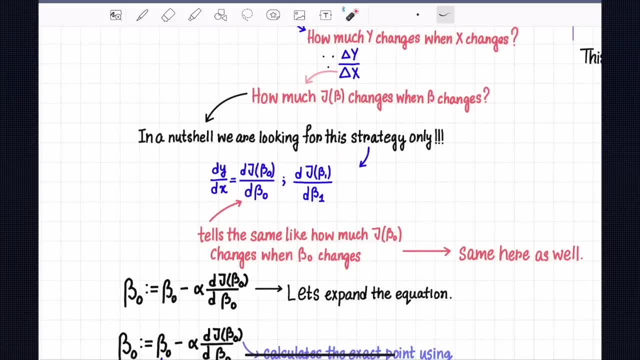 we're just looking for that strategy, and we're just looking for that strategy. and here we go, here we go. so here we go, here we go, here we go, so here we go, here we go, here we go. so here we go. where it tests the dy by dx, where you're. where it tests the dy by dx, where you're, where it tests the dy by dx, where you're taking out that, where, where, where we taking out that, where, where, where we taking out that where, where, where. where we have when, when you take out the strat, have when, when you take out the strat. 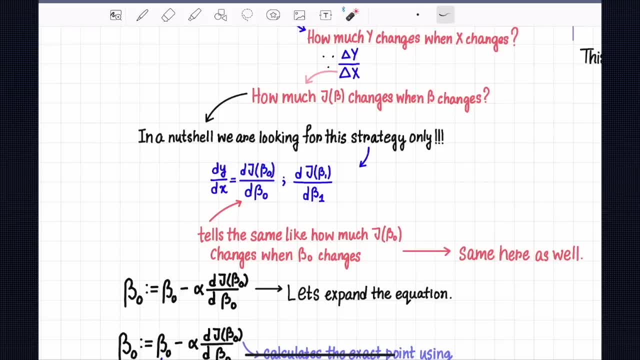 have when, when you take out the strat, when you you have to do for individually, when you you have to do for individually, when you you have to do for individually for different different parameters, for different different parameters, for different different parameters, because you have two parameters beta, because you have two parameters beta. 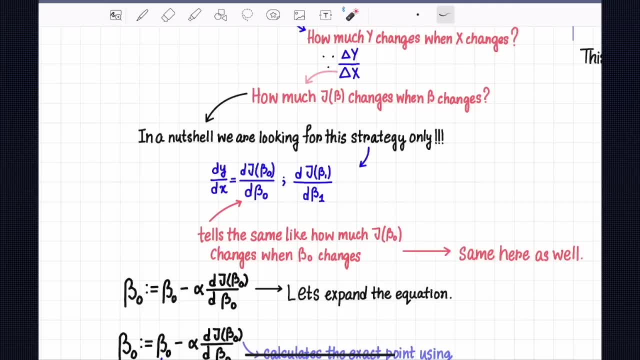 because you have two parameters: beta zero and beta. one right. beta beta zero, zero and beta one right. beta beta zero zero and beta one right, beta beta zero. various- one is slope and one is biased various. one is slope and one is biased various- one is slope and one is biased term, but it's not something like it's. 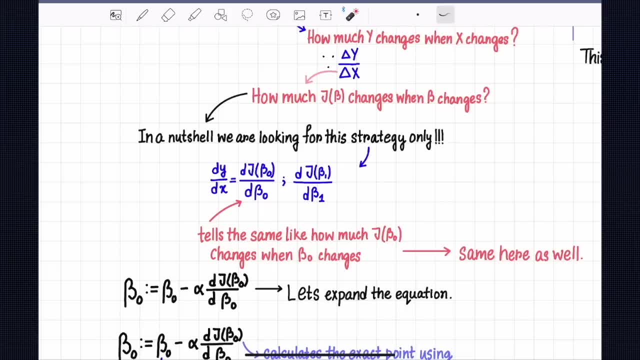 term, but it's not something like it's term. but it's not something like it's the best of now, but over here is the is the best of now, but over here is the is the best of now, but over here is the is the optimization problem. so you 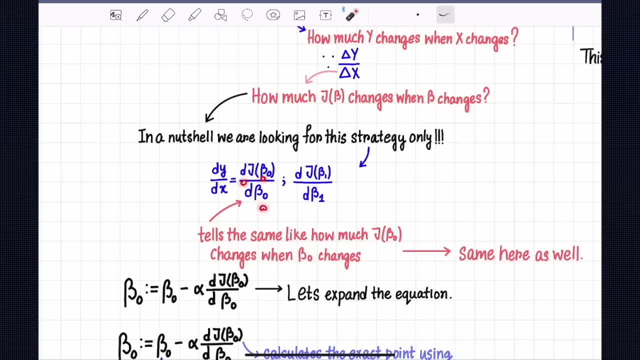 the optimization problem. so you the optimization problem, so you eventually take out the derivative of. eventually take out the derivative of. eventually take out the derivative of your cost function with respect to beta, your cost function with respect to beta, your cost function with respect to beta zero and derivative of the cost function. 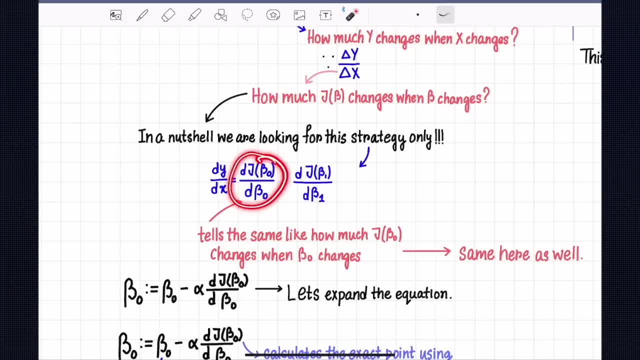 zero and derivative of the cost function. zero and derivative of the cost function with respect to beta one. because you, with respect to beta one, because you, with respect to beta one, because you have to do so, it tells you it, this tells: have to do so. it tells you it, this tells. 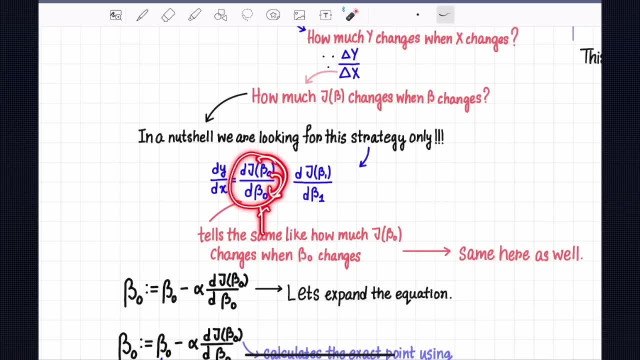 have to do so. it tells you it. this tells you how much your cost function. will you how much your cost function will you how much your cost function will change if you change beta zero a little change, if you change beta zero a little change, if you change beta zero a little bit, how much this cost function will. 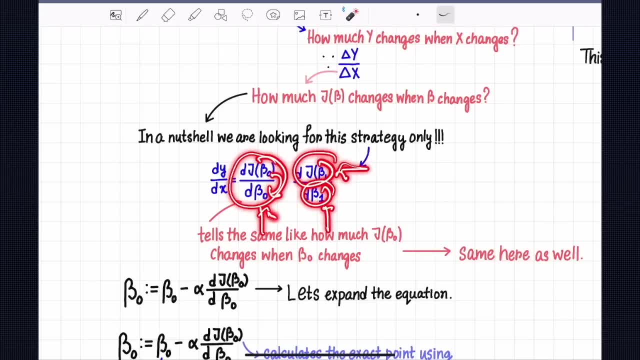 bit how much this cost function will bit how much this cost function will change when you change beta one a little change when you change beta one a little change when you change beta one a little bit. so if that changes, if this it it it bit. so if that changes, if this it it it, 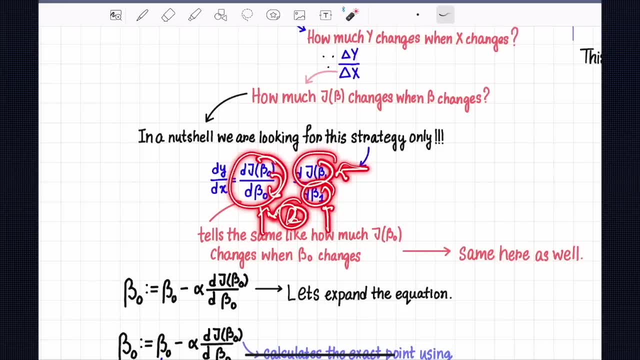 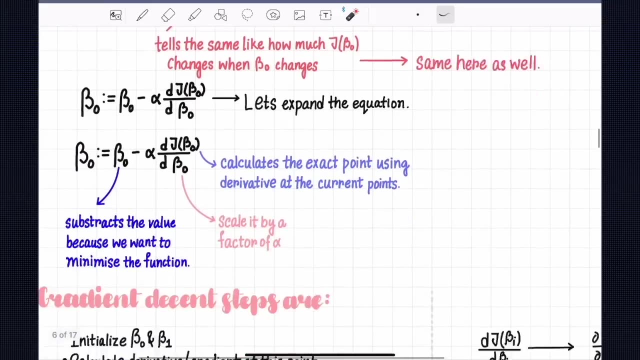 bit. so if that changes, if this it, it, it will happen in every iteration. so the will happen in every iteration. so the will happen in every iteration. so the second iteration: assume that it changes. second iteration: assume that it changes. second iteration: assume that it changes. i hope that you're getting what exactly? 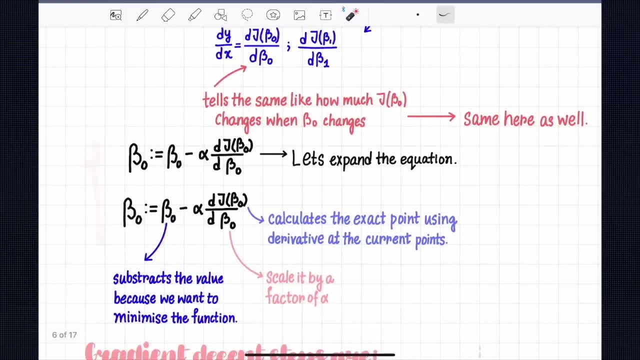 i hope that you're getting what exactly. i hope that you're getting what exactly i'm trying to convey. i'm trying to convey. i'm trying to convey now. here's your algorithm. here's your now. here's your algorithm. here's your now. here's your algorithm. here's your algorithm. here's your algorithm. 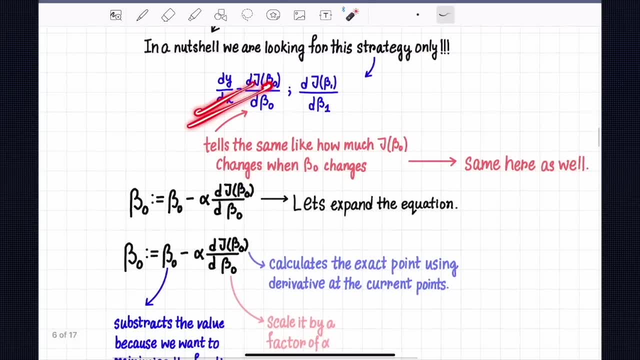 algorithm. here's your algorithm algorithm. here's your algorithm: um for updation. like you get a change: um for updation. like you get a change um for updation. like you get a change: now you get a change. now you have to. now you get a change, now you have to. 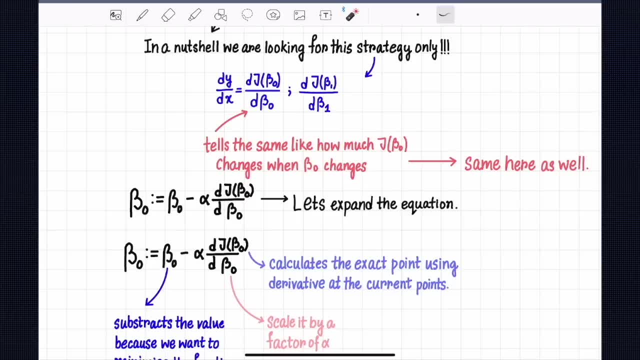 now you get a change. now you have to update. now you have to update your values. update now, you have to update your values. update now you have to update your values as well. and then you look for another as well, and then you look for another as well, and then you look for another beta value, right, so you update the. 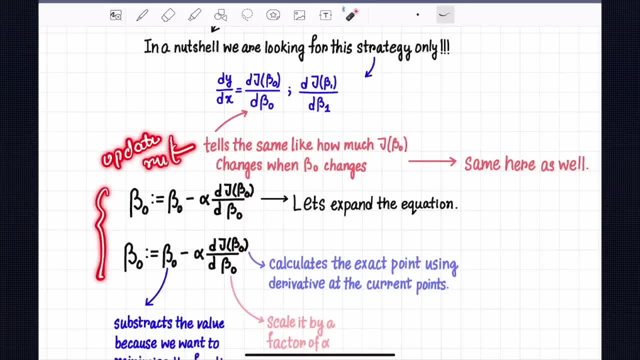 beta value. right, so you update the beta value. right, so you update the. this is: this is called the update rule. this is: this is called the update rule. this is: this is called the update rule. this is called the. this is called the update rule. this is called the. 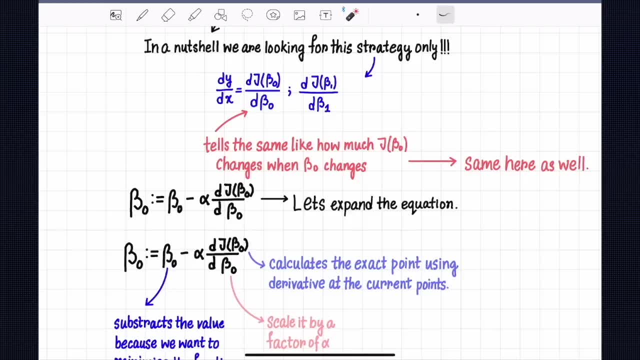 this is called the update, update, update rule, where you first of all update, update, update rule. where you first of all update, update, update rule. where you first of all update beta 0 with old beta. so update beta 0 with old beta, so update beta 0 with old beta. so basically, you have a new, new beta 0. 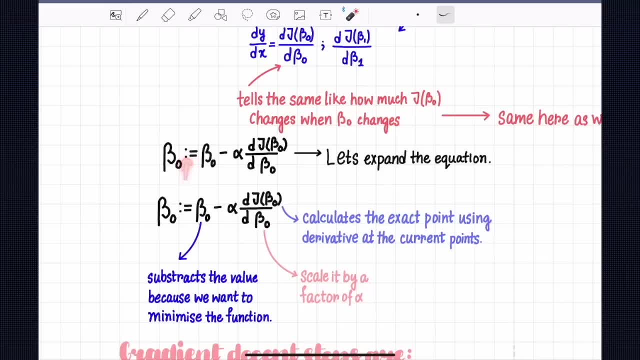 basically you have a new, new beta 0. basically you have a new, new beta 0, new beta 0. and then you assign this: we, new beta 0. and then you assign this: we, new beta 0. and then you assign this: we. this is assignment operator, where you 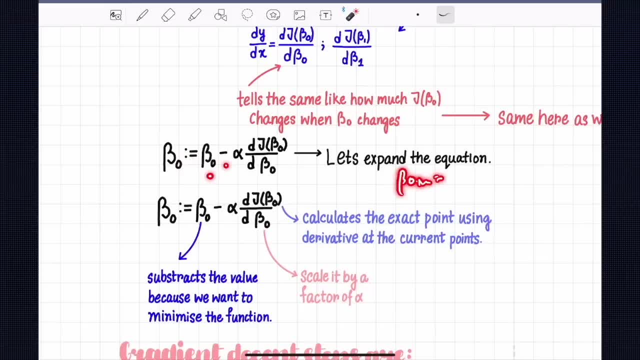 this is assignment operator where you- this is assignment operator where you have new beta. new beta is equals to old. have new beta: new beta is equals to old. have new beta. new beta is equals to old beta minus the learning rate and I'll. beta minus the learning rate and I'll. 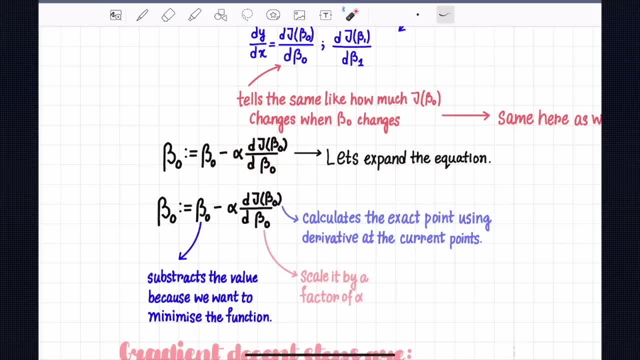 beta minus the learning rate, and I'll talk about that times. the change in X. talk about that times, the change in X. talk about that times, the change in X with respect to the, the change in your with respect to the, the change in your with respect to the, the change in your cost function. how much your day of the. 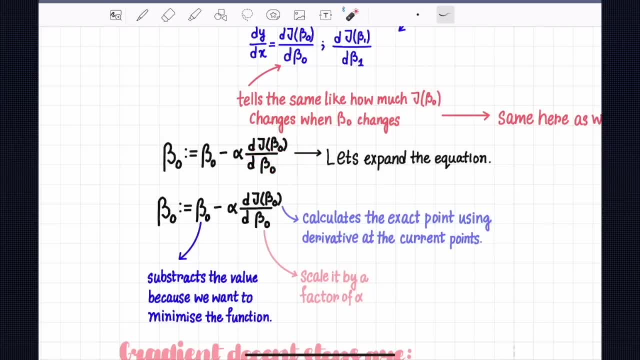 cost function. how much your day of the cost function. how much your day of the. how much of error changes when beta 0? how much of error changes when beta 0? how much of error changes when beta 0? changes will expand. this will will take. changes will expand. this will will take. 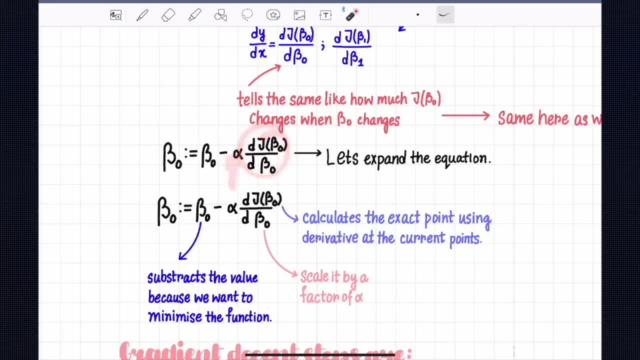 changes will expand. this will will take out the derivative- adjust a second. but out the derivative: adjust a second, but out the derivative, adjust a second. but assume that so we multiply the learning. assume that so we multiply the learning. assume that so we multiply the learning rate with this. so what is learning rate? 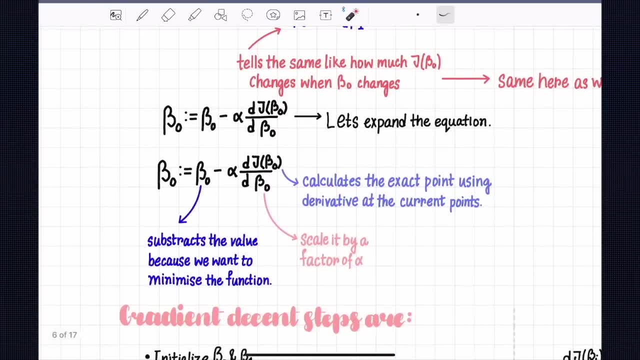 rate with this? so what is learning rate rate with this? so what is learning rate? what is learning rate, so, but, but before? what is learning rate, so, but, but before, what is learning rate, so, but, but before that will, will, will, will talk about that, that will, will, will, will talk about that. 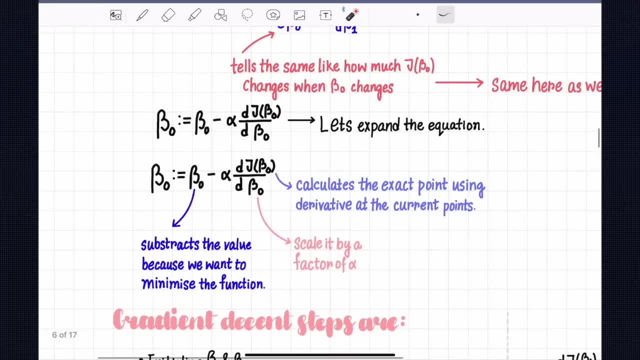 that will, will, will will talk about that learning rate later on. but let's let's learning rate later on. but let's let's learning rate later on. but let's, let's stick at some point over here. beta 0 is. stick at some point over here. beta 0 is. 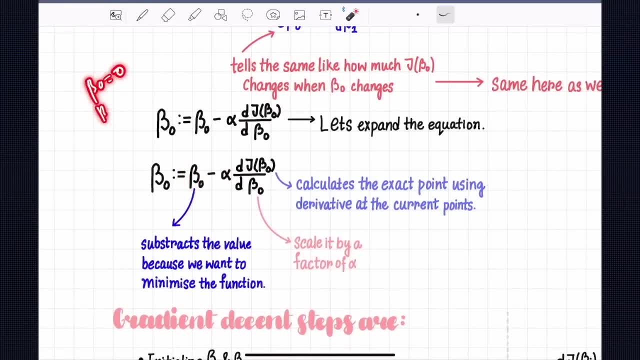 stick at some point over here beta 0 is. is the old beta 0, like over here? if you is the old beta 0, like over here. if you is the old beta 0, like over here. if you have beta 0 to be 0 and beta 1 is also. have beta 0 to be 0 and beta 1 is also. have beta 0 to be 0 and beta 1 is also 0, then this is the old is now we have the 0. then this is the old is now we have the. 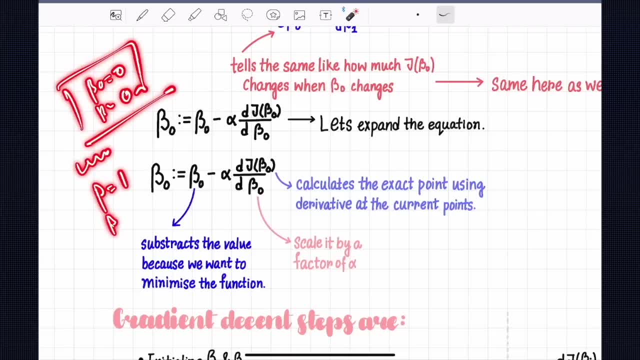 0. then this is the old is. now we have the second iteration, second side. second second iteration, second side. second second iteration, second side. second iteration here: beta 1- beta. so you have iteration here. beta 1, beta. so you have iteration here: beta 1, beta. so you have been new beta and you have to take out. 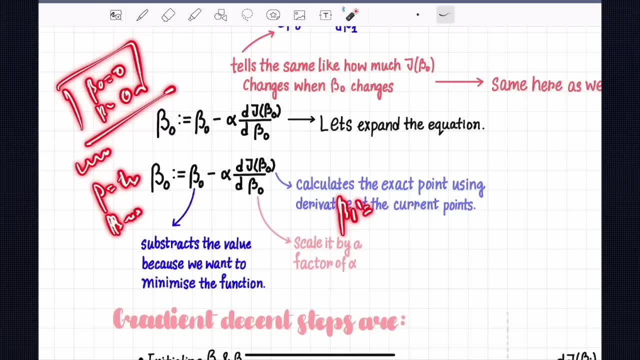 been new beta and you have to take out been new beta and you have to take out the new beta, so you have the when you the new beta, so you have the when you the new beta, so you have the when you actually convert beta 1. is you be assume? 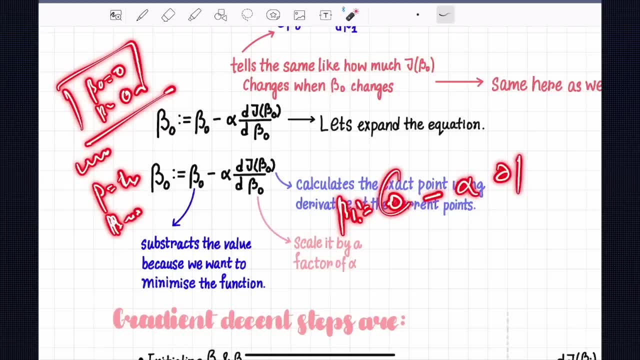 actually convert beta 1? is you be assume actually convert beta 1? is you be assume that you have a 0 minus the learning, that you have a 0 minus the learning, that you have a 0 minus the learning, that alpha the respect. so basically this: 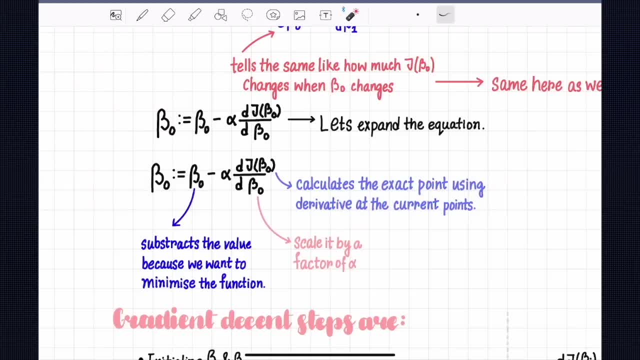 that alpha the respect. so basically this: that alpha the respect. so basically this is a old old be task over to previous. is a old old be task over to previous. is a old old be task over to previous one? the P, the previous beta. okay, the old one. the P- the previous beta. okay, the old. 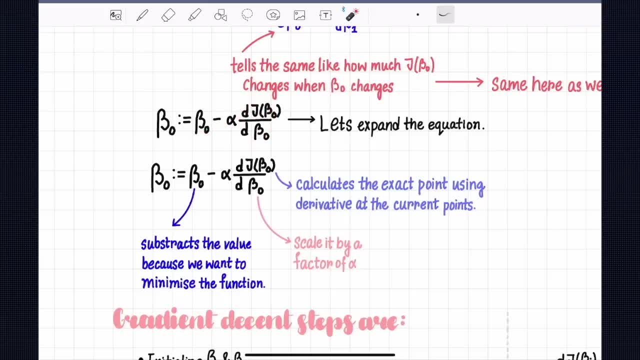 one, the P, the previous beta, okay, the old beta minus the learning that alpha and beta minus the learning that alpha and beta minus the learning that alpha. and this change: change of rate of change of this change. change of rate of change of this change. change of rate of change of rate of cost function with respect to: 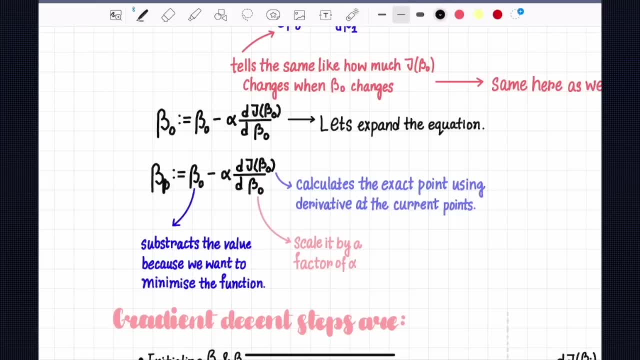 rate of cost function. with respect to rate of cost function with respect to this beta 0, and then you do for beta 1, this beta 0, and then you do for beta 1, this beta 0, and then you do for beta 1 as well. I'm so sorry, this, this, this should. 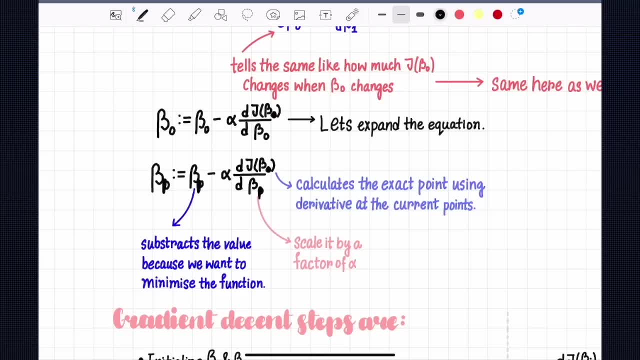 as well. I'm so sorry this, this, this should as well. I'm so sorry this. this: this should be beta 1. this should be beta 1. okay, be beta 1. this should be beta 1. okay, be beta 1. this should be beta 1. okay, this should be beta 1. now over here, oh. 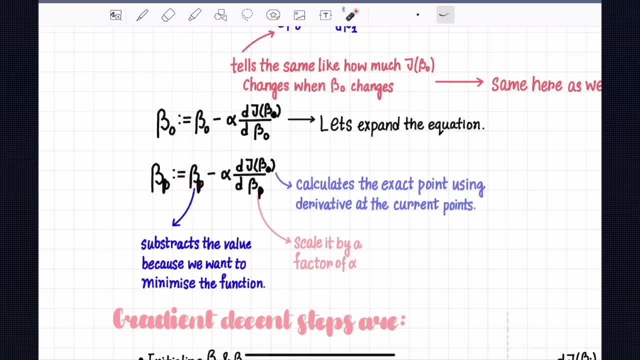 this should be beta 1 now over here. oh, this should be beta 1 now over here. oh, yeah, so now you may have several. yeah, so now you may have several. yeah, so now you may have several questions. the first question is: would be questions. the first question is: would be: 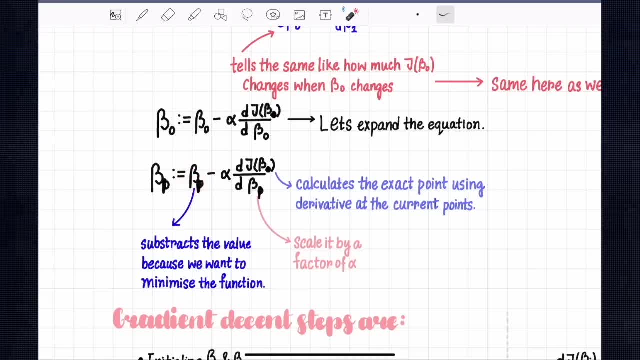 questions. the first question is would be: why are you subtracting our old beta, the? why are you subtracting our old beta, the? why are you subtracting our old beta? the reason why you're subtracting because? reason why you're subtracting because? reason why you're subtracting: because we want to minimize our function, right. 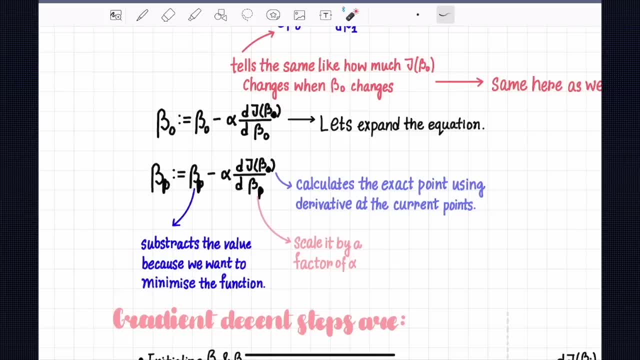 we want to minimize our function, right. we want to minimize our function, right. one way to think about it: it's, it's, it's one way to think about it. it's, it's, it's one way to think about it. it's, it's, it's. it's not something legal, but we can. 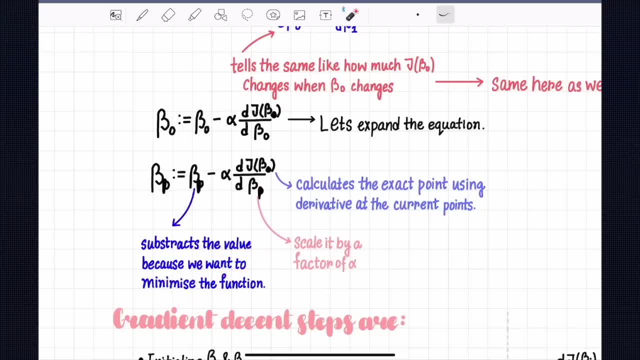 it's not something legal, but we can. it's not something legal, but we can think about that. we are to minimize our think about that. we are to minimize our think about that. we are to minimize our function rate and we want to go down and function rate and we want to go down and. 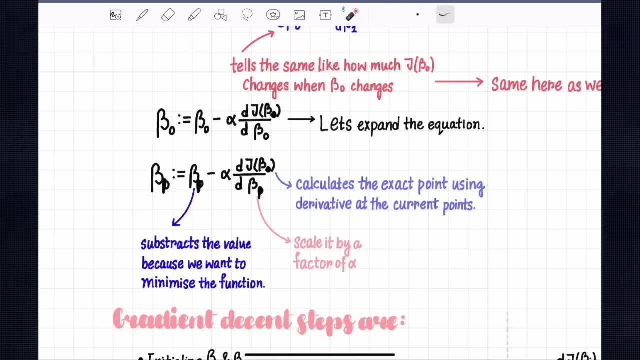 function rate and we want to go down and minimize our function so that our error minimize our function, so that our error minimize our function, so that our error is less so we are to minimize. that's why is less so we are to minimize. that's why is less so we are to minimize. that's why we subtract many, if anything, you to 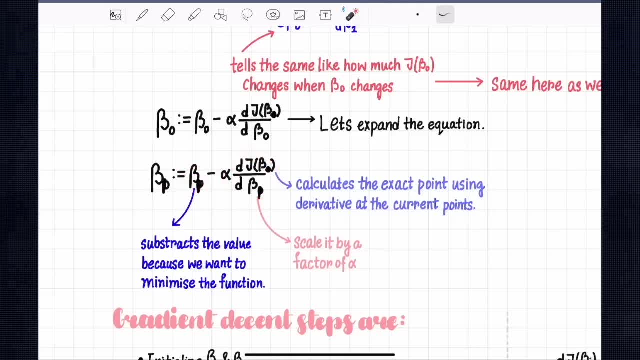 we subtract many. if anything you to, we subtract many if anything you to minimize or to subtract. and then it will minimize or to subtract, and then it will minimize or to subtract, and then it will tell you: it will get this, this change. tell you, it will get this, this change. 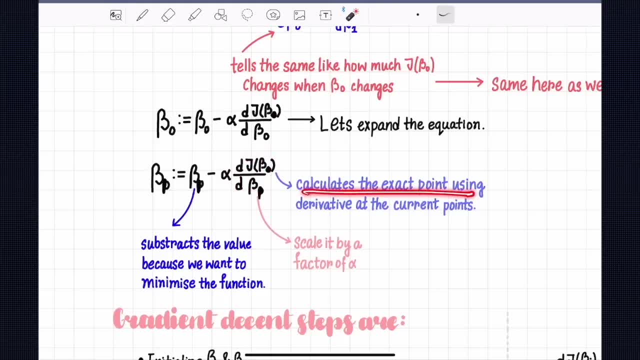 tell you it will get this. this change this. this calculates the change it. this: this calculates the change it. this: this calculates the change. it calculates the exact points using. calculates the exact points using. calculates the exact points using. derivatives at the current points: okay, derivatives at the current points, okay. 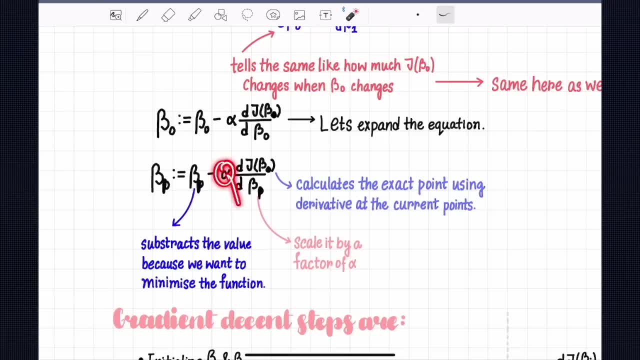 derivatives at the current points. okay, and of course it is this the change, and, and of course it is this the change, and and of course it is this the change. and we were learning that alpha which is, we were learning that alpha which is, we were learning that alpha which is nothing, which is nothing which is. 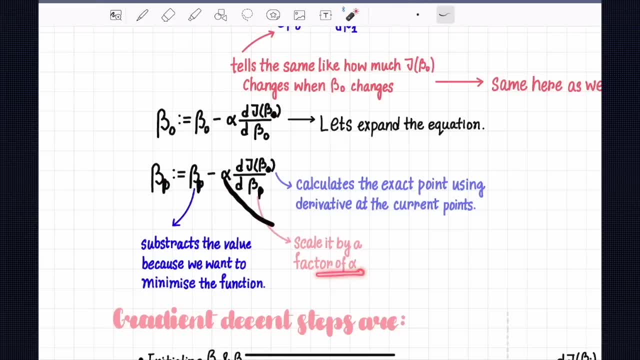 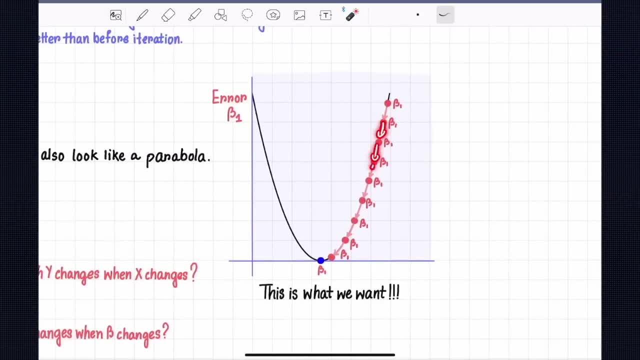 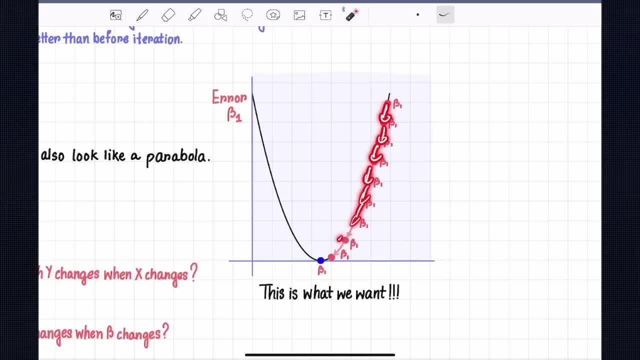 you're going down at a certain rate. so you're going down at a certain rate. so the rate of going down, the rate of going, the rate of going down, the rate of going, the rate of going down, the rate of reaching to a global minima is nothing. 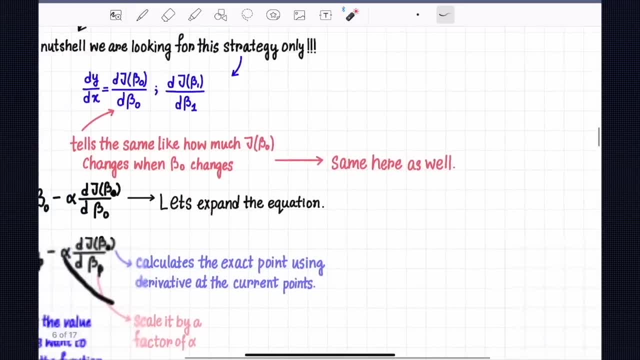 reaching to a global minima is nothing. reaching to a global minima is nothing but called the learning rate. okay, it's, but called the learning rate. okay, it's, but called the learning rate. okay, it's something, but called the learning rate. something but called the learning rate. 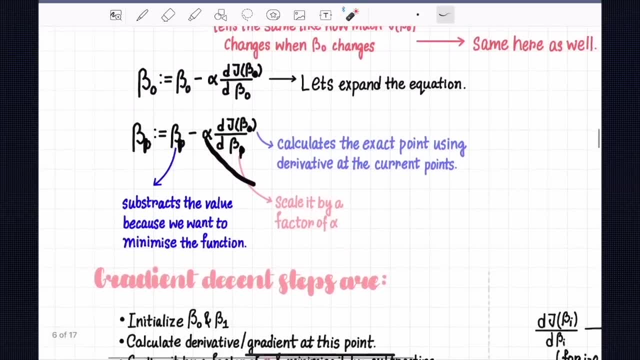 something but called the learning rate, the rate or by which we going we, we, we. the rate or by which we going we, we, we, the rate or by which we going we, we. we learn with the, the, the read by which we learn with the, the, the read by which we. learn with the, the. the read by which we learn is also known as learning. it will learn is also known as learning. it will learn is also known as learning. it will take a look at. we'll take a. we'll have a. take a look at. we'll take a. we'll have a. 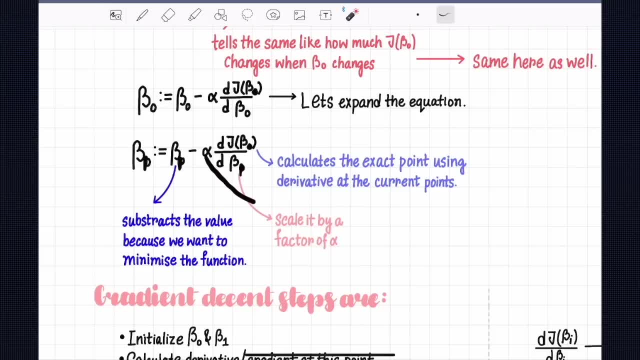 take a look at. we'll take a. we'll have a separate video on the learning rate, separate video on the learning rate, separate video on the learning rate. we'll talk about some of the best cases. we'll talk about some of the best cases. we'll talk about some of the best cases and cases of learning that in great 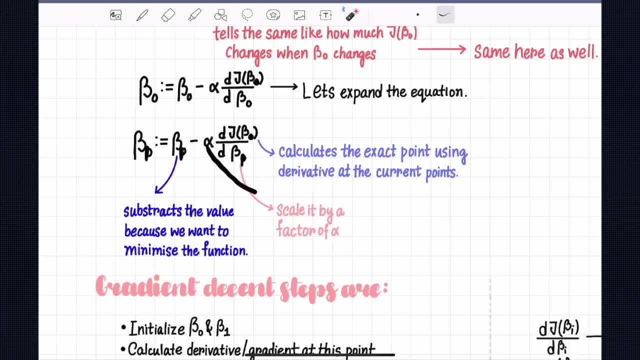 and cases of learning that in great and cases of learning that in great detail. but even assume, as of now it's detail. but even assume as of now it's detail, but even assume, as of now it's case, the fact it scales the scene by the case, the fact it scales the scene by the. 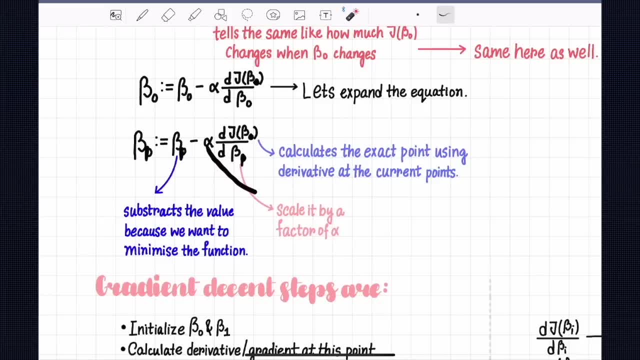 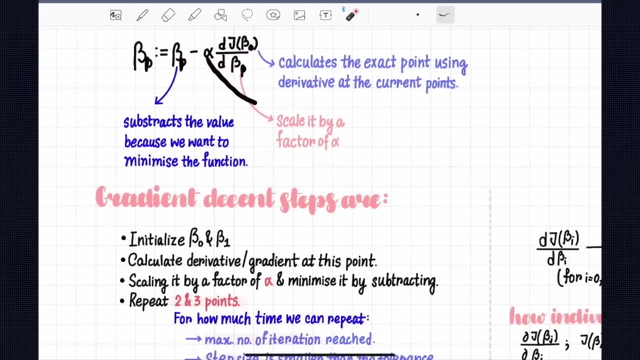 case, the fact it scales the scene by the factor of alpha and that is the rate factor of alpha, and that is the rate factor of alpha, and that is the rate of learning in a geometrical perspective, I of learning in a geometrical perspective, I of learning in a geometrical perspective. I hope you are understanding. cool, let's. 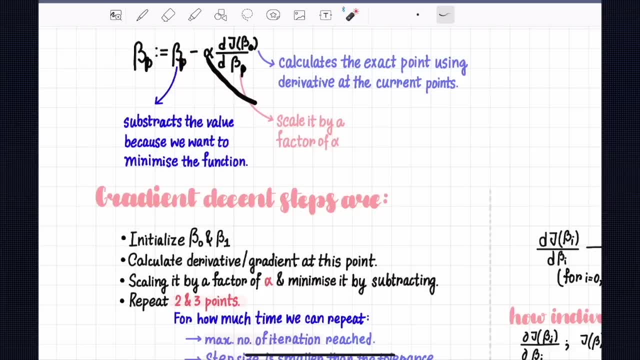 hope you are understanding cool. let's hope you are understanding cool. let's get started. huh so the. what are the get started? huh so the. what are the get started? huh so the. what are the steps? it is to summarize, you initialize steps. it is to summarize, you initialize. 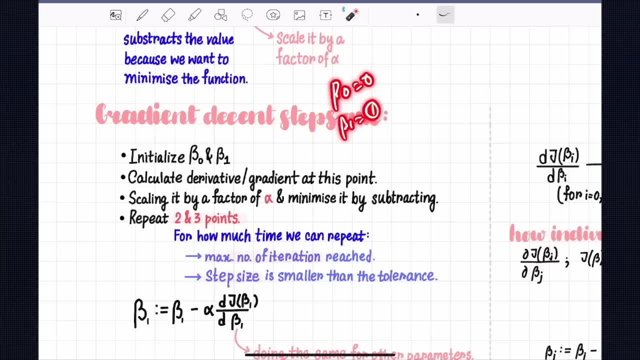 steps. it is to summarize. you initialize your beta 0 to Ben. beta 1 equals to 0. your beta 0 to Ben: beta 1 equals to 0. your beta 0 to Ben: beta 1 equals to 0. assume that your initial a beta 1 does. 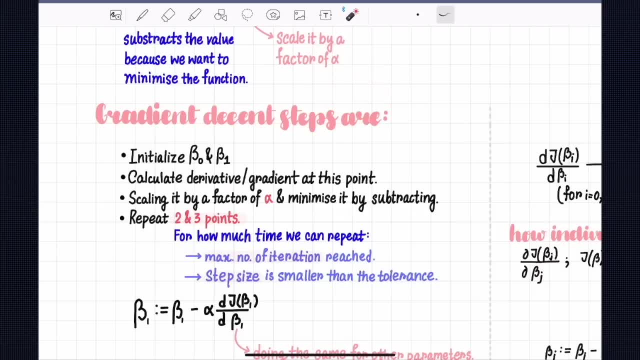 assume that your initial a beta 1 does. assume that your initial a beta 1 does any number, any random values, and we any number, any random values, and we any number, any random values, and we there is a initialization techniques. there is a initialization techniques. there is a initialization techniques. will study in deep learning, not as of 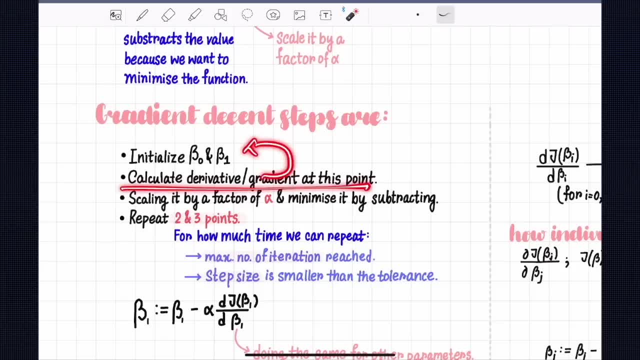 will study in deep learning, not as of will study in deep learning? not as of now, but you can ignore it. you calculate now, but you can ignore it. you calculate now, but you can ignore it. you calculate an gradient at the current point with an gradient at the current point with. 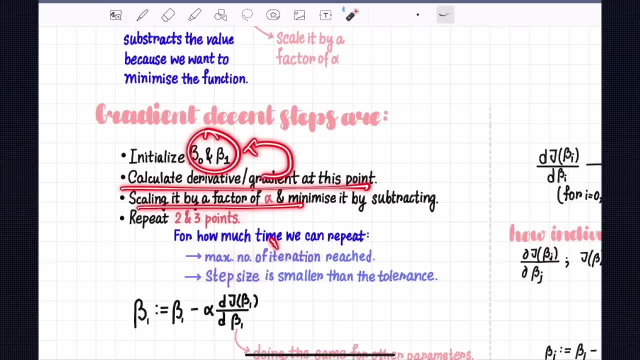 an gradient. at the current point, with the current current value, of course the. the current current value, of course the the current current value, of course the error will be high. you scale it. a factor error will be high. you scale it. a factor error will be high. you scale it. a factor of X mems. minimize it by subtracting you. 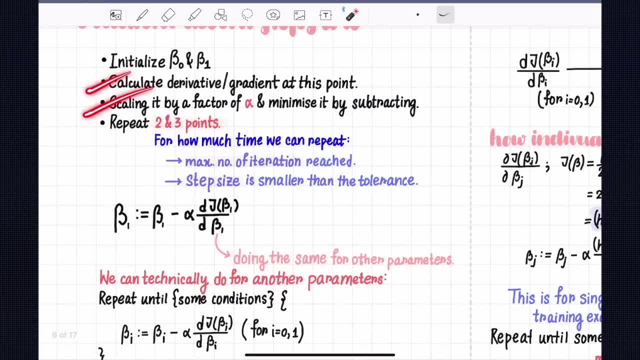 of X mems. minimize it by subtracting. you of X mems. minimize it by subtracting you. subtract the old bit us here the update subtract the old bit. us here the update subtract the old bit us here the update rule app happens and they repeat two and 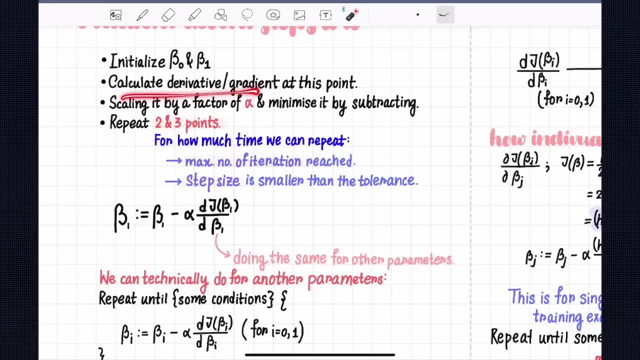 rule app happens, and they repeat two. and rule app happens and they repeat two and three points. two and three points, right. three points. two and three points, right, three points, two and three points, right? you repeat: calculate you for you and the. you repeat: calculate you for you and the. 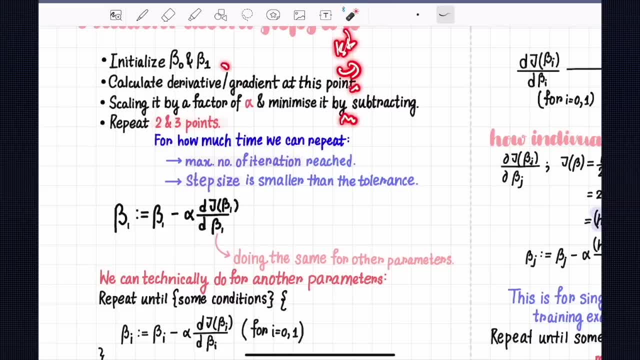 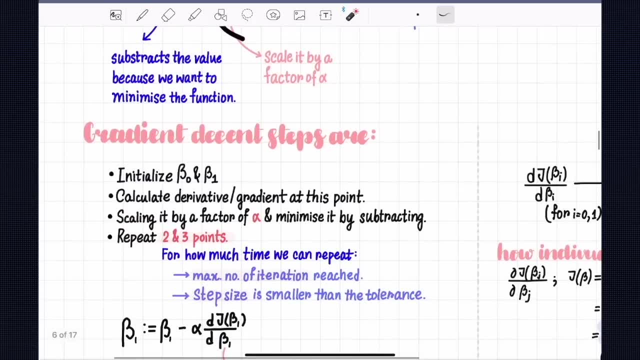 you repeat: calculate you for you and the first iteration. you calculate the first iteration, you calculate the first iteration, you calculate the beta, and then you go to third edition and beta, and then you go to third edition and beta, and then you go to third edition and then you know you it now your beta are: 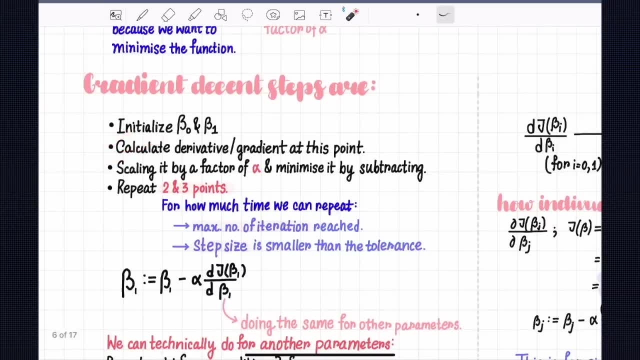 then you know you it now your beta are. then you know you it now your beta are of the second iteration. so you scale to of the second iteration. so you scale to of the second iteration, so you scale to repeat the two and three points. how much? repeat the two and three points, how much? 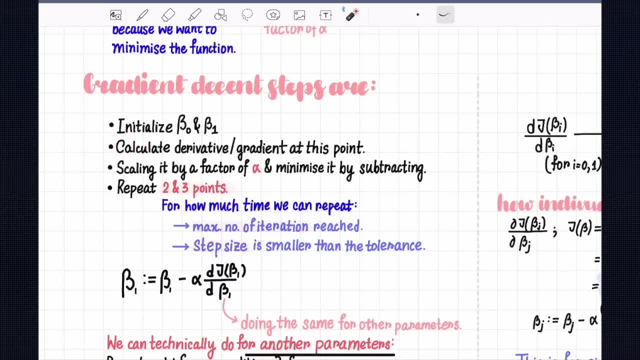 repeat the two and three points. how much? by how much will you want to repeat? by how much will you want to repeat? by how much will you want to repeat? first of all, we can do it for like we. first of all, we can do it for like we. 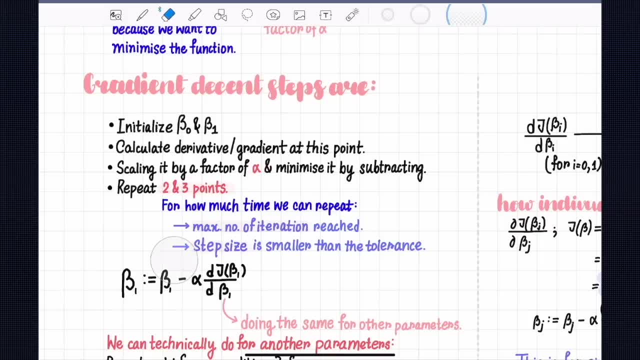 first of all, we can do it for, like we are not a beat for 20 iteration, 30 are not a beat for 20 iteration, 30 are not a beat for 20 iteration, 30 iteration, 40 iteration, or we can, we can. iteration, 40 iteration, or we can, we can. 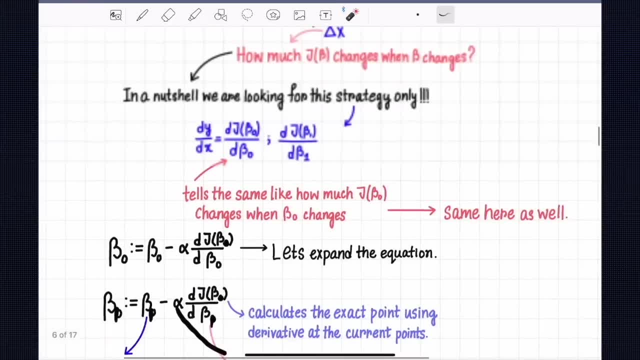 iteration, 40 iteration, or we can, we can learn this when you're, when you're, when learn this when you're when you're, when learn this when you're when you're when you're when you actually converge, when you're when you're when you actually converge, when. 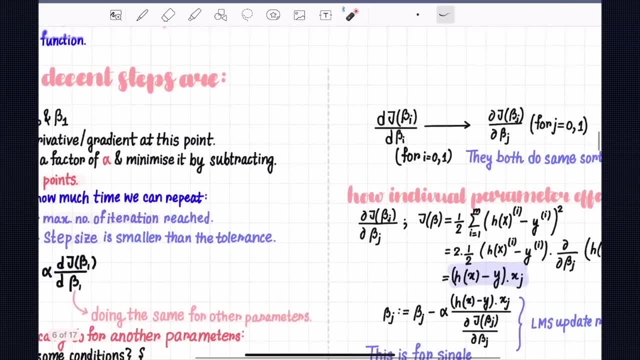 you're when you're when you actually converge, when you actually when your beta, you actually when your beta. you actually when your beta, when your beta is actually when you're when, when your beta is actually when you're when, when your beta is actually when you're when you're when your algorithm is. 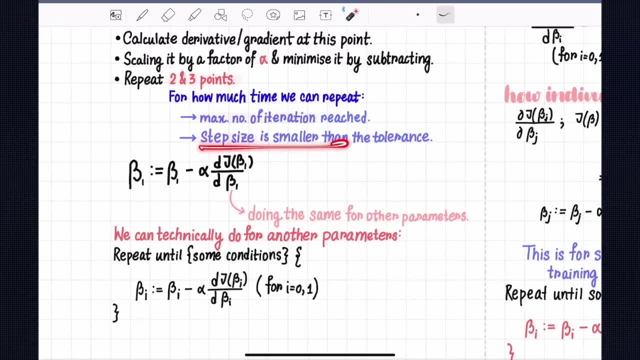 you're when your algorithm is. you're when your algorithm is converged, so what? what? what we say converged, so what? what? what we say converged, so what? what? what we say converged is that your step size is converged. is that your step size is converged, is that your step size is smaller, like a step size smaller than smaller, like a step size. smaller than smaller, like a step size. smaller than the tolerance. and then the learning rate: the tolerance, and then the learning rate, the tolerance, and then the learning rate stops when it reaches the global minima. stops when it reaches the global minima. 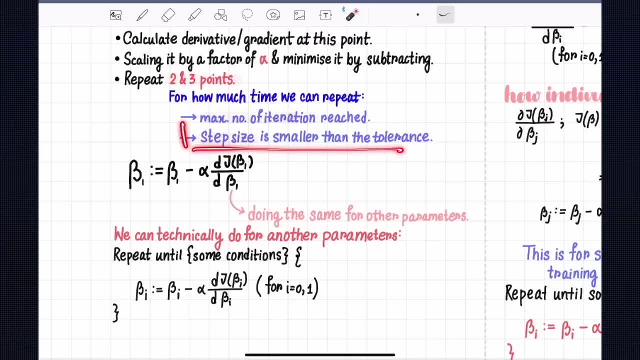 stops when it reaches the global minima. okay, and you will learn about this. you okay, and you will learn about this. you okay, and you will learn about this. you can ignore this as of now, we'll have a. can ignore this as of now, we'll have a. 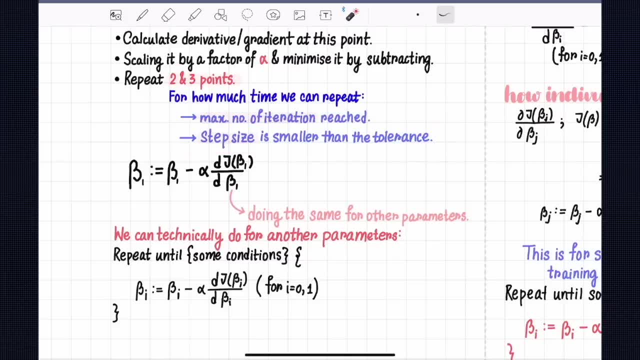 can ignore this. as of now, we'll have a separate video on learning rate. to make separate video on learning rate. to make separate video on learning rate to make you better understand about it. okay, so, you better understand about it. okay, so you better understand about it. okay, so, and then we do for beta 0, and then we do. 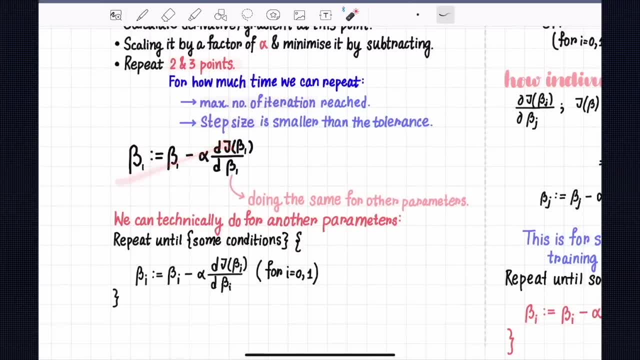 and then we do for beta 0, and then we do, and then we do for beta 0, and then we do for beta 1 as well, and then you do for for beta 1 as well, and then you do for for beta 1 as well, and then you do for beta 1 as well. okay, doing the same thing. 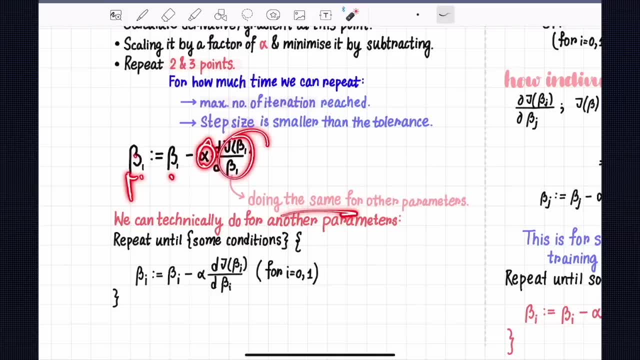 beta 1 as well. okay, doing the same thing. beta 1 as well. okay, doing the same thing. very updating the beta 1, the new beta 1. very updating the beta 1, the new beta 1. very updating the beta 1, the new beta 1, the old beta minus learning the alpha, the. 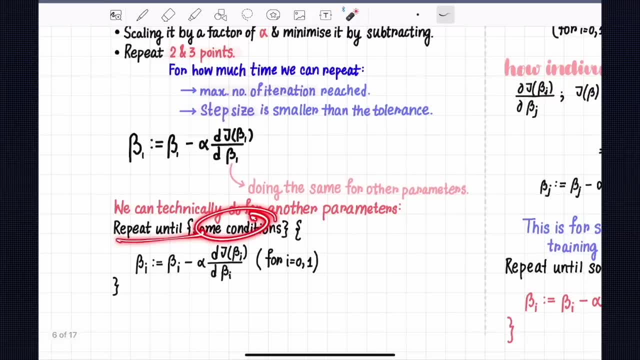 the old beta minus learning the alpha the. the old beta minus learning the alpha the. change okay, and then we repeat until change okay, and then we repeat until change okay, and then we repeat until some conditions. what is the number of some conditions? what is the number of? 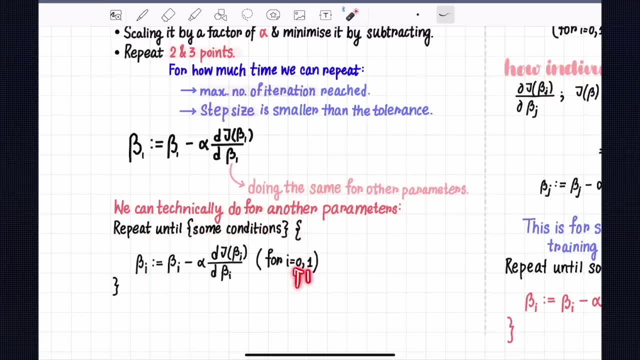 some conditions. what is the number of iterations: repeat 24 or 20 iterations. iterations: repeat 24 or 20 iterations. iterations: repeat 24 or 20 iterations. where you I for beta, I goes to 0 and 1. where you I for beta, I goes to 0 and 1. 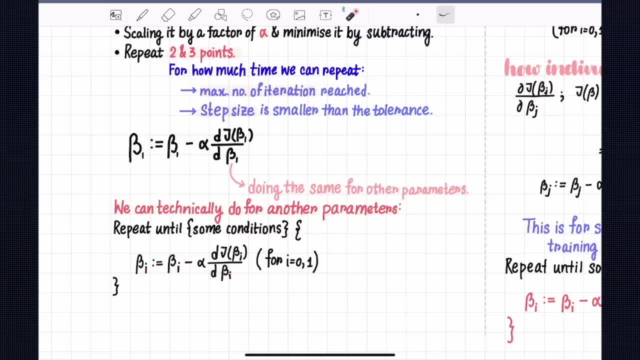 where you, I for beta, I goes to 0 and 1. we apply the folder for beta 0, and then we apply the folder for beta 0, and then we apply the folder for beta 0 and then we update with me, simply, simply, do for. 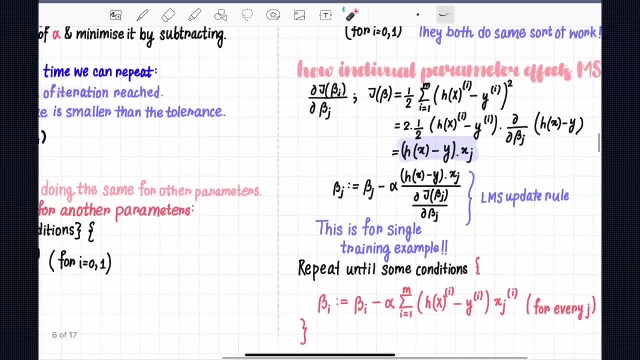 we update with me, simply simply do for. we update with me, simply simply do for. all the betas out there, whatever beta 1, all the betas out there, whatever beta 1, all the betas out there, whatever beta 1 and beta 0, you do for both. fun, okay now. 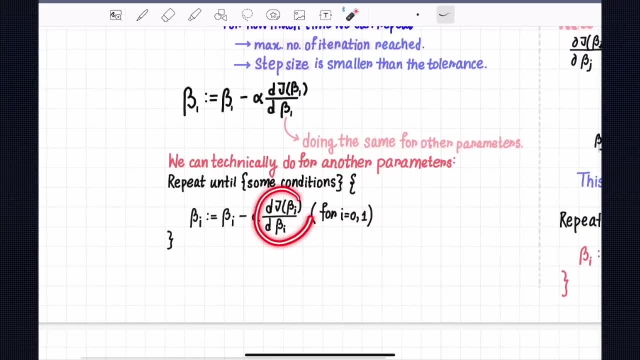 and beta 0- you do for both fun, okay now. and beta 0- you do for both fun, okay now. now, your question would be: how can we now? your question would be: how can we now? your question would be: how can we calculate the derivative of this? so 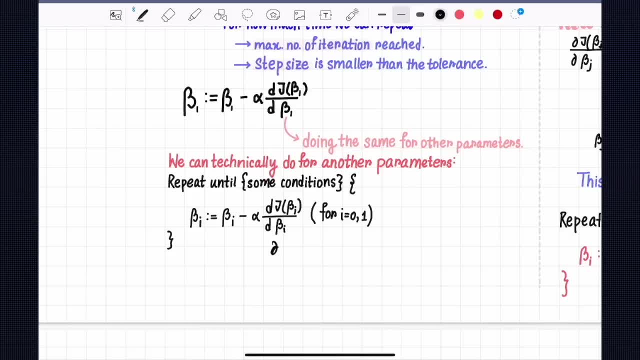 calculate the derivative of this. so calculate the derivative of this. so eventually you don't use, usually use the eventually you don't use, usually use the eventually you don't use, usually use the derivative. you use the partial derivative, you use the partial derivative. you use the partial derivative of G of bi with respect to bi. 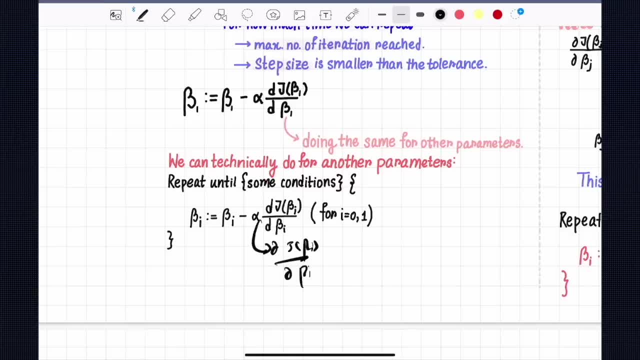 derivative of G of bi with respect to bi. derivative of G of bi with respect to bi. be beat I so this, this exactly means be beat. I so this, this exactly means be beat. I so this, this exactly means that in both means exactly the same, but that in both means exactly the same, but. 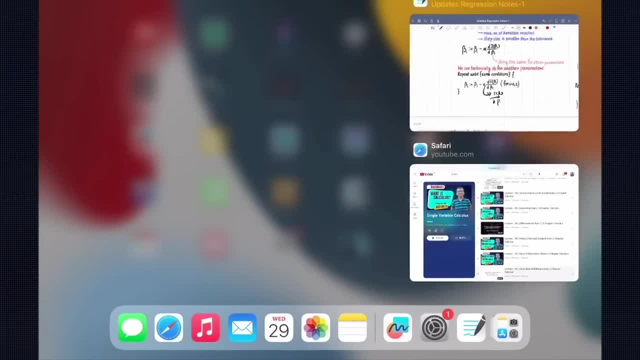 that in both means exactly the same, but this is a partial derivative which is: this is a partial derivative which is: this is a partial derivative which is applied in a vector calculus, if you want, applied in a vector calculus. if you want, applied in a vector calculus. if you want to learn more about, you know, calculus. 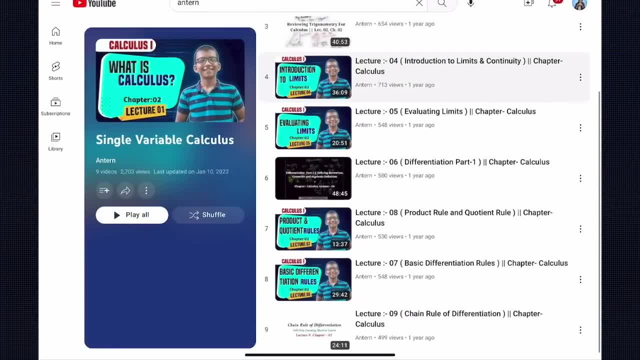 to learn more about you know calculus. to learn more about you know calculus and everything. if you haven't yet, I and everything. if you haven't yet, I and everything. if you haven't yet, I recommend you to watch this playlist. recommend you to watch this playlist. recommend you to watch this playlist, which I created over a year ago, which is: 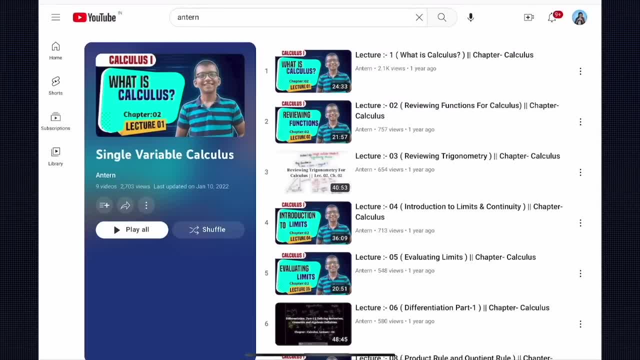 which I created over a year ago, which is which I created over a year ago, which is quite famous playlist, not by so much of quite famous playlist, not by so much of quite famous playlist, not by so much of people, but eventually it is very nice people, but eventually it is very nice. 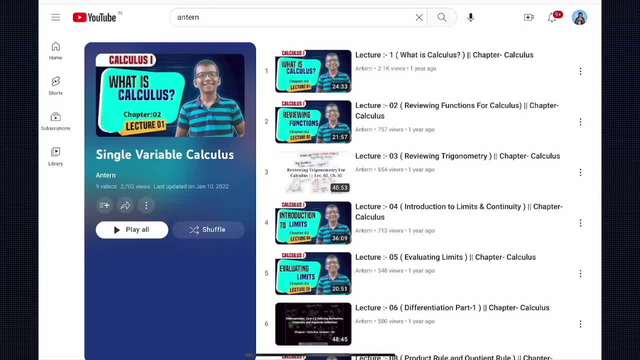 people, but eventually it is very nice. if you to, if you wanted to learn about, if you to, if you wanted to learn about, if you to, if you wanted to learn about calculus and great detail, I've tried calculus and great detail, I've tried calculus and great detail, I've tried, I've considered everything which I know. 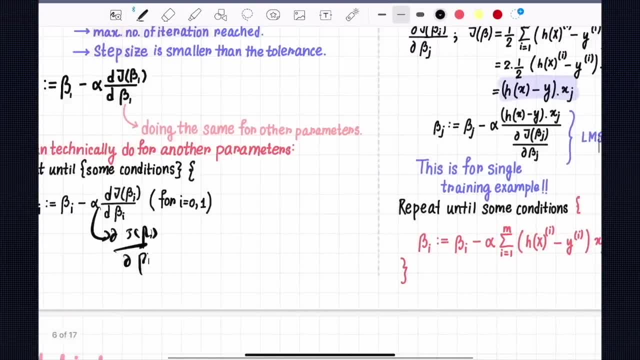 I've considered everything which I know. I've considered everything which I know about calculus over here. so how can we about calculus over here? so how can we about calculus over here? so how can we take out the- this partial derivative of, take out the- this partial derivative of? 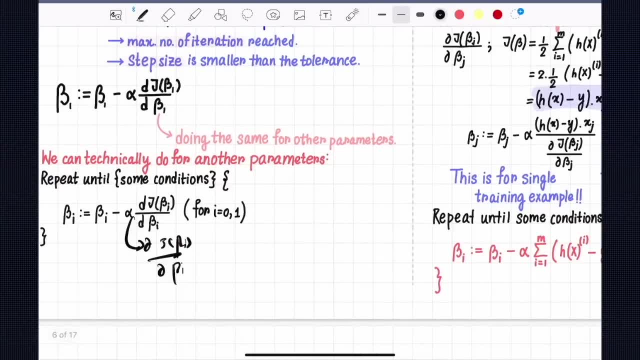 take out the this partial derivative of G of. how can we take a partial that G of? how can we take a partial that G of? how can we take a partial that derivative of your cost function with derivative of your cost function? with derivative of your cost function with respect to particular parameter this: 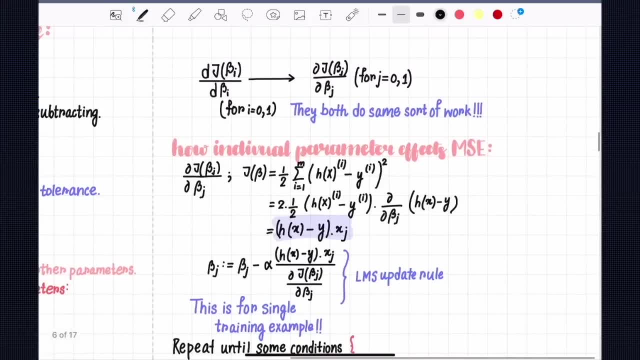 respect to particular parameter. this respect to particular parameter, this exactly means the same that how much a exactly means the same that how much a exactly means the same that how much a cost function changes when you beat up cost function changes, when you beat up cost function changes when you beat up beta changes. okay, I hope that this makes 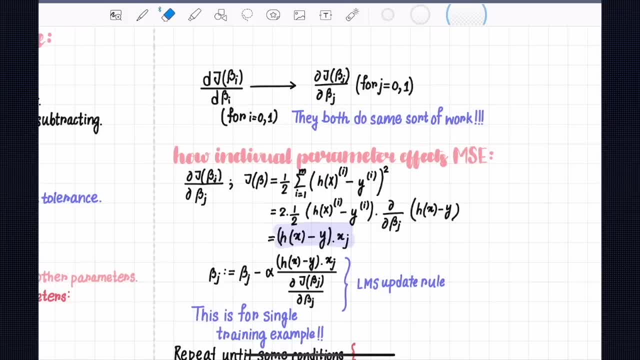 beta changes. okay, I hope that this makes beta changes. okay, I hope that this makes sense. so you see that they do the same sense. so you see that they do the same sense. so you see that they do the same sort of work overall. you seem simply sort of work overall. you seem simply. 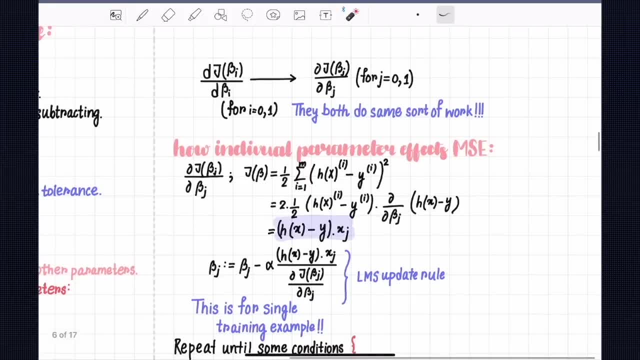 sort of work. overall, you seem simply same sort of work, but this is so the same sort of work, but this is so the same sort of work, but this is so the vector calculus. so how individual vector calculus? so how individual vector calculus? so how individual parameter, like eventually, how? 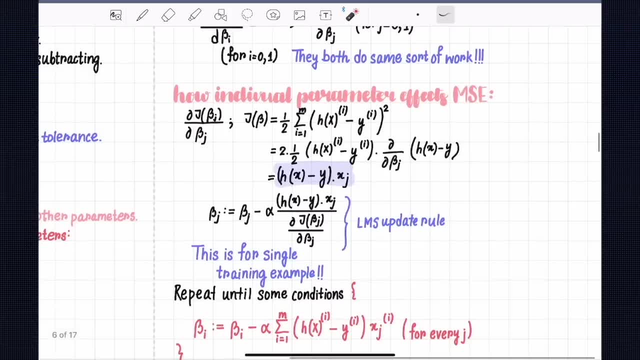 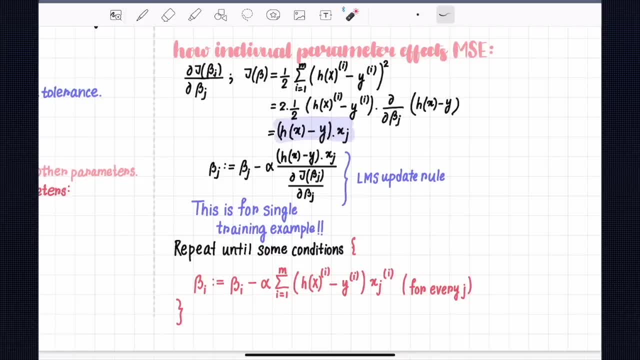 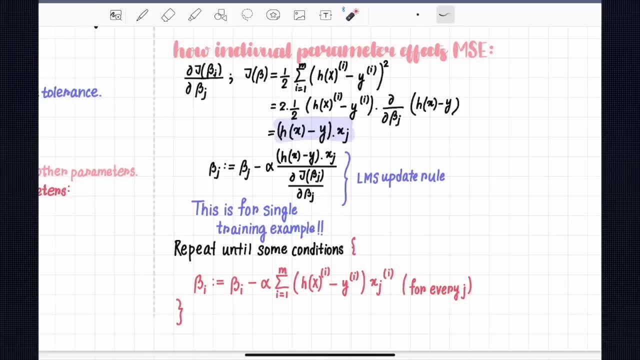 we'll talk about that for a single. we'll talk about that for a single training example in a free form. so I'll training example in a free form, so I'll training example in a free form. so I'll just talk about when, even very less you 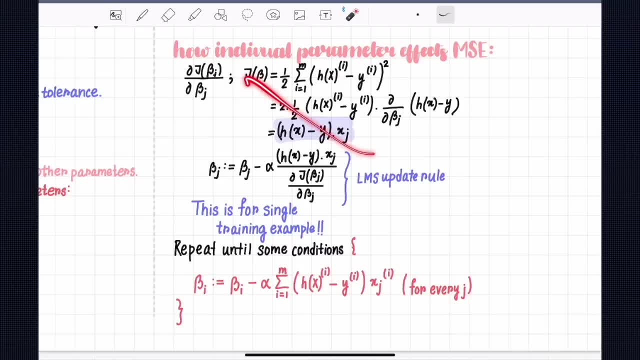 just talk about when, even very less. you just talk about when, even very less. you do a real-world example. no, then then do a real-world example. no, then then do a real-world example. no, then, then then I'll show you the derivation you can. then I'll show you the derivation you can. 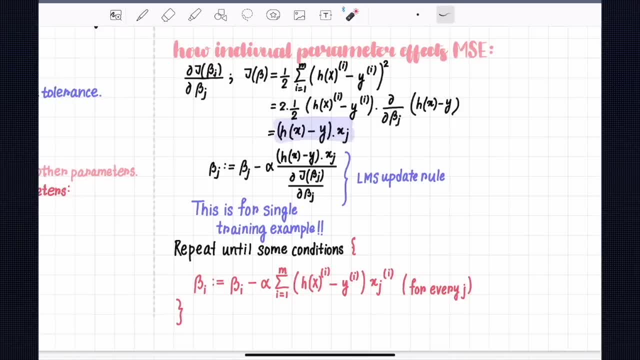 then I'll show you the derivation. you can know this as of now. this just for know this. as of now. this just for know this. as of now. this just for notes purposes. I'll show you a book notes purposes. I'll show you a book notes purposes. I'll show you a book example, hands-on, so that it fit. it is. 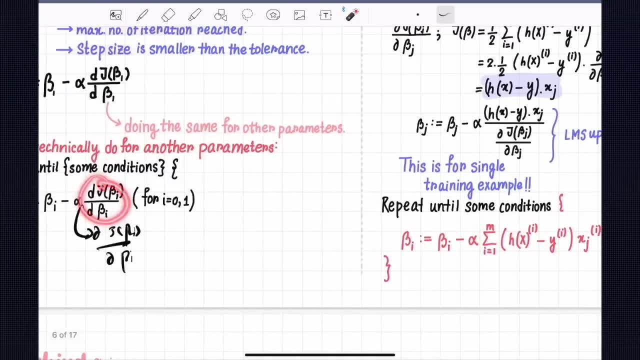 example, hands-on so that it fit. it is example hands-on so that it fit. it is more clear. so now when you, when you more clear, so now when you, when you more clear, so now when you, when you actually calculate when this will yield, actually calculate when this will yield. 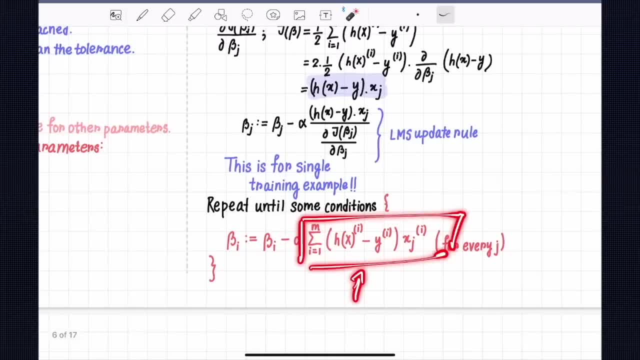 actually calculate when this will yield to this formula, to this formula, we to this formula, to this formula, we to this formula, to this formula, we learn how to utilize this formula and learn how to utilize this formula and learn how to utilize this formula. and for now, you plug in the values now over. 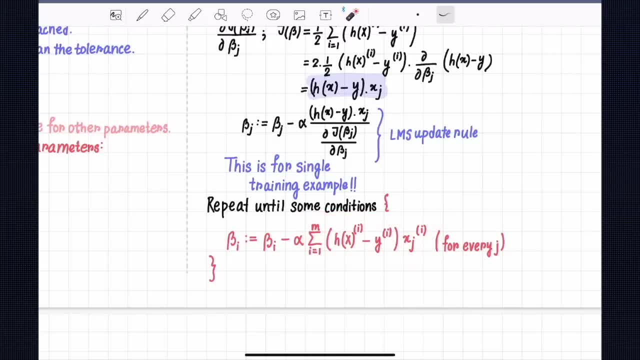 for now. you plug in the values now over for now. you plug in the values now over here. this: this will give you the rate of here. this: this will give you the rate of here this. this: this will give you the rate of change. okay, listen you the rate. 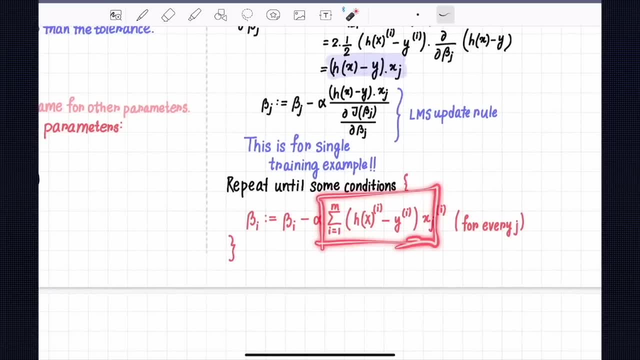 change. okay, listen you the rate change. okay, listen you the rate of change. so we'll talk about what is the of change. so we'll talk about what is the of change. so we'll talk about what is the interpretation of this? well, what? why? interpretation of this? well, what, why? 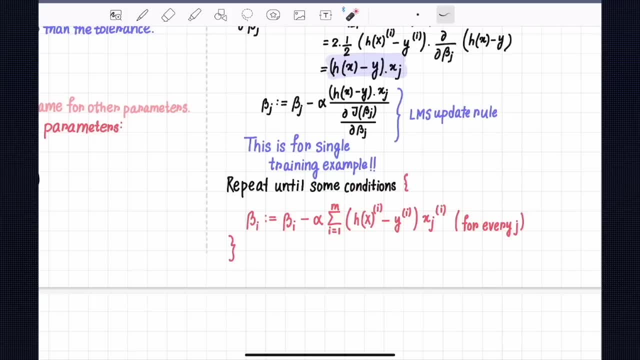 interpretation of this. well, what? why do we use derivative? what is the? do we use derivative? what is the? do we use derivative? what is the interpretation of this number and interpretation of this number and interpretation of this number and various things? this is just a starting. various things. this is just a starting. 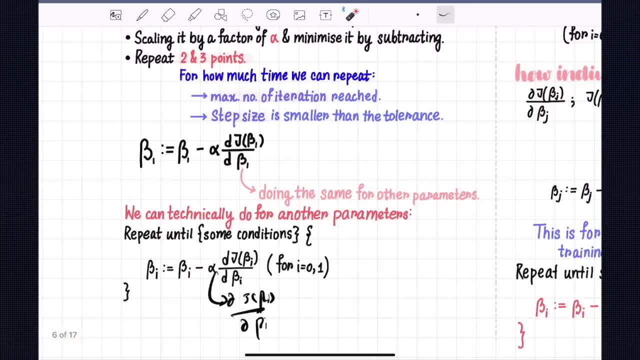 various things. this is just a starting point. my aim was to make you understand point. my aim was to make you understand point. my aim was to make you understand that we have an update rule, and then we that we have an update rule, and then we that we have an update rule, and then we have this. give you a storyline. for what? 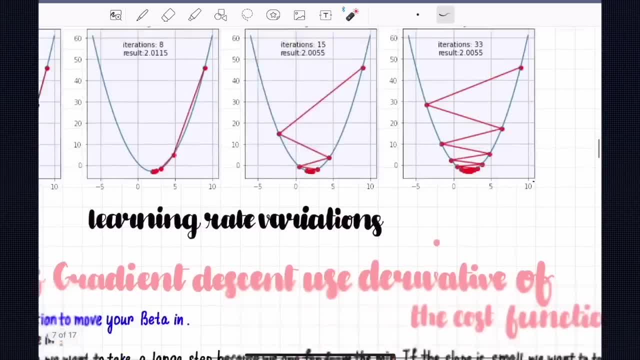 have this? give you a storyline for what? have this? give you a storyline for what? exactly how do we learn? and this is the exactly how do we learn, and this is the exactly how do we learn, and this is the story behind the learning point. okay, so, story behind the learning point. okay, so. 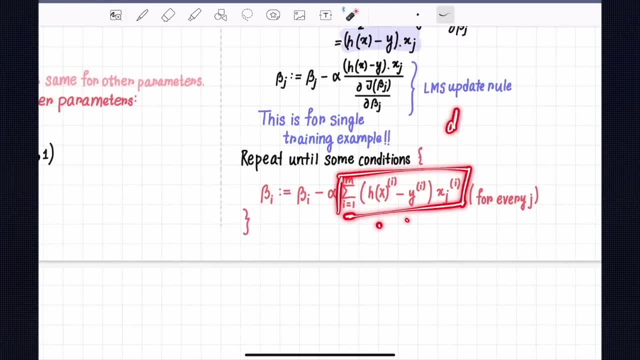 story behind the learning point. okay, so you can see that we are having the this. you can see that we are having the this. you can see that we are having the. this is the derivation when you calculate the. is the derivation when you calculate the. is the derivation when you calculate the derivative of the cost function: the cost. 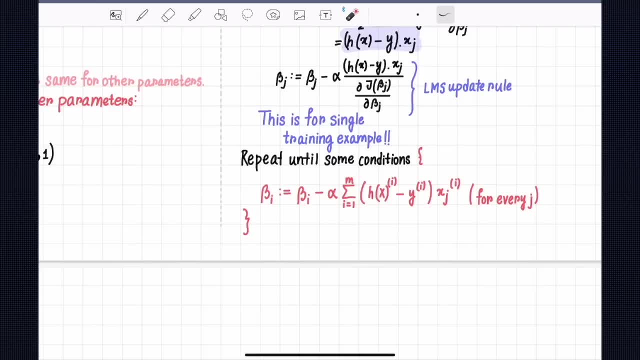 derivative of the cost function. the cost derivative of the cost function. the cost function is which I've seen with function, is which I've seen with function, is which I've seen with respect to particular parameter. you get respect to particular parameter. you get respect to particular parameter. you get this particular equation. okay, we'll. 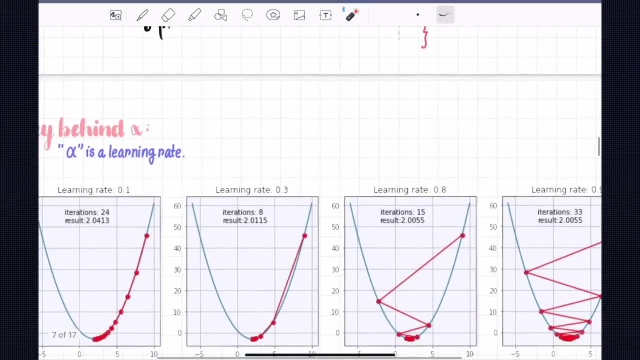 this particular equation, okay, we'll this particular equation. okay, we'll click, we'll talk, we'll talk about this. click, we'll talk, we'll talk about this. click, we'll talk, we'll talk about this. and just just in next section we're. and just just in next section we're. 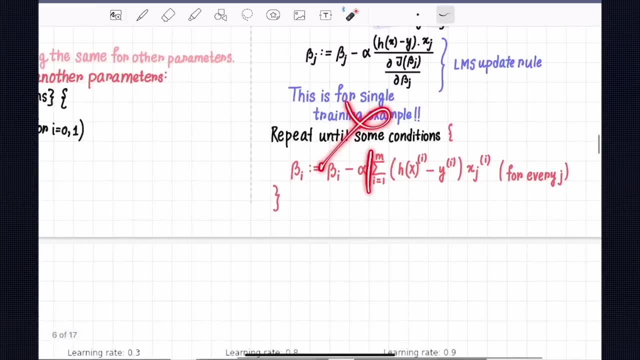 and just just in next section, we're talking. we'll work on, for example, talking. we'll work on, for example, talking. we'll work on, for example, pleasing- no dad of snow, but just pleasing- no dad of snow, but just pleasing. no dad of snow. but just remember that this is the derived. if you remember that this is the derived, if you remember that this is the derived, if you don't want to do the calculus stuff, you don't want to do the calculus stuff, you don't want to do the calculus stuff, you can actually ignore the next section as can actually ignore the next section, as. 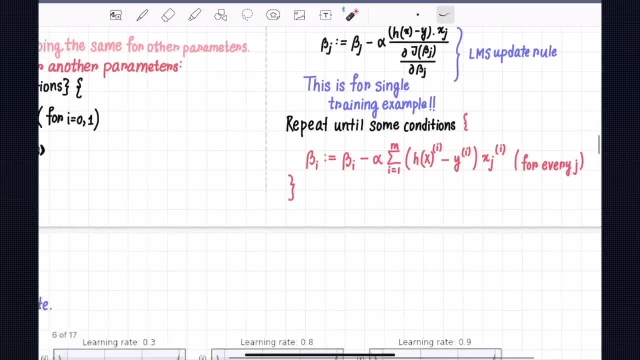 can actually ignore the next section as well, but I really really recommend if well. but I really really recommend if well. but I really really recommend if you want to fully understand greatest, you want to fully understand greatest, you want to fully understand greatest and you should be able to learn about. 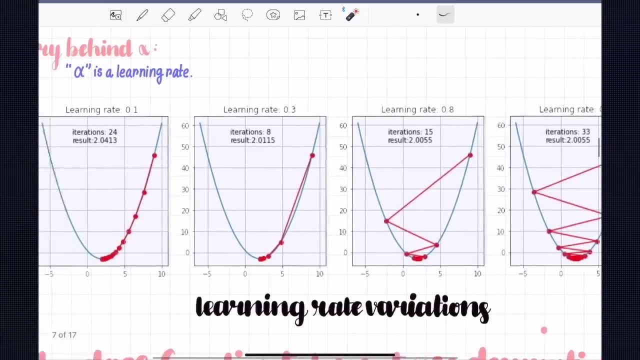 and you should be able to learn about, and you should be able to learn about it. okay, now I have listed some examples it okay now I have listed some examples. it okay now I have listed some examples of learning rate. so over here we which. of learning rate. so over here we, which. 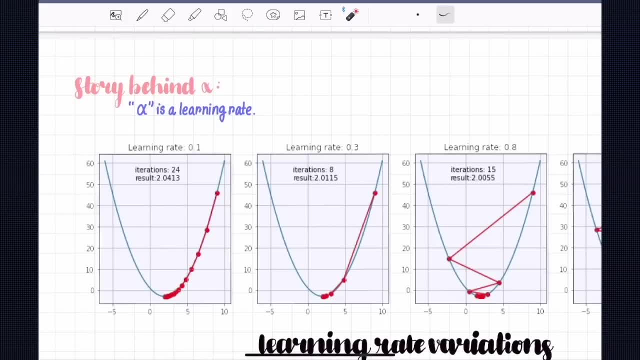 of learning rate. so over here we. which which which have seen learning rate alpha, which which have seen learning rate alpha, which which have seen learning rate alpha is a learning rate which decides by. how is a learning rate which decides by? how is a learning rate which decides by how much? you should converse the rate of. 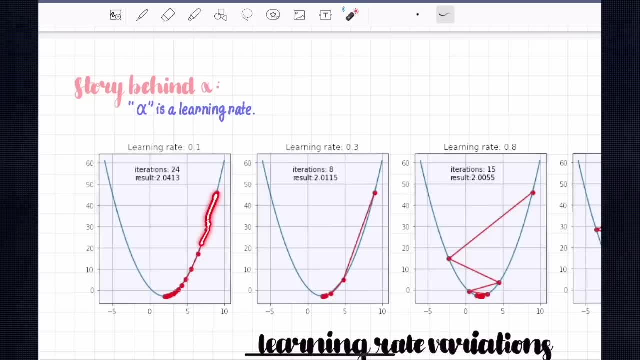 much. you should converse the rate of much. you should converse the rate of learning. okay, so we have learning learning. okay, so we have learning learning. okay, so we have learning. reserve 0.1 starts with this and then it. reserve 0.1 starts with this and then it. 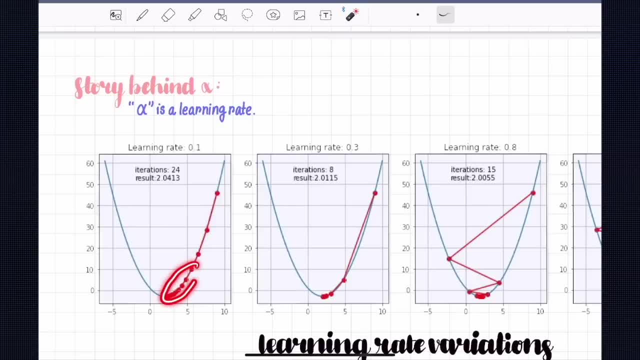 reserve 0.1 starts with this and then it slows down and then it converges slowly, slows down, and then it converges slowly, slows down and then it converges slowly. so if you see that at this point at this, so if you see that at this point at this, 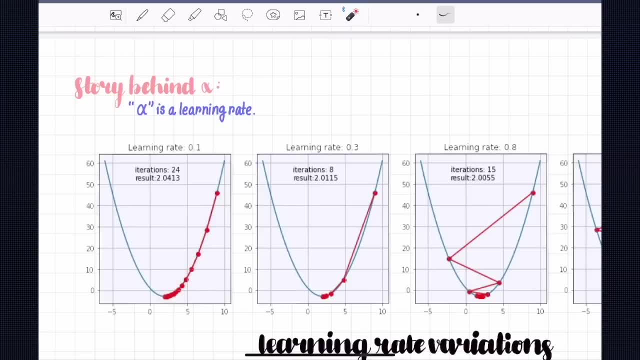 so if you see that at this point, at this point, it is very, very slow, why? because point it is very, very slow. why? because point it is very, very slow. why? because at is at as it is learning, and, and and. at is at as it is learning, and and and. 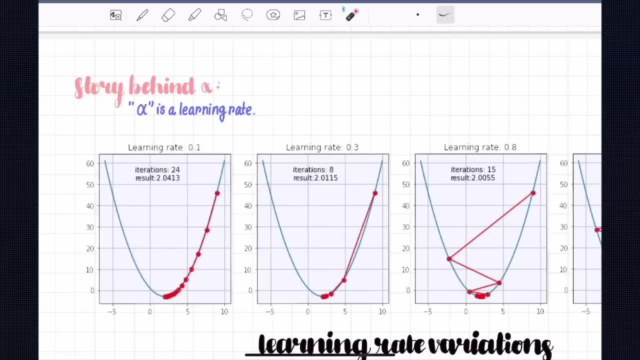 at, is at as it is learning and and. and. it knows you can understand this to be. it knows you can understand this to be. it knows you can understand this to be. it knows that, second. it knows that it is. it knows that second. it knows that it is. 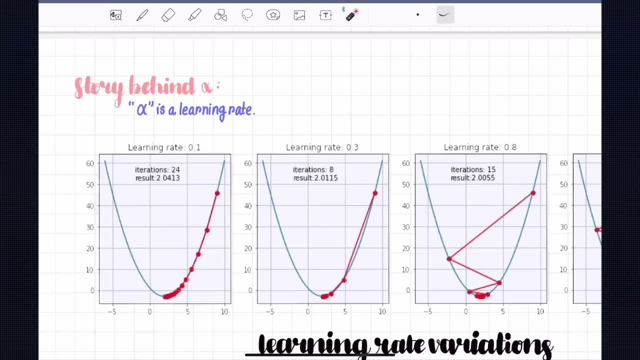 it knows that. second, it knows that it is our mind my conversion rate is coming. so our mind my conversion rate is coming. so our mind, my conversion rate is coming. so I have to be very cautious because I'm. I have to be very cautious because I'm. I have to be very cautious because I'm occurred so I have to be a bit slow. occurred so I have to be a bit slow. occurred so I have to be a bit slow. because when you have a, when you drive a, because when you have a, when you drive a. 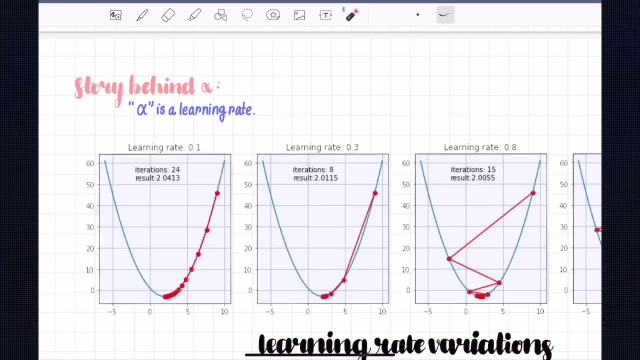 because when you have a, when you drive a car, you don't drive it up in the same car. you don't drive it up in the same car. you don't drive it up in the same speed, right, you don't have it. stay same speed, right, you don't have it, stay same. 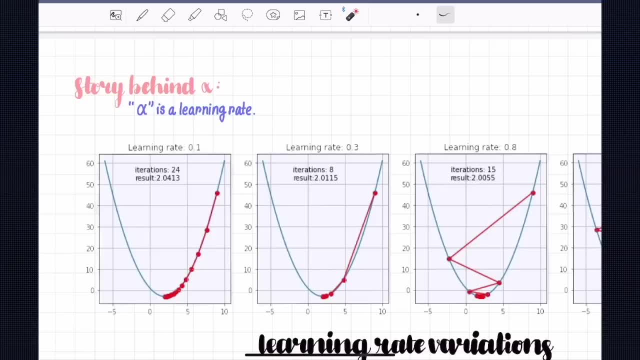 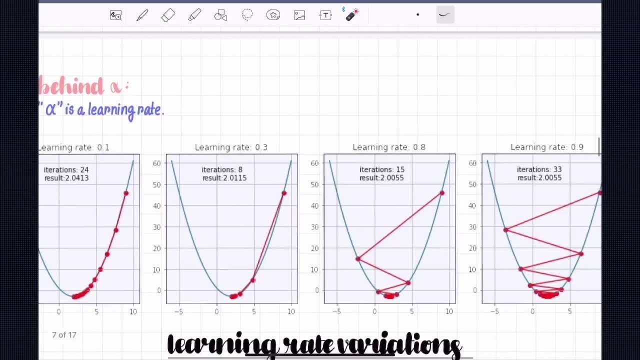 you strive same speed, you drive that fast. but whenever required the breaker comes, you slow it down. right, or whenever the stoppage comes, you slow it down. that's why the stoppage is slows. but if, but, if your error, if you, if your learning rate is too high, you. this is the learning rate. 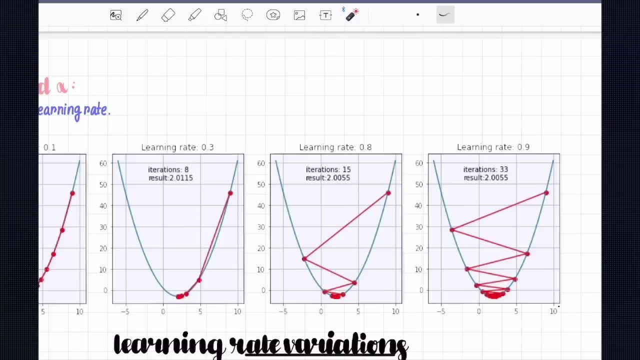 which you have to choose according to your problem statement, according to the data, which we'll talk about that later on, when actually the practical. but this is something which i have to tune like try out several and see what works well. so if your learning rate is too high, it will mostly diverge. 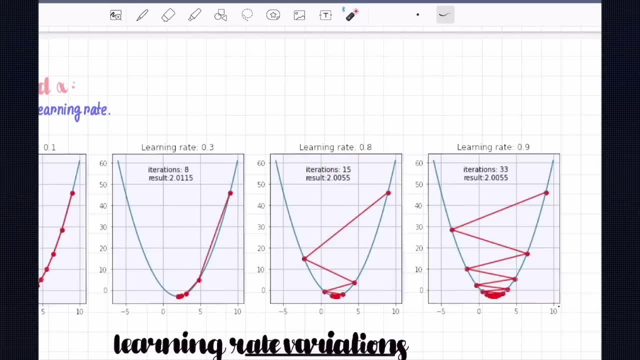 so, for example, if, if, if your car is going on okay with the high speed, so if you push a brake, if you push like 100 kilometer per hour, so push a brake car is most likely to fall down. right, but like it, it, it will most likely to fall down. it will most like to crash like hell. 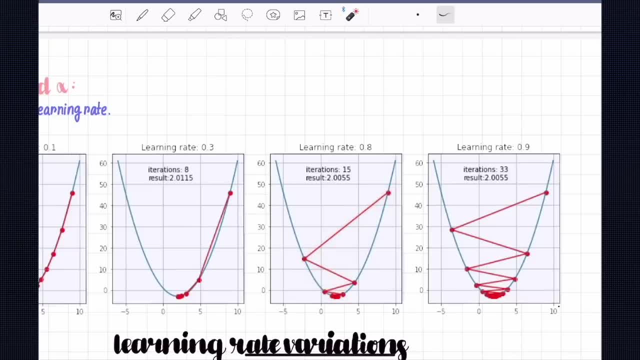 so if the learning rate will diverge like this, it will never converge to the minimum, it will simply keep on diverging, you'll. it will never reach to a stoppage. and if your learning rate is too small, then it will never converge, you, okay, because it will be two per so, super, duper. so if you drive at one to one, uh meter per per, 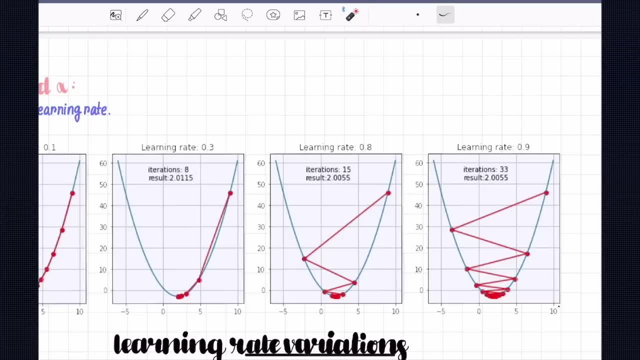 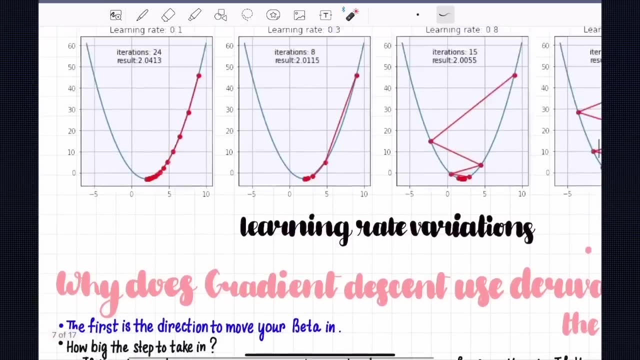 kilometer. you know it's, it's. uh, i mean i i just mess it up. so if you drive slowly, you'll not be to reach. okay, cool this. these are some of the learning rate variations. uh, we'll talk about that later on, but i hope that you understood about gradient set in upper level. now let's go and do. 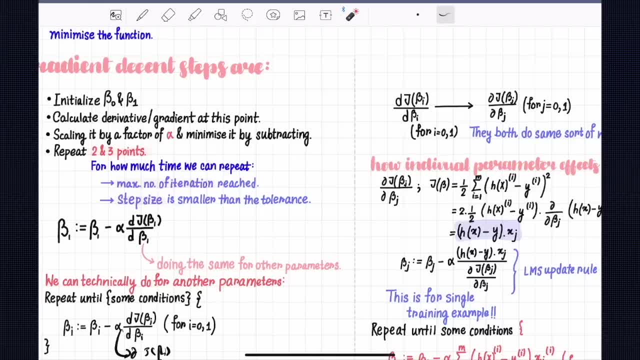 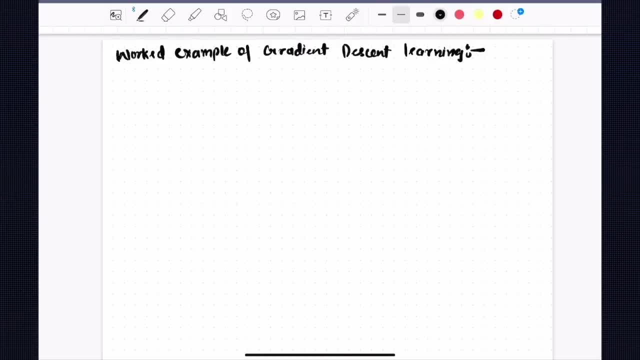 the world example and the derivations and all to make you more, uh, understandable about all of this thing. so, hey, everyone, i'm back, uh, with a world example of green descent learning, and we'll eventually take a sample data and perform a real time learning on that and then i'll show you how, it is super simple to understand, creating. 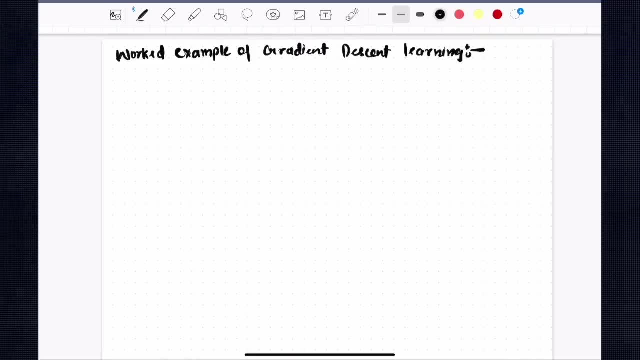 descent, even with mathematical reasoning. uh, if you're, if you're not comfortable even with math, i would recommend you to watch it right, it will be much more better for you. so let's get started over here. i wanna, i wanna, take a sample data. so, sample data which i'm, which i'm gonna take, is you? 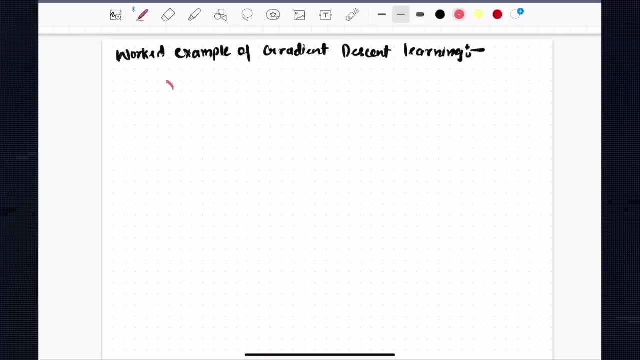 have a one input feature, one input feature which is going to be a sample data. one input feature and, oops, my mind is so diverted. i'm using yellow and white, so x and y, and in this x and y you have one, two, two, four, three, six, four, eight. please note, i'm not going to take a huge data, otherwise it. 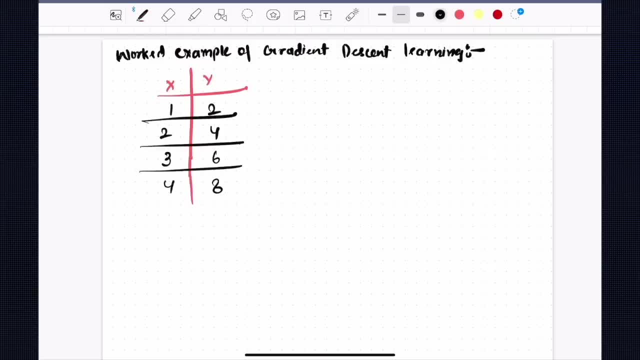 will take me years, but i'm going to take a sample data. but i'm going to take a sample data. this is sample data where you have only one independent feature- independent independent feature- and then you have your output variable- output uh variable or target variable. okay, you have one independent. 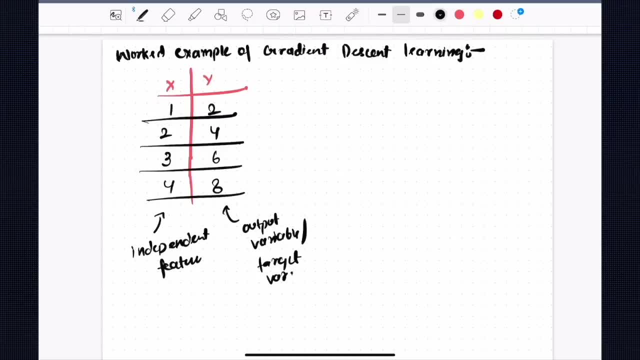 feature. and then you have output variable and target feature, target variable which you're going to predict. so in a builder function f, in a builder function f, or takes the value of this- x is the value of this- and maps it to y. so to build a function f that i have. 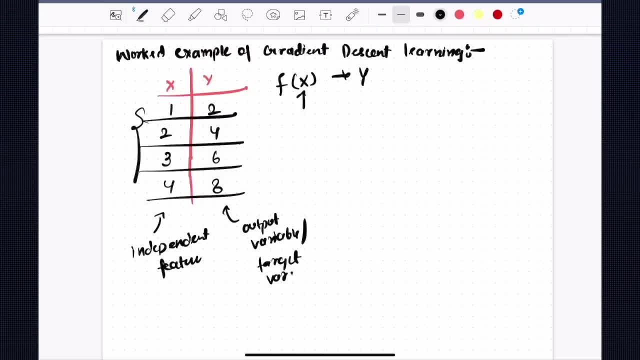 any sort of relationship between these two, right? so, basically, this for for you it may be super simple, right to understand the relationships, but eventually i'm going to take an example to show you how our machine learning algorithm will interpret this, how our machine algorithm will go on understanding the relationship. okay, because i 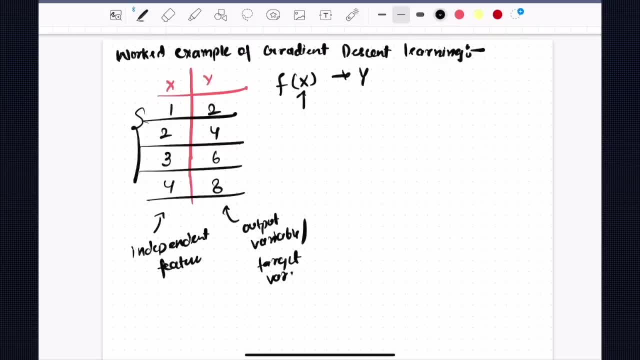 am always a believer- or of understanding from the baseline, so that you understand the core of it, you will understand even the big things of it. so your f of x is um. when you, when you're taking a value of and you put a put, put, put in the value of x, you'll predict y. so build a function f. so you'll build a function f. so. 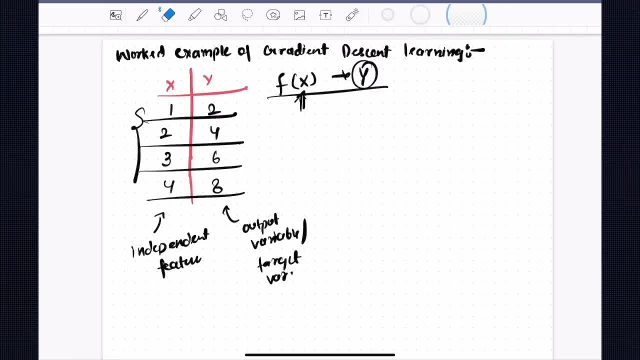 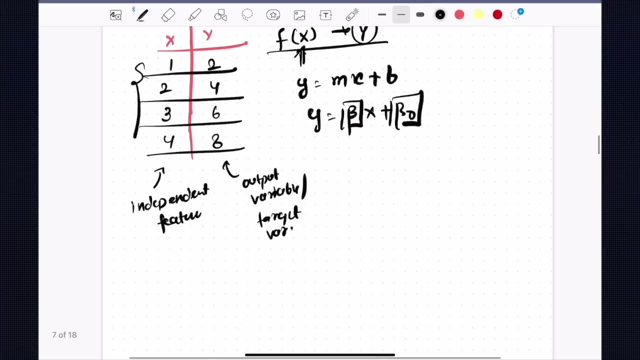 your equation, so equation, so sorry. so. so your equation for this line, so equation for this line: or y equals to mx plus b, or y is equals to beta one times x plus beta zero. so your point is to take out beta one and beta zero out of this using gradient descent. so what's our first step? the? 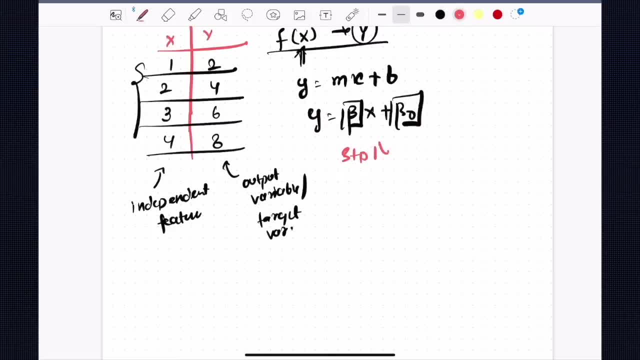 first step of ours is nothing. step number one. step number one: initialize. initialize your beta zero and beta one. so i'm going to initialize beta one to be one and beta zero to be zero. so this is two, two things which i'm going to initialize initially. okay, because anything you have to initialize first. 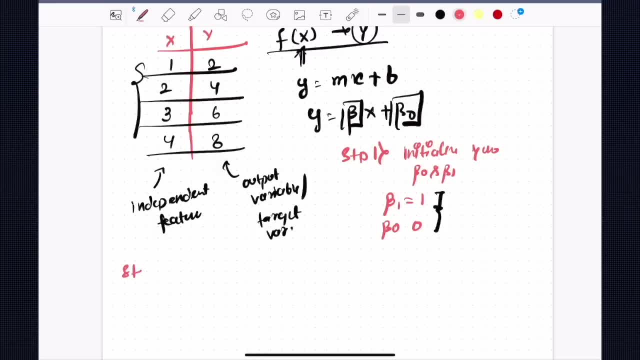 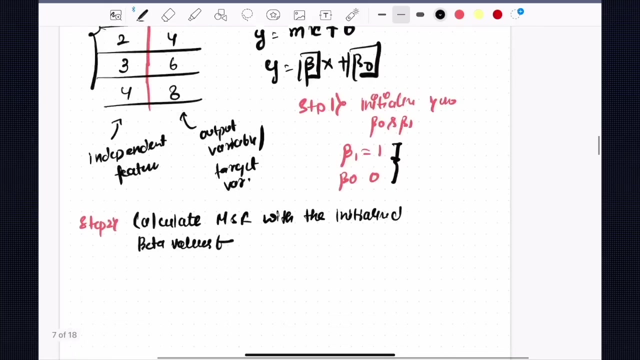 then the second step, which, which, which you have to do, the second step which you have to do, the second step which you have to do is calculate. the error is: calculate the mse, calculate the mse with the initialized, with the initialized beta values, with initialized beta values. and so how can we take out? first of all, it's very simple. 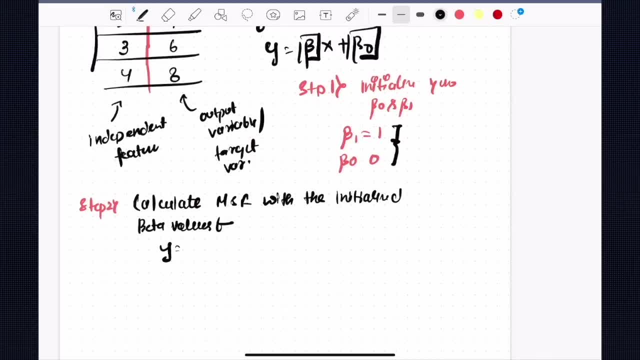 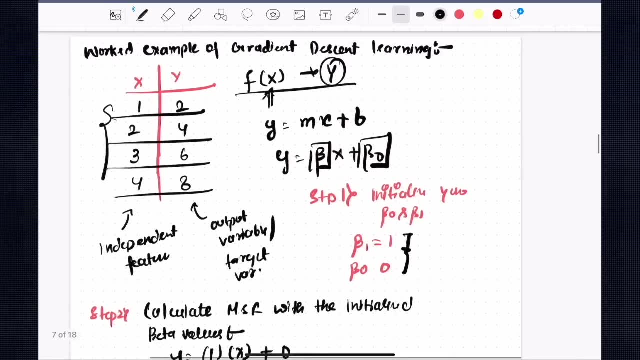 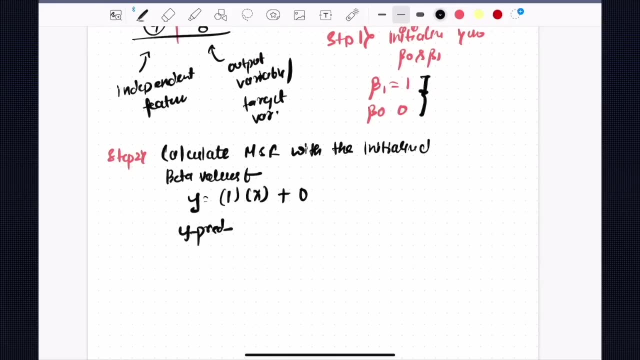 you have, your y is equals to beta. what? what was the beta one? beta one will one times x plus zero. this test was equation. you plug in the values of every x over here. you plug in the value one, two, three, four, right, so uh, the y pred one, so y pred one, which is equals to nothing but. 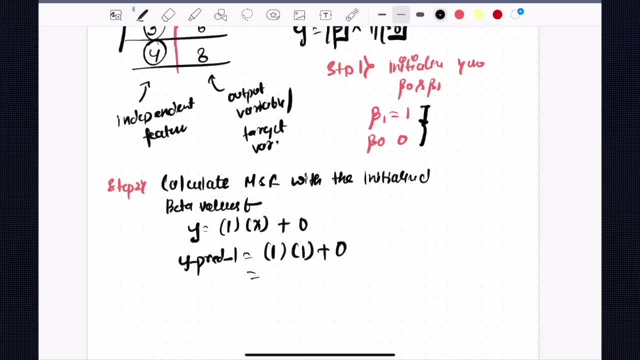 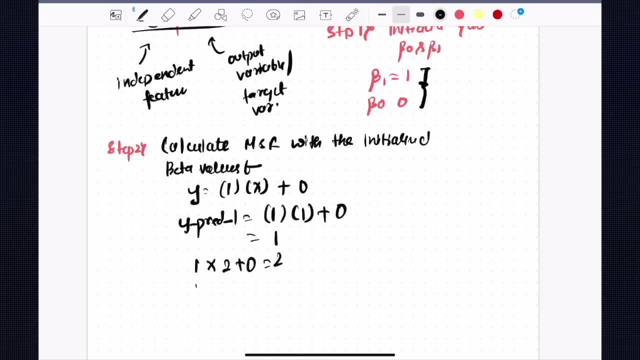 uh, one times one plus zero, which is nothing but equals to one. so you keep, keep on doing for every sample. so, y pred two, y pred three, the prediction which is one times two plus zero equals to two, one times three plus zero equals to three, and one times four plus zero equals to four. okay, 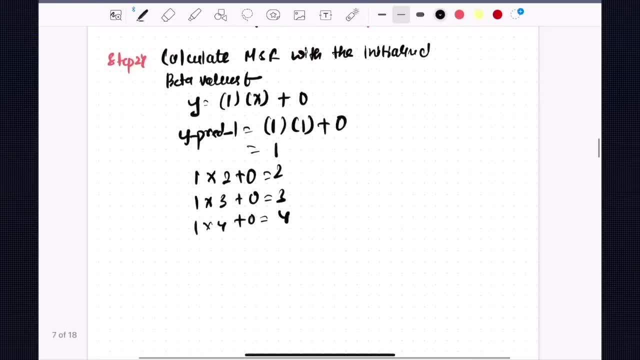 so now you have to calculate the step now you have to have, after taking the predictions, now what have to do is calculate mse is calculate, is calculate mse. calculate mse by nothing but one, by m. i is equals to one all the way around to the m. i is equals to all all the way around to the m. 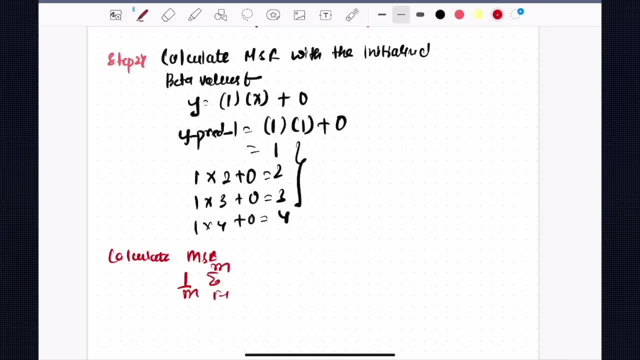 so what exactly we can do, we can simply um say that one thing is, we can also use our formula, which which we had, of that one by two, m, which is nothing but 7.5 divided by two, which is something. yeah, so what exactly we can do. what exactly we can do is we can either use two over here, but as 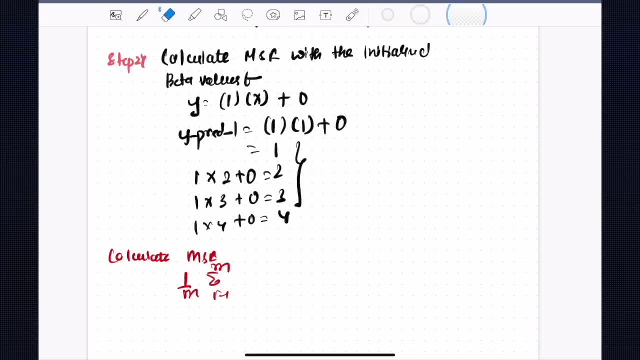 of now. let's ignore two as of now. what do you say? let's, let's ignore two as of now? uh, because of uh, and just just just just for sake of simplicity, more, but eventually we'll use this two. so maybe let's add two over here as well, one by two m, but uh, but eventually we are, we're just going to take. 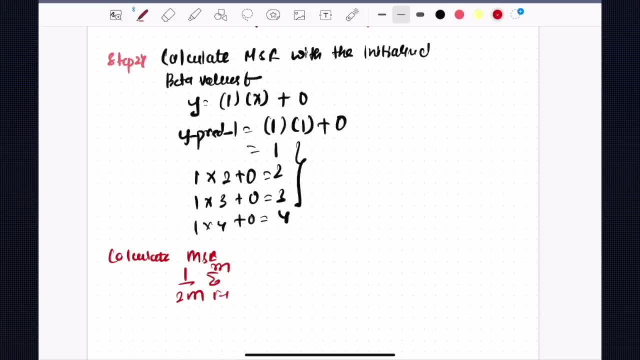 the squares, nothing else more. so let's stick to this one. what do you say? let's stick to this one. it's much more. you? uh better. so one by m? um, of course we will. we'll change it later, but my point is not to make it. 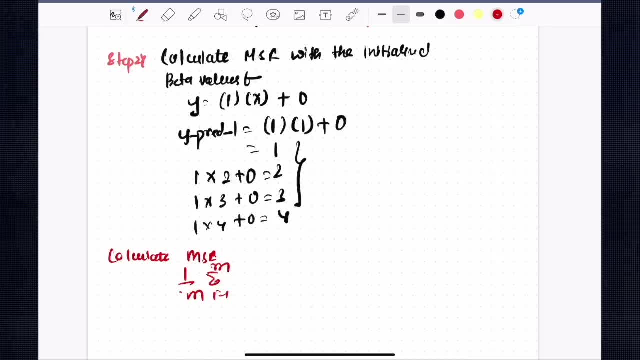 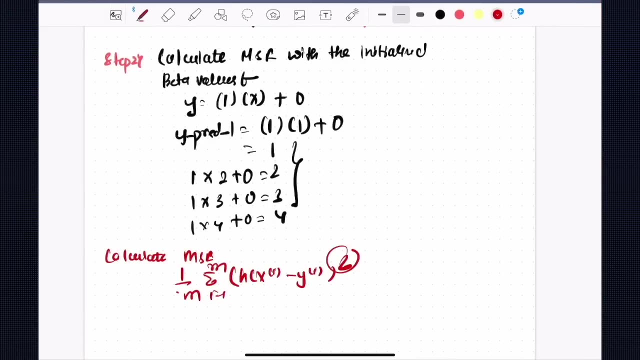 perfect, accurate, but as of now, uh, if, if, if you see in your machine a machine learning libraries, they're consistent enough. but let us use simple, very simple, without using two or anything, which is one by uh, and you have your edge of xi, edge of xi minus yi, squared for the square for removing 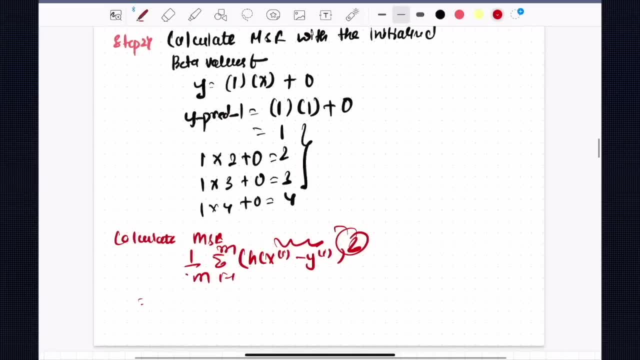 and the difference is a square for removing the negative sign. so now you items u and u, that is a simple gray, and the t, which is put together in a three-dimensional kind of system where basically theенкоT, oh the, is devoted one and now it will yield to one minus. 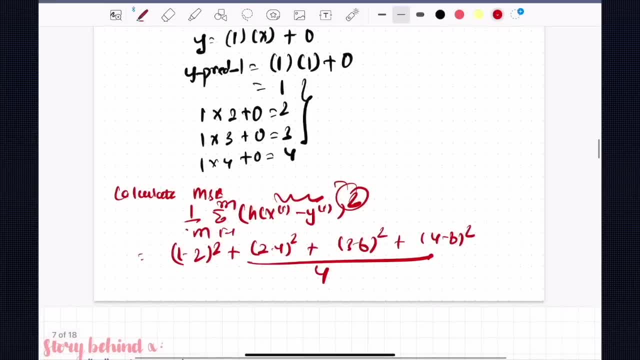 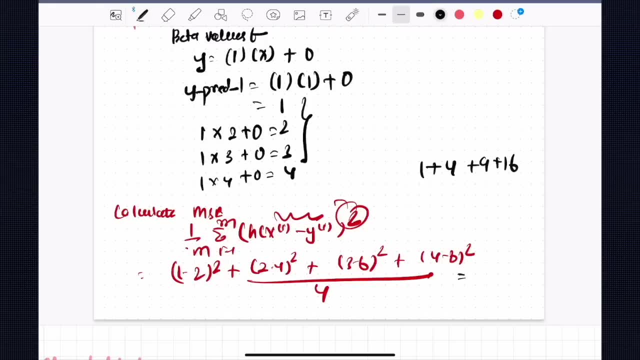 two squared plus two minus four squared plus three minus six squared plus four minus eight square, divided by four, divided by four, and that will yield. that will yield nothing but one plus four. one plus one plus four plus nine plus sixteen divided by four, and that is the third: p plus four. 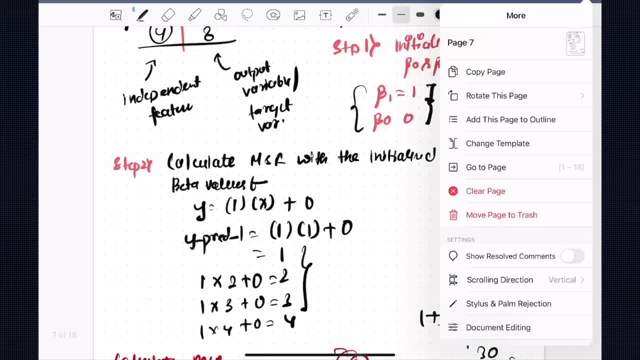 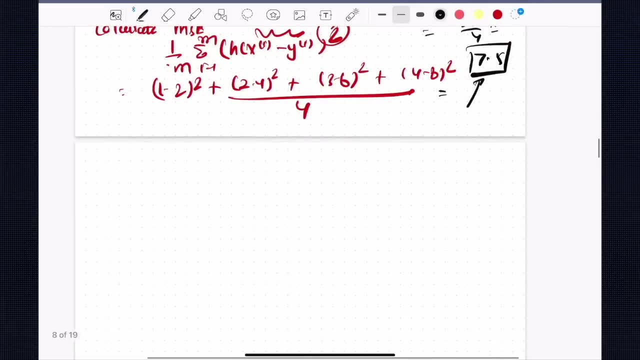 which is nothing but seven point five. okay, this is your error. this is your error if you utilize these two, two values. now let's add one more page. let's add one, one, one, one more page now. once you have the once, once you have the MSE, now you have to use gradient descent. 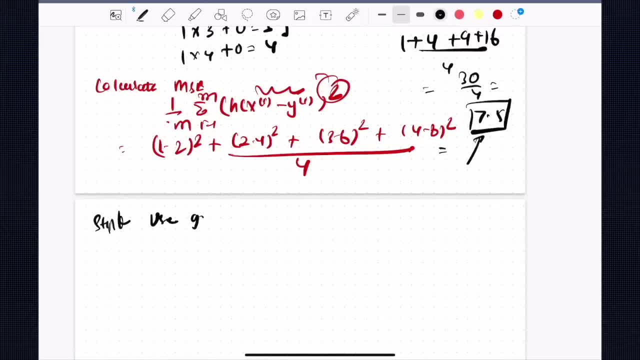 now a step is you have to use, use gradient descent. use gradient descent to minimize, to minimize your, your cost function, which is G of beta, which is G of beta. so to use gradient descent to minimize that cool. so let's eventually talk about how can we eventually do it. so your cost function is. so I'm going to. 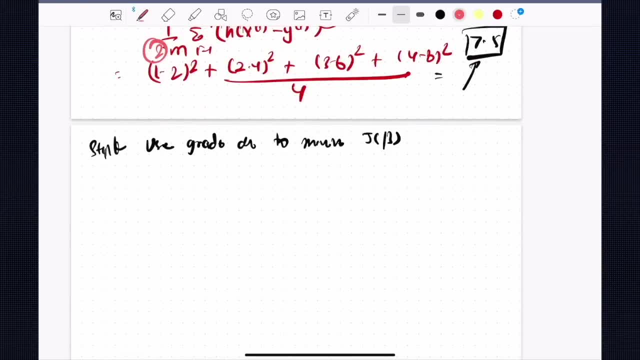 rise the conventional cost function to show you what exactly this two means, in how exactly this to eventually help us. so this it will make you more clear. so 1 by 2 M, your I is equals to 1, all the way down to the M edge of X I minus Y I. 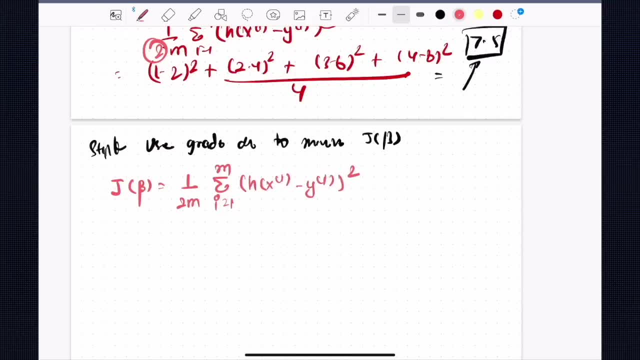 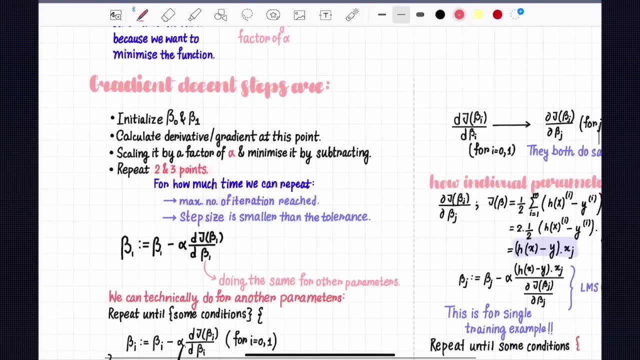 squared. so this is your cost function. so, basically, what our goal was: to take out the partial derivative of this, of this, because our, what was our gradient gradient is the formula formula, was this formula right? so we have to take out this. we are will take a, will take out the derivation, will will take out the. 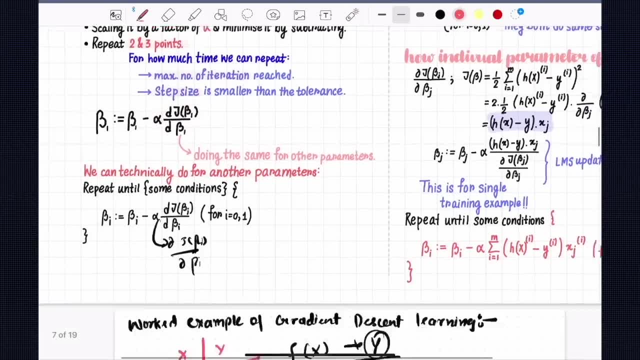 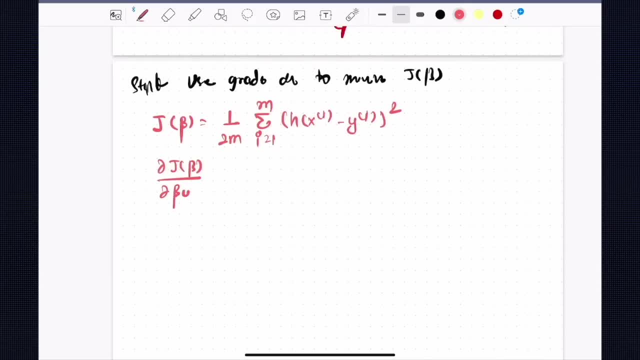 field. do the calc will. they could do the calculation of this. how, how you're going to do, you will see it right now. so you're going to go. the derivative of G of beta with respect to: with respect to beta 0. first of all, let's, let's do for. 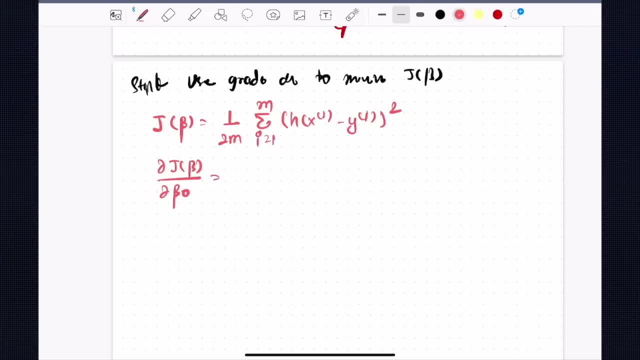 beta 0. okay, so what, this is with. well, we'll turn it will tell how much cost one pergola 당신 When your beta 0 changes. so it is nothing. it is nothing. so what, what we're going to take of the derivative of this whole set of function, this whole function? so how does this? 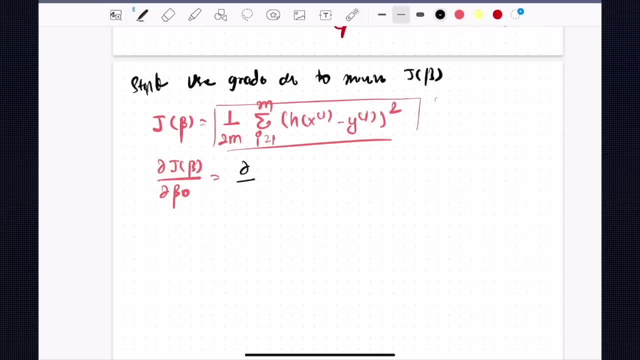 fail. so which is nothing but derivative of of the whole function, will write that, with respect to beta 0, whole function is 1 by 2, M is equals to 1, all the way down to the end edge of X. i minus y, i squared. okay, this is your. this is which, which keyiva the y of x and y square. okay, this is your subst. 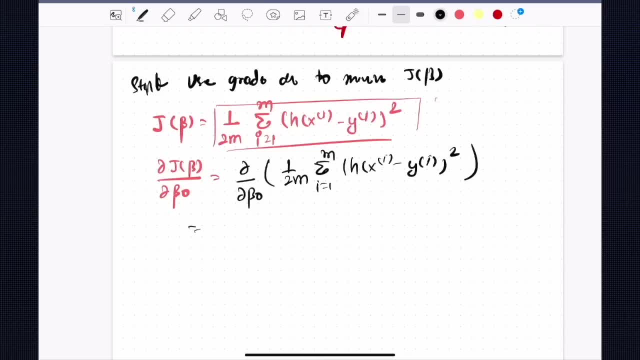 going to solve. So what I'm going to do, I'm going to take out the sum rule- sum sum, sum outside. so I'm just going to take out the sum rule outside, which is 1 by 2m. 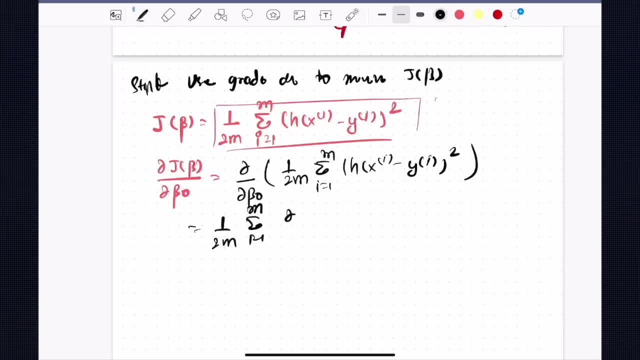 i is equal to 1, all the way down to the m. Then we take out the derivative. then we take out the derivative of your, of your, this function, which is over here you're going to apply the chain rule. over here you're. 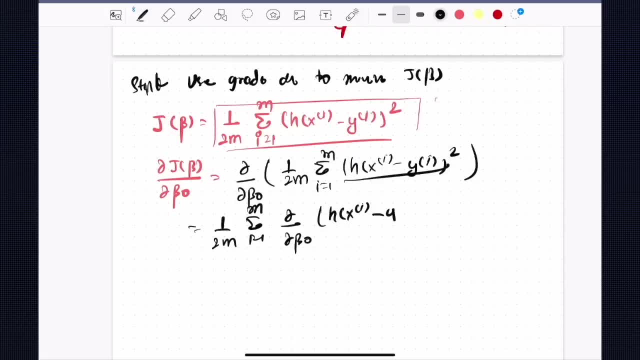 going to apply the chain rule on this particular function. so x of i minus yi squared. okay, Now you're going to take out the derivative of this. How are you going to do it? We have a two function, one inner one. 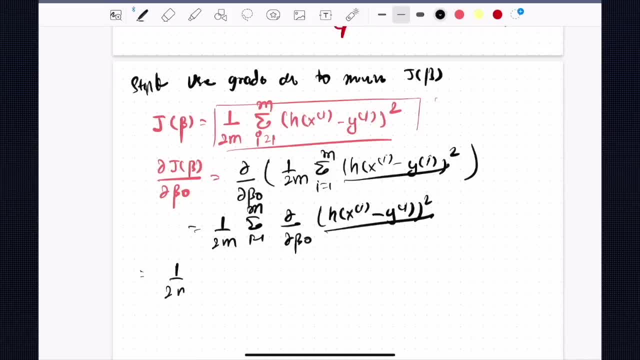 outer. So you will take out the 1 by 2m. 1 by 2m i is equal to 1, all the way down to the m derivative of this particular cos. function that derivative of this particular cos. 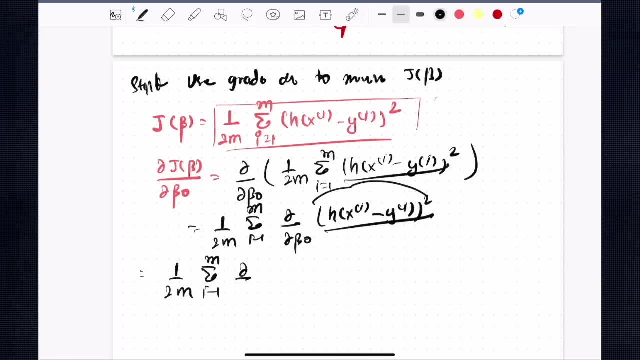 over here you put the outer function multiply. this is over. here we're going to apply the chain rule. over here we're going to apply the chain rule of calculus. so we are going to take out the derivative of outer function, leaving as it is inside. 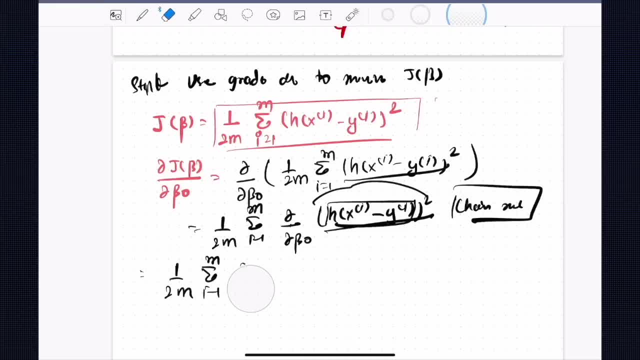 times the derivative of the inner function, The derivative of outer function is nothing but equals to 2, comes over here by the power rule, and then we subtract minus 1 from here, so 2, and we leave the inside as it is, as it is for outside. 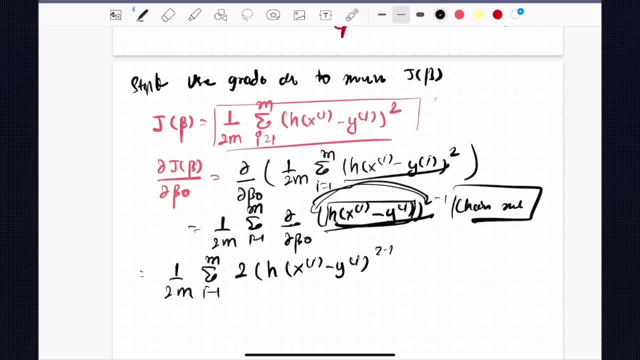 derivative, and over here, 2 minus 1 is nothing but equals to 1, multiply times your derivative of your inside function, which is beta 0, and say: inside function is nothing but minus yi. okay, So this is your. 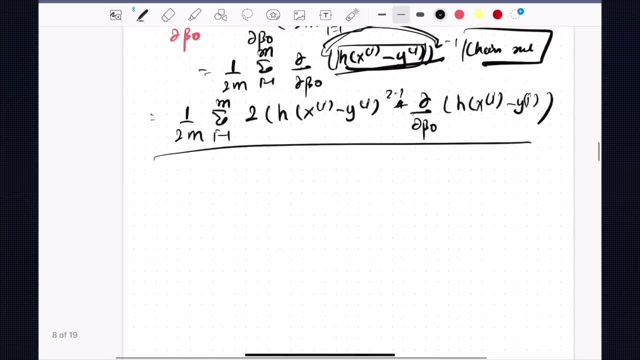 equation that you're trying to solve Now: 1 by 2m. 1 by 2m i is equals to 1, all the way out of the m, all the way out of the m, and then you simply solve for it. 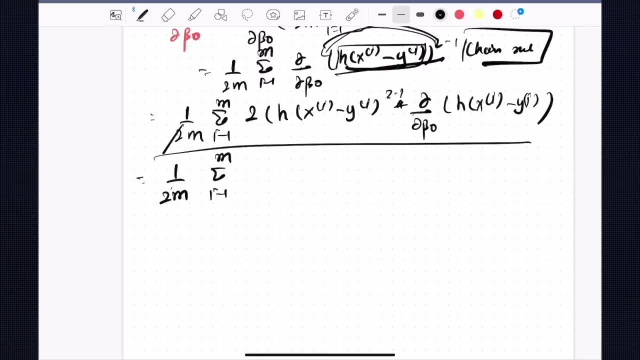 which is nothing, but your 2 and 2 cuts out. so you see that 2 and 2 cuts out, so now we will not write 2, and then your final answer would be: 1 by m, h of xi, h of xi minus. 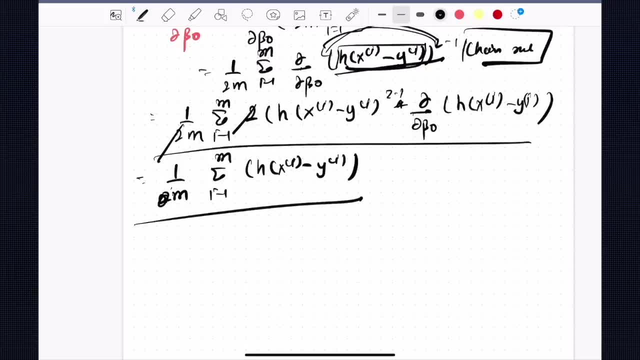 yi. This is your derivation. this is your derivation. You might think: Yayush, what happened to this? This becomes equals to 1, this becomes equals to 1.. Why, Why do we say that this is equals to 1?? So let's. 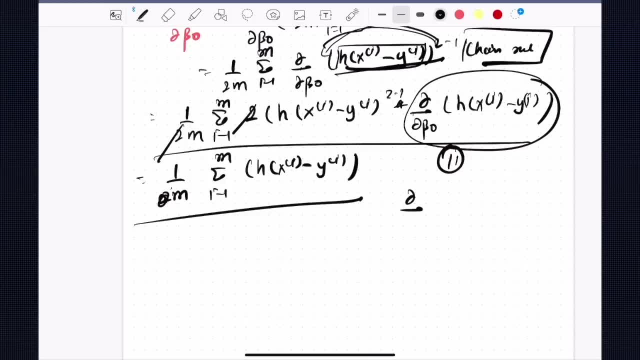 talk about why exactly this is equals to 1.. So, when you take out the partial derivative of this function, h of xi, h of xi minus yi with respect to beta 0,. with respect to beta 0,, what exactly if we expand this h? 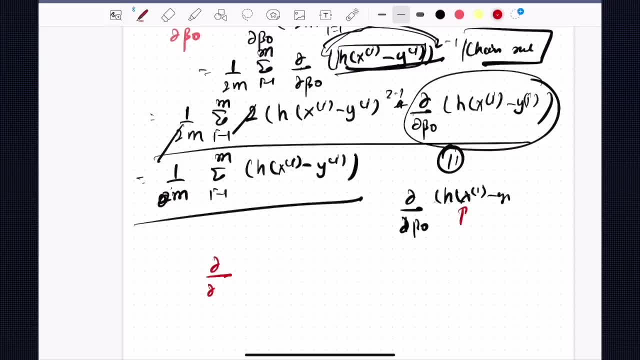 of xi is nothing, but is nothing. but let us assume the beta 0 plus beta 1, xi minus yi with respect to beta 0, right, So over here we are going to take the with respect to beta 0, so except beta 0,. 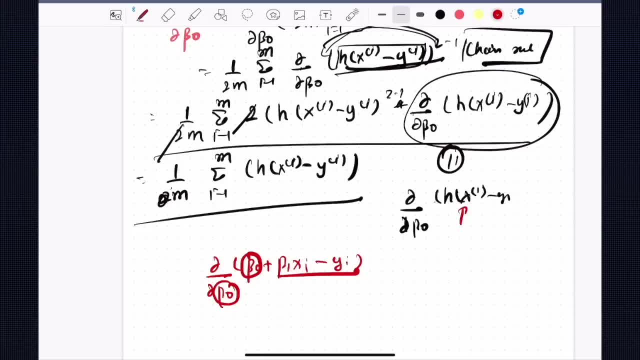 except this: everything is constant. everything is constant. so that will be nothing but equals to 1.. That will be nothing but equals to 0. So everything is constant and that derivative is nothing but equals to everything is 0, okay. 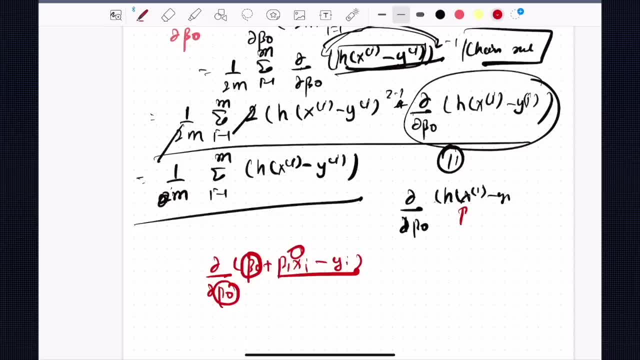 Now over here, now, over here, now, if you go and if you see that everything will be 0, because it is except 0, which is nothing but, and the derivative of the constant is, you know. so, now, now, you see, now you add the derivative, now this, this one, because this respect this. 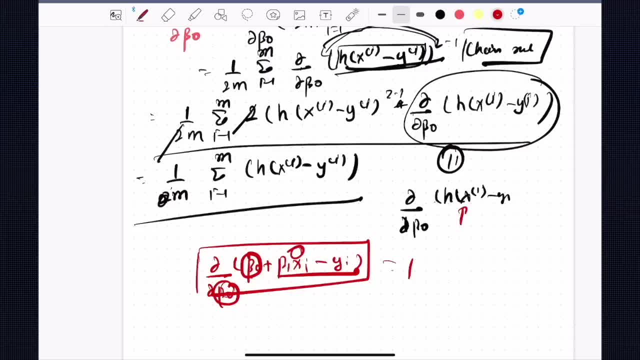 is, the whole equation will come to equals to 1. why because? because because, when taking the partial derivative with respect to all the letters except the, except beta 0, are treated as constants and their derivative constant is nothing but 0, and then you have beta 0 when you take out the. 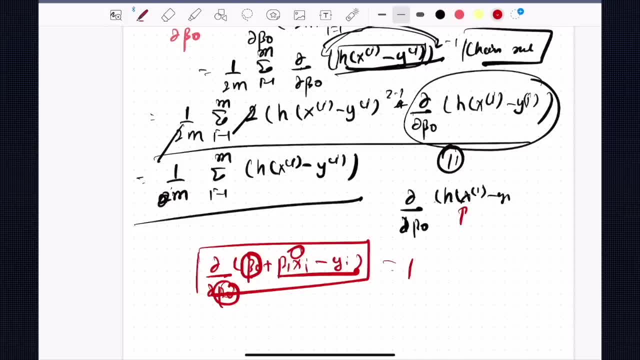 derivative, that is nothing but equals to 1, and you have 1 over here, and when you actually do that, because it's it it does- it does not have any constant and even if it- as as we know that a v, it, it has a constant x 0 and x 0 is nothing but equals to 1, right? so i hope that it makes sense. 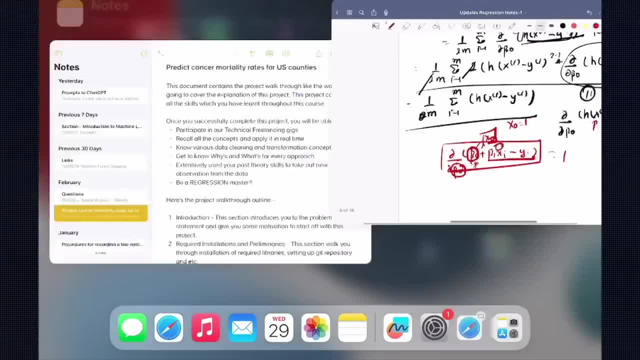 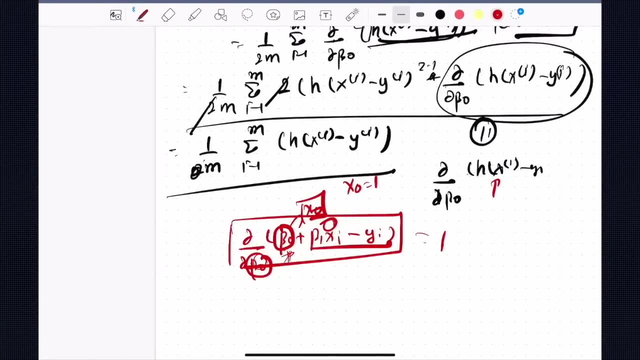 to you as well? uh, if it not, please see my calculus lectures. please see my calculus lectures out here. it will make much more sense. if you see. i'm not going to go in depth explanation, but you can understand this way that we come up with, when we actually take out the partial derivative of: 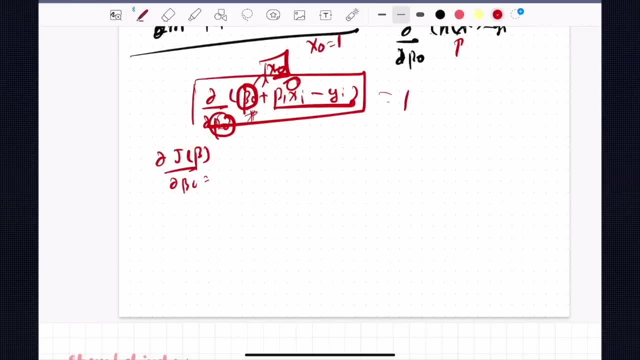 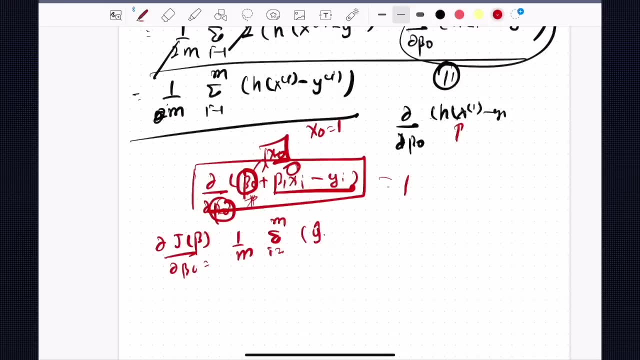 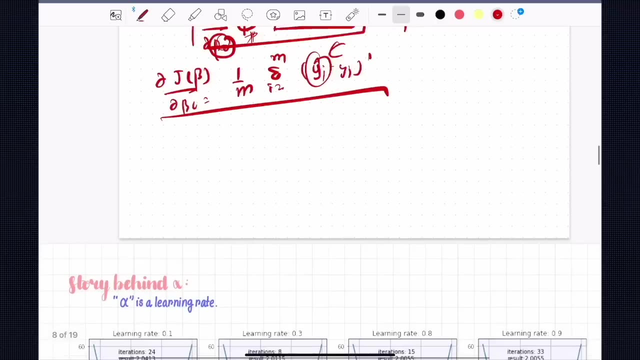 geo beta with respect to beta 0 is nothing you, but 1 by m. 1 by m i is equals to 1. all the order of the m, y hat i minus y i and y hat i is nothing but the model predictions plus okay. so this is your beta 0. now we'll do for beta 1 and now we'll 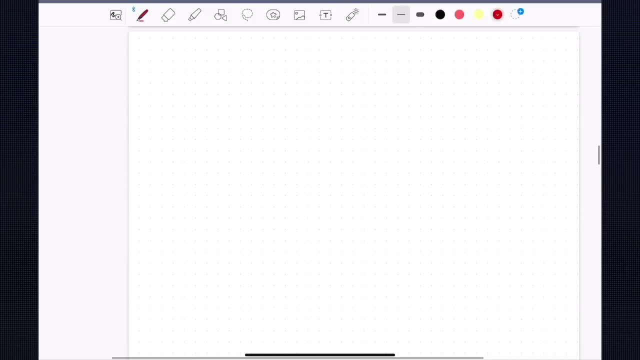 do for beta 1. okay, beta 1, exactly the same. the only thing changes instead of 1 now. so when you actually uh, every, everything remains the same. so, and when you actually take out, the derivative of beta with respect to beta, 1 is nothing but equals to: everything remains the same. everything remains the same over here. 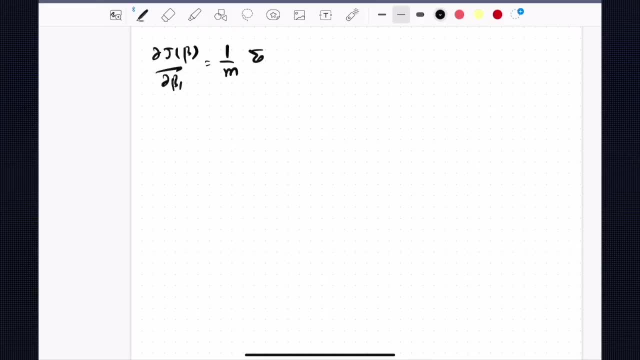 everything remains the same: 1 over m, 1 over m. uh, i goes to 1. all the order of the m- y hat i minus y, i multiple multiplied by x, i multiplied by x, i, y multiplied by x, i. because now, in this case, now, in this case, when you actually take out the derivative of this, 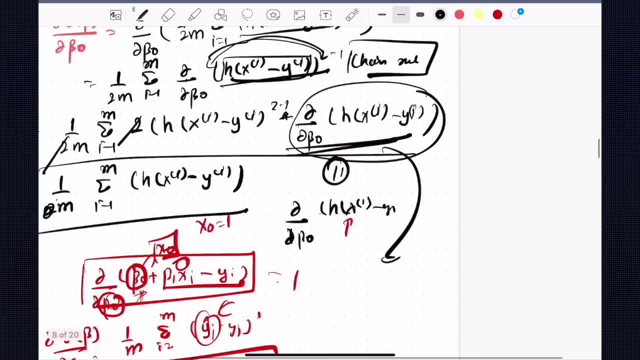 take out that derivative of this, you will notice that now h of x i is supposed to beta 0 plus beta 1 x i minus y i. right, so now take the derivative of this: everything except this one is constant, this one, this one, everything is constant. now over here, then actually have beta 1 times x i, the 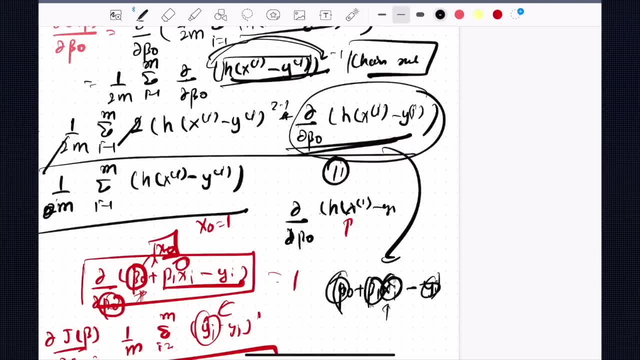 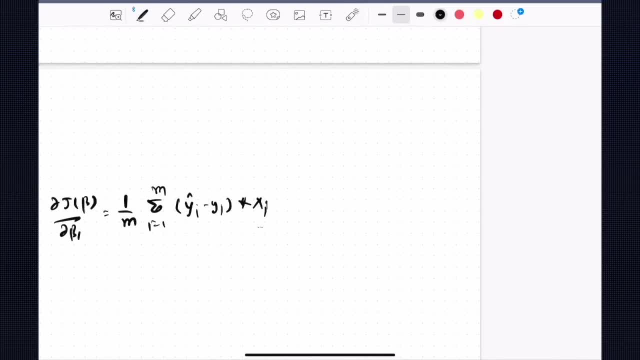 constant is that the, the, the. this is the coefficient of the curve x- i. so this is x, x, x. i would be over there, okay, so x, i will be, uh, written over there. please see my lectures. uh, if you are confused, like how this x, i? again, this is a rule of calculus and all. if you don't know, please ignore. 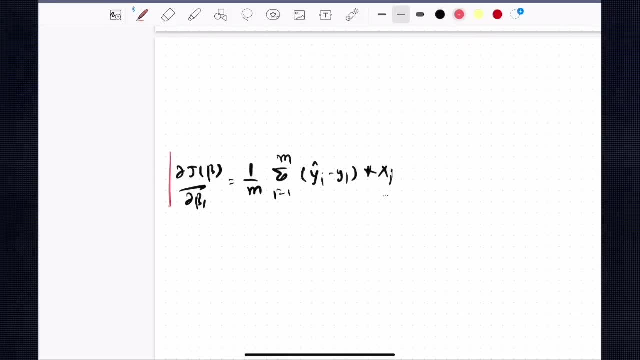 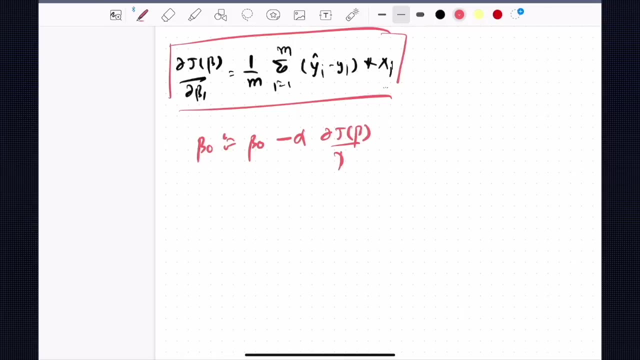 it. uh, now, over here you have you. you got this for beta 1 as well. right now what you need to do. we had an update rule. now we have to update beta 0- old beta- minus learning, the alpha, the derivative of beta- with respect to beta 0. and then we have beta 1, beta 1 minus learning alpha with respect to. 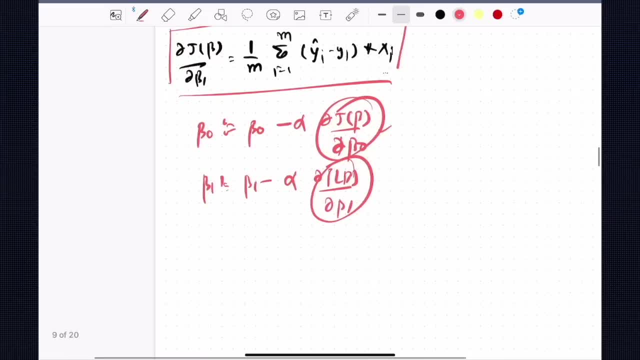 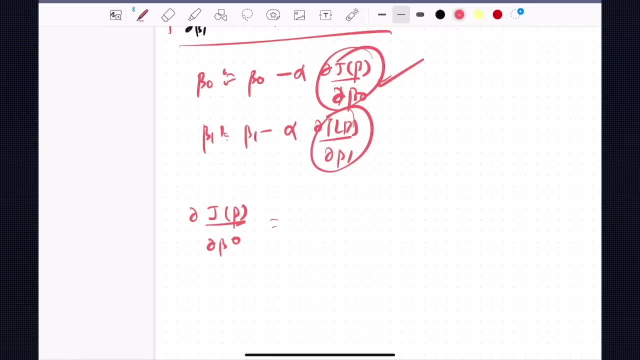 beta 1. right you, you have this, you have this. so let's calculate this one, let's calendar the first, first one. the partial derivative of beta with respect to beta 0 is nothing. but we have already taken out, i've already taken out the equation. this was our equation, right this? this was our. 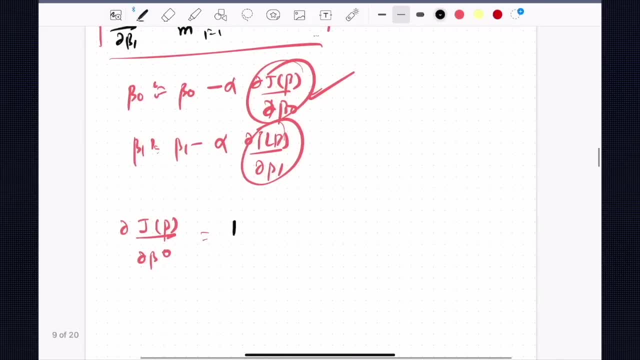 equation. so, first of all, our prediction, our prediction: 1 minus 2, multiplied by, multiplied by- uh, 1 minus sorry, yeah, 1, 1 minus 2, we and we are multiplied by 1, so it's, it's we, we should not write anything. 1 minus 2, and and then you have 2 minus 4, which is your prediction, minus the actual. 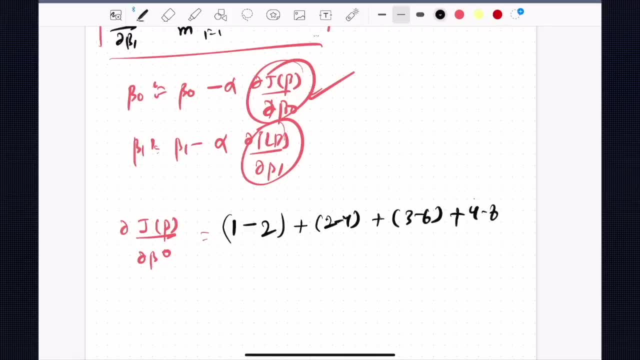 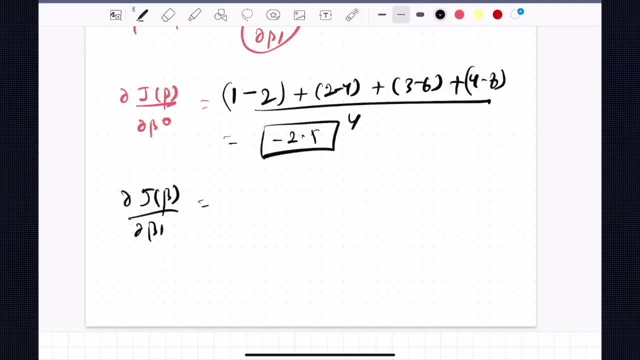 value plus 3, minus 6, plus 4, minus 8, and then you divide by the total number of values, which is 4, which is nothing but which is nothing but minus 2.5, which is the rate of change. okay, you do the same for j of beta. with respect to beta 1, which is nothing, you will get nothing but 1 minus 2. but 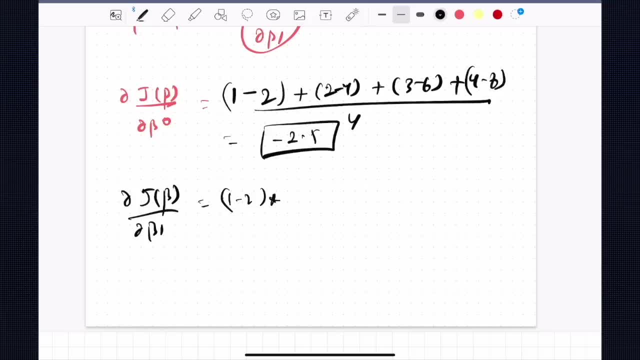 this time you're multiplying with xi and the first, everything you're multiplying with xi and the first everything you're multiplying with xi and the xi, which is x1, and this is for x1, right? the x x1, is that nothing but equals to 1? so if you go, 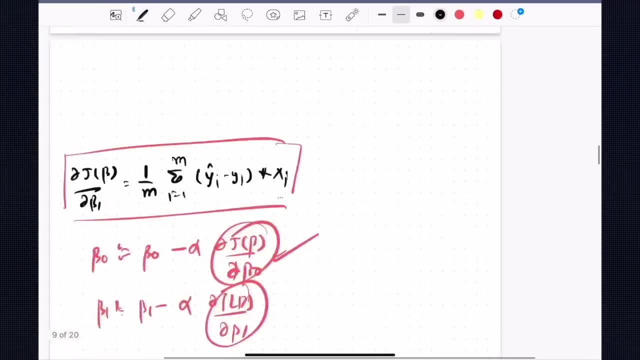 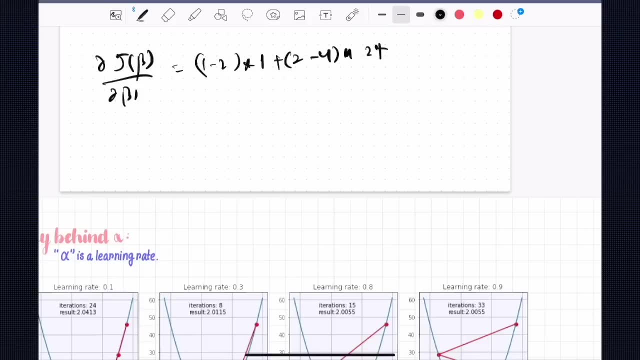 and see that x1 is nothing, but is now you. now you do for sec, sec second one, you do for a second one, which is uh, 2 minus 4. you simply add plus 2 minus 4, multiplied by 2, plus 3 minus 6, multiplied by 3. 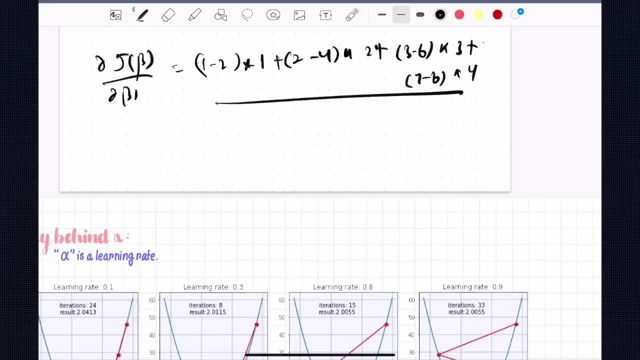 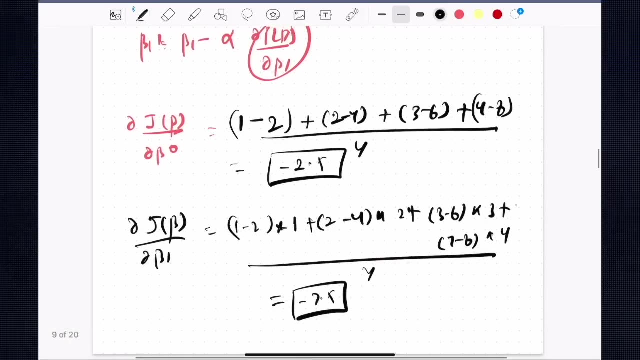 plus 4 minus 8, 4 minus 8 multiplied by 4, and then you divide the total by 4, you get nothing but minus 7.5. you get nothing but minus 7.5, minus 7.5 when you calculate. so your uh, with the current value of beta 0 to be 0 and beta 1 to be 1, 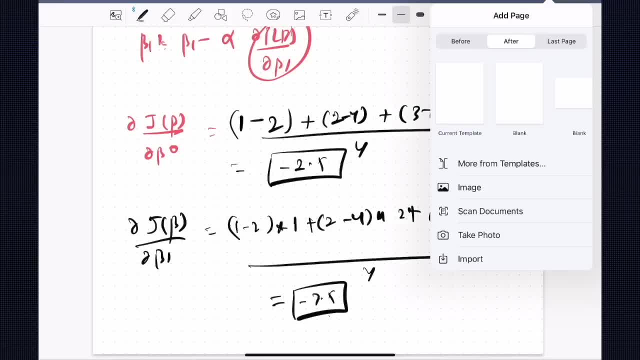 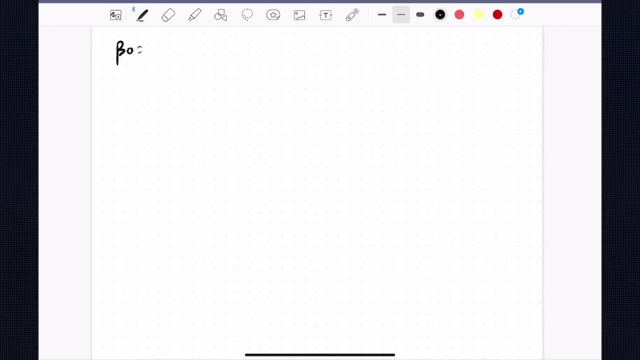 is nothing but minus 2.5 and minus 7.5, which is the rate of change. now, once we get it. now, once we get it, we can simply apply our update rule. our update rule was: first of all, let's, let's do for beta 0. our old beta 0, which we initialized, was 0 minus learning. let us assume that your learning 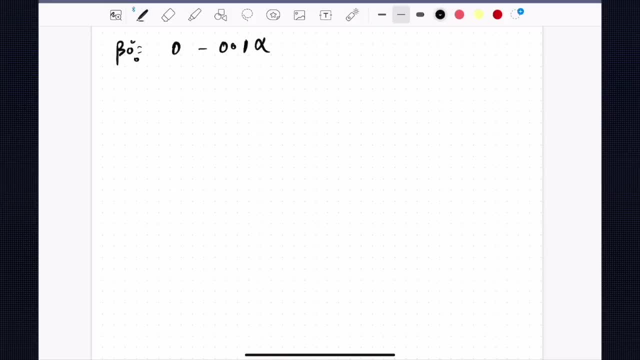 rate is alpha. we'll talk about learning the alpha in great detail multiplied by this learning rate, multiplied by the rate of change. and then we'll talk about learning the alpha in great detail multiplied by the rate of change. and the rate of change for beta 0 was minus 2.5, right, and the 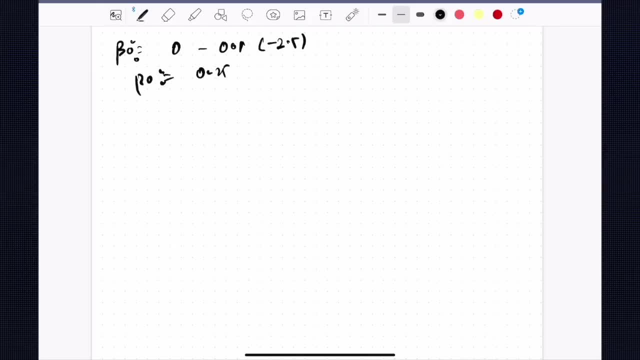 beta 0, the updated beta, beta 0, where is 0.25, and then your beta 1. you do the same. you have 1 in this case, because the old beta was 1 minus 0.1. multiplied by minus 7.5, you get nothing but 1.75. 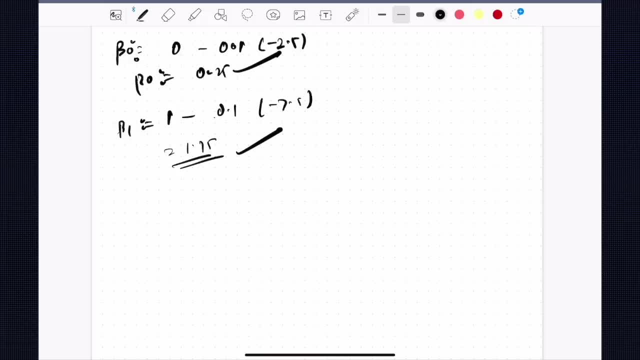 that's an output. okay, this is beta 1. this is updated beta 0. updated beta 1 after in the first iteration. okay, as because it now you were: what now, what you're going to do is you're going to do what you do now. this. this is now. you're done with the baby: beta 0 and beta 1 in the first iteration. 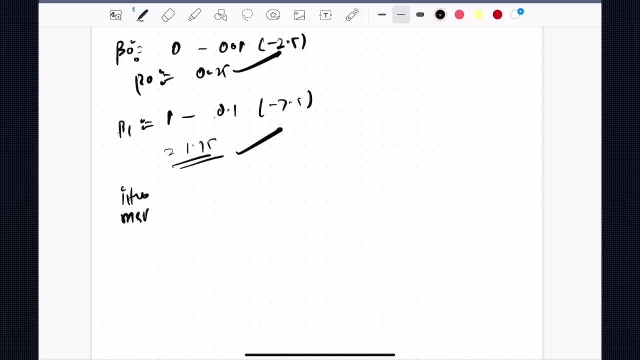 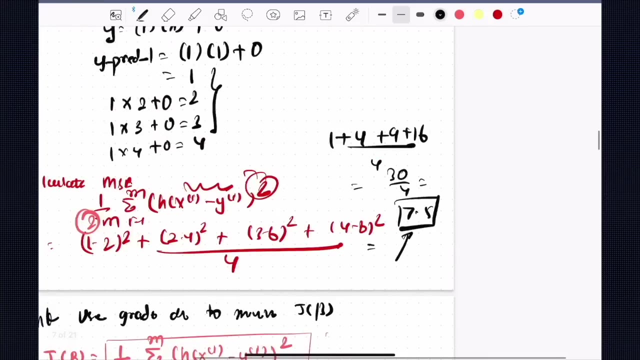 in the next- it's done in the first iteration- you calculate the mse and the updated beta 0 and beta 1 calculate the mse and you'll be noticing that your mse and m msc is low is low. so when, when you calculated, when you calculated the msc with uh, with this uh, with beta 0 to b, with beta 0 to b1 and 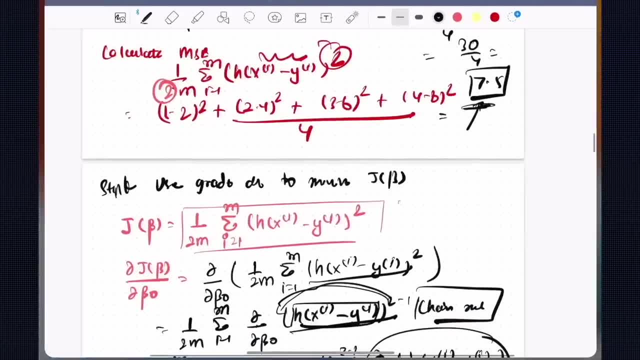 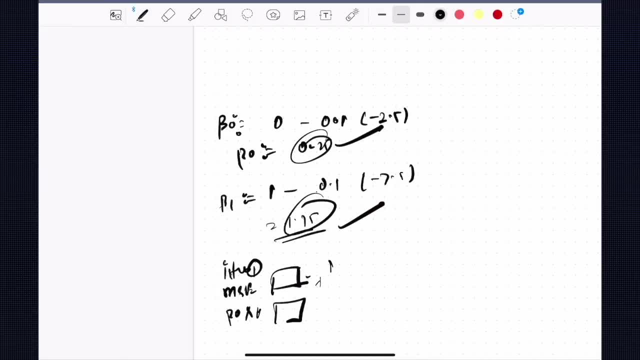 0. it was minus it, it was seven seven, seven point five. but when you'll calculate your mse with 0.25 and 1.75, it will be less as compared to previous one. please note that you can try it out as well. and then you do the. 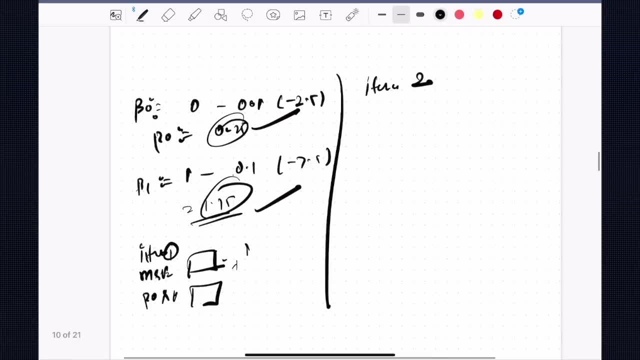 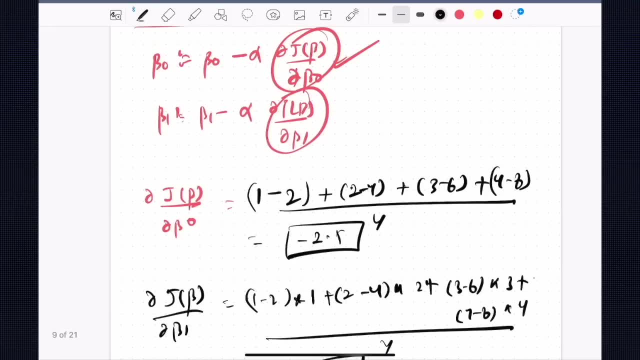 next iteration number two, maybe an iteration number two? you do the same step. now, what you do? you calc, you calculate the mse, you plug in the values of, you plug you again. you again make the predictions. you again make the predictions with new beta value. you again make the predictions. 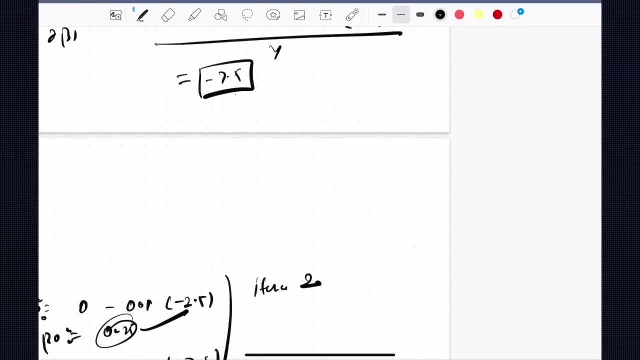 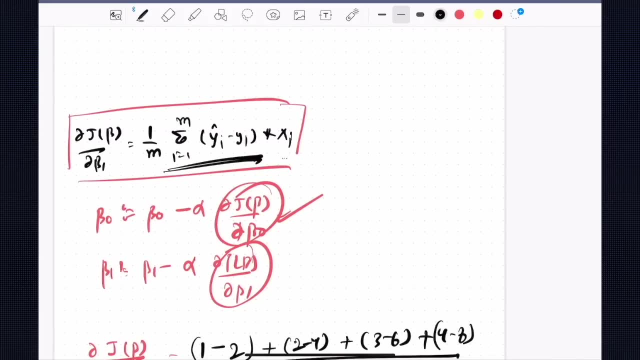 with the new meta value and then you uh, take out the error. and after taking out the error, you simply apply the update rule after calculating this derivatives once again, how this derivatives is calculated, you have your new predictions right? if your new predictions and new predictions, you will get that once again, and then you have to calculate that once again. you're getting new. 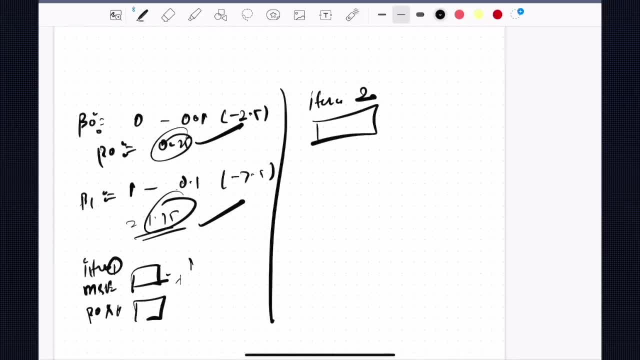 derivatives, and then you calculate and then you have the iteration number two, iteration number two as well iteration number three. you do the same and all the until you reach to 20 or whatever number of iterations which are fixed up. okay, i hope that you're getting whatever. whatever i'm trying to tell you can try out this by your you may be. 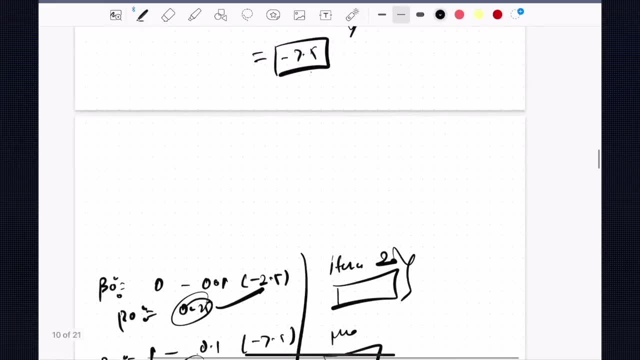 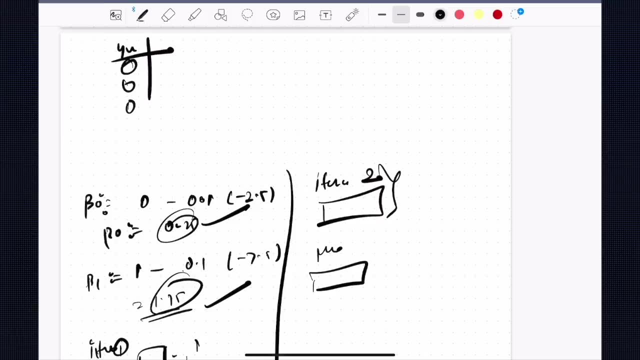 confused about iteration number two, so let me just be clear about it. what exactly i wanted to, what you can do? you can, first of all, you be you. you have got new betas right. you make your y thread once again, once again. now you get your four predictions. after getting four prediction, you 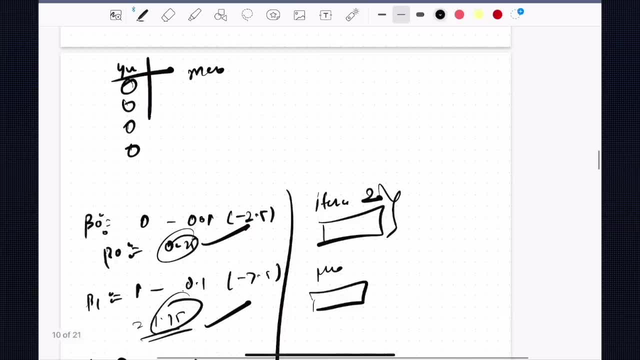 take out mse. with these four predictions you're taken out. good, now what you do? you have- you all already have- your uh partial derivative of cost function with respect to beta one and beta two. you have some equation. you plug in the values, now the. now the derivative you'll get is very different. why? because your predictions will change. because you 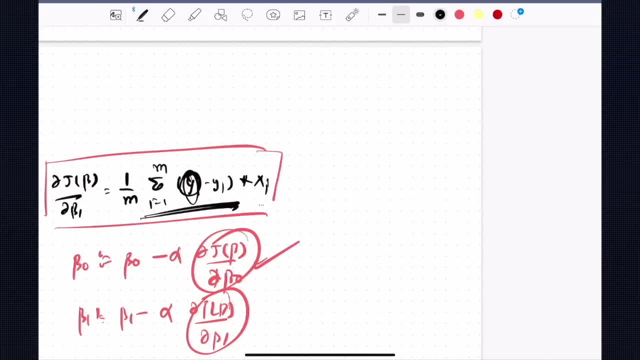 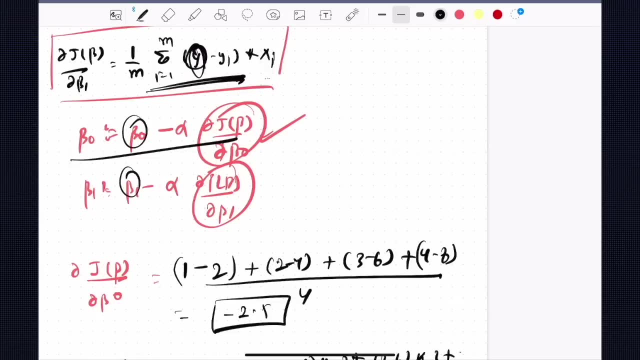 have because you're using new beta value, new parameter value, and your predictions will change, of course. so beta, the, that derivative also change. and then you plug in the derivative over here. now beta 0 and beta 1 will be different. where beta 0 is 0.25 and 0, beta 1 is 1.7. 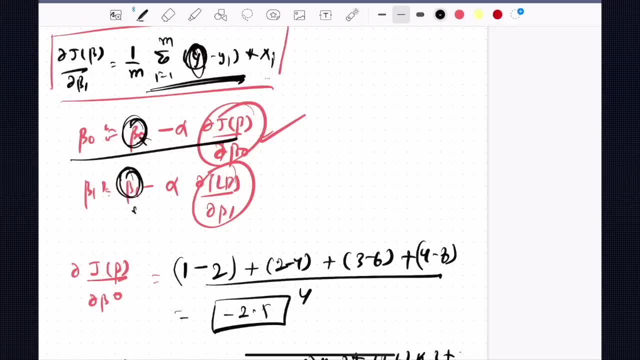 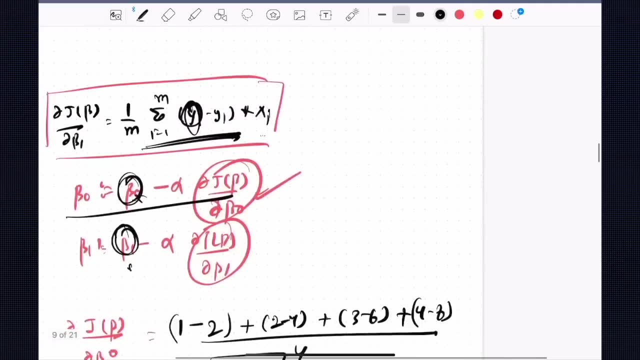 uh 75 minus 2.5 and beta 1 to be 1.75. right now again, you will be getting new betas where the mse will be lower as compared to previous one. i hope that this gives you a good sense and i really hope that you understood this as well. 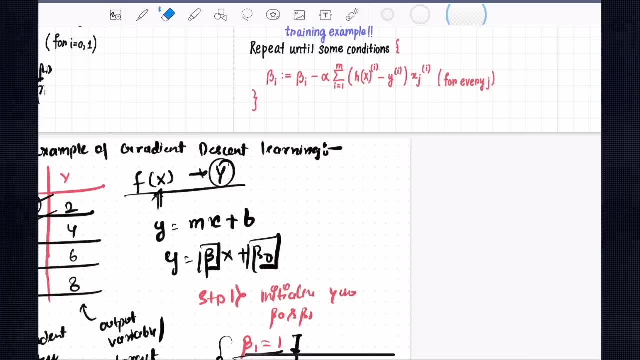 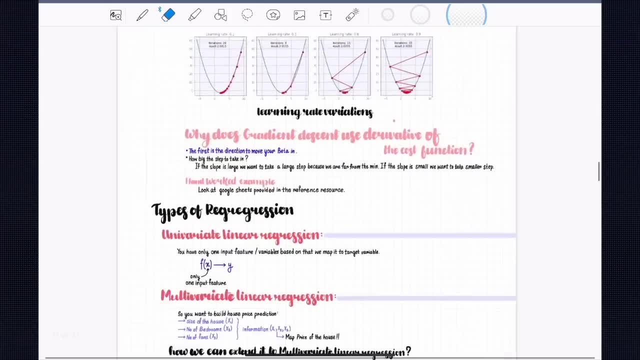 now. i'm just going to uh. now we'll ask you to take brain, because this was something you know. uh, very tiring as well for me and it may be tiring as well for you. in the next lecture we'll talk about uh. why does gradient descent use derivative? what is the significance of it? and i'll give you a. 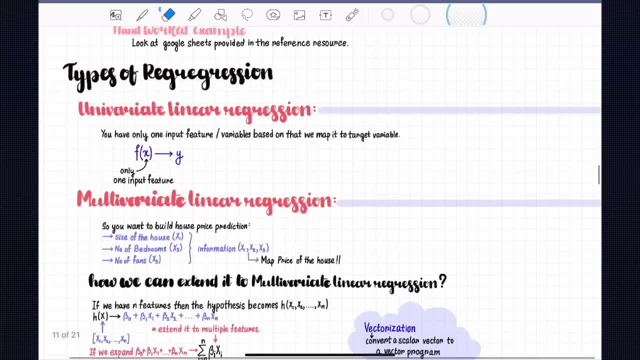 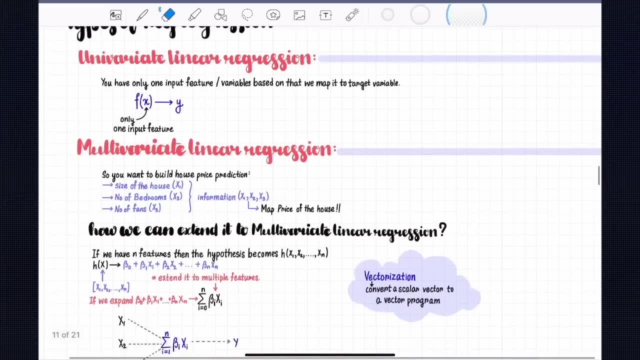 google sheet where we have- we have one more solved problem of it, and then we are finally done with learning, and then i'll recapitulate you everything, make your summary so that you understand it, and then we'll go to other forms of linear regression to study more about a lot of things. so let's catch. 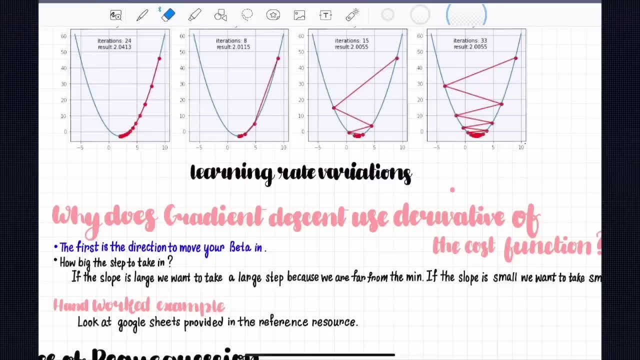 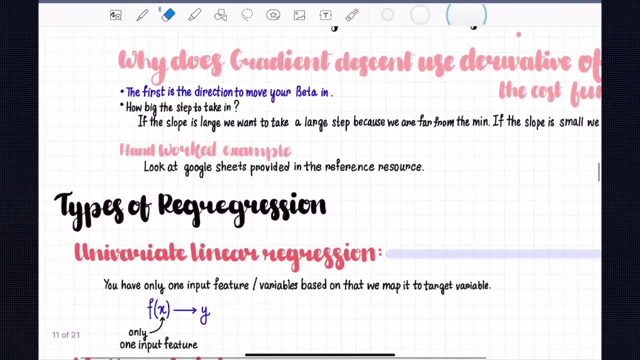 up in the next lecture. hey, everyone, welcome to this lecture. uh, so, basically, what i'm going to do today is talk about some of the key terms which may be, uh, useful for you, and then we'll talk a bit, have a bit of discussion around, um, some of the types of regression algorithm, which is the 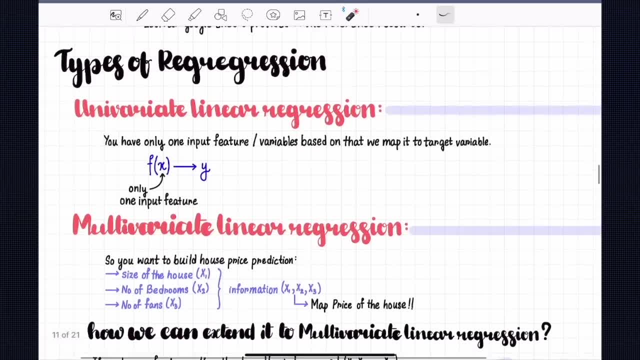 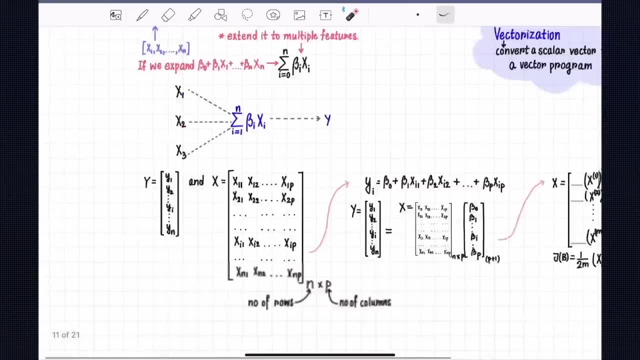 univariate or simple integration, or multivariate and multiple linear issues. we'll talk about the differences and all in great detail, okay, and then we'll get started with extension form, which is quite easy to understand with if you have understood the previous one. so first of all, let 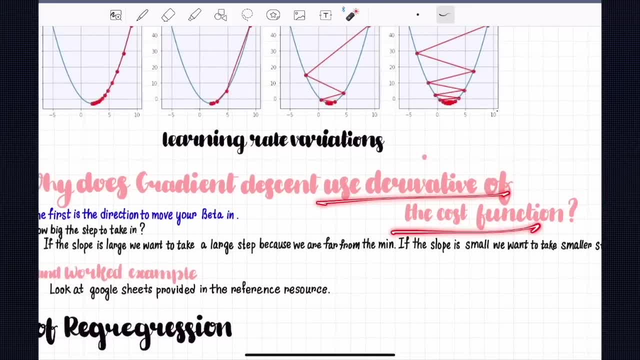 let us understand. why does gradient descent use derivative of the cost function? so first of all, let's figure out that in so, in. so, basically, in linear regression, so in linear version, what was? what is your eventual goal? what is your eventual goal? that's a nice question to start forward. so your eventual goal is nothing but to. 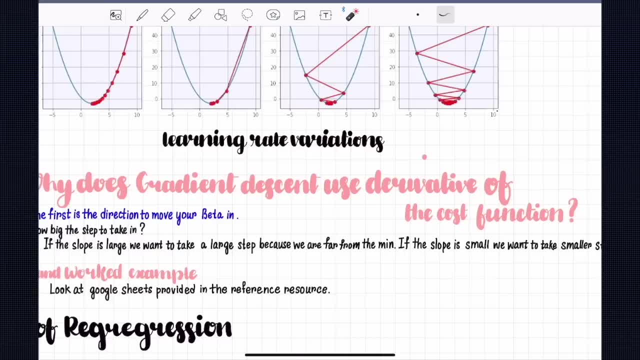 minimize, but to minimize your cost function or your mse so that that is a goal and and and your error between, or to minimize the error between your predicted and actual target value, so that we take that partial derivative, partial derivative of that cost function with respect to a particular. 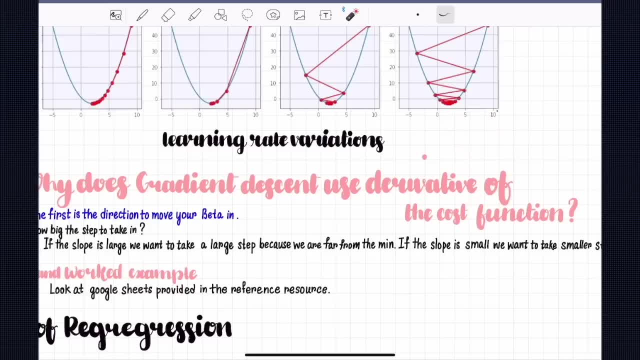 parameter or a coefficient- assume that, in this case, beta zero. okay, so particular parameter coefficient and which? so what does that derivative gives us? of course it gives us the rate of change, but what in terms of how does this help us to go down? or how how does it help us to reach to global? 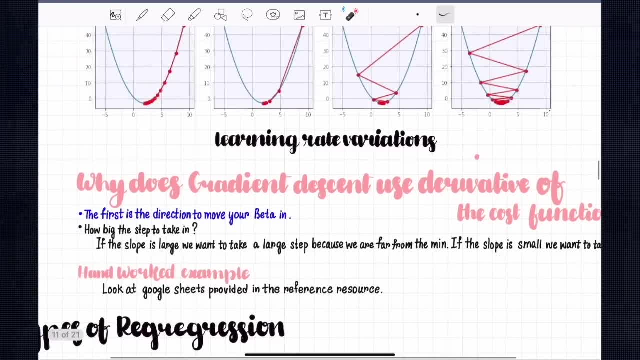 minimum? that's a very nice question to ask. the first it gives. the first is the direction to move your data. be right, whether to increase the beta or whether to increase, decrease the beta. right, so it also gives whether we should increase the beta, increase the value from one to increase or decrease. 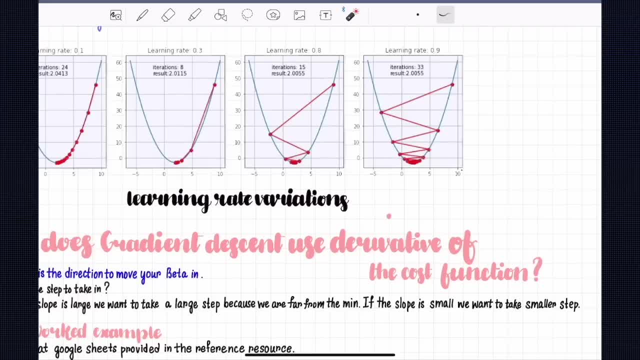 the beta. that's what it gives, so direction, to move your coefficients or parameters in in order to minimize you, your error. so, for example, if you have a current zero, should we minimize or macro? so should we move, should we decrease or should we increase this? so this exactly, the derivative tells and it tells in. 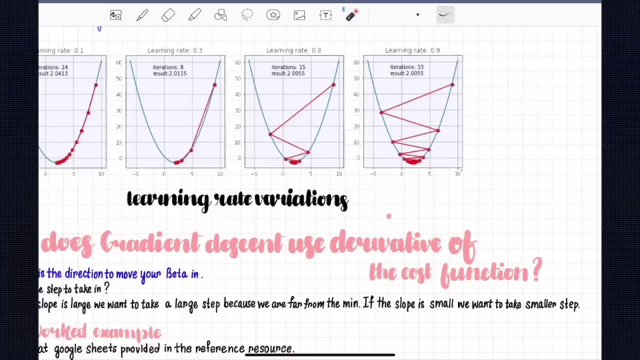 such a way that it minimizes the error, minimizes our mse. okay, so the derivative of your mean squared error with respect to a coefficient, with respect to a coefficient or a parameter value or any kind of beta zero and beta two, sorry, beta one and beta zero provides the rate of change of the mse with. 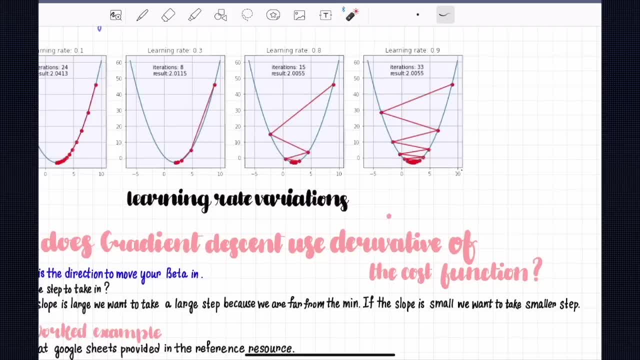 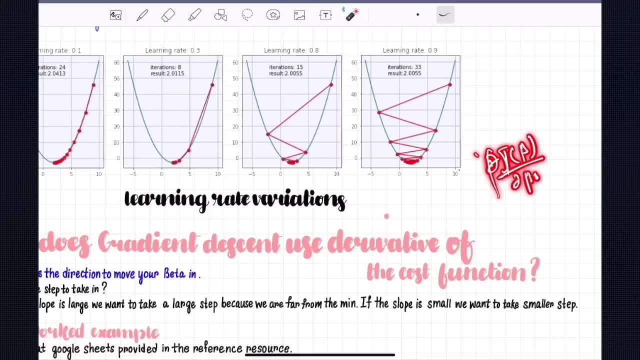 respect to particular. so how much that changes when this changes. and in support example, if you're derivative, if we, if we, if you did a derivative, if you're derivative is positive, the derivative is positive, which is the rate of change is positive, then increasing the value of coefficient will decrease. 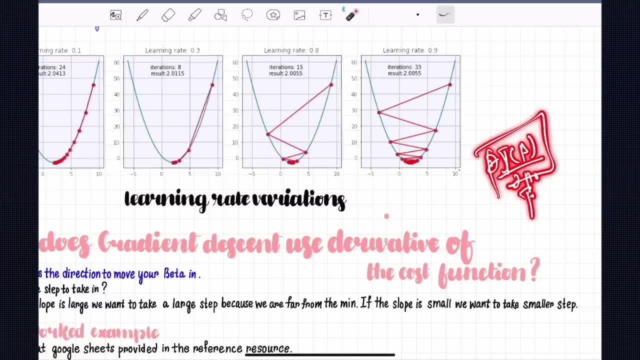 the error. okay, first, please note that what I've, whatever I'm telling, if the derivative is positive with respect to this, so it tells that if we increase the value of beta, if we increase the value of beta, if beta is increased, then the error will decrease. so if it is positive, then we increase. 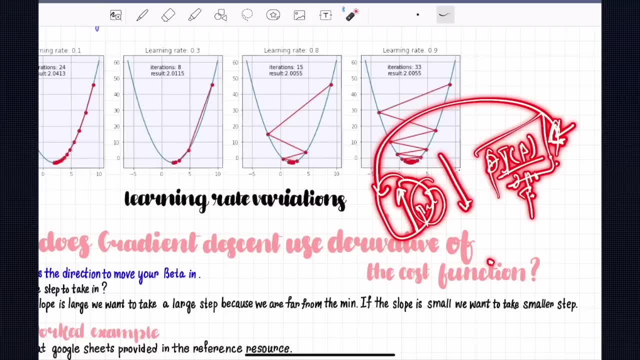 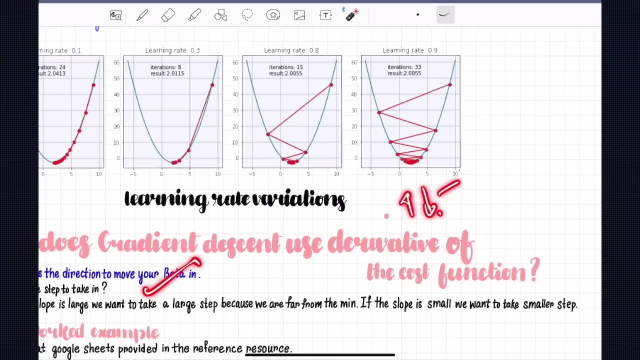 the value of beta. please note that this is the most famous question when we when we talk about the interpretation, because this, this derivative, also gives the direction to move, whether to increase or decrease, uh, digi or theta, in order to minimize the error, right? so if your derivative is, 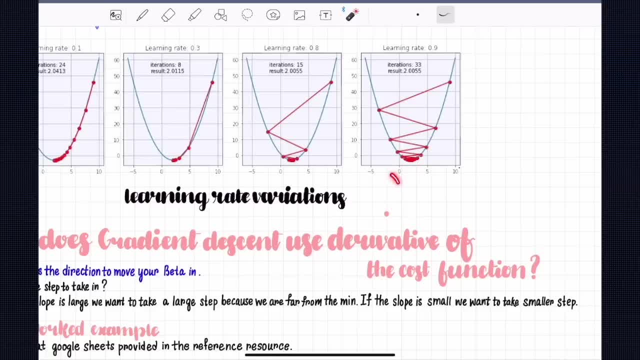 positive, then if you increase the beta, your error will decrease means if the, if it is positive, if the derivative positive, it increases your beta. okay, and if your derivative is negative, then increasing the value. so, for example, um, yeah, so, uh, just, uh, just for a note. uh, over here i think i 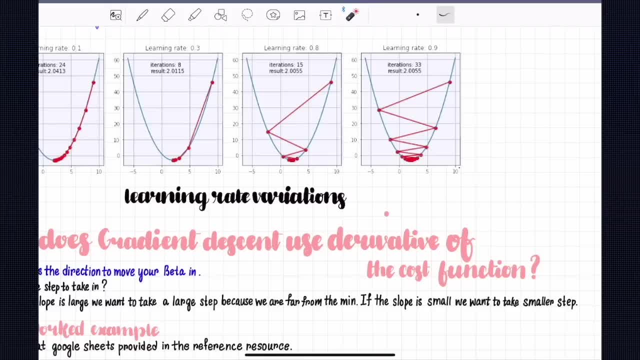 i. i had a very wrong interpretation. i'm going to retake it. i'm going to retake it. okay, so now the derivative of mse with respect to a particular coefficient provides the rate of change. how much cost function will change when you change the coefficient. so, if your derivative is positive, if your derivative is positive, so whatever the 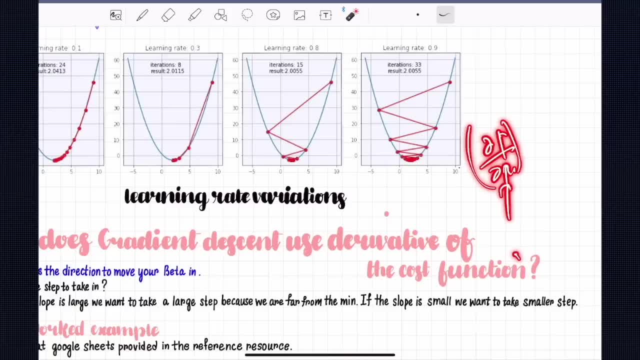 derivative which you've taken, whatever the derivative which you which which you have taken, if this is positive, which means that if you increase the value of beta, so basically, derivative, what does it gives? it gives the direction to move, to increase or decrease the theta. that's, that's. 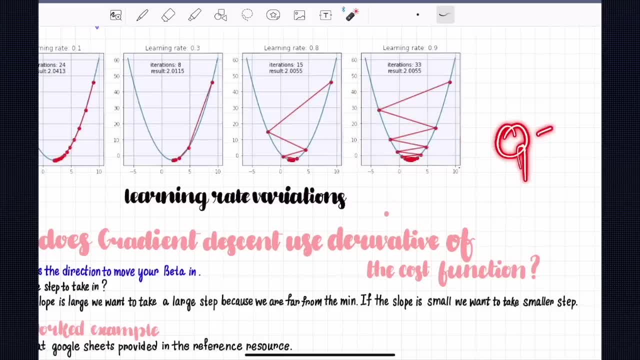 what it gives right. so if we increase, if, if the derivative is positive, the derivative is positive. so if we that, that means that if we increase the value, if we increase the value of beta, our error will also increase. so we'll have if the so. so this tells: if increased. 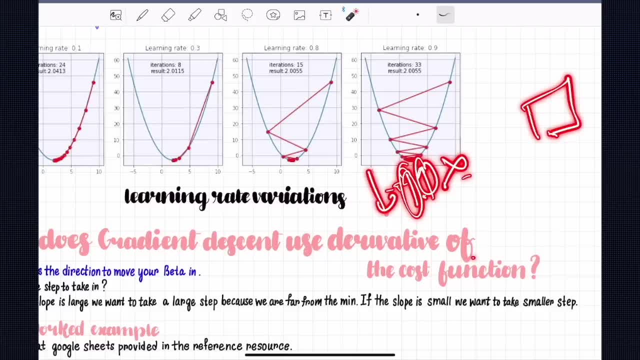 the value of beta, our error will also increase. so so in, so over here we decrease it, okay, but if your derivative is negative, if your derivative is negative, which means that if you increase the value of a coefficient, if increase beta by some factor, by increase beta and increase beta from, 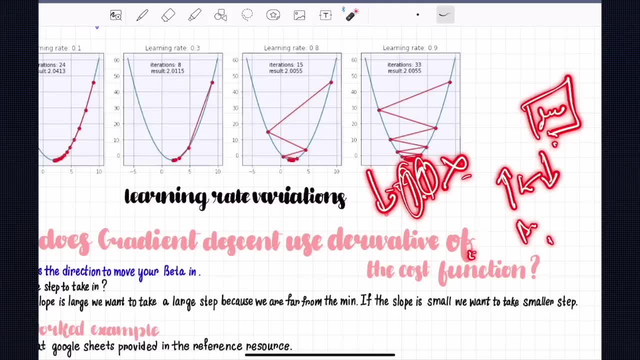 the previous one. it will decrease the error. it will decrease the error, right? so over here we just go with this change, okay? so basically, this derivative gives us the direction to move your beta in. if, if the derivative is positive, that means if we increase the beta, our error will. 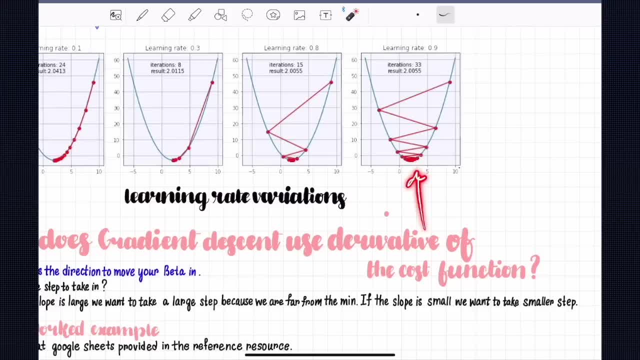 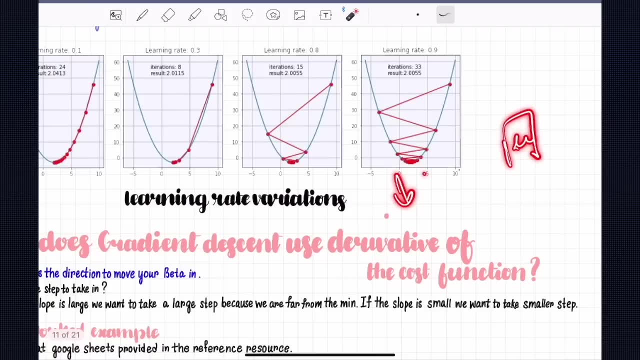 also increase. but if the derivative is negative, if it means if we increase the beta, then the derivative will decrease- okay, i hope so. if the derivative is positive, then we decrease the beta so that our error also decreases. okay, i hope that that gives this gives you a good sense. 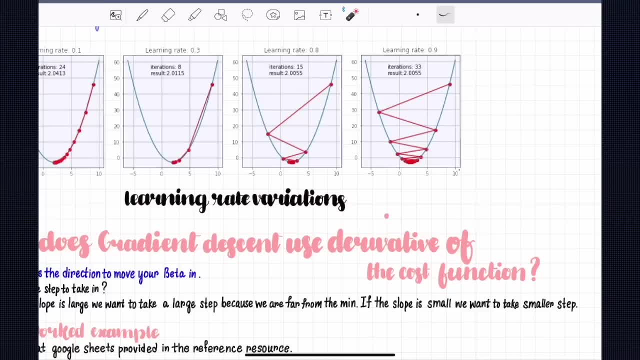 so by computing the derivative of these of this mse with respect to every individual parameter, we can determine the direction in which each coefficient should be changed, like to increase degrees in order to minimize our error. okay, i hope so that you got it. and now our gradient descent. 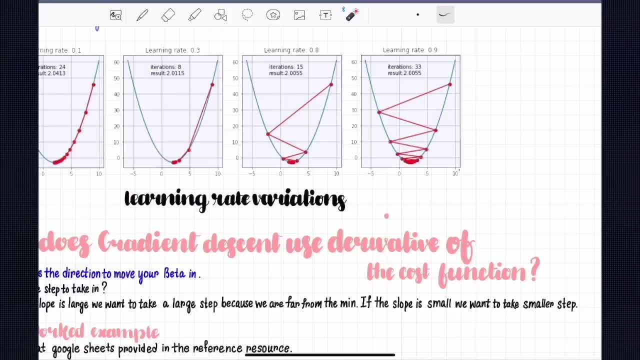 uses this derivative. our gradient uses this derivative of the of the mean squared error to update the parameters in the direction in the direction to update the parameters in the direction it minimizes. so this degree. we'll use the gradient descent to in the direction that it minimizes the 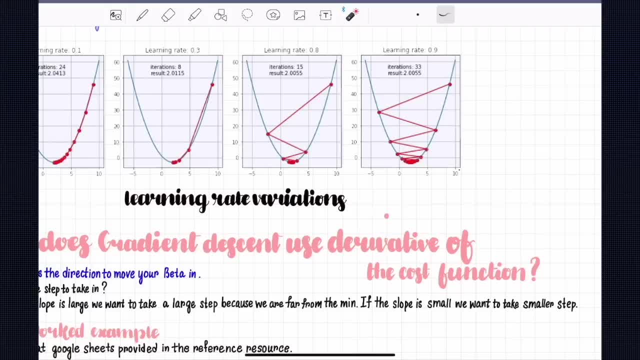 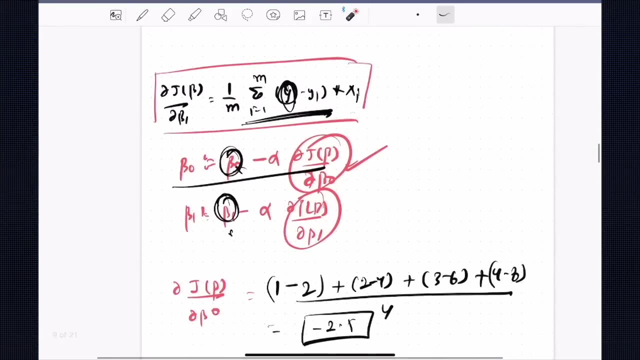 particular error. so at every iteration to, at every iteration, the, the, the gradient of m, the, the gradient of mean squared error is computed and the coefficients are updated in the opposite direction of the gradient. as we have already seen how exactly gradient descent works, and, and and it. 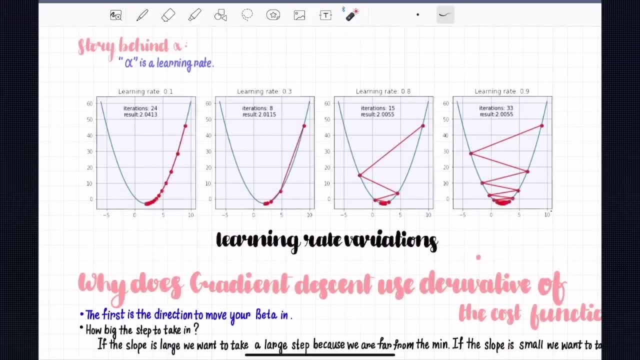 keeps on, it keeps on, you know, changing the direction, increasing or decreasing keeps happening. you opposite of the gradient, of opposite of the gradient, and keeps on the come, come, coming up until unless we converge to the global minimum. so basically, the whole idea behind: first, it is the rate of change. 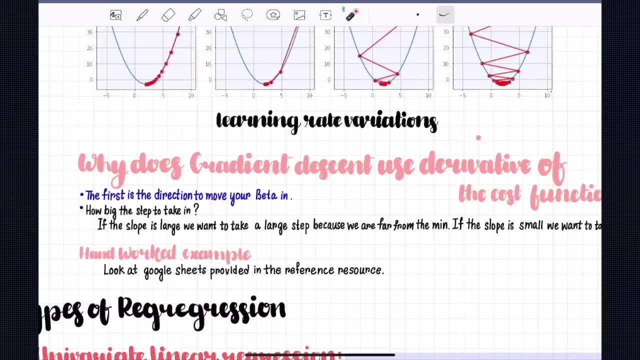 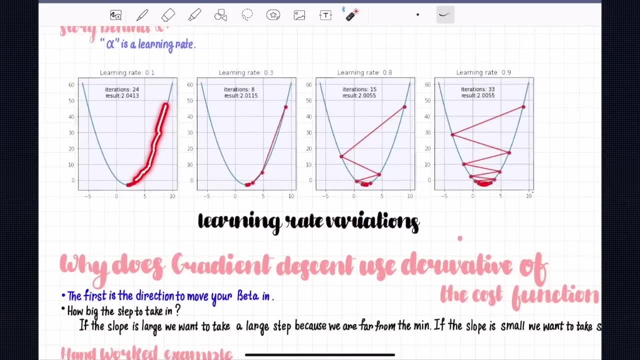 derivative is the rate of change. second, it tells you the direction. and second, like, how big the step is. in this case, if you see that it has to, it's starting in the big big step, but eventually the start is small right. so if your slope is large, if your slope is large, we want to take a large step. 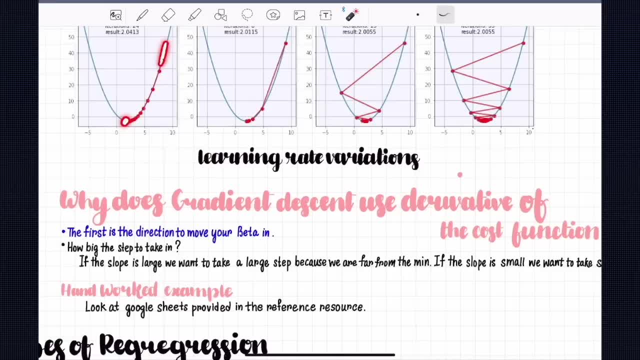 because we are far from the minimum. we want to take a large step because we are far from the minimum. we are far, so this over here slope is large right, so over here it is far from the minimum. so so we take the big step. but as we go towards the minimum, our slope becomes small and that's why we have to. 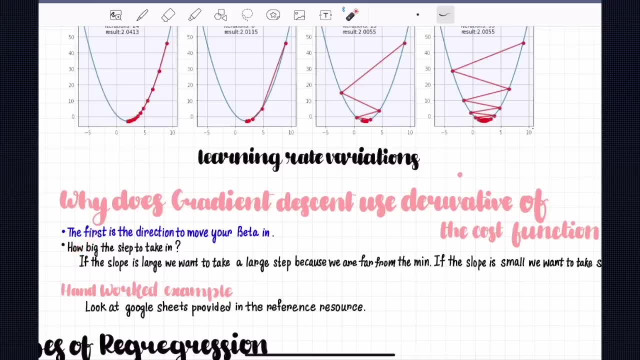 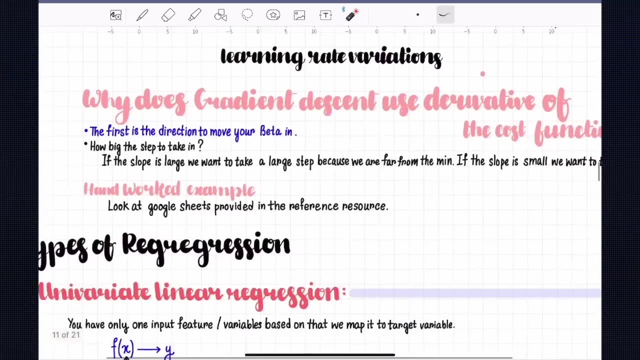 take a little little step. so the your debt derivative tells that how big this step we should take. i hope that this gives you a very clear sense about what exactly our debt derivative means, and i hope that this gives a good sense about why do we use trade where- if for the cost function cool. 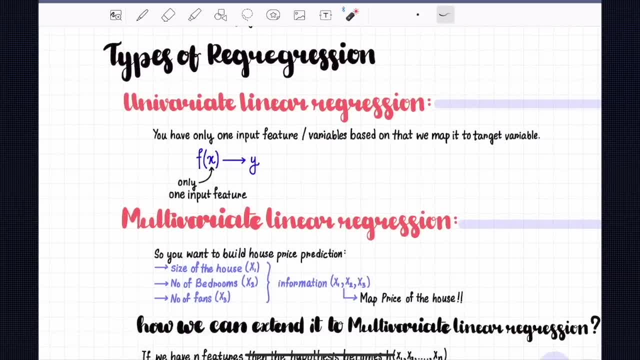 when we choose, do you use as non chi if not an all chi, because at the end you see that this people are acting like animated. it actually means that we actually use a bearing in our system quite a bit, because the size of this thing is going to form up like I wanted it to, and if it doesn't, 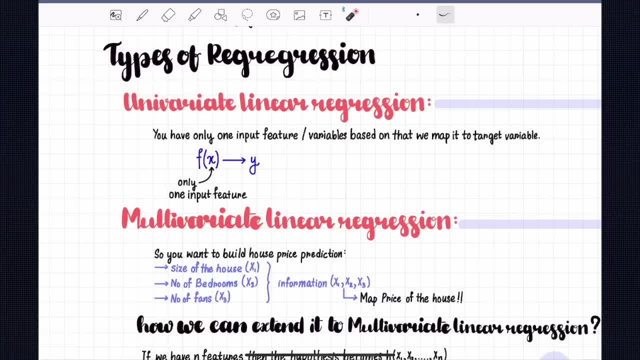 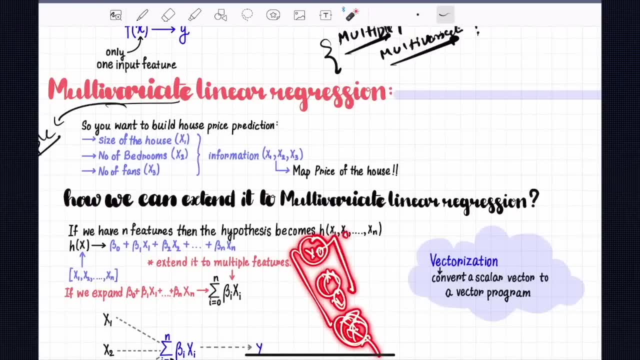 found. when I say something, it should explain itself. one more time term. I said: this is how our chain here- well, where, even though we have to take this part, essentially meaning the the quickly loop- is very plano going to become, because the way I possible is going to become. 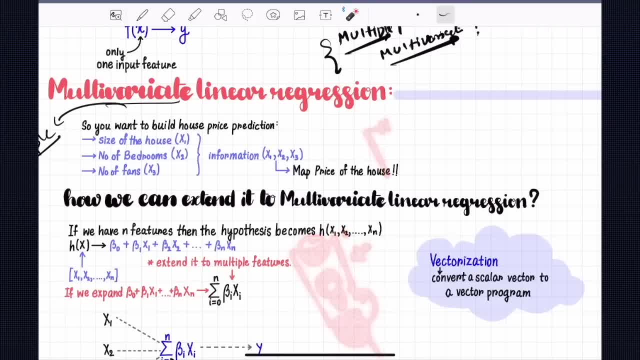 and then, and, and then you have a x1, x1, x0, x1 and x2, and then you make a, and then you make a parameter vector, and then you make a parameter vector, and then you make a parameter vector beta 0, beta 1 and beta 2, and then you take the dot. 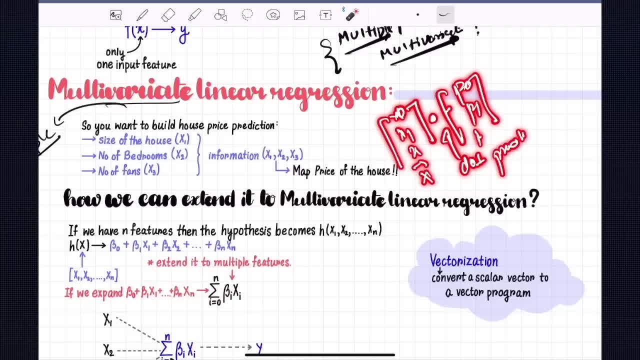 product between both of them, dot product between both of them, dot product between both of them. so when you take the dot product between both of them, what is it? does X 0 beta 0 plus X 1 beta 1, X 2 beta, beta 2? so we studied the linear. 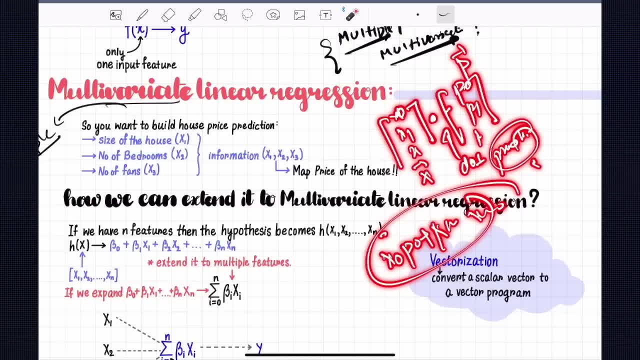 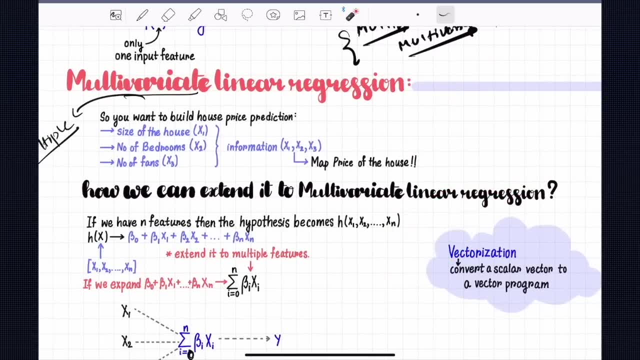 algebra. this read heavily reduces the computational time because it follows something as a broadcasting, where it simply multiplies and adds at the same time, and the calculation, the dot product which will perform the way of taking the vector X X 0, X 1, X 2, and then beta 0, beta 1, beta 2, they take the dot. 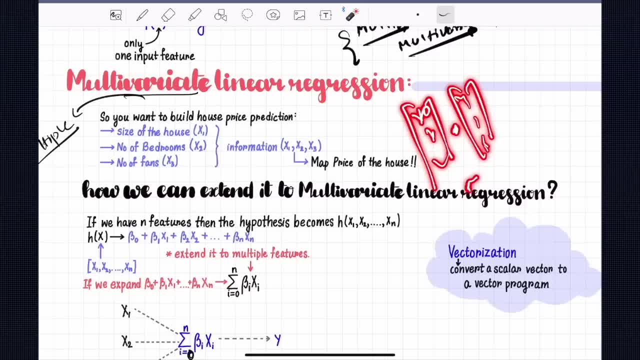 product. it will be super duper efficient. so we have several frameworks to do this, which is now X 0, X 1, X 2, and then beta 0, beta 1, beta 2. they take the dot product. it will be super duper efficient. so we have several frameworks to do this, which is now: 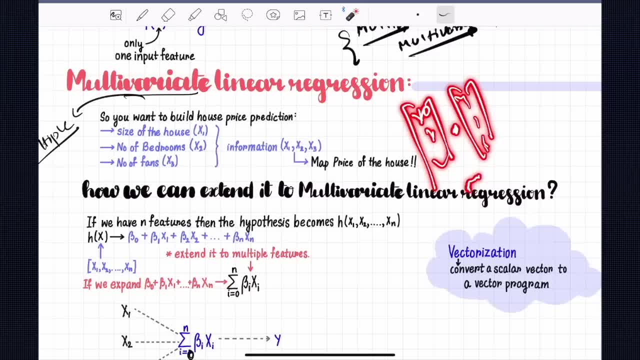 pi framework, you know tensorflow, which provides the optimized versions for the vectorized option, this called the vectorize operations. that's why linear algebra comes into place. okay, now, how can we write the dot product? so, if you have the beta, if you have the beta, which is the parameter vector which contains 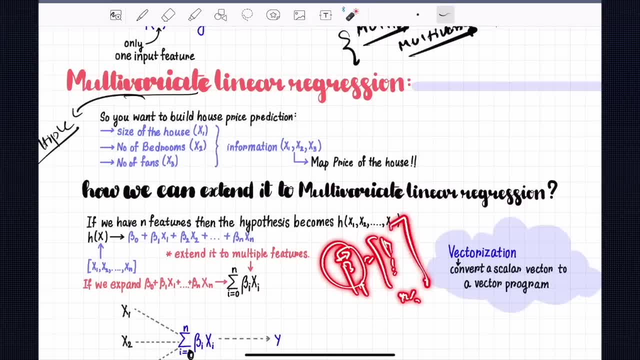 the beta 0, beta 1, all the way on to the beta, and number of a beta, the number of it has nothing but because of number of features which you have. and X, X, X vector contains your X 1 all the way on to the X 0, all the way on to the X n. then you take the dot product. 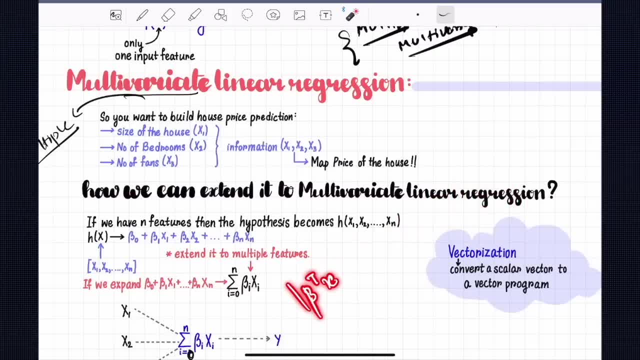 product by beta, transpose x. this is, this is how you can write. or you can say: beta, dot x. okay, you can write in this way. so you basically take the dot product, but but we'll come to dot product. we'll come to dot product later on when we solve a real world example, but as of now, this is how it. 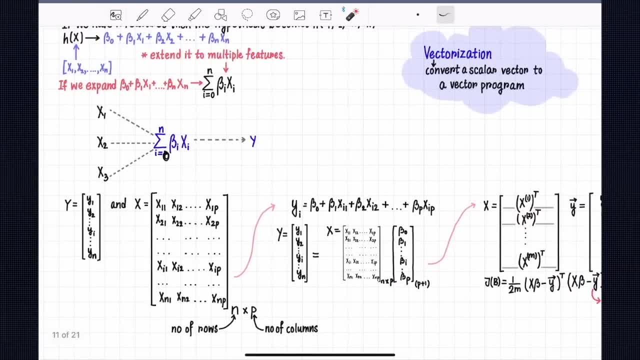 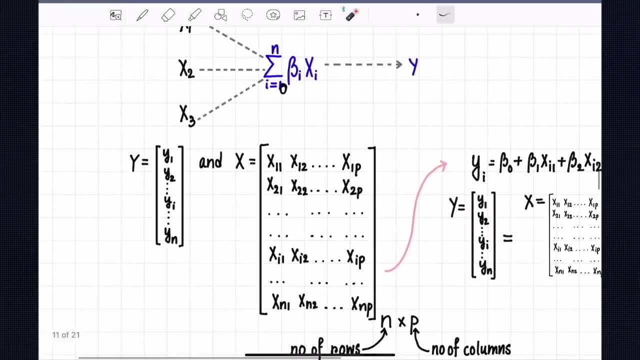 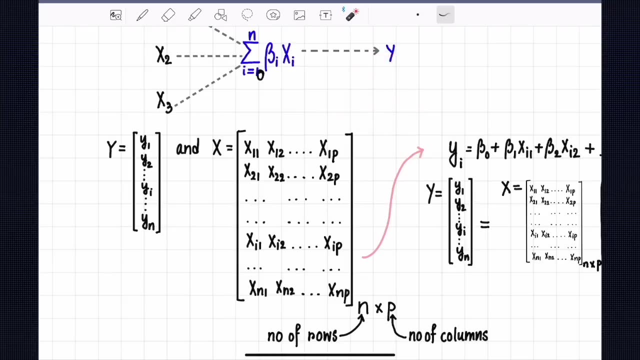 works. now let's get started with more detailing thing. okay, first is: let's prepare our design matrix. let's prepare our design matrix. so this is: let's prepare design. design matrix is nothing but your data. how can you convert your data into a matrix, a csv data into a matrix? so in this case, 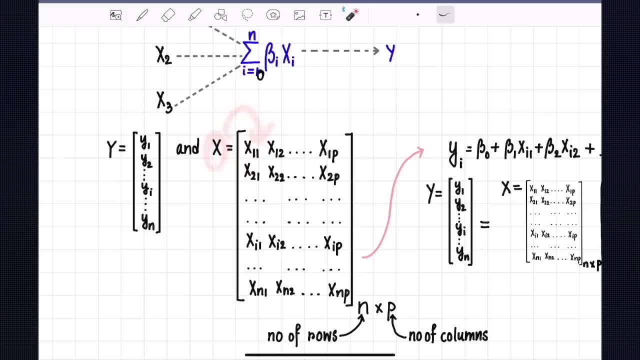 in this case you have your design matrix x, okay, x contains your data, okay, so assume that you have x1, x2, x3, all the other number of features. so x1 size of the house, the number of bedrooms of the house, the number of so it can have n number of p, number of information. so here we have written p. 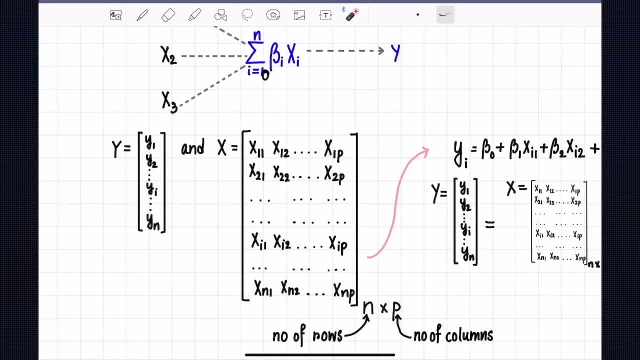 in the instead of n, so we have p, number of information. okay, and the and the first data point can be represented as. if you have seen the matrix lecture, you could have understood this very easily. so the first data point in your, the first data point in in your data, is x11, which represents 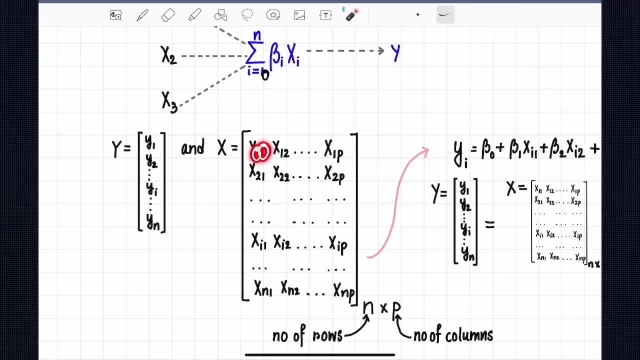 that it is the first row and first column, which means is it's the first, it is the first, it is the it. it is available in the first row. which of the first information, for example, if there's the size of the house, this is the first. okay, now this is the second row. first information: this is the second. 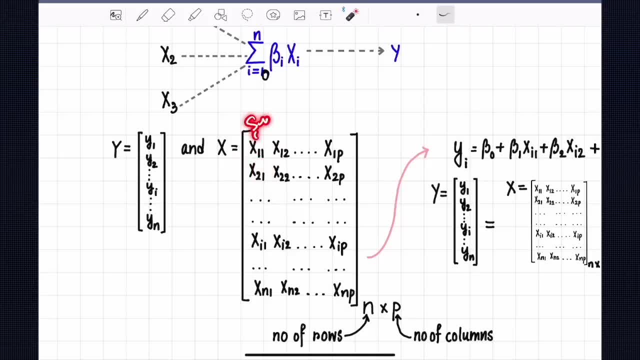 row of the first information, which is assume that this is the size of the house. the first information of the size of the house. second information of the size of the house. so you have same information but different, different samples. then you have price of the, then you have number. 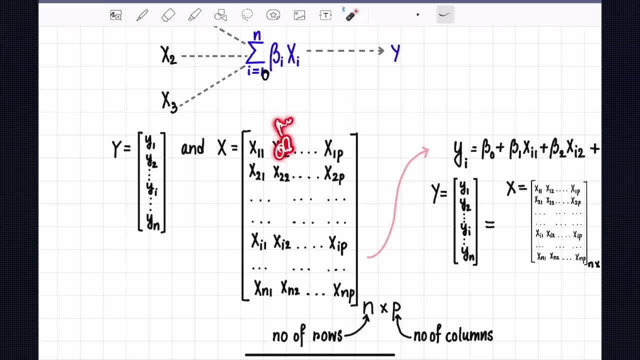 of bedrooms. so first, information of the second, second feature, which is the number of bedrooms. second, information about the bedroom. so you have several samples for the same right. so you have on over here. you have different, different features or as a number of columns, and then on the number, 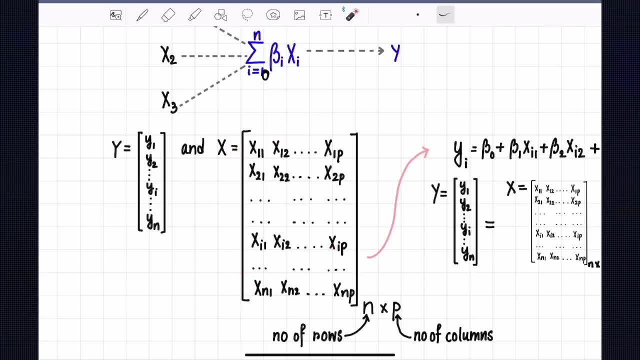 of rows has an n number of a number of rows. okay, first data point: first column, first row. first column second: first row. second, column support, first row, third column, all there are. the first row, p, column, okay, and then at last you have a and the nth row, first column, and a throw second. 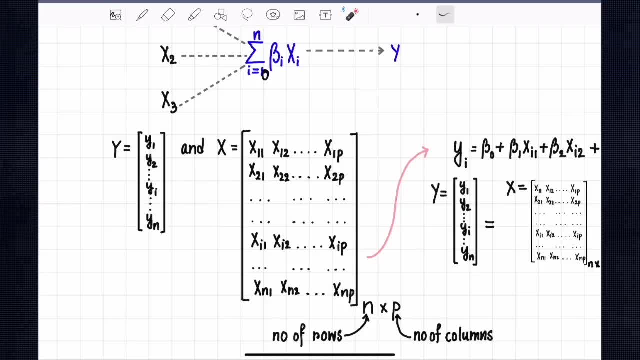 column and a throw p-th column, okay, so it says that it can have p number for columns or n number 4 and N number of rows, okay, so this is no, nothing known as design matrix. this is nothing known as design matrix, okay. and then you have this y and y. then the, the y, y n will be equals to x, n, okay, so the number of 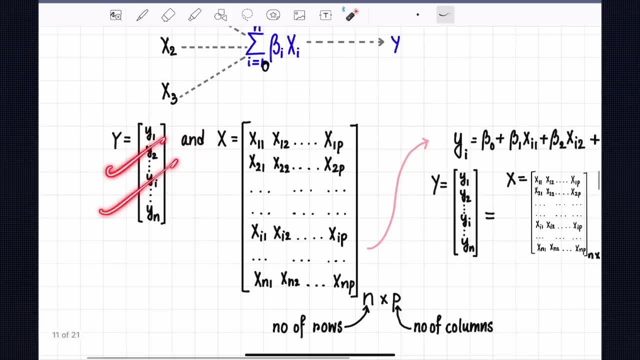 rows. the number of elements which you have in your parameter y vector is equals to the number of rows which you have in a design measure, because it is a super supervised learning problem and every individual row has its y 1, y 2, all the way around to the y n, every has its own label, so it 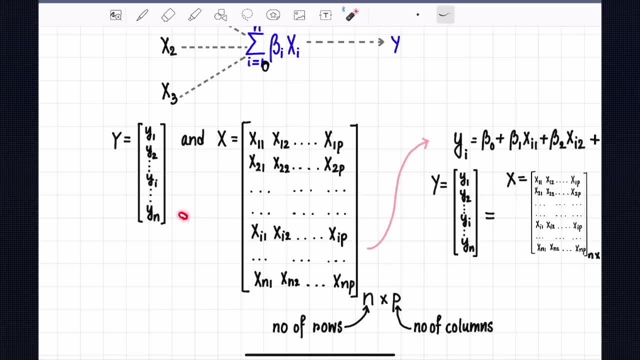 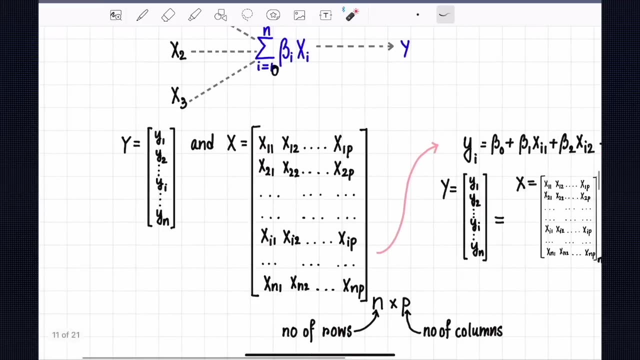 it. it may be small, it not be smaller than it. x n is equals to y and the number of elements in y n should be equals to number four data points in x n. okay, cool, now what we can actually take out. we can actually take out our y hat i, y hat i, which is the predict prediction. so now you might. 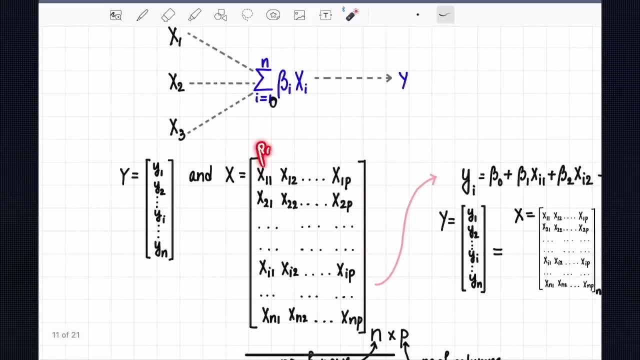 be thinking that, okay, every individual parameter has beta 0, beta 1, all the way around to the beta p. okay, p number of four. now should we? are we going to multiply beta 1 with all the variables over here? beta b, beta b, beta is the two with all the variables. and how exactly the hypothesis function, how exactly is will, will? 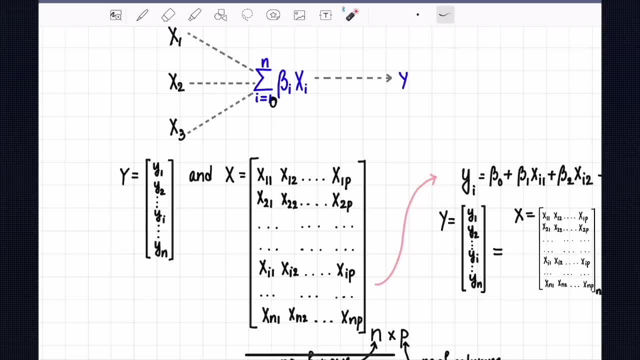 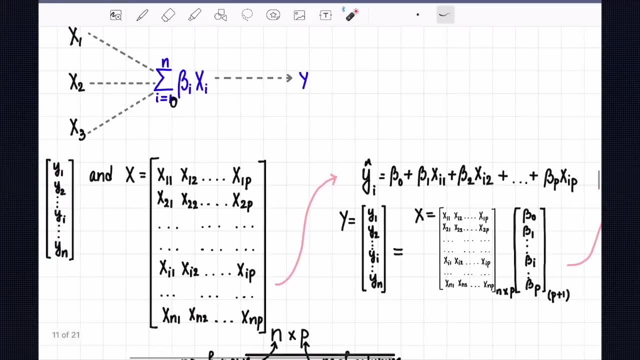 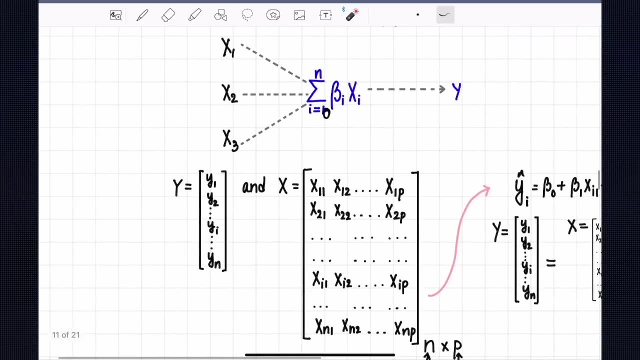 this work a very, very interesting question. so your prediction, your prediction: y hat i, y hat i, which is your prediction? first of all, you have beta 0, beta 0 by default comes in beta 0 times x 0. so basically, sometimes you know what we do. we actually have. 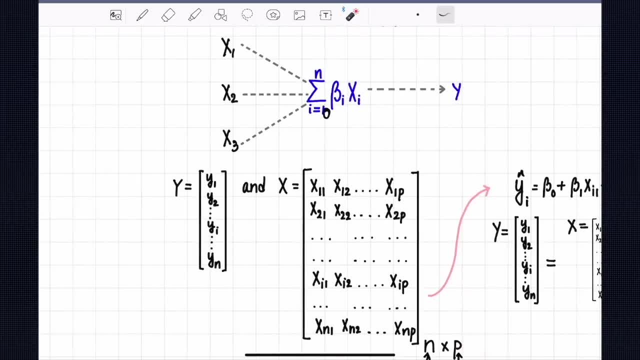 n times x 0, so we actually have n times x 0. so we actually have n times x 0. so we actually have n times p plus 1, n times p plus 1. in this case, we add another column of 1, 1, 1, 1, 1, 1. we'll talk about. 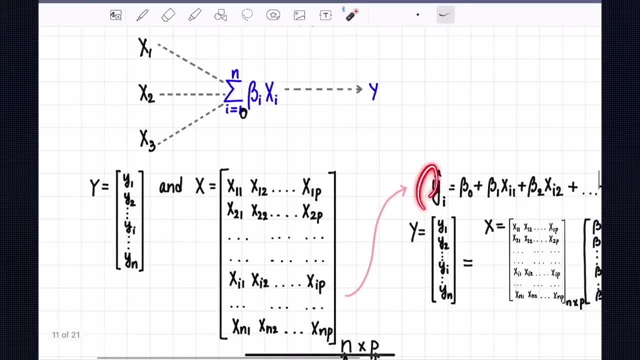 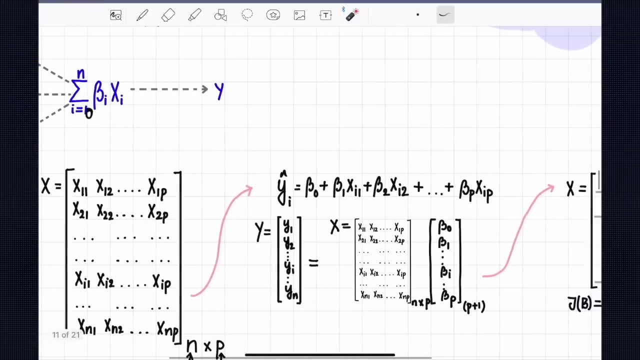 that? why do we add 1? okay, so you're you. you get a predict. you, you actually have this prediction: y hat i, which is beta 0 plus beta 1, x i 1, beta 2 x i, 2 plus beta all the way around: beta p x ip. what does? 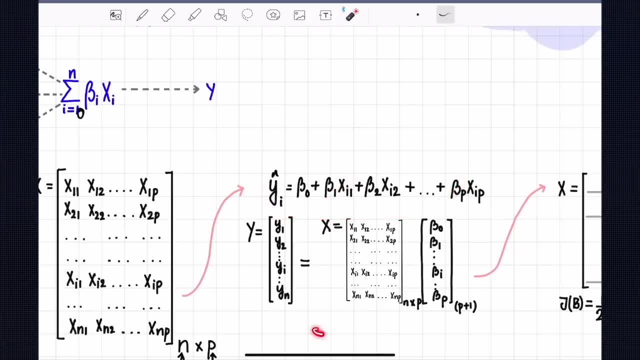 this mean? this, will you? you'll only be able to understand if you understand this thing. okay, so you can get your prediction. you can get your prediction, which is y hat i, which is y hat i. you can get your prediction. you can get your prediction you. you can get your prediction from your model by. 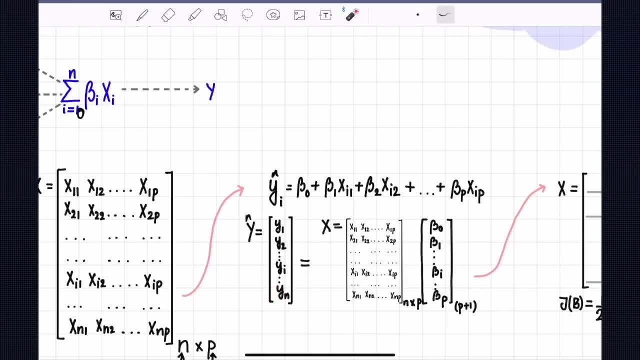 for example, we eventually have to make you, you have to make a prediction for calculating how well your equation is right. so you actually have a parameter vector which is beta 0, beta 1, all the way around, beta p, which is the which is of size of p plus 1, p plus 1, because there's a p number of. 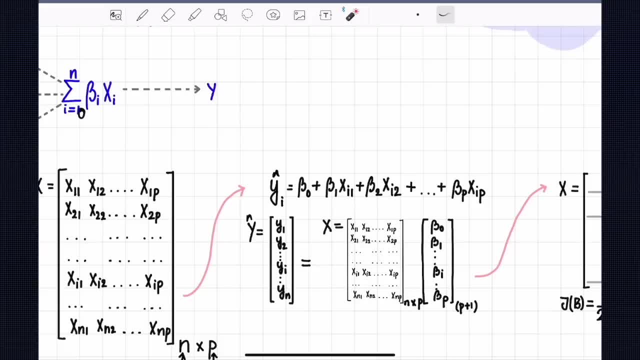 features plus 1, which is beta 0. okay, so you multiply it. so basically, in this case we also have 1 over here. so i'm just going to add to make sure 1, 1, 1 all the way around to be 1, so only 1. 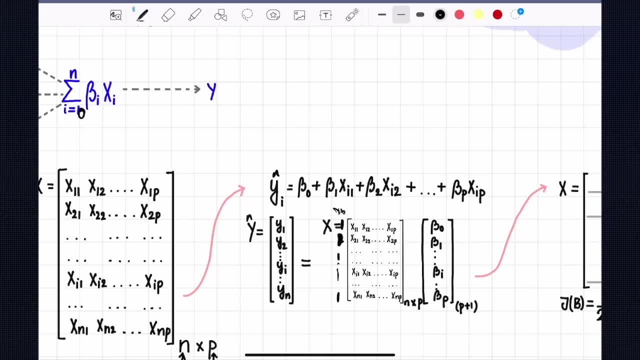 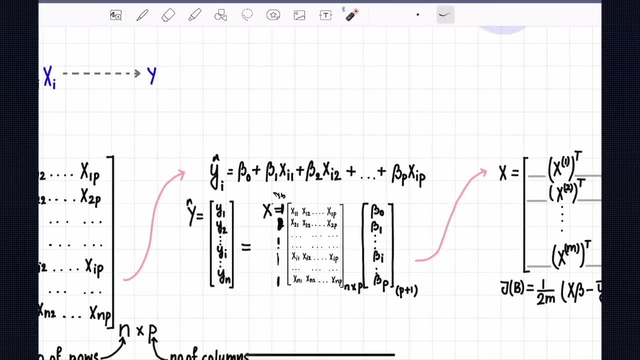 so this: this indicates x 0. okay, so that beta 0 gets multiplied with this, we'll talk. we'll talk about that, uh, in a bit. so you have this particular and now, when you multiply this matrix with a vector, it should lead you to a vector of your predictions. so every individual sample will have 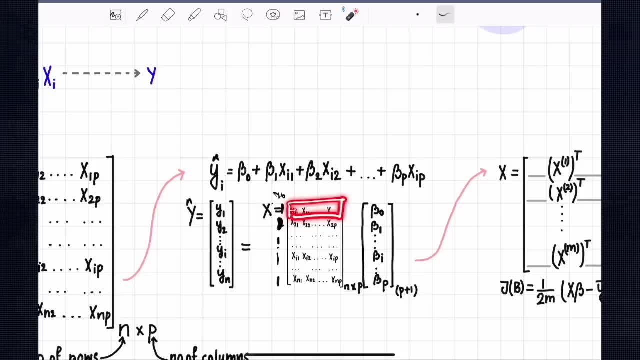 it because up, because a row is a data point, second row is another data point. so basically it's a column columnar difference. you know what i'm speaking about is assume that, assume that you know, make you you have a data like this. you have a data like this. 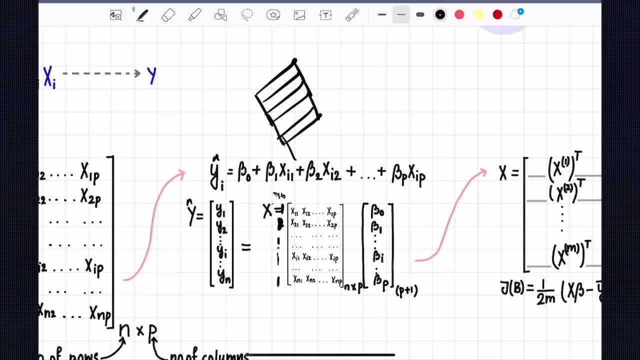 have data like this, okay, data like this, and data is mostly, you know, like this, so you have. so this particular point has this label y and now you have to make the prediction for this y hat i, so that you can compare the both and then the take out the differences. so take out the y hat for this. 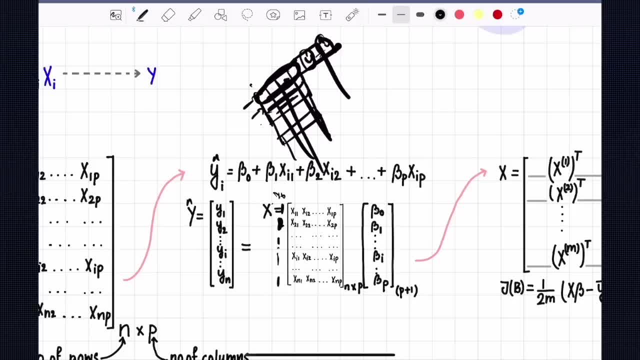 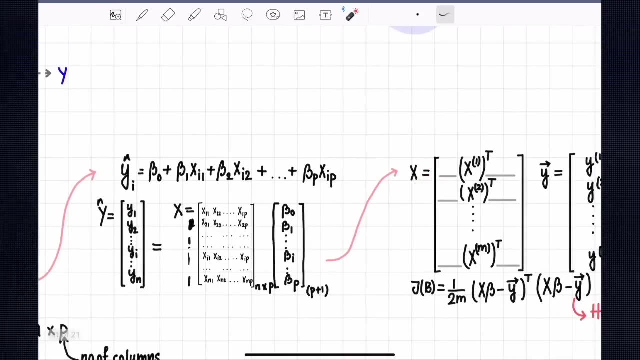 particular data points for this part, because every row is a data point. every row is a data point. okay, what is it that that will eventually help us in taking our learning from our data? okay, hope so that it makes clear. we'll talk about this, uh, this, in a bit, but before that, what i exactly want to. 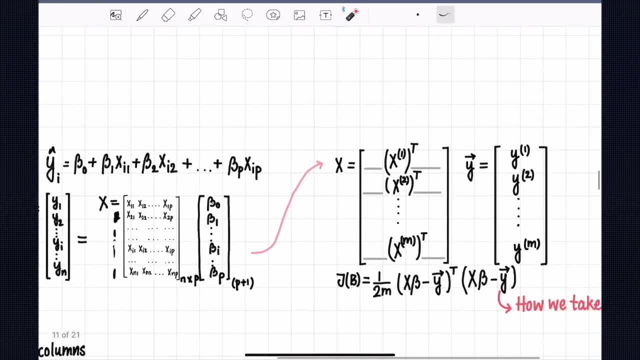 convey to you all is: you can actually convert this. you can take this x1, you can take this x1, you can take this x1, which is all the this, this column, into into a, a row vector. you can actually convert this to x1 transpose, which means: 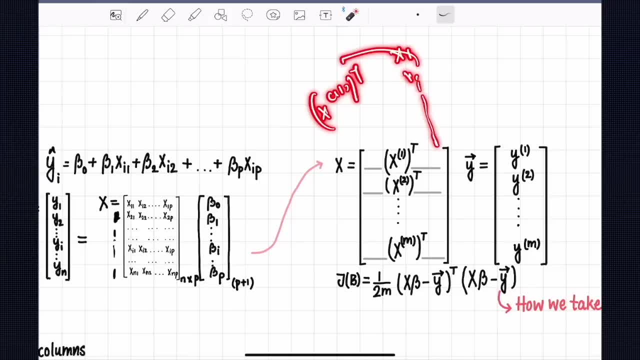 eventually x, x1 or s, like, like. like this you can convert like this and then you have x2, transpose x and transpose. you take this and convert this into a row vector. take this: converts into a row vector. this, this, this has its own benefits. we'll talk about that- and your cost should become like this: 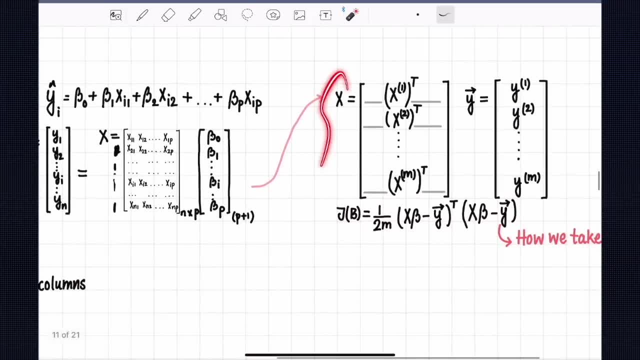 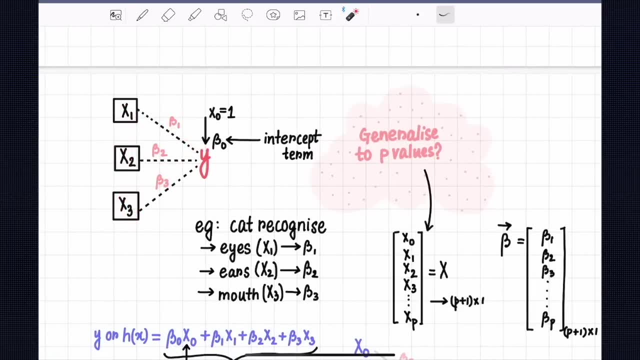 we'll talk about this, all of this in detail. just we'll, we'll, we'll come. come to this. please ignore as of now. cool, so you have x1, x2, x3, x3, all the way it's it. it has some feature. we have x0. 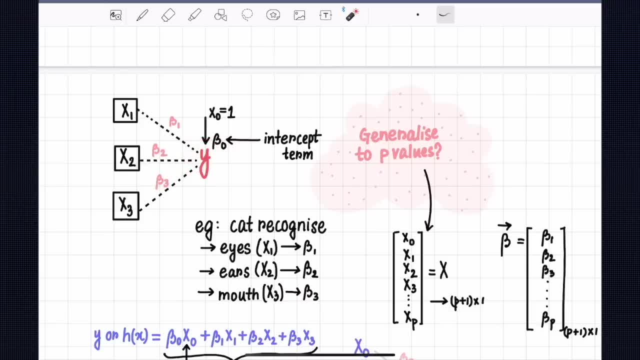 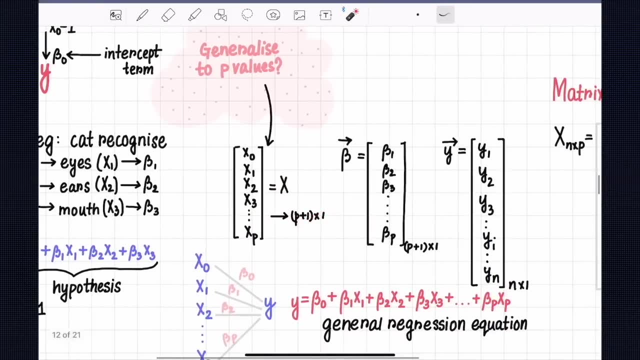 which is beta 0, and then you get a prediction y using our thing. okay, categorize, as i've already talked about this, your p number of samples- they're generalized to p samples- and the parameter vector p, and we have y, vector y, which is the ground truth. okay, you have a matrix distribution, which is: 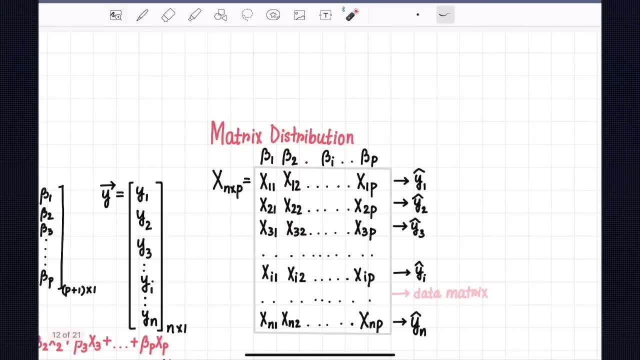 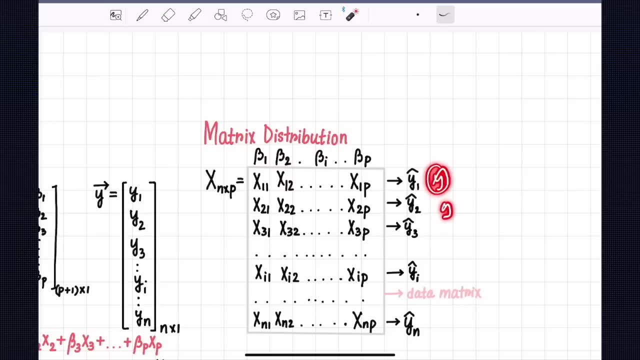 nothing, which is also the data matrix and the design matrix now based on this, now based on every individual data point will have its own prediction. uh, will have its own prediction, and then we compare with the ground truth, the actual prediction, and then take out the error. and then take out the error. okay, so every data, date, data point has its 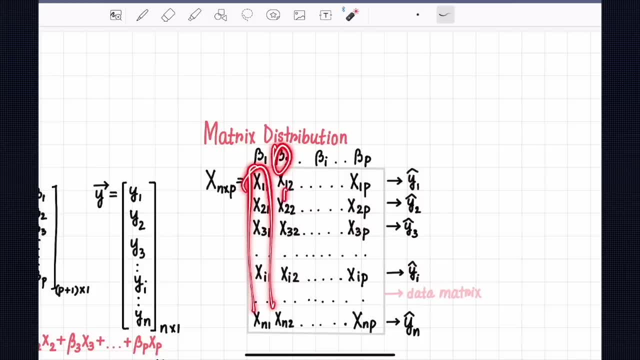 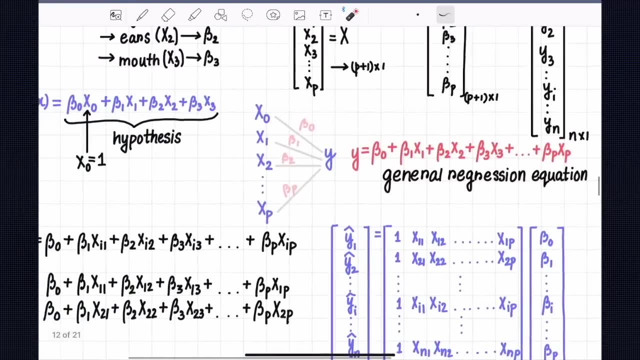 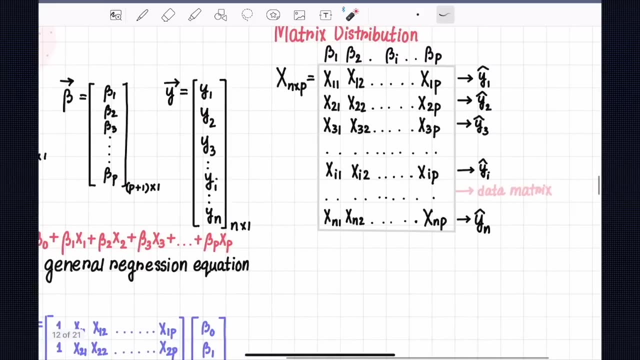 own prediction and then, and every column has its own b2, which is the uh beta values. okay, understood, in this case, you're seeing that exodus might be going to be aggregating of the information. now let's get started. let's get started in: how can we actually, how can we actually take out the y hat? 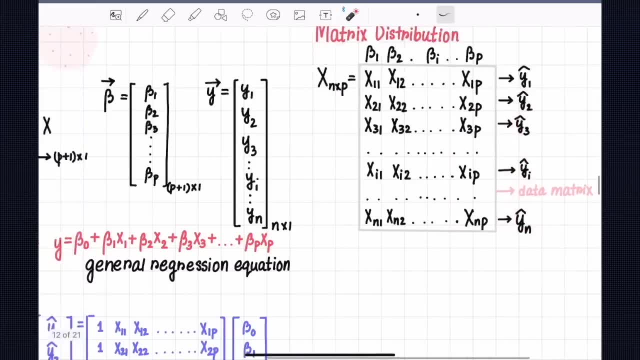 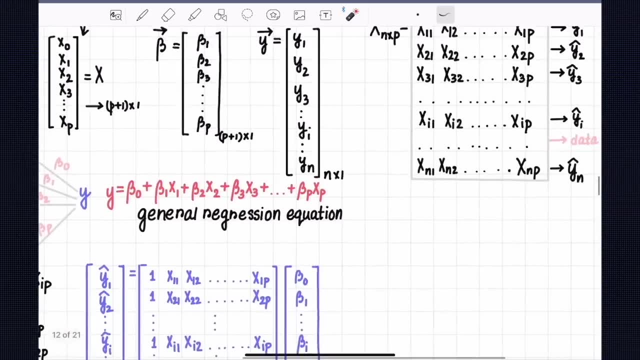 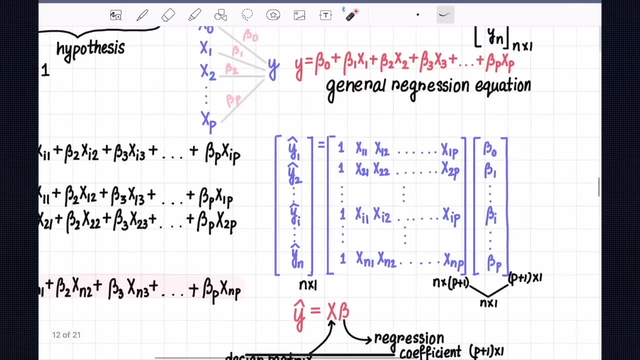 two, y hat. three, y hat i- all the way around the number of features which we have. let's exactly work on that. so y hat one which is equals to beta zero, which is equals to beta zero, which is, uh, equals to beta zero. so where i am going to write it up, i don't know. yeah, in this case, see this: 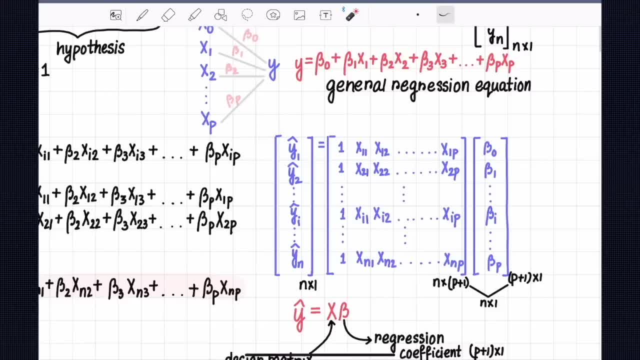 example: uh, now over here, i think i did, i written. now you want to make, now you know, now you want to get a uh predict prediction. you know a prediction vector, and then you have your y, uh, and and and then you have a ground truth over here. but your prediction vector, and first of all you have this: 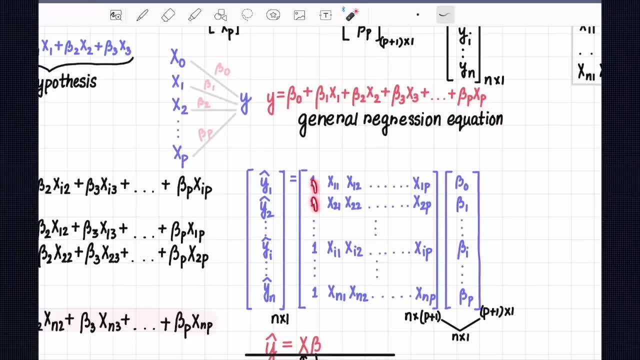 one, you, you, you made a, uh, a column where you have one, one filter, okay, y, you will notice. and then your parameter, vector b: okay, when you multiply this matrix, this is: this should be equals to, this should be equals to: so, when you multiply this matrix with the multiply with this matrix, to 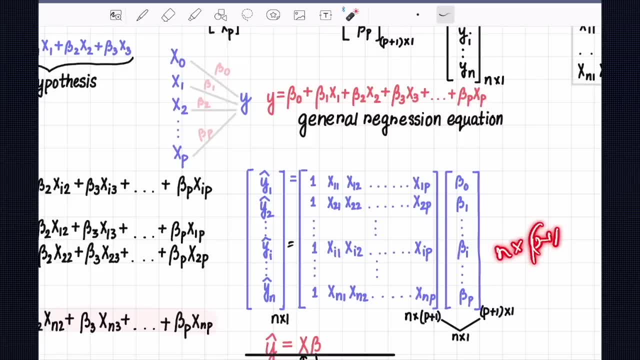 the product. the matrix is n times p plus one, y p, number of columns, plus one column which we added right right now. times you have p plus one times one is p, number of columns, which is one, and when there is only one column, so when you, when you actually 300, take out the 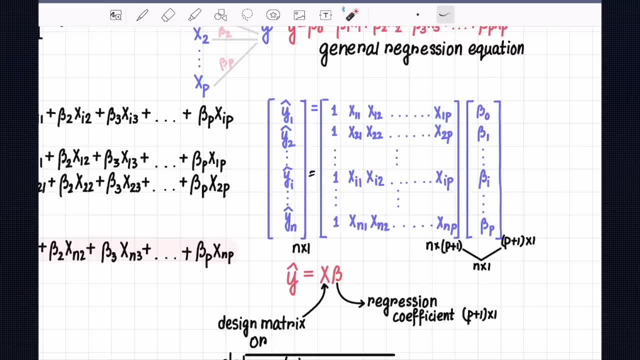 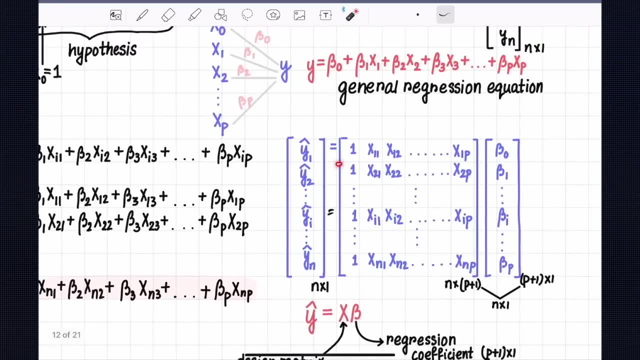 take, take out the multiplication between both of them, the dot product between both of them, multi multiplication vector product. okay, in this case, what we'll do? you have beta zero. as i said that every individual point has its own prediction. okay, it should not be like this. it should be like: 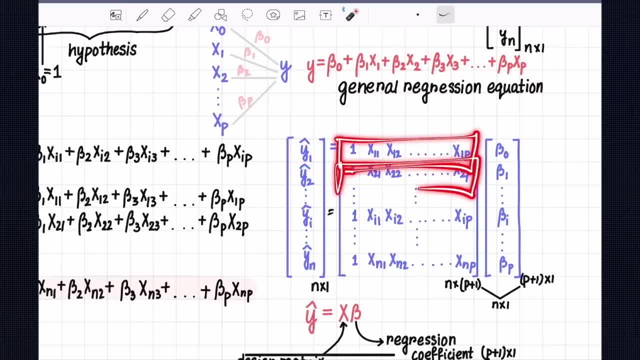 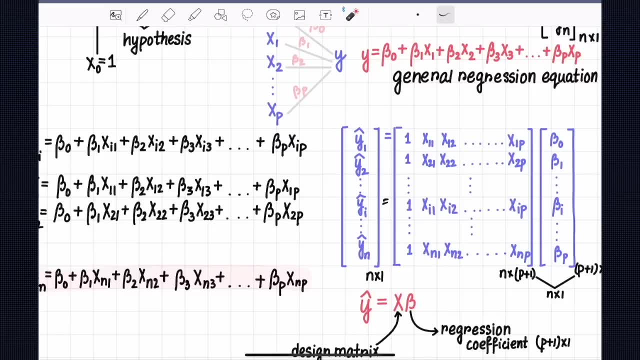 this everyday data point is: is is a row, okay. so beta 0 times 1, beta 1 times x, 1 1. beta 2 times x, all the way out of the beta p times x 1 p. so basically, you take the first row, you take the. 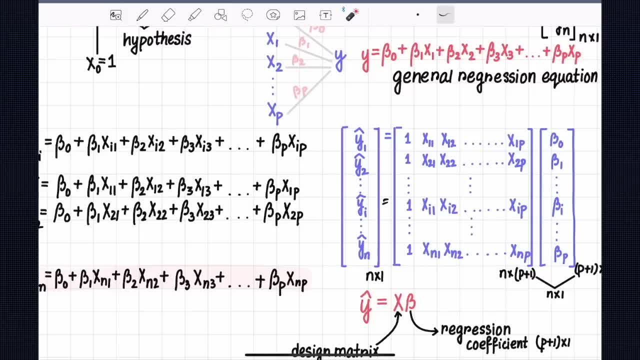 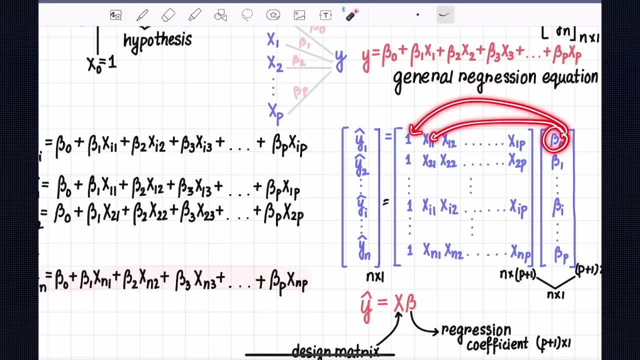 first row of the vector. multi. take the, take the dot product between the first row of the design matrix or data matrix with the first element of the vector. understood what i'm trying to say? you take the beta 0 and up and multiply with every element of the first uh row of the, every element. 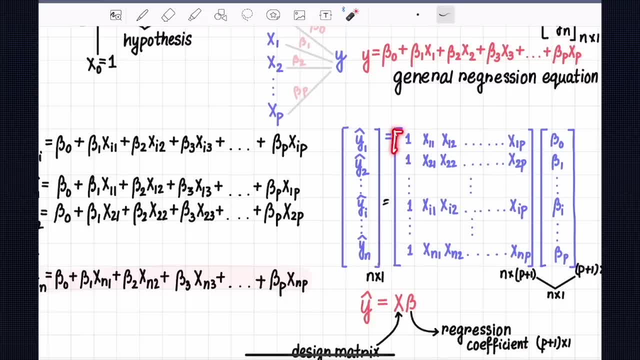 i think i just messed it up. i think i just made up. you take the first row of the. i just, i'm sorry, let's you take the first row of the design matrix and then you take the vector. so basically, you have your call, you, you have your row vector, you multiply with the, you, you, you multiply with. 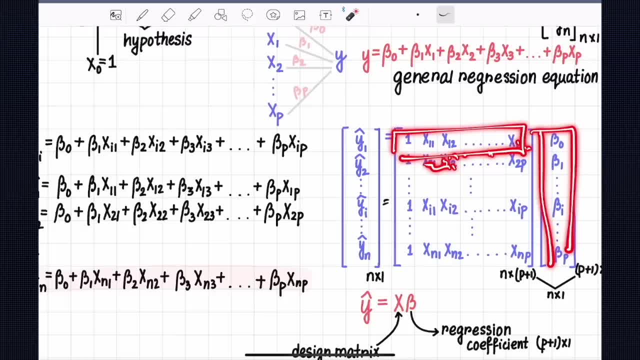 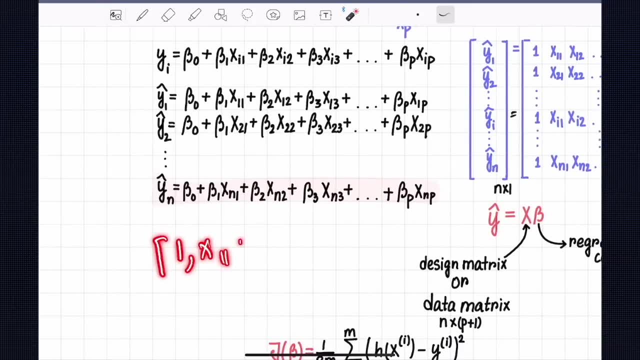 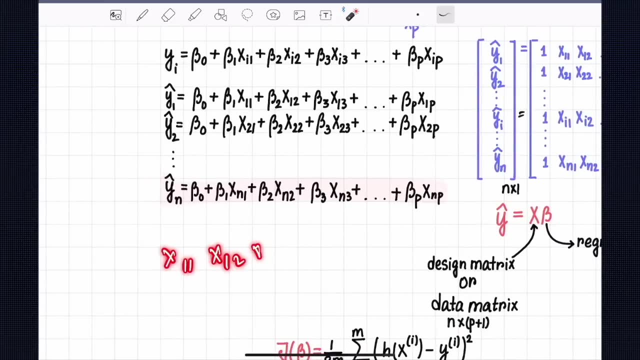 the column vector. so take the dot product between the row vector and the column vector, row vector and the column vector, which is nothing. you'll come up with 1, one, one x, one, two, all. there are the this x, one p. so x one, one x, one, two, all x, one p, all around. 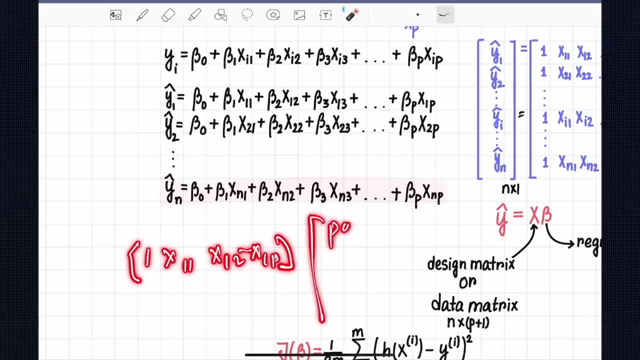 x, and there is one. so take this and then you have a column vector which is beta zero, beta one, beta one, all the other. take the dot product between both of them, so dot product will yield to something like this: so beta zero, this beta zero, multiplied with this one, beta one, multiplied this, then plus. 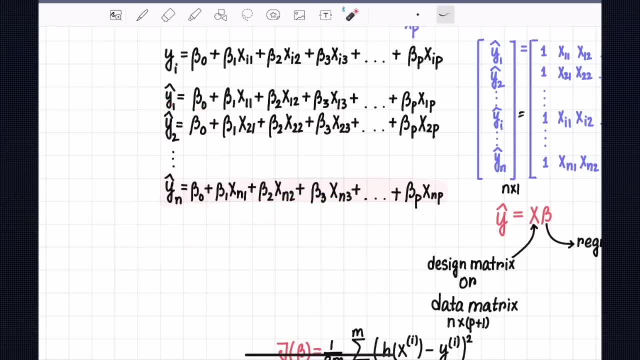 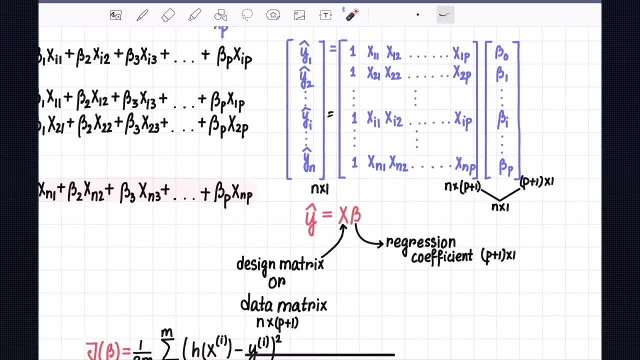 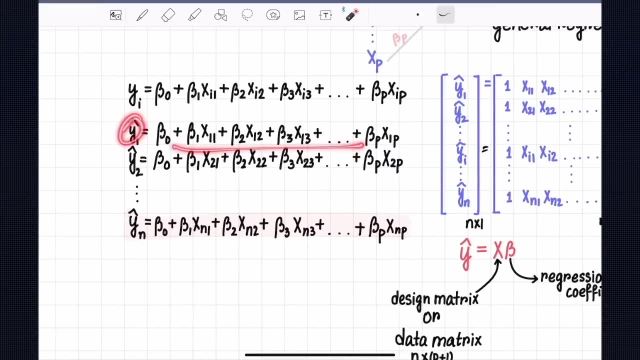 of course, beta, beta three, beta three, multiplied with the third information, beta four multiplied with the fourth information. fourth, fourth information, the fourth information, a particular data point in that fourth information. okay, i in that, i in ith index, and then you have got your prediction. you just take out this and then go to your prediction. now you go to y2, which is the. 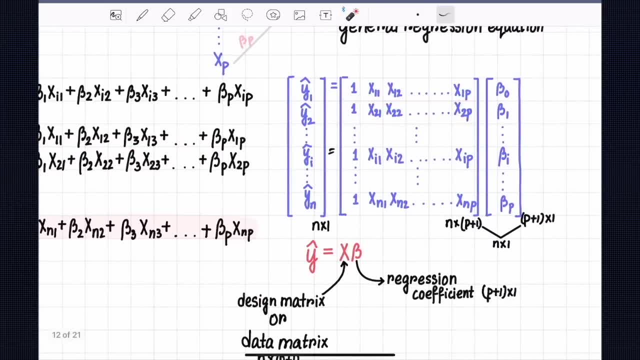 which is the prediction for this second row. okay, for this second row. so basically, you do the set, you take the second row, you take the second row, and then you take the uh, and then you take this vector, do the dot product between both of them. it is beta, zero times. one beta, one times. this is the. 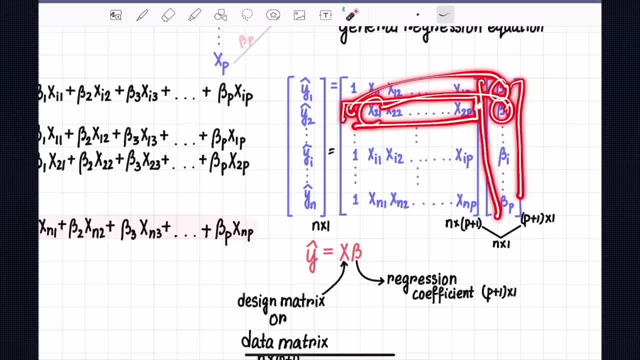 same information. this is the same information. it is. the x21 is. it is saying that it is the 2nd data point of the first table of the same. this: if the size of the house is the second data point, okay. second of the point of the first information. so beta 1 times x, 21, beta 2 times x 22, beta 3 times x23. so you, 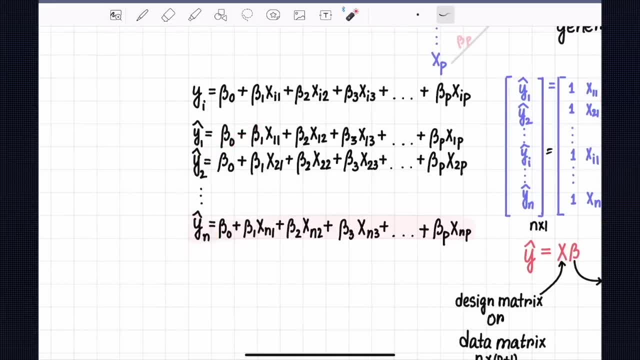 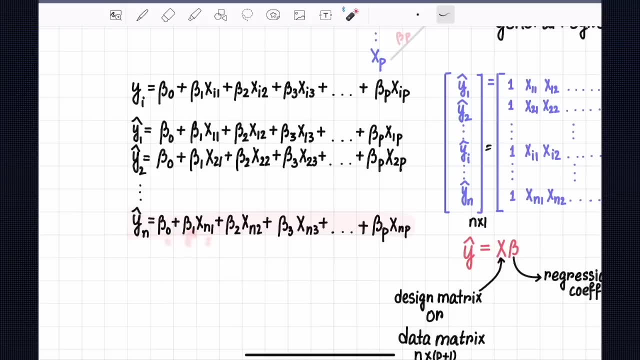 have this by 2 all the way around the ym, all the var 1961, which is a y uh n number of a predictions. it's beta 0 times beta 1, x n 1, which is the nth data point for the first info. nth data. 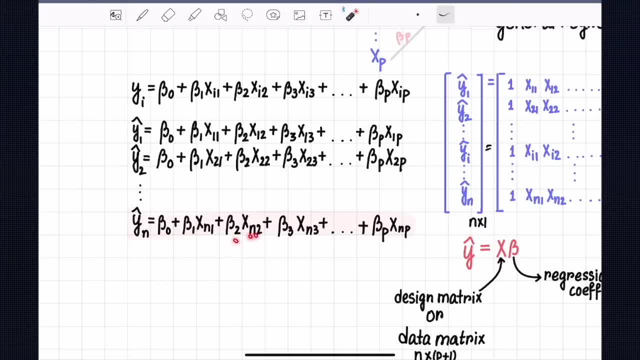 one for the first information, the beta 2 times x2, xn2, which is nth information for the second. sorry nth data point for the second information, nth data point for the third information and nth data point for the pth information. okay, And in between you have yi, which means that you have beta 0 times, of course. 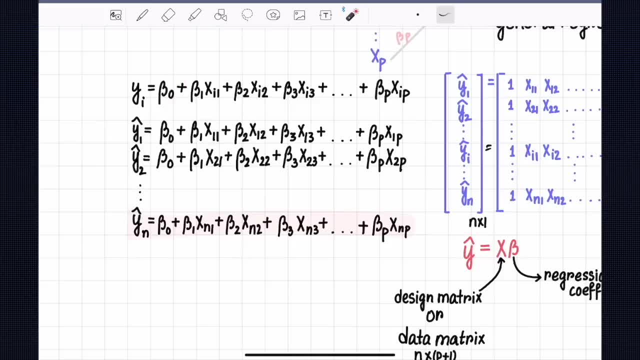 1, times, of course, 1, because everything is 1 in that first case, beta 1 times xi1,. i-th data point for the first information. i-th data point for the second information. i-th data point for. 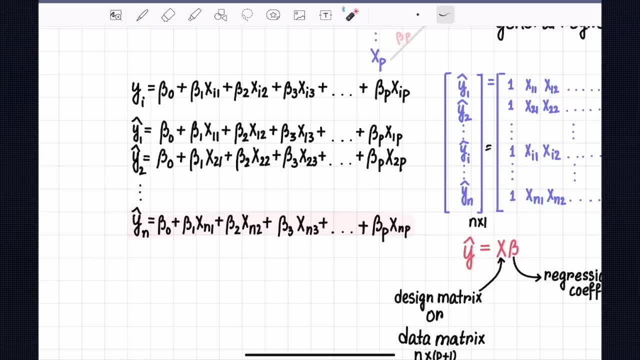 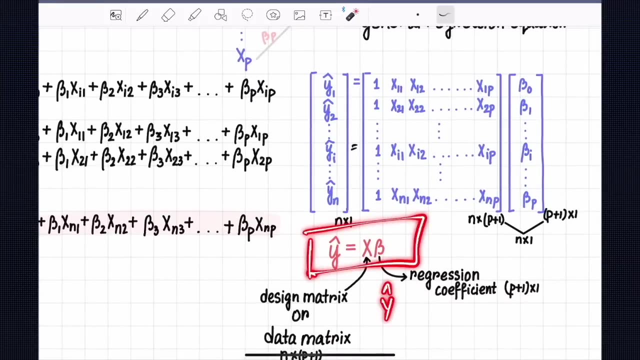 the third information and i-th data point for the pth information. right, And this is nothing but your prediction function, for nothing but your simply multiple linear regression hypothesis function. okay, You can write this in a vectorized format, which is: y hat is equals to xb. 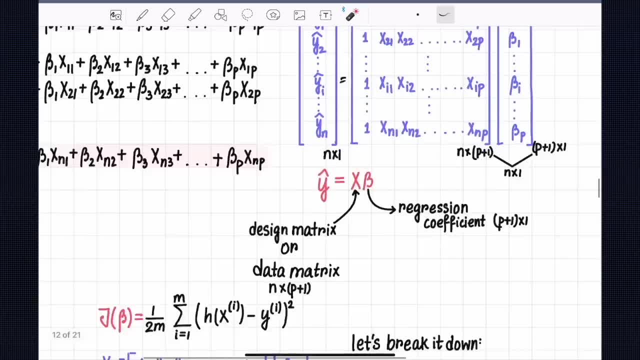 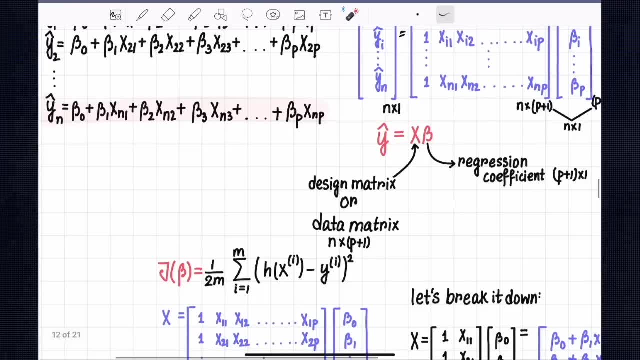 and this will yield to n times 1 vector. I hope that this makes sense. okay, Now, over here, now, once we have this, now, can I actually now, once we have the multiple, we have the hypothesis function, we'll do a worked. 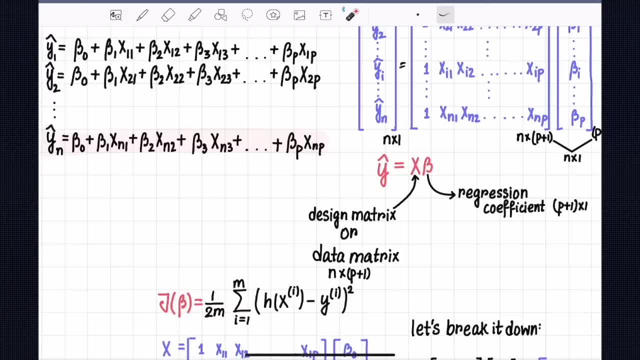 example, just like we did for linear regression, simple linear regression. we do a simple worked example for you to be better comfortable in: okay, Cool, Yes, So now you have this, now you have this, now you now what you have to do. now you've got your y, now you compare this. 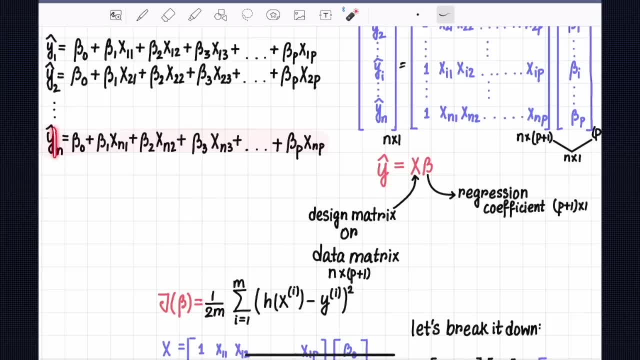 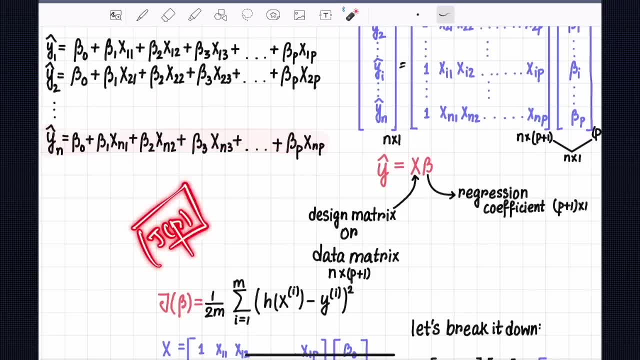 to do now. you have to do now. you have to do now. you have this j of pira, which is your cos function, which is nothing but equals to this, which is for, defined for simple linear regression, but eventually you will notice one thing. you will notice one thing: you have your. 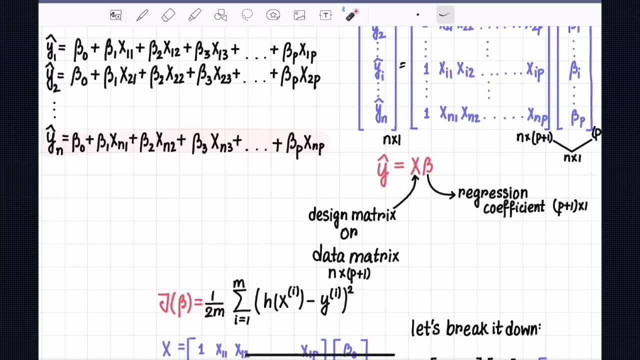 vector in this case, you have your vector in this case. you have vector in this case. you have vector in this case. right, Of course you can write your vector. not a big deal. you can actually what you can do. you can actually, you know, take out something. you can take out something like: 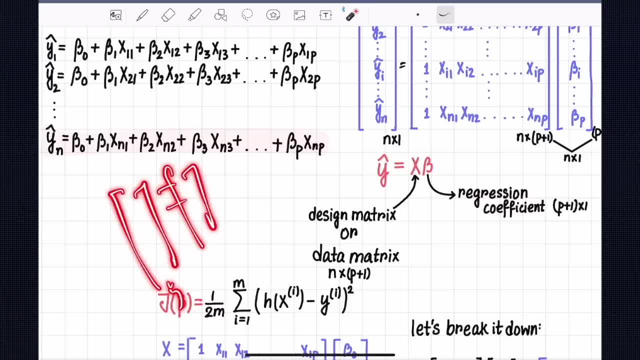 this: you're going to have the y hat and y and then subtract it, and then you're getting another vector, and then you're going to have the y hat and then you're getting another vector, and then you simply add all the elements in that vector and divide by the number of terms you can actually. 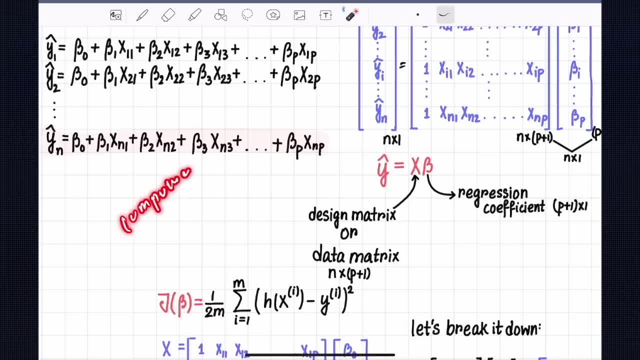 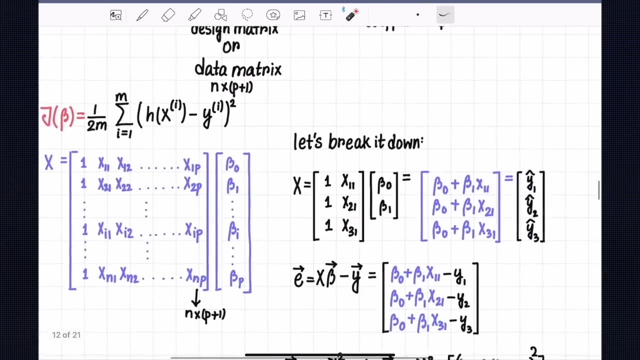 do this, but this is computationally, computationally expensive and computationally expensive. we avoid in machine learning because it's already too, too much. you know what do you say, but you know very, very time-taking. so what we do, we have a vectorized, as we have the vectorized hypothesis. 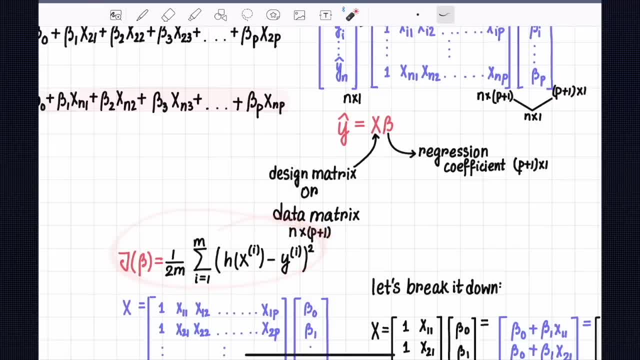 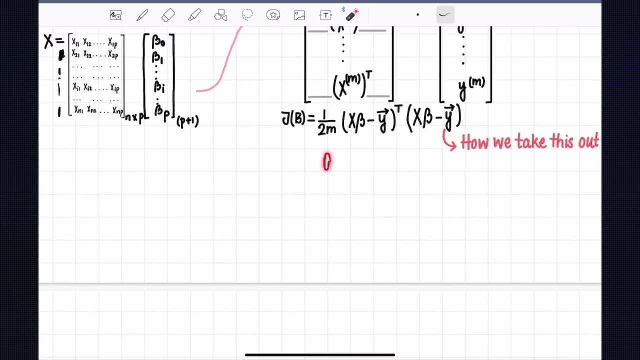 function if something is vectorized, which is computationally good. we have vectorized cost function, and we have a vectorized cost function, and we have a vectorized cost function as well, which is defined by this, which is g of beta, which is 1 by 2m x beta, which is your. 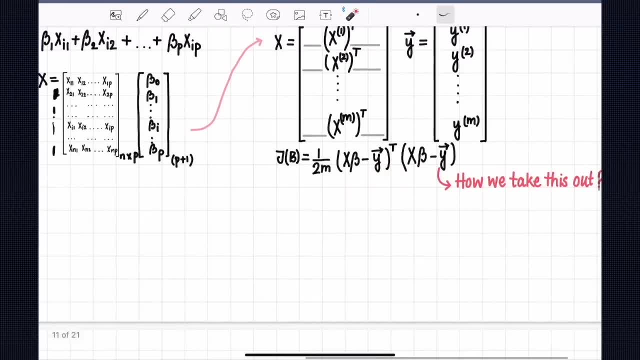 prediction function, which is the prediction, which is y hat. eventually, y hat minus y. transpose x beta minus y hat. well, sorry, y not. this is your prediction and this is your ground truth. prediction, ground truth. so you have this vector, this, this, this also, it's the. 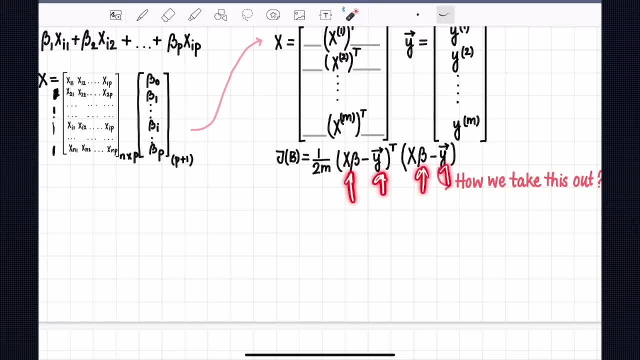 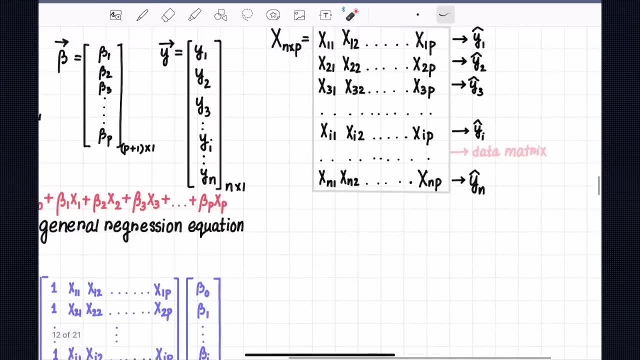 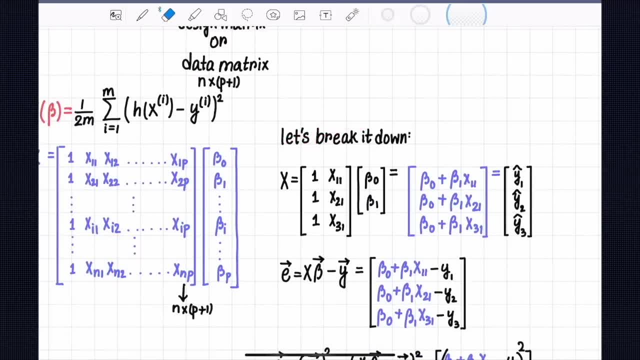 let's, let's not take this, let's take a very simple example: where you have, where you, where you have a vector x, where you have 1,, 1,, 1, and then you have first first information, first. 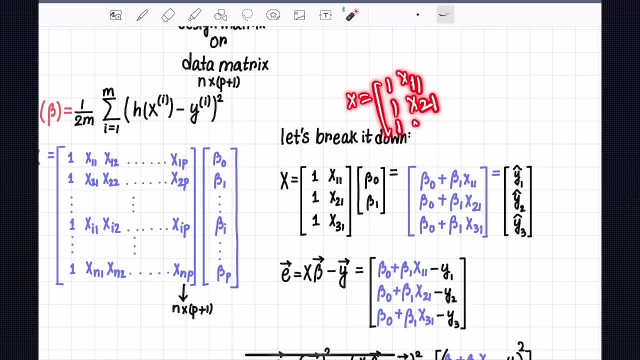 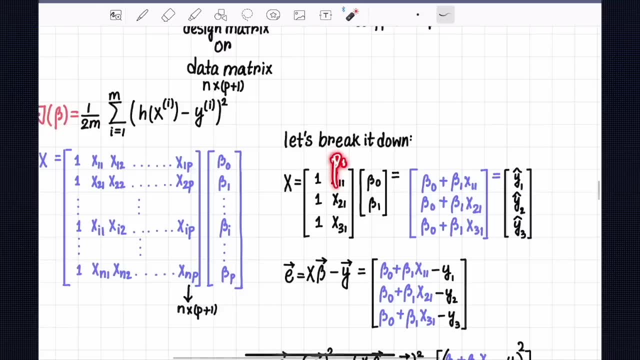 first data point of the first information for second data point, for the first, and you have only one predictor, which is an independent variable, and then you multi and, as you have only one information, you have beta 1 and beta 0, as as as a simple integration. but let's frame. 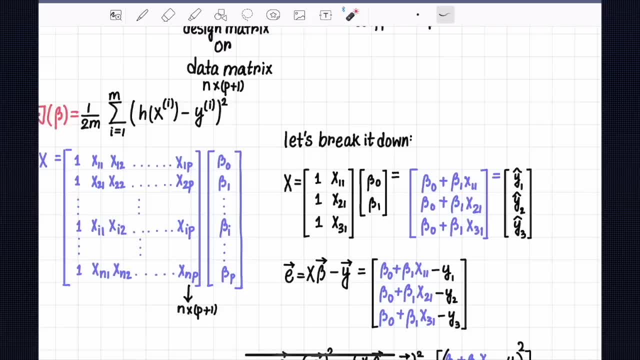 this in a multiple thing, okay, So when you, when you want to take the prediction, it's nothing but x, beta, so you take the beta 0 and beta 1, this, this the first row. multi take the dot product. between these two the. 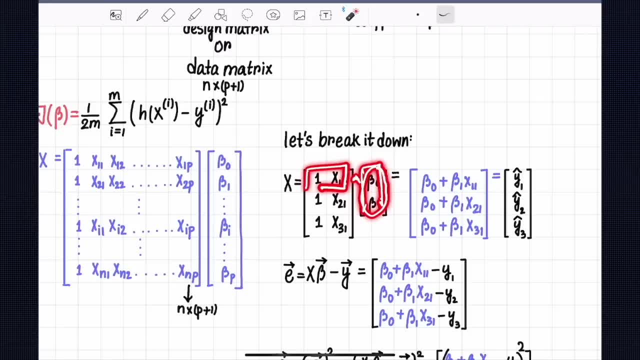 the vector, which is the parameter vector and the first row, and then when you take the dot product and then the and then you write the equation over there and then take the, this, this, this particular vector and then multiply with this vector, sorry row. 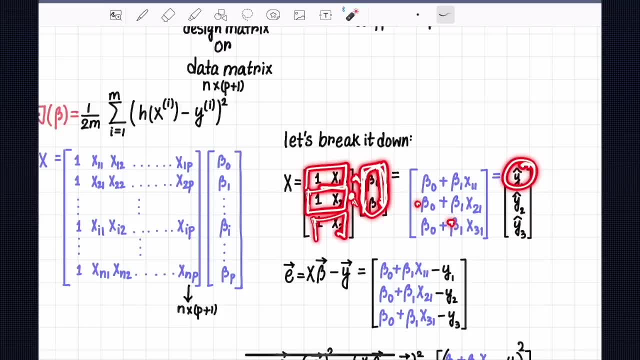 vector. then you dot the dot, the dot between the, the dot between the row vector and this vector. so you'll get the three data points out here. Now, what do you do Now? you have this, Now the what will. so you have the prediction, for you have the prediction from your model. 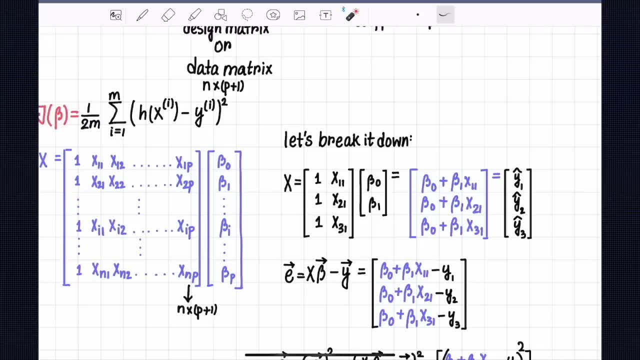 Now, what do you have to do? As I say that you want to, you want to identify what, what is the differences between both of them? right, as? please note that if you want to know the geometrical perspective, of course, please see my previous lectures, because I've already told this, I'm not going. 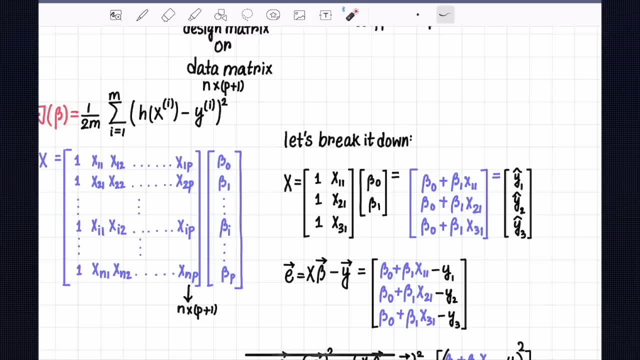 to tell again and again. So you have. now you take out the errors, the residuals, how, how, apart from they are. so you simply have the prediction function, the, the prediction which, which which you got x like xb, which is equal to nothing, but the vector minus y hat which which. 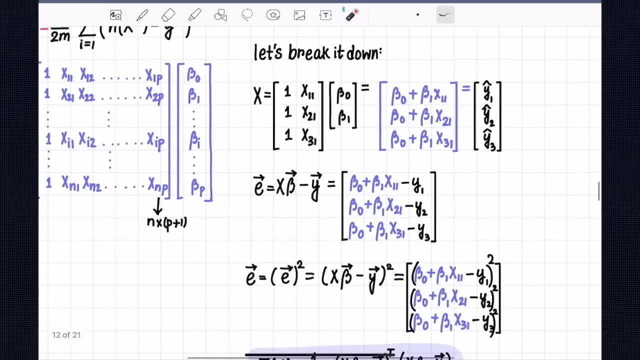 is nothing but what, which is nothing but a ground threat. okay, So, when you see this, when you see this, you will simply have this, and now we have to, as as as to as to remove the, you know the squared sign here, sorry, the negative. 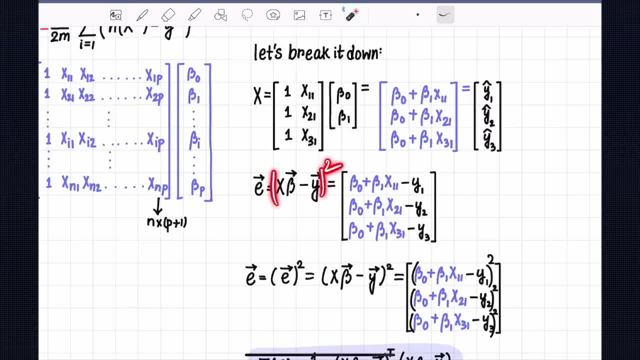 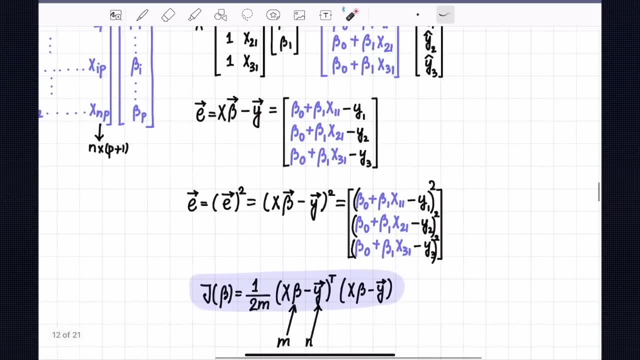 sign: we square, we square, so this is going to be a squared. so, if this is going to be squared, so every individual parameter is going to be squared. So, when every individual parameter is going to be squared, now you can see that this is. 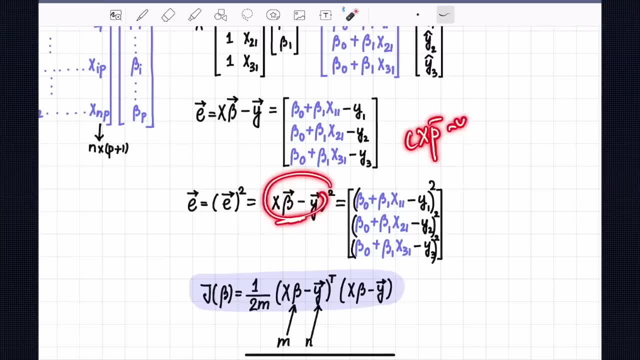 going to stay, so you can. actually you have x beta minus y beta, Sorry, x beta, which is the, which is nothing but which, which will yield the prediction function, which vector minus the ground truth transfer. so basically, let's remove transfers. 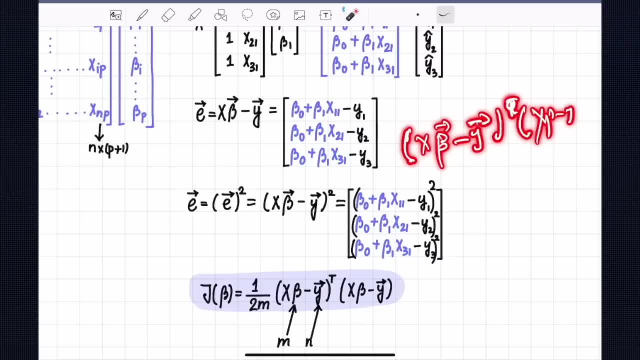 as of now. so you have a couple of times x beta minus y. so you simply take the transpose for vector multiplication of both of them and eventually you will be getting a very nice. so you have noticed a pattern. you know using vectorization it will eventually helping. 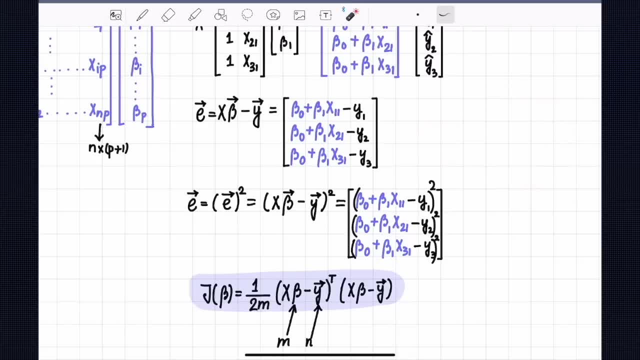 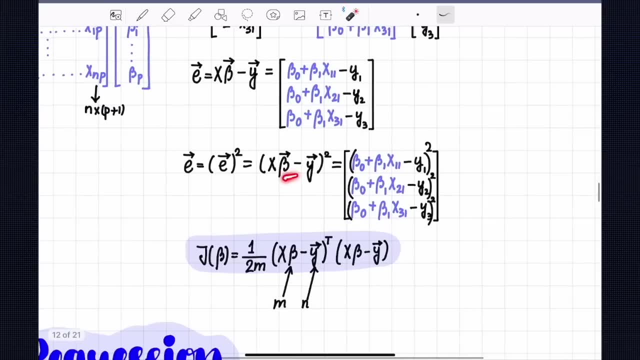 you, it is helping you out. it is helping you out very, very easily. it is helping you out. so, basically, you, you, you are simply multiplying. you are simply multiplying this two times this, this, this square of this. so, basically, you have this, you have. 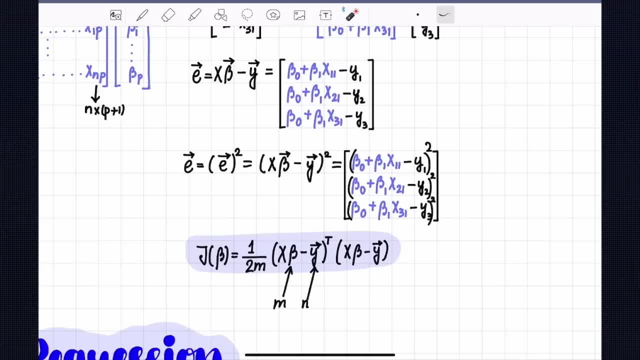 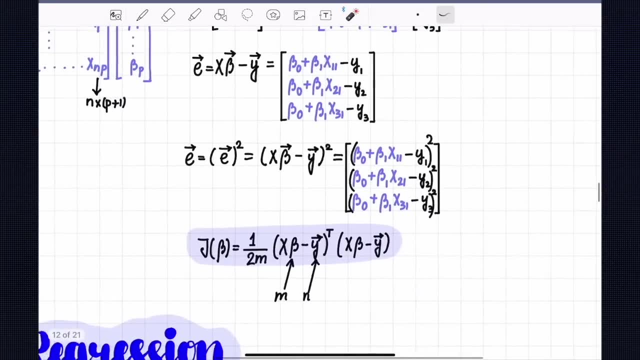 this transpose for better computation. you can see for that if you, if you will do one sample example just to see how does it work. so now, rather than doing this extensive computation, you can simply, you know, multiply the subtract, the vector, and then take, take out the dot. 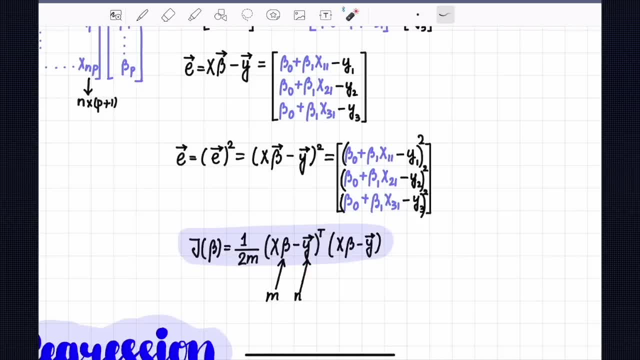 predict in both of them to actually get the answer. okay, hope so it makes sense. okay, you have the dot predict in both of them To actually take out the answer and then you divide by 2m, or 2 over here is added. 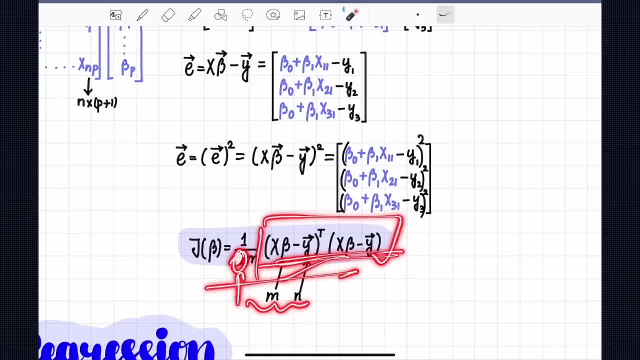 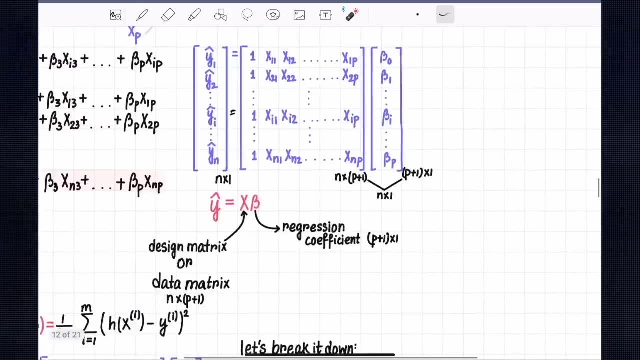 because of the gradient descent convention, but you can actually remove this 2 as well to take out the what average. I hope that this gives a good sense about how to. how do we came with this cost function? efficient cost function. 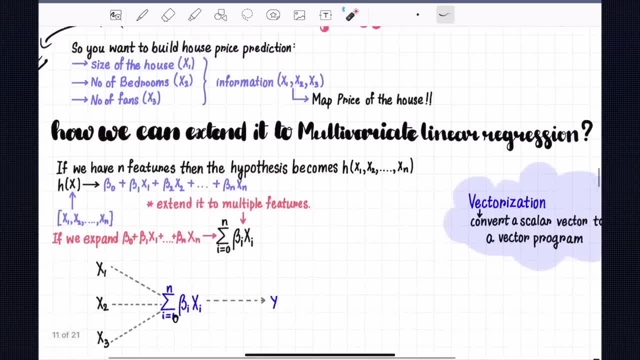 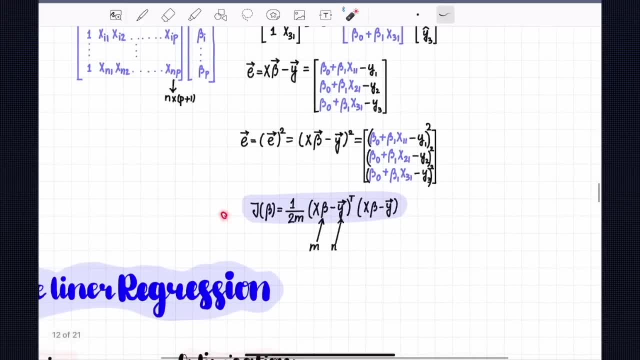 Apart from that, I think we covered pretty much very, very well about this multiple linear regression and then now, once we have this cost function, now we are able to evaluate it, now what we will do. now we want to minimize, we want to minimize the cost function. you. 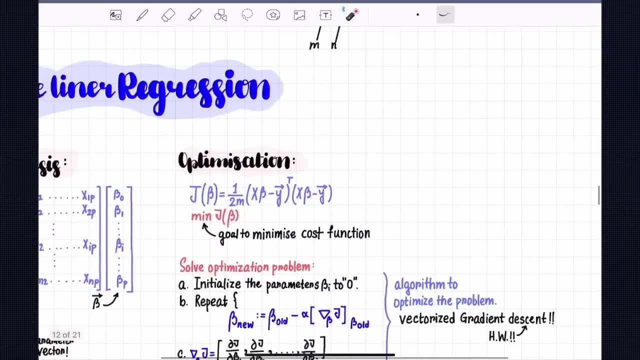 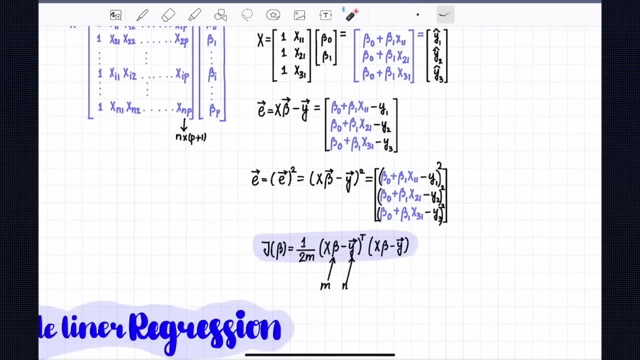 will see that how I do that, How I do it using again gradient descent. I'll show, I'll showcase you the difference between the partial derivative, as we are using the partial derivative, why we are using a partial derivative- a very interesting question. but I'm just, I just wanted to be with the. 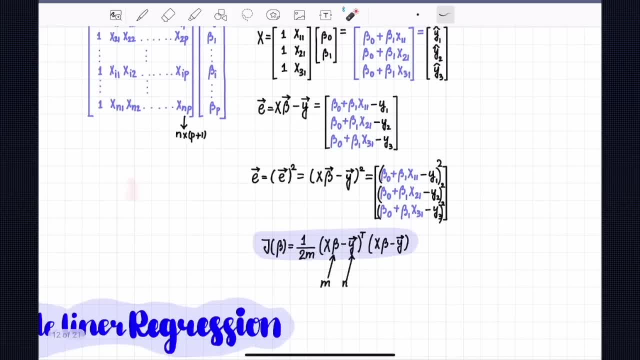 convention. I just don't want to use that d. d is used for scalar programs, but this partial derivative is used for what is used for vector formula. but but basically I think I'll just note it down for you. 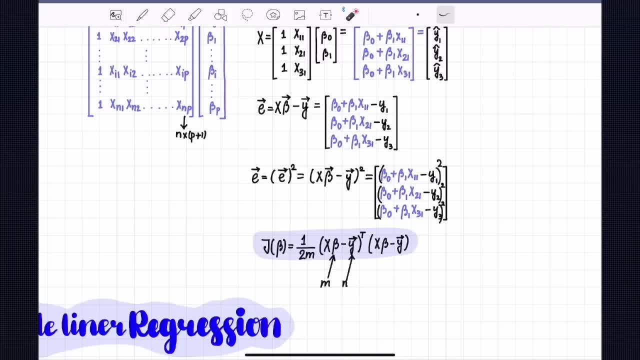 For for you all that, okay, here we are using, in terms of future notation, the. the reason why I use that partial derivative in that, when actually we were solving gradient descent, is for so that it so, so that it works perfectly for our future notation, which. 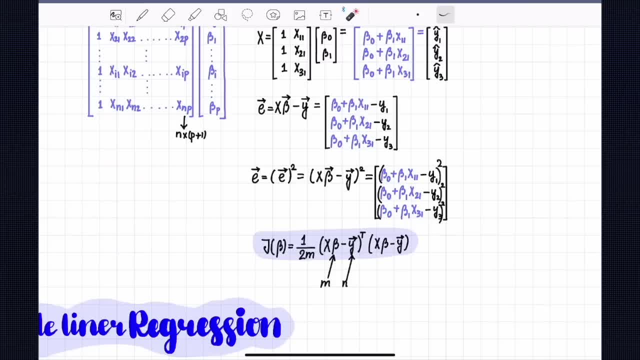 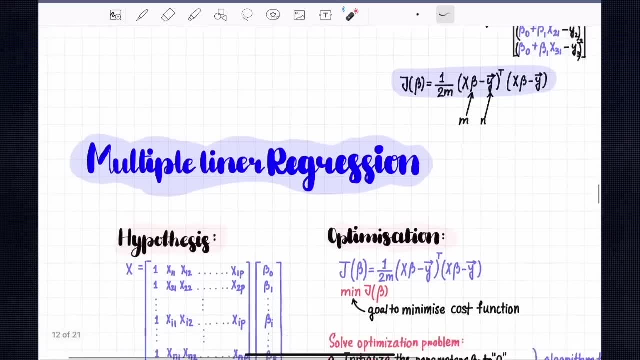 we'll study right now so it makes you be a bit handy. otherwise I could have introduced various, so you might be confused. so that's why I didn't introduce over there. Okay, so cool. I think it's now. in the next video we'll talk about how can we optimize. 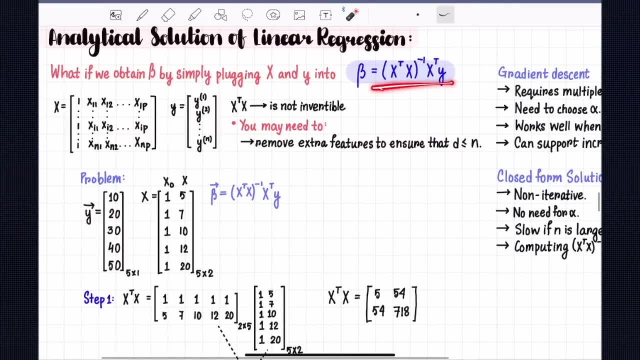 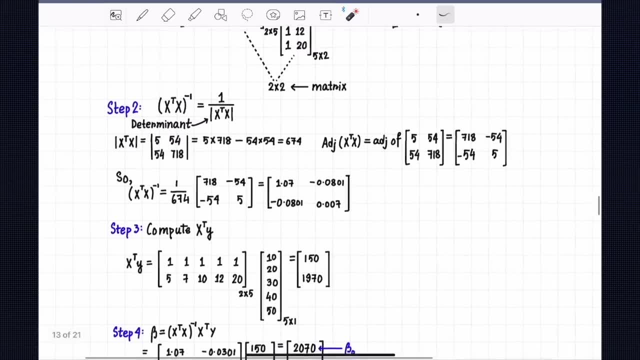 our cost function. and apart from that, I'll show you an analytical, analytical solution. how can we, without any procedure, we can just take out our beta's value in matter of no second, in in matter of no time, with, with, calculating, and then we'll talk about. 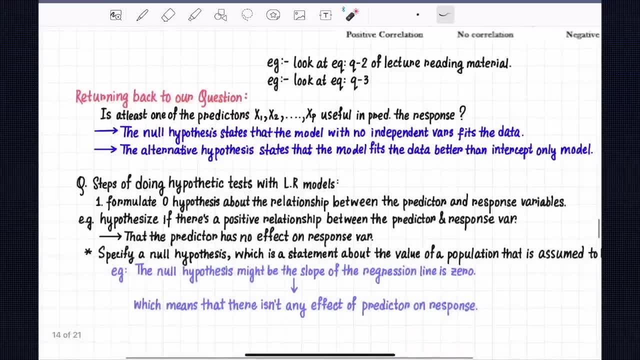 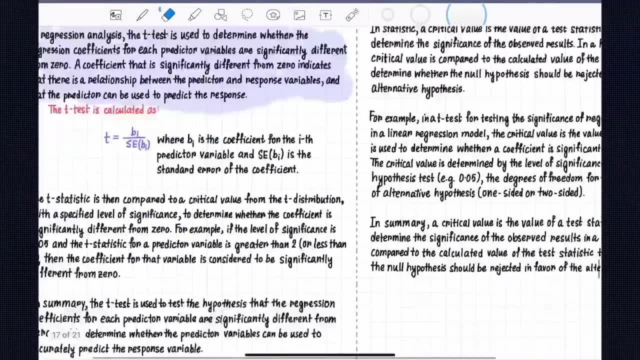 how can we evaluate. and then we'll talk about some of the hypothesis testing, which is t test, f test and a lot of things going to come up, and you'll be eventually enjoying all of this thing. and after that, what we'll do? we'll talk about something known as assumptions. 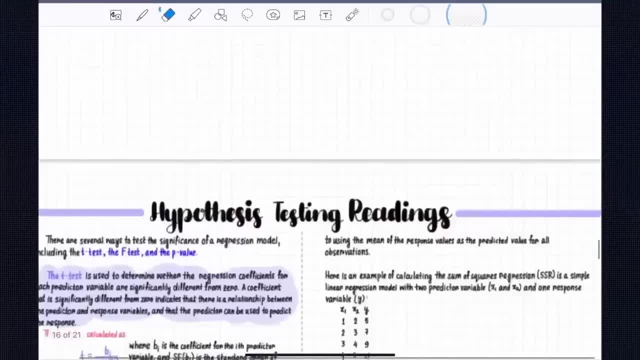 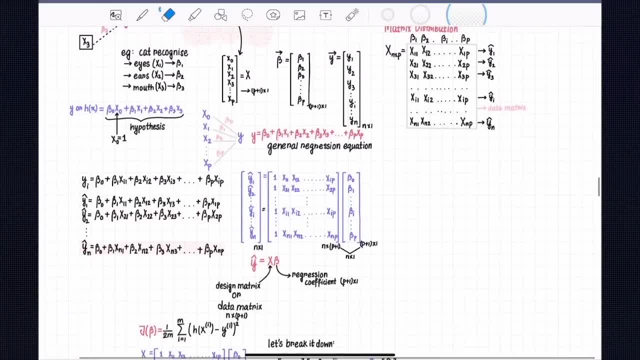 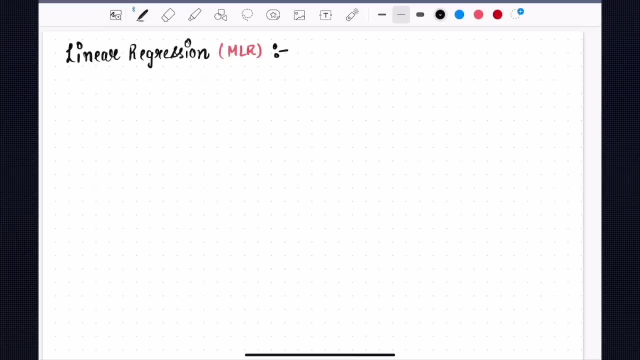 super duper enjoying that as well. i, if i'm enjoying to teach you all of this. so let's catch up in the next lecture, linden, bye, bye, hey, everyone, welcome back to this lecture. uh, so basically, uh, we are at linear regression, where we'll be talking about multiple linear regression. i already have the 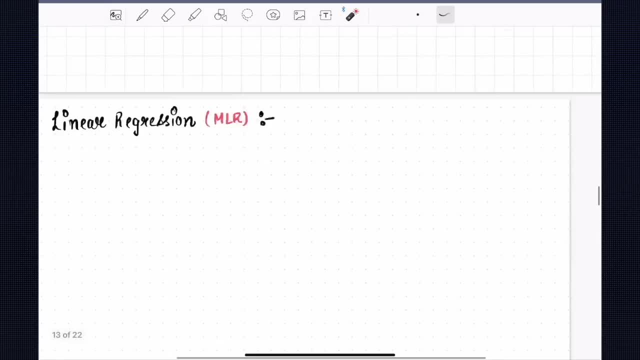 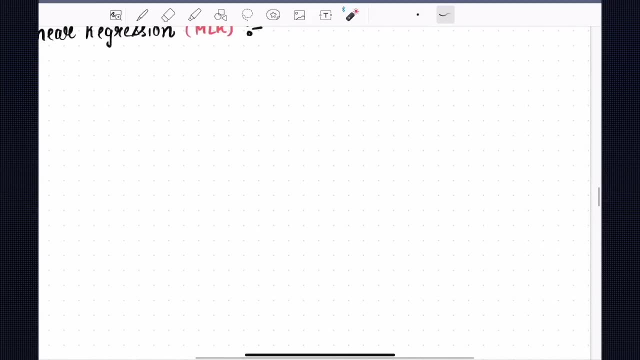 notes for you, but that's a bit less so i just want to elaborate with you, uh, to you, with some examples which may help you to understand much more better. so we'll do a. we will have a set of worked set of examples for you to better understand all of these things. okay, so let's get started now. 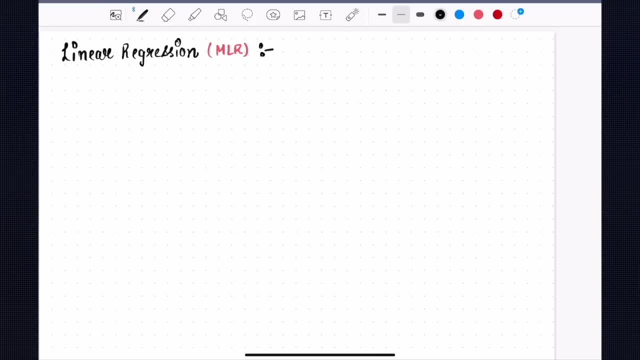 so basically, uh, let's have a, let's have an example so that i can show you the vectorized operation and everything. so assume that example over here is x1, uh, x2, x. in x1 you have 1, 2, 3 and 4 and x2. 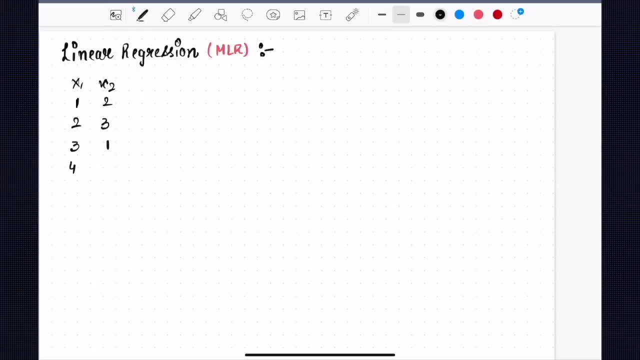 you have 2, 3, 1 and 3, and then you have the. you have a, two independent variables and then you have one uh uh dependent variables, which is 3, 4.5, 4 and 6.. so you have the data available, you have a data. 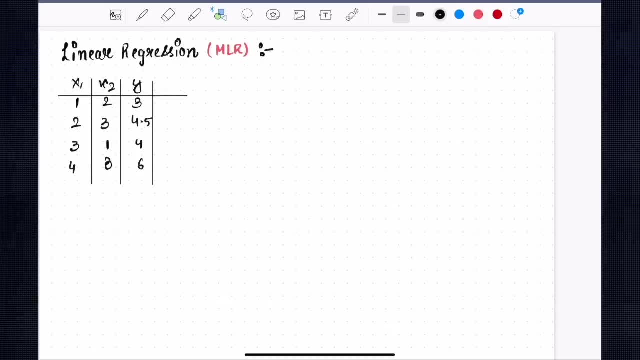 available like this. so let me just draw a straight line: you have a date, you have a data available where these two- uh, these two variables which is out here- these two variables are independent. independent, as this is no dependent output variable and this is nothing but your y. 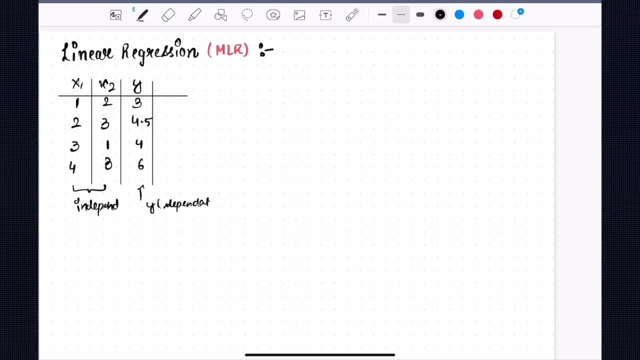 or your dependent variable, or your dependent variable. okay, so this is the data now. so now you have the, so now you can make a design matrix. so you know. so now you can make a design matrix. first of all, first of all, we'll, we will calculate the, we'll have the hypothesis function out there. 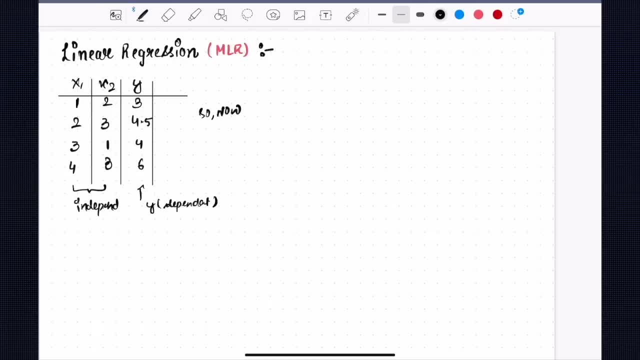 okay, so we are. now we are not train our linearization model on top of it. so how we'll train, first, we will, uh, put, put that in form of a matrix which is nothing but um one, two, two, three, three, one and four, eight, and then, if we have one, one one, i'll show you what is the use case of the matrix. so 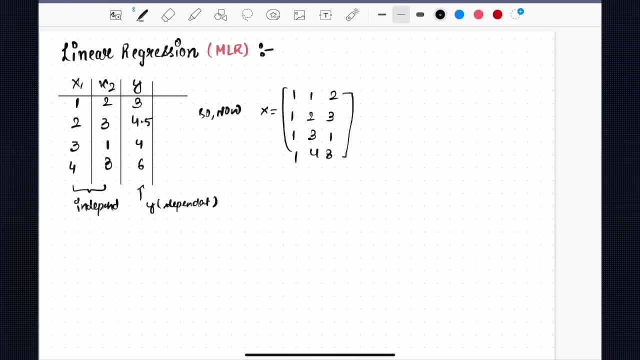 of this one, just in some, just in some, you know moments which you will see that why we are adding one more over here. so let me just have this in a nice way. you have x equals to 1, 1, 1, 1. so with the: 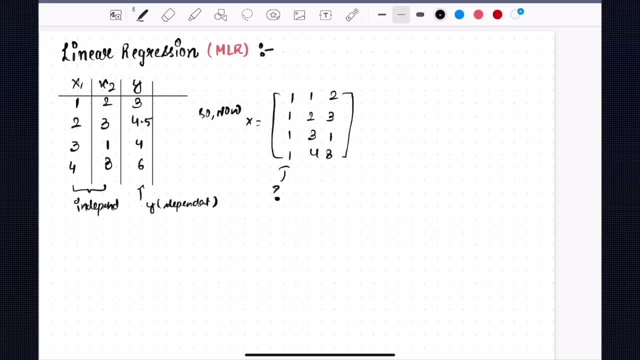 we have the design matrix- we'll talk about this later on. we'll talk about this later on- and then you have beta and then you have beta. so basically every individual feature has its own beta right. so beta 1 and beta 2, beta 1 and beta 2 right, beta 1. but but we also have something called. 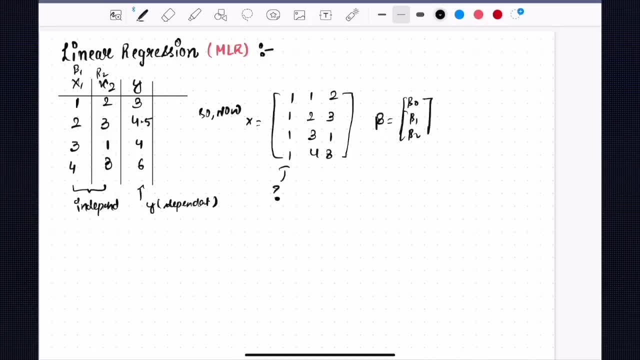 beta 0. right, so how beta 0 will? basically when we do the multiplication. so basically we take the first row, multiply with the uh, then take the dot product within the first row and and the vector b. so basically the here is here. we have only two, for example. assume that we haven't taken this. 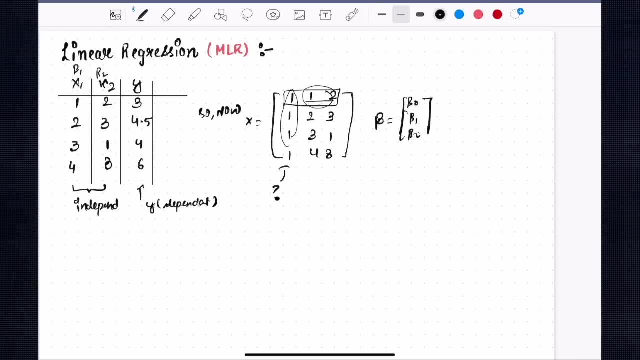 particular, 1, 1, 1, then we would have only one, two and this. this would have been left. so we have to multiply beta zero to one as well. right, because beta zero times x, zero, x zero is equals to one. that that's why. so you assume that you, that you have initialized your beta with- uh, maybe. 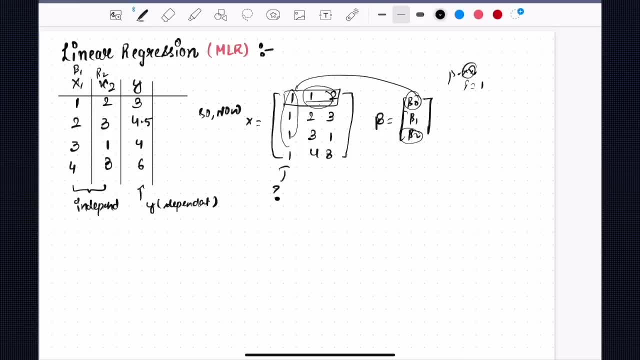 zero. so, but before that, you have the beta over there, and then you have your uh ground truth, ground truth vector, which is three, four point five, four and six. three, four point five, four and six. okay, so you, so you have this uh ground truth, uh, over here now. what you do now. let's now with. 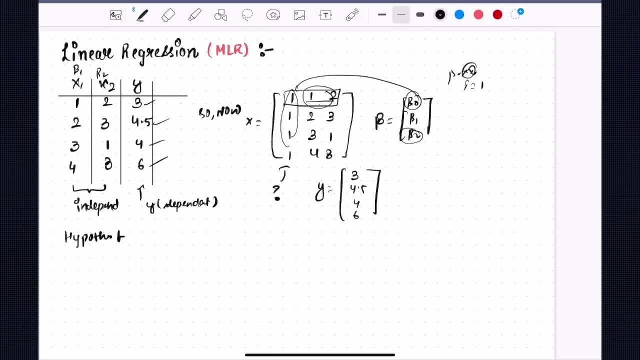 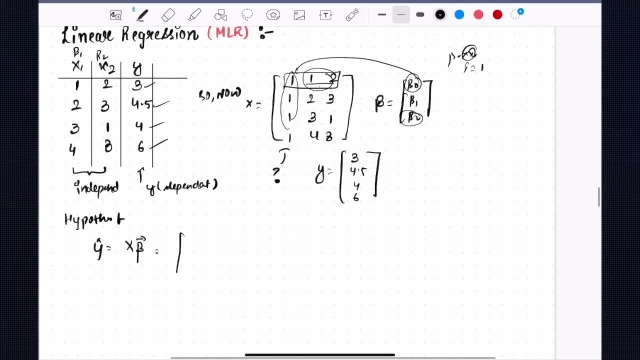 available settings. now let's let's do one thing. let's form a hypothesis function so you can get your prediction vector by multiplying your design matrix with the, with the parameter vector, and this will yield to, to um. this will yield to a vector. this will yield to a vector which is equals what? 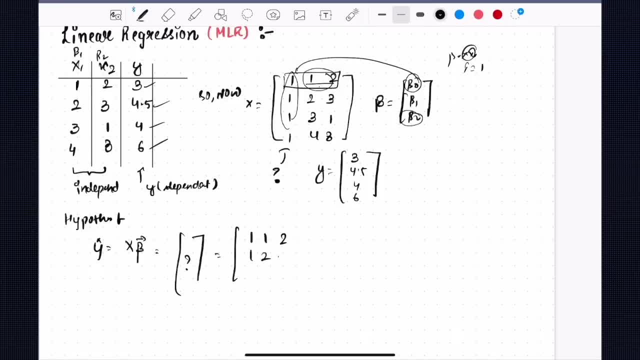 what was our design matrix? design matrix was one one, two, one two, three, one three, one one, four, eight. and then let's initialize our beta value: beta, zero, beta one, beta two, all, all, every to zero. because we have to, you have to find the best setup. so, in the first situation, what do you? 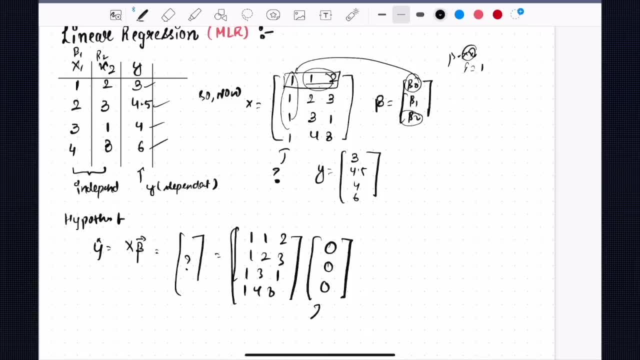 do you just initialize. okay, i hope that this really makes sense. uh, to you now, once we have that, now, once we have that, what we will do after initializing our beta values, after initializing our beta values to zero, what we will do? we'll simply have this zero, zero, zero and 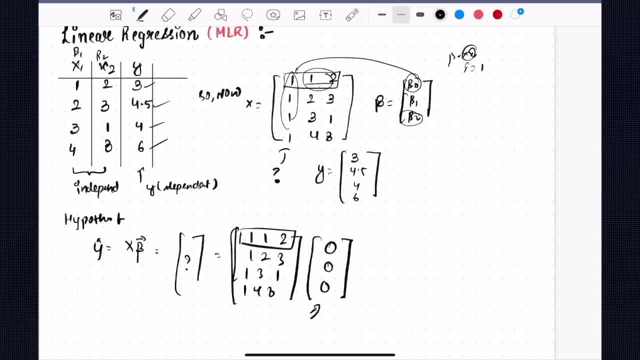 now we're going to initialize our beta values to zero, and then we're going to initialize our beta values to zero, and now we're going to initialize our beta values to zero. and now we're going to take the field. we will take the dot rate between the first row and the column of that, the first. 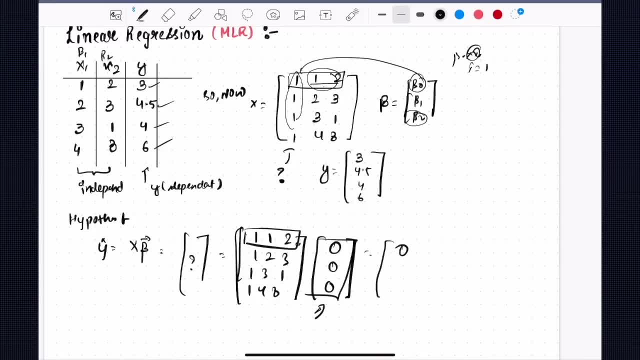 row. the dropper within both of them will yield nothing but zero. the dropper between the second row and this vector will lead to zero. this and this is zero and zero. so your predictions, your predictions, are zero, which is your y hat. so, once you have the predictions from your model, when your 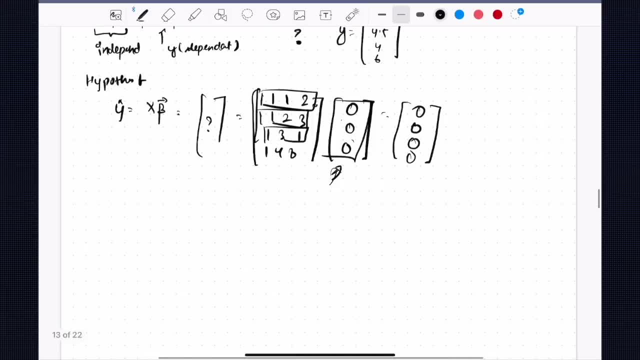 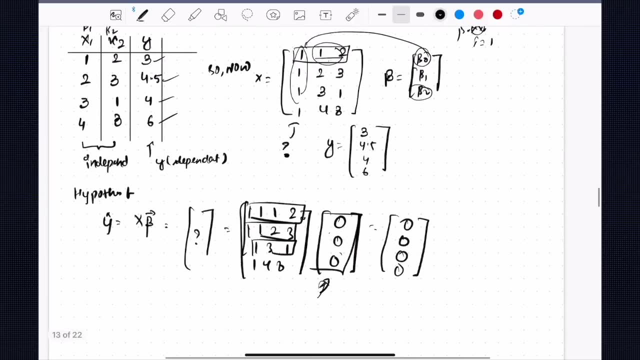 betas are all set to zero, you'll be having that, okay, and then and then. now we have to compute the cost. once you have the model prediction. now you have to compute the cost. once you have the cost. once you have the model prediction, now you have to compute the cost once you have the. 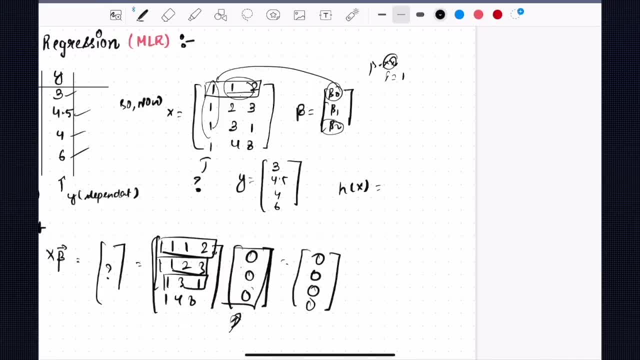 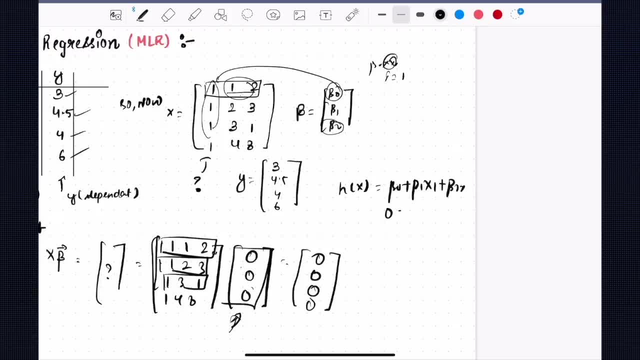 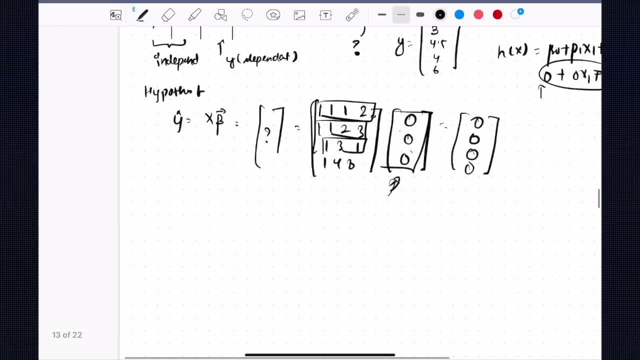 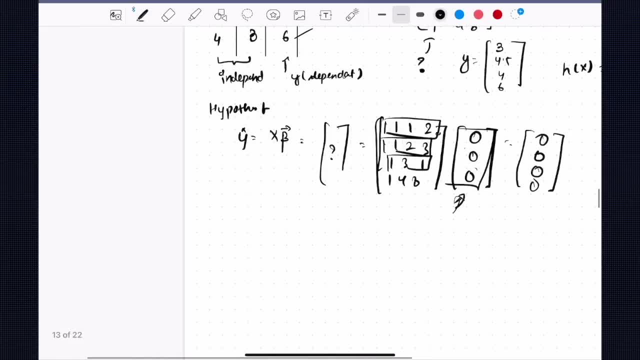 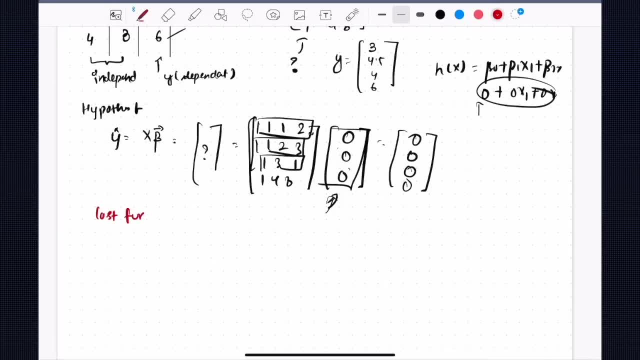 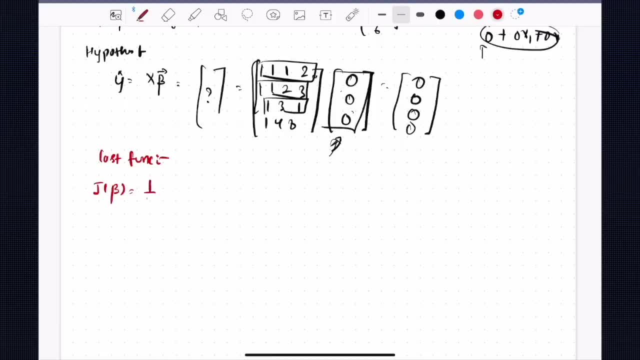 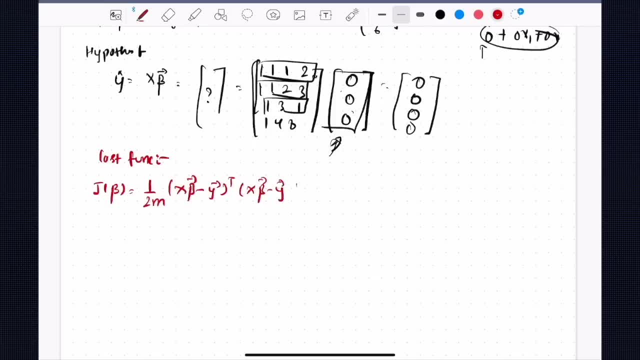 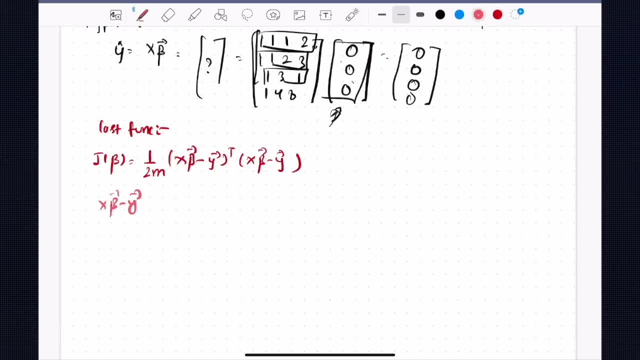 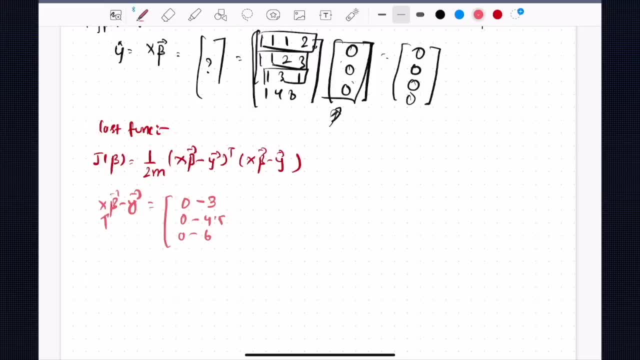 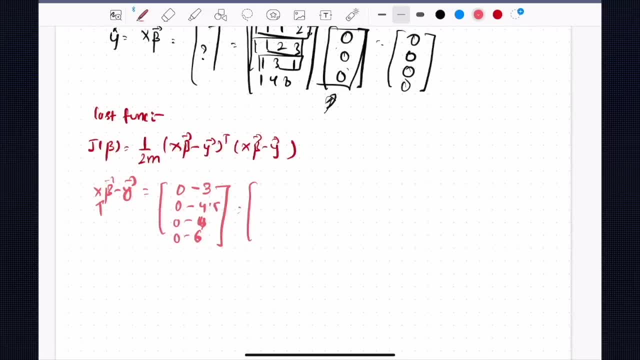 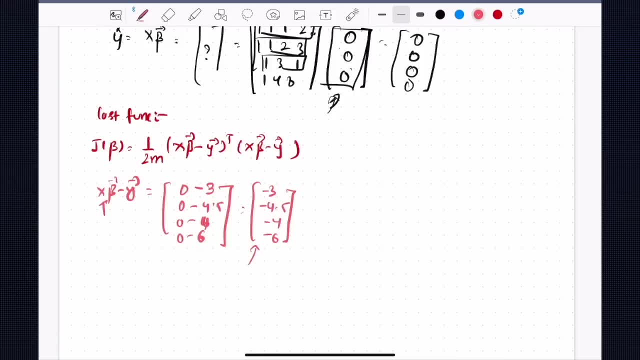 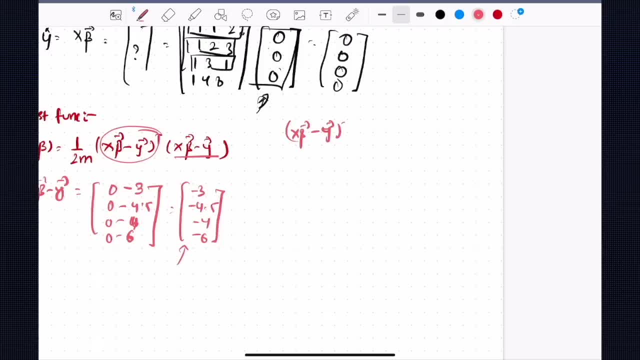 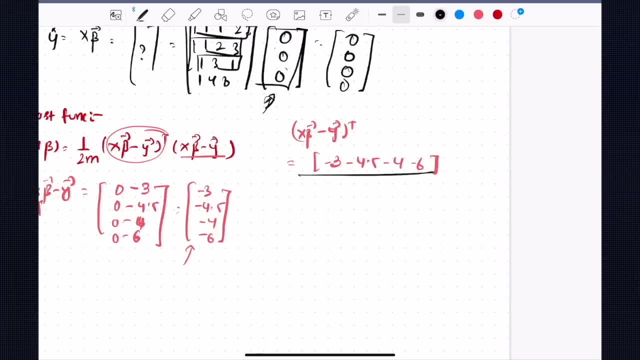 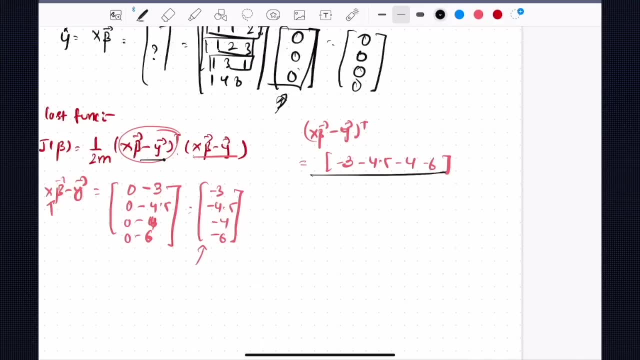 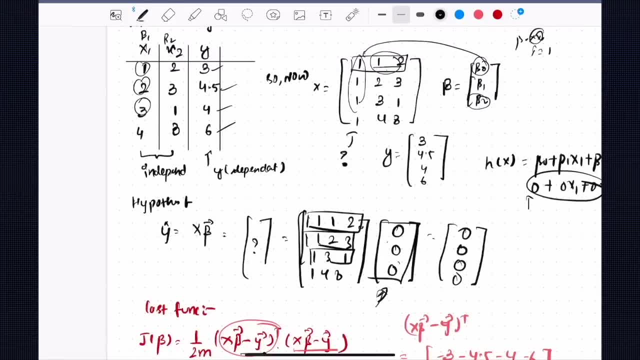 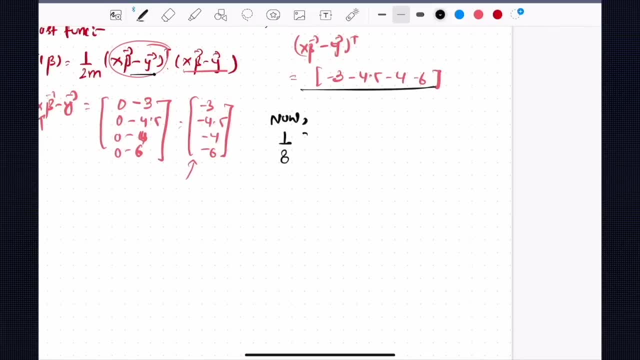 you have here. you have four examples. M is goes to 1, 2, 3, 4, 4. data points: 1, 2, 2 by 4 is goes to 8: 1 by 8 times 1 by 8 times minus 3 minus 4.5, minus 4. 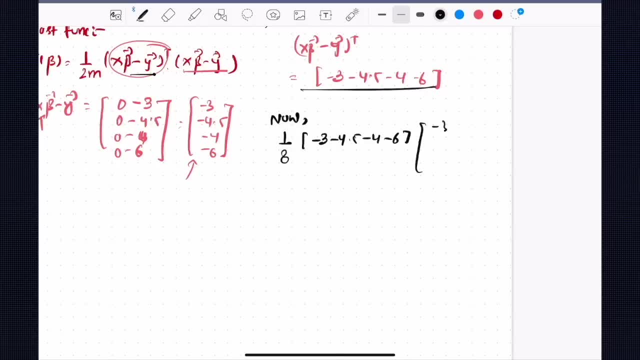 minus 6, and then you have the non transpose vector, which is minus 3, minus 4.5, minus 4 and minus 6, when you actually calculate this up- and you can actually calculate this up, which is nothing, but which is sorry, this is nothing but 9 plus 25, so 9 plus 20.5 plus 16 plus 36, as you multiply the 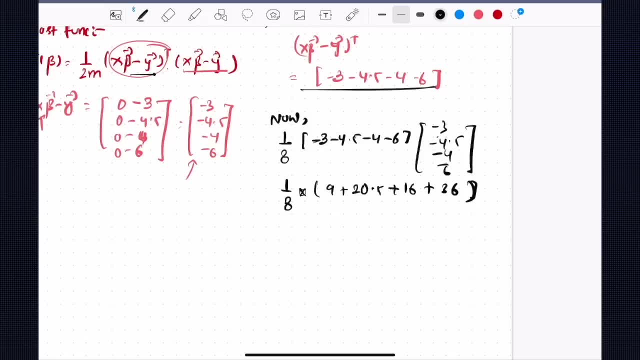 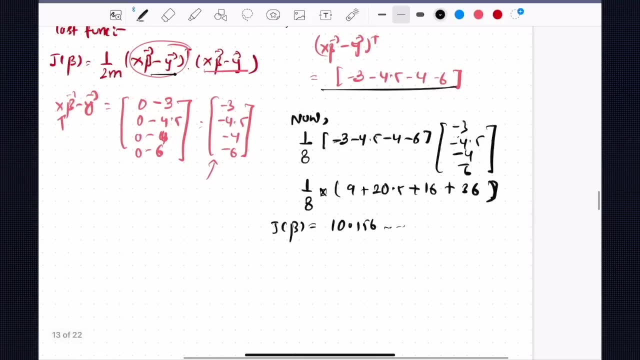 element wise operation. and then what do you do? and then you simply add it up and that will do your beta in yield to 10.156, so you'll have this cost function out here, okay, so you have seen that how we have taken an account of this. at what? 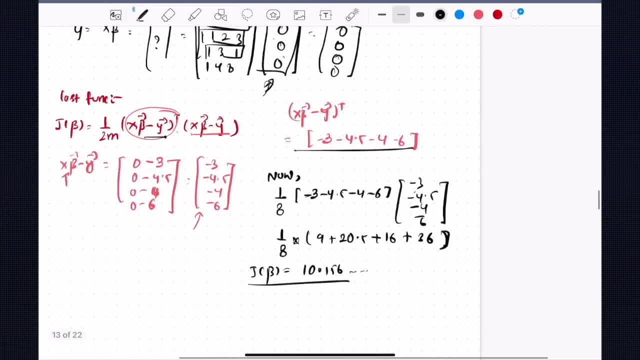 this is function. after that, we have, at this, taken out the and and we have taken out the cost pension out there. I hope that this gives you pretty much a good sense about how exactly we cover up things. now. this was that vectorized operation out there, right, so how this vectorization really helps. so this is a 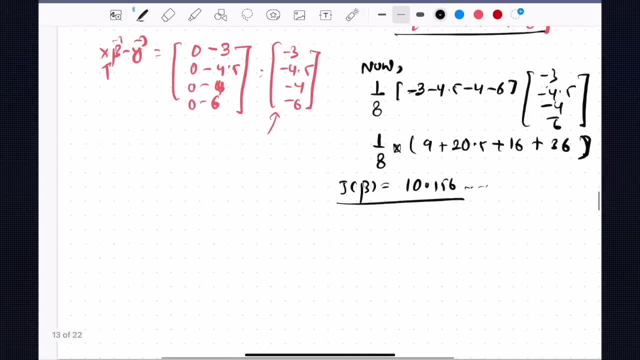 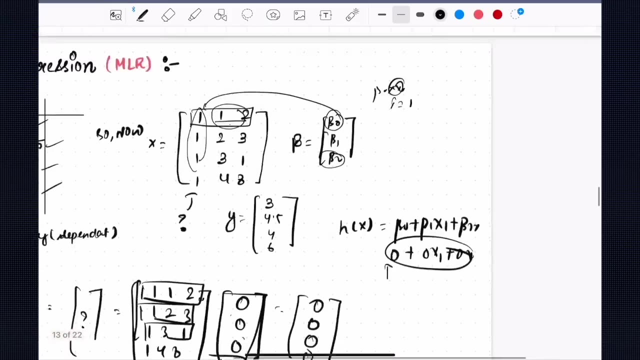 very important topic to talk on. maybe it's very useful as well to talk on, like, how vectorization question, how vectorization, how vectorization helps, how vectorization helps. so if you were to do this normally, you know if you, if you were to do this without any vectorized operations? first of all, let let us 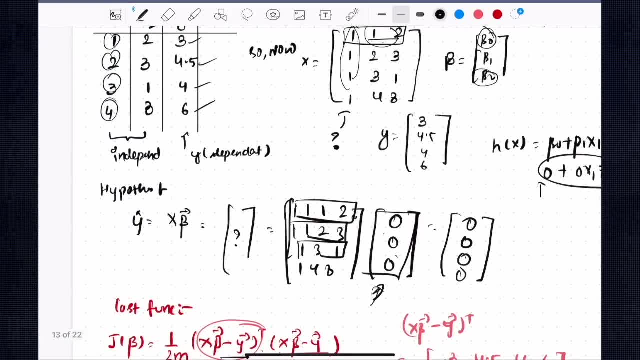 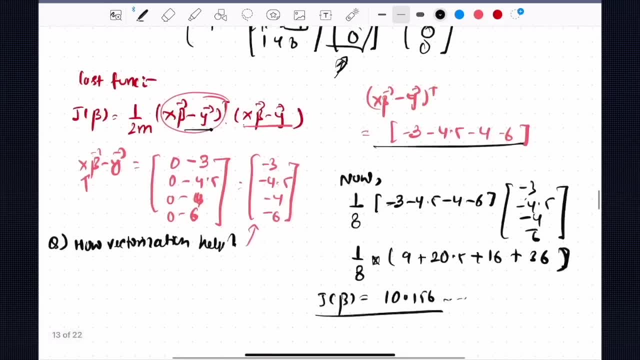 assume you know you don't want to do it with any vectorized operations, first of all, even with calculation of hypothesis, will take too much of time. no nested loops will come in. it will take too much of time. so when you have this, particularly your design general form, which is the 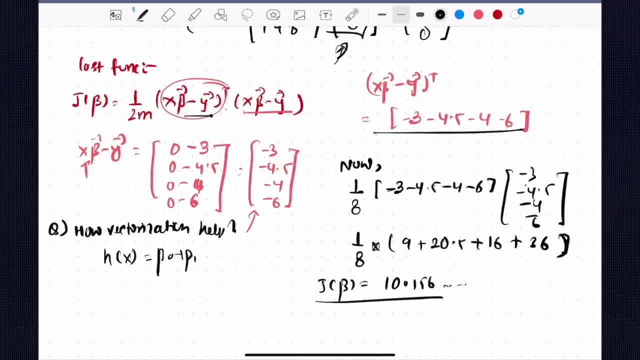 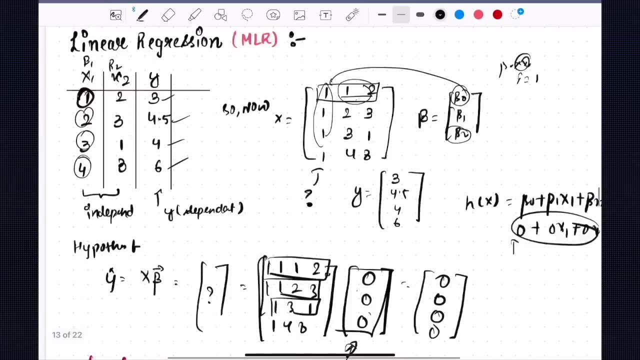 sword number part, which is when you are write word and you put a, all the time start to calculate the a. this is what you put, the a-line value of x. you have to put h of x. this is your know. your going to write further with h of x, your h of. 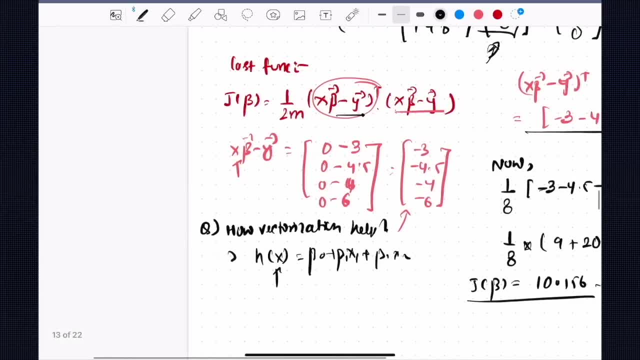 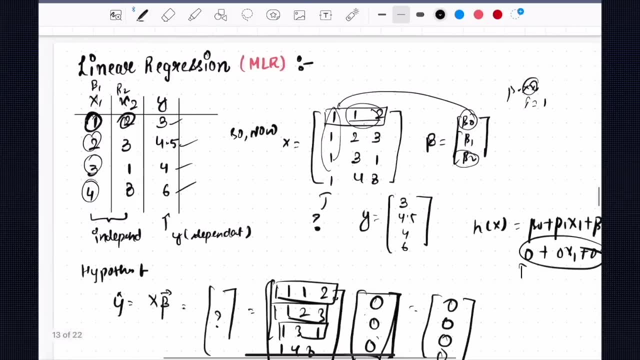 a. it basically is the size of an x enаци. that means h of x and h of x and you have n for products and x for business. h of x will be h of x and h of a once we go over to x1. ok, this is where you need to do, as you all the 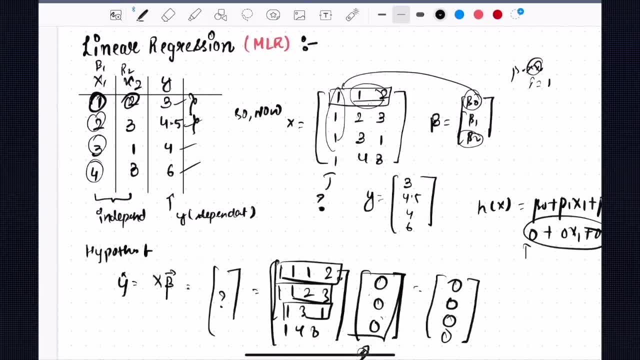 n that you need to. therefore, when we do this for big data, when you do h of a- 很好 -, h of x is kth into beta zero plus bita20 it. Melissa, in the background, we know what we're doing now because we have zeta 0 plus x, 1 plus zeta twice we. 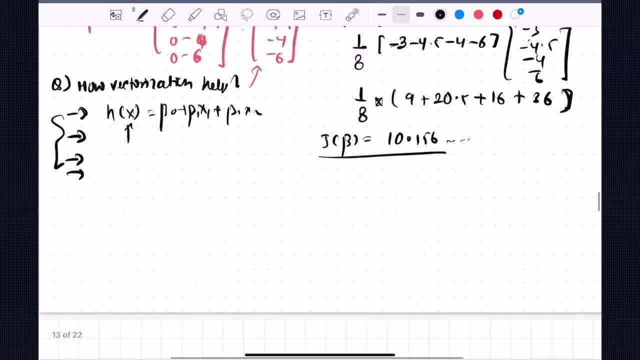 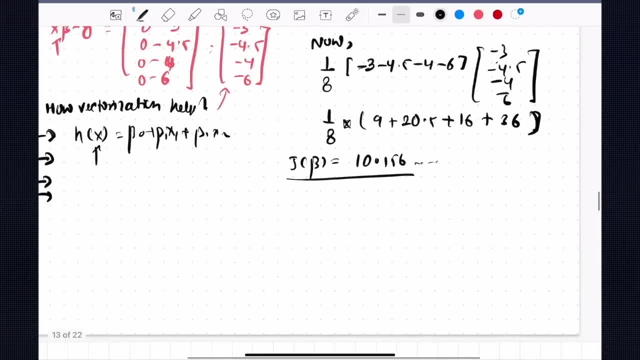 for every individual right. so that will take a ton of time, right? so that's why we we over here. you have seen that how simplicity by at the only one time. it just calculates our error. okay, cool, so, um. so what are the? what are the operations involved? what are the operations? 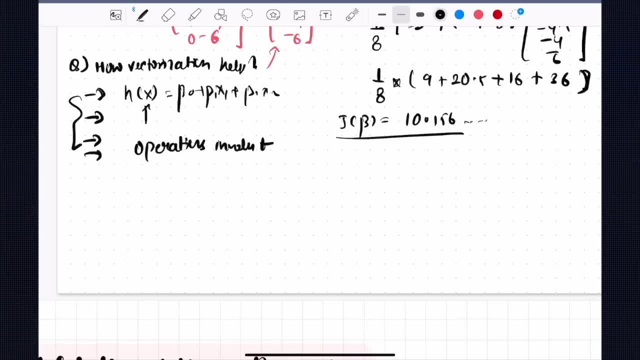 involved, which you have studied right now. so operations, the first operation which is involved is compute the compute, your hypothesis, or compute xb, which is nothing, your x is nothing but m times n plus one matrix, where you have one included for one one, one column, and then you have a beta, which is nothing but n plus one matrix, and and then you have nothing. 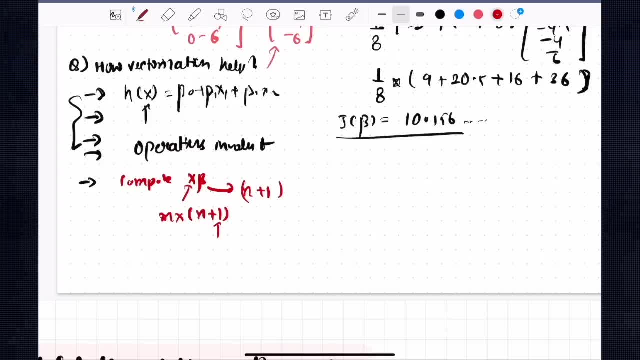 but n plus one matrix. okay, and then you have a beta which is nothing but n plus one matrix- uh, sorry, an n plus one times one matrix. or the vector where you have betas are also included. that's what you have. and then you have a beta which is nothing but n plus one matrix. 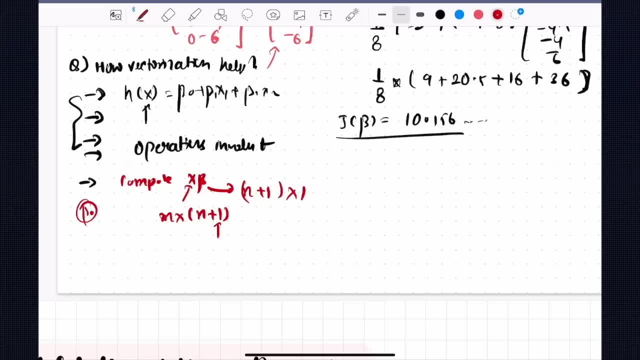 that's why we we have this plus one, okay, so compute this. so computation takes the. the complexity will take uh some order. so that's the first and uh operation is involved. second operation which is involved, which is the which is taking all the error, like this: and then 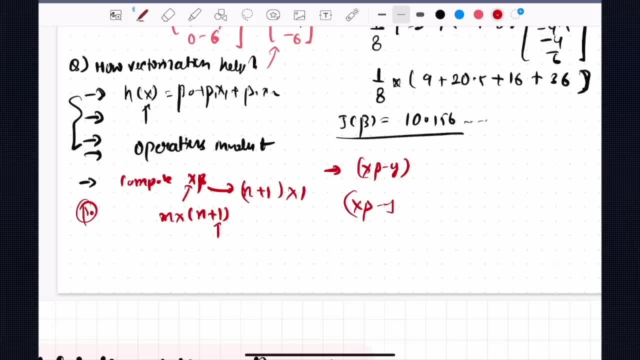 what you do, and then we take the transpose of this, and then we take the transpose of this and then we multiply it. okay, so this is the second and third information and after you multiply if you will be getting your answer. so the total time takes it's very less, as 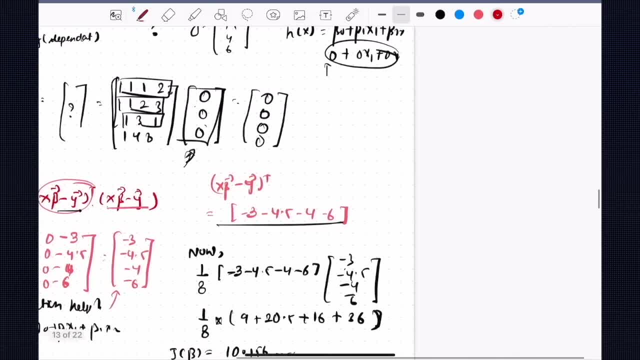 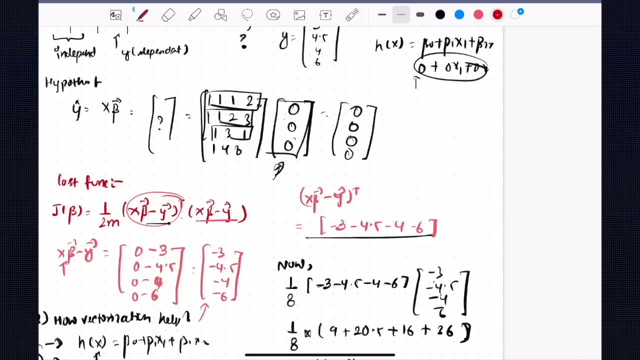 compared to the. you can also take out the runtime complexity if you want. so now, i hope that this gives a good sense about what exactly we're trying. we're trying to offer now, what we'll do now. we'll go forward and talk about: uh, how can we perform a gradient descent, how can we perform gradient? 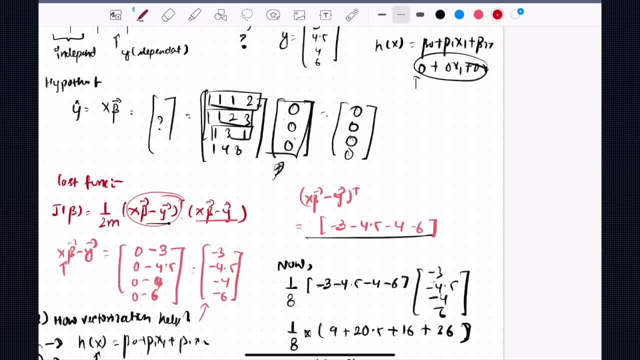 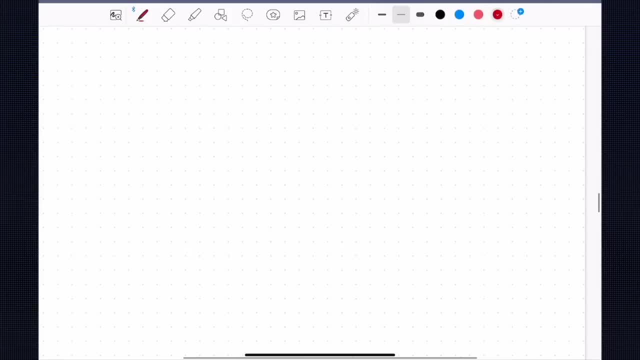 descent out here, okay, so that's the first question to tackle. so let's go ahead and have this current template and let's get started. how can you perform gradient descent? okay, so, basically, so, basically, um, how can we perform? let me just write: gradient descent. amazing question, right? so how can 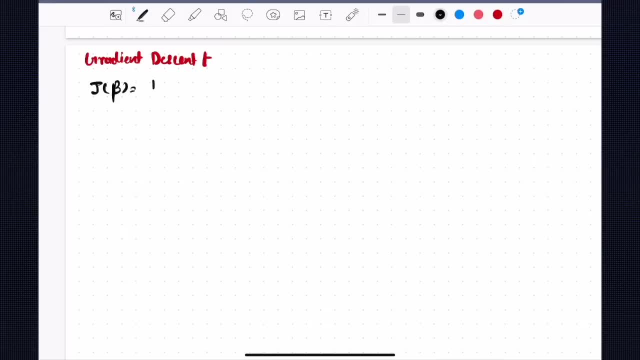 we perform. so you have j of beta. your cost function is nothing but one by two, m: x beta minus y. transpose x beta minus y. so this was a cost function, right. so now this was: this is a cost function, as i've studied that you have to take the partial derivative of your cost with the gradient. 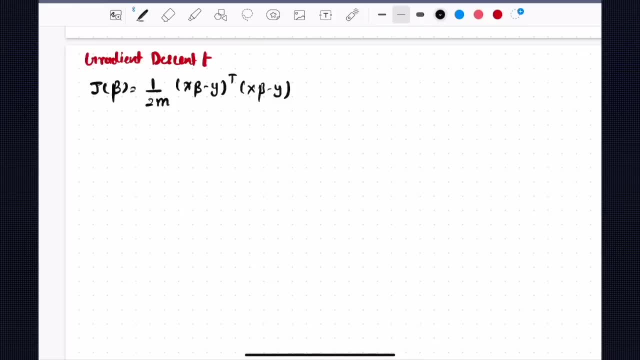 of your cost function. so there's a difference between partial derivative and derivative. so there's a difference between partial derivative, of course, function with respect to a parameter and uh derivative of so previously. so basically, this we use if we have the scalar program, if you have a scalar program, just just, just like we saw in our uh previous: simple, simple. 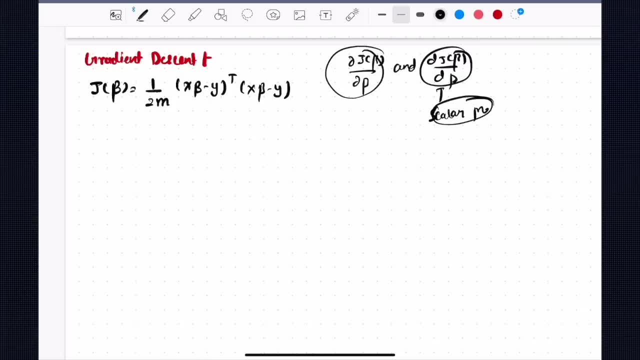 linear regression. but in this case, but in this case, but in this case um this particular thing, we have a vector program which we saw in a multi, multiple integration. but i just introduced you this into the first one so that you'll be comfortable with what exactly both mean: the exact. 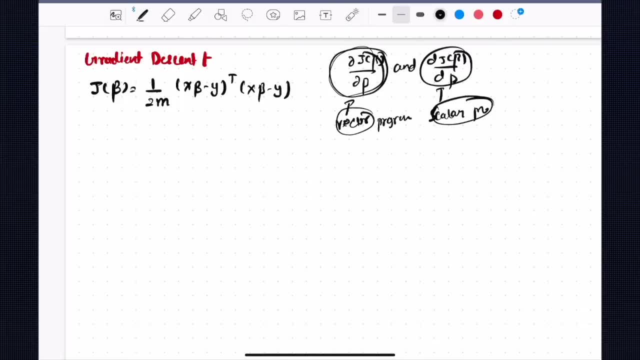 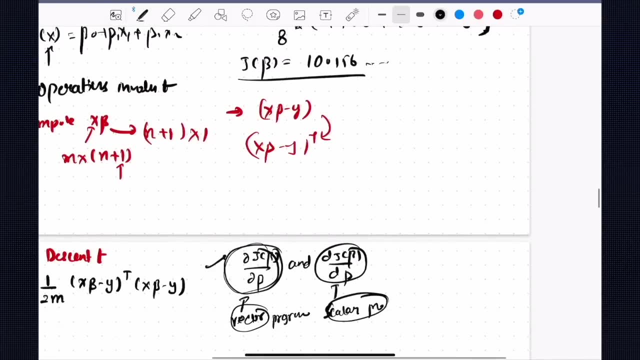 same thing, but this is for vector programs. this is for vector programs and this is for a scalar programs. so basically, uh, whenever you have, whenever you have, betas in vector, you actually use this, and then, when you have the same scalar, you actually use this. okay, so what? you do? so what? 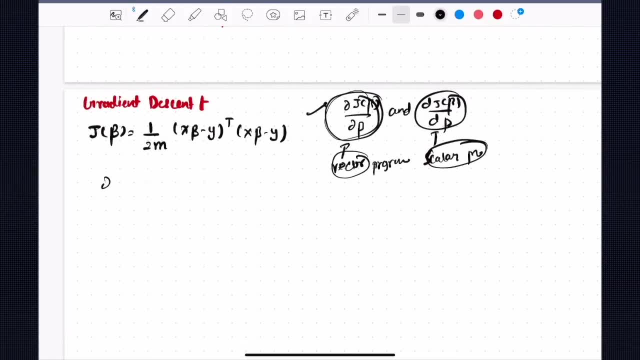 you do, you take out the you, you take the debt, you take the derivative part and you take the derivative partial derivative of g, of beta with respect to a particular beta, y. we take out and everything we have talked that it gives the rate of change, it gives about everything. the whole story of 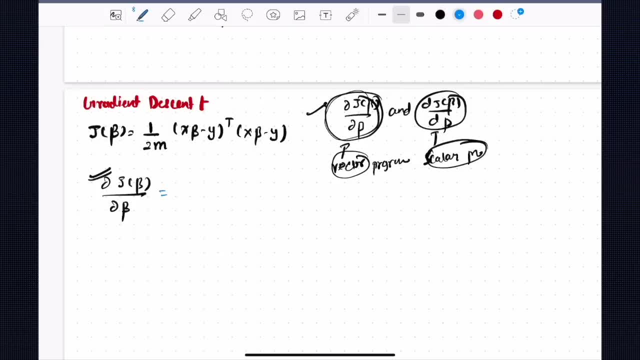 geometry we have already talked about. so you take the partial derivative of it so that you can identify the rate of change, how much the cost function is changing, where the beta is changing, so that when you take out the derivatives, which actually gives 1 by m, x, transpose x beta minus y. 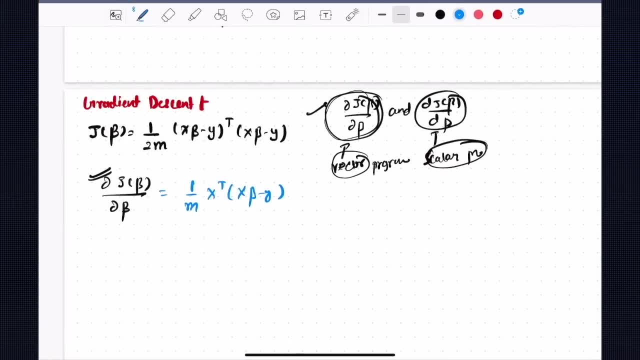 so when you actually take out the derivative- i'm not going to talk about the um- how can we derive it? it's not required, maybe for you. if you're not a character, i think you're going to have to do it with a student, but we, of course, have the reading materials for you to get started with it, okay, so 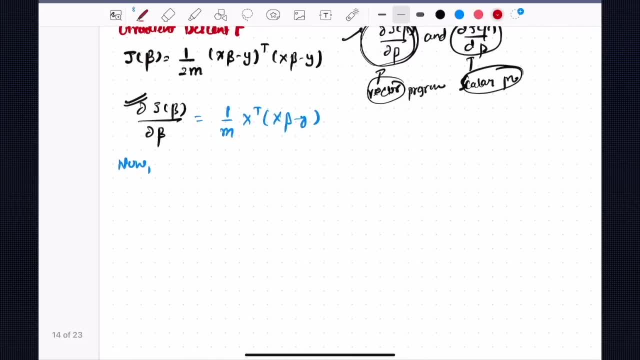 so what is? what is the gradient descent algorithm? so once we have the gradient once, once we have the gradient calculated out here what you can do, we have the algorithm following. so you go for i, for i in, uh for i in range number of iterations you wanna perform, you're gonna perform, you're gonna. 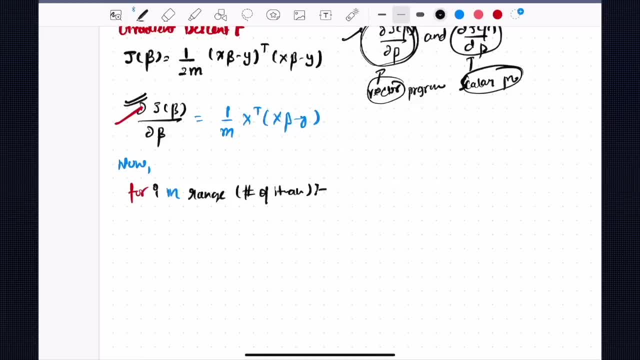 change the variable so that you so, so, so, so, so that you can converge them on a specific number of iterations. the beginning of the tutorial. you don't have to tell us what is, what is, what is, what does this mean and what does this mean, but you need to. 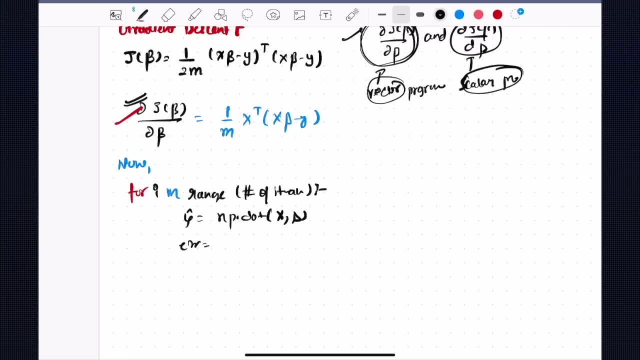 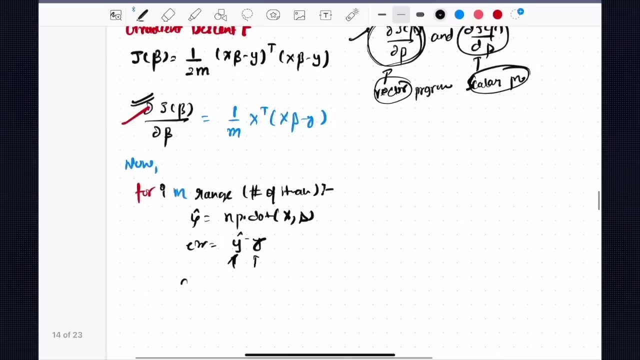 understand, you're able to tell what the gradientzahl Boltz rate is, because this area represents when, when you think about the screening point for the improvement of the model, we can see that we have a third and full run and we have salt probability of 3sini. that means this value pleased. 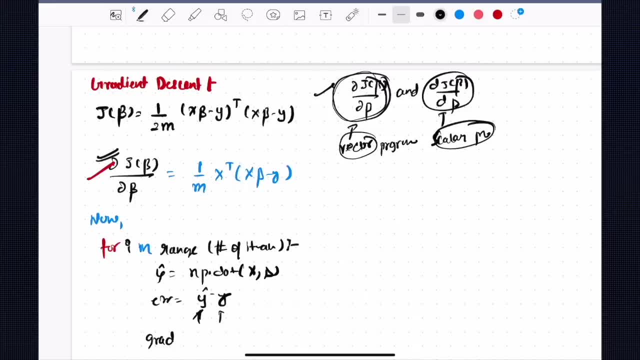 is this value? so what is this value? so if you plug in the two points here, sigma plus sessions, on the other side, we have the explicit parameter which is our derivative. then what is the gradient? extraordinarily, and all of this, we have right. so we have two of theseала, or we have any number of ordered ones, which is the diagonal and the retailers. we take out first of all the hypothesis. find you using hypothesis function. 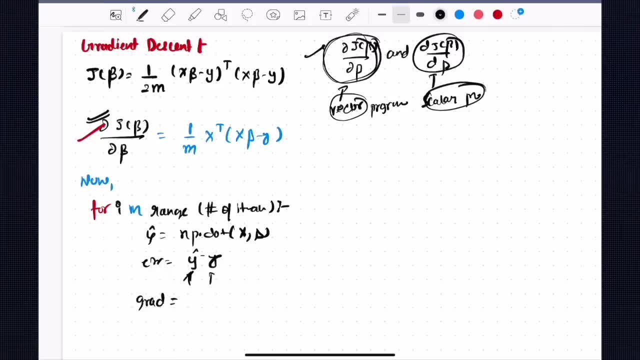 point which tells us how much, how much change we are getting in a cost function if they change the beta a little bit, which which, which was nothing but which we have derived, which is nothing but 1 by m times the doctor, between the dot product, between your, your pure. so, basically, this is the 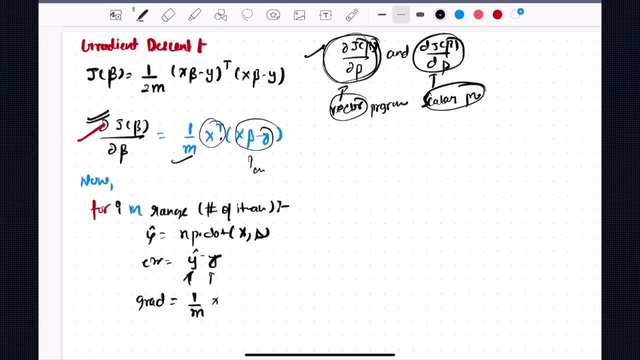 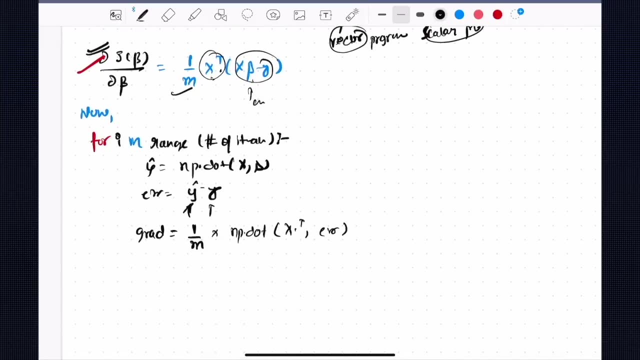 dot product. between the error- this is the error and it's the transpose stake of the dot product- between the transpose of your x, which is this, and the error, which is this. so just simply multiply, okay, yeah, now, once you have the error, once you have once, once we have that, once we have. 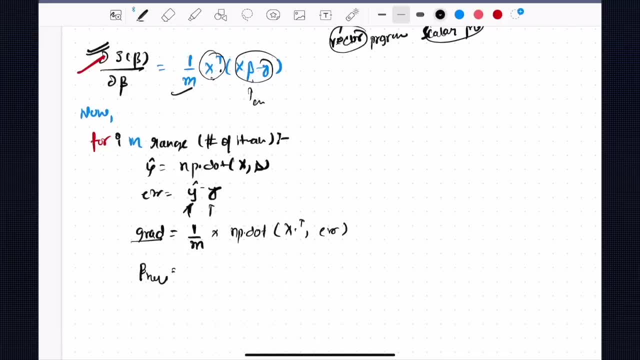 the gradient, we can actually use the update rule, so your beta nu will contain beta old minus the learning rate alpha, which is nothing but learning rate alpha, multiplied by the gradient. multiply with a gradient which is out here right. this is the derivative, which is nothing but a. 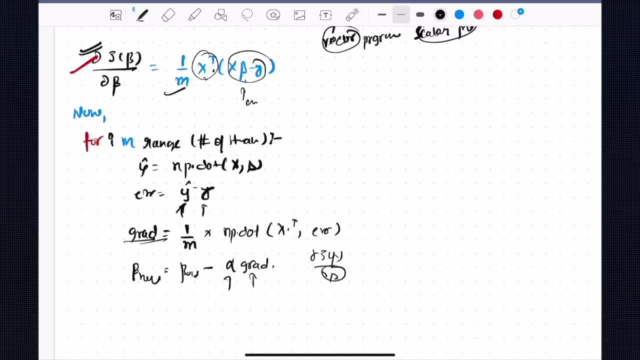 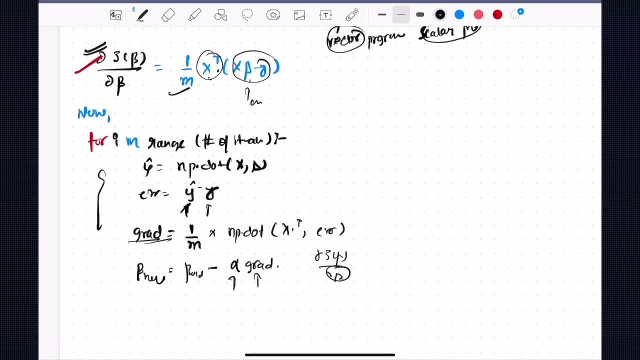 partial debt derivative cost function with respect to particular, uh, very even. okay. so i hope that this, this is the algorithm which is for multiple linear regression. let's try to do one thing. let's try to solve. solve a very simple example of using a gradient descent. okay so, 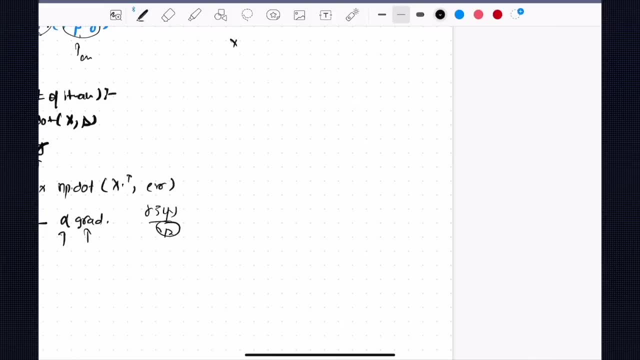 assume that I'm going to take a very simple data set which is X, 1, X, 2 and Y, which is 1, 2, 2, 3, 3 and 4.5. so, based on this, on a predictor variable, Y, so your design matrix will conclude: f: 1, 1- okay, because that this is important- X, 0 and. 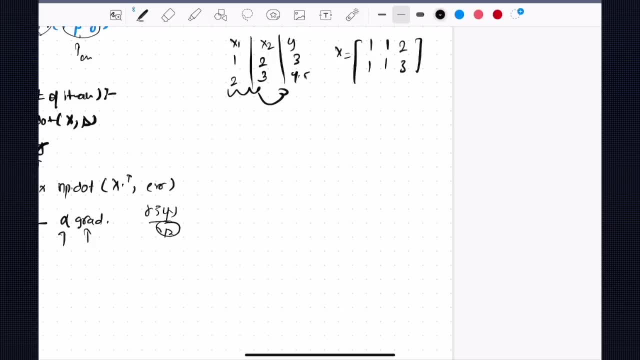 then a 1, 2 and 2 and 3. this is a design matrix. this is a design matrix, okay. and then you have a output ground truth vector which is 3 and 4.5, and then you have parameter vector which is 0, and then you have beat 0, 0. so beta, 0, beta 1. 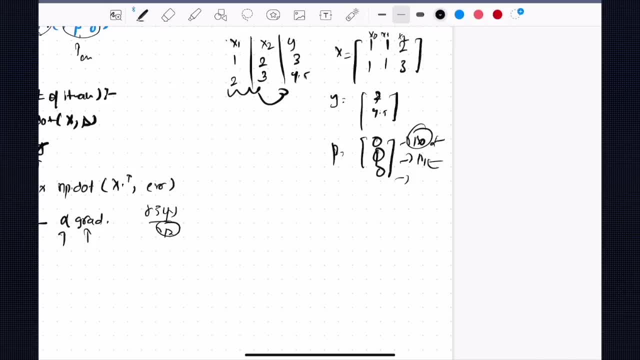 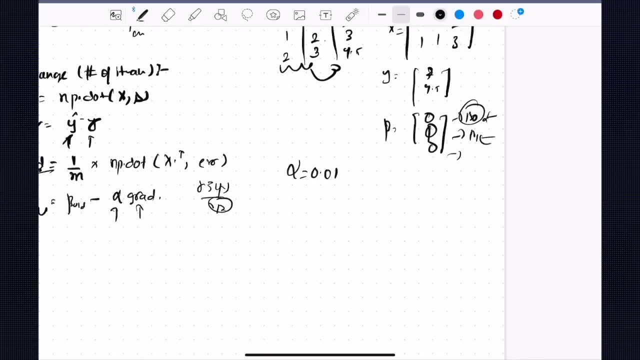 and beta 2, beta 0, as it for for biased on beta 1 is the parameter of X 1 and we are doing the parameter of x2. okay, assume that your learning rate alpha is 0.01. and then now what you do? now you compute the gradient. so now what to? 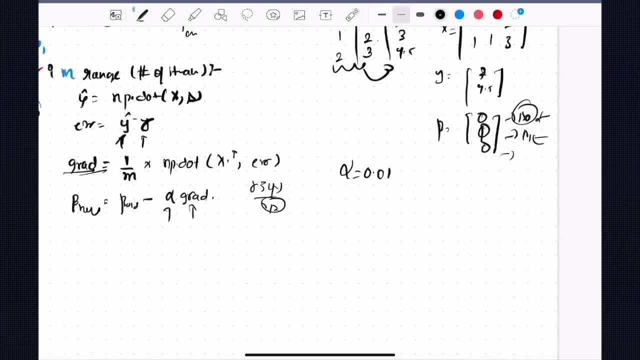 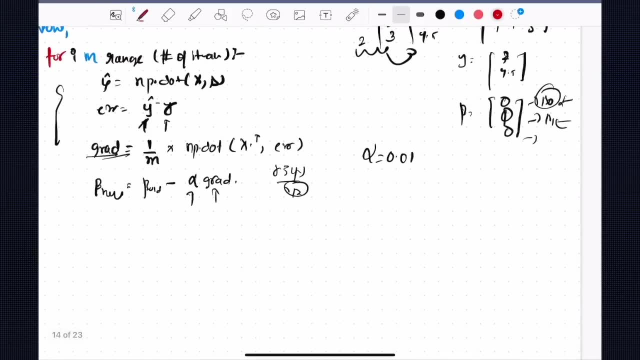 know, know, because. but before that, what you do, but before that what you do. you compute the you you write, you run this algorithm. the first step in this I've been been run running this algorithm gonna calculate your y hat and the calculator y hat, which is nothing but X, beta, is nothing but 0, 0. okay, you calculate it. I. 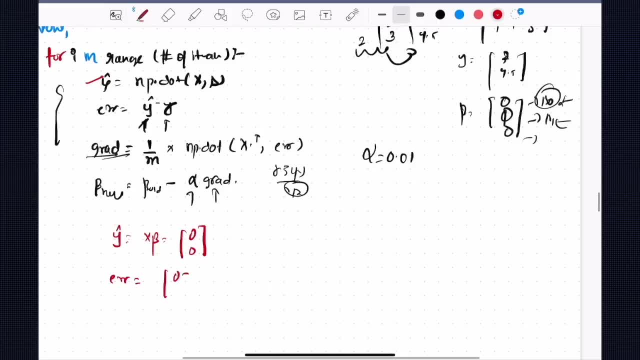 calculate the error, which is nothing but over there, which is nothing but your: 0 minus 3, and 0 minus 4.5, which is nothing but minus 3, n minus 4.5, which is nothing but this is anything but the error, that difference. now, once you have the, 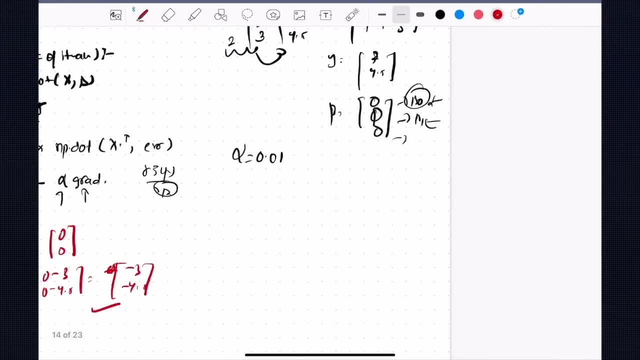 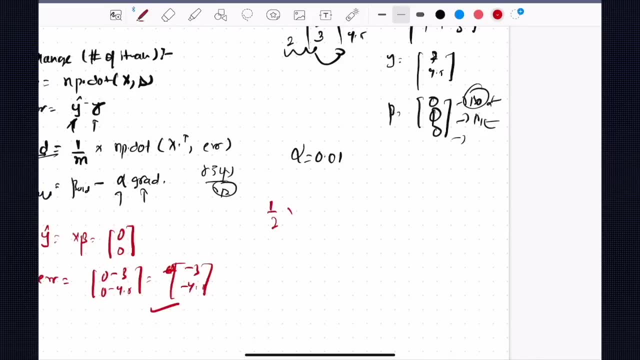 difference. you calculate the gradient at that particular point. when I calculate the gradient in that particular point, which is nothing but 1 by 2, 1 by 2, which is over here, MS goes for 2. that's why 1 by 2 multiplied by your, your dot product. 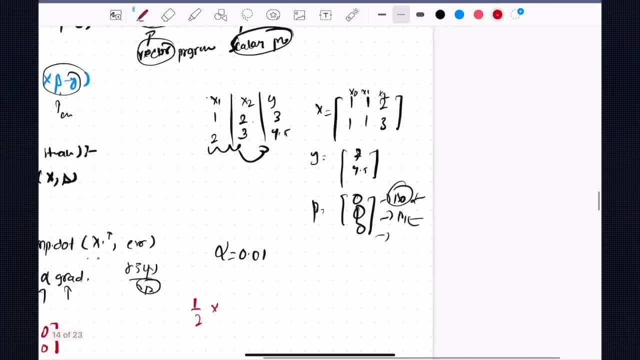 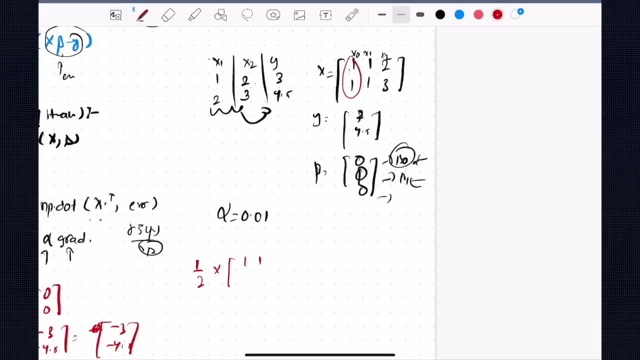 between your X transpose the design matrix and the error. the doctor, between the design matrix, which is the design matrix over here, is 1, 1, okay, which is 1 once you attempt to transpose of it to the 1: 1, 12 Chalmong 7. 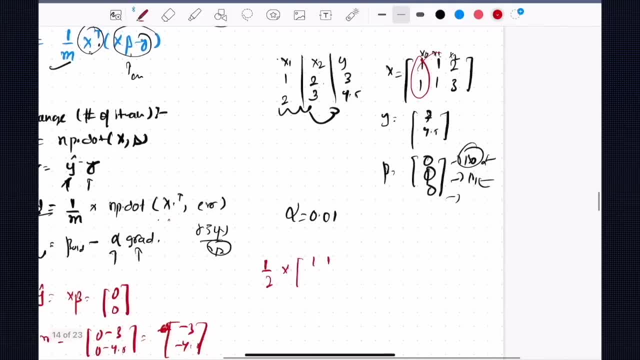 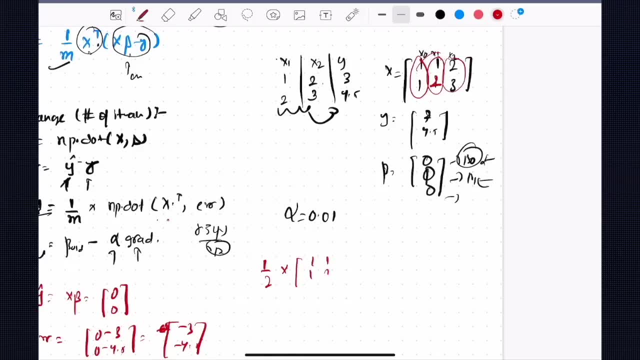 two. sorry, sorry, i guess i did a bit wrong over here. it should be one: two. okay, so one two and two three. okay, so one one, one two and two three. so when you take out a transpose of this particular matrix, you'll get this multiplied by, multiplied by oops. 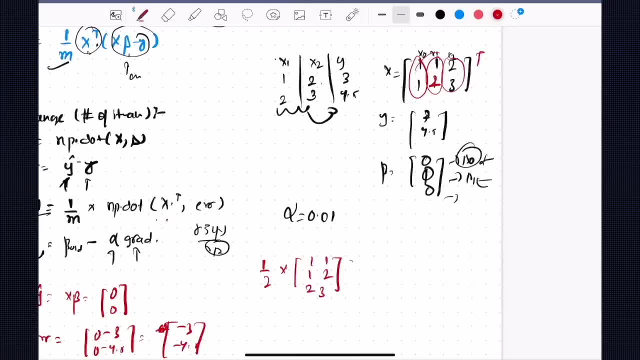 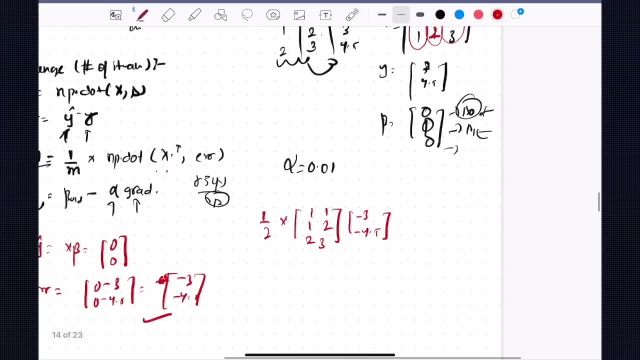 multiplied by your uh, error, error or difference vector, just this. okay, so when you calculate the gradient, you calculate the gradient you will end up being with. you'll end up being with uh, this particular variable, which is nothing, but you'll have c, c, c. let us assume that you have. 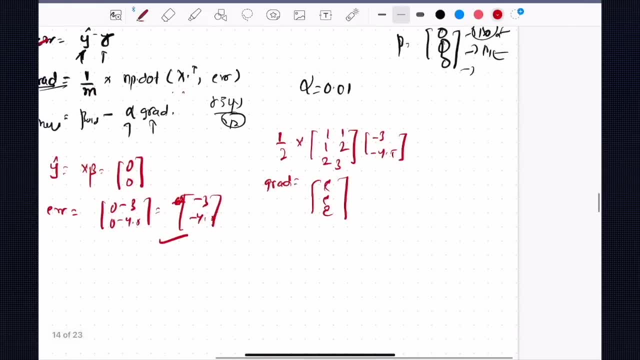 gradient. now what you do? you have a gradient, so when you actually work on it, when you actually work on it. so this is the new set of betas. now you come to the gradient here. this is a good this: when, even when you solve for it, you'll, you'll, you'll. autumn automatically get it, okay, you'll. 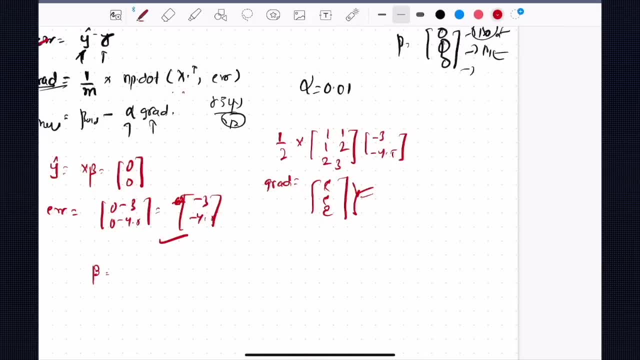 automatically get it just when you solve for it. okay, so you get all the values and you solve for it, and then you have the new beta is equals to old beta, minus learnings and grad. okay, this, this particular grad, and is also a vector. okay, so your new beta will be a vector, which is a three elements which: 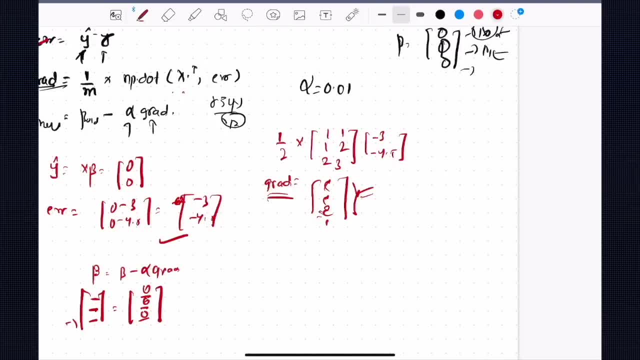 old beta is also three, zero, zero, zero, okay, minus 0.01, multiplied by your vector. multiplied by your vector, which is the c1, which is c2 and c3. in this case, if we exactly want to focus on exact numbers, this will be nothing but. 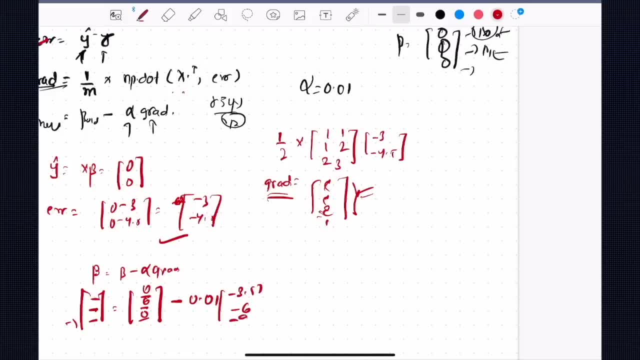 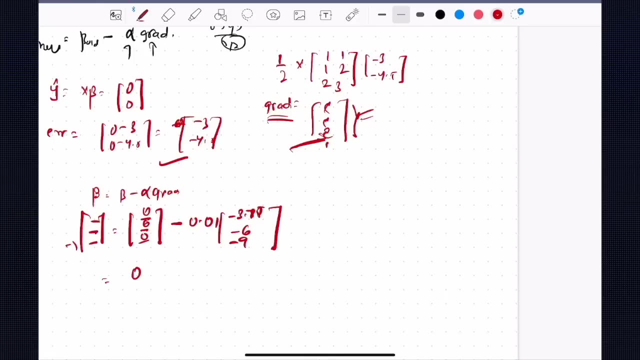 minus 3.75 minus 6 and minus 9. okay, so this is the basically, uh, the, the, the c will, when you calculate, will come out which is nothing but your new set of betas. new set of betas will be 0, 0, 0 minus 0.01 times minus 3.75 minus 0.01. 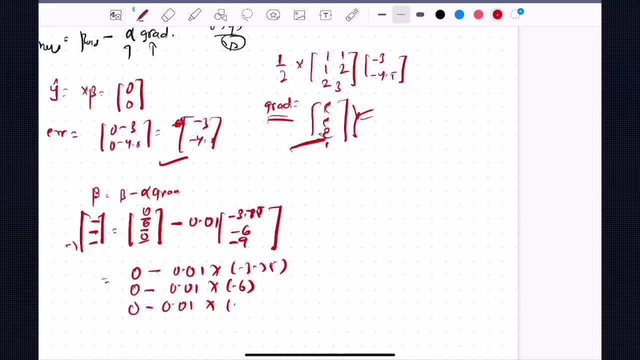 times minus 6, minus 0.01, multiplied by minus 9, so you have this one and then you actually calculate this: 0.0375, 0.06 and then 0.09. so this is your new set of vector after first iteration. okay, and this is the first situation. now you 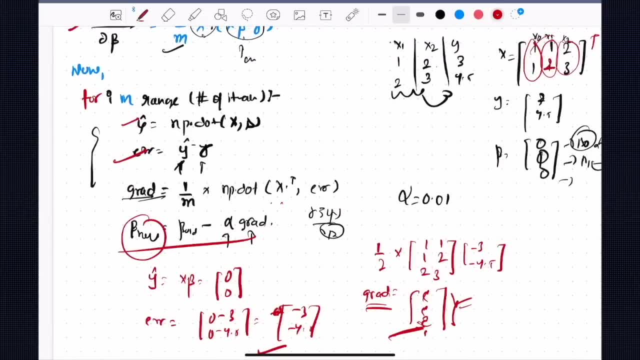 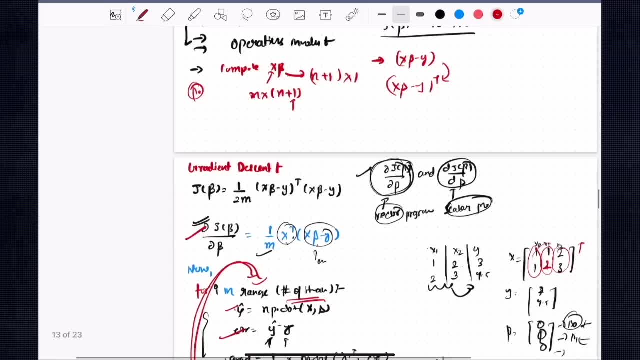 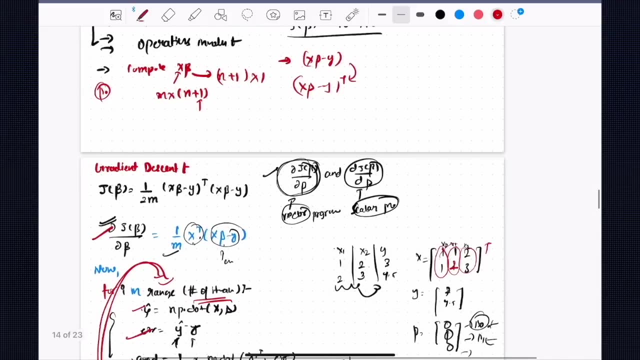 reached. i hope that this gives a good sense about how exactly we work through and um, for geometrical perspective. we have already talked a lot cool um, so i'm just trying to make sure that you have every worked example into your hand so that it's much more better for you to understand it. next, what you? next, we are done with mostly um. 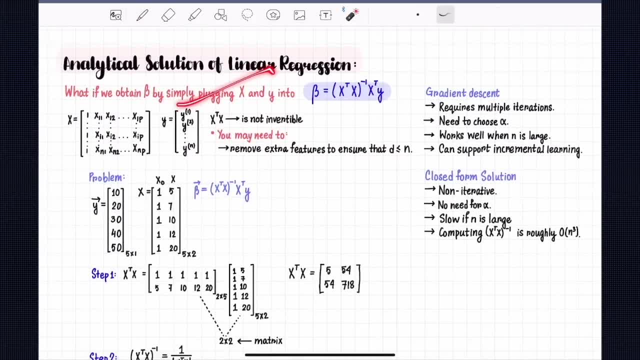 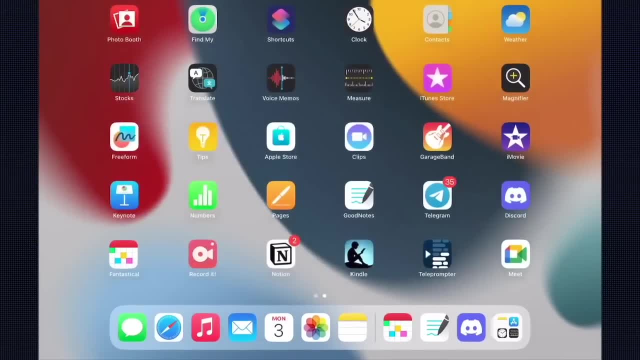 this. we'll talk about a bit about analytical solution of linear regression, and then we'll talk about how can we evaluate our model, uh, specifically, and then after that we have a lot of things there, so let me just go there. so, after the calculation, we'll talk about the. 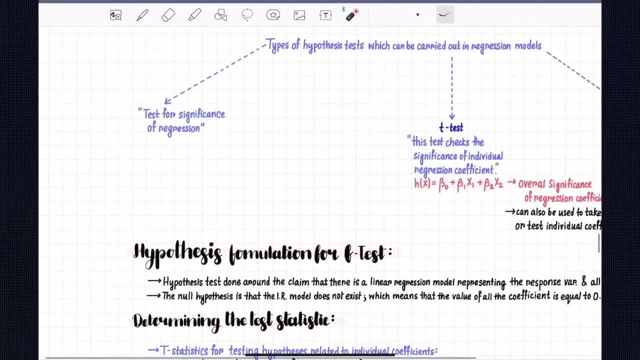 hypothesis testing, which is one of the most important thing over here, which is the how can we test our model, the significance and everything. and then we go to the next step, which is nothing but actually talk about assumptions of the model, and then we'll do one project and then wrap up. 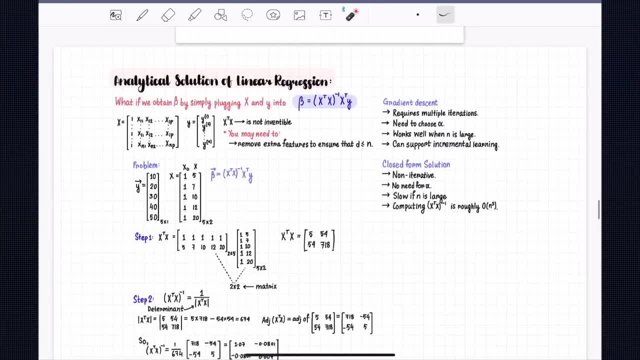 this course. in this video, what i- what exactly i'm going to do is talk about something- was analytical solution of linear regression. so, basically, what exactly we'll talk about the and what exactly we will talk about in the analytical solution of linear regression is: you have direct 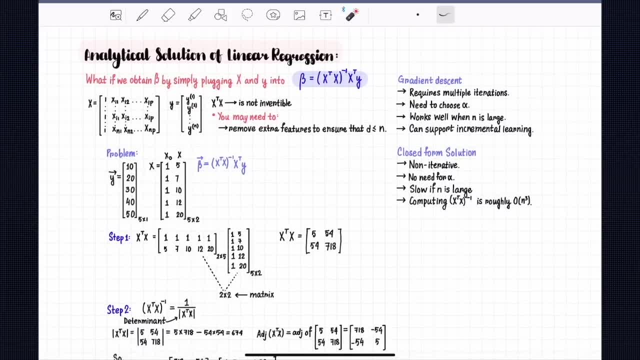 formula. you have direct formula for taking out your beta values by putting your x and y's into it. so how this is derived and everything, i'll be linking a very nice resources in this particular reading section of this, or you or you can see in the resources section for this particular lecture. 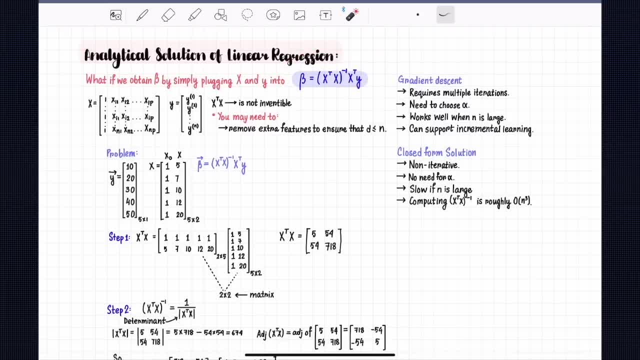 i'll, i'll, i'll give you how do we derive this formula, but it's pretty easy. if you get to it, you'll have the assignments as well for on it. so basically, uh, we have the direct formula when we plug in the values of x and y and then we get our output variable y, sorry, our betas, right. so we have. 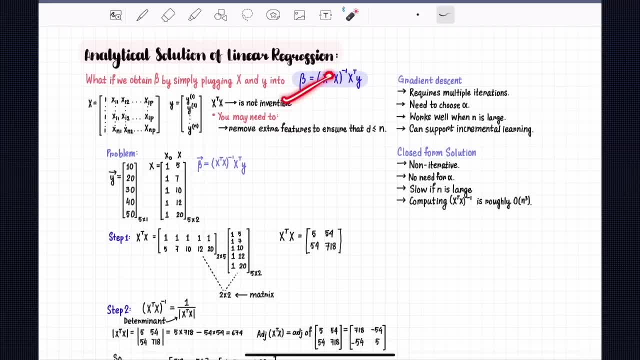 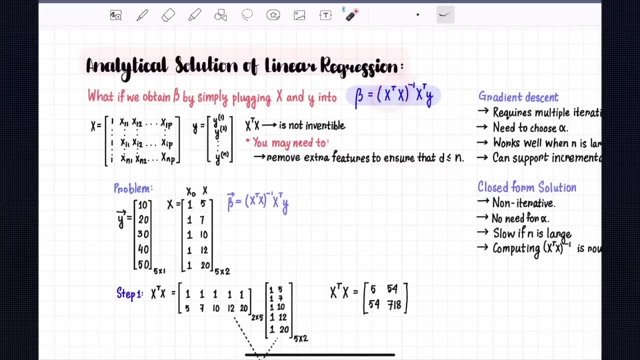 optimized beta, which is converged beta, which is the best beta, right? so there's a direct formula, which is which we call an analytical solution. that so basically, uh, so basically, the formula is x transpose x, then we take the inverse, multiply it with x transpose y. so so let's talk about, let's. 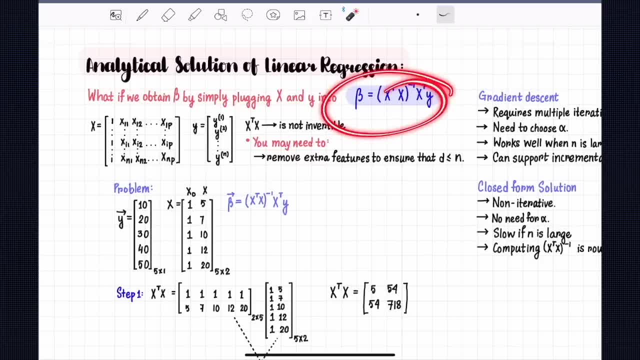 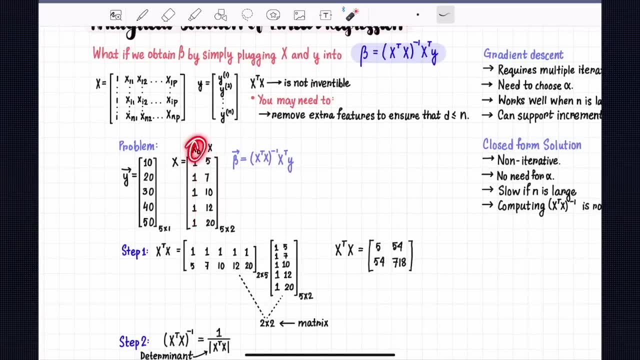 let's talk about um and let's try, let's talk about by taking one particular example. so assume that this is a particular example. you have one, one, one, one x zero, and then you have one independent feature and one uh x zero, which is nothing but four beta zero, and then you have out, and then you 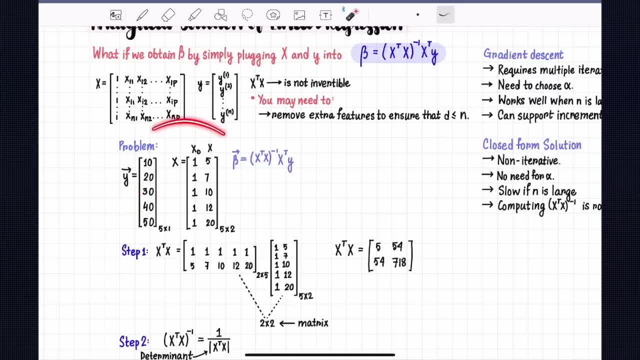 have a variable, uh, which is y, which is a ground truth over here. now we utilize both of them to actually take out the analytic, to take out the beta's values, right? so basically, the first step is to calculate the x transpose x, x transpose x. so when you take out the sodium, take out the. 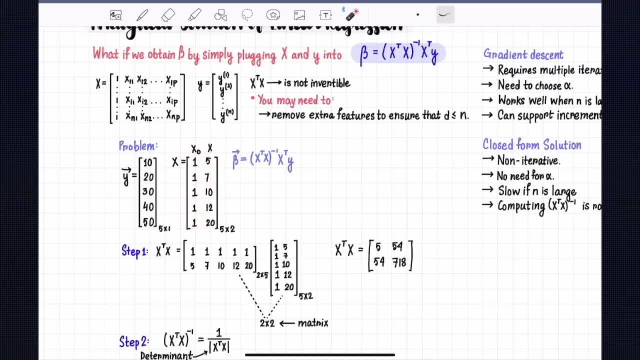 transpose of this. so this column, this column becomes the row and row becomes the column. so basically, one, one, one and five, seven, two, zero, and then you have the particular matrix out here, which is two. uh, two by five matrix, multiplied by five by two, that will yield to two by two matrix. so 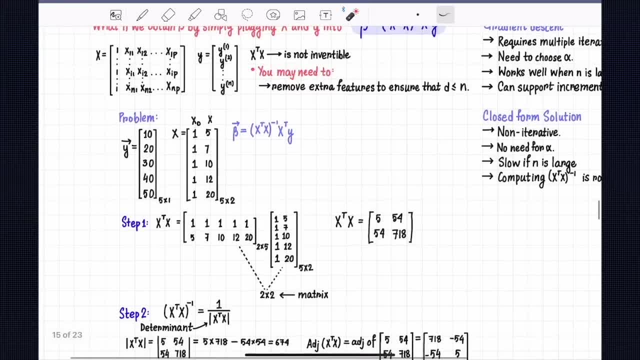 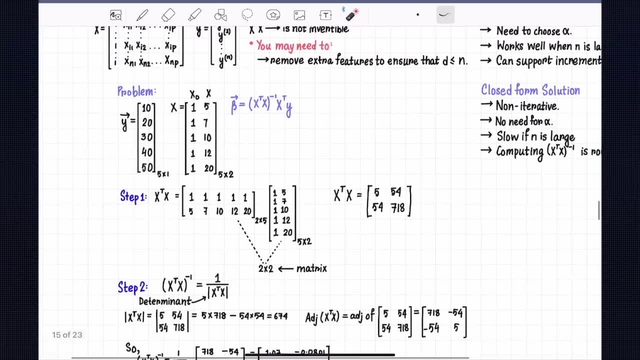 which is nothing but this one. okay, now the next step, what you do is take out the inverse of it. so what is the inverse of it? inverse, or any particular thing, is one by this, okay, one with the determinant of the inner value, which is one by determinant. and when you take out the determinant, 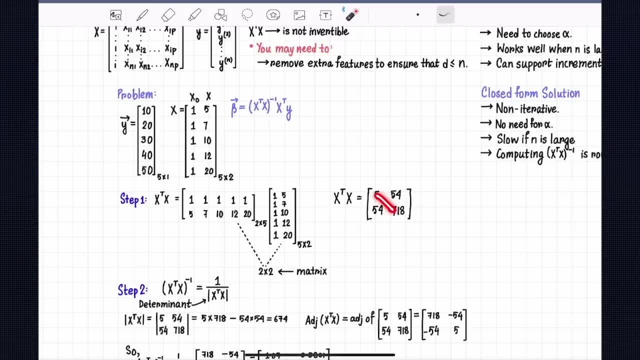 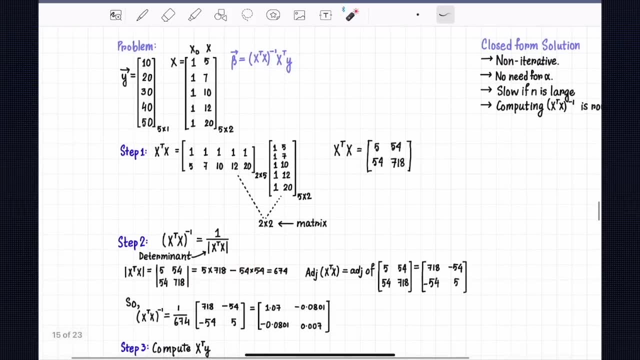 of this particular, which is nothing but uh, which is nothing, multiplied by this minus multiple, minus uh, 54 times 54. so this is a determinant, this which is not not nothing but the area under a parallelogram. we have already talked about the terminal, everything in great detail. please see the. 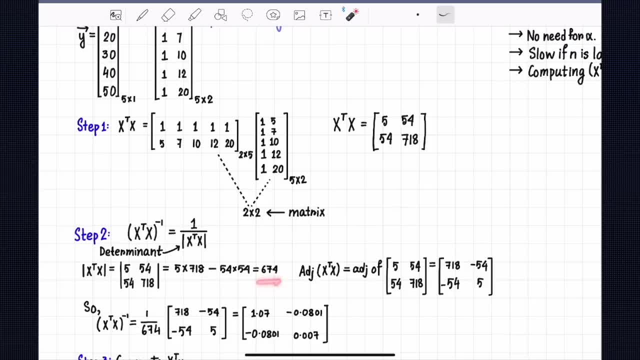 lectures. so when you take out a determinant, you will have 674, and then what you do? you take out the aggregate of that and then, and then you take out the aggregate of that. so as you get of, that would be nothing but, uh, this one, this particular matrix, and then you multiply with one by this: 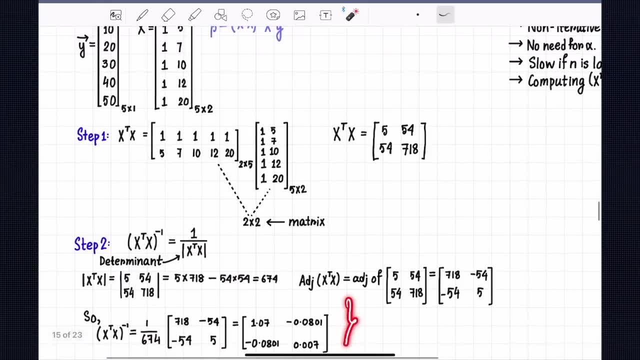 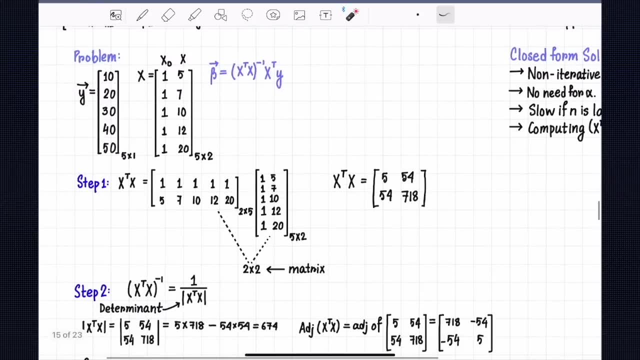 with the, the azure gate matrix, where you will get the, your inverse of a particular matrix. now, once you have the inverse of a particular matrix, now what you do? you compute. you compute x, transpose y. which is this one? you now, we compute x, transpose y, you'll get this particular. 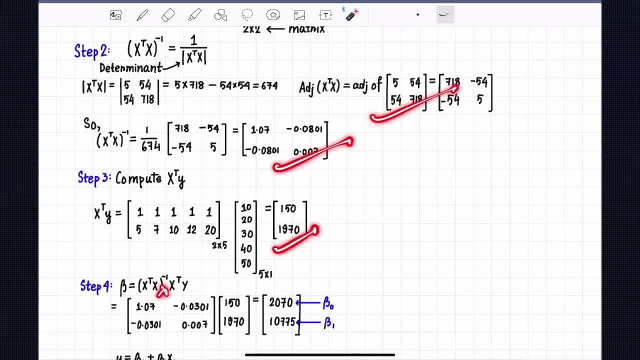 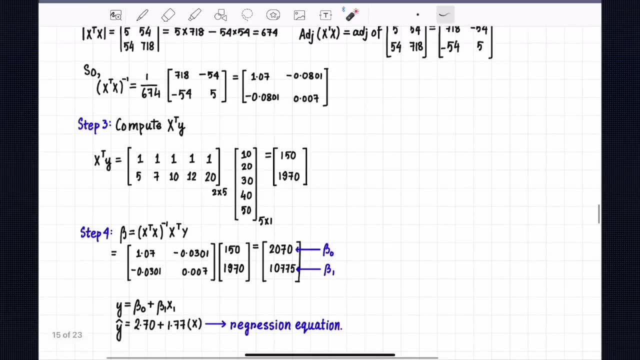 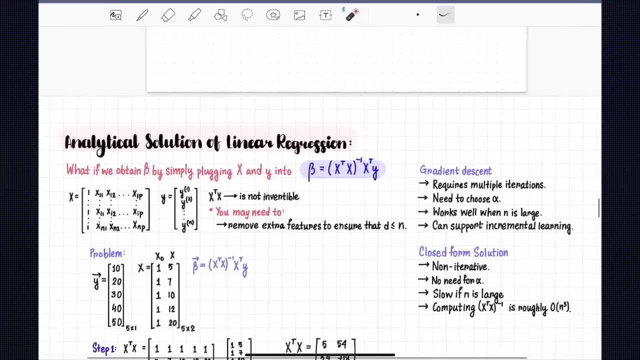 thing and then finally multiply this particular matrix, this particular matrix and this particular vector by forward, getting beta 0 and beta 1, and that's the required beta 0 and beta 1, which is your regression equation. okay, i hope that this makes much more sense. uh, now, uh, so, as the as this: 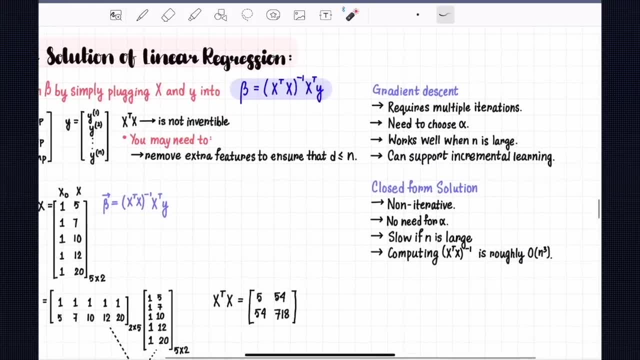 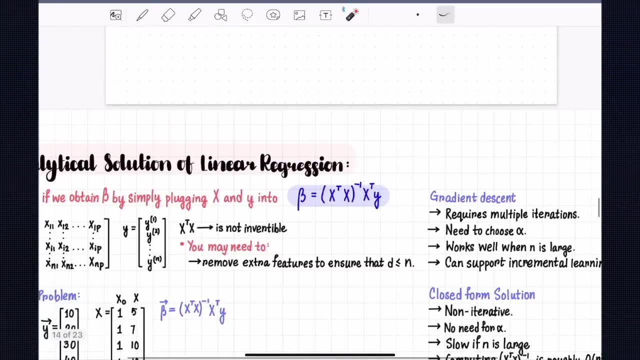 was very simple example, uh, for the calculation of this, but i actually want you to just don't uh remember how to how exactly do this? this is something which is, uh, softwares are made to do it for you, so you don't need to worry about this. what you need to. 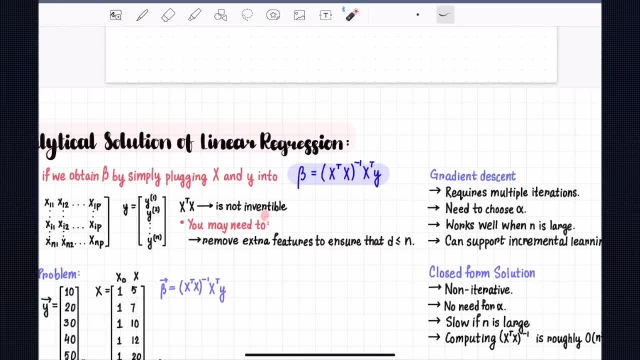 worry about is, uh, uh, is this particular thing like what? what exactly this test tells is. here we have the formula which directly gives our beta values. okay, uh, if this, if this is not, if you, if your, this matrix is not invertible- invertible is it cannot be inverted- then you. 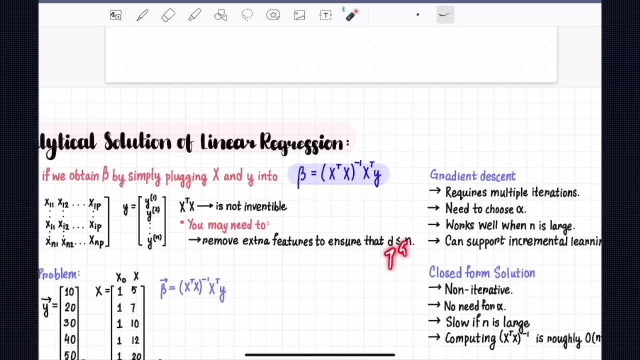 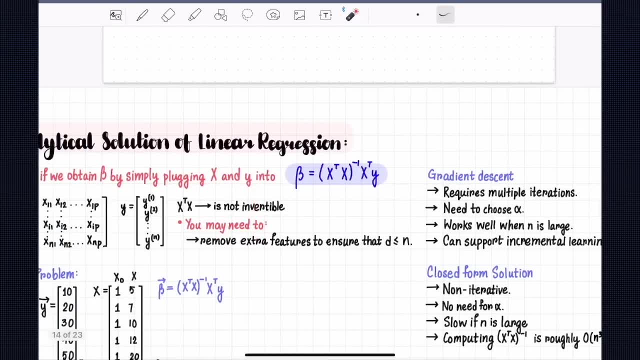 need to remove the extra features to ensure that your d is smaller than r equals to n, so your, the number of features is less okay. so, uh, this is a very general, general thing which you need to know, but, uh, but let's talk about what is the difference between this. this is important. this is usually 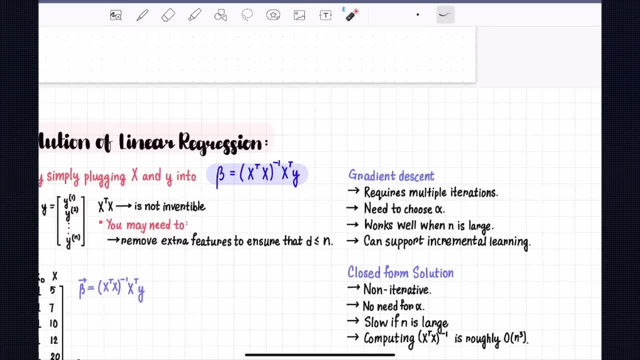 asked in interviews what are the difference between gradient descent and closed form solutions? gradient descent requires multiple iterations. okay, so we have one iteration second, and it requires time and you need to choose the alpha value as well, and it extremely works well when you have, when you have, a large number of features. it is not. it does not works well when. 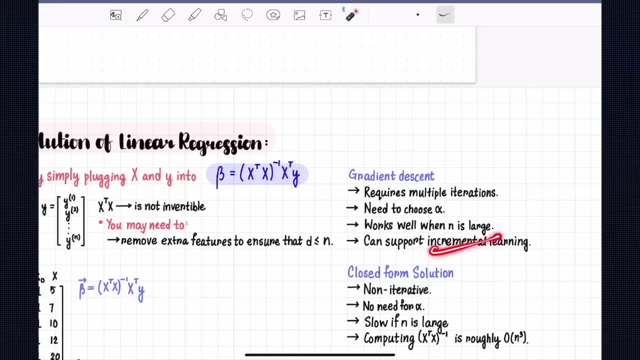 you have a large number of features. okay, it supports the incremental learning. it supports the incremental learning. okay, it is a non. the enclosed from it is non-iterative. it's just we plug in the values and then we get up values and then it's no need for alpha values. you don't need that. it is slow if n is large, if 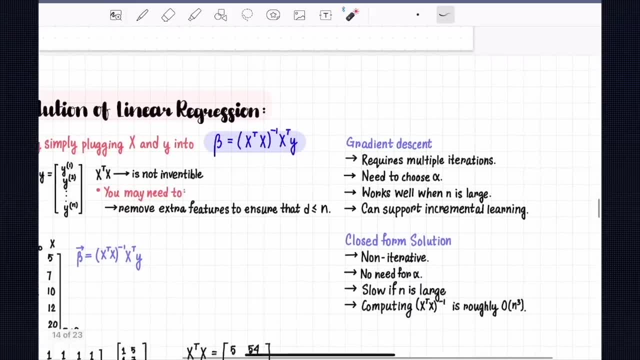 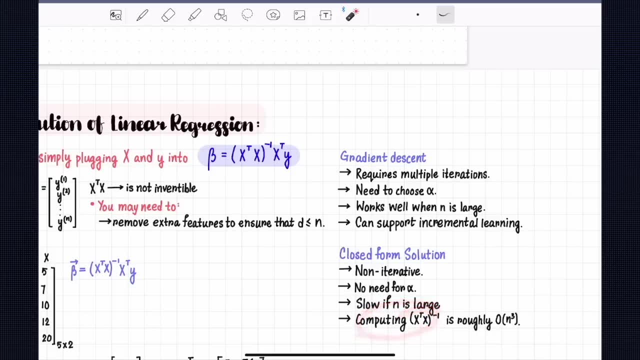 the number features large. it is slow because it'll compute all the operations, which is linear algebra operation, which is quite expensive. and then you have this particular thing, which is nothing, but you can: you compute x, transpose x, uh, which is roughly order of n, cube, which is extremely. 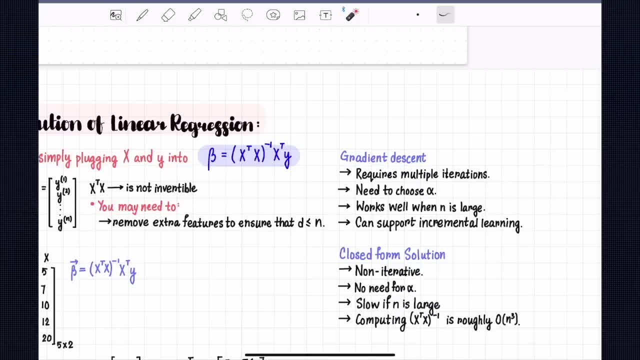 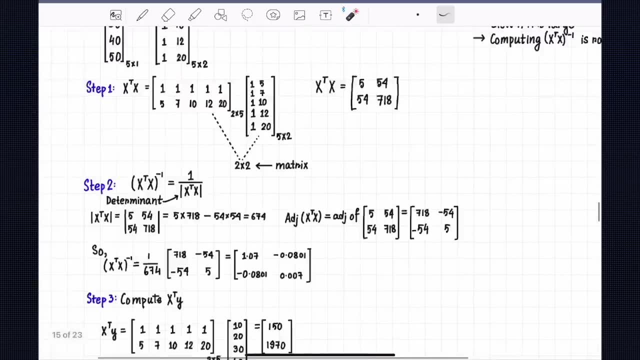 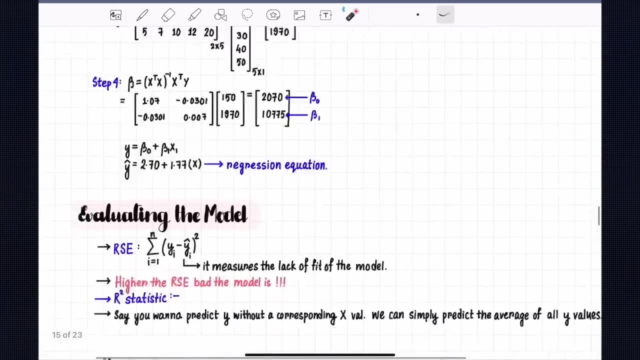 extremely time taking. so if your, if your data is small and is small, then i suggest to go close form. you know a large, then i support incremental learning, which is gradient descent. okay, i hope that this, this, this gives you a very great sense what exactly this analytical solution means. now. 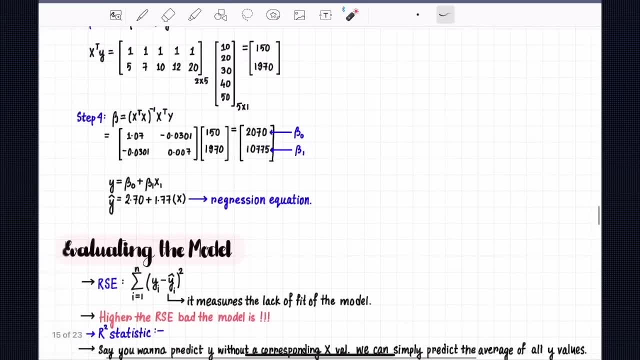 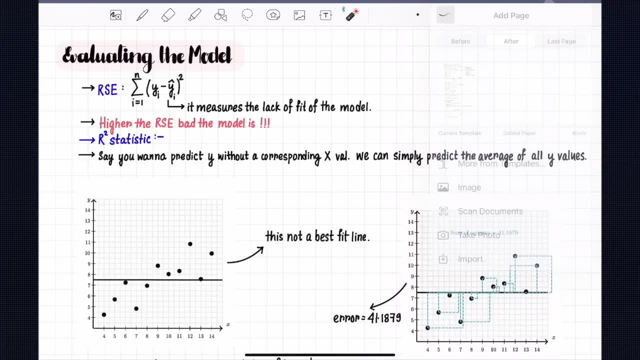 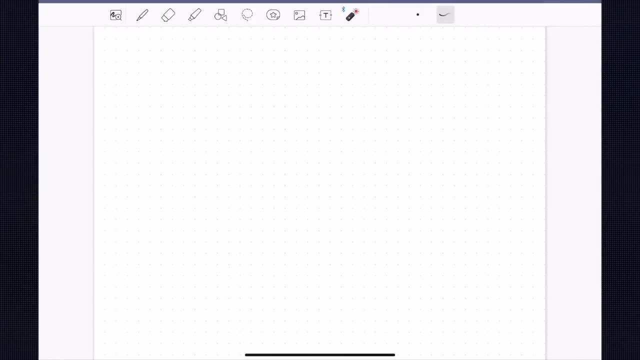 what we do now. what we'll do, we'll talk about how can we evaluate our machine learning model by going on to the next slide. so let me just make a template. let me let me just make a template. uh, over here so dotted paper, and over here what i'll do. i'll talk about some of the methods, how we 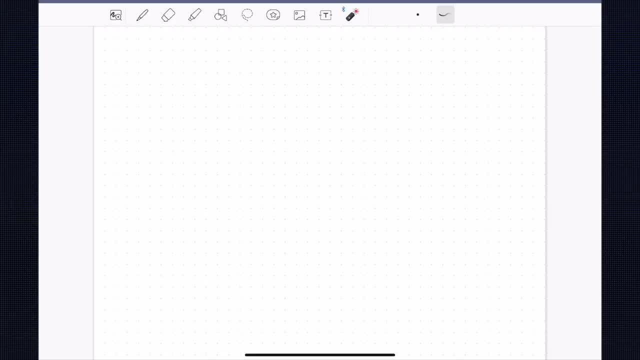 can eventually uh talk about how can we evaluate our machine learning model in a right way? okay, so, uh. so the first, this is the first measure, which we have already have seen earlier- is nothing but known as mean squared error. so the first measure for evaluating how well your model fits the data: 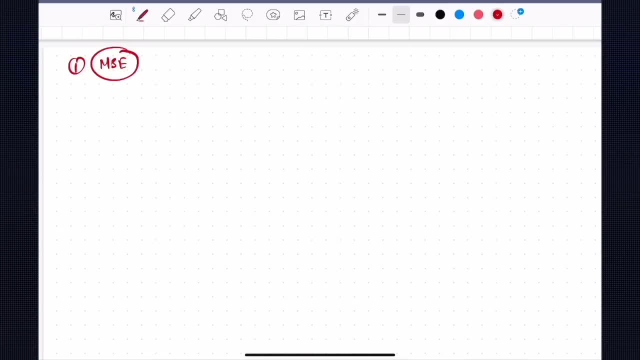 which is nothing but mean squared error. so what exactly mean squared error is is the average of the squared difference between the predicted value and the actual values of this subject. yes, this eats in all the higher second area, so that means the in higher second area here. the size of the question about how 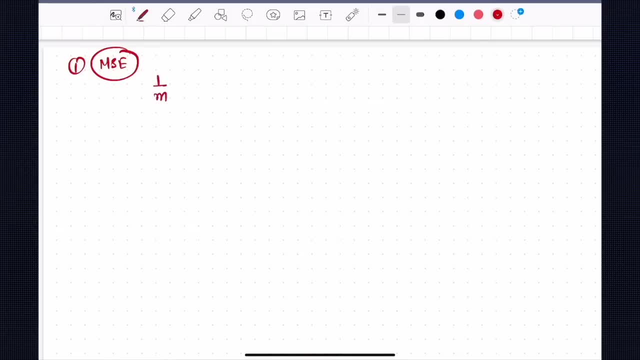 pleased is. the object right here is just the relation between the predicted value of part of the divided straight line, the thirdası function, and this, sorry, the third tissue, or the variable of the rated дет. atualizeienenofивается the impact of larger errors on overall errors. so 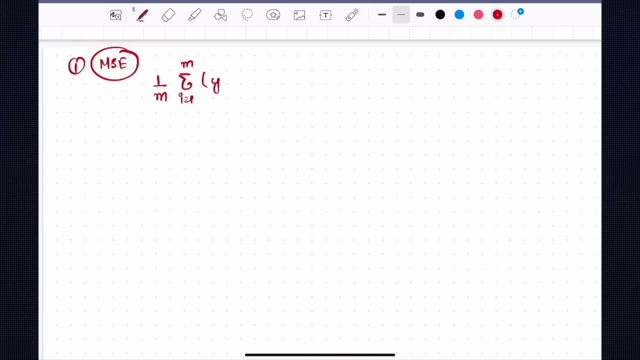 basically what exactly this justtells? you have the msc, which is nothing but one by m, some sometimes sorry. you take out moral prediction minus yi, which is minus your ground, truth and Square to remove the negative, to remove the negative sign once if, to remove the negative error, if there's any right. 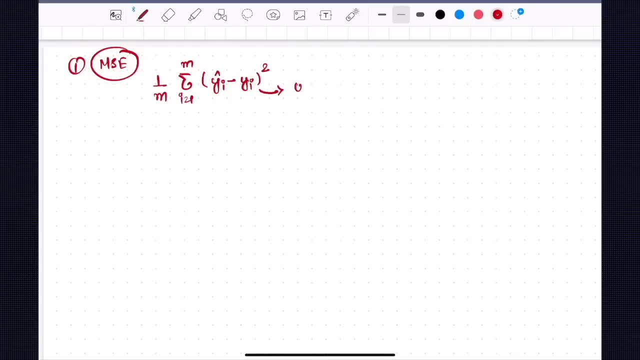 So, basically, what does it tell? what does it do? It gives you, it gives you, it gives you the The, the differences, overall differences, the overall differences, the overall, the overall differences, the overall differences In your model. but there's a one note to be taken out up, one note to be taken out here: 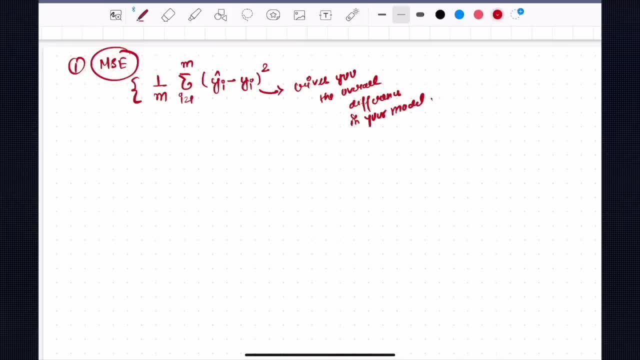 You see that we are taking mean. you see that you are taking mean. so mean is highly affected by outliers. So assume that you have a two, three, two point, five, six and then ninety, nine. You understand this. this can easily affect your MSE. How are you models for finding this? 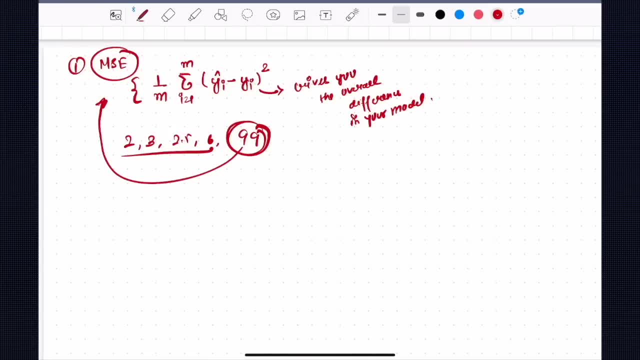 Only one example is it perform Very worse right. so over here your MSE will yield to very bad exam, to to a very misleading- You know, miss misleading error, because it is a. it is waiting eventually gonna mean and there's something giving us a misleading outcome, right. 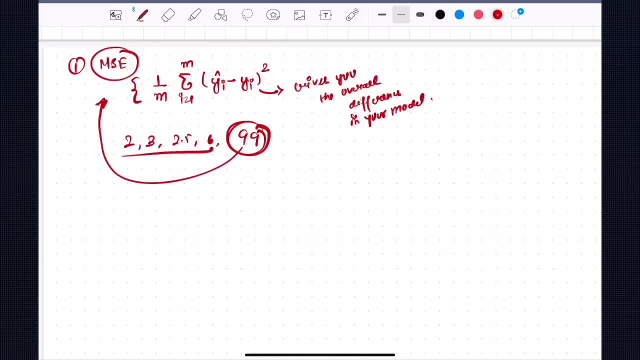 This is something which is to give a give, giving out the misleading outcome. So basically, we say that it emphasizes the impact of larger errors on the overall sense. so if you've got the if you, if you, if you, if you're getting the enlarge MSE, that means that it is not 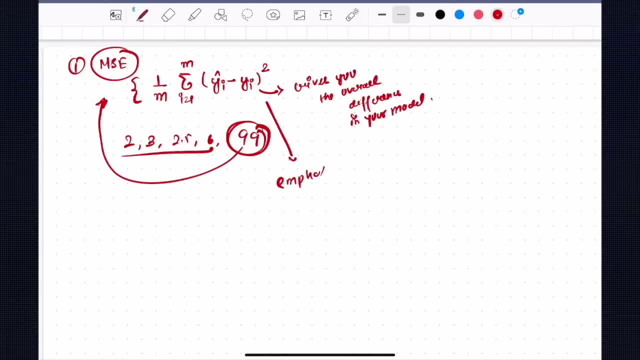 Something like every errors performing it emphasizes. it emphasizes what is emphasizes the impact of large errors. the impact of Large errors like this, like this, in overall sense, in overall, in overall sense. But I just told about it- MSE, those. that's one of them. Another one is: 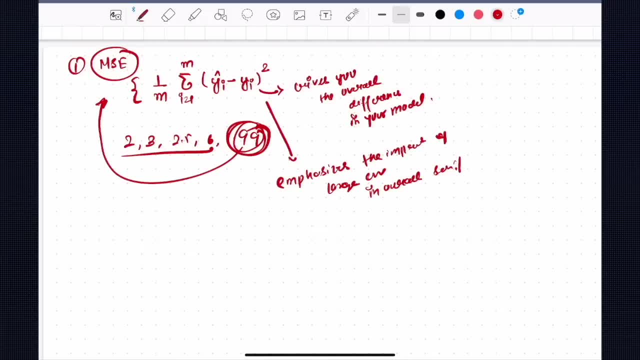 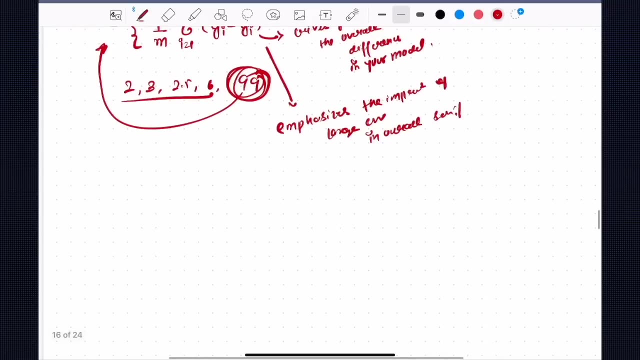 Another one is is about mean absolute error, mean absolute error, So it's the average of the magnitude of error and it measures the absolute difference between the predicted and the actual values. it Measures the average magnitude of errors in a set of predictions, without considering the direction. 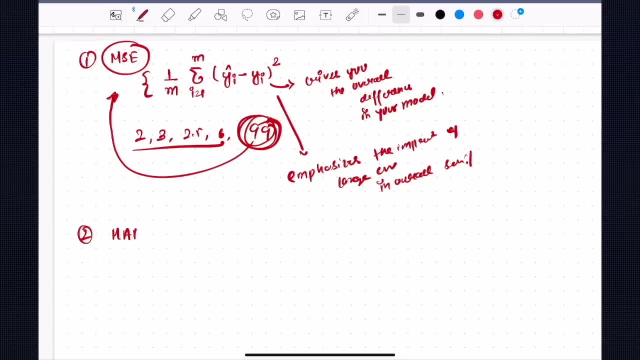 So, basically, so, basically. what is stress tells that you have mean absolute error, and what does it tells that the first of all, the formula for this is a nothing but 1 by M. I Is equal to 1, all the amount of the M. and take out absolute value of Y, I minus y. 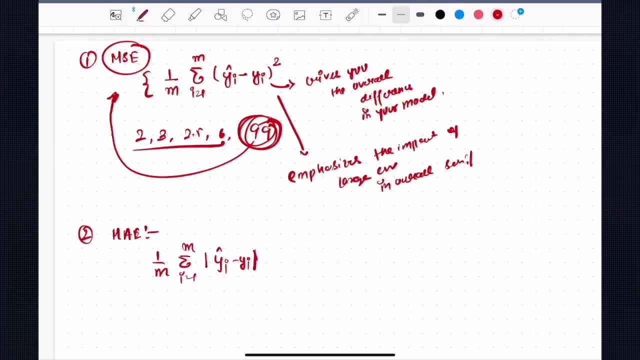 not squared over here. please note that we have that. we don't need to square. so basically, what? what? what we're doing? and rather than you doing a square to remove the negative sign, we're taking the absolute value and so that we get rid of negative terms. so basically, that means that if 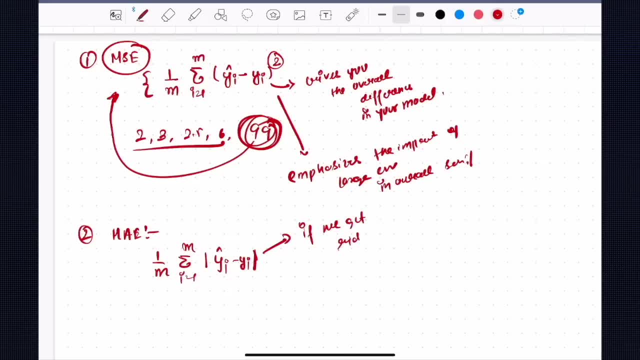 we get rid of negative terms, if we, if we get rid of negative terms, if we get rid of negative terms, what does it mean? it means that if you don't have, if you don't have any direction, it does not. if, while you take out this, then it does not have negative or positive reduction, it just says we. 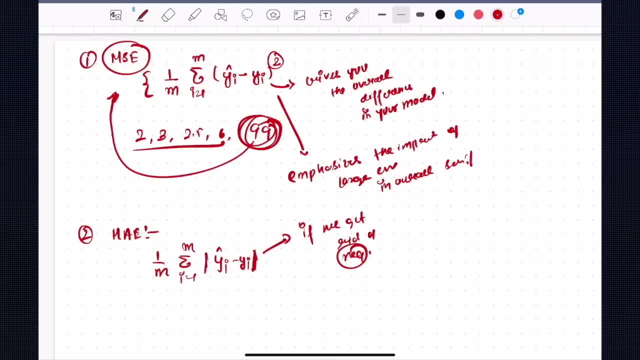 don't have direction. so if we get rid of negative direction, which also means that we get rid of the direction without the considering the factor of whether it is positive or negative, it does not focuses on that. okay, so it does not consider directions, but it takes the average of the. 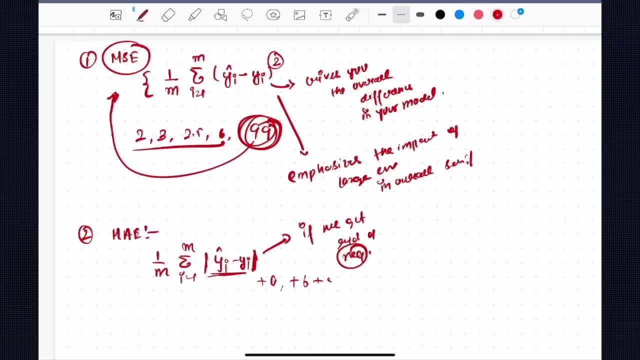 absolute. when you take the average, you'd be positive, positive b, positive c. take the average. okay, it is not taking on differences that consider that is going in other direction. it all in the like, consistent like it's. it's like we're not considering directions in this case, so that's. 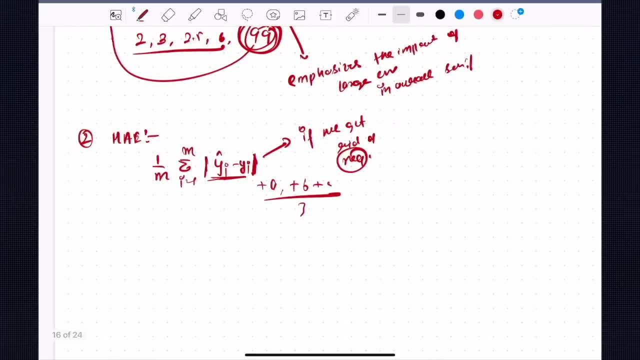 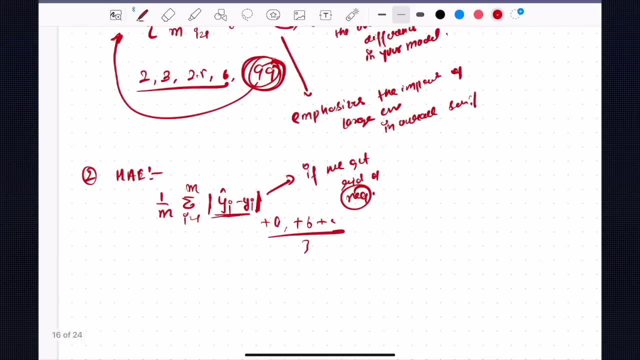 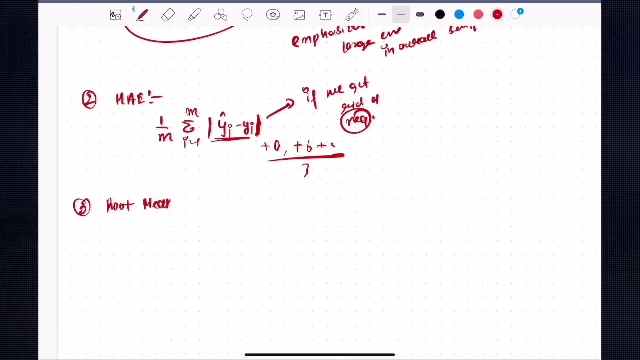 mean absolute error. that's one of the way we do think about it. okay, and that and another one which we have is nothing but called root, mean squared error, which is nothing but called root, mean squared error. so let me, let me just write: root mean mean squared error, or somewhere we call rmsc, so what? 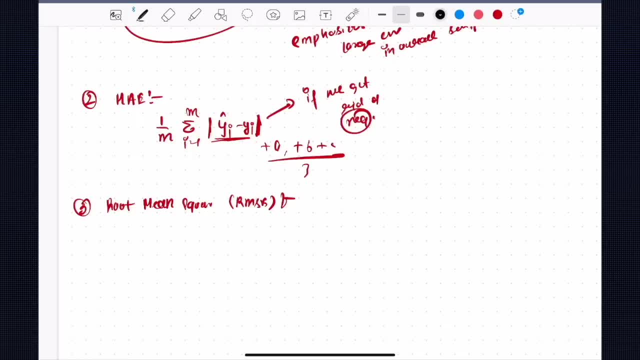 does rmsc means? this is a very important thing to talk on- rmsc is nothing but a square of your mean squared error, square root of your mean square. so when you take out the square root of mse, that will give you r? mse, which is root mean square error. okay, that is the square root of that. it has the same units as 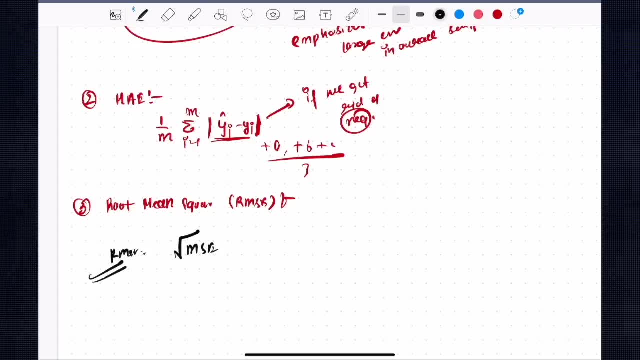 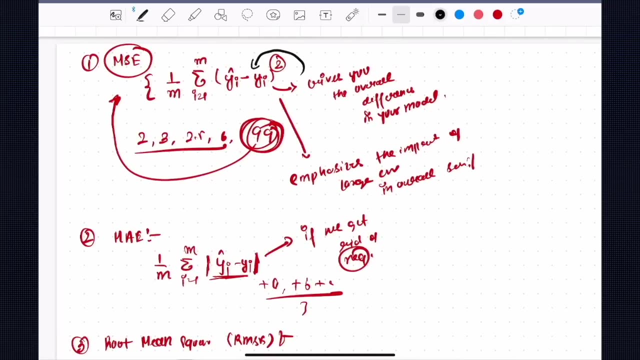 the dependent variable. so why does we um, why do we take out mse? because the units are same as the dependent target variable. that's why it is easier to interpret. you know some, sometimes we take out the m, mse because we want to come back at this format where it was. okay, you can understand in. 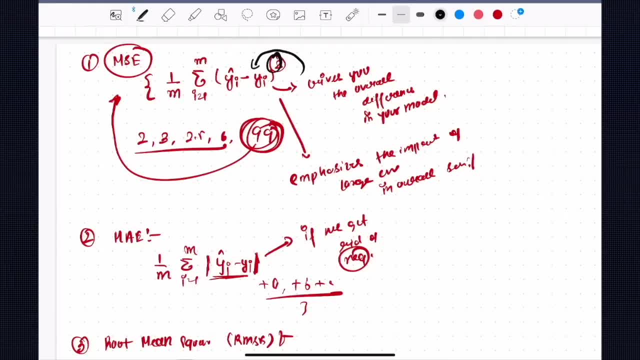 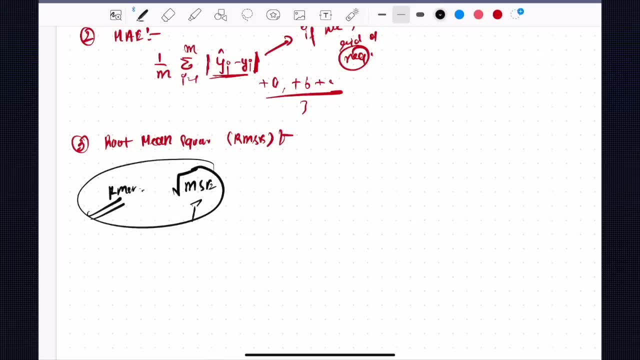 that way. here we squared it. no, we want to come back at where it was, without considering the negative sign. so here it tells you the it. it converts back to the units which was previously in. okay, cool though. so these are very small errors which i really want to talk on. uh, one of the 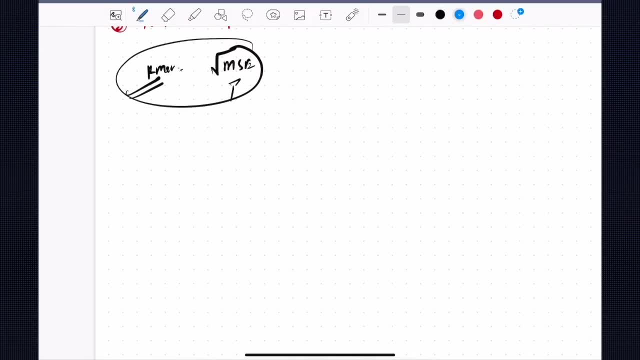 important and most important is nothing but called r, r squared error, r squared error, and in that we have sst, which is, uh, which is total sum of squares, and residual sum of squares, which we'll talk about. that today. okay, cool. so let's talk about these. 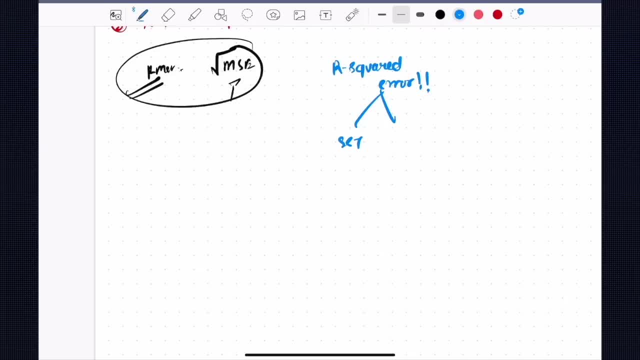 both in great detail so that, um, you have a very nice understanding of what exactly you need to do. okay, cool. so, um, let me just start off with one example. so let's say, let's consider a very simple example to illustrate the, the, the, the, the r squared error. so assume that you have a data set with one independent feature, okay, and one. 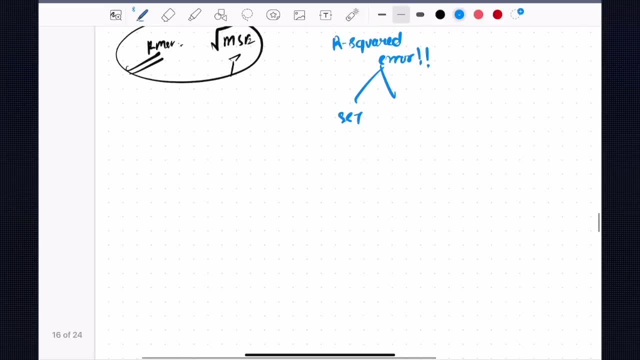 dependent feature. okay, so let's consider your, the, the index number, the observation number, which is observation number, is one. so we have x, which is the index, which is one, and y, which is also, which is the target, which is three. okay, so two, two, five, and then you have three, three, seven and four, four. 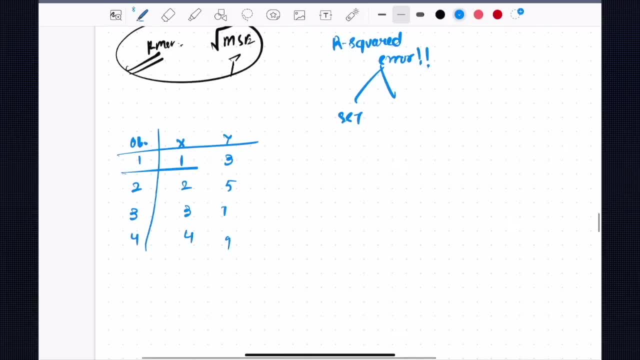 nine. so you have the index number, the, the obs, the observation number, the observation number, and then you have, and then you have the independent feature and the dependent feature. so basically, you're going to map a function x to the output variable y. okay, so now. so now you built a linear regression model on top of it. uh, when you 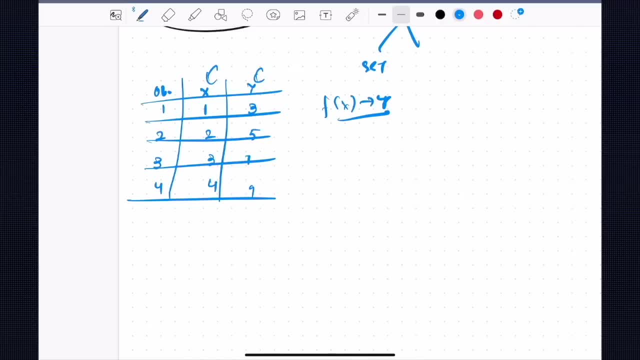 built a linear regression model on top of it. uh, basically, we need to do the hypothesis test. we sorry, we know we need to predict. we need to predict the y hat right so that we can calc, so that we can. so that let's take an example: beta 0 is something there- 0.1- and beta 1 is also 0.2. 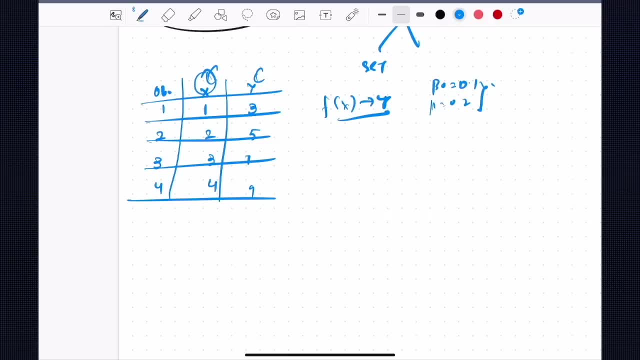 test it right. so you have to take, you have to say you, you have to perform the predictions on the x and then compare the prediction y hat with y, right, so your y would be nothing. but so your, your actual y was 3, 5, 7 and 9 and your model predicted 3.5, 5.5, 7.5 and 9.5, which is the model which which. 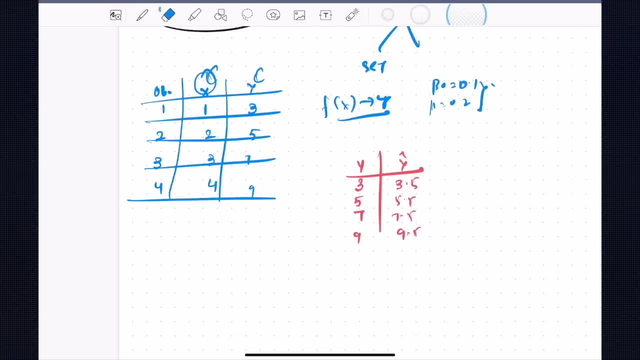 your model has predicted. okay, now we have to compute the r squared. we have to compute the r squared. so the formula for compute- we'll talk about the geometrical in just in some minutes- but the formula for computing the r squared. the formula for computing the r squared is nothing but 1 minus s s r divided by s s t. okay, this is the formula for calculating. 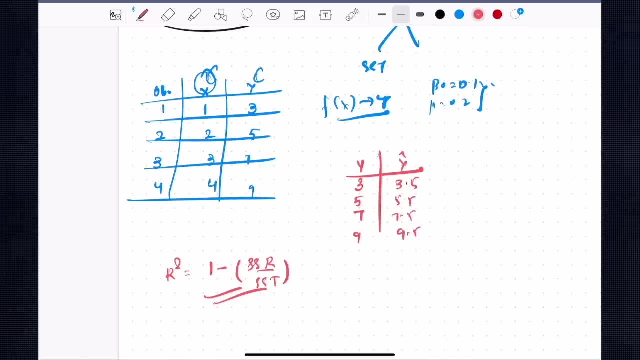 the um, what formula for calculating your r squared. but let's talk about, let's break down what is s s r and what is s s t. so s s t is nothing, but it's the total sum of squares. so s s t is nothing but the total sum of squares, which is total sum of squares. what does it tells s s t represents the. 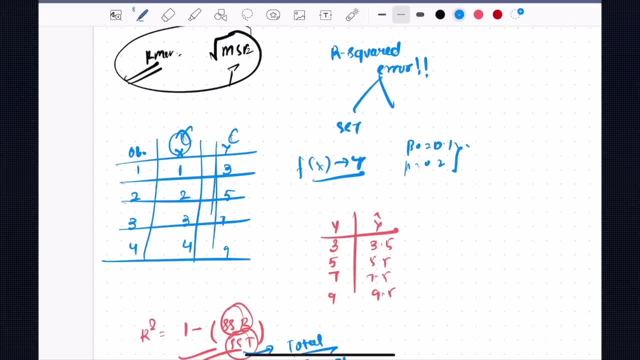 total variation in the dependent, which is the variation in this. so let me just highlight this: the variation, the total variation between the dependent variable is represents the total total variation in the dependent variable. how differences, what, what differences? what variation it shows between whom? so it shows between the. it shows that the total variation, how much variation? you get into this okay. S s t is nothing but 1 minus s s t. one square x minus 4 square x minus 4 percent is nothing but 0.5 times the total amount of respect of your r squared unit. as来 and Freiburg gives you with any number you give some magnification, you say that s s r plus r squared Foreign. 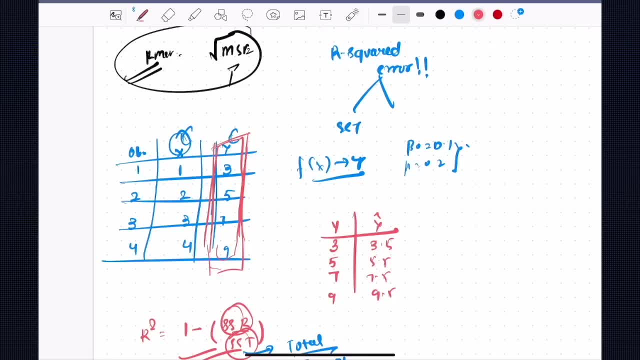 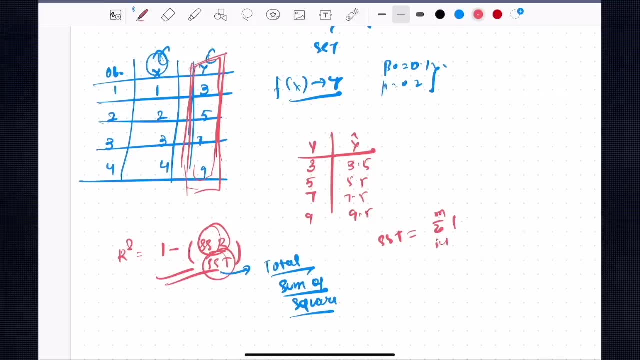 it shows that by showcasing the difference between the actual value and the mean. so your sst, your sst formula is nothing you go for. i equals to 1, all around the m, y, i minus y, which is the mean diverse, and and and squared okay to get rid of negative sign. so what does it tell it is explaining about? 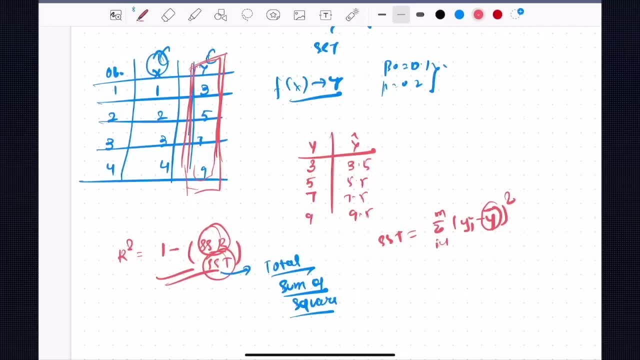 your y. it is explaining about a target variable. it is where the where we take all the differences between the differences between your uh prediction, your, your, your act, not a prediction ground to explains the variation between the ground and the mean of this. so what is the average? so assume that 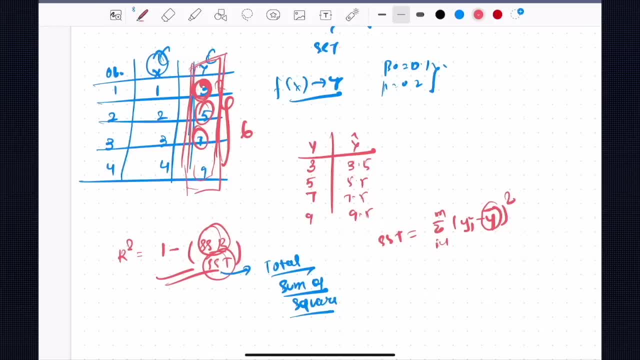 average is six, so the. what is the? so three, three minus six, which is minus three, right so the variation between your variation, between the actual values and the mean. so what is the most common value, value in this? and what is the? what is the who, who are in beside of them? what is the? 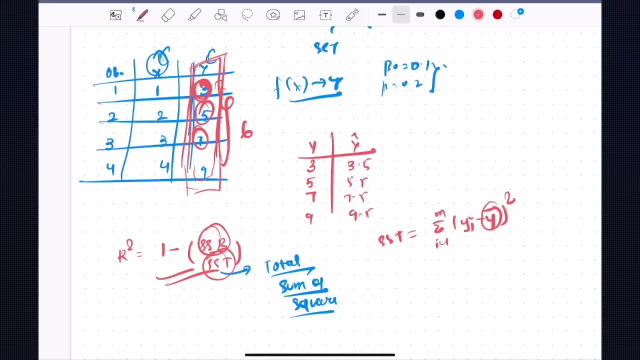 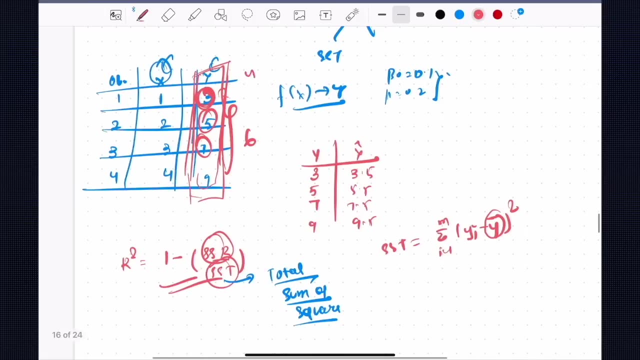 variation is over over there. so that's what it does. so basically it is saying the very- we have already talked about variance, a lot i don't know discuss, just discuss it once again. so it measures the variability of the target variable without the considering the influence of the independent variables over here. are you seeing? 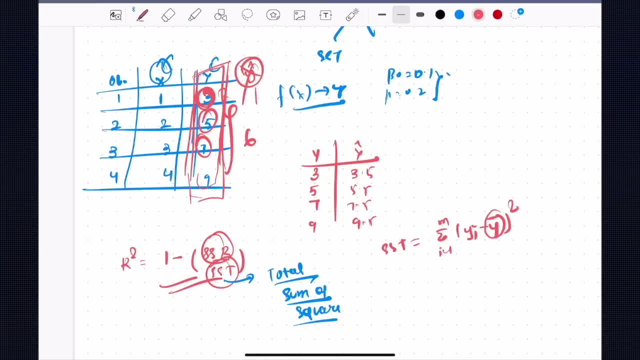 i'm taking y hat, i'm not taking my head, i'm just taking out. i'm just taking out the variability of my target, where how much my y is spread out, how much my y is a target variable which is dependent variable, is varying out. right, it's varying out without considering. 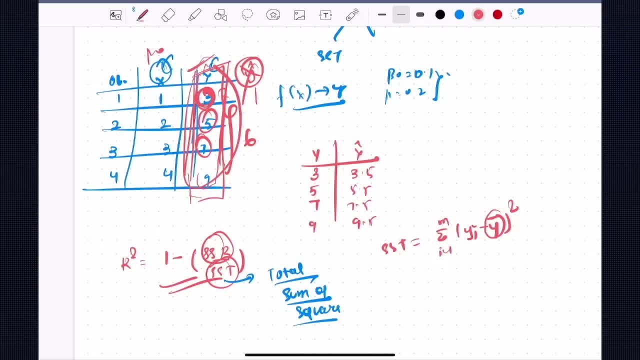 our beta zero and beta one, because over here, this is, this is our data. right, we are not considering anything, we're just taking the y? uh, which is we are just taking the y? uh, which is the mean, and then we are just trying to take out the variance, we are just trying to take out the 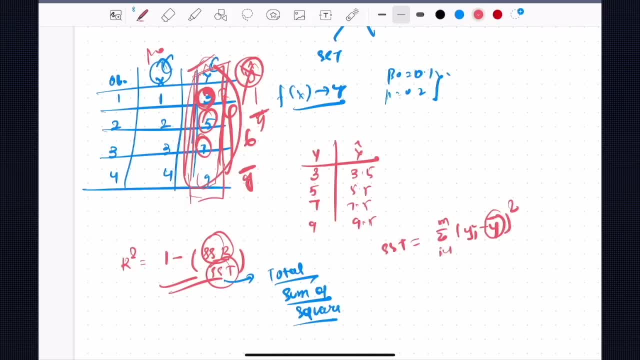 variance between: uh, with with that mean. so basically, we are not men, we are not doing any sort of. there is no, any influence, there is no influence, no influence of your independent variables. we are not used, there is no influence of these independent variables or literally anything over there when we calculate. so so your? 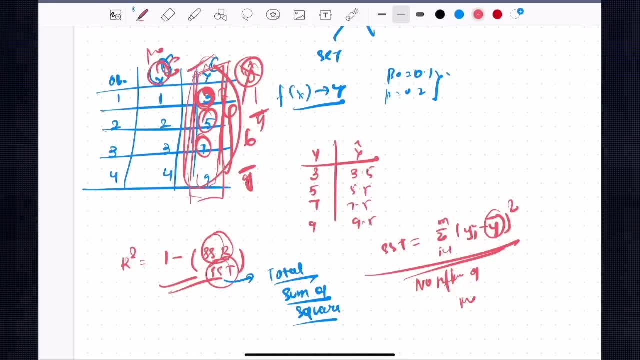 formula for that was ssd. was this: where to summarize that you're taking out the differences between your, predict, your, your not predicted, with the ground truths, values, the target where the, the actual target values and the mean of that to take out the difference? uh, so to take out the variation. 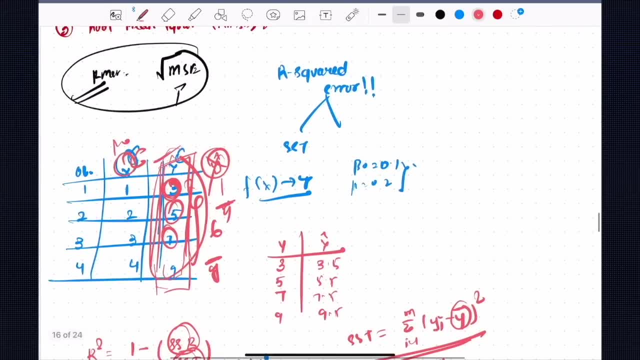 in that particular, or the variability in that particular variable. okay, which is why, then you have nothing, but something known as ssr is nothing but ssr. so which is which is the full form is nothing but residual sum of squares. so the formula for this is nothing. 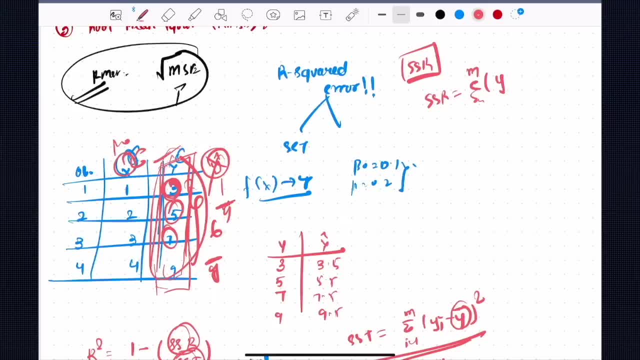 but ssr is equals to uh, i is equals to one all the way down to the end: y i minus, y hat i square. so this is something which you, from which you're familiar with. here we are taking out the, taking out the, the variability of the dependent variable. so, basically, we're taking out the variability of. 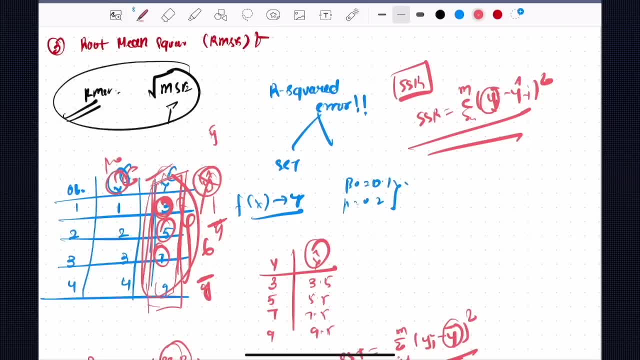 the dependent variable, considering our y hat, considering our hearts. we're going to take on the variability of this here we are just taking out the variability without considering the y y. here we are over here taking all the variability where they're considering the y hat, because we're 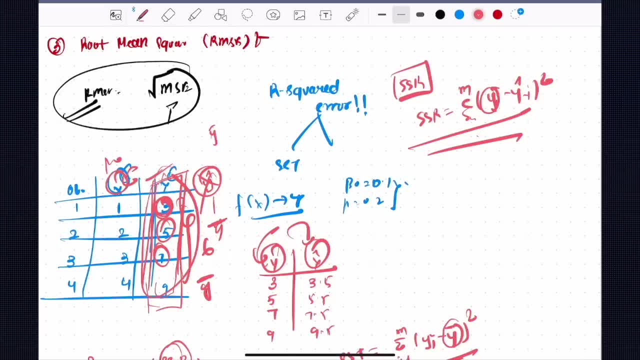 going to definitely take all the residuals through its explains. it represents the unexpl uh the it. so basically, higher the variability may, higher the variability method key, more the difference and more the difference back the model because your model could not be able to predict so higher the. 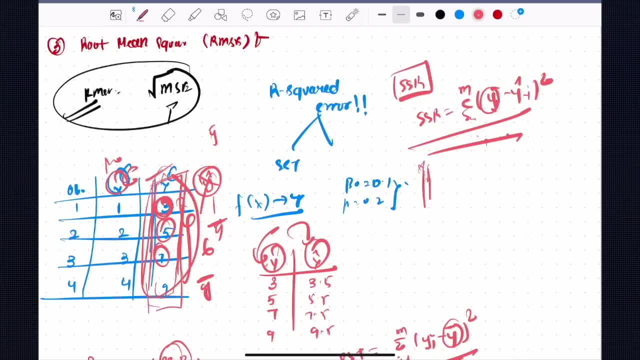 variability explained in this, which means that the more the model is not able to capture, which means that more is not to explain again. i'll summarize in very simple terms: the ssr is nothing but which you have studied, so i'm just going to reframe in different terms that you're. 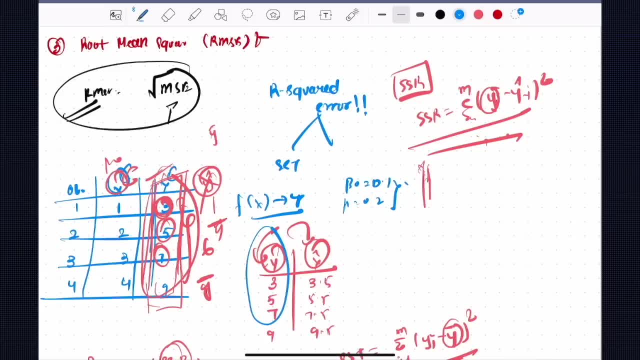 taking out the variability of your dependent variable, taking on the variability of your dependent variable, considering the effect of y hat. how you're doing that previously in ssd. what you're doing, you're taking on that variability of y hat without considering of y hat, just taking on the. 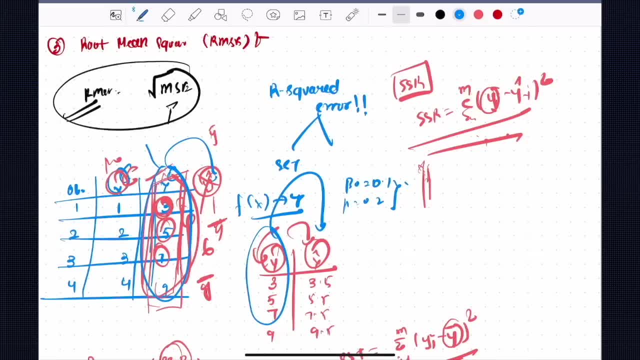 mean of that, and then just taking out the way, the very with the variation. but up here you're taking on the variability. with the constraint so higher, the variability means that your three is far away from 3.5. that's what it means, you know. so if the variability is high, that means the errors are high. 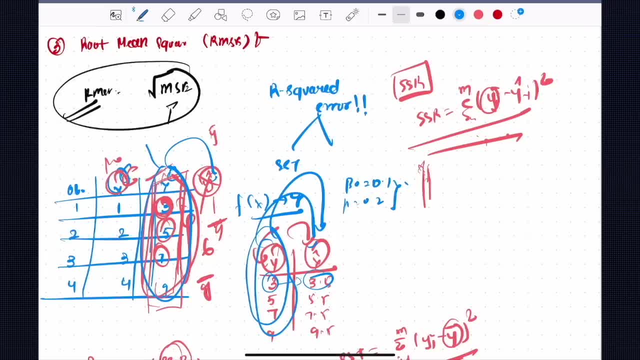 variance is this: how spread they are from the mean. so basically, the, the variability is also, which means the way the variability is high, the model could not capture it, the model could not learn it in the nice way. okay, so ssr over there is and indicates that this is the formula. so now once. 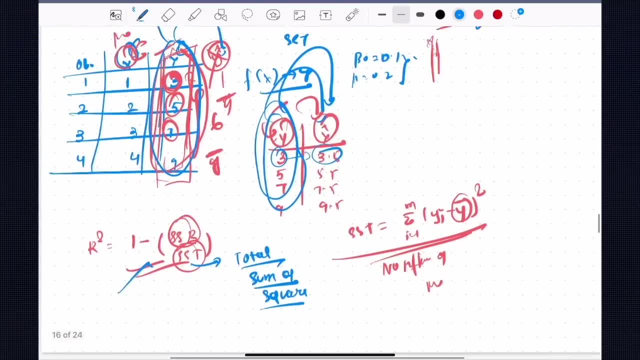 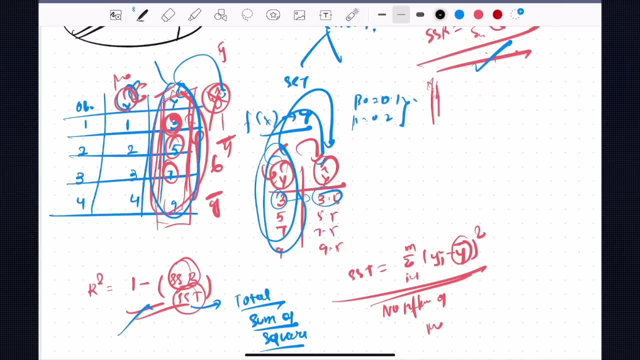 you about know about ssr and sst. now you can easily come back to formula. and what does it tell? let's, let's talk about that. so your formula tells me. your formula tells me. so assume that we want to take out the r squared, so first of all, we want to take out the r squared, so first of all, we want. 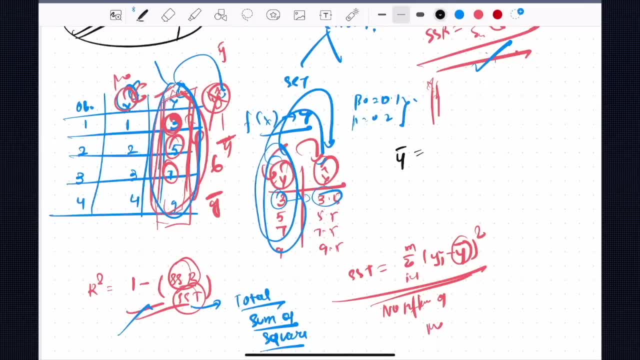 let's, let's take out y uh, which is let's, let's, let's put, let's take out the r squared for this, which is number three point three, plus five, plus seven, plus ninety, whatever four, which is number six, and then you have sst. you take out the sst, which is which you'll get a twenty, and ssr, which 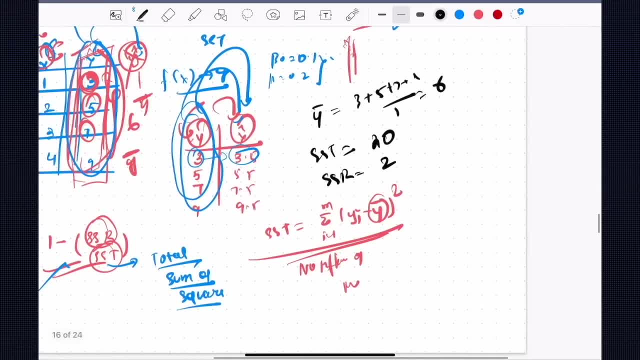 is residual, which is nothing but two. okay, now we can easily compute it. now we can easily compute it. which is r squared, which is nothing but one minus two by twenty, two by twenty, which which will get one minus 0.1, which is 0.9, which is when you convert in percentage term, which is 90. 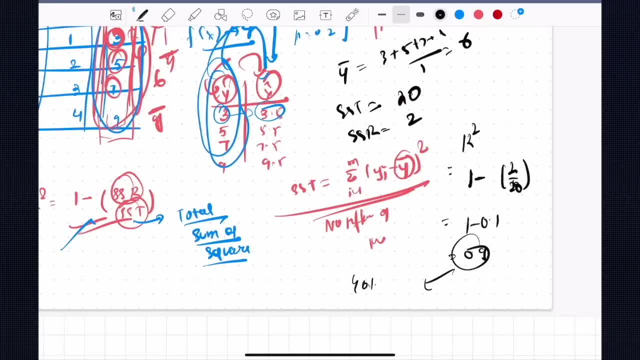 so the r squared value is 0.9, which means that 90 of the variation in the dependent variable y can be explained by the independent feature x using linear regression. so if we are able to explain if, if our if, if there is a 90 variation in the dependent variable means that 90 of the 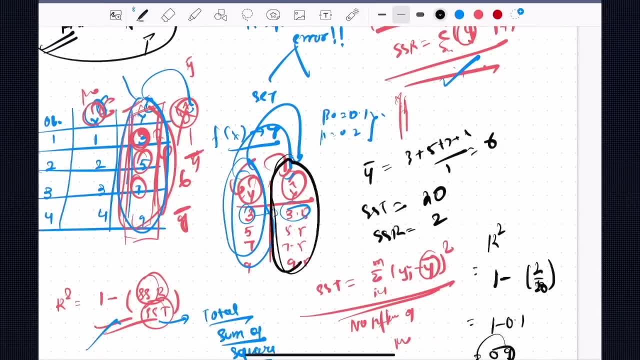 answers are able to correctly are your linear regression is model is able to give 90 of the correct answers. you- this is 90. this, this is your model- is able to correctly identify 90 percent of the examples. you're not designing this way. 90 percent of examples are correctly identified- okay, but it's not exactly what. 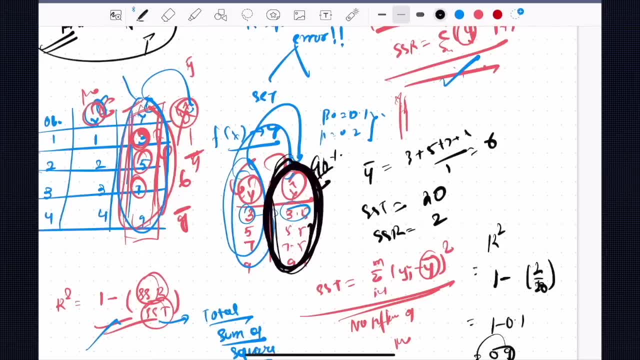 i'm saying is something like 90 variation. 90 variation is explained by your model, which means the 90 of the variation, which is which is perfectly explained. so the if, if the variation is low, for example, is 20, 20. so this is pretty pretty much low. so your model is not able to. 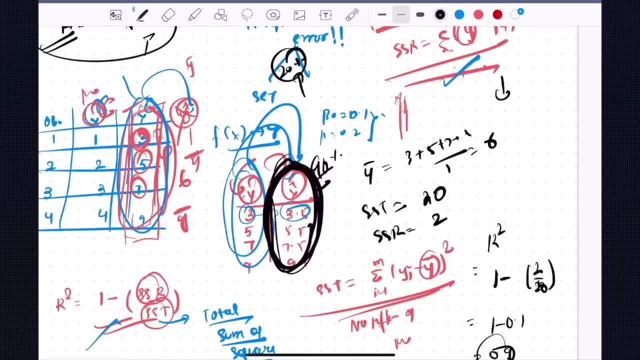 uh exp. your model is not a best fit because it is not able to explain your model. if you nine 90 by 90 percent, your model, your linear vision, is able to explain the x, x, x. explain. the independent is explained. okay, i hope that this gives you good sense. what exactly this just says? higher the r. 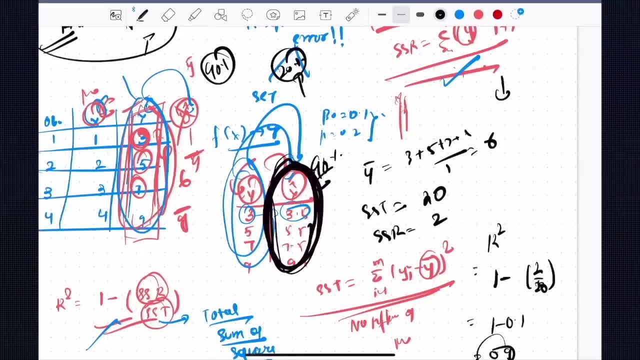 squared value. good the model is because it's able to explain more variations in the dependent variable y, given or explained by the independent variable x. so x is able to uh, which is your linear model, is able to uh, explain your wife. okay, but one thing to be noted over here: there is what there there is. 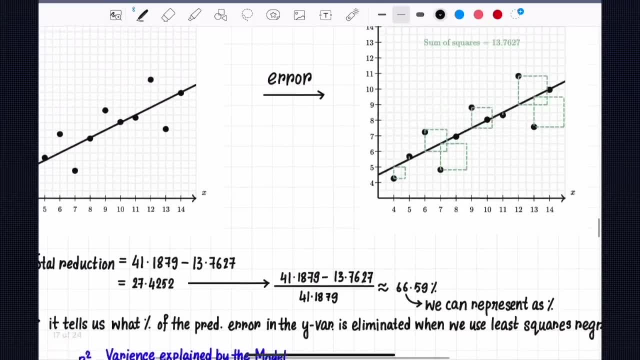 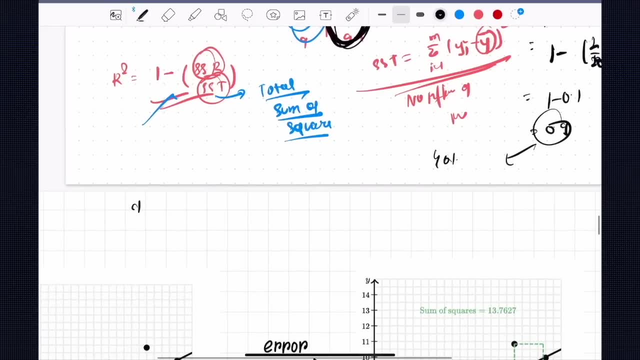 there is one thing which i really want to write, one thing which i really want to write over here, over here, maybe let's write it out. so the r squared, which means that the x percentage of x percentage of the variation, of the variation in the dependent variable, in the dependent variable, 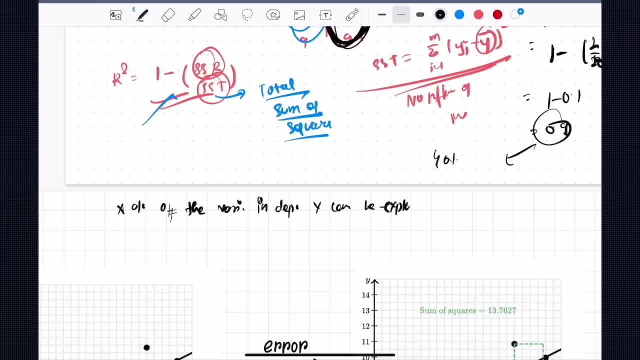 y can be explained, can be explained by x using lr. so this is what it said. so if the variation is large, then then your model is good. but if the variation is less than your model is not, but depends on problem to problem as well, okay, uh, but but over here, see over here that you have x. so what does it tell then there's, if there's 90? 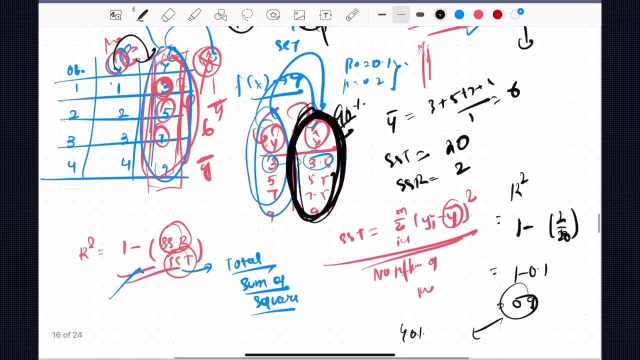 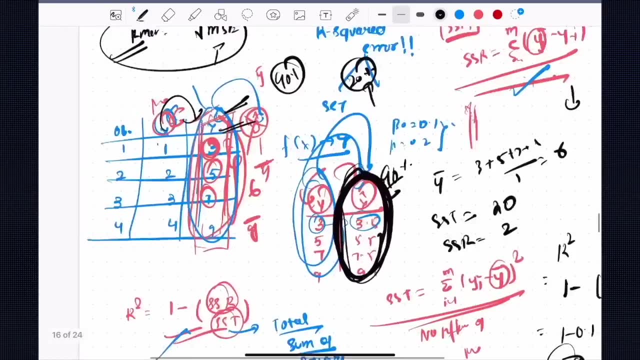 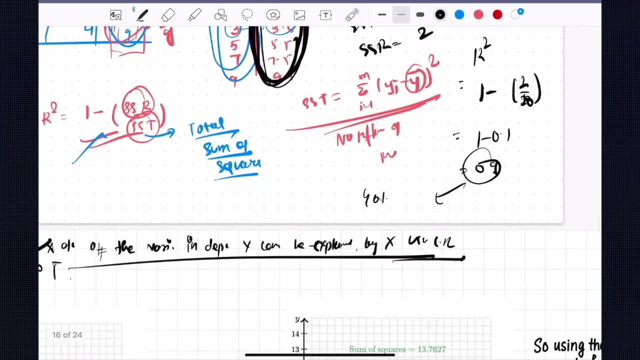 of the video. in this example, the 90 percent of the 90 percent of the variation in this particular y and 90 percent of the variation, 90 percent of the variation in this particular y is explained by x, is explained by x. so x seems to be useful feature is explained by x using our linear regression. okay, 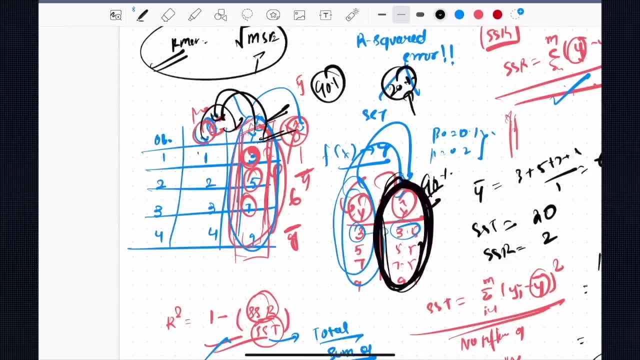 so 90 of variations explained, you can understand your your, you are able to your you, given the information, you're able to correctly identify 90 of them. okay, so this is this is one way to understand it, but yeah, this is a very messy thing. to help you understand r squared, we'll have one. 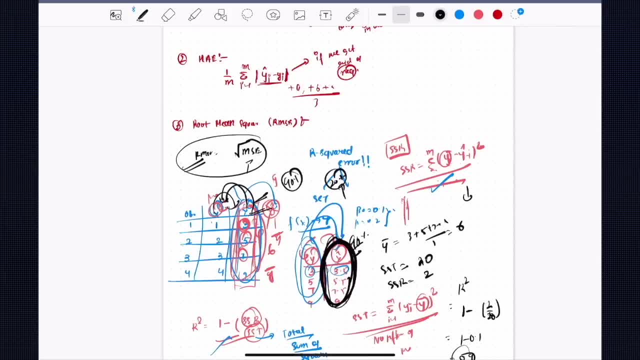 practical example to have one. one more lecture on square and there is something known as adjusted r square. we'll talk about that bucket. it's the end end of this lecture. i really hope that you really enjoyed this, and now we are coming to the ends of our lectures, specifically cool, so uh. 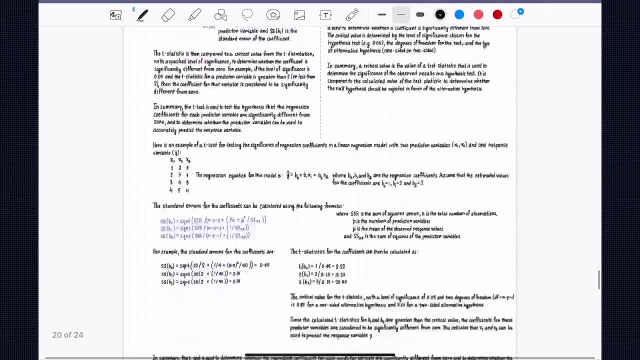 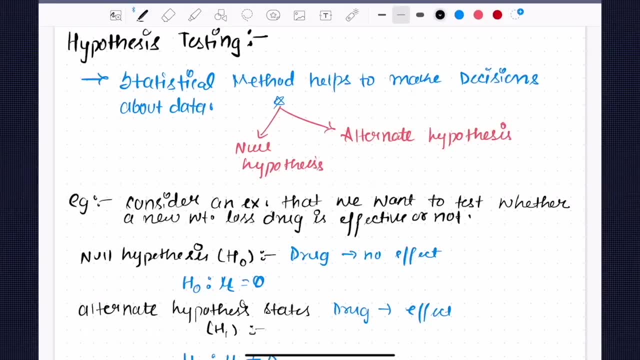 we'll talk about, uh, hypothesis testing, which is one of our last phases, and then we'll talk about assumptions, uh, which is one of the my favorite topic, and then we'll do a project, and then we'll end up this lecture. hey, everyone, welcome to this video. is uh, in this lecture, what exactly i'm gonna? 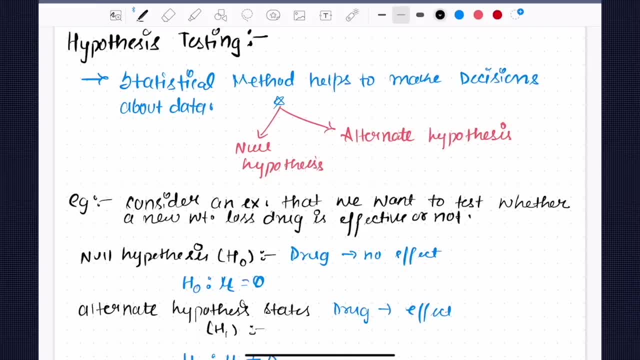 do? i'm gonna talk about one of the second last topic of uh whole regression analysis course is about hypothesis testing, and hypothesis testing is one of the most you know ignored as well as one of the most asked questions. um, that the topics from which the interviewers asks in regression analysis and we'll talk about this in pretty much. 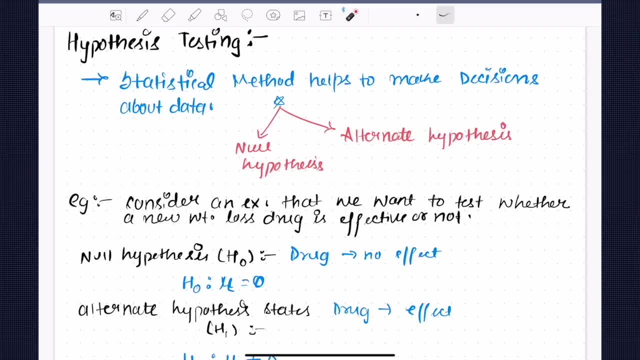 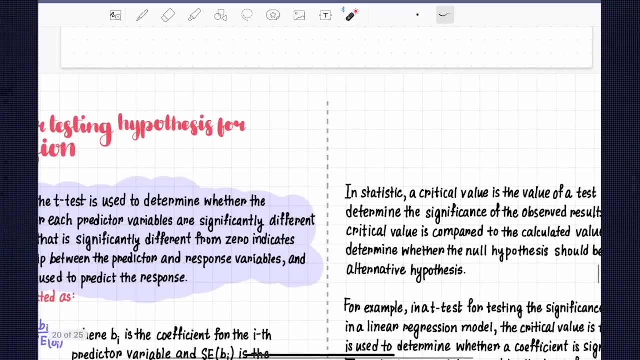 very detailed, with several examples as well, like: how do we use hypothesis testing, a linear regression? we'll have the practical implementation of it as well in various terms. and uh, and then after, and then after uh, working on the hypothesis testing, uh, we'll go forward and talk about uh. 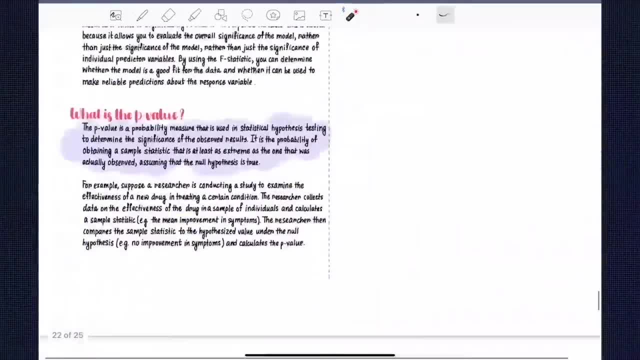 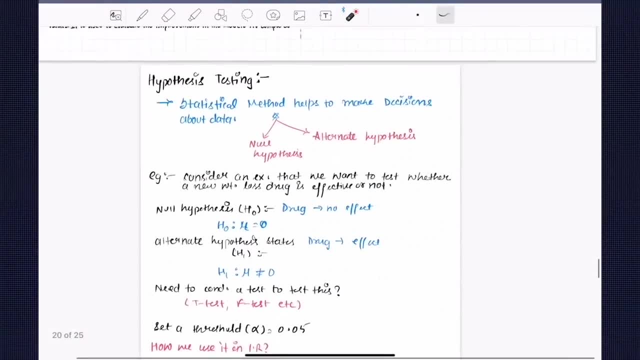 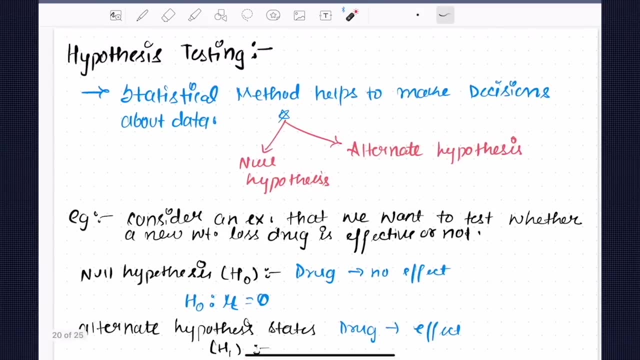 we'll go and forward and talk about something called, as some, something known as assumptions of linear regression, where we talk about something, but that's for later purposes. currently, our aim should be finished this hypothesis testing in very detail. now, one thing which i recommend over here is: sometimes you will see formulas. i would suggest you to completely ignore those formulas, okay, um. 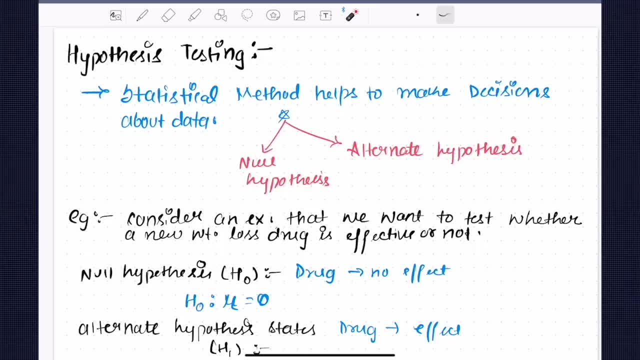 sometimes, you know, there is a some, some formula. this will come up. the main idea from which which you have to take up is how you, how you take up the idea of what you have to take up, is how you take up the idea of what you have to take up. the idea of what you have to take up is how you. 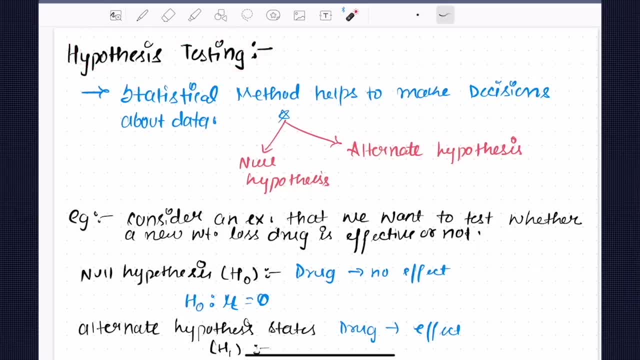 can understand the concept, the core of it. formulas can be seen later on as well. so how can you understand the core of it? by understanding the crux, by several examples, which i'll try to take. okay, cool, so now what? so now what we will do. we'll try to start off with this, but before that, i just 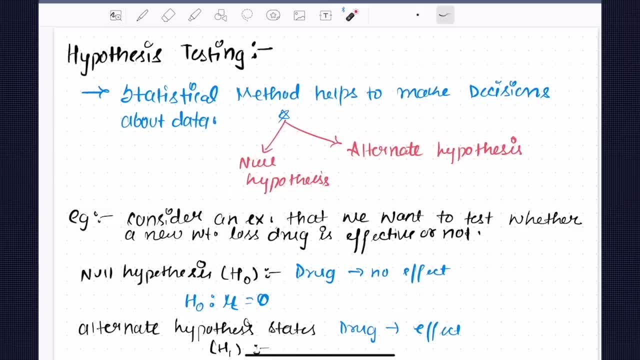 want to clarify some of the things that uh, as, as i say, formulas will come. please ignore if you, if you're not able to understand it and at any point, if you're not able to understand, i suggest go to a discord server. go to a discord server and ask directly by giving the timestamp you should tag. 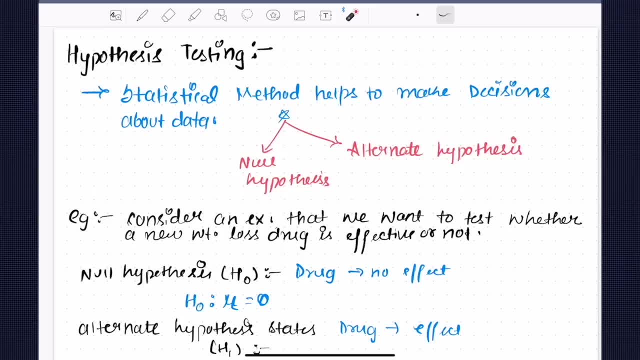 the help, or create a ticket directly out there and then ask the question, uh, in machine learning section about, uh, any such questions if you have. so let's get started eventually, uh, with this, with this, um, basically, uh, you, you have. you must have studied about hypothesis testing in statistical. 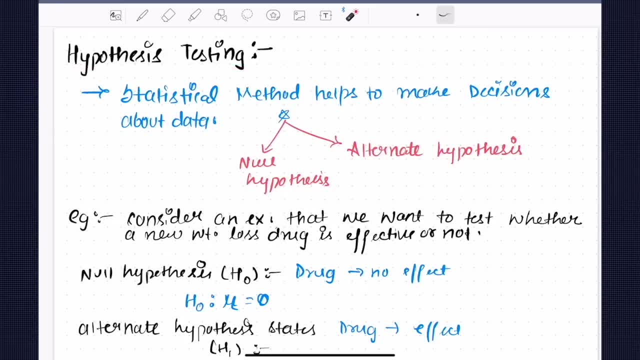 and probability lectures. uh, if you haven't, please. i consider to watch a little bit of lectures around hypothesis testing, because i assume that you know a little bit about hypothesis testing. however, i'll, i'll, i'll also describe over here if you don't know. but, uh, i if, if you're not comfortable with. 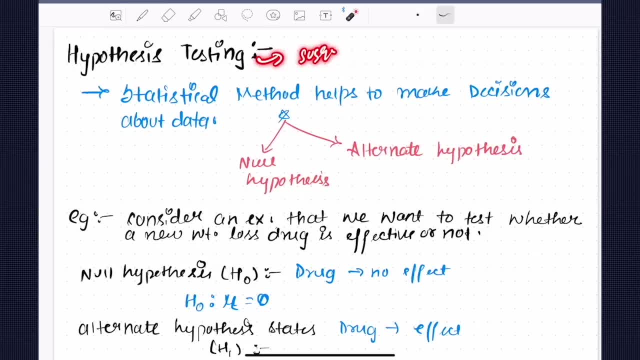 statistics and probability. i would suggest- the highly suggest- to go and watch our stats and prop lecture. stats and prop lecture, which is one of the most important you know uh lectures. but it is available on our course, which is cs01, or you can say machine learning, course, machine learning. 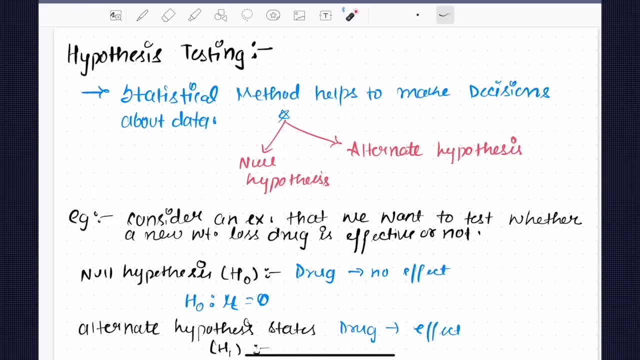 course, by anton you will be able to see everything out there, but let's get started with actually this, this, this lecture. so, basically, what is hypothesis testing? hypothesis means some sort of statements or to be made. sometimes some sort of statements which is not yet means like: this is the hypothesis which we want to test. we say now, this is a. 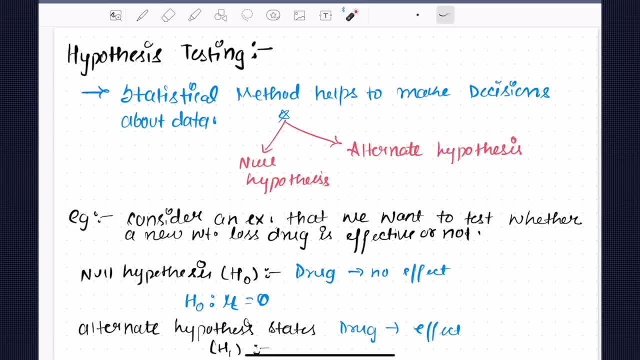 hypothesis which we want to test. so the formal definition if we go to hypothesis, the formal definition if you go to a hypothesis, so hypothesis states that the the hypothesis states that is what, that that the statement or the explanation like for a statement is made based on limited evidence. 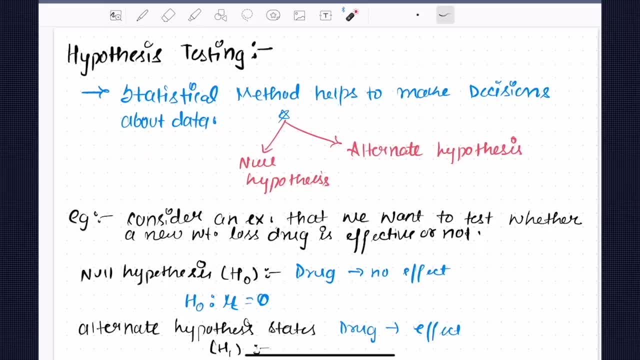 but if you have test purely based on limited evidence, then the data are solid so that you cansweise test for Hall au log, which is the other part of hypothesis land grant, and these are lots of examples how to test made. these are lots of examples to discuss whatsoever. today's were not in the actual textbook so that was all just a small. 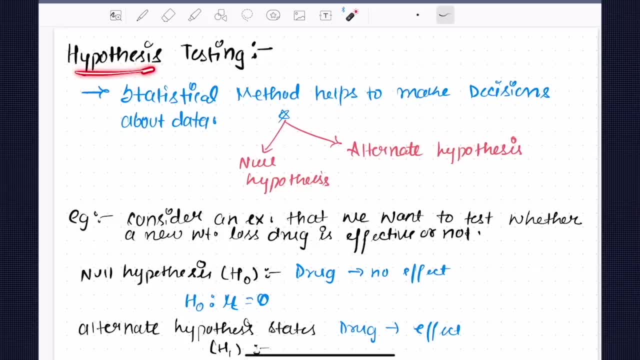 amount of evidence, for example, for the, for example, one of one of the example, that that one of the example can be: if you stay up late, then you feel tired the next day. that's, that's one of our hypothesis. that's one of our hypothesis, right? um, so these are some of the hypotheses. so how can we? 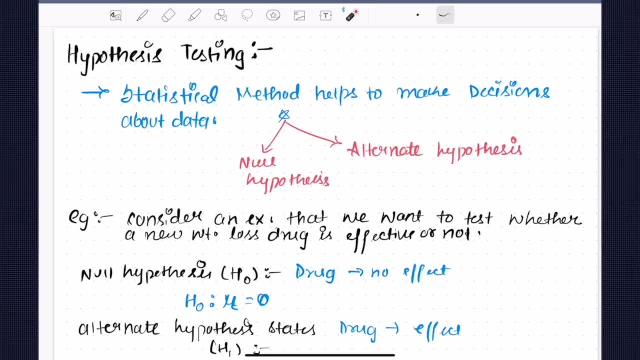 Stay up late, then you feel tired the next day. That's one of the examples. So how can you identify stay up late? if you stay up late, how can you validate it? So hypothesis testing deals with validating your hypothesis using several tests. 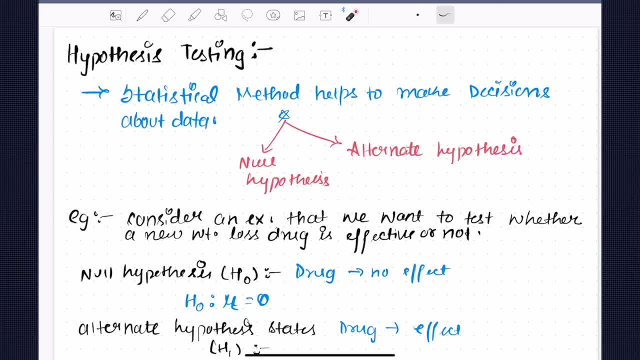 You know you conduct tests for identifying that, But never mind, let's actually talk about, let's keep talking about hypothesis testing. So it is a statistical method in terms of statistical maths. It's just a statistical method which has to make decisions about the data. eventually, 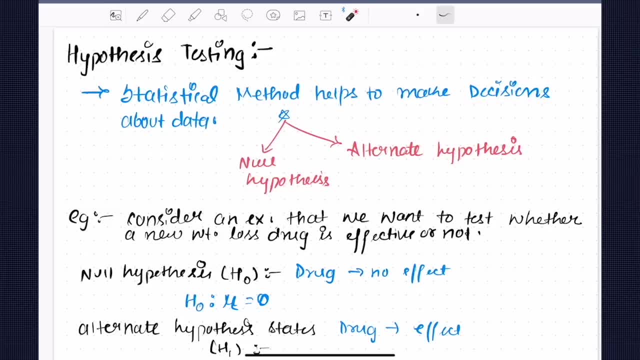 For example, that statement: what was that? If you stay up late? if you stay up late, you feel tired. If you feel tired, okay, that's one of them. Another one is: let's say, for the sake of an example, another hypothesis can be daily. 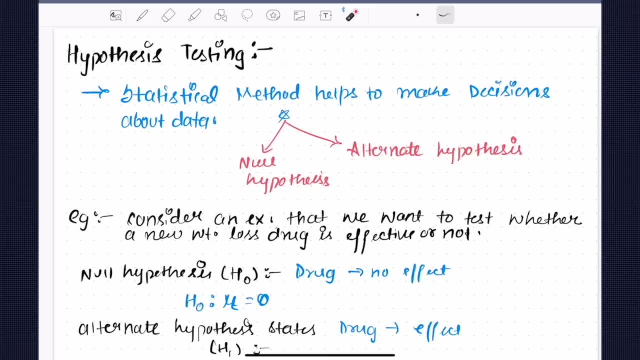 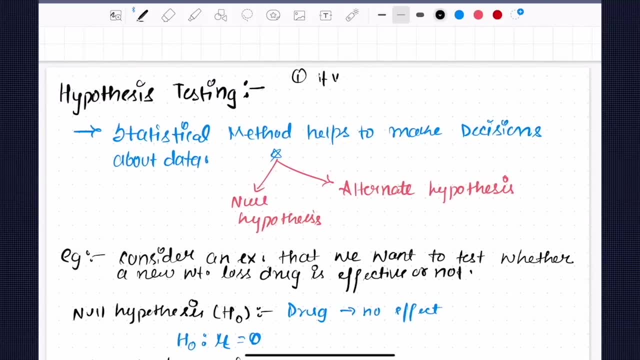 exposure to sun leads to increased level of happiness. That's one of the hypothesis. So previous hypothesis was that. The previous hypothesis was: if you stay up late, if you stay late, if you stay late, you feel tired, you feel tired, you feel tired. 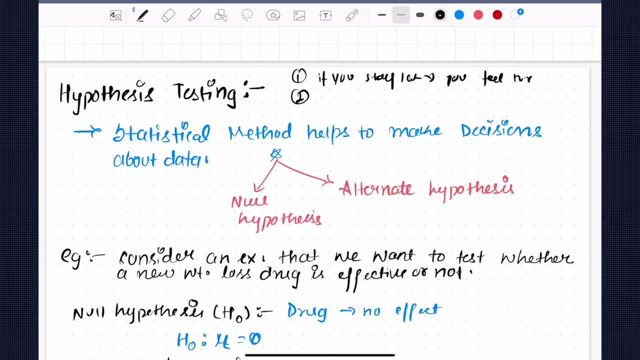 Second example of an hypothesis: exposure to sun. exposure to sun, what does it lead? It leads to increased level of happiness, increased level of happiness, increased level of happiness. So this is one of them. So these are some examples. So basically, hypothesis testing: 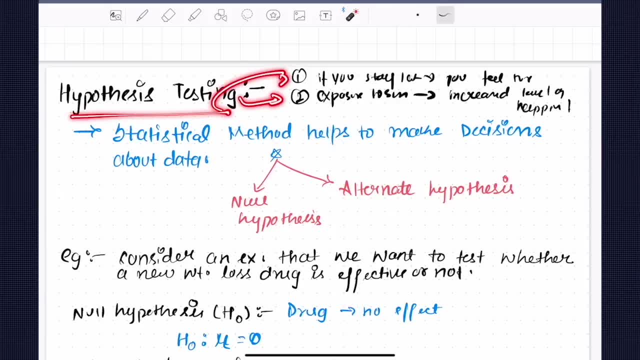 What is it? What does it do? What does it do? It validates. it validates whether this statement is true or not based on the data which takes the decision: whether this statement is true or not, based on the available data, based on the available evidences. 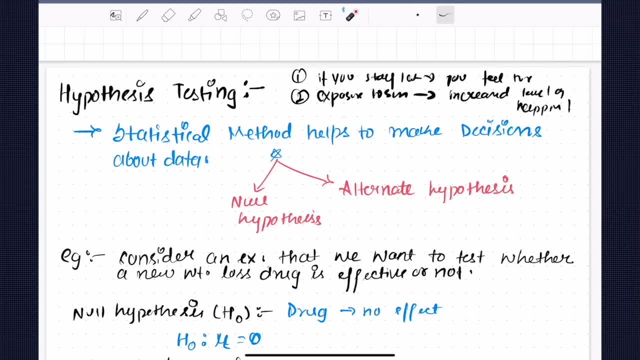 Okay, So there are eventually two types of hypothesis which we generally know, Something known as a null hypothesis and alternative hypothesis. or you can say H1, so S0 and H1. So what does it mean like null or an alternative, and blah, blah, blah. 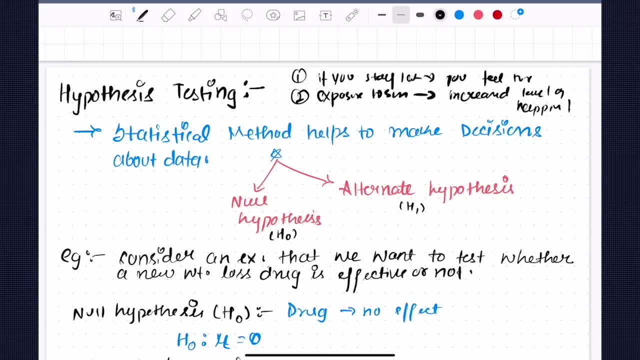 So let's, Let's talk about, uh, both of them in great detail so that you, you, you, you, you could understand in pretty simple language. Um, so let's take an example that you, that, uh, that, that your hypothesis, is that, that your hypothesis? what is your hypothesis? which you're on a? 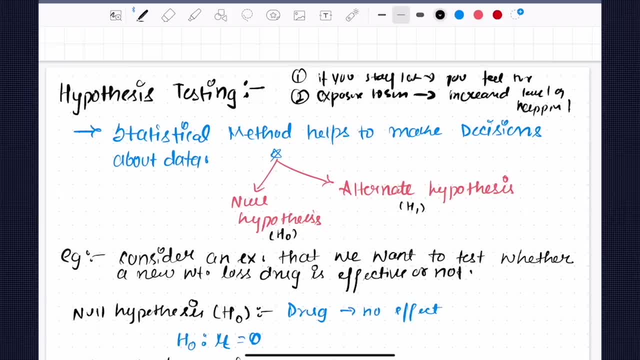 validate you're on a battle, validate whether, whether you're you may. let's say, in a pharmaceutical. a pharmaceutical company, uh uh, invented a new drug of weight loss drug. Okay, So they, they invented a weight loss drug. 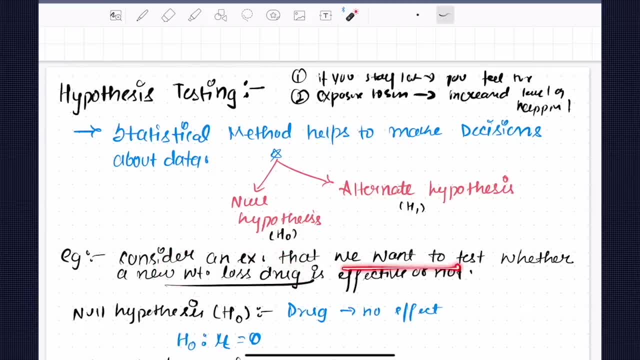 They invented a weight loss drug And they want to test, they want to test this hypothesis that the weight weight loss is effective. Okay, And if the hypothesis is true, then we say that if this, this is the hypothesis, what is hypothesis? 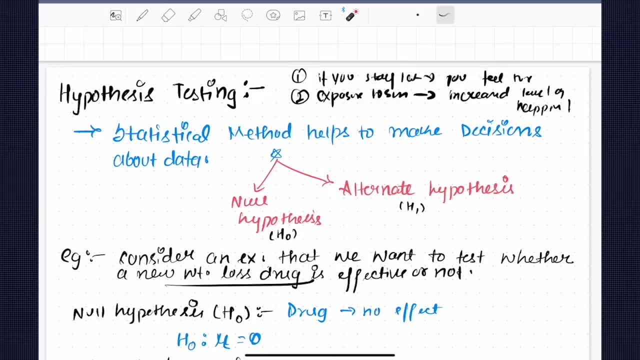 Weight loss drug is effective. Okay, So we test this hypothesis: whether this weight loss drug, the company invented with the new weight loss phase they have invented, is it effective or not. So this is a hypothesis which we want to test. which we want to test. 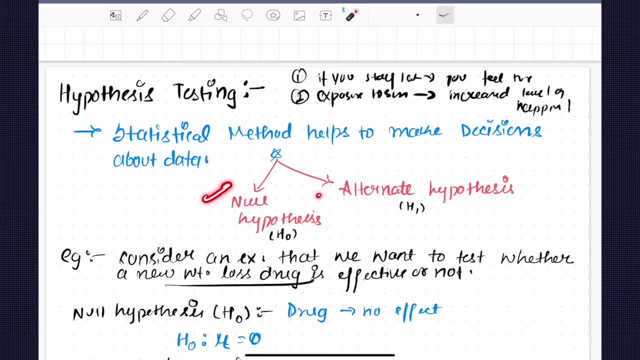 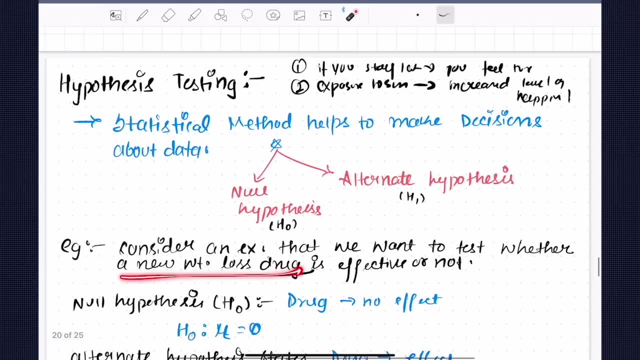 Okay, So there are two types of hypothesis: The first one is null and second one is alternative. So what is the null? The null hypothesis in this particular example, the null hypothesis in the? in this particular example, the new drug, the new way to drug, which is, which is which is published or which is invented, has no effect on decreasing your weight. 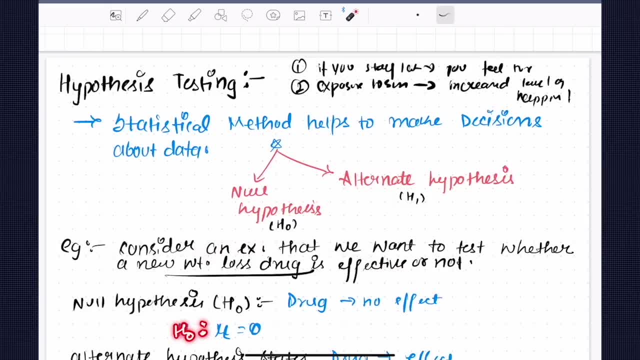 Okay, So we say that. so we say that your null hypothesis: the in the in the population- this is a population mean which is at that indicates in the pop. in the pop the drug effect on the population is zero, means the drug effect on a lot of people is zero. 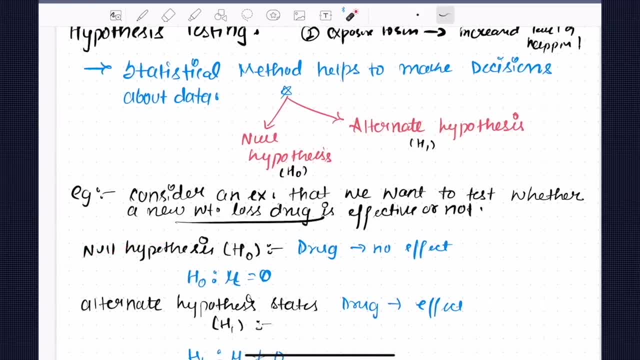 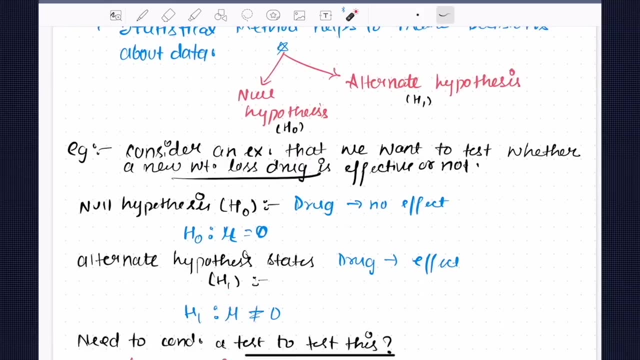 Okay, And that's null hypothesis. What exactly So? the null hypothesis states it says that a drug has no effect. but it alternative hypothesis: what does? it states It states that your drug has an effect. Your drug has an effect on decreasing the weight loss, which means that a population with the, the, the in in in the population, this is working, which is not equals to zero. 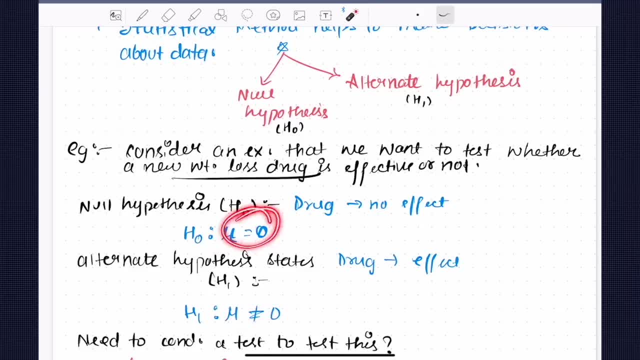 What does it mean Equals to zero And what does it mean You mean the population mean equals to zero, which means that it has no effect. population which is not equal to zero, which means that it has some effect. Okay, Okay. 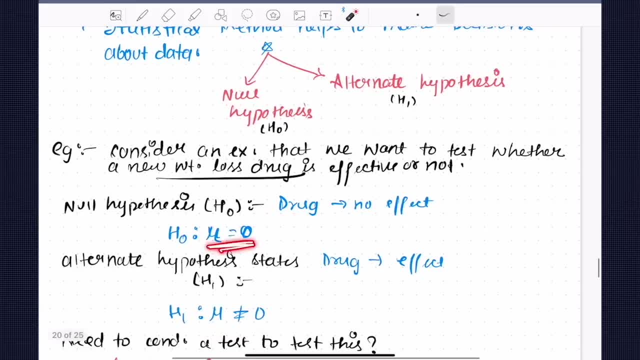 Okay, Okay, Okay, Okay. So what does it mean? is zero? the on the number of people, for example? this: this is going to assume the number of people which which this drug is affected is zero, which means that the drug does not affect, but over here it is not because of this. 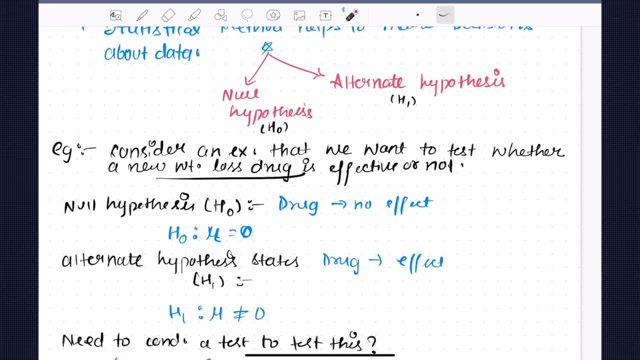 So the drug eventually affected the population. Okay, So how can we validate? how can we test it? So, basically, so basically, we want to test, we want to test whether, whether, whether we will consider null hypothesis or alternate and a particular example. this particular can be either classified in: 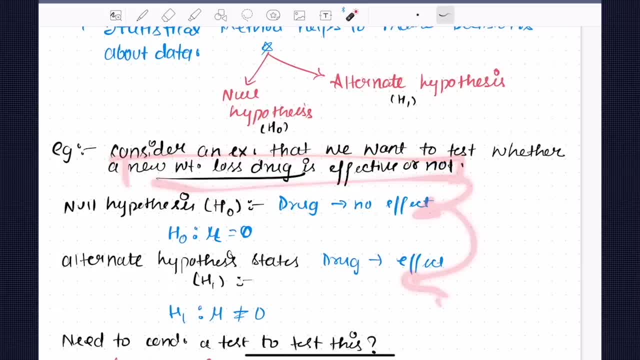 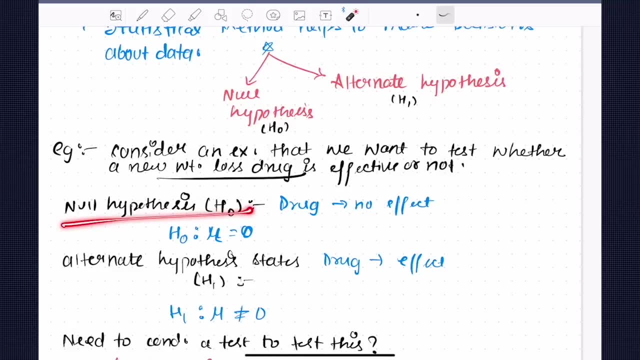 So, in a context, we want to conduct a test. we're going to conduct a test. we're going to conduct a test to identify whether it is null hypothesis, which means the drug has no effect, and an alternate hypothesis, which means the drug has an effect. 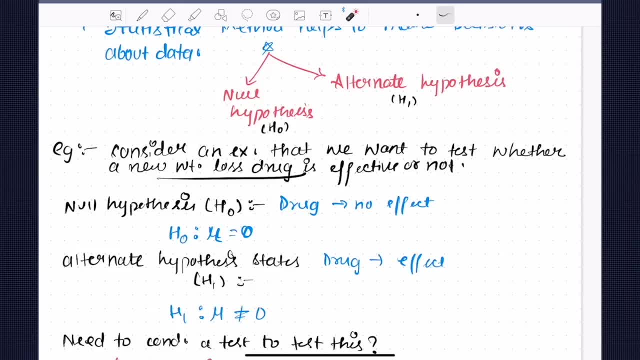 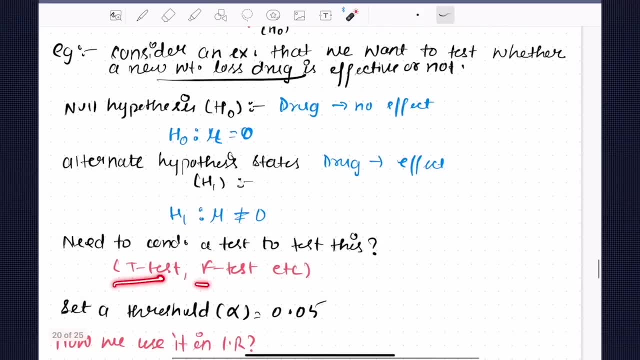 Okay, So this is two of them. which one to go forward? So we have several tests in our statistical tools to conduct, whether whether the drug has effect or not. Some of them are T test, F test and there are several other as well. 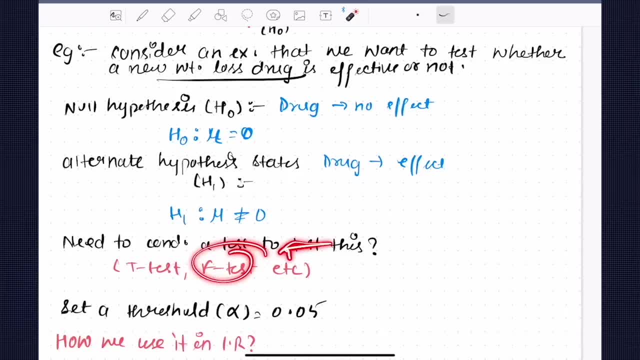 So we'll study about T test In great detail. F test will be given to you as an homework to actually work on your by yourself, because we want you to be not even spring food like this. We just want you to be explored in everything by yourself as well. 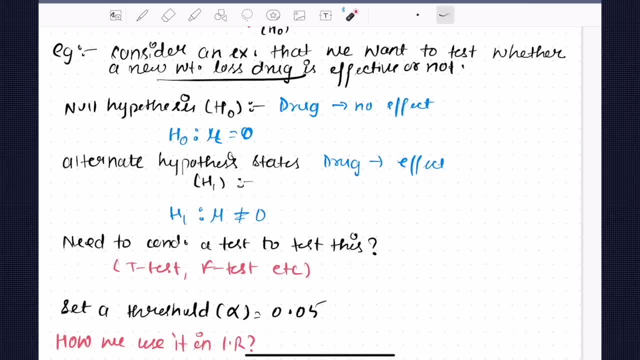 So you, now, now, now, you're at a journey where you have to explore things by your own right. If you have came over, came over here, this means that you have achieved a lot in your career as of now in terms of learning. 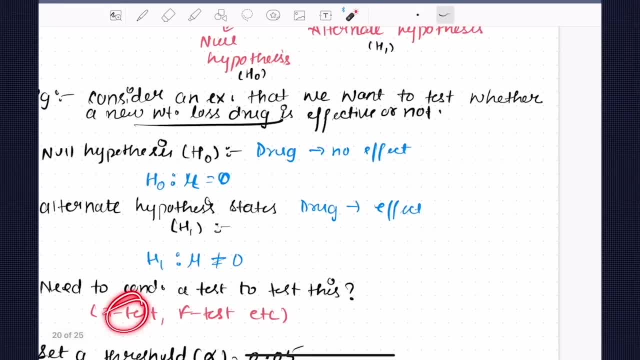 Okay, So now, so now. so, of course, when you conduct a test, it will give some sort of number. assume that C, right, So in what? and then what we do? We, for example, you got C, so so we, so we classify, you know, classify, you know, you have to classify whether, whether this is a null or hypothesis. 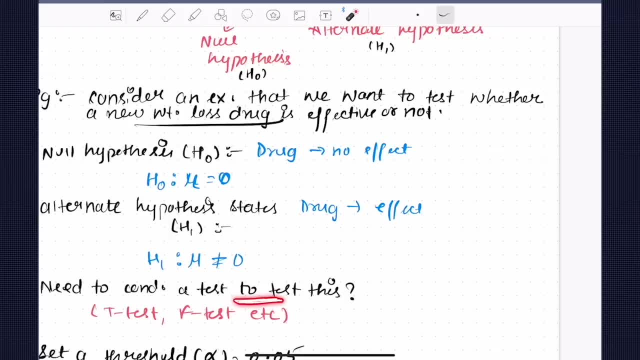 So, if, if, if, assume that you conducted a test, don't worry, we'll talk about each test in great detail. You conducted a test and then you got some number C. okay, You got some number C. So we check, we check with a significance, with which a threshold and we say that if your, if your, if your test value is is smaller than is smaller, 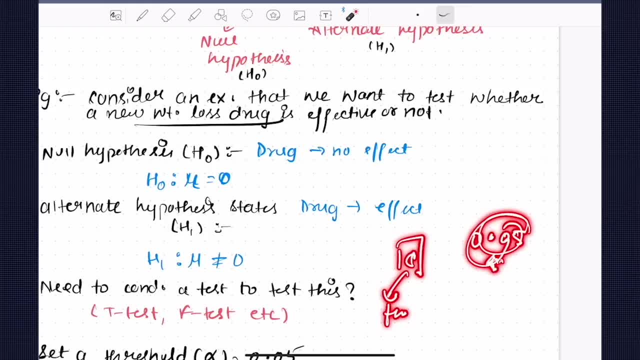 Is it smaller than this particular 0.00, which is 5%, which is 5% smaller than 5%? then what we do? we reset the null hypothesis and then we accept the alternate hypothesis, which means the drug. then we reset, then the drug has an effect. 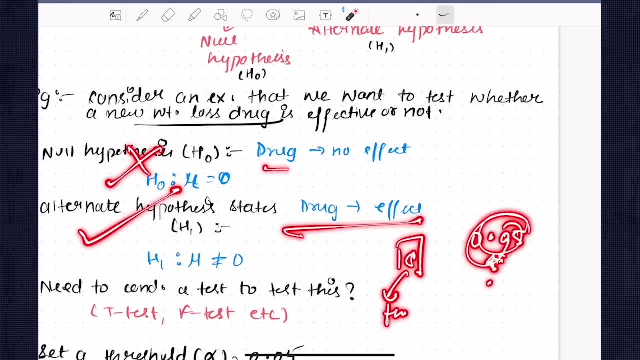 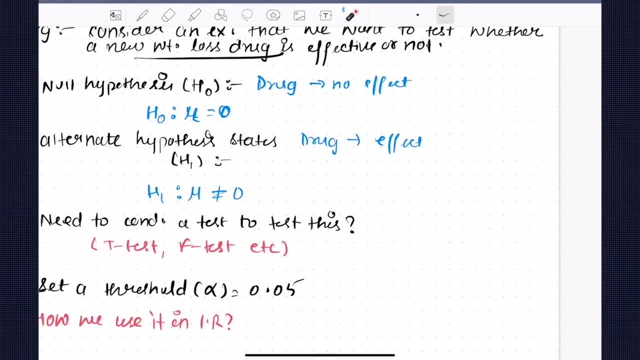 So, if, if your, if your, if your value from the test which you conducted is smaller than the significance value, which is 0.05, which is a standard threshold which we keep for, for, for, for, for, even when we used to test. 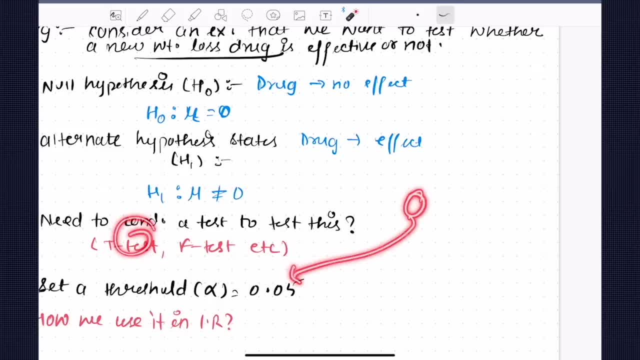 So T test will give you some number and then you and then you compare with it If, if, if, the test value is smaller than this, then we say that the drug has an effect. Why We'll talk about that later on in great detail as well, about this. 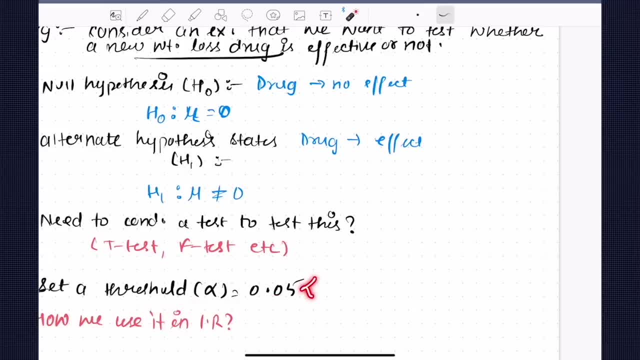 Don't worry. Okay, And then if, if it is, if, if it is greater, if it is greater, or your T value is greater than this, then we say that it is a alternate hypothesis. Sorry, We reset the alternate hypothesis and then we accept. 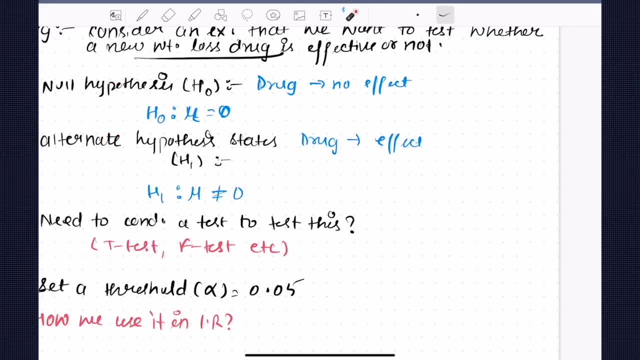 Basically anything of which anything above the 5% and your, your value, T value or the test value is greater than 5%, then we say that the drug has no effect. Then we say the drug Has no effect. 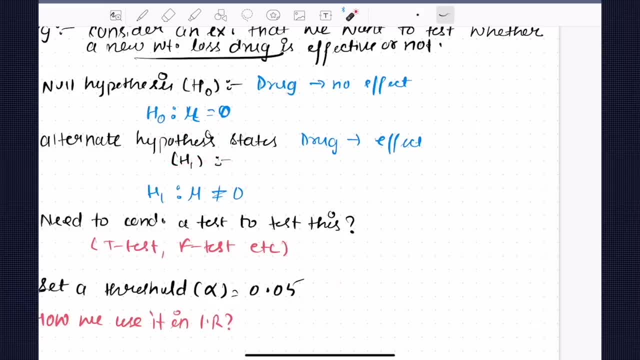 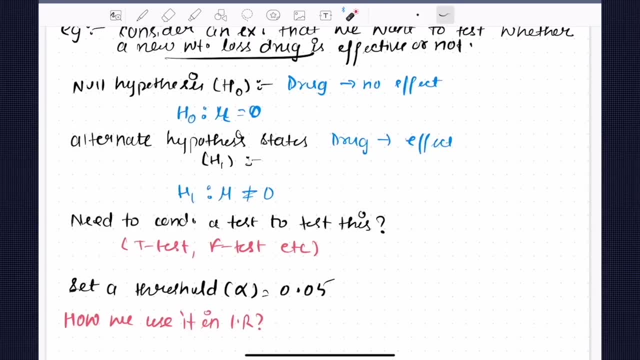 It is smaller than 5, 5%, The drug has an effect. Okay, That that was one of one of the example let's talk about in great detail This. this was just an example to showcase you the hypothesis testing, but how we use the hypothesis testing in linear regression. 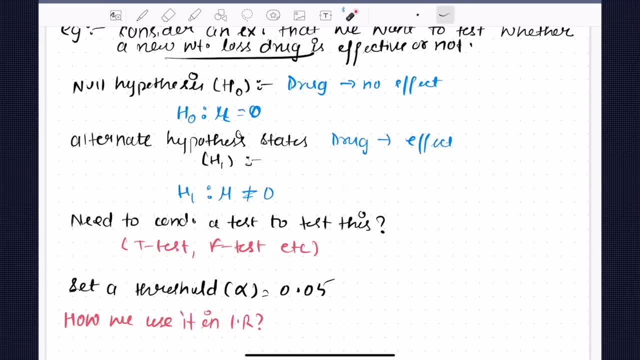 That's what. that's one of the most famous questions to talk on. Um, I just w, I just was, uh getting a red bull. I'm so sorry for that. Okay, So uh, how can we think about in terms of linear regression? 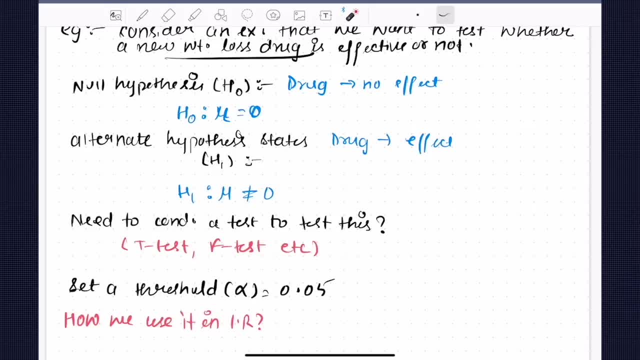 And this is something Which Everyone needs to know about. this, This is something which every everyone needs to eventually know about. So let's get started with that as well. Yes, So how can we use that in a linear regression and linear regression? 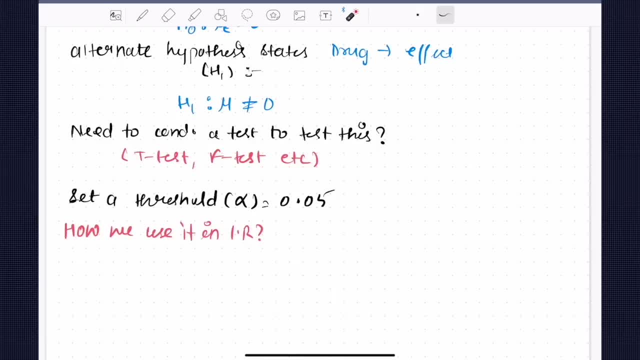 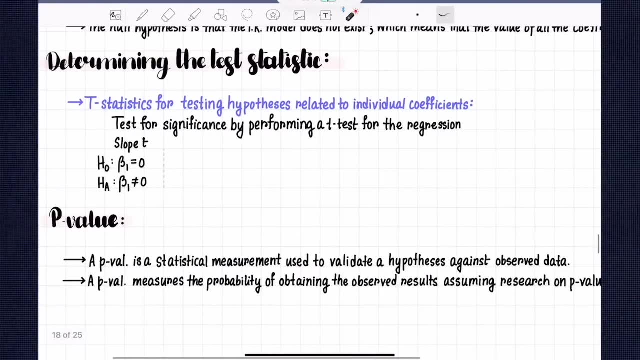 So, basically, so, basically, um, I'll just go through a past example so that you could be understandable in the easy way. I'd add: the preferred, all of this thing. Okay, So this is, this is one of them. This is one of them. 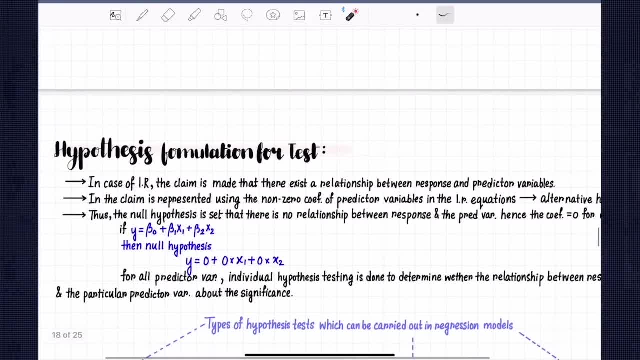 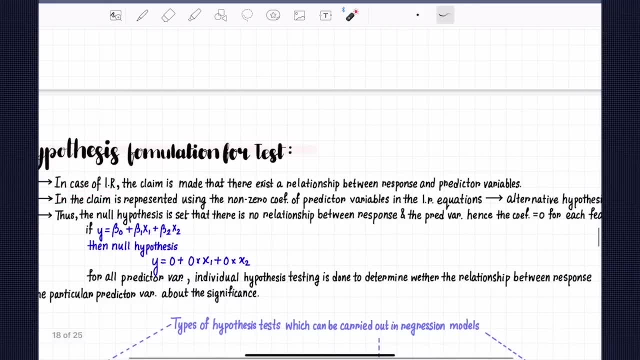 Where we talk About FTS. Yeah, So basically, how does we formulate our hypothesis in terms of linear regression? So, in the case of linear regression, the claim is made that there is a relationship. So what is an hypothesis? Hypothesis is that there is- there's exist a relationship between a response and a predictor variables. 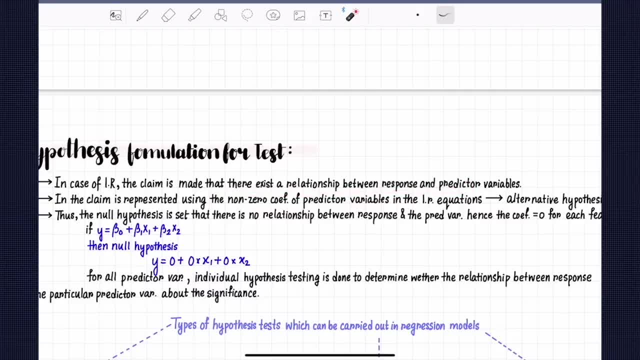 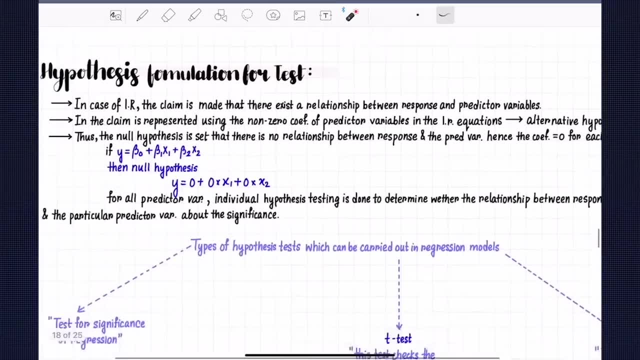 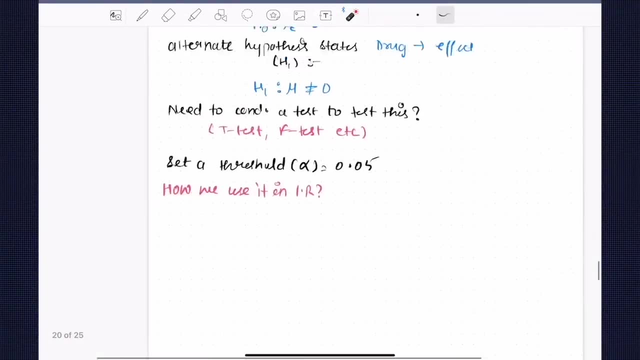 Now you might be thinking: why do we need hypothesis testing? Why do we need hypothesis testing? So basically, how and how does it helps and how does it helps? now, This, all of this, might be in your question, But first of all, I I understand that your question is, so let's go ahead and talk about why exactly we need hypothesis testing. 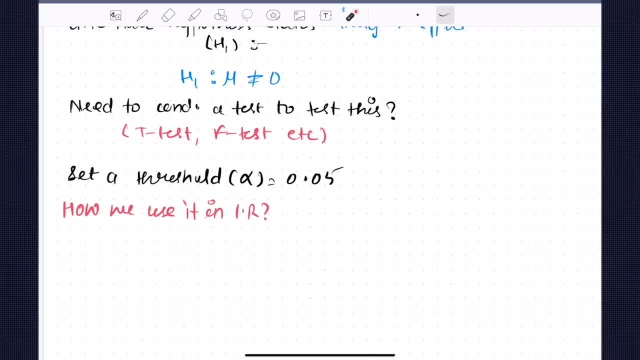 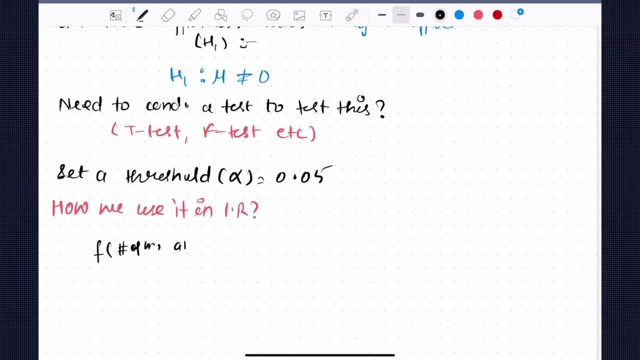 So assume that, assume that um you, you want to build, a you want to build. you want to build a function F that takes in the number of hours of study, number of hours and attendance percentage of a particular child and then predict what, what will the exam score? 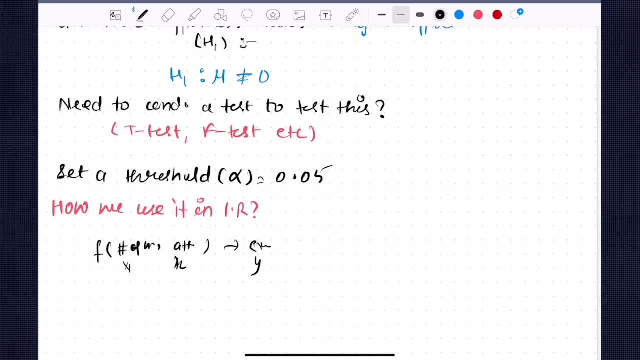 So so it takes the X one and X two and predicts Y, which is the exam score. Okay, So it takes X one and X two and predicts Y, And this is a Nice Uh, this is the function that you have to build. 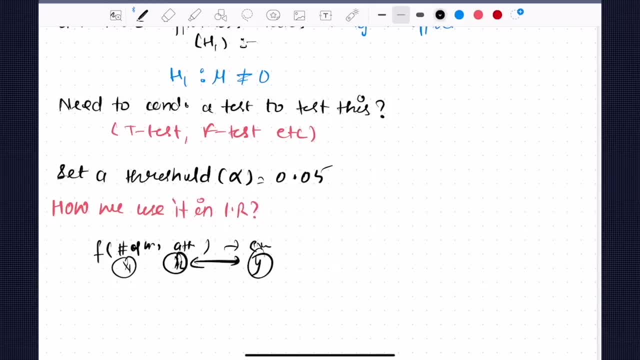 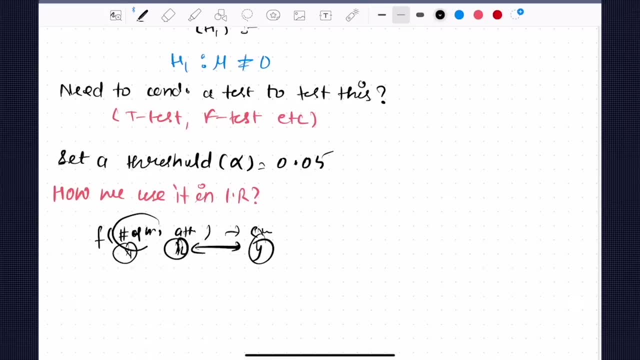 This is a function that you have to build up. Okay, So you have um now, now. now it may happen. Now it may happen. Now, what, what? what do you want to do? You want to interpret right? 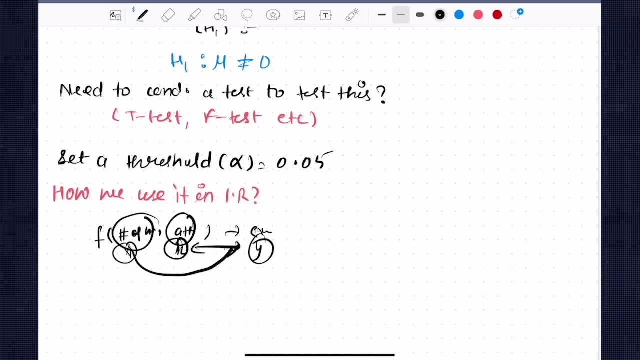 Is this significant to awkward variable? is this information? is this particular independent X one is significant. What does that mean Significant? significant means important. Okay, It's like like you can understand, Is it? Is it, Is it significant? Is it even reliable for this? 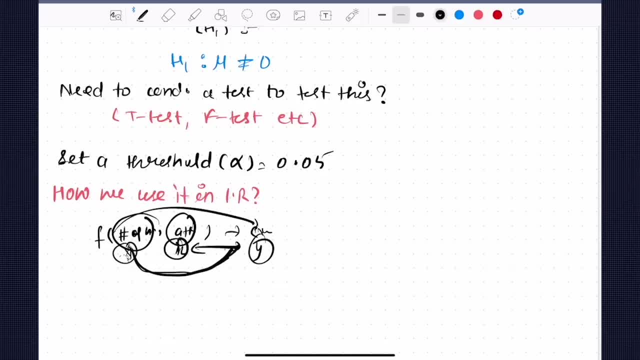 So, basically what we do, and the first hypothesis formulation is: is there exist any relationship between both of them, Yes or no? How can we identify relationship between both of them? How can we identify Is there any relation between both of them? 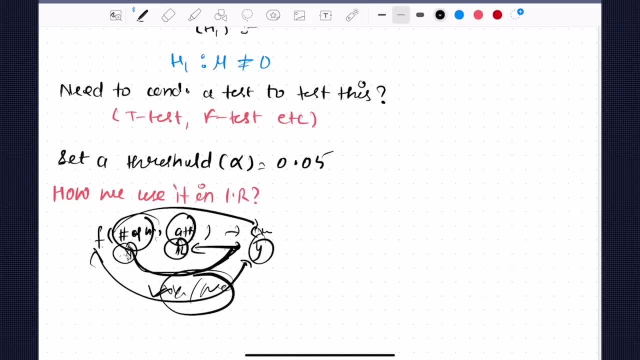 Uh, the input variables and outer variables, by calculating the significance, Okay, How much this value X one is significant to this output variable. Why? Okay, Because this is important in terms of the, the reason why it is important, The reason why it it, it, it is important. 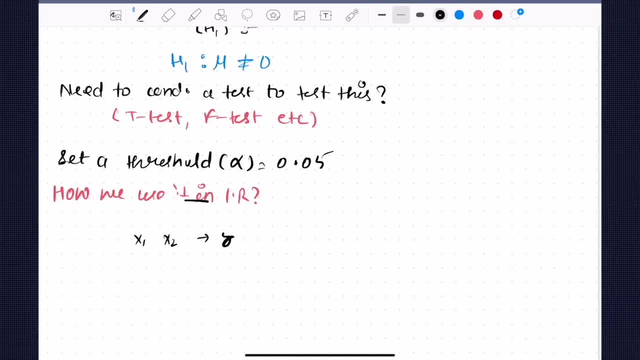 See example X one and X two and they're getting the Y. So so, basically, you identify the relationship between both of them. So if there is no relationship, then your machine learning model will be not able to perform well. So you can tell to stakeholders that there's no relationship with the N into the uh number of hours a particular student study, that that, whatever number of our student the particular study uh, it will not affect exams. 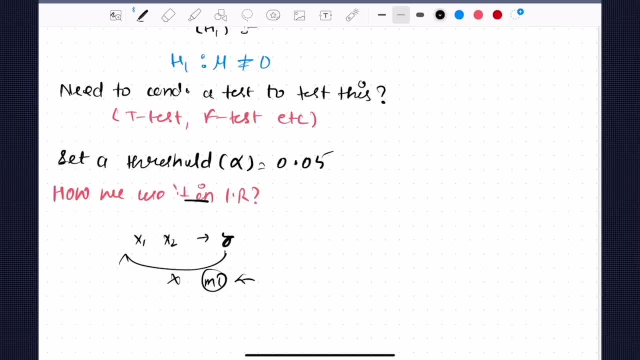 Course, exams course will be the, according to some of the factors. Okay, So this can be one of the possible factors. So, if we should first of all, uh, Make sure ourself that there is a relationship, Okay, This is, this is one of them. 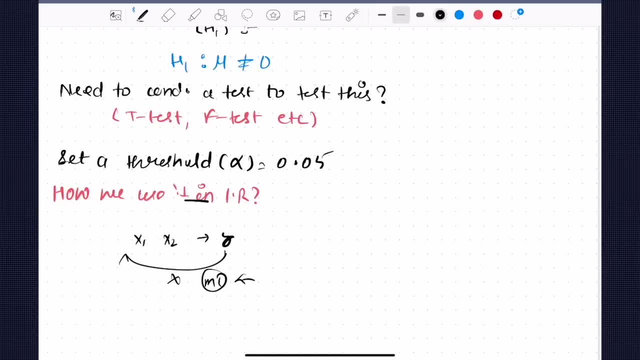 So there is a religion. How can we identify there is a relationship between input variables and output variables. We can identify the relationship between the input variables and output variable by identifying the significant, the significance of our input variables to our code variables. Okay, 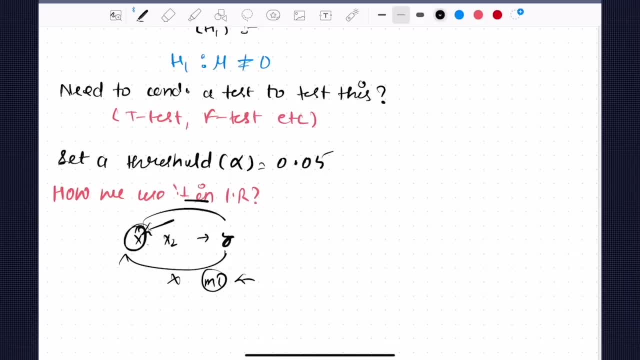 So we can say that okay. Okay, So this is a. is this significant to our output variable? Yes or no? Yes Or no? Is this significant? or output variable: Yes, No, X one is significant If is is. so question is: 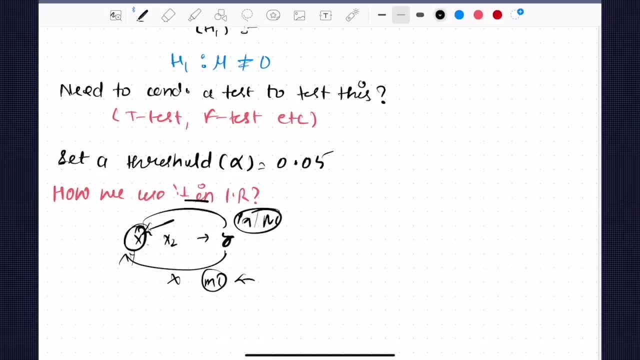 Is is your number of hours study is significant to your exam scores. So this is the hypothesis formulation. Hypothesis formulation: what does it say? It says that there is a relationship. there is a relationship, there is a relationship between input and output variables. 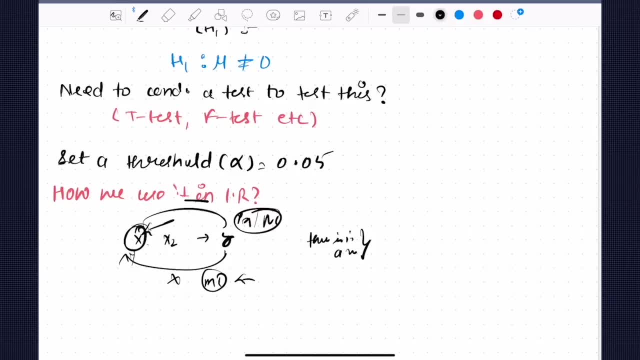 or independent features and dependent features, okay. And then we go to the X2 and then say, okay, is this something related to? is this something is the X2, is the attendance is also significant output variable. Well, yes or no, okay. 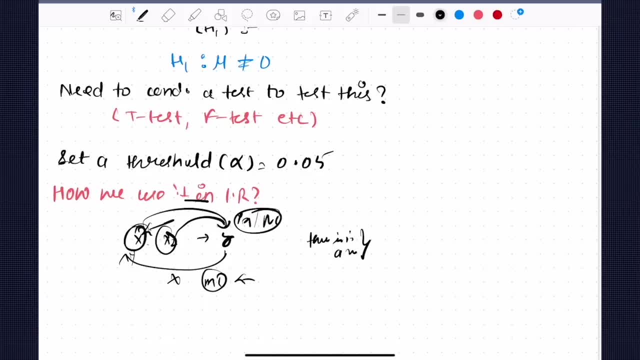 So this is how we- this is why important- because we want to identify: is there any relationship? and assume that X2 does not have a significance. So we can drop this column, we can drop this feature. If we drop this feature, it will definitely help us. 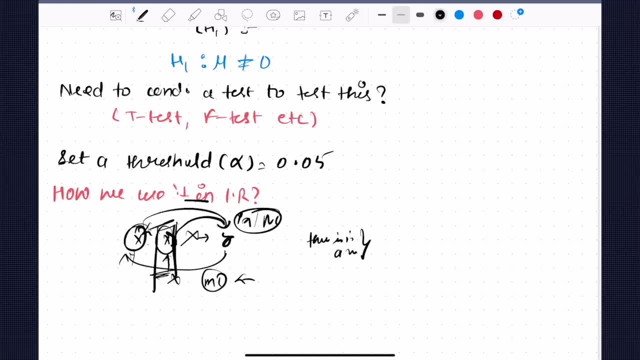 in getting the robust model, because this is just unnecessarily over here, because it's not contributing to your output variable, does not have any relationship with output variable. Understanding what I'm trying to say? I'm just trying to convince you. just I'm trying to convince you that there is a relationship. 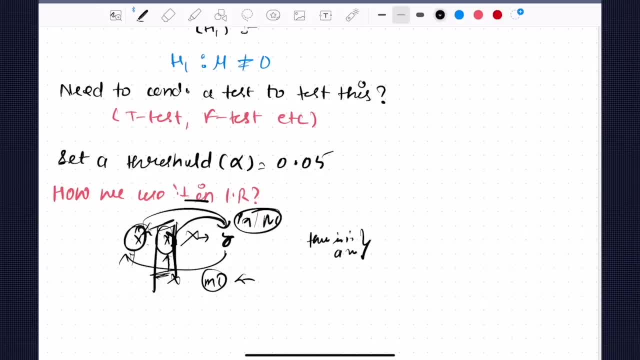 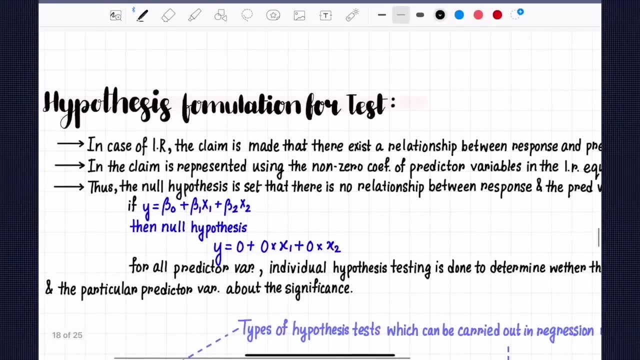 there is a relationship. there is a relationship If there is a relationship. that's the build of a hypothesis formulation. We'll talk about all of this in great detail, but you can understand There's exist a relationship between the response with the Y and the predictor. 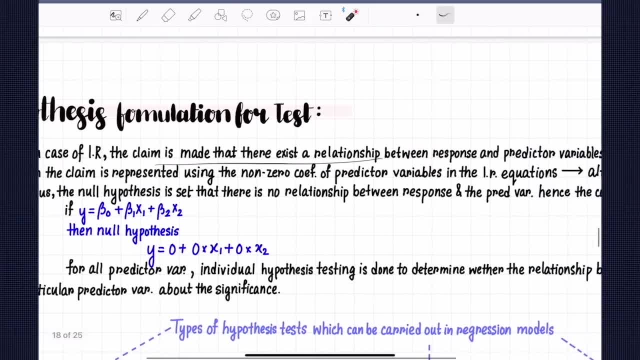 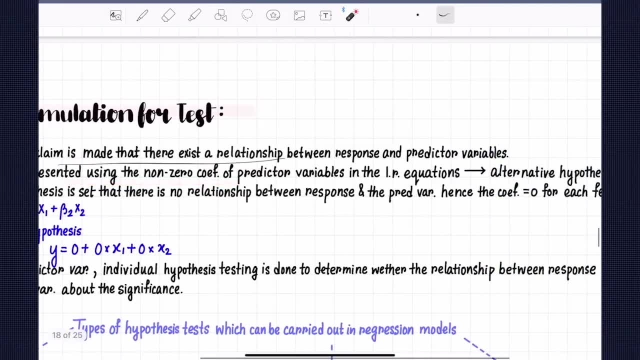 So that's the hypothesis formulation. okay, So the formulation of hypothesis says that if the claim is represented using the non-zero, then the alternative, this is the alternate hypothesis. and if your beta value, if your beta value is the non-zero, 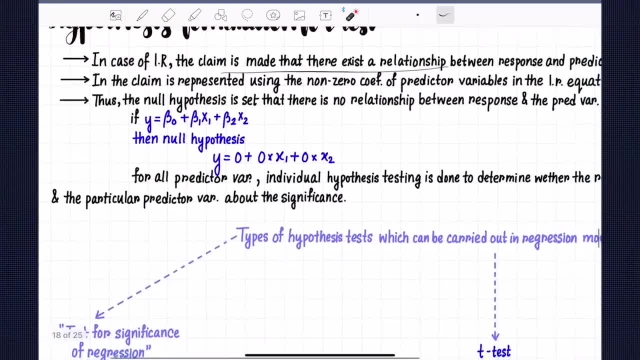 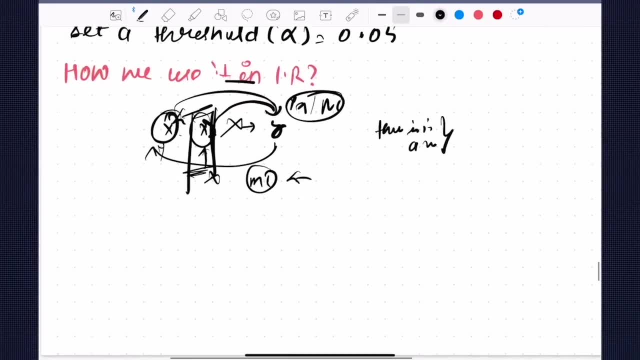 then this is a null hypothesis. I know you didn't understood anything. Let's talk about what exactly that statement says. So what will be our null hypothesis in this claim and what will be our alternate hypothesis? Null hypothesis says null hypothesis means 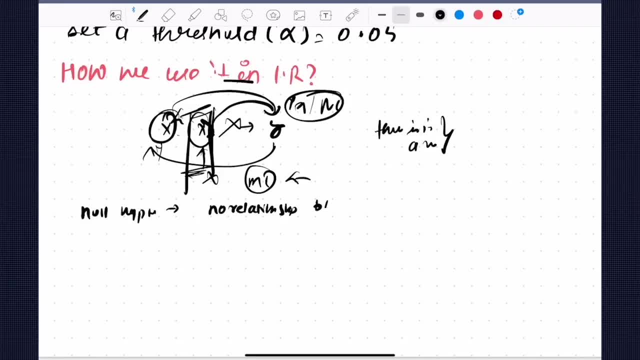 that there are no relationship between whom? Between your independent X1, X2 and Y. There's no relationship between X1 and X2, Y. And what is the alternate hypothesis? Alternate means completely independent, Completely opposite. okay, That there is a relationship. 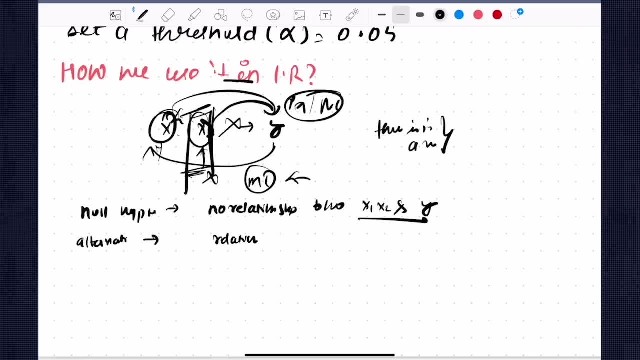 There is a relationship between X1 and X2 and Y. Okay, So now, how can we say that? How can we even make it more mathematical? So null hypothesis. can we say that null hypothesis where your beta 1 and beta 2 are equals to 0?? 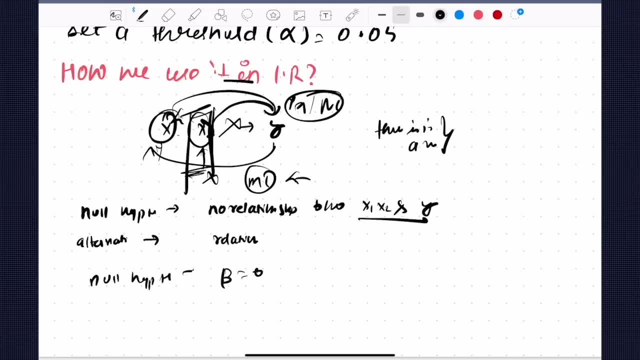 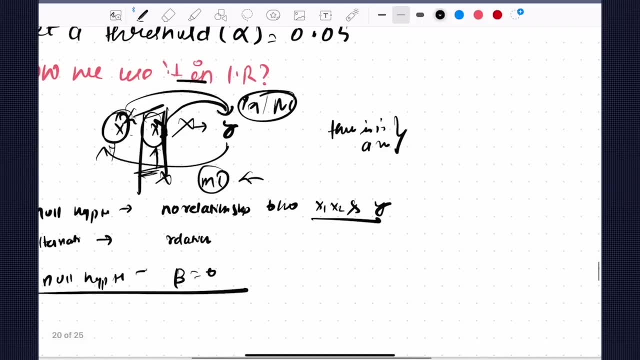 Or we can say: all your betas are equals to 0? Or all your beta 1 and beta 2 are equals to 0? Null hypothesis means so. if so, for example, let you. I know it's very simple to understand the concept. 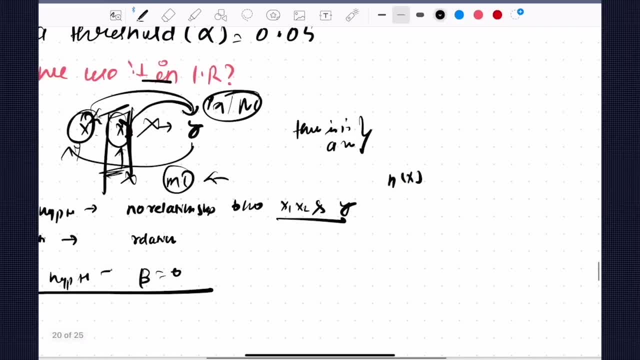 Please apply your mind now over here, That you have your hypothesis, which is beta 0 or beta 1, beta X1 plus beta 2, X2.. Okay, you're understanding. So if we say that, if we say that, 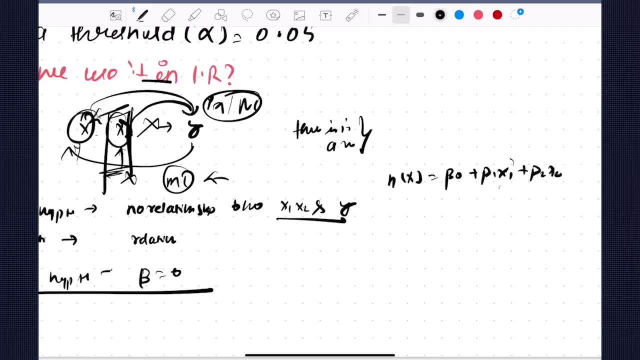 that if, if, if there is, if there is no effect, if there is no effect of this in output variable, which means that this is equals to 0,, this is equals to 0.. Bro, I'm just trying to say that. 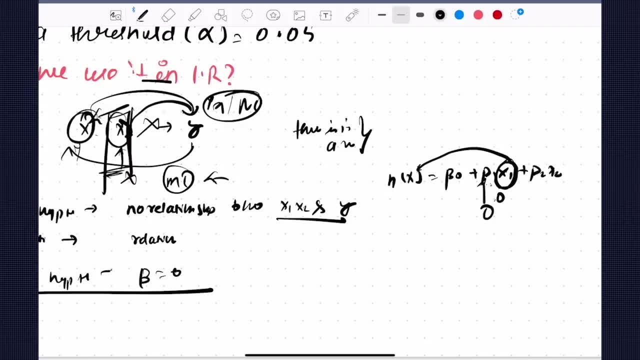 If, if this is equals to 0, that means that will yield to 0 and that will does not. that will not affect your output variable. But what about eventual null hypothesis saying that your X1, X2 does not have any significance, right? 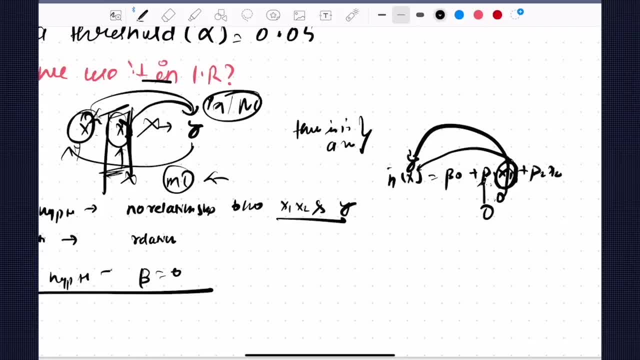 So if your beta 0 is equals to 0, that means that X1 does not have any significance. If your beta 2 is not is equals to 0, that means X2 is also does not have any significance in output variable. 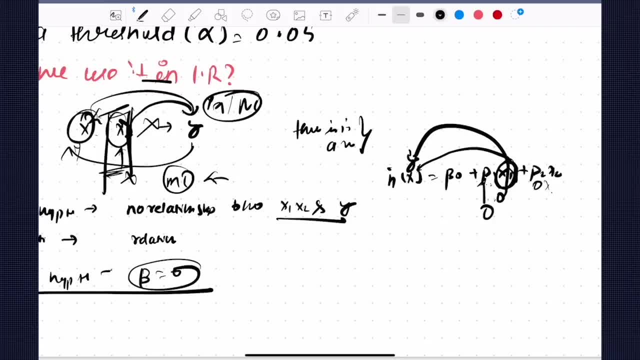 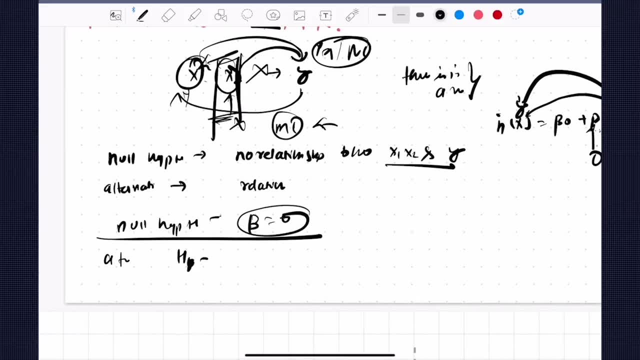 Okay, so your all betas will be equals to 0.. In null hypothesis, all betas are equals to 0. in null hypothesis, An alternate hypothesis says that alternate hypothesis, which means that all the betas are not equals to 0,. 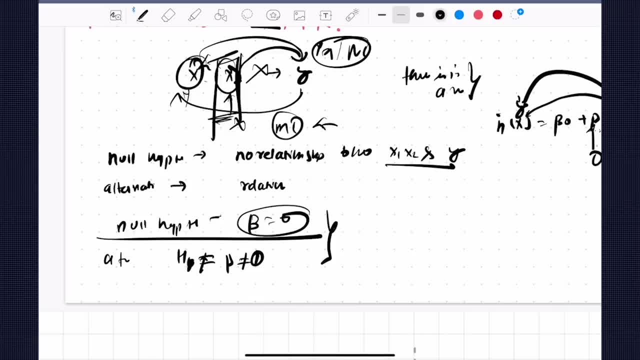 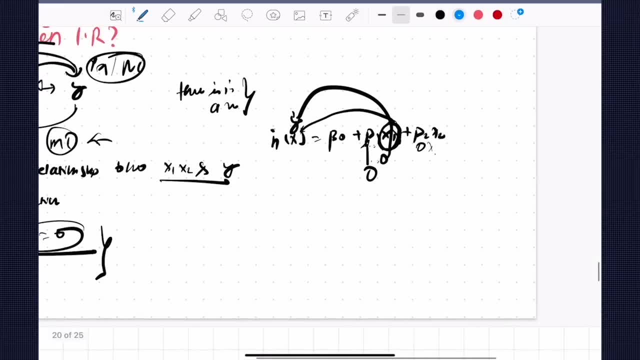 are not equals to 0. That's your hypothesis. this is your hypothesis. Now you might be thinking a bit of how this, how this is coming Again. I'll summarize it for you: That your H of X is nothing but equals to beta 0. 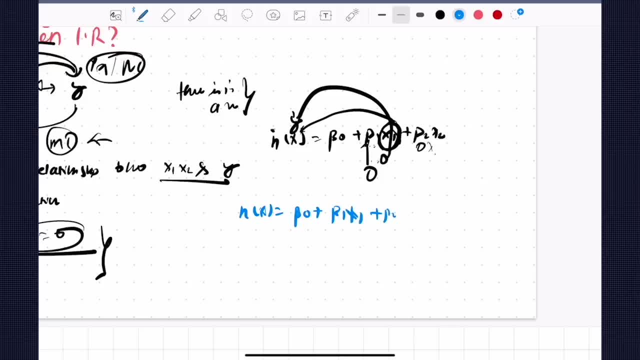 plus beta 1 X1, beta 2 X2.. So null hypothesis. What does it say? That there's no relationship. If there's no relationship, that beta beta 1, if we make beta 1 to beta 2 to be equals to 0,. 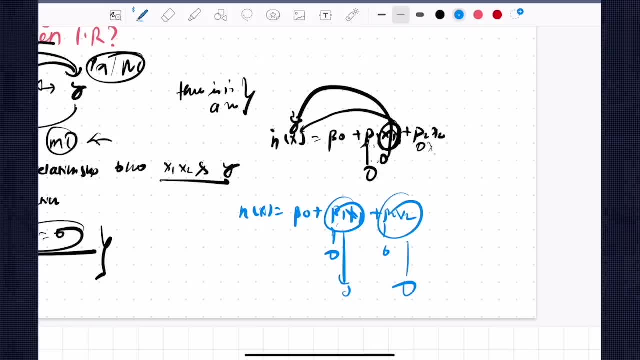 that means it will. it will be whole yield to and this will whole yield to 0. Which means they're not affecting any output variable. Right, But what if? if there's, if there's something out of 0, that is alternative. 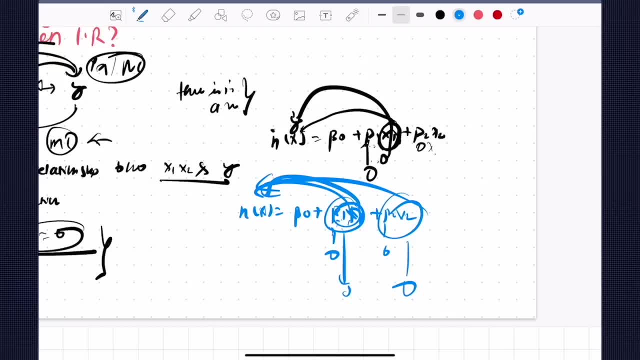 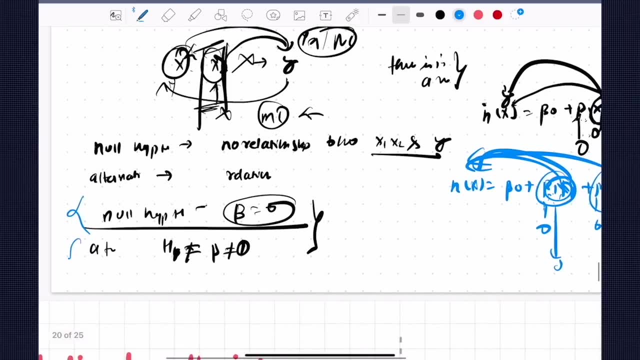 which means that that it is affecting some sort of output. It is affecting some sort of output variable. So in null hypothesis we say that all our beta value are nothing but 0, but alternate, all our value is nothing but not equals to 0. 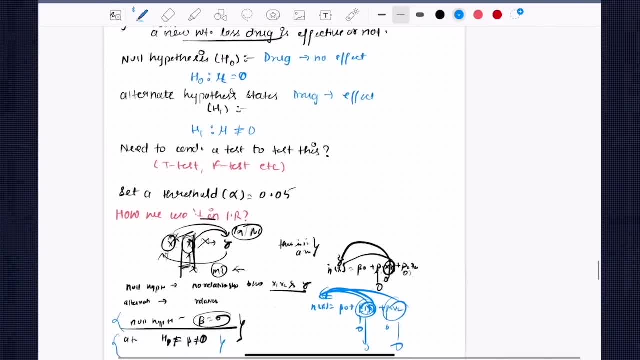 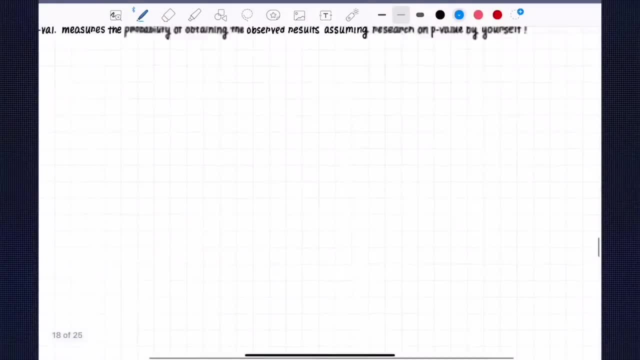 This is our hypothesis formulation in linear regression. I hope that this gives you a very good understanding about what exactly we we aim to start solving about this. Okay, So, so now you can see that if everything is equals to 0,, 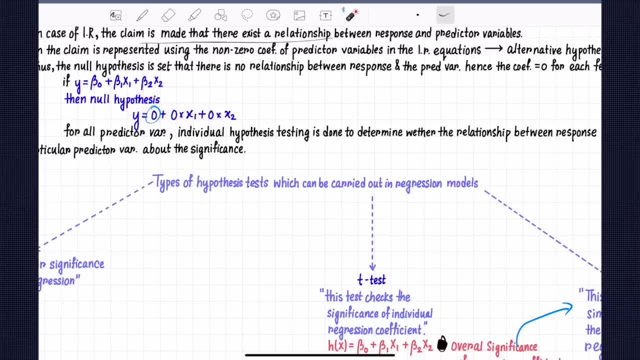 if everything is equals to 0, that means this is a null hypothesis, which means that does not have any output, that does not have any consequence on output variable. But if there's not equals to 0, that means they have a consequences on output variables. 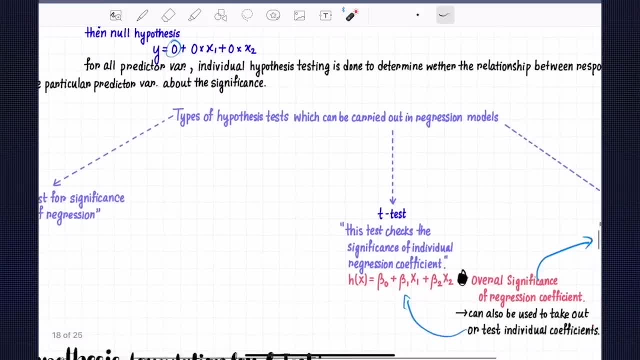 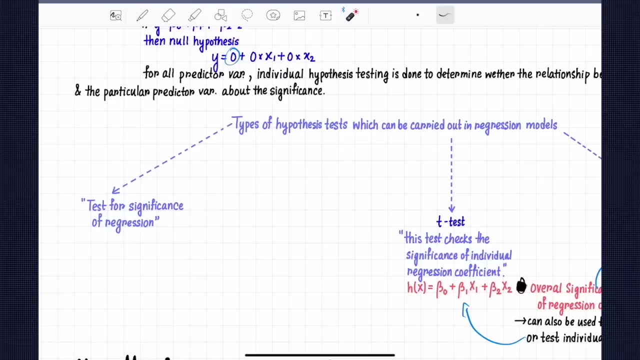 So there are three types of tests we should talk on. which is test for significance of regression? Is it a regression problem or not? Maybe it can be easily classified when we'll talk about. maybe it can be easily classified when we'll talk about. 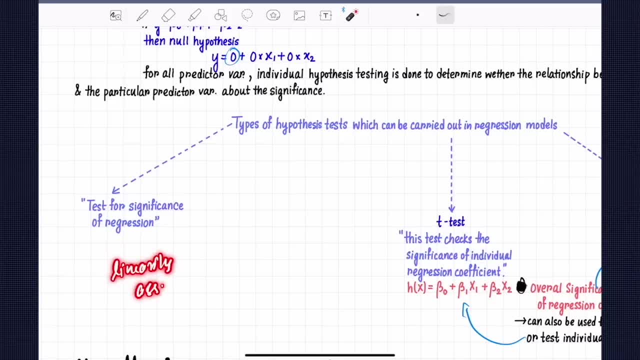 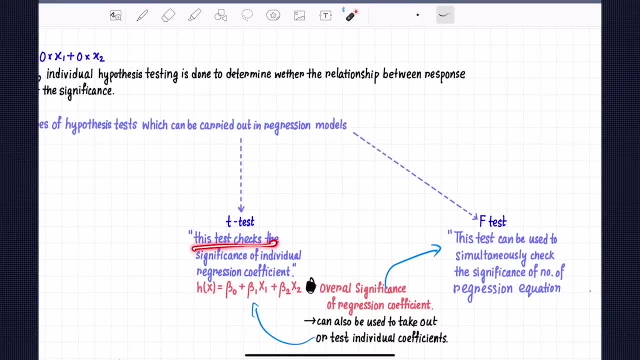 maybe it can be easily classified when we'll talk about linearity assumption. It can be easily talked about linearity assumption, which we'll see that later on. One is test t-test, which checks the significance of individual coefficient, regression coefficient. 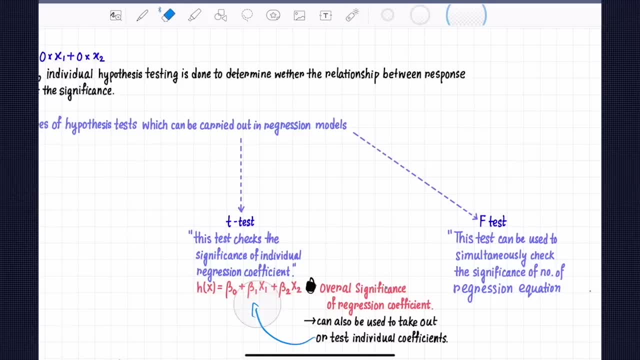 So what does it tells? So what does it tells? I think I did a bit wrong. Yeah, yeah, So it. what does the t-test? does T-test, as I said, that we have an hypothesis where our s0,? what does a null, null hypothesis indicate? 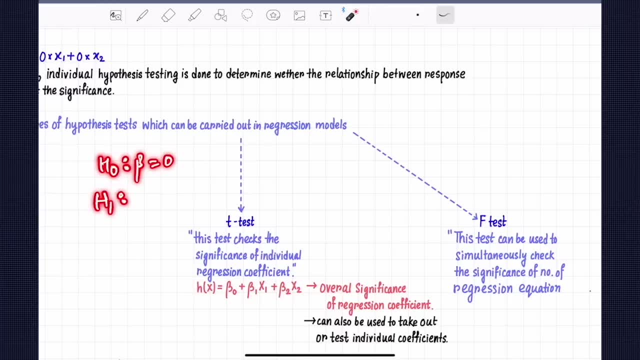 That our beta value is nothing but equals to 0.. And our alternate hypothesis. what does it indicate? Our beta value is not equal to 0.. It's not equal to 0.. This is our formulation of our hypothesis testing, which we're going to test. 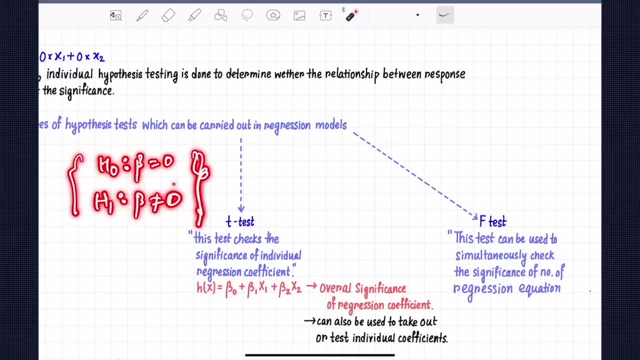 Which we're going to test. So in a test we're going to test whether there's exist relationship or not. So we have a test right, We conduct a test and then we get some certain value. let's assume c. 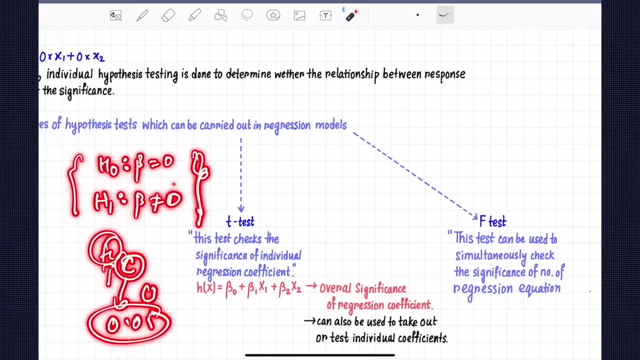 So if that c is smaller than 0.05, is smaller than 5%- we'll talk about that- this again significance, just in a second- But if it's smaller than, then we say that we say that we reject the null hypothesis. 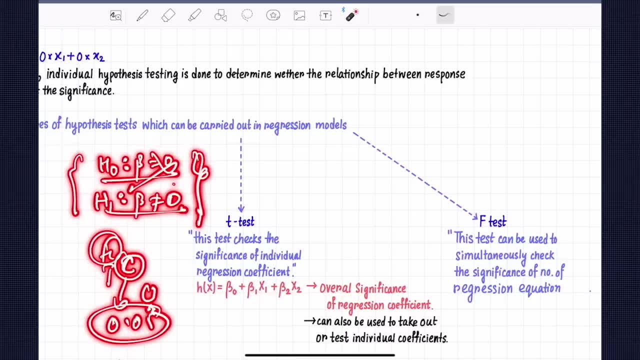 that means there's a null. we say, except that there is a relationship. But if it is greater than 0.05, that means that we reject the alternative that there's no relationship between the variables. Okay, Reject this alternative, and then we accept this. 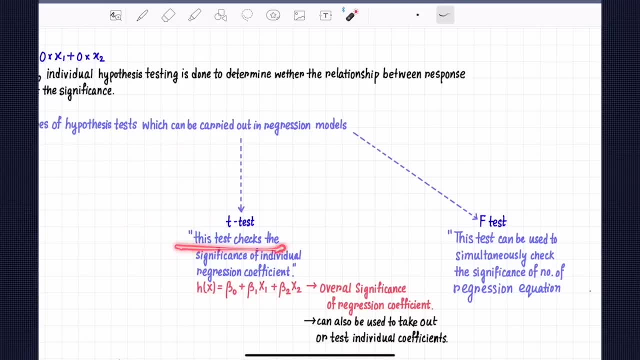 We'll talk about the significance just in a second. So this test checks the significance of individual regression coefficients Individually, okay, Not something like it checks that whether this x1 is significant to output variable or not, or whether this x2 is significant to output variable or not. 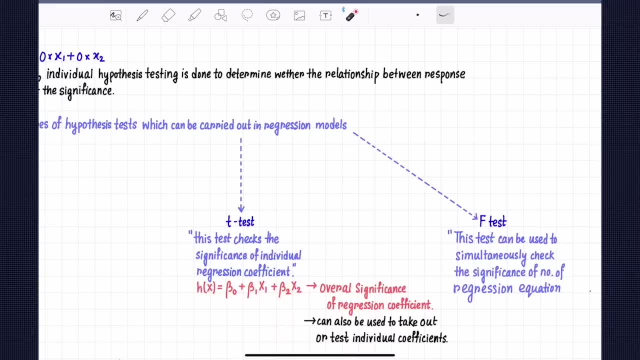 How does it check That? if your beta2 is is equal to zero, so your hypothesis will be a zero where beta2 is equal to zero, and h hypothesis, where beta2 is equal to, is not equal to zero. So this is a hypothesis. 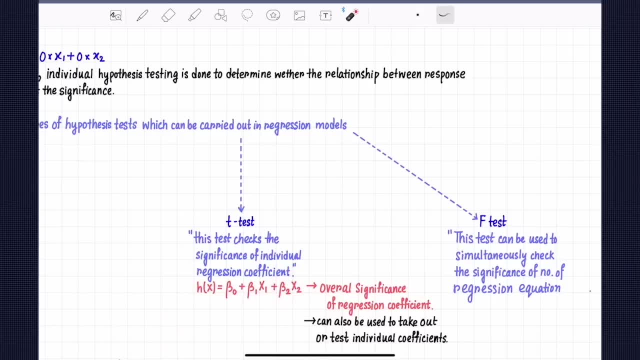 It checks individually, It checks individually and once it checks individually, we can easily take out the overall significance. Okay. So if we take out individual significance, then we can easily say, okay, this x1 is not significant, then we can remove this x1.. 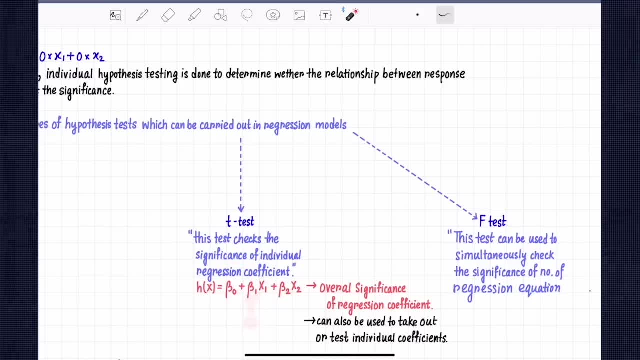 How can it? if the beta1 of x1 is zero, that means that it is not significant. And then we have something known as t test, and then we- sorry f test, and f test is used for taking out the overall significance. 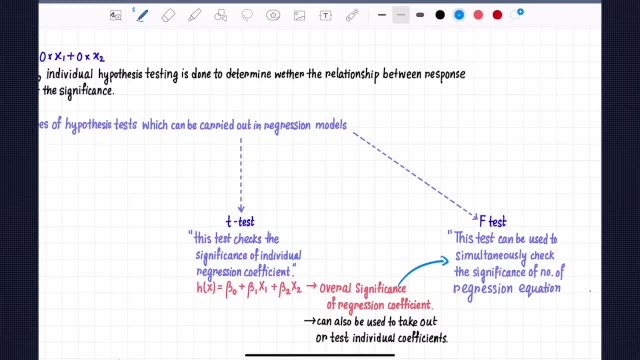 the overall significance. overall significance of your regression values overall, which means whether this overall equation is significant or not. Okay, Significant means overall, so the hypothesis formulation would be: the null. hypothesis would be: beta, all the beta values and the null alternative. 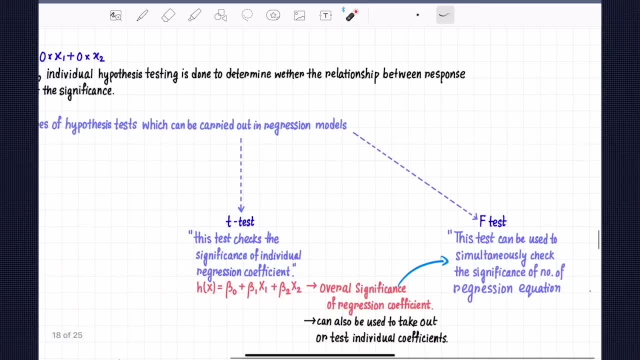 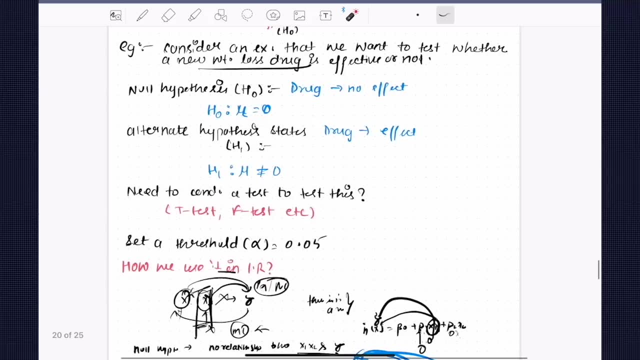 which is all the beta values, not equals to. this is the hypothesis formulation: Three tests. let's talk about the first test. t test, f test will be left upon you to explore. I hope that I'm giving you a very great knowledge out of it. 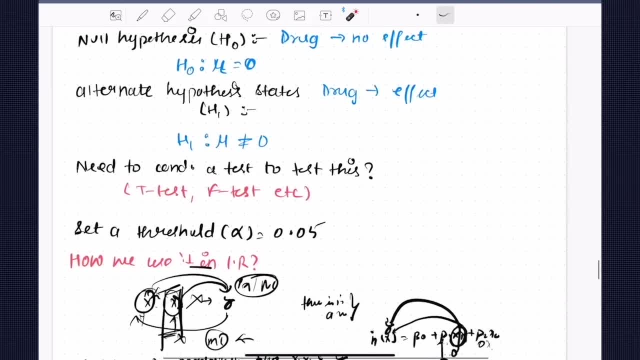 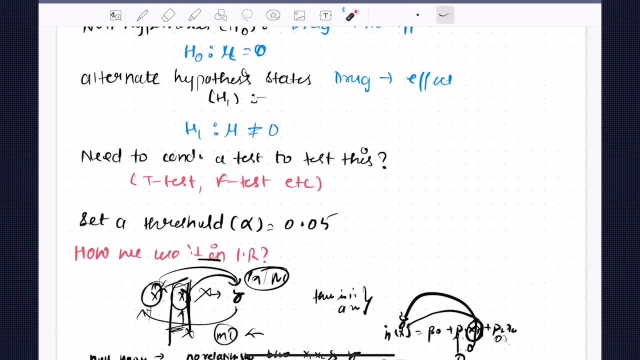 And I really hope that you'll utilize this information, because for me, it takes a ton of time, you know, to develop this And I hope that you will, that you will, that you're enjoying this force out till here And, if you are, till here, 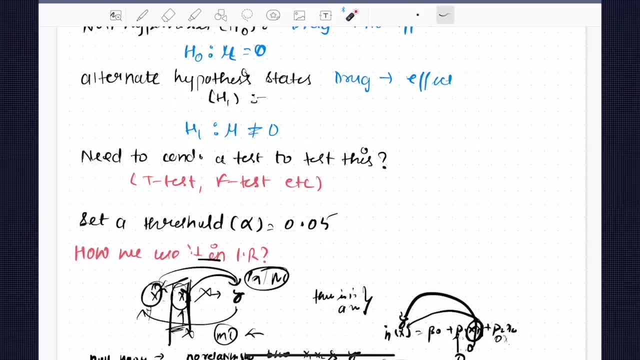 that means that something you are a special guy. you know that you're a special guy and you're always up for ready to take challenges out there, Okay, cool. So now I've been talking about something known as significance value. 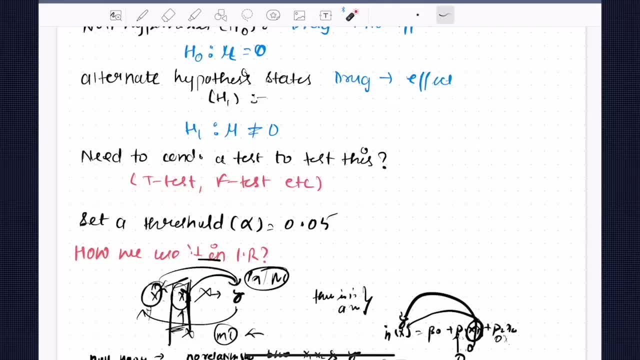 So we'll conduct the t-test. So how can we? how can we conduct the t-test? So there are some steps for conduct, for conduction of a t-test. I'm directly going to the you know t-test formulas, so that it is. 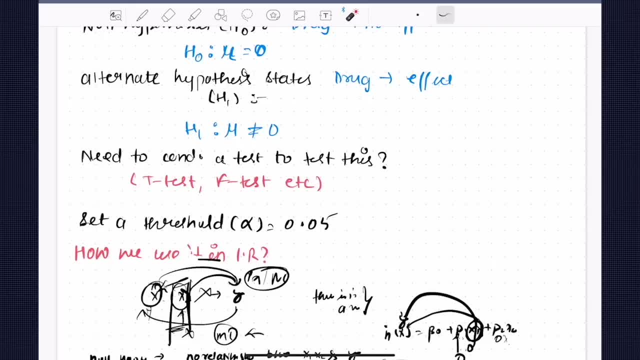 it will make much more sense to you only when we'll do one example. Okay, So let's go to one t-test example. Yes, So you're. so you're first, so you're basically again, I'll just write the t-test example. 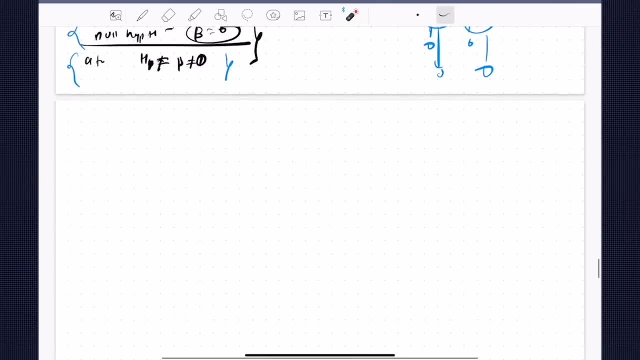 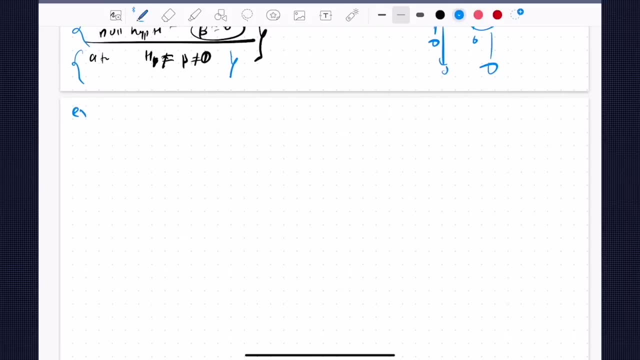 so that it makes much more sense. Yeah, So your. so your hypothesis formulation is. hypothesis formulation is, so assume that let's take an example, because I really like to take examples in every bit, whatever I'm explaining, because that's something is. 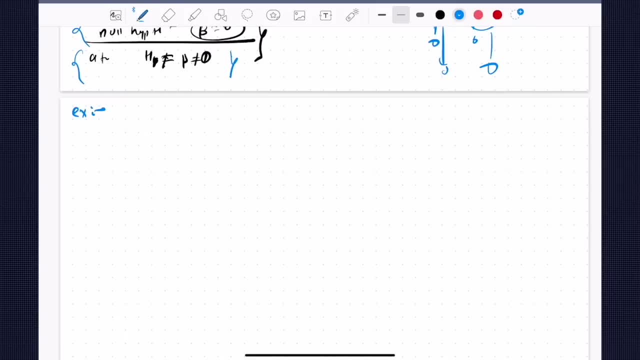 makes me motivated to, like you're able to understand, by the simple examples. So example what does? example says. Example says that you want to build a simple linear regression model. We'll build a simple linear regression model. we'll build a simple linear regression model. 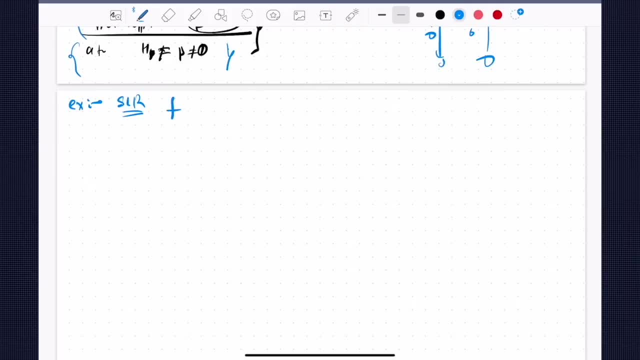 And what does that simple linear regression model do? It will build a function f. build a function f that takes in the, that takes in the square footage, the square footage, or you can see the size of the house. size of the house. 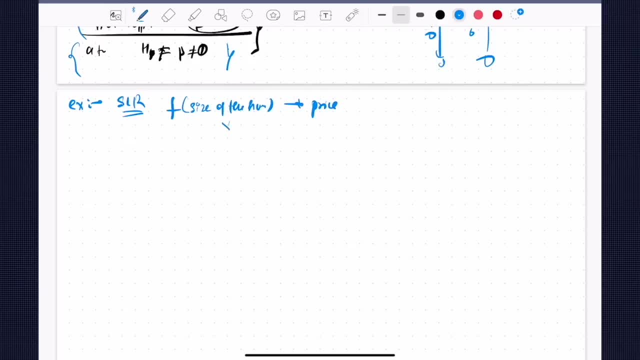 and predicts your price and predicts your price. So, given the x value, so you're gonna predict y. I'm just taking a simple linear regression to make you understand. So, in this case, what will be our null hypothesis, Null hypothesis. 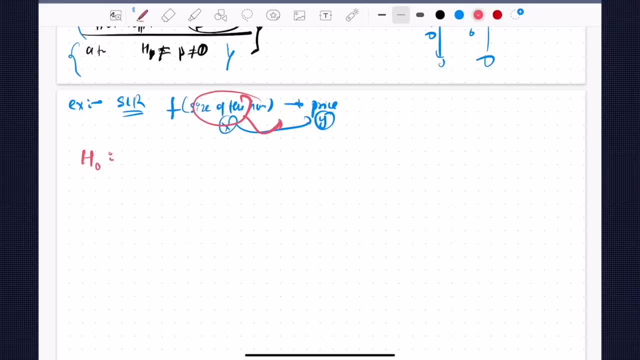 which means you don't have significance to output variable, which is null hypothesis. nothing but your beta one. beta one is equal to zero, Okay, And alternate is means that your beta one, which means the beta one. 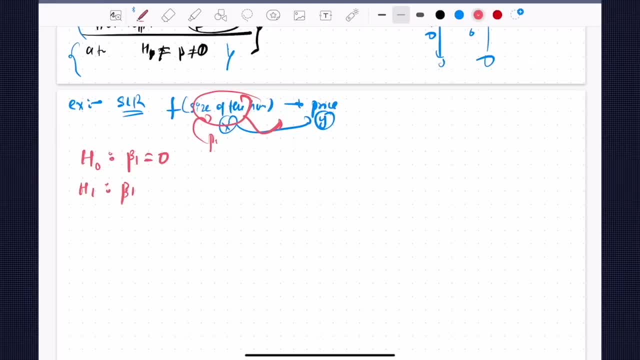 which is the beta one is the say: is the coefficient of this x one right Beta one is not equal zero, which means that there is a this. this means there is there is no relationship, no relationship, relationship. 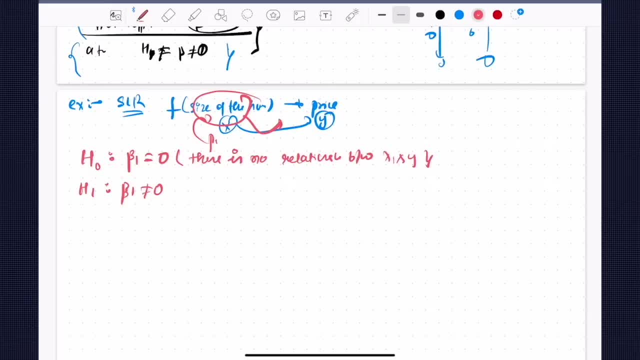 between x one and y, which means that no relationship between size of the house and price. size of the house does not affect size of the house does not affect price, And this there is. this alternate means there is a relationship between x and y. 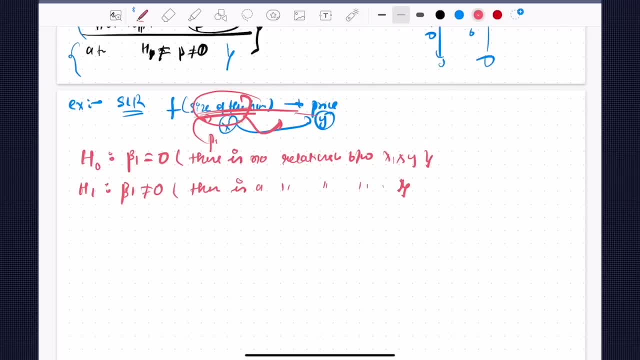 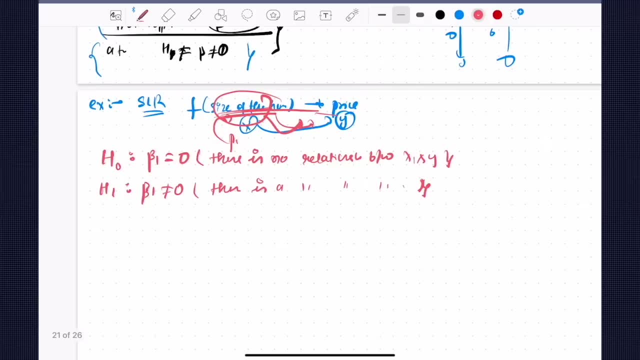 That means that that means that there is a relationship that size of the house definitely affects this price. Okay, So when you fit, when you fit the linear regression model, when you fit the linear regression model, you have the following equation: 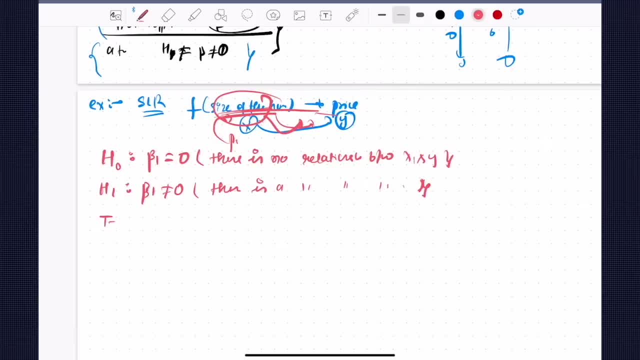 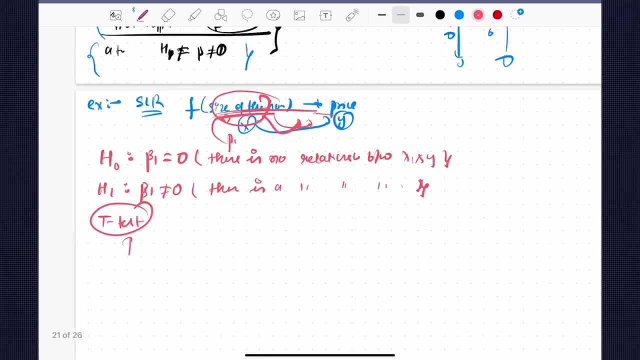 Now what you do, you calc, you do the test, Now you do the t-test. How we'll do, we'll talk about just in some seconds. but the formula for calculate, for the formula for doing the t, for the formula, 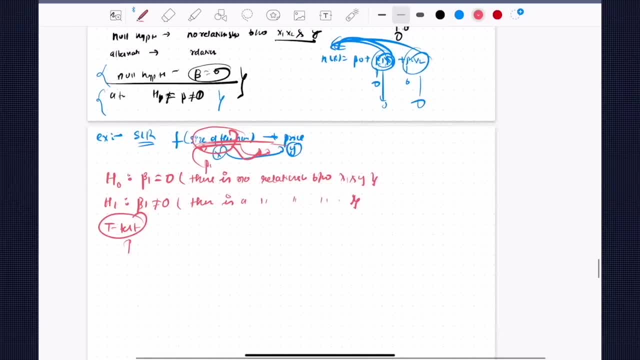 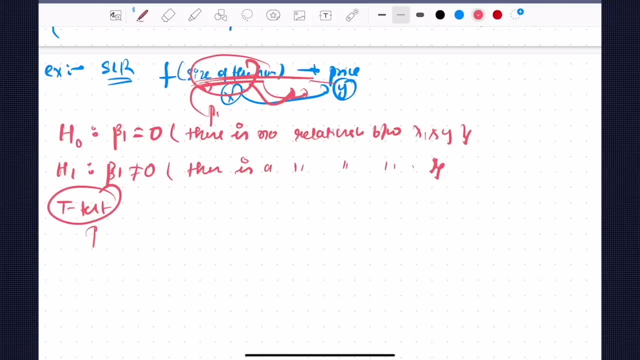 for doing, for for for doing this test is we is we do individually for every parameters. right, If we do the individually for every parameters? So the t, we calculate the t-statistic, the t-statistic for whom? 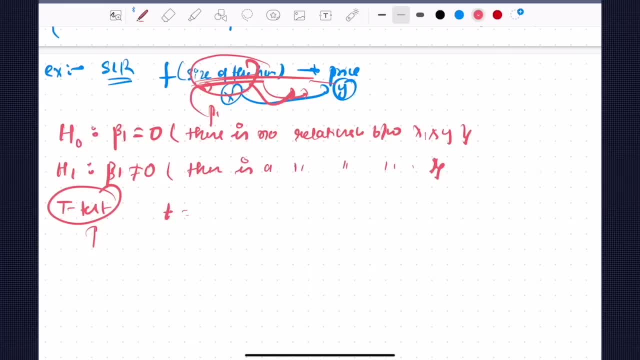 T-statistic for the size of the house because it does individually assume that it assume. so we'll take, take out the t for every individual parameter. So currently I'm doing for only one. So it takes a t-statistic for the size of the house. 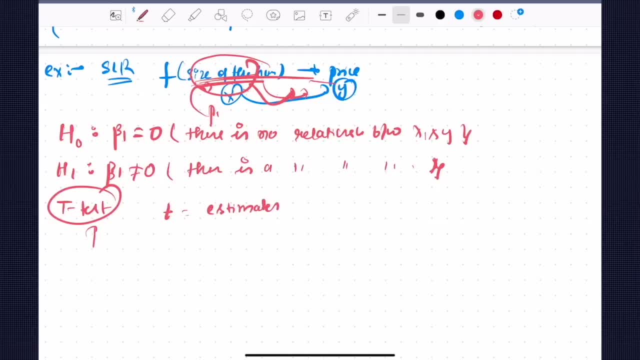 which is estimated coefficient. estimated coefficient: the coefficient value. So in this case it will be beta one minus zero. beta one minus zero divided by the standard error of that beta one. A very nice equation of very confusing to a lot of people. 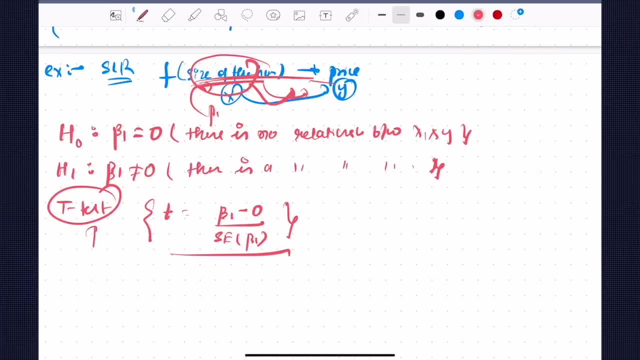 Now let's talk about: why does that confusing? And let's talk about each and every integrity of it. Okay, Each and every integrity of it. So we'll talk about: are we subtracting it? why are we dividing with standard error? what is a standard error? and yeah, 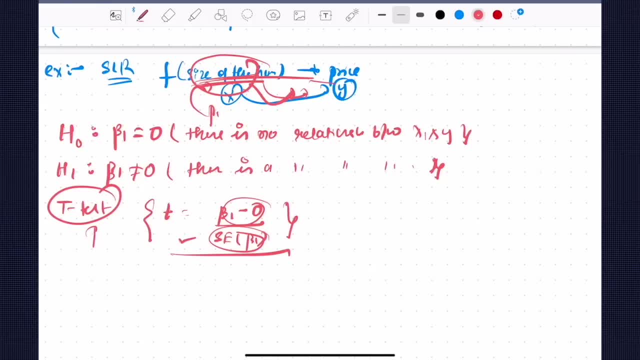 so and and and after conductor, after conduction of this test, what we do so that it makes much more uh sense to you in your initial stages as well. okay, so let me just let me just open my uh form uh calculator, because this is something which i'll be required, which will be required. so let's first 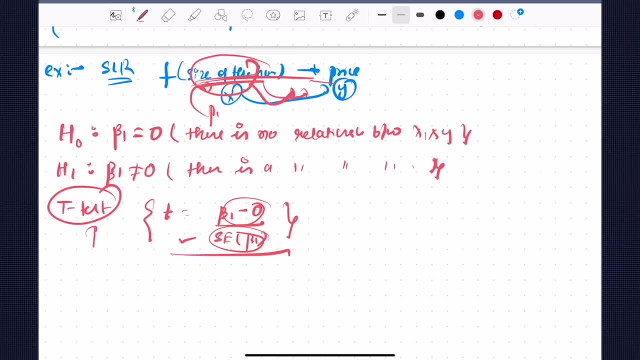 of all talk about. let's first of all talk about the general formula. so the general formula for calculating the t? t value to a statistic, for a particular beta, for a particular beta, is nothing but estimated coefficient. there's coefficient which is estimated because we have to take every this hypothesis. testing only can be tested if you, if you have a fully trained 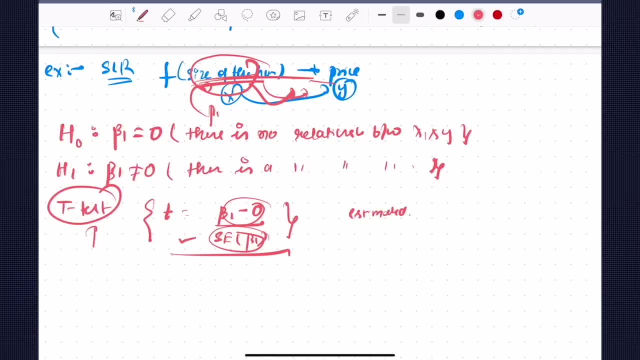 model so that you can test your hypothesis. okay, estimated coefficient minus 0 divided by standard error of that coefficient, standard error of that coefficient. so what does it measures? what does it measures? so what we don't saw? what we saw is that in the theory of sign母 10 we had the 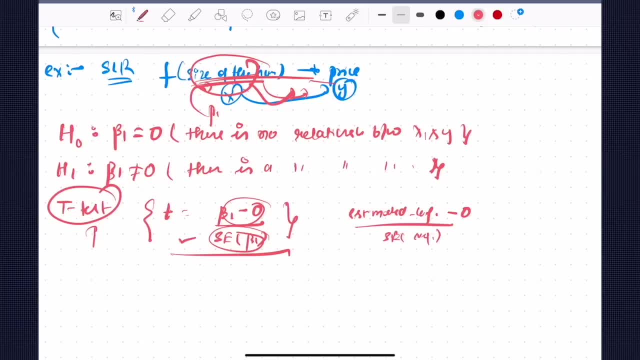 do what we are doing over here. so basically we are calculating the t statistic and then we are subtracting the hypothesized value from the estimated coefficient. so you might be thinking: what is hypothesized value? this is something which is confusing to most of the people, so 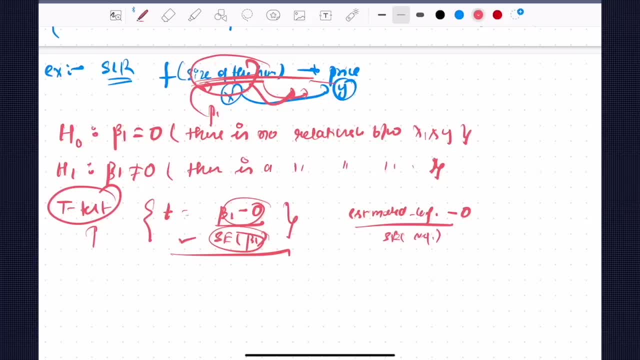 hypothesized value is the value of a coefficient under the null hypothesis. so we first of all assume: okay in, uh, basically what? basically what we do: we hypothesize something, we make a, we make something like true, like there is a no relationship. we prior to assume that there is no. 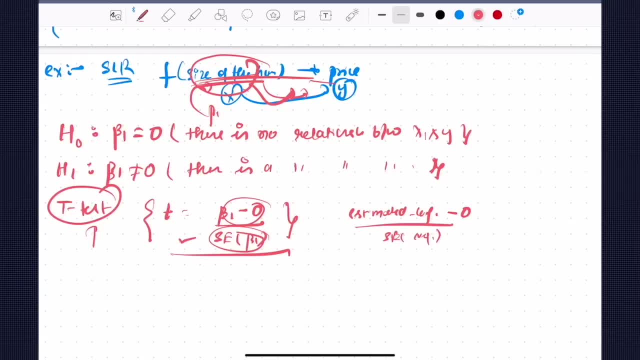 relationship. okay, and then we disprove that. and then we disprove that. so hypothesized value is zero in this case. because your hypothesized value is zero, okay, so estimated minus the hypothesized value, which means the value of the coefficient under the null hypothesis. okay, this. 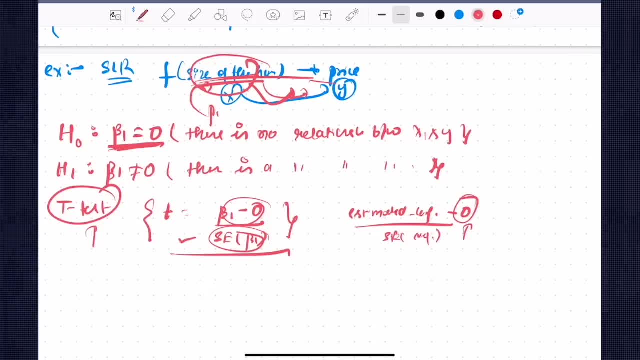 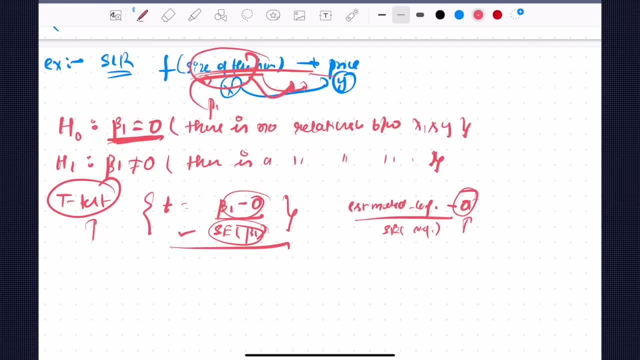 is the hypothesized value which is under the query. and so if, if the beta one is equals to five, that that means you have to write a five over here. okay, if the in but but, but you should, but it should be a null hypothesis. so we pre-assume things, that we that that that we already assume that there's no. 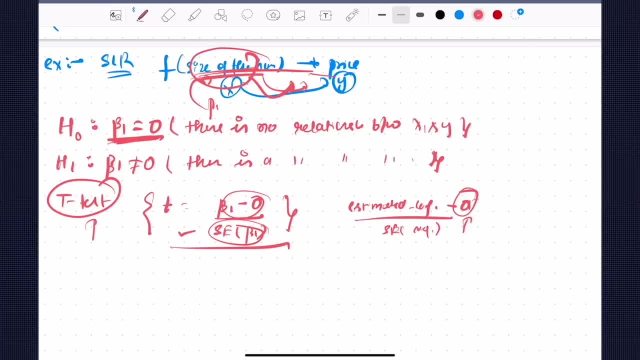 relationship. now we disprove that, uh, with, with, with t statistics. so if you're not able to disprove that, that means there is no relationship. but if you're able to disprove, then we accept the alternative hypothesis. okay, so over here, this is usually that there's no relationship. so basically, 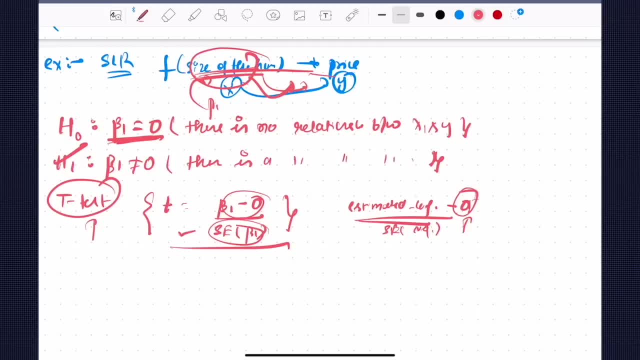 we subtract the hypothesized value and then we divide by the standard error. so what does a standard error means? what a standard error means? so let's just go and talk about- uh, let's just go and talk about a very nice explanation of standard error, because this is something also also people 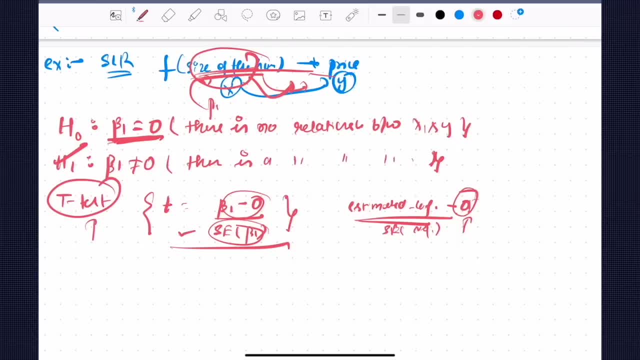 you know uh worry a lot about. so standard error is nothing you know uh worry a lot about. so standard error is nothing you know uh worry a lot about. so standard error is nothing, is nothing. but um, uh, it's, it's, it's nothing but accuracy: the accuracy of an estimated value, the accuracy or how much uncertain, or how. 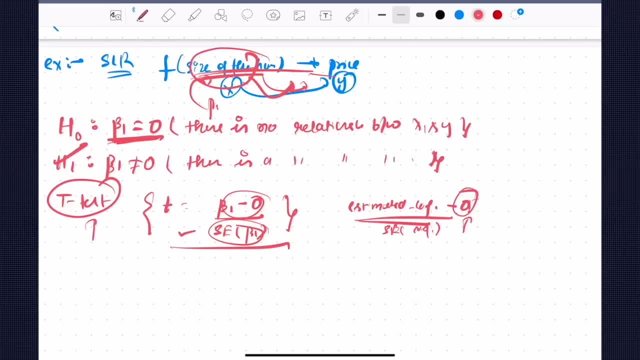 much uncertain your uh regression coefficients are. so I'll take a very simple example to make you understand about this. um, so basically assume that, uh, so assume that you built a linear regression model and the standard error is the measure of uncertainty of the estimated coefficients. and then 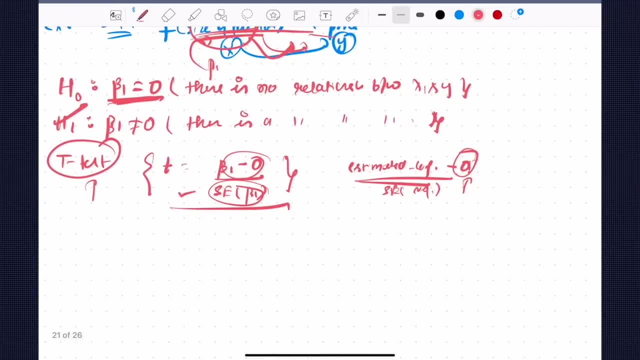 you describe the ratio basically: uncertainty, uncertainty, uncertainty means the standard error, so I'll just write it over here: standard error, it measures the uncertainty, uncertainty, uncertainty or the accuracy, accuracy or preciseness, or the preciseness of the estimated coefficients, of the estimated coefficients. this is a very important uh to talk on, that, that the standard is nothing but. 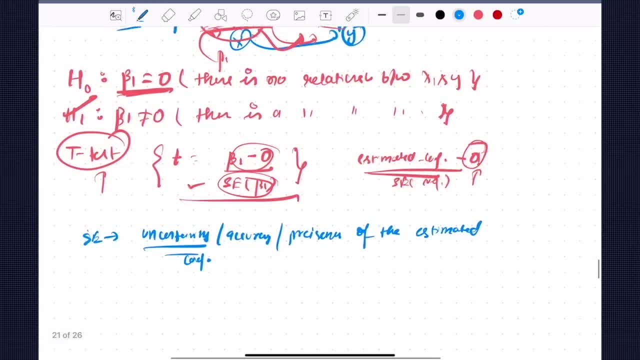 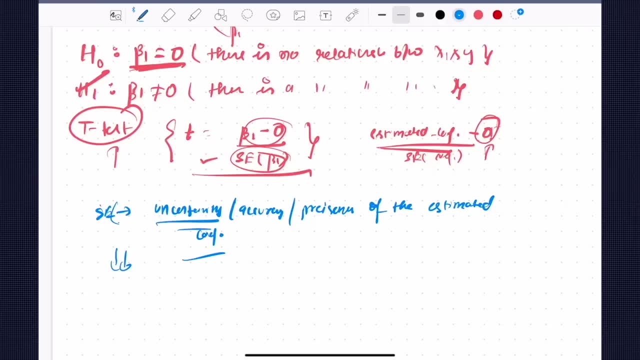 the accuracy, uncertainty, preciseness, so lower the uncertainty means better your coefficients. so basically, it evaluates. basically it evaluates how your coefficients are uncertain, how, how your estimated coefficients are accurate, how your uh, how your uh, how your estimated coefficients are precise and all. so these are certain uh, certain words to talk about. so basically, so basically, you calculate, so 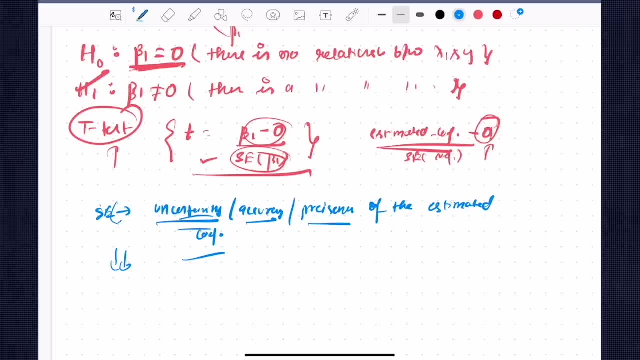 basically, you calculate and say that, okay, this is something is used, this is something is used to indicate how precise or or precise or accurate your estimated value are. okay, so again you might be. you might be thinking so you might have beta 1 equals to 2.. beta 1 is: 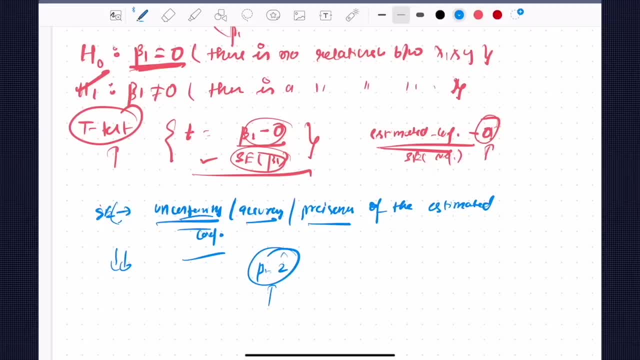 equal to 2 by estimated by your gradient descent. okay, uh, best, estimated by your gradient descent. that's one of them. so when you estimate a beta 1, so how precise, how much? how much precise this is? how much precise is? how much accurate this is is how much, how much uncertainty it contains, how much. 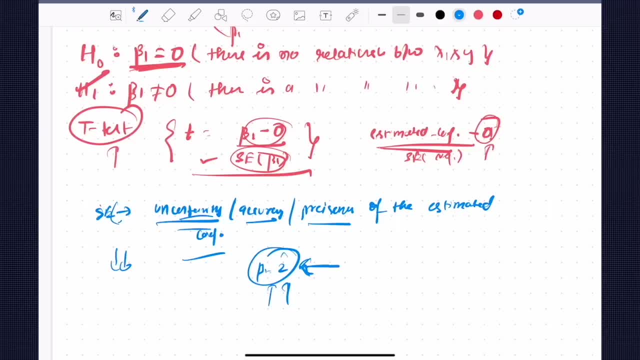 how much we are sure about this. we quantify that. so we quantify how much we are sure about that. we quantify how much we are accurate about a particular beta value. that's what the standard error means. standard error means how much we are sure about that particular beta value. okay, how much you're. 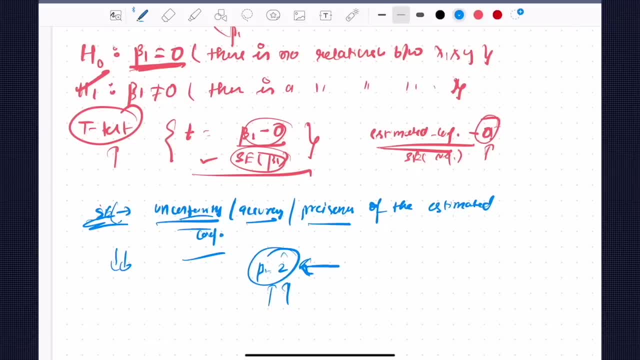 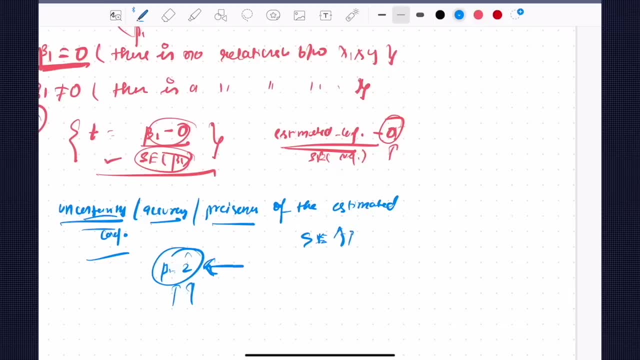 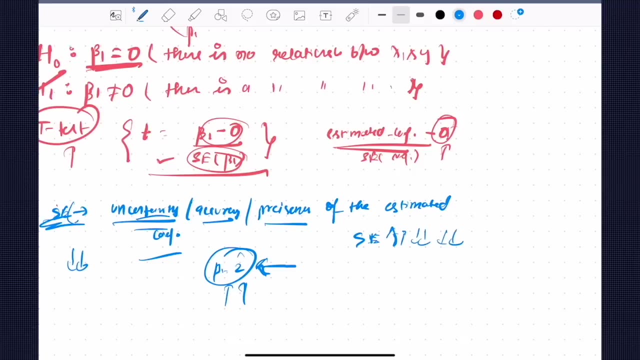 sure about that. I hope that it, that I hope that it gives you. so, if your standard error is high, if your standard error, if it's, if you, if your standard error is high, that indicates that there is more uncertainty, more uncertainty and less accuracy, less preciseness. okay, so if your uncertainty is, 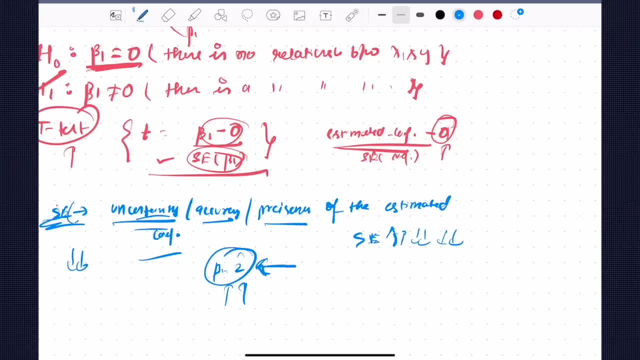 high, which means not sure about that. that means that is bad. no, if you're not sure about, if you're not too much sure about the particular coefficient, that means that that that means that there's something wrong with it. if it's super accurate with that and you and you're also not accurate. 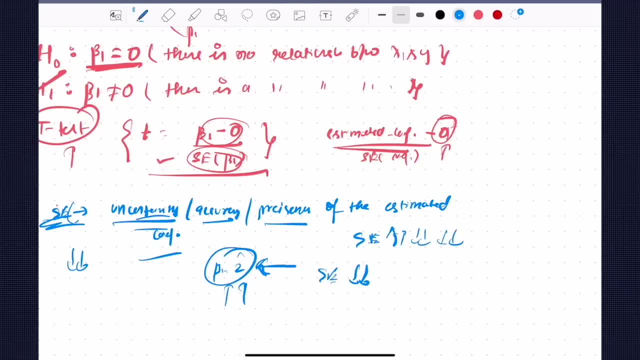 so if your standard error is small, that means that your uncertainty is low, which means you are too sure about you are able to quantify things. you're able to quantify how much sure and unsure you are if you, if unsureness is too low, which means that you're sure of that. beta values to that. that means 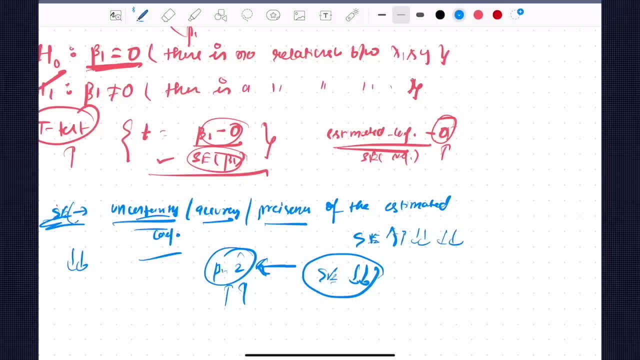 that is, uh, that is good. so your standard error should be less. so basically what we are doing. so basically what? what we are doing? we are simply subtracting. we are simply subtracting, sorry, we are simply, first of all, the. now you know, you understand this full equation. you have you. 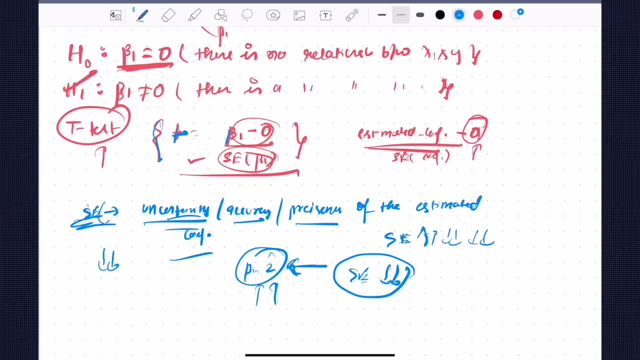 calculate the p-value. calculate the p-value which is beta 1 minus 0 divided by the standard error. so now, what does the division gives you? what does the division gives you? this is something is you, which is usually taught in the uh statistics classes, and I usually recommend you to not even uh. uh, which is the which is the which is not even. 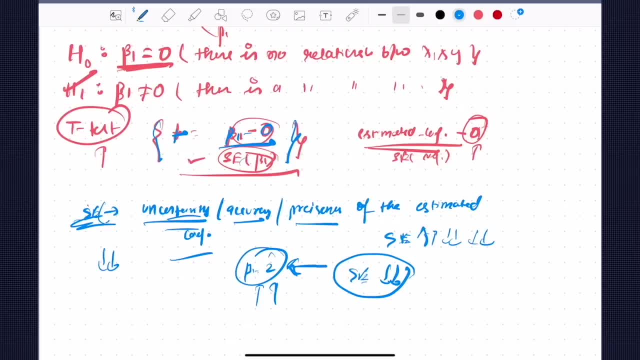 recommended for you, even if you, if you, if you're just curious, you can just go ahead and talk about things. uh, but what exactly? what I'm going to do is talk about my interpretation from what I understood, because that's something you know. I I also have to take care whether, whether I understood. 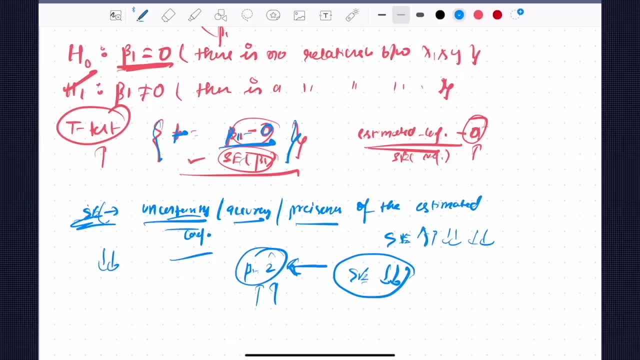 it nicely or not, right? um so, uh, let's talk about that, otherwise it will be bit off to me as well. so the t-value which you're going to get over here, the t-value which is going to get over here, which will give you, which will 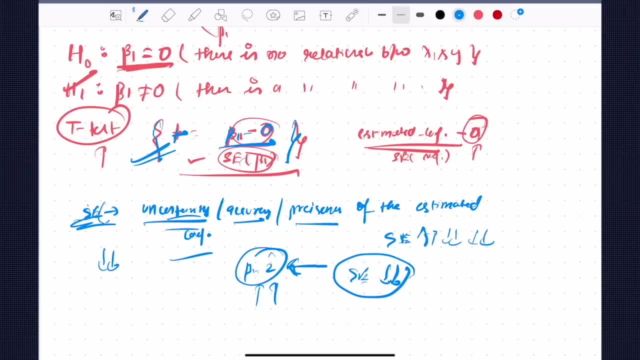 give you a number so that we can compare with the threshold we'll talk about to the threshold just in some second, just just after this topic. so the t-statistic, this is called the t-statistic, this is called the t-statistic. is the is, is, what is the? what is this test? it's helps. 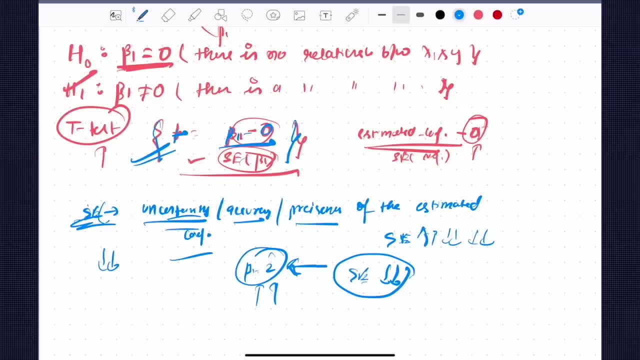 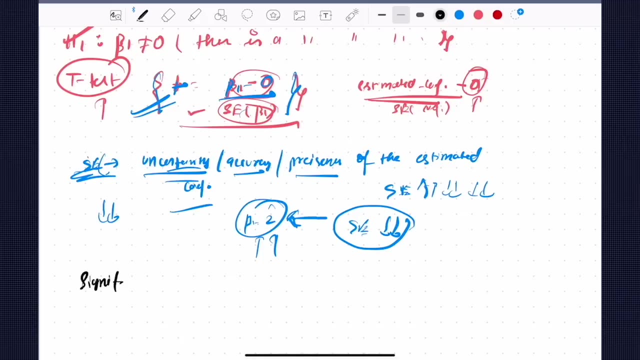 to assess the significance of the coefficient relative to the variability or the estimate or the uncertainty of our estimates. so what does it tell? again, I'm going to repeat: it tells you, please remember the significance. it tells I'm just taking in, say very, I'm not taking very mathy, you know if 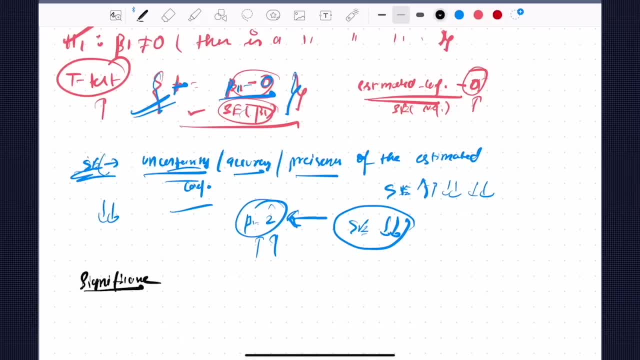 you if you go online. no, everybody is taking so mathy mathy things. I'm not able to even understand why they're taking mathy mathy things, but it tells you the significance. it tells you the significance coefficient of a coefficient relative, relative to the uncertainty, uncertainty, uncertainty of the 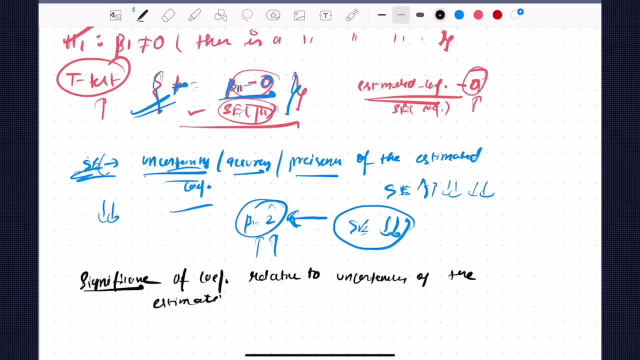 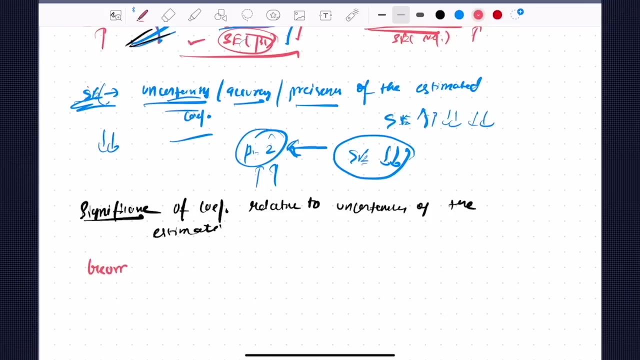 estimate, of estimate. that's exactly what it. what, what, what does it? t-test gives you in geometrically. if you understand it geometrically, it can be thought of as: how many standard errors the? how many standard errors the estimated coefficient is away from the hypothesis erised value. so again, geometrically meaning. geometrically meaning, I know this is something. 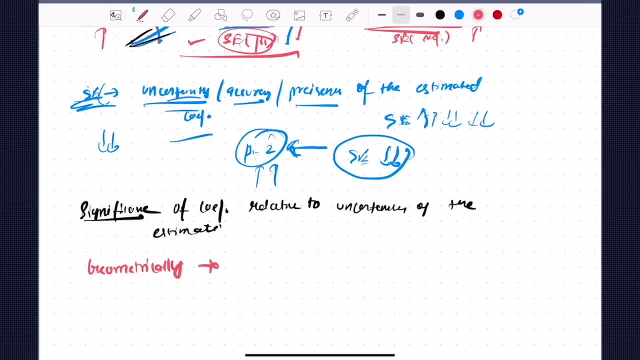 this is something I'm confusing as well. I can. I can actually ignore it as well, but but if you just want to understand in much more depth, it will be easy for you. so it can be thought of as though it can be taught. it can be thought as it can be thought of as: how many standard errors, how many? 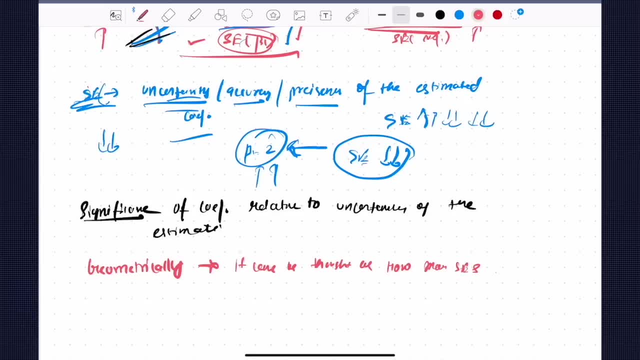 standard errors. as standard errors are away, are the, the, the coefficients, the coefficients, the standard errors of the coefficients, is away from the hypothesized value, is away from our what is hypothesized value, which means that we already assume it, which is our beta. our beta is nothing, which is which hypothesized value which is equal. 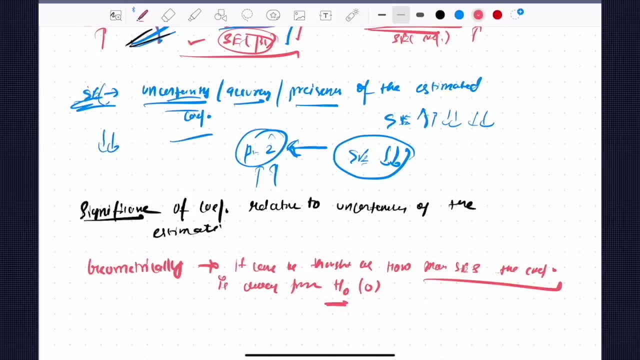 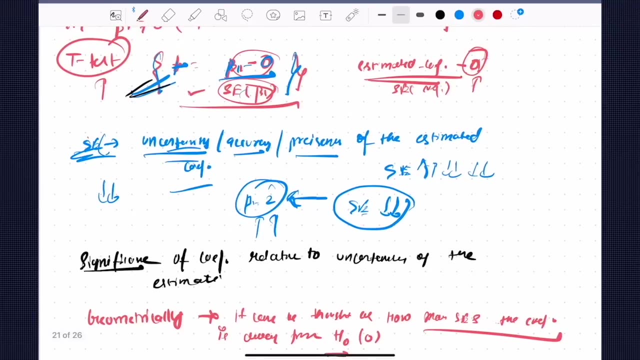 to zero. so what does it give? now, this is something which which almost our standard errors are away from, that are away from that. okay. so now, what does it give? the t's test, the? what does it give is it gives so if, once you calculate your t, once you calculate the t statistics, so we 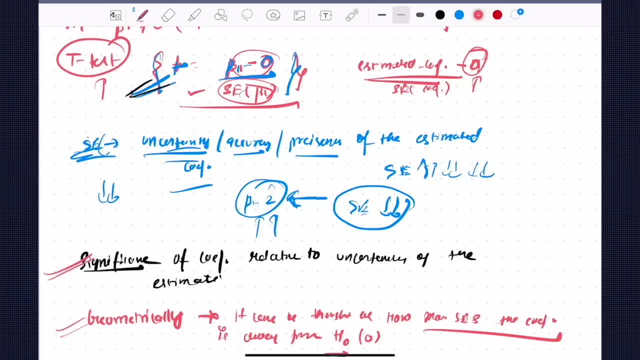 can understand two ways, either by this particular example or this particular. what does it give a significance of a coefficient relative to the uncertainty, unsureness? what is the significance of a particular coefficient with respect to the or relative to the? there is uncertain. uncertainty of the estimate higher than certainty, like it's. 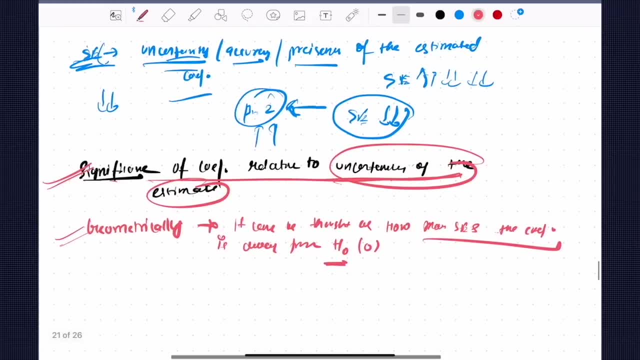 not good, right? so the large t statistics. so now let's talk about what does it mean if you have a large t t statistic, if you have a large t statistic, what does it mean if you have a large t statistic? so if you have a large t statistic, you, it indicates that your estimated coefficient. 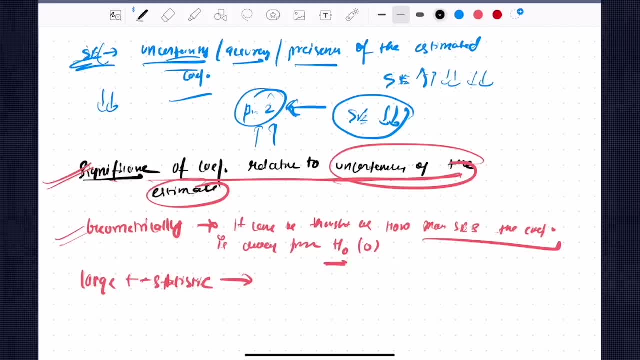 is different from the hypothesized value is different. so, lastly, statistic means that your, that your estimated coefficient, that your estimated coefficient is different, is different from the hypothesized value, is different from the hypothesized value, is different from the hypothesized value, which is s 0, which 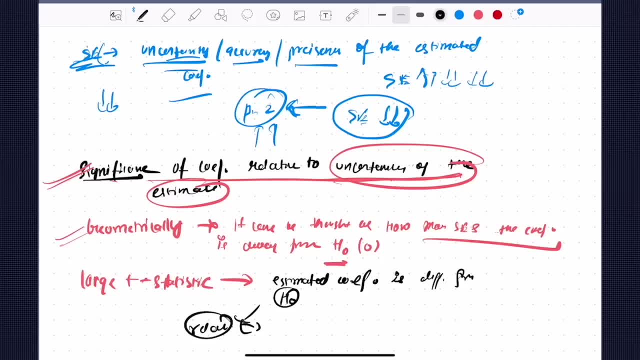 means that there is a relationship, that there is a relationship between your h j, which is between your beta 1 and y. okay, so this is what large t statistic means. we will we'll be talking, but usually it depends with the. if you have the p values, we have to compare. 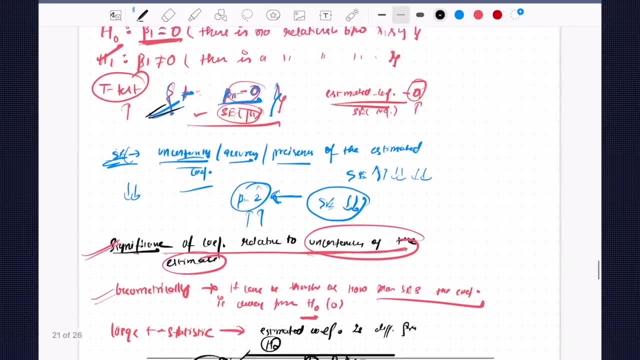 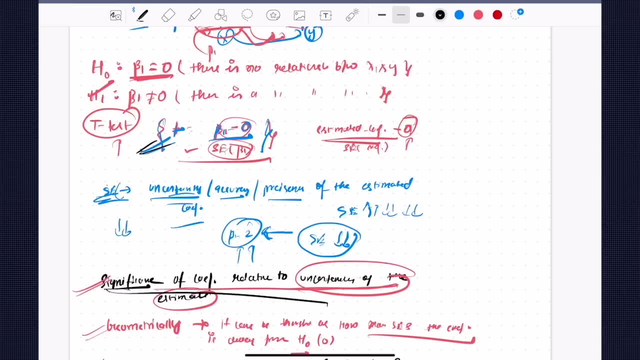 with our p value. but, as of now, why do you divide? do we divide? we divide because because it tells you the significance of our coefficient. now, once we have the significance, now, how can we say that, okay, this is the perfect. like, how can we identify whether to accept the null hypothesis? 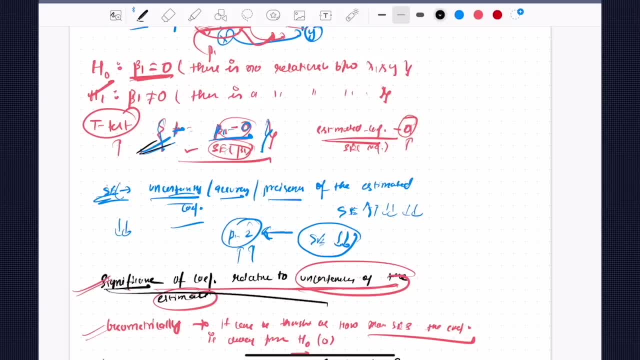 or whether to expect the hypothesized value, which means that the pre-assumed thing, which is that there's no relationship- or should we accept it, or should we reject that there- is that we have evidence to say that, that there is a relationship between that. okay, uh, let's talk about that this. 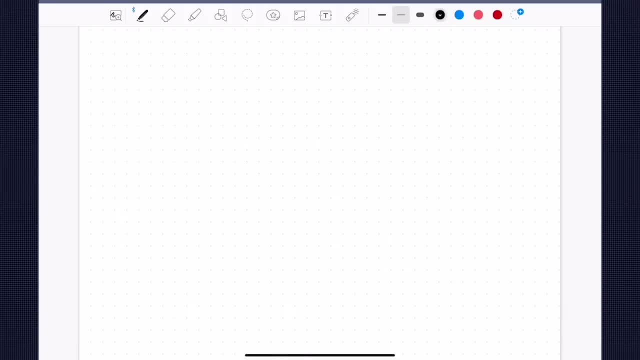 is something important to talk on as well. i'm just talking uh too much. i'm so sorry for that, but it's actually 38 minutes but that. but this is something which is important as well, uh, in terms of understanding level as well. okay, so let's talk about uh. p value. let's talk about p value. 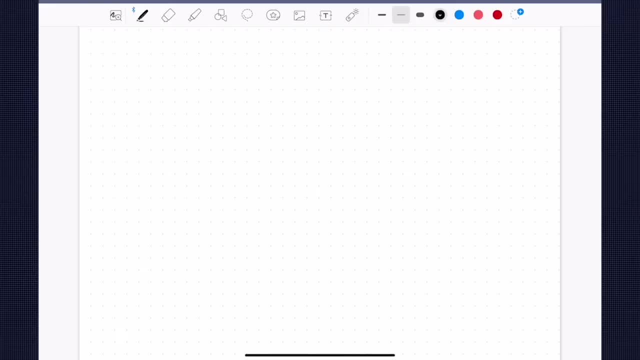 so p value over here? what is it p value means? so? so once we have the t t statistic, we, once we have the t, we compare with the threshold value. usually this threshold value is 0.05 or five percent and we say that if your t statistic is less than five percent, is less than five percent, then there is 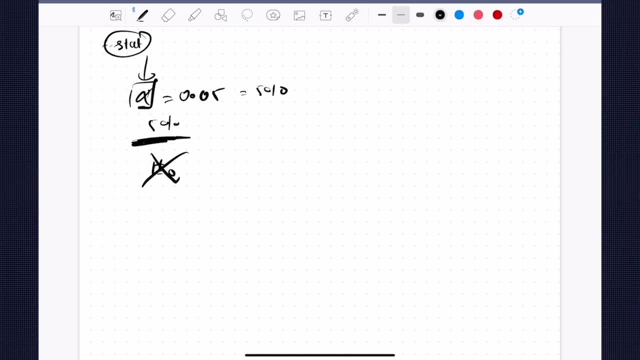 then we can reject our null hypothesis. and then we can reject our null hypothesis and say that there, there is. if it is greater than five percent, then we say that, okay, this is something um null. then then we have, we have. we can reject the altered hypothesis that there is no relationship. then we can say that there's. 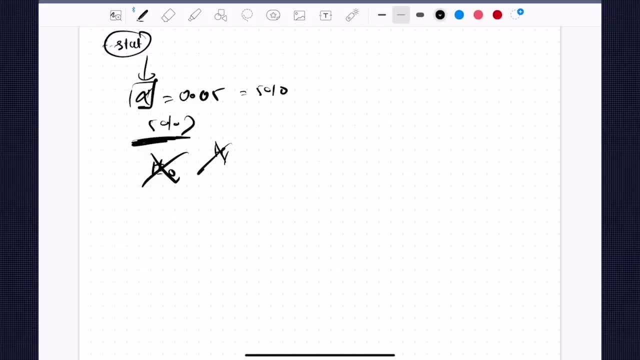 no relationship if your t statistic is greater than, like the t critical value. a t critical value- okay. uh, currently t statistic is different from t critical value. t critical value, which we'll talk about it just in a second. but assume that you got a some critical value and then you compare with. 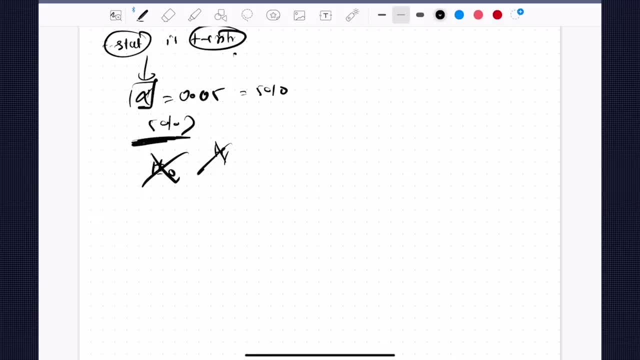 it okay, okay, so, uh, you can take a break as of now. even i'm speaking for the last 40 minutes, but that's all right. this is something which we have to do if you want to understand, uh, hypothesis testing in detail. um, so, so, basically, what is the so? so how can we say that? how can we say that? 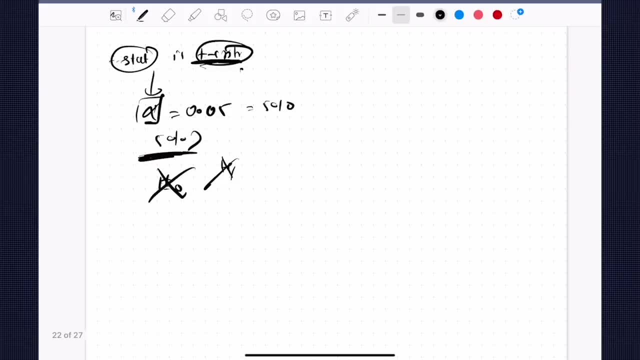 that if your t critical value, the critical value, the, the value which will get, the probability, the, the critical value which will get is: if it's more than five percent, then only if it is. how can you support that statement? we can say that, how can we say that, how can we say that? as i say it, as i say that the null hypothesis 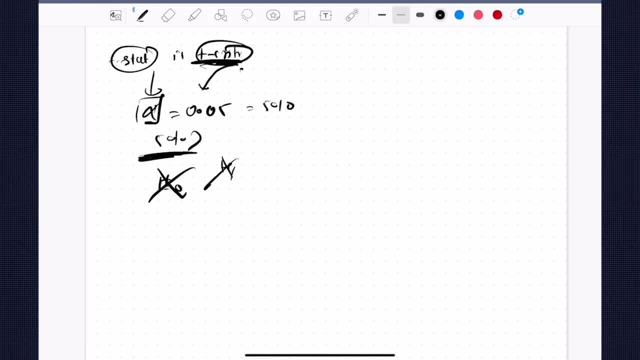 is a statement that assumes that there is no effect. there is no effect or the relationship. so there's there. we introduce a concept of something known as p value and threshold value, or is also called nothing but p value. so what does p value means? it says that. it says that. 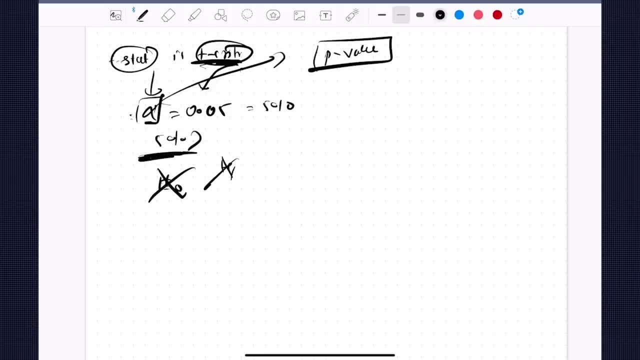 the observed result is unlikely to have a t critical value and the t critical value is unlikely to have a caught by chance alone. and so, basically, what does it mean? i know it's something, uh, chance and all. it's something which is also very great to understand it. but i'll take a very simple example. 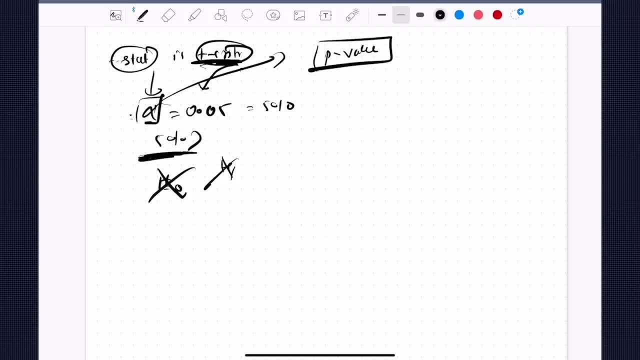 uh, so that you have, uh, a nice interpretation. so assume that you want to do a test if new weight loss supplement is effective on weight loss or not. again the same example which you have taken up. so you conduct experiment on two groups of people, so group number one and group number two conduct 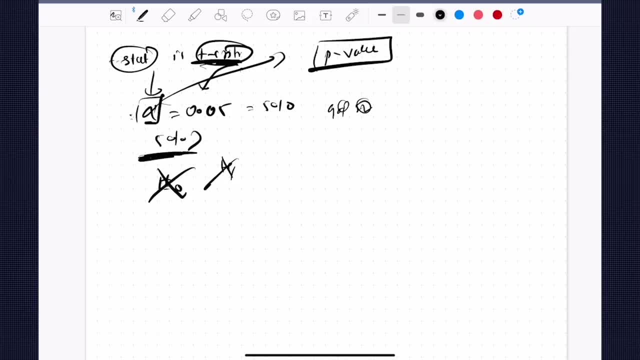 two groups of people and then, once you are one groups that takes the supplement and other takes the um place, which is the other takes the supply. one, one group takes the supplement, other does not take that supplement. okay, so hypothesis, what this null hypothesis says. null hypothesis, is that there? 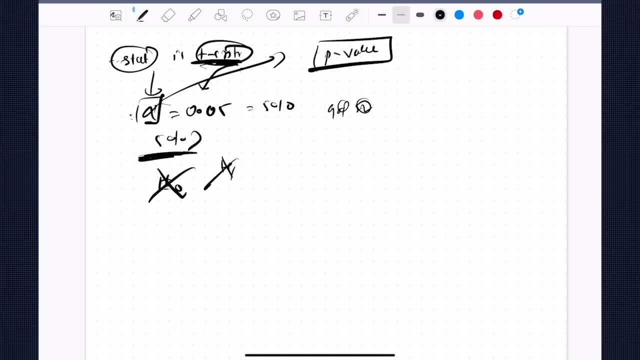 is no effect of that supplement, okay, that there is no, no effect and and no difference, there is no effect. so basically there is a two groups again. there is a two group, group number one, group number two, so each taking their own treatment effect. the supplement, those the supplement number one, and 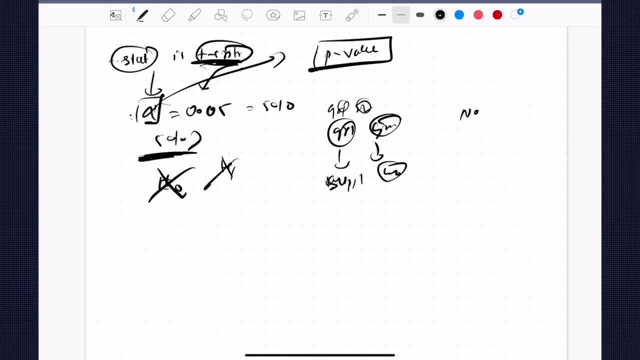 supplement number two: okay, so the null hypothesis states that there is no difference between these two, so i don't know if there's any difference. that's the hypothesis and the hypothesis. the alternate hypothesis says that there is a difference, which means that if there's a difference, that means there is something hooking in that, so we can, of course, use that for tritium. 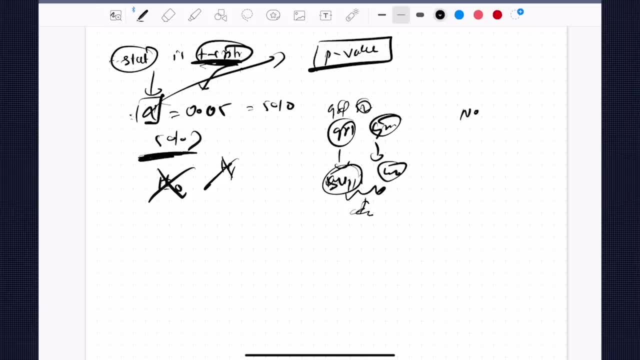 effect, but i bought the null hypothesis, that there is no difference. so after you conduct the experiment, you calculate your critical value and then, what do you have a significance? you, and then, and then your critical value comes, t critical value: 0.02, 0.02, okay, and 0.02. so your 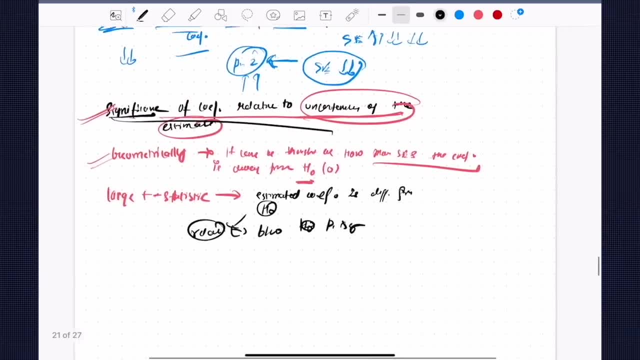 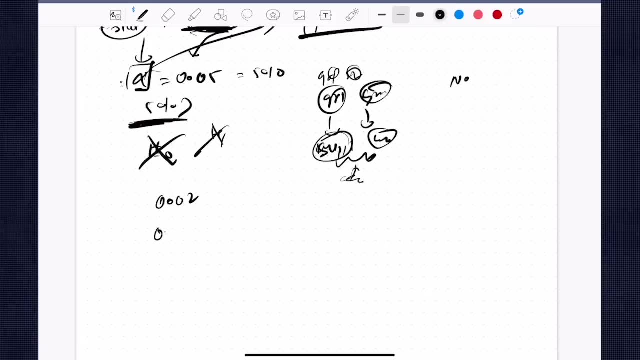 value is 0.02, which is the t critical value. by by doing the, by taking all the t statistic, you calculate 0.02. now, now, your threshold was 0.05, 0.05, right so? so so what? this means that that means that there is enough evidence to support that the weight loss supplement has an 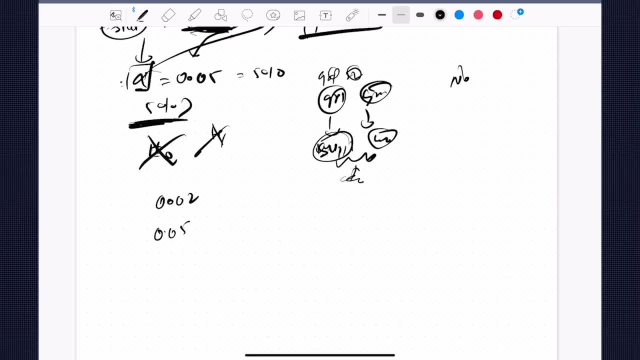 effect on the weight loss. so there is a. so we x, we reject the null hypothesis. we reject the null hypothesis why we require by, why we represent. so if, if your critical value is is a smaller than your significance value, then we say: then we reject, then we reject our null hypothesis and accept our uh alternate hypothesis. now you 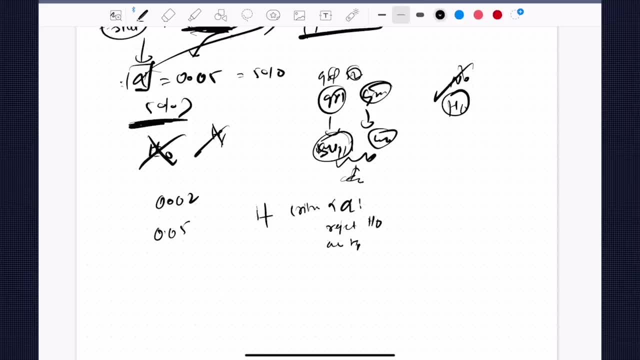 might be thinking: why, why does it happen like that? why does it happen like that? um, this is something, uh, this, this is something which also you need to understand. so this is a general thing. if a critical value is smaller than this, then we say that, okay, reject the null hypothesis. 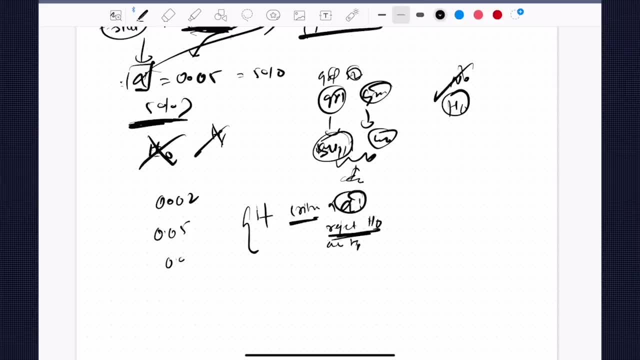 and then we accept, uh, that there's a so, but, if. but if you got 0.07, that means that you have to reject. but you have to reject your alternate hypothesis. accept the known hypothesis. okay, i know this is something hard to understand as well in the initial level, but you have to understand it anyway. 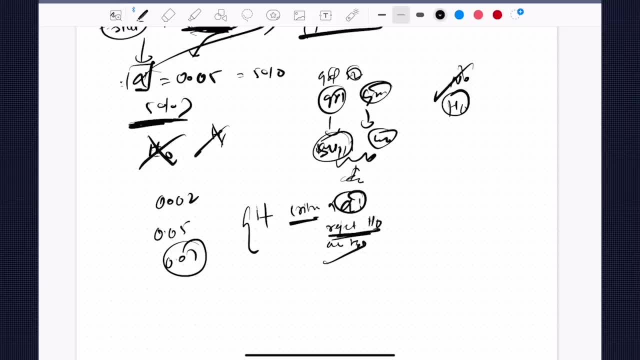 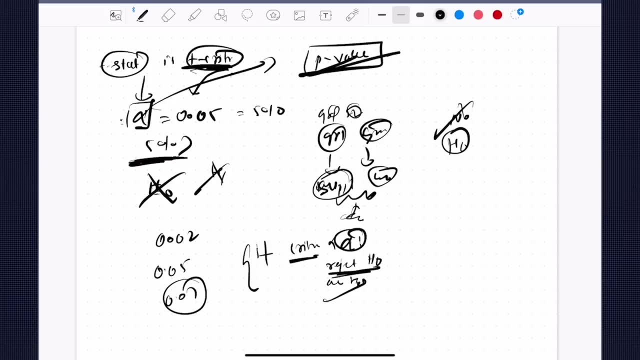 assuming that you have brain for this, cool. so how can we connect this? how can, how should we connect this p value, the concept of p value, to linear regression? so the so in linear regression, your null hypothesis states that the independent variables- independent variables has no effect. your independent variable has no effect on the independent, which means so all your betas are. 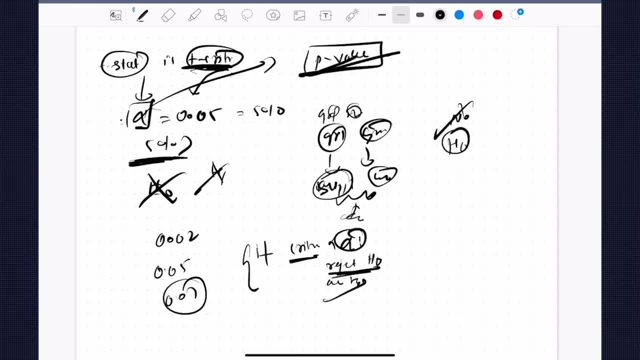 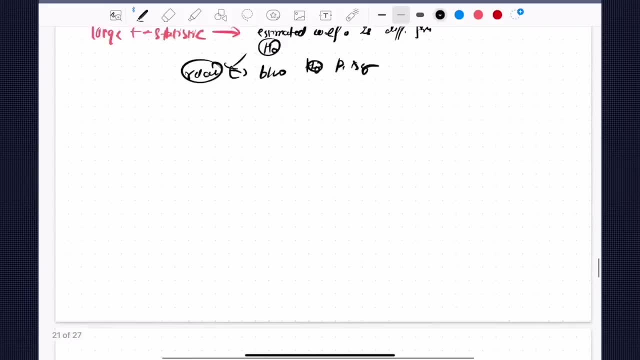 equals to zero and the p value associated with every coefficients help us to determine uh. that has a significance with us. so, basically, you have a critical value. in this case, you'll, you'll, you'll be having critical value for every uh betas. okay, so currently we'll be having critical, critical. 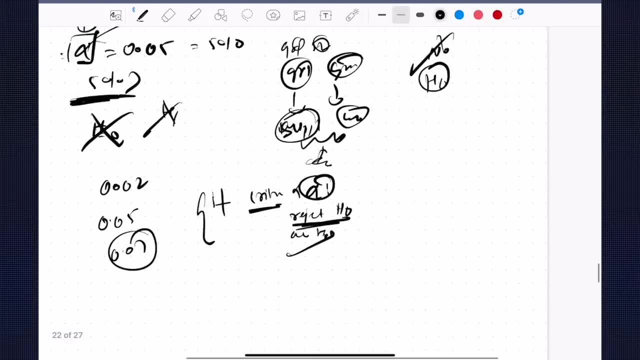 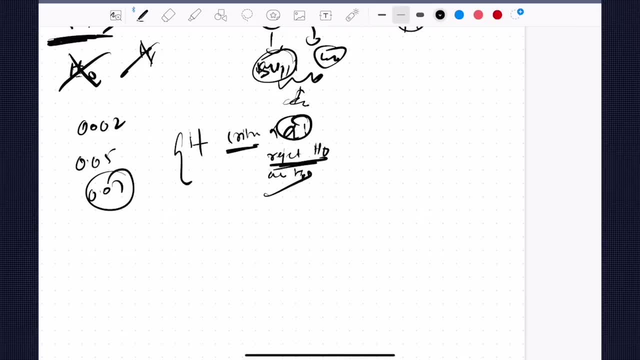 critical value, or the p, p value for this size, which states that, which states the significance of our size of the house on on the price. and so in this example, in this example, as we have seen, so you obtain, so you obtain the p value, or we can see, so there are p value or we can. 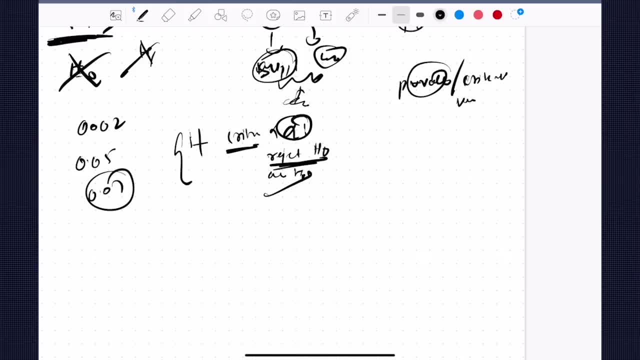 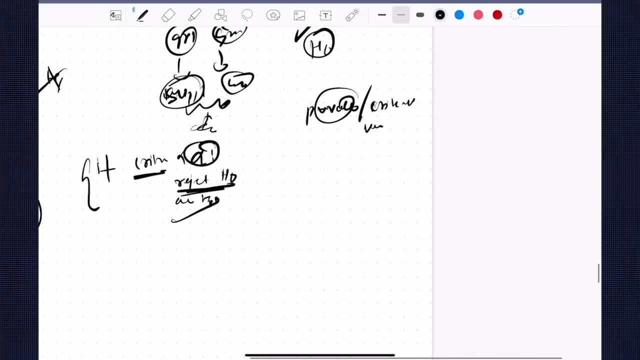 say critical value. we can say critical value by taking the t test and then and then comparing with the t test distribution. we'll talk about that, we'll talk about this. you calculate the t test after calculating the test over here, after calculating this, after calculating this, you. 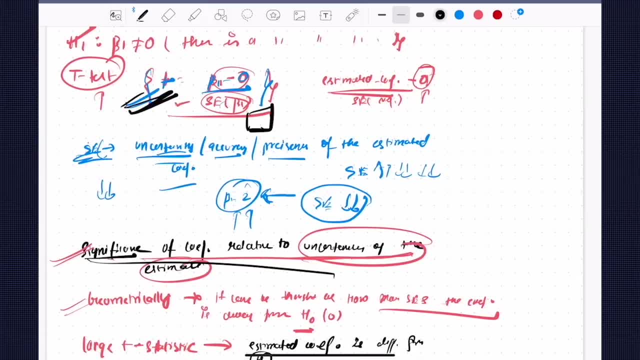 compare after you take out- you know, i've, you take out some number. you compare with the table, you compare with the table and the table. you, it is a table which is already, uh, published on the internet. okay, you, you don't need to remember everything, you don't need to worry about how this came. you compare, okay, this, this is something over. 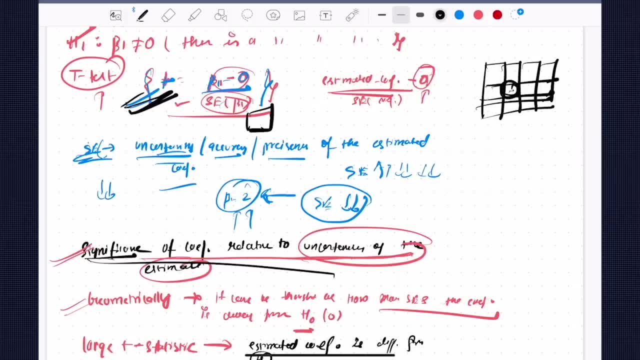 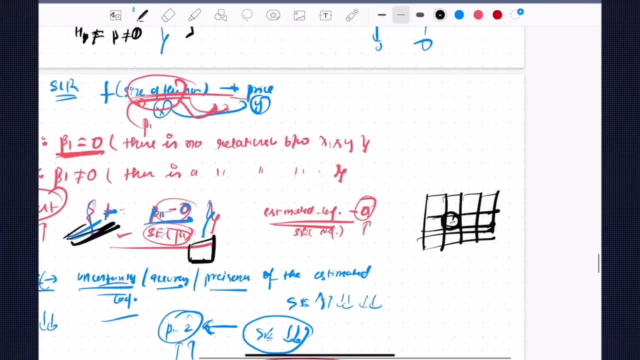 here now. this is, uh, we have to. we'll. we'll select the. how do we select the pp values as well later on? but you, you calculate how much significant, how, what is the probability that this is. that is, that size of the house is significant. okay, you calculate that p. you calculate the p value for. 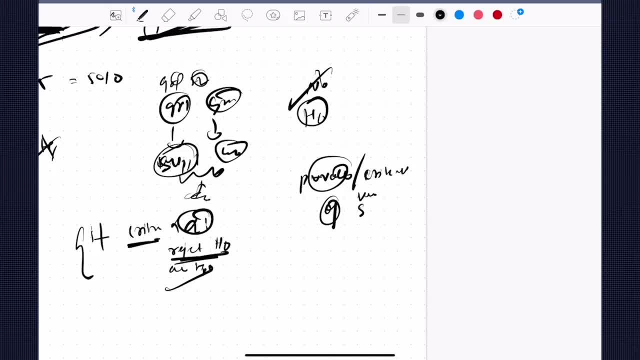 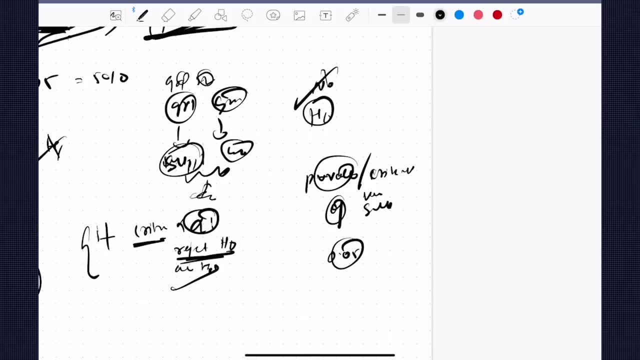 the coefficient of what over the coefficient of your size of the house. and now we say that if your p value is less than 0.05 is a threshold, which is the threshold, you reject the null hypothesis. you say that there is not enough evidence to accept the null hypothesis. so you 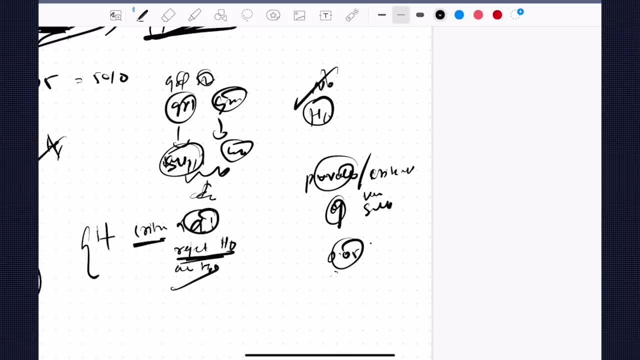 might be thinking: what does it mean, bro? why do we? why do we don't? don't say this: if it is, if your p value, like if your probability is higher, that means that it is something uh, significance. it is not okay. p value is always related to the 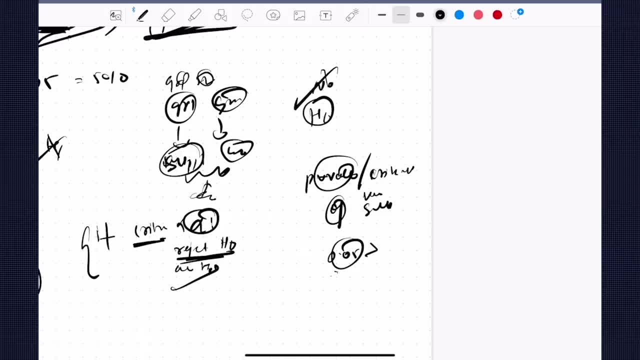 null hypothesis. so higher the p value is, the more you're providing evidence that there is no relationship. lower is that there is an evidence to uh reject them. there is evidence for alternative that there is a lower chance, that there is a lower chance of um of uh. there's a lower chance. 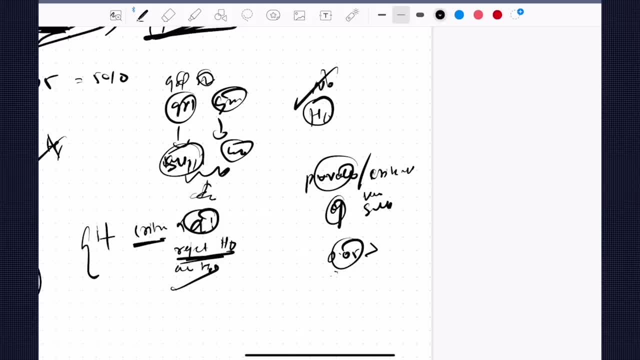 that it occurred that it is a uh, null hypothesis. okay, i hope that you are understanding what i'm trying to say. if you are not, then please watch the lectures once again so that, uh, you are able to understand uh in much more easy way. um, so, if, if, if you want, i can actually take an example, i can. 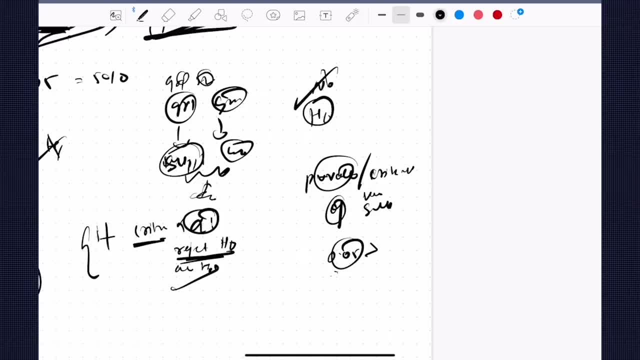 actually take an example to help you understand that. what is chance and all. but let me know if you wanna understand about that, like, how can we there's a support to statement? how can we say how? how can we say how can we say that why not greet up? why not get a? currently you can. 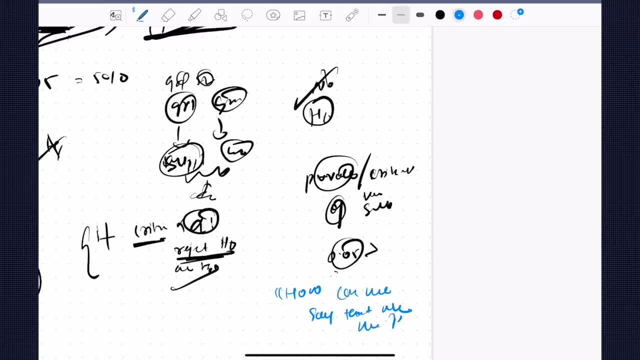 understand this with that if the p value is smaller, if the p value is more than 0.05, you reject the null hypothesis, except the alternate hypothesis. okay, if you, if you want to know, please let me know about that as well, because i have a very nice. 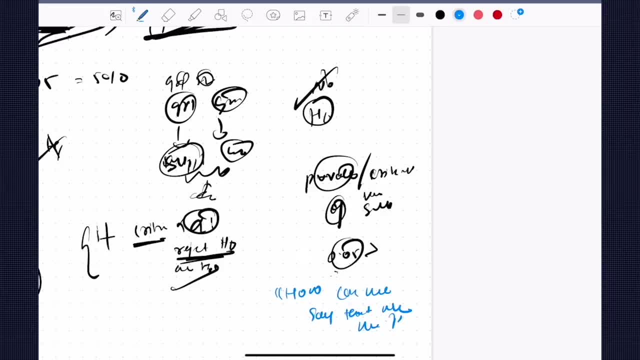 explanation, but that is a bit of out of the context of the course, but it's all right, i can actually understand. like, uh, i can actually understand this. this is something which people face as well. cool, so now. so now, once we have that, we announce if it's more, it's greater than. 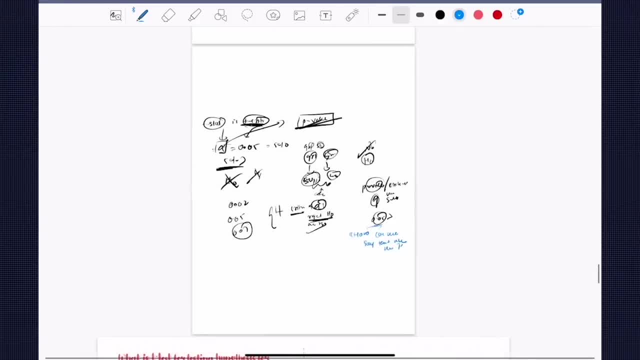 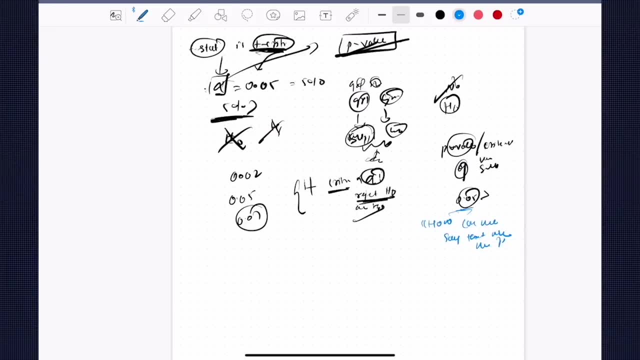 or smaller than we accept or reject unknown hypothesis. cool, i hope that this gives a good sense. now let's do a very nice example, a numerical worked example, so that you understand it, and nicely. and then, uh, we'll be done with the t test, you'll, you'll be left. 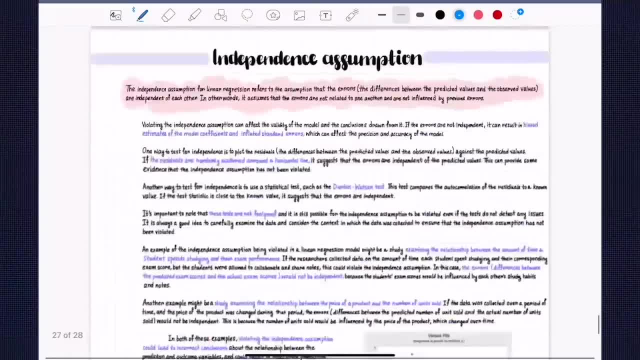 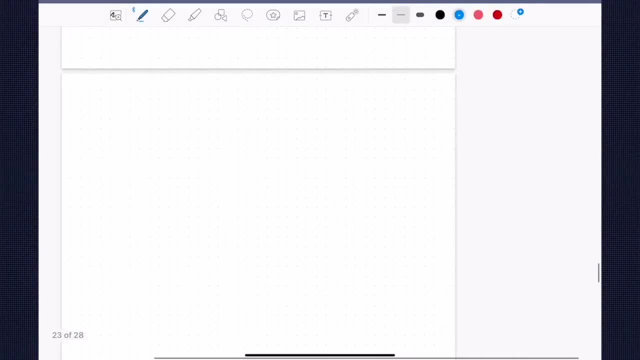 with f test by your own. you'll be left with the f test, uh, which you have to explore by your own. i'm not going to talk about that, so let's talk about uh. let's continue. our previous work example, our previously worked example, was that your, you have a square footage. you have a square footage which is: 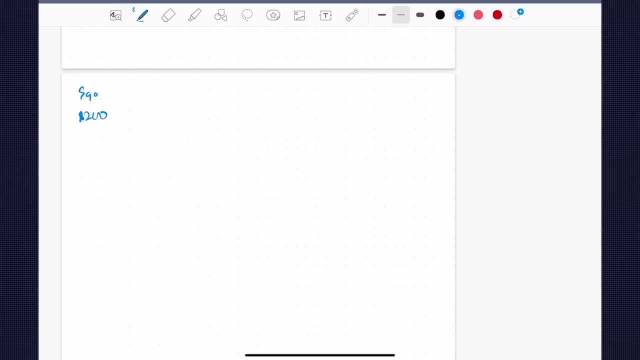 1200, 1, 200, 1200, and then you have 1500, 1700, 2100, 2300, 2600 and three thousand, okay, and then you have nothing but the y that we have the price of the house. you can understand some sort of price, okay. 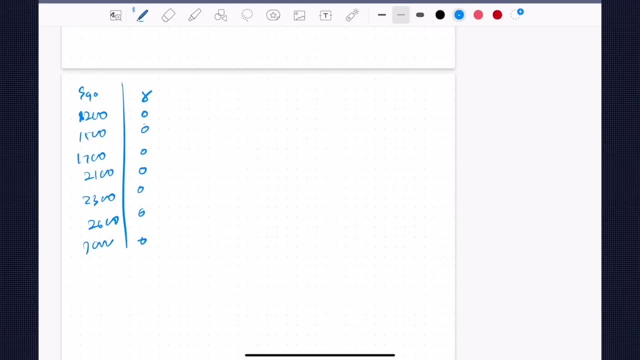 i'm not writing the data, but i'm just making it like this. okay, so your equation will be beta 1 plus beta zero. sorry, beta zero. sorry, i think i did it wrong. beta y is equal to beta zero plus beta one, x. okay, x x one. so assume that your beta zero, assume that your beta zero is nothing but. 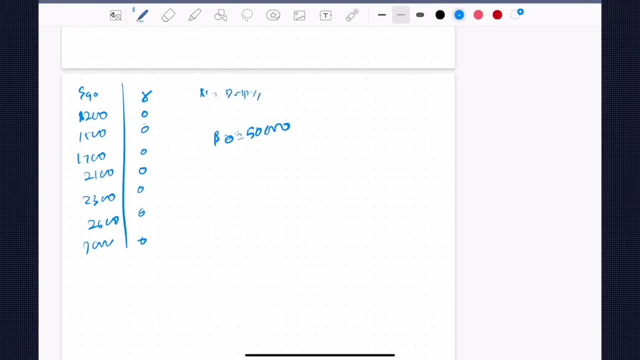 five, fifty thousand, okay, fifty thousand, and your beta one is nothing but equals to hundred. okay, so we can. so first, so let's state our null and alternate. so null is h, h zero is h zero is where all your beta values h one is the alternate is: they are not equals to zero. 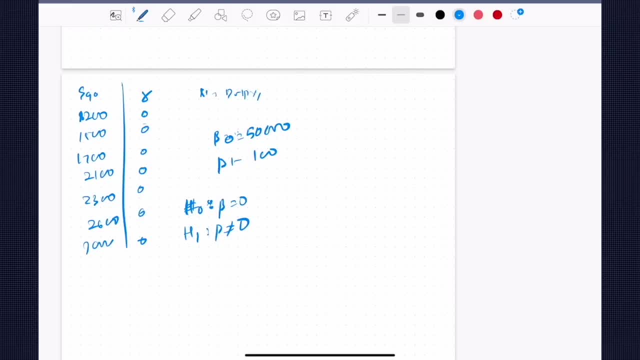 that there is a relationship existence. you calculate the t statistic. you calculate the t statistic, t statistic, how, how it is calculated, estimated. we are going to calculate for beta one. okay, because we are going to take out the significance of this x one. you calculate the beta one hundred minus. is the estimated minus zero? well, because, because the null, because minus. 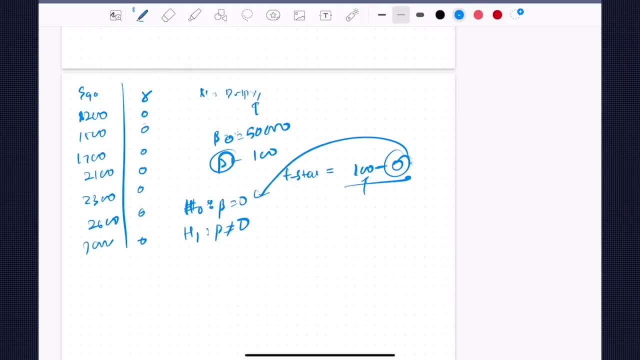 the hypothesized value. in this case it is equals to zero divided by divided by the standard error. standard error of that coefficient. the standard error is also: it's: it's a nice formula for calculating of a standard error, but in real world you don't need to worry about the formula. you can actually 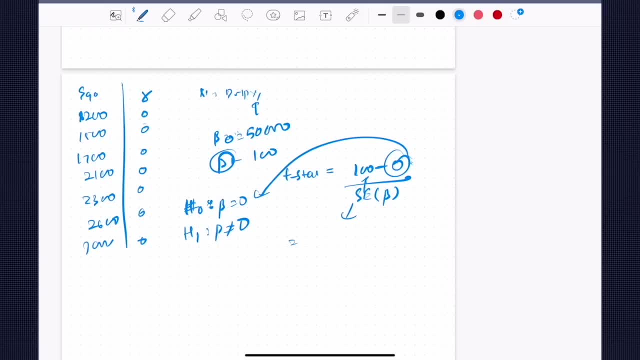 look on the internet to calculate the standard error formula. so the standard error which which you are going to get, the standard error which which you are going to get, is nothing but the. the whole calculation will yield the whole cal. the whole calculation will yield to hundred divided by ten, which is nothing but equals to ten. so your t? t statistic is: 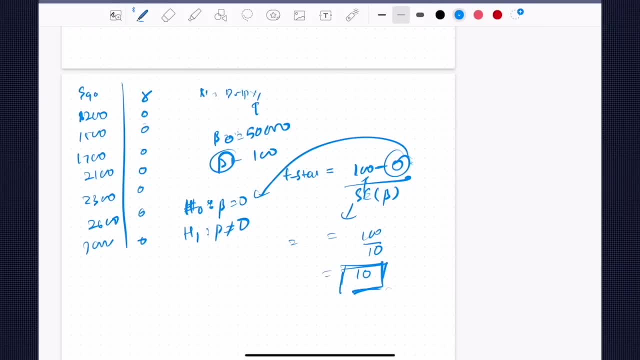 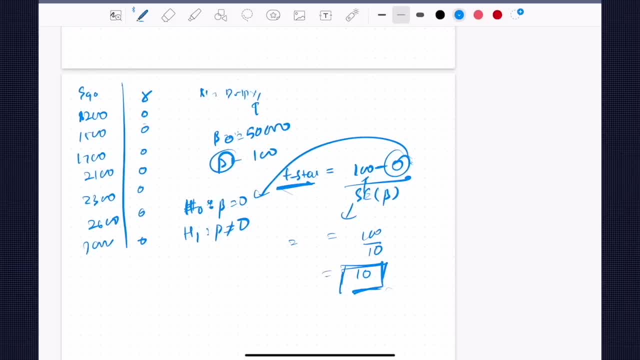 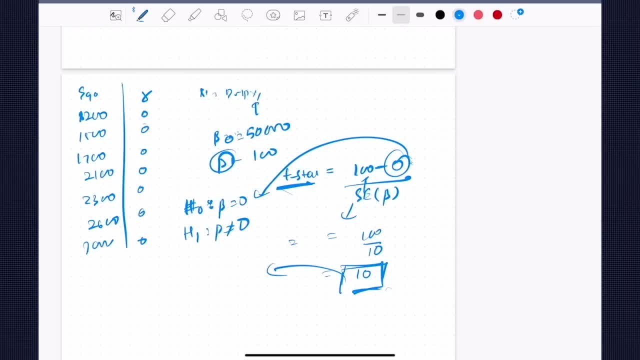 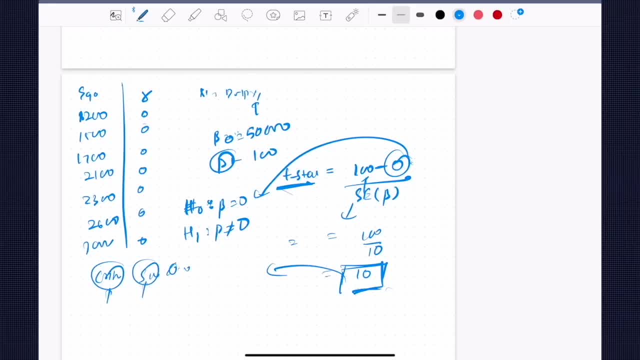 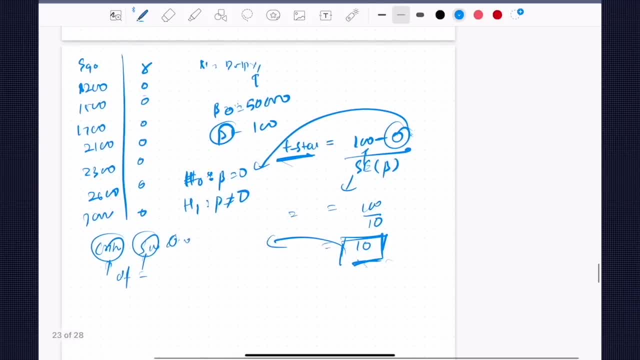 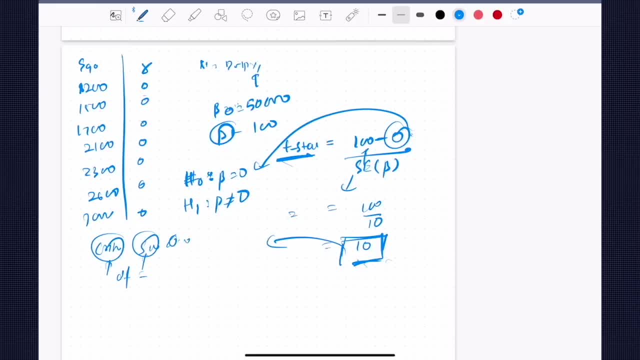 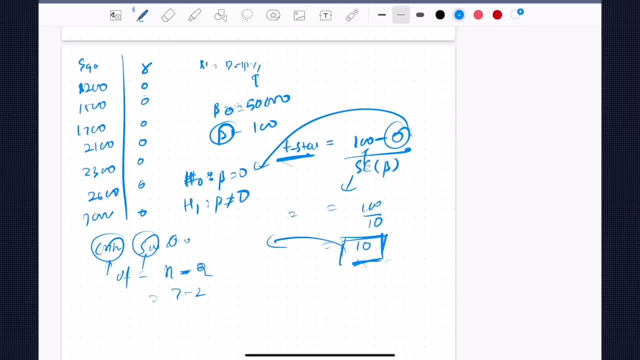 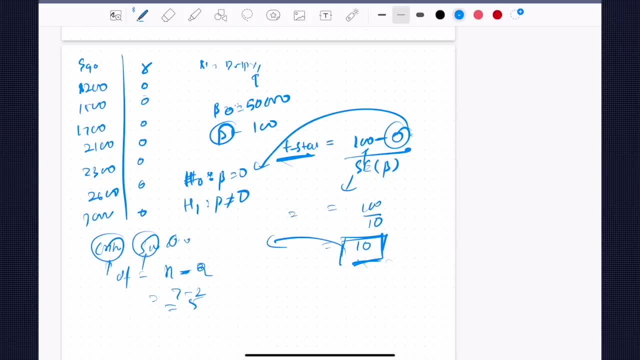 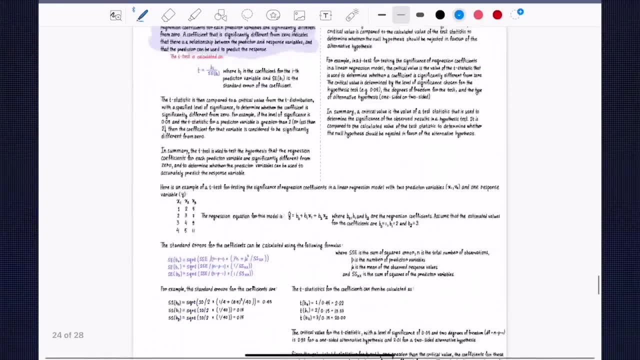 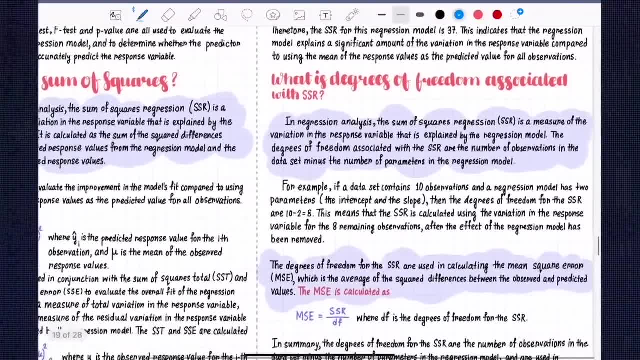 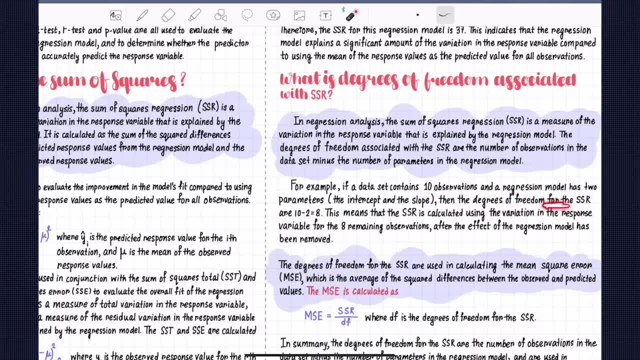 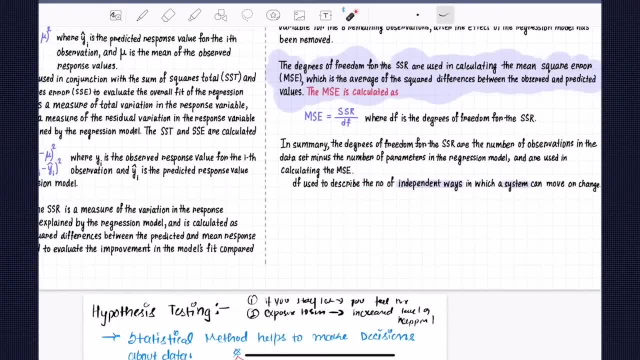 the t statistic. now you can calculate the t statistic. now you can calculate the t statistic now. was intercepted in a slope. the degrees of freedom is equals eight. so what is degrees of freedom is used to decry the number of independent ways. a system can change number of independent ways. 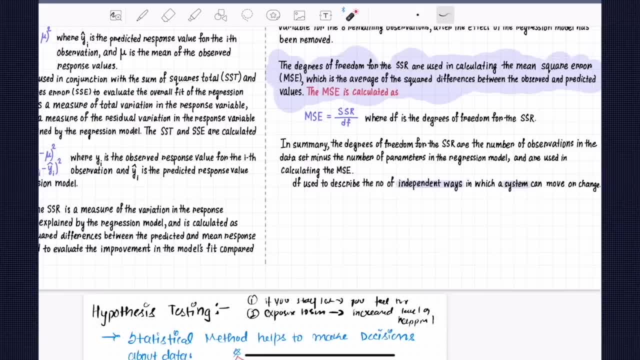 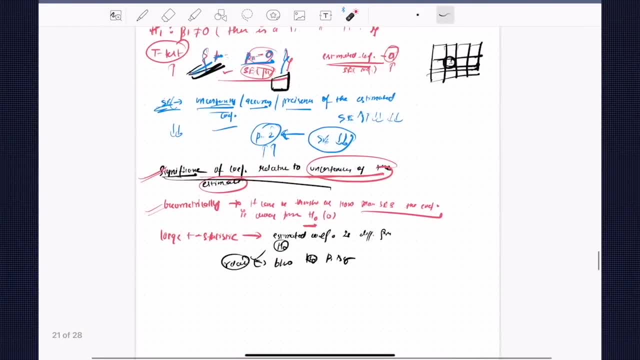 the system can change. this is used for calculating. if you're not able to understand, i i i would say: ignore it, but eventually you know. but. but eventually this has a statistical meaning where it says that number of a number of uh, independent uh values, or the independent values, 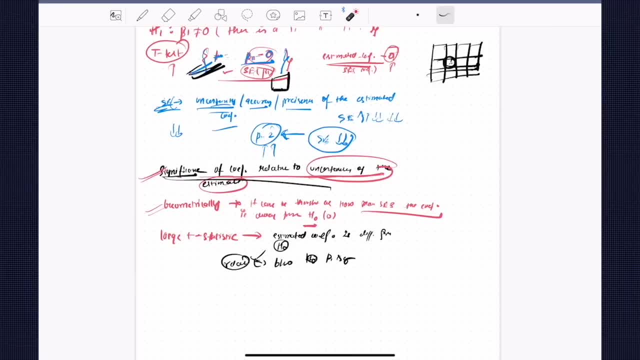 in your data set. so basically beta 1, and beta, of course, is dependent right number of independent values of your model, the number of independent. why we say that that is number of independent. we can search online about more about degrees of freedom, but this is number of independent value. 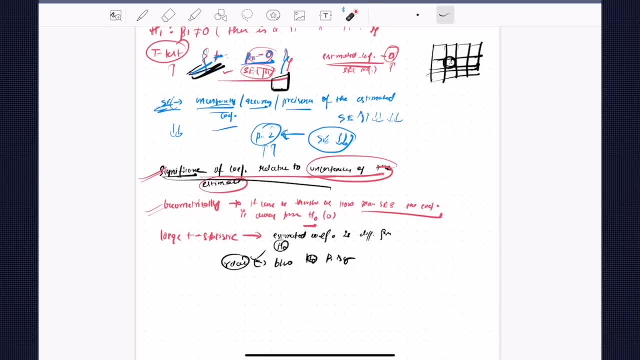 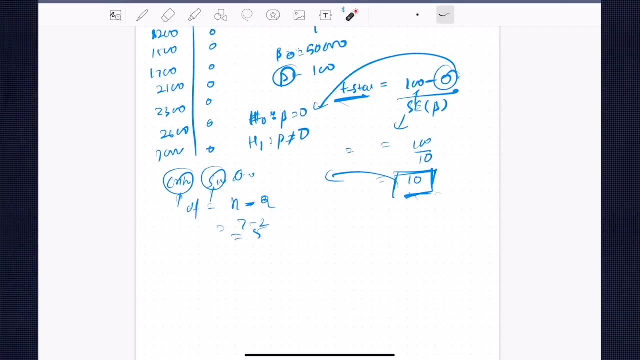 which? uh. so basically the two are dependent, because it's slope and intercept which is dependent, so we can subtract it from our whole data number of observations. we'll eventually get your output variable by the degrees of freedom. degrees of freedom. so once you calculate the degrees of freedom- in this case is five. okay now 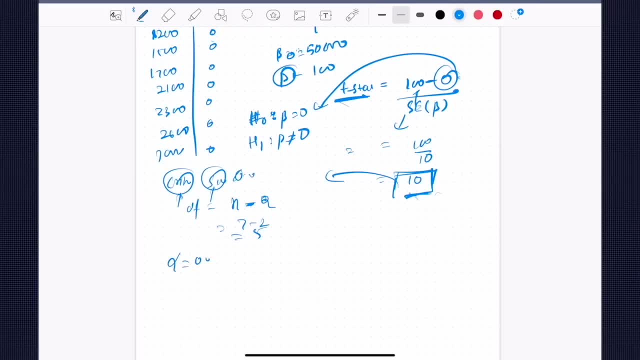 now. so now, now, your significance value is 0.05. degrees of freedom is uh. five degrees of freedom is five. degrees of freedom is five. okay, so your significance is this: degrees of freedom is this. now, let's go ahead. now, let's go ahead and talk about something known as uh. 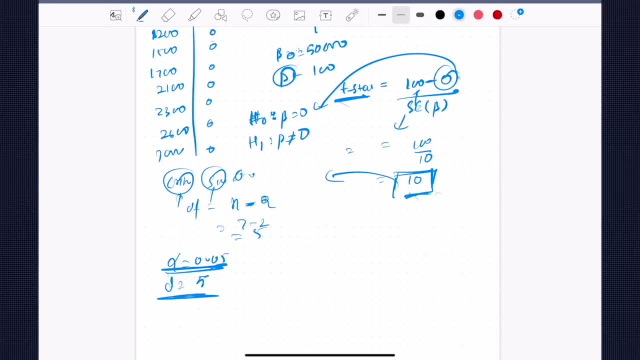 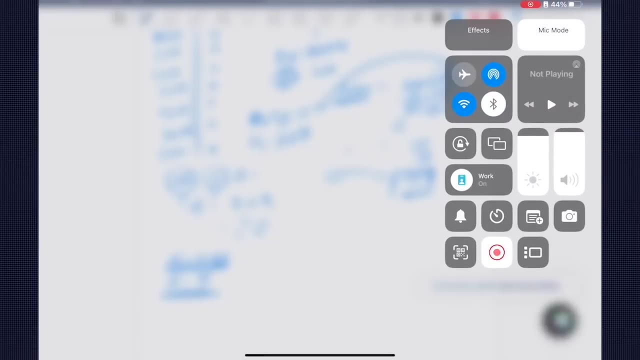 now let's talk about something known as uh table distribution. so a cd: open up the t table distribution. to do that, you'll need to be online. oops, i'm not online. that's pretty bad, so yeah, so i'll put up the. i'll. i'll put up you, you. you should open it online by your. 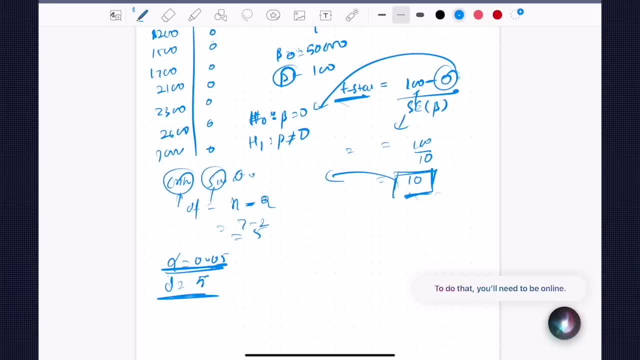 by your own. i'm not online as of now, so i suggest you should open by your own so that you understand it by yourself. open that online and then just go to a table and then if you see, And then if you see, on x-axis, on the top of it you have nothing but t values, the probability, which is you have to go to two tails. 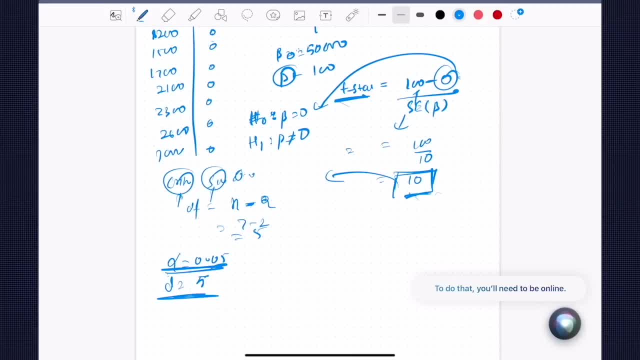 In regression, you always use two tails, not one tail. The difference is listed in the reading materials. Please see that. So, in two tails, you see that 0.05,, you see that 0.05.. And then, if you see the fifth, the degrees of freedom is 5.. 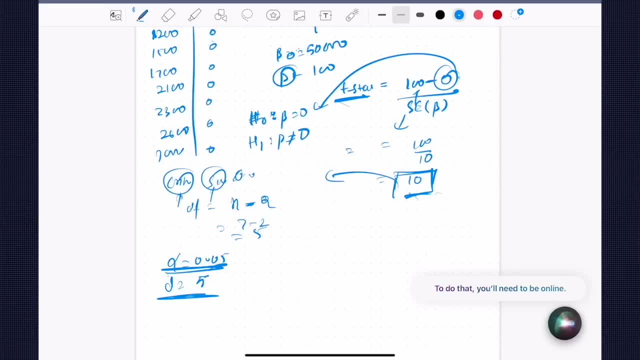 That is, the 2.57, 2.571, 2.571 is your, is your critical t value? is a 2.571 is a critical t value? is a critical t value? Now you compare the t statistic, t statistic, with a critical value, with a critical value. 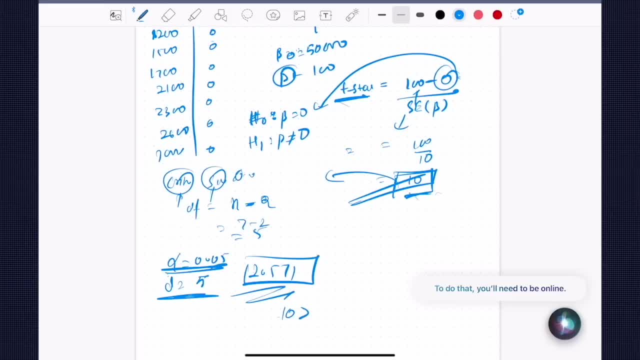 So it shows that. it shows that if you your, of course, t is greater than 2.571,, t is greater than, of course, 2.571.. So we Reject the null hypothesis because this means that there is a significant relationship between that. 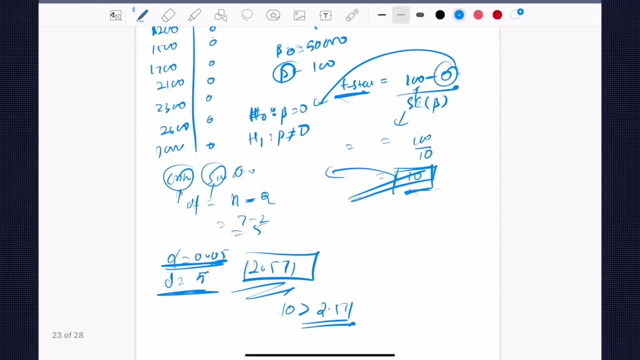 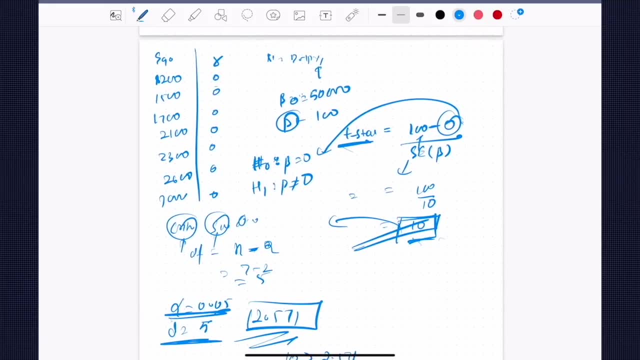 So you, you, you, you might be saying that, yeah, you should. just some, some seconds ago you told that that it should be smaller than the critical t value. So not not about that, but in this t test of course we do in several examples, but in t test we simply do this, is we simply reject the null hypothesis in the favor? 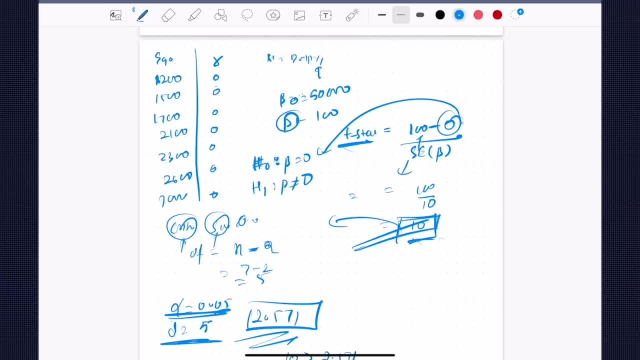 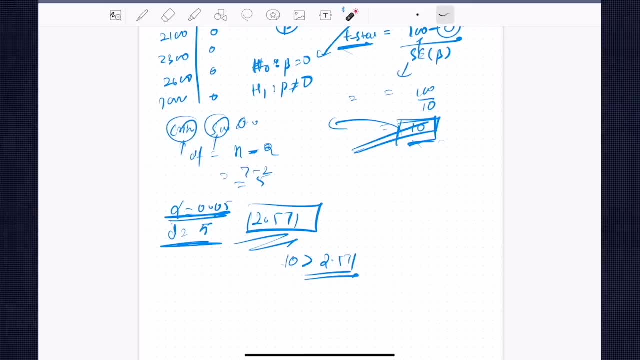 If it is, if a t statistic, if a significance level is, if a significance is greater than the approximated critical value, Because of course it changes, no, it changes. So, as I say, your t statistic should be greater than should be. sorry, should be greater. 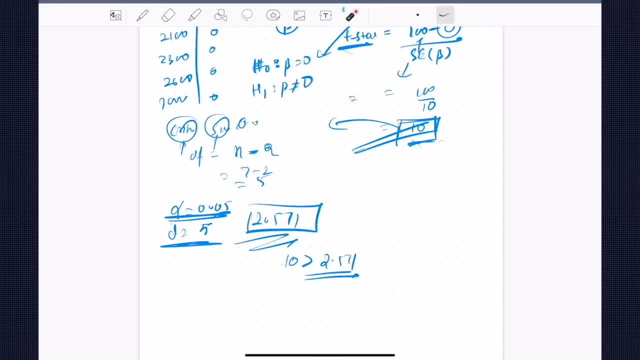 If the, if the significance is greater than your approximated value, then we say that okay, So something that we predicted nicely. So I hope that this gives a good sense. If you want to know more about all of these things, I would really suggest go forward and talk about. I have also given several examples of 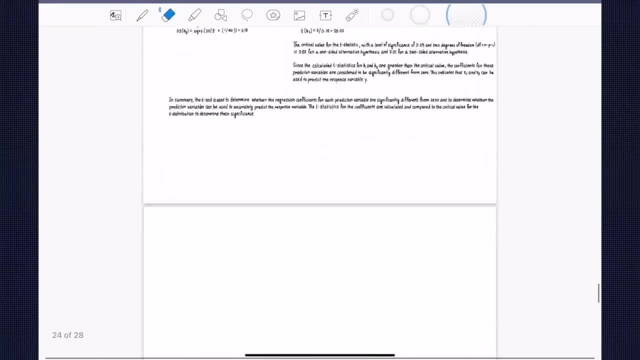 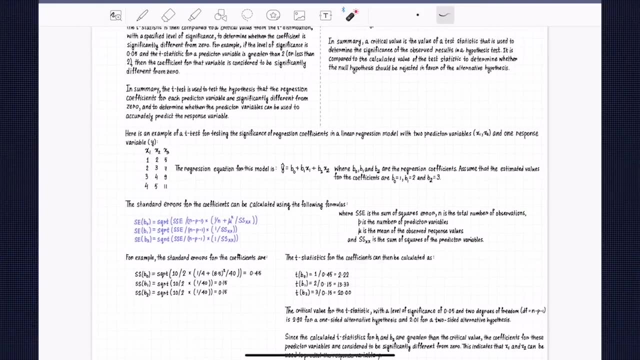 So if you go and see several examples of mine of t test, of t test, you can go over here. I didn't talk about like for every individual predictor variable, for every individual predictor variable. you should be able to view it nicely. 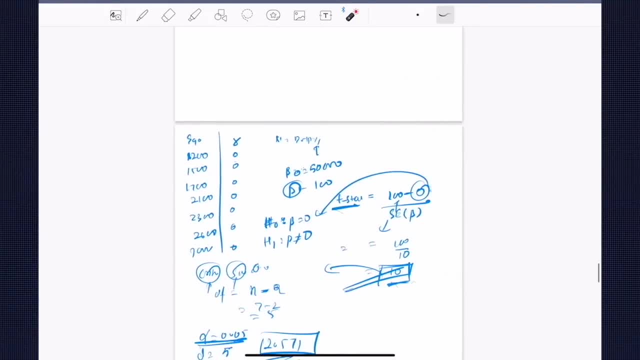 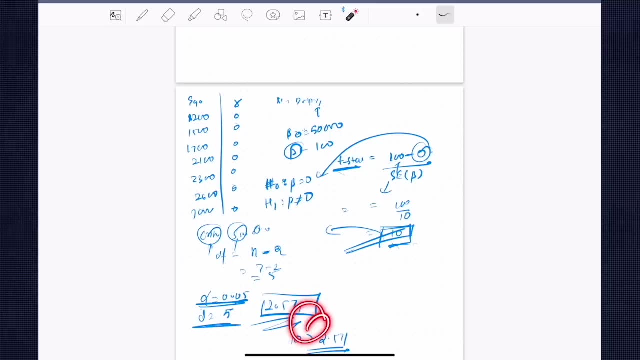 But my point was that you can easily use the materials to actually t test, to calculate t test statistics and then approximate a t critical value and then compare the and if the t test is greater than approximated critical value, then you go forward and accept it. 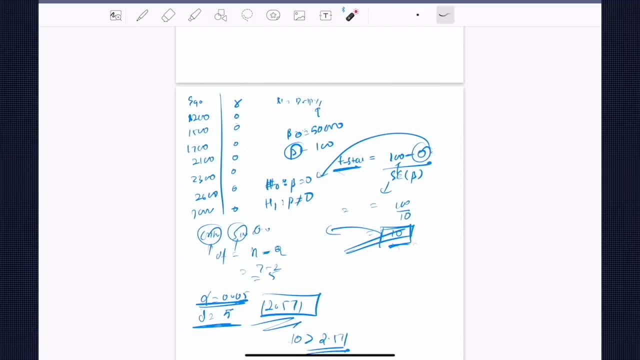 Okay, Cool, But but you know, but you, but you have to also make sure that you're, but but it depends on several. What are the problems from the test to test? So that's that. that was pretty much about our t statistic. t test statistic. 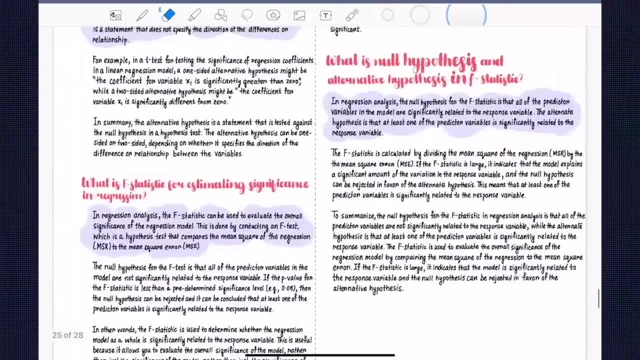 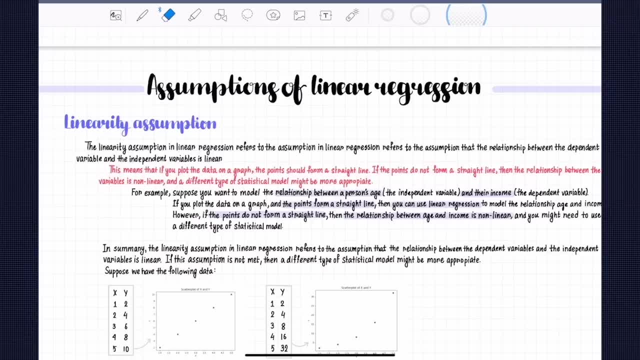 Now what we'll do now we'll- now we are done with almost hypothesis testing. Now we'll go ahead and talk about assumptions of linear regression and then we'll wrap up our whole course with a one project. Hey, everyone. 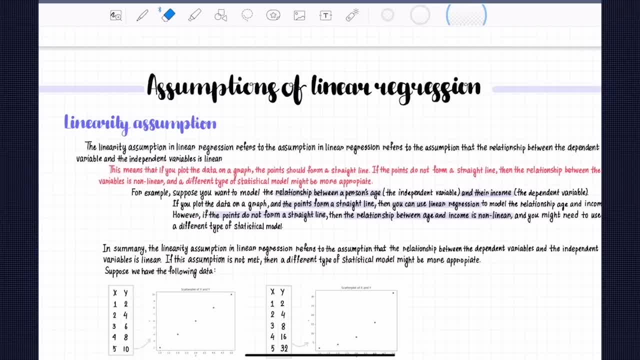 Welcome to this one of the our last of lectures. I'm super excited that we came along over here and I hope that you really understood each and every integrity of everything which should, which you should know. We have talked a lot of things. 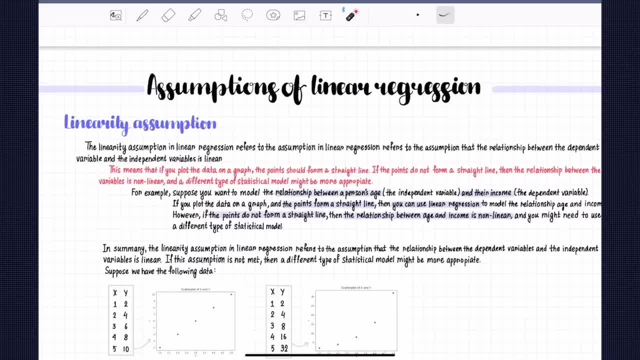 As of now- and it's still not ended yet- Let's say we still have a lot of things to explore. We still have a lot of things to cover up, And one of the things to cover up- which is one of the most famous interviews kind of thing- is assumptions of linear regression. 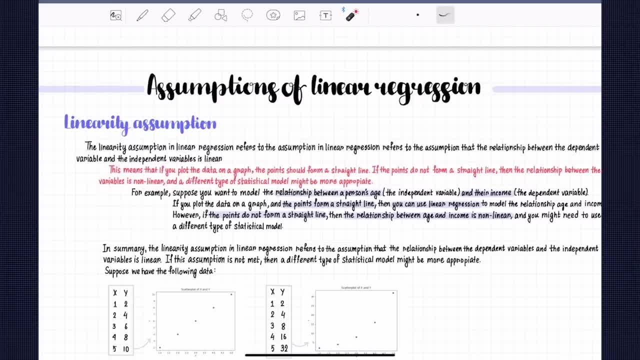 So basically, what I'll do is I have tried to make it in a unique way or a structural way, Okay, So basically we have several subtopics to cover in this. There's subtopics are linearity, Then you have, you know, independence. 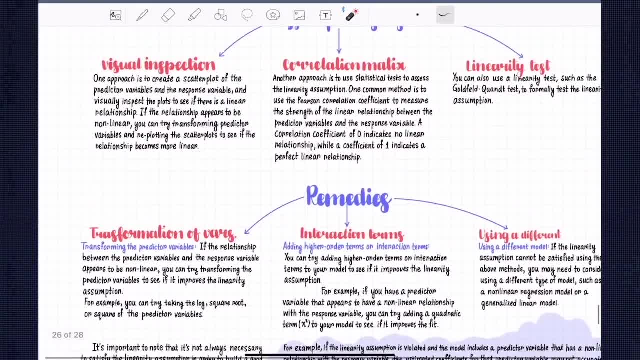 Then you have normality assumption And there's several other assumptions Listed out here. So what I'll try to do, what I'll try to do, I'll make sure that you understand each of the subtopics in great detail And I'll make sure that you also do your substantial research by yourself. 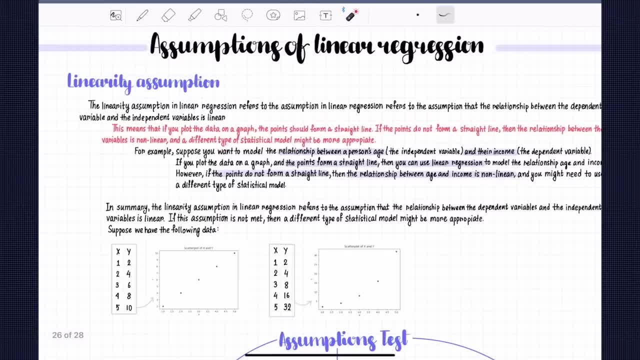 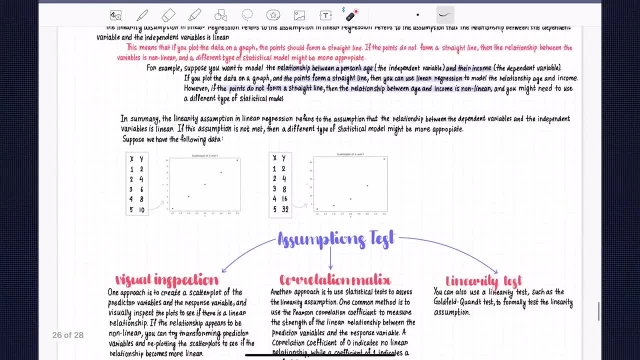 Okay, Cool. So basically, let's start off with the first assumption. Let's start with the first assumption. These are the notes for you to you know, review quickly, But I prefer using my own hand right now, So let me just open my new hand, which is this one: 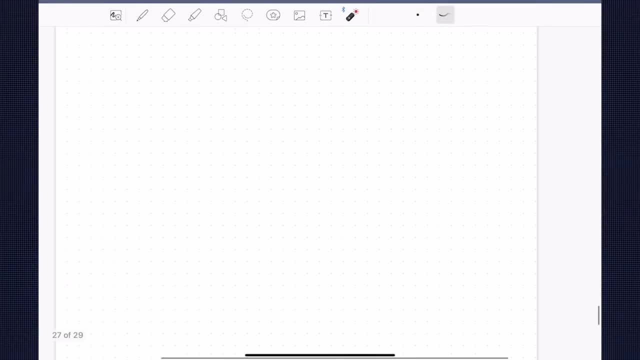 Let's open a dotted paper. So once we open the dotted paper, let's get started now. So the first assumption. But what exactly assumption is? Now? you might be thinking, hey, Ayush, okay, this is an assumption. 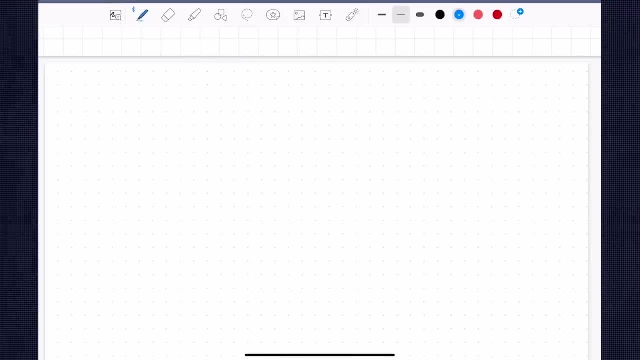 But what exactly assumption is And why do we need to study about this? So assumptions, Assumptions. So what is the definition of assumptions? So tell me the definition of assumptions. So first of all, let's get it clear about what exactly the formal definition on dictionary says. 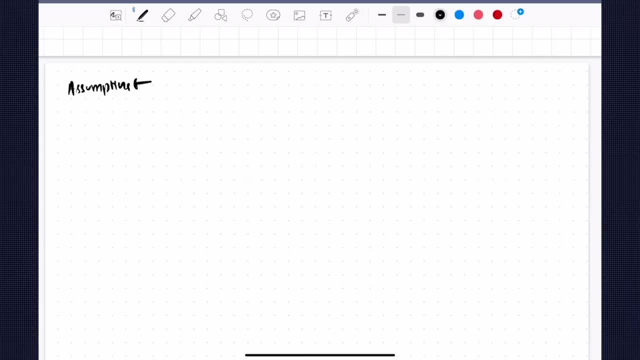 Because anything which I learn about anything, I just make sure that I know that definition of the topic. So thing is: What is assumptions? The thing that is accepted as true or as certain to happen without any proof? A very nice definition. 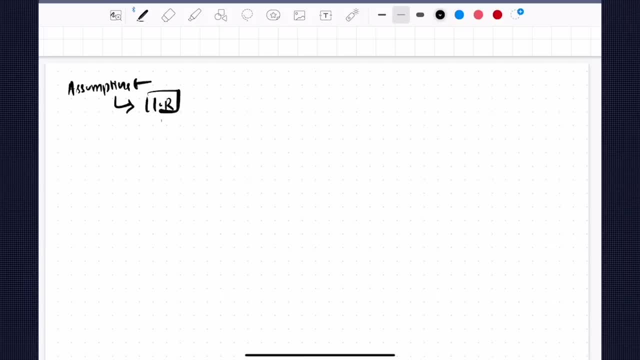 So what this says is when you apply a linear regression model, this linear regression model assumes several things without any proof. It assumes that your data should be linear. It should follow linearity assumption Or no constant variance assumption. There are a lot of assumptions. 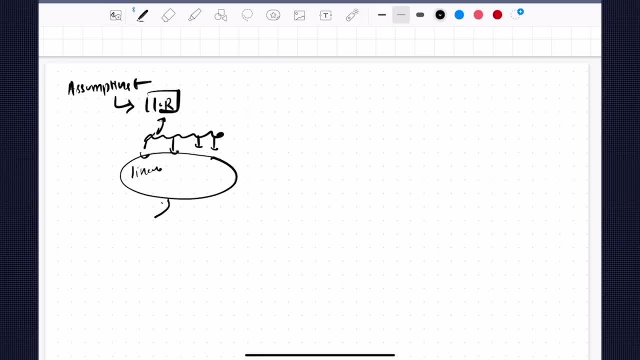 So it assumes all of these things, And assumes all of these things, And then you can expect your model to work fine. So if any of those assumptions fail- Like if any of the assumptions fail- then you cannot expect The LR model will only perform best. 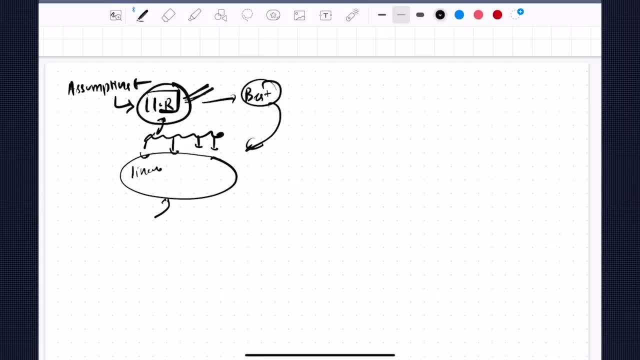 It will only perform best if, and only if, these assumptions are met. Assumptions means certain things are met, Like, for example. For example, when we have something like- Let's take an example- when you prove something Or when you say: assume that this is something. 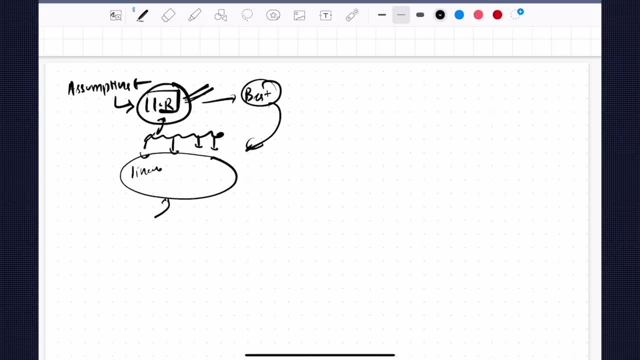 And then you put an argument. So when assumption is that not true, Then how can you say that particular thing will work Right? So assume that we have some certain assumptions to be there And then we expect these assumptions to be true. 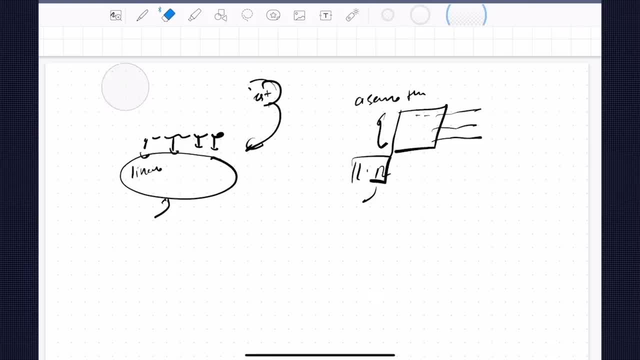 For our LR model to work perfectly fine. Okay, So this is one of the definition of assumptions in a great detail. Now what I'll do. Now what I'll do I'll talk about. There are several, So, as I talk, 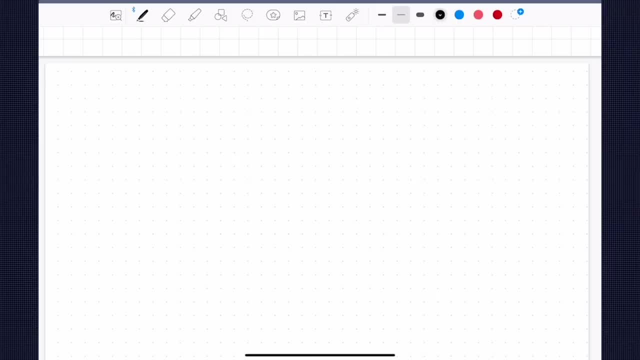 There are several assumptions, So I'll talk about some of the most important assumptions For you to explore it out right away, And then we can further get started onwards. Okay, So the first assumption which I'm going to talk about: 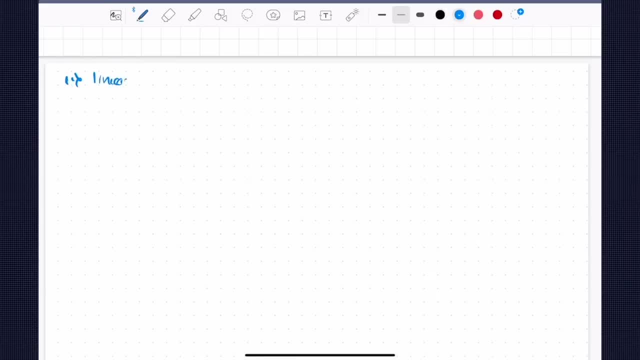 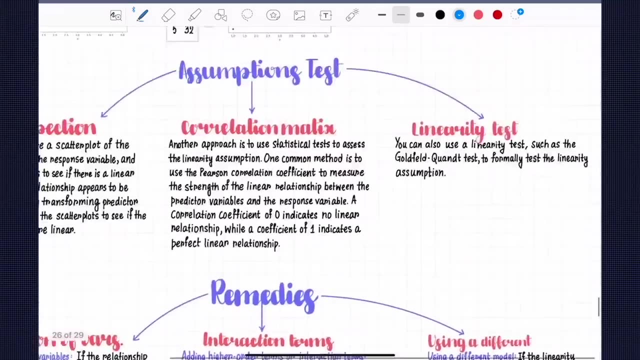 Is something known as linearity assumption. Linearity, Linearity assumption. Please ignore my handwriting. I have to write it super quickly, That's why I'm writing it super duper quickly. So linearity assumption says that. What does it say is that? 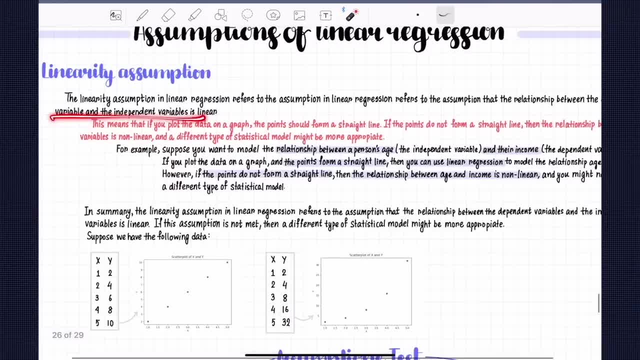 It says that the relationship between the dependent variable And the independent variable is linear. Okay, So what does it say? is the relationship between, as this linear regression? So it's expects the linearity assumption Where it says the dependent, the relationship between the independent and the dependent variable are linear. 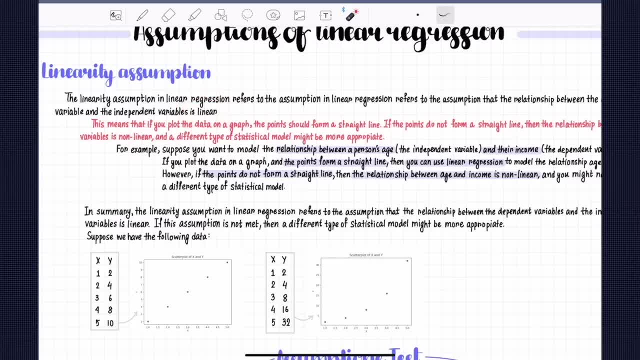 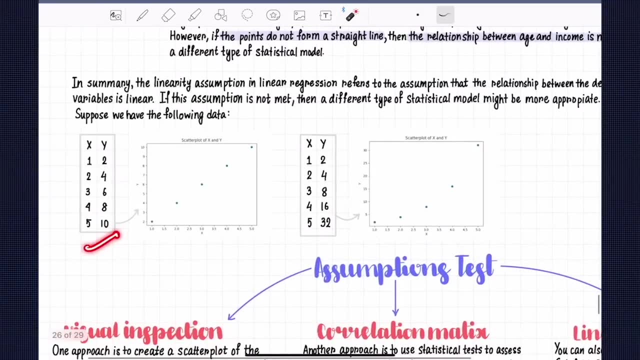 So what exactly linear is? as I've already talked about, It means that we can have the straight line which can represent or approximate our data. So we can have a straight line that can reasonably approximate our Data. Okay, So over here, this is a very nice example of the linearity assumption. 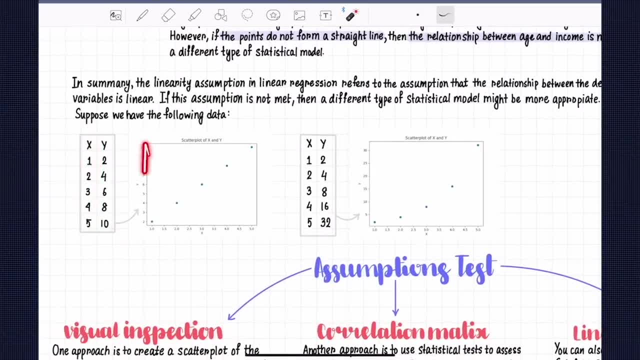 This data, where we have only one input feature and then the output variable. You plot this: y onto this and x onto this. Now, over here it can be. your data is linear. Why? Because it can be approximately on the straight line data. 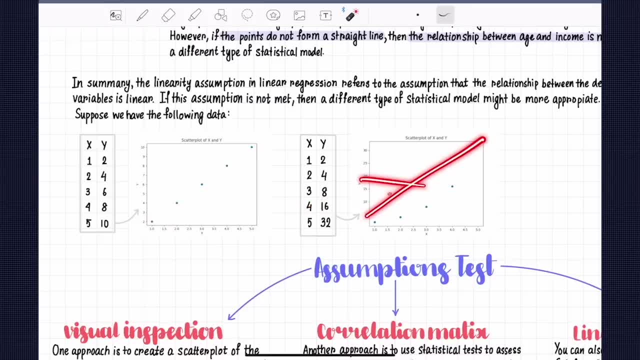 But in this case this is not a linear. over here You cannot make a straight line to data You it? it forms something like this, which is not linear: Okay, It cannot be reasonably approximated as a straight line. So that's what the linearity assumption says. 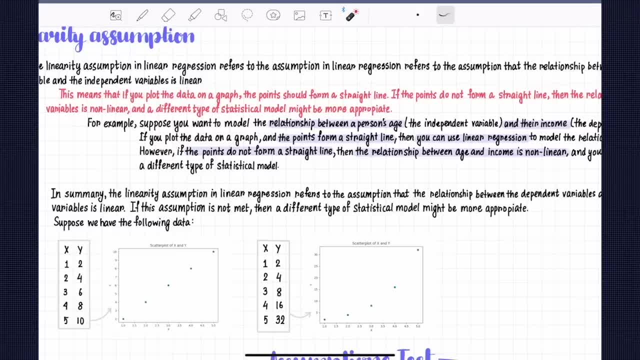 Okay, So this is important. Why this is important? or by why this is important? because accuracy of the linear regression model relies on the underlying relationship, which is nothing but linear. Okay, So if your model is not linear, assume that in this example, assume that in this example, the errors will be super, super high, as and if the errors are super high, which means that your model is not performing well and it can fit in any way. 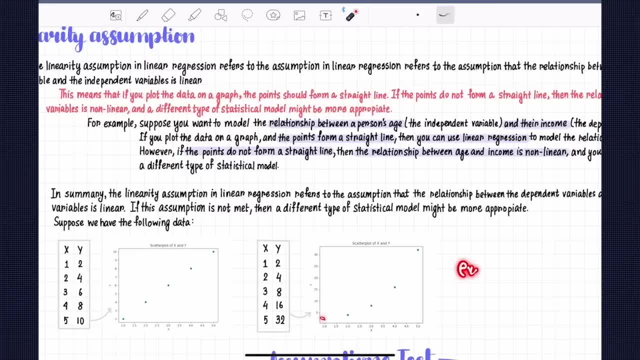 You will not be able to perform well. You have to use extensions of linear regression to work On this data, but we'll talk about that later on. but over here it will not, definitely not work well, pretty well, Okay. so this is something which you should know about. 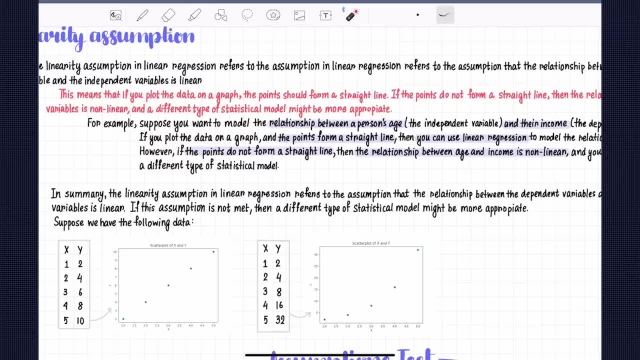 Like this is an important assumption because it will lead to an accurate predictions because of high error, Okay, cool. So once we have those assumptions, like once we have those assumptions which you can see if you plot the data on a graph, the point, the point should show that it should be reasonably represented in straight line. 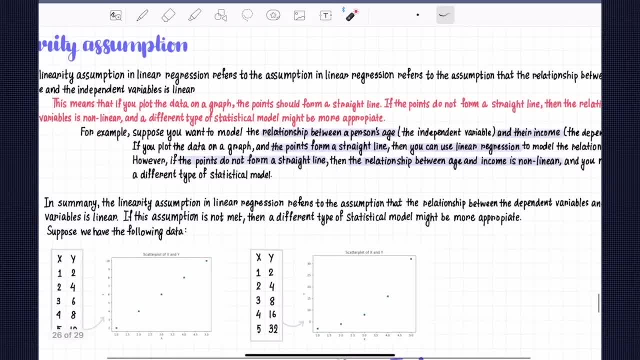 And if there's not form, the straight line, this means that they are not significantly appropriate. or we should use other significant, Significant Model, which is a polynomial regression or other regression, to actually make it more appropriate. Okay, cool, So this was one of the example. 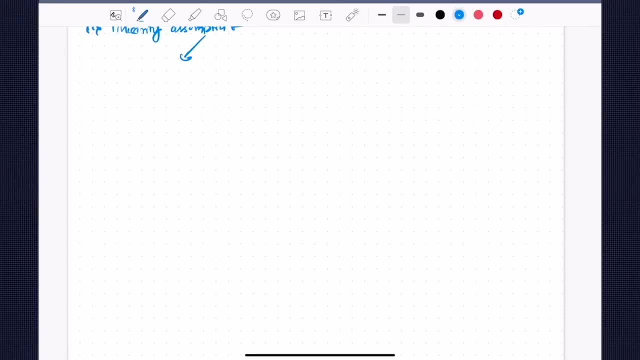 Now, as I told, once we have these assumptions, once you took it, this is assumption. Now, how can you test? How can you test if, the if if that particular problem or data set follows linearity, as I'm so not linearity, assumptions or not? 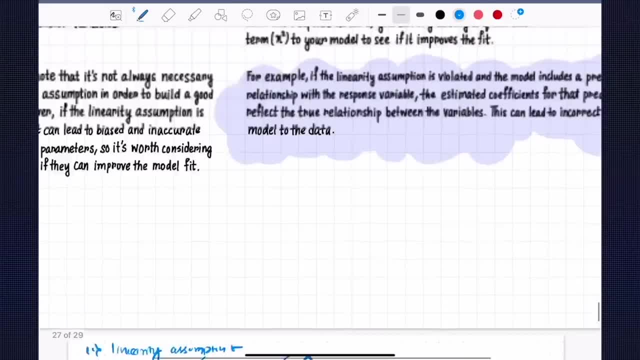 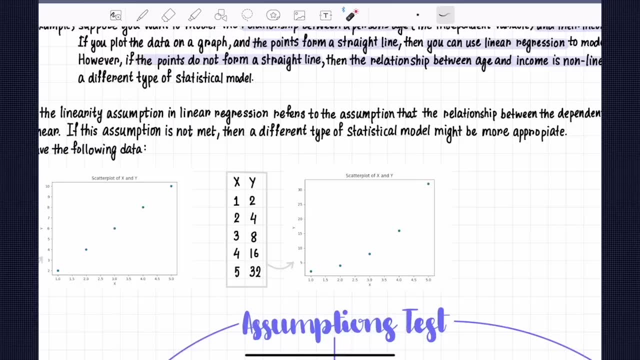 We have to test now. So we haven't. How can we test it over here? What we did? We just did a visual inspection. We just did a visual inspection. Okay, this is something which you can draw a straight line. But what if you have a higher dimensional dimensional for data? 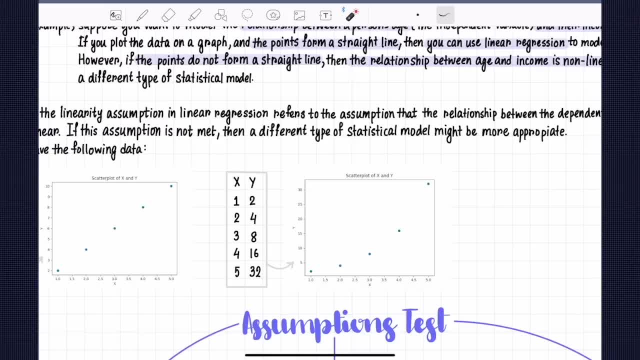 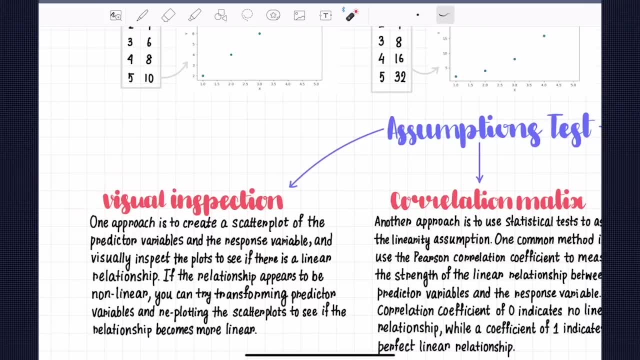 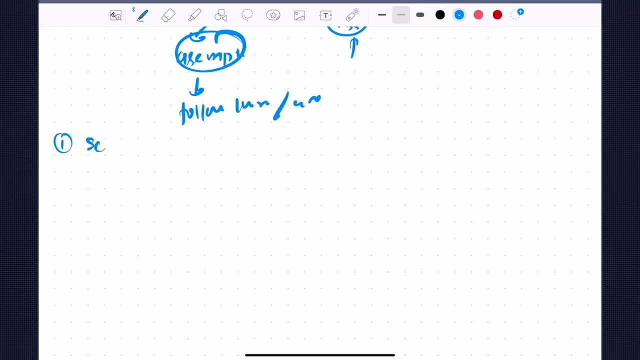 So there are several ways to test your model. Okay, the first test which you, which is which is very popular, is nothing but visual inspection, visual inspection. So, in that visual inspection, in that visual inspection, what you do, what you do, the first thing which you do is scatter plots, scatter plots. 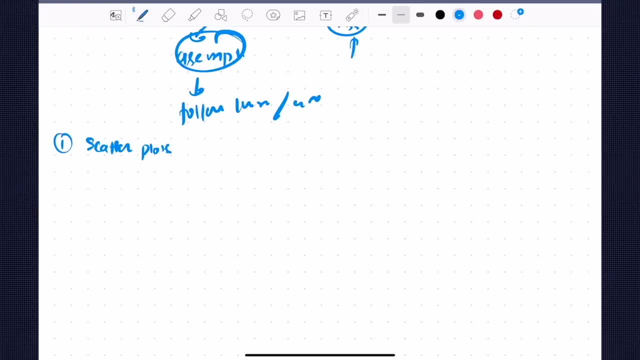 The first way to test, if that, if your model, for if your data follows linearity, assumption Not is apply scatter plot. So what exactly scatter plots does? So what exactly scatter plots does? What is it? does we? we simply take an independent and or dependent variable. 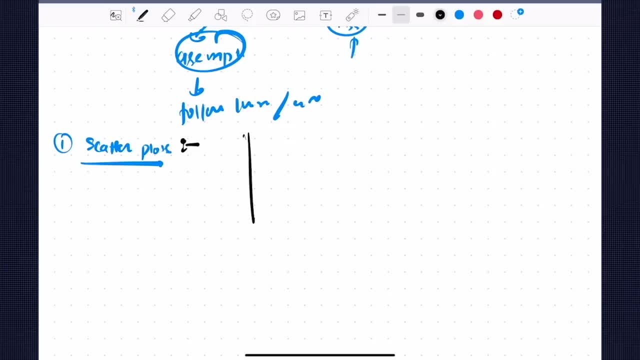 We have to of course, do it in a 2D plane, of course. So when you have the on y axis, you have the dependent variable. x axis, We have independent variables and you plot it. So if the relationship shows the straight line or the or the linear data, that that means it is falling. 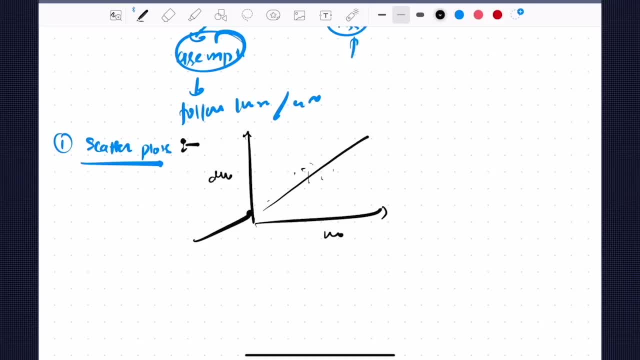 But if it does but it does not, then then it is not. your assumption is not satisfied. So visual inspection is one of the most common ways As well, but we have. the only downside too is if you have a more number of variables, large number of variables, input features, independent features, sort of plotted against every individual, and see if it works. 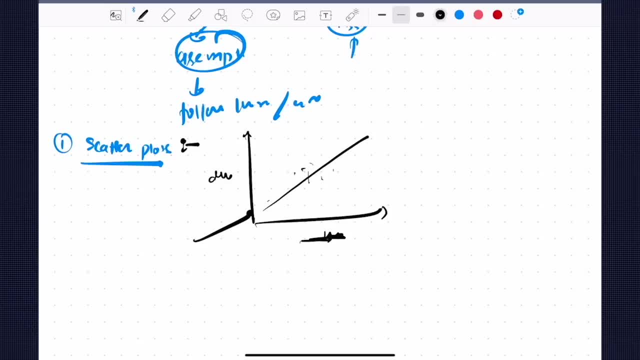 But. but you know it's sometimes not good as well, but eventually it helps you to get a better understanding. But this is scatter plots to eventually help, OK, so so this is. this is one of them. Another one is which is more common. 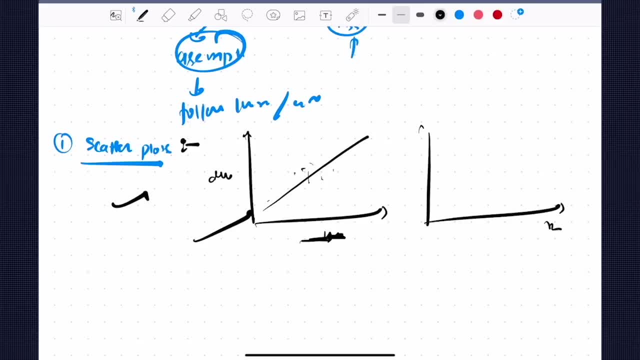 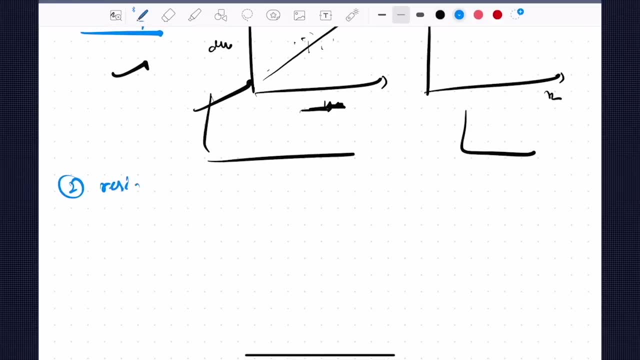 Like over here, we have to plot for every individual independent feature, X2 and then Y, and X3 and then Y, and all we have to do for a scatter plots. But but another example is that I said how can you test with residuals plots, residual plots. 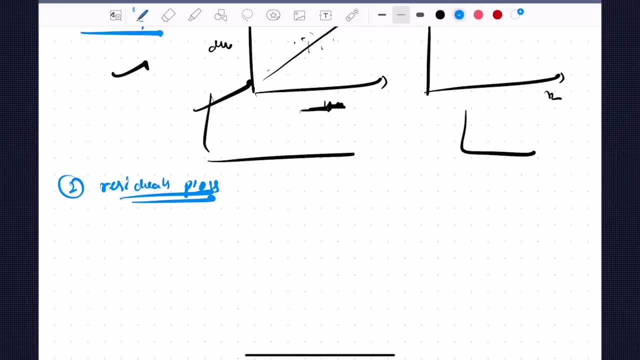 So residual plots plots is one of the most common ways to, to test those assumptions. What you do, you simply put you simply and you simply take the. you simply take the residuals and then put it on a Y axis against the predicted or the predicted values or the independent variables. 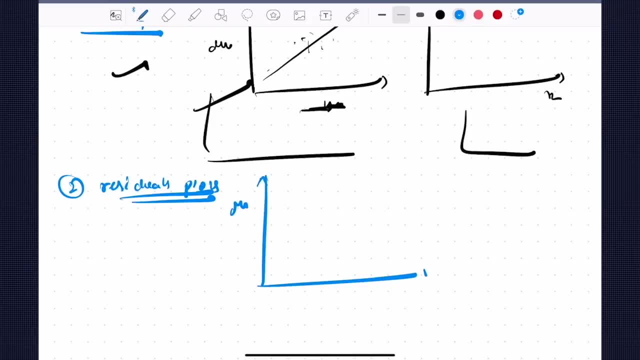 Basically, you take you on Y axis, You have the residuals on by Sorry. on X, You have the prediction, the prediction OK. on Y axis, you have the residuals on Y axis, Y axis prediction- sorry residuals and put on the over here prediction. 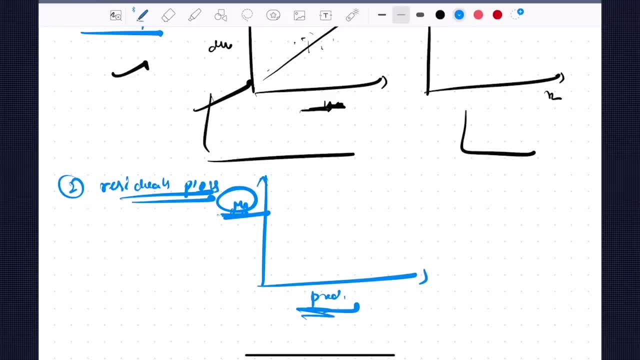 So you might be thinking here: how does it even make sense, Right? So let's, let me show you a very nice example of how what exactly residual plots looks like, so that it makes perfect sense to you. So I'm just going to take a very nice example. 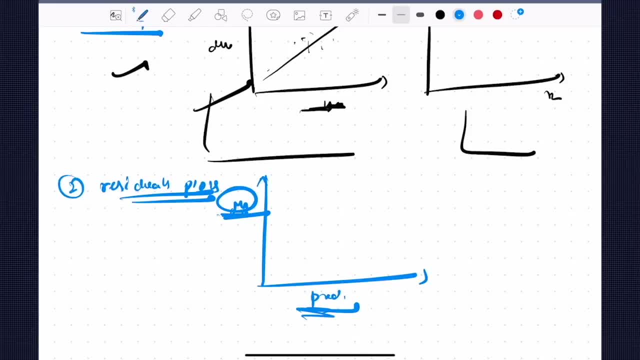 Maybe that will make much more sense. So I'm just drawing out a very nice example so that I can Actually send it from Mac to my iPad. That really works. You know, sometimes it works and sometimes it does not. So let me just open up a very nice 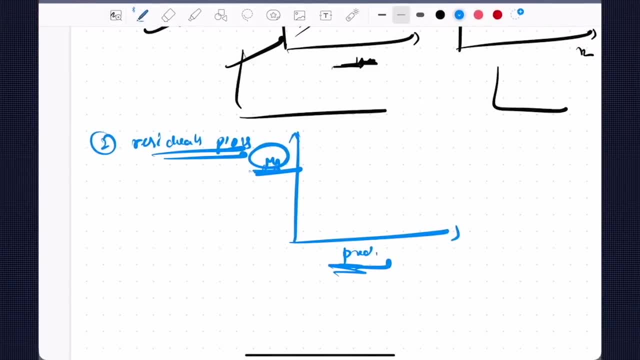 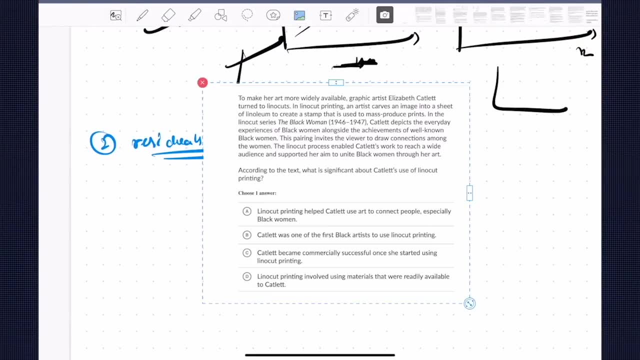 So open up a safari. Where is my safari? Yeah, So, yeah. So how can I download this? Oh, so I send this on my laptop, from laptop to over here. Now I should be able to show to you. So this is the example of a residual plot. 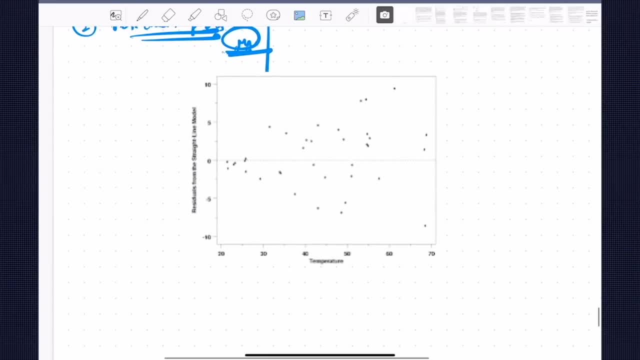 This is an example of a residual plot. And what does this plot sees on on x, on on x axis, you have the temperature and then y axis you have the residuals. now, if you see that, now, if you see the when you, when you plot the related values against the residuals, 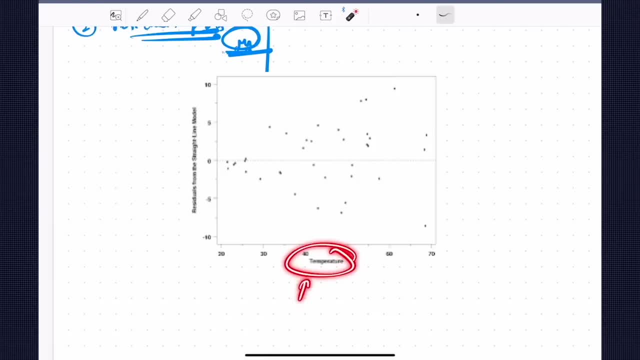 against the residuals, the odd, or even attempt, or even the independent variables against the residuals. it should show what it should show. it should show a very, uh, a very random scattered point. so over here, you know, you see, they are very randomly scattered. there's the, there's not the. 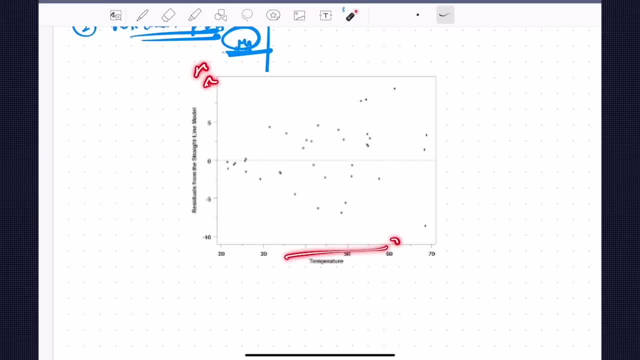 residual plots. there is the. on y axis, you have residual. on x axis, you have the independent variable. so this does not forms any sort of you know, a pattern like this. uh, what, what patterns i'm talking about? for like this, or like this, or like this? it is not forming, it is. it is a very 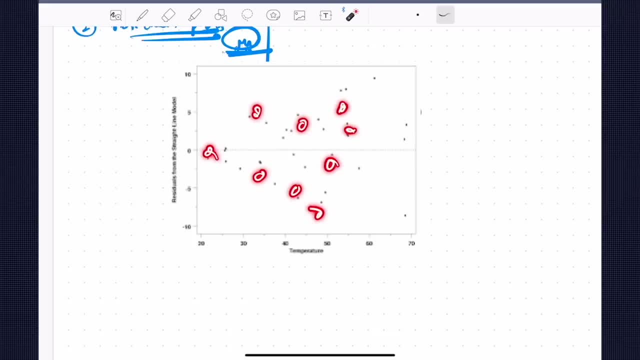 random one. you cannot even fit any sort of model. it is very, very random. and they're around zero. only they're around zero, okay, so so, if, if, if, if the linearity assumption holds, if the linearity assumption satisfies, the residuals are: uh, the residuals are scattered randomly. are scattered randomly? okay, are scattered randomly. 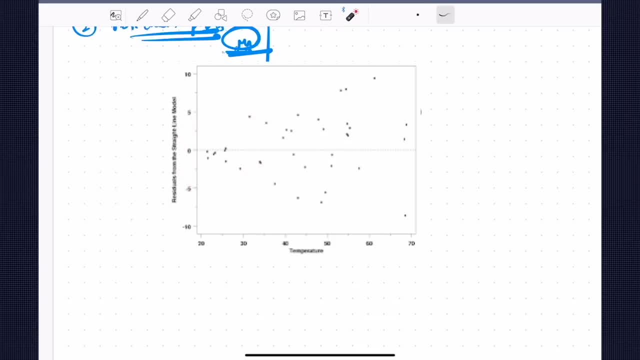 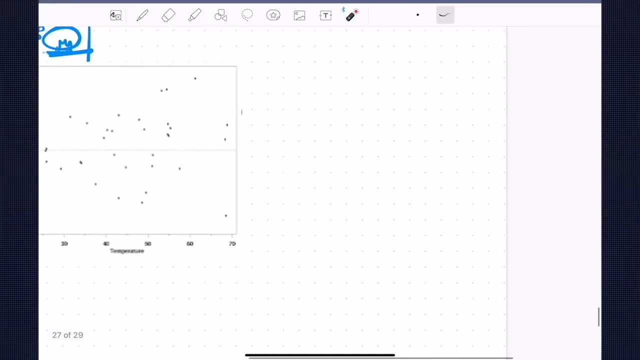 and they're around zero. they're around zero. okay, i hope that you are. you are unable to understand this pretty well? uh, this is. this is the visual inspection. this, this is what you do for visual inspection. another way, is something known as uh is is is something known as partial regression plot. 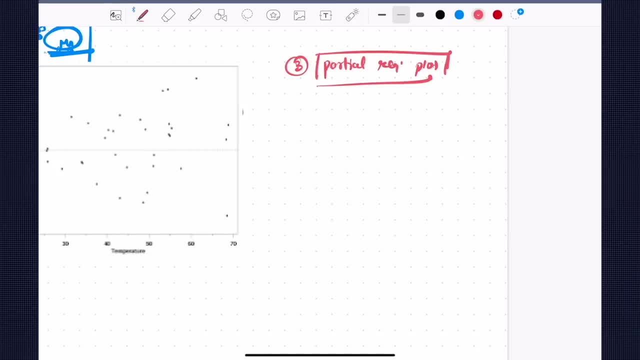 partial regression plot. partial regression plot, and this is something which you have to explore by your own. this is something explored by your own. i'm not going to teach, teach about that, but you have to explore by your own. uh, because this? um, because now you are at a stage where you have to explore by your own, as 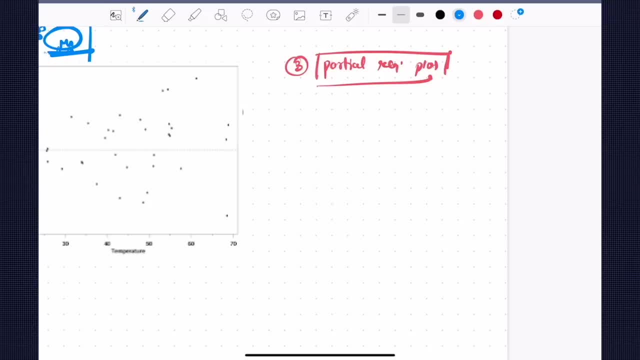 well, i cannot spoon feed you everything but this. this is one of the way which you, which you should explore right now by yourself, another way to test, another way to test: it is nothing is nothing, but something called as statistical tests, statistical tests. so we have seen our, our hypothesis testing. 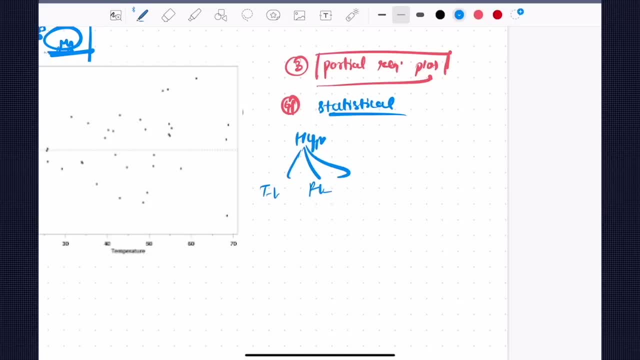 in that hypothesis testing we have several tests. which is t test, you know now? so there are there's several tests for space testing the significance of our coefficients or independent features. so just like that, you have a tests for testing the linearity assumptions, for example. one test is nothing but a rainbow test is nothing but rainbow test. 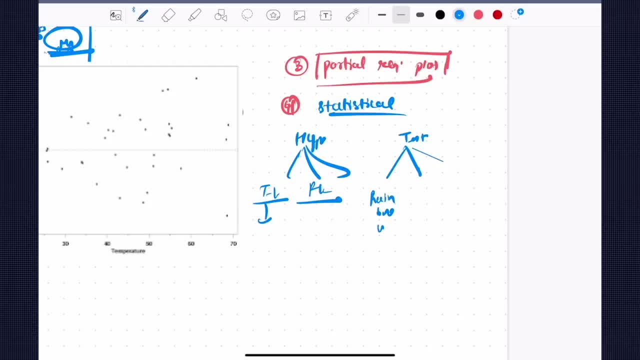 rainbow test. i'm not going to go in mathematical details of it because this is something you're not studying statistics in detail. if you want to study statistics, just go and search more. if you're interested, you know. but i don't suggest you to go in so mathy details of it because nobody usually 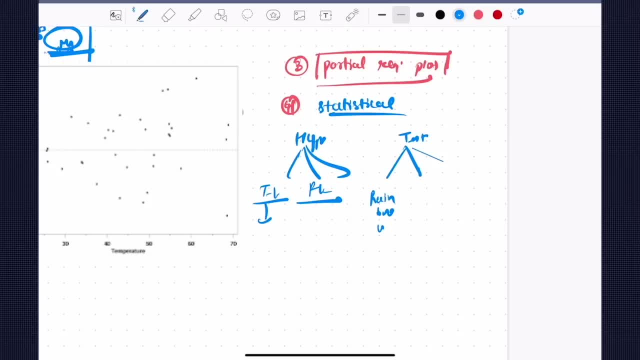 asks: you just need to know. okay, there's something test available have to use for testing this linearity, or maybe something known as Harvey-Cohler test, which is one of our one of the most statistical tests, which is often used for testing the significant other like: how can we eventually talk about things? how can we eventually test if, if the model is linear? 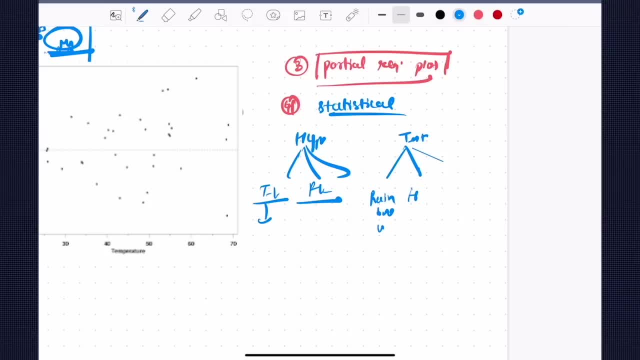 or not. okay, so just you can. you can explore the mathematical thesis. how do we test exactly? but it just follows the same thing which i've studied. the test assesses we have a null hypothesis. the null hypothesis states that. the null hypothesis states that. what is it test? it states: 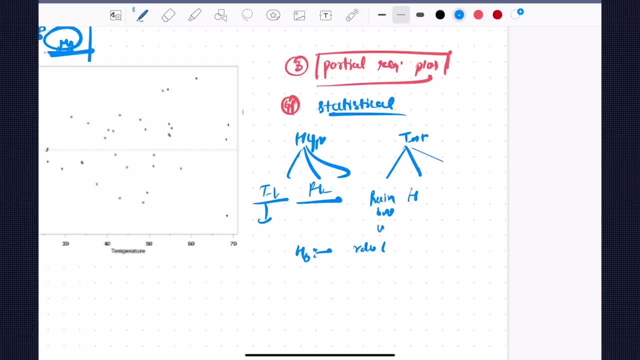 that the there's the. the relationship between the relationship between your x and y is linear, so it. it assumes that the it already assumes. now we have an alternative. it says that it is not. the relationship is not so. so so what we do? we conduct the test and once we have the critical, uh, the p. 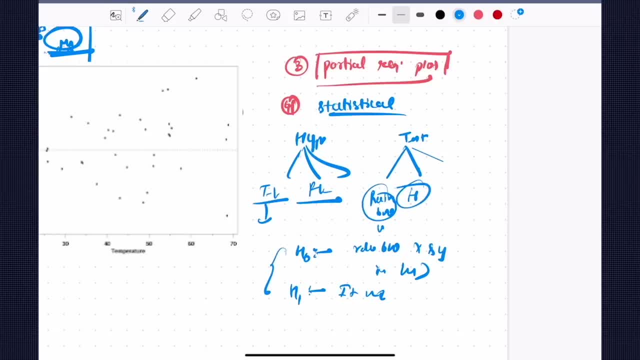 value. if the p p value which we get from after conducting the rainbow or the these tests, if it's smaller than 0, 0, 0, 0.05, which means, which means that uh, which means that you can reject the null hypothesis. and if, if it is more than you can reject the null hypothesis, which means that assumptions is. 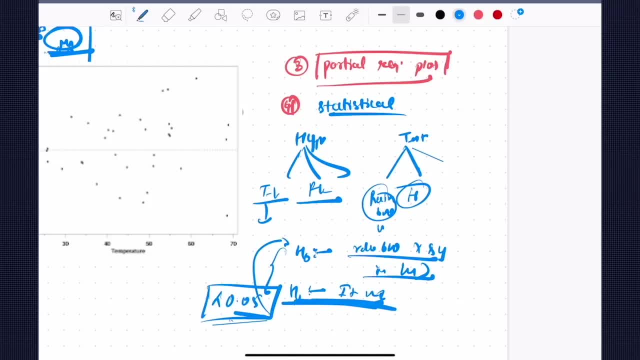 is not satisfied because you're seeing that it is not linear. okay, so this is one of the- this is the. the same same concept holds for every hypothesis testing. another, another example is another example. so these are some of the- uh, some of the ways to summarize up: linear regression assumptions holds. 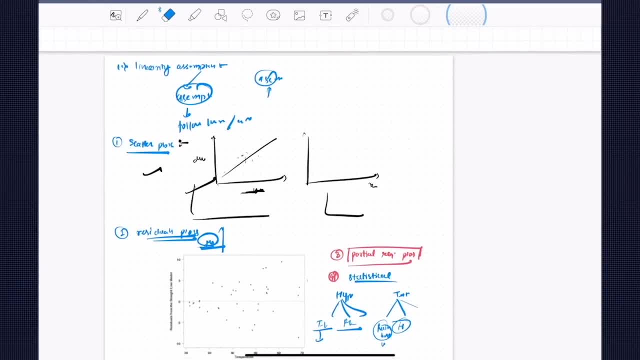 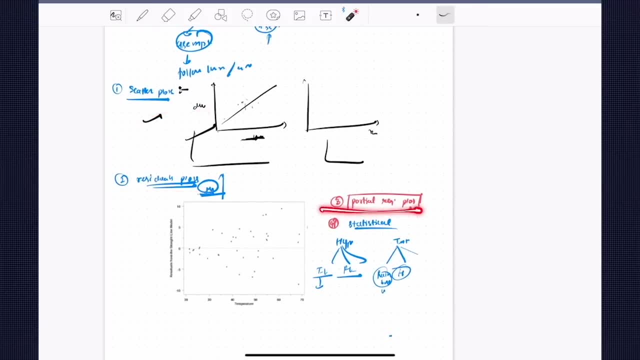 for you know, uh, there should be linear significance, significant relationship between the two variables. uh, we have scatter, scatter plots, then we have residual plots, and then we have partial regression plot and statistical plot, and that we have, uh, hypothesis and tests. uh, sorry, there's several hypothesis tests available to test with the darts whether it follows. 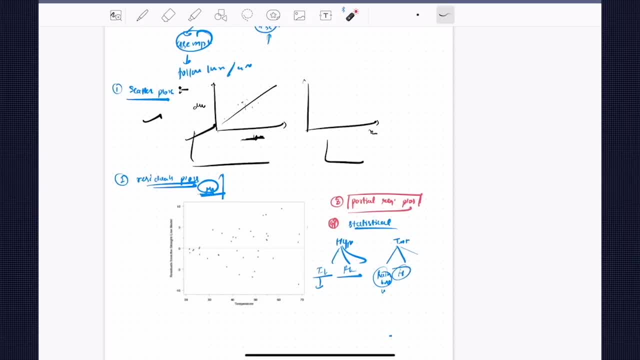 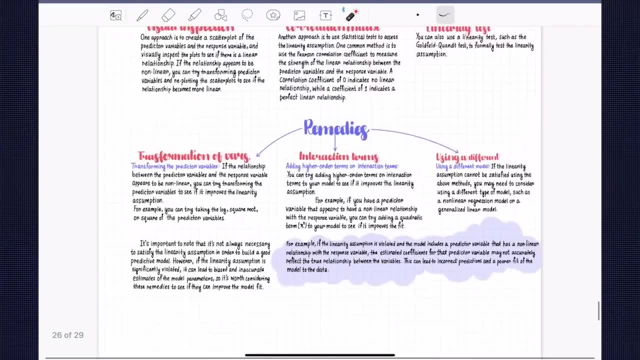 statistical or not. okay, i hope that this gives a good sense about our linearity assumption. now, what we'll do? we'll talk about something known as another assumption, which is nothing but called as, uh, the remedies of it. yeah, yeah, this is. this is one of the. 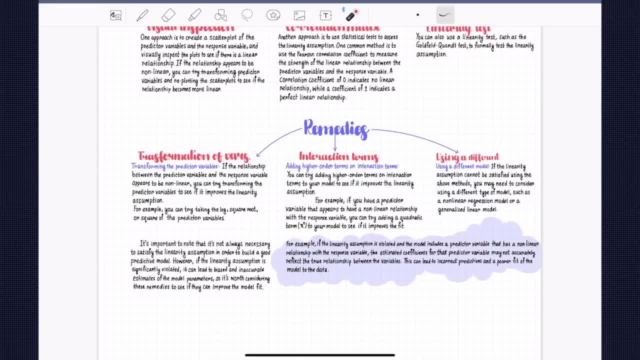 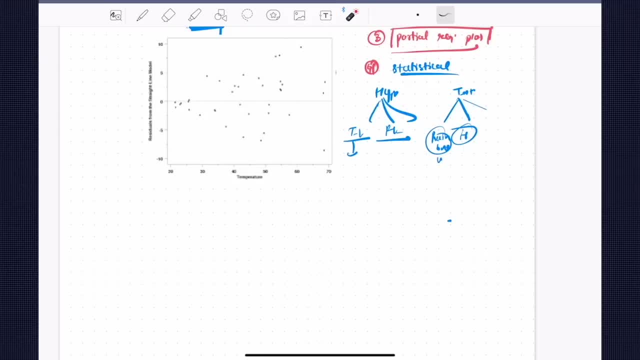 to think about. yeah, i just forgot like we have some remedy, remedies about how can we fix so once our assumption, so assume that your assumption is violated. so assume that your assumptions is. assumptions are violated. assumptions are violated now if the if your, if your model does not satisfy. 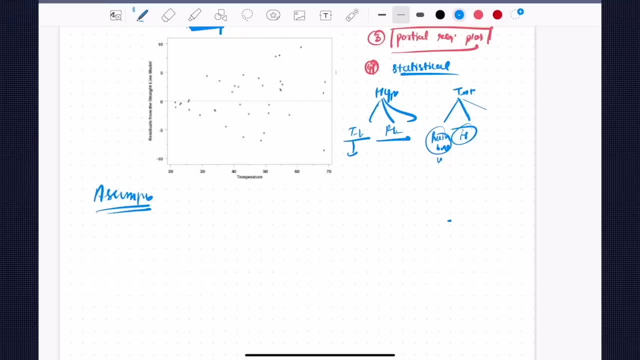 linearity assumption, which means that your model is not going to work well, right, so so we give. so you here. you might be thinking: okay, you told about that, this will not work. well, so what we should do if this does not work? so i will say that fix that assumption, make it the make, make it from. 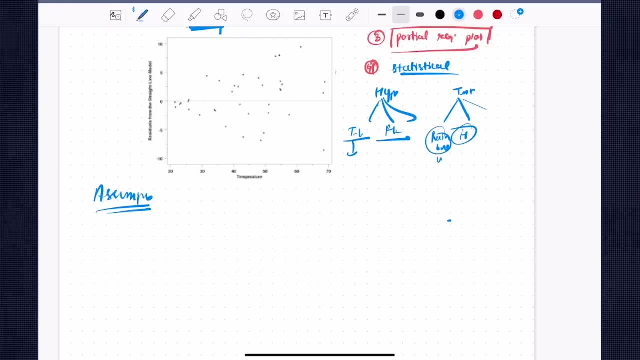 non-violated to non-violated assumption. okay, and this is what you have to do. so there are several remedies for it. you know, remedies mean something to fix if they, if it is, if it is being violated, we have to fix that as well. hashtag fix, hashtag, hashtag fix is also a very famous thing, so you 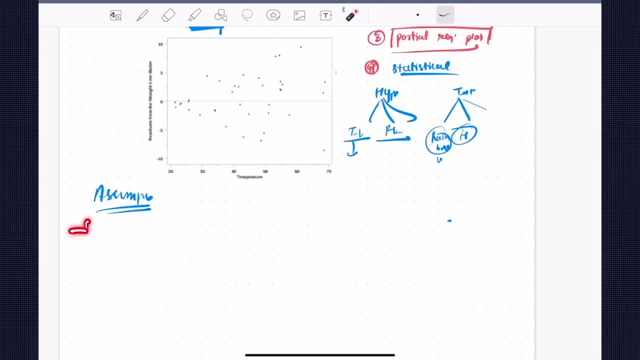 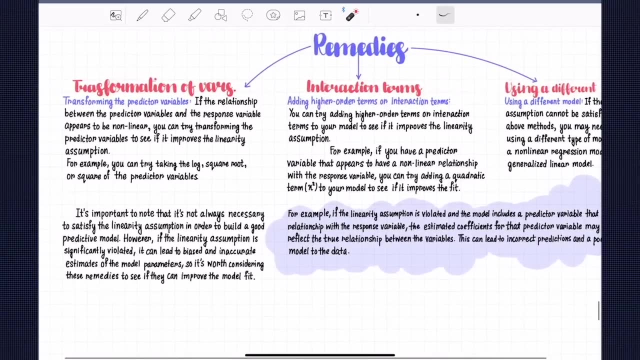 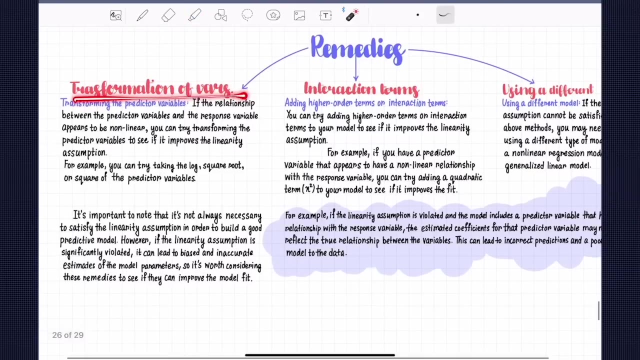 have to fix that assumption. so there are several remedies. the first remedies is nothing but called transforming variation variables. the first remedy is we call transforming of our variables transforming of our variables. over here you can see that we transform our variables. so this is one of the transform. 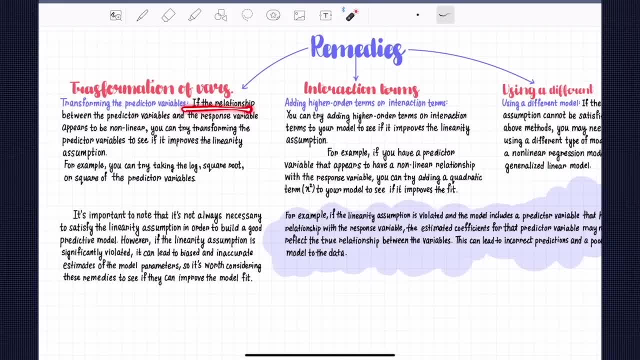 variables. so what does that mean? transformation of our variables, which means that if the relationship between the predictor and the response is appears to be, you can try transforming the predictor or to see. for example, you can take the square root or log or or a square of a variable, for example. 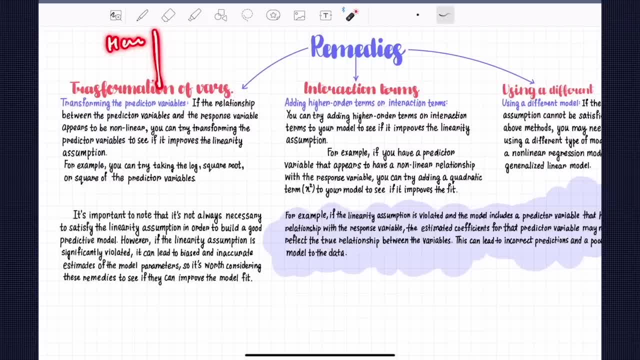 assume that you have a house price square and then you want to predict based on the. so you know, based on the size, and predict the house price you have. you have something to 1000, then you have 200,000, then 250. sorry, 1 to. 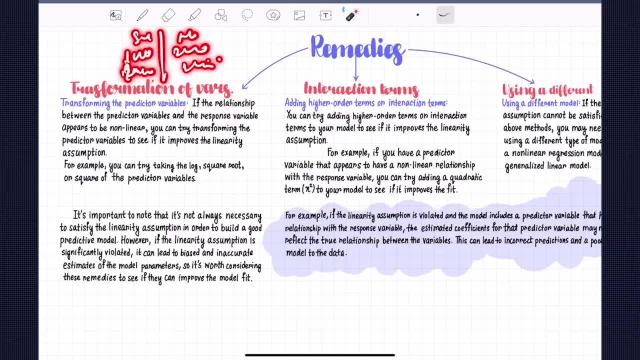 200 square feet, then you have to 250,000. so you, what you can do, you can apply the log, you can apply the log or the square root. you can apply the log or a square root on, you know on maybe, on on on variables. okay, on on variables, so that it comes on a it it becomes linear. okay, so you apply. 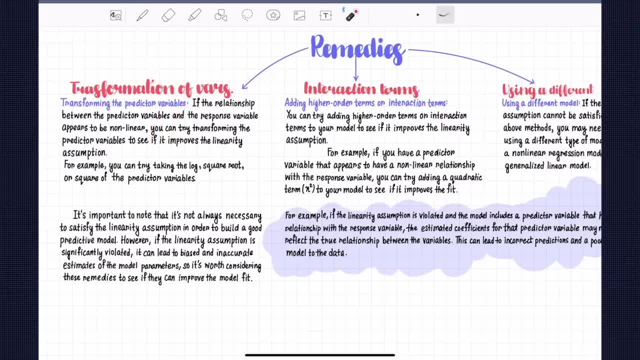 the transformation on the variables. you apply the transformation of variables to study more about feature engineering. so if you want to study more in detail about all of these things, i suggest to take the course which is cs01b04, which is one of our famous course available online, um, so you can. 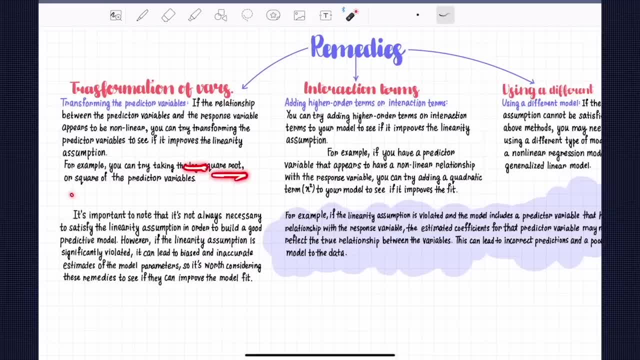 actually, uh, talk about this, so we get, we, we take this log, a square root or a square of the predictor variables or independent variables out there, so that it works perfectly, so that you bring that, bring them back into the linear way. so i think the log, it of course comes in a linear uh. so this is a 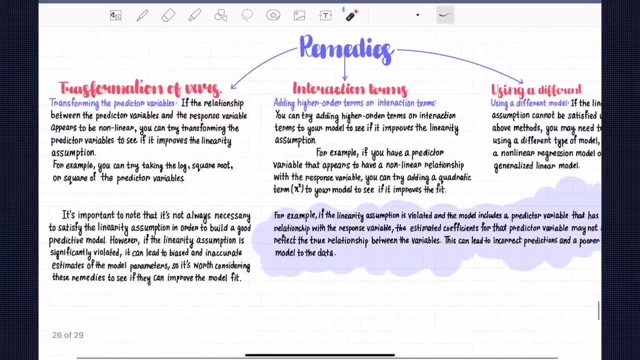 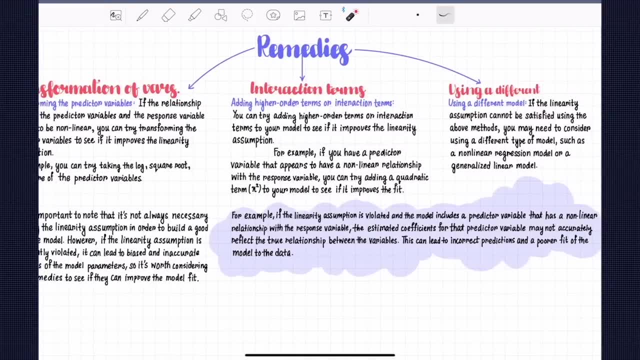 very nice uh. so this is a very nice uh. so this is a very nice uh. note to make sure. so that's one of the transformation of variables. another one is add higher order terms. add higher order terms or interaction terms, which means that if you have your x variable, then you make another variable, x, but you square that. but you square that okay. 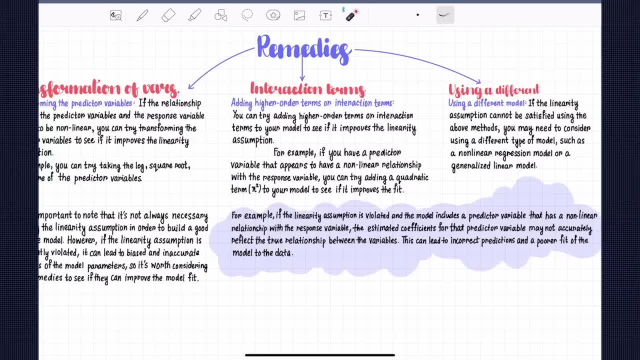 so you add the, so you add the cubic, per cubic terms or quadratic, to help capture even the non-linear relationship. so eventually this introduces a concept of polynomial regression. and this introduces concept of polynomial regression- but that's something for later on- where you introduce the higher order of you know uh, intra the variables, where you just take. 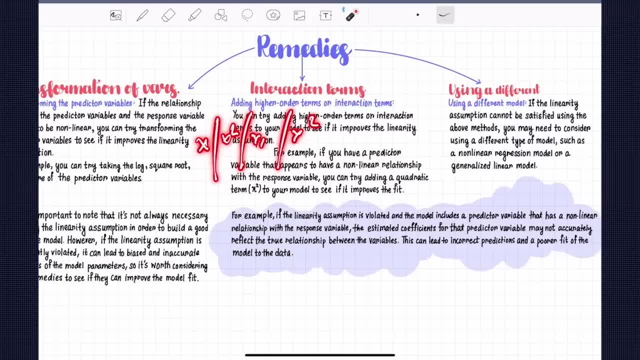 the x and then take the x squared and then you have x 2x- 1- take the x 1 squared. so you just introduce the higher order uh terms, for example quadratic or cubic, which helps to capture the non-linear relationship. another one is like: if nothing is working, then you should start going on. 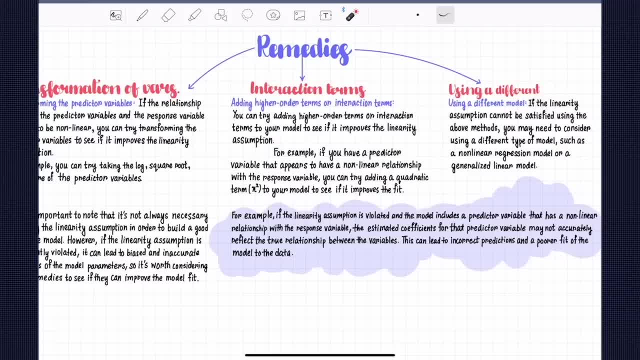 to take out the different model. okay, different model means you can consider using g-relativism, GAMs or decision trees, models like random forest, which can better capture. if your data is nonlinear too much and not able to satisfy the assumption, then I think you should go to random forest, or 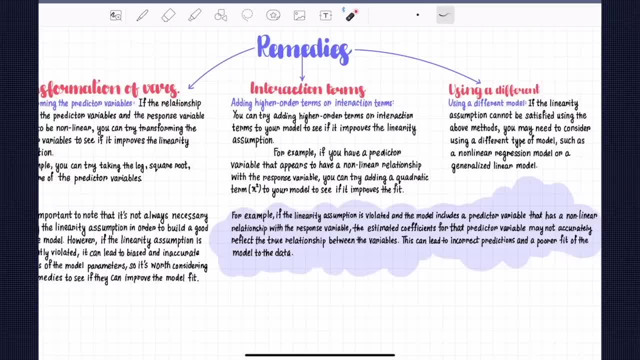 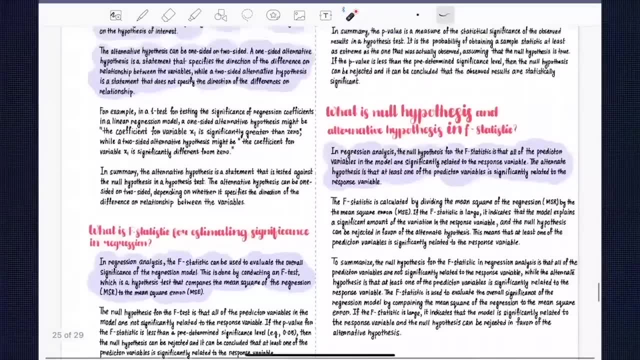 somewhere like that to actually cover up our assumptions of random forest. Okay, cool. So I hope that gives you a very nice understanding about linearity assumption. What the next which we'll talk about, is something known as independence assumption, which is also a very nice assumption. 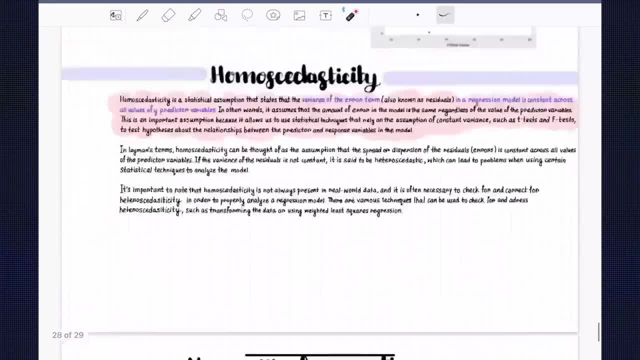 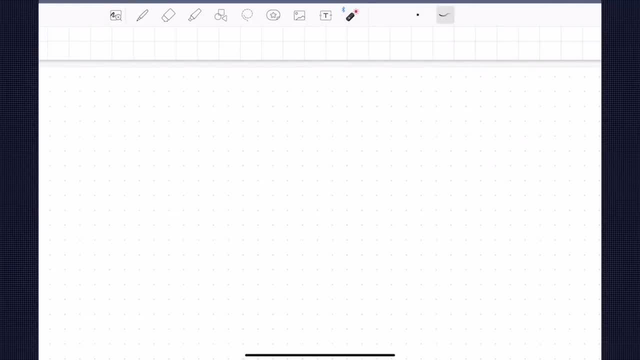 And then, after that, we'll talk about homoscedasticity and normality assumption, And then we'll wrap up the lecture on this. Everyone, welcome to this video. In this video, what exactly I'm going to do is going to talk about independence assumption. This is one of the- again the second. 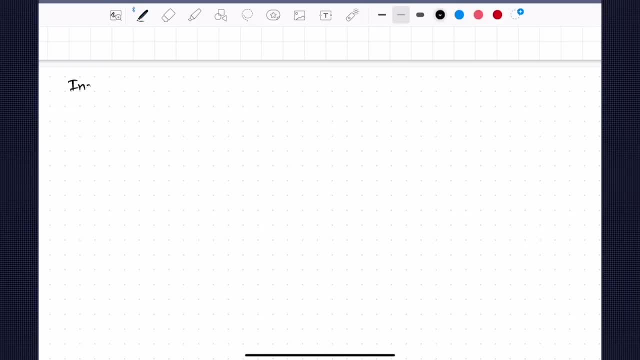 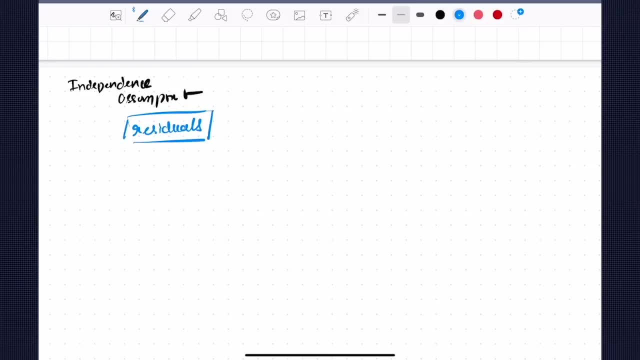 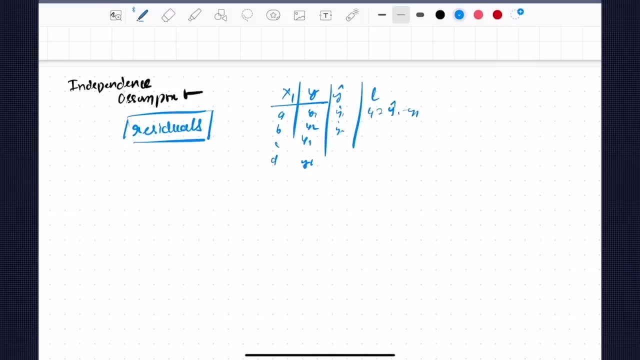 will be will be: error one is equals to y hat one minus y one. error two is equals to y hat two minus so, so the error number one should be independent of error number two, or error number two should be independent of error number one. Okay, so errors or residuals associated. 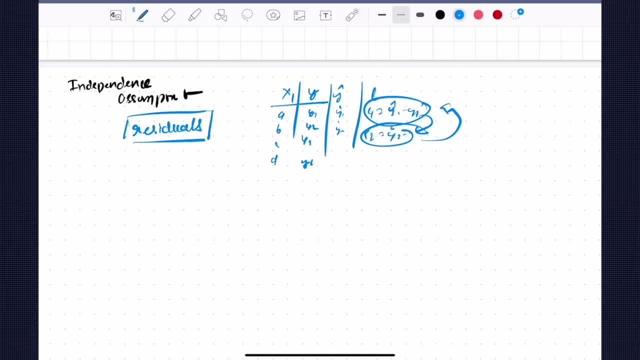 with the in this the data or the observation should be: should be uninfluenced by any other observation out there. So error number two should be uninfluenced by any other. So error number two should not get affected by the error number one, okay, or error number two should not. 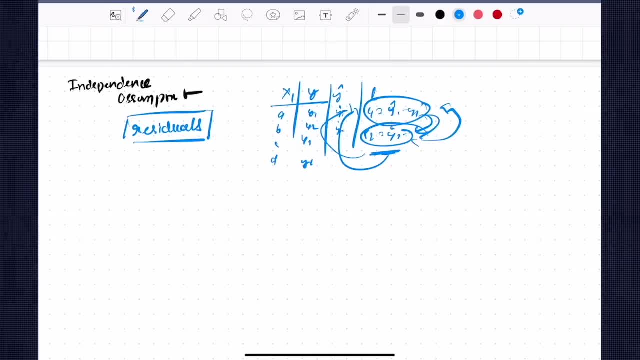 get affected by anyone else. So I guess the independent assumption states that the assumption switch it holds, that that your observations associated with one observation should not influence the error associated with the another observation. Okay, if you don't fix this, you will end up with biased results, inaccurate estimates, unreliable predictions and a lot of things can. 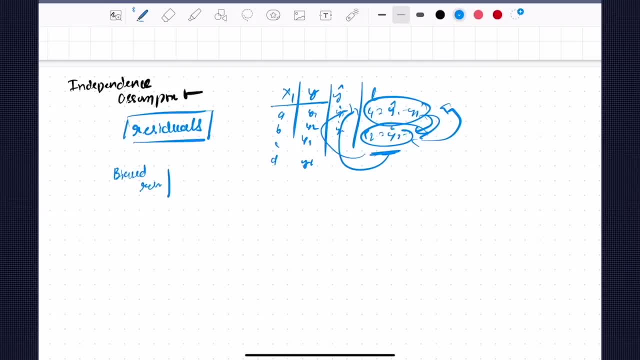 happen. So this is the, this is what the assumption state that your, that your error should be independent. So let's take a very nice example. So example states that that you have. you have something known as electricity. So you know, predict the electricity based on the, based on the temperature in a city, based on 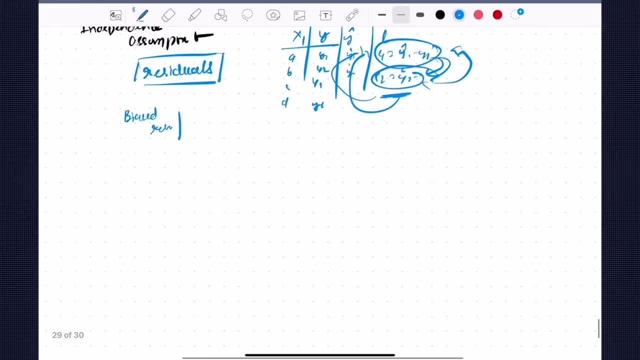 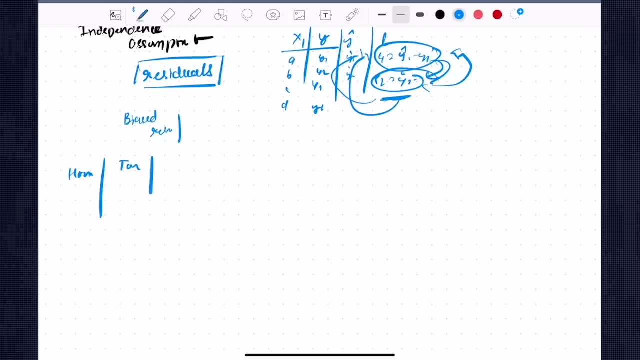 the hour. Okay, so we collect the hourly data for the entire month. So you have hourly data, which is, and then you have temperature, okay, and then you have your electricity demand, temperature, electricity and demand. So let's say this is an hour, you know, and you have a temperature of 33.15, 1617. dot. 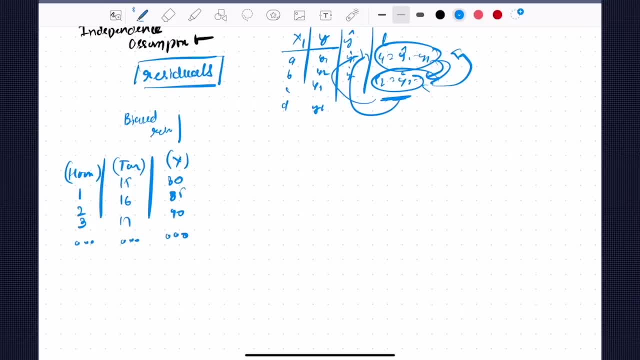 dot dot and 8085 and 90. dot dot. So this is, this is one of our, you know, this is one of our, this is one of our data which we, which we have in our annual test, whether this assumption has holds the independence assumption or not. So if you see that the demand for electricity 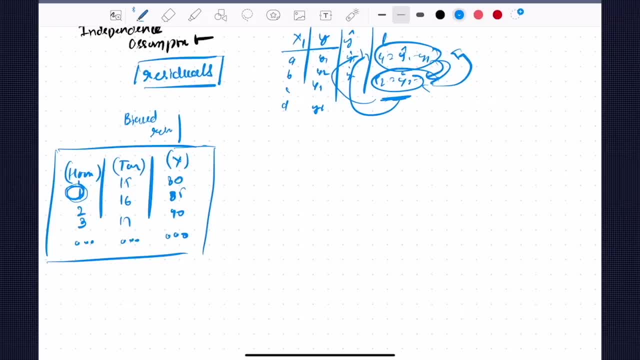 at one hour, at one hour, at one hour, might be related to the demand of the previous one, right? so, basically, so, basically, what? what is it trying to say you? it's, it's something which is trying to tell you that assume that the electricity demand at at hour two might be. 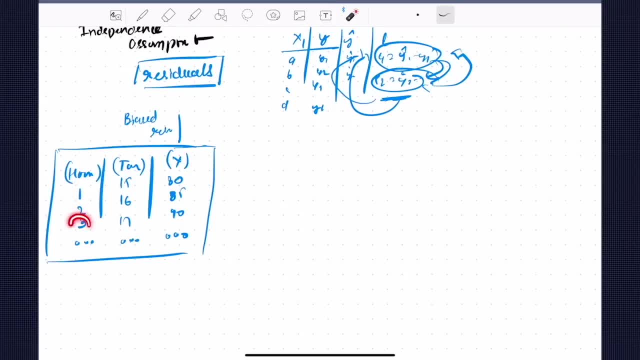 related to previous hour. right might be related to previous hour, electricity at three might be related to the previous hour. hour number three might be related to the previous hour. so you see that there is some sort of relation and, as we said, that there should be not any relation, of course, if 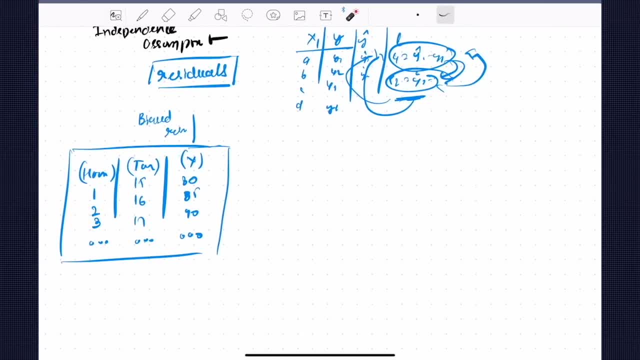 this is related, then of course, errors will be also related. okay, so electricity uses strengths to show a pattern. so when you when, as we are using electricity, it is being so that we have it is greater than the previous one. that's what it is showing. okay, it is as the hours increases, your 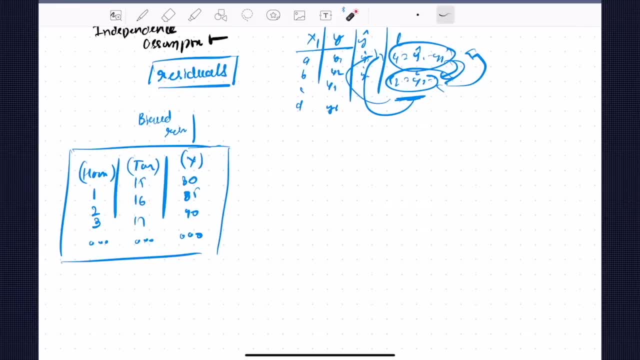 demands. also in this it is showing such some sort of pattern over the course of a day. so it is, of course, showing the pattern over the course of the day because it is related to each other. so what is it showing? for example, over here, higher the demand is higher in the day and lower. 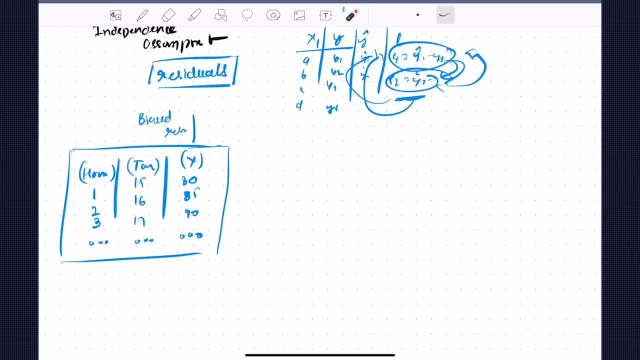 demand at night or lower demand at night. so this is something which is, which can, which can be showcasing the patterns. so, over here, this is showcasing the trends, which is not good, right? this means that our, that our points are independent, violating the independence assumption, and that's one of our important major issue. so that's this, this is what assumption indicates. 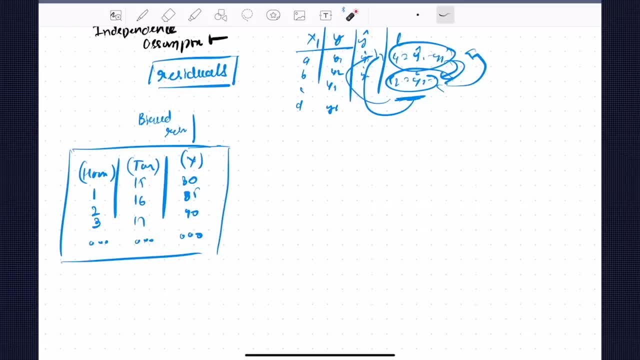 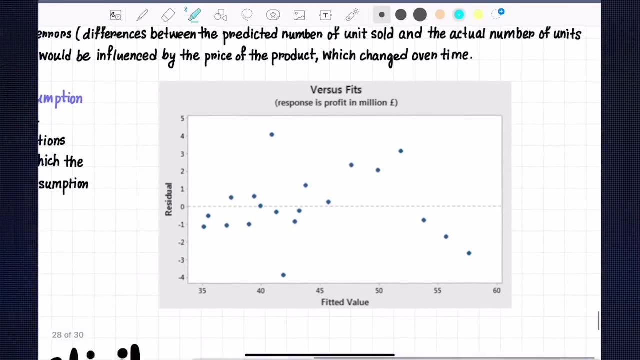 how can we test our assumptions? for testing our assumptions, for testing our assumptions, we have couple of things. again we can talk about residual plots and residual and plots, so that again, you, you can, you can take your residuals and plot it and plot it, or like like this: you take the residuals and plot it on a y-axis and you take the fitted value, the prediction. 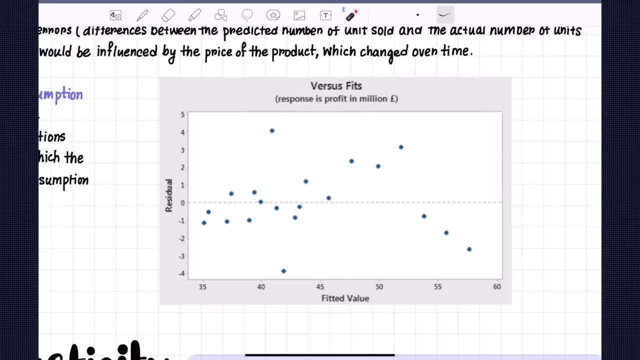 value product on x-axis right, and when you plot it, and when you plot it, you will see, you will see that, you will see that, uh, you, you will see that, uh, you will see that there is no patterns or trends of the residuals. so there is no patterns. there is this. there's no certain patterns. uh, over here. 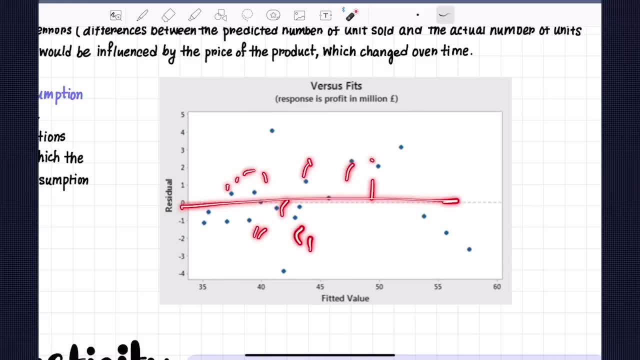 there's over the line. they are distributed randomly or scatteredly. if there's some sort of patterns like this, you know, like this, so we can say that that's that something does not hold true. but over here this does not have pattern, but but in the case of this it will hold a particular pattern. when you when this particular example, it will hold. 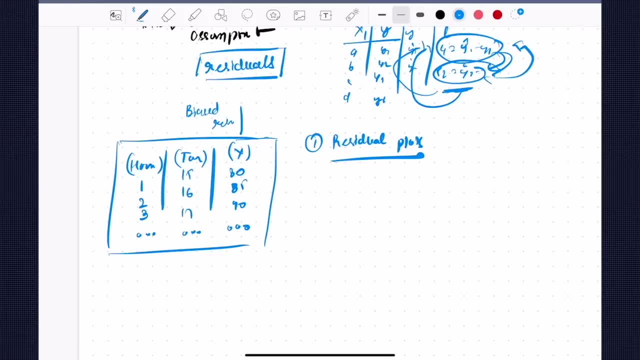 a pattern, okay, uh, so you, this is a visual inspection, uh, from which you can see the another one is nothing but called statistical tests, statistical tests and statistical tests. what does it say is that you have couple of tests, which is a couple of tests, and you have a couple of tests. 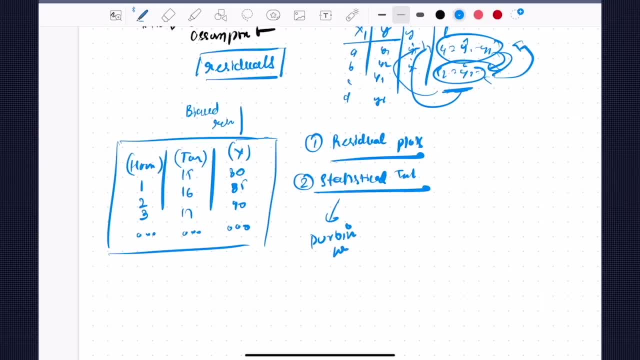 durbin watson test. durbin watson test, which will give you some sort of number, and then we say that, okay, that that number is greater than the significance of 0.05, which is a p value. then we say, okay, we can reject the null hypothesis and say, okay, this is something which is 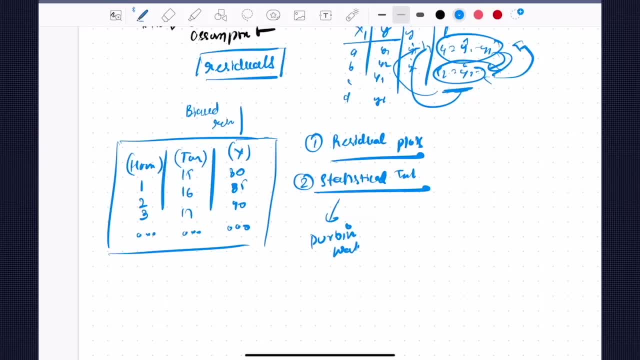 correlate. so we'll talk. these are tests which have already seen the way we conduct tests and all in previous lectures. but durbin, watson test and worship godfrey test, godfrey test. so let's talk about a bit about durbin, but your, your stance should be that you are making it. 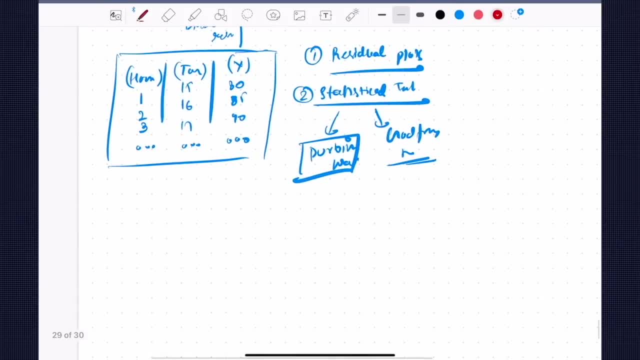 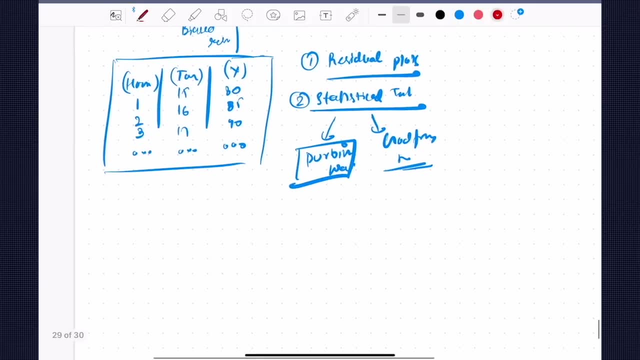 researching a bit more about it. okay, and so how can we so that? so there is one of them is: um, is what we can do? so what exactly the durbin watson test means the durbin watson uh is specifically was introduced what, how, why it? why it was introduced: it was introduced to detect the 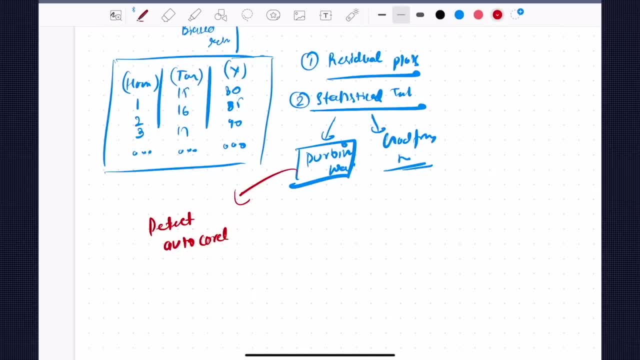 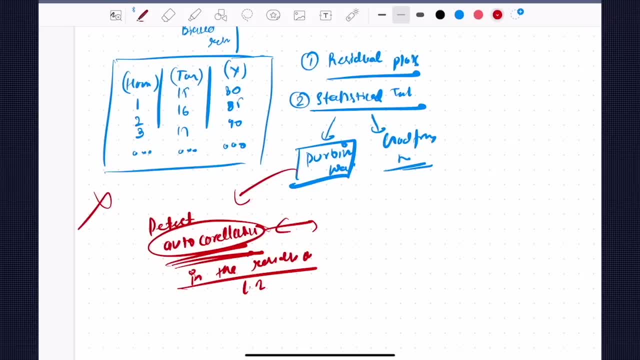 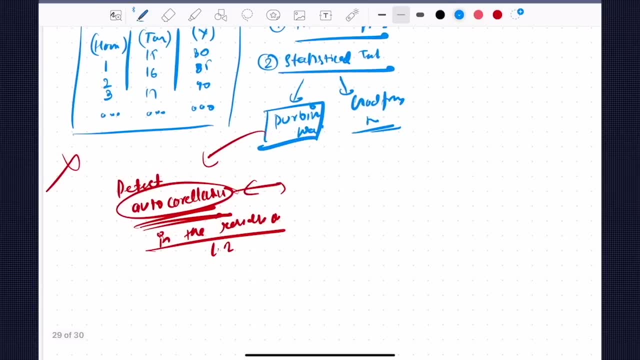 they don't. they don't satisfy this, that the independence assumption, and if they are not correlated, then then that they satisfy the assumption. okay, so your durbin watson, the durbin watson test, which you have, it lies between 0 to 4, 0 to 4, and if your durbin watson gives test, 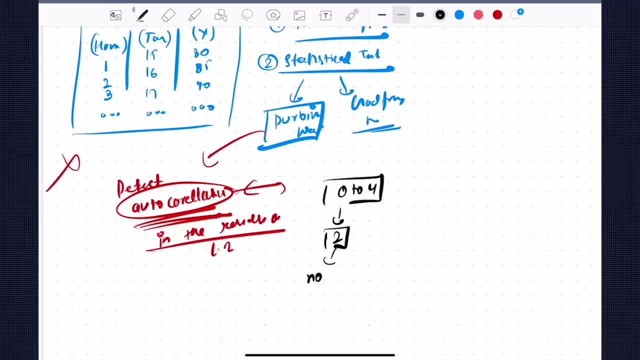 of a 2, value 2, which means that there is no autocorrelation. and if there is no autocorrelation between the situations, that means the assumption satisfies because there is. there is no barrier correlated with each other. okay so, but if the values are less than? if the values are less than. 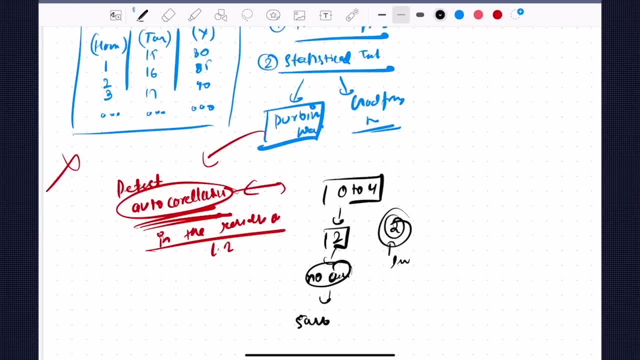 2. that means there is a positive correlations, which means there's a positive. we have already talked about positive and negative correlation. please see the lectures of probability. if you haven't bought the course, please go and just enroll in a course if you haven't studied about. 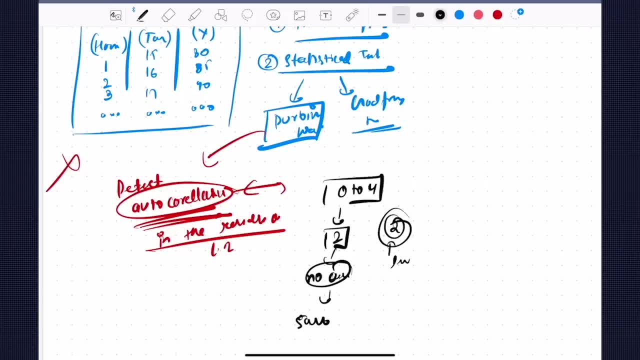 probability statistics. so value less than 2 suggests that the positive correlations are nothing but are nothing but the positive correlations which you have is nothing but a value less than 2. if your durbin watson test statistics give less than 2, that means they have a, they hold a positive. 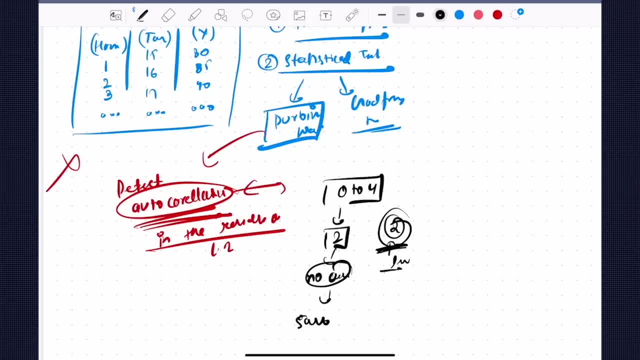 correlation, but which means the residuals are positively correlated across observations. but your value is greater than 2. suggest negative correlation, which means that residuals are negatively correlated. so your value should be 2 if they want to satisfy this assumption. if they are less than 2, that means they are positively correlated. if they're greater than 2, then they 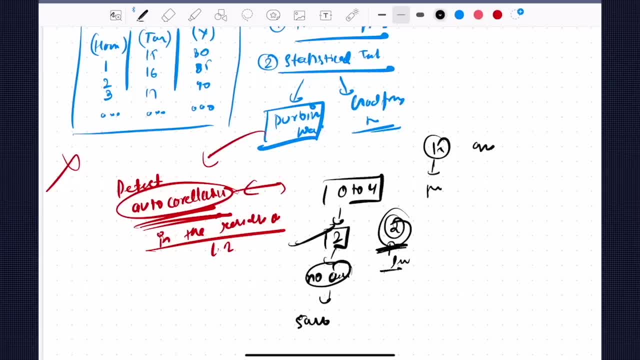 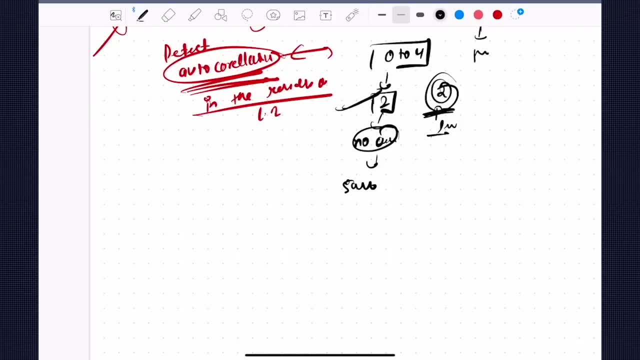 are negatively correlated across the observations. okay, um, yeah, so, uh, how can we perform some of the steps? so what do you do? you first of all fit your data and then you calculate the residuals. you calculate the residuals, you calculate the residuals. after calculating the residuals, what you do? you take out d and, in details, you're taking on the t value over. 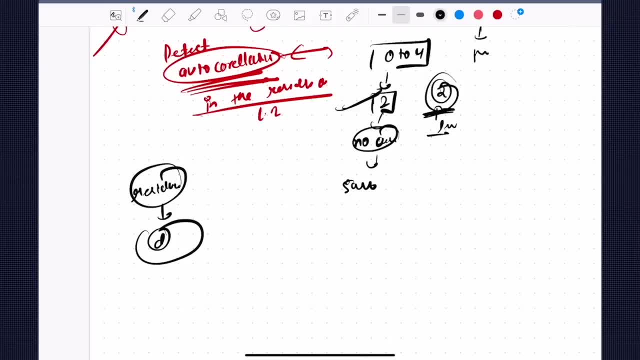 here. you don't take out the test statistic, which is d? um you. you can search online for the formula, but formula is not even required. you know, there are automatically tools which does for this. now, once you have this d now you, what you do? you compare the. 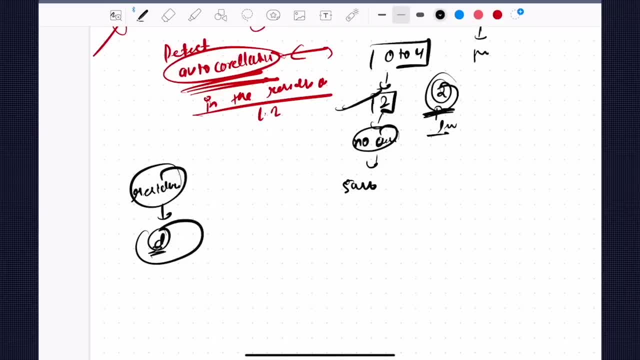 statistic to the script: critical values for the durbin. what's the, the, the table which we have? okay, the tables are statistical software. you compare it and if your d is less than that lower critical value or greater than that, then we reject the null hypothesis of no autocorrelation, which 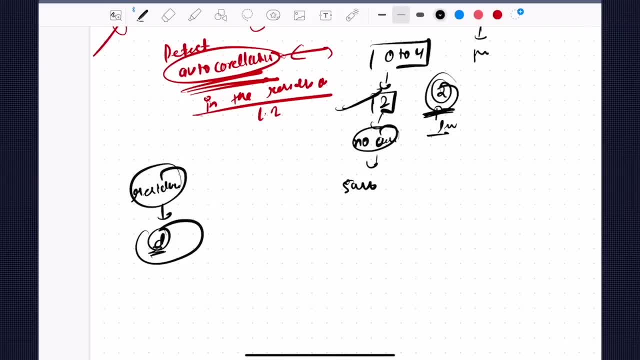 means assumptions is likely violated. for example, what does it say? what does it say? that you conduct the test and then if, and then we again our null hypothesis and alternate hypothesis comes into play, and if it's greater than that, and then we reject it. and so this rejection automation will. 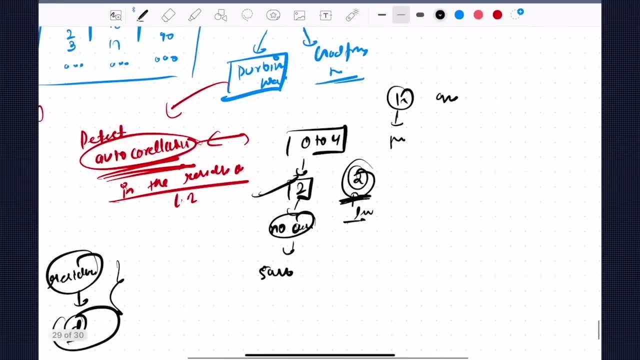 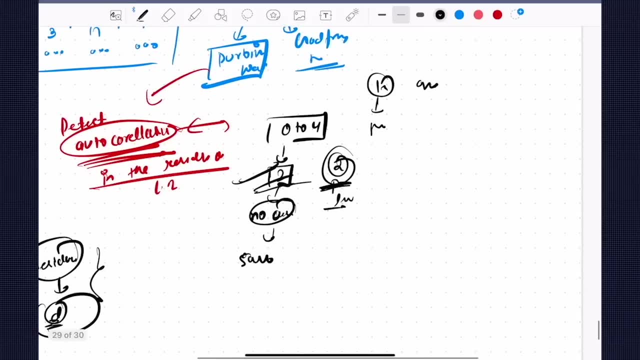 eventually happen. okay so, but but mostly what you do if your good d statistic gives two, that means there is no autocorrelation. but, however, you can perform test as well for detecting autocorrelation. but one of the more drawbacks of it- the durbin watson test is- is more for you know what it's. 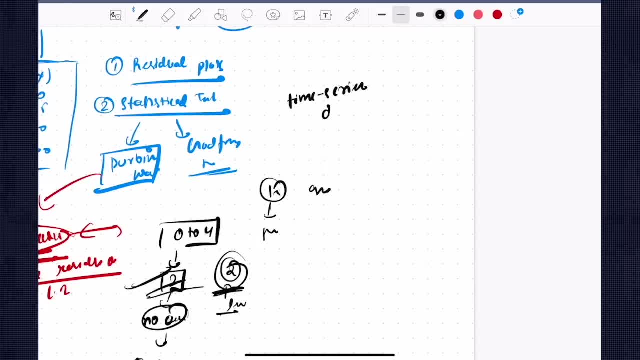 more for time series data is more for time series data. okay, so that's why, uh, we have to use a. we have to use proper, you know, tests for all of this thing. i hope that you understood about how can we test our independence assumption. there are several remedies for it. so there are several remedies. 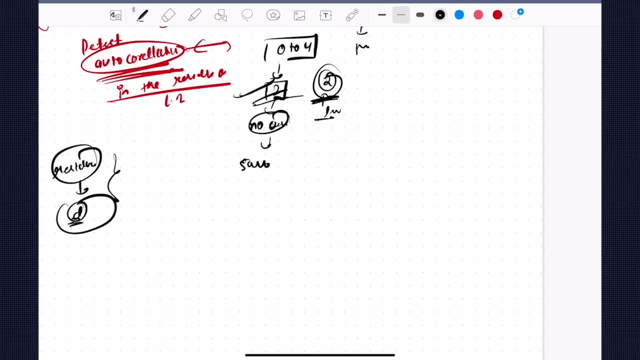 if the assumptions are violated, how can we fix it? so one of the way to fix it is add additional variables, so you can actually add additional variables you can actually add. the first one is: add additional vars, add variables. so, for example, if there's any underlying factor which 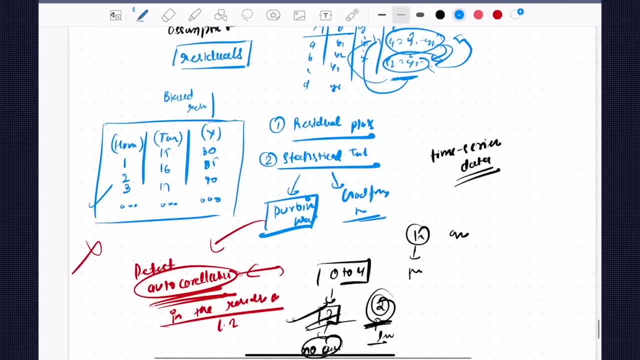 is causing, for, for example, in this case which you have taken, example, that your this, this, this, this has a this bullets independent by, because it might be related to previous one. so we can find a factor which is causing, we can try to find a factor which is causing that dependence, and then we can you. 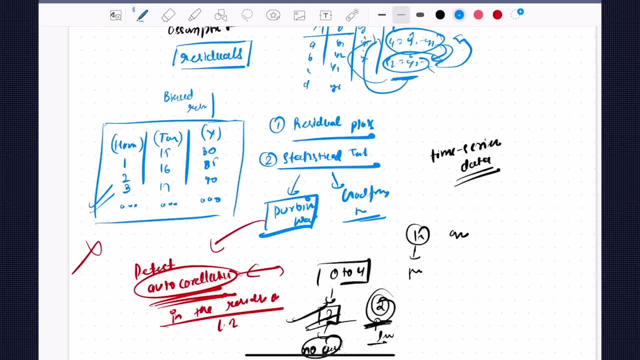 know, add this factor as an independent variable. okay to, uh, we can add this factor. so adding more variables definitely helps. definitely helps for it. for example, in this example, what we can do: we can introduce another variable. we can enter, introduce another variable. we can introduce another variable. what variable? time of the day? time of the day, in this case, the time of time. 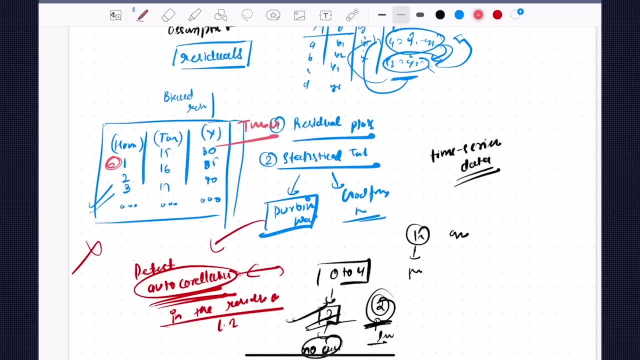 time of the day. so you introduce another variable, so time of the day, which is night, night, morning. so how does it help? how does it help? this helps how? how does it help if we, if we convert, we can actually take it, that we can actually understand the pattern your model could understand, the 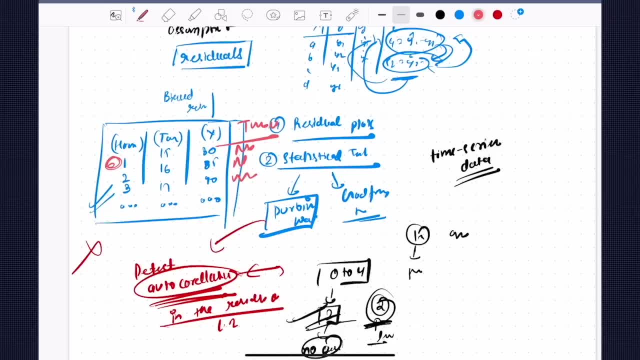 pattern. okay, this is something is um daily patterns. your model should be able to capture the daily patterns. that's that. that was the factor. so you can consider adding more variables according to what. what is causing those this factor? so, basically, at night time, so we can actually explicitly add this to actually help so that your model does not be dependent. so this is. 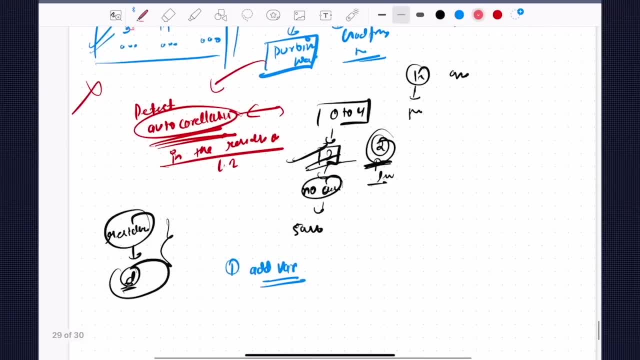 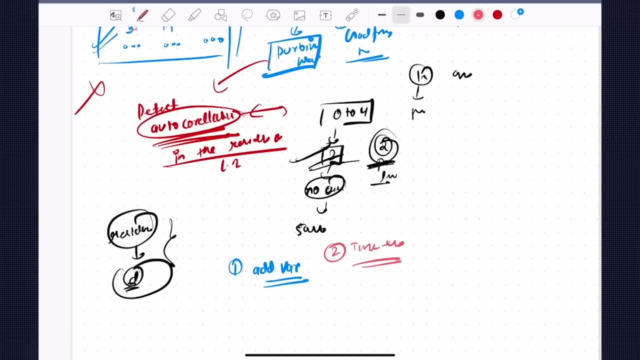 one of them. you can add more variables. uh, we'll do one proper example as well, don't. don't worry, you can use time series model, for time series model relatively works well in these type of examples, and then at last you have nothing but called uh, mixed effect models. but that's. 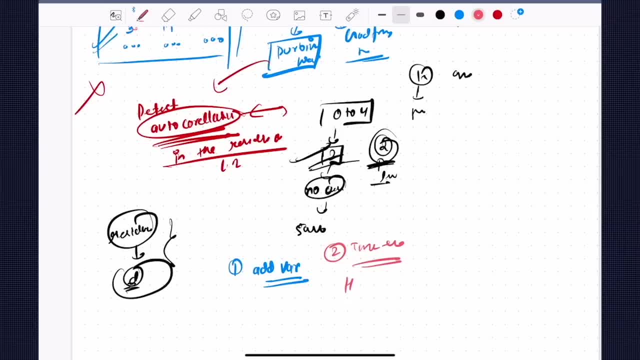 something it's like. that's something you can use hierarchically- hierarchical linear models- but i suggest you to explore. by that alone it's not too much use, but exactly that's what people actually use sometimes if if you have hierarchical data. but i suggest you to learn about hierarchical linear models- hlm- a very nice uh concept around it. okay, so adding. 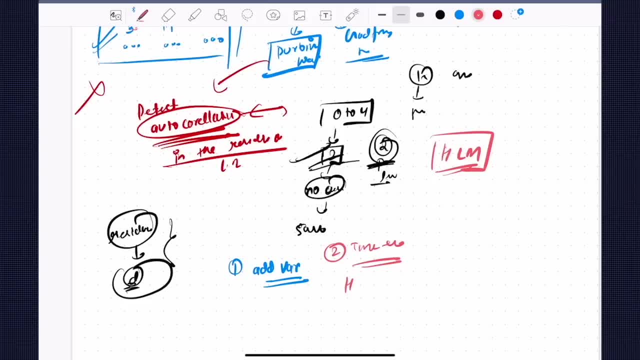 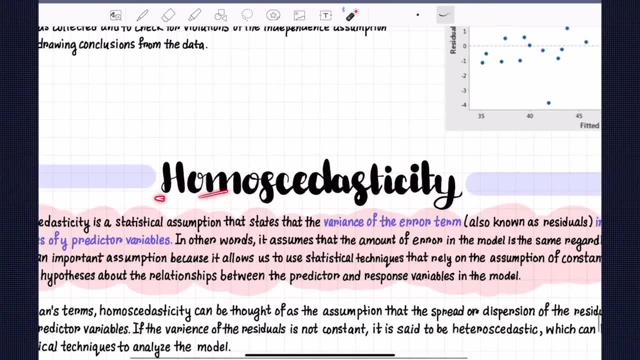 more variables. you know time series using another algorithm. all of this really helps cool. so i hope that you understood about independence assumption. now we'll talk about uh, homo scat district assumption, uh, which is also known as non uh constant constant variance or constant variance across it. so we'll talk about 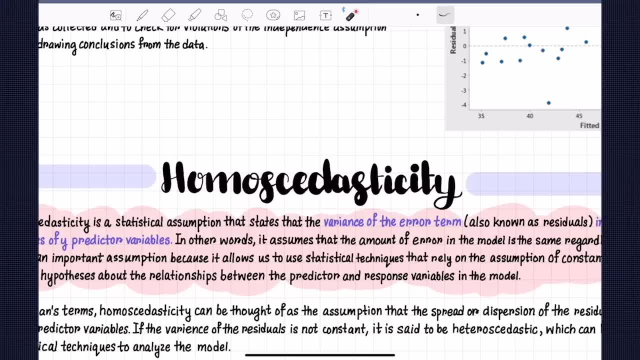 that uh, where your variance of all the residuals are constant across all the levels. so we'll talk about that homo, this no, constant, very uh, constant, various assumption uh, and then we'll take one example, and after that we'll have our simple last one, which is normality, and then we have no, no. 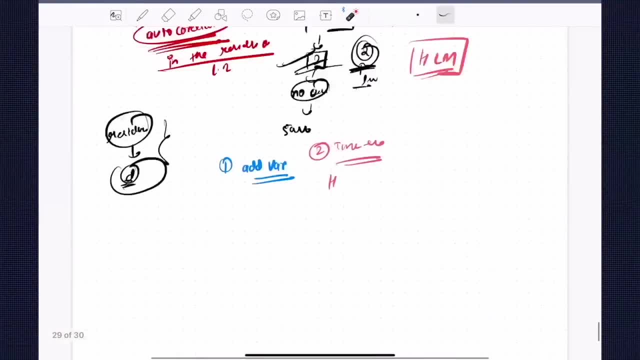 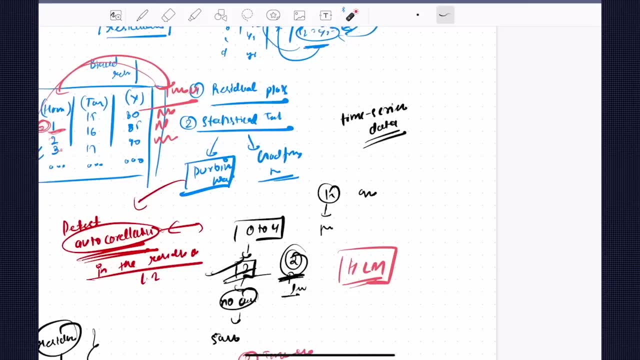 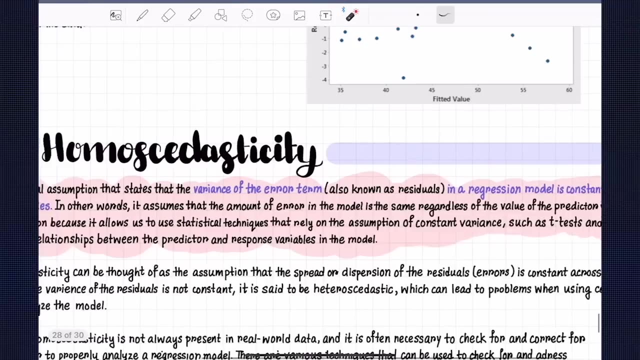 multicollinearity, which is left upon you to for you to explore. so let's get started with: um, what? homo city assumption, or even say no, constant variance assumption? no, okay, cool. so what does this homo scattered city assumption states that i? i really have a hard time, uh, understanding, you know. 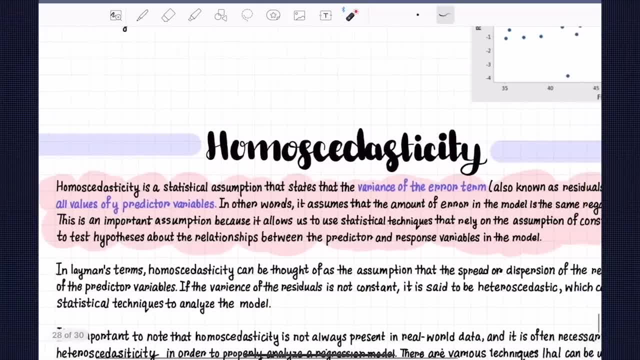 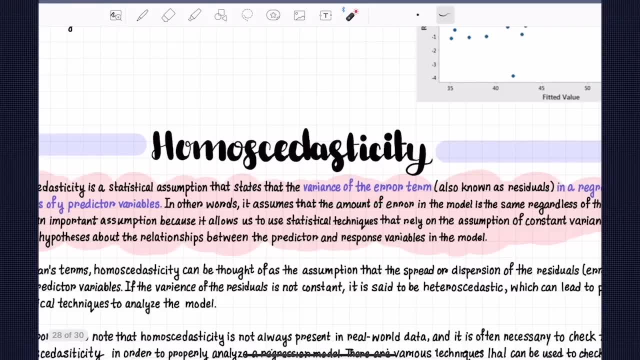 pronouncing this, so please you know if i sometimes pronounce it wrong. so most characteristic assumption is a statistical assumption that states that the variance of the error term also is a spread or very. what does it mean? the spread of the values? variance means spread of the values. okay, how, how? 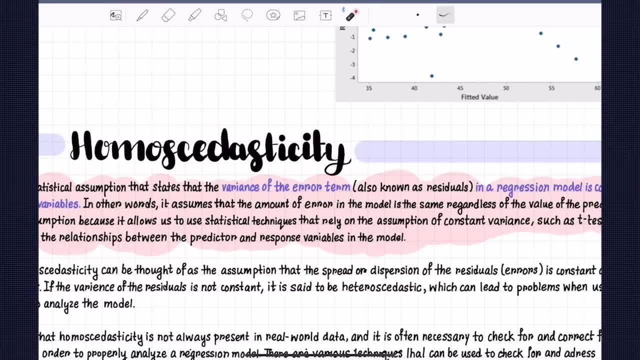 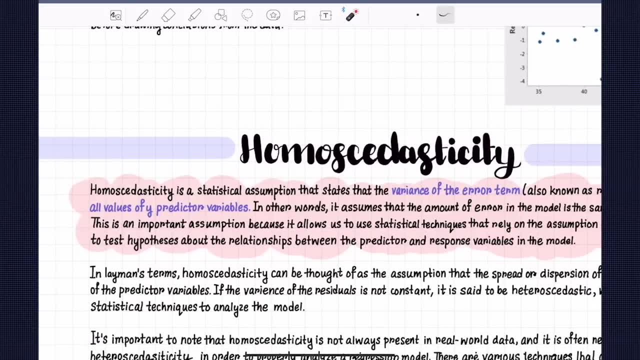 does it spread across the mean. so the mean of it, how does the way variance is a in a regression model is constant. the residuals or the variance are constant. okay, they're constant across all the all the predictor y variables. you may be thinking: yayush, what the 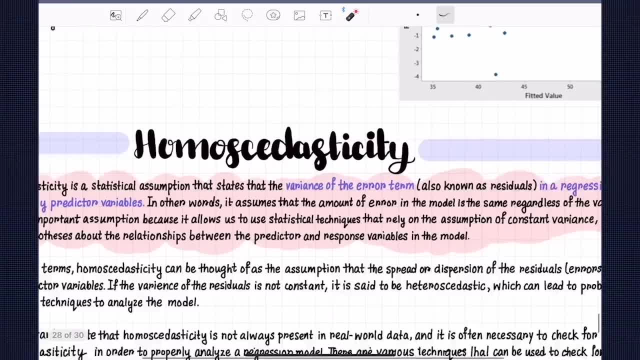 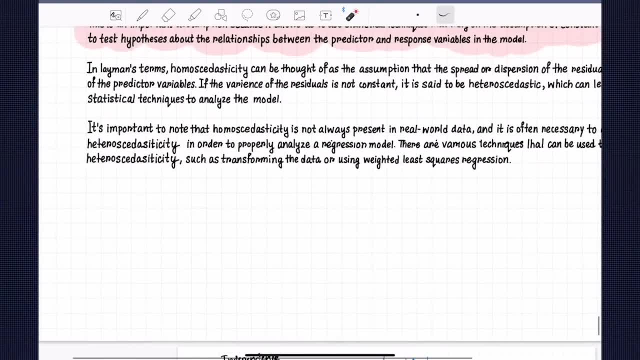 okay, so what? what? what just you told? okay, so, uh, you have, uh, you, you, you might be confused how, what exactly does it mean? so let's talk about what exactly does it mean. so you can assume that it is. uh, it states that your variance- i assume that you know variance- the spread of values. 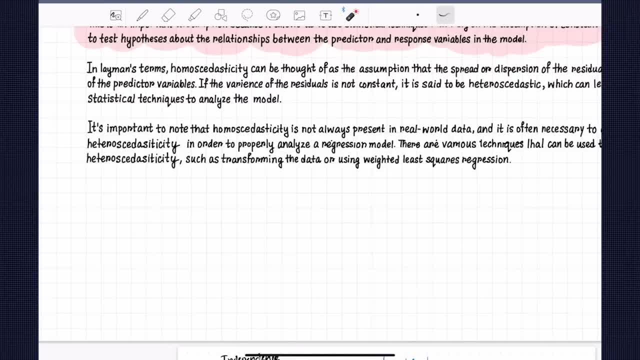 of the residuals is constant across all levels, they do not change. or you can say: the spread of the residuals should be approximately same for all values of the independent. so you have x, row number one. you have row number two, row number three, row number four, row number five, so your 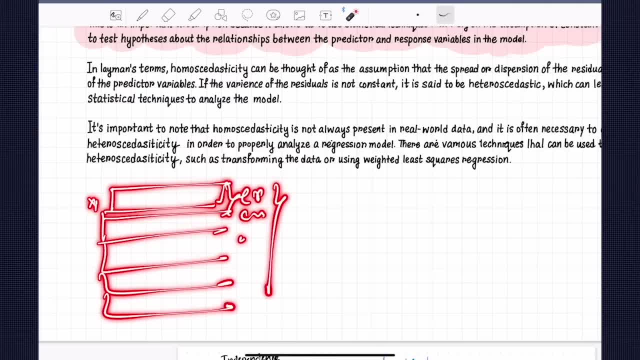 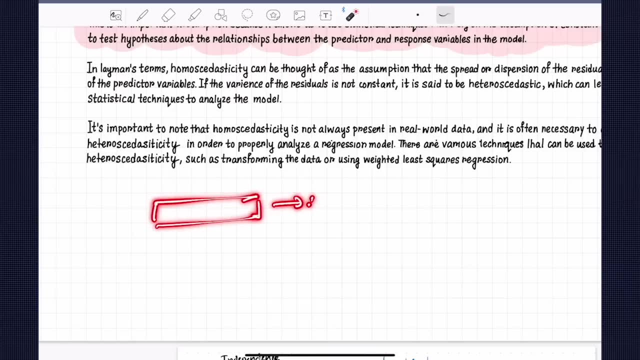 so your error on number row number error on. so they should be constant across all independent values. okay, they should be constant. if they are not, if the variance of the residuals increases or decreases dramatically, for example, at at row row number one error is something c and over row. 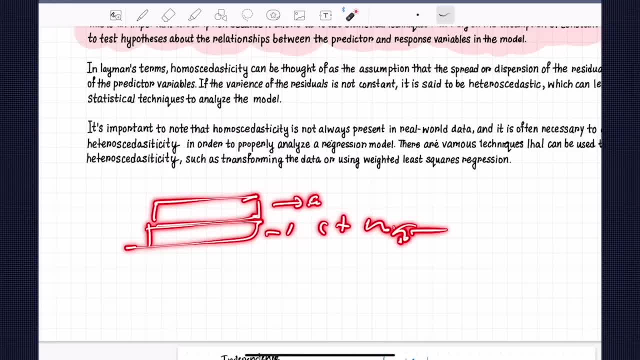 number two error is c plus 100. that. that means that is, that increases. and at row number three, c minus 100. that means it decreases, you know. so it increase or decrease dramatically, which means that it is not following that assumption. that is not constant. the variance is not of constant. 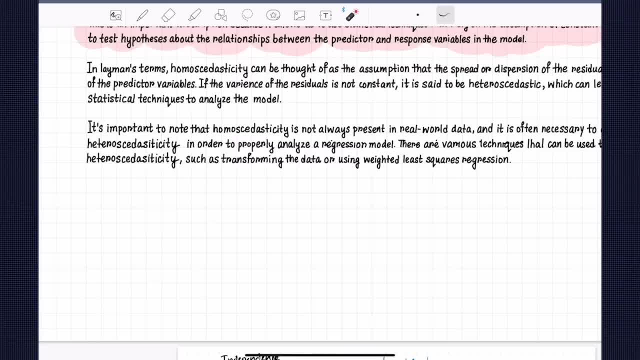 across the individuals of your samples. then we say that it is not following our assumption. that well, it's the assumption, okay. so uh, i hope that really helps about that. again over here for testing it. we have nothing but called residual plots. we have nothing but called residual plots. 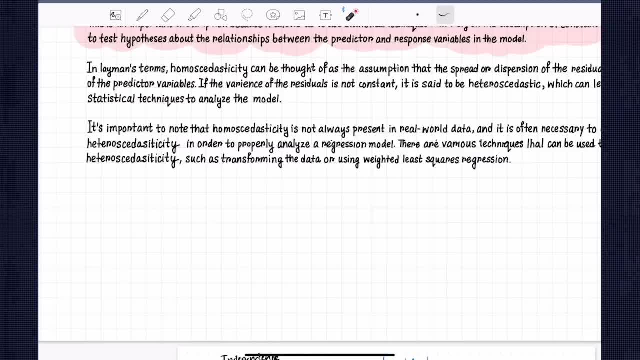 which really helps to test the homoscedasticity assumption. so what is uh? so let me, let me just again: if there's no, any patterns, then you can conclude that there's no such assumption. so just going to uh make you aware about, like a very nice example maybe for you, which will be super helpful. 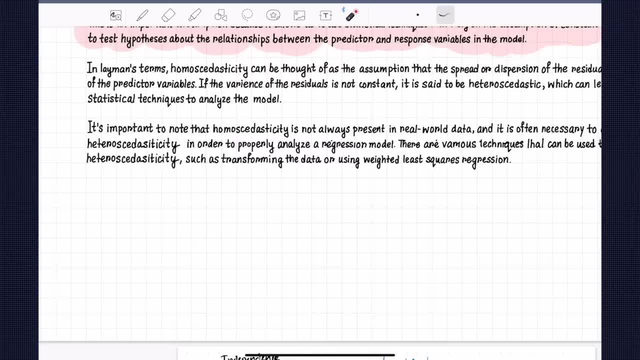 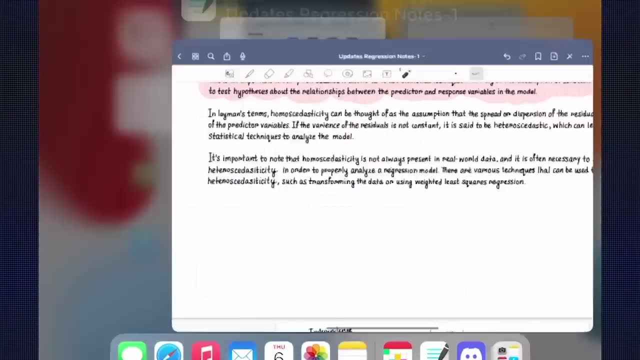 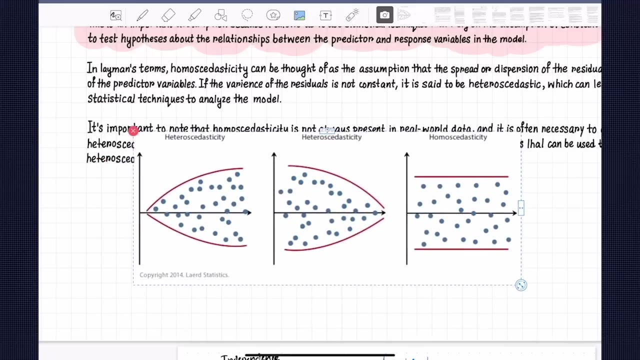 if you understand it the nice way. you so just going to have it over here, the png file, uh, uploaded right here, share done and then i'm going to share again airdrop and ipad, oops, yeah, so this is. this is one of the nice image which i usually use to explain it. so this is. this is called the residual plots we have. 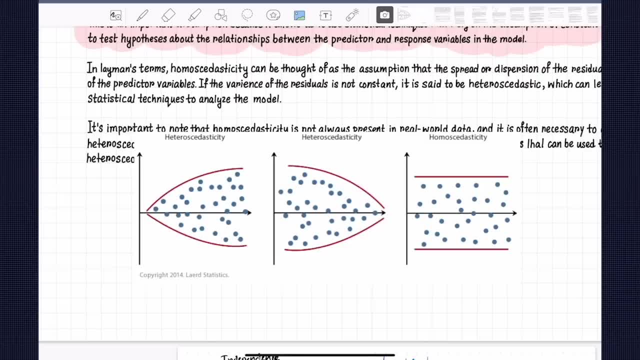 the residual plots, which plot and y-axis residuals. on x-axis we have some sort of uh fitted values. you have fit if we have uh fitted values or the predicted values or the model predicted values on. on y-axis you have the uh on y-axis. we have what? on y-axis you have nothing but uh residuals on. 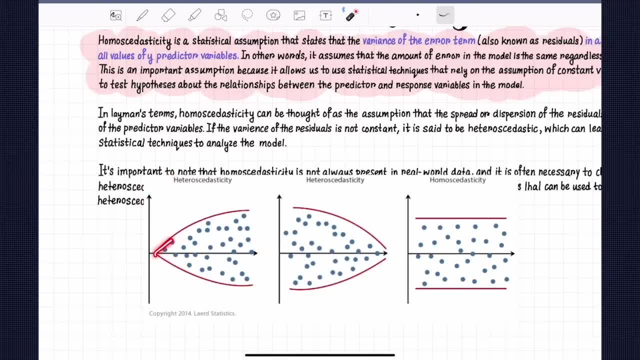 x-axis, we have fitted values and when you plot it, if it shows some sort of patterns over here, you see that it is showing some sort of patterns. over here it is showing some sort of patterns, but over here it is not showing any sort of patterns, right? so in this example, if, if your model shows: 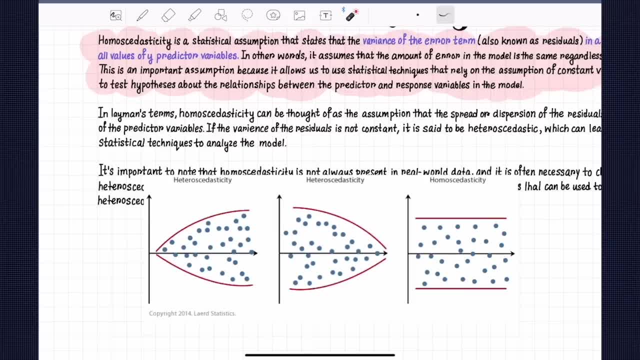 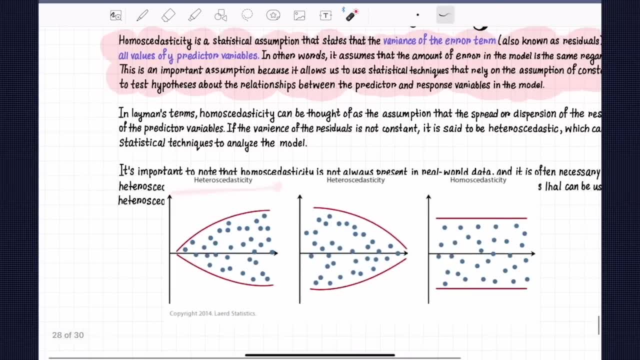 something like this: that means assumption is satisfied. you can go ahead with it, but if the this like, if there's some sort of showing patterns, that means that assumption does not hold. this is- this is example of a heterostasis, heteroscedicity, and this is also example of heteroscedicity, but 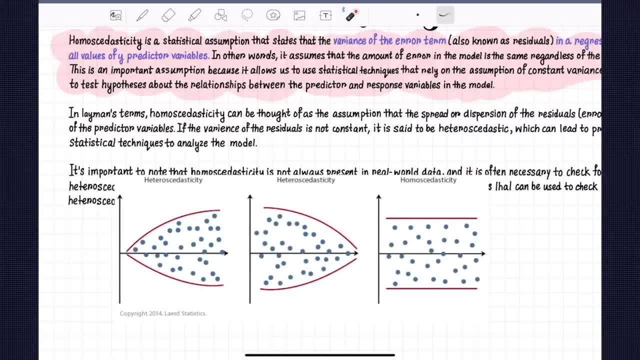 this is an example of homoscedicity, which means that it was homoscedicity assumption is true. it's constant. your variance, your errors are constant across the uh, your residuals are constant across the independent variables. okay, and there's no trends, or there's no trends over. 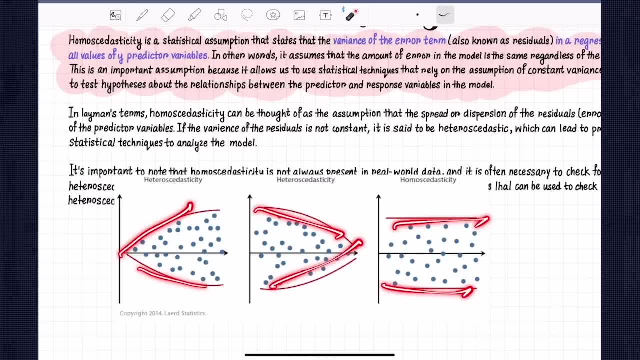 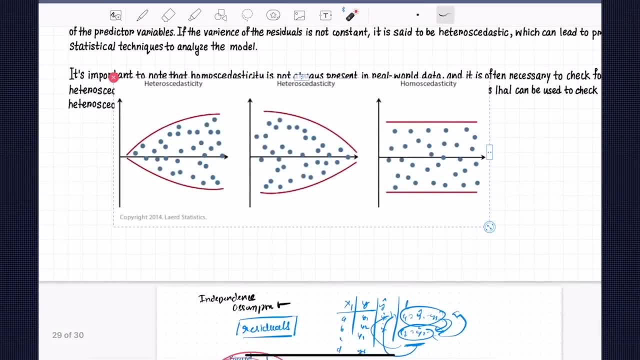 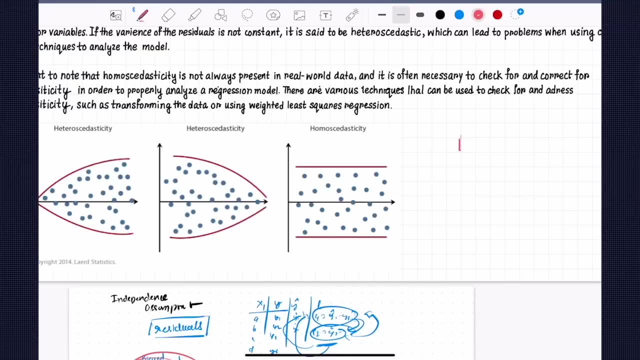 here it is increasing. over here it is decreasing. over here it is constant across all variables. okay, uh, this is what this is, a visual inspection. another one is nothing but called: uh, we have several, you know uh, statistical tests, just like as the previous one, which is called the pagan test. 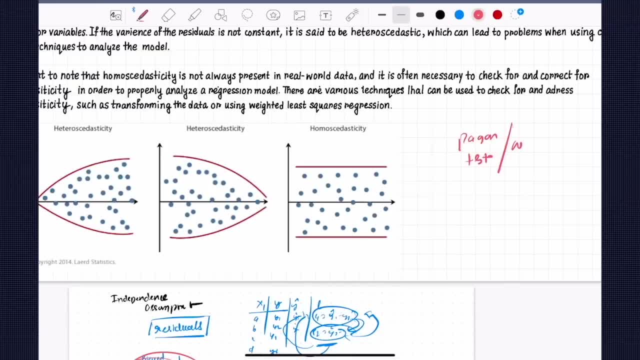 pagan test or white test, white test and all of this. you don't really need to, you know understand what exactly, uh, it does. but again the hypothesis testing formula looks and you have the end null hypothesis alternate and then you perform the test and then checking the significance value. 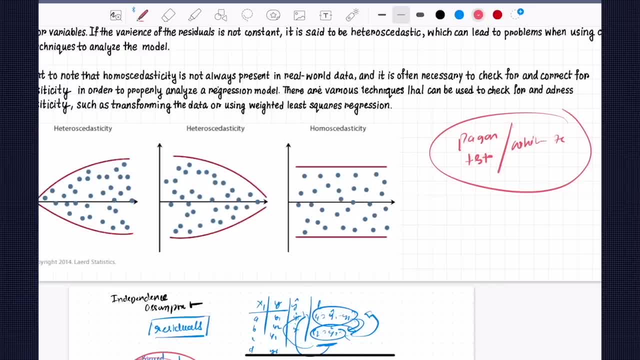 and then you perform the test and then checking the significance value, and then checking the significance value, and then you say, okay, there's something greater than then. we reject or accept statistical test. but all the statistical tests which you have to understand by your own by searching online, i'm not going to do with it because it is out of the scope of the course. 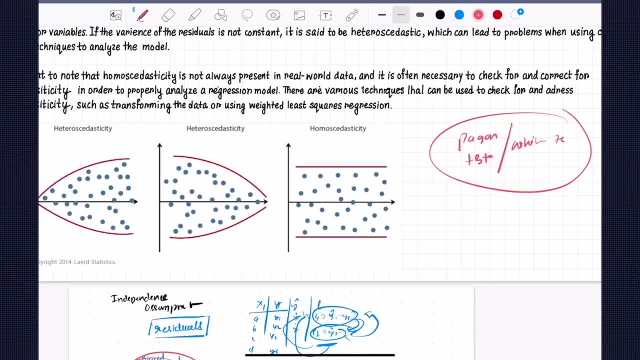 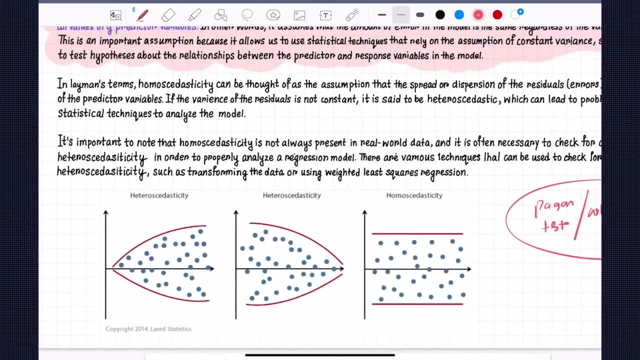 as well. it is not required as well for for for initial steps at least. so once you, once you assume that your, your model does not satisfy. so what are the remedies? how can we fix it? so, fix and can be happen in two or three ways. two or three ways, okay, so, uh, two or three ways. so let's talk about what. 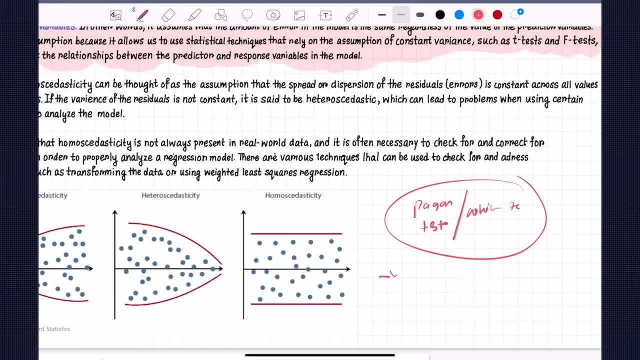 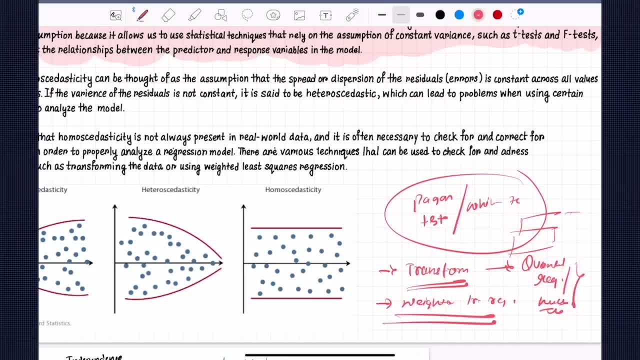 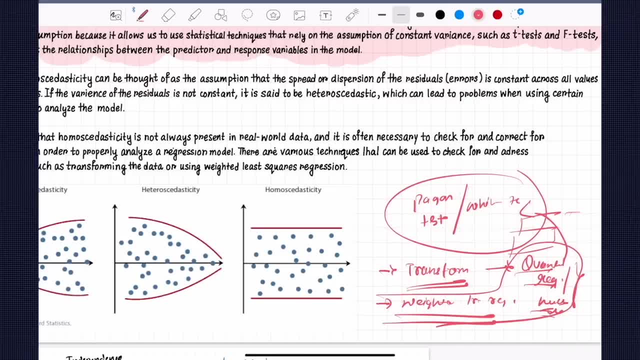 types of extensions of linear regression, which helps to satisfy this assumption. so i really want you to go ahead and then stop this lecture and then go over and search about this, learn about this, make a note and tag me on linkedin. okay, cool, so i hope that you're done with this homoscedasticity. 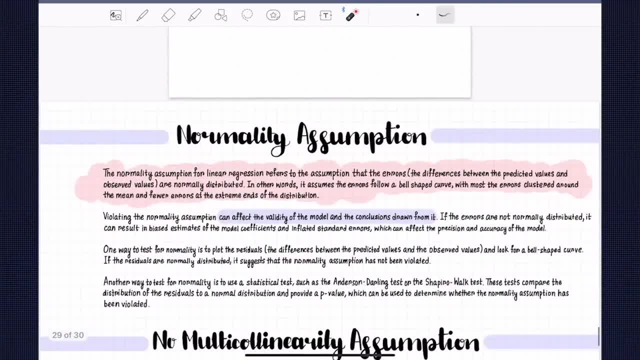 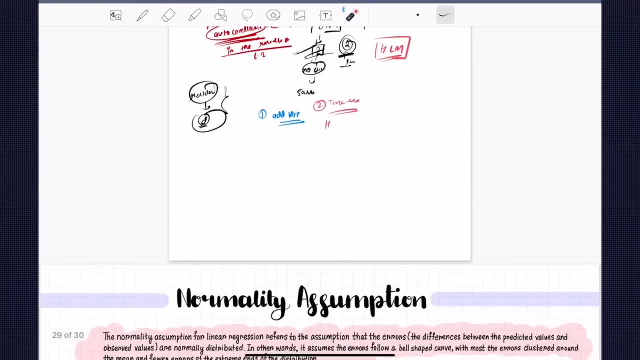 assumption. uh, now, at last, we'll talk about nothing but called normality assumption, which is our most you know as well as it's not. you know what most is something which is required for everyone, you know, cool, so let's get started with normality assumption. so what is it normality? 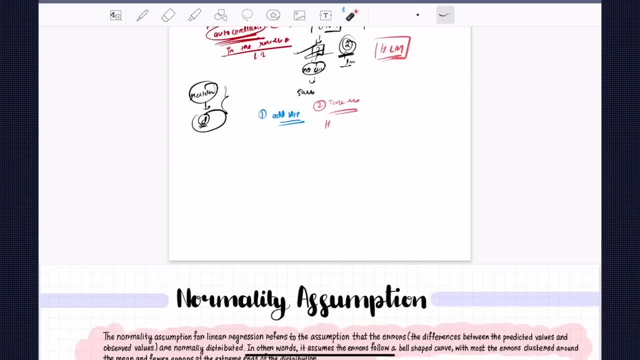 assumption states that normality assumption states that normality assumption states that that the residuals, now previously in independence, and the constant and homoscedasticity constant- you know independence, independent of each other, constant, and now we talk about they should be normally distributed. you know that. what is? 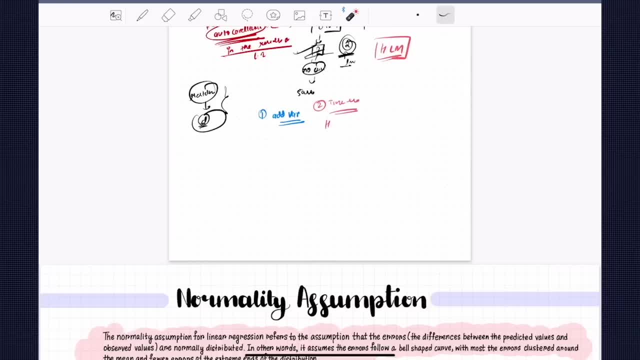 normally distributed. you know what is said to be. write me in the comment box. what is it said to be? a normally distributed, a? very nice, uh. so i'll just wait for five seconds. what does it means? so tell me. what does it means your residuals to be normally, to be normally distributed? 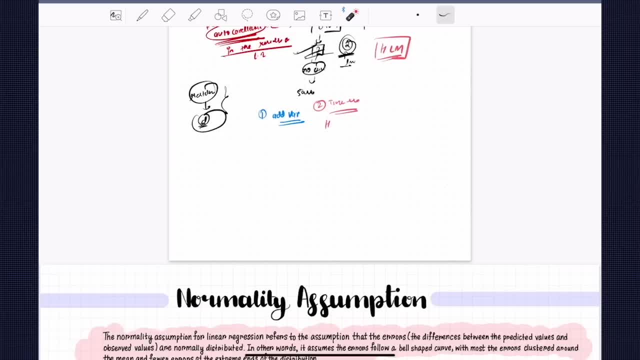 so let me, let me just write the question so that i can- at least i can check for it and you and in the comment box, uh, yeah, so please go ahead and write it, uh, so that i could understand. cool. so what does it say to be a normally distributed which means? which means that your 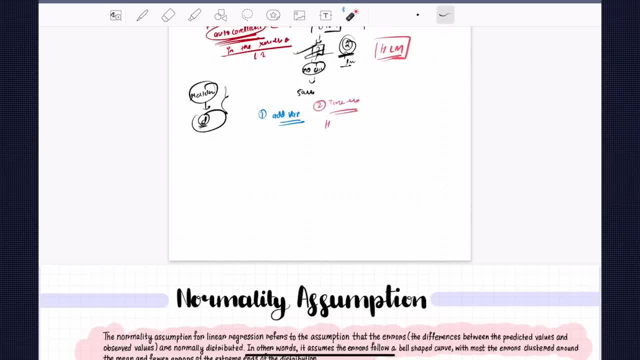 mean? is that that that your distribution is following a normal gaussian distribution? okay, your mean is following a normal gaussian distribution. okay, so let's go ahead and write it: normal gaussian distribution, that your residuals are following the normal. when you plot the residuals, they should follow something like this, where most of the values should lie between this: 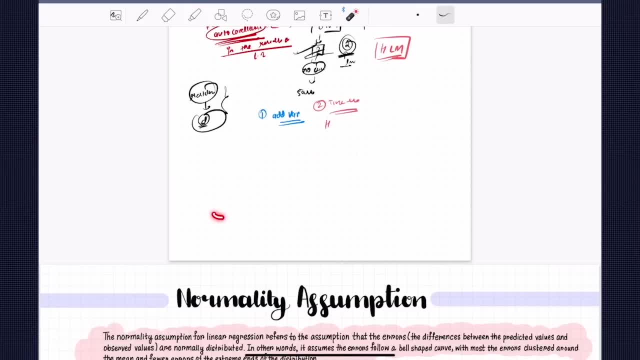 range. okay, should, should, right, should. uh, this should be symmetrical. they should be symmetrical. most of the value should be around the mean. your mean is something that nothing but mean is equals to zero. and then you have the bell-shaped curve, which is symmetric, which is, which should be, which? 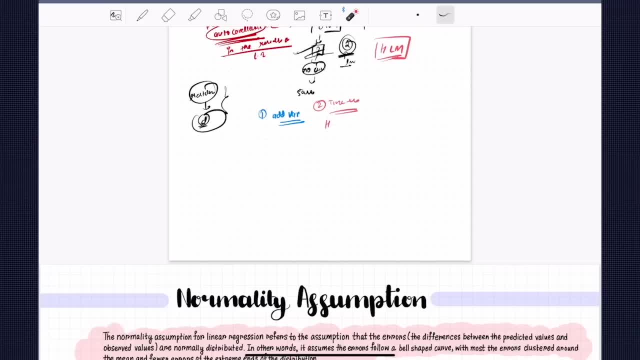 should, uh, where the mean should be close to zero in the case of residuals. in the case of residuals, mean should be close to zero in the case because residuals are, of course, zero, right, because we don't want our residuals to be high, so it should satisfy our normality assumption. it. 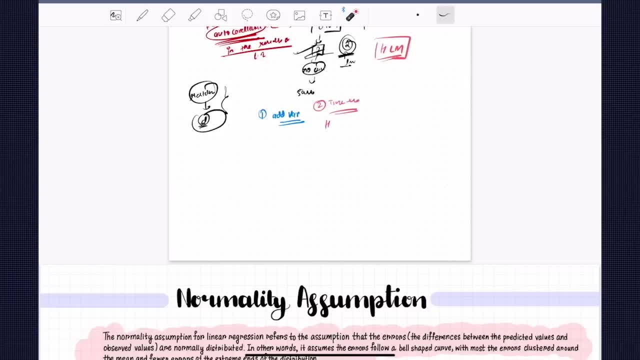 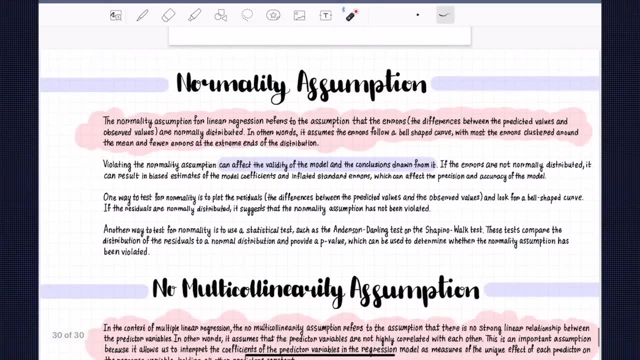 should satisfy our normality assumption? i hope that. so, basically, uh, normality assumption states that. and what does normality assumption states that? that your normality assumption refers to assumptions that the errors are normally distributed, in other words, that your, uh, it should be well shaped, bell shaped curve, with a symmetrical positions, with most of 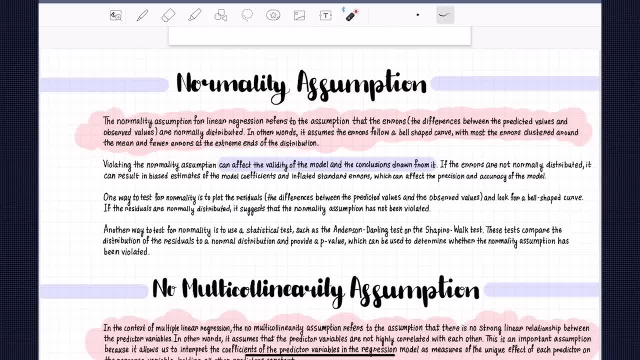 the errors clustered around the mean and fewer errors, so most of the errors. so when you, when you plot it, so most of the errors should be over here, so it should be constant. so you see that it is related to the previous one, this constant, so your most of the errors should be constant. it should be independent and they should 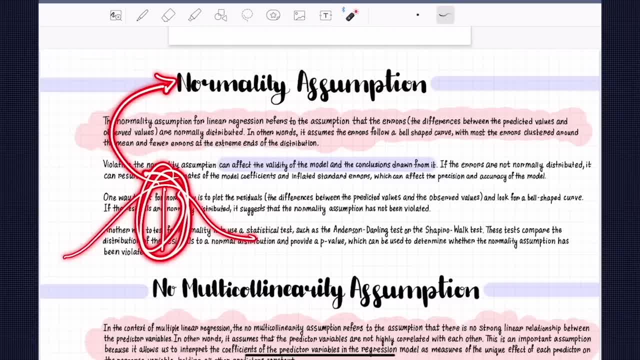 be around. they should be similar. it should not be this. it should be very one, one of one or two errors should be at extreme, like very different, but it should be most. most of them should should be: uh, between, like it should be around the mean: okay, uh, over here you can see that if you violate, 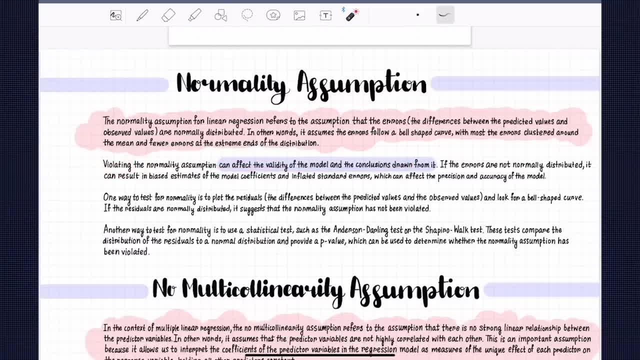 this. it can affect the validity and the conclusions your model is going to make, and it can also often result in biased and inflated standard deviation- errors again, which can directly affect the accuracy. so there are several ways to test the, and the easiest way is to plot. a distilled plot is a. 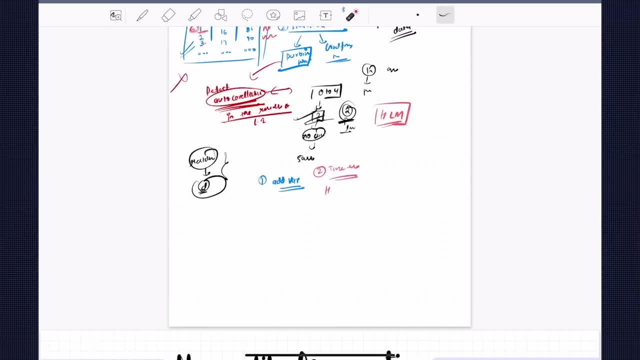 normal plot and not which is nothing but a histogram or something like you know, histogram with a bell-shaped curve, uh, which you which, which you usually do. so let me just introduce you with a very nice image for this as well, maybe for you, which will help you. we have two, two types of plots which we can use. the first one is: 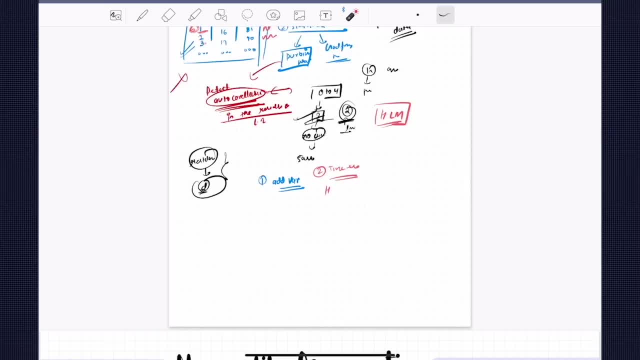 quantile plots. the second one is a histogram plot. so assume that i just want to take a very nice example. which example i should take? i don't even get it, um, so i just gonna use this. so assume that. assume that you have this particular example where you plot the residuals on a y-axis. 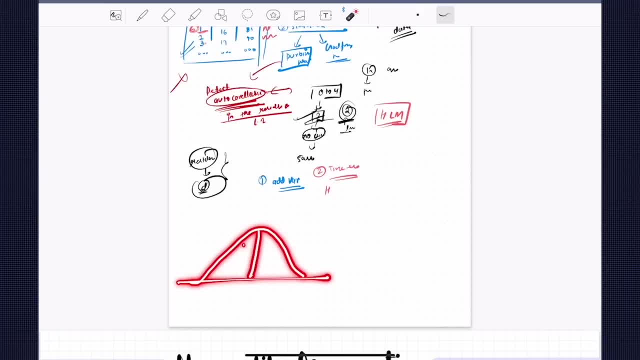 where you plot the residuals on a y-axis, where you plot the residuals on a y-axis and then see: okay, your, eventually, your, your, your bell shape should form like this, it should. it should form like a gaussian distribution. that's one of them. when you plot the dev versucht way, where you plot the histogram, where you plot the histogram. 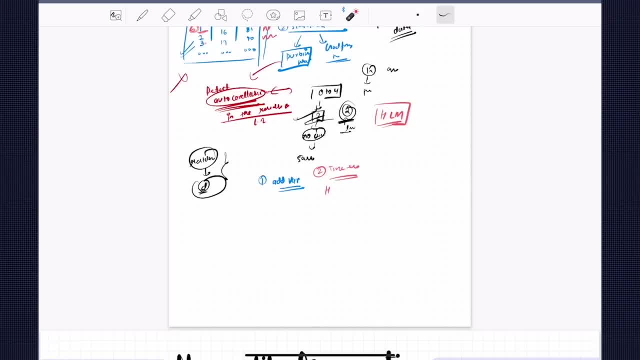 and then what you do when you plot the histogram with the bell shape curve and then, and then you apply the distilled plot on top of it so that it looks like a density plot. you know the density plot and should look like a, a gaussian distribution, or you can. what you can do. 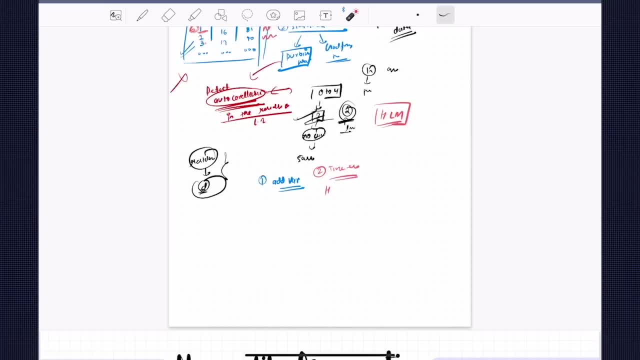 you can create a quantile-quantile plots. quantile quantile plot means it means that what does quantile quantile means that it means that if the residuals are normally distributed, should fall approximately along a straight line. now, this may be a bit off, you know, a bit off to you, so let's just go ahead and talk about it. so what? 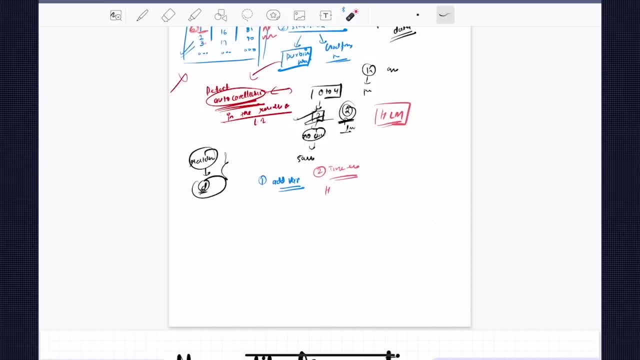 i'm going to do is have it like over here quantile plots. i'm just going to send it out to you over here. you usually you know what i do, i usually teach along with it. i i just don't, like you know, to teach it like, uh, like, like, like just having a preparation, because i feel like having a 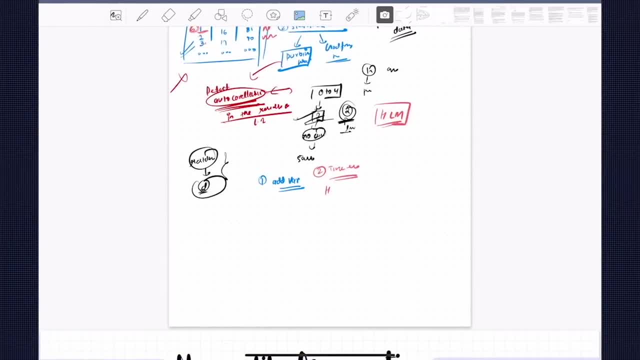 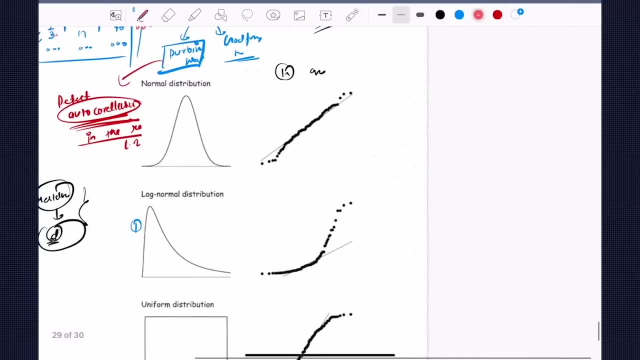 preparation really affects. you know the way we teach. so of course i have a preparation, but not too much, because i like to be very natural. so over here you can see that you have a qq plot and qq plot. if so, what is qq plot and indicates the qq? 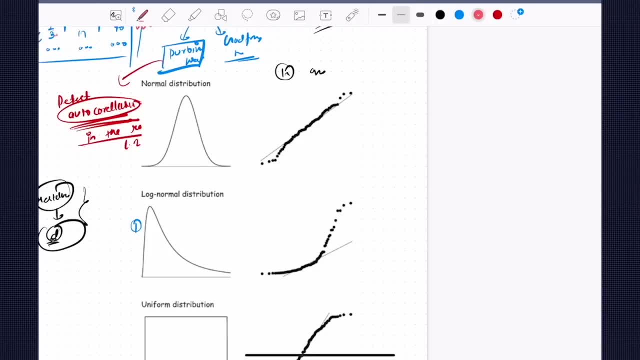 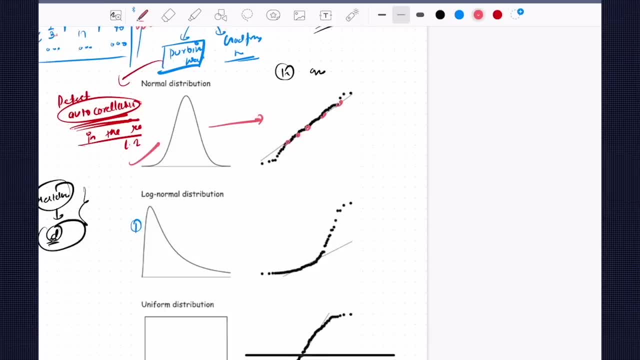 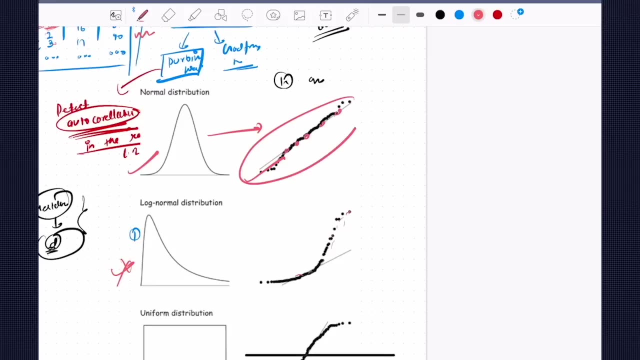 approximately over here. this normal distribution there lies approximately on the straight line. but over here this is not a normal distribution, log normal distribution. so your points are, the points are divorced. the points are not on the straight line. over here this is also not on a straight line, but over here this is on a straight line. so if, if you get the quantile plot like this: 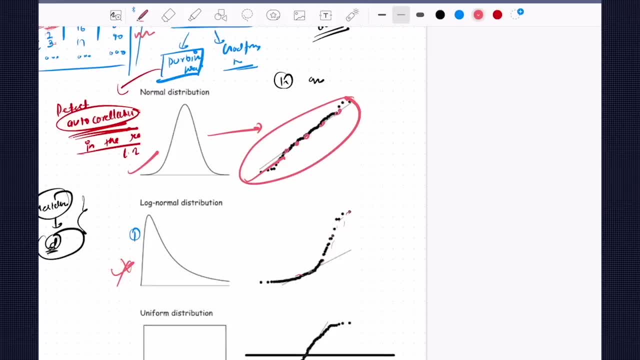 then you say, okay, this satisfies our assumption. and then you have several other statistical tests, just like um, a previous one, like which is over here, we have sapiro will test, or you can say smirnov test, where it is used. but we'll what, we'll perform the test, one of the tests in practical. but you, there's that, that something. 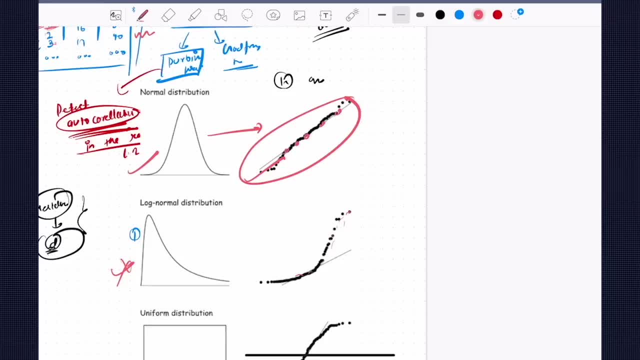 is according to you, if you want to do it, but i like to do it by normality assumption, which is just by visual inspection. what are the? what are the remedies for it? transformation is one of the most popular remedies: removing the variables, which is which is called the transformation. 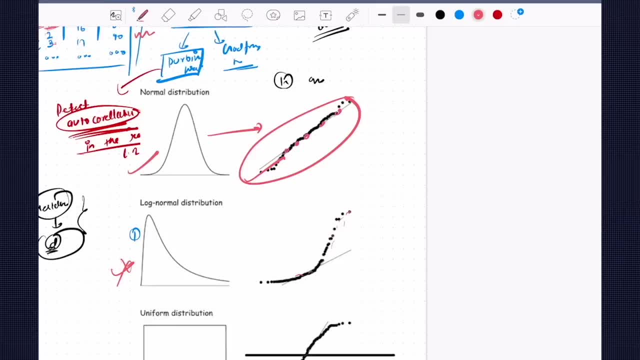 which is causing to be it in non-normal, so you can remove the variables which is causing to be non-normal, or you can talk about, or you can use different other algorithms, such as quantile regression, as i told that you should be comfortable with that. um, and actually in the course you know, 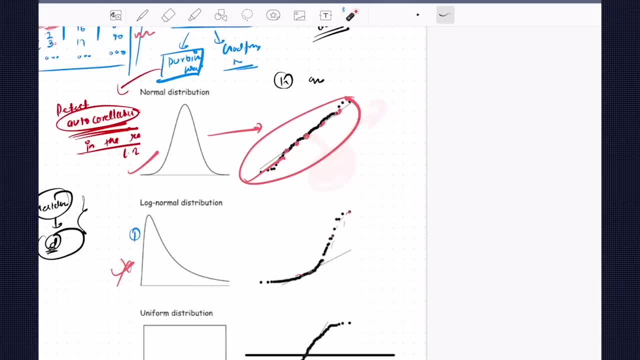 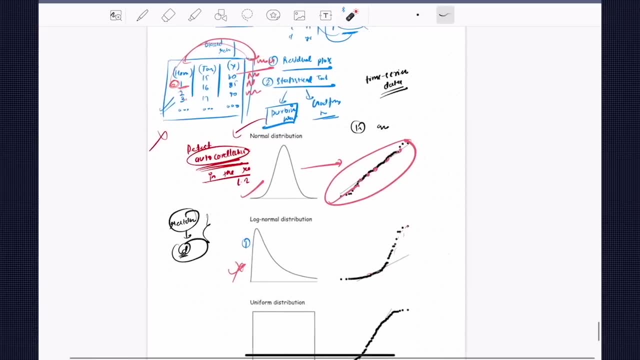 the course which which which we have cs01, we teach about all of these extension as well, but as of now, i feel like, as we made it for fee, we just wanted to explore by your own as well. okay, so this, this is about normality assumption, where we, where we are, ask our residuals to follow a normal distributed 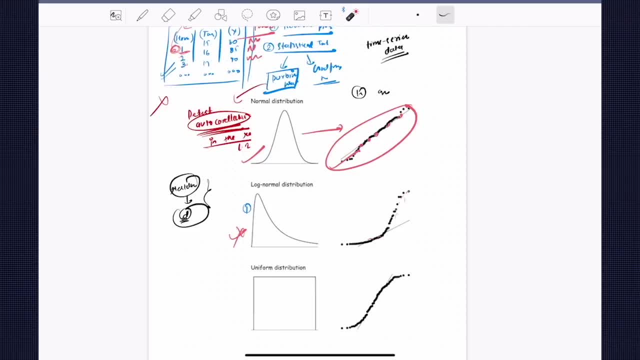 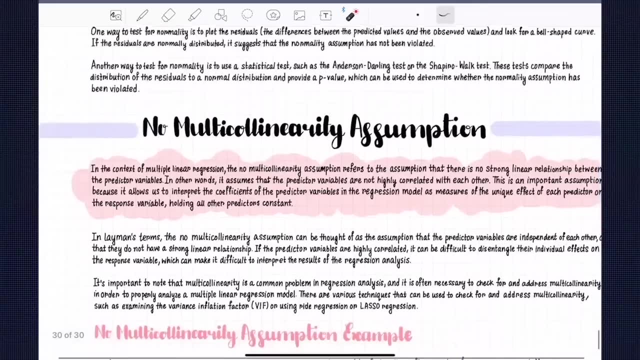 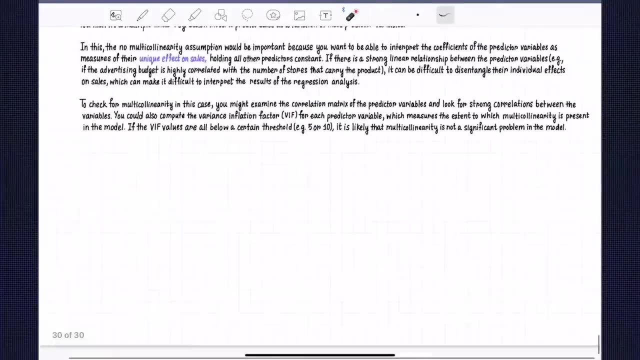 plot. okay, cool, so i hope that really makes sense. uh, now what i'll do? i'll just wrap up. so now we are. we are done with almost all the assumptions. now what is left is something known as no multi-coloniality assumption, which is for you, as a homework, to uh understand. it's very easy and very, very tricky, as 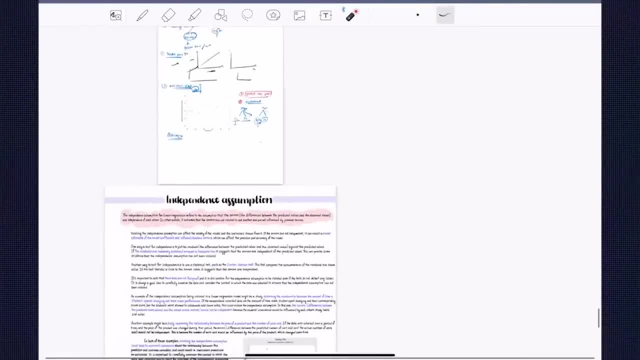 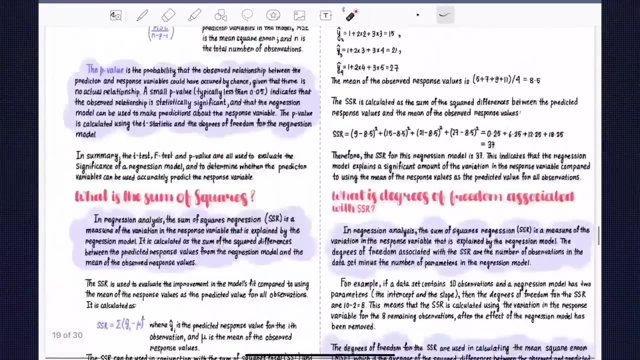 well if you don't understand the right way. so, but that's, that's something which you have to deal with, deal by yourself. we have already talked about 10 hours of lecture. that's something which you have to do by your own as well. right, and we have a talk in very things, in great detail, and i really hope. 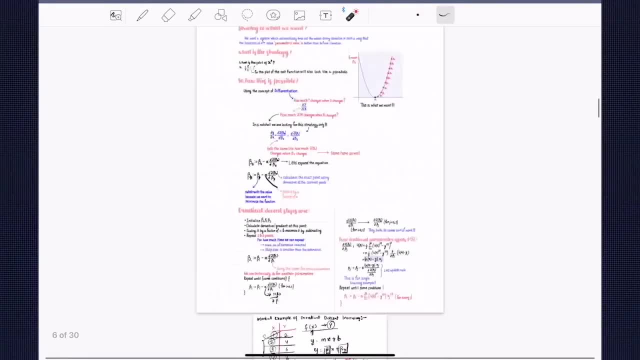 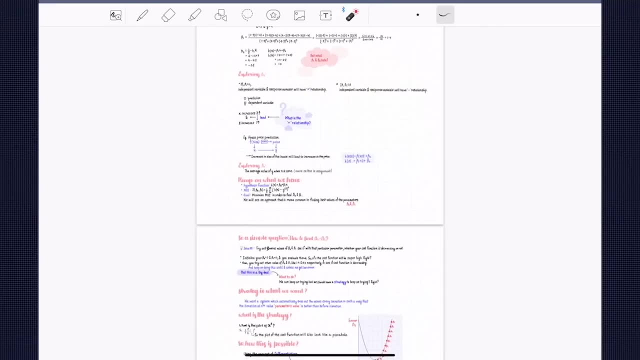 that you understand all of these things. you have a lot of time, you have a lot of time, you have a lot of time. we have come to an end, actually. so we are done with the assumptions and everything. now, what's next? the next is nothing, but we'll go and do a sample process, one simple linear regression. 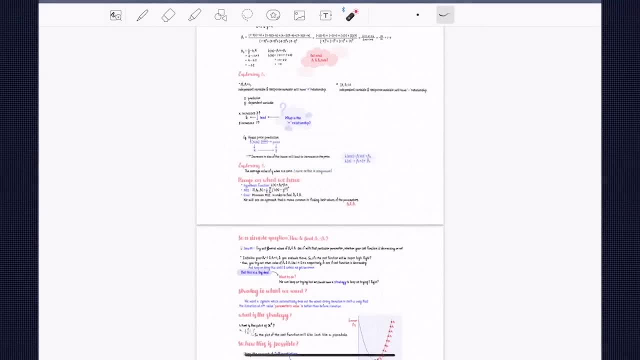 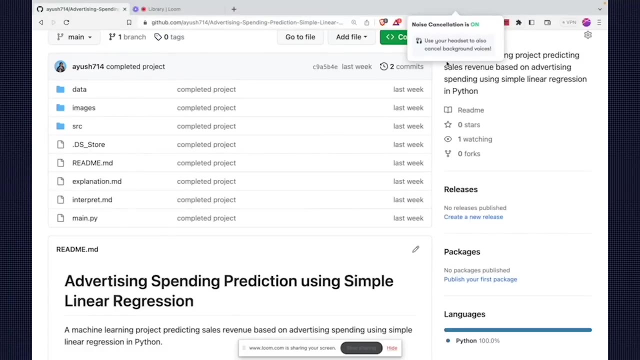 and one multiple linear regression to showcase you several other things as well. so you don't need to worry about lot of things. let's get started with the final section of the course and then we'll say goodbye the lesson. hey, everyone, welcome to the mostly the last section i've been telling in the practical. 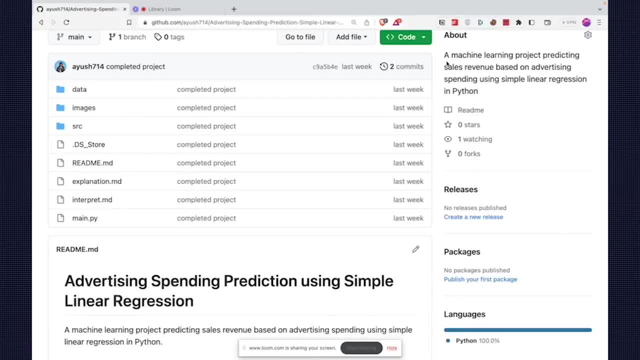 session, so we'll so. uh, so we'll now now start off with the practicality stuff. get you comfortable with what we have learned and how to implement that as well. okay, so we will definitely do that, but but prior to this, you have a programming assignment for you, so that you could, you could. 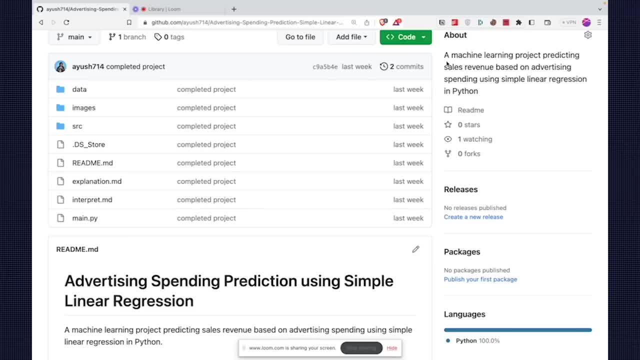 implement linear regression from very scratch by your own. i'm not going to do that. what i'm going to do, i'm going to utilize libraries, teach you the core and concepts and crux which nobody else teaches. that's my aim. so, uh, we'll, we'll, we'll be doing a short, a couple of linear regression. 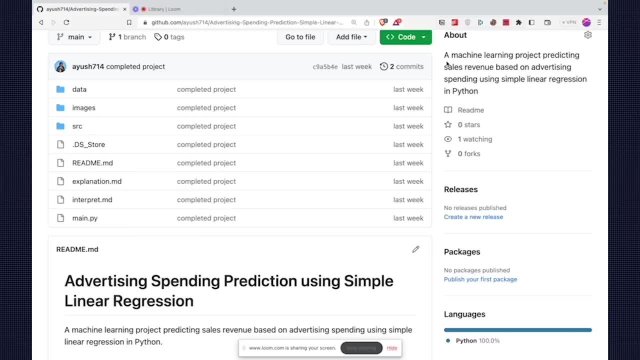 project. one of the one of them is using simple linear regression to give you a basic idea about how we go about building a very nice report, how do, how we go about interpreting the results of linear regression and etc. and, as my as as my strategy suggests, we'll start with the baseline. 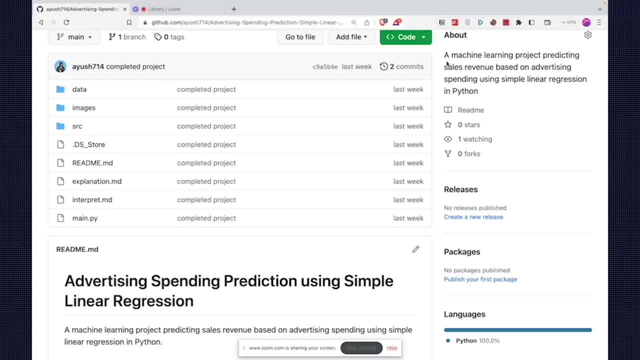 and then we will slowly extend to the, to the multiple uh variables as well, right, so, so what? so what we can do? we can actually uh do that in terms of uh having more sort of, you know, adding more sort of uh projects in future if you want to go with the free one. but as of now, let's, let's get started with 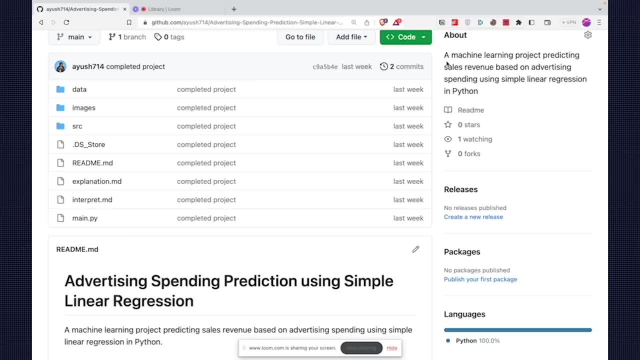 the very simple example on how we can use linear regression for identifying predict advertising production. but before that, i'm pretty much sure that you might be confused about what exactly the project is and how we're going to go forward with it. so basically, let me show you what exactly the project. i'm going to start over the problem statement and then after 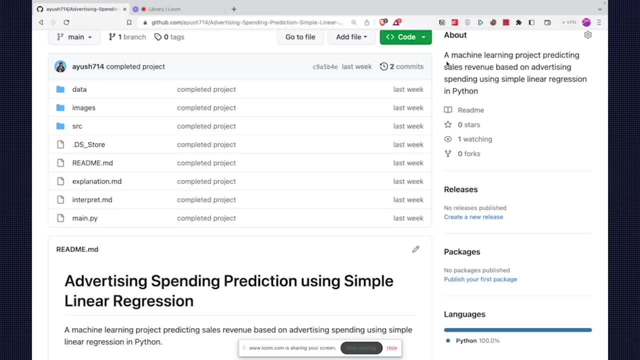 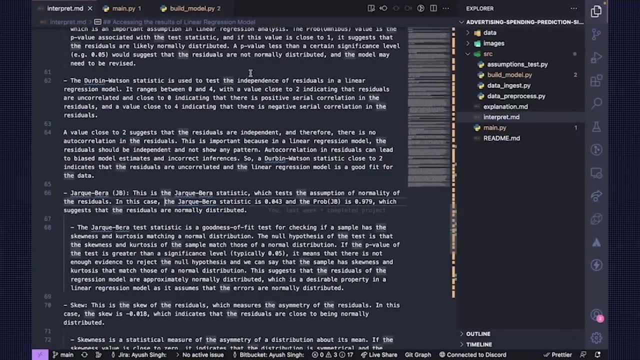 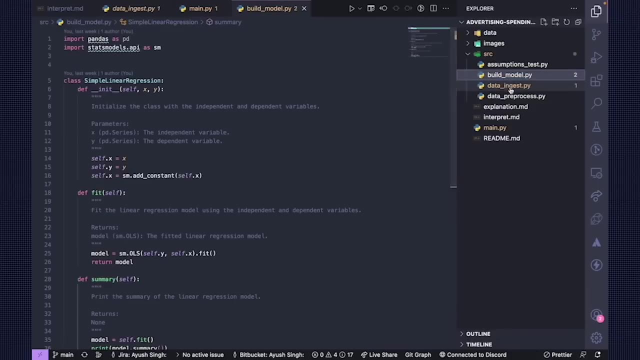 the problem statement. i'm going to make you familiar with something known as uh, with some, with something known as uh, like what? uh? simple and linear regression. and then we'll do a couple of stuff like 40- 40, for example, data ingestion, and then we'll talk about how we will deal with the 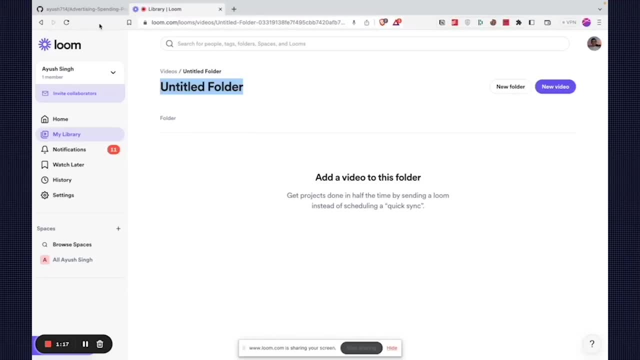 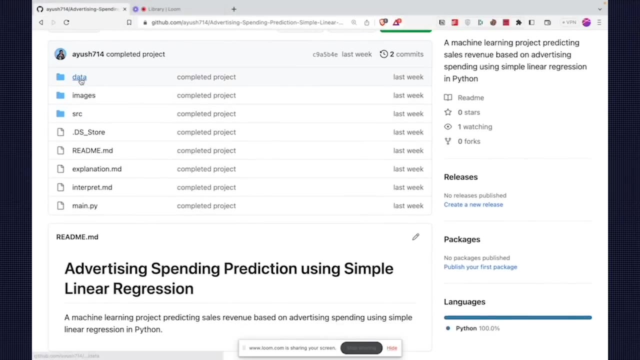 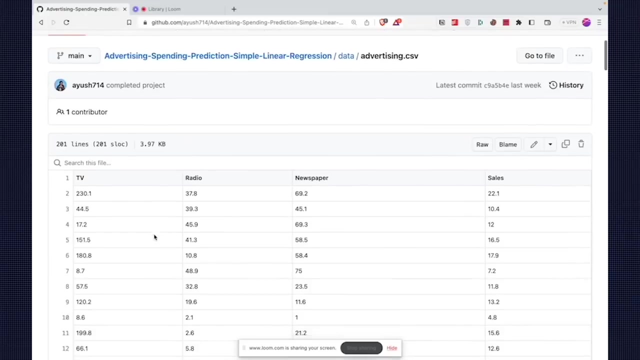 model, how do you test the assumptions, and etc. so i hope that that really makes sense. uh, apart from it, and and, on the other other hand, uh, let's get started, uh, eventually talking about, first of all, what exactly the data is. so, first of all, we have the advertising date data set, as we have already seen a lot, uh, and you and you're also 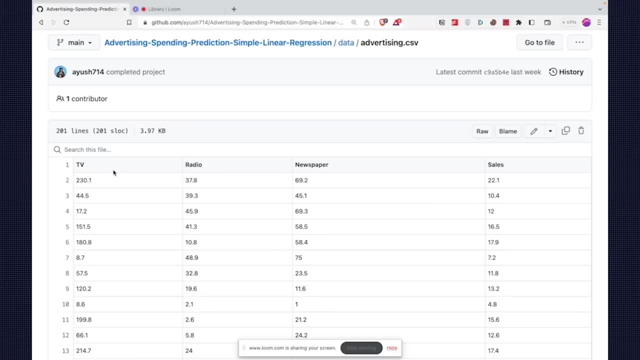 seeing the programming assignment which you'll be doing. uh, please see the course website where we have listed for the same. so, over here, over here, you have three variables. you have three variables, which is tv, radio and newspaper, and these are listed num listed, listed, listed um expenses. 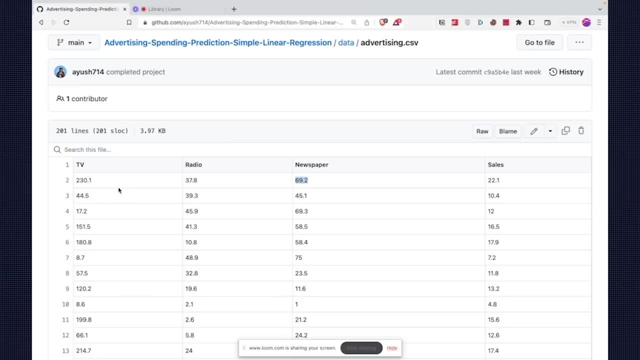 which which a particular company has put on. for example they have: they have spent around 200, that 230.1 uh on, uh on on the expense on tv, uh at advertising on tv, 37.8 thousand dollars on radio and six sixty nine point two on newspaper advertising and based on the advertising they got. 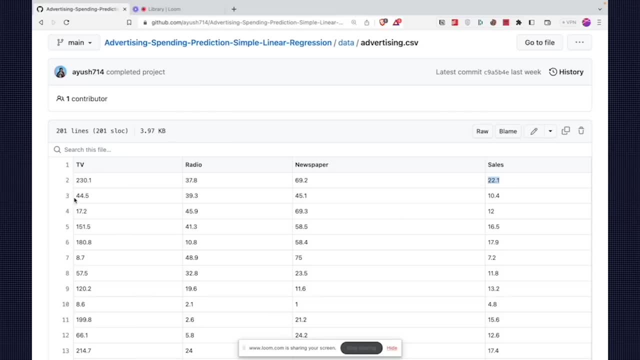 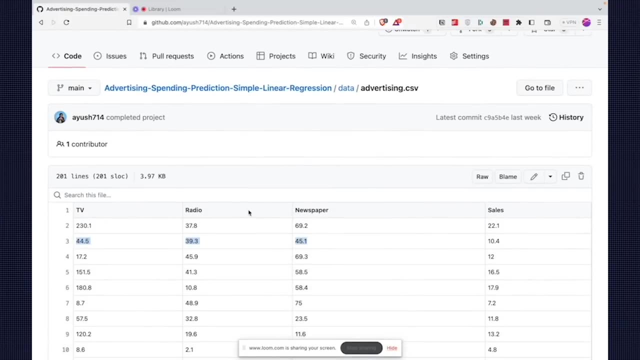 22.1. this much sales, okay, so so basically, we had, this is over. here we have the expenses which every company has did on tv, radio and newspaper and we are going to predict: uh, what is now? what is the significant number of our sales? so now your task as a data scientist is to identify: 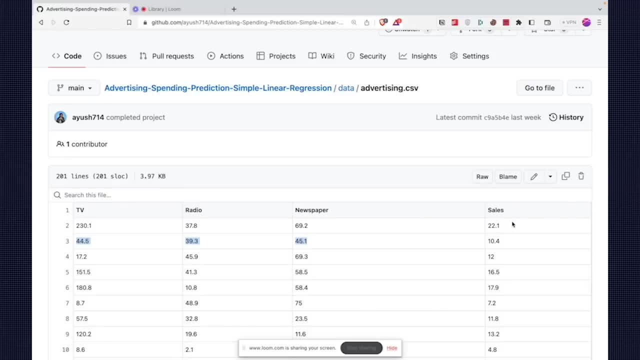 which, which, which mode of advertising is much more liable for? is which? which a company should increase pins to get the sales? and which one, um, which, which one source we should completely vanish it like, we should completely ignore it, for example, in some cases, okay, you, uh, you, you might say okay. 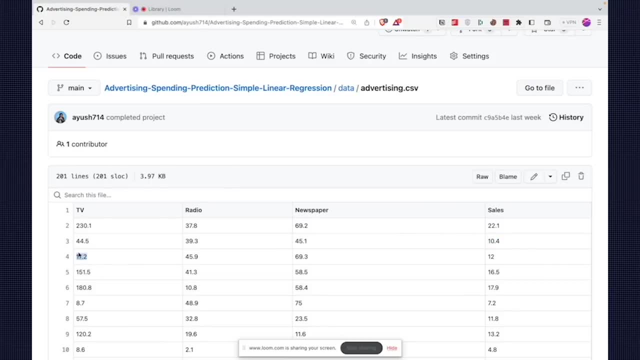 for this particular example, you might gonna go with tv because it is more significant in getting more sales as compared to newspaper or radio. right, so so your comp. so so that's that's what your work should be as a data scientist: it's help to take, help the stakeholders to take better. 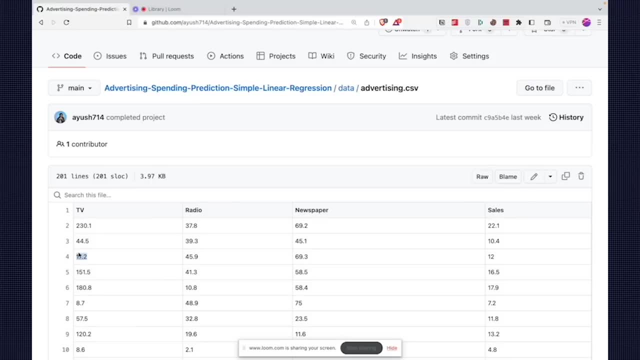 decisions out there, right? so what decisions they they have to take? they have to, they have to take the decisions of about, like, whether to use tv, whether to expand and spend more on tv, radio or newspaper or couple of them. so we have to identify, we have to identify which variable independent. 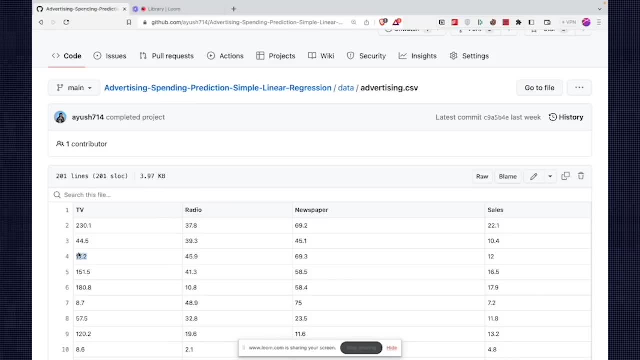 variable is giving most of the most amount of contribution to sales, which particular medium of source is giving most amount of information to the sales, and that's our problem statement. so what? i'll uh for being super simplistic as as, as i told, it's not a full-fledged project project, it's just for. 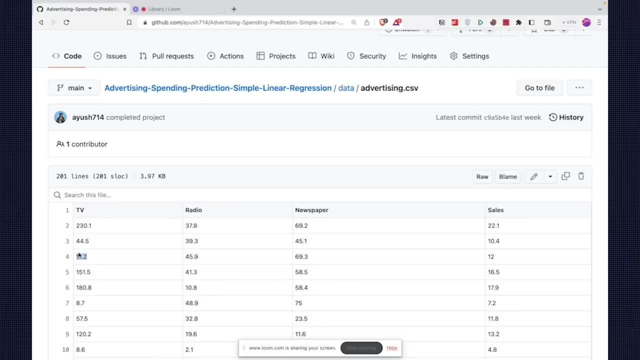 the learning purposes, not for the putting on a portfolio. so basically, uh, over here what exactly i want to do. i want to take this tv and i want to take one of the and take one of the advertising source and understand his impact, understand its impact on the awkward variable sales, for example. 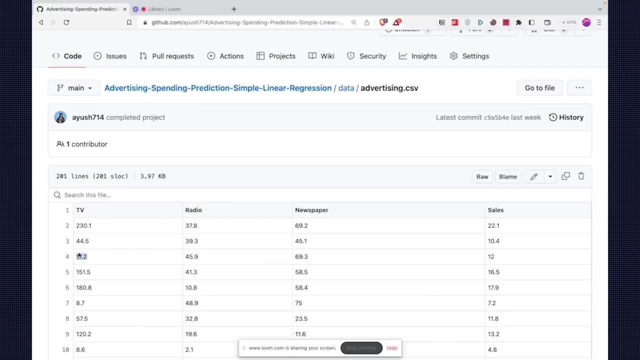 i could take tv and then understand its impact sales so i can build a linear regression on top of it where, given the tv, the expense curve given on tv, it will predict me the sales so that i can identify: okay, this much. and then i can do for. 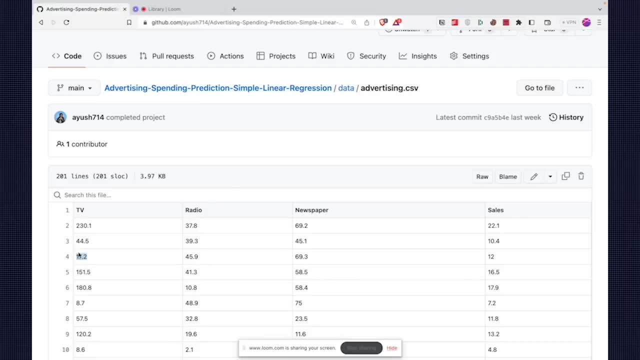 separate variables and then i can do for separate variables and then see which is which is having the most amount of contribution. however, this is not we do it. we actually use the multiple linear regression, where we use the three of them to actually predict the sales. but that's for you. 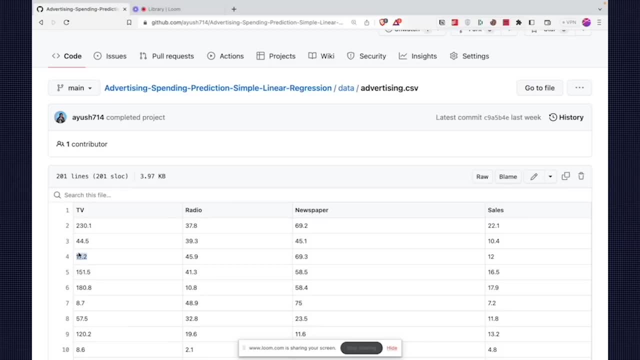 to try out, not for me, as a programming assignment. we have listed detailed programming assignment for you where we will we'll do a small thing and then you have to extend it to further, okay, so over here, oh, over here, what we'll be doing, we will, we'll be making the data into a simple linear regression. 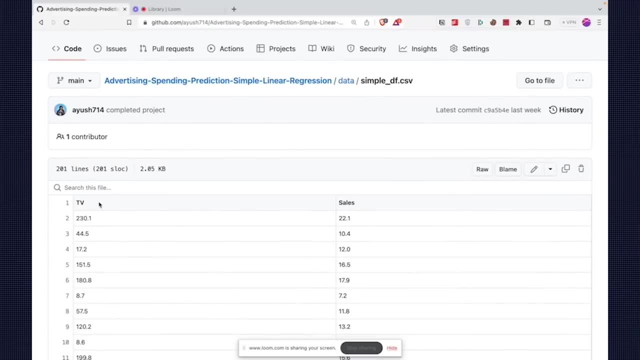 which is a simple pdf where you take the only one column as of now so that you have x1. we have only one entry and independent feature and then one dependent feature, and over here we're going to identify the significance of tv onto the sales. the significance of tv or 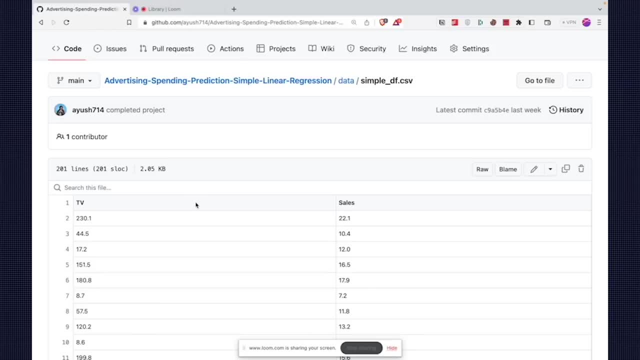 the sales. however, you can also include other variables if you want to understand the significance. but as of now, let's, let's get started with it. uh, you'll be also doing a very nice programming assignment where we'll be actually understanding, answering that question of which one to go. 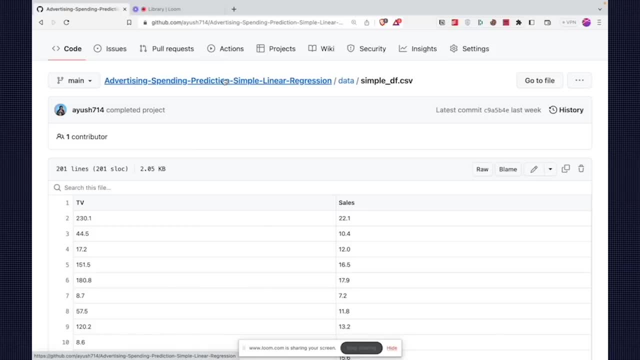 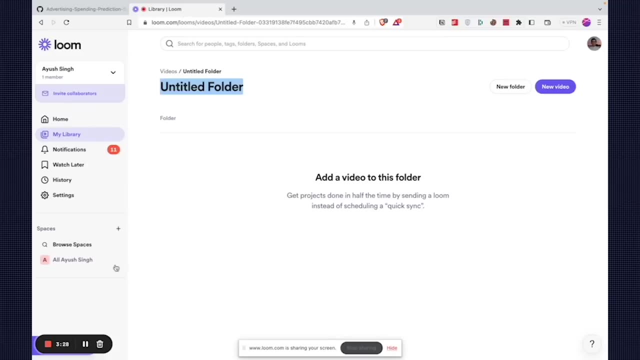 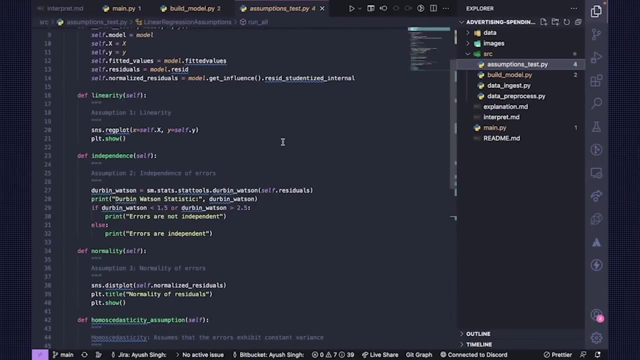 forward with which one of the medium source to go forward with. so let's get started with actually talking about, uh, the how, how can you code in a complete? so, uh, here we went back to this uh lecture, uh to this project. so i'm going to start off with the data ingestion. so 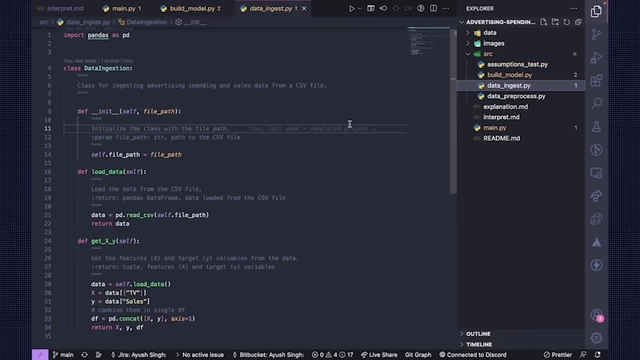 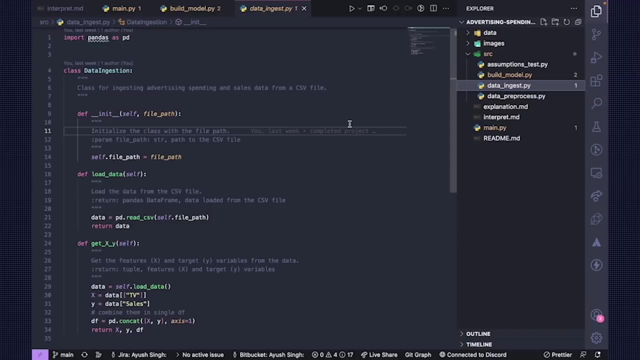 the first step of any machinery project is to ingest the data, and i'd really like it to be in sort of class and everything. so basically, over here, over here, we have- um, yes, we have a class and we have a data ingestion class which ingests the data advertising and then lowers it down to 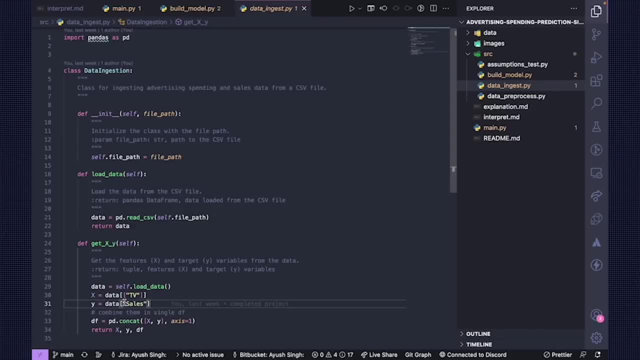 only one way to uh to a simple for, to a data set where we can use simple integration on, where we have only one independent feature and one dependent feature. the first step is to initialize the class for the file path, so we require the file path when someone 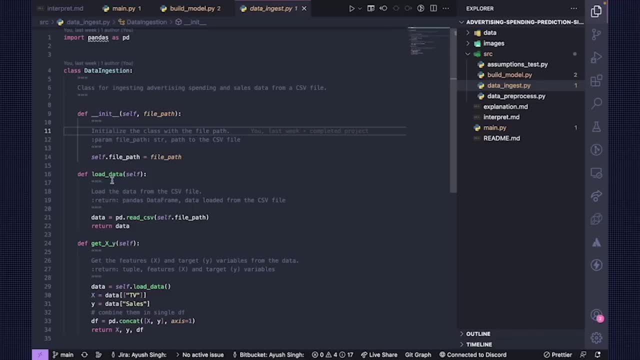 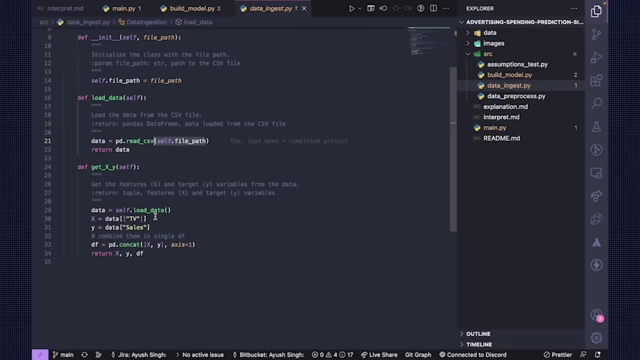 instantiates this cloth class. and then what? and then what we do, and then we have a method called load data which reads the csv, which reads the csv from the specified file path, and then we get the and then we get our specified. as i said, that it that we want the specific tv and say it's only. 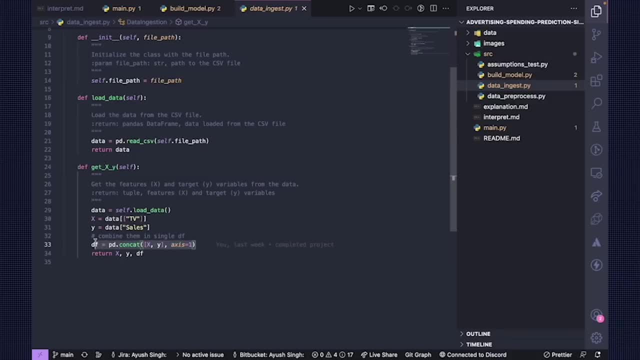 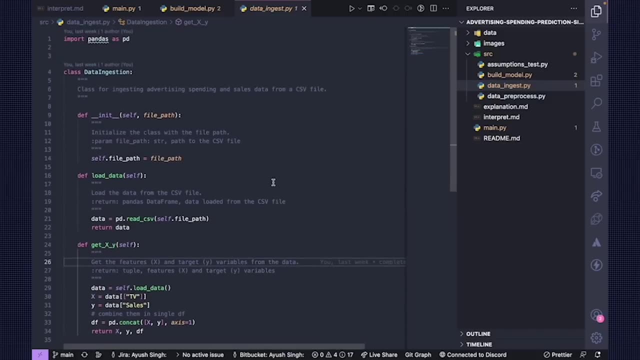 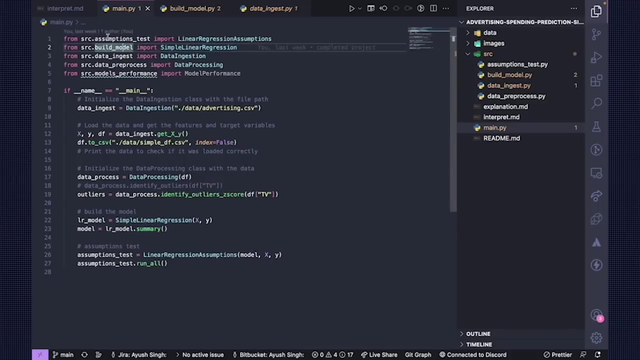 so that it is for learning purposes, and then we concatenate both of the x and y variables and then we return that data frame. okay, so this is a basic data ingestion class, not a big deal to understand it. okay, now we can actually use this. now we can actually use this over here, over here, which is: 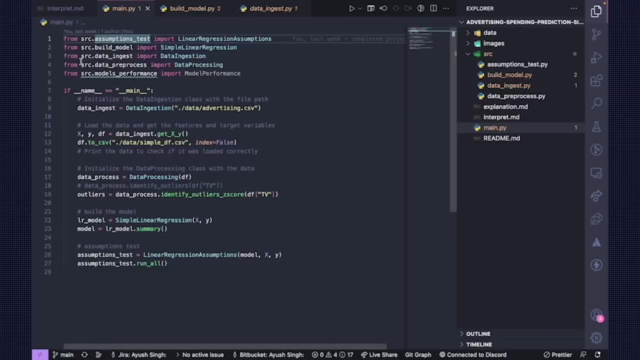 uh, where? where we are importing, so ignore everything, just just just go over here. you can. you can say from source, which is the source folder, dot, data ingest, with the file name import the data ingestion class. and then you say, okay, this instant instantiate a class, and then um, and 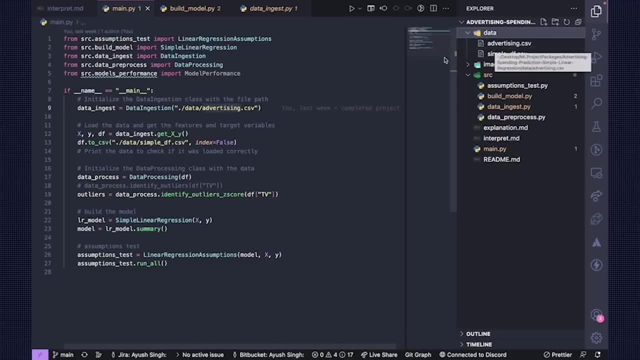 source it to the or the make it to the advertisingcsv and that gives your simple df. that that, that will give you the data frame, which is a simple df, which we want to perform on. okay, now internal injection is done, so let's run our file to actually see. okay, that will make much more sense. 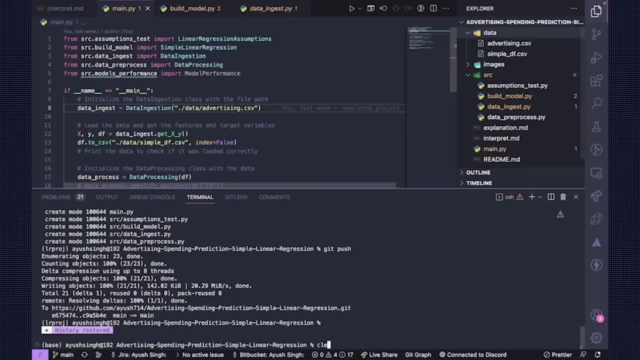 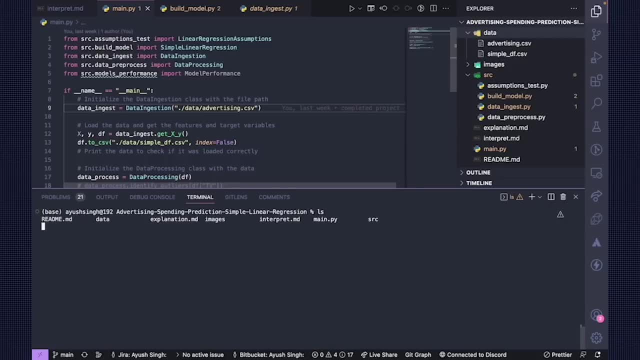 and i'm going to use something like: uh, very nice over here, so i'm just oops, clear ls, and then i'm just going to have this: uh, if i have actually an environment prediction, so i'll just, uh, environment variable. so what was the name? lr crotch maybe, i'm not sure. yeah, uh, so honda. 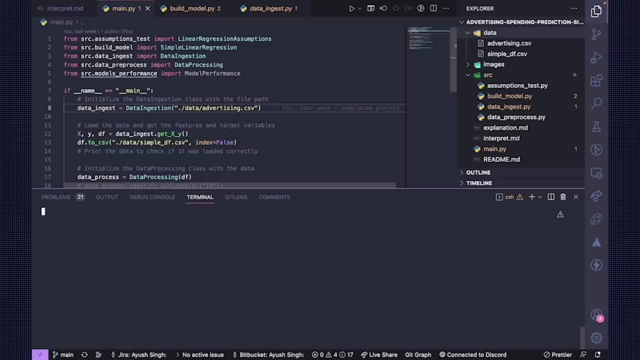 deactivate. so that's clear. okay, so, uh. i have activated my environment. if you don't know how to activate, you will be also in the reading materials for that or the other. otherwise, in the next set of projects, i have showed you how to do this. okay, so uh. 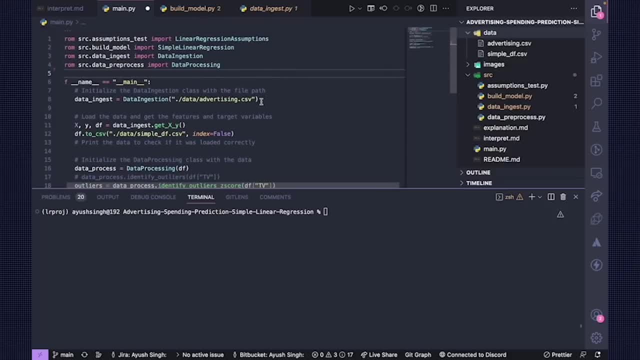 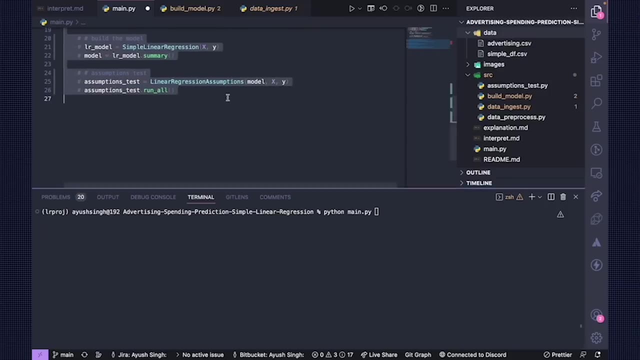 i'm just going to remove this because that's not required. yes, over here now, what we will do over here now, what we what we will do is we will simply uh, run this python dot, python mainpy, and i'll just, i just want to run that. uh, just going to make it comment and i, i just want to. 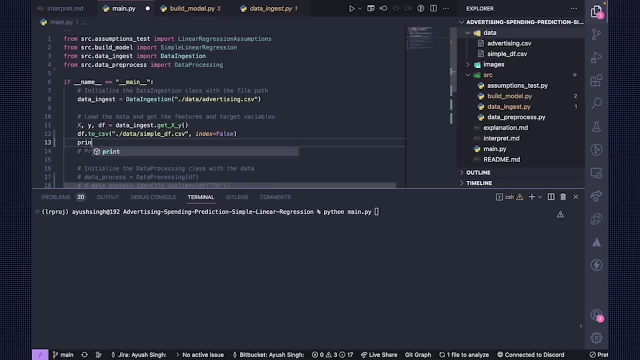 take a look at what exactly the data frame looks like. so, just going to print that data frame, print that it, uh, the data frame, so that it may seem it's good to use, so that you can see what exactly the it's working on. so so when you, when you run it, you'll be eventually getting a date, a data frame. 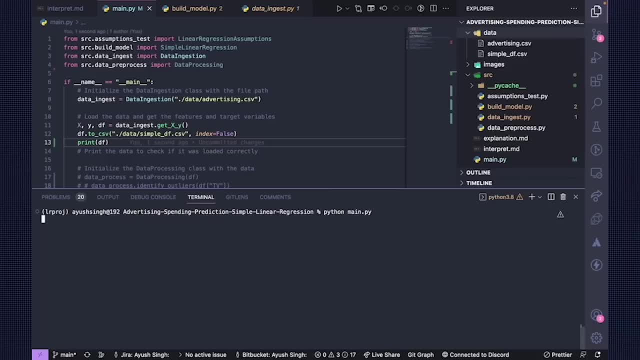 where, where you have only one column which is then x and then y over there. okay, so it eventually takes time initially, and then it works fine. so you have the tv, which is the expenses on tv, and then the sales which happen if you advertise on tv. so that's, a data ingestion is done. now the 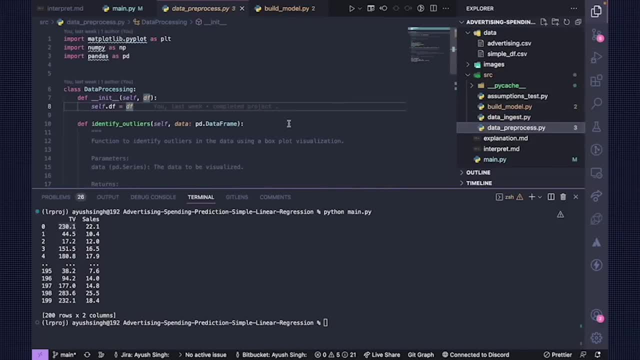 next step is i'm going to do a basic data processing. please note that in the next project which we'll do, we'll have the very extensive data processing thing. but as of now, i would suggest you can ignore this as of now, okay, uh, maybe, uh, you it just for. 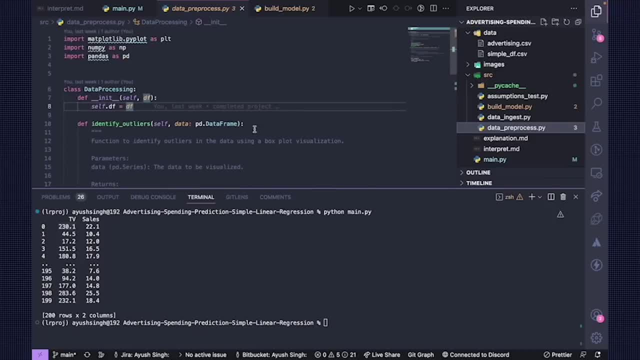 information purposes, if you want to know how we, how we are performing, basically what we're doing. we are, we are importing a class, known as data processing class, and in that we are instantiating, uh, instantiating with the data frame object, sorry, uh- which which takes an input, which is data frame. 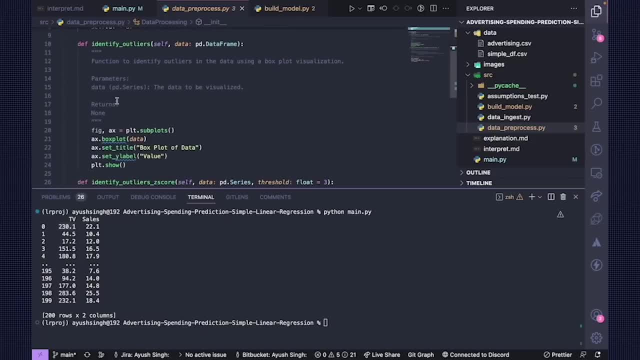 and then performs couple of methods. the first method it applies, it identifies if there's any outlier. we box plot. we box plot and see if there's any outlier. we box plot and see if there's any outlier in that particular tv's variable because linear regression is, it's sensitive to outliers. 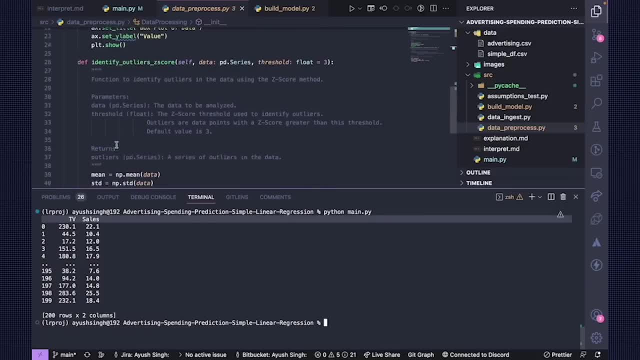 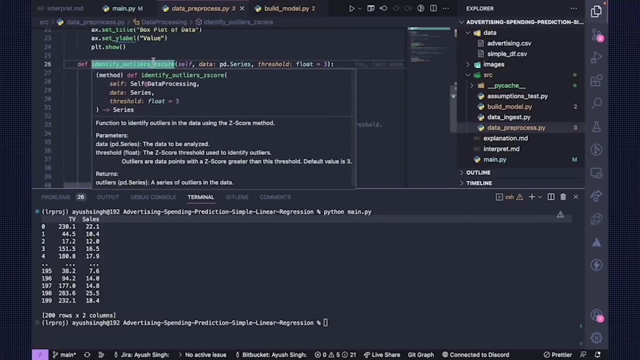 so we have the tv and then we just see if there's no pliers. if there's any, we identify uh, the out, who. who are those outliers? numerically okay, and there are several ways to deal with capping, trimming and several ways to identify as well, which we'll be seeing in the next lecture. please ignore that. 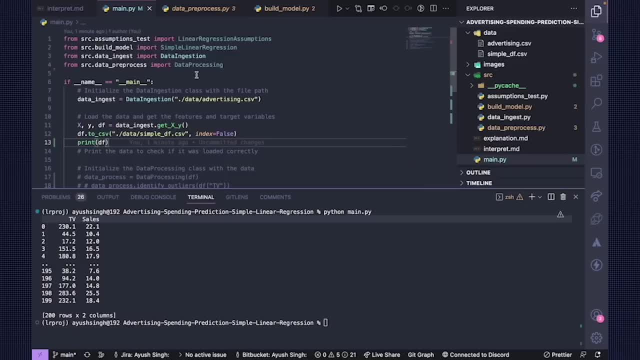 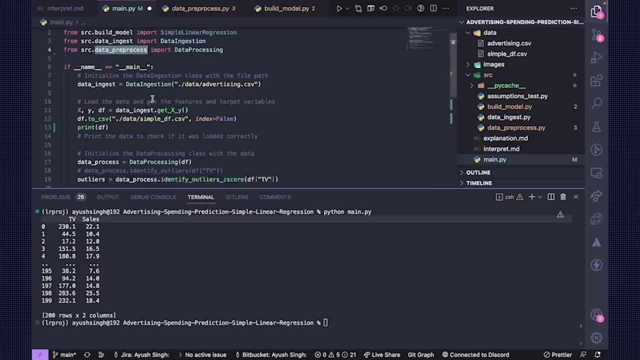 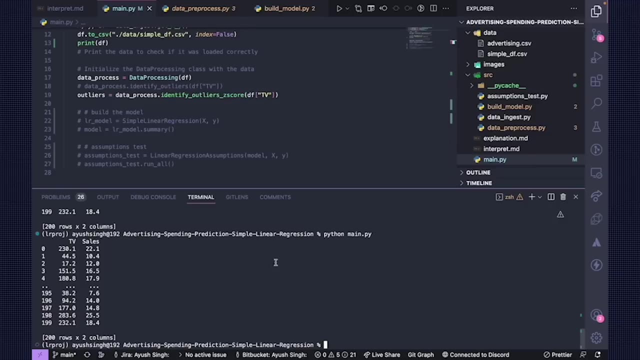 as of now. so when you go to mainpies, now, uh, now you can just import the same thing we can import, which is the data processing, from that data source folder in the data data pre-process file, and then you simply run it. so let's when, when we run it, it is okay, let's identify if there's any outliers. so, 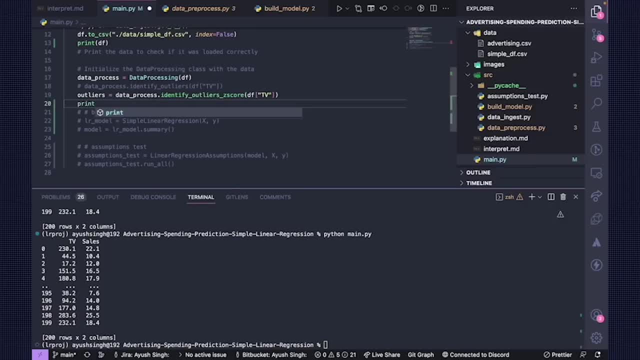 it says that there's no, any of that. so let's print it out. let's let's print out books. i haven't printed out so outliers, so if i just print it out, you will be able to see that there's zero outliers in that particular column. okay, of uh using z score, but you'll identify your method to actually uh. 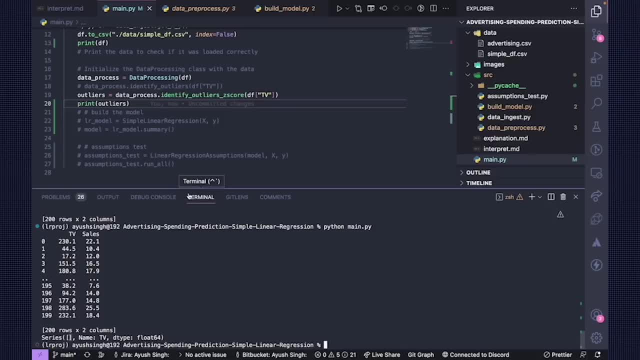 identify which are outliers and outliers, which are outliers and outliers, which are outliers and outliers. i recommend to. if you don't know about outliers, you should wait for the next lecture. as of now, you can ignore this. this, this is not the scope of this uh video project. the scope of this project is: 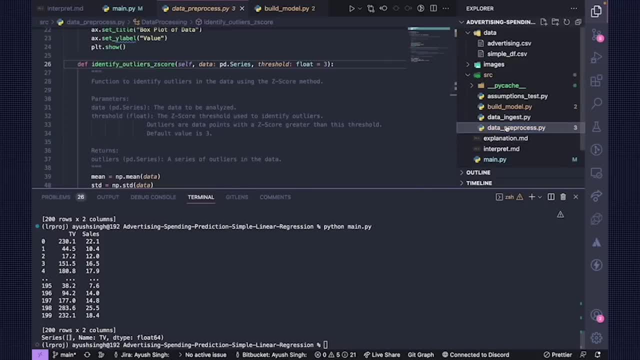 focused on model building only. so now, once we have the bit of processing, i just want to show you the process. nothing else like. okay, after data ingestion, we process the data in a good way, and then what we do? we go on. how can we build a linear regression model? so how can we build that? so we'll be using 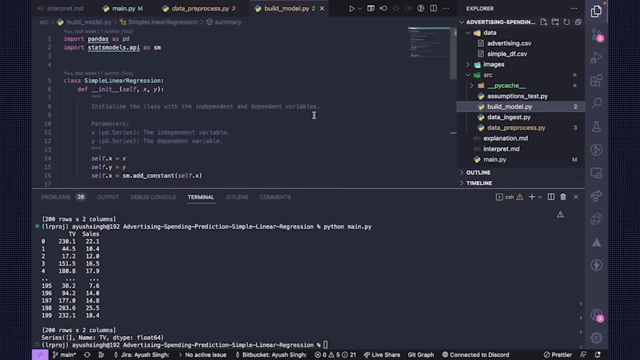 a stats model api, because i really like that as compared to the scikit-learn, because, um, i don't know why, but yeah it, it is more interpretable, it gives more results, it gives more explanations when we after after building up the model. okay, so basically, we'll build a class. 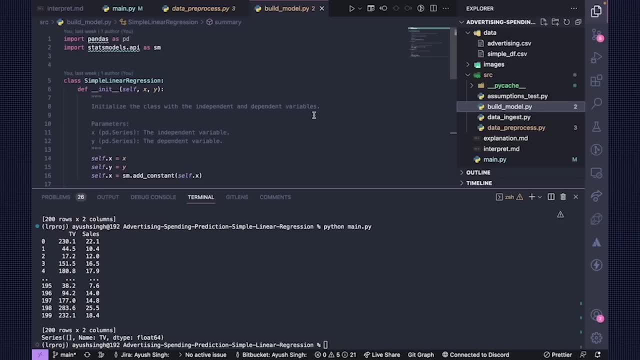 which takes in, which takes an x and y, which is the independent and dependent variable, and then we, and, and then, and then what we do? we add a constant which is one, one, one terms- you know, in x is a design matrix- and then one, one, one, one, one, uh, a column of one, so that we multiply with. 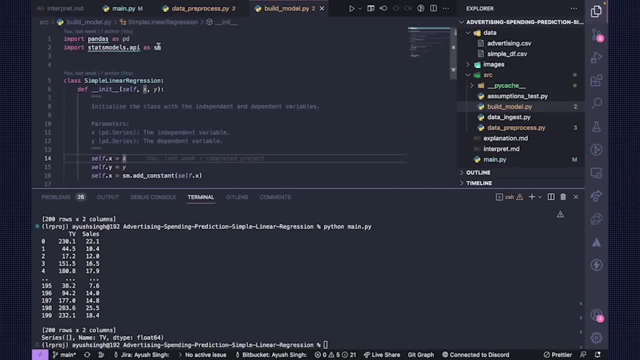 beta zero and one which is sm dot add constant. we have sm as an alias and then we multiply with beta for this, a for for this, uh library, and then what we do, and then we make a method called fit and that fit, what it does. we are calling, or we are we are calling, orderly squares, which is equivalent to: 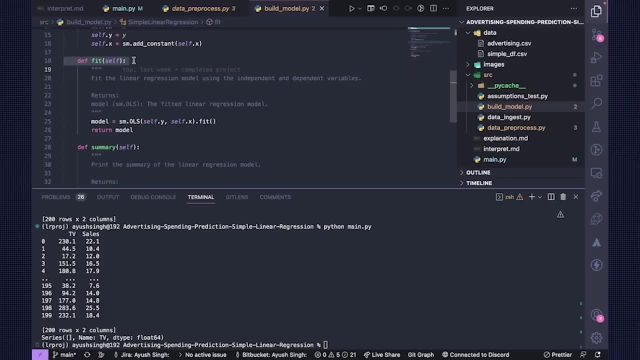 linear regression and then we're calling dot fit. and when we're calling dot fit, by giving your independent variable independent, sorry, dependent variable, independent variable, we were saying: okay, this is something as a dependent independent and this something is independent. so model that relationship using linear regression first. first, what this fit fit will do, it will perform all the. 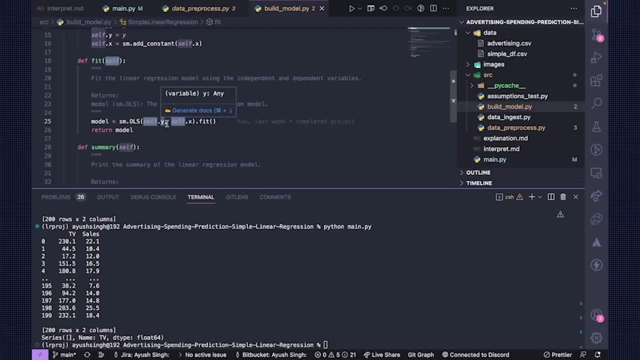 steps. first step: hypothesis. second, calculate the cost. third is perform the gradient descent on top of it until, unless your model is confused- we have already talked about what exactly fit method does it fits the method. for example, we have already seen what the algorithm is. take out the hypothesis. 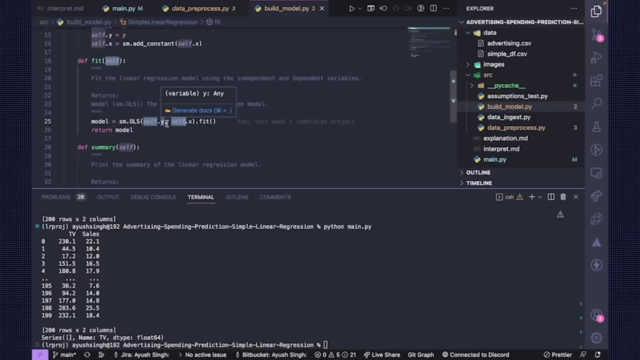 take out the error, take out the dead, take out the derivative and then perform the gradient descent n number of times, just after you updating and updating beta's value. so that's what fit does. okay, fit means it trains your linear regression model by the number of iterations. so when you 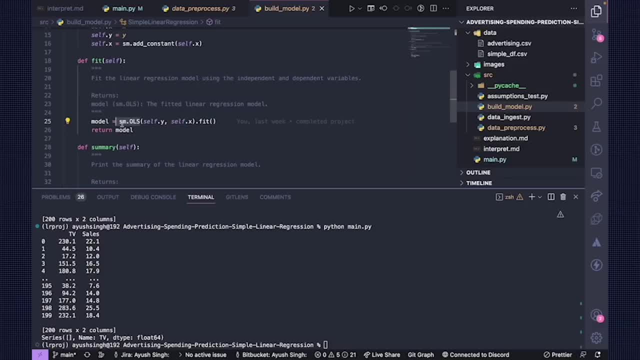 actually go and see what it. what exactly isn't that all what it says? you will be seeing all this stuff, but but basically it trains your using gradient descent algorithm- cool- and then return the model and then we can print the summary of our model. what exactly, after training our model? what exactly the summary? 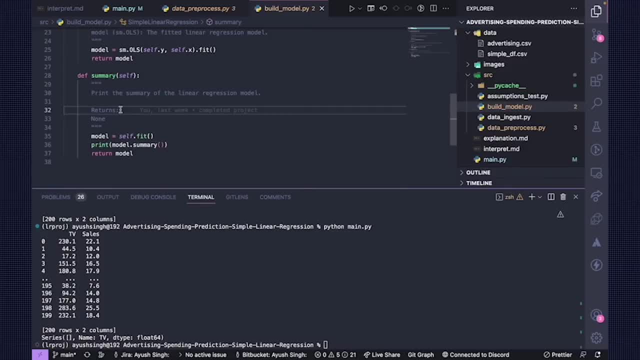 of our model looks like, what exactly the summary of our model looks like and if you, if you're getting confused what this dot fit method does, please take a look at online from for scratch implementation of linear vision if you're still not sure about how do we programming it up. but 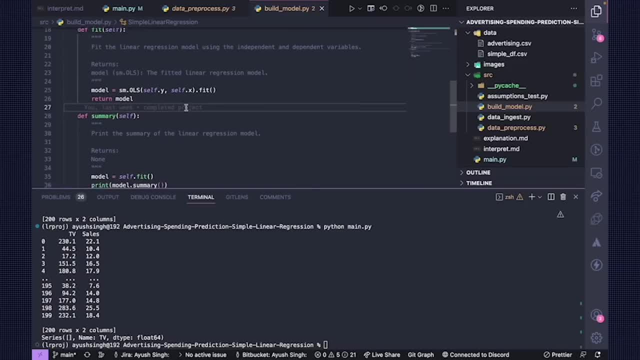 if, but you have to attempt a programming assignment for this. for better understanding, you print the summary of the linear regression model, which is model is equals to selffit. first of all you train the model and after yourself you train the model, and then print the summary of the model and return the trained model so that anyone can use it for a prediction. 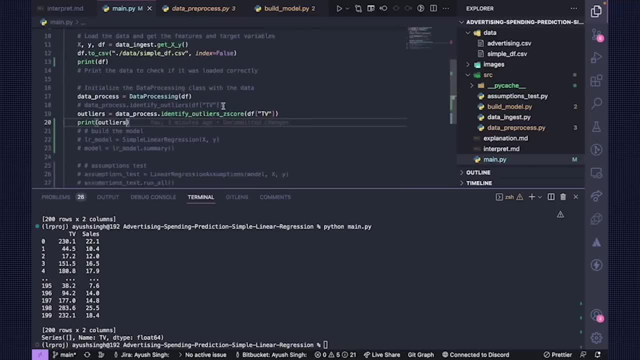 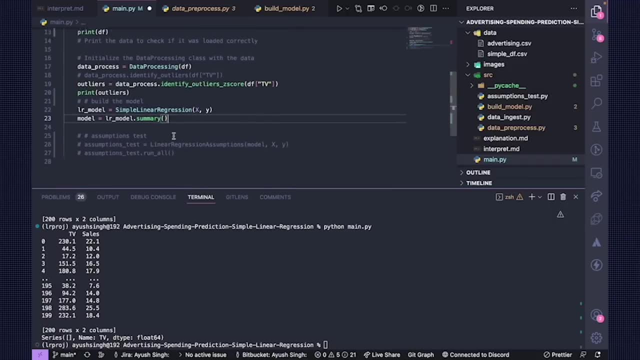 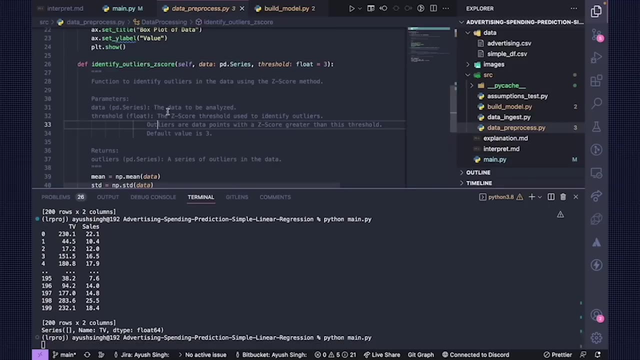 so over here, when you actually uh, when you actually uh, use that, so let's, let's, let's have a basic, uh, simple integration model over here and let's print it out, let's print, print that stuff out. so, um, basically, we are, we're just calling dot summary, we are just calling dot summary, and when 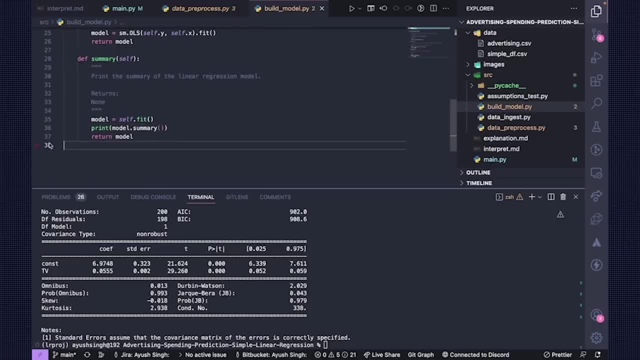 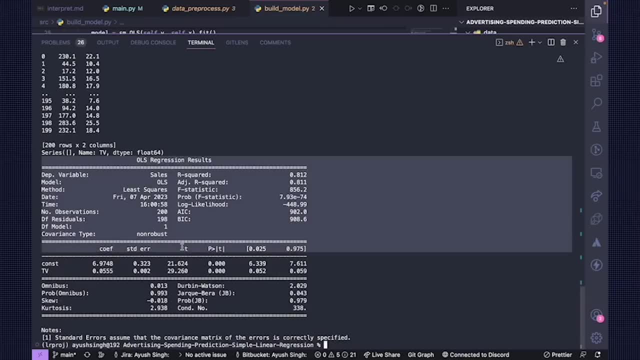 you're calling dot summary. it first of all trains the model, prints out the summary and then return the model. so how does that summary looks like? which is the most important part of this lecture is we have this ols regression results which is telling: okay, this is the dependent variable. what? 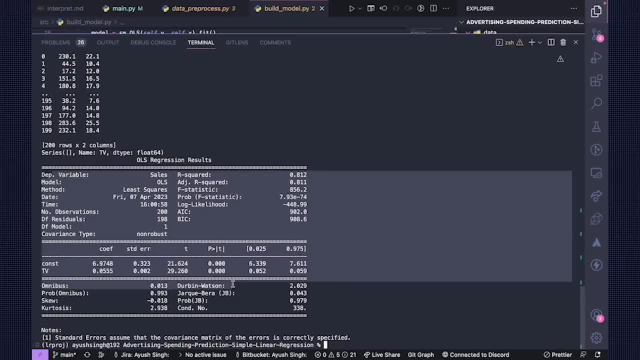 model we are using and a lot of things. we should talk about that in just a second, about how we can interpret the ols results- regression and then, once we have our uh ols results- now we are, we have a with a full report of how it is performing, how our model is performing, how how they're performing. 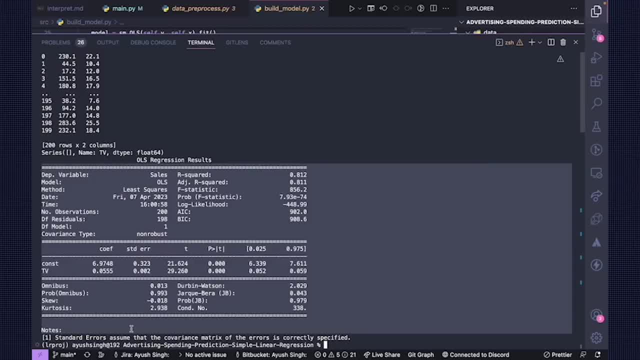 in different, different tests and etc. and etc. so this is something which will, which, which which we'll talk about. okay, uh, each and every integrated what exactly this, what exactly this, what exactly this report says and everything in greater detail. so let's talk about how can we interpret each of. 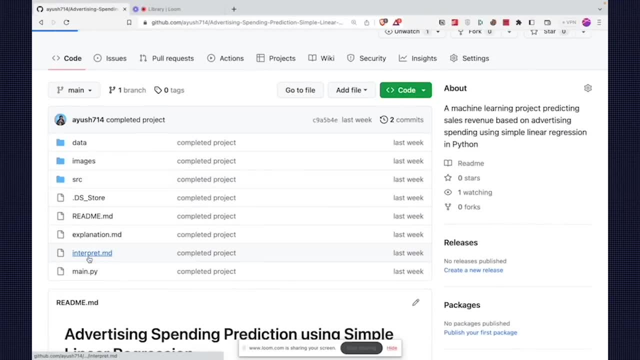 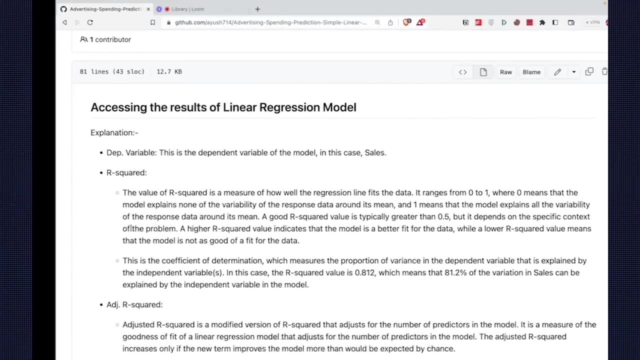 them in a nice way. so i would suggest if you go to interpretmd. so when you go to interpretmd, you have pretty much everything listed out there. so i'm just going to focus on important you know, explanation of which is required for you as of now and which is in the scope of the course. 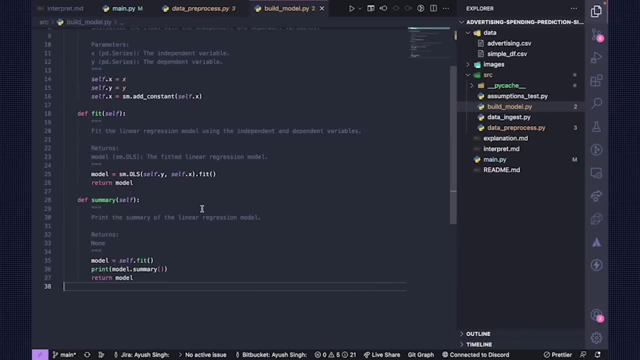 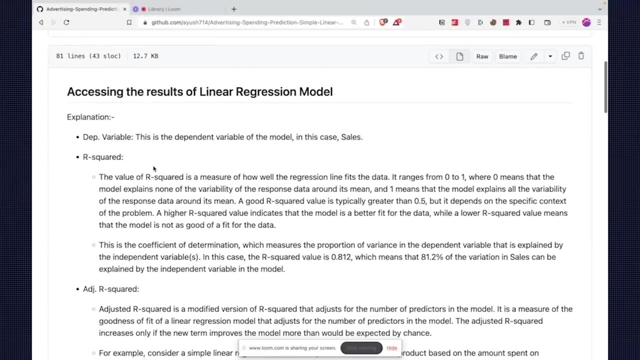 uh, like, contrary to the intervals, which which we haven't had a talk, so i'm not going to talk about that, but we're going to talk about most of the things, which is the starter, which is also very, very important. cool, so let's talk about that. so, first of all, let's let's- let's- assess the results. 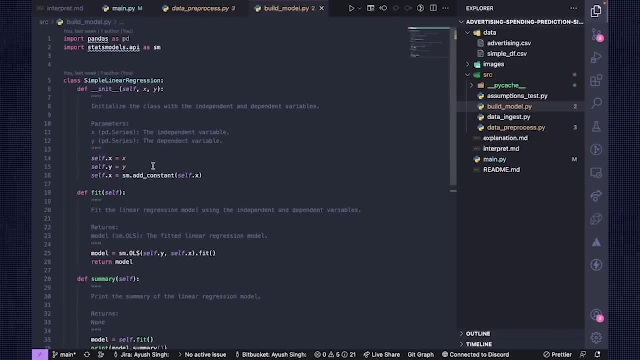 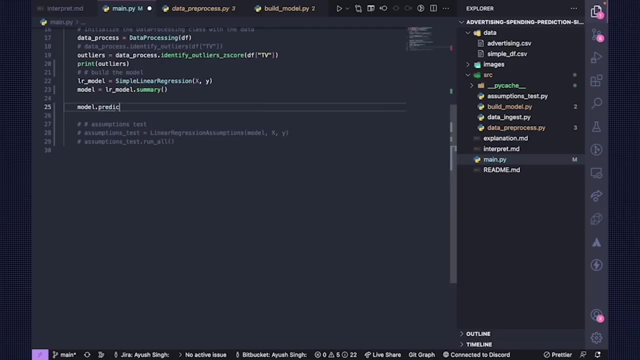 so now we have trained a model that can take in the tv expenses and then could predict, and that can predict what, the what, what will the, possibly the number of the sales which which you're going to get. so what you can do, you can simply go over here. you can simply go over here and then say okay, and then say even modelpredict. 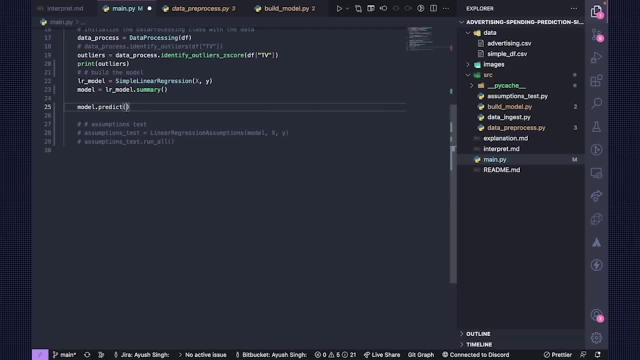 modelpredict, you're given the you, you you're given the value of tv sales and then that will give you you're given the value of tv sales and that will yield you to the particular variable, which is the uh- so tv expenses- and that that will give you the sales. okay. so this is what. 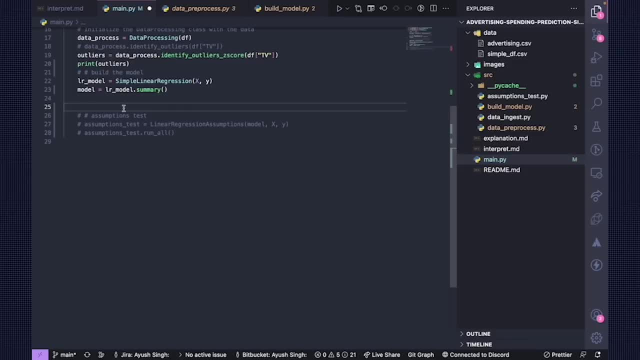 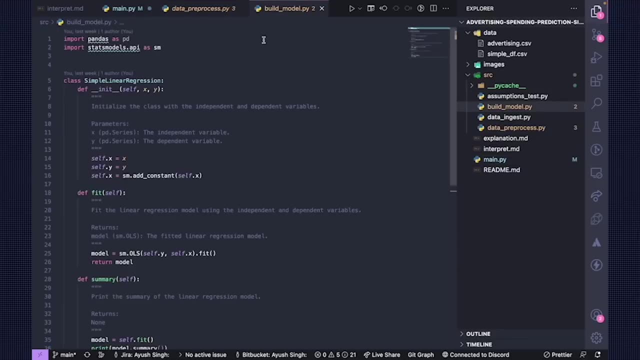 what you're going to model or predict, but that's something for you know, i just like you, can easily do that. i assume that, because that's something which i would also explore by your own. okay, cool. so over here you have the first first and first one is dependent. 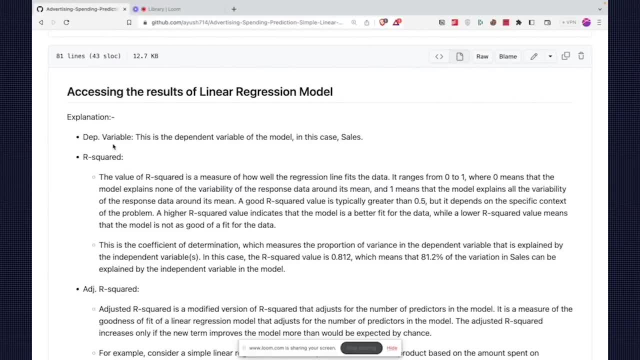 variable and dependent variable is a dependent variable in the model, but in this case it's the sales going to predict the sales, given the tv expenses. second one is r squared. as you know, we had a talk on r squared right in great detail. how do we evaluate our? how do we ever evaluate our? 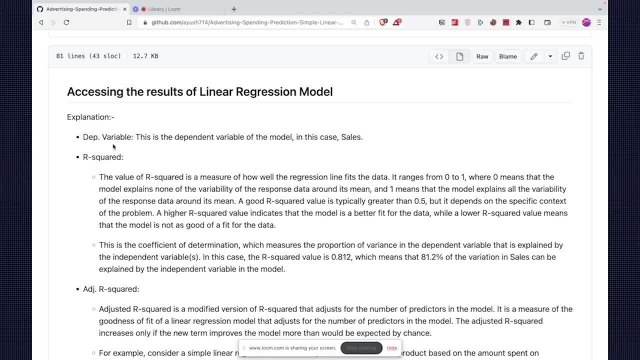 linear regression model. so over here. so over here, our r squared, our r squared, which is nothing but the r squared, which is nothing but the r squared, which is not good, okay. so that means that 81.2 variations of the sales is explained in our tv. that means that it's pretty nice, which is 81. 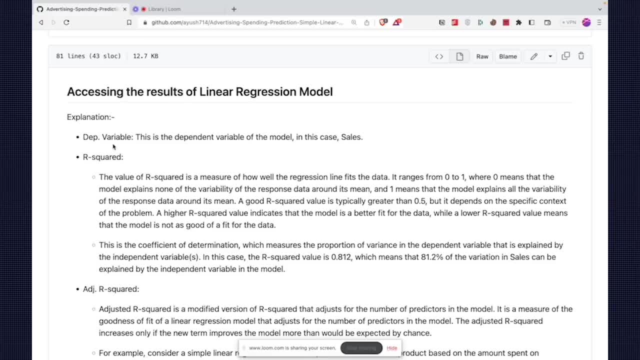 percent of variations in the sales. whatever the variations comes in in the sales is being described by your tv expenses and that's pretty much good. it's good. so higher r squared indicates the model is better fit to the data. where lower is not good, okay uh, but but it also depends on problem. 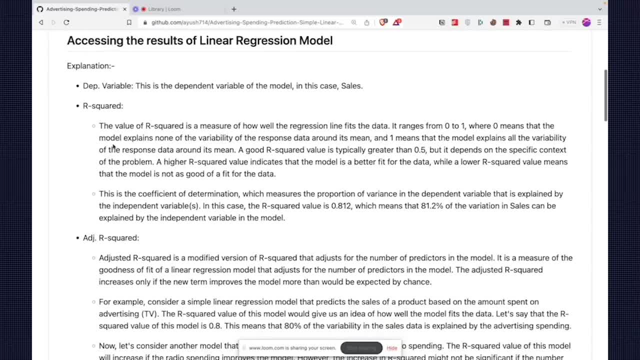 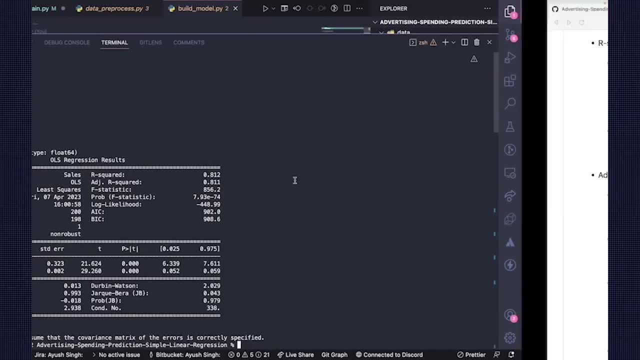 to problem, so you'll. so you might have to worry about that as well, but but basically, over here it explains pretty well: uh, what is adjusted r squared? adjusted r squared in this case is almost the same. it's almost the same, which is 0.811. and what is what exactly adjusted r squared is? it's, it's. 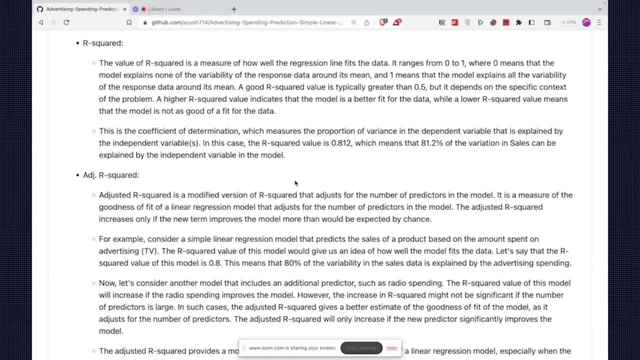 nothing but a modified version of your r squared. modified version of r squared. so what is modified version of r squared? for example, it is a measure of a goodness of fit for the linear vision model that adjusts for the number of critics. now you know you might be confused in this, so let's. 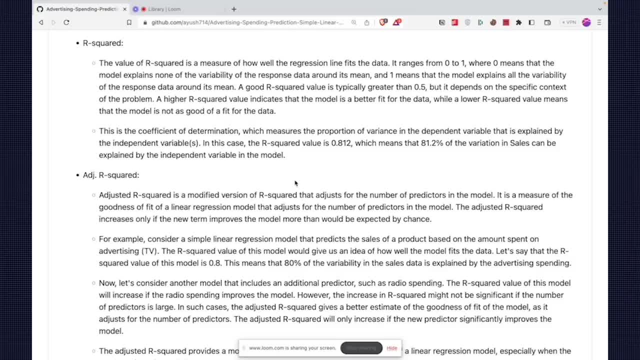 consider a very, very simple example. consider that linear model that predicts the sales of a product for the amount of money spent on advertising. okay, so r squared will give us an idea about how more, how well the model fits on the data, how well your sales is being described by your independent variable. okay, now let's say now: 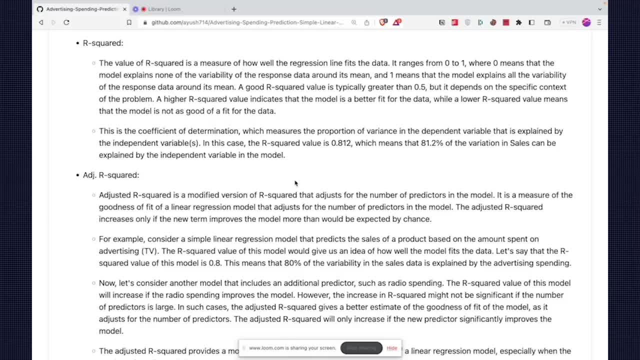 let's say that you add an additional independent variable, such as how much your, how much your company spent on radio spending. okay, so the r squared value will increase if the redo, for example, which which we have will increase if the radio is spending, improves the model. okay, like if if the 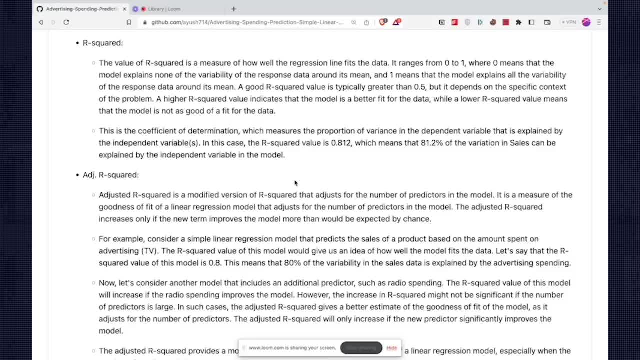 radio spending improves, the model r squared will also increase, right, so, basically, so, basically, it will increase, even if one of the predictor is not improving the model. okay, so you put another variable, x, and then if it is, if, if, if it is not improving, but a radio is improving, then increases. 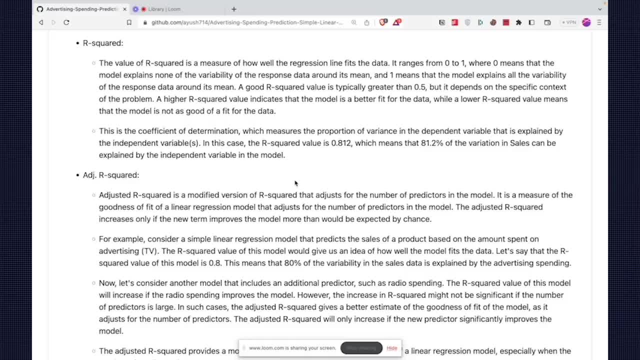 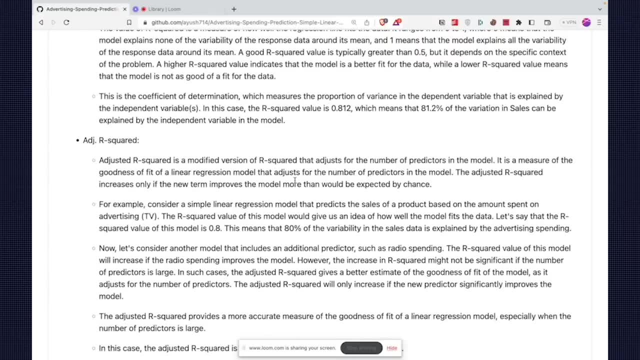 so r squared might not be significant if you have a more, lots, lots of predict independent variables. okay, lots of independent variables. so i just r squared is pretty much the same because we have only one variable and they are almost same because over here we have only one to check the, that to, to check how much they're explaining to the output. 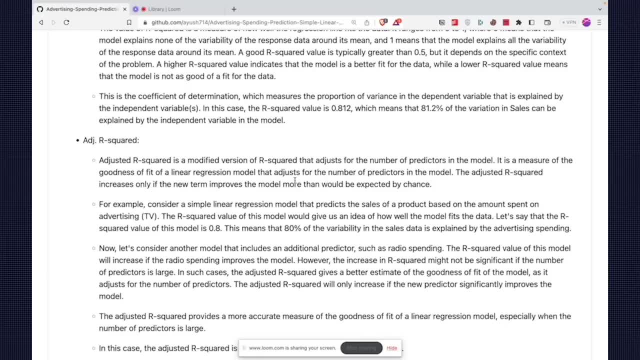 variable y. but, for example, if you introduce to one of the variables like radio newspaper, then you will see a massive difference. because, because if you have a large, large number of, even if one of them is increasing, is improving the model, your r squared will increase, but r squared 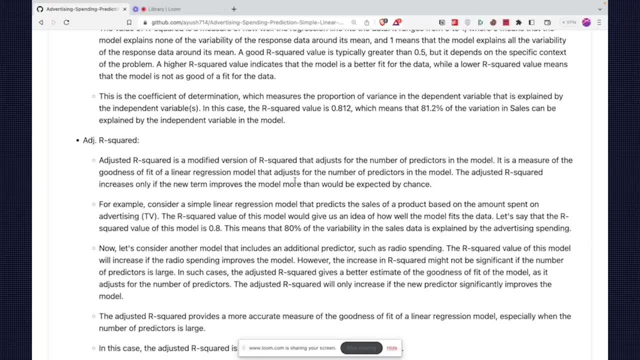 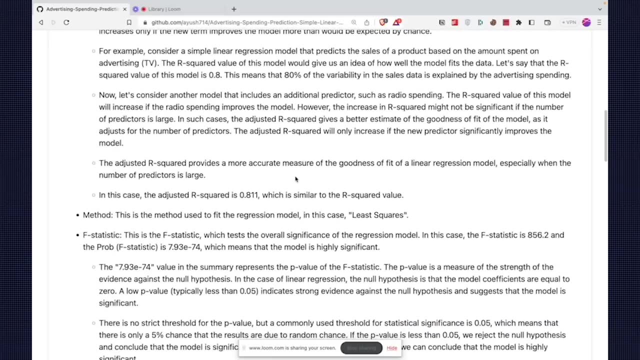 just increase the rs, but adjust r square. what does it do? it only increase r square if and only if, if, if and only if, if your overall it just if your overall model- is improving. okay, so that is our adjusted r square. you can take a look if you want to know more about it. another one is method. what? 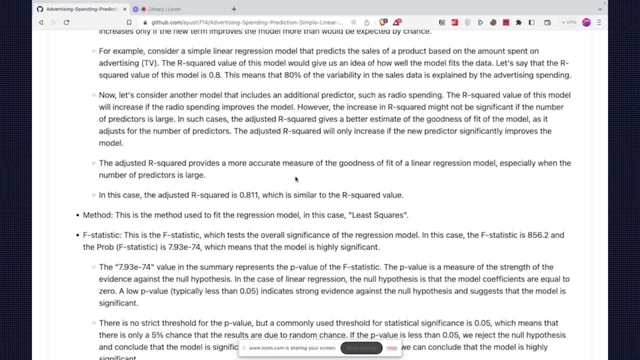 method which you're using, v squares method, where we are using gradients of uh green- is almost same, but a little bit of difference at all. but we are using gradient descent algorithm to optimize it and then we have something that's f statistic, and then we have something called the gradient descent. 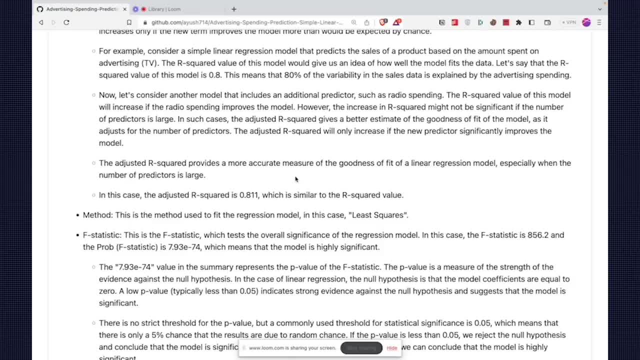 So F-statistic, which we have already talked about in hypothesis testing, an F-statistic which tests the overall significance of the regression model. In this case, the F-statistic is this much, which tests how much your regression model is good. 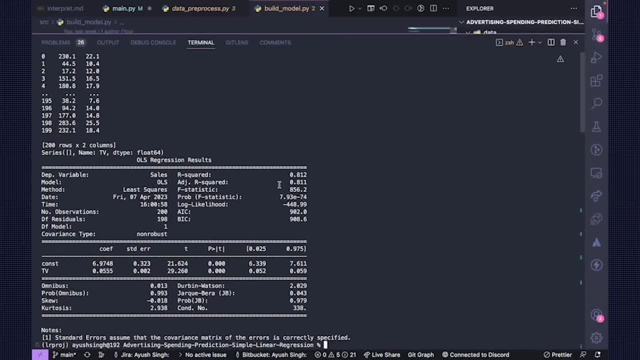 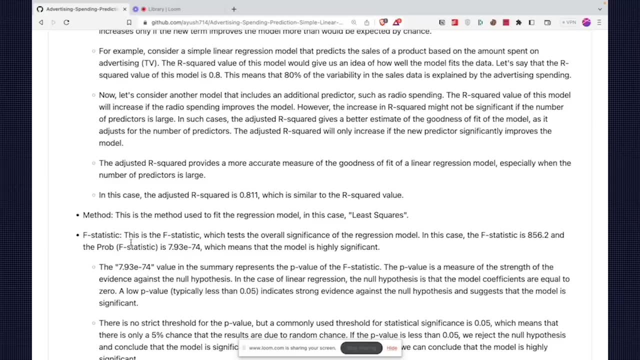 So basically over here which you see, the F-statistic which does overall significance of a particular model, And if you convert that to a probability of F-statistic which is around 7.93-74, which means the model is highly significant, 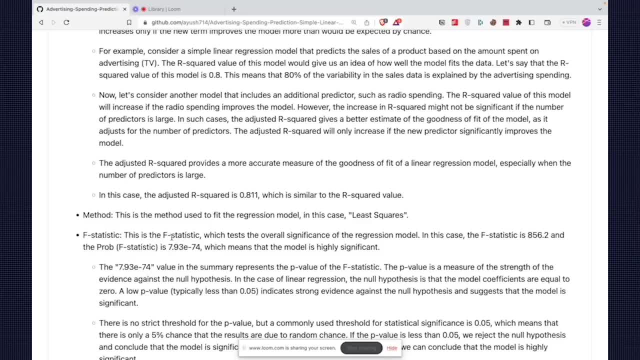 How can we say that the model is highly significant? So you might be thinking, hey, 7.93-74 is very, very small, very, very large, But it's not Actually. if you know math, then you'll be able to understand that it's actually a very, very small number. 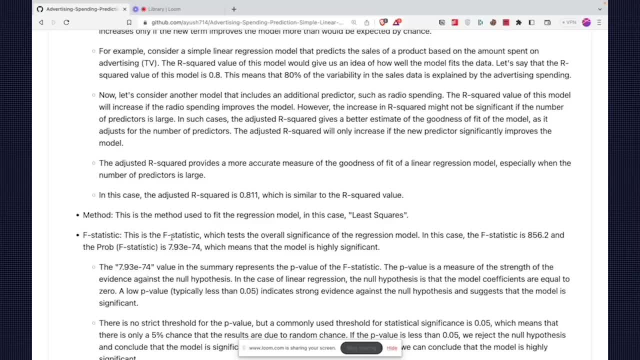 So what we'll do, we'll compare that value, the probability of F-statistic, we'll compare that value against our p-value And then we can see over here. And then we'll compare that value against our p-value And then we'll compare that value against our p-value. 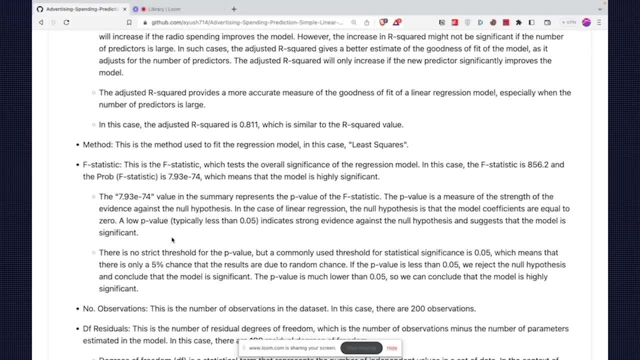 And then we'll compare that value against our p-value And the p-value we can test. in this case we can have a null hypothesis that the model coefficients are equal to 0.. A low p-value indicates that the evidence again. 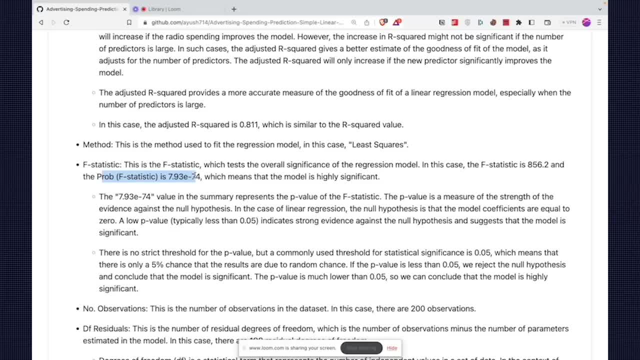 so we can. so p-value, which is the p-value, p-value lower than 0.05, so that will. if it is, then we'll reject it. So over here it's actually lower than 0.05.. 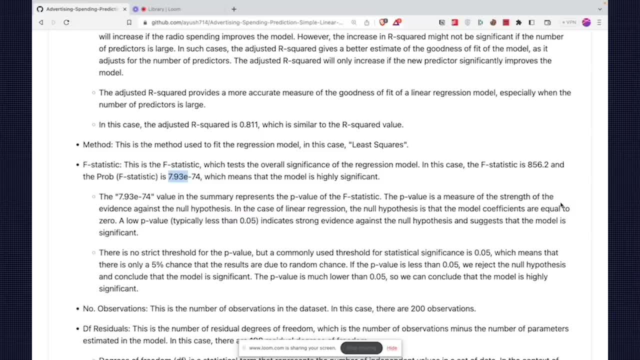 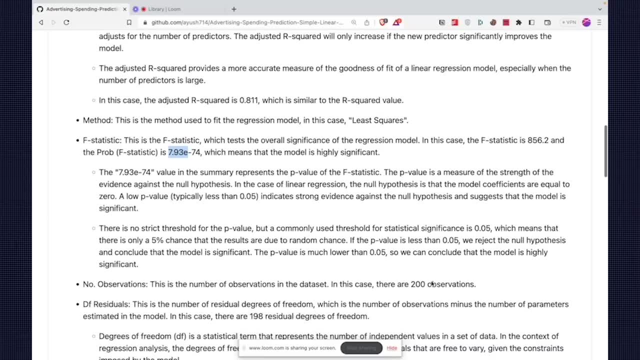 Then we'll say, okay, let's reject our null hypothesis. The null hypothesis was that all our betas are equal to 0.. so that is not so, so we can see that it's pretty very zero. that model is highly significant to our 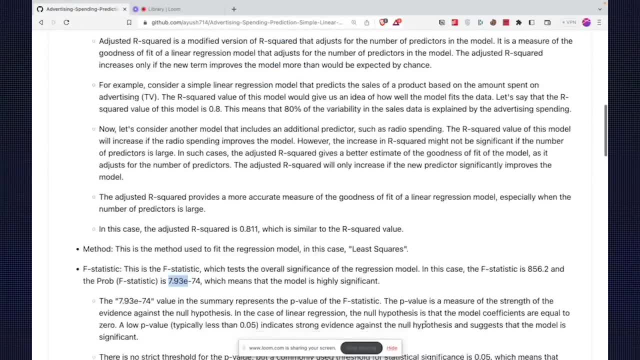 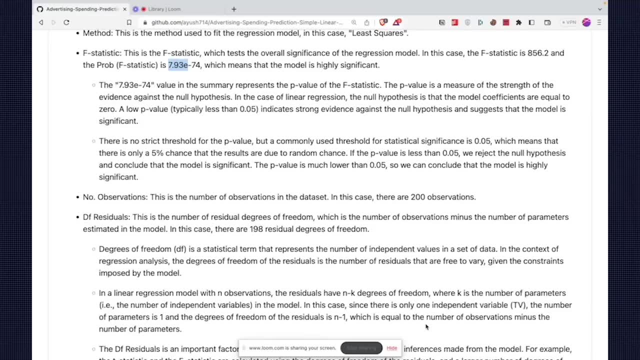 uh, so your, your, your dv is highly significant in predicting that. but but, uh, you see, but this, this, this f statistic can be for several other values as well. it does the overall sense. so if you also see the highly significant, then if you use three of the variables of radio, newspaper and uh, what? 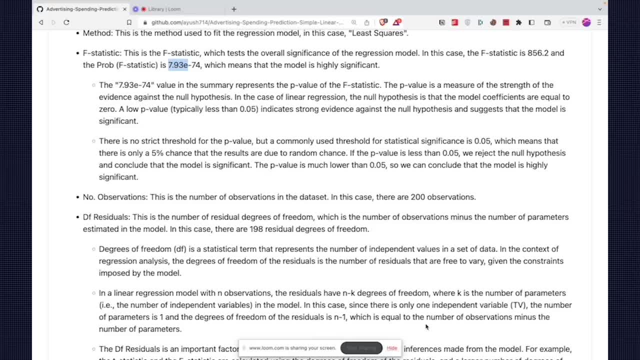 the tv. then if it's highly significant, you say okay. three other variables are very highly significant as well in predicting the sales. okay, uh, number of observations: there are 200 observations as of now. as i said, there's degrees of freedoms, so degrees of freedoms in this case. 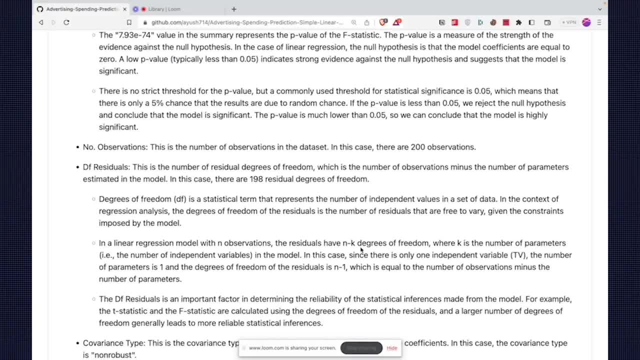 is 198, because you have 200, 200 number of rows, and then you simply have number of rows or number data points minus the number of parameters, in this case, only beta 1 and beta 0. beta 1 is related to tv and beta 0 is the constant term. uh, is this the bias term? so what exactly degrees of freedom is? 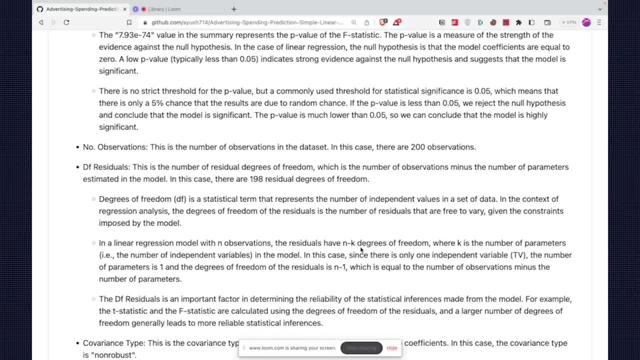 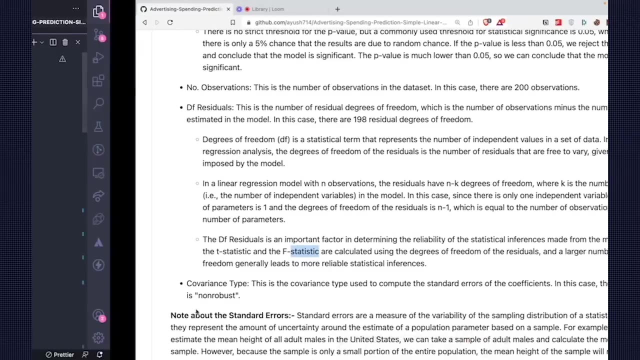 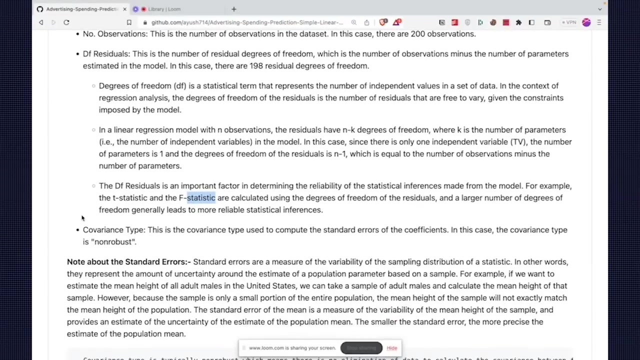 so what exactly this does is represents the number of independent values in your data set. number of independent values. okay, this actually helps in calculation. this actually helps in calculation of t statistic or f statistic and a lot of other way. but this is what the df residuals is. it's saying their df residuals is nothing but your 198.. okay, so covariance type. 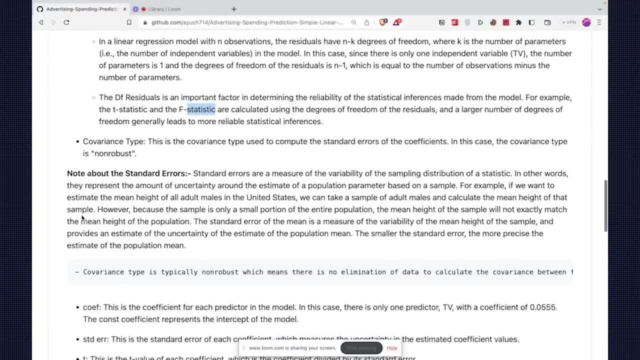 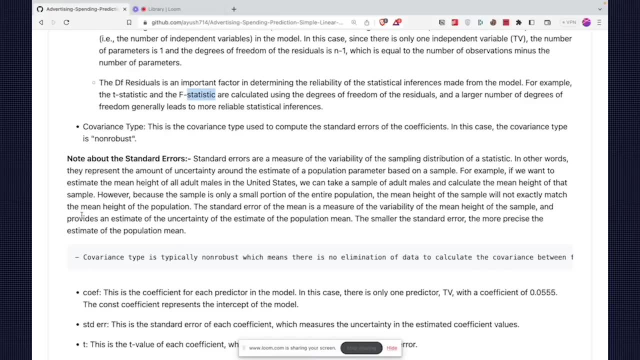 so what is covariance type? covariance type over here is nothing but, uh, non-robust. we'll talk about that. what does that? what does that mean? what does it mean? but the covariance type is the type of the covariance used to compute the standard errors of the coefficients. 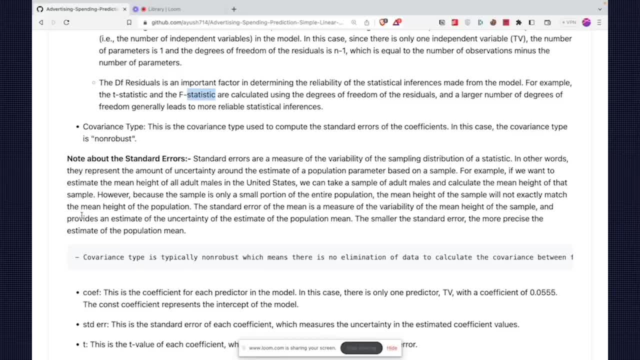 again the blah, blah, blah. it's really difficult to understand, but i'll i'll explain in a nice way so that you understand it. so, over here, what is it telling that your standard matters first of all? what is standard errors? we have all dropped the other. how efficient, how efficient or 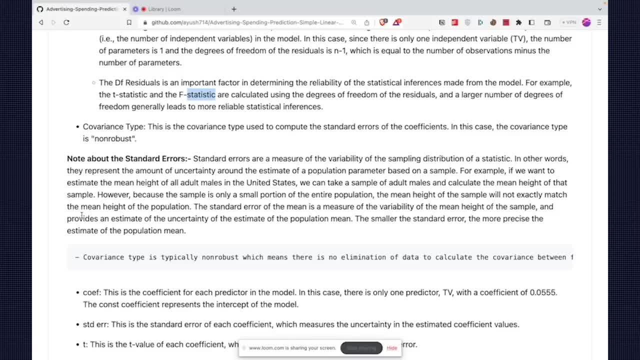 accurate or how reliable our coefficients are for example a very nice example which was which we'll let me'll have to go to so what standard error we have the standard error what does it tells it tells that the measure of the variability of the miles � porc with respect to the 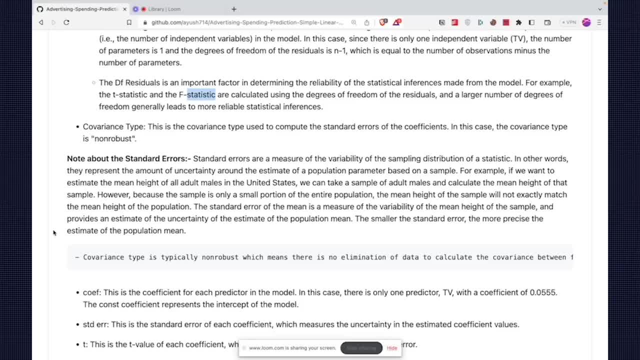 population, population. right, we're here for the population mean height of the human adult males means the population of equality is quite limited. or, you know, we cannot calculate the sample ofthe population of audience male, for example. this is a die hard ability of the height of the sample which provides what is the? what is the? it provides an estimate of. 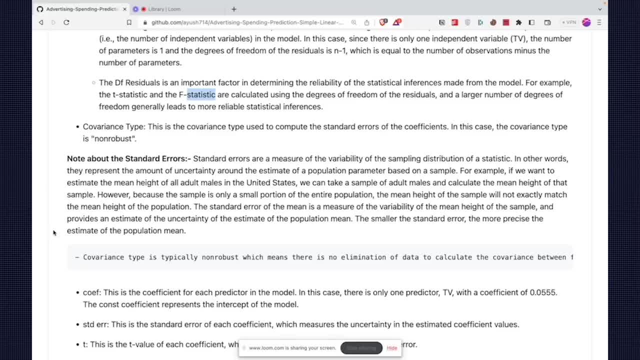 the uncertainty. so how much we are sure about how much our sample mean is accurate, how much the sample mean is accurate according to the population mean. so smaller is smaller. the standard error is more precise, the estimate for your population estimate. so you're based on sample mean, you're predicting the population mean, which means that we're using- uh, we are, there is some. 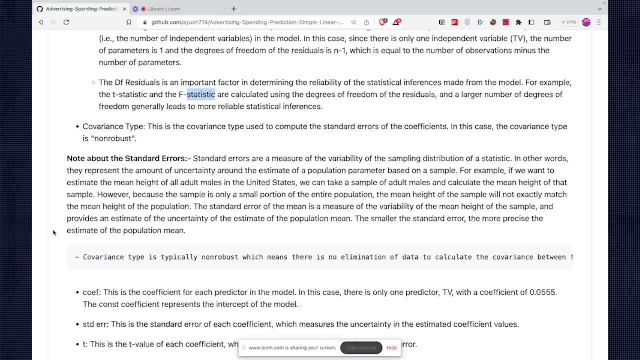 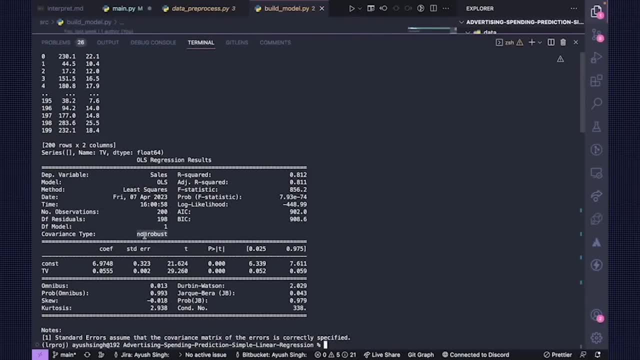 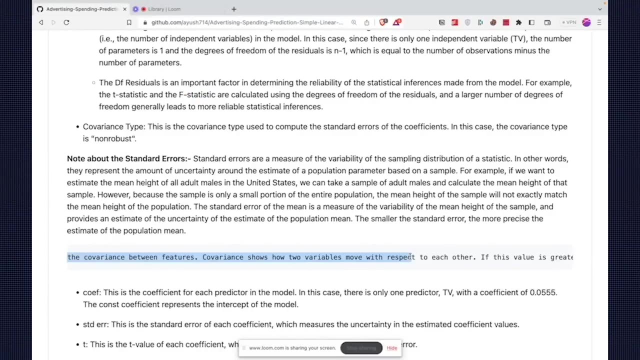 sort of standard error switch. does that okay, how much precise we are in getting the population mean given? we have the uh sample mean and in this case covariance type is non-robust, which means we calculate the covariance of our matrix without any el elimination of the data, without any elimination. 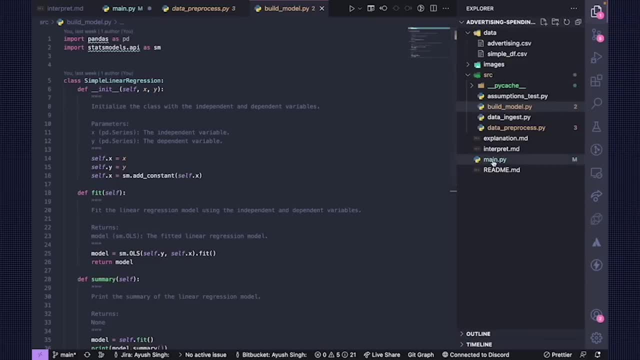 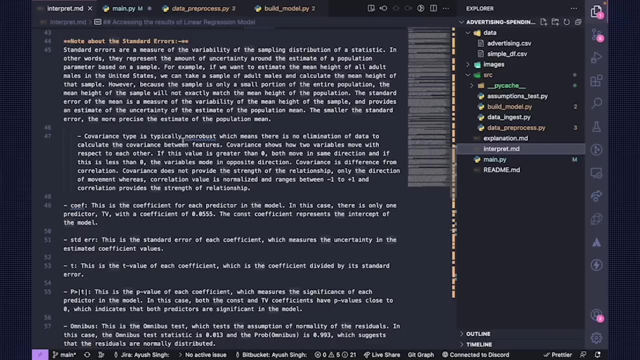 of the data. so what exactly does this tells? what exactly does this says? i'm just just going to go over here and then tell you about that. so over here, if you read, read this out: it's typically non-robust with the standard error switch, which is the data analysis. so it's typically non-robust. 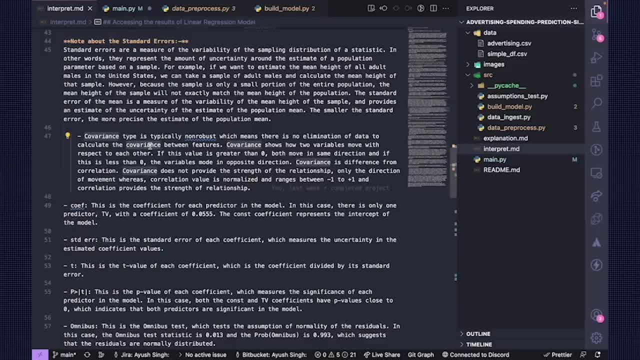 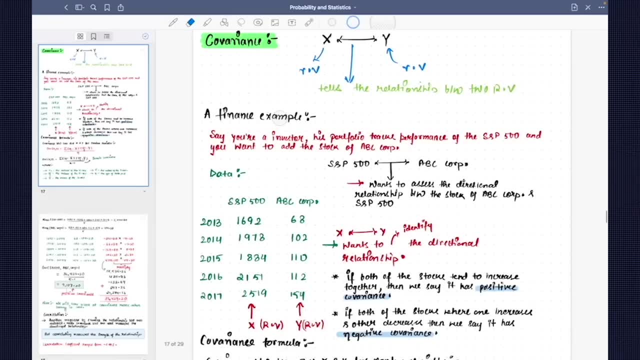 is no elimination of the data to calculate covariance between two features. but what exactly covariance is? covariance is a nothing, but it tells you the relationships between two random variables. so, for example, you have two stocks, which is s p 500 and abc corporation, you're going to assess 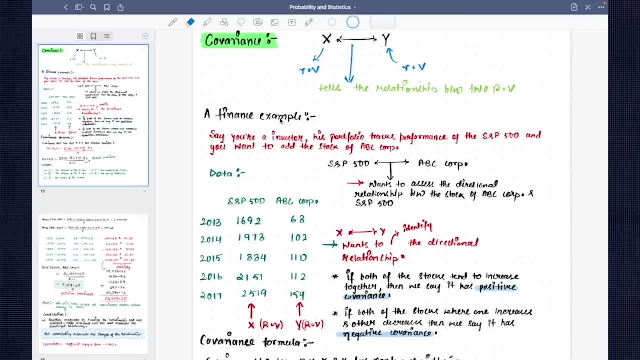 the directional relation. what is directional directional relationship? so if sp is increasing, what is happening to abc corporation? so what is the covariance between sp and abc? so it tells either one is squeezing or one is decreasing. so basically, this is the data, is an example, and it's x random variable and so y random variables over here. both are increasing that. 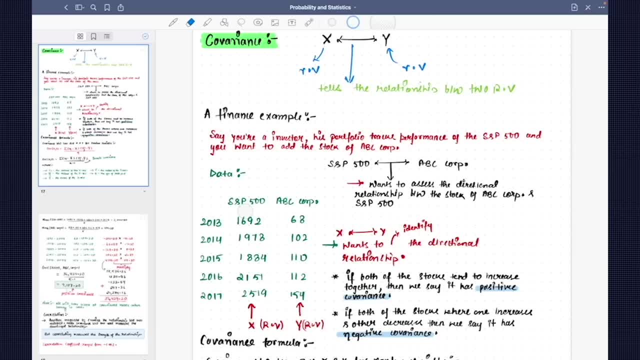 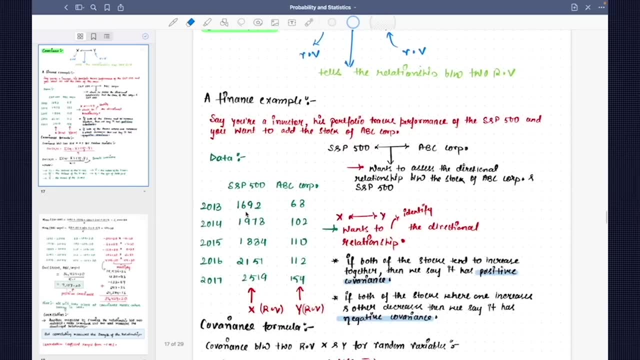 means they have a positive covariance. this one: it tells you the direction of the relationship, not like, if one is losing the word, then what is happening to another? so if both of the stock decreases, then we have certain certain things. so that's what the covenants is. it tells you the 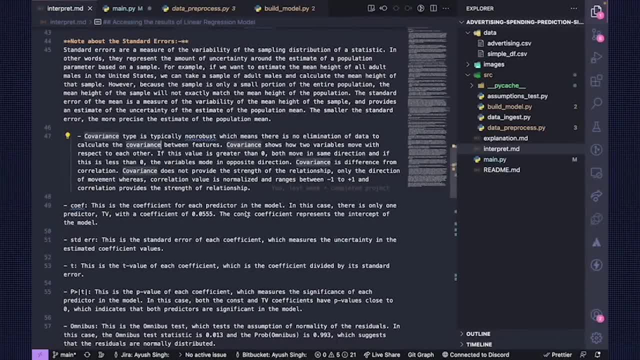 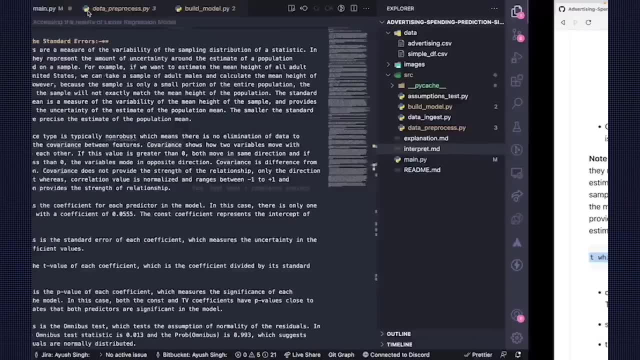 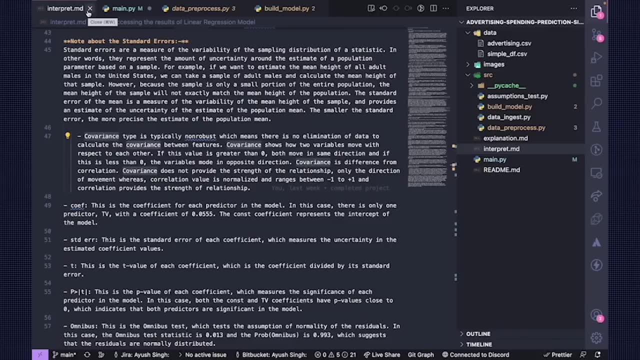 relational. uh, it tells you the relationships between two random variables. okay, uh, cool, so i hope let me just just ensure that. uh, yeah, it's running cool. so covariance shows two various between, uh, how they move with respect to each other, and blah, blah, blah. it just tells you about everything over here, okay. 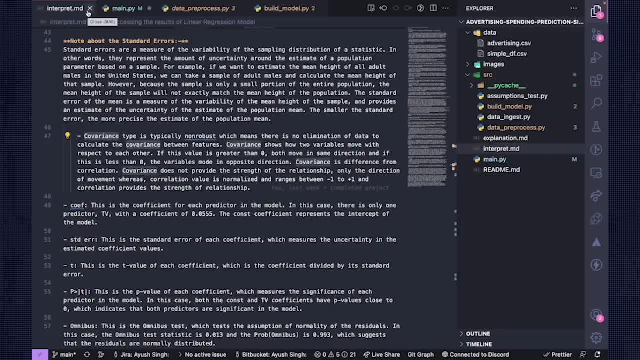 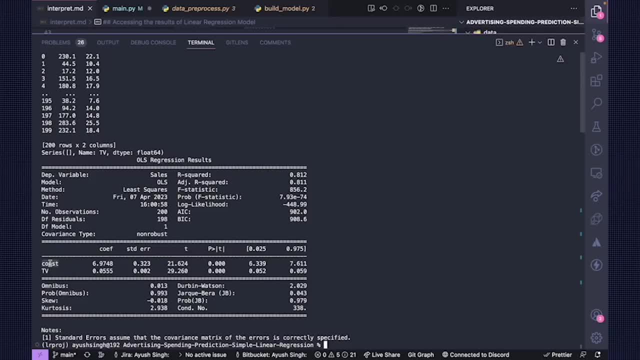 uh, no, that's non-robots, which means that we don't eliminate any data. okay, which is most commonly coefficient. so coefficient is coefficient is nothing, but coefficient is nothing but for constant, which is the bias term, which is beta. 0 is 6.978, which is the average. when x is x is equal to 0. 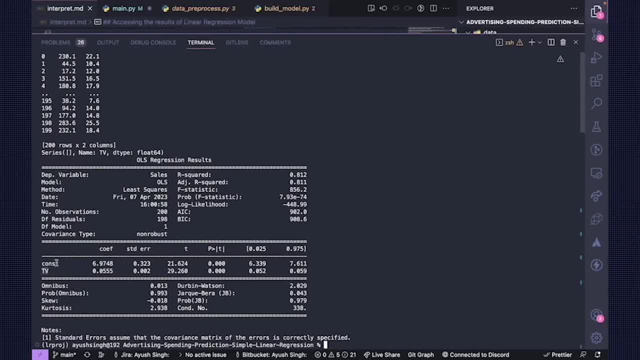 and dv is 0.00, 0.055 and constant for the santa. error for the constant is 0.323, which is how reliable, how reliable our, our constant or or the our, how accurate or precise our estimate is for bias term and how the estimate. 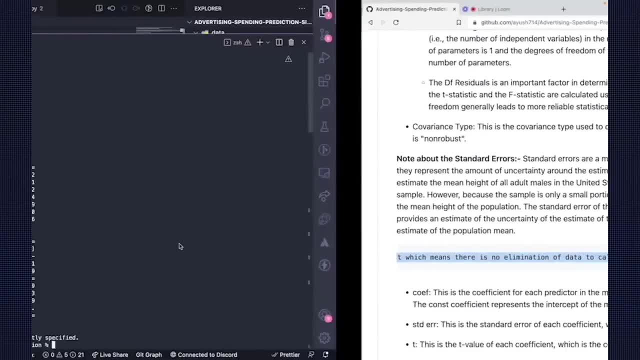 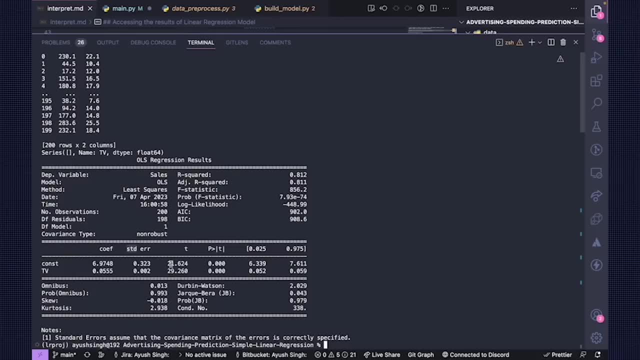 how good i estimate for tv, which is pretty much very low for both of them. and then you calculate the t statistic, which we had a talk, which, which, which we had a talk, which is t statistic, which is okay, t statistic for constant, like how? because these statistics, what is it? it tells you, it tells 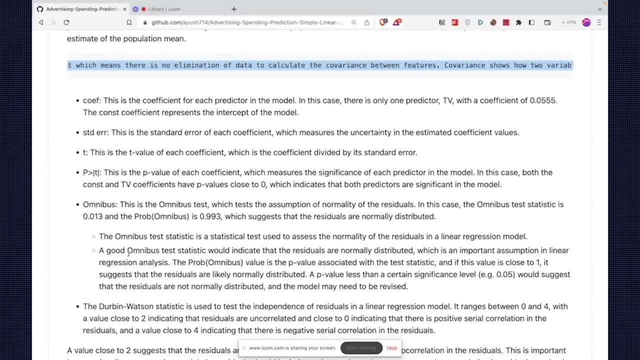 you the a sig, the, the significance of the individual parameters. it, it tells you this. it it tells you for individual parameters. okay, so we just calc, which is calculated by dividing the coefficient by the standard error of that coefficient. so how? so? basically that's the t statistic. now what you do? you compare that t statistic. so this is the. basically you have the. 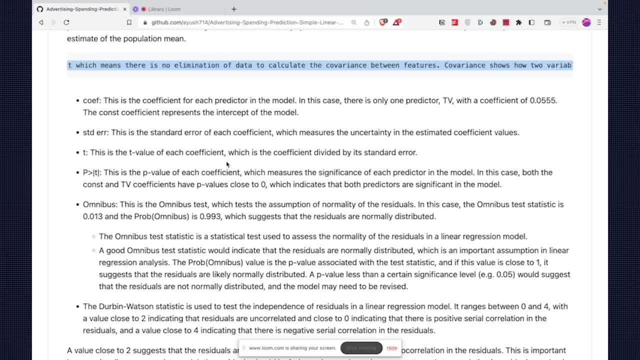 p value: uh, you have the p value for each coefficient which measures. now, if, uh, and you can see that both of the p values, uh, both of the p values are close to zero, which means that they are, that they are pretty nice, you know, they are less than 0.05 and they're both significant to the 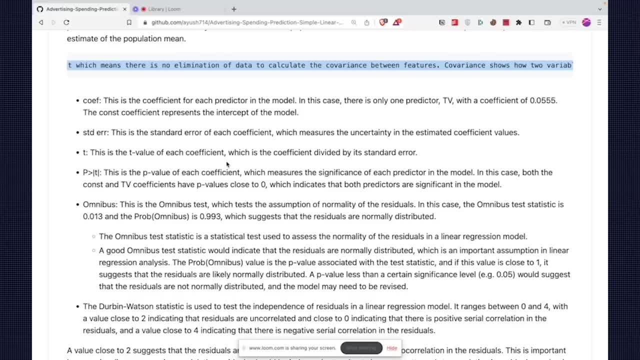 model. okay, we have omnibus test, which tests though now, now, now over here, we are done with a couple of things, which is the testing significance of a model. now, what we do? we have the omnibus test. what exactly omnibus test does? it tests us, though we have a assumption, which is normality assumption. 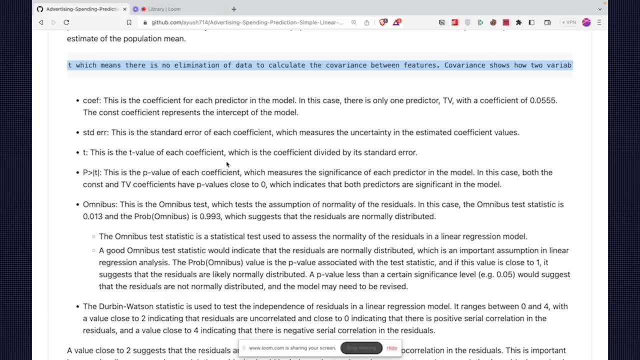 in a linear regression with tests, whether our data follow our residuals are normally distributed or not. so omnibus test statistic gives you exactly uh helps to validate the assumption. that's why i really like stats model api because it tells you everything which you need. you don't need to. 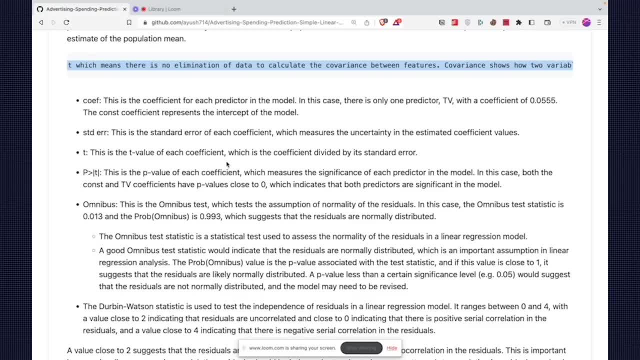 calculate further on. so omnibus, test statistic, which gives you 0.013, and the probability which gives the prop, the p value which is 0.993, which suggests that residuals are normally distributed. how can we say that they are normally distributed? so over here, which you, which, which, which you can. 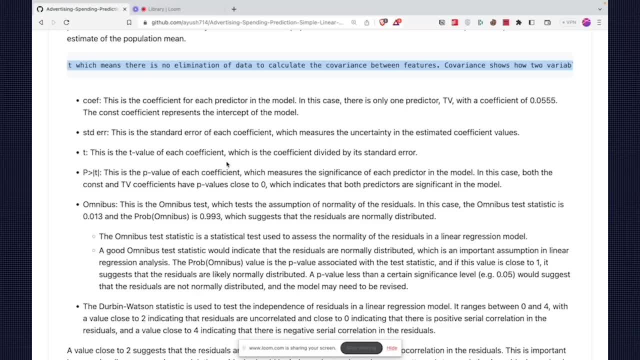 see the, the, the, the probability, the probability that you get, the probability that you get, the probability that you get the value, the probability of omnibus value, is the p value associated with the test statistic which was calculated. okay, so t, t statistic, you know t statistic which we can calculate, and other things. 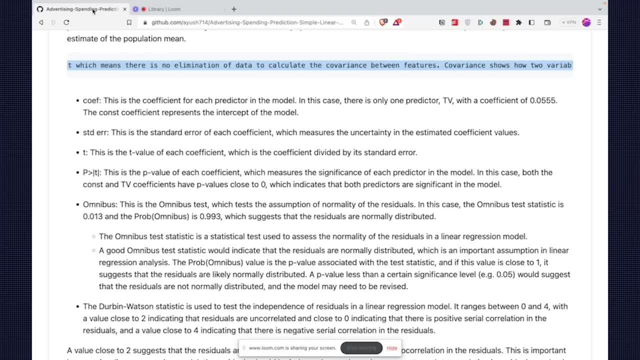 so over here. the probability common omnibus is the if, your, if your value of the prop, the probability of omnibus value test test, is close to one, that means are likely normally distributed. and if they are less than that they are if they are less than 0.05, which means they're not normally distributed. 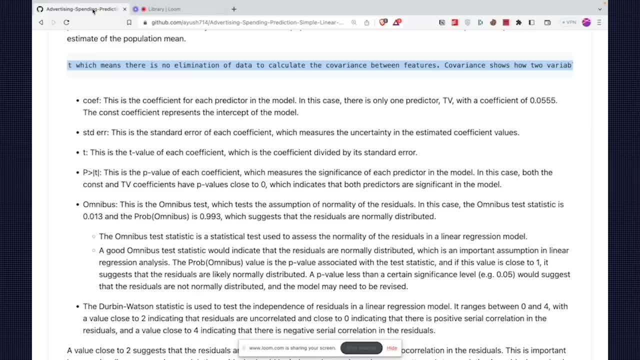 right. so over here, which is 0.993, which means they're close to one, that means they're normally distributed. another one is durbin watson test, which was used for testing the independence of residuals, whether one into one. one error does not affect the another which we had a talk, so it usually ranges between 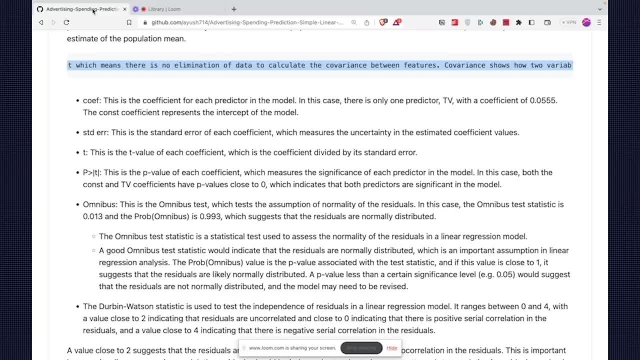 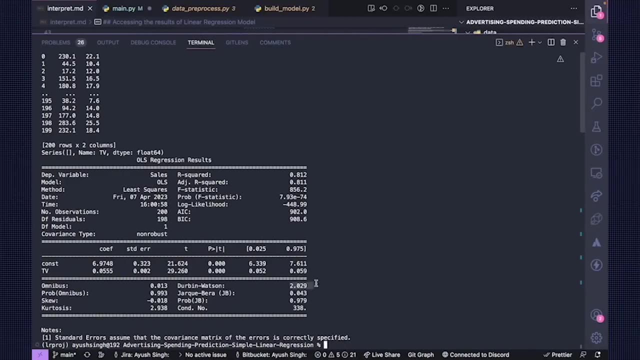 zero to four and the value indicating two, which means they have, they follow the assumption, but less than they are, you know, uh, positive, and greater than they are, greater than two, they are negative. correlation, right, so, um so, uh, but so in this case, your durbin watson test is around two, which means that they also follow the 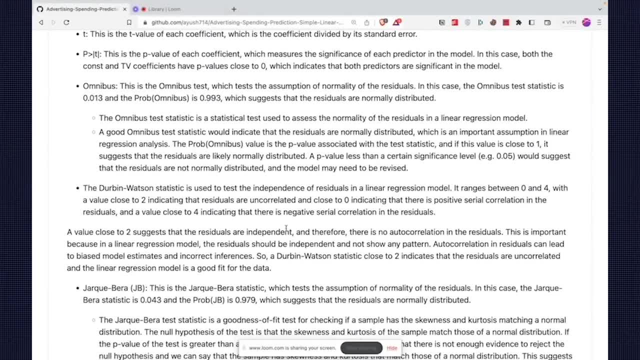 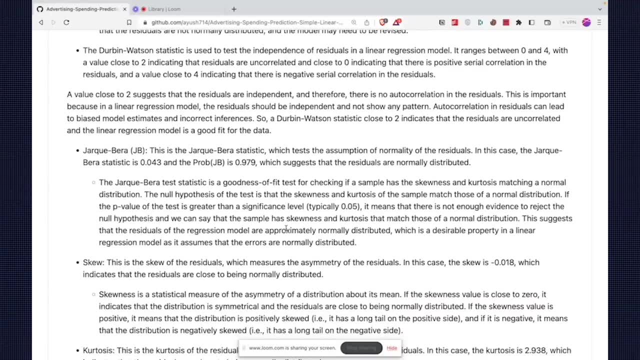 independence assumption- now we don't need to check for too much- and then value close to- as you can see that you can uh read over here. and then we have another test, which is another again for normality assumption, which is jarred beta test. you know there is a lot of pronunciation. 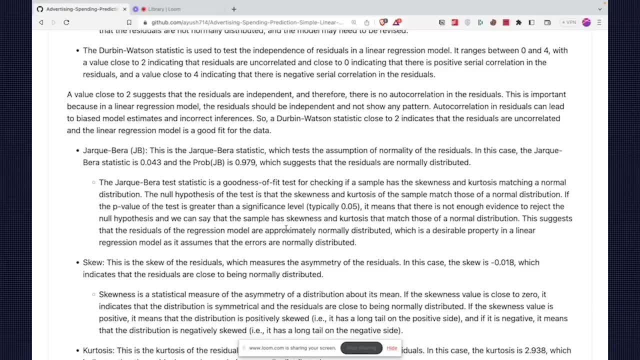 uh, for the same, like harik beta, you know jarred beta, so depends on what you use. so you, you have another test. you don't need to understand how exactly the mathematical working works. that is, it's just for statistics purposes. so which tests assumptions of a normality of the residuals in 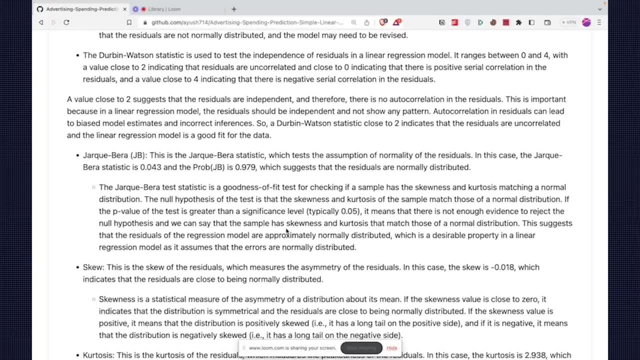 this case your beta statistic. as you know, first, first you have a t value and then the critical value, right? so first of all, calculate the beta statistic, which is this much, and then you calculate the probability of that which is from the table distribution, which is 0.979, which says: 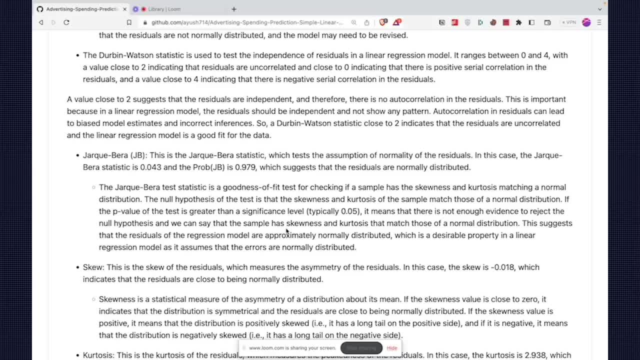 that residuals are normally distributed. what is the probability which is the so so, so that we have the problem, so that we can compare with the significance right alpha value. otherwise, how can you compare this? this is, this is not a property. convert that to a probability. so we suggest that. 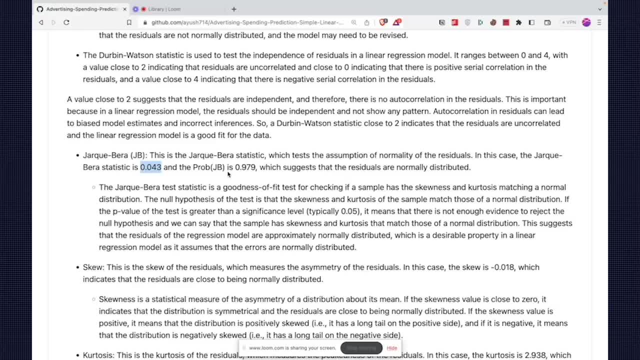 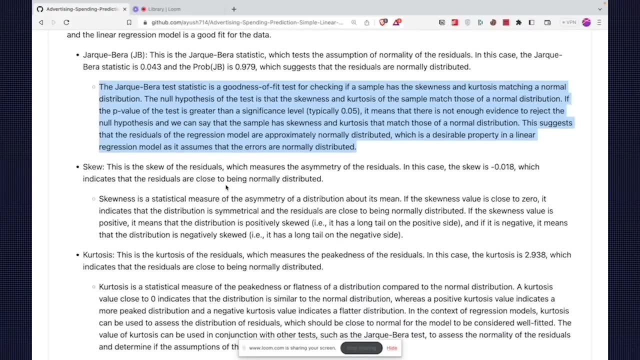 the residuals are normally distributed. how can we say that you can read that? how can we say that we have actually written you everything which is over here? uh, that that also test suggests. now, now you have skewness. skewness means that skewness means. so how can i explain your skewness? skewness is a. 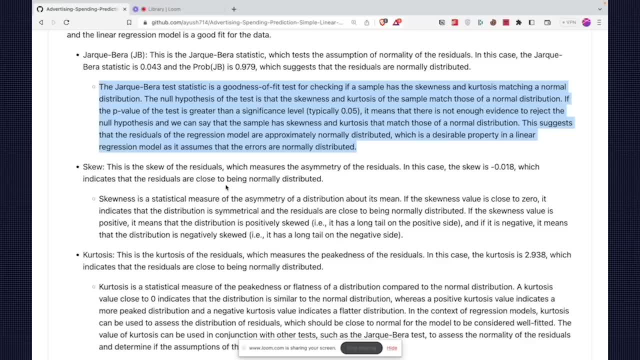 statistical, you know, uh, i think that if you have to enroll in my course for learning about all of these things, but, but basically, um, but, but basically, skewness means that a skewness also suggests some normality assumption, okay, uh. so basically it also also helps to calculate our normality. so over here, in this case it's minus 0.08, which means the 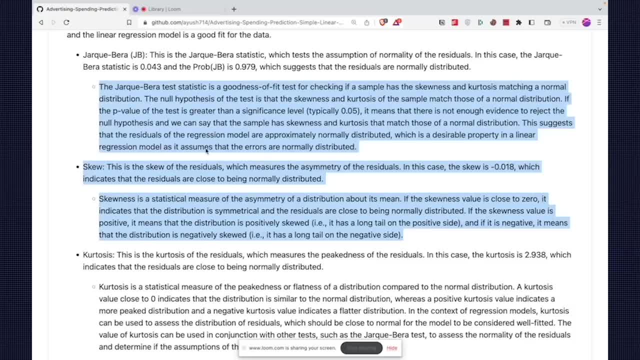 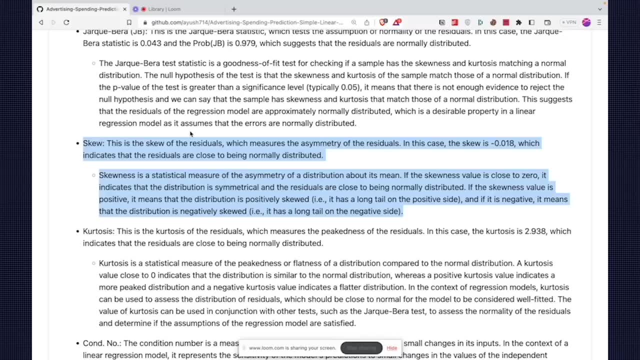 residuals are close to being normally distributed. i suggest you to you know, have a look at in detail about skewness and couturis, because this is something which you have to and it would indicate the valid validates our normality assumption over there. but i suggest you to 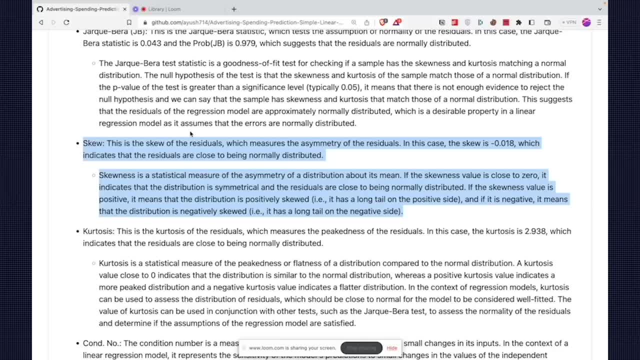 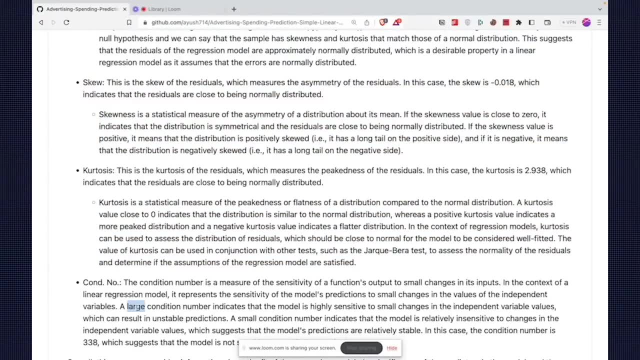 explore by your own, because something is takes a long time to explain. that is that, that that i explained in my probability course. okay, cool, and this is the condition number. uh, this is not important, you can actually ignore, but actually condition number if you, if you want to know about, like, uh, and so you have a condition. 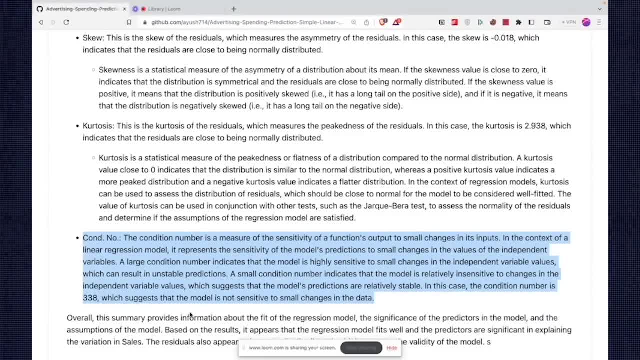 number over here. condition number: what does it state? it represents the sensitivity of the predictions, of the model predictions, to small changes in the value of independent variables. so how much your model prediction will change if you change the training data and then retrain the model? okay, so if you reach, if you change the training a little bit, and then how much that will? 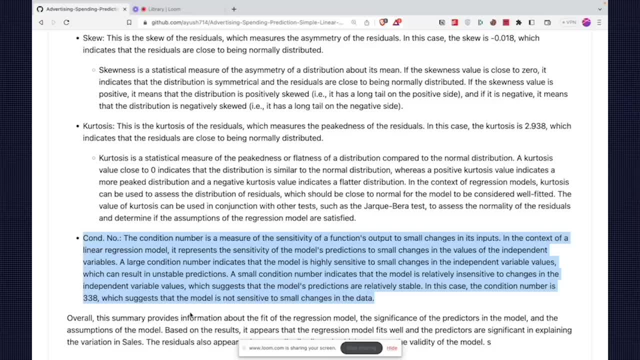 change, so higher. the higher the condition number is better. sorry, a small condition. small condition number indicates that the model is relatively insensitive to changes, which suggests are relatively stable. okay, so they're not sensitive. so basically, smaller condition number, which means that even if you change the data, your predictions will be remain stable. it will not drastically. 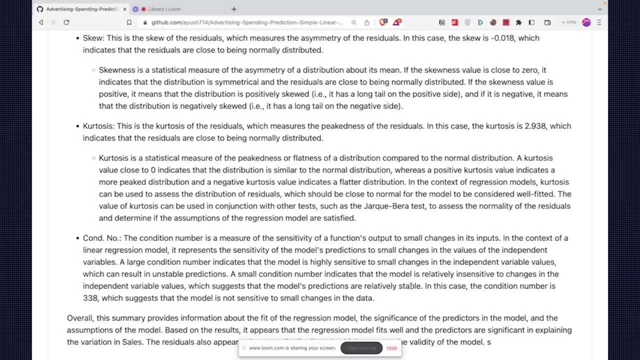 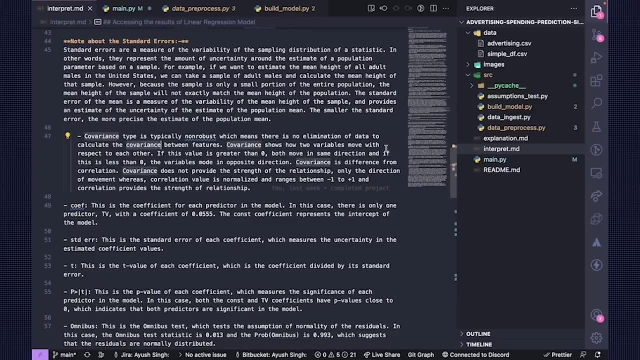 change. i cannot trust it. it will not drastically change, so i hope that that really helps. um, that really helps now. uh, hope that this. this provides a very nice explanation about our condition number and the summary of everything: now, what you can do now. you can have now now. now we have, now we are done with. 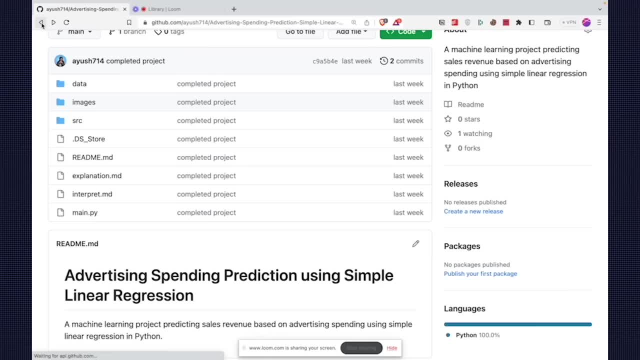 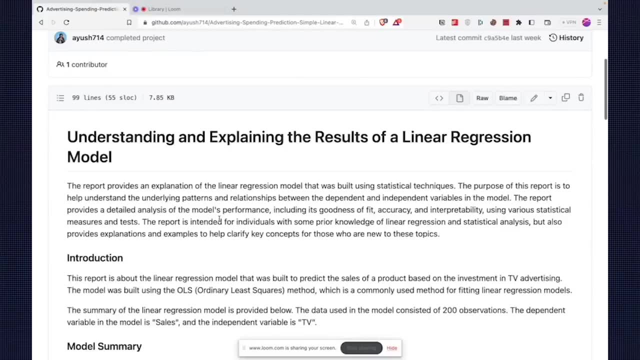 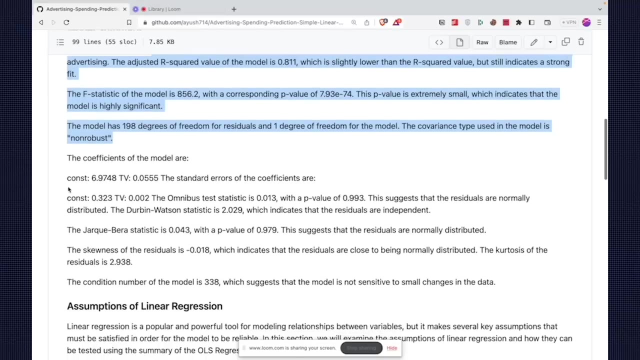 this interpretation. now you can actually go to something known as by your own, which is explanation, and explanation consists of everything which we have talked on a lecture, like i had. uh, over here again what exactly the report is. what is the small summary of the model over here. i've interpreted that. i've interpreted every the the important, you know. 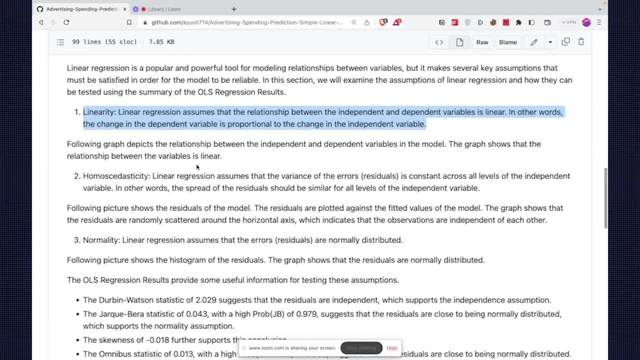 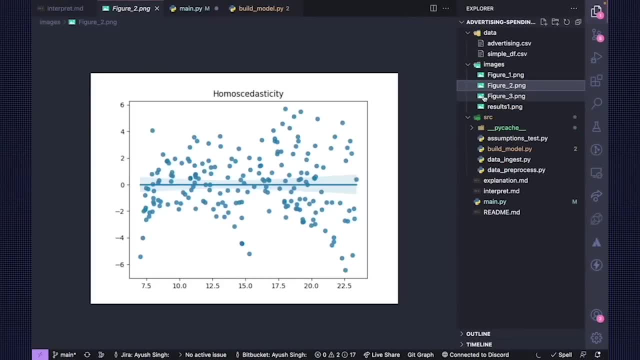 everything. i've also validated the assumptions. i've also validated assumptions. if you, you can also go on uh images and then see figure one, figure two, figure three and all which, which, which will give you a very nice as uh for for every assumption by your own. okay, if you want, you can actually tell. 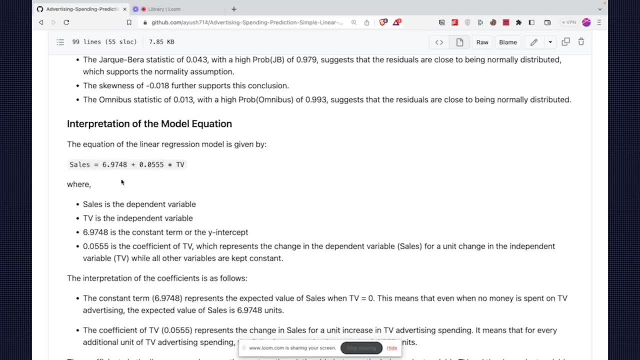 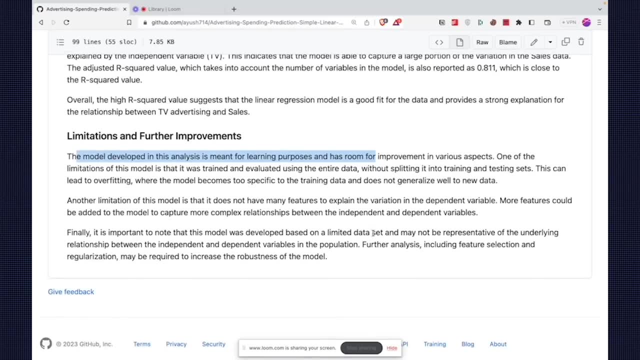 me in a comment box if you want to, if you want me to develop for it, but you can see that i have written a very nice blog for this, so that you don't need to worry about too much- and also, just what are the further improvements or limitations which can be listed out there for you to work on. 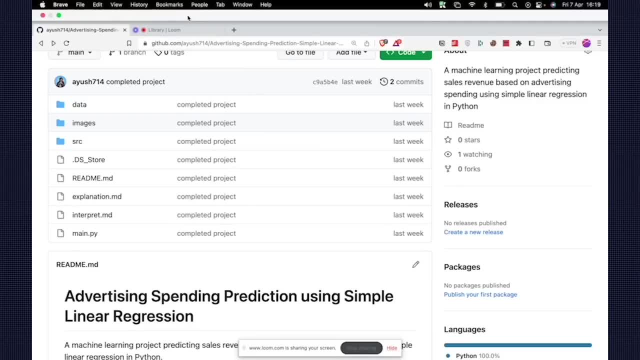 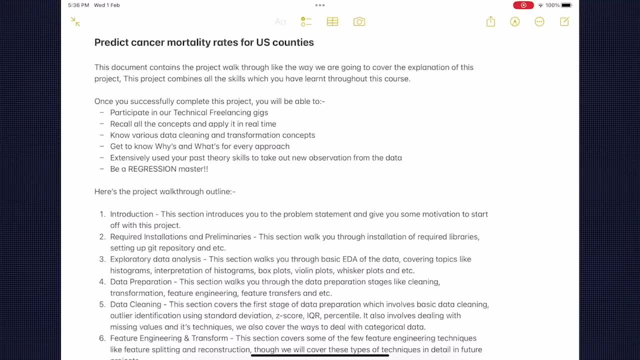 and that's pretty much it about this project. i'll be catching up the next project. till then, bye-bye, hey, everyone. welcome back to another lecture and section, which where we are going to eventually talk about one of the last projects for the midterm. so on regressions, on on regression part. 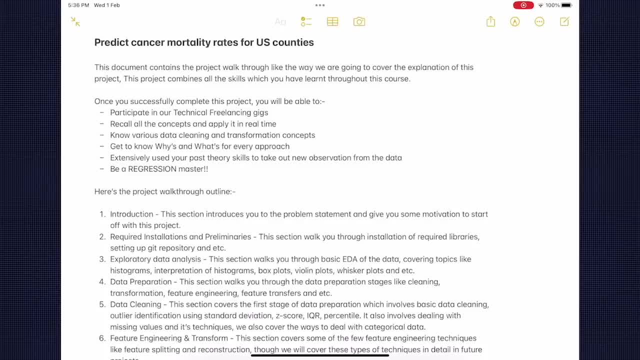 and then we'll move on to classification projects. so, basically, what this project indicates this: this project says that that in this, uh, in this, we'll try to predict cancer mortality rates for the us countries. right? so what exactly this uh, what exactly the problem statement is? 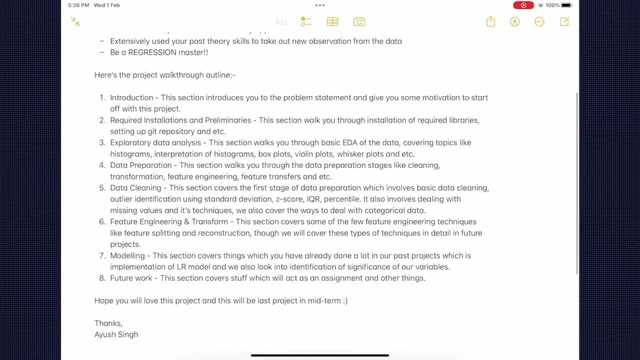 etc. so here's the walkthrough of the product which will go through it first. we'll start off with the introduction, which is this lecture. so we'll start off with the introduction lecture and then give you some motivation to start with it, and then we'll, uh, go through through the 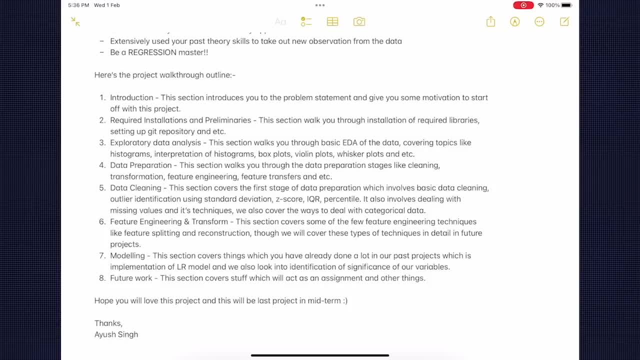 rick, what are some of the required installations and what is the virtual environment? setting up the virtual environment, setting up your workspace, etc. and then we'll go forward and i'm going to show you some of the things that we're going to be talking about today. 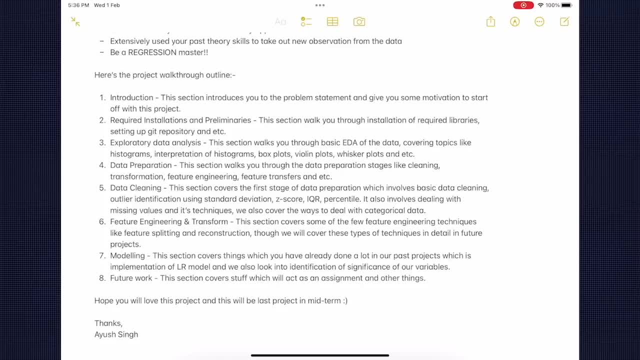 understanding uh exploratory data analysis. so in ex in exploratory data and analysis, we'll try to do some, you know, a basics ed of the data set and we'll try to understand uh more about the data and then after that we'll go through uh preparation of the data. what is the? 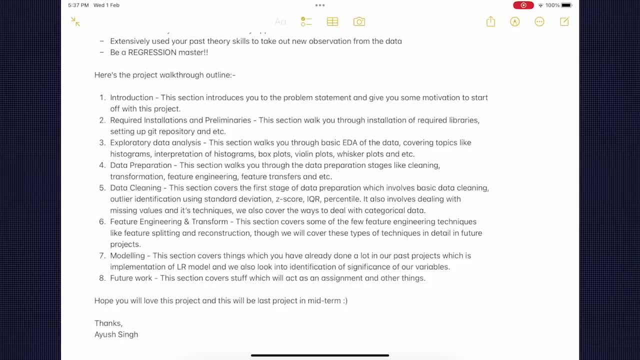 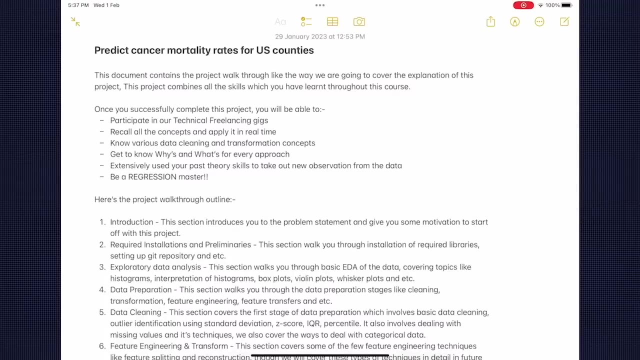 preparation of the data means, which means cleaning up and then featuring, etc. and then we'll model our work, uh, where we'll implement our linear regression model to predict what is the death rate for that particular country in that particular country, for the different different states. i hope that makes sense now. now, uh, what i'll do is uh, make you, make you, make you go through. 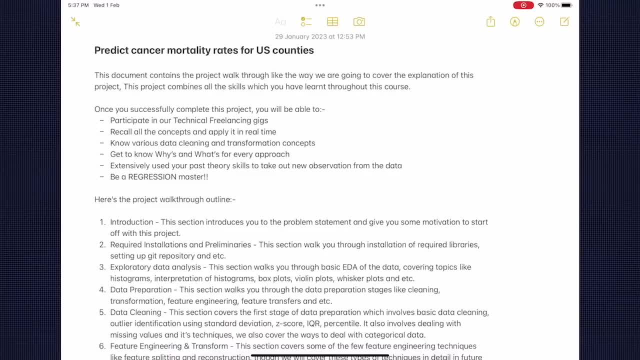 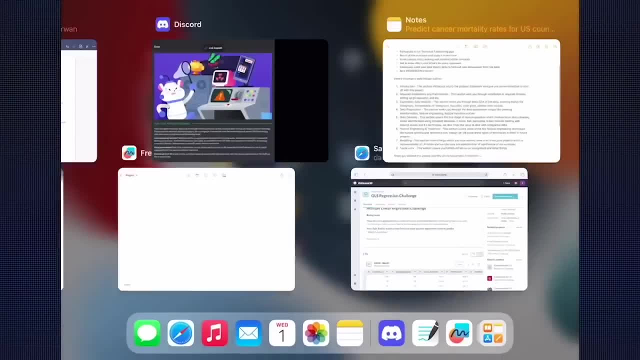 all the. the first part of this project walkthrough is introduction section where we let's talk about uh, what exactly we are going to solve in today's lectures. so basically you can go to the uh given link. so wireless regression challenge. so you'll be having the link in the readme of your 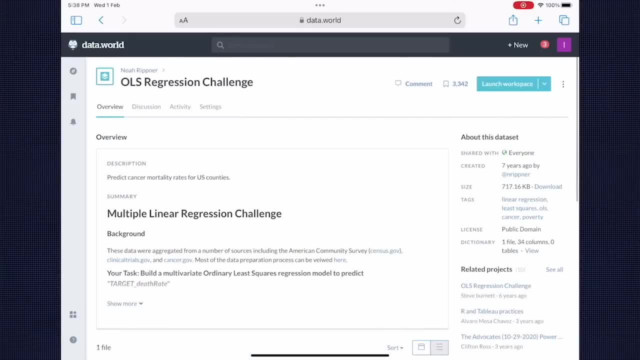 project and so if you go over there, so basically this is a challenge- uh listed by dataworld which is one of the good challenges which i've ever seen- and basically this challenge says that that you want to predict, that your task is to build a model to predict what is the rate of cancer mortality. 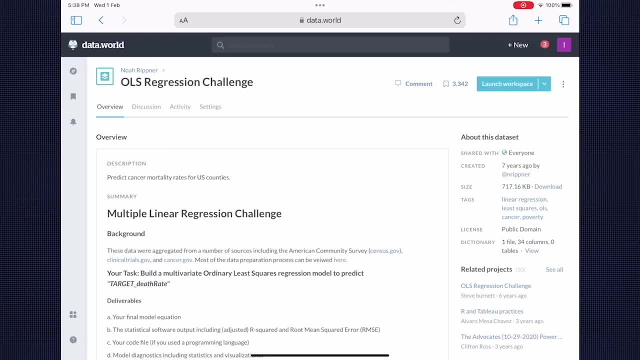 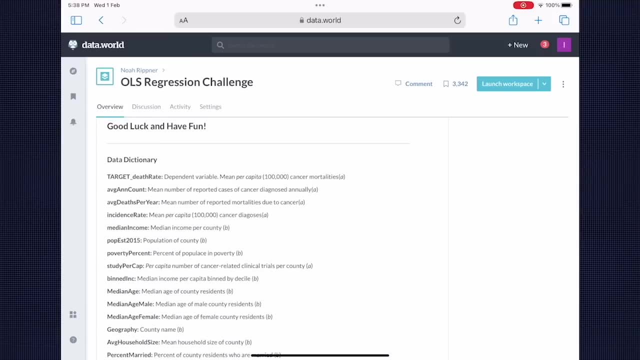 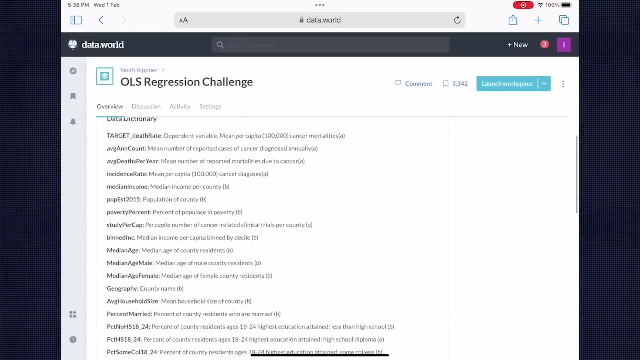 what is the rate of the person dying with the cancer for us countries? okay, so, if you go and see the data, so the data, the data dictionary, where you have several independent features and then you have one dependent features, so what is, uh, let's, let's talk a bit about on this, is you? 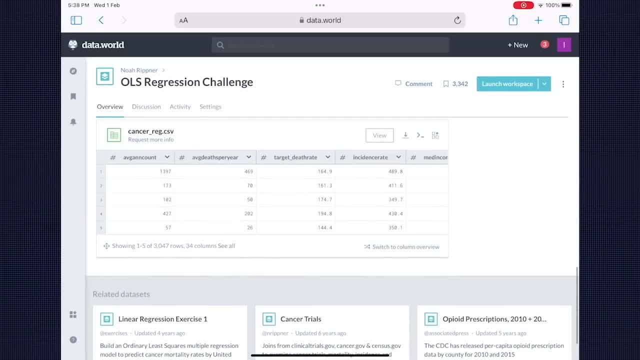 have the data dictionary. let's let me show you first of all the data. the data which you'll have is over here. this is the data which is which is in csv file. okay, so you have a total of 3047 rows and 34 columns in which, in which there is one column which is a target variable. so let's talk. 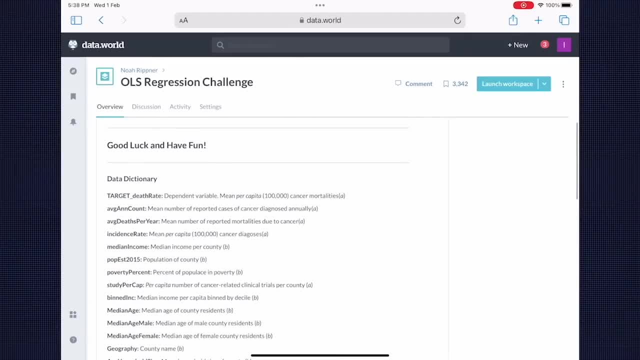 about what is which is the column, which is target variable, which is target death rate, with the target is the death rate, which is a dependent variable. it says that mean per capita. which is what is the death rate? uh, in per capita, which is 100 000 cancer mortalities. and then you have again the same thing. 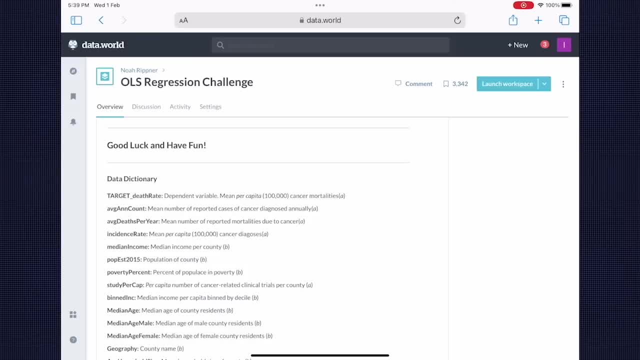 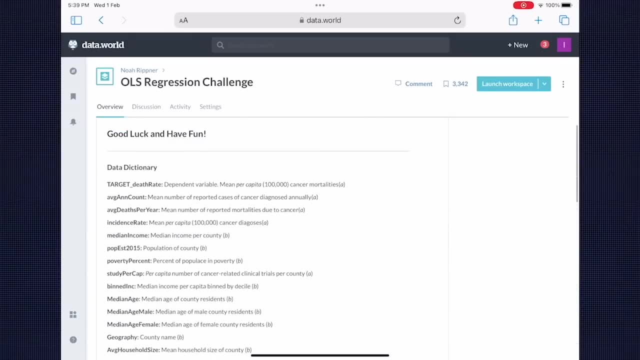 average mean number of reported cases of cancer diagonal diagnosed annually. so you have these features, which is average counts. if you go down you see average count and then you have average dates per year, which is mean number of reported mortalities due due to the cancer average date. 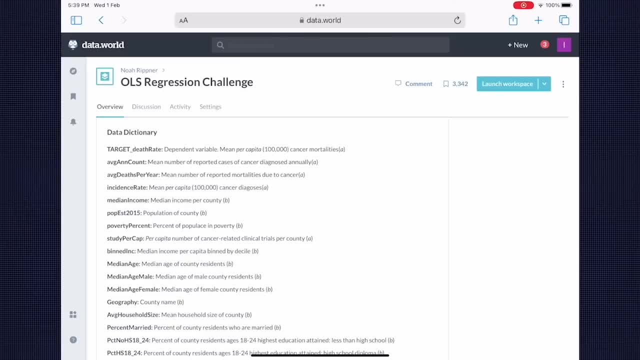 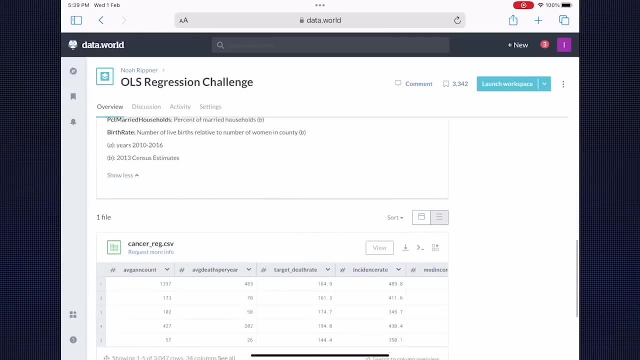 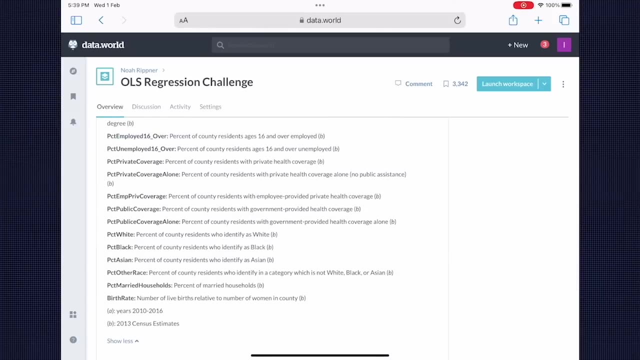 then you talk about incident rate, mean per capita and the median income per country. then you have population of that country, percent of population country. so you have the features out here. you have the features out here and every feature has its own description listed out here. so i 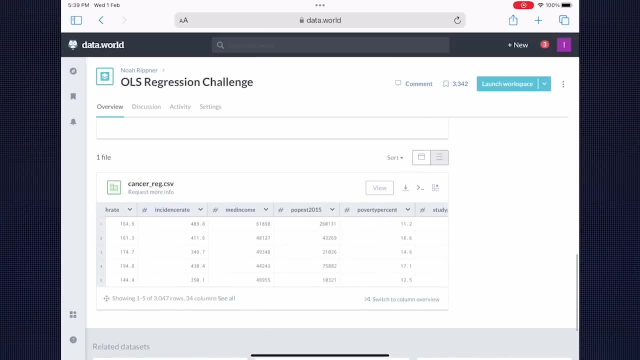 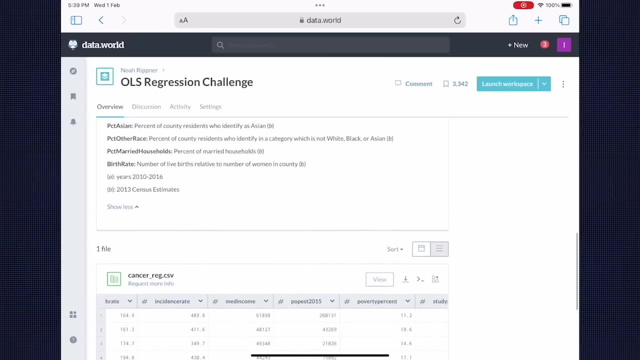 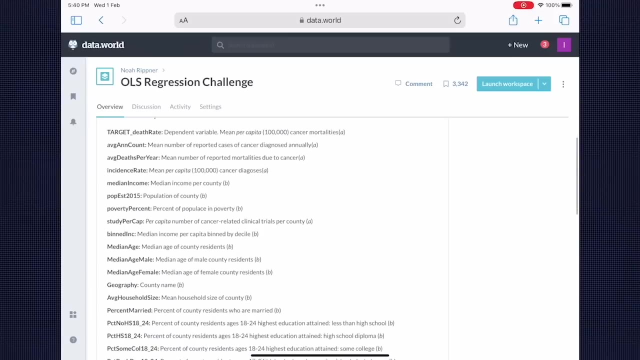 suggest, without doing anything: go through the understand every feature and try to first of all understand what exactly each feature is trying to tell you. okay, um, so basically the the the years of data it contains is from 2010 to 2016, and between that you have several number. 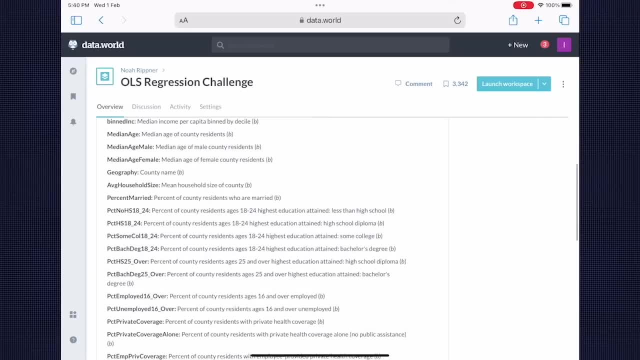 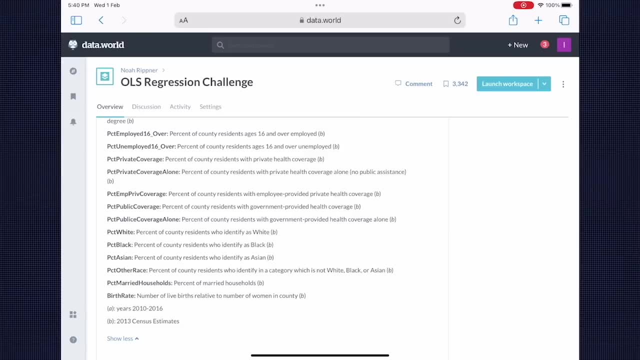 of information out there, right? for example, you can just go and see um some birth rate, which is the number of live births relative to number of country women in the country. which is the person of married households. person of country testing who identify in a category which is not white. so 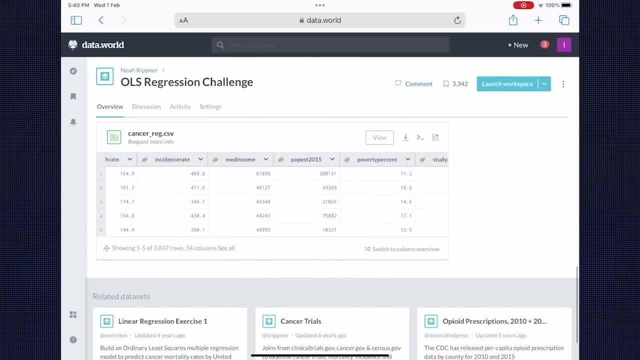 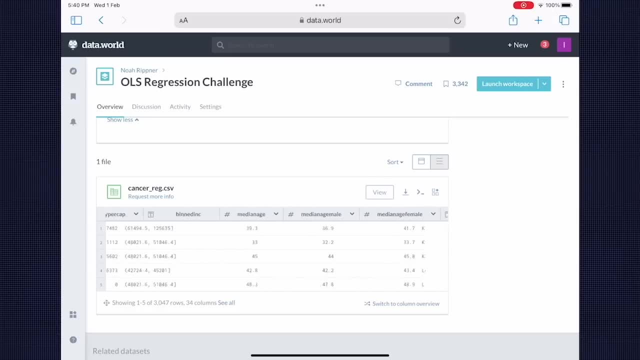 basically, these are the information for a particular observations. okay, so let's go with that example, so they'll be coming up later. but, uh, we will put the date first for each one of them. so if you've given them information for you, you have to predict the time they will show up, means when. 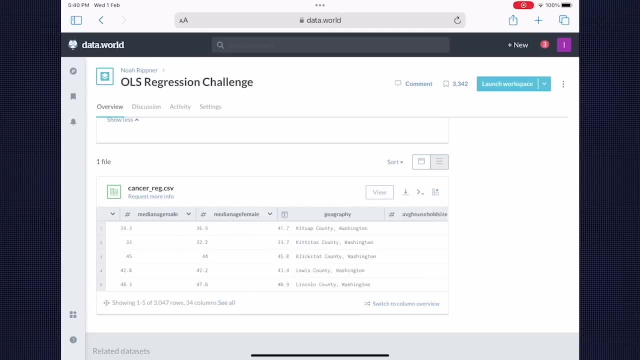 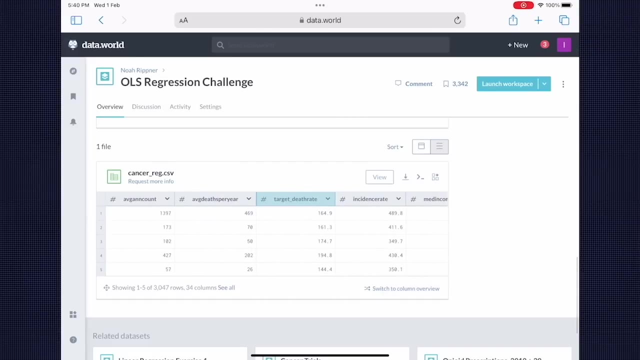 they will show up. um, then this is the time they will show up, or the time the test where they will show up means, because each one of them is using the same fruit, so you are able to take every condition and jungle examples, which means that you can Sk plague their data and then also you 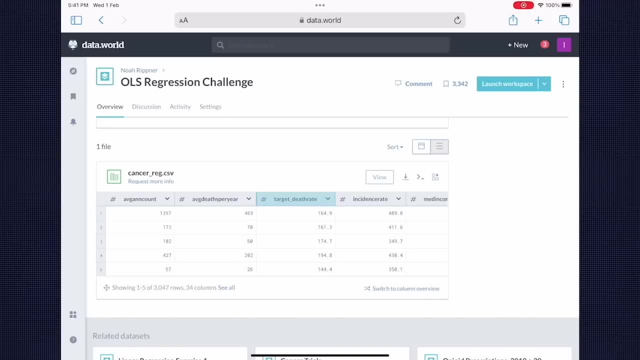 can predict the rate of death as well, so that is meant to be mentioned as one of the most important details. you need to have lerich on the screen, butterfield, where theうん ex represal, whereas here. so what exactly we will do? let's- uh, let's, go to this now, given the data. so, basically, we need to. 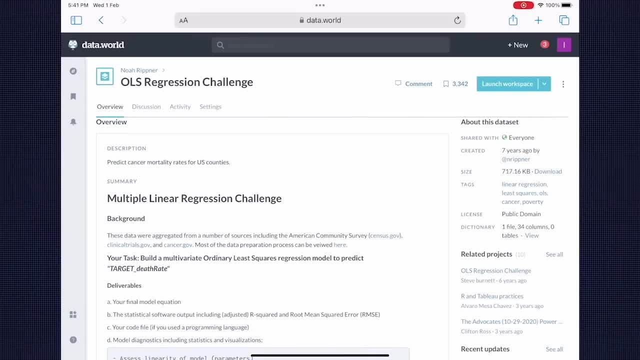 predict the rates. so, cancer mortality rates for the us based countries out there, right, um, which is nothing but how many people died? uh, we have to predict the death rate using of death rate which will happen, uh, using cancer, okay, with the cancer diseases. so build the task is to build a multivariate. 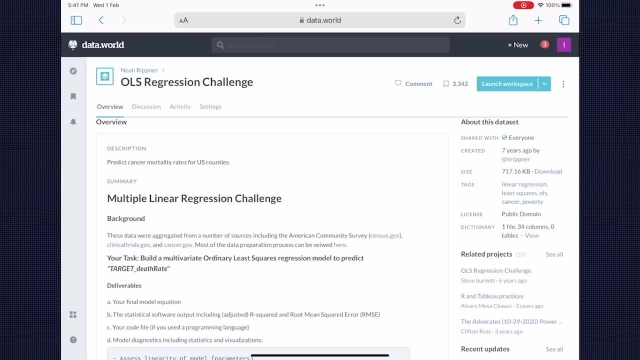 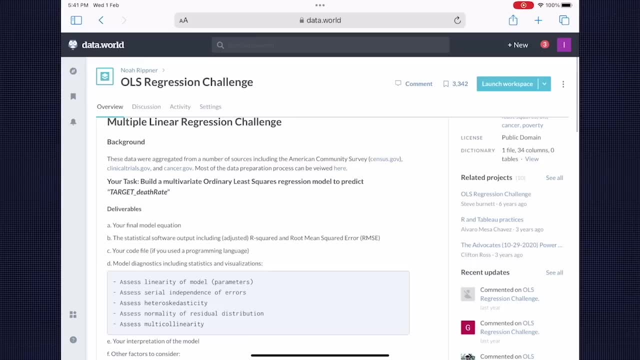 which is multiple, um, like linear regression model to predict the death rate for the us countries. right, so what? what should be the deliverables when, when you, when you, will complete this task? what should be your following deliverables, like what you're going to deliver to, uh, the task master? 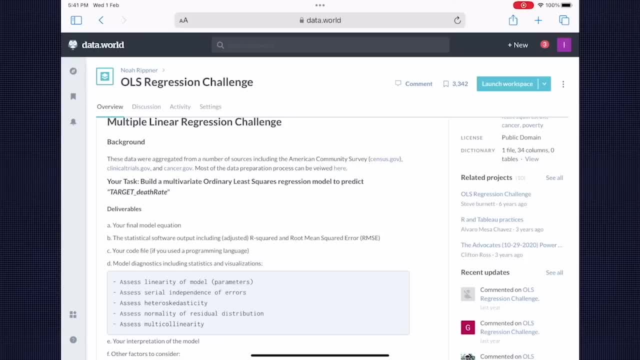 whoever is checking your assignment is: first, is your should be model equation. where you're, where you should have a model, you should have a statistical software. we are telling about r, square, mean squared, your code file and the model diagnostics whether your model follows the linearity assumption. independence. 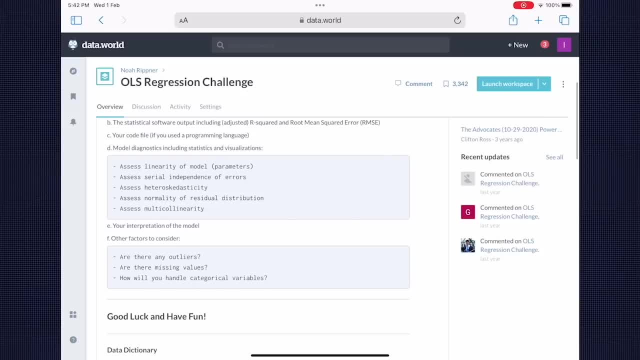 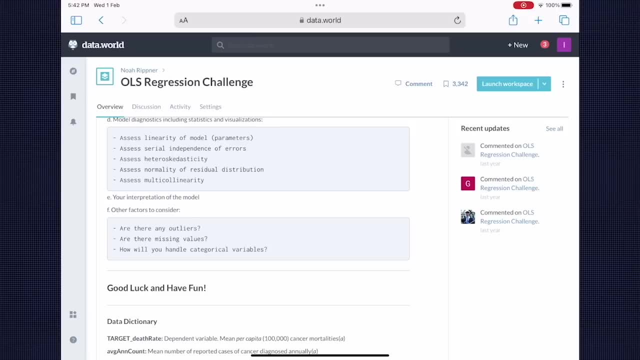 assumption, etc. and then your interpretation of the model, and there are other factors to also consider in this. okay, so i hope that this, this will tell you a lot, and now i hope that this gives you good sense about what exactly we have to do now. we, you- you may be thinking we'll be. 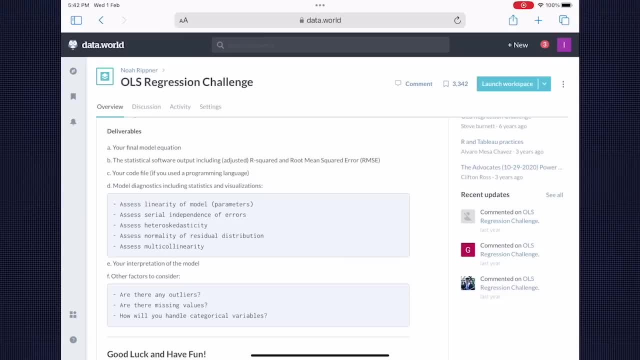 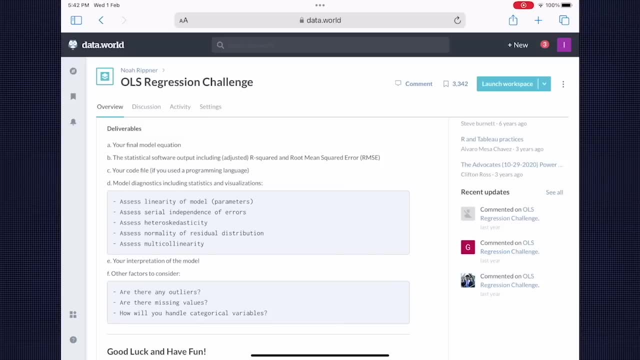 covering each and every part, as you might have already noticed that we have covered this part which is assessing them, which is model assumption test, as well as the evaluation part, so these two things are in your assignment. however, we'll do the big chunk of portion of this project to help you better understand mainly the data processing steps. 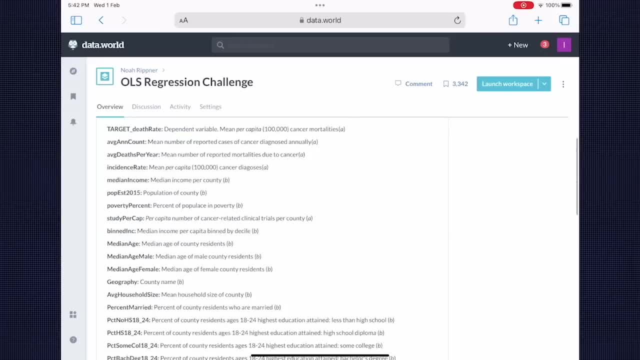 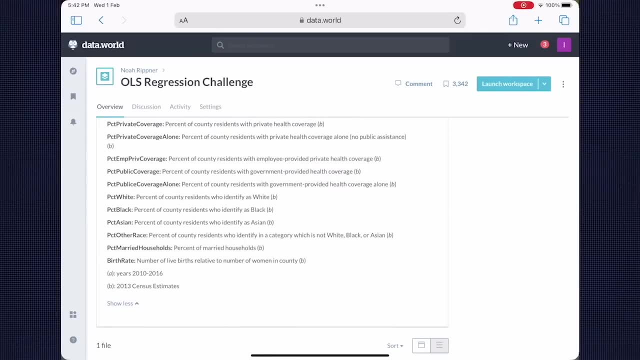 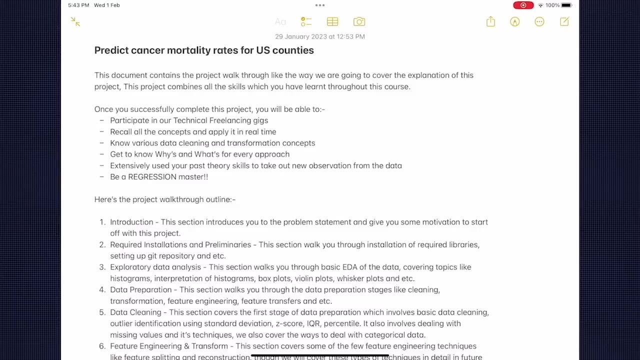 and all. so i hope that this gives you good sense about what exactly we are going to do. um, so, as i told our our aim, we have come. we have come. given you the short introduction about the problem statement, problem statement is nothing. we have to predict the death rate per. 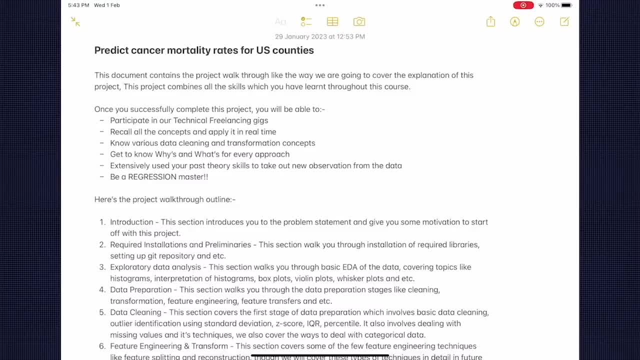 which is which? which is the death rate and what is the for using? which happened with cancer mortalities? okay, now, uh, you might have some issues like understanding variables. so here's you have to do if you're having a very high hard time in understanding cancer and whatever the independent 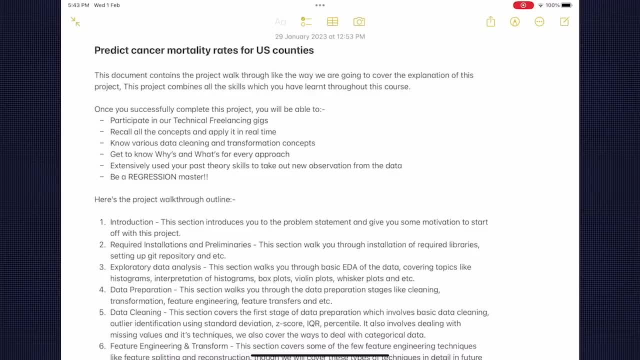 features, then i suggest you to search that particular term online on google, and then you'll be automatically understanding what exactly you need to do. right, but as of now you have to predict what. what will the death rate in that particular country, given that in that sort of 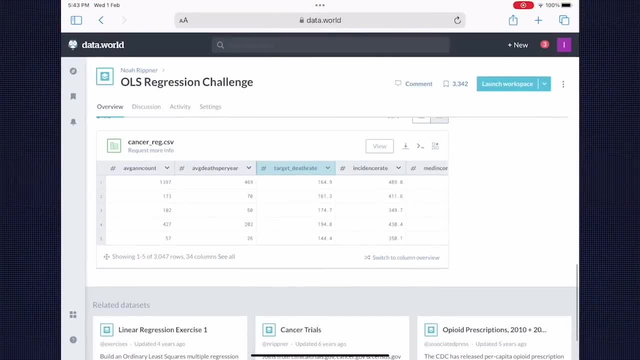 information. so, basically, if you go out here, if you go out here, you will see a geography in that geography, in in that geography, you have the geography as well as what. for that particular place and for that particular year, you have all the information available. i hope that this gives. 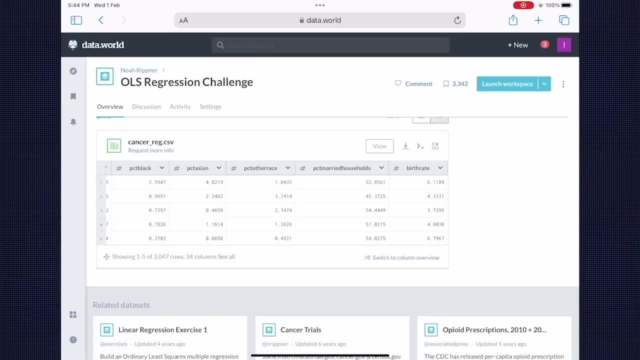 you a good sense what exactly the problem problem statement is now in the next set of lectures. what i'll try to achieve is i'll make- i'll start off with a very basic introduction of what is the require required installations which you need to do. what is environment variable? so we'll start off with the basic introduction to environment. 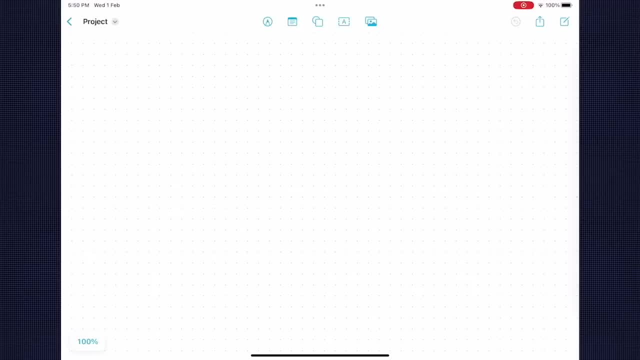 variables, and then we'll move forward accordingly. hello everybody. um, now we'll talk about one of the theory theoretical concept. today is a bit about on programming basis, but this should already be covered in your python if, but if you don't know, i i widely use this, uh, virtual environment, uh, in this. 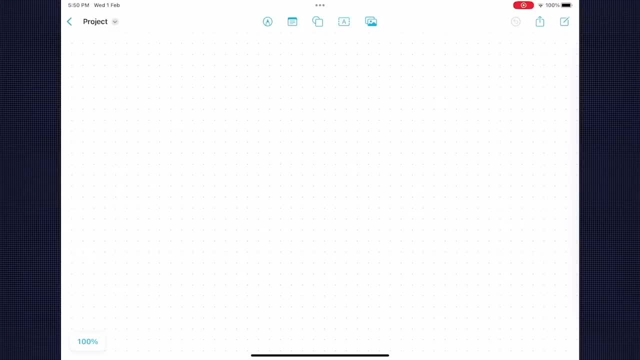 text. so if you, if you don't know about virtual environment at all, uh, this lecture is for you, maybe, uh, but if you don't know completely python, this, this lecture, is not for you. please, complete your python stuff, like in python, you, you're taught, you're taught in these, all these things. so please, 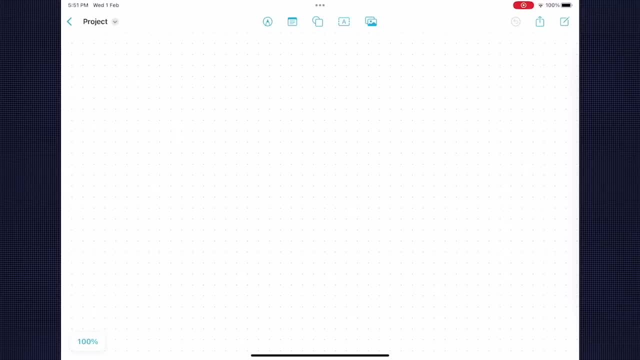 make sure that you have some idea what exactly these things are. but if, even if you don't, if you have basics of stuff not done, then you will be able to solve things up. cool, so let's get started. uh, actually is first, is i will what our agenda today to talk about virtual environment variables in python? 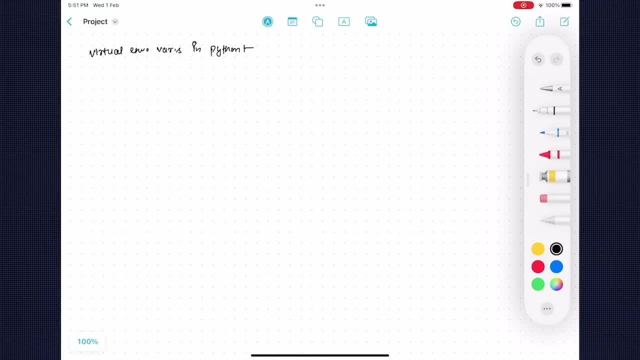 our agenda is to talk about this, especially in this particular lecture, and uh first of all. let's let's talk about uh. what exactly they are right. so virtual environment in uh is an isolated working copy of your, of your python version that allows you to install any sort of packages or dependencies. 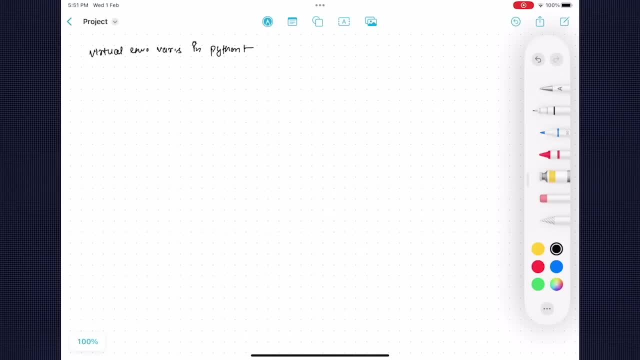 for a particular project. so i know it's something which is a very big definition. let's let's say one thing: you're working on project number a, you you're working on project number a and also you're working on project number b. project number b: you have a python, you have python installed, you have 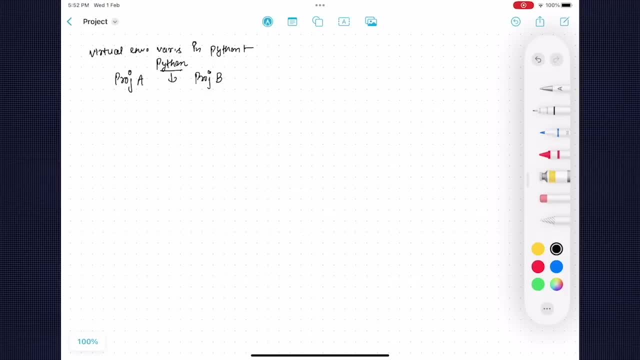 a python installed right, and then in that python you have several libraries installed, such as numpy installed, panda has installed, matplotlib installed, blah, blah, blah. so in that python version you have dependencies and packages are also installed right. and now, now, now, you, now, now you have this package packages in the hat, so your project a also downloads in your base version. you're in project a. 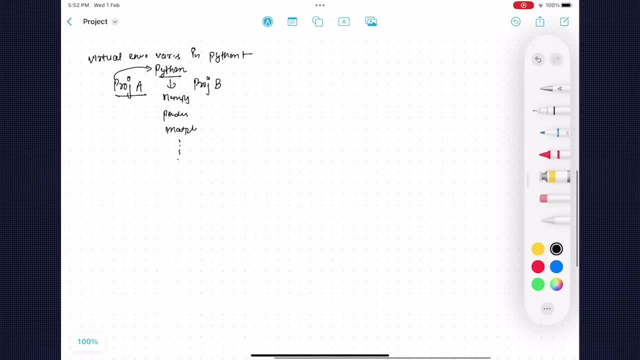 you download your whatever, first of all, download your packages required for project from these um which these, and every library has its own version, right, they have their v1, v2, v3, etc. and project b might also have the uh, some, some sort of similar libraries or different different packages installed. okay, but, but, but you 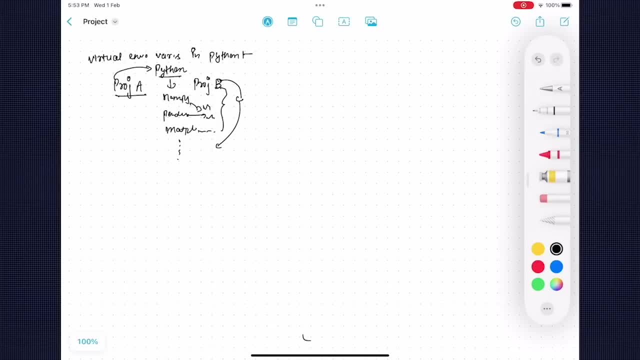 may be thinking: but over here. but over here project a is utilizing my. it might happen that project a might have different versions requirement, different versions requirement, and project b might have different versions requirement. right, that's one of the way to think about that. if your project a requires, if your project a runs on numpy 1.0, then project if project b works on. 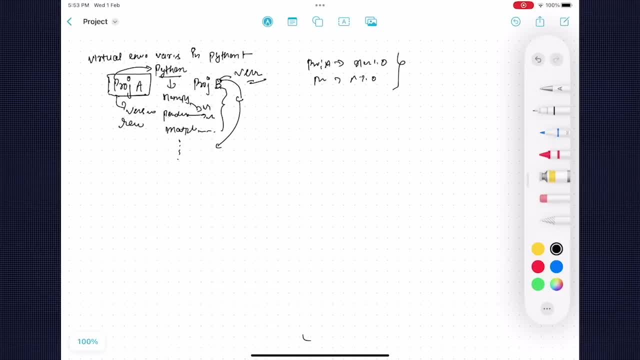 numpy 2.0, then that's an issue, right, you, you cannot uh run project b on that first library, right? on the other hand, you might be uh having questions like: um, so, so, so, so we need uh. so you, you might be thinking: key, how can we solve this? there's one way to solve this is that we can have 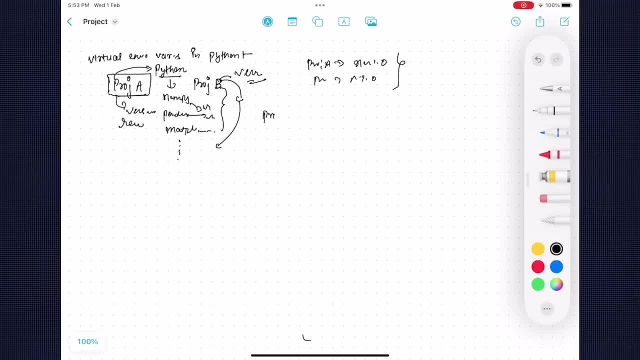 every project separately. so we can have a project, project number a. we can have a project number a with with its own python version, with its own python version, with its own libraries versions, with its own libraries versions, with its own dependencies, right? so, for example, numpy can be dependent on several other other. 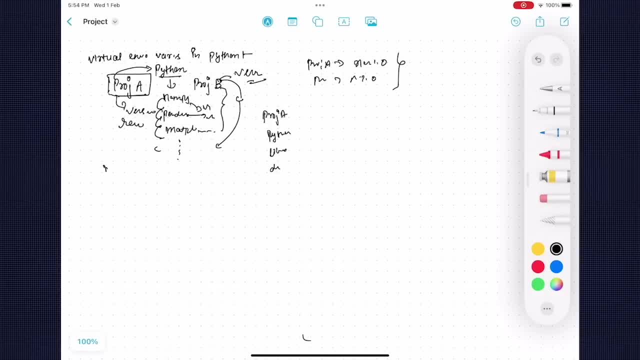 packages to work. right, so numpy pandas can be dependent upon numpy matplotlib. right, so a single library can be dependent upon several other uh packages. so one way to think about: why do we need, first of all, what is virtual? first of all the problem which that a particular project, project number a, might have different requirements of your python version. 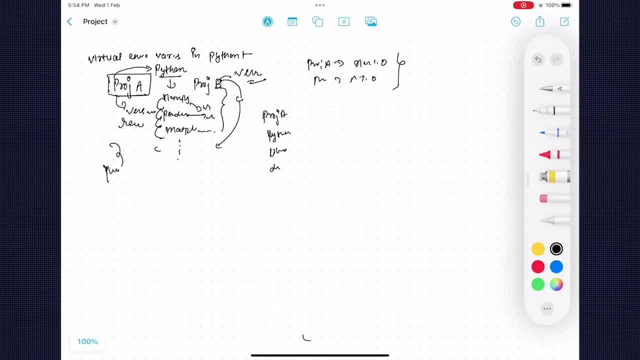 they require 3.8, but project b requires 3.9 and they might require several other other other set of versions of your libraries and maybe there that there might be different, different dependencies. so, for example, numpy can be dependent on pandas and matplotlib, but pandas can, may not be dependent on. 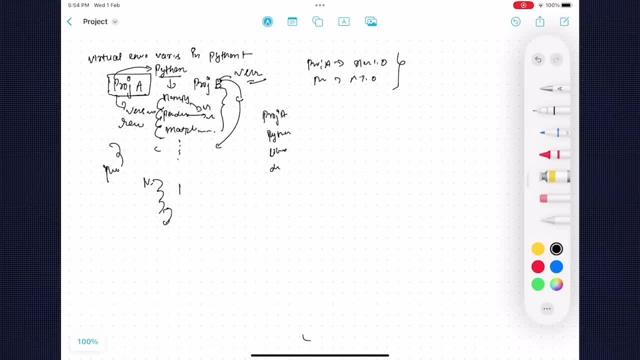 up right. so this is dependency, conflicts between which may can happen, and etc. so what is the ideal solution? we can have a container, we can have a container sort of thing, we can have a container sort of thing, or the variable sort of thing, a variable sort of thing or an environment sort of thing, for every project. so we have two projects. 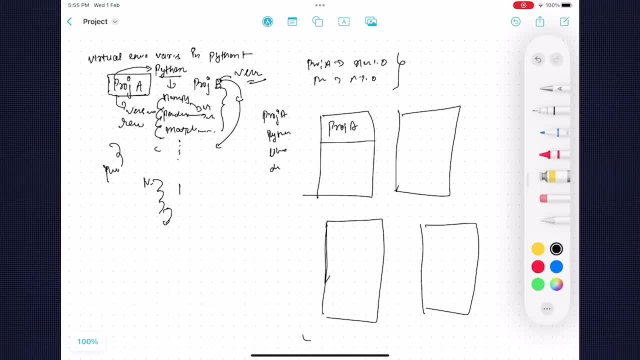 so project number a. so we create an environment for that particular project number a, and in that project number a you might have installed your own python version, your previous, that same such like a vuri address over there we called a single library byte directory on that particular. 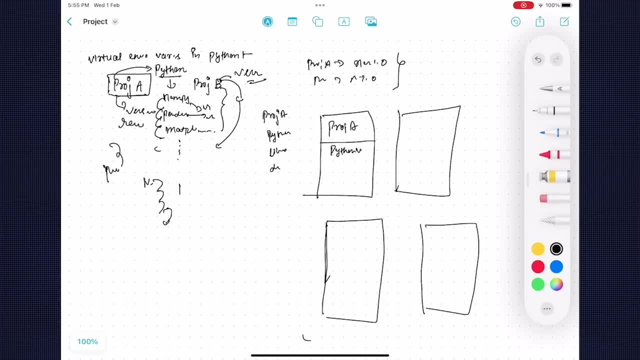 project number a, and in that project number you might install your own python version, your thyme, your own python version. you might also install your own libraries, your own libraries. so now you can run that project a using this and whatever versions you have, and then you make. 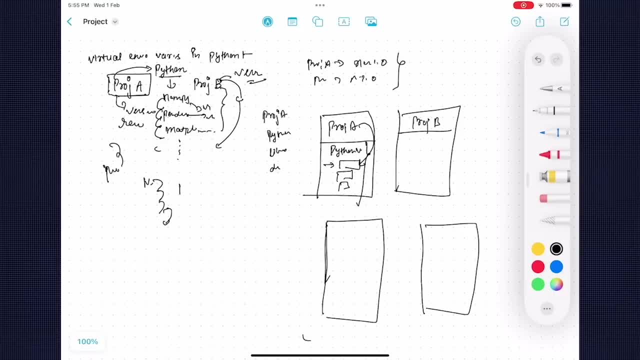 this another environment for project number b, for a project b, and in that project b you can have different, different versions. so you're gonna numpy 1.2, number one, 1.3 and then you can activate this environment. if you're running this particular project you can have project. 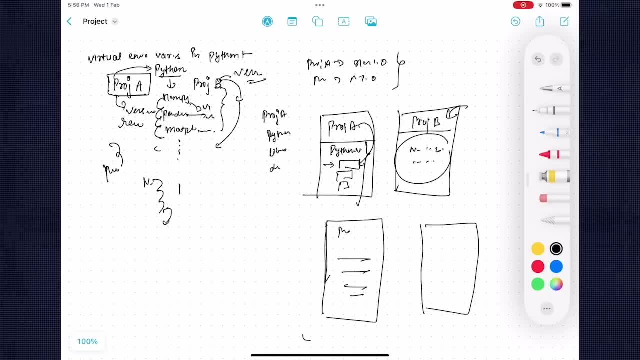 c with different versions, with different versions of your libraries or python, and all right. and then, if you want to run project number 3, you can activate this environment. if you have project number d, then you can have several other versions, and then if you run this project, 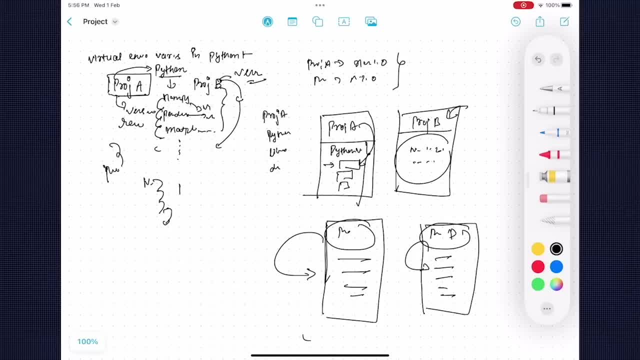 then you can activate this particular environment. okay, so this is one of the way to think about it, right? so basically, you can, you can, you can have a different different versions of packages and different, different for the different different projects, for the different different environments, and we can create this and this will not affect anything on a global means. 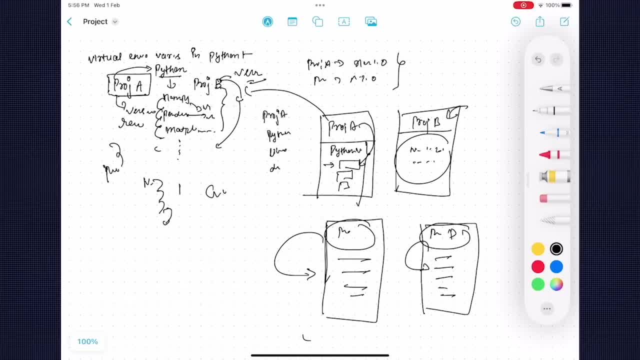 where you have global means, which is which is setting over. here you have certain packages installed, python installed on a path environment, but in that one you have several of the virtual environments available. right, there are different, different tools that use to create these sort of environments. one of them is venv, another one is conda, another 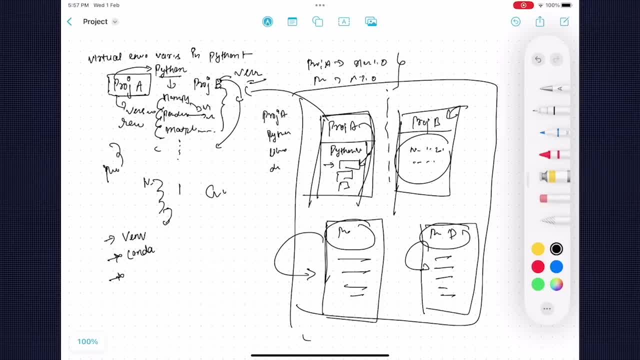 one is uh, one is venv, another one is conda, another one is uh, let's, let's say for us, for a second example: uh, pi nv, pi nv. so we have these three where you can simply create your virtual environments out of these tools, right? so let's talk about a bit about you know, a bit of reasons. 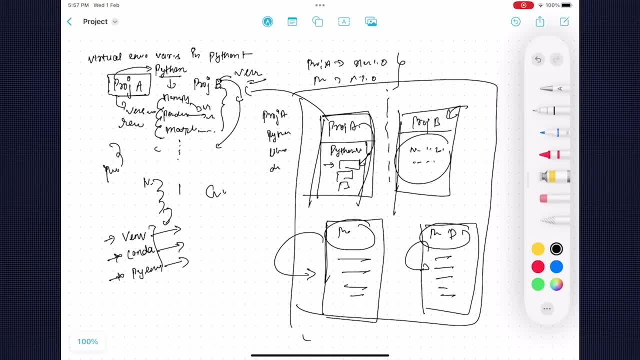 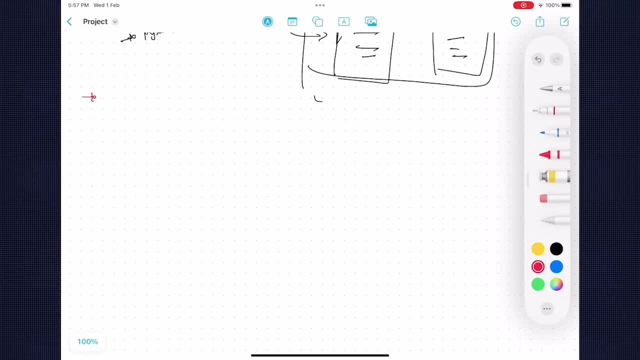 why exactly we need a virtual environment in our daily life, as is something which is super important. so there are several reasons which we might use for virtual environment. the first one is package package management. so this is the first one which is in package management, in package management. 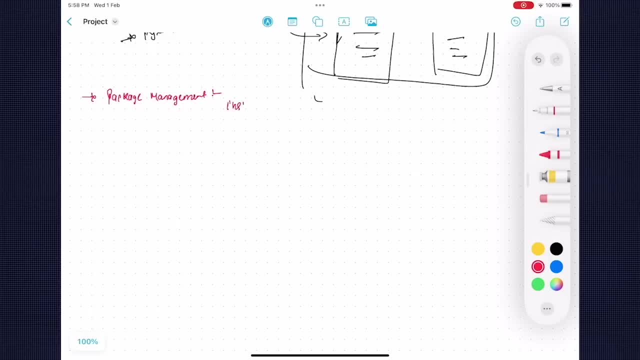 in package management. you can you what you can do. you can install your packages. you can install your packages. you can install and manage your packages or or libraries, libraries for particular projects. you don't need to install in such a way that it should be applicable on every project. it can be for a. 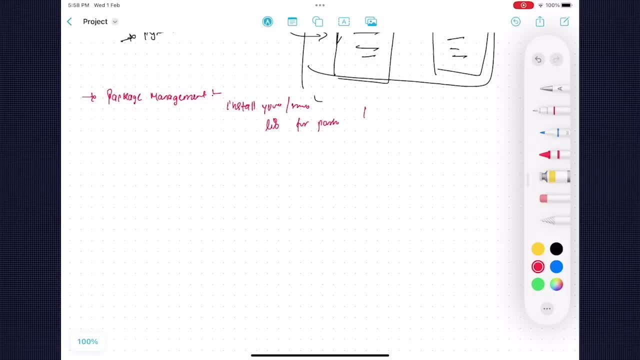 particular project and this: like you install a, like you install, you manage your project. you, you have a project and then you have several other dependencies. you have to only in package this. you can package this without affecting the project number two on which your work, so you might have. 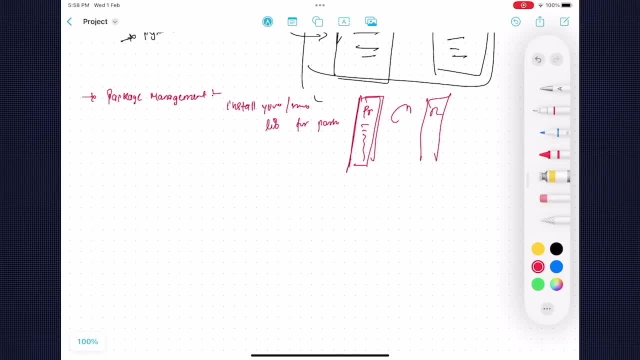 noticed in my previous projects, i always create a virtual environment so that it does not affect my other projects- dependencies, right. another way is we isolate our projects, which is another one is isolation, another one is iso isolation. isolation means that if you have lots of environments, you have lots of virtual environments for project. 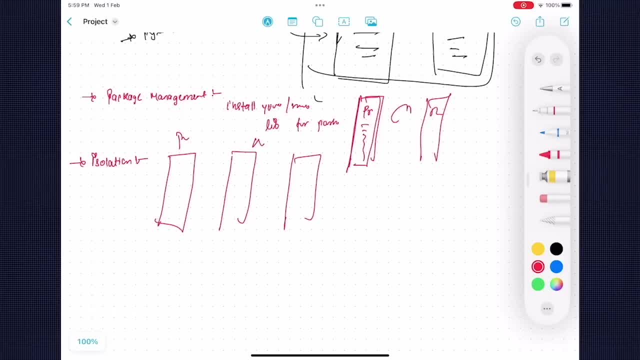 number a, project number b, project number c, so you can have these virtual environments. so changes in the project number a does not affect the changes in project number two. even they, if they have a same lab because they have all installed separately, they have all are installed separately by creating. 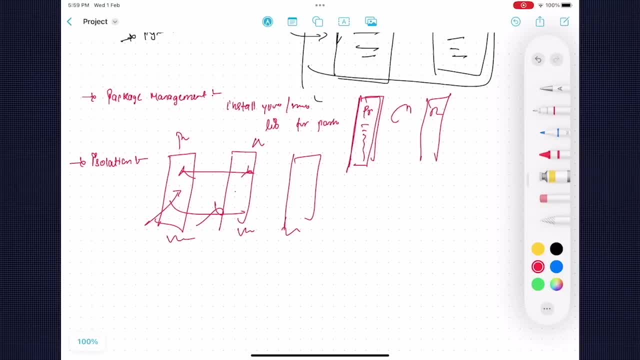 a folder, so everyone has their own folders and in that they have their own packages. so every environment has their own different, different versions, or it may be same as well, but one is the other. so in coven 19 we used to isolate now people, so in just wave over here as well, we isolate you. 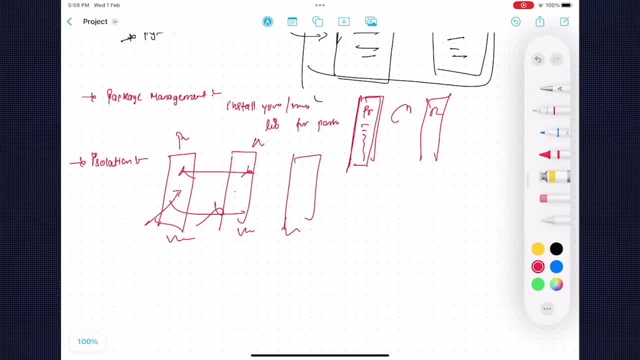 guys. okay, now you might have another one- is which is the another one is reproducibility. the rip bro do Z ability. okay, so this another reason of repressibility, which means that- let's take an example- you run a particular project, number a, you run a project number a and that there has 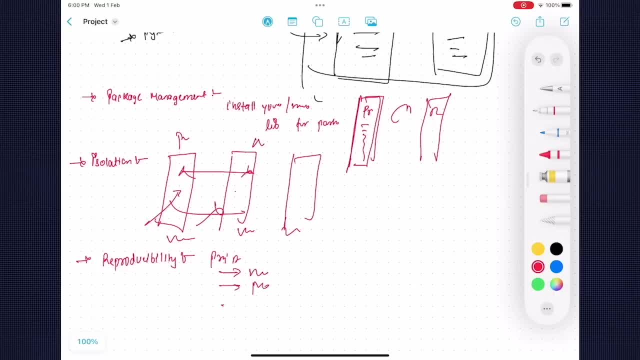 its own requirements. you know, has has short, should have numpy, should have pandas in that project, should have seaborn, should have this, this particular requirements, all the all the technical requirements, right. so when you have, when you package this up, you can exactly set up in such a way that it will work on other systems as well. you can also deploy to production. so whatever you, 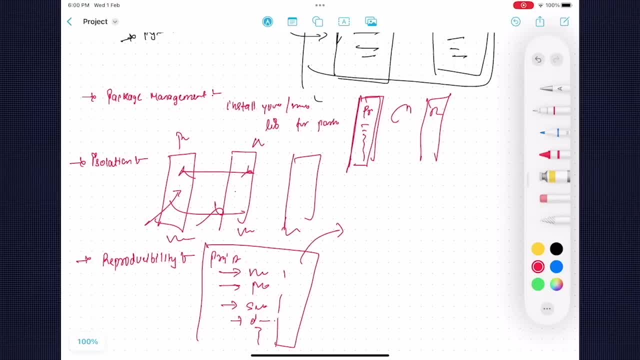 change, change it over here, changes in production as well, so you can actually have a very good reproducible pipelines out here and i hope that this gives you a good sense about what exactly you need to. you know she should be able to, but the reproducibility is not nothing but sharing of. 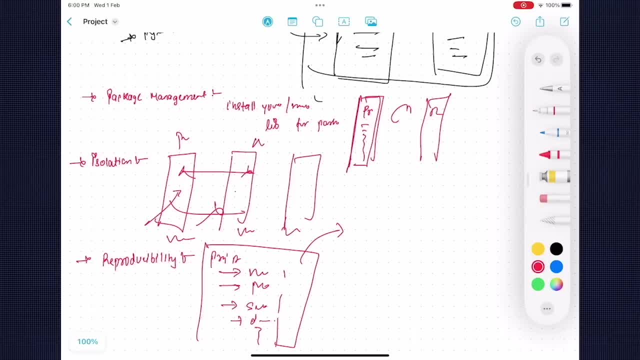 your project to others or deploying your project to a production. and that's why- because it may happen that you have a global slave, say, for example, of global environment, and in that you have hosted project number a. so, even if a single dependency error occurs, the system which is 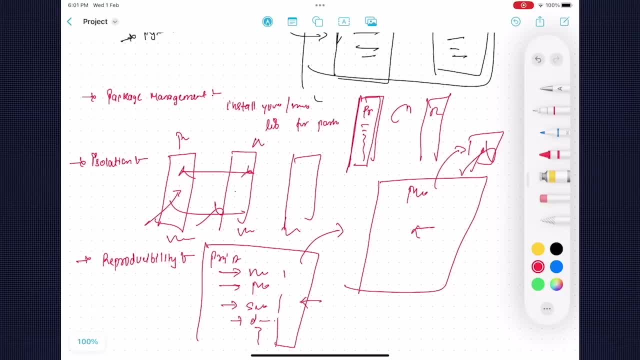 running for users and production will fail right. so you have the separately so that your model is so. so it's, our production is containing a single container or a one environment. i hope that that this gives you good sense about what exactly we wanted to talk on our packages and all now what we'll do. we'll 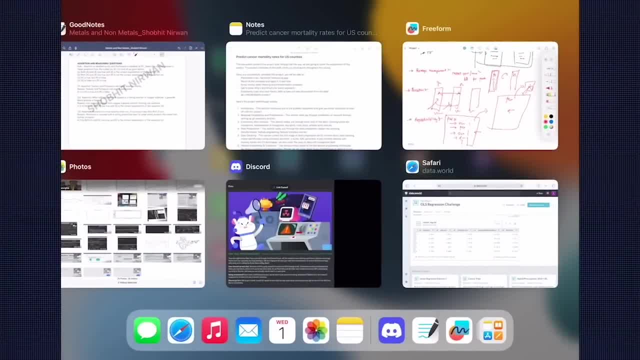 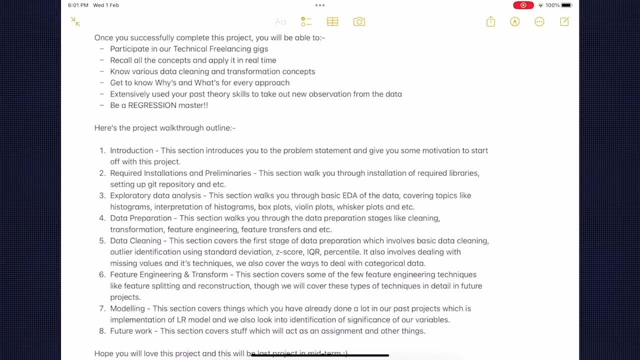 try to get into a bit of coding part. so now we have completed, complete, a bit of theory, which which which was needed before. it now what we'll do. we'll try to install our packages now and then we'll get started with basics of, you know, exploratory data analysis and try to understand. 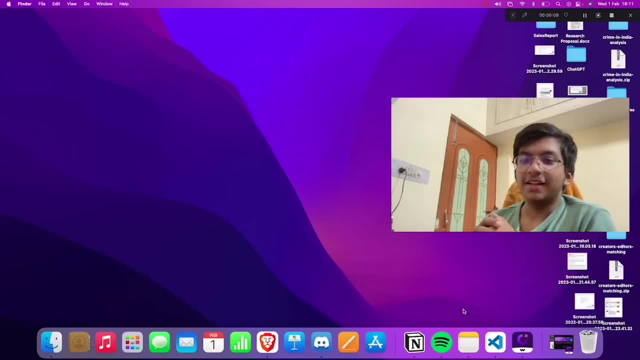 from there. hey everyone, welcome to this. another video on what what you're going to do. we're going to set up our project and make sure that you're also following. you have the downloaded materials and all, so you're also following to that throughout the course. so what i'll do today is make you a bit comfortable with a bit of you know. 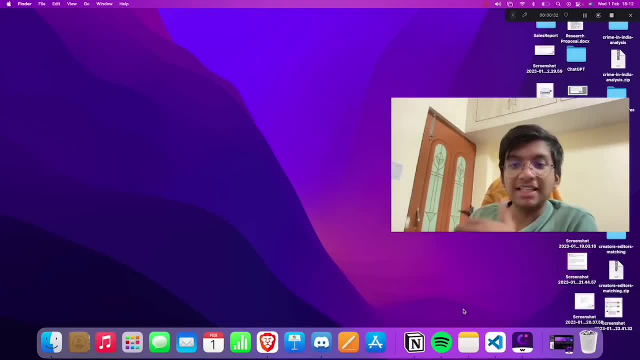 setting up the environments and installing required libraries, getting you through the notebooks which we have, getting you through the important steps out there, right? so let's start with that. first of all, i want to show you one thing which is a document file. which is a document file. 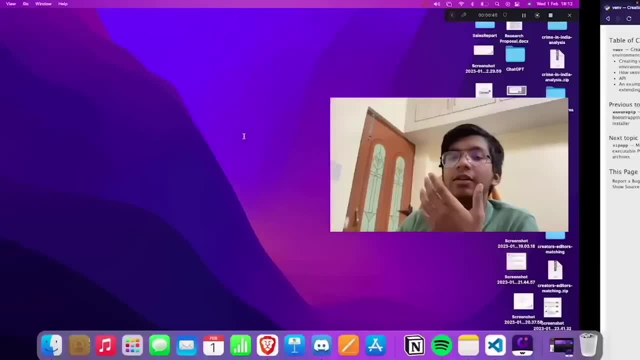 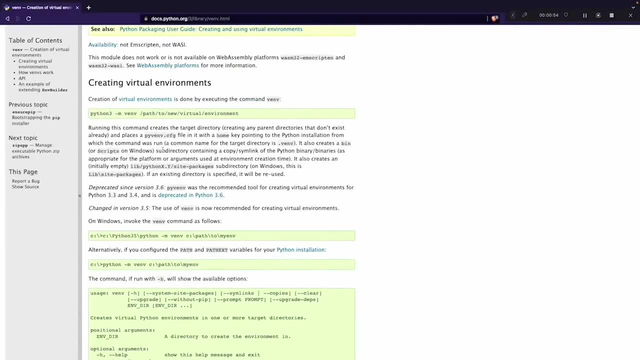 which is a documentation of python, which where it says that we'll be using vent. we'll be using vent to actually create the environment variable out here. so, um, so now, if you, if you want to create the virtual environment, if you, if you really want to create the virtual environment, then what we can? 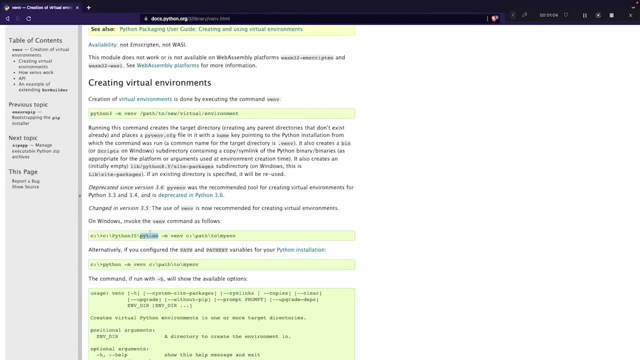 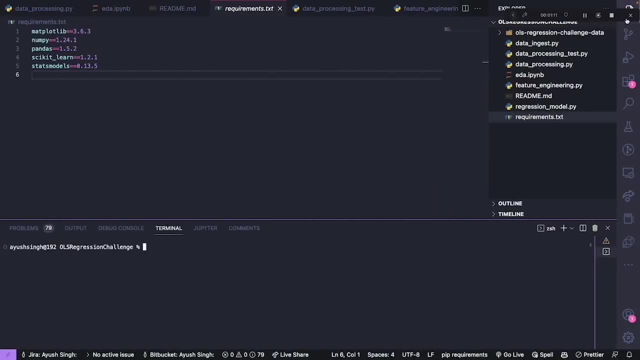 do? we can simply have this, maybe this one which is python mvnb, which which says that. so, basically, i have opened my you, even when, when you unzip your file. when you unzip your file, you will be having a unique library of всё. okay, so now you open your terminal. open your terminal and go to that. 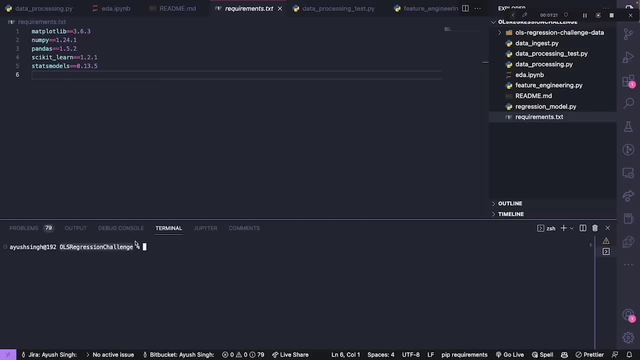 folder when, which will get you that Oxford, your and right. so if you try to create one name for your that whs0 and write yourgarock virtual environment as a ols regression challenge, so just write oh ols, which will be the name of our environment. 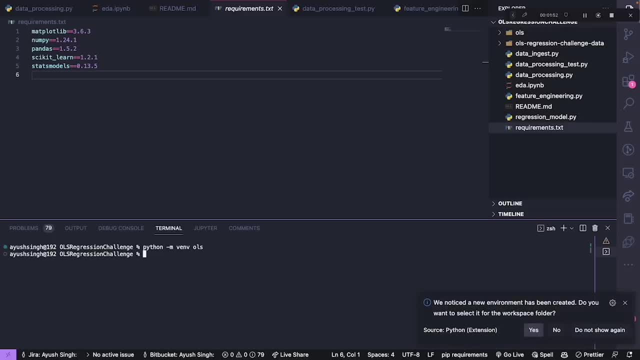 and then let's click on enter and that creates. and that creates. uh, we noticed. do you want to select it for the workspace folder? yes, i want to select it for workspace folder. now we have created a virtual environment. we have created a virtual environment named ols, where it says that you 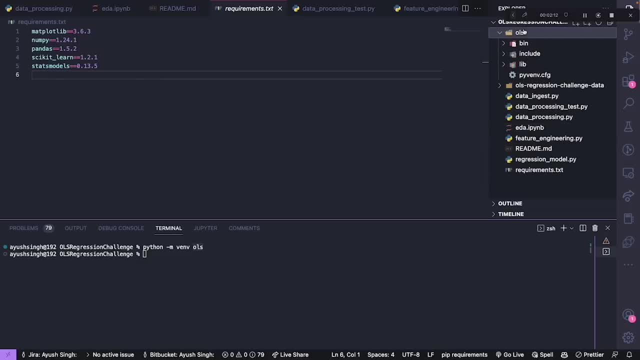 can see that a new folder has been created where all our files will be installed. all our packages will be installed. now it's containerized in a particular environment, so now our project will only run if that environment is activated. if this environment is activated, okay, so how can we act? 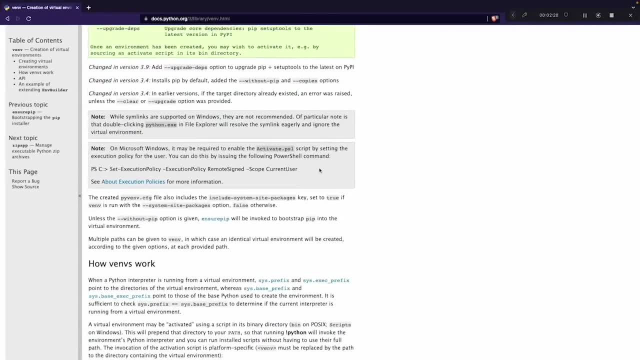 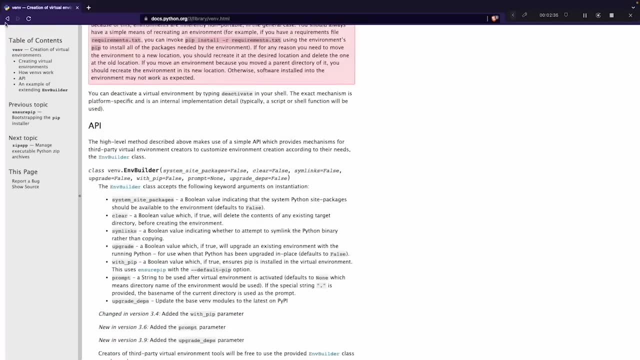 how can we activate this? this is, this is pretty much uh, like, like i'm, i'm totally, you know, uh, trying to make sure that how, eventually, if i'm, if i'm uh, you know, uh, in initial versions how i'm going to uh, you know how i'm going to. you know how i'm going to uh, you know how i'm going to. 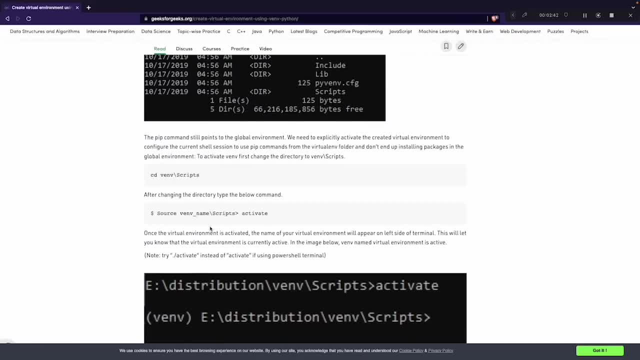 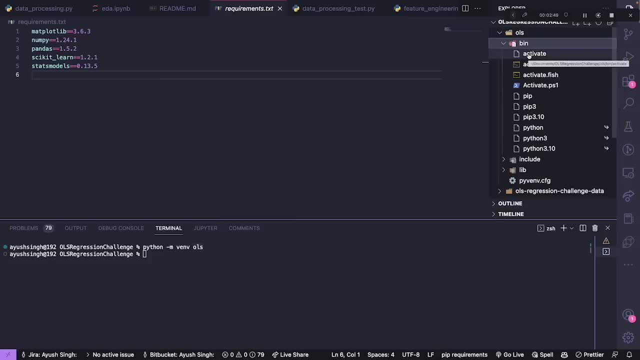 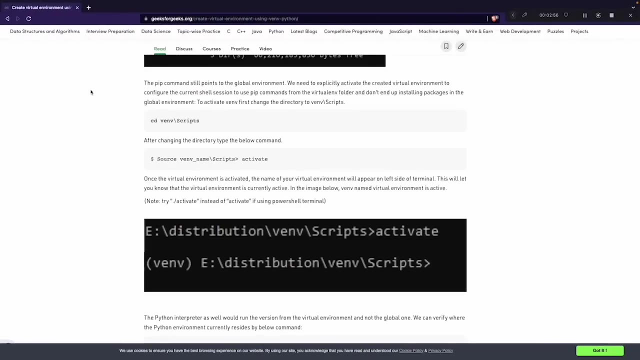 make sure that you're able to, um, get it. so so, basically, uh, if you go to the, you know so, if you go to the bin for bin file, and then you have something which is activate, which is something which is activate, so you can either go there and then, uh, confirm it right, either you can go there. 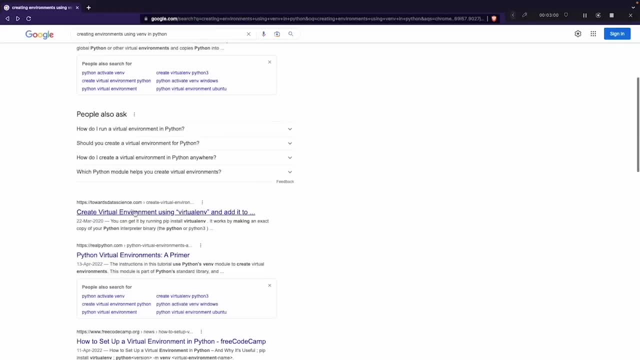 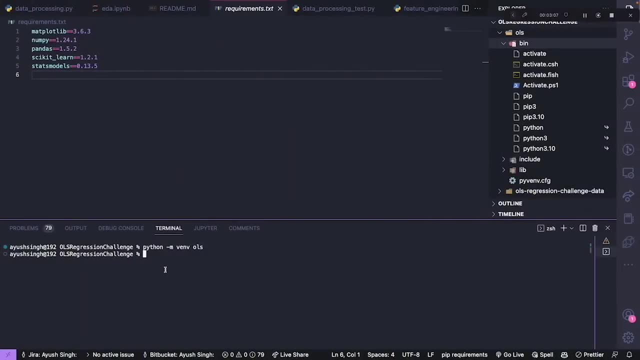 go there like cd and blah, blah, blah, you just go there. or you can just have a uh sets like, let's say uh, let's say uh, you want to go it, uh in the folder of cd, you want to go it, uh in the folder of cd. 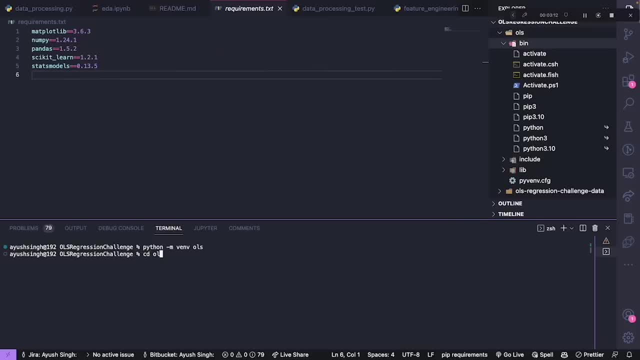 you want to go it, uh, in the folder of cd ols, cd ols, cd ols. eventually i- i actually use pi envy, to be honest, uh, because because of my organization, because in previous organizations they were using pi envy, but i recommend you to use ben, because it's just initial version of 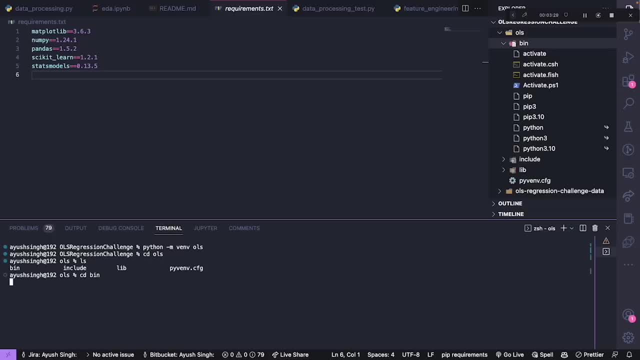 yourself. that's why i recommend to use that. then i go to select, go to ben and then click on source, source, activate, or maybe you can run simple, simply the activate as well. it should run very fine. so now, when you see over here ols, which means that now your particular, now you can run your. 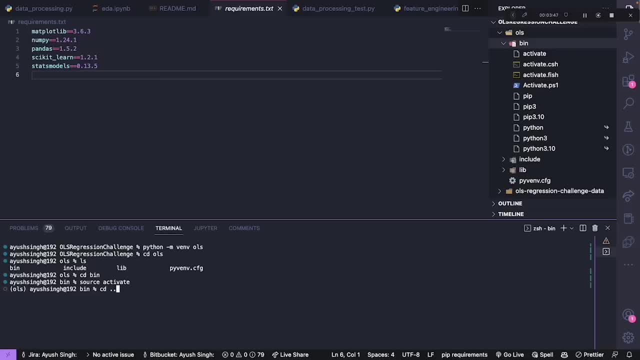 project with that particular environment. okay, now you can go out of that. however, you can also write source and then you write, uh, you know, ols, ols, and then you simply write our bin, and then you simply write activate. okay, it should work perfectly fine, right? so i actually go on and showed you the step. 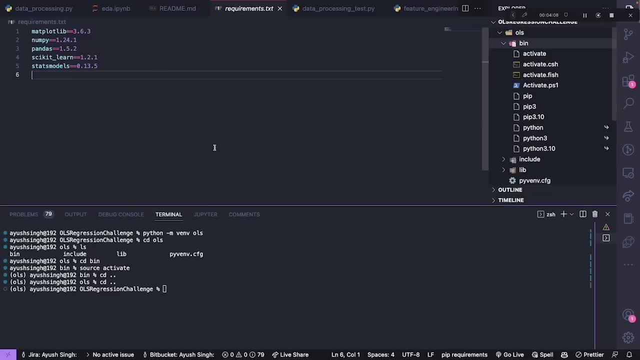 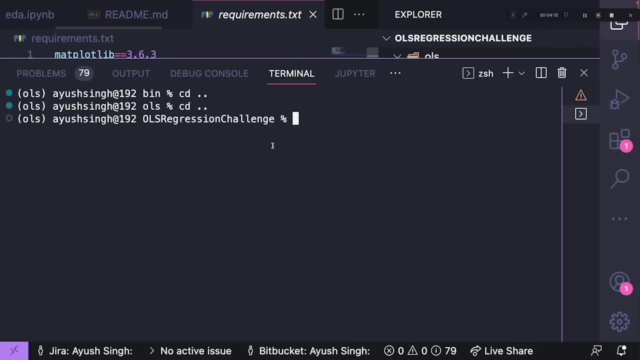 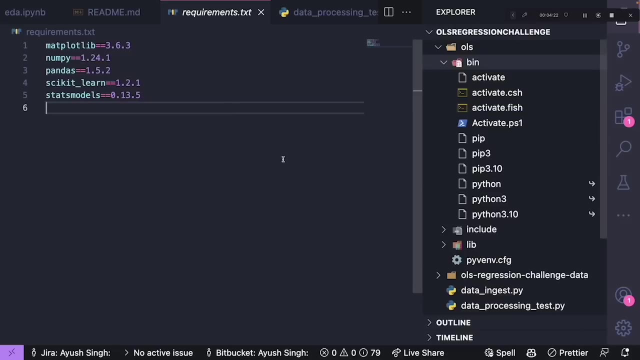 by step uh solution of that. right, let me just zoom in a bit. maybe it may be beneficial for you uh to notice uh which is out here. so let me just zoom in a bit. yeah, so now we have, now we have activated environment. now what we need to do now. as i said, now, once we have activated our environment, now what we have. 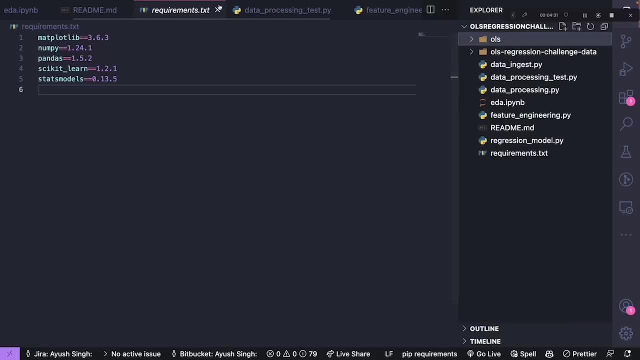 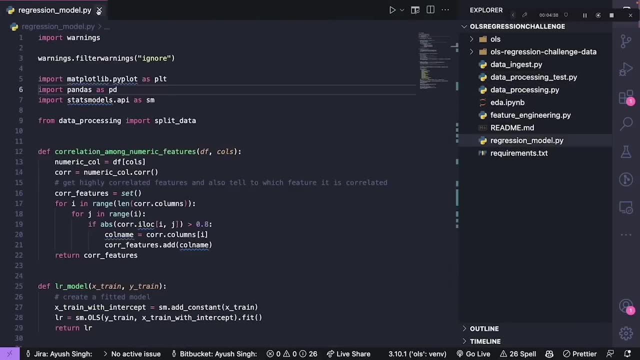 to do. we have to. um, let let's, let us go through the uh project, let us go through all the files. right, that's much more better rather than showing it like this. so now you're the now. now we'll see something like this after every end, after you have activated your environment. 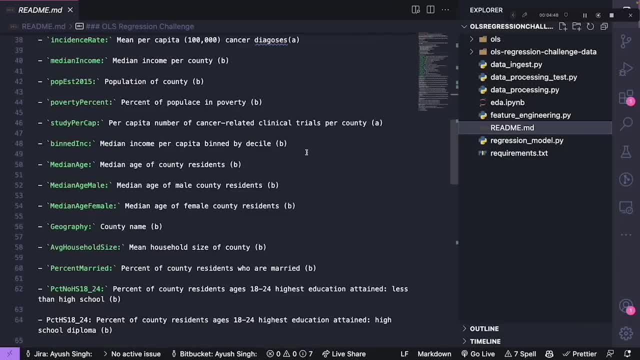 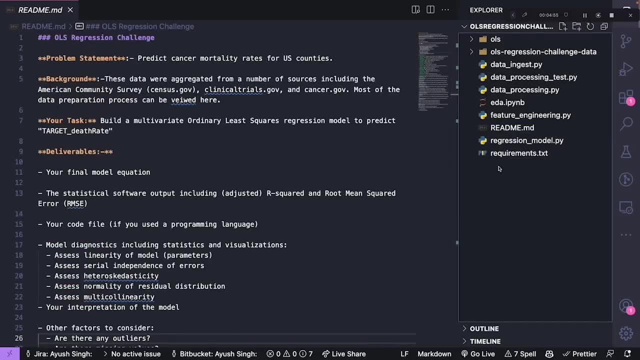 so, though, so i'll recommend you to go to readmemd, and this is read memd. you'll find everything which you need, which is what exactly? the problem statement, etc. now. now what we need to do. we need to recall and we need to install the required libraries, which we'll be going to use in this. 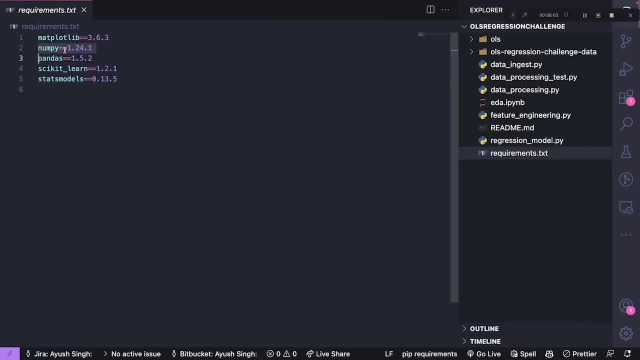 project. so we'll be going to use this, this project, as well, as we have some other libraries to install, so we'll install that for sure. so, as of now, we'll install these libraries and we're going which which have created requirements, which says that these are the requirements for this. 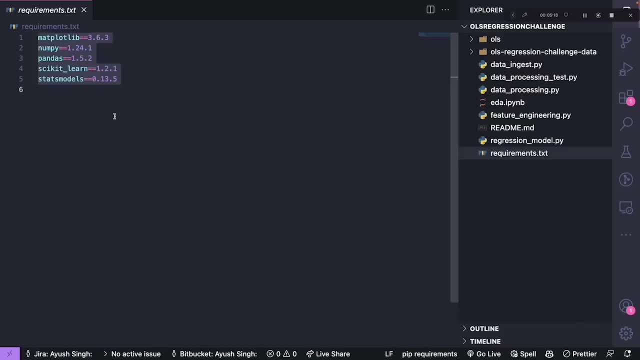 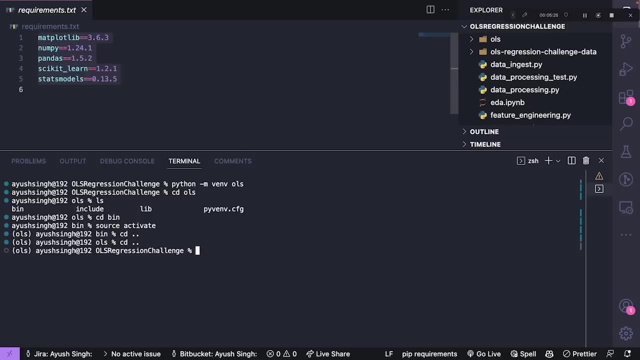 particular project, which means these are the libraries, which or packages which needs to be installed for this project. so when you're going to go to there and then what you can do, you can simply add: first of all, which python? so let's they think about which is the python which which you're 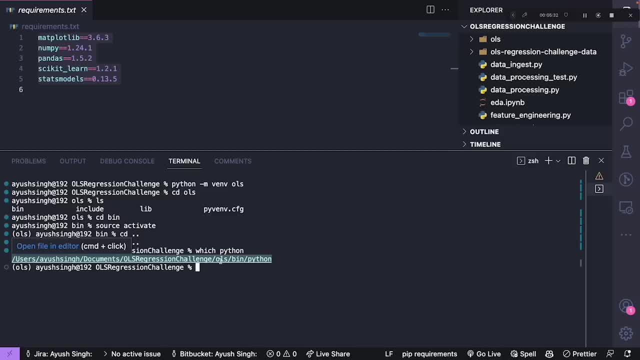 using over here. we are using the python which is created for this environment, and then let's talk about which pip you're using. using pip for this particular you can see that ols bin and pip, so pip for this particular environment. now, what we can do, we can simply install pip, install our dash, our. 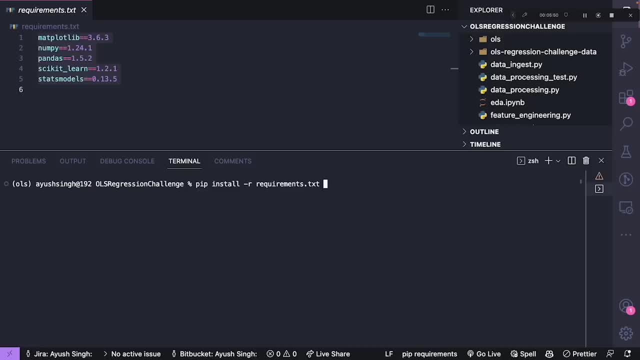 requirements. so what, what this does, what this does, so it you, you can simply name all the file, name all the libraries with, with the specified versions which you need, specified versions which you need for that particular library. we will come to that how we got, how we created this at the end. 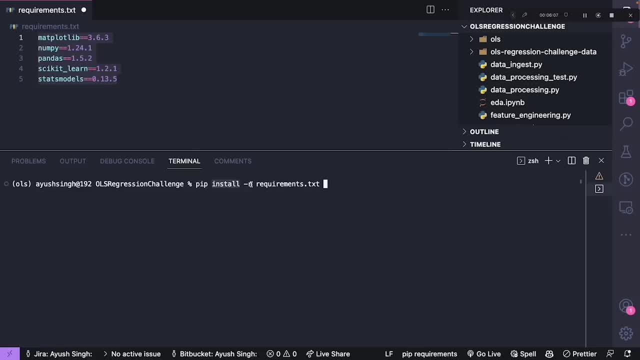 but as as of now, you can simply have this pip install and this this indicates that you know you can also install it individually, but i was i've added in the file, so so i can install it all at the once by a single command which is in the requirements file, and then it goes in the first install, the. 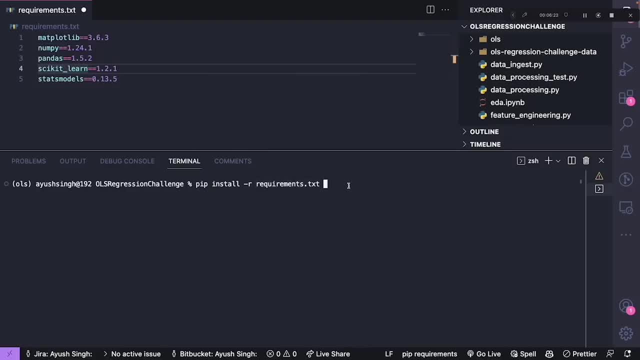 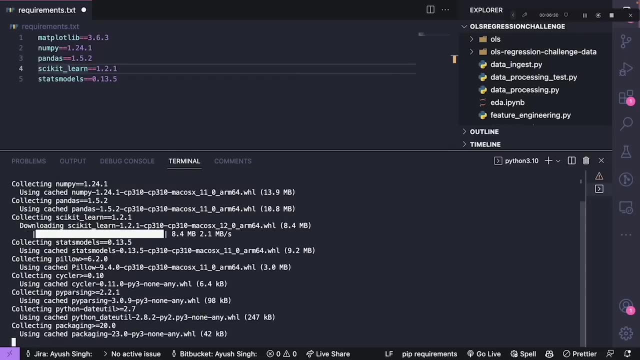 first, second, third, fourth, all around the end, and then simply click enter. once we click enter, it takes it takes a bit of you know um time to do that, um, and then you will see that it is being all the packages are being installed. so all the packages are, i think, uh, being installed. 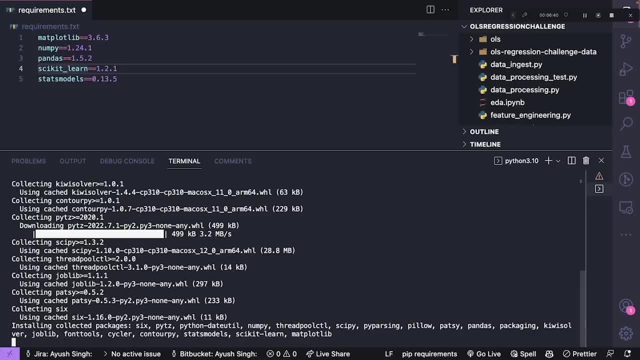 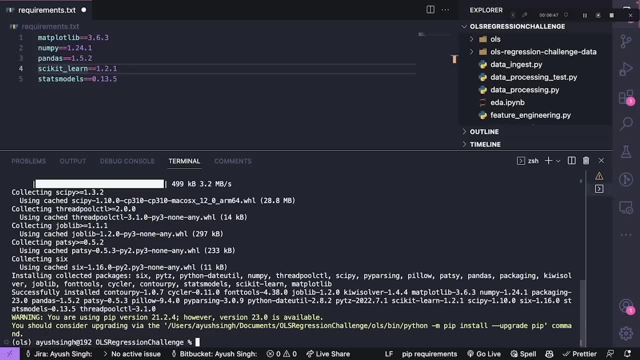 over here where they're installing matplotlib, they're installing numpad, they're installing cyclone, they're installing stats model, and then we are done. so we got a bit of warning over here. what that warning says? that that the pip version which we are using, the pip version which we are using, it's not upgraded. so let's upgrade our pip version. 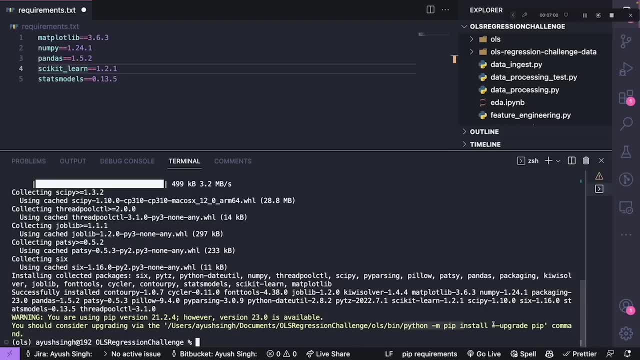 so let's, let's upgrade our pip version so we can simply add python and then use this particular command. uh, so just saying that, use to use this python, which is our python. the, the absolute, the, the path of the python, python is over here at the end, because the, uh, the, the path of the python is. 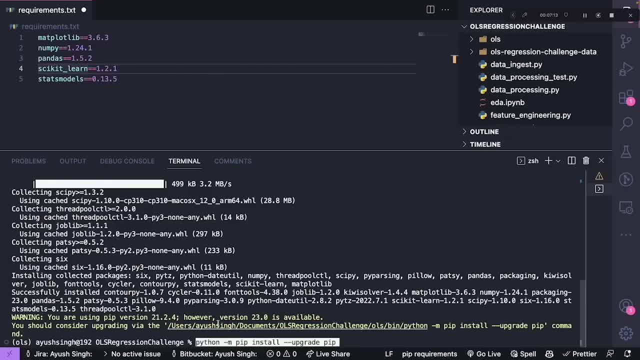 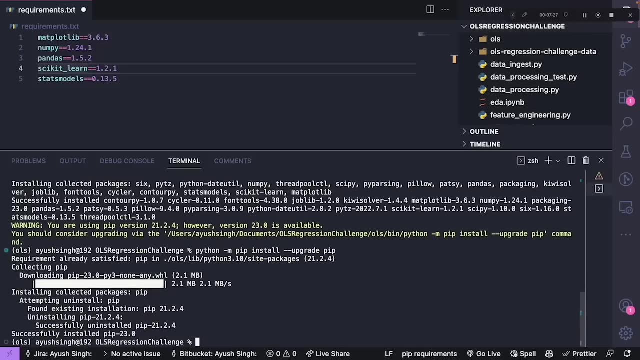 But you can actually absolutely use that Python because you have just checked that Python, the which Python, the Python is like the environment Python only. and then you installing Pip install and then you upgrade the pip. you simply upgrade your pip and then click enter. now It upgrades your pip to the latest version, which is 23.0. now that warning can be removed. 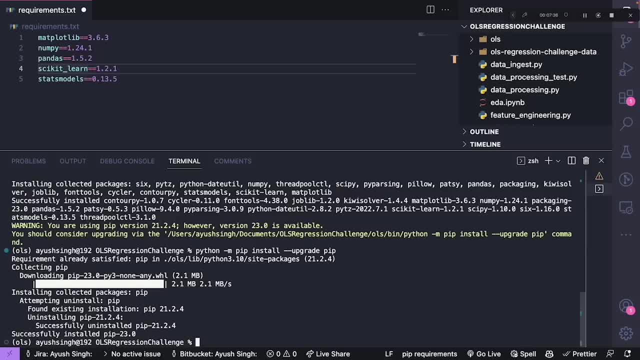 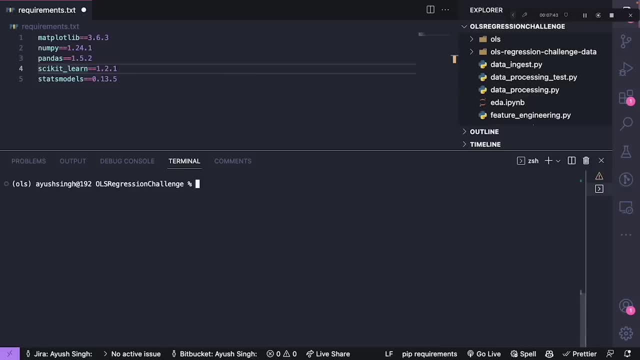 So I hope that this gives you good sense about what exactly we wanted to, wanted to do. now We have the working, we have the working Available things out here where we set it up, a project. now We are. now we are ready to start off with our explanation of the project. 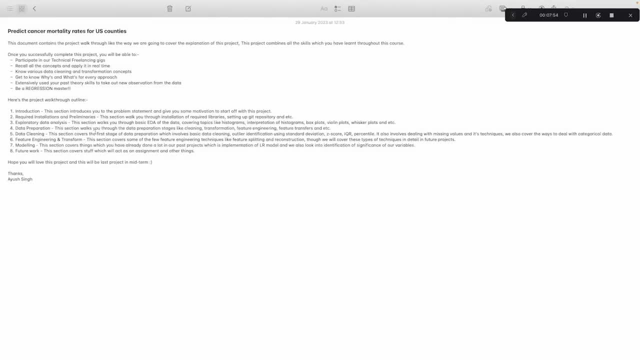 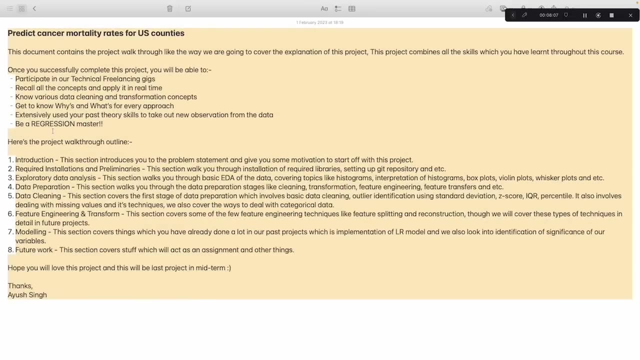 So if you open our notes, if you open our notes, we had this notes out here, We had this notes out here. Let me just move it, but you have to Introduction: we have done with introduction, all the setting up, everything. However, we haven't covered the setting up get repository, which we will do at the end, not right now. 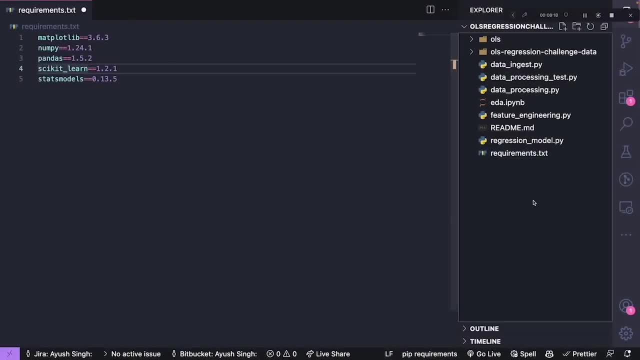 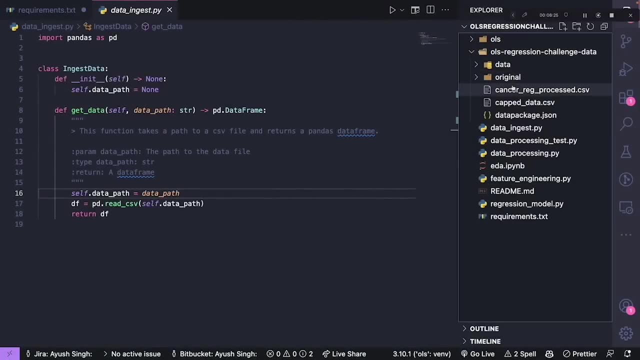 so. So now we have the required and things, now, what we'll do will: now we have the data. So when you, when you, when you open this data folder, you have, you have a lot of things available out here. you, you don't, you ignore this. these two as of now, because 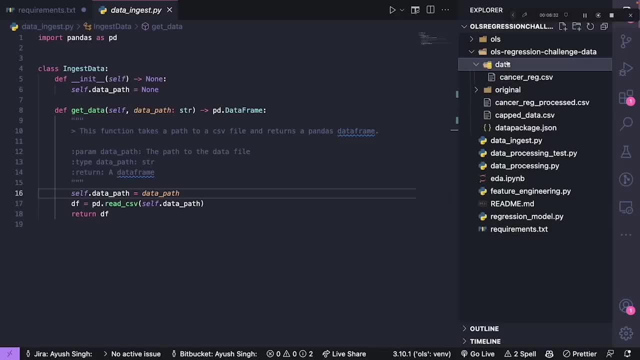 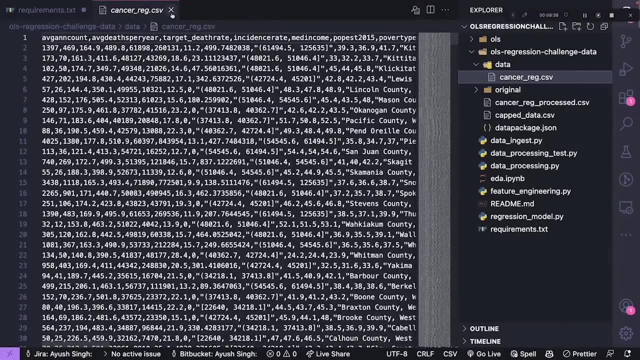 This is something which will be built in the project monthly. You will see. that is the data and this is the original data, right? So I suggest to go in this data and this data. you will find out the data which is available out there. So let me just open that. so I think 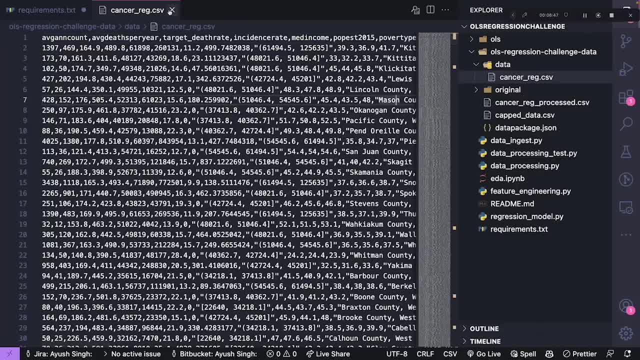 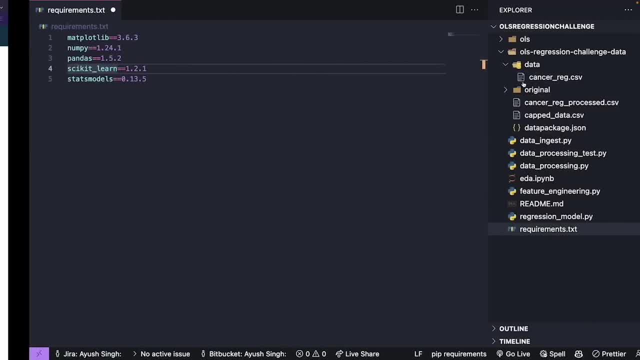 When you will open this in CSV file, it will look much more better. I have already shown you in the introduction session. very, very good. If you go over here, you will be having cancer regression, not CSV. You will be able to see the data out here. 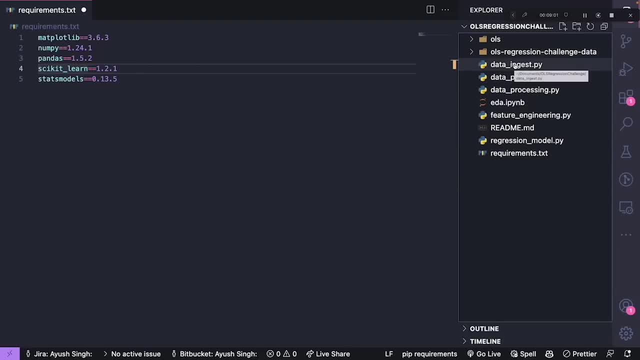 Okay, Now over here, the first step is: will the first step, which is see a very simple, very, very had a class Where we are taking out, ingesting the data, and second, what we'll do will start off with Understanding our data. Okay, so I have created a very nice notebook where we did a very extensive 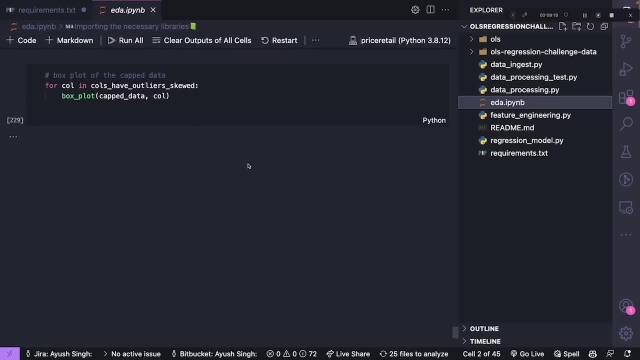 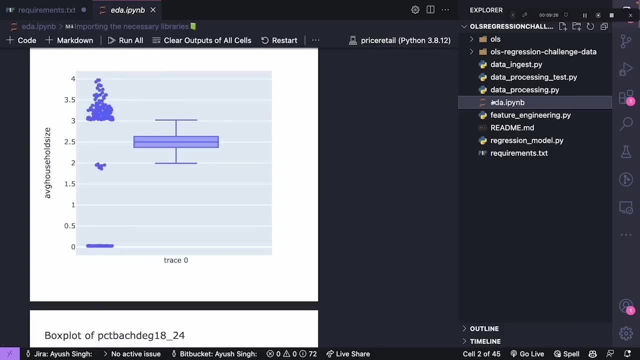 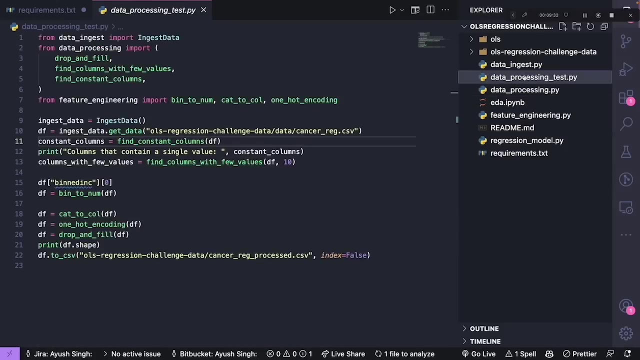 We did deal to be it. you know outliers, we deal with a lot of things out, So we'll cover that in very day. So I hope that and then we'll after the, after the, after the EDA will cover some pre-processing techniques, We'll cover some feature engineering techniques, then we'll cover some pre-processing steps and cetera. I 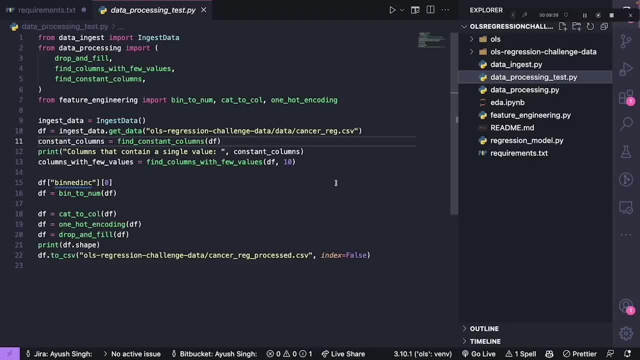 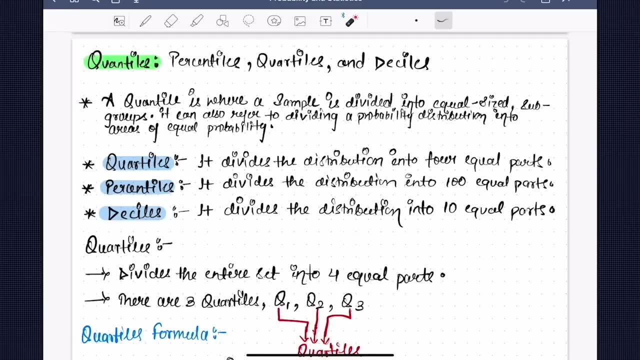 Hope that this this guides you super well. let's catch up in the next set of lectures to understand the EDA and everything out there. So everyone, welcome back to another lecture, especially on our Some theory part which we'll try to discuss. you know some. I will start off with this basic EDA and then with the basic area. 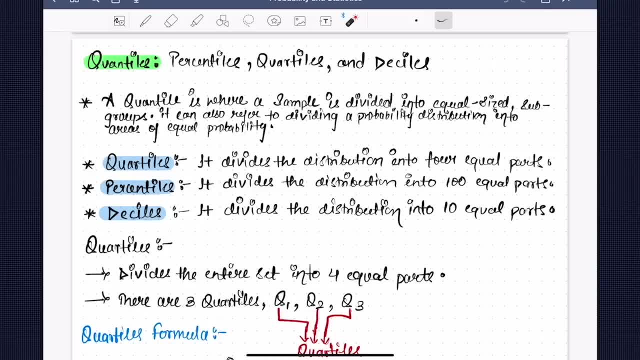 We'll try to figure out what is the possible. you know our data Cleaning techniques and data preparation techniques which we have to go forward with, right. So let's let's start talking about- actually about all of these things, But before that, going to review a quick concept which we have to go through is about quartiles, right. 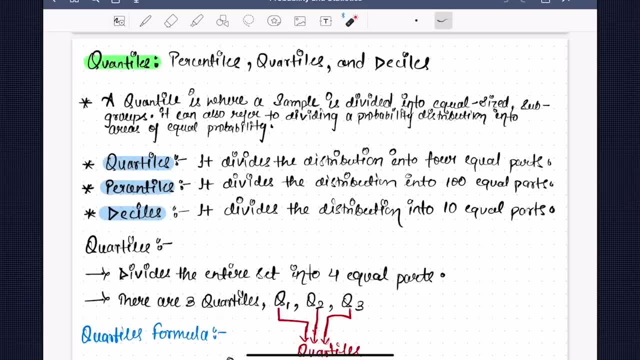 You can read about deciles, percentiles, in the previous Lectures taught in the probability and statistics part. I would like to go through only one concept of over here, which is quartiles. So what is quartile? quartile is something which basically quartile is a part of quantiles where we divide our data into some sort of distribution. 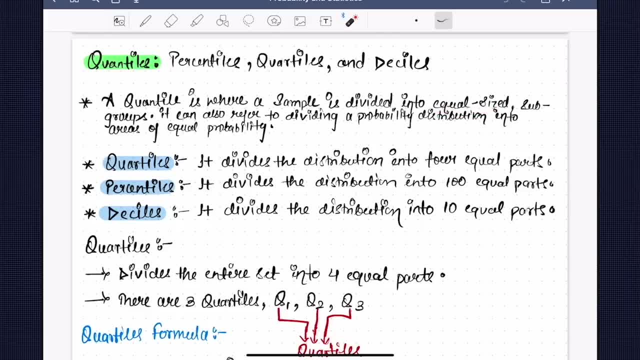 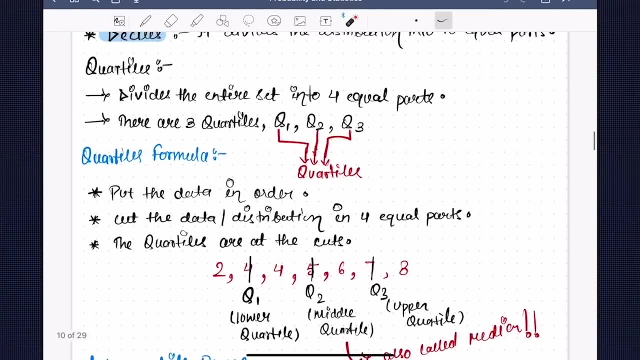 Which are equal sized, right, or subgroups. Okay, so we divide our data into subgroups, right? So we have already studied that. it divides our distribution into four equal parts of quartiles, divides our distribution of four equal parts and there are three quartiles. so here, assume that you have this data, this data, so assume that this. 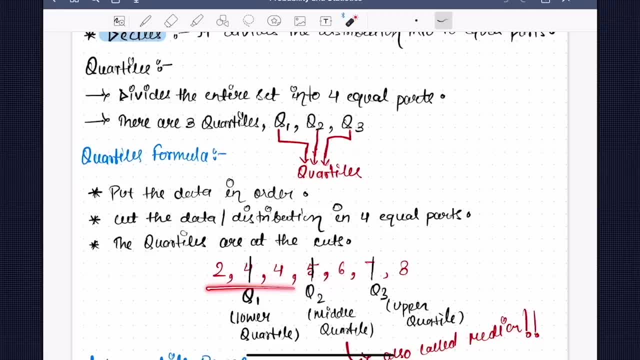 is a column: two, four, five, six, seven, eight. so divide this data into equal equal parts, where you have first, first, second, third and fourth. so you'll see that the all are equal, equal parts. and this is the quartile number one, this is a quartile number two and quartile number three. 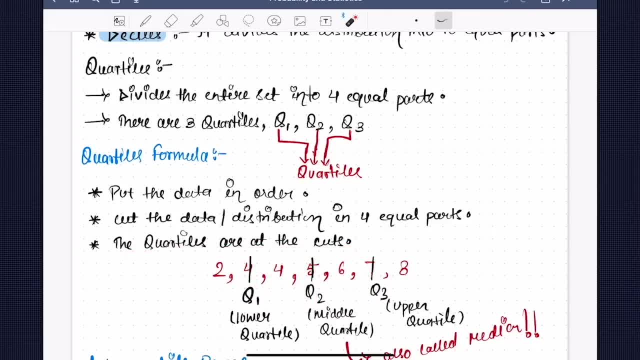 so quartiles are at the cuts where we divide our equal parts, right? so the first step of this for taking out the quartiles. so what is quartile? quartile is where we divide a distribution for four equal parts and quartiles are like q1, q2, q3 are the quartiles where which are present at the 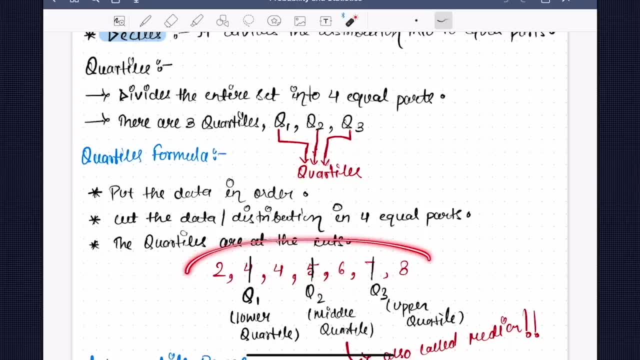 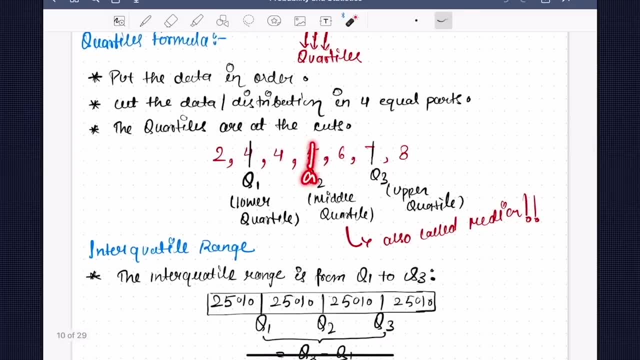 cuts and they. first of all, we have to put our data in a ordered format. it should not be unordered, otherwise it will not work right over here. over here, your quartile number two is the median. quartile number two is the is the median, so let's talk about quartile number one and quartile number three in great. 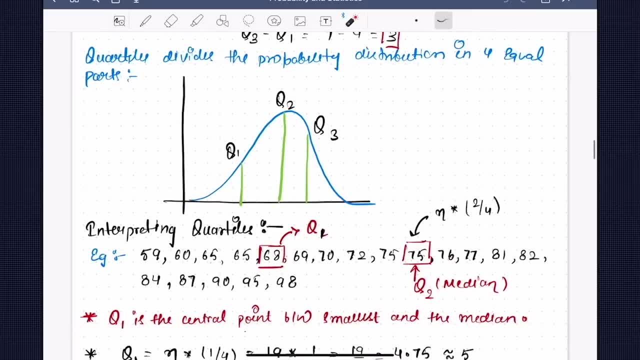 detail. so, basically, you're seeing in you, you're seeing in front of you that you have a date, that that your distribution of your particular data right and this is quartile number one where, and this quartile number two and this quartile number three. so, given this particular information, q1 is 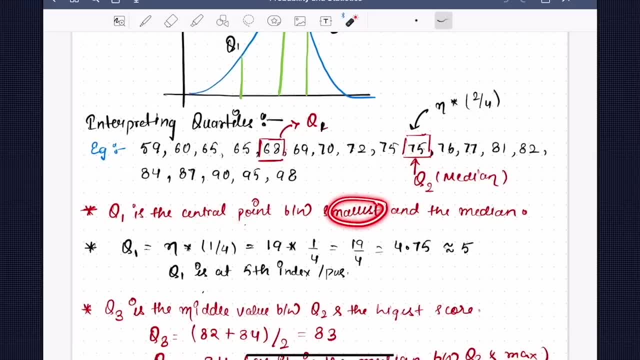 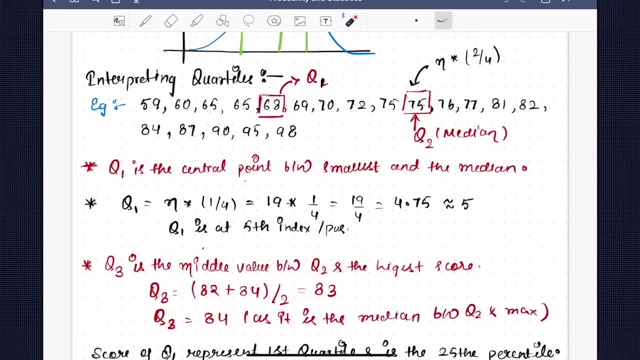 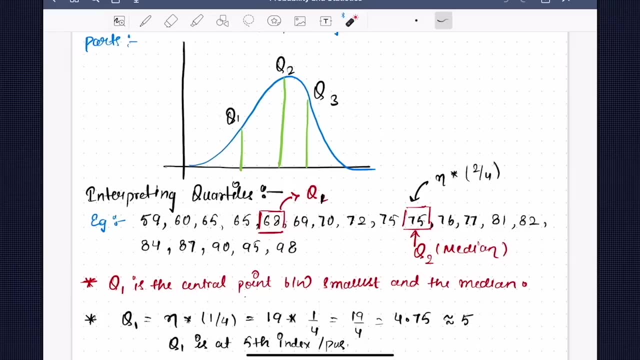 the central point between your smallest value and the median of your column. okay, q3 is the median, the q3 is the median and q2 is the highest score. so, basically, what? given this example, so assume that this is this. this is an example of your marks. you got right, this is, this is an example, so you 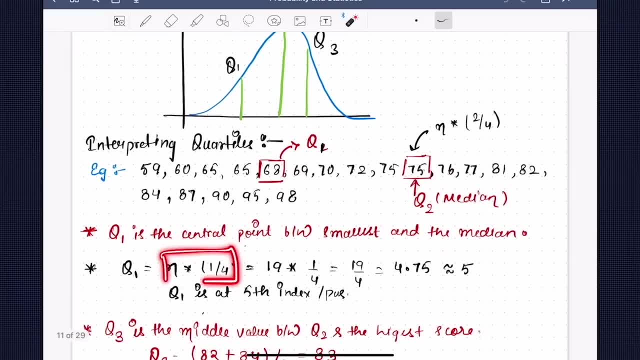 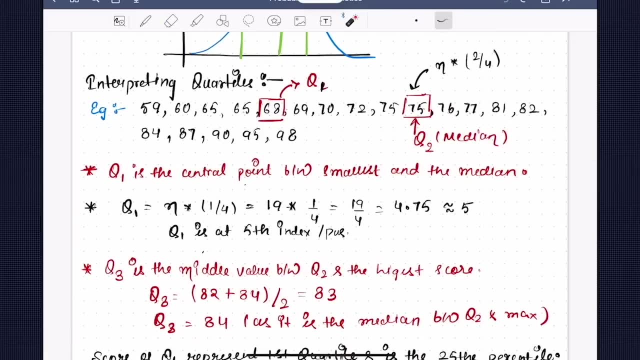 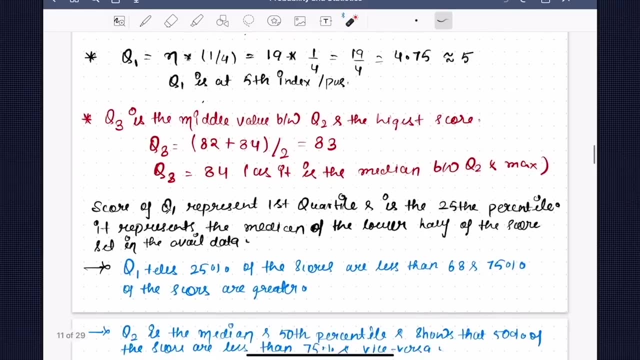 put in order format. now you take out q1 by this formula, you take out q1 by this formula. you take out q3- sorry wait, you take out q3. you take out q3, which is the middle value, by this formula, and you take out q1, q2, q3, which we have already taken out. right, and now what q1 tells you q1. 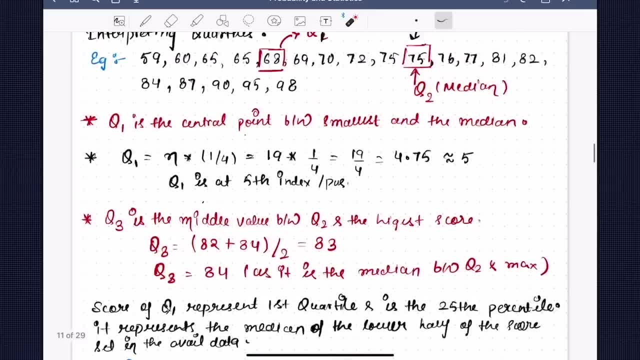 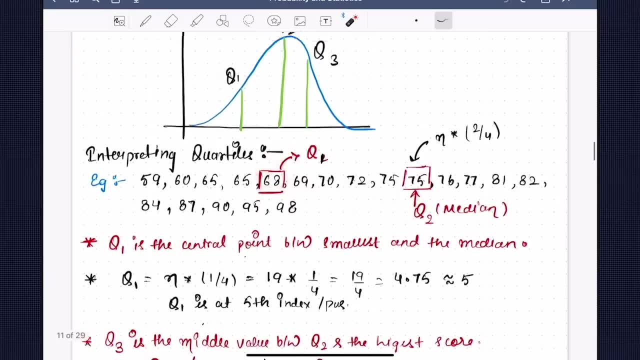 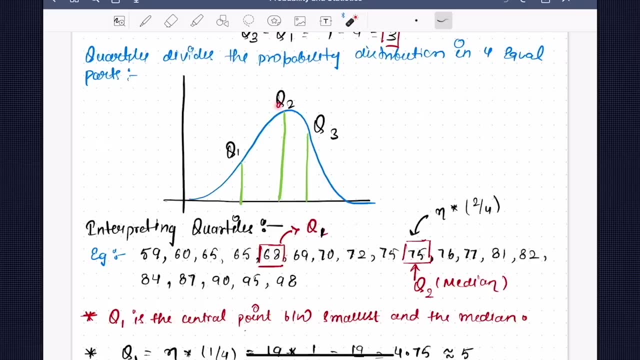 tells you that 25 percent of the scores are less than 68. so if you have the quartile number one, if we have the quartile number one which is at the position number five, which is 68, so we say that there is 25 percent of values, there's 25 percent of values which are less than 68. quartile number: 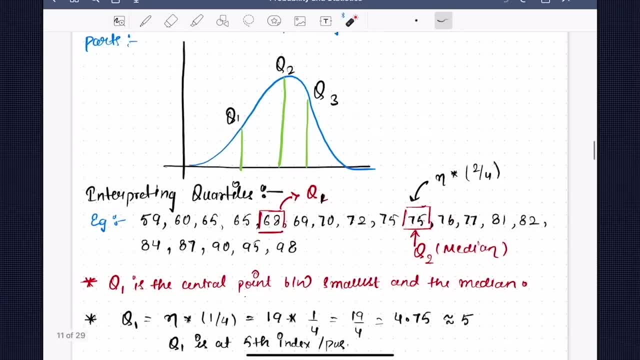 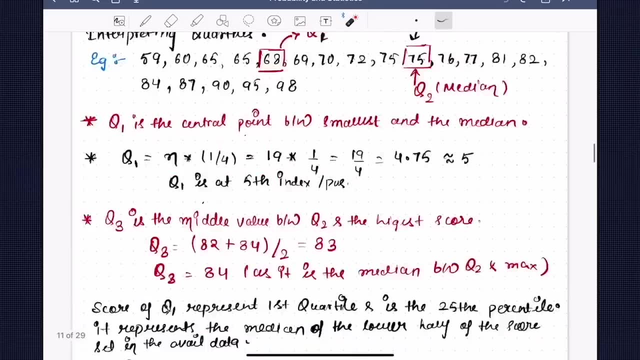 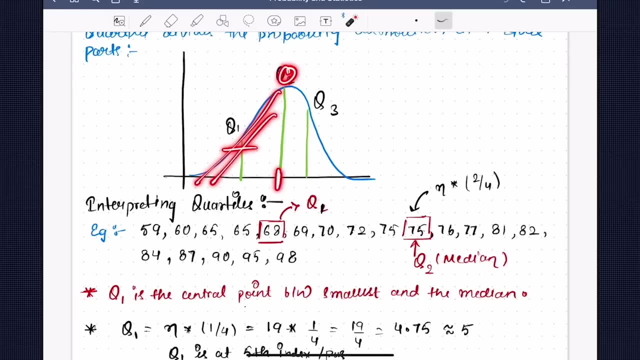 two tells there are 50 percent of values which are smaller than which, which are smaller, which are smaller than you know. so, whatever median is, there is 50 percent value which is smaller than this particular median right, 50 percent values like this, 50 percent and the 50 percent who are greater than this. so that's why q2 is called the median. 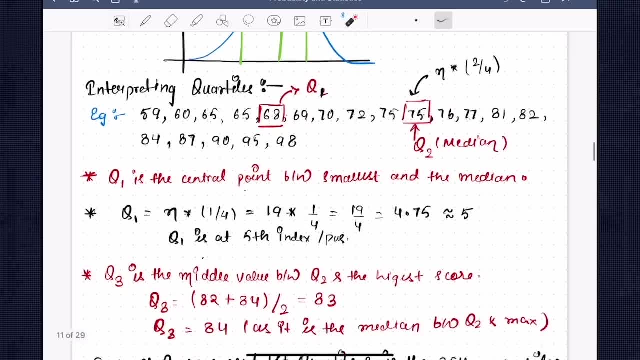 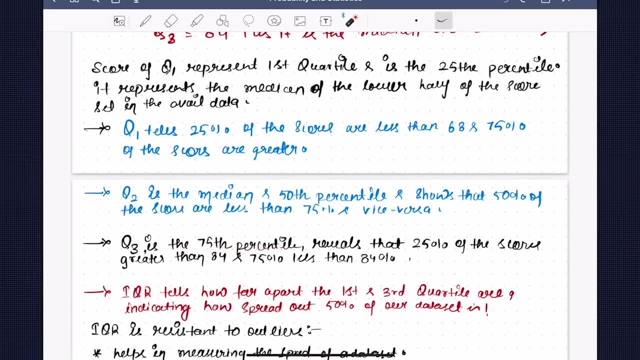 which is the middle value, with 50 greater than this and 50 percent smaller, smaller than this. we have q3 where we say that, q3 which says that, which is the 75th percentile. or you visit where it contains the top 25 percent of the scores which are greater than 84, right? so basically it is saying: 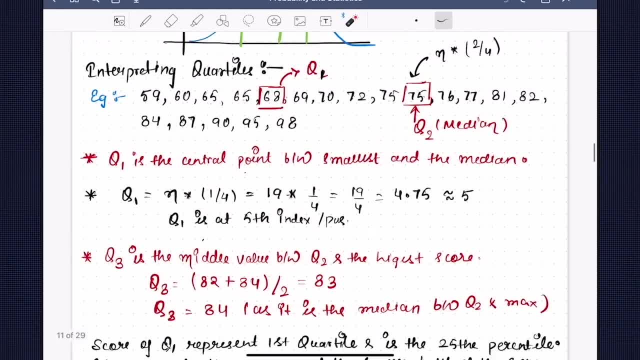 that whatever the score which is greater than 84, that's what. the greater than 84 are the 25 percent of the values which are 20, last 25, top 25 percent of the values, right? so this is also called the 75th percentile, where it says that 25 percent of the scores are greater. 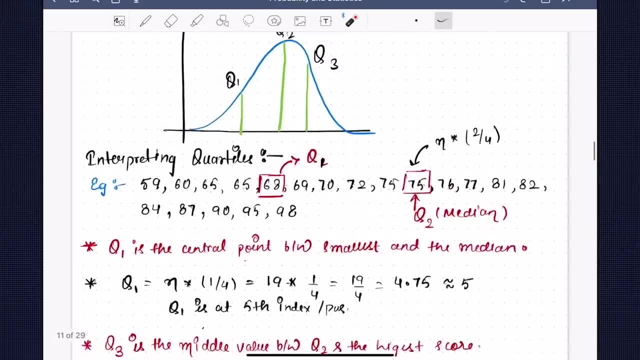 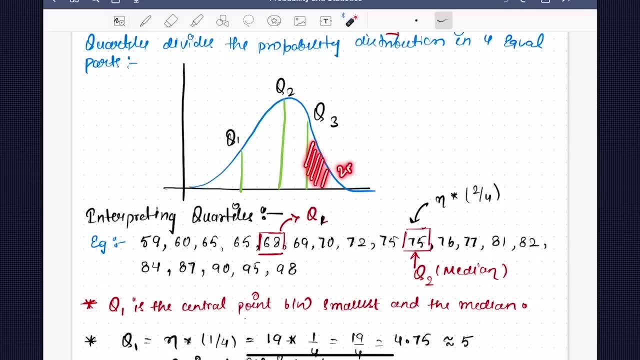 than 84.. and 75 percent less than 24.. so, basically, out here, out this, we say that there is 25 percent of the score which are greater than 20, which are which are greater than 84, because that's the quarter number three for the. 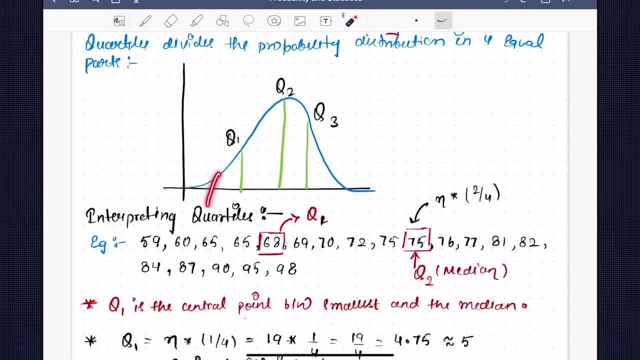 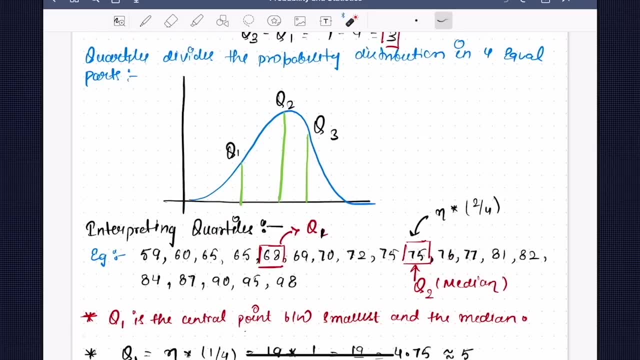 this particular example greater than 20, 84, and there's 75 percent of the examples which are less than this. okay, again, i'll repeat: quartile number one says that the 25 percent of values are smaller than this q1. whatever the value over here, 50 percent of values are small and quartile number 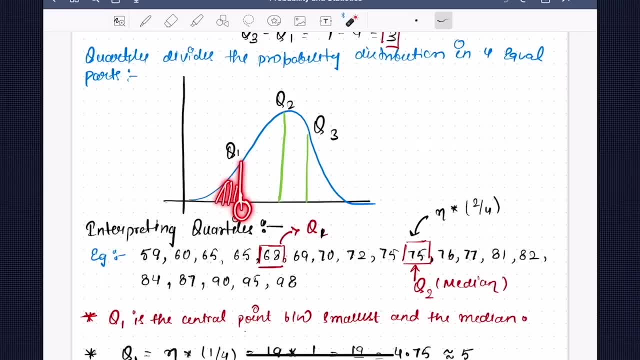 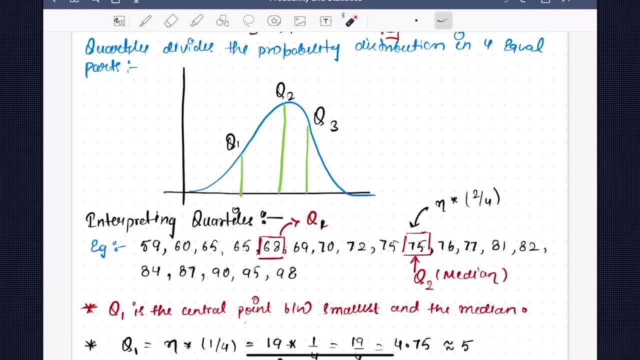 one says: the 25 percent of values are smaller than this particular value and 75, sorry, and 75 percent of values which are greater than this particular quartile, and how you can take out. you can take out by this formula. okay, i hope that you're getting one way to interpret it. q1 is the 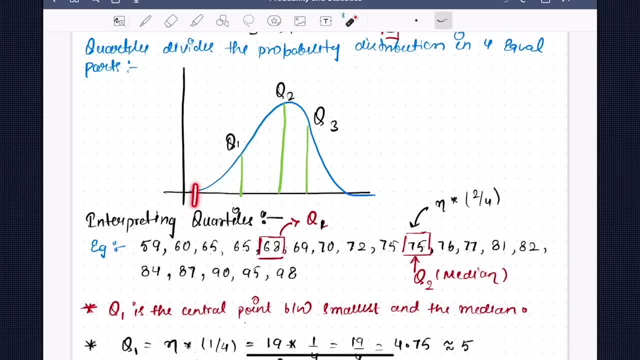 middle point. q1 is the middle point between the lowest value in your data and the median of your data. right median of your data: that that that is the because 50. what is the half of 50? because the median is called the 50th percentile. so what is the half is 2, which is a 25th. so you have to. 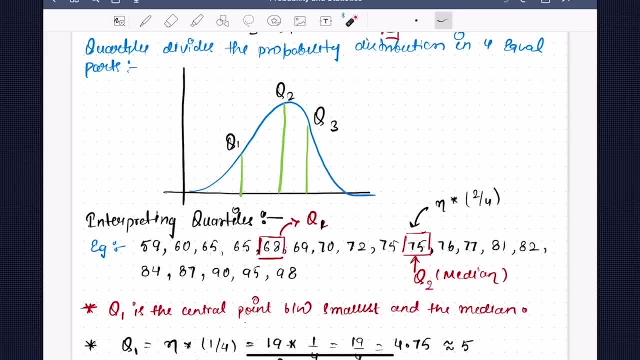 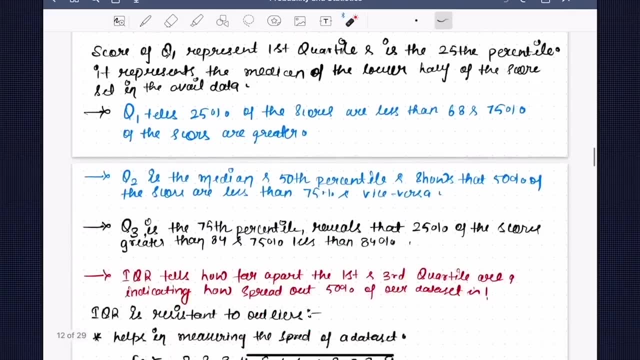 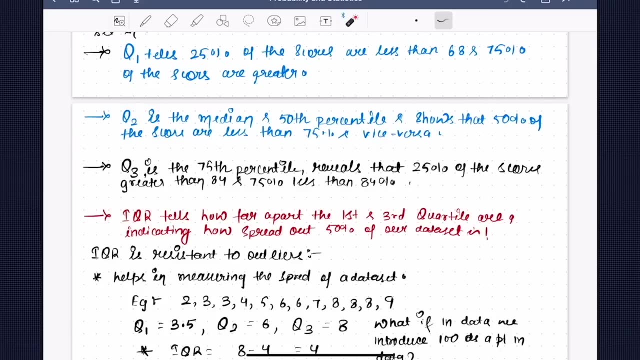 take the median, this is the central point between both of them, and q3 is the central point between median and the largest value, maximum value in your data. okay, this is the one way to interpret it. another one which, which which we are going to talk today, is iqr. what is iqr? iqr? it tells us how far 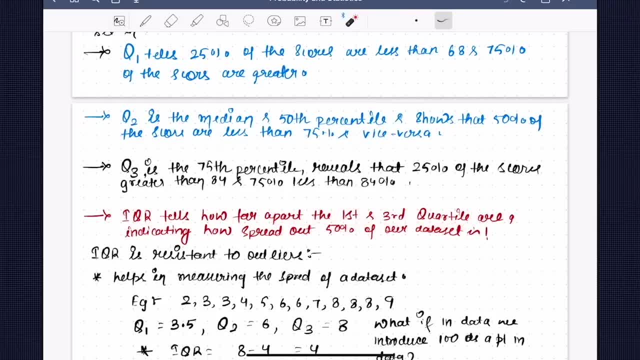 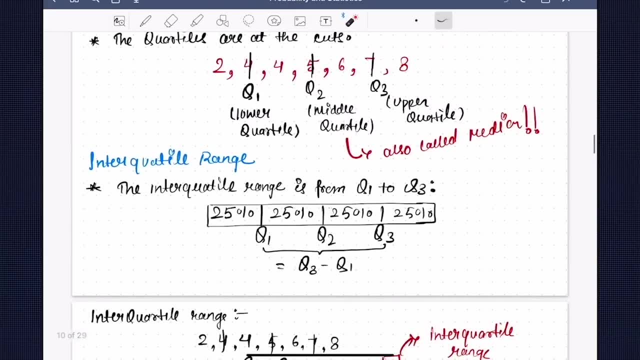 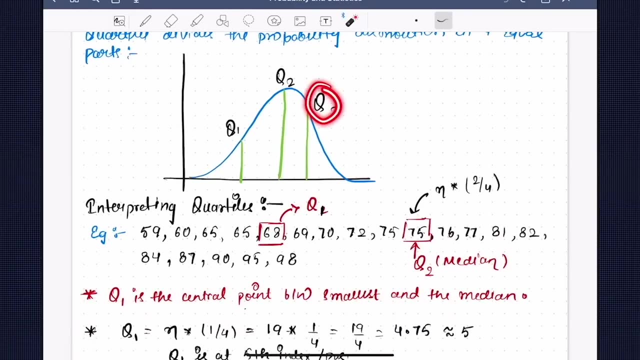 apart. your first and third quartiles are okay, indicating how spread out your 50 percent of your data is. so what it is telling. so what it is telling that um, um, what it is telling that you, um, take out your total number three and quartile number one, right, so let's talk about it in this. 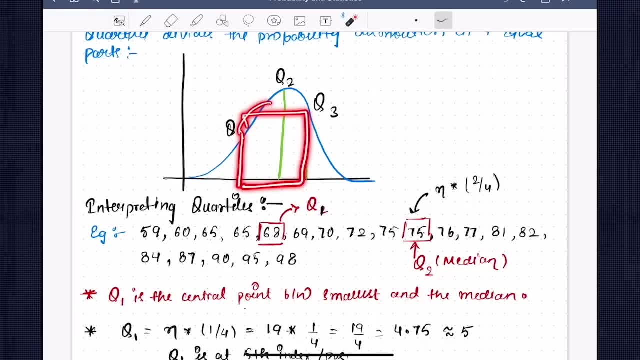 video. okay, what it is telling is that there is some social error. n equals three. at the first quarter, number three and quarter number one. okay, where it says that, because most of the most of the data lies between these two. right, because most of most of the data lies over here. 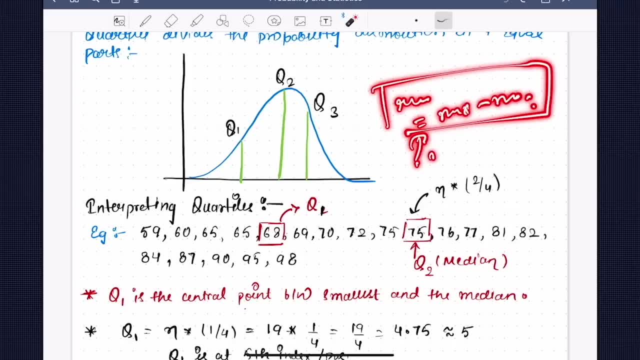 right, so we are not take out the range. how do we take out the range? first of all, if the simple range is taken out by maximum minus minimum, right, but that is, that is. that is um. that is um it is if we use our formal range, where we take out the maximum value and maximum and minimum value. 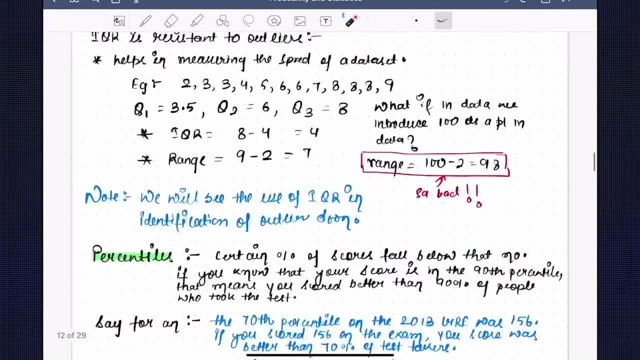 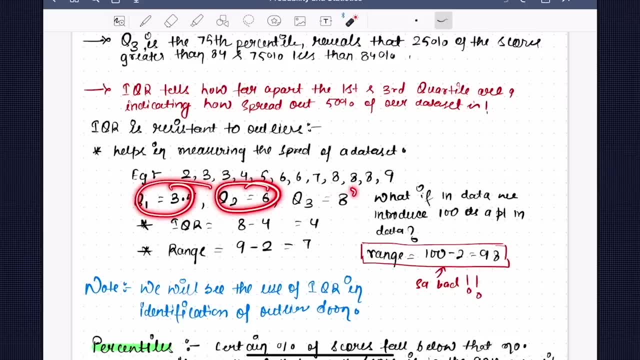 then it can lead to outliers, why you can see over here which we have listed it out. for example, you have this data out here right now: you have quarter number one, 3.5, quarter number two, six and quarter number three eight. okay, which are the cuts? so what? so we can say that there's 25 percent of 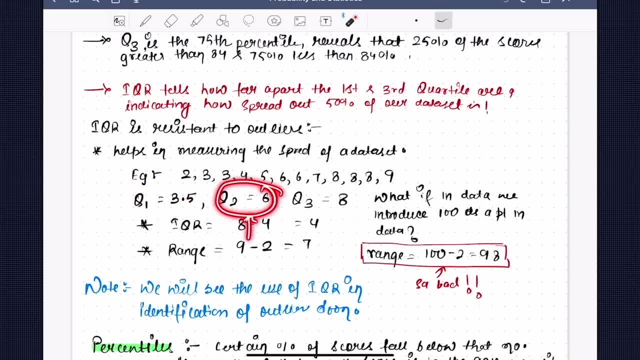 values which are less than three point five, fifty percent of values which are less than six and eight, with twenty five percent of values which are greater than eight. okay, so, so assume that, assume that you can take out IQ R, IQ R, which is which is the quarter, number three, which is which is the 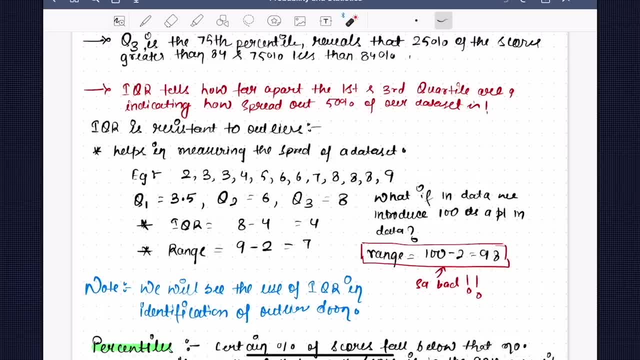 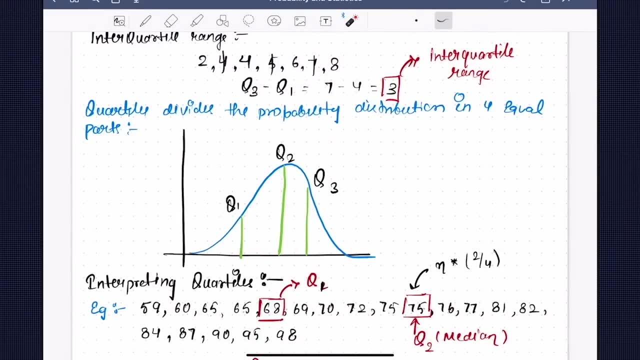 range of the range, of the range of the values, where your most of the data are present. okay, where your most of the data present, you should think logically as well. in this, over here we it is. we are taking the range of this particular. where are most of the data lying right? where are most of the data? 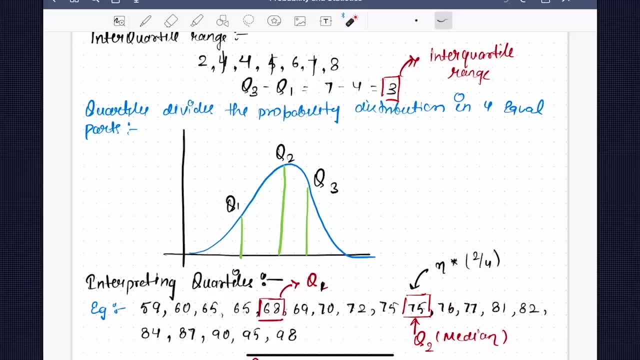 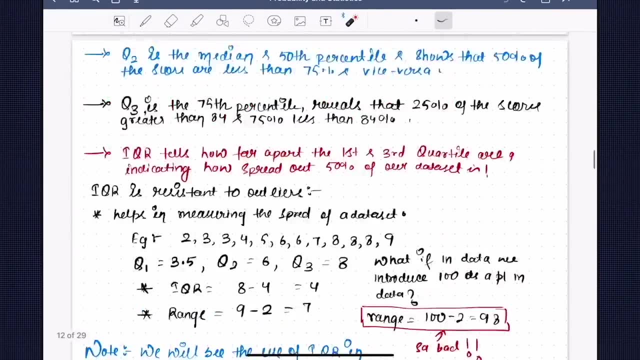 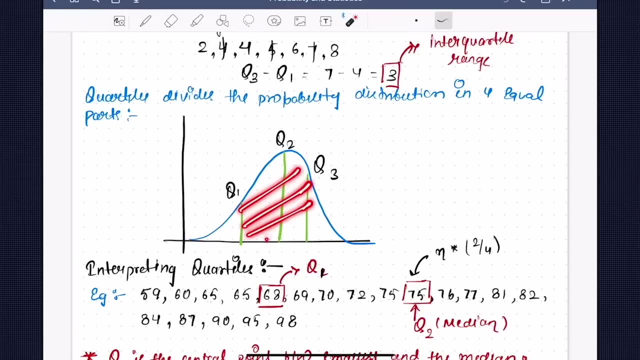 lying so they are not likely outliers. outlier are the one where they are out of the distribution, where they are out of the distribution right. so iqr is the it tells, it tells, it tells the range, it tells the it it describes the range between these two uh quartile number one and quarter. 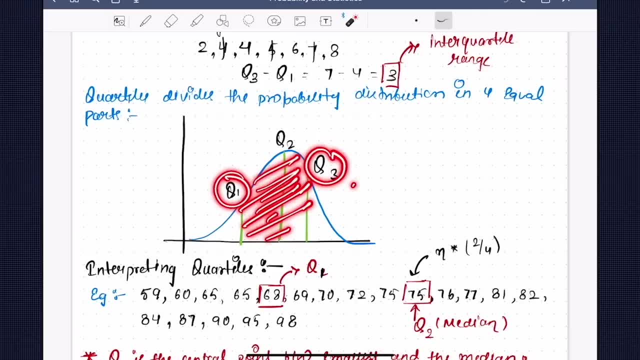 number three, where it says that how much your data is, um, uh, you know, uh, spread out, just like the range where you talk quarter number three minus quarter number one, because we just take out the range of this particular part of the data. that's why square number three minus quarter. 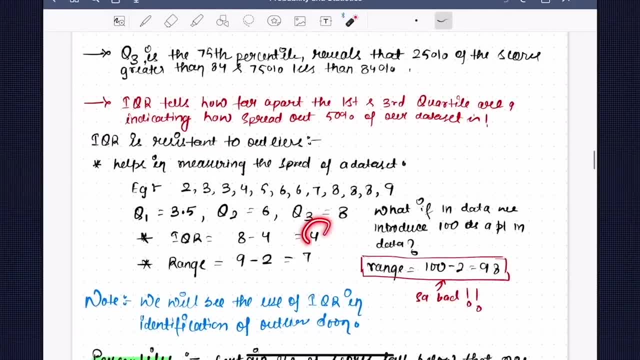 number one. we do so you get four and range is seven. but why we don't use range? why we don't use a range? because- let's take an example- we introduce hundred over here, hundred over here, so 100 minus 2, which is 19, 8, right. but but we, if we take a but quarter, but quartiles will not change over here the quartiles. 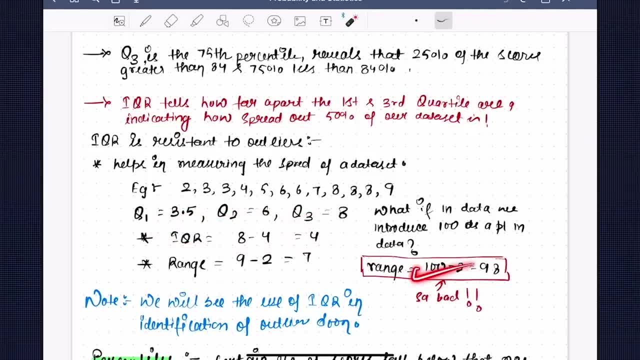 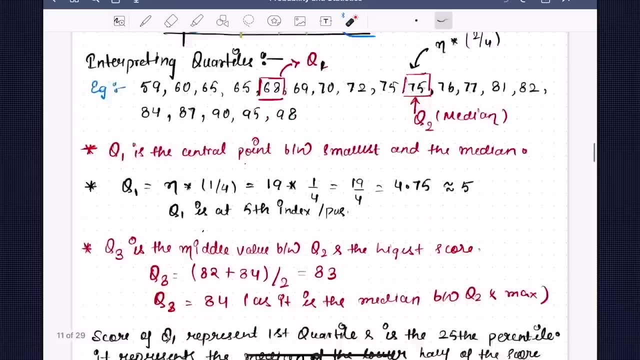 will not change. so our iqr will be resistant to even these outliers, but range will be affected, right? so that's why. so that's why where are most of the data are present? we take the range of that. that's what, the interquartile range. i hope that that gives a good, good sense of what exactly we 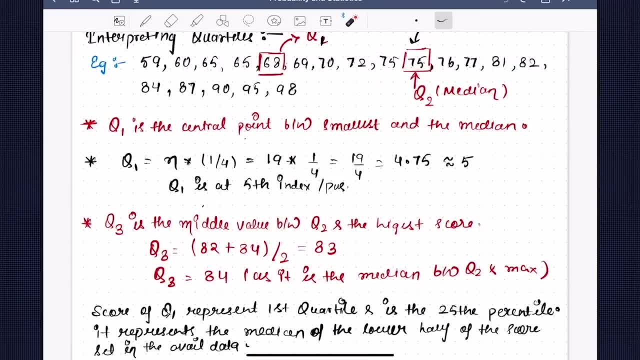 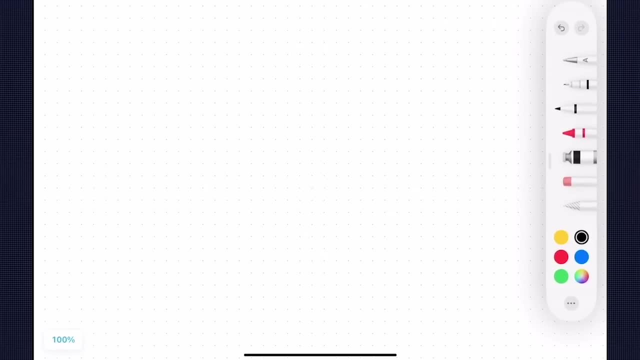 wanted to have a talk on now what i'll do in the next, uh, after the review of this, will talk about a very nice stuff, which is box plots. so, uh, let's go into the next lecture and talk about something known as box plots. so, hey folks, welcome to the another lecture on box plots. so 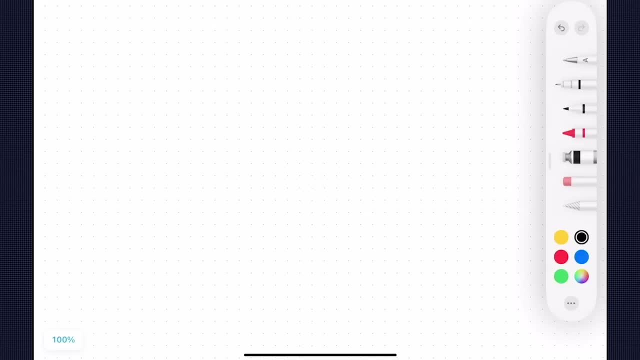 uh, eventually we have. i think we haven't had a good talk on box plots and all, but it's very easy there, relatively easy if you know about quartiles, and all right. so assume that, assume that you have a data, assume that you have a uh data out here. so let let me just first of all give 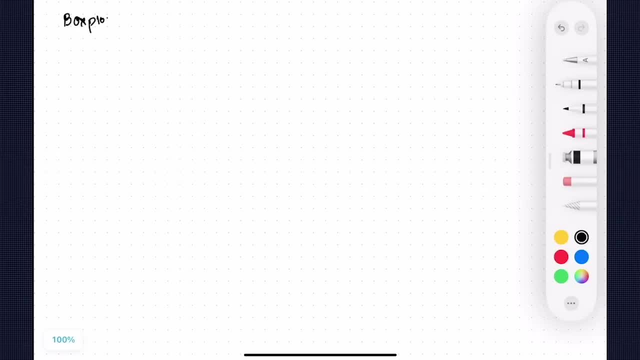 the title as box plots, right, box plots. i know my handwriting is not good, but that's something which i have to bear with, and we'll extensively use this box plot to do video night, to to do a nice thing, okay, um, so basically, assume that you have this data- 18, 34, and then you have 76, and then you have. 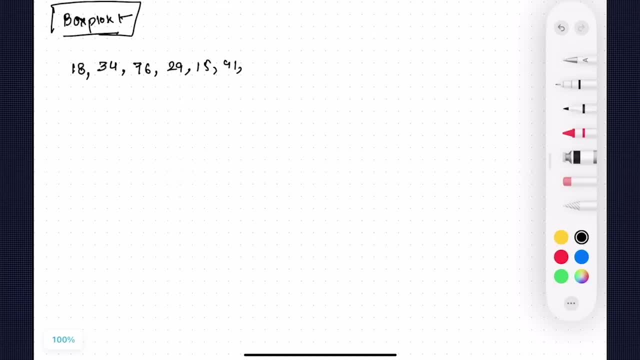 29, then you have 15, then you have 41, 46, 25, 54.. 38, 20, 32, 43 and 22.. so you have this data available out here now. the first step, as i told, the first step, the first step is to sort it right in an order. so when you sort it in an order, you'll have 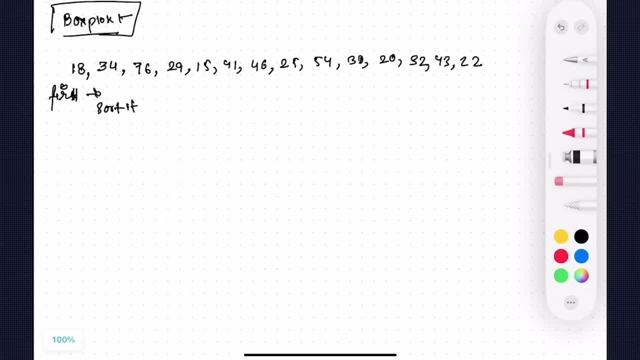 15. okay, let me let me use another pen. um, assume that you'll sort it on another order, which is 15, 18, then you have uh, 15, 18 is 20, then you have 22, then you have 25, then you have 29, then you have 32. 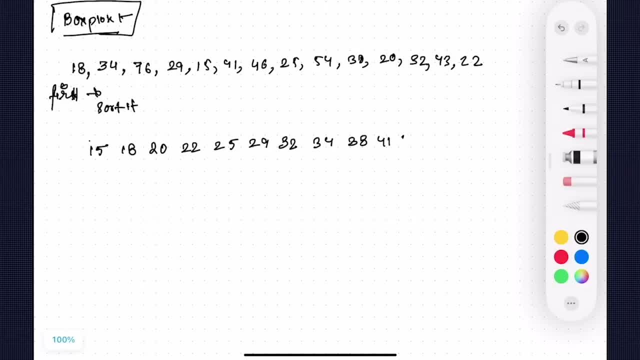 and then 34, 38, 41, 43 and 46, right, so this is our sorted data now. so now, once we have the sorted data, now, um, and then we have 54, sorry, uh, then you have 50.76. so now we have the sorted data. so now we have. 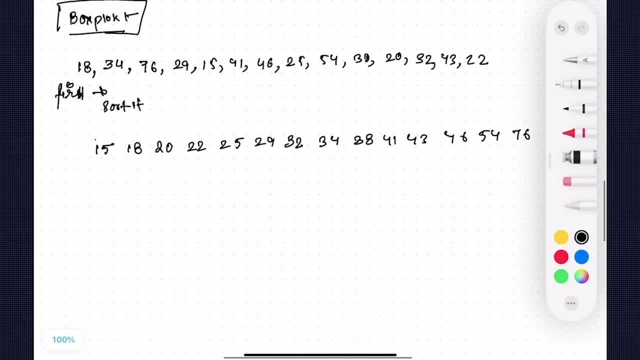 we have the total total now what we need to do right. so now, once you have that sorted, later you're going to take over quarter number one, quarter number two and quarter number three. right, that's our goal to take out. so how can we take out this? as i said, divide your data into. 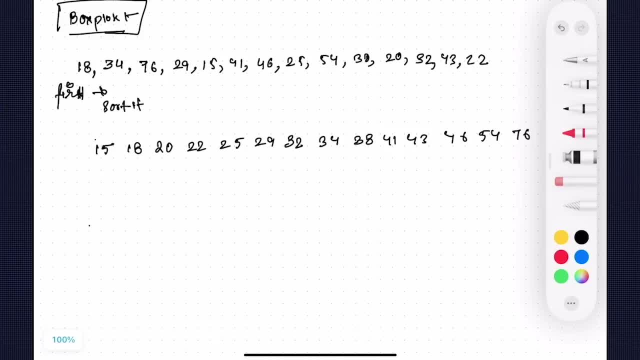 equal equal parts. first is divided your data into equal equal parts. so first of all let's find the middle value. so middle value, so first of all let's let's count the number of values: one, two, three, four. okay, so let me just one, two, three, four, five. one, two, three, four, five, six, seven, eight, nine, ten. 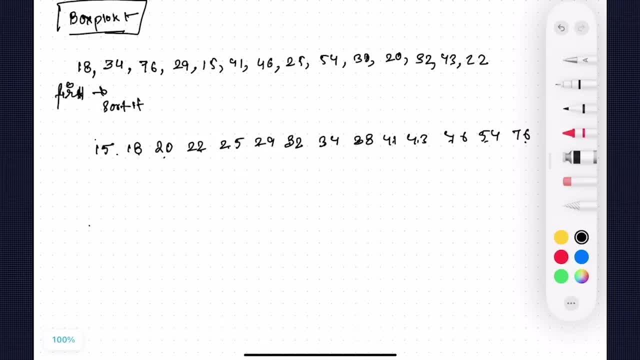 11, 12, 13, 14, so you have an even number of values, right? so that's something. so, basically, i've already conducted it. so when you take out the median of even then it, then then i think you should tell me the formula in your discord. so go over there and tell me the formula for median you. 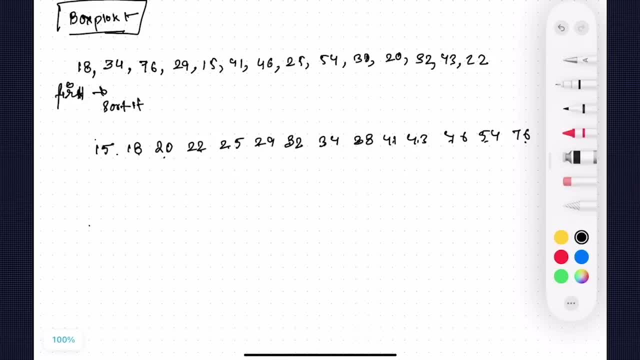 should, you should be able to. we have already covered this um, so the the median will come, will come, which which is over here, which is the quarter number two, which is around 33. so the values over here are the. the values at this side, on the left, left side, are the 50 percent of values. 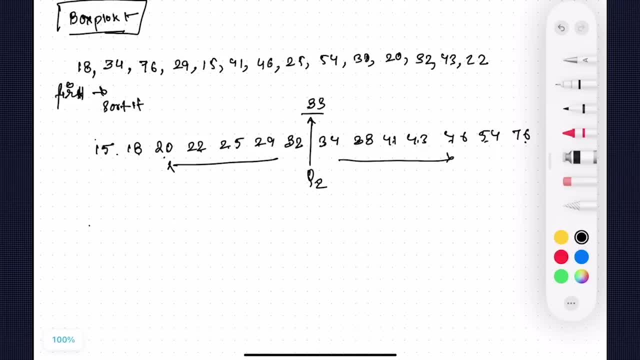 which are smaller than 33, and the values which is over here are greater than 33, which is the 50 percent of the values. i hope that that makes sense now. so now, once we have this quartile, quartile number two, now we are going to go forward to quartile number finding one. so quartile number. 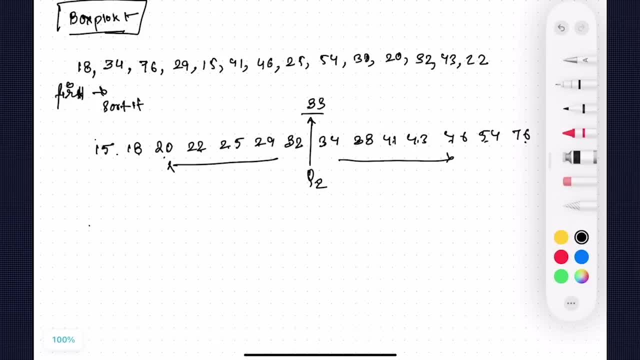 one we have to find. we can use that formula to find the index. i have already used it. so this particular is the quartile number, quartile number one. this particular is quartile number one. this particular is quartile number one, right and now and now we we want to find the quartile number three, which is over here. 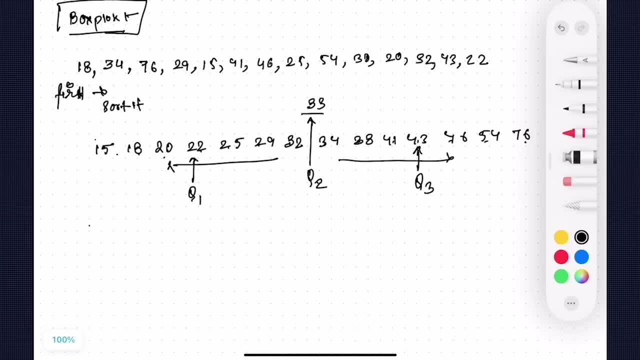 which is over here, which is quartile number cl我是三キ Z, so forward program three. so now you see that we have divided our data set into four equal parts: one, two, three and four. right one, two, three and four. so we have already divided our data into four equal 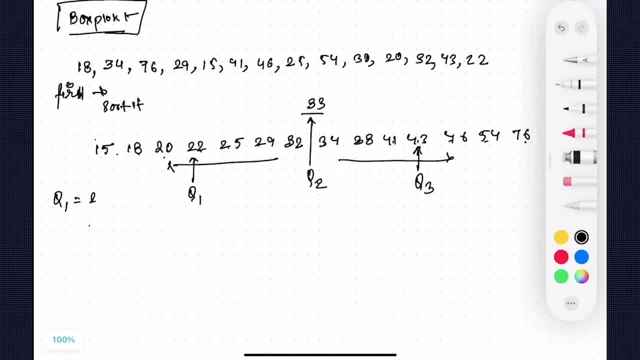 parts. so now your quarter number one is quarter number one is twenty, Quarter number 2 is, which is the median, which is 33, and quarter number 3, which is 43. So you have 50% of the values which are smaller than 22. Sorry, 25% of values which are smaller than 22, 50% values of smaller than 33. 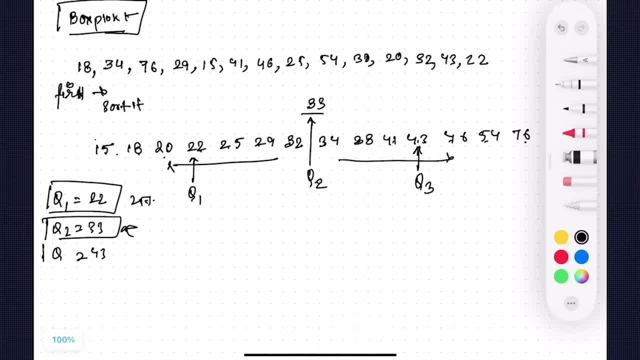 And then, and then there's 43 or sorry, 25% of values which are greater than 43, okay, So currently you have this particular example With it, statistically, which you have now, what, what, what we're gonna do the, as I told, let's take out the IQ. 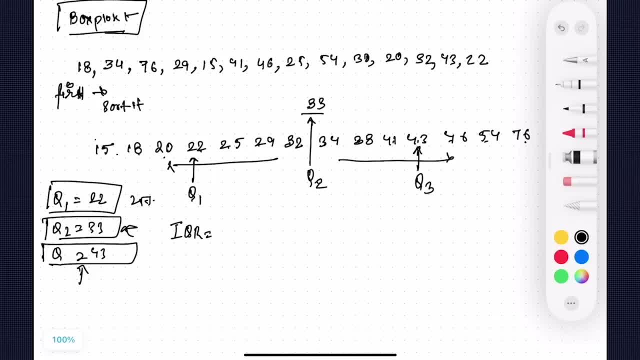 Are as well. IQ are right. What is IQ are? IQ are is the range where all the data lies in, right, which is Q 3 and minus Q 1? Where all your data lies in, which is 50% of a data, which is 43 minus 22, which will give 21,. okay. 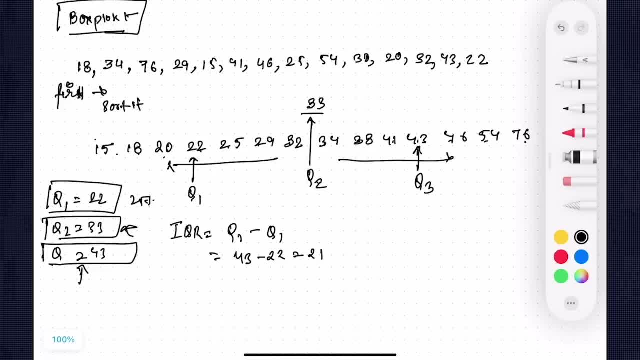 So that's what IQ are, so that's your IQ are. now what we need to do now: What, what? what we need to do, okay, first, is we can go forward if we can go forward with taking out the maximum. You know, we can take the minimum and then take out the maximum. 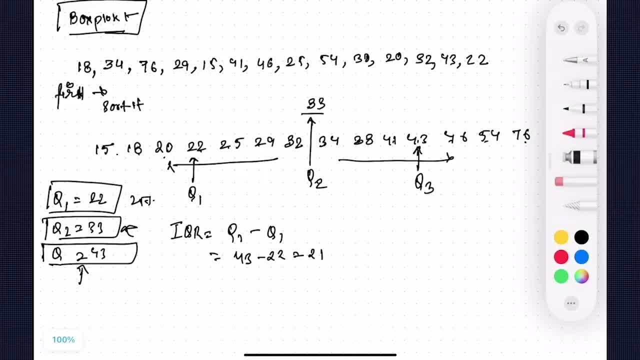 And then make a box plot out of it. but for outlier identification, for outlier identification, We need to make a viscour. Viscar, okay, you make this curse. So what is this curse? viscours gives you that a maximum, a maximum and the minimum value in your data, a. 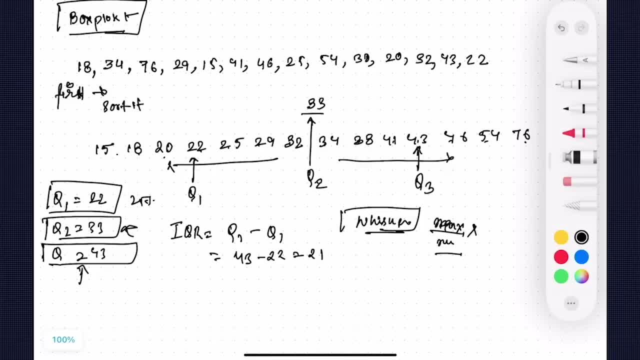 Maximum and the minimum minimum value data according to the IQ our range, right, according to the IQ, our range. so it gives the maximum and The minimum value in the data according to your this value, 21 according to this mass. So basically we have the maximum. and then if you say, if any data points go above this maximum, 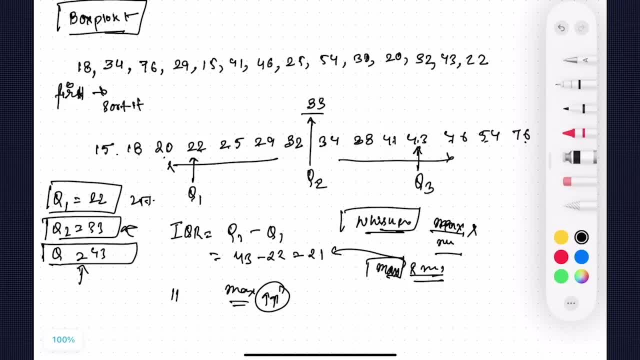 Then that's an outlier, or any data points which go below this a minimum, and that's also an outlier. So for outlier and the identification with respect to our IQ, because our IQ is resistant outliers, so we're gonna take out. so we have a viscours which gives us the 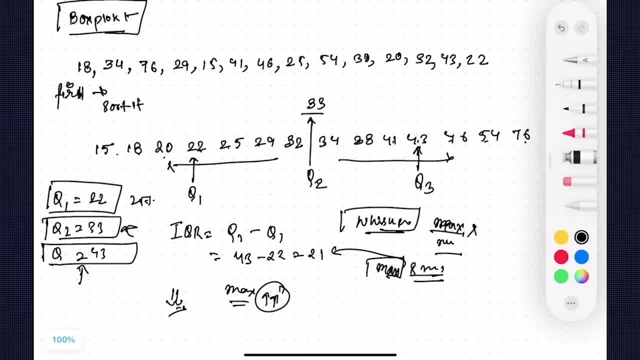 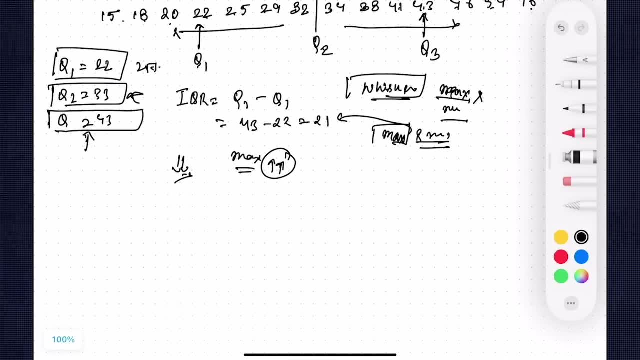 The, The min, a maximum, minimum values which are also resistant to our data, which which helps under Detection. you will get to know. just wait for a second second. now We want to take out the maximum and a minimum value. So minimum value can be taken out by the minimum value can be taken out by Q, I think. 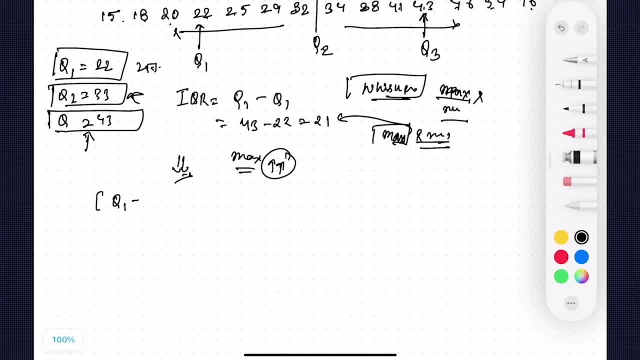 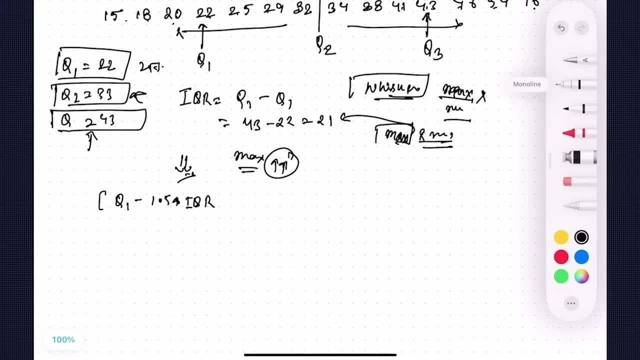 We can take out q1 minus 1.5 times IQ R. Right, That's the minimum value. That's the Minimum value, and then maximum value can be taken out: q3, q3 plus 1.5 IQ R. okay, so this is the formula for minimum value, for taking the minimum value in the data with respect to this out: IQ, our range and 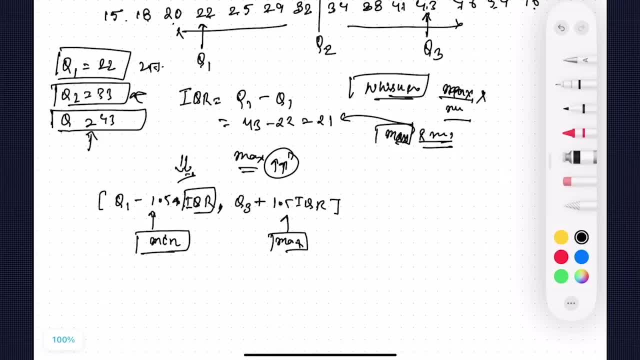 This is for maximum. Now you may ask: how that? how does this game? This is something which you can go forward, even if you want to recess. well, how does this derive? But that's a very general explanation behind this. but that's not a scope on this, my scope on this, to tell you that we want to 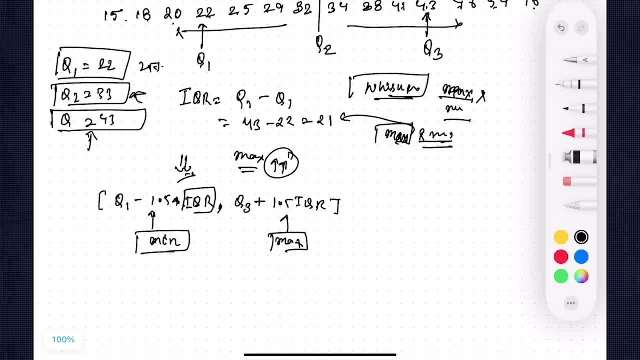 Find out the maximum and minimum values with respect to the outlier range. if there was simply the range or something, You're just taking the minimum and maximum values right, but that cannot be used as the outlier. I'll tell you that at last. why Q? why we cannot use the minimum and maximum, why we need to take out the minimum maximum with. 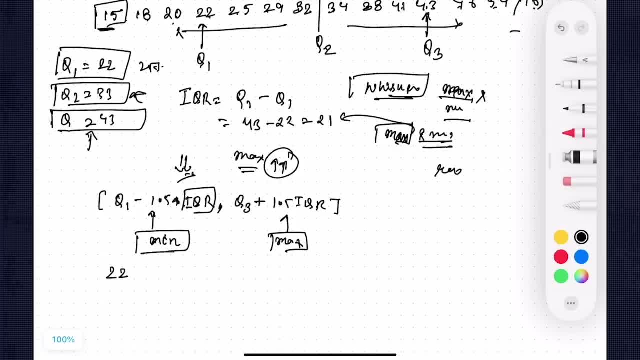 respect to IQ R. so if we do the calculation to 21 minus 1.5 times your IQ R, which is 21, and then Comma, because this for minimum and this for q3, which is 43 plus 1.5, Multiplied by 21, you get, you get 9 point minus 9 point minus 9 point 5, and then you get 74 point 5. 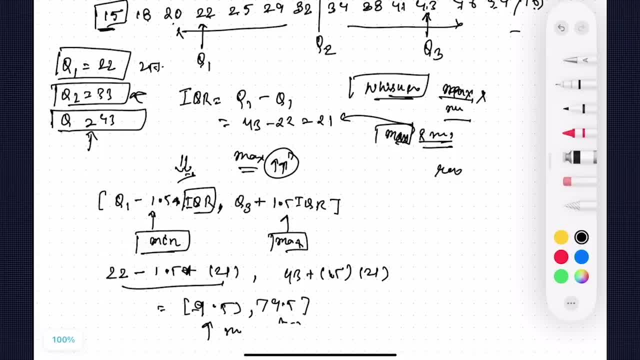 So this is your minimum value and there's a maximum value. So if anything goes above this sort, if anything goes below this minimum, if any data points go low, go below this data point, We say that 9.5 minus 9.5. if any goes above this, this is called the upper limit and this for the lower limit. 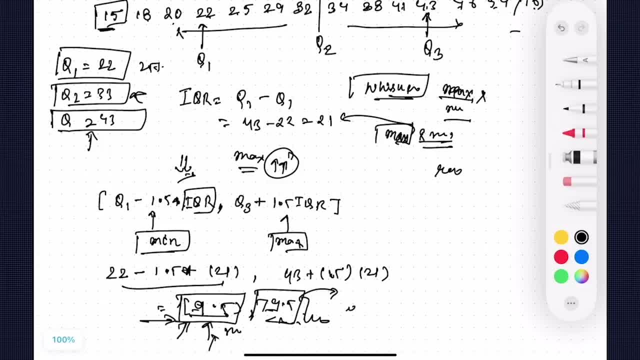 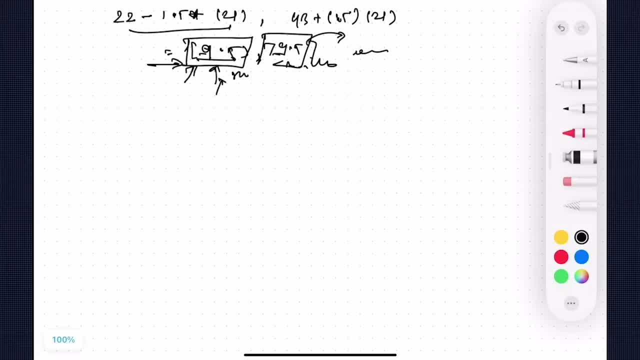 So, if any any goes above this, we say that that's thoughts an outlier. So let's try to do with the help of an diagram. So let's try to do with the help of an diagram. So I'll make a very nice diagram right now. So assume that you have a diagram over here. you have the diagram over here, a number line. 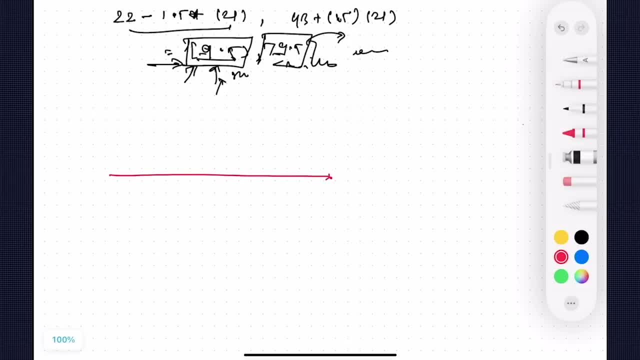 So let me just make a diagram like this and let me just use another pen. Yeah, so you have 0, then you have 20, 30, 40, 50, 60. let's make, let's extend this 70, 80, 80, right, so you have to. so you have this number. 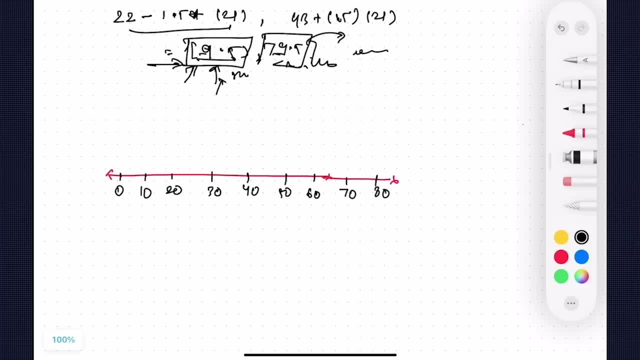 Number line out here now. now, basically what? what was our outlier? What was out our outlier? our, Sorry, what was our quartile? the quartile number one was 23, co quarter number two was what, 33? and quarter number three was 43. so it is slightly over here. So we simply make something like this: 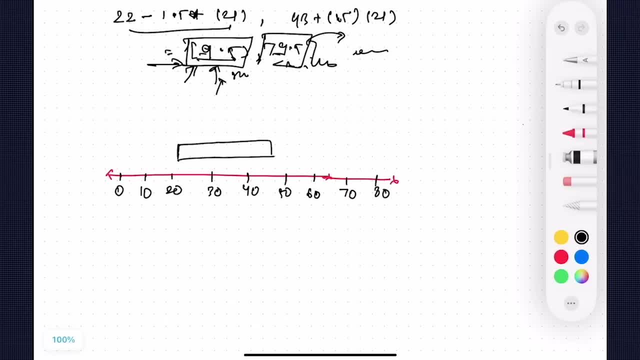 Okay, I know this something is not great, But this is, this is what it looks like and This is your quartile number. so now, this particular is quarter number one, This particular is quarter number two and this particular is quartile number three. as it makes it, it is 22, it is. 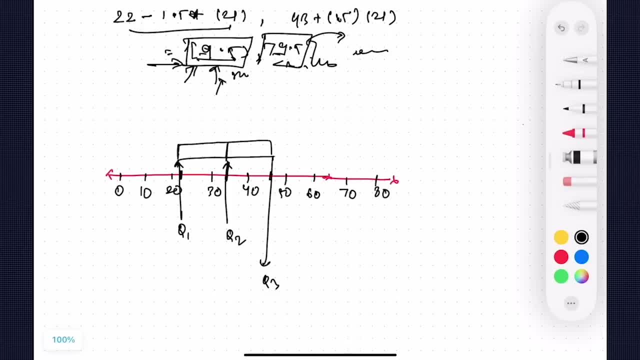 Cut, I think 33, and this is 43.. Okay, so you have these three outer court Quartiles as of now, which I've already seen. Now, we wanna, we wanna now one thing which we can do. we can simply say that something like this: we take out the minimum and maximum and then just 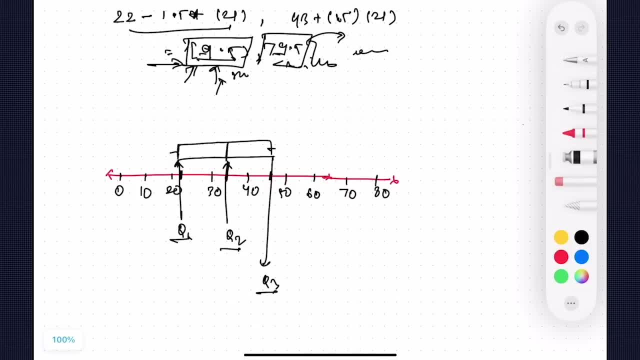 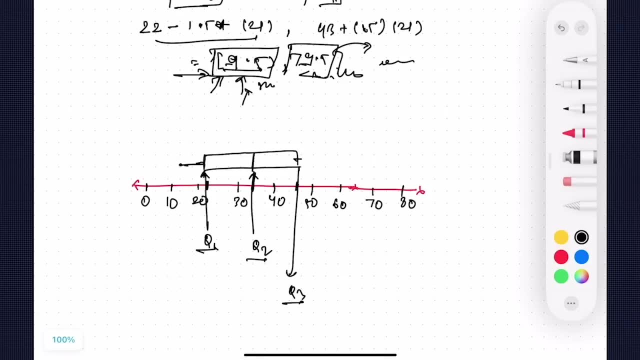 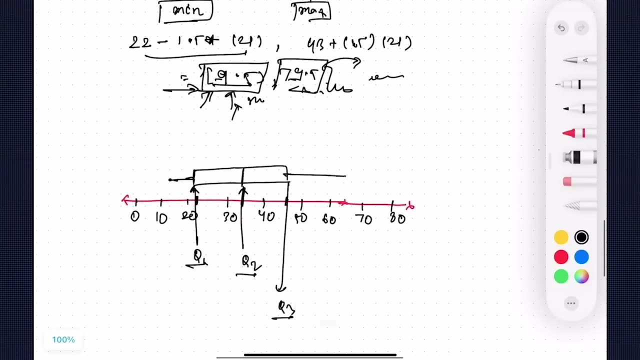 Add it. for example, in this case, the minimum is, in this case, the minimum is a 15. so we can have over here, you know, we can have like this minimum case, and then what is the maximum? maximum is 76, Maximum is 76, so we can have something like this: Okay, we can have something like this: 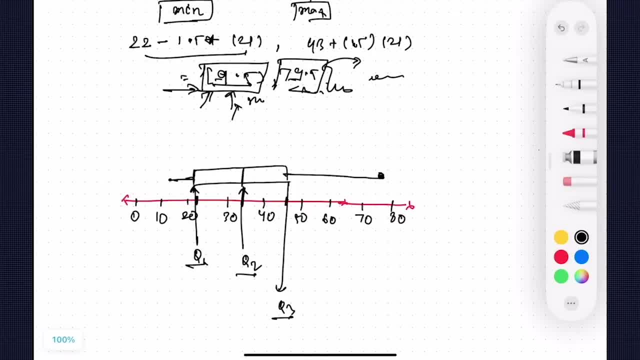 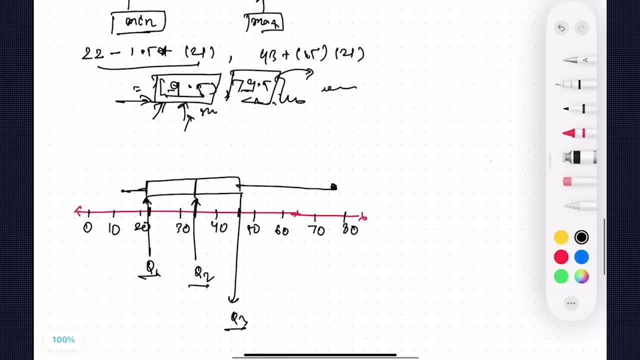 But it. but I'll tell you why it will not work. First of all, you see that 76 is out of it, bit out of the distribution, is bit outlier, or just by seeing it right. so So I'll tell you why. Why it will not work. first, as we said, as we say that IQR is resistant to outliers and IQR represents the 50% of our data. 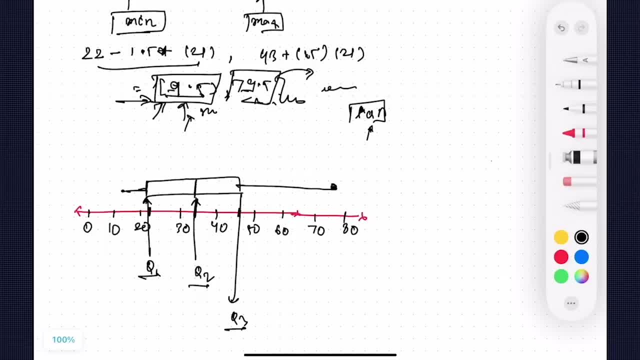 So if we take out the maximum and minimum value using IQR, that makes makes more sense because we'll be able to identify Where are most of the data lies. So if any of the- if any of the data goes out of that lie is spreading out, will consider that as an outlier right. 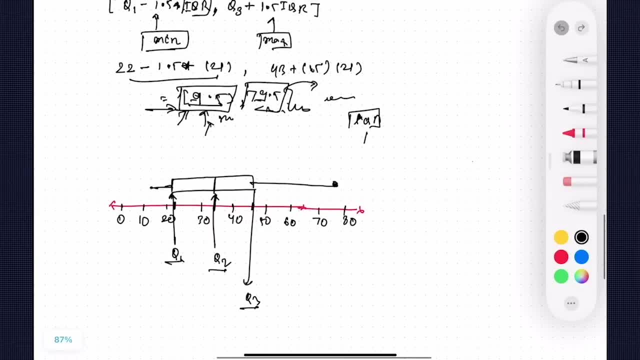 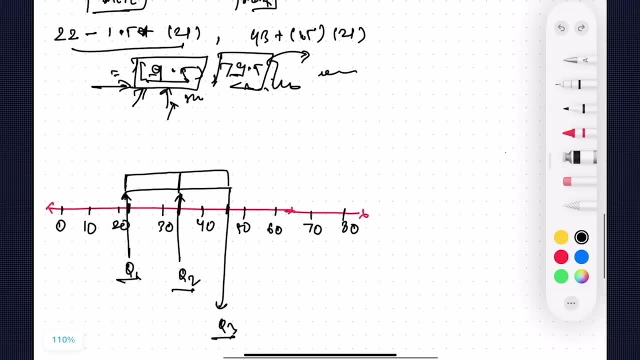 So now. so now I think it will makes more sense if you just try to now makes it make. make it more sense, Sense, sensible, yeah. So now we wanna. we have this minus 9.5, We have this minus 9.5. Where do we say that here? 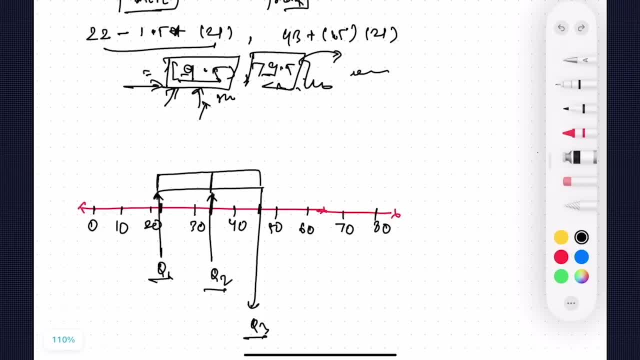 We say that we have, we make a vesha, We make a vesha, make a vesha which is minus 9.5, Which is minus 9.5.. So, and then you have the service 70. I think what was that? 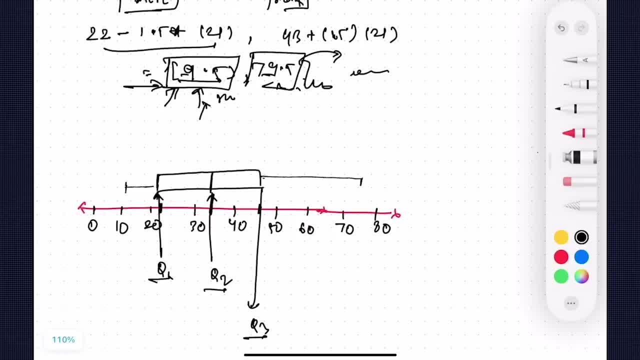 It will be something over here. So anything, anything which is now now, anything which is which this is for, This is for the maximum, for the maximum value, And this is what: the minimum value, okay, so, maximum, and this is for minimum value, okay. so anything, anything, any. 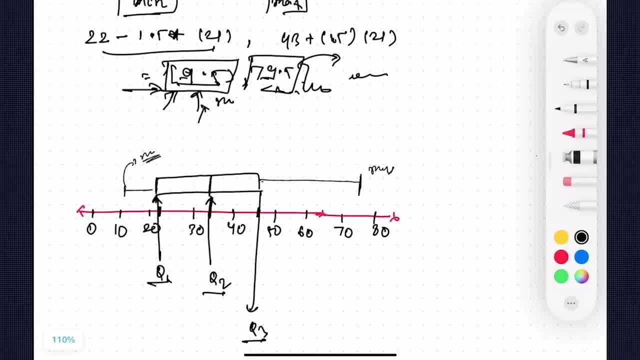 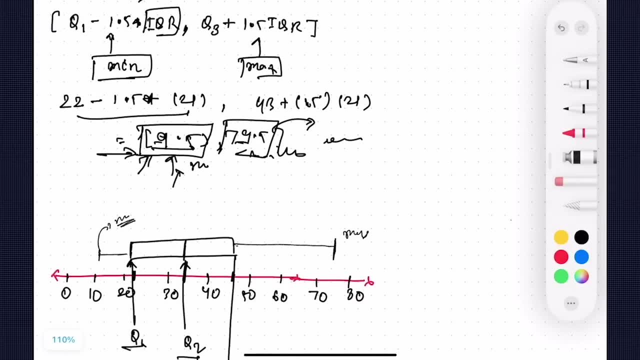 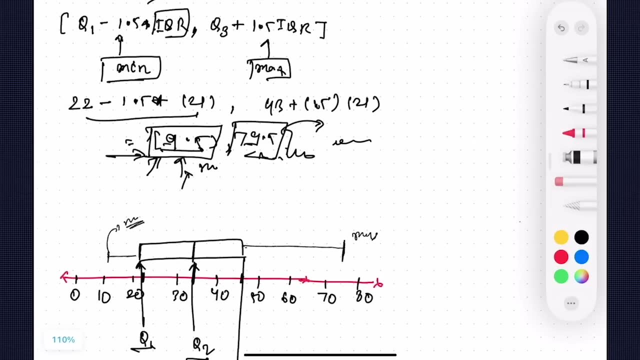 our data. so how can we use this to remove our data? how can we use this to remove outliers from our data? so we say that anything below minus 9.5, anything which below minus 9.5 is outlier, anything above my, above 74.5, is outlier, because this is the distribution, this is the range of our, of our. 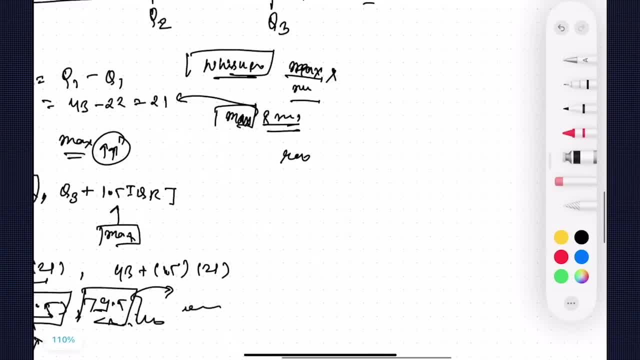 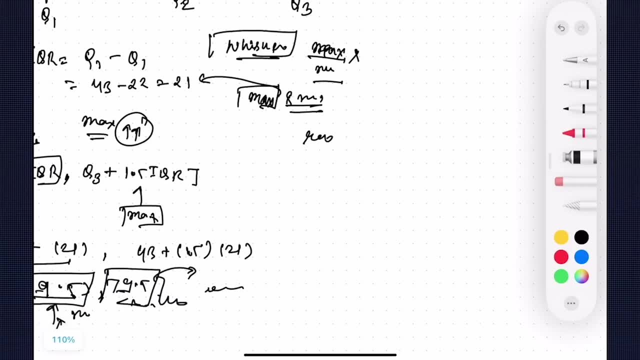 maximum data. where are most of the data? so anything above this. so, if we see our data, anything below minus 9.5, there is no anything below minus, but there is um above 74.5, which is 76. so we simply say that we consider this particular thing as an outlier, this particular thing as an outlier. okay. 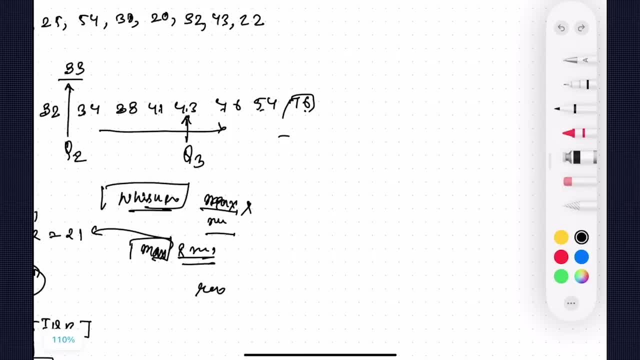 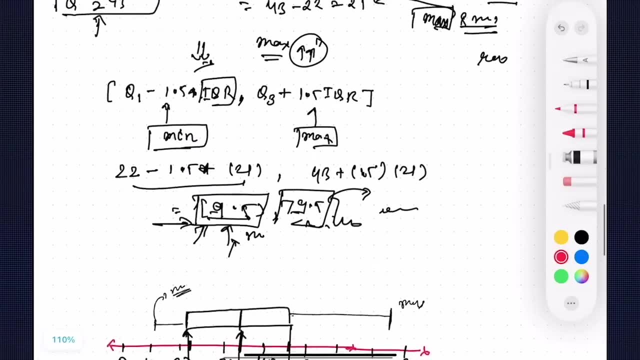 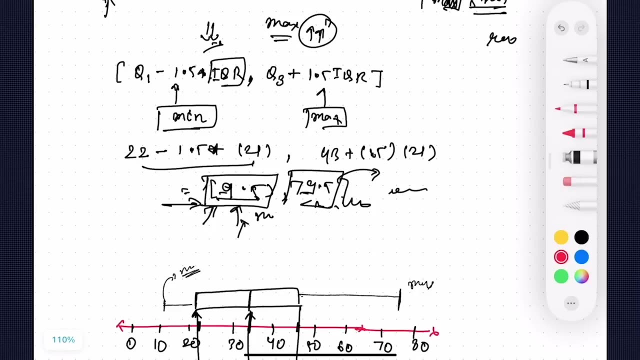 this particular thing as an outlier, this particular thing as outlier, and we remove this data from our plot, right from our data. so we remove that outlier right there. you know the linear regression there other, there's lots of algorithms that are sensitive to outliers. okay, so you have to. 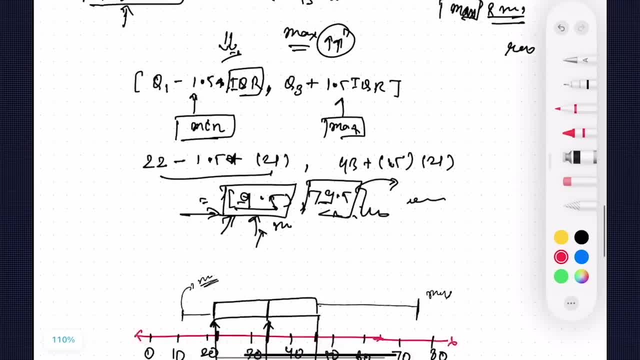 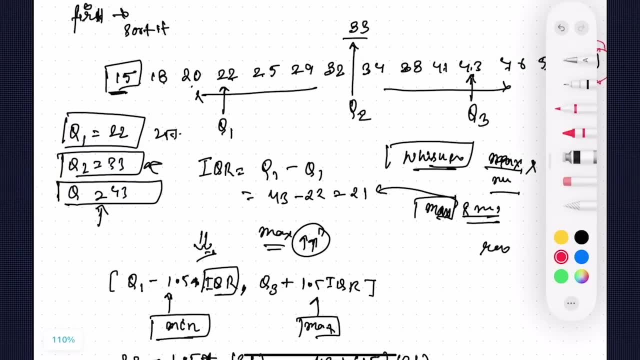 remove these outliers will, which will study later on as well. so we'll remove this outlier by a box plot where i'll summarize the concept. you take out the, you take in order, you take out the quartiles, you take out the iqr, you take out the maximum and minimum value by this formula: 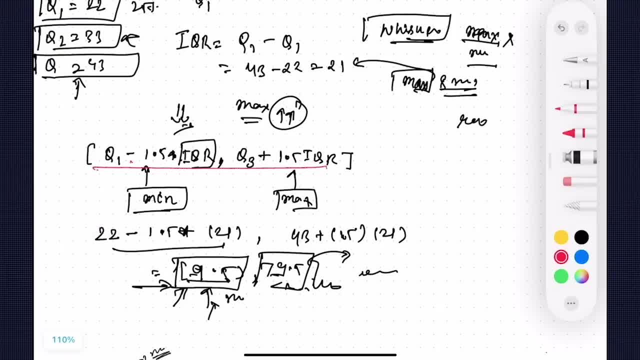 by this formula, which is, which is out here: q1 minus 1.5 times iqr, q3 plus 1.1 for maximum, for minimum. anything above this is bad, anything above this is outlier. anything below this is outlier. i hope that makes sense. let's catch up in the next lecture to actually see the practical effect and 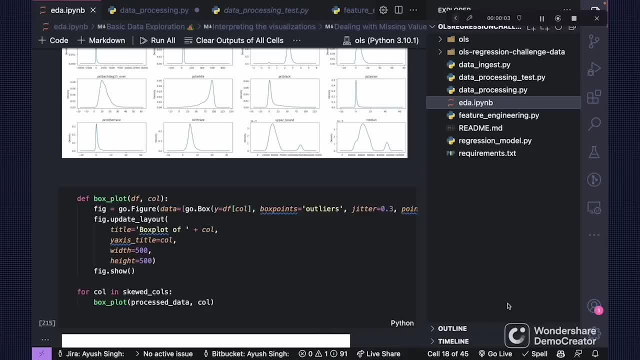 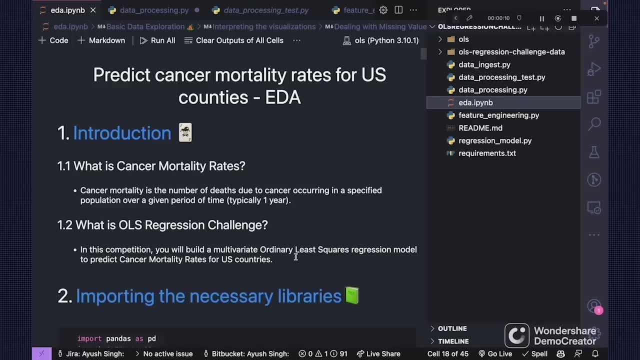 how we actually do it to identify outliers and how we actually do it to identify outliers in your data set. hey, everyone, welcome back to another video. um, so now what we'll do. we'll start off with you know eda stuff and uh, processing stuff which we eventually need for our project. 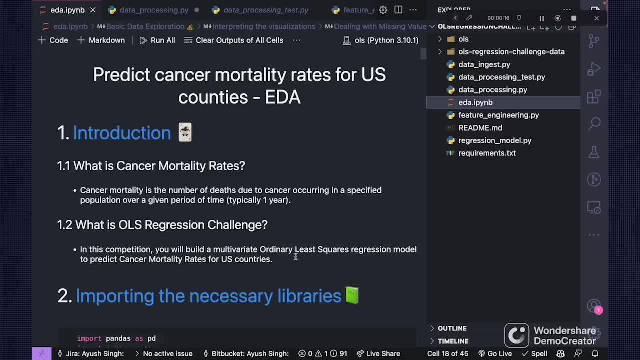 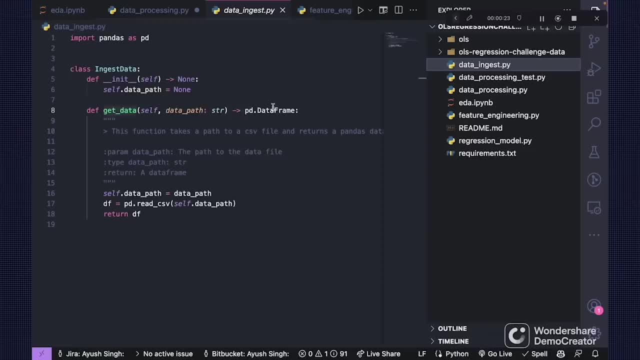 and i'll make sure that you understand each and every concept in great detail. uh, so you can actually read all of this thing which you have, which you have done, done it for you. but let's start off with: uh, we have, we are done with the ingestion of the data. now let's start off with. 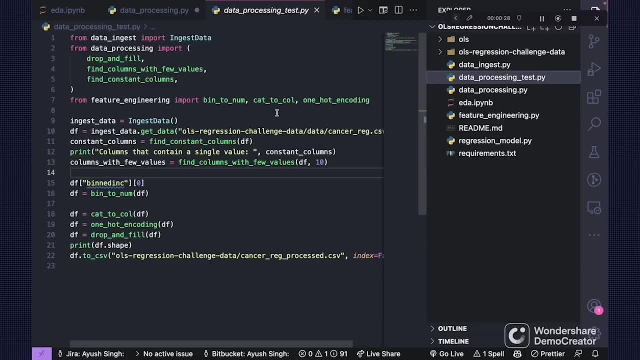 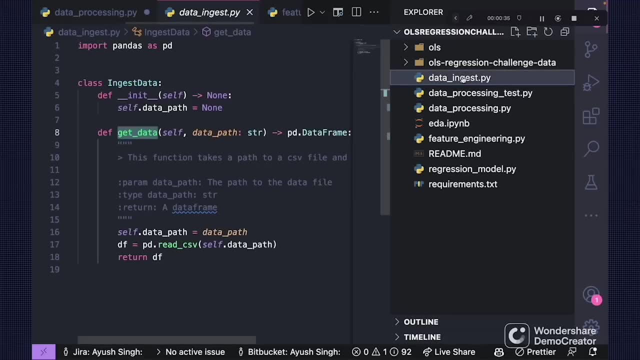 this file. don't know what's. what's this file? don't worry, we'll figure it out. the first line of the first line of the code says that we ingest the data from our data ingest file. so it goes in data ingest file. it ingest this class. so if you click over here, if you click over here, you'll be going. 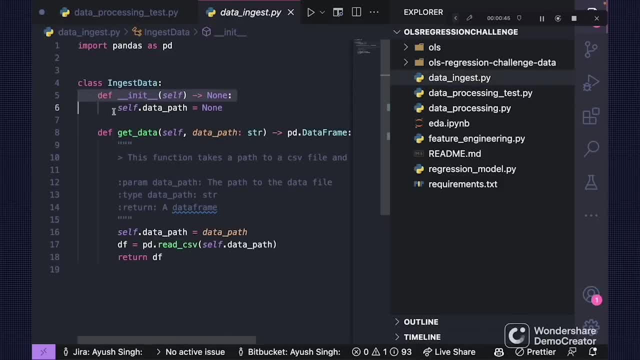 to this ingest data class and over here in this class you have the init method, which is a constructor, and then you have a method which is get data, which where we ask for the path of the data, where the data is present in your folder, and then we read the csv. if it is a csv file, we read. 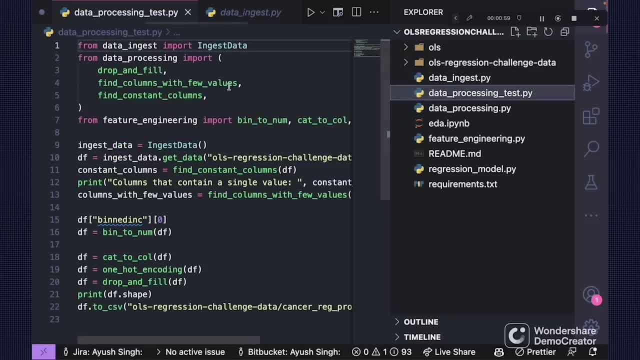 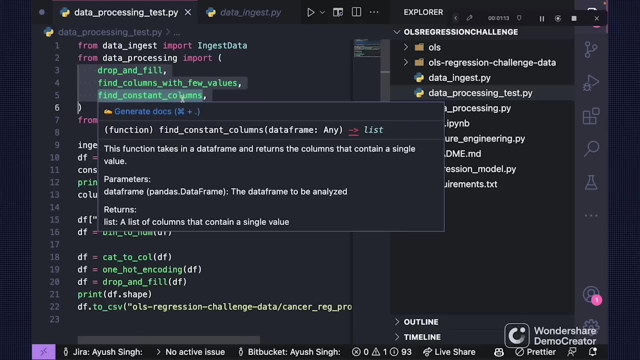 that okay, and then we return the data frame right. so let's see, it goes into ingest file and then we ingest data. it's, it just imports that class. then it goes in processing data with it, goes in processing file and then it imports the following columns, which will take a look in a bit. you have 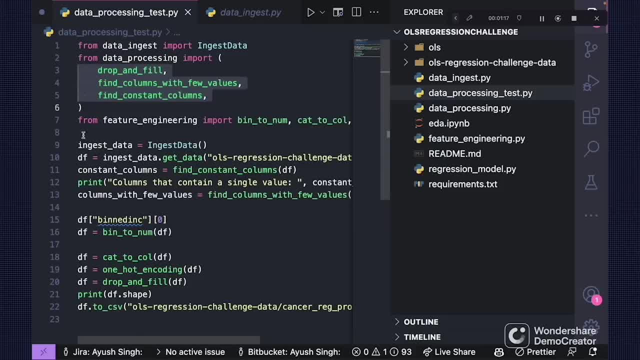 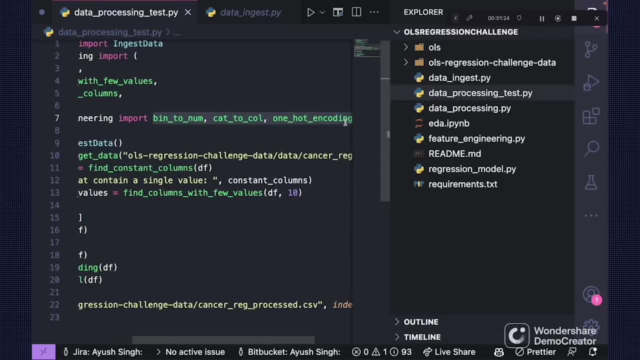 to just wait for a sec, right, which will take a look in a bit, and then you have for from feature engineering we are import via. there is another feature engineering file. they're importing some functions which is important to us as of now, right, which is important to us as of now, right. so now, 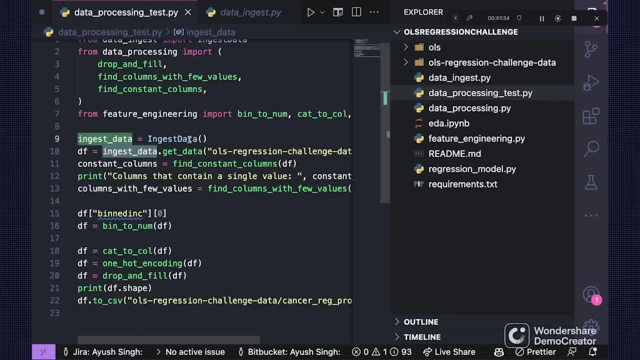 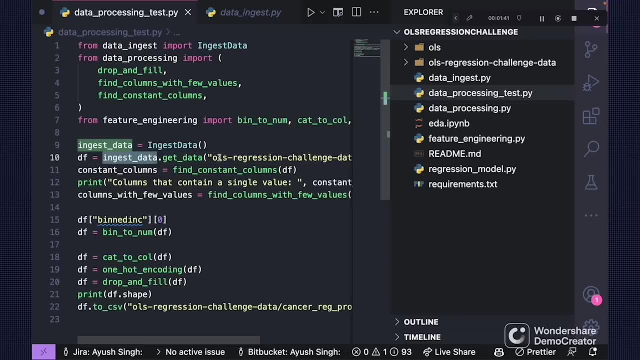 we have ingest data and it's we, we are, uh, we are. you know what? what we are doing? we are simply um, instantiating a class and then using that class, as we say, we are using the method of the class, if you see that method methods get data over there. so, using the method, ingest data, which is the object. 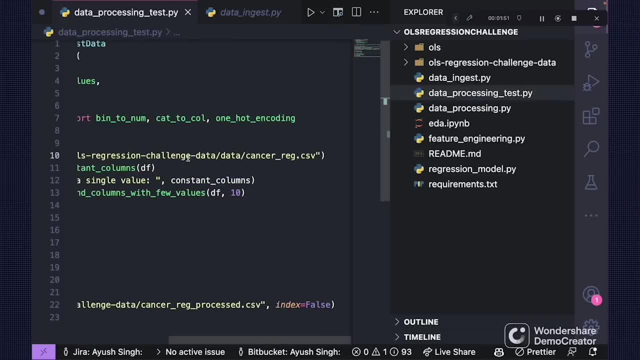 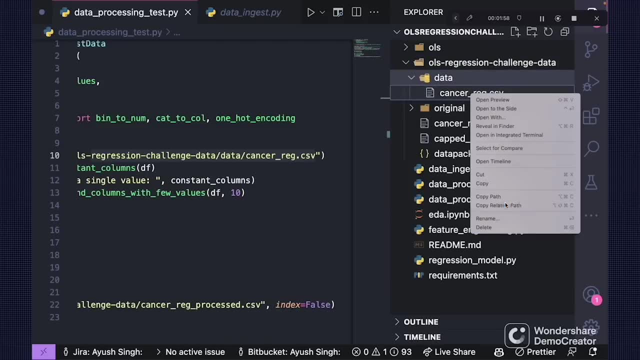 which is the blueprint of the class. we say that we will get the data from the following, uh, from from from the following folder. so we go to ols, we go to data and then simply copy the relative path of it, right, and then we import that. and then now, once we have the data, now it's ready to start with some of the processing, which is: 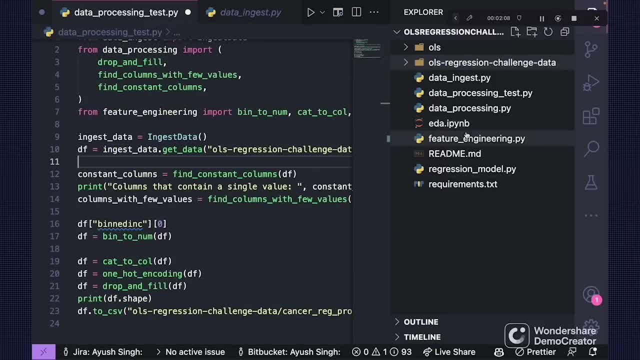 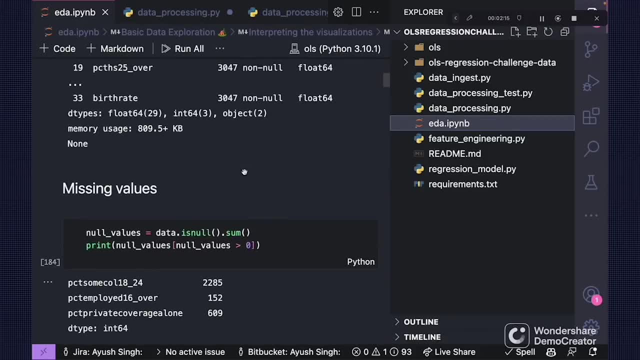 required as of now. but before processing- uh, what? what i usually like to do, i usually like to, you know, go through all the basic data. you know, see how, how's the data looks like. you know, see some of the missing values, if, if i have any, and talk about distribution. right, so let's, let's, let's. 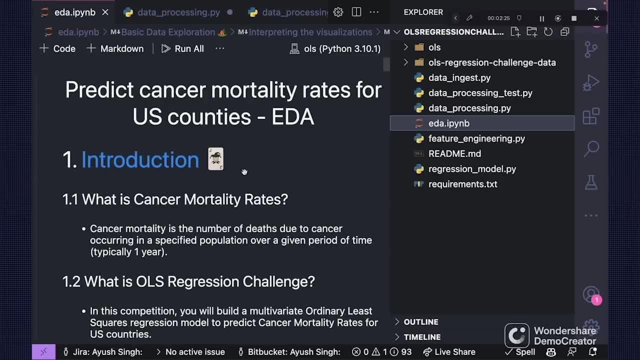 before going on the distribution one, let's before going on a processing one, i would like to take a time to explore a bit of, you know, explorative data, analysis and analysis and all. so let's go through all the basic data. so what's, what was our project? our project was to identify the number. 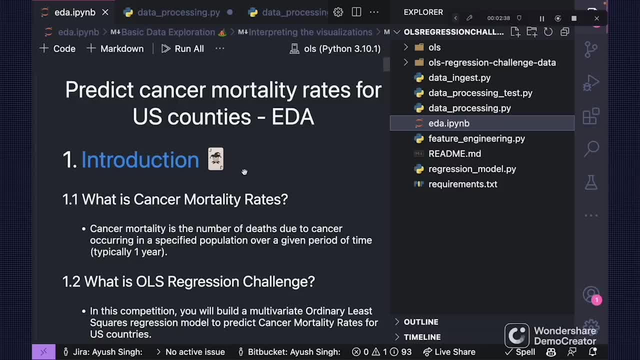 of deaths which was due to the cancer in a specified population for over a period of time, typically one year. so mortality rates are nothing but a number of deaths argued for a period of time. in this case we have. we have given already. in this competition you have to build a multivariate, least squares. 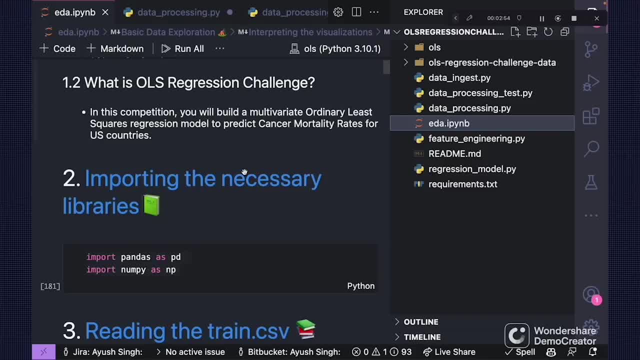 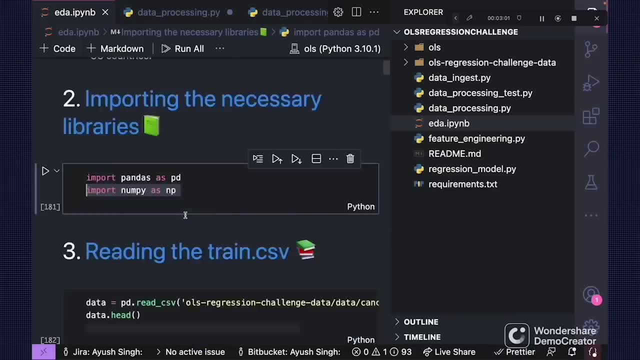 competition to predict the cancer mortality rates for us countries right? the first step is, of course, we are going to import the libraries. of course, sometimes i've imported in a bit between as well along. so we import our libraries as of now. we need pandas and numpy. we pfpd as an ally so that we 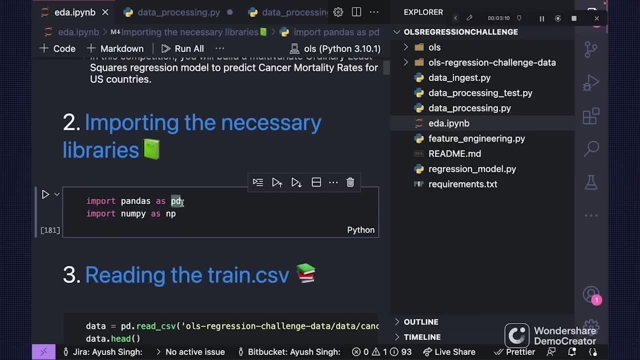 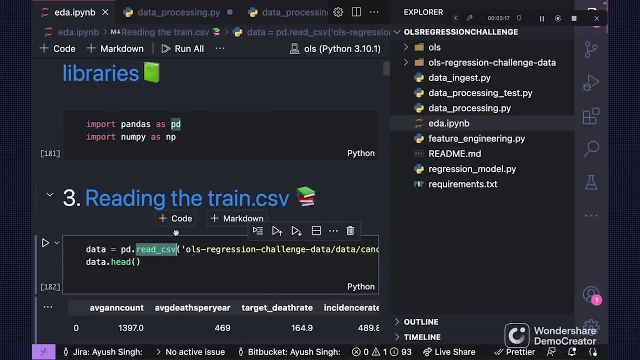 don't have to write pandas dot every time to use panda. so we have pd where we can use this pd. now, one thing that you, which you do using a way, we are not importing that class just for sake of you know, simplicity. i just added it, you know we can give it to any people, so just for simplicity. however, we 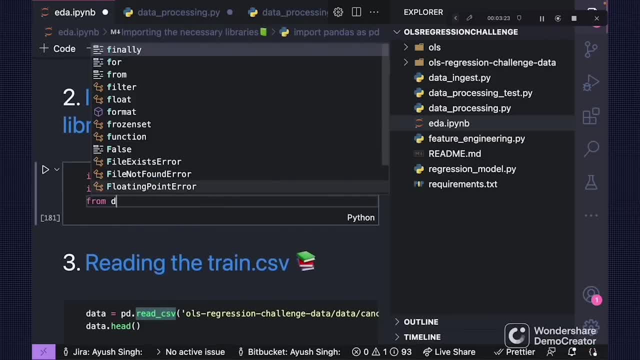 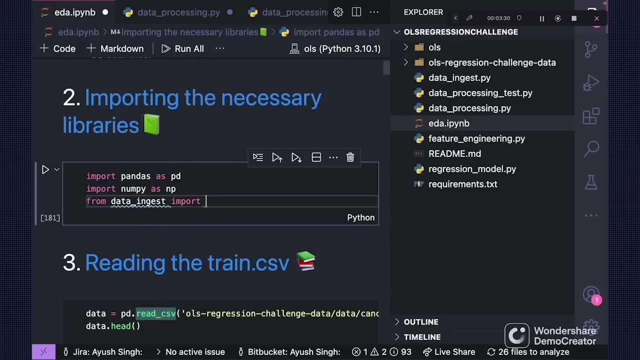 can use that. we can simply import the you know from data uh from data ingest, uh from data ingest, and then we simply import the. i simply import the ingest data file and then we simply make a you know, uh ingest data, which is- i just going to comment it out- you. 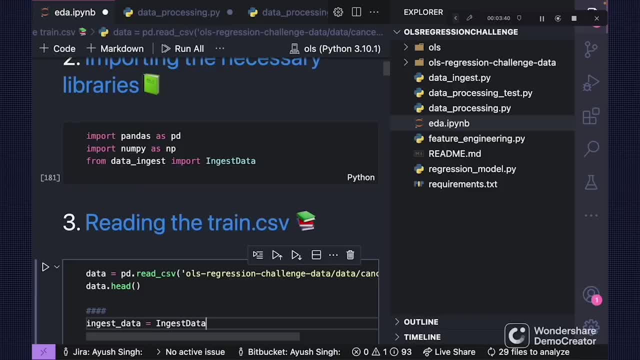 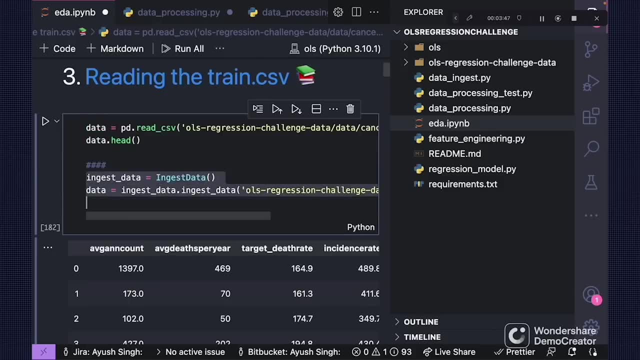 know ingest uh data, which is ingest data, and then simply say, uh, data is equals to ingest, so you simply have this uh to actually import the data. but as of now, i just imported that because of simplicity, so that you could be on the same page rather than going over this. so if anyone is seeing 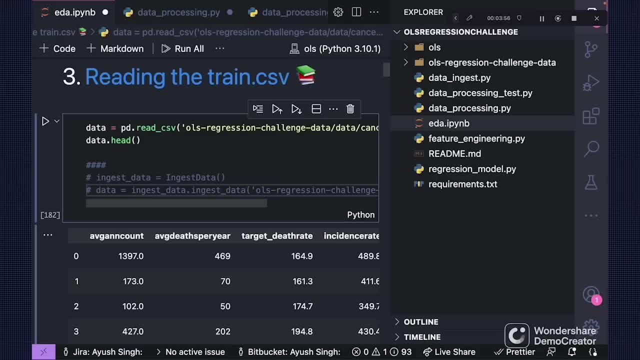 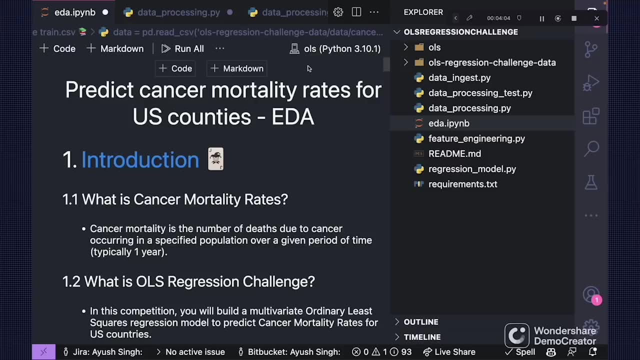 adh, they should be able to understand it very well. so now, once we have the data, so now let me start running it. so before that, i would like to just tell you that we have to uh over here. you have to activate your environment in jupyter notebook as well. 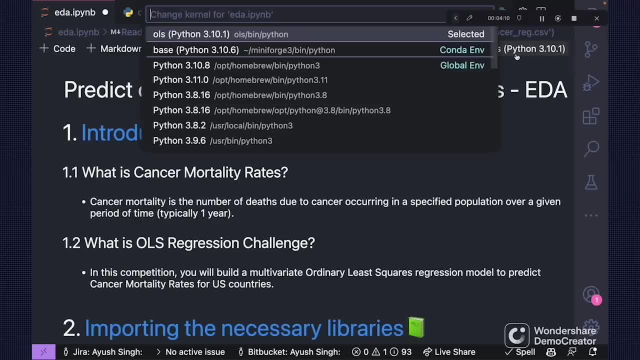 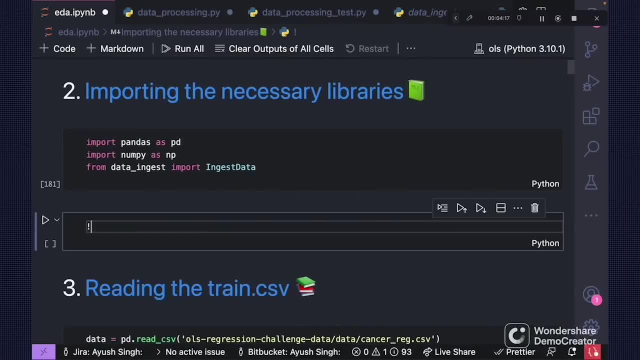 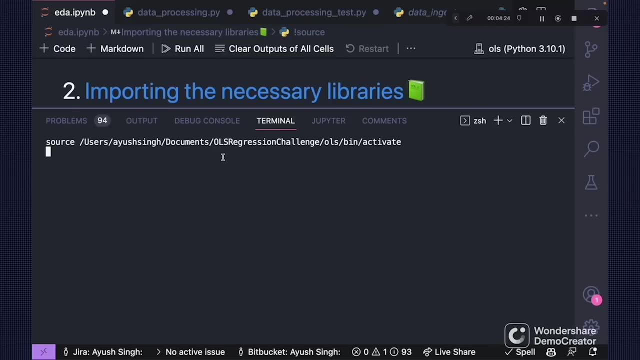 in in. uh, in vs code we have this. we have this select selecting of our kernels. but in vs code you can simply write. you can simply write like this, a source, and then you simply have the following command, which we have used earlier. so now you see that we are using source and then it. 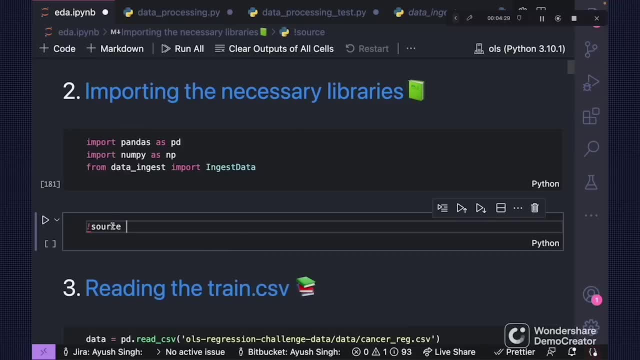 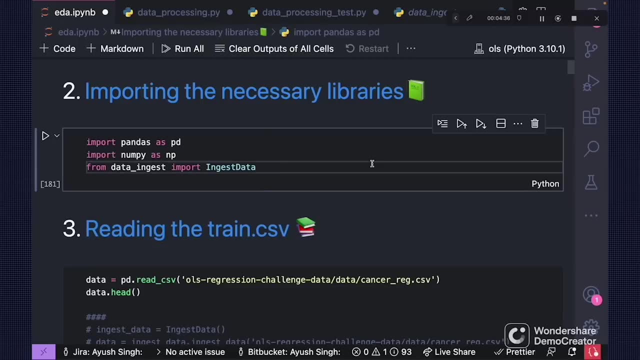 is activating it, so you can simply use this as well. you can simply use the this as well. source: simply give the activate, it will be able to activate for that particular environment. however, you can change the kernel as well according in your vs code if you have issues. if you're having issues, 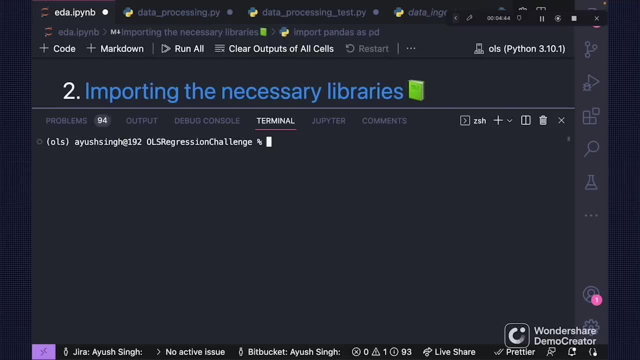 over there. please let me know. i'm just deactivating because sometimes you know conda, i have also a conda installed so i have to. um, it's my system thing which i have to deactivate. it doesn't really matter, it is a base thing. but i'll deactivate for a safer thing. but as of now, 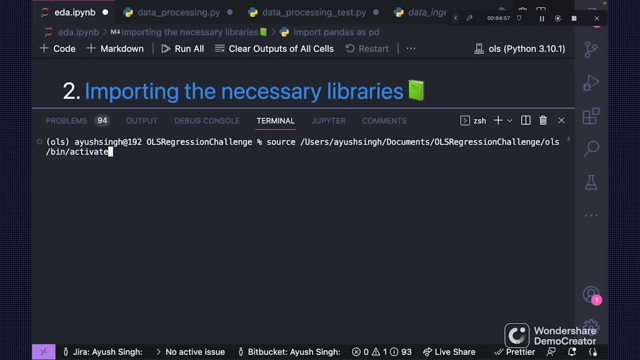 you just simply source, then you have uh which, which you have used source, and then you simply activate it. okay, and then you just simply activate it. and then you just simply activate it, okay, and then you also this uh base base also gets activated, but it will it mean it may not be shown, but but it is. 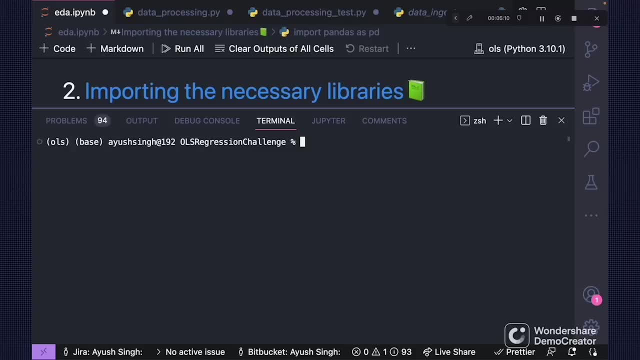 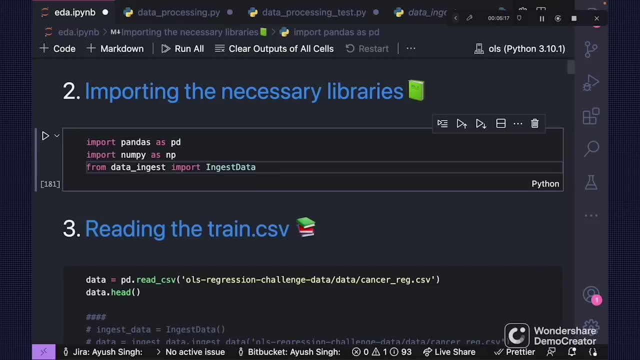 not going from here. it is my system things. i don't know what's what, what, what happens, but i think i need to uninstall this on now. but never mind on that. but uh, you can. you can first of all activate that environment whenever you enter. enter the project, first step, activate that environment. 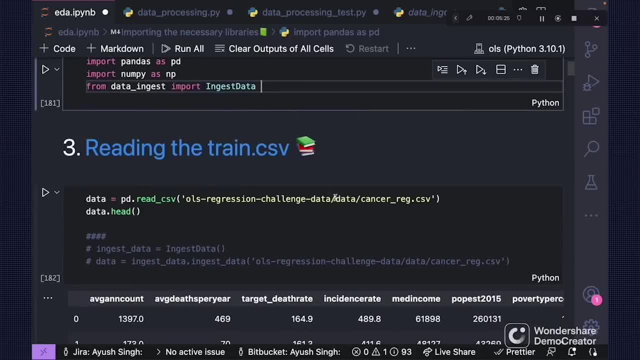 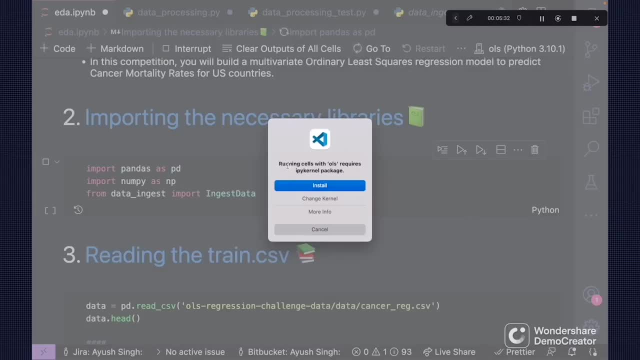 because that's what the project right. once you have activated the environment, now you should be able to run it. so let me run the first first cell. i usually use um vs code because it's much more so. it says that for vs code we are going to download, we have for for this particular. 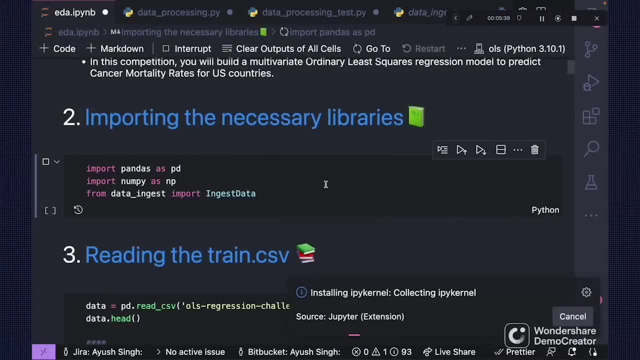 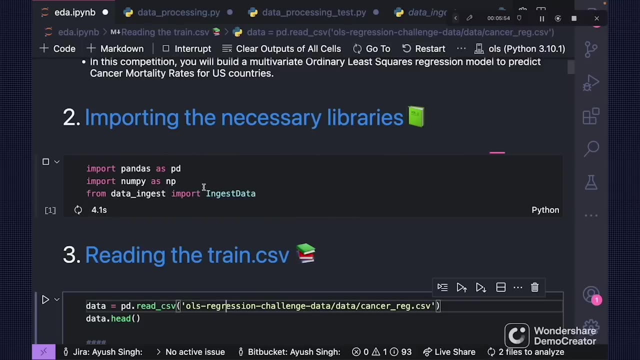 environment, we have to also download the ip i final ip kernel. however, however, if you're using vscode, you, you don't really need this. okay, you don't really need um to download every time, but i don't know. but yeah, for vscore we have to now. it runs now. it runs now. you see that it takes some. 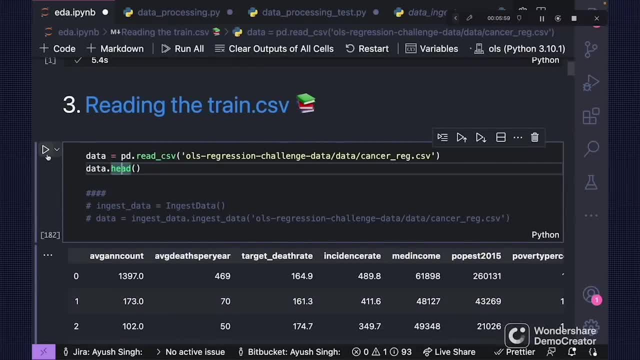 seconds to run it, and then we simply say, etcha, now, let's, let me import my data. so this is what your data looks like. this is what your data looks like. your data looks like you can use it. you can type uh and then say, okay, press the anytime button and then, uh, run this and it will access the data. how? 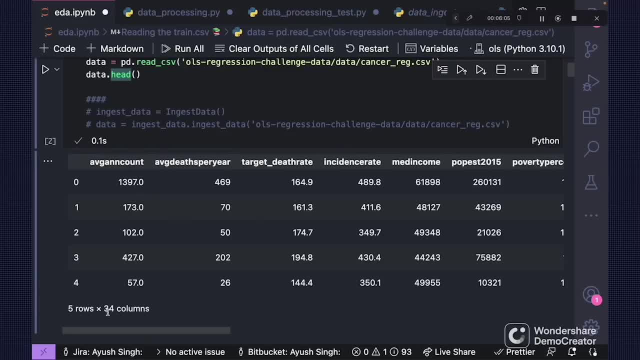 does it apply to it? so now that's how this is. your dailyあga symptoms looks like це там ép esse me to go Patram. your data looks like where you have the 34 columns and five rows where it where we are asking to show. 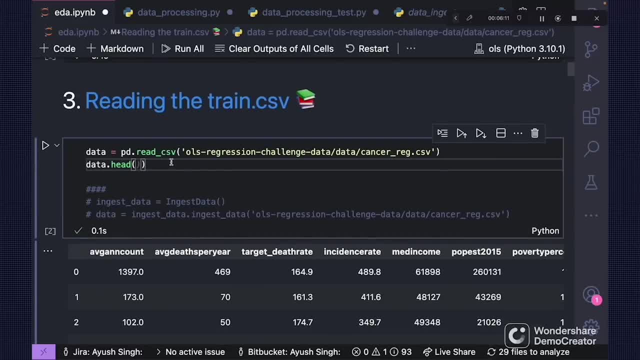 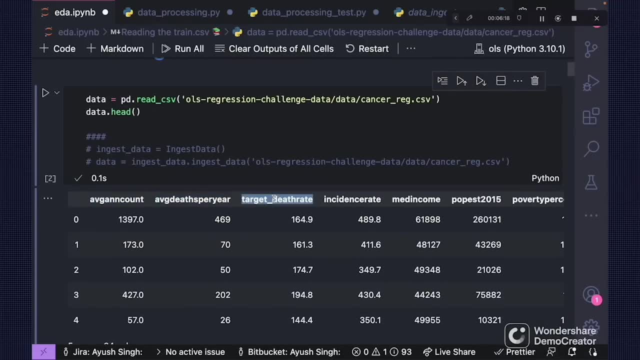 the five columns. you can also specify on it. so it's 10 or 5. it is just for the top five columns and over here and over here it says average in an account: average death per year. this is a target variable. the death rate in that particular span, incident rate, median income rate, power type study. 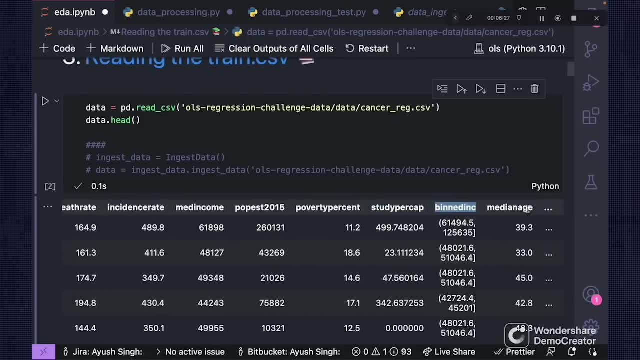 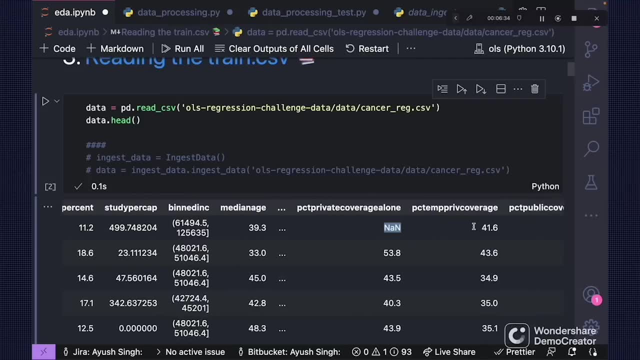 case study recap: bind dink, which is and media range. so you see that this is something unusual. you have to work on this, so i'll come back like something you have nan values, omg. you have missing values available. you have. you also have. you know um what you also have if you've explored the data. 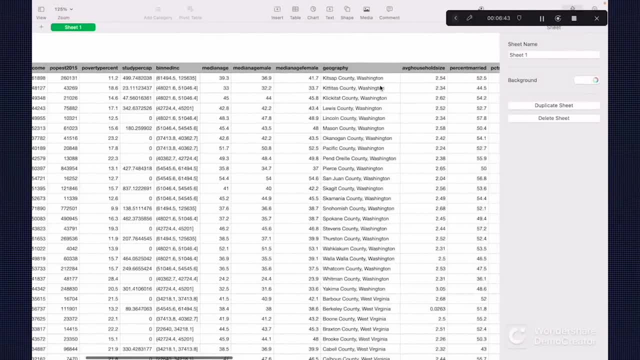 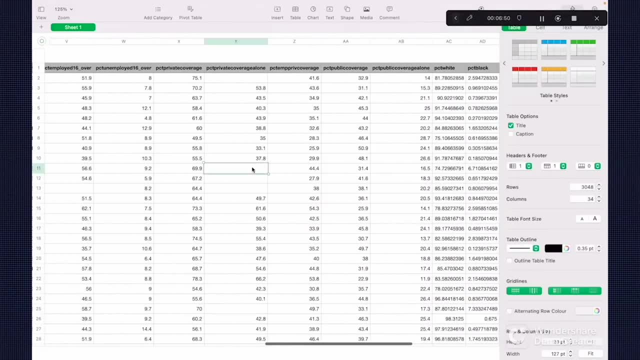 if you explore the data, you also have, you know over here, which is the english, which is the categorical values, which is this text value. so how are you going to deal with that right, missing values, categorical values in, in type of interval, in type of in interval, type of thing. how are we? 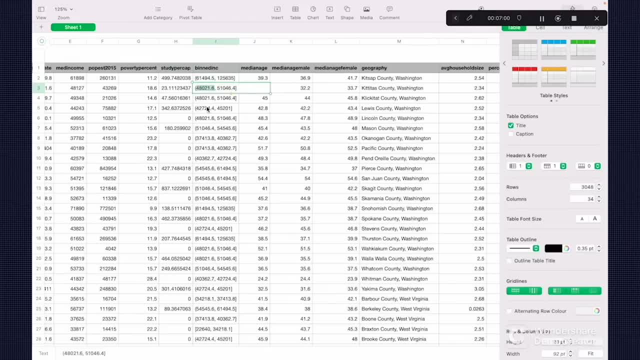 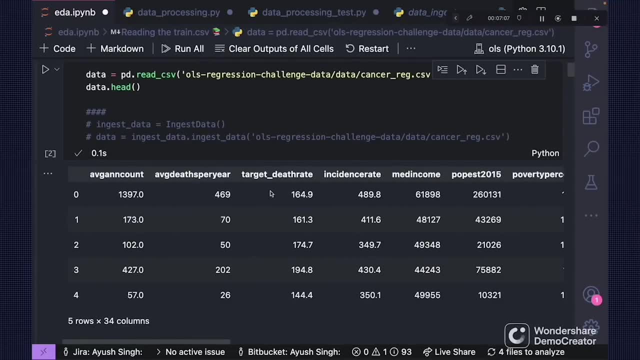 going to deal with this, because we cannot just read it to them, because model in make, because this, this acts as a string right now, so that model will not make sense. so there's a couple of things which you have to take care. missing values- right, the first is missing values. 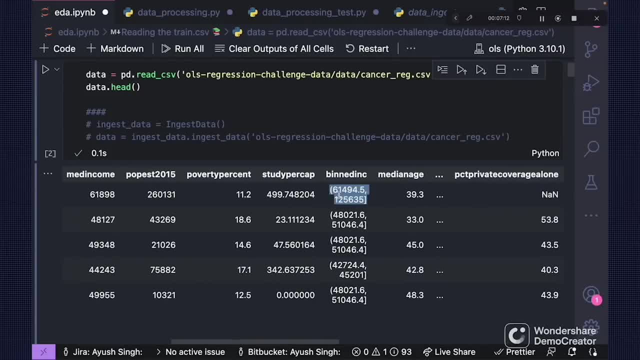 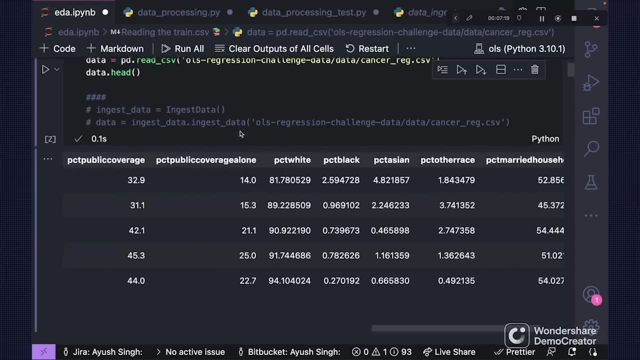 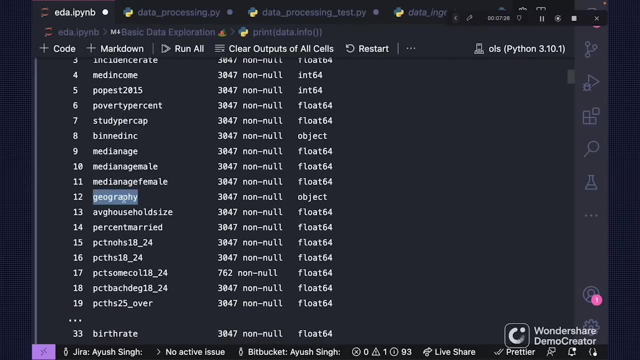 second is over here, which we see that this is something unusual. but there's something unusual where you have the lists in every column and then you have, you know, um, text category, text variable, okay, object variable. we can use simply datainfo to take out things out here, to take out geography. 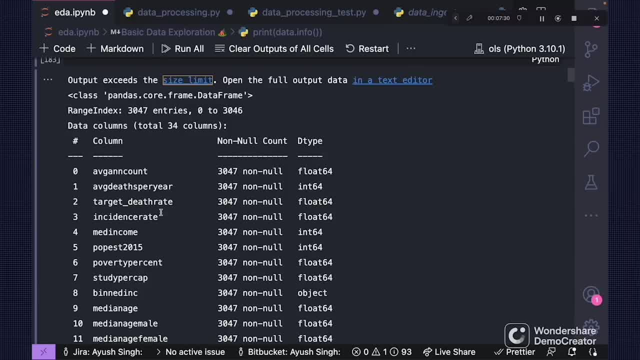 isn't a string. and then you have enough, all you can use simply datainfo to take out things out here, to take out geography isn't a string. and then you have enough, all all values of float target that is float, and then you can take out the null and then it gives you. 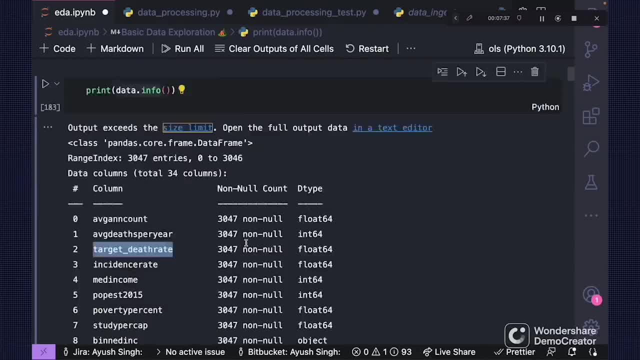 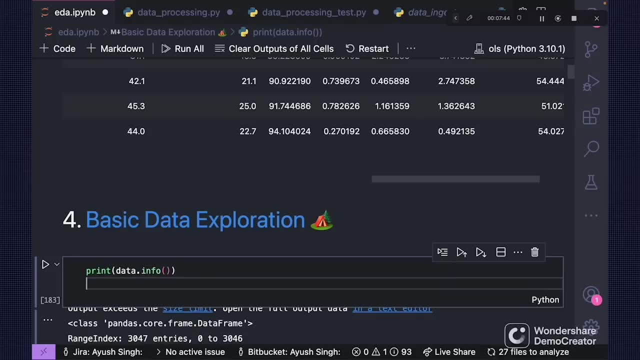 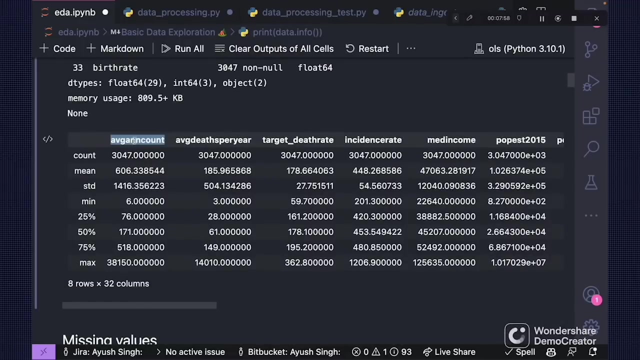 good information. so now let's take out. so now, once we are done with exploration, you can also take out describe. you can also write describe. so um, data, dot, describe, and then over here when you do the describe, then what it does for every column. it describes some of the useful statistical analysis. for average a and n there are three zero four, seven. 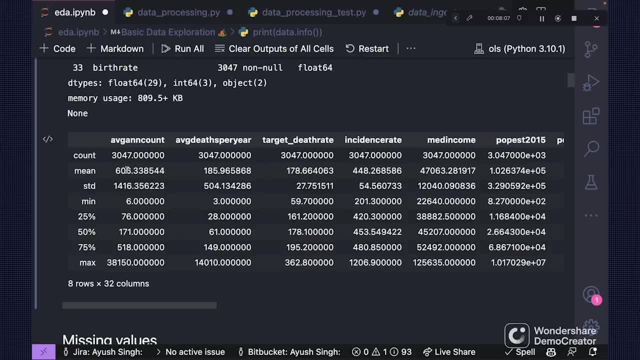 count with the number of values in that particular column. what is the mean? mean is 606. a standard deviation, 14 and 16 minimum value in that column six, twenty five percent of the values, which is seventy six, where we see that there is this twenty five percent of the percent of the value which is 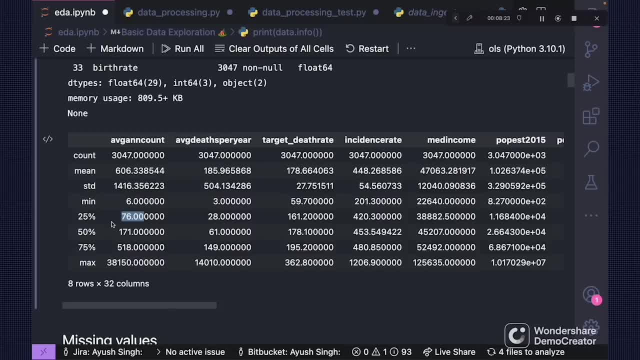 smaller than seventy. six fifty percent of value which is smaller than one to one, seven, so 171, and seventy five percent of the and less, less, twenty and more than and so and twenty five percent of values which are greater than 518, or we can say twenty seventy five percent of values which is 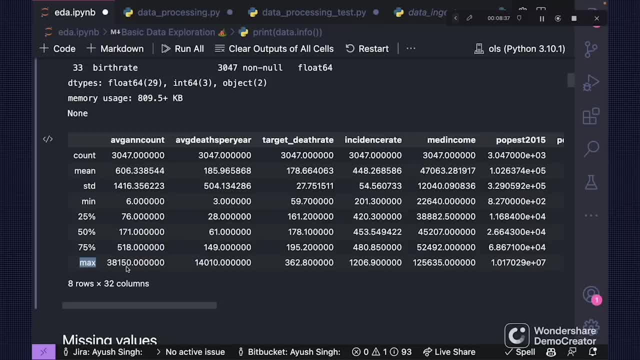 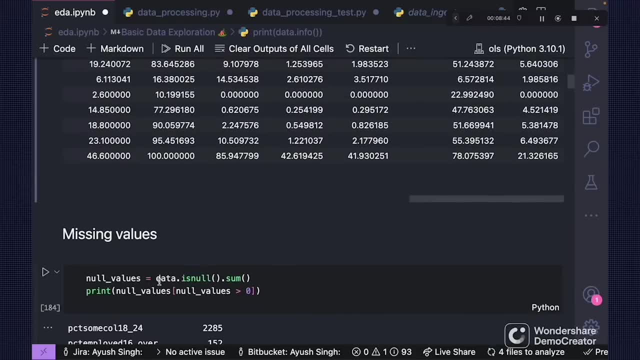 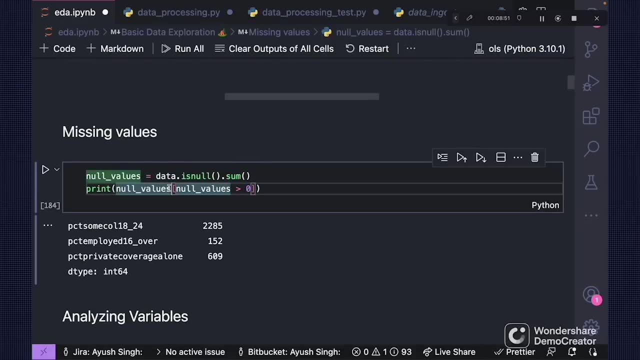 lesser than 518, all right, and maximum value in that column is 385150. so you have now, for every column list listed out here and then now. now, once we have the basic things, now what we do, we simply go ahead and simply take out some of the ask, because we have noted on three, three things. 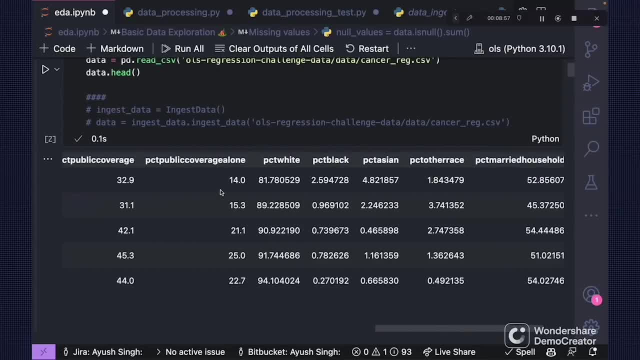 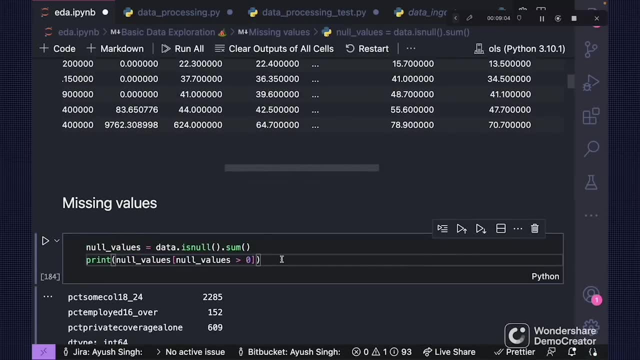 that bin, uh, that bin wallah thing, and then you have nan values, right, and the category. so let's take out, let's take a look what number of meaning missing values which we have in which which columns. so if we run this, if we run this, we say that null values, we, we put the null values. 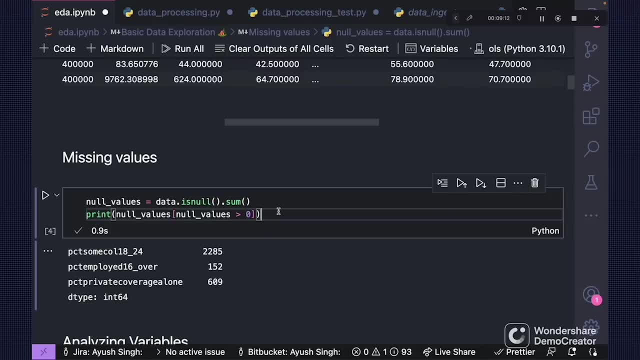 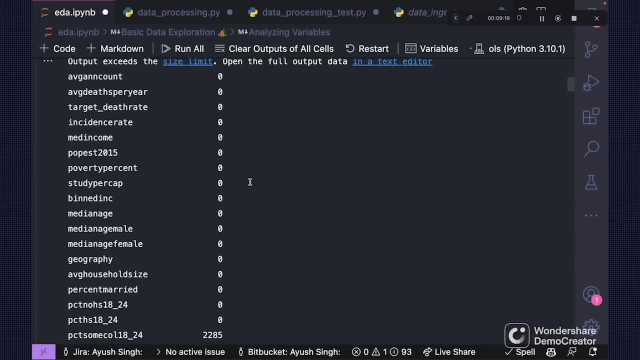 and we say data, that is null dot sum. so what this is gives um, uh, this gives um. you know when, when we print out normal values, this should give you know this- every column with the number of null values present out. there, with the number of present one out. there are only three columns. 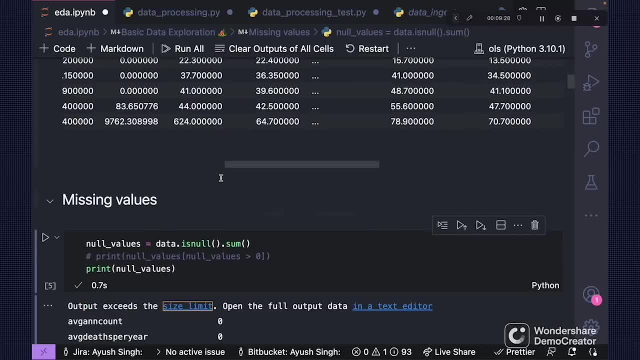 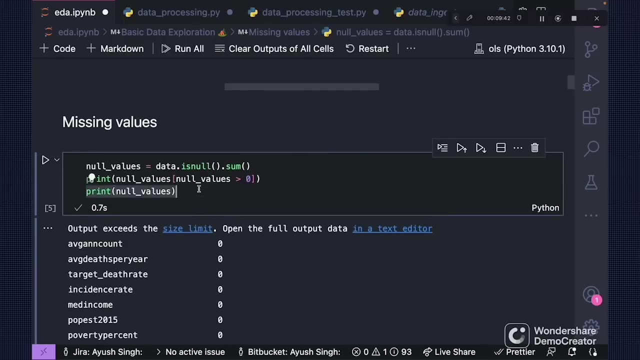 where your null values are present. there are only three columns which are where your um null values are present. so we say that you print the null value, print the null from from, from the null values from that series, take the null values, take the null values whose global value greater than zero, right, so we simply print that. and then we say there are three columns. 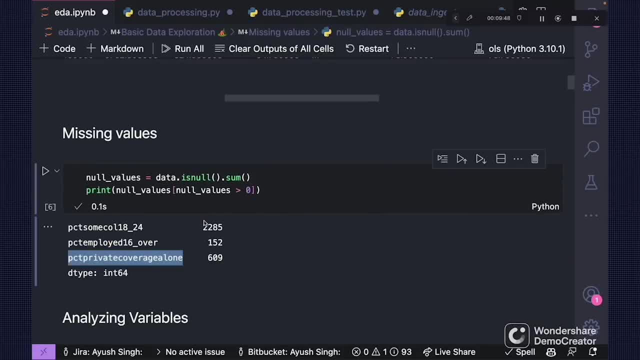 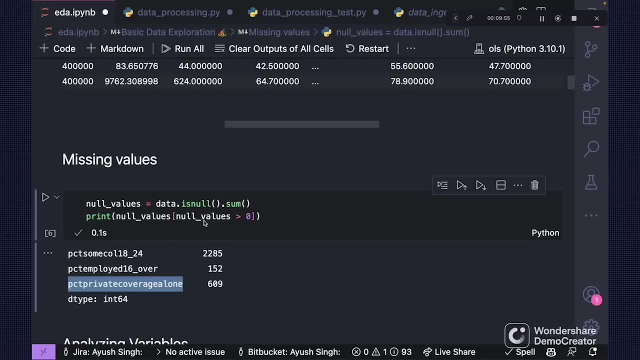 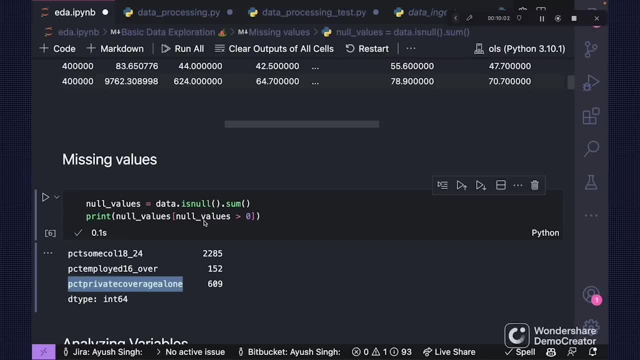 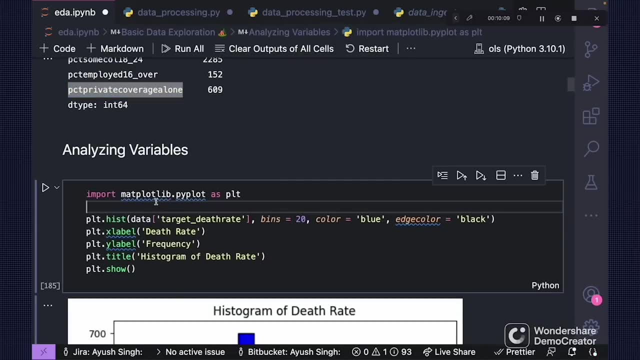 blah. so there are several techniques for dealing with missing values, with their pros and cons, which we'll deal with in very detail. then we have now once: once we have this, let's worry about other things, let's let's start exploring each and every variables. so once you have the basic, you know. 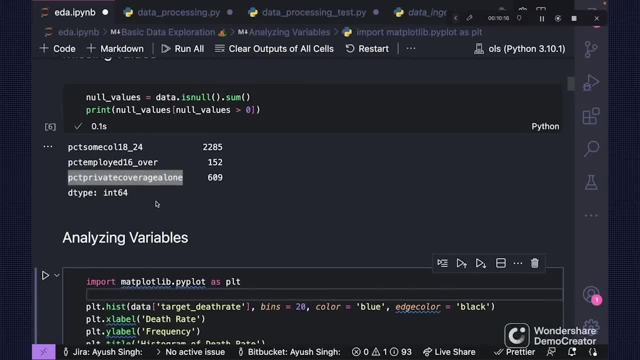 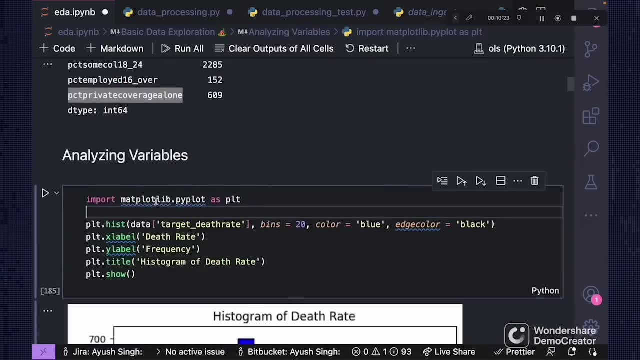 missing values, exploration of the data. now let's go ahead and talk about how we can. um, now you have to analyze h and l variables in your data, to further analyze your data. so now you may be thinking, hey, ayush, how are you coming up with these, these things? 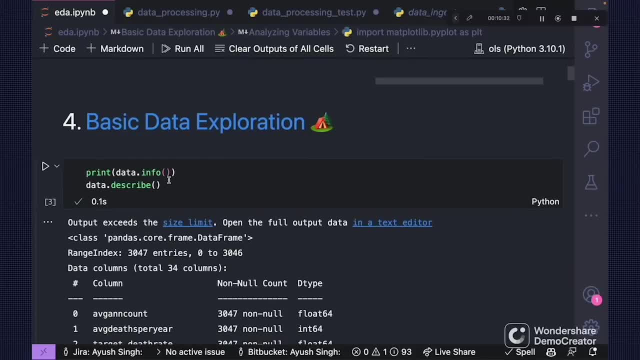 the first step is in anything is to do a basic exploration. okay, have a template basic exploration where you talk about: what are the number of there? is there any missing values? is there? what is the data types available for every column? what is the maximum minimum values? what? what values are greater than this? what value is smaller? this more than? and the next step should: 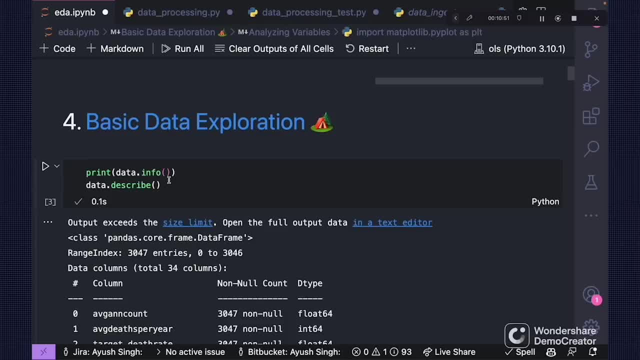 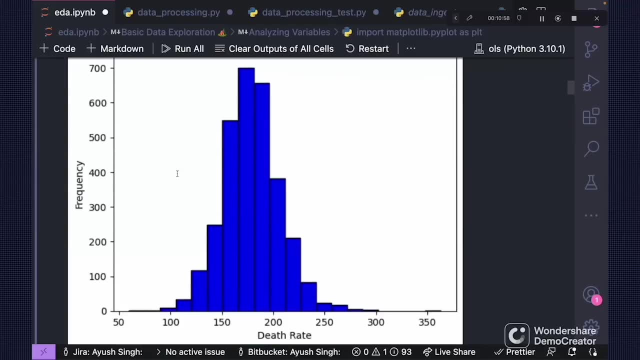 be to analyze each and every variable. okay, each and every variable out here. that will give you a very good set of thing. first is we are going to analyze our target death rate. we're going to analyze our target variable- right target variable- in which we say that plothistogram, you're plotting. 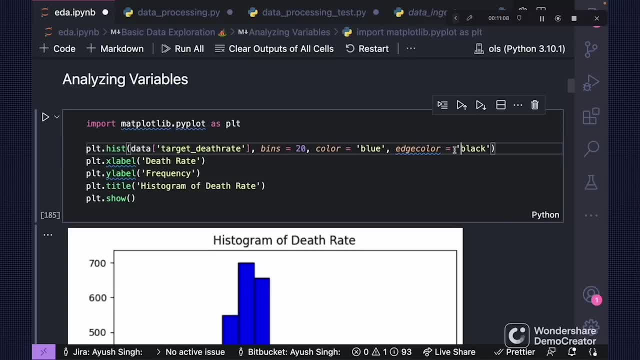 the histogram then should be 20, color should be blue and it should each of the histogram should be black and then we say: on x-axis label that as a death rate, on y-axis label that frequency, and then title should be histogram of the day three. and then we show that plot, show me the. 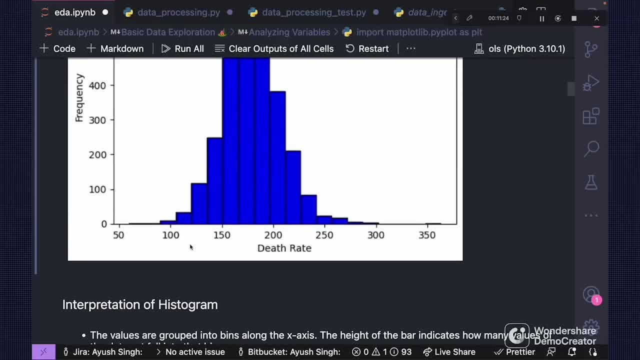 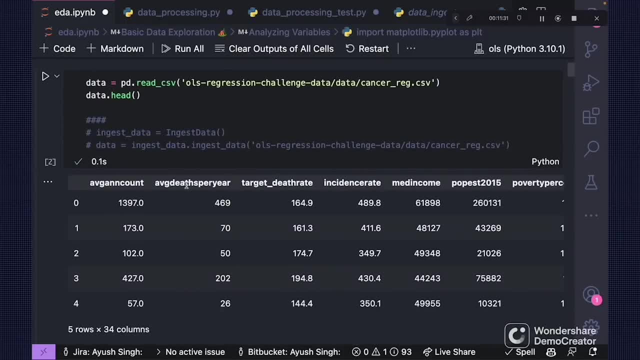 plot right now. that's what it is saying and i'll talk about what is the interpretation of this. so when you, when you actually take out the histogram of this target death rate, of the histogram of this particular column, of this particular column, this will result in this: 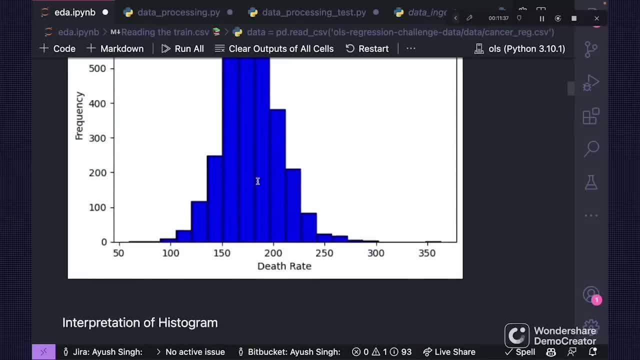 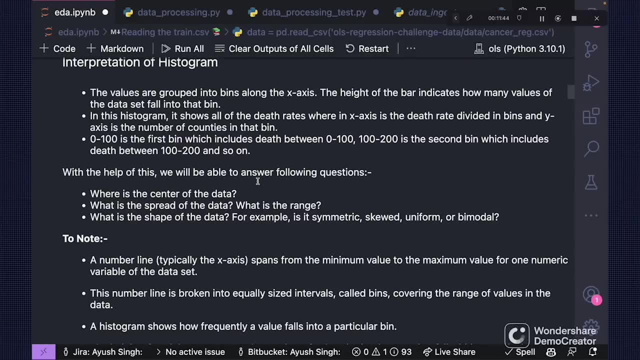 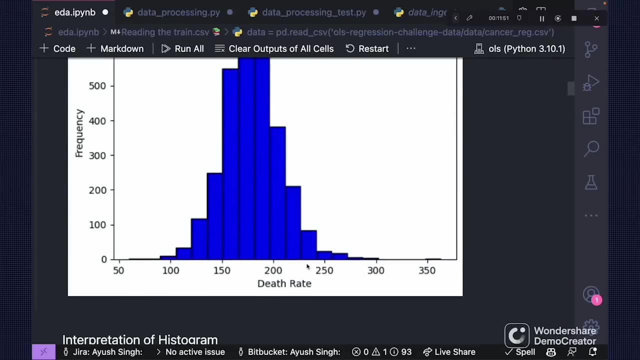 particular histogram so you may have high time in uh interpretation of it. so let's talk about interpretation of your histograms: the values, which are grouped into bins along the x-axis. so the values, the values are grouped along with bins. so you see over here, you see over here on the. 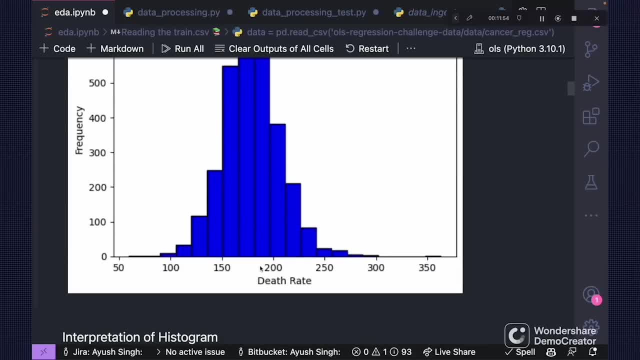 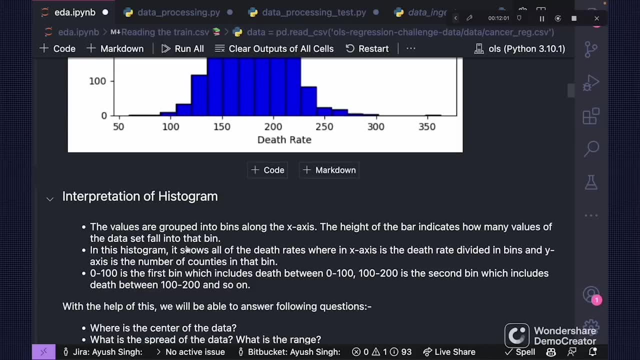 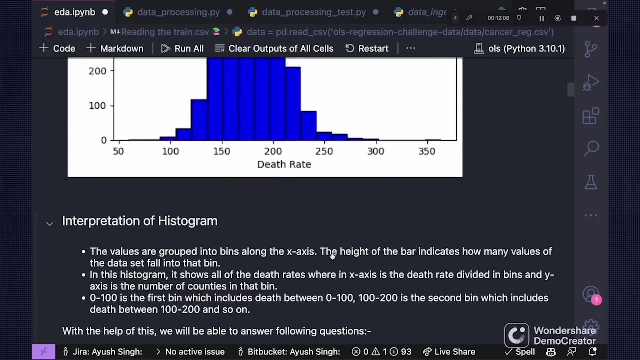 values on x-axis. they're grouped in bins, they're grouped in bin. so uh, we'll talk. we'll talk about uh as of now, which you see over here in this histogram. it shows all the traits which are data divided in the bins, and y-axis on the in the counties. you know the frequencies in that bin, okay. 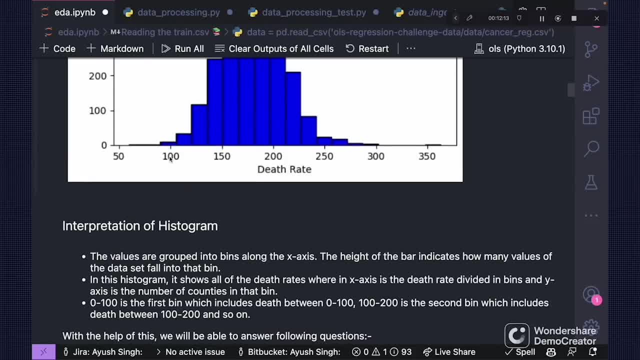 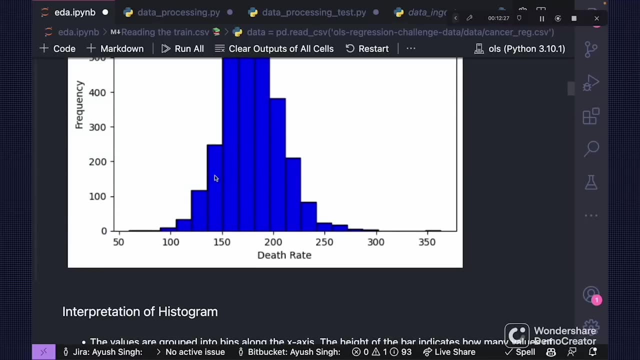 so we say that zero two hundred, zero two hundred is the. i think uh, fifty two hundred, not zero two hundred. uh, zero two hundred is the sorry. fifty two hundred is one bin, 100 to 150 is another. but over here you might have noticed that we have 20 bits as of now. but if you notice it very nicely that 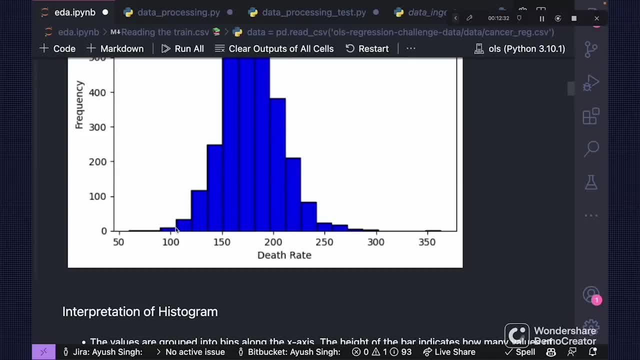 this, the, the, the range of this, the, the. you see, you see the mouse right now. you see the mouse there where i'm indicating. so this is 20, you know 20 bits. so we say that, that, that in this particular bin, what are the number of frequencies, what are the in this part, for this particular bin, what is. 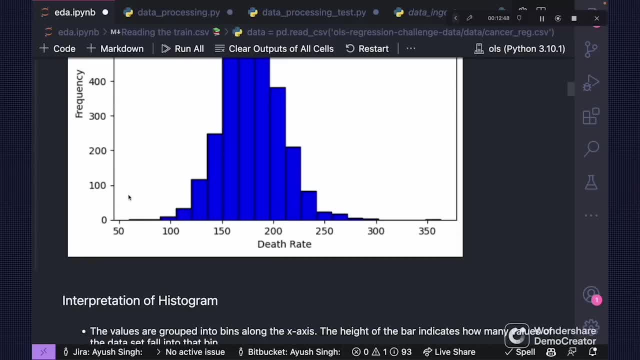 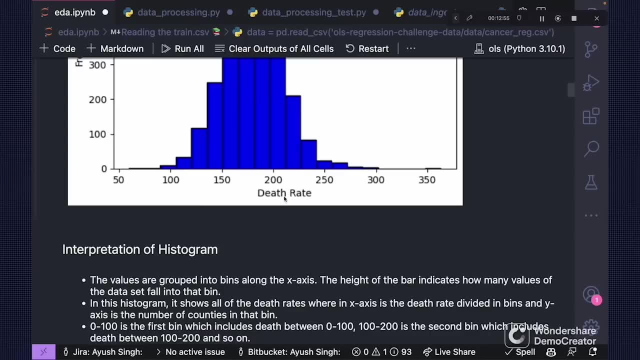 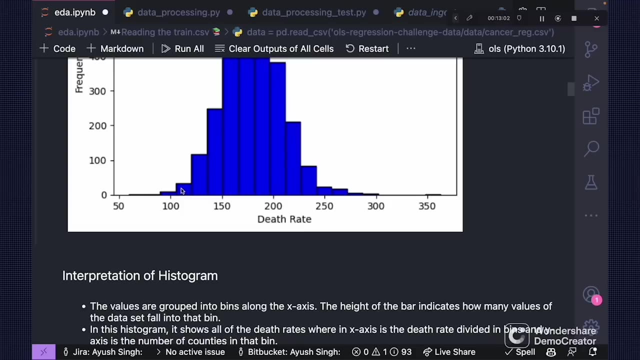 the frequency right for this particular bin. what is the frequency? so that's what it is telling, that it shows all the traits in x-axis with the bins over here we have 20 between 20, 20 and bins. uh, 20, 20 right, and y-axis is the counties in that bin. so for, for this particular bin, this will be the. 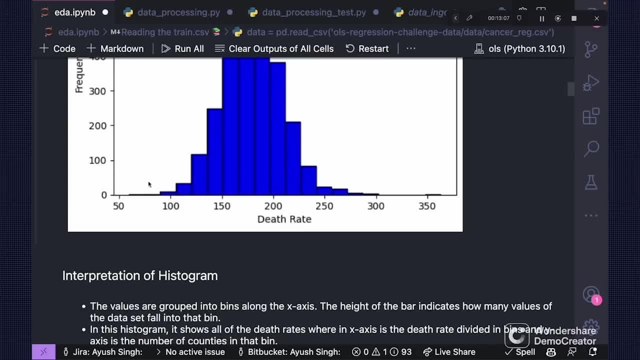 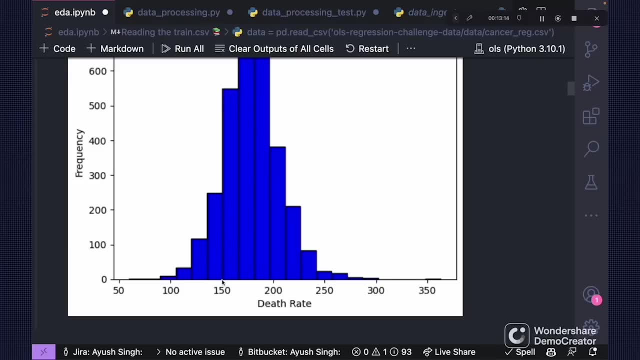 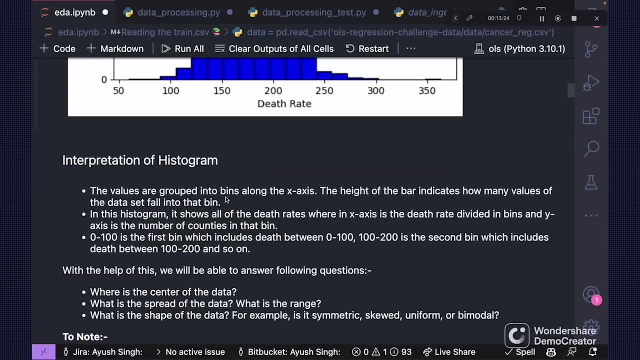 counties on. we simply have this 100, we have this, this bounties for this, we have this much. this is 550 around for this particular, so for for 150 to maybe let's take an example of this particular bin. so we have this, uh, five type of thing. so now, this is the simple interpretation of histogram. 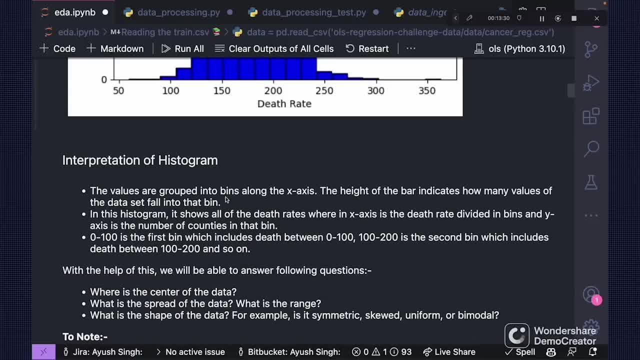 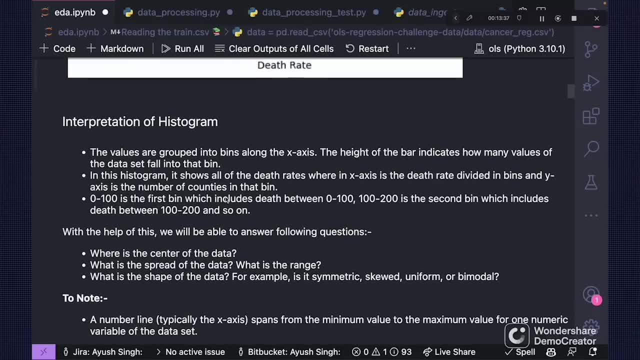 which you've already seen, but, but it has. but now, once we have the basic understanding of histogram, what will how? this will help us right. first, it helps us to identify our how. how does help us to understand a particular variable in terms of statistical format. first, it will help us to. 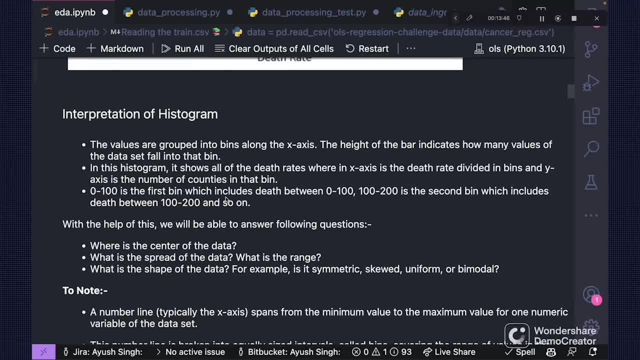 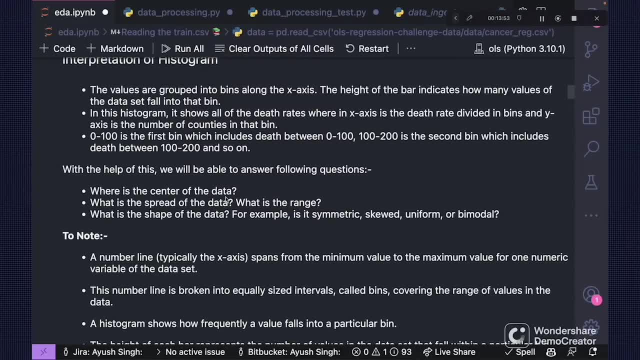 identify. what is the center of the data, what is the spread of the data and what is the what is? eventually, what is the range and what is the shape of the data? right, so let's talk, let's answer these three questions: what is the center of the data? but but before that let's to note something. number 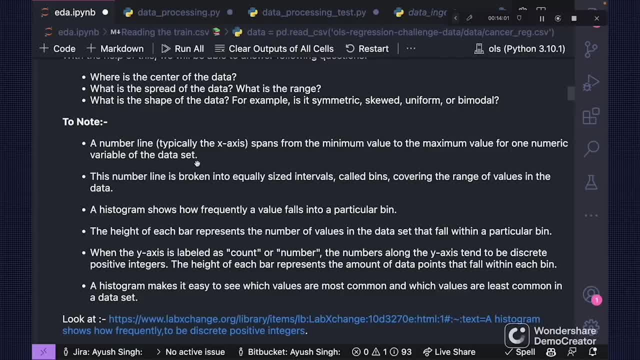 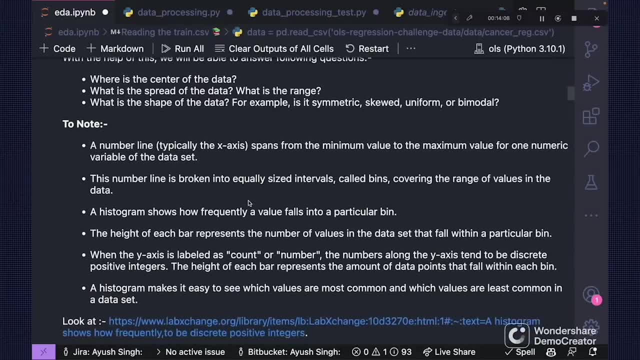 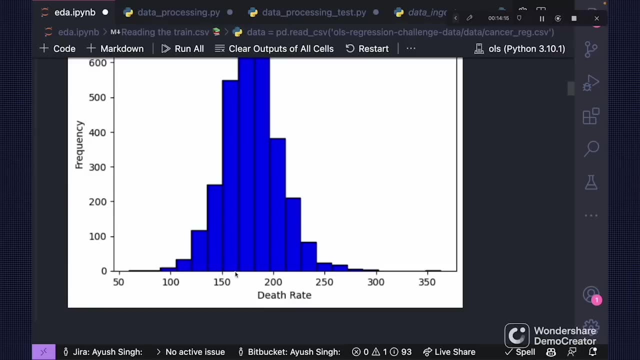 line is spams. from the minimum value to maximum value. the number line is the number of the data is broken into equally sized intervals. you see that all are equally sized. these are nothing but called bins covering the range of values. over here it is 150, 150 to this will be: uh, maybe we have 20. 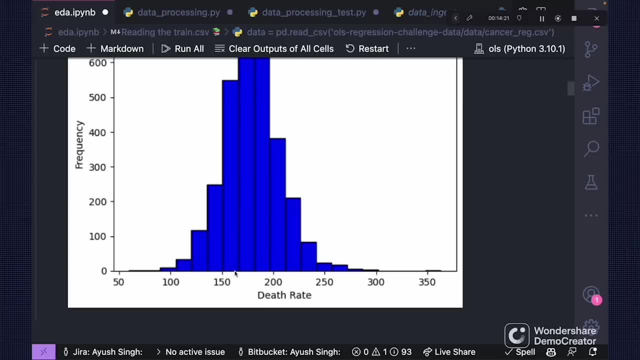 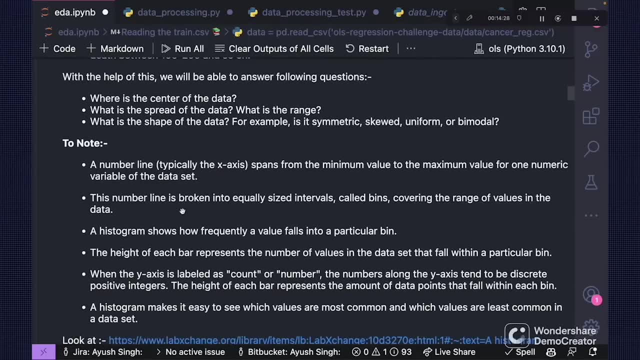 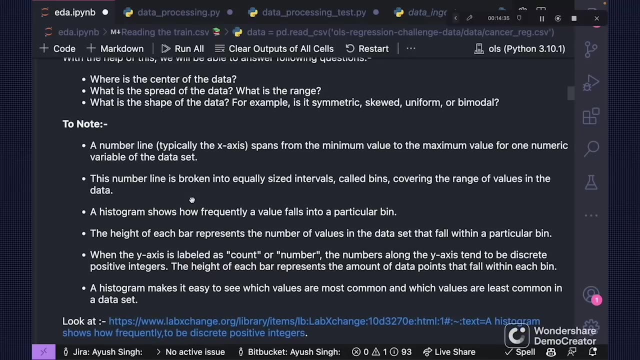 bins. so then, this particular, we have all the values, all the values which lie in this range, right, which lies in this range, okay, um, where we said number line is broken, equal called bins, and it have the every bin has the range of values in there, that a histogram shows how frequent the values occur in that particular bin. so his histogram. 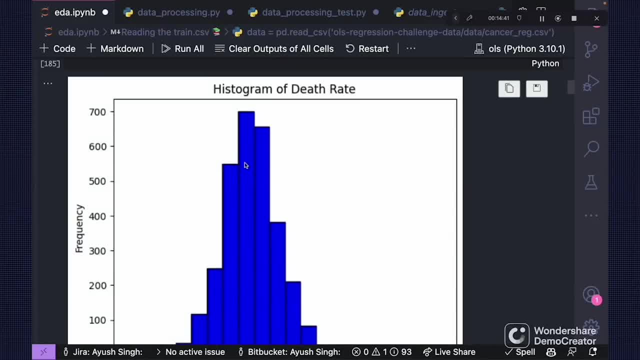 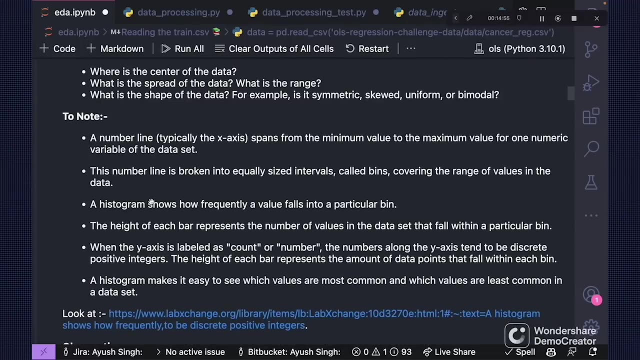 it shows how. what is the? how frequent the, the range of values occurs in that particular, how frequent on bikes is is for this particular bin, there is 680. that is the frequency right. so that is the frequency. the height of each bar represents the number of values in the data set that fall. 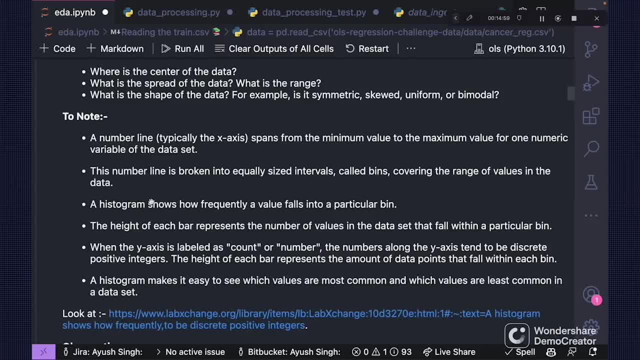 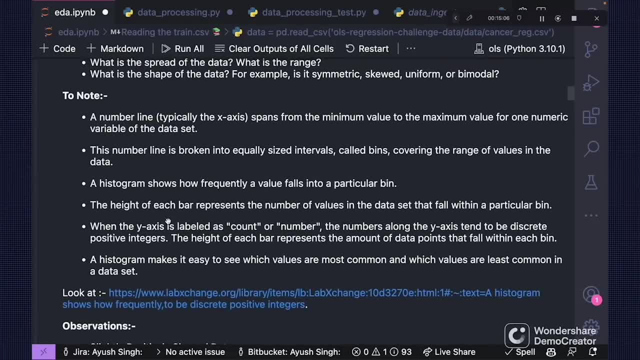 within a particular bin and when the the higher you know, the higher number of you know thing is. and then you have y axis, which is the counter number, the, which is to be discrete, which which represents the amount of data falls in that frequency, of course, and the histogram. 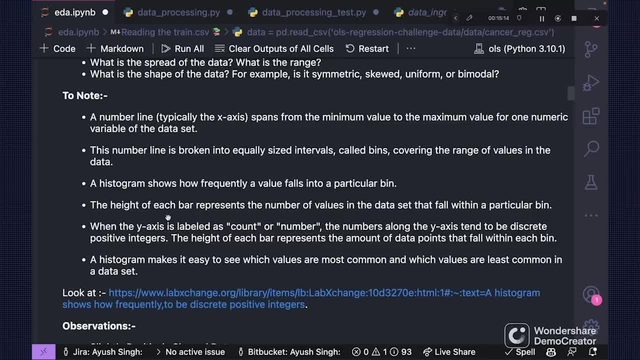 make it easy to see which values are common and which values are less common, or which range of values are less common in your data set. okay, yes, now, now, once. now, once we have that, let's go to some of the observations. so i've linked the resource, which is good for you. 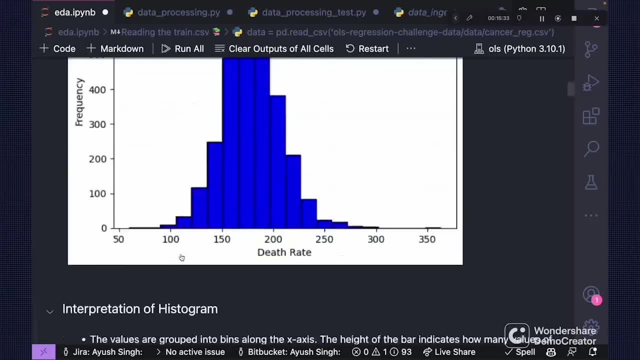 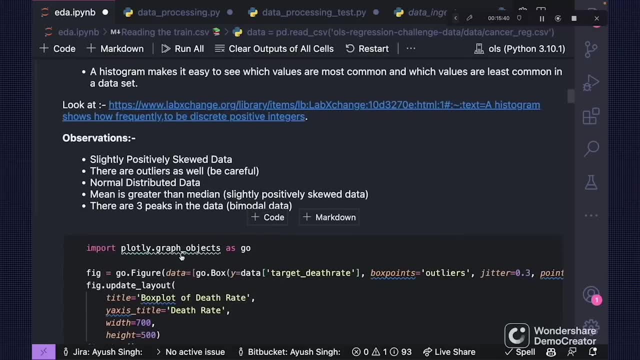 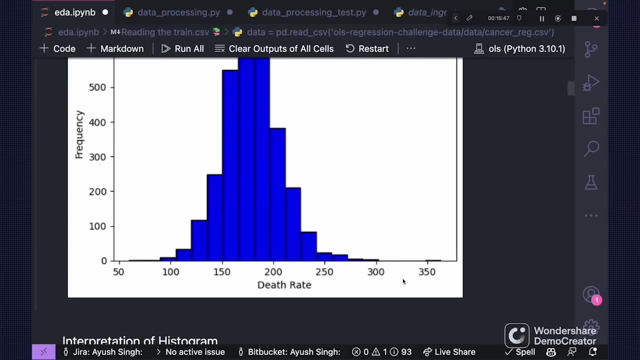 uh, first observation is: it is slightly positively skewed data set. so if it is not completely normal, it is very slightly positively skewed data set, right? and then there are outliers as well. yeah, so you see that over here, you see over here, you see over here, you see over here say this: these 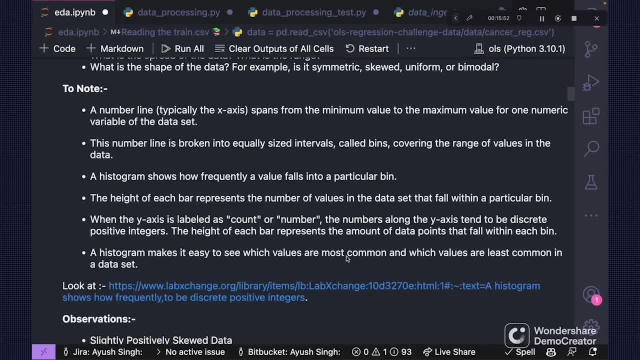 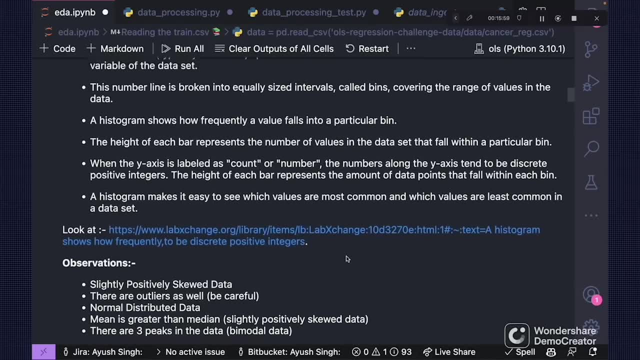 are out of distributions and these outliers, nice. so we got an idea. this is an skewed data set or slightly, and you have the outliers and this is also not. this is not a completely normal distributed. this is it is not completely normally distributed and this mean is going. 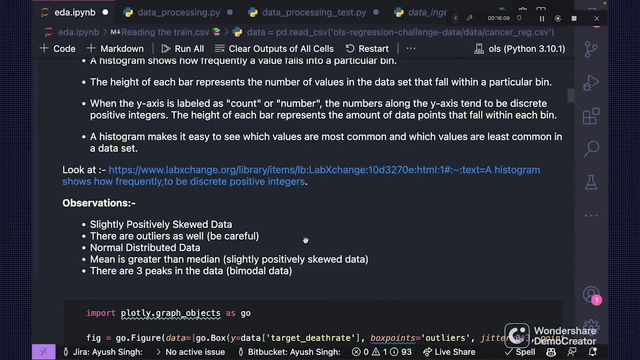 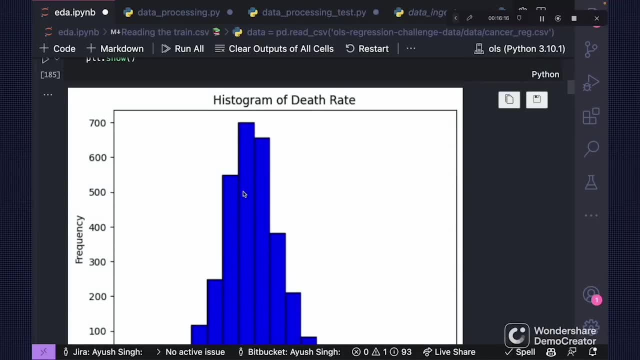 to be skewed data set. okay, so if you have a data set which is slightly skewed, data set which is greater than median and slightly positively skewed data set, your mean is greater than median and you have three peaks in the data set. so you have by model data where you have three. 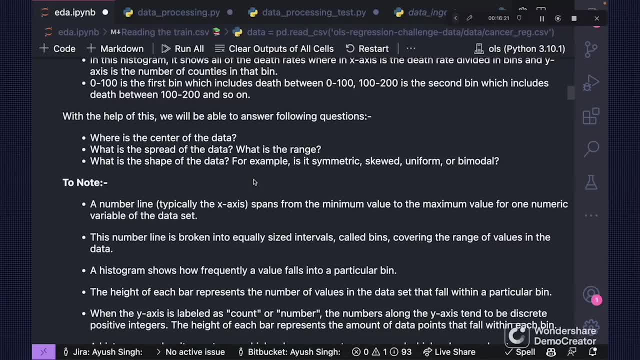 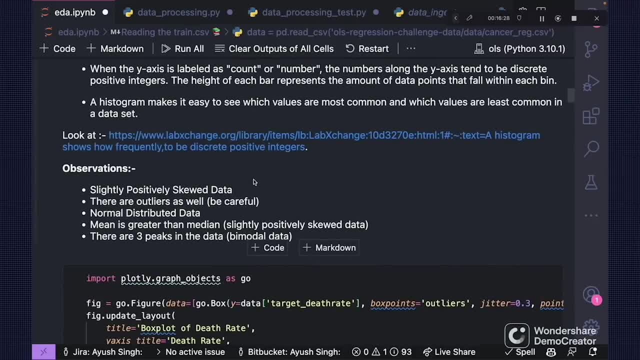 peaks in your data set right for that particular range. this is the high. this is one. two, three, these, these are three picks. that's why we say: by model data. but the most important key takeaway, which which i'm going to take from here, which i'm going to trans translate, is the is we have this, the? 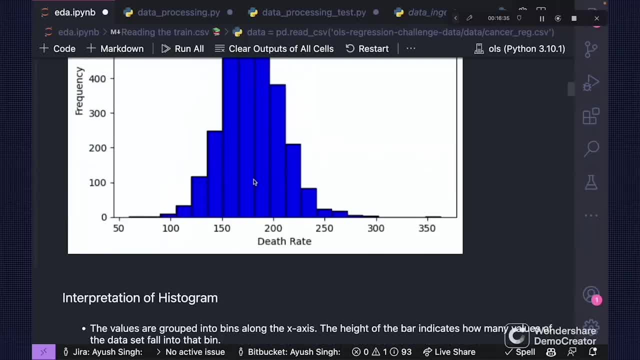 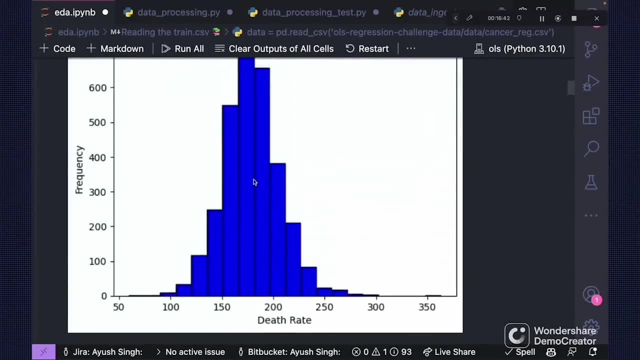 columns, which is slightly secured. we have the column which is normally distributed, we have the, however, um, we are not going to. uh, we have, we will just take care later on about the outliers, but that that is for this particular variable. so we do this for every variables, but that, for example, 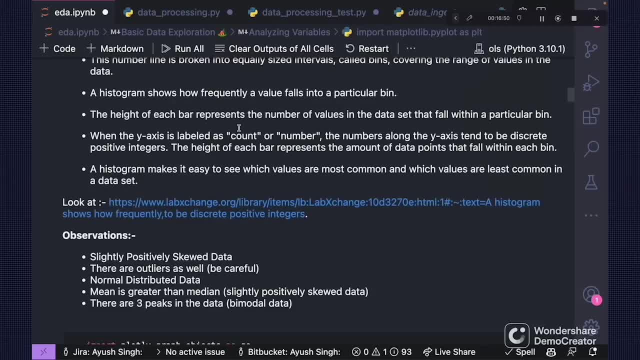 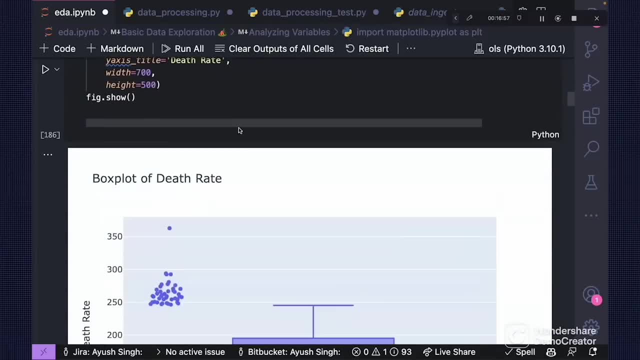 if a thousand variables, how are you, how you're going to do it? that something is a uh talk to talk on specifically, but i hope that this histogram gives you a nice sense about what exactly we're going to deal with the next. so next, what you're going to do. as you've identified, we have outliers. 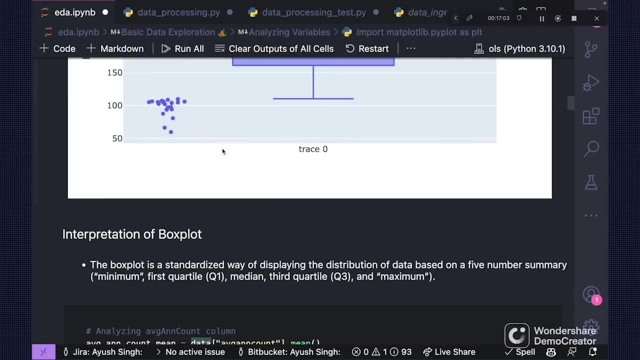 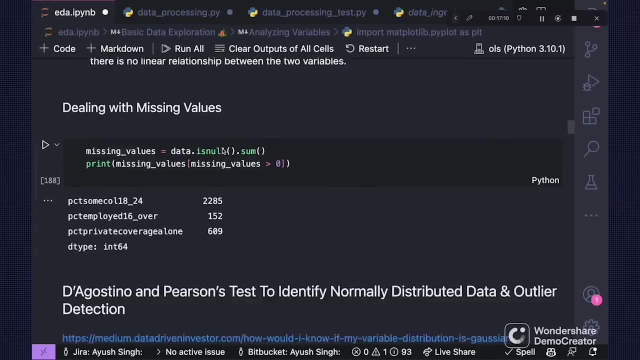 we're going to use box plot to see whether we really have outliers in a great sense, right? so we're going to do that and then have a have a very nice understanding of that and for every variable we'll do the nice exploration and then we'll learn about outlier detection, removing a lot. 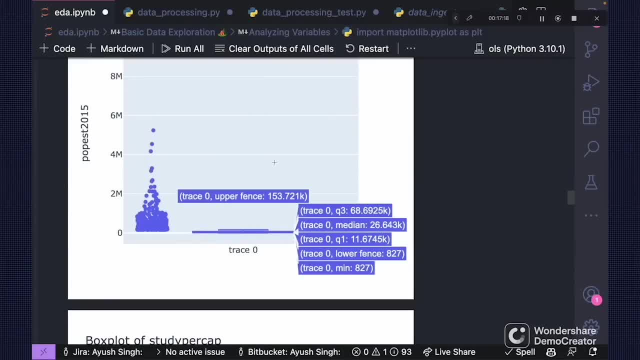 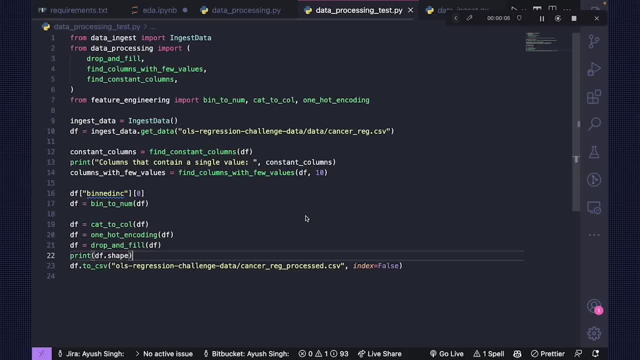 of things to talk on. you know there's a very lot of things to talk about, so let's go and go to the next lecture and talk about that. so, everyone, let's get started with our data processing techniques, which we wanted to. so you will find a file, uh, which is data processing test and data processing. 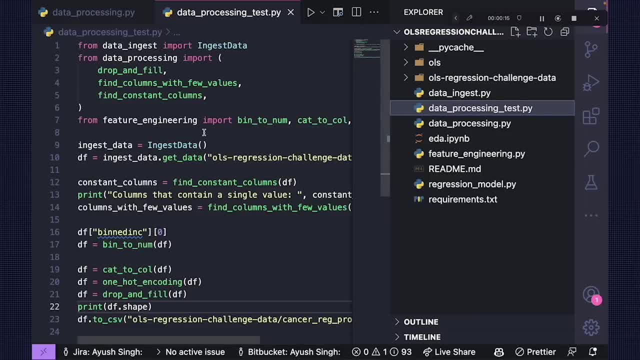 data processing. test is a really specific thing in data processing, so there are a lot of things to talk about and you can use them for your data processing, and then we'll go through a lot of different things. so we will try to uh go through step by step what exactly we are doing and why we are doing that. 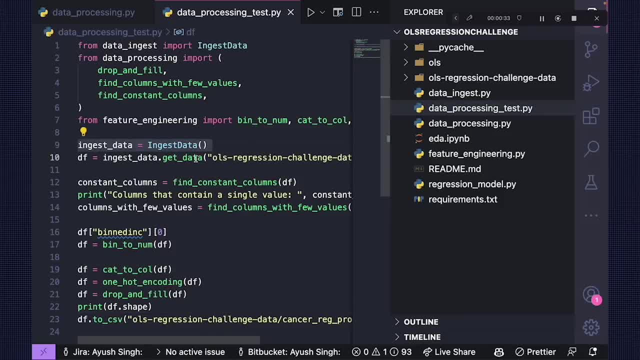 right. so first of all, let's get started with what exactly things which are going to use. first, we ingested the data, we get the data, we imported data using csv file, and then what you're doing? you're finding the constant columns. so this is not appropriate for every case. so basically this: 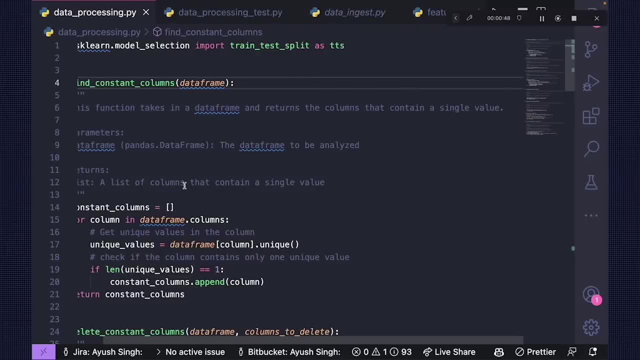 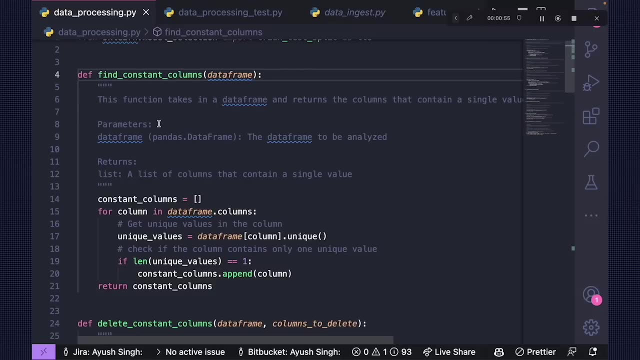 this function takes a data frame and it turns the columns that contains a single value. so if your data frame, if your column, has only one single value, that's the very, very bad thing which can happen, right, so it will remove, it will find the columns which is constant, right, which has a single. 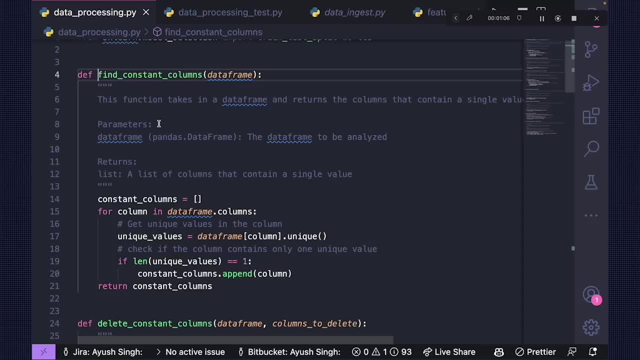 values which can indicate either of categorical variables or the variables, which does not provide any sort of values to your, to your data, right? so we find the constant values, constant which has that a column columns that contains only a single value, either a 1, 1, 1, either 2, 2, 2 or whatever. 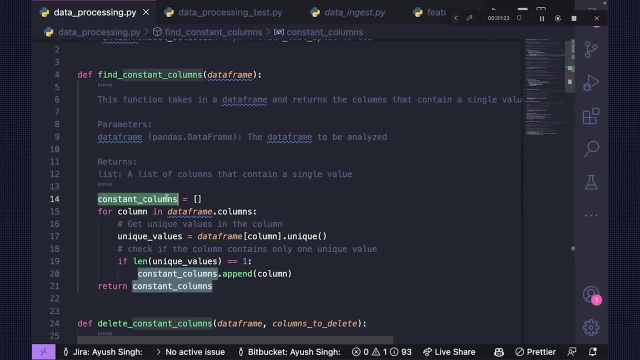 so constant columns, we make a v, we make a list, empty list, constant columns and we iterate through the the columns, data frame, data frame, dot column, where we ask for the data frame as an input to the function, and then we iterate through the columns and then we say that find the number of 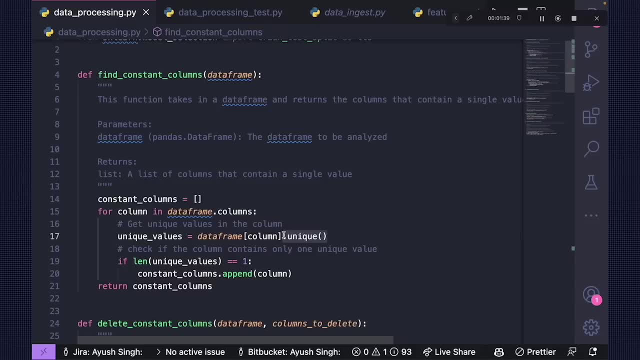 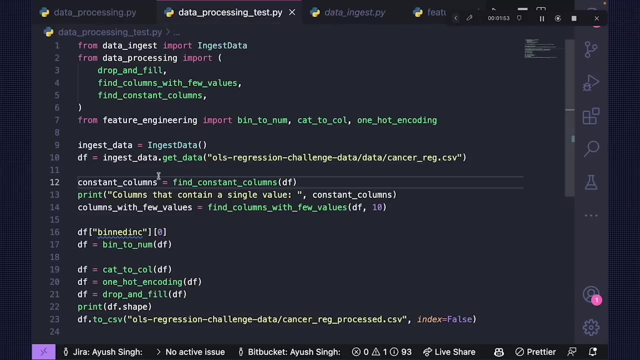 unique values in that column by using unique method, and then if that unique method is greater than one, then append that particular column in this constant columns, which are which which we are doing over here, and then we are returning at the end the the the constant columns, right? so that's the first step which which we are doing over here. so it says the columns that 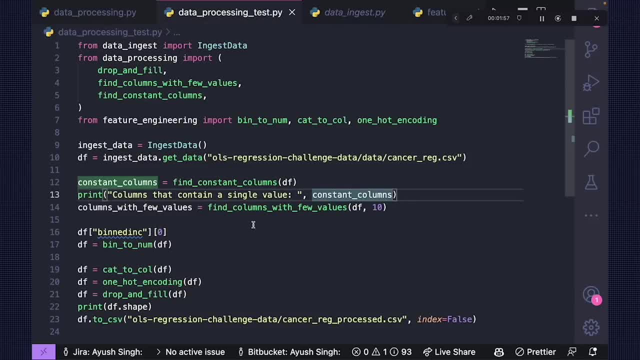 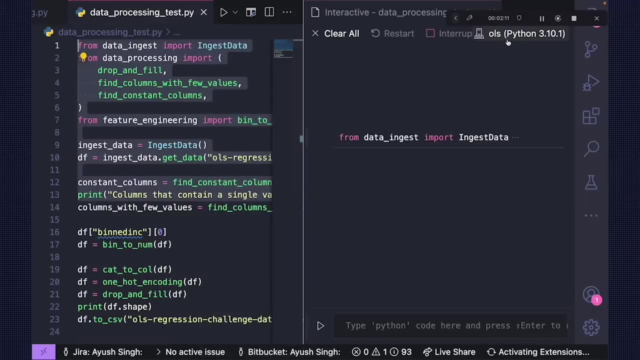 contains a single value, and then print out the constant columns and then let's try to run it. so, uh, what? what? exactly? what i'm going to do is maybe go to uh run my, you know, uh, it's interactive window, so i'll just run my interactive window. so we have ols activated in this as well. so you see, 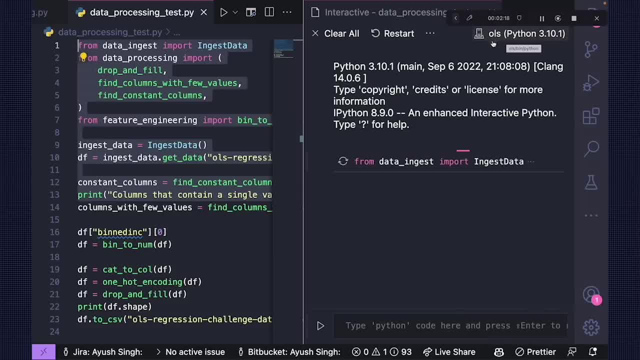 in virtual environment, which is ols, is activated in this now. so we have that. let's wait for a few seconds, then it should work really fine. so, over here, what you're seeing in front of me is it is running. uh, the two thirty lines of code which i've selected, you might use reapiter notebooks. 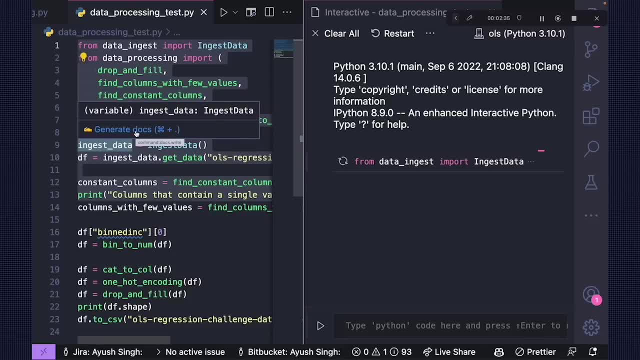 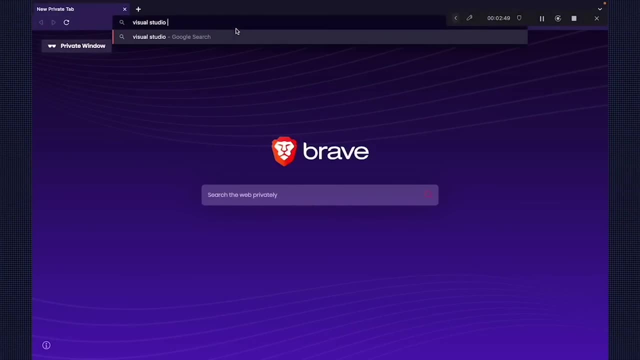 or you might run the whole notebook step by step. the the way i like is interactive. you can also go online and search about which visual studio code interactive notebook you will be able to find out. so if, if, if you go and then search out virtual- sorry, visual studio code interactive interactive notebook. 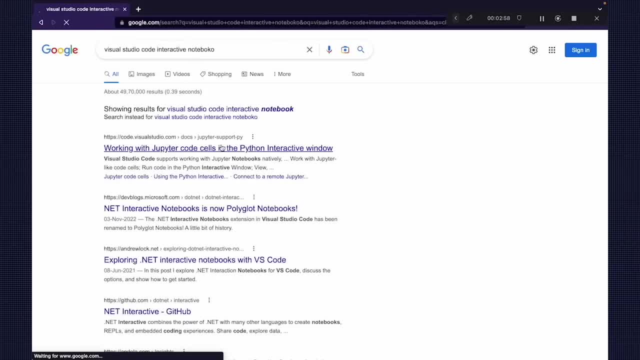 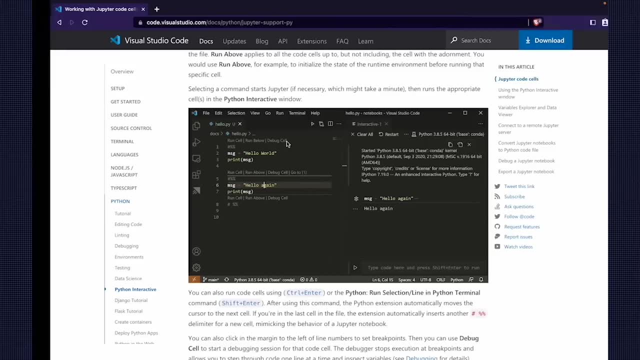 then if you go and see, then you'll be able to see that python interactive notebooks where you can actually download each and everything and then run the run that thing interactively by select, selecting the number of cells. so now it says the columns that contain the single value is nothing. 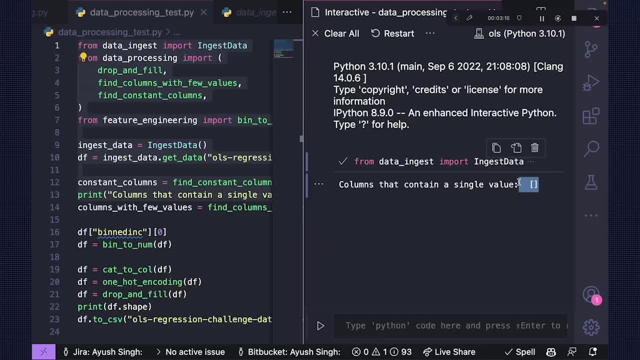 so you have a. so so you have a column which has at least more than one value, so at least it has a good spread. so that's, that's something which you don't have to worry about. sometimes it may happen that the columns contain a single value, and then you want to take a look if your data set is too. 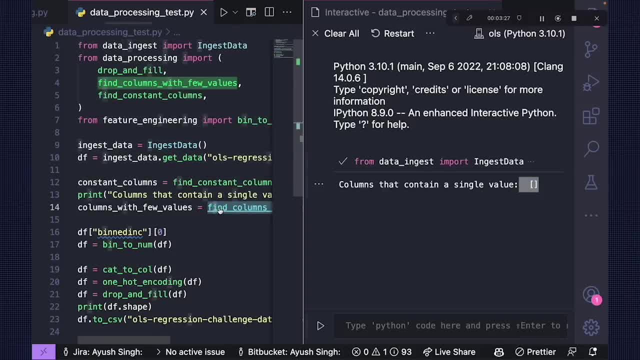 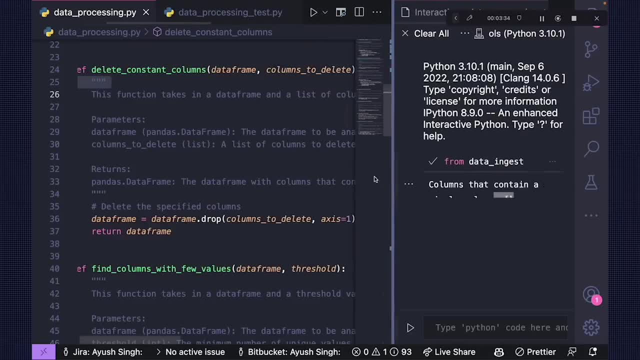 large enough. now you go to columns which contain the single, very few, few number of values. so i've also written: delete constant columns. so these, uh, this, what, what this particular method does? this drops the columns which are constant, but in this case we don't have any constant columns. 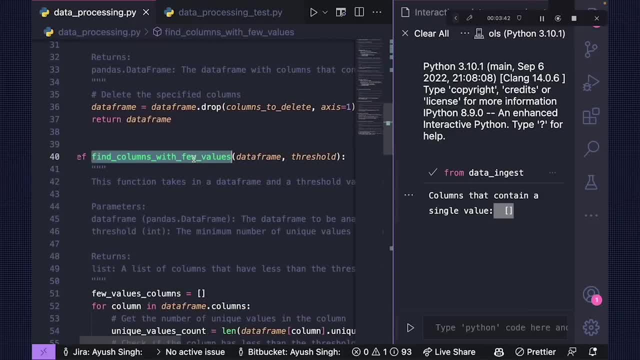 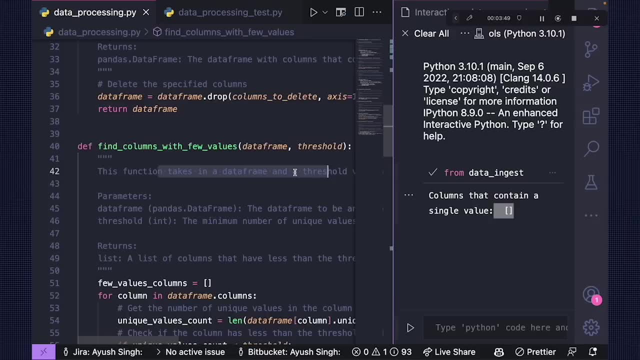 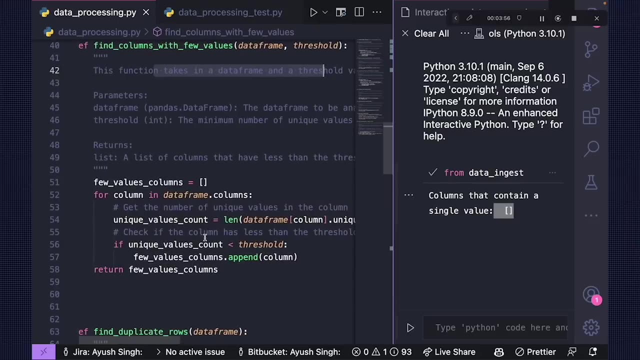 now we search for columns, which is with few unique values, where we say that function takes in a data frame and a threshold as an input, like what number of constant values, and then returns. so, for example, some columns may have fewer number of values in that column. so we say that we what we do, we simply say that we make an 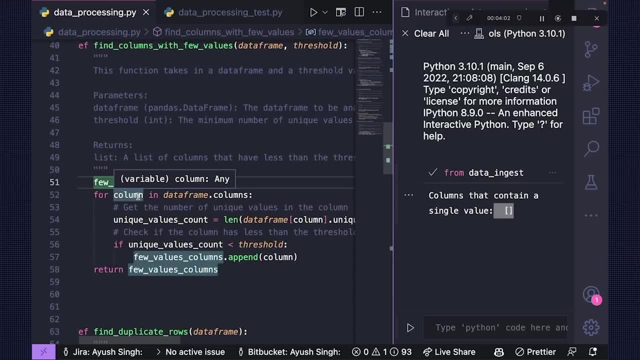 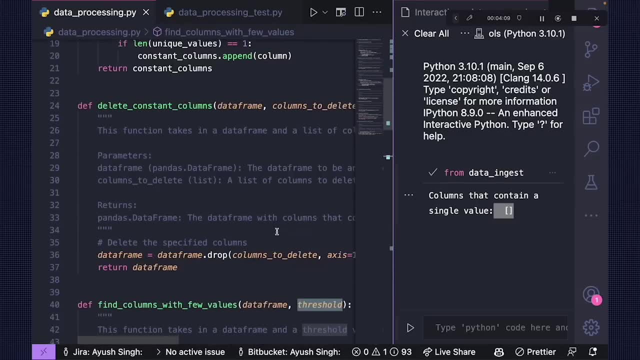 empty list and then we do. then we iterate through all the columns in your data set and then we find the unique values for every data frame and then we say if the unique value is smaller than threshold. so, for example, you say that you want to take a look at the column and then you say that you want to. 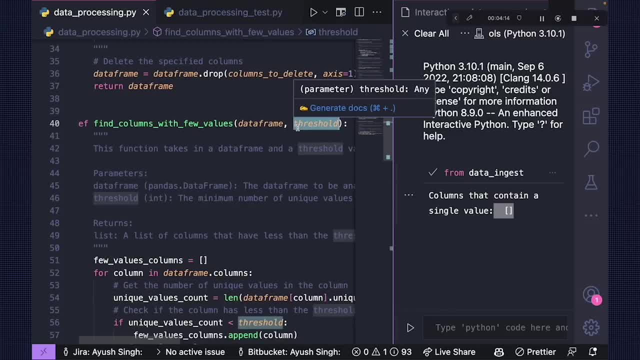 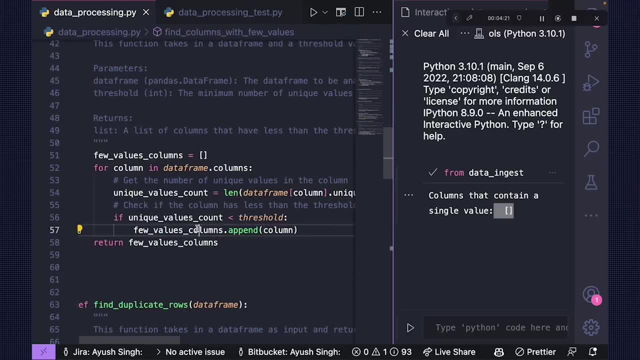 take a look at the column and then you say that you want to take a look at the column so you can see that it says that you want to have tree columns in that particular column which has, which has less than three, uh, less than three unique values in that particular column, right? so if, if that is, 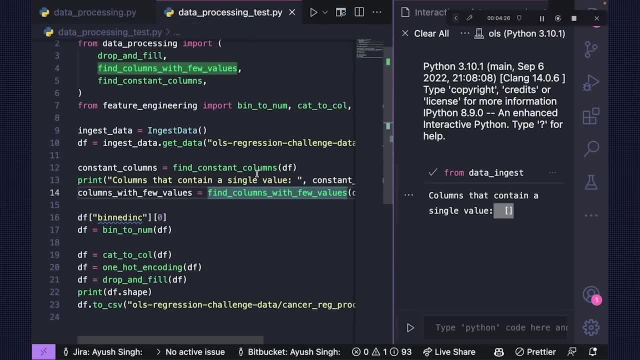 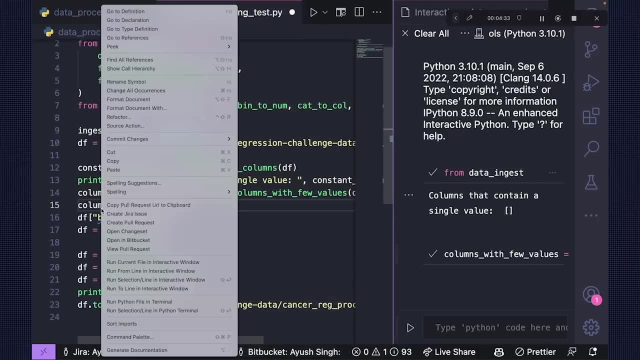 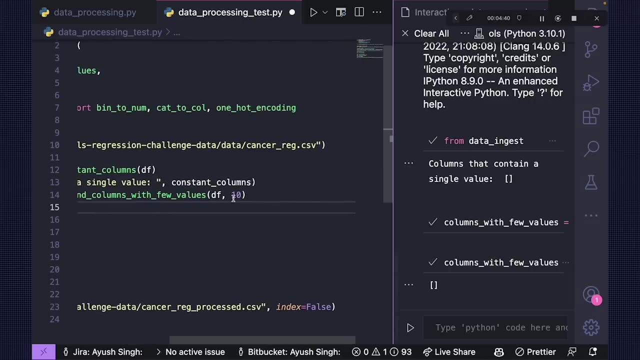 smaller than threshold. then it says that: append that column so you basically have the columns which has few, fewer, fewer unique columns. so it should also give you a empty slide which is: seeing, if you print this out, so i can just print it. print this out works like a jupiter books. so it says that: 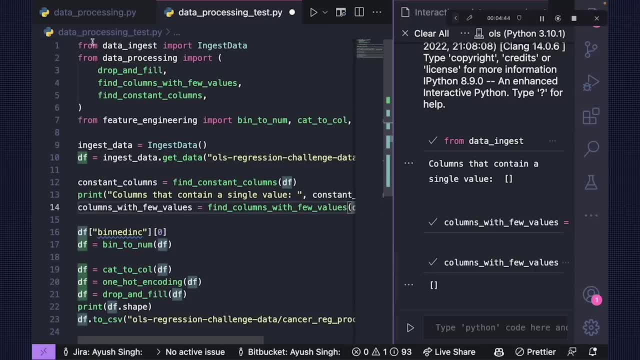 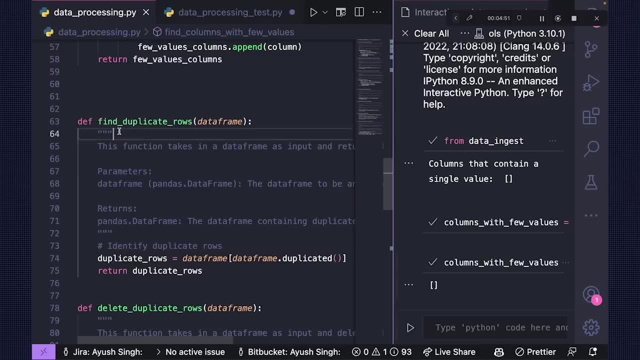 okay with that threshold- 10. you can. you can change your threshold. so, similarly, i have several methods for as a template for you to make this work in your further projects, like find duplicate rows. so it may- it may sometimes happen that you have a duplicated rows as well, so you can actually. 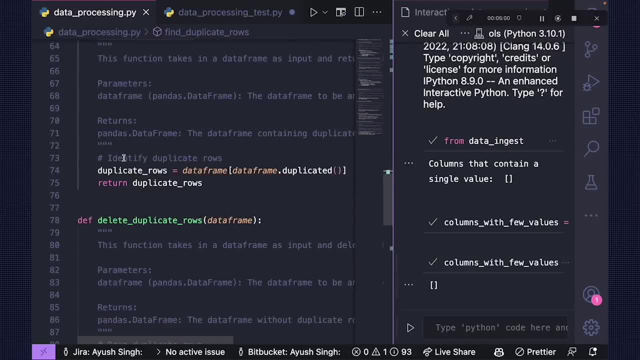 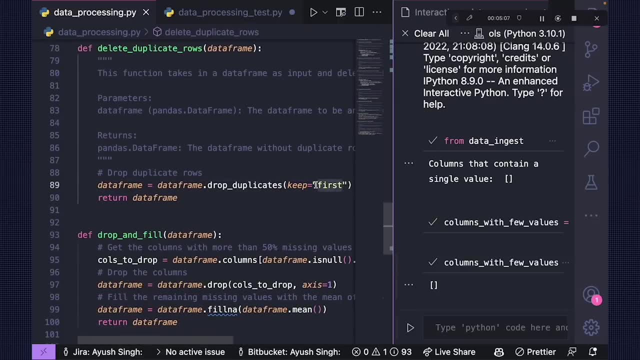 delete the duplicate rows by using these two methods, where you first of all find the duplicated rows by finding dot duplicated and then you simply drop the duplicates by keeping the first duplicate, so you so you might have first duplicate, second duplicate third, where the second and third are. 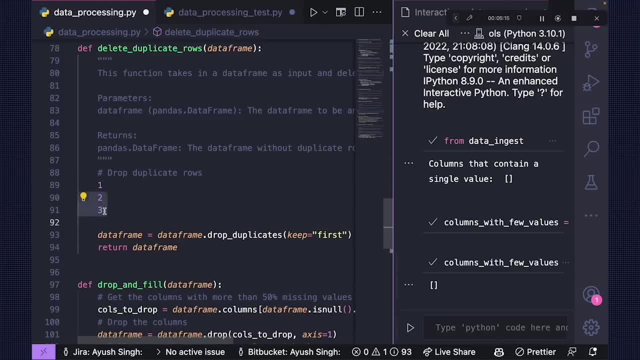 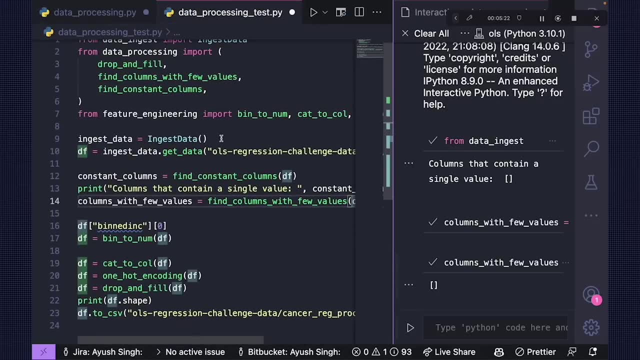 the same as first, then it keeps the first and drops the second and three, right, so you delete the duplicate etc. so you have a couple of methods now here, but but we are not, but we are not using that. so now you have the basic, you know basic things, which is just for us exploring things. 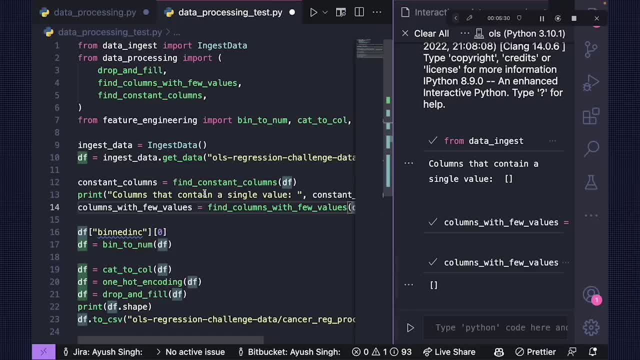 there's a lot to left in data processing. now we have all of this left. now what? what we'll do? we'll do some more sort of a basic feature engineering or feature construction. okay, that's called feature construction, right, feature splitting and construction. this, whatever I'm going to teach right now, is called 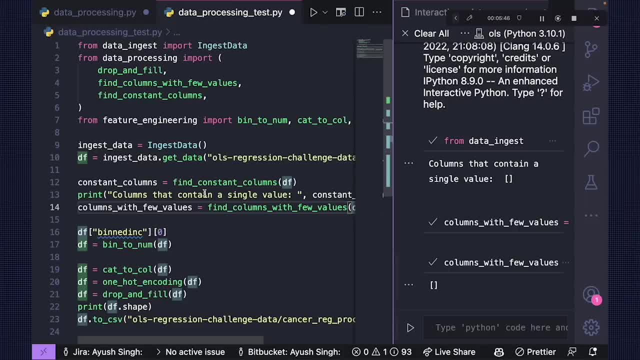 feature construction, feature splitting. so let's do that in the next video. so now, what you're going to do. we are going to talk about something known as feature construction and feature splitting in our data. so one thing which I would just want to highlight for you is: if you, if you see our 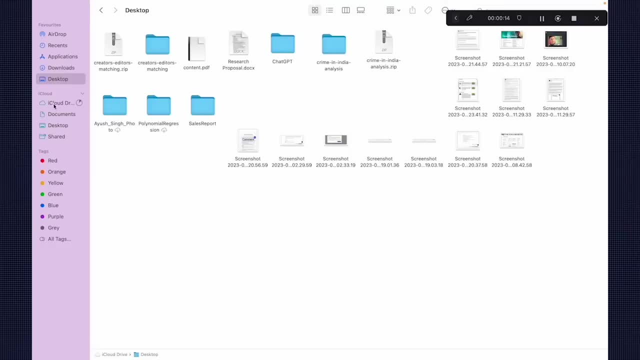 data which we have. if you see, our data which we have is: let me, let me just go to desktop and then let's let me go to my OLS regression challenge and then you have the data. now let's go to data and then let's open this data and then worry about two of the columns out here. 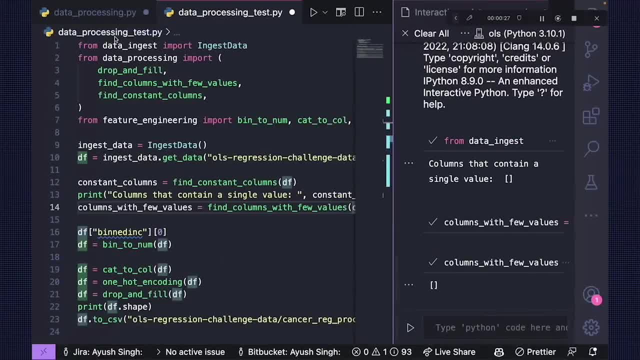 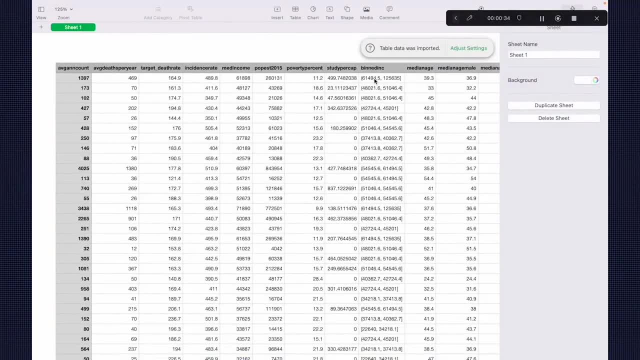 the first column out here is our bend. you know, you, we have seen where the columns for in a in terms of interval format. so you've seen bend bending where it says that your column is an interval format: six one, nine four. so this is your lower bound and this is your upper bound, right, this is a lower. 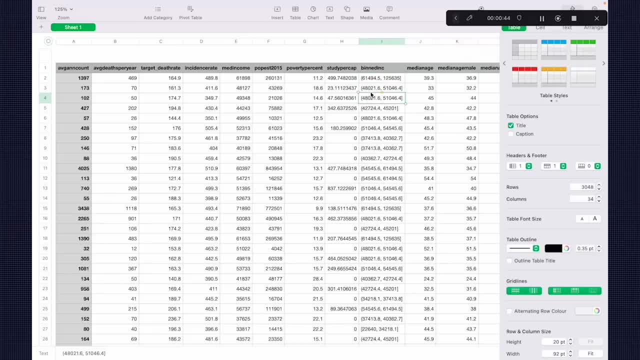 bound and this is your upper bound, right. so you have this column, so so it will. it is this of object type and the model will not make any sense out of it if it is left alone. so what we need to do, we want to take the first element and make you, we store the first element in. 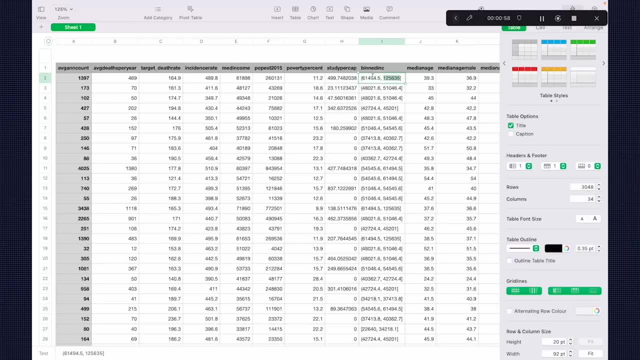 another column and take the second element and store that in another column. this is called the first lower bound and this is called the upper bound right. so what we'll do is split out. this will split out the where the values from this column into different different columns, by making 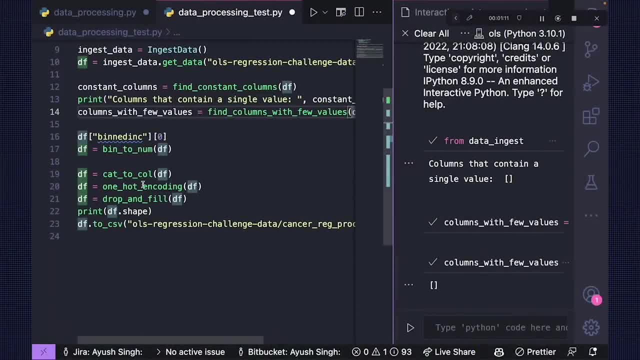 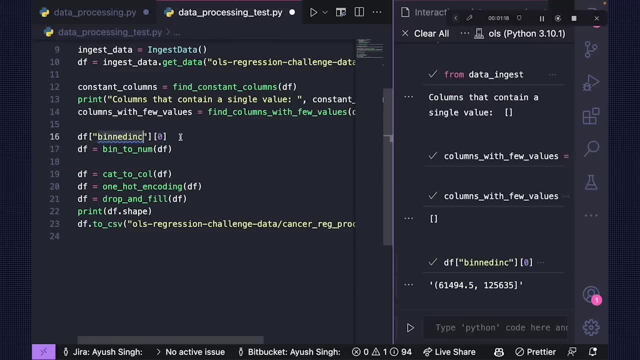 different, different columns, right? so let's see how we are going to do it. so we're going to use uh. so first of all, let me show you first of all what exactly that uh we are doing. we are using df data frame and then assessing that column, and assessing the first value of the column, and then 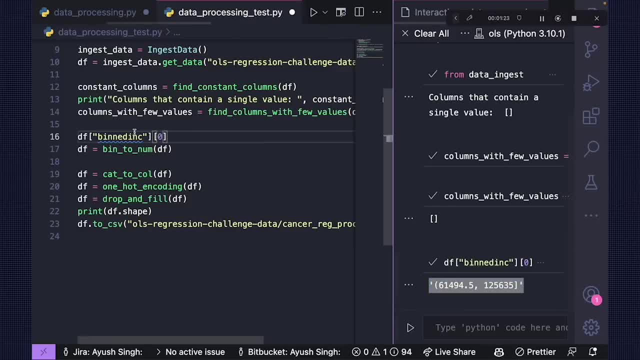 from that and the first value is this: if you see the type of it, if you see the type of it, so type of it is nothing but your string, i guess. so if you see the type of it, it is nothing but a string. so now you have that string, now you have make the column so that it should make sense, otherwise it. 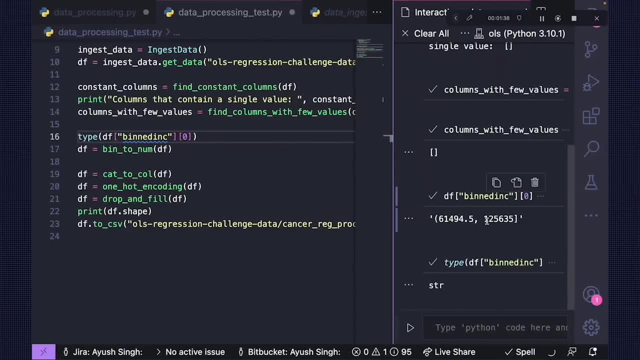 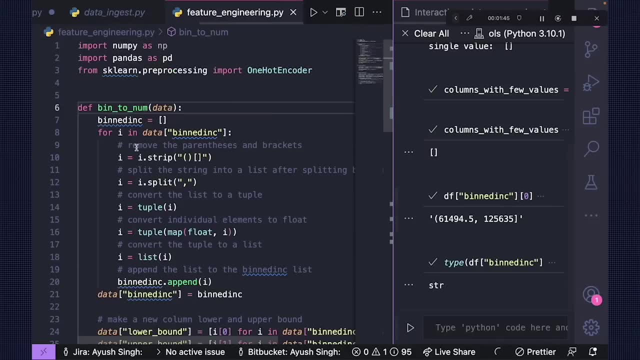 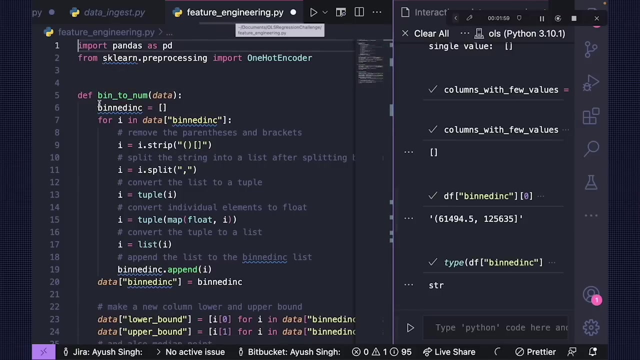 will not it. the model will not accept it. so whatever you're seeing in front of me is over here. we are just ignore whatever we have imported as of now, focus on this function. so this function is made in feature engineeringpy file and in this what we are doing, we are making a empty file. 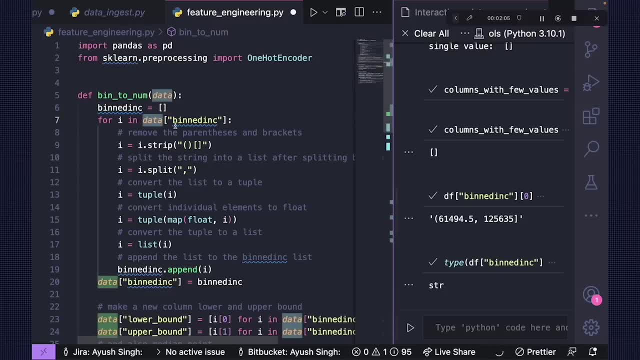 bin a dink where we are iterating in the in that column. so we are iterating for i in that particular column. so it will go through first value, second value, third value, etc. and then, first of all, it will remove all the parentheses. my point is that it will remove the parentheses and the square bracket, so it is saying i to strip. 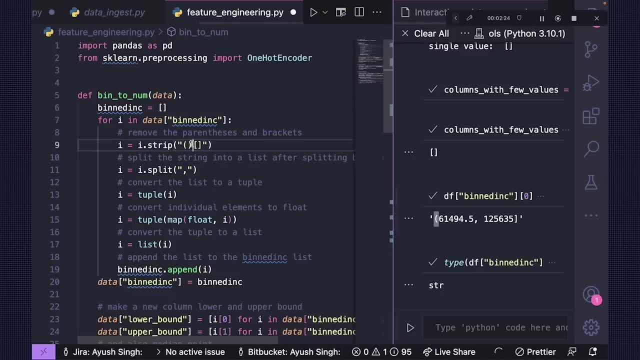 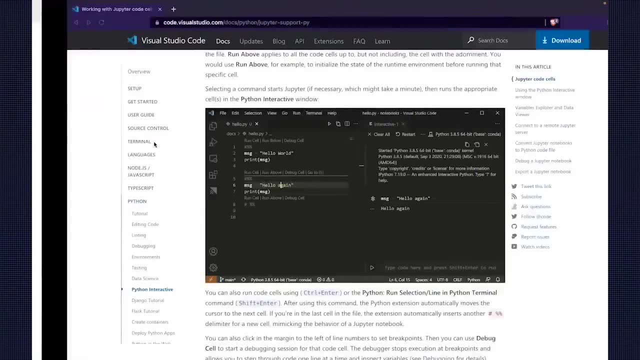 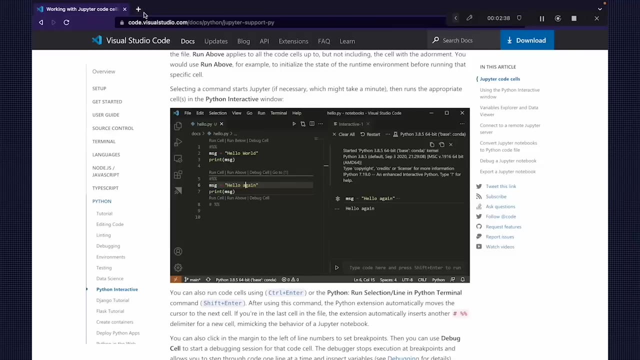 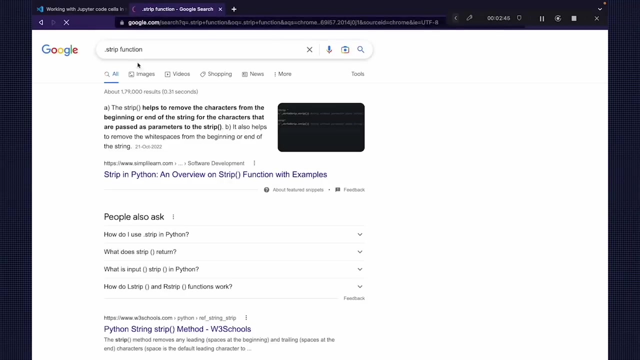 and then um, and then this particular uh, parentheses and squared brackets. so it will it. it will remove it. so if you see dot strip function in python, if you see dot strip function in python, if you see dot strip function, i mean um dot split, which helps to remove the characters from the beginning or the end of the string. right, so it. 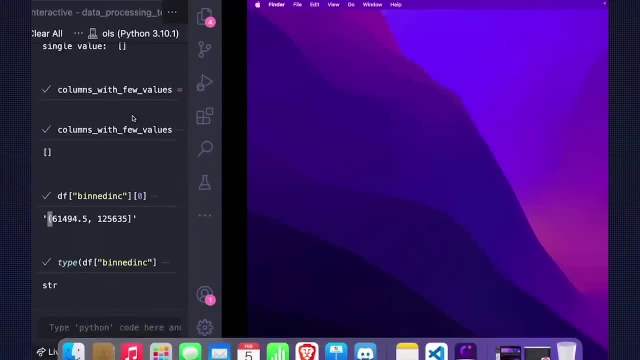 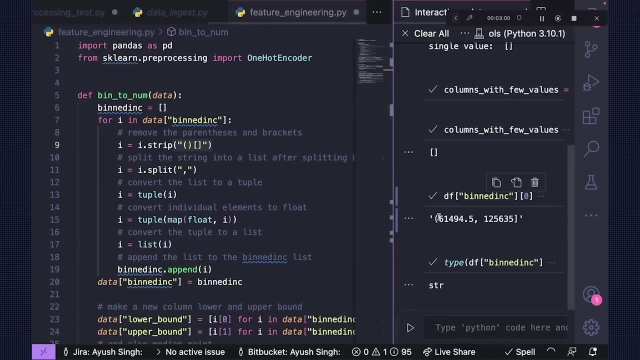 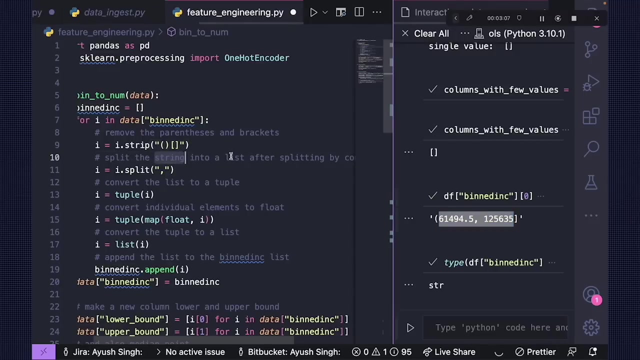 strips out. it removes the white space, uh, and any sort of values which we wanted to remove. so it's split. it removes the parentheses and brackets, in this case, this parentheses and brackets. now we have removed the parentheses and brackets, now we have this, um, and then what it does? it split the string into a list so we can actually, uh, split that string into. 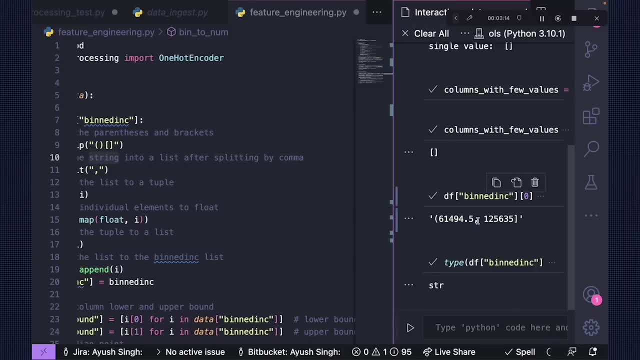 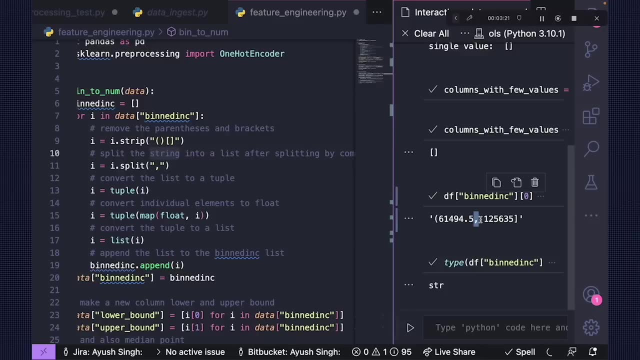 a list, when, where you see. so it. it says: whenever you see this column, split that, split that list, split that string into a list by this. so when, when, when, when, the. when the push program sees this particular column, it says, okay, this is the first element, and then splits these two differently. 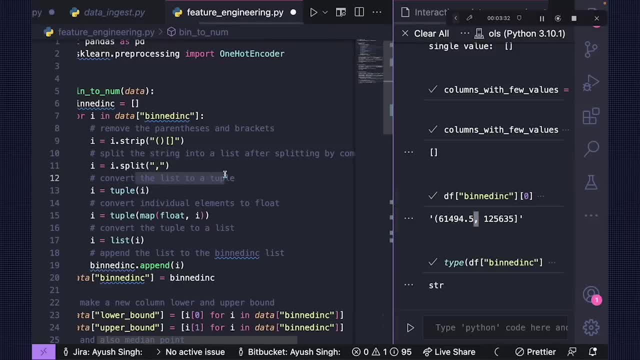 right. and then what it does? it converts the list to a tuple- um, considering that we should have a unique stuff. and then it converts the, converts individual elements to float. right, so it from the tuple, it maps every individual to float. so each and each individual is mapped to float. and then, finally, 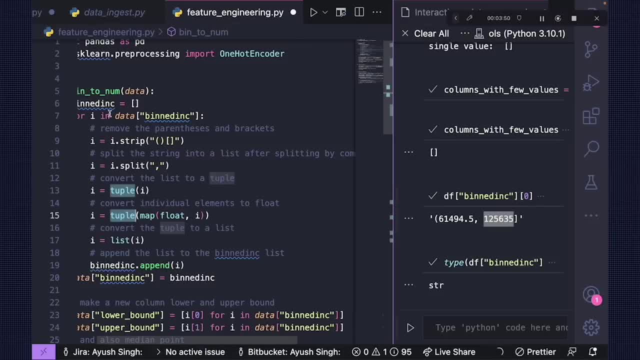 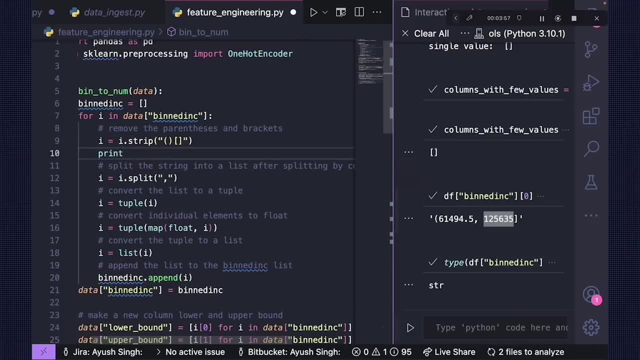 convert that list to a tuple, to a list, and then you append that particular- uh, i, that particular value into this. so if i could show you, if i could show you what exactly each steps looks like, each steps looks like, so let me just show you each, each step. this should make much more sense, i guess. 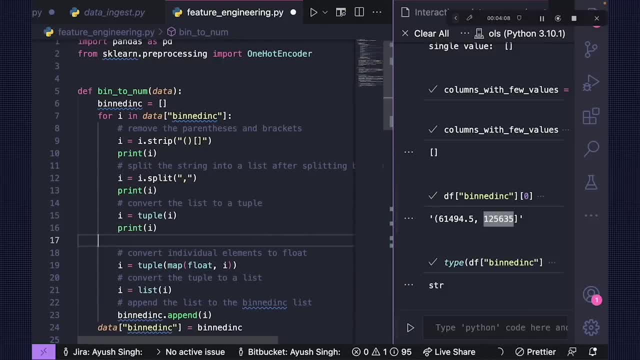 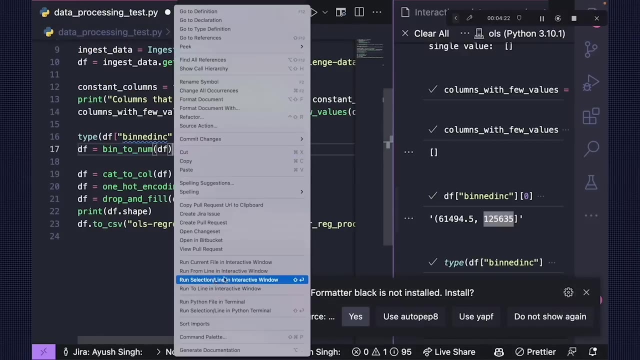 so let me just print each and every eyes, uh, whenever you actually uh, go ahead and then see that, right, that should make much more sense for you. um, let me just go to data and chest data test and then let's run it. first of all, we have to, you know, save. that it will not work if you don't save. 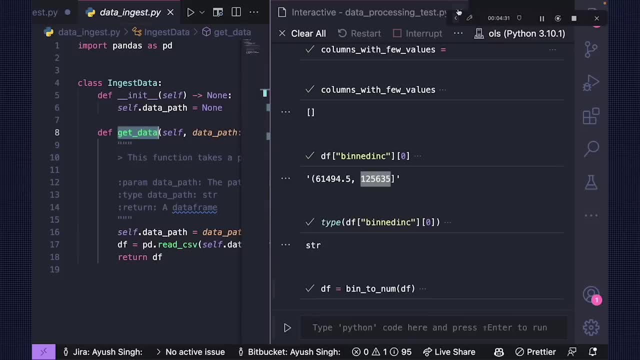 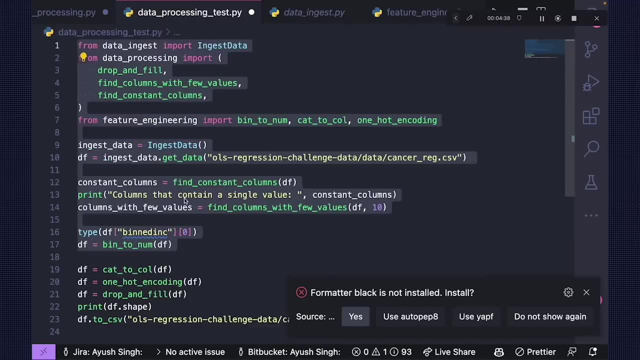 it. so we have to save that. we change running and then just save it, and then we have to save it, and then we have to save it, and save it first of all and go to data test and then now run it from here to there in an interactive. 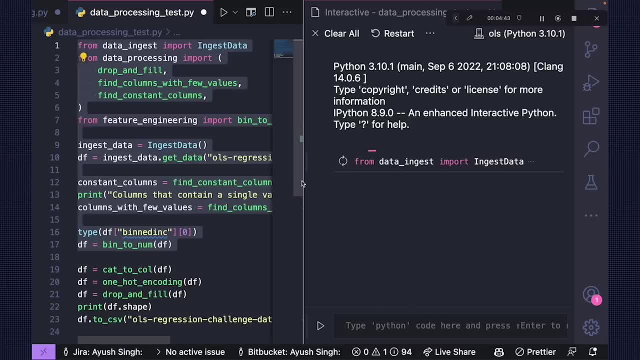 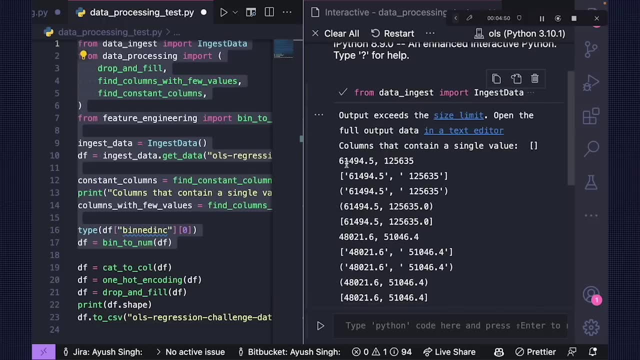 window. it will take some time to run it. so now you see, now you see the. for the first it was this, it was this, it was this, then it, then it converted into this particular thing. that then it converted into this particular thing by removing all the parentheses, by removing all the parentheses. right now by removing all the parentheses over this fire stolen. it means that weáb기가 is a parent. this dollar. there are only six states. a lot of other states, a lot of other states are two states, a lot more of like a capital states per one state, but a specific state there are. 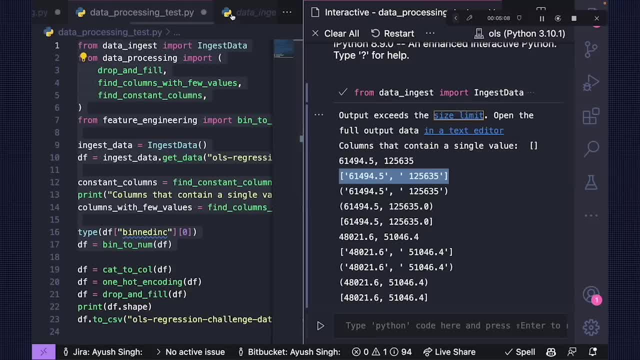 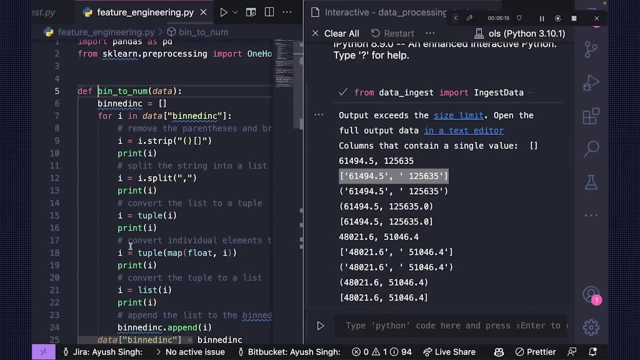 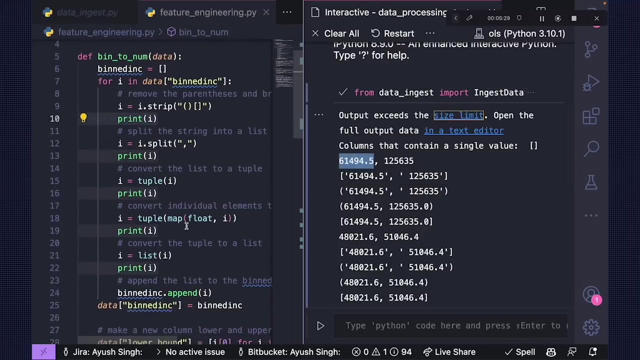 So basically, you can see now Where I was data engineering. So you can see, over here we are first printing I, the first printing I, with the removal of All the values out here, with all the values out here, and then we are getting the value of I. we are getting the value. 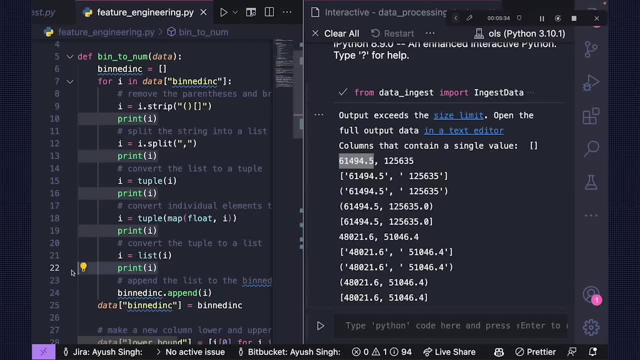 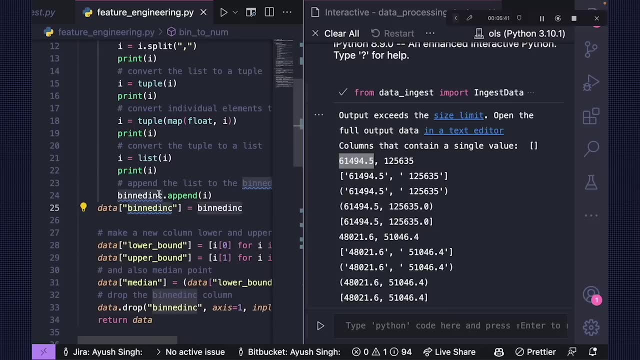 Of I, which is, you know, Specified value, right, which is the which which we wanted. now you can simply say, you can simply what, what? what you can do Once you have the value, once you have the values, which is removing all the processing stuff, which is converted into a list. 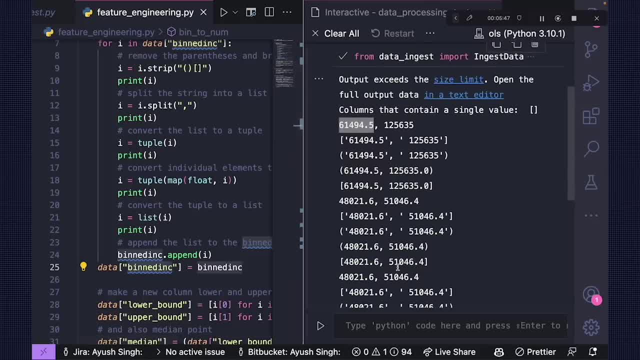 Which is going to convert into a list, which you can see over here, Which is converted into a list. now that list can, now that list can be added instead of those strings, right, And then what we do? we say that we, we make a new column data. 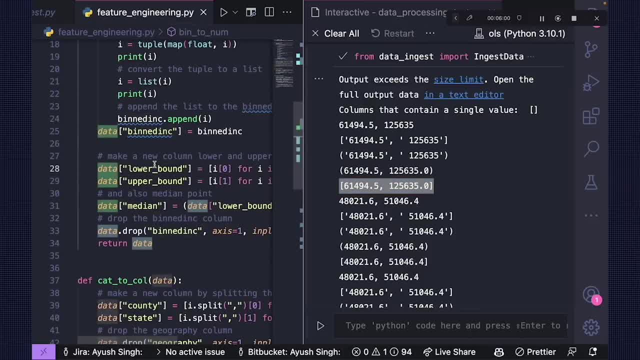 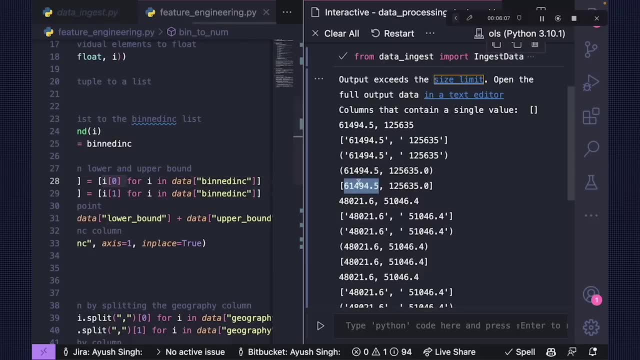 Which is of lower bound, make a new column, and then we say that now that list can be added instead of those strings, For I in that Bendec, Take the first element in that list, take the first element in that list, and then we in up in upper bound. 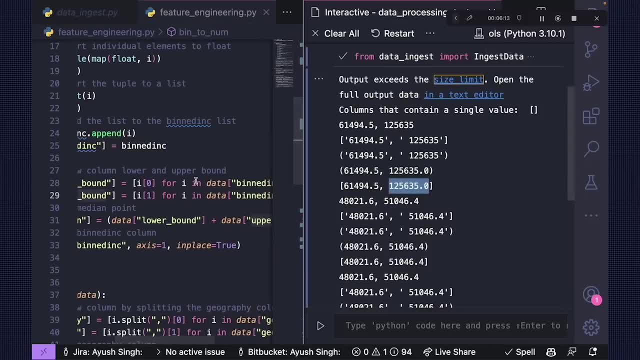 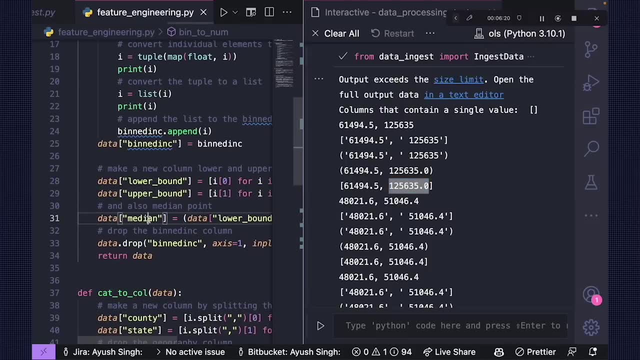 We say that take the second with the zero, the first element in the, in the lower bound zeroth, and the first one first. So we said for every, each and every values, right. We also make a column called median, where we see me lower bound plus. 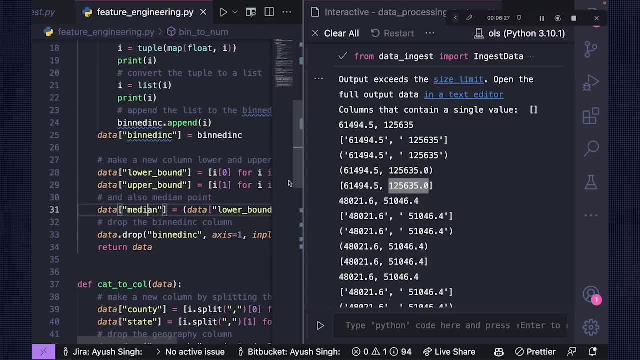 Upper bound divided by two, that will give us median, and then we finally drop that column, which was useless in this case. So we simply drop this column, Bendec, right. So this is how, basically, what you're doing is simply taking this value, putting this another in one column named lower bound. 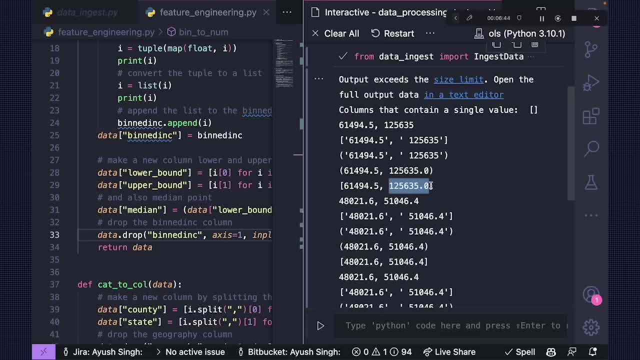 Taking this value, putting this in another column. We named all upper bound- and then we are taking the median of both of this, like this First element plus second element, divided by two and may storing that in another column. that might be useful, right. So now this will start making sense. So what we did? we split it. the feature is split at the intervals- and then we used 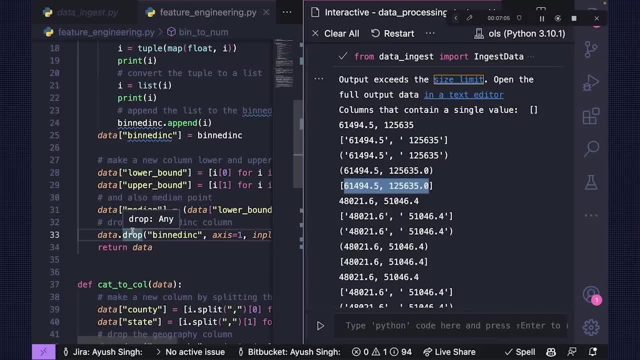 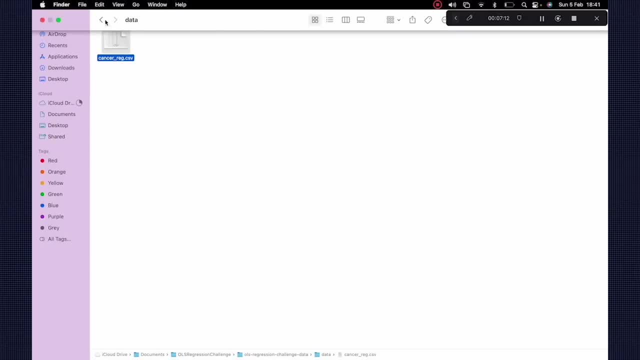 Accordingly, according to a statement, and then we drop the columns which are useless. So now we have the information, which is good. So this is what? quite what we did now, if you go and see our data which we have. So let me, let me just show you the data which we have. 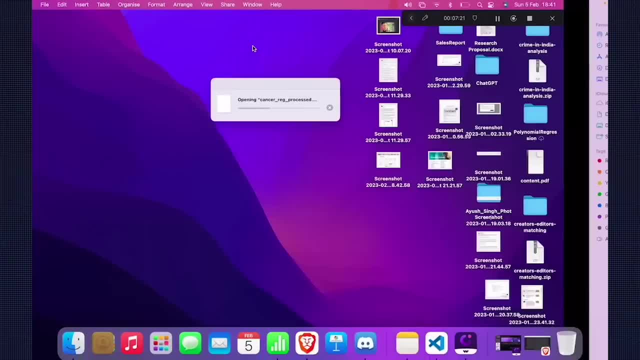 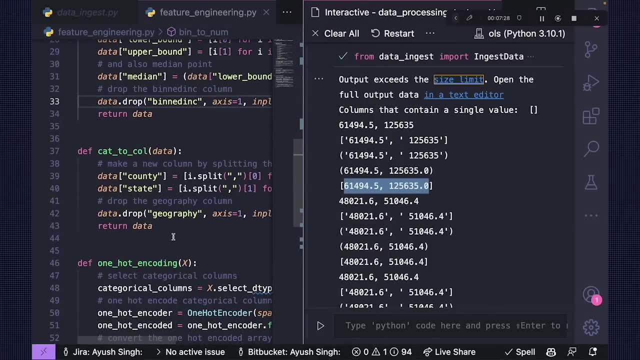 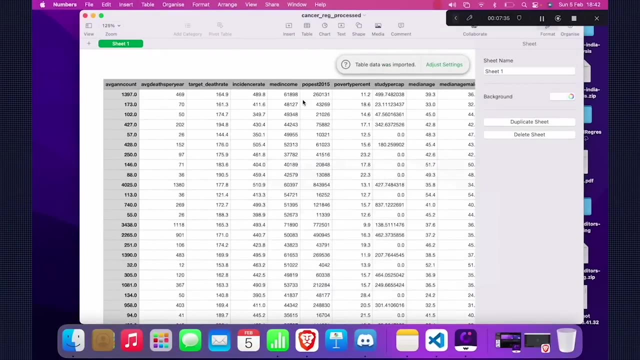 You should wait for a second Still opening. it's very big, to be honest, Yes, and then. and then we'll go to categorical, to column, and then we'll talk about categorical encoding in the next set of lectures. So if you see out here that spreadsheet now, if you see over here now, 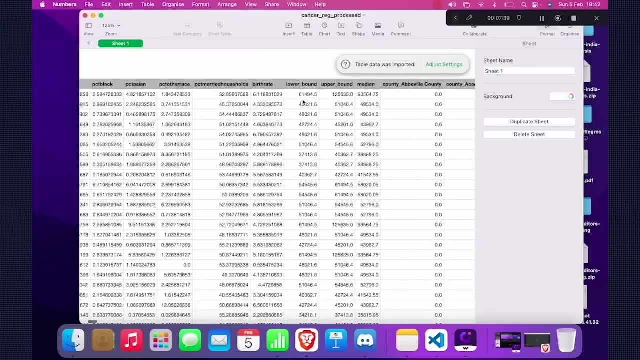 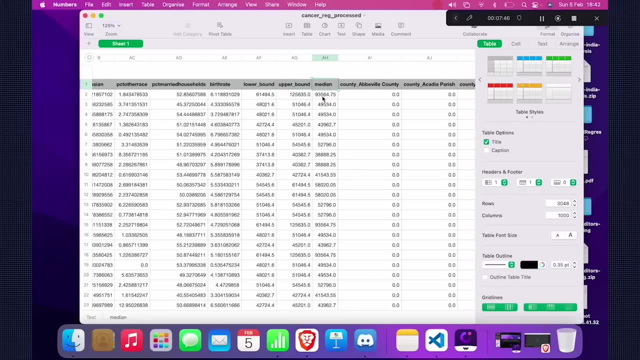 If you see, over here you have something known as upper bound and lower bound. So let me just show you to you, first lower bound, So that lower bound have this particular values, upper bound had this particular values and median is this right? So we have. did we remove that? because that was more not picking sense because of interval. that was a string and model will not. 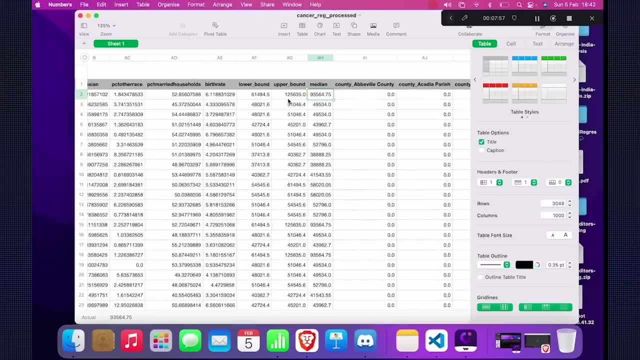 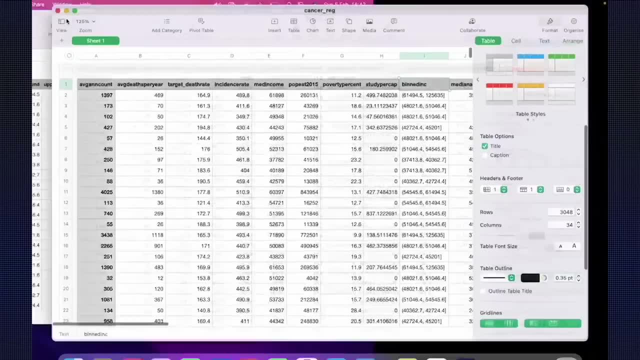 Make sense out of it. We made something like this, which will make sense to our model. right Now we have something that's categorical. so now, Another issue which we had, and another issue which we had. I'll just want to show it to you. 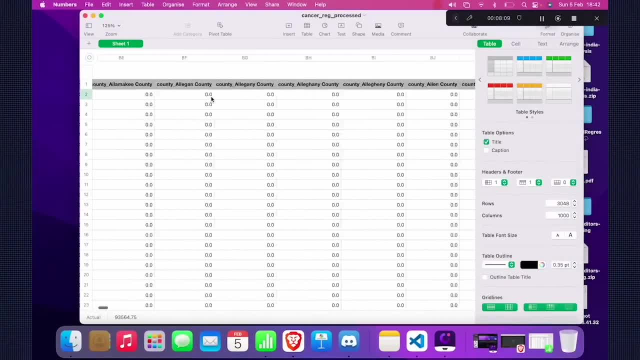 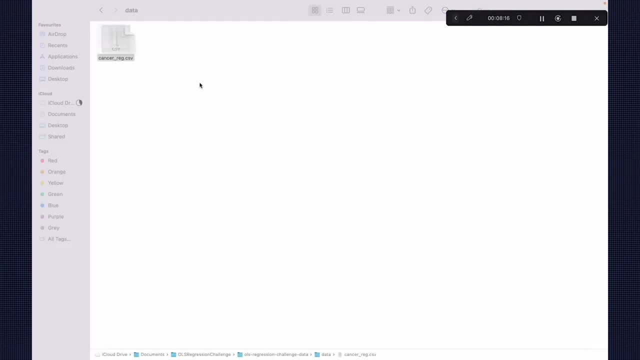 What issue which we had is this particular column? Where is that column Data? and then we just going to show it to you. That's much more better. Yeah, so see this. now we are done with this. now you see a geography column in geography column. 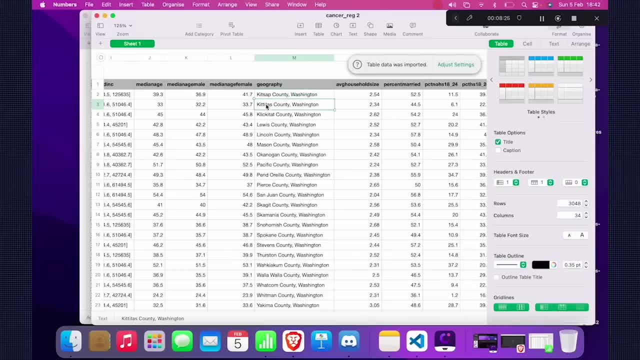 We have the county and the state, right, county and the state, so both had the same point right. So can't we have a spark and we split this feature again and then have Count in another column and State in another column? that will make much more sense, right. 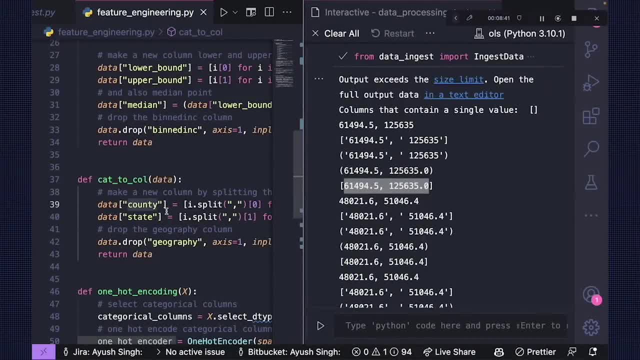 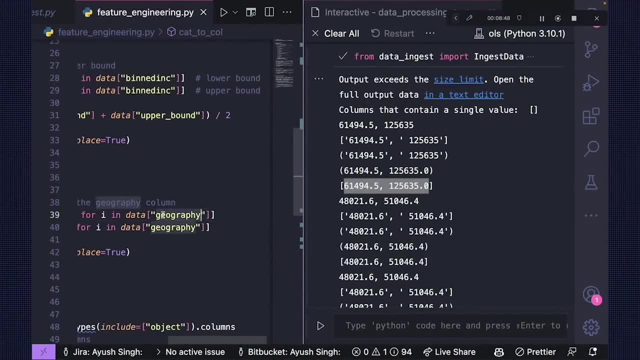 So what we do? you simply say, you simply say: count e. we split that with that comma, because comma is there, so we split, we're using the comment. then we say that for, for every column in Geography, and then we say that click in, in this case, 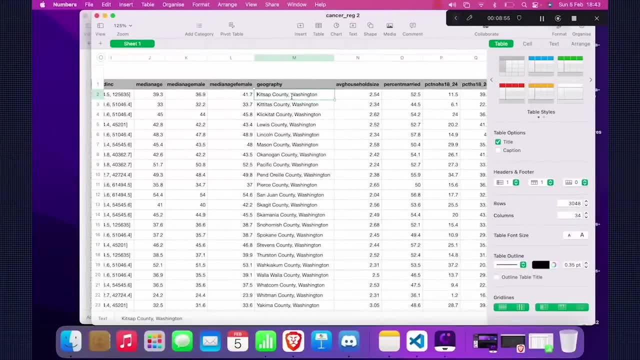 We are absolute of a zeroth element because this will be converted into a less now. now we take the zeroth one because it was splitting the impendant with the help of Famasot 8 paper, convert into list and then we take the first element. 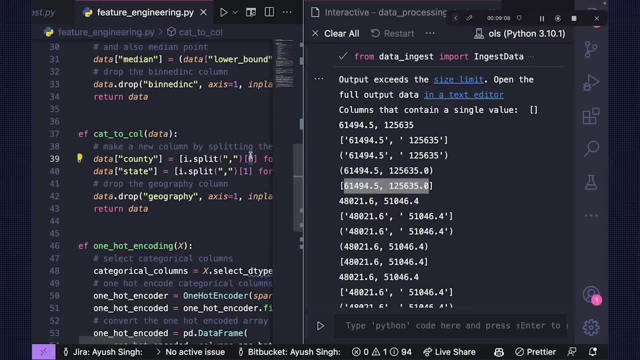 and then we take the first element and store that in a county column. and then we take the second element, which is of course worse because it starts from zero one. so let's take the second element and store that in a state column and then we drop the geography. so now you have another. 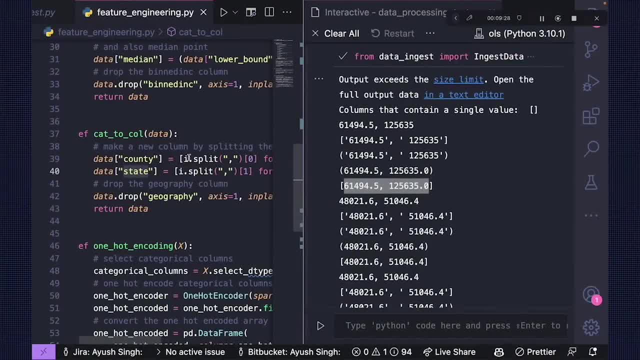 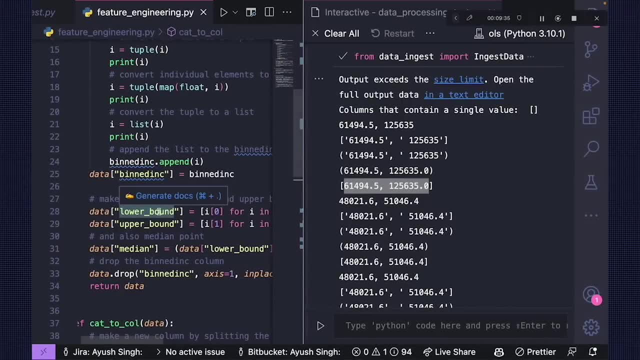 column for kits app for counties and states. right, so that that is feature splitting and reconstruction. this is this is the processes called feature splitting and reconstruction. i hope that you got it very nicely and that's it for this right now. so what i'll do in the next. 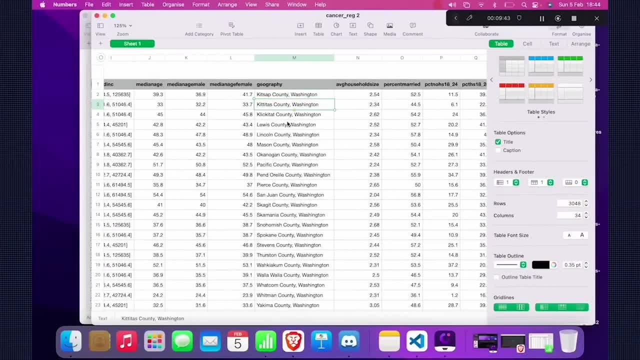 set of lectures is actually talk about. we have this, something now. we have the columns, which is splitted. now we now, how can we convert, how can we make use of the state and the counties? and how can we convert that, how can we make sense out of it? by different, different methods of categorical. 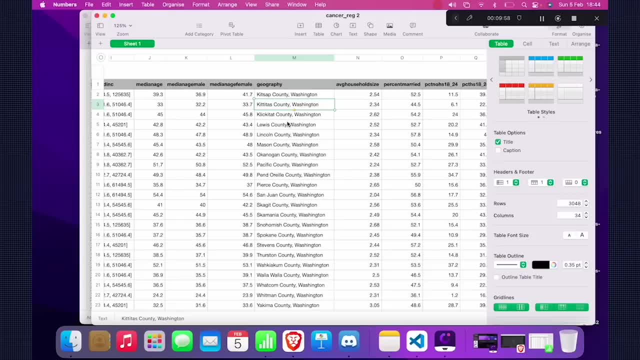 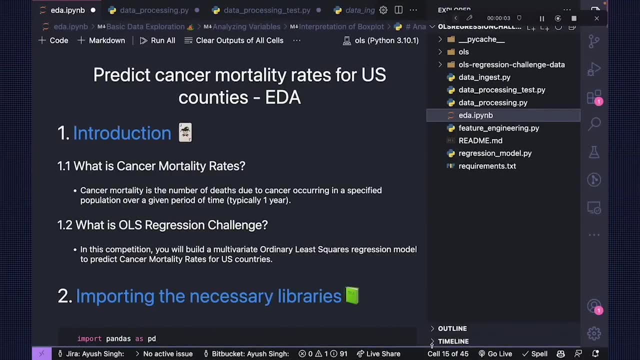 encoding. that's also super useful for you to understand. let's go back and let's go to the next lecture. so, hey, everyone. so now, uh, in this, what i'll try to achieve is just what i'm going to achieve is try to give you a very nice and complete our feature engineering techniques, which is 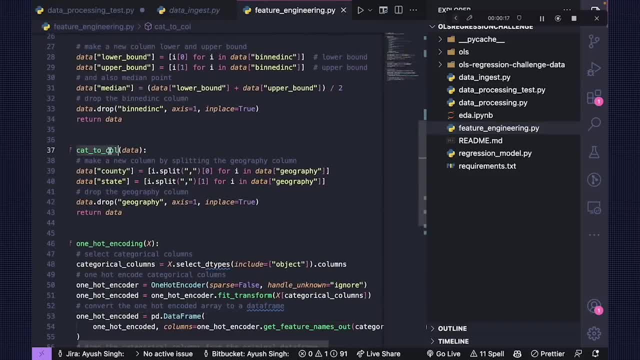 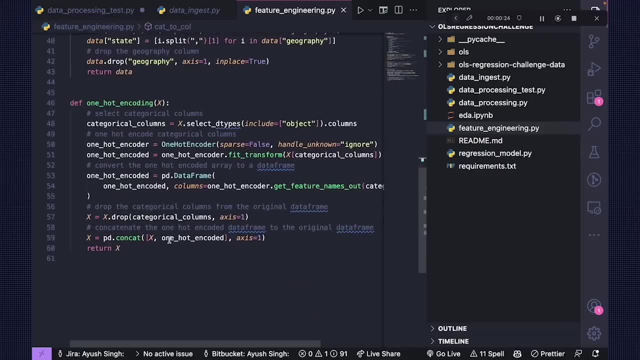 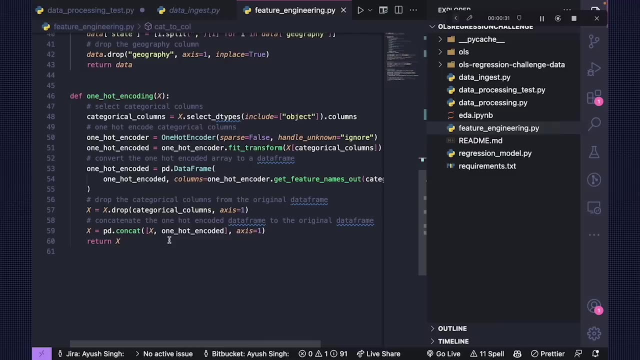 till the previous lecture. we have completed this categorical- uh sorry, to the in geographical column. we have converted the geographical column into two sets of column, which is county and state. what i'm going to do next, it is talk about one hot encoding, which is- we have seen the, the, the data where we had the values, which is categorical, so now we had the two. 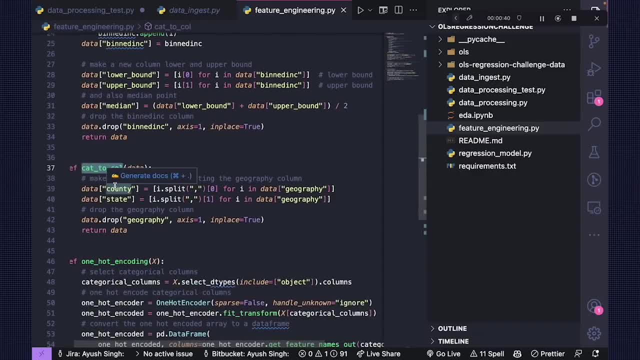 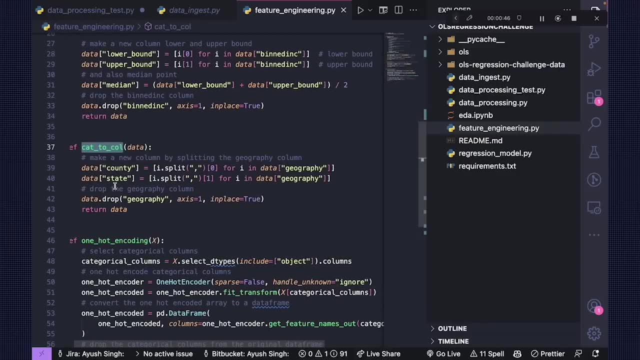 categorical values, which is this county and state, and county we have some other, and state we have some other set of values. now we have to convert this into some sort of integer or numeric that should make sense to the model. right, that's your. your model should be able to interpret it right. 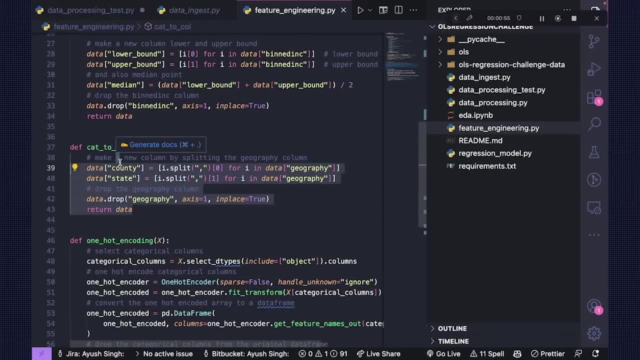 so now what we need to do? we need to: um, you encode those categorical variables, right, so we learn encoding techniques later on, but we'll encode those categorical variables, or try to make sense out of that english, otherwise it will give a very a good error, because your model will not accept. 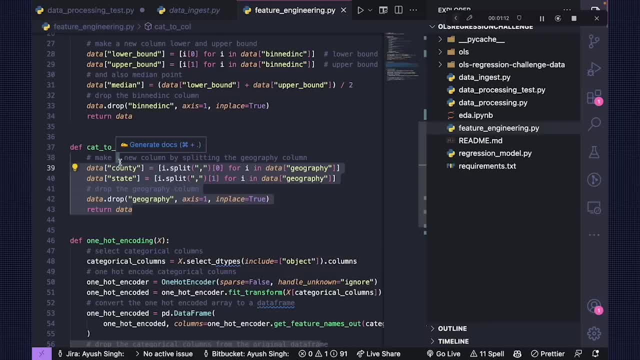 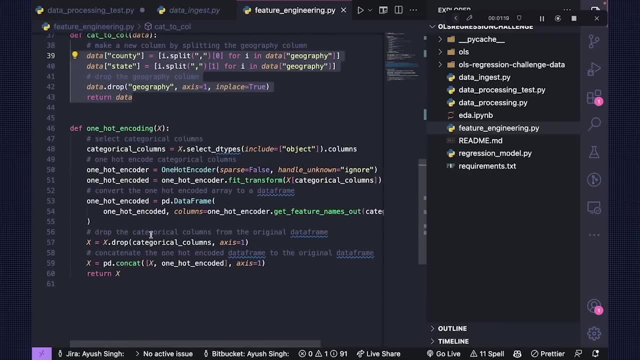 the english stuff. it will accept only the numeric, and you have to make in such a way that it should make sense, okay, so so what you? what exactly? i'm doing it over here? whatever you're seeing in front of your screen is you have a categorical columns in that categorical, categorical columns. you are. 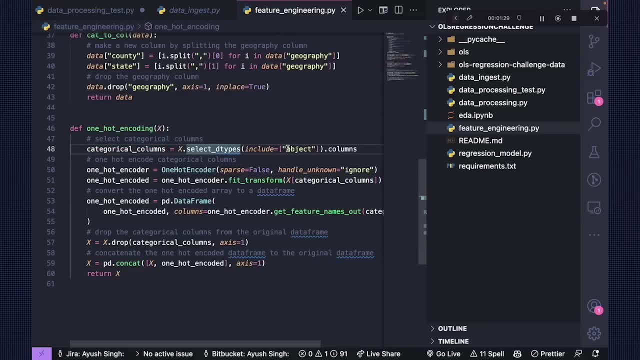 selecting if in that data table, selecting the data types, which is, the categorical columns which are of object, and they're selecting the columns, so basically what this category column states that this is a list of category columns whose object is data type. so most of the category categorical columns whose data type is object, right, so that's what we first of all select: the. 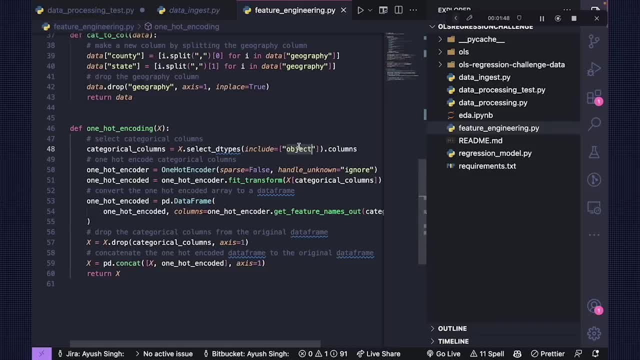 categorical columns. and then what we do. we have the one hot encoder, you know uh instance. we create an instance with the following parameters. so let's try to go ahead and then talk about what is what exactly, one hot encoder. so i'm just going to go ahead and then talk about 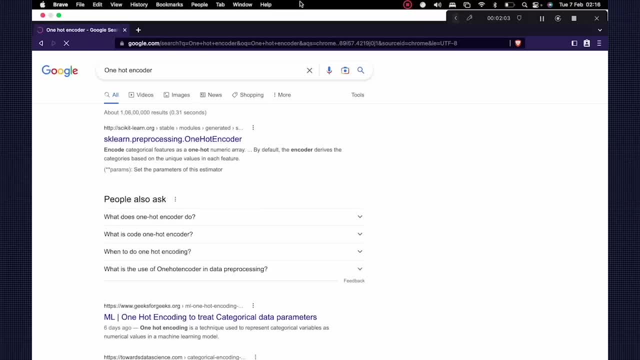 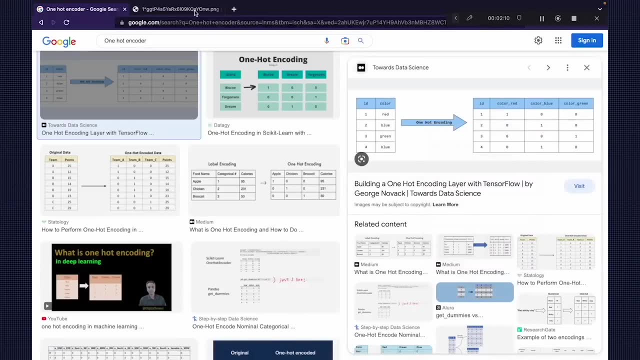 this one hot encoder and then i'm going to show you a very nice visual, a quick, uh, understanding of that. so whatever you're seeing in front of my screen, uh, so see this: you have the categorical, very variable. you have a categorical variable which is color, and then, in that you have red, blue, 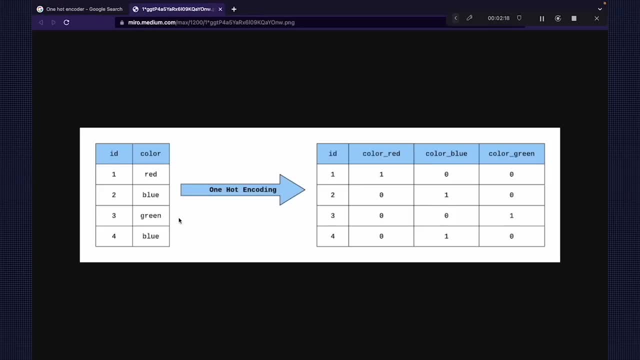 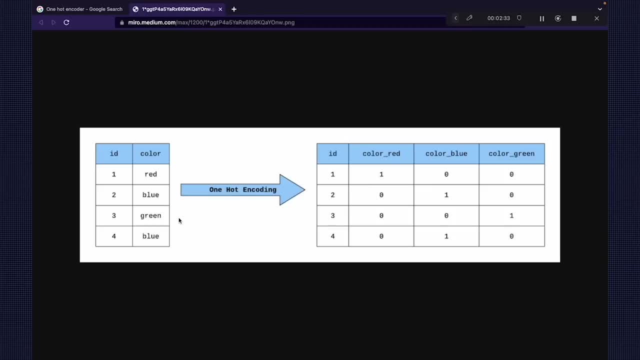 unique um values in that particular column will be the equals to the number of new columns which will be created. and now for this. assume that color is uh for the. for the example, in id number one, id id number one- we have color red, where it says color red is present but color blue is absent. 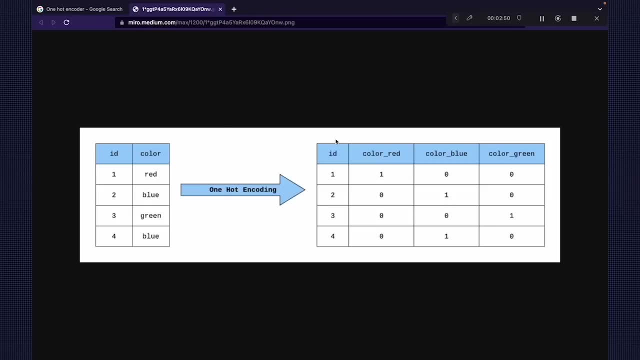 green absent and zero blue is absent. right same goes with color blue. and then in first id color blue is absent, but you see, the color blue is friend, so that's why it's one. so basically, what we, what, what we are doing eventually is removing uh is is is converting that into a dummy, variable type of thing we're creating. 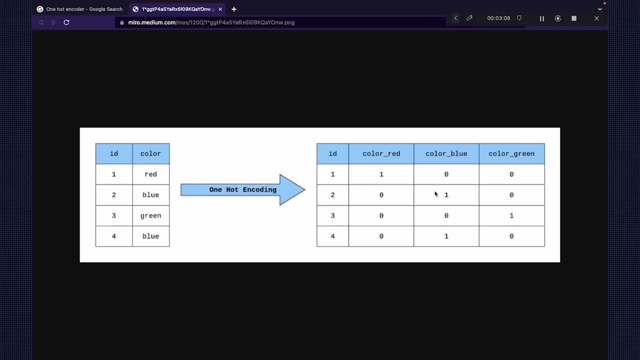 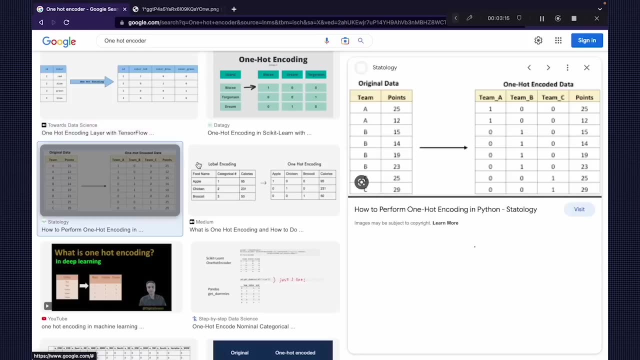 creating some sort of dummy variable for every values and then we are seeing if that particular variable is available or not in that right. so i'll tell you a very nice example in this so you can also go and see the other set of examples. so let us assume that you go and see this one. 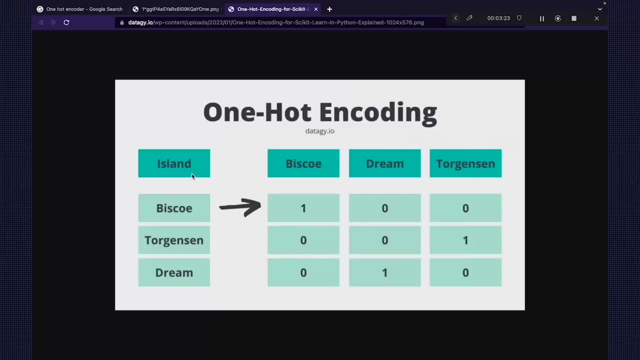 assume that you have seen this example, and in this example you have island as a categorical variables and then for every categorical variables you have the, you have the columns created for every means, the unicategorical way, uh uh, counts in that. so biscoi, and then in biscoi the first id is one, because it is present, but tungsten is not present. 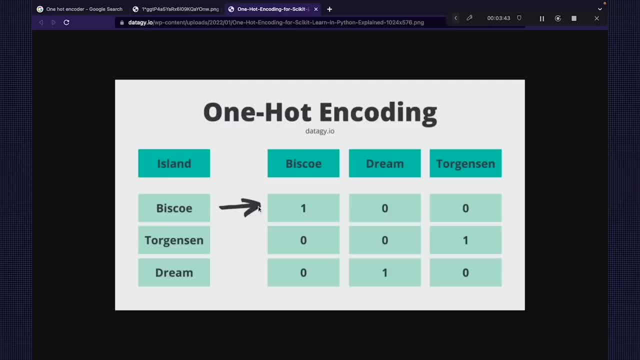 that's why zero in the first id, in the, in the first id right and see my mouse. so in the first id, biscoi is only present. then a second id, at the last column, dream is present, and the third we have second, tungsten is present, right. so this is how we create new set of this. this, this is how we. 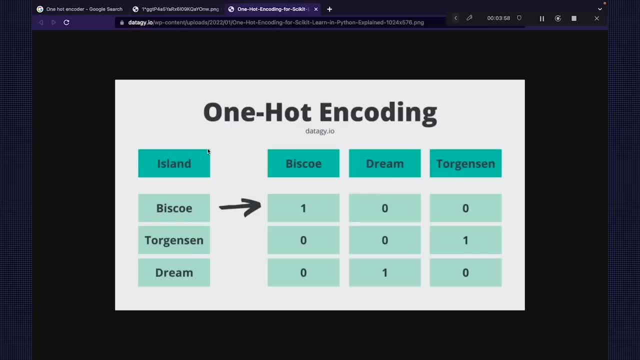 convert this particular one column to the number of occur to the number of columns, that we have a column which is equal to the number of unique values in that particular categorical variable. and in that and and how we do it, we have the particular id and then we see that id is present. 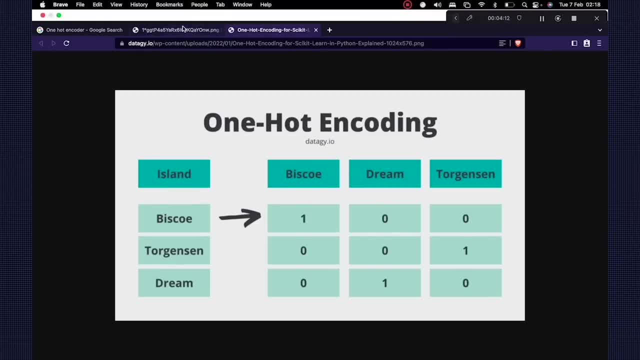 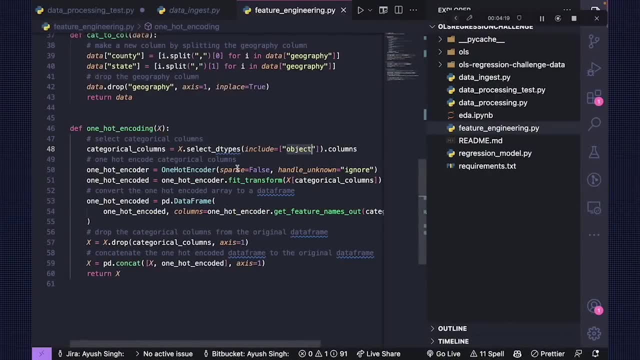 in that particular column, or not, right? so i hope that this makes sense. i'll be giving you a very, very nice example as well. so this is what the one caught encoding will do. which over here, what is this? parse is equal to true, and then handle unknown is equal to true. so what is this? uh, variables. so 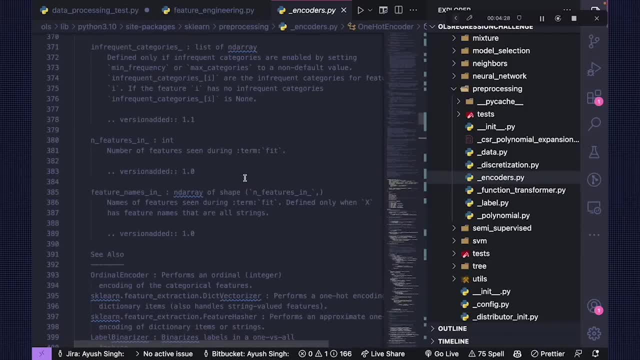 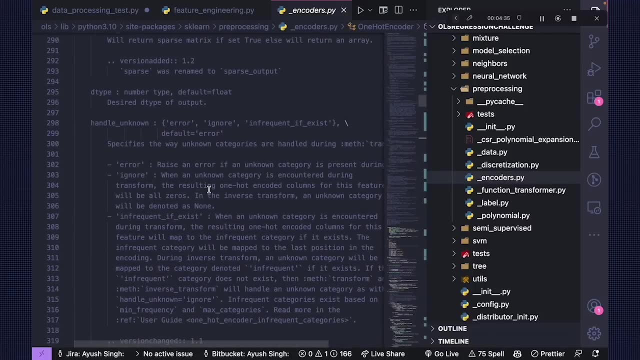 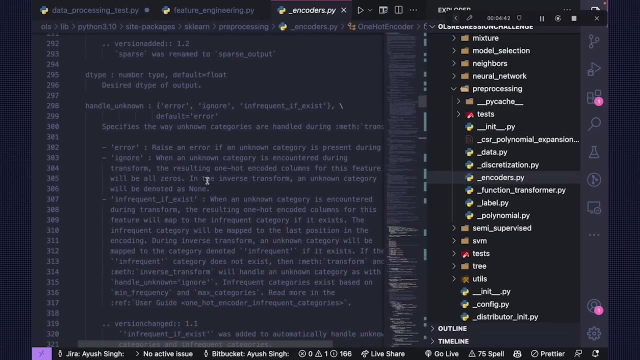 handle. unknown is nothing but, um, i think that there is a very nice set of yeah, so handle, and unknown, which is this specifies the way i think there should be some. uh, yes, so when giving an input. so, when given an input, uh, if there is any unknown. 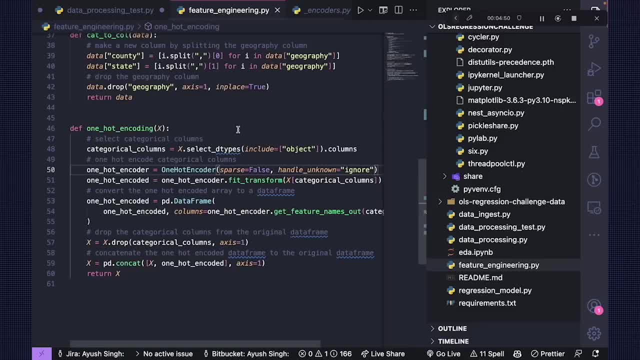 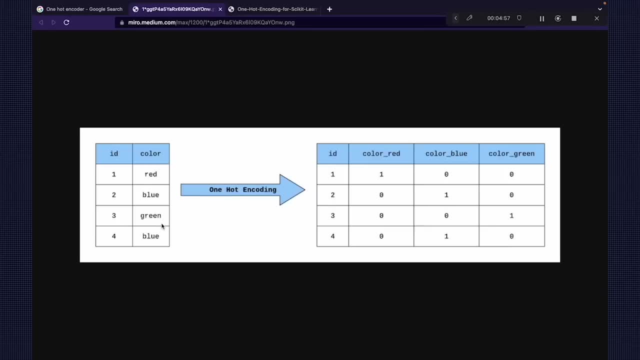 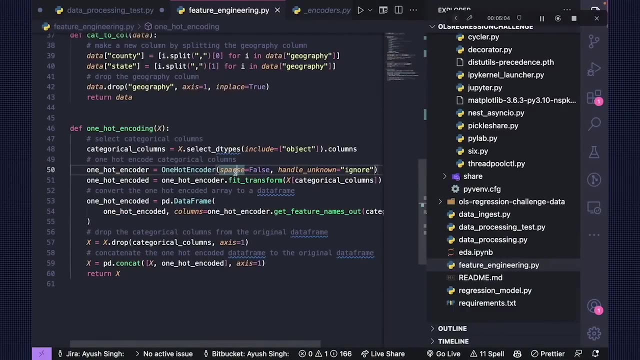 values comes in, so ignore that. for example, for example, in that categorical variable, apart from this, apart from red, blue, green, apart from this, some other you know, a violet color comes in, but that's not present in your data, so we have to. it is asking to ignore that part. okay, and then sparsity. we are saying that as a false we, we, we don't have. 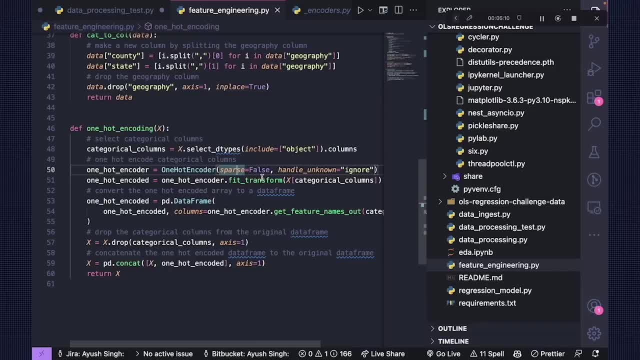 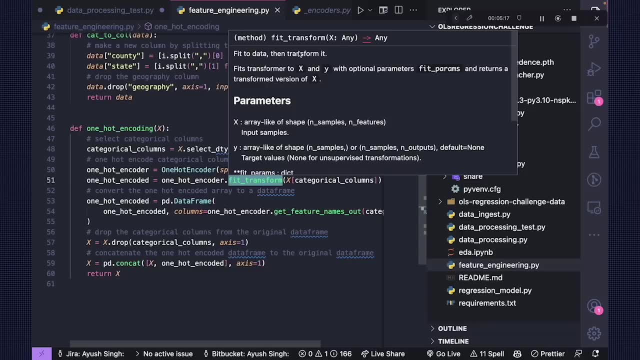 a sparse data, right. so now we instantiate, then we say fit, transform, fit, transform it fits and transform. so basically fit the transformer to x and y, uh, which is a fit the data, and then transform it like. first of all fit the data like: have the? uh, all the, all the cat, all the things out here fit? 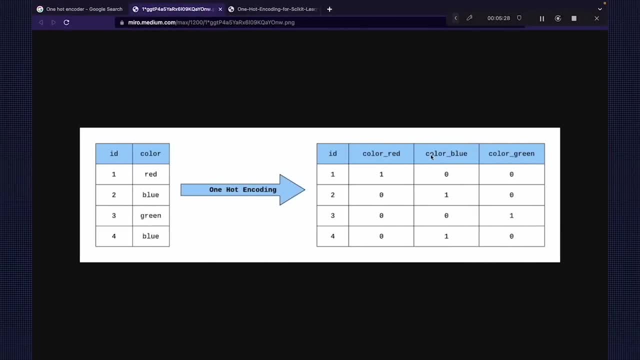 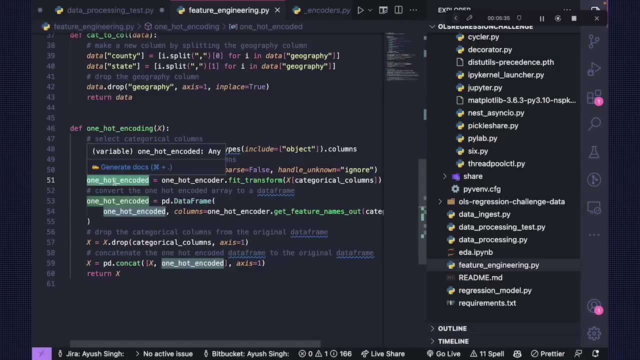 the data and then transform it like: convert that into the categorical variables over here, right? uh, for all the category variables on your data set and you have one hot encoded which is the data set, which is one hot encoded. now you convert that data into a data frame, but and then you name. 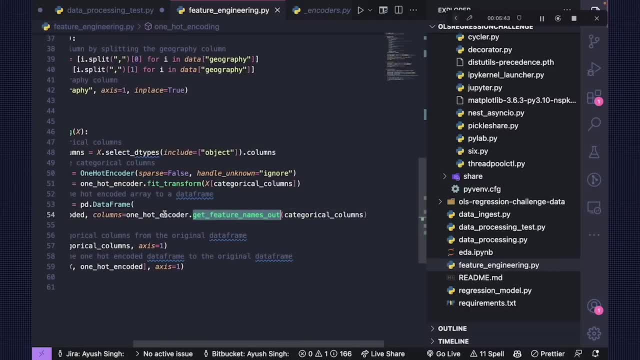 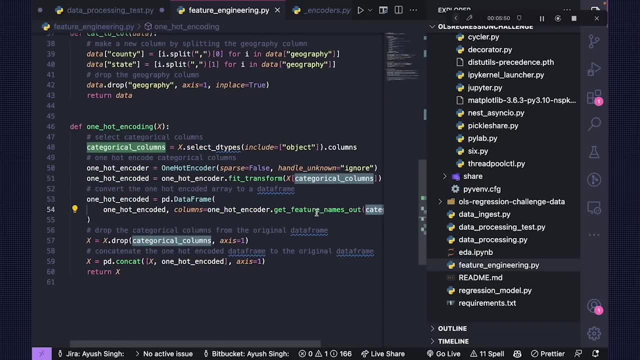 that feature by getting the get features names out, using the one hot encoder um object and then using get features names out, by giving that particular categorical column right, you name that as a columns. and then what you do? you drop the categorical columns which are now you have. 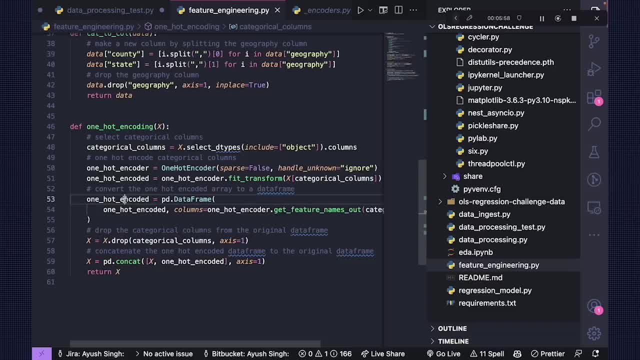 the geography. now you don't need the english column, you already have the numeric converted new encoded column. so you drop that and then you concatenate the numeric which, which, which was there, and then the official data set. okay, so i know it. it might make sense to for you to maybe understand. 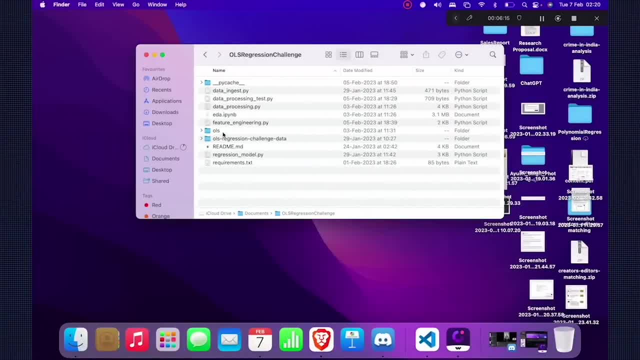 it, but let me just make you clear with things. so let me just open that uh ols and then let's go to uh processist. let's go over there. it will take some time because it is a very huge data set now which is which is being created, and i'll explain you every part which is happening over here. 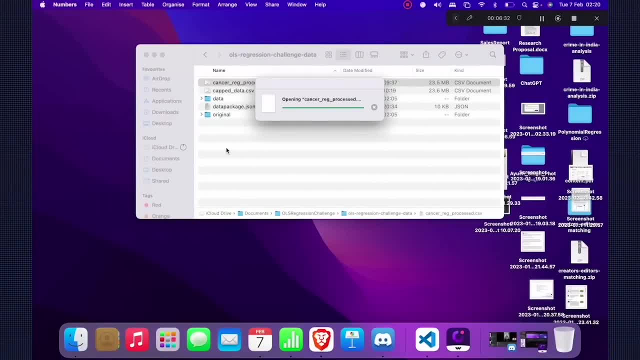 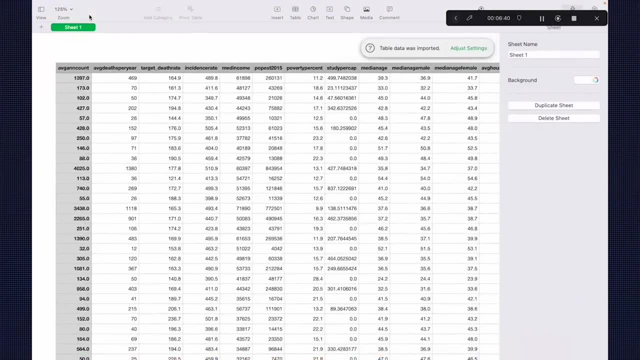 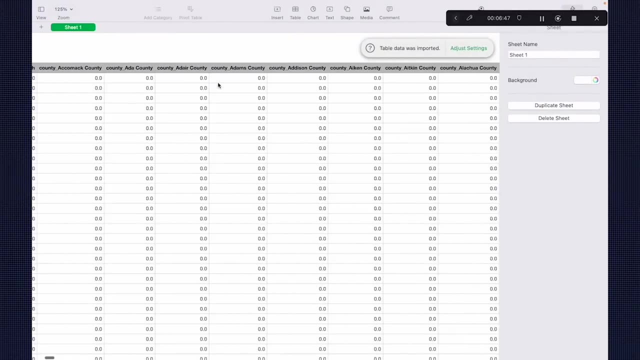 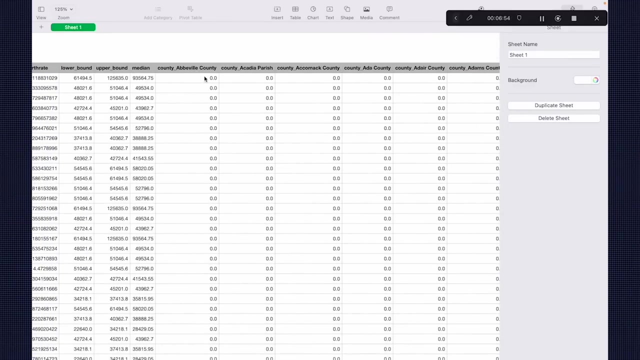 so let's, let's, let's just wait for opening. yes, so you're seeing in front of, you're seeing in front, you're seeing in front of me, which is, uh, your first categorical column, which is that geography, that geography is now converted. so now you see that we have county of abelia county and that first id, it is not present. so 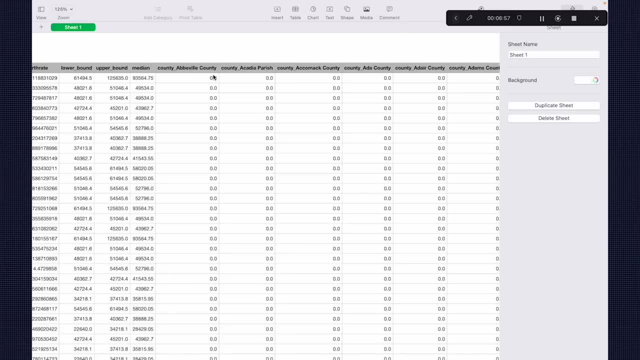 every unique id of that particular county. uh, that's that every unique value of that county variable is converted into the columns. now, if they're converted into a columns is now, if you see that if that ability is per present in the first row or dot, it says no, it's. 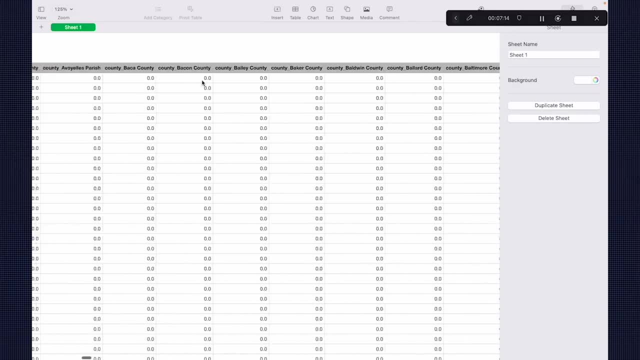 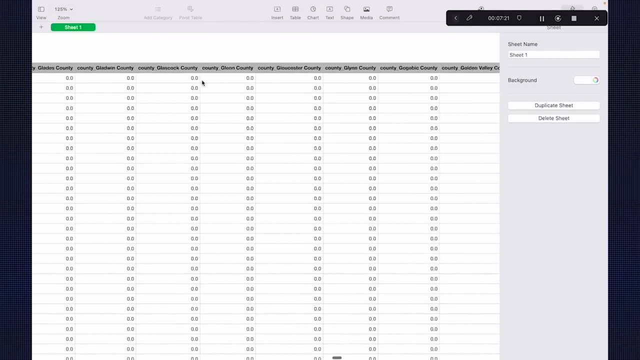 not present. but if you see now, this is that there are so many unit values, that's why there's so many counties are created, though so many variables are created, and that's the downfall of it. that's a downfall, but we cannot do anything. that's what the one hot encoding says. then you have state: 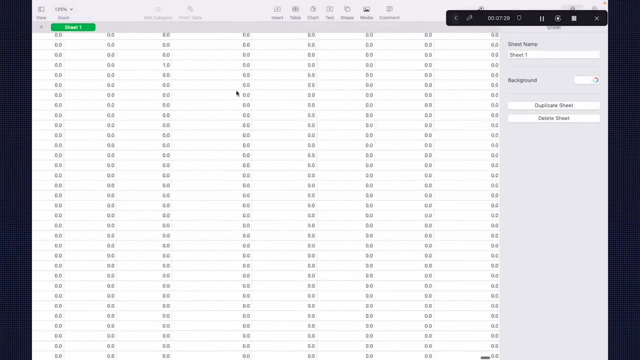 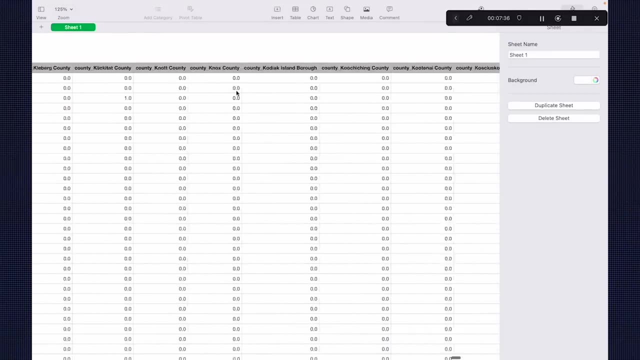 then you have, you know, a state, i think it. it it does not full, but you have a state and for state as well, for state Washington states, Los Angeles and etc. it is showing off as well. and then you see that it is. it is mostly, you see, by zero, but at some point you will see that there's one as well. 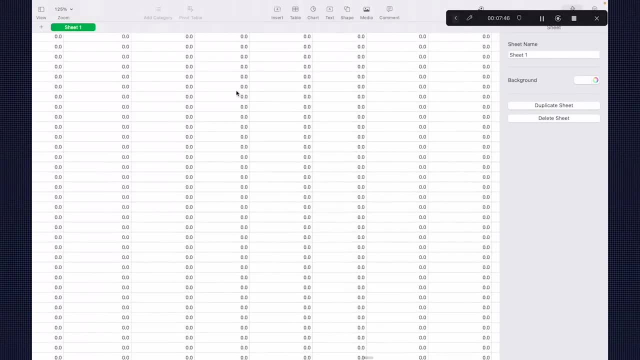 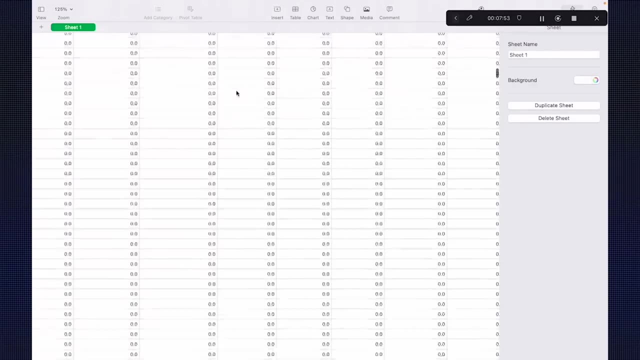 there's this one as well, where it indicates that that particular County is present in that that particular variable. okay, I hope that makes sense. I don't want to repeat it once again. so this is how it got converted. this is a very huge data set which is being formed, that there's a 1935 columns and only few rows. 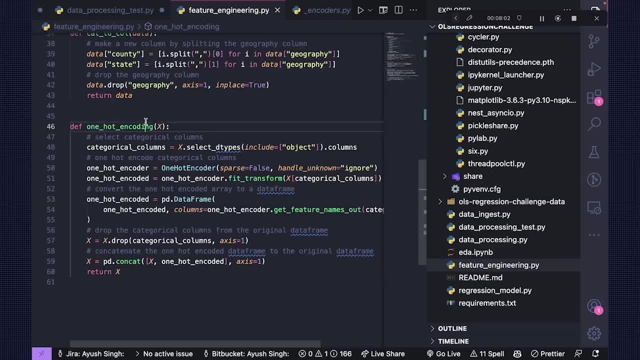 right, but we'll deal with that. so this is how one of 100 coding is where you convert our numeric to. there's one hot encoding, but but we'll take a look at other encoders. like you know, there are other in encoders as well where we'll 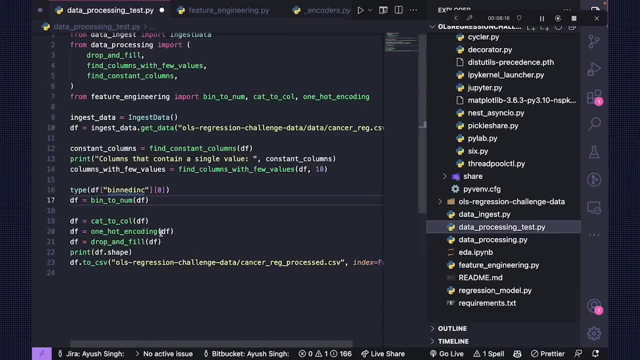 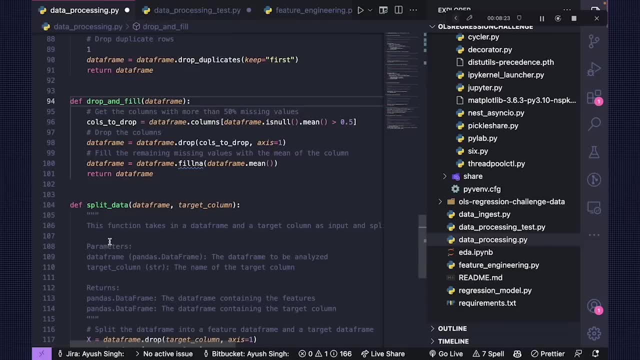 take a look at that and then now what you can do, you can simply say that one hot encoding and then you simply encode the variables. now you have that. now you have also seen, now you have converted the to the numeric. now you what you want to do, you want to, you want to fill out the. 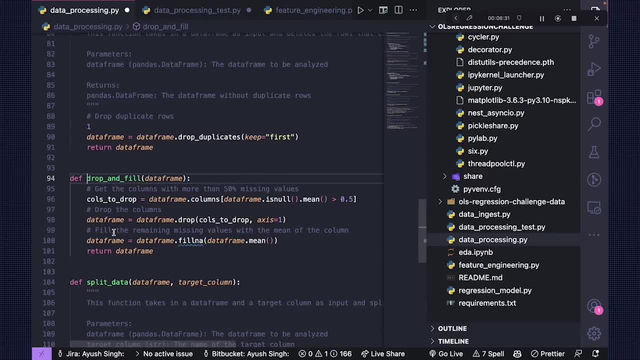 missing values, so missing values in the data set. however, we'll be having another section of dealing with missing values, but currently, what I'm explaining, you see, first is, first of all, we take take the columns which in which we need to drop right. so here's my plan: what I'm going to do if the missing values exceeds 50%. 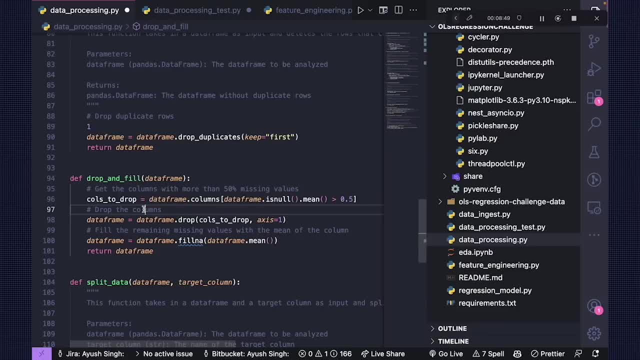 of the whole data. then we say that remove that particular column, right, but if that is below 50%, we'll say that let's deal with it with our techniques which we have. so the first of all calls to drop first the variable contains the call columns which we have to drop. so we select the columns from the data. 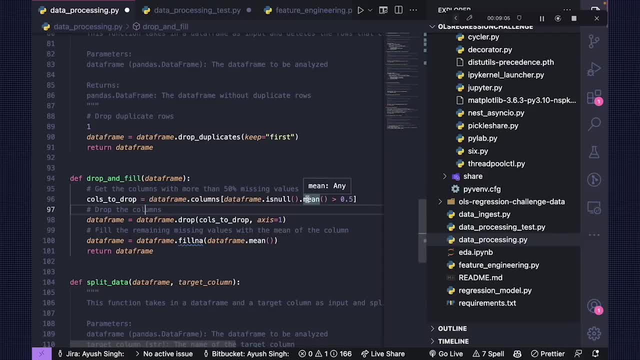 frame where our null values and where the null values, the mean of that null value, that in that particular column the mean is greater than 0.5. if that percentage is greater than 0.5, then we simply drop. if that, for the particular columns with that particular column in the data frame is: if the null null. 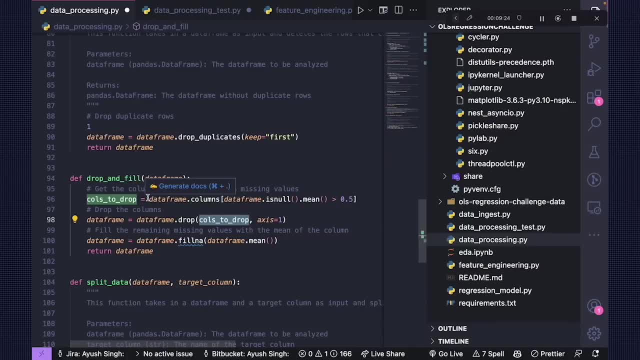 values in that particular column is greater than 50%, we say that drop it, which is drop, x is equals to 1, because it is a column. if this was a row then we would have written x is equals to 0. then if the values which are is smaller than 0.5, the missing values are less than 50%. 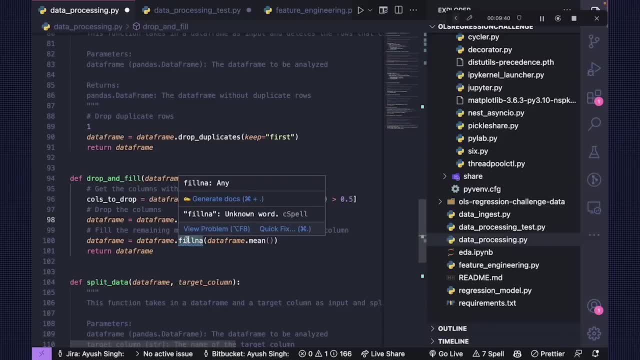 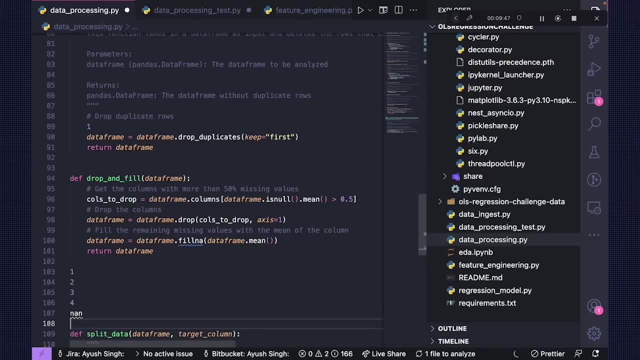 50%. then we say that fill the missing values with that mean of the particular column. so for example, you have one, two, three, four, nan, and then six, seven. so now you have only one value. so you fill this by the mean of all the values in that. 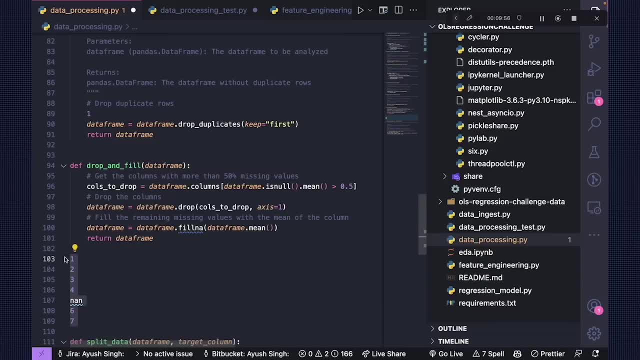 particular column, right? you have other methods too simple: imputer, canonimputer. there are several other techniques for imputing missing values, which is a whole set of interview questions, but we'll deal with that in the next section. uh, like, we'll study in detail, right, so we don't have to worry about that now. this is something which is dealing with missing. 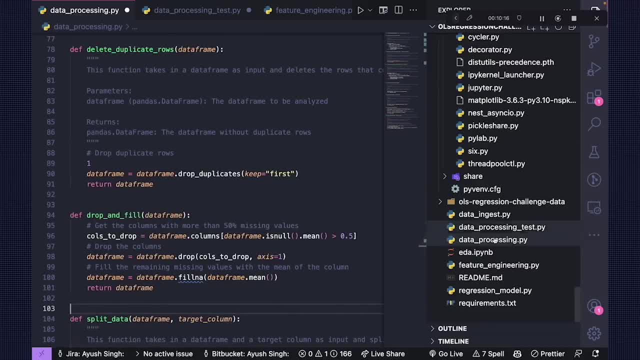 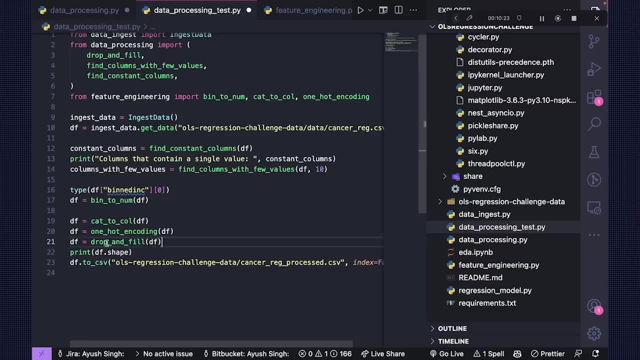 values now. now i hope that now you know what you can do. you can simply use this uh in one hot encoding, drop and fill and then print out the shape and then you can simply convert that. now we have the process data, where what we did- we first ingested data, we found basic values which 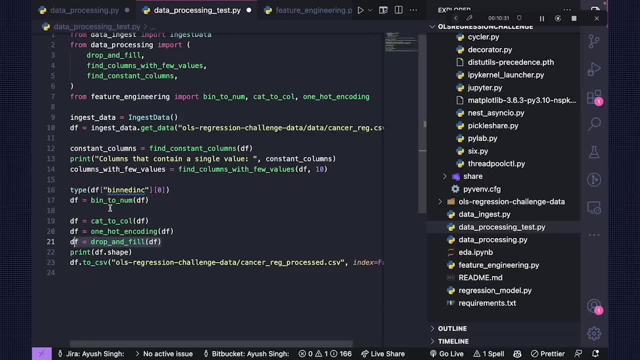 is converted that intervals to bins, categorical, categorical some, some some call it splitted- the feature reconstruction, feature splitting, feature engineering of converting categorical variables into numeric, and then we simply dropped and filled the missing values. now we have the perfect data to do the analysis on it, to do the analysis on it, where now we'll deal with something known as. 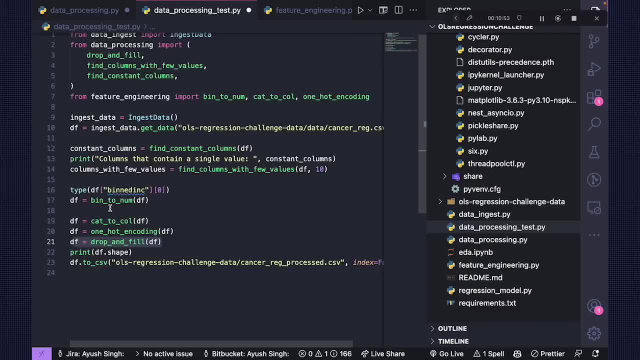 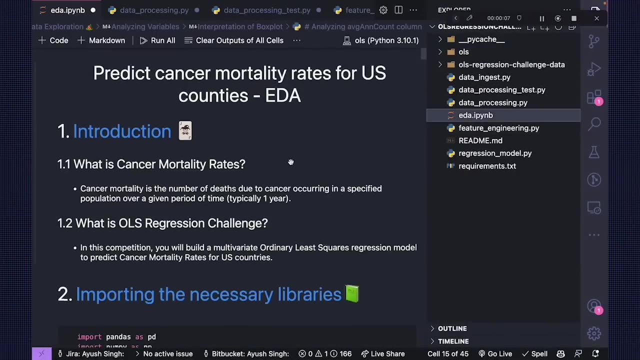 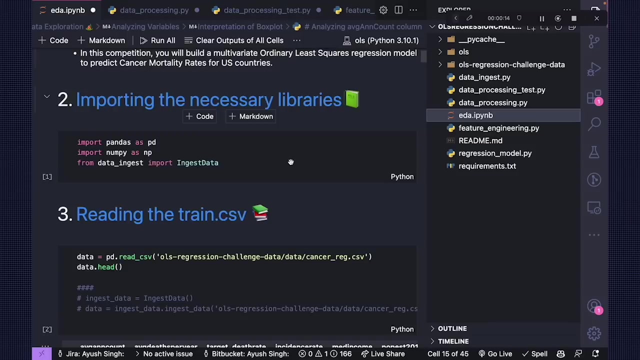 outliers. so, uh, that something is the whole set of discussion for the next set of videos, so let's catch up in the next video. so now, what we'll do now. we have done with the preparation of a data set. now, once we are done with the preparation of the data set, now we'll go and explore some of the most amazing things. 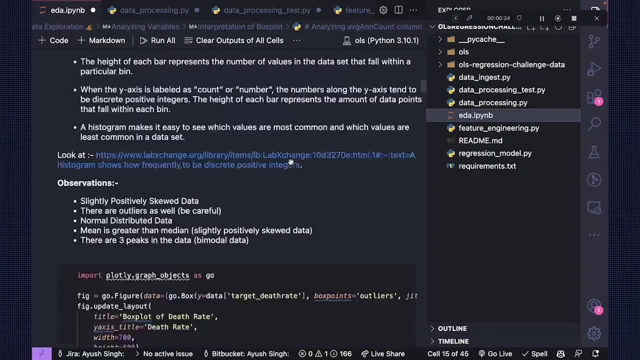 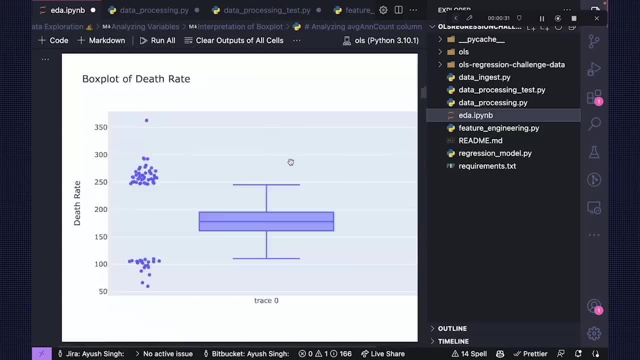 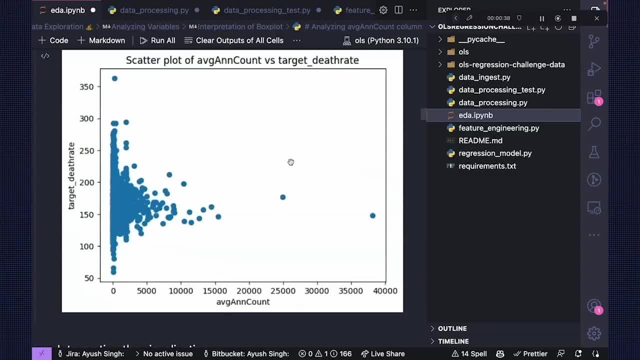 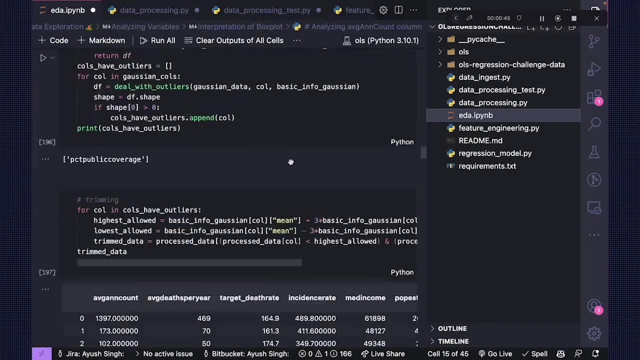 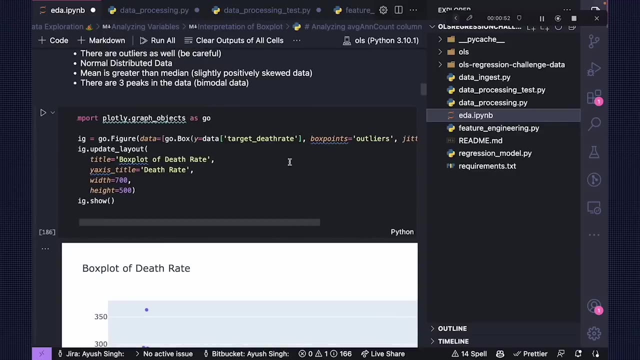 out here, right? so, um, in outliers we have seen a very nice explanation of the outliers, but we'll talk about some of the methods for dealing with outliers and i think this will be a very long video, uh, so bear bear with me up, right. so first is what we're doing. we're taking out the box plot. 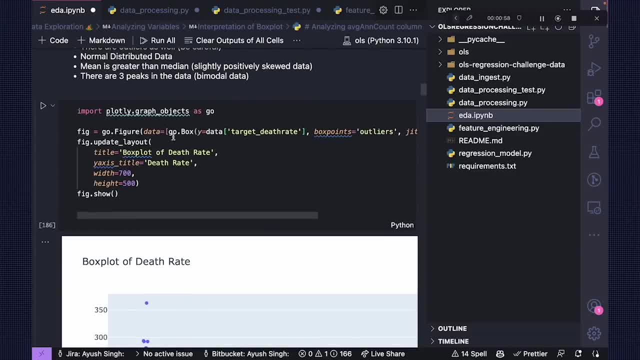 of our target that rate, where we say that we- i'm using plotly, so i'm using plotly- where we say that we're going to create a figure. in that figure we're on y-axis, we should have the target death rate and then it should have point pose jitter. 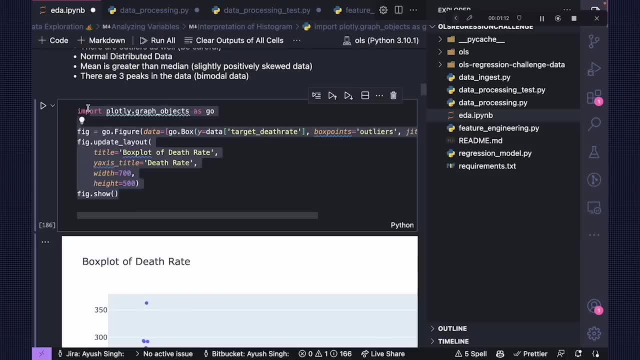 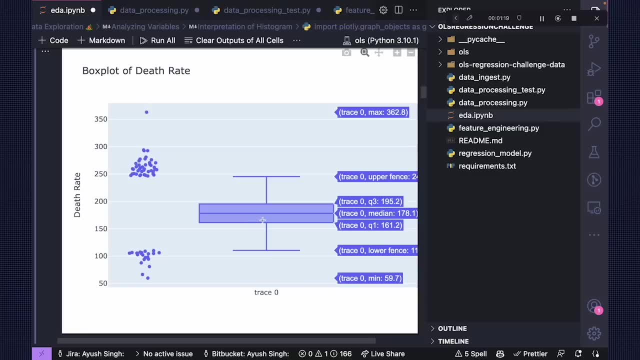 box points to be outliers etc. so this is a i'm using plotly to plot my box plots. so out here, out here you can see my first quartile, my first quartile, which is um 161.2, and then my second quartile is 178 and my third quartile is 178 and my third quartile is 178 and my third quartile is: 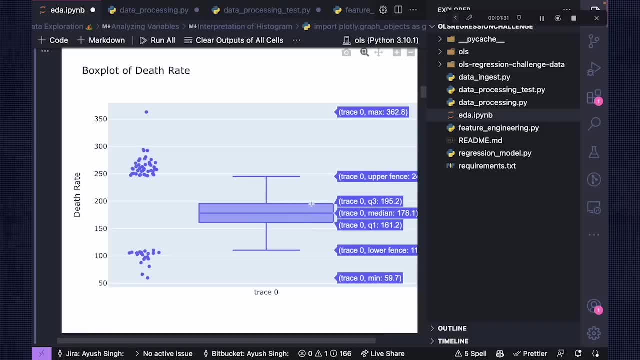 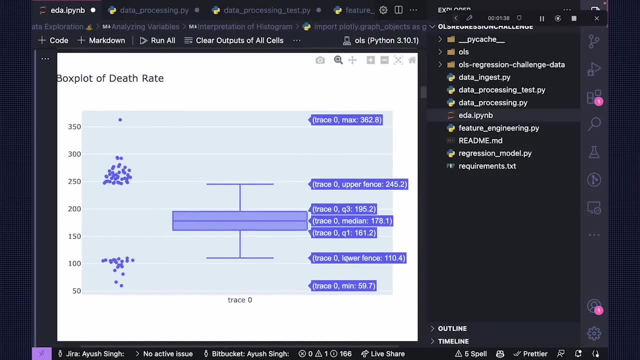 194, right, and then you have something upper fence. up upper fence is something which is your maximum, and there you have lower fence, which is this much so whatever goes above this are are said to be an outlier, and whatever goes beyond this, whatever goes um below the minimum, are said to be outliers. 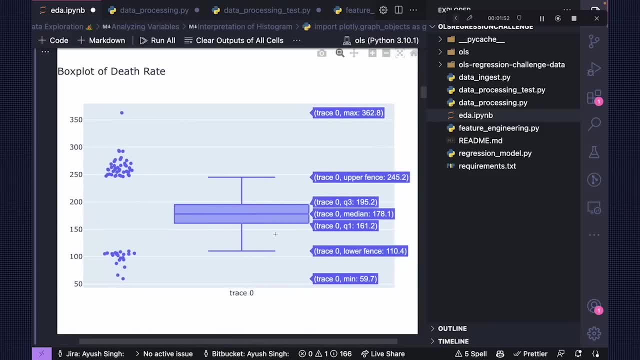 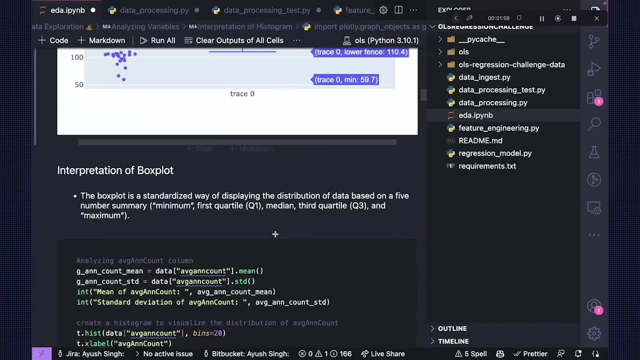 but this is this is what we have learned, right? but this is something that you will take a look at later on, but as of now, let's go ahead and let's talk about: uh, let's analyze, rather than this, target column right, let's analyze other the columns as well, rather than that. so, first of all, 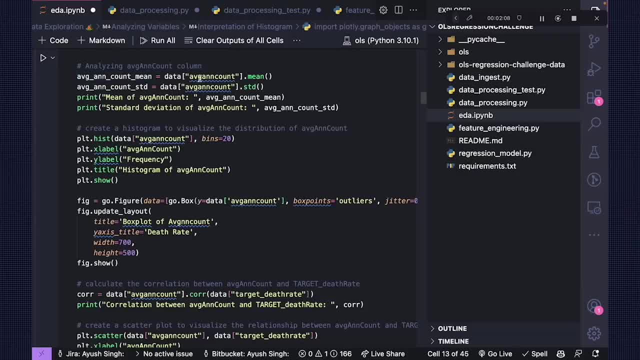 what i'll do. what i'll do is we have a column known as average ann count, right. so this is a column in our data set. now we're what we're doing: and taking the mean of that column and then taking the standard deviation of that column right and then we're creating a disc histogram to visualize. 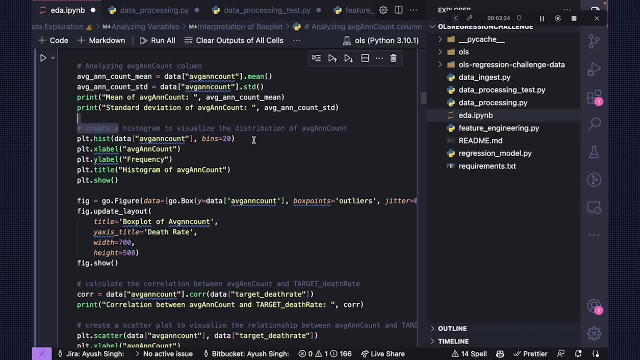 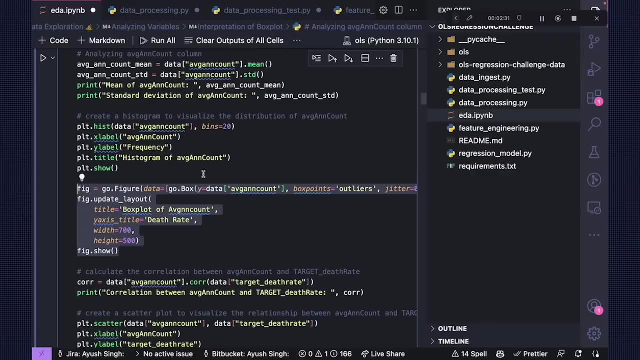 what is the distribution of that average ann? and then we plotting the box, plot using uh, plotly. so uh, for line by line, i i'll be giving you resources for learning plotly. okay, so i suggest you to first of all learn plotly, because that's very pretty much easy, so you can first of all, 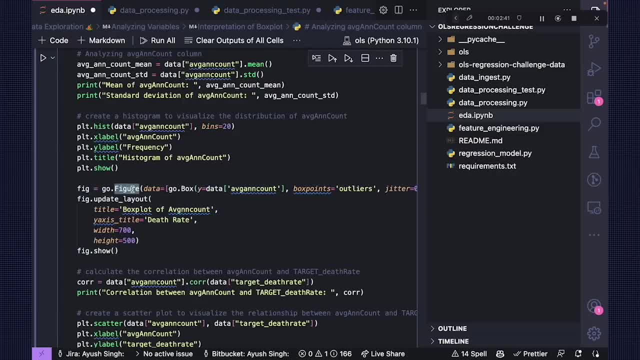 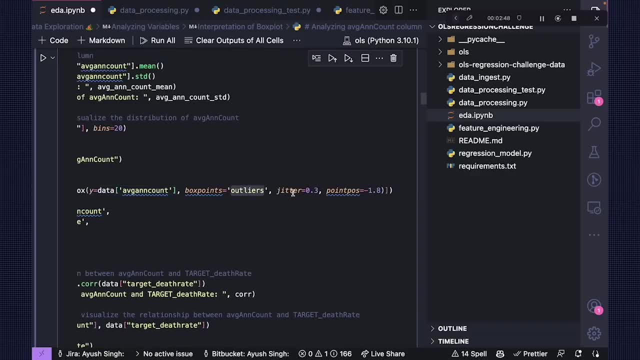 i suggest you learn plotly where you're saying: create a figure for that data and then that data i'm going to, we're going to have the box plot of this particular column and the it should be outliers. zeta is equal to 0.3 and point post is equal to 1.8. however, you don't need to remember. 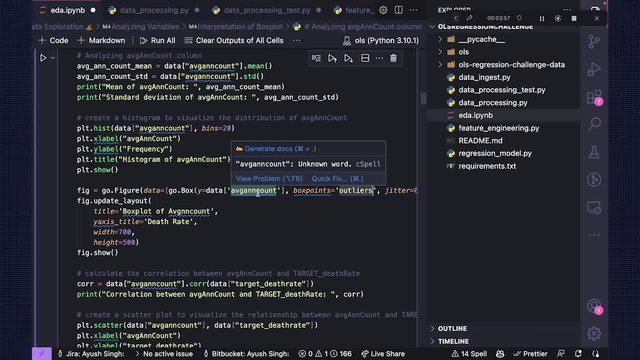 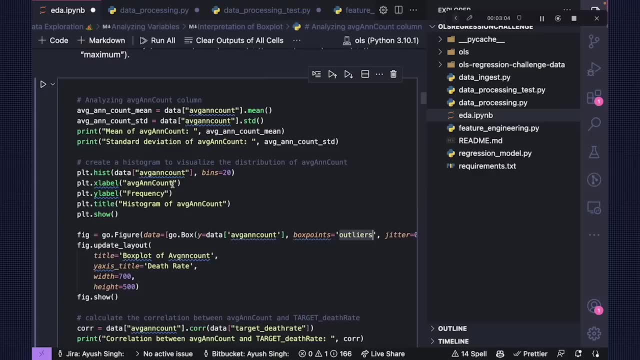 all of this what i usually do: i just copy and paste things. so even i, even sometimes i forget a lot of parameters, so it's so going to be eventually so what i'm doing right now. i'm taking out the now. i'm going each now why i'm doing this. first of all, let's understand why i'm. 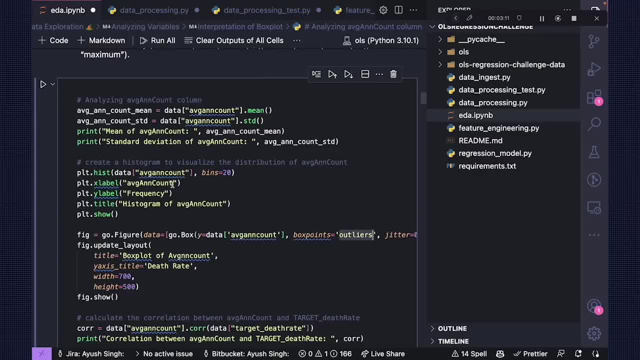 doing this, the reason why i'm doing this: i want to identify outliers in my columns. so, just for explanation sake of thing, i'm giving the tools how i go about learning more about how my individual variable looks like, how my, how this average ann. columns are is. what is the distribution? what is? 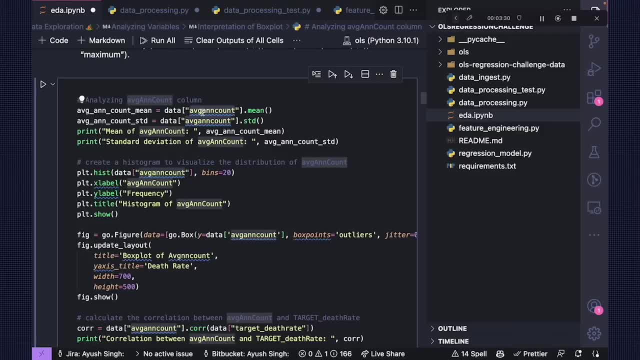 the mean? what is the standard deviation? what is the standard deviation? what is the standard deviation? what is the? what is the correlation coefficient? correlation with my target variable. what is the number of outliers present, etc. etc. etc. so, in this um, this is a step which i follow. 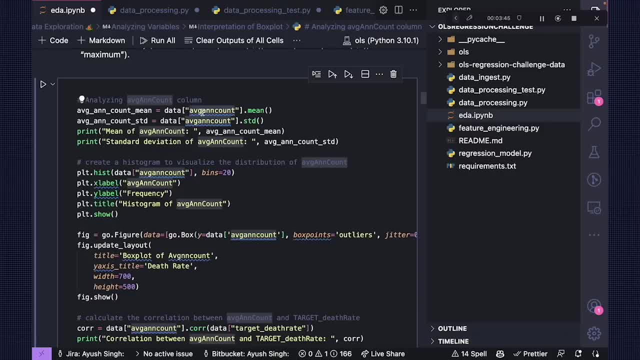 the framework which i follow is the reason why we are doing this. we need to summarize this instead. summarize this column: average, ann, count statistically. so whatever you're seeing in front of me, we we have. we are printing the mean of that particular column and then you're plotting the 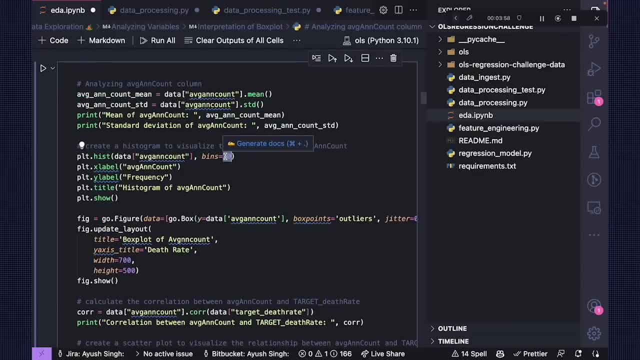 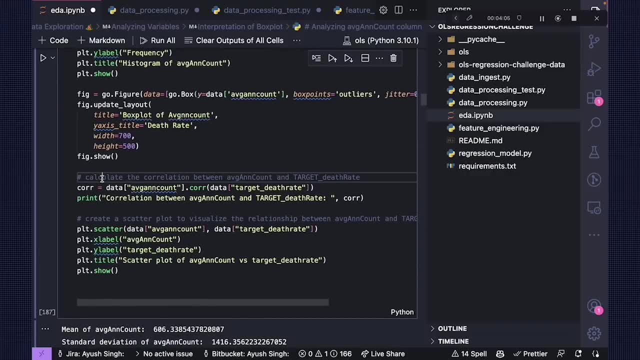 histogram bits is equals to 20, which you have seen the way i'm doing it- and then you're plotting the in interpretation of the histogram. then over here, we cal, and then you simply box plot it, and then over here, you calculate the correlation between the average ann count and target death rate, which 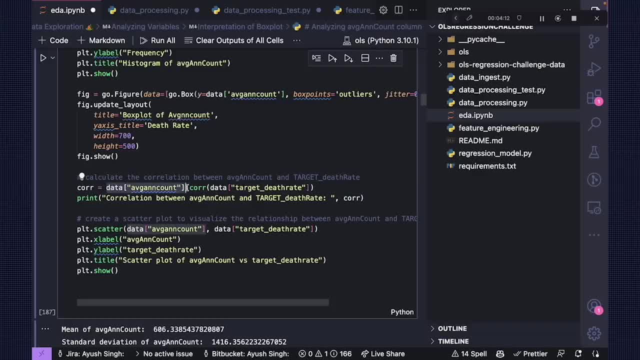 is. we are seeing correlation is equals to this particular column. this is assume that this is a vector dot correlation with whom target death rate? right? so we need to identify what is the? what is this direction, this strength between your average ann count and the number of death rates in that? 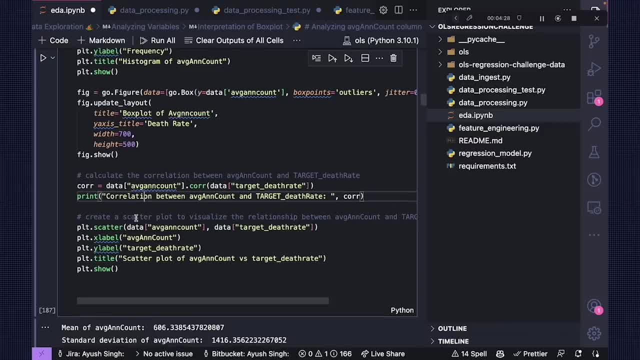 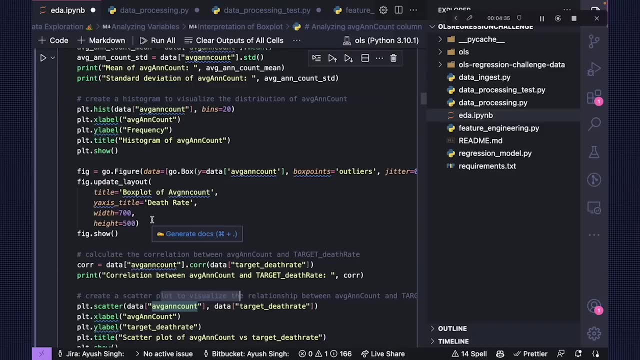 particular country, so the correlation it will be given by this, and then you create a scatter plot to visualize the relationship. so, uh, here's what i. here's why i did first of all, i create, first of all, i did two basic statistical analysis of this numeric column mean standard deviation. i, i, i wanted to know the distribution. that's why i. 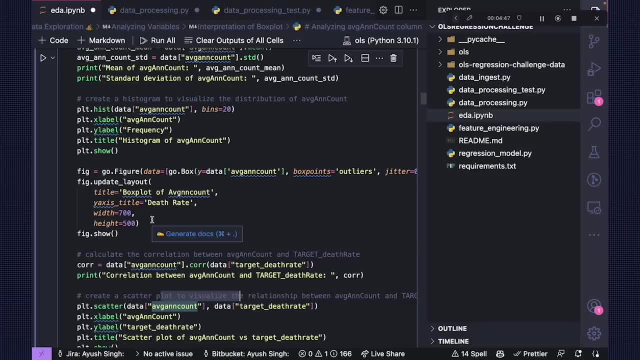 added a histogram. i want to know the outliers. that's why i added: you know box plot. i want to know the correlation between both of them. that's why i added this. now you may think we are going to do this for every column. if you wish to analyze any particular column, you should do this and then. 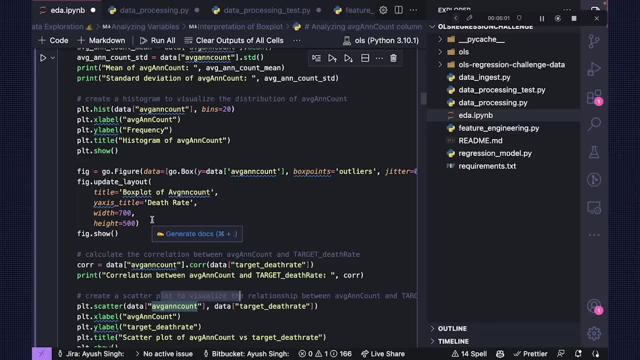 do it right. if you wish to analyze, if you wish to know more about the data, you should do all of this step for each and every numeric variables right. that will give you a better understanding about holistic understanding about data. so over here, and then you're plotting the scatter plot to 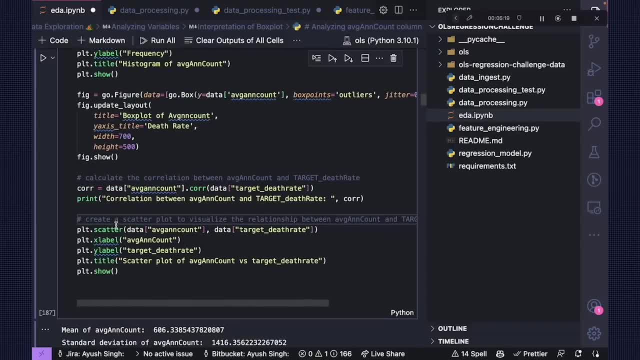 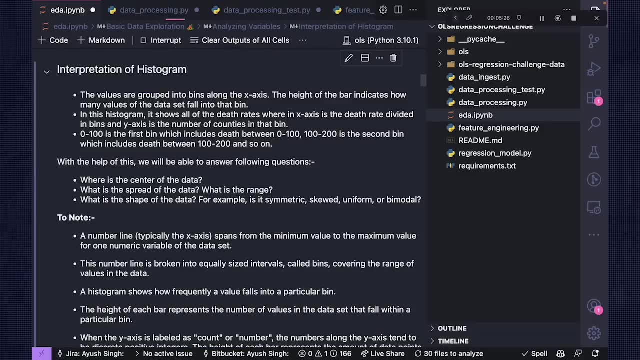 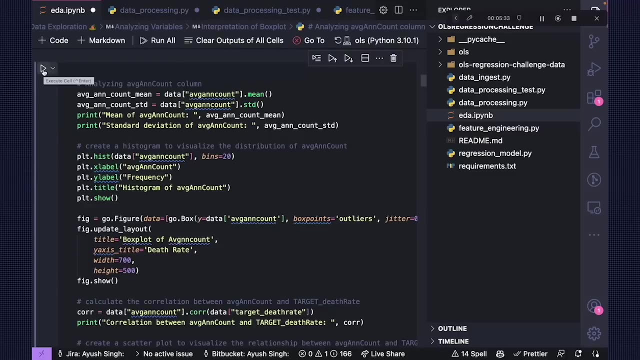 visualize the relationship between a of average ann count and target death rate. so let's first of all print this out from starting, then it will make more sense. so let me just run it eventually. so it will take some time to run it, so we'll just give it. give it some time to um run it. i think yes. 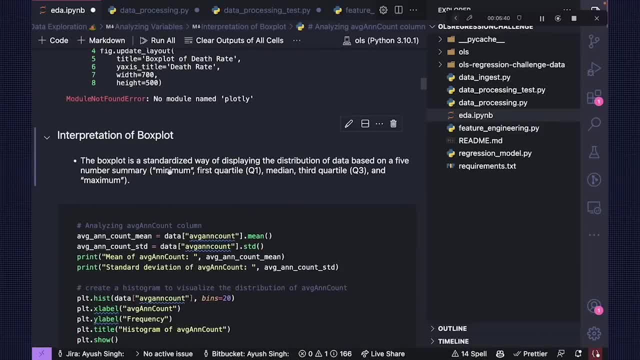 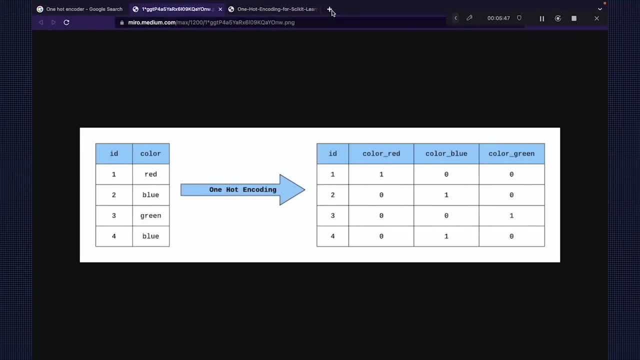 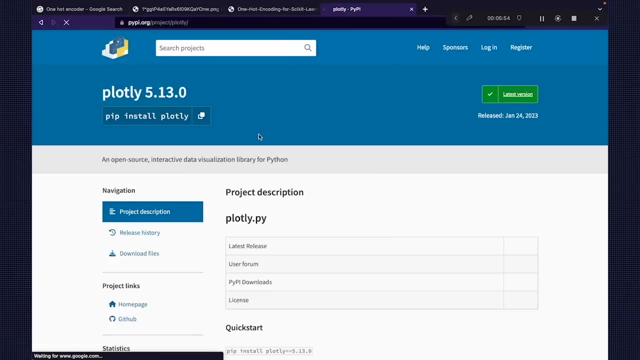 plotly: no module name plotly. so basically it is saying: the plotly is not installed. so let me quickly install plotly. so plotly install pip, and then i'll just install plotly by using pip. install plotly by making a plotly, and then i'll just install plotly by making a plotly, and then 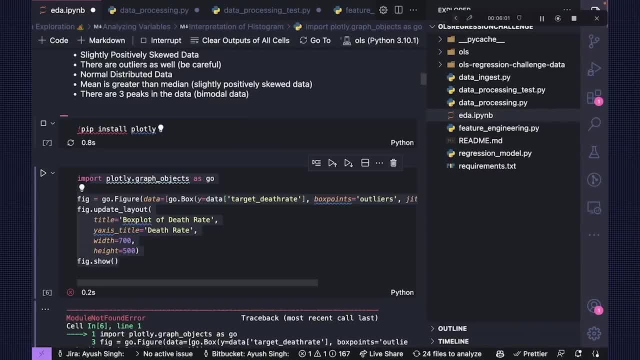 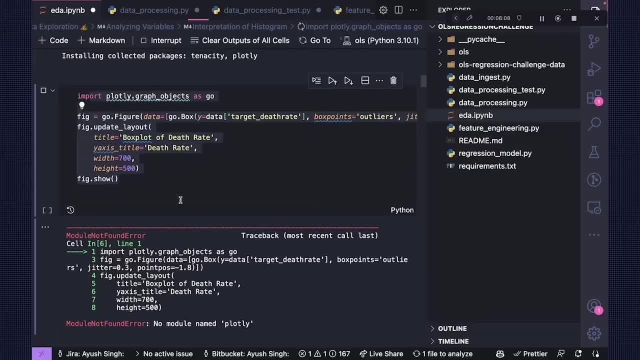 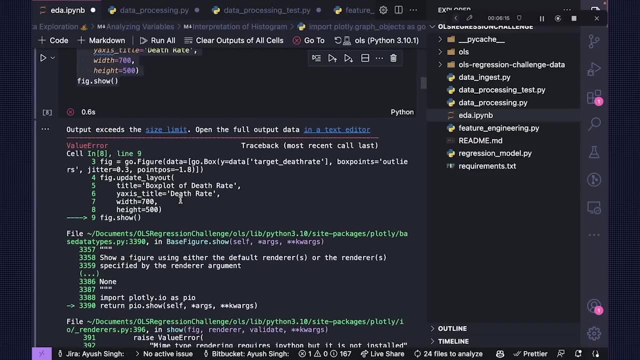 i'll just install plotly by making a nice pip: install plotly, let's wait a few seconds to get it. for getting it installed, i think it's get stalled. so once it gets stalled, we'll just run this. you should wait for some time. whoops, it is saying a minimum. uh min mine type of rendering. 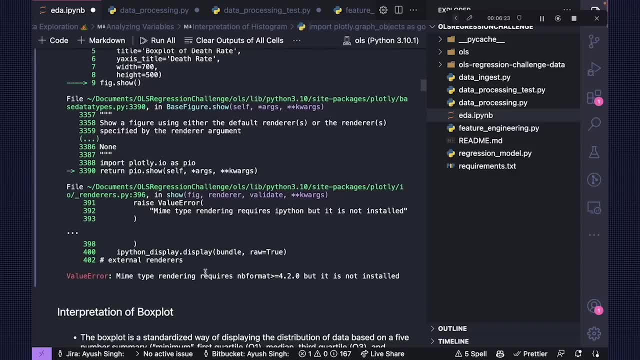 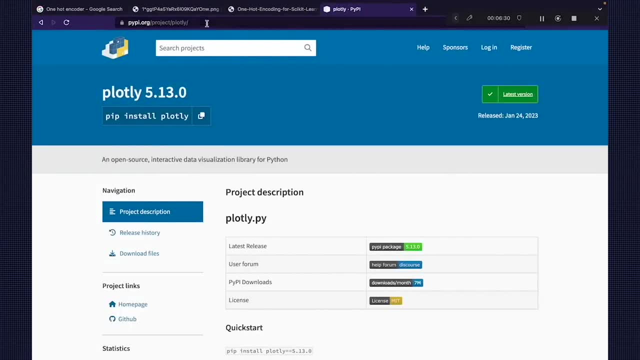 requires nb format 4.2, but it is not installed. interesting question, so let's go and search for it. so this is how it works. so let's go and search for it. so this is how it works. so let's go and you should search if you. i don't know the. currently i don't know the solution to this. 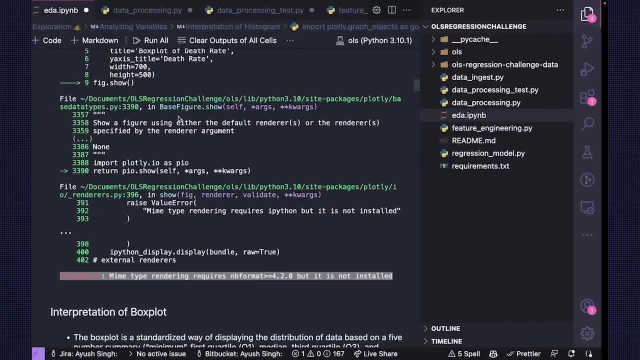 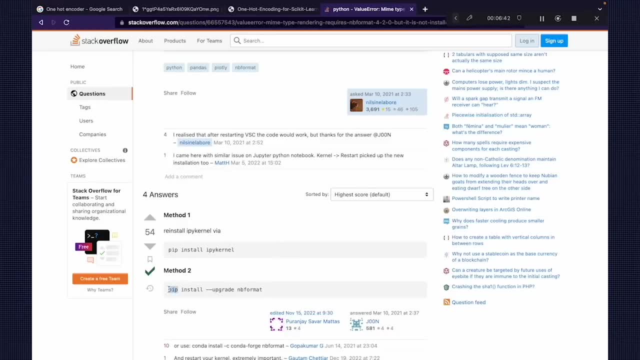 problem. okay, now let's try to debug it. so just saying that there's something to do with this format. right, there's something to do do with this format. i think that you have to update your kernel. you have to upgrade your kernel. you have to upgrade your jupyter notebook. that's why it was. 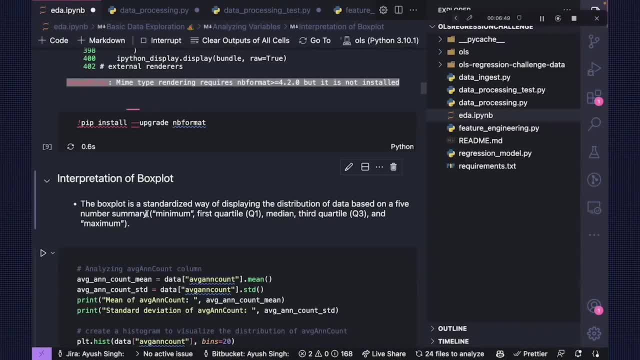 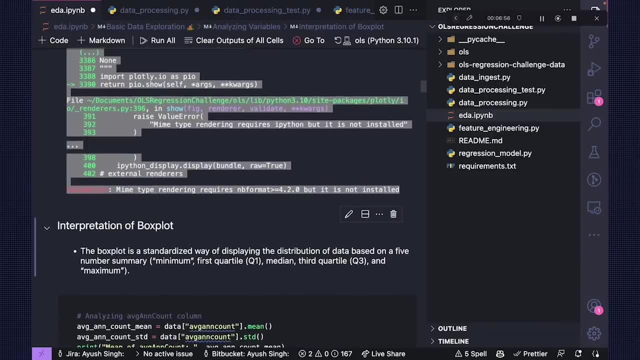 saying you can simply go and then simply run it, and then you will see that it will work completely fine. then you see that it will look completely fine. so let me run this out, and then you see that, and then you first of all restart the kernel. so you have to also restart the kernel, to be honest. 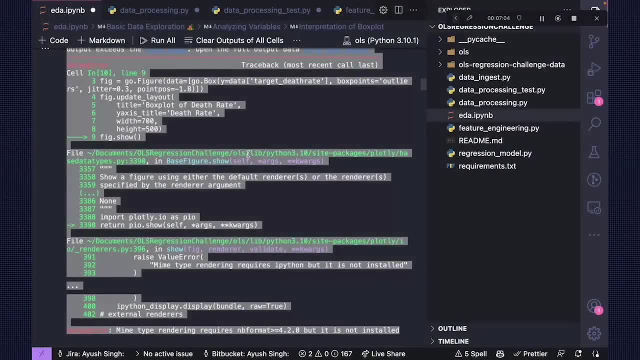 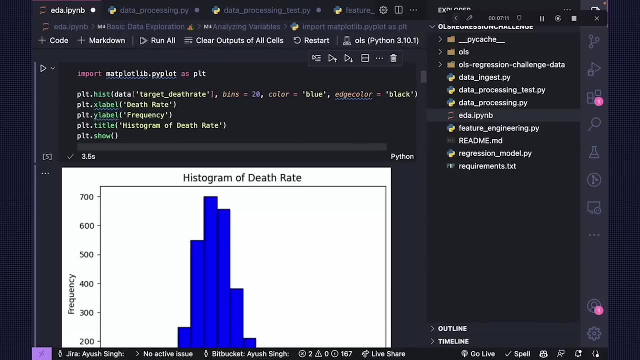 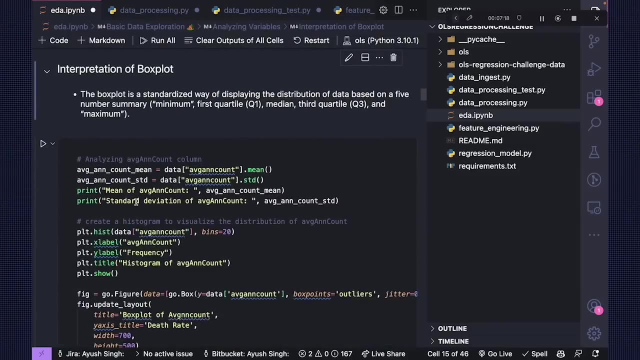 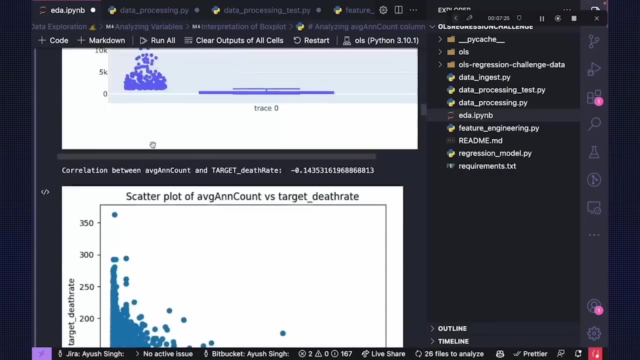 restart, because once you install the libraries, you also have to restart so that it makes sense. yes, now we are, we are done with that. now, what we do, we simply have this: um, so let me just first of all run, run it out: so it says that, what it says. it says that for a 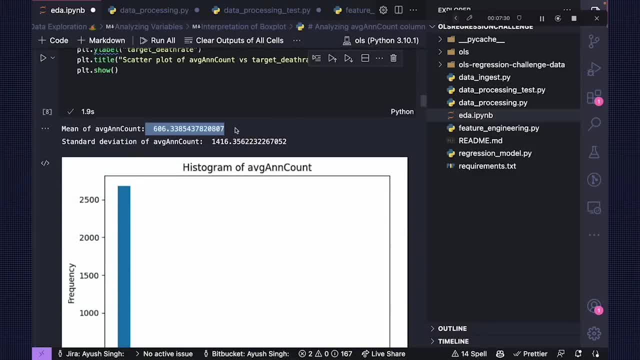 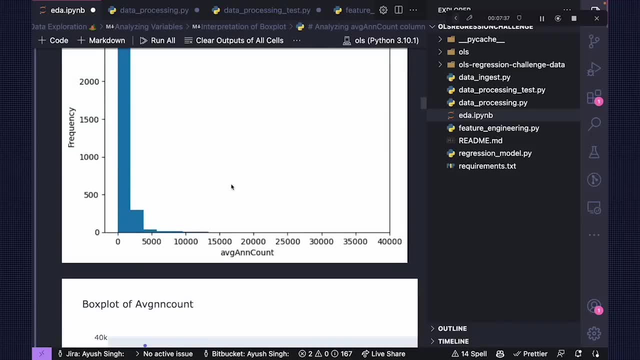 particular average ann kernel. it says that for a particular average ann kernel. it says that for a particular average account you have mean of average count standard deviation histogram. you see, it is a positively skewed. it's not normal. it's a positively skewed data set where most of your data lies between your 0 to 5000, where there are some outliers also present. 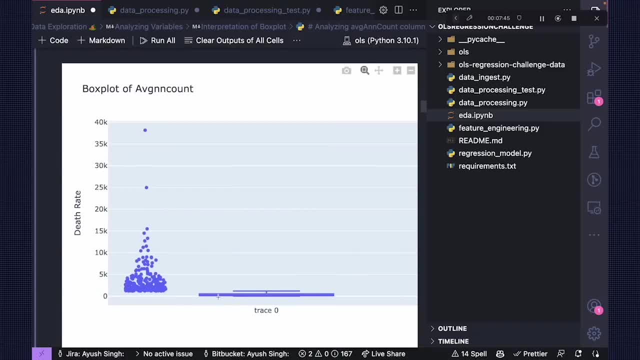 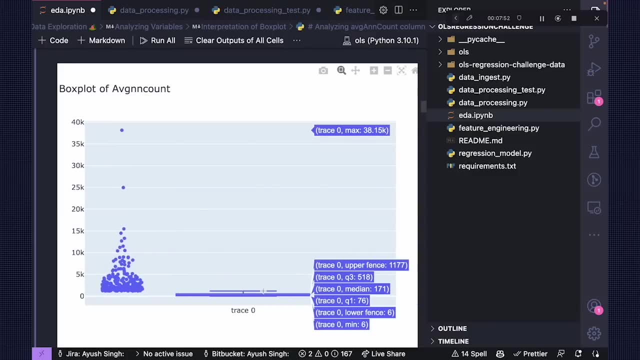 you can see that there are a lot of outliers present. you see that that this is your upper upper fence, it's your lower fence and in this upper fence you have, 117 is the upper fence. so values above this are outliers and whatever values below the six are outliers. but you see that most. 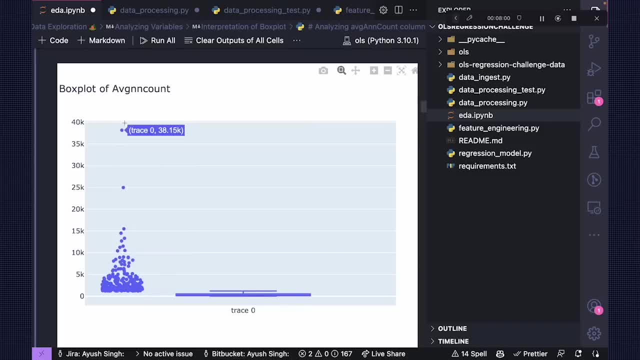 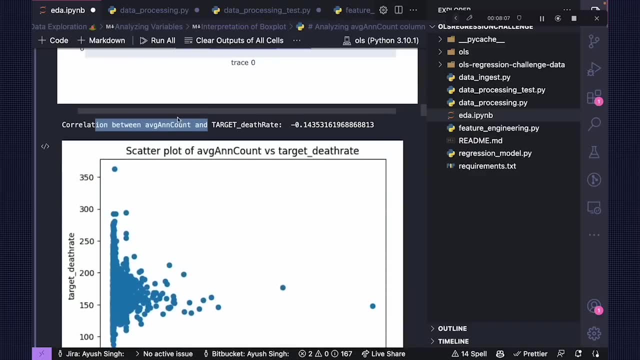 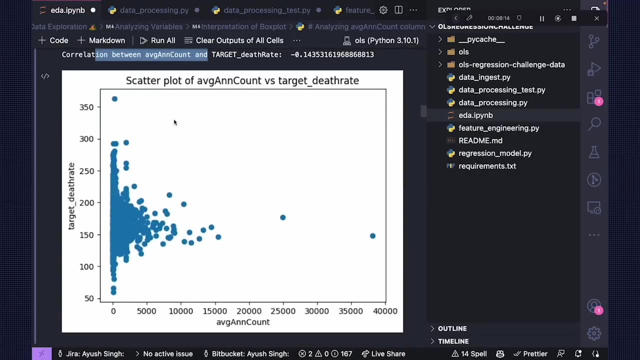 of the values lies between: uh, you see, these are the values which are omg, these are outliers. and then correlation between the target is negative correlation, where one increases then other degrees. so it is saying that, um, yeah, the the negative correlation, what it is, one increases and other decreases, right, right. so, as 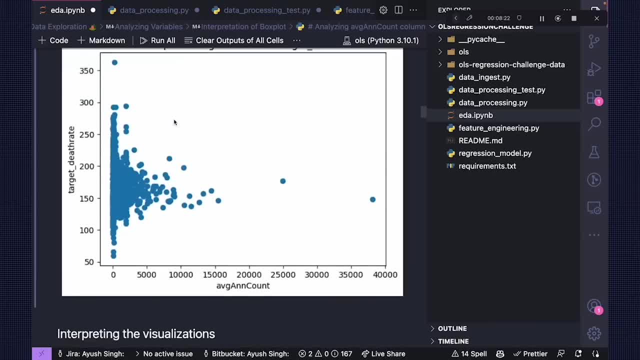 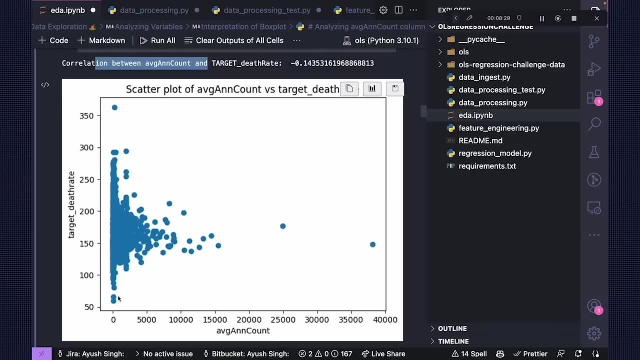 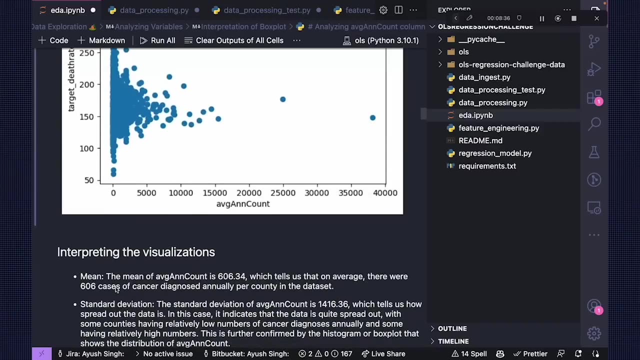 assume that. um so now you see over here, now we feel now this is scatter plot, where on on x axis we have average in and count of y axis we have a target death rate. you see that there is some sort of giving a very nice stuff. but you see over here that uh, but, but let's, let's, let's interpret it so. 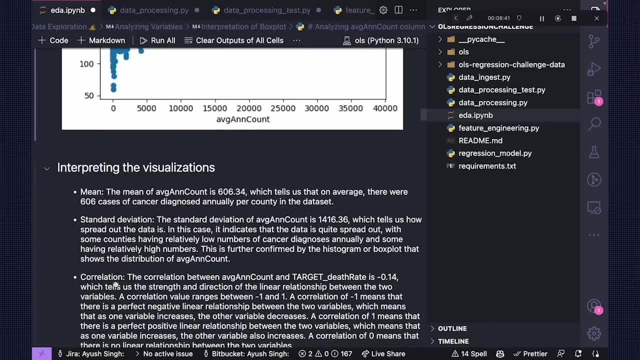 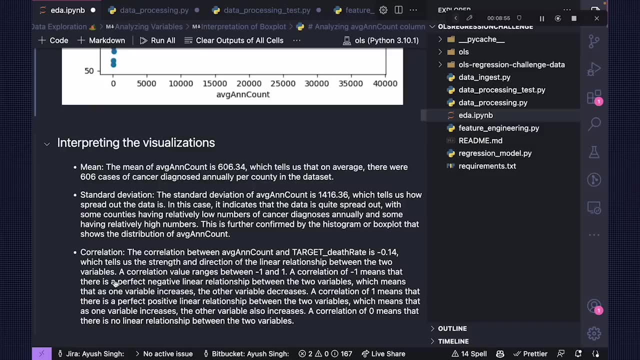 it is saying the mean of average in and count is 606, which tells us on an average there were 606 cases of cancer diagnosed annually per county, right six and average. the standard deviation tells how spread out your data is. indicates you it is quite spread: 14 to 16 is quite spread, with counties having relatively low, low numbers of. 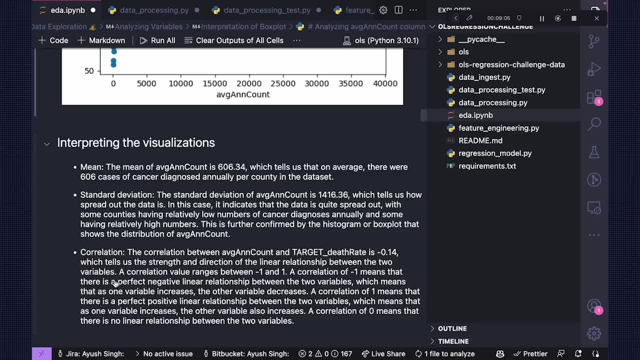 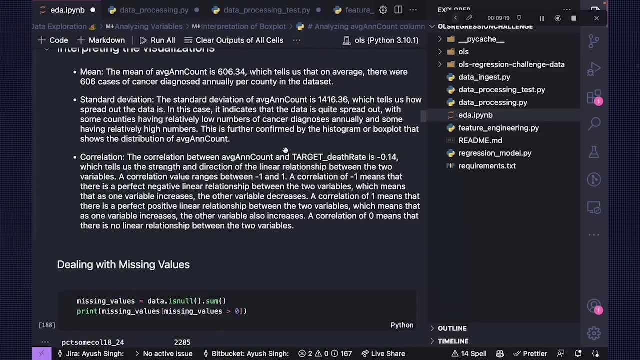 with count, some counties having a relatively low number of cancer diagnosis annually and some count is very relatively high. that's why the standard deviation is high, because the spread is high. in this case- and this is further confirming, which you can see that this further confirmed in your histogram or box plot, you see the correlation is minus 0.14, which tells us the 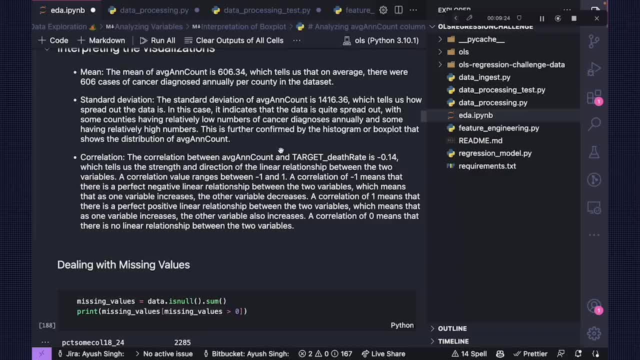 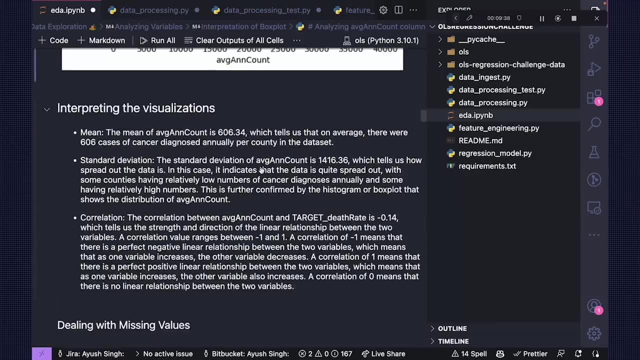 strength, and then strength of a linear relationship. correlation of negative. one indicates that the perfect linear relationship, which means that one increases than other variable decreases, a correlation of one means that there is a perfect positive relationship between both of them. right? so this is a very correlation about? uh, how can we interpret it? so if, in this case, if one? 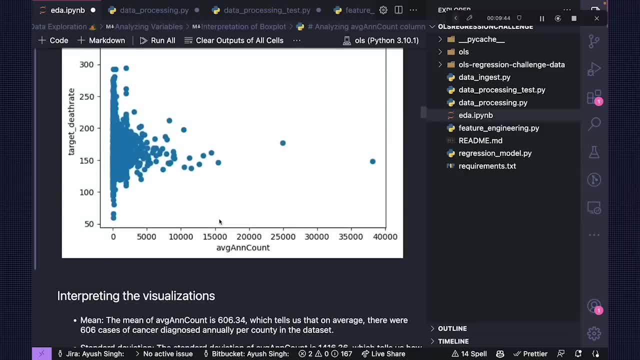 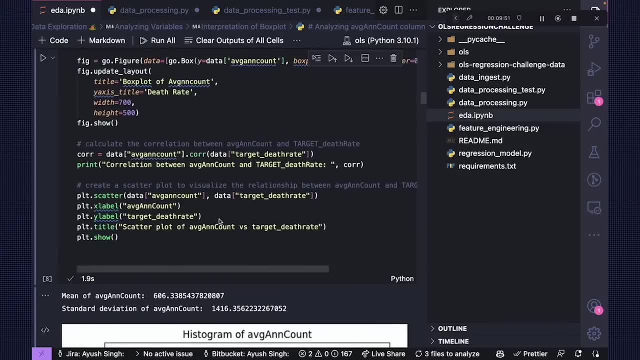 increases, then other other decreases, but it does not imply causation. please see my lectures initially on correlation does not imply causation, but only thing which i want to tell is to: this is how you can visualize or summarize your correlation, and then you can interpret it as a linear relationship. 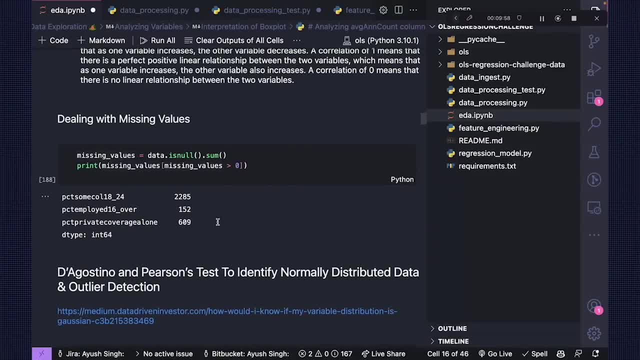 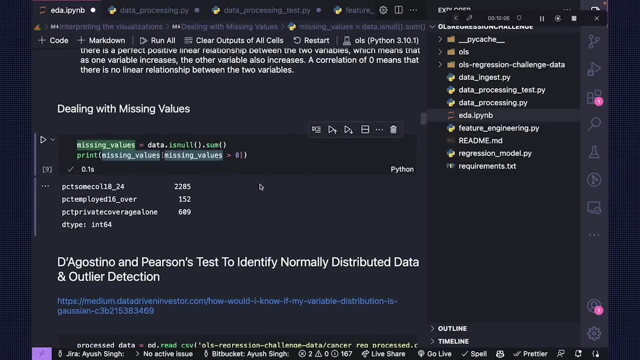 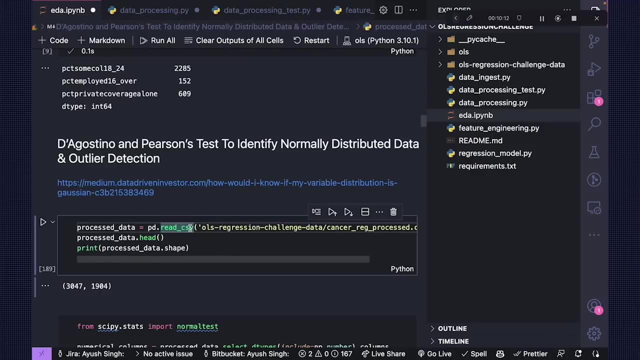 and then you can visualize your correlation and then you can interpret it as a linear relationship, particular variables. by dealing with all- all of the shirt sticks, you have several missing values as well. um, i think you have several, several missing values. however, we are going to import the process data to deal with anything, literally anything, right. 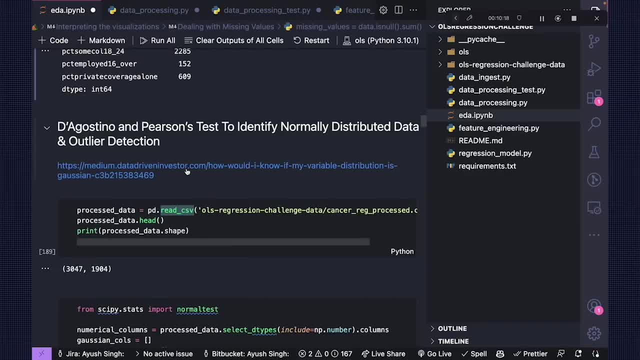 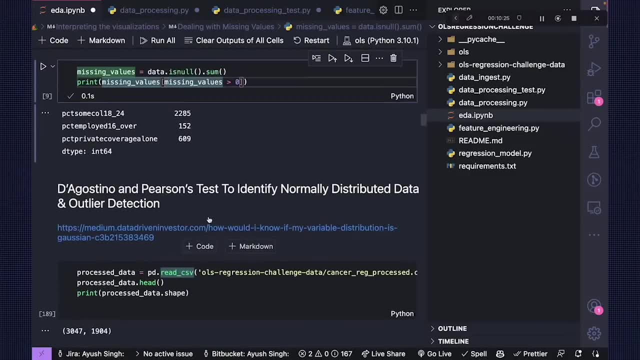 so you can actually ignore this as of now. so what you're going to do? we're going to import our process data, but now over here, but now over here, you will be a bit shocked to uh see the outlier detection. so let's try to learn about outlier detection in the next set of lectures. 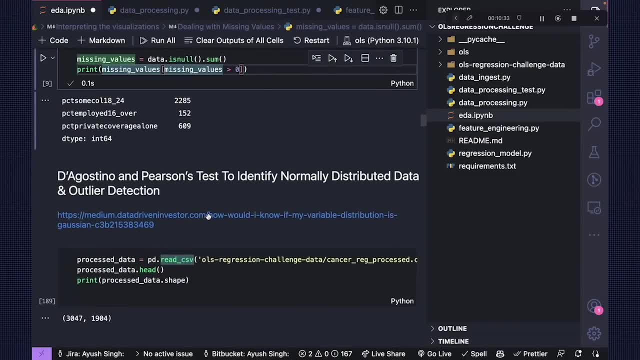 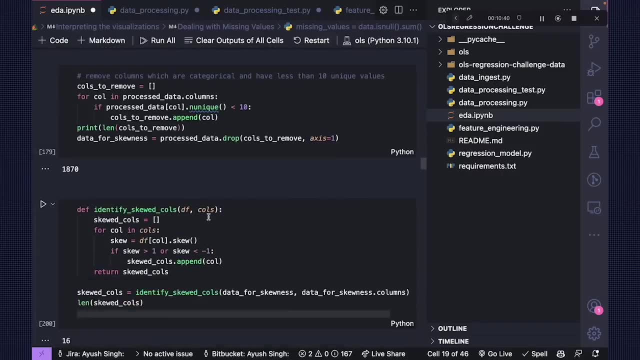 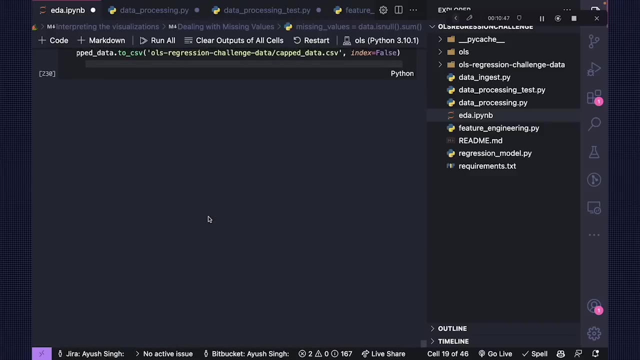 on how we can utilize, how we can utilize, how we can utilize several tests for outlier detection, how we can eventually utilize other things like um, like skew. how can we perform outlier detection, skewed data sets? how can we remove it right? how can we remove our uh outliers from the data set? 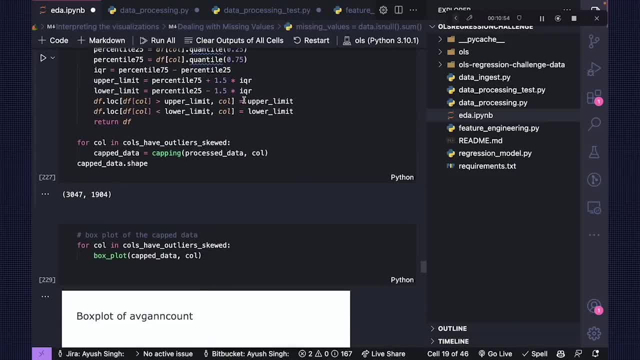 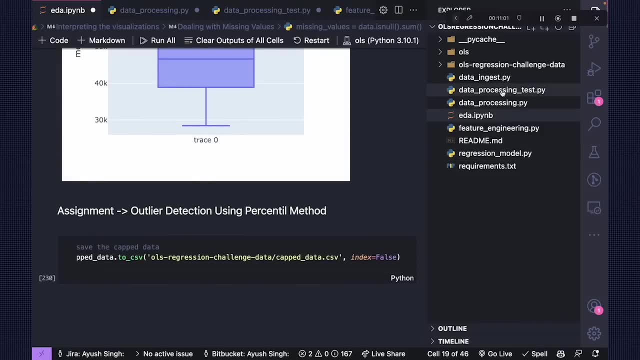 by and how can we use several trimming, capping, this with several of the techniques we can utilize for dealing with it. we'll deal with that and then, at the end, we will just save it and then we'll go to model building, which is super duper easy part in this, where we simply have our model to eventually. 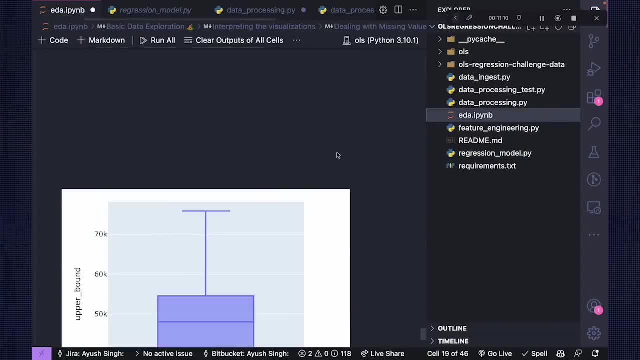 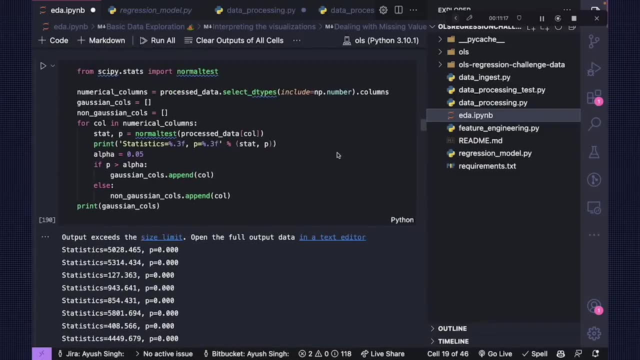 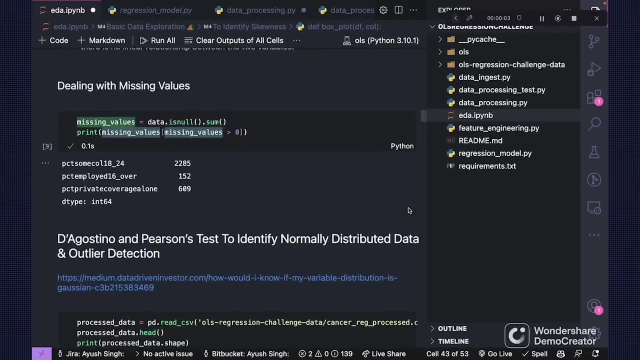 train a model, but the most important part of this project would be the outlier, dealing with outliers and working with data. so let's meet in the next lecture talking about things which you have not imagined till then. bye, bye. so, hey, everyone, what i'll do today is talk about 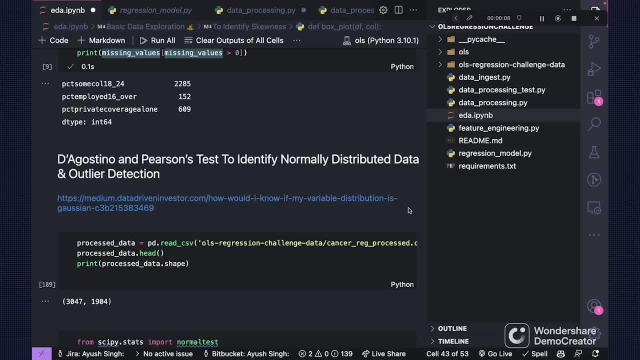 outlier detection, which is the most important, you know lecture till now which we, which which we're going to deal with today, is that the most important lecture and we'll try to achieve. talking about outlier detection using z-score method, we'll try to achieve outlier detection using iqr, you know, interquartile ranges. 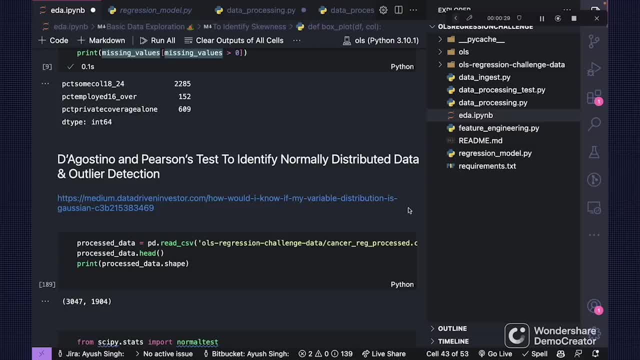 we'll also try several other techniques, like: and how can we how what is trimming, what is capping, etc. in these sort of lectures? so so let's get started actually with all of this. so whatever you're seeing in front of your screen is for normally distributed data, so um. so, first of all, 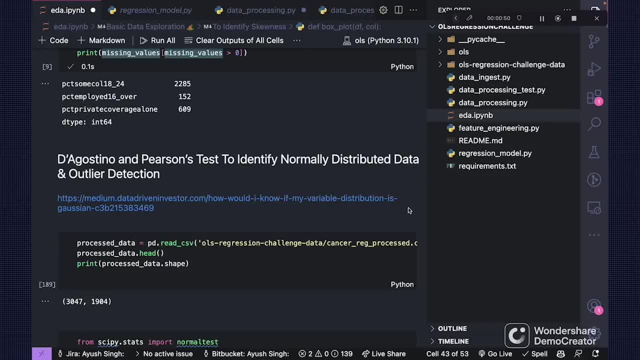 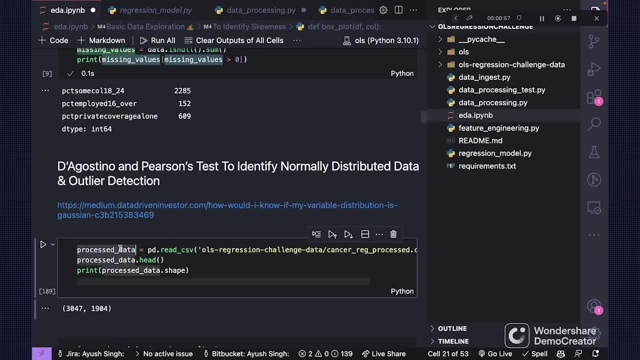 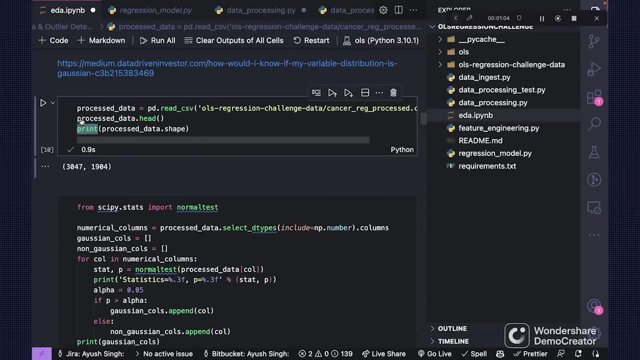 we'll try it off, try and try it, try it, try out outlier detection using outlier detection using um, z-score and over here, first of all, we import our process data, the one which we process very nicely, and then we take a look at the head of this and then we take a look at the tail of this. so let's try to print out our head, our head of the 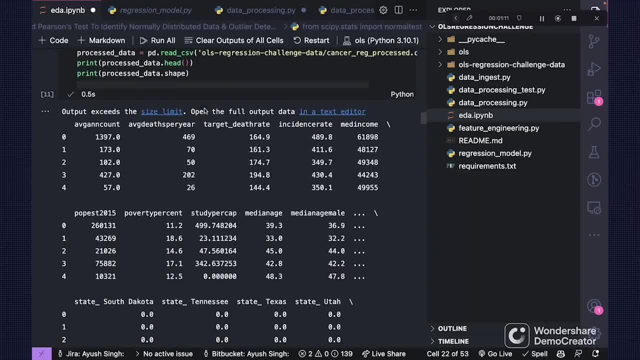 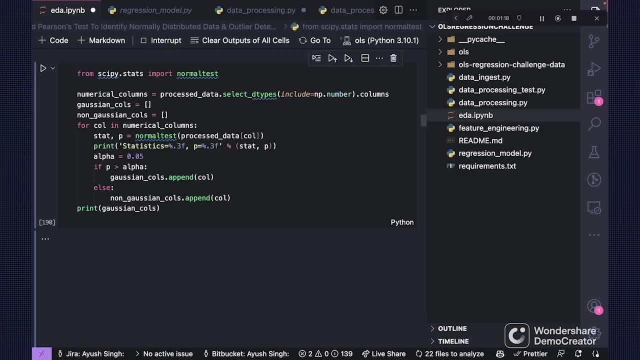 data and then let's first of all head of the data and we print out the head of the data. this is how it looks like, but i think which we want this to be in a form of, rather than printing, let's print out something like this: it should look like this: where you have five rows, nine out of four columns, right. 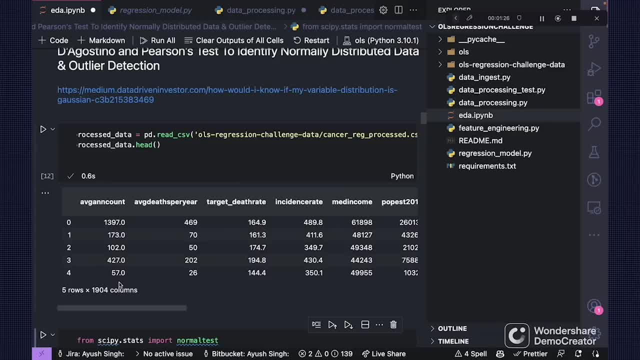 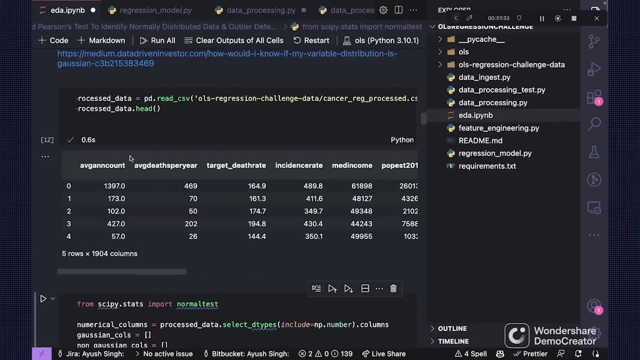 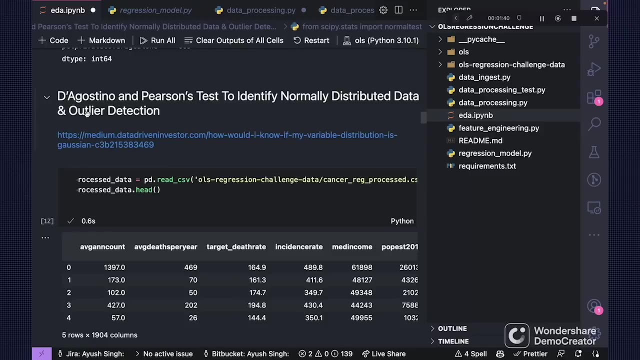 because why? why this is nine of four columns? because every value of that categorical values has become a new categorical column. now now, now for z score we are going to use out. we are going to use z scores. we have studied these scores in our probability lectures, so please go there and 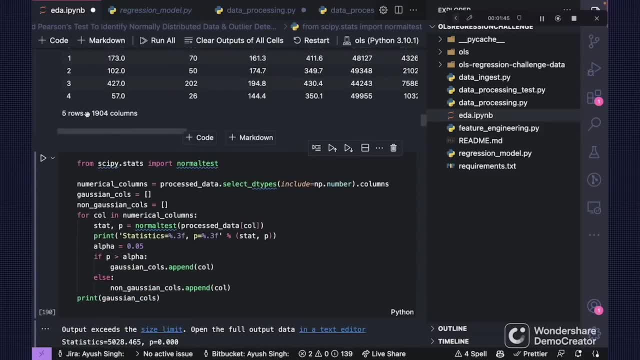 review it back. um, so we also z scores. are you and we are going to use these code for outlier detection? right, we are going to use z score for for outlier detection. so, basically, so basically what. what we are saying over here is that, um, there's one condition for z. 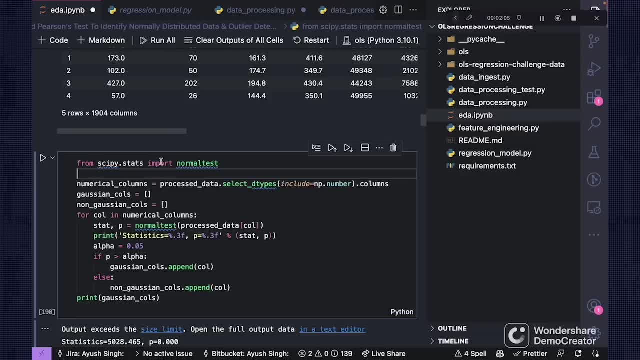 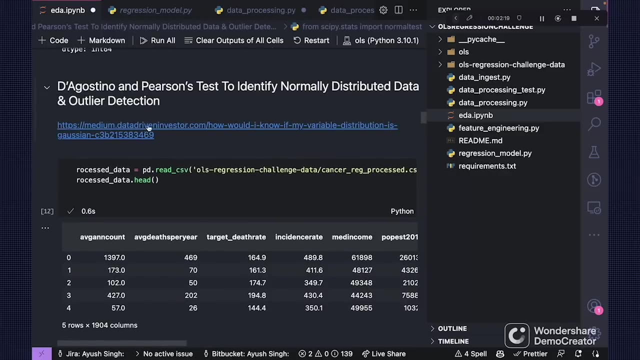 score that your particular column or data should be normally distributed. so we are not deal. so we first of all want to select the columns which are, okay, normally distributed. okay, it is not like hi fi and all. so you can go and see over here as well: how do i know if my distribution is, uh, gaussian, if 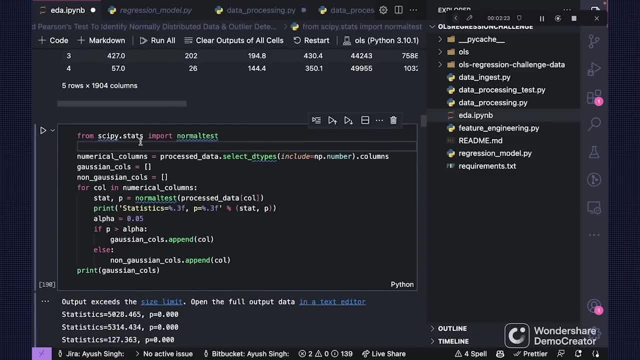 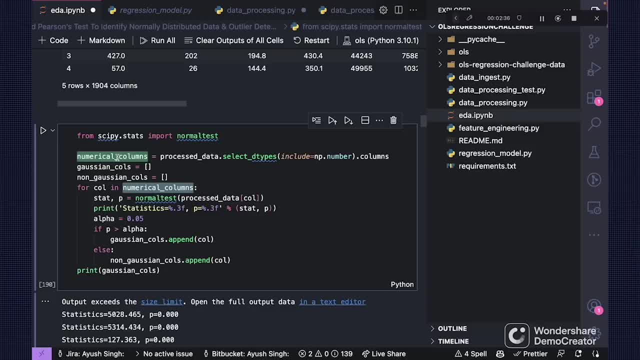 the numerical columns. you want to select the numerical columns, so only because we're going to deal with numerical columns, and then you have gaussian columns and non-gaussian columns. we make a 2 empty list and then you say for call in numerical columns, for calling numerical columns. 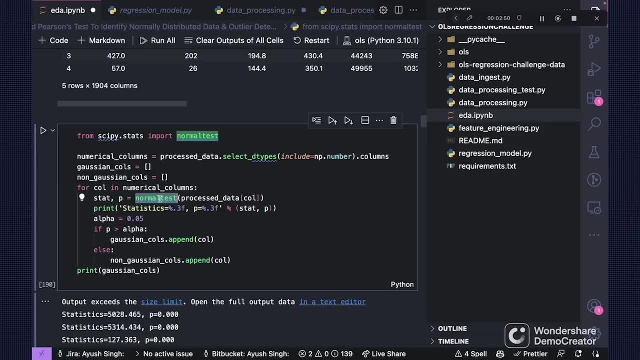 we are taking out the stat and p, p value for the normal test, which is which is conducted on that, conducted on that particular column, and then a printing of statistics and p value. and if now, there's, now our piece, our signature is: alpha is 0.05. so if a p value is greater than that alpha, 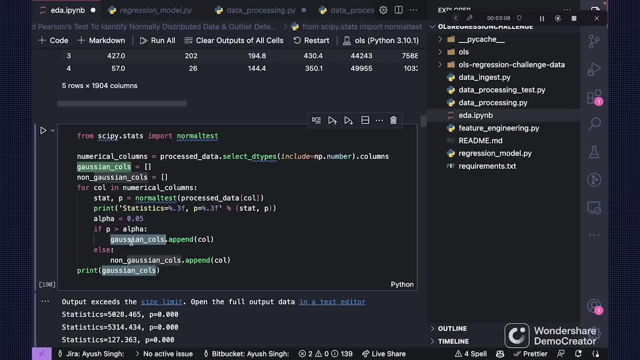 they're greater than the alpha, we append our column in that. uh, so it it. so, if so, what we say? we reject our null hypothesis. we reject our null hypothesis. and then we say, okay, that, if that p, if the significance of that particular column is greater than 0.05, we say that the, that, the, 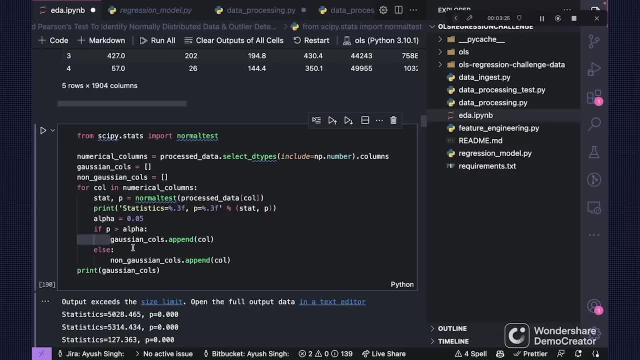 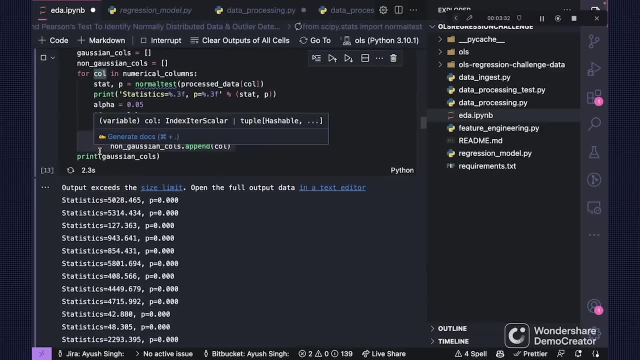 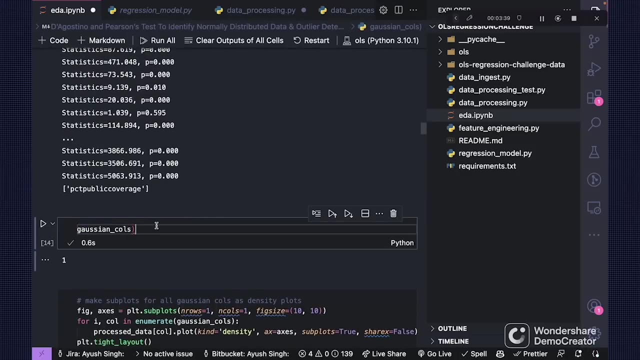 particular variable has the is the caution call variable and otherwise it is not caution. so, uh, we, we run it, then we run it. it will take some time to run it. so you see that we ran it. now, if you take a look at the length of the gaussian columns, there is only one column, which is normally. 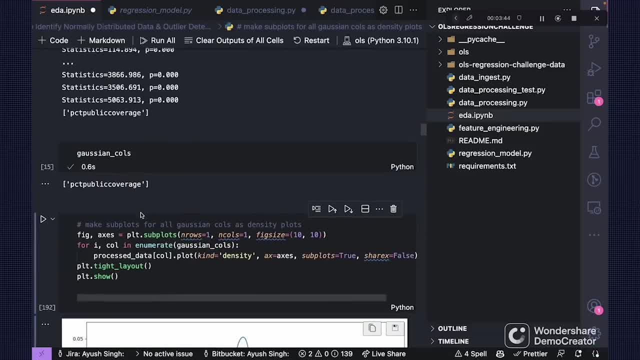 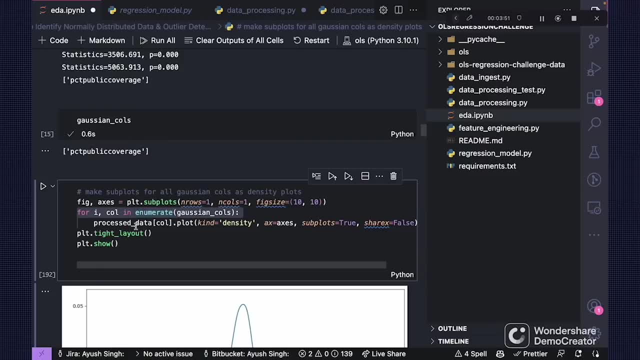 distributed. there's one, only one column, which is normally distributed, which is pct public coverage. now, in this, what you now we have now, let's check with that through the pct public coverage and we can see that we have now, we have now we have now, really, you know, uh, gaussian columns out here. so when you subplot it, and then here's the, 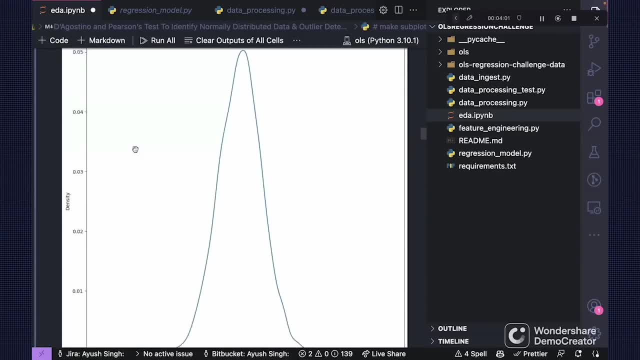 explanation of this code. so what you're doing, you're creating a subplot with 10 by 10 size. so this is: whatever figure is created is of 10 height and 10 width using a subplots function from the matplotlib library and there's n rows and n rows and n columns parameter. so you see, there is. 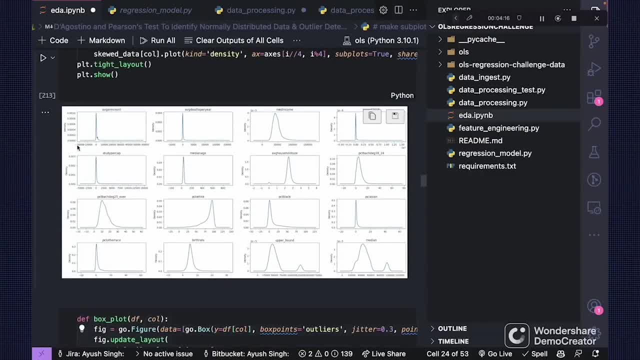 something known. as you see, if you this is how, so you have, and what is the number of rows and what is the number of columns if there's more columns, if there's more columns which are gaussian, gaussian or nominal columns, then you have a number of columns which are gaussian, gaussian columns. 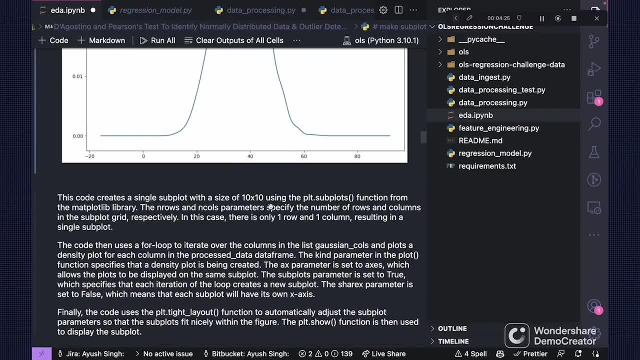 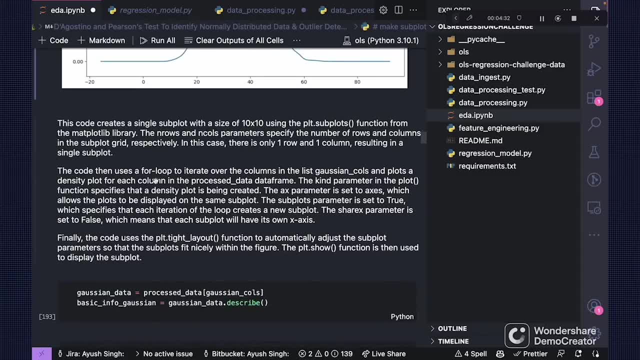 are normal distributed. we most likely go with this, you know, specify the number of rows and columns and there is only one column or one row because there is only one value of gaussian columns, and then we could use for loop to iterate over the columns. there is only one column in the gaussian. 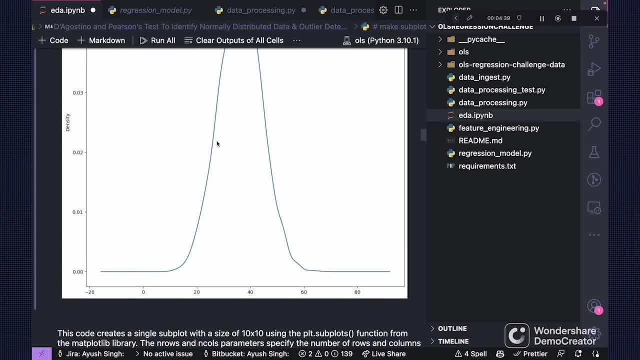 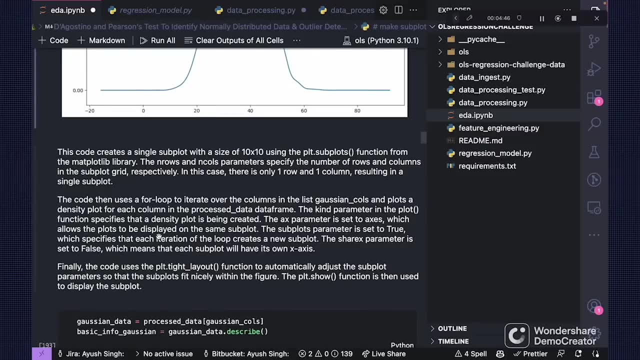 call. that's why we just iterate once time. and then we plot the density function. then density plot of that function. right, density plot of that function. the x parameter is set to xs, which is which allows the plots to be displayed on the same plot, and the subplots parameter set to true which. 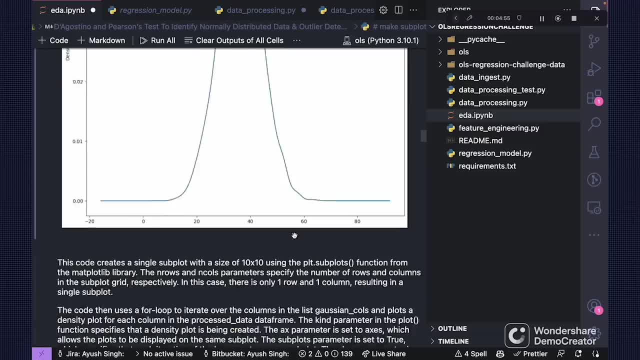 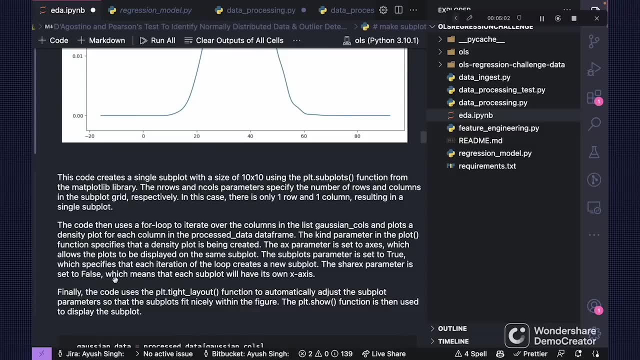 specifies the subplot values, which gives the function its number. and this is what we can see: that each iteration of the loop it should create a new plot. right, that should create a new plot. that's why subplot is equals to true, and then the share x parameter is set to false, which means that 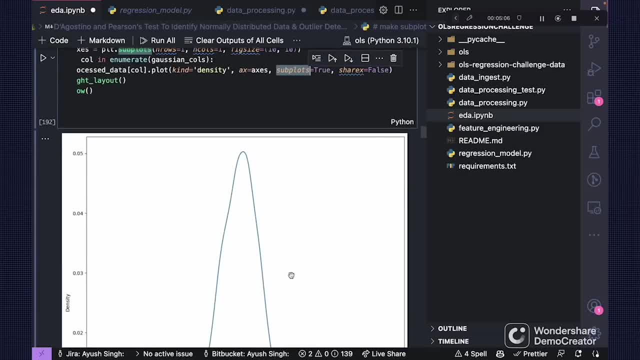 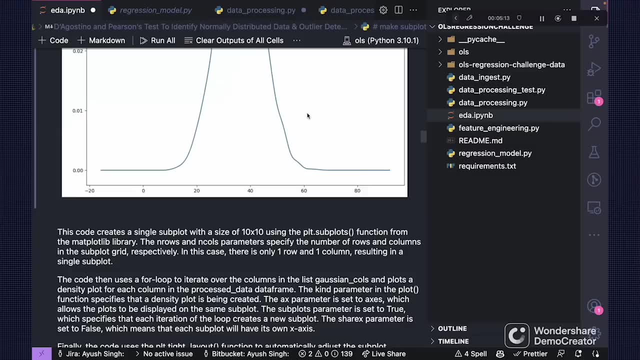 each plot should have its own x axis. so each plot should have own axis. that's why share x, which is sharing the x axis, should be false, right. and then we tight layout. tight layout means to automatically adjust to fit nicely within the figure. so it it ought, it should automatically. 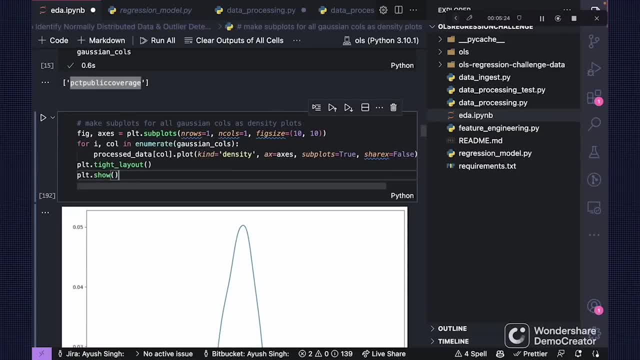 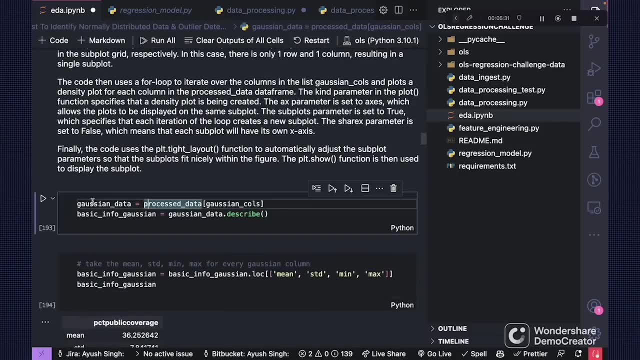 adjust so it fit nicely on the computer. then we run it. now we see that this is the only column which is normally distributed, which is normally distributed now. now, what? now, what we're gonna do? now we're not thinking: now we have the column, now, we have the only the column right now, so we print. 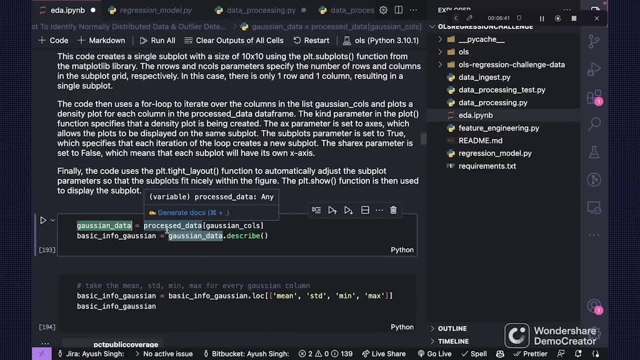 now we're going to take the, whatever data present in that column, right, because we want to identify outliers in that particular column, right? so we're going to take out the data from that column and then we're going to describe that data. so when you now you have the, now you have the. 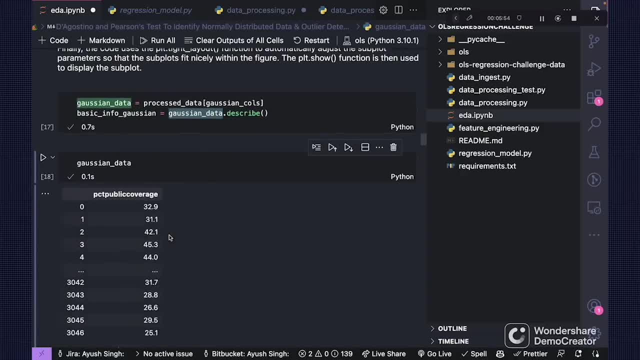 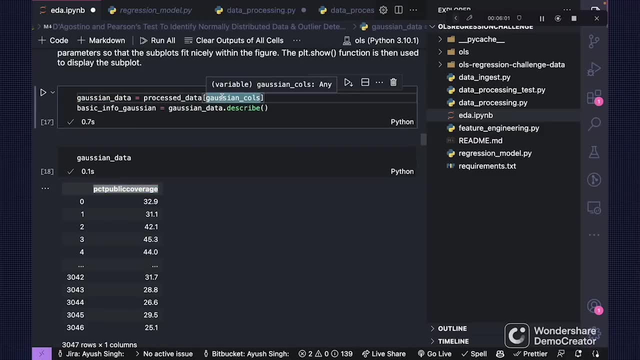 gaussian data, if you, if you print out the gaussian data, so you have only one column, pcti, which is gaussian, because we want to process data, and then we just have taken the gaussian columns out here, right? so it is just giving the column columns which are gaussian, gaussian, so now we have the 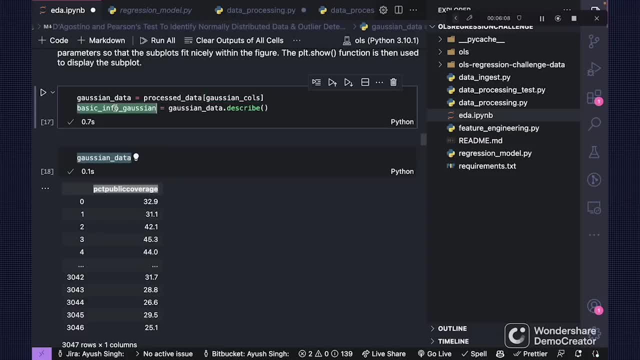 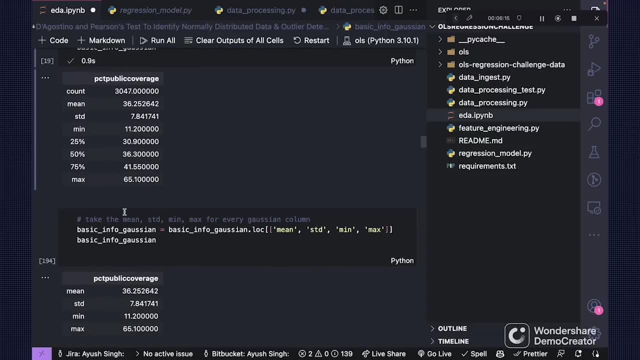 gaussian data- now we can perform our outlier detection on this- and basic info, which is basic info, which is mean, standard deviation count, you know 25 percentiles and 50 percent, etc. which is the good statistic which we'll use later on. then what you, then what you're doing, we are taking on. 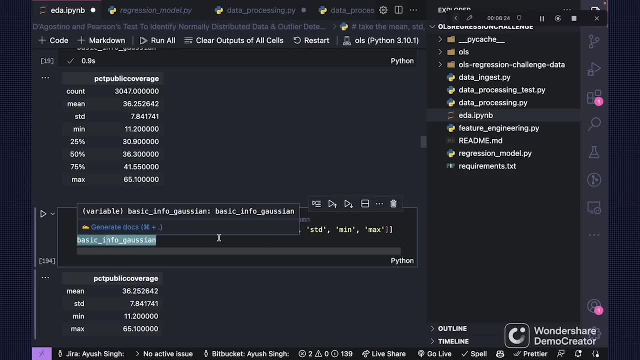 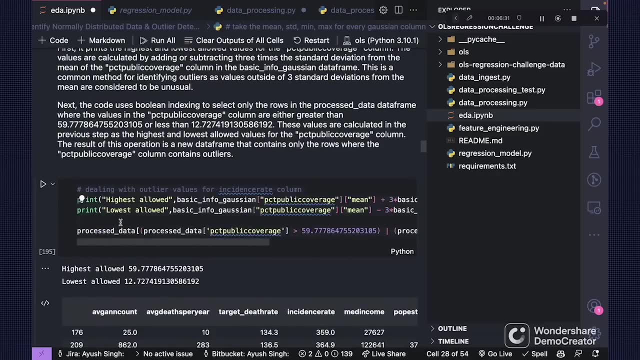 basic info so that we should, which we'll be using in our b info, which is mean standard deviation, minimum and maximum, and then what you're doing, and then and then over here, now, here the part come. as i told you that in, as i told you that we need to identify the highest and the lowest right. highest: 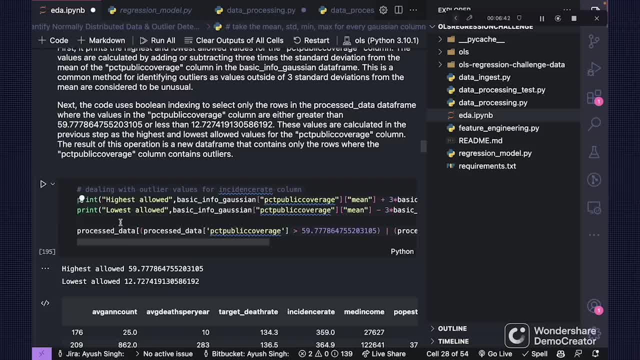 allowed in the lowest allowed and we'll be using the z score in that right. so what? what? eventually we are doing what? eventually we will be using z score for eventually taking out, you know, uh, highest and lowest. so what, what you're doing on this case? we are taking that particular column and then what? that? 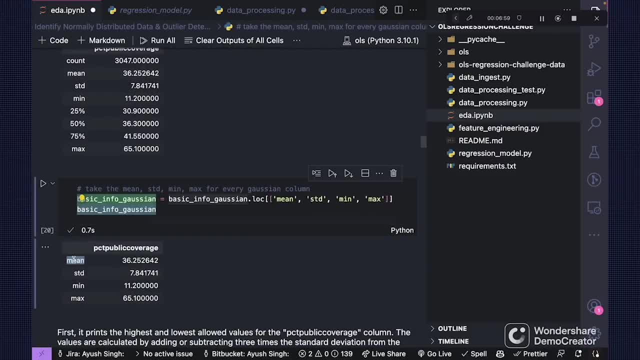 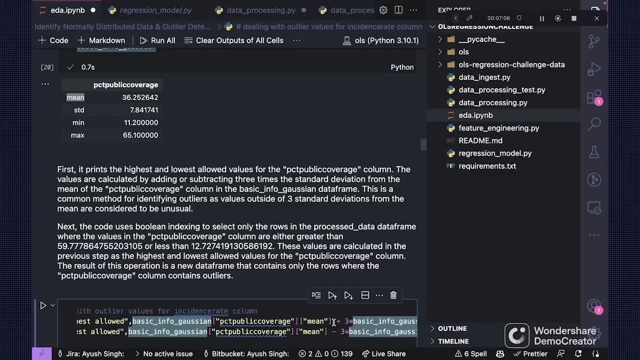 mean, because this is a basic info, basic info, gaussian. taking the mean of that minus, sorry, plus, that's the maximum thing, plus three times the basic info, then the standard deviation. okay, this is the currently we're using z score. that's why we have this formula. why this three, three? 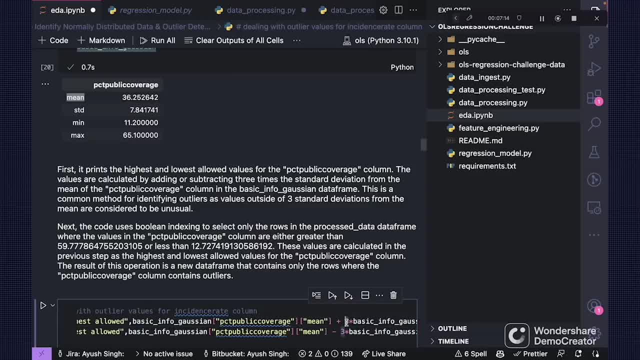 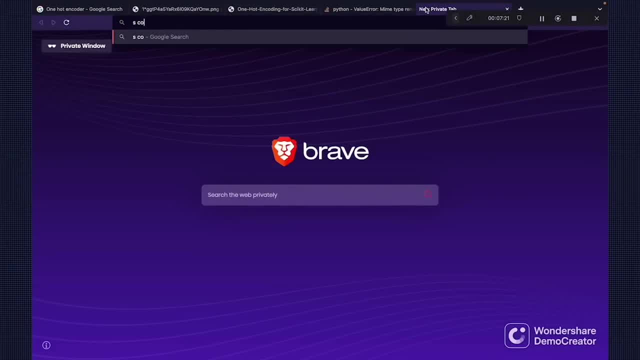 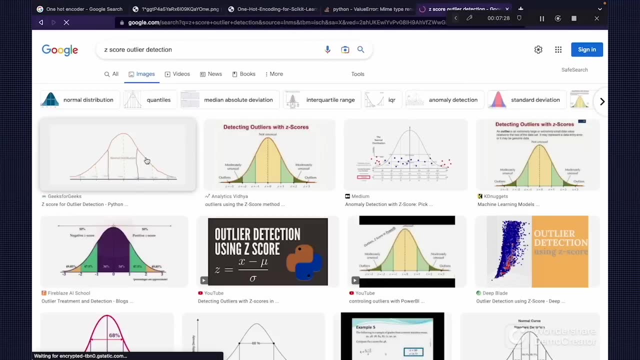 three can be changed. we're going to uh know, know the you know values which go outside of that. so if you go and see you know, uh, z score outlier detection, z score outlier detection, let's go to this so you can see that anything which goes and anything which goes. 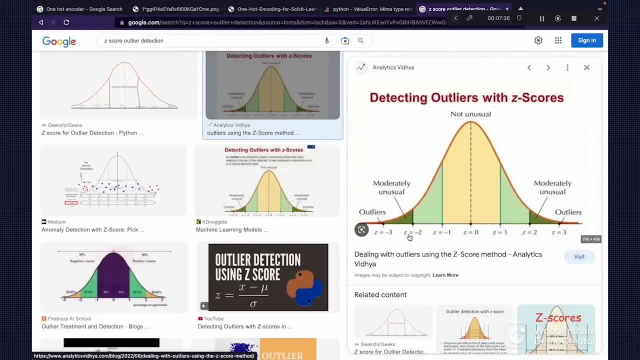 beyond this three, then that's outlier beyond, beyond minus three, below minus three, in that outlier. and beyond minus b, beyond three, and that's also out outlier, right. so the formula was this, formula was this, but you can see over here: ending z, score: anything below minus 3. ending above 3, above 3. 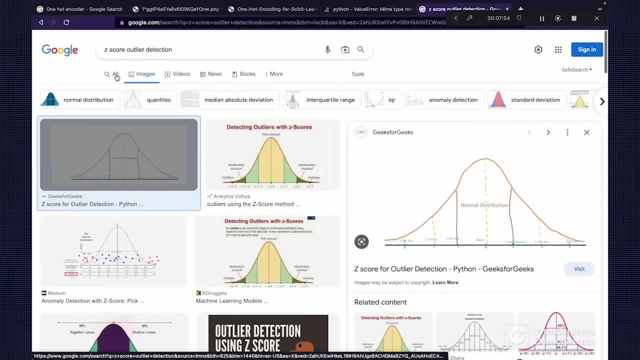 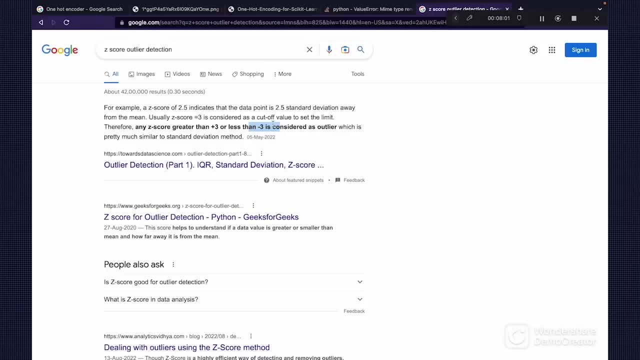 standard deviation three. they are outliers right. so if you see over here that there's the nice, any z score greater than plus three, which is standard deviation, or minus three is considered as a less than standard. minus is considered as an outlier right. so which is pretty much. 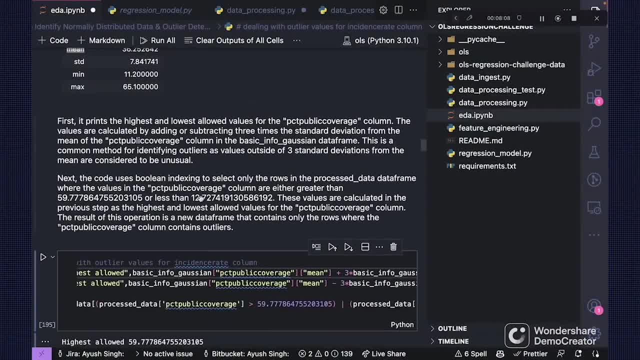 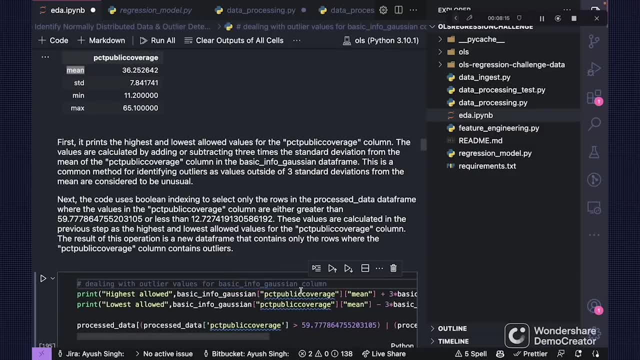 seen as the standard deviation. this is also called the standard deviation method. some people call it, but we're not going to call that. so we have the. we are going to take out, you know, for pvc column, not for incident. yeah, for this column. right that this is the. this is the highest allowed. so 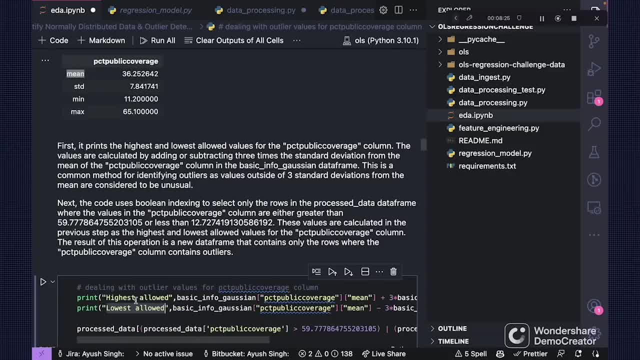 anything which goes above this, anything which goes beyond below this. so this is for plus three values and minus three standard deviation. so anything which goes, this is the my, this is the top of the plus three and this is the value of the top below of the minus three. so we say that highest allowed. 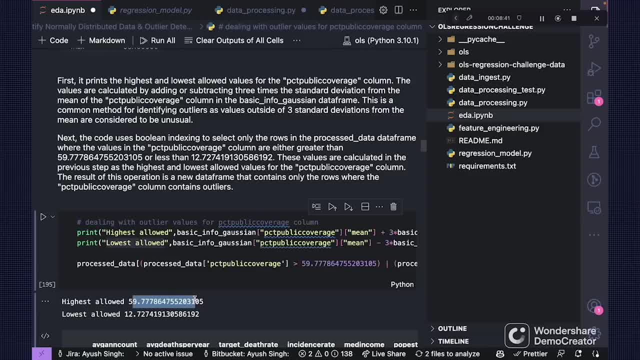 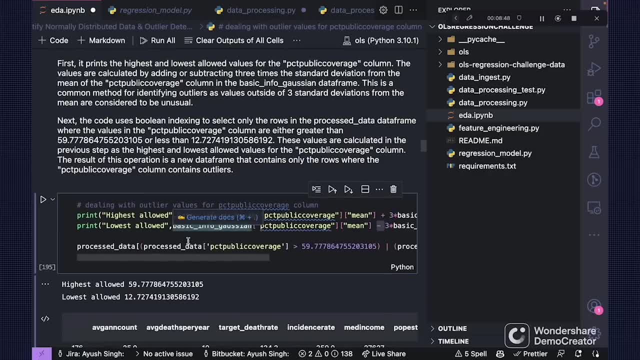 in that column is for 59, which is the plus three, which is the z score in this is plus three and is, in this case, a minus three. you lowest and where we subtract it. and then what you're doing? we are saying, we are saying key in process day, now you're going to print out. so we say the process data. 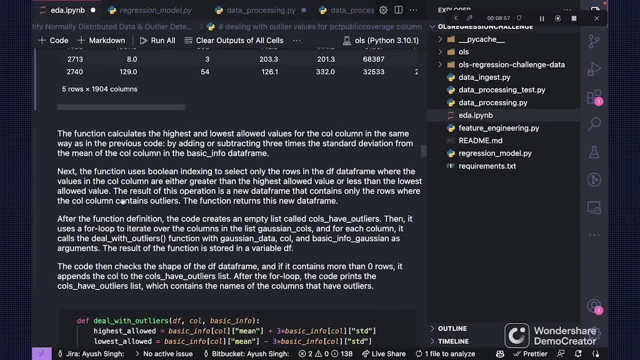 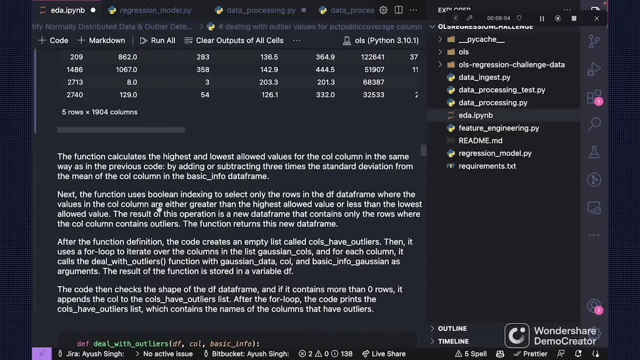 so you can see out here that what exactly we are doing. we are using. the function uses boolean indexing to select only rows in the data frame where the values in the column are either greater or the low, or greater than the highest allowed or less than the lowest allowed, and this results in: 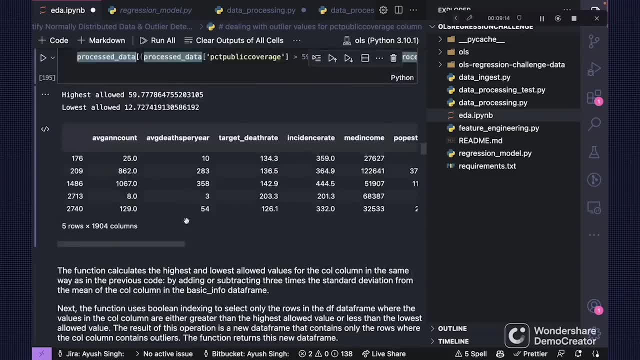 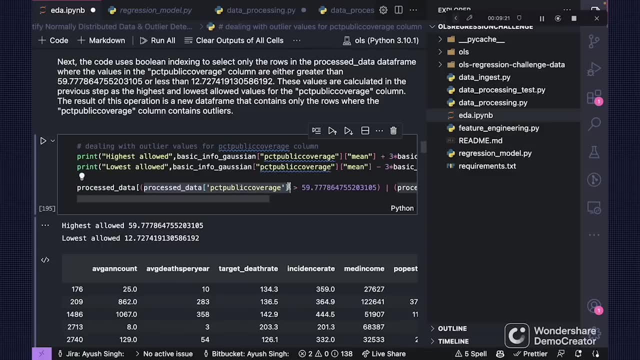 the new data frame operation and this is called the data wrangling. this is called the data wrangling and in this case you have pop processed and then we will go to go to the particular column and therefore loop, iterate to every rows, and they say any rows which is greater than that. print out or. 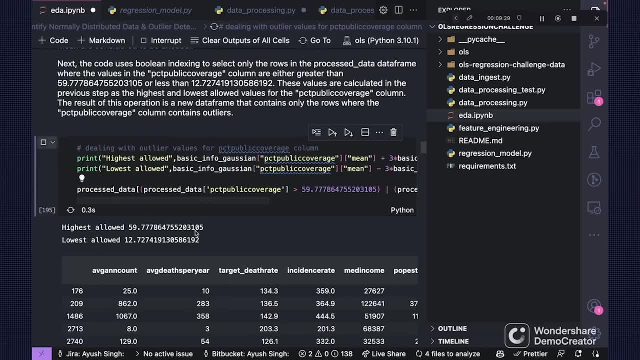 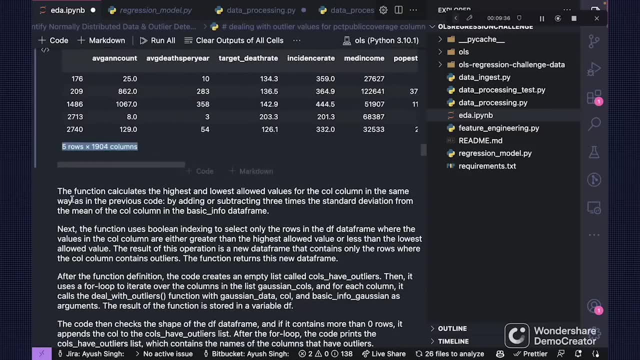 any rows which is more than this particular value and print this out and that prints out very nicely your columns. and there is only five rows which are which are acting as an outlier. there are only five rows which are acting as a outlier. so what we do, we make a function, we make a. 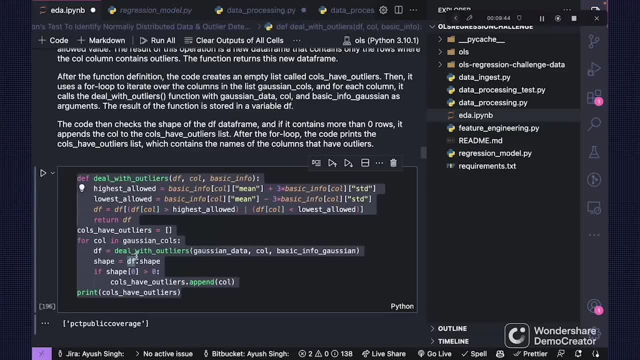 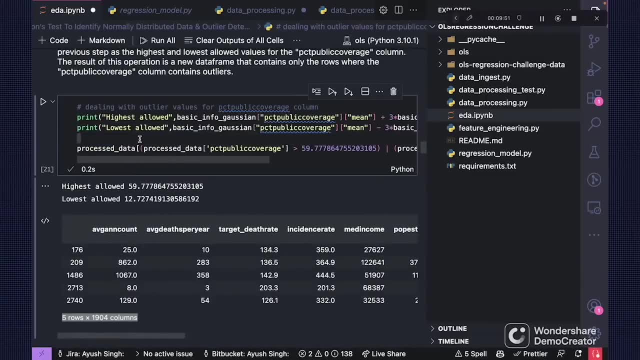 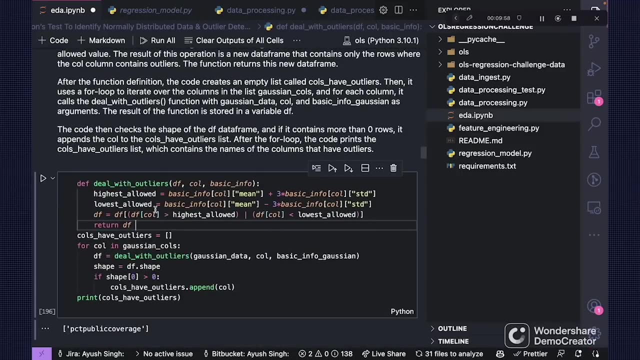 we make a function where we talk, talk, where a function that checks that deals with outliers, that checks whether that for that function is outlier. just we implement the advanced version of it where anyone can put you know column name and then he'll be able to able to get your the, the, the data frame right. so over here you have deal. 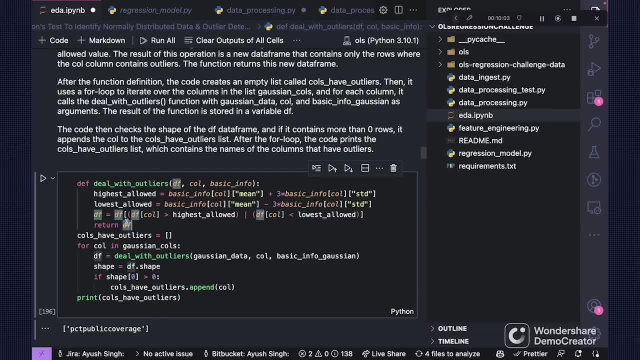 with outliers. so it deals with outliers where it returns the out there. it returns the data frame, which which is the outlook outlier data frame in that particular column. okay, it is for that particular column, so it is highest allowed lowest load, as we talked about, and then the data frame. 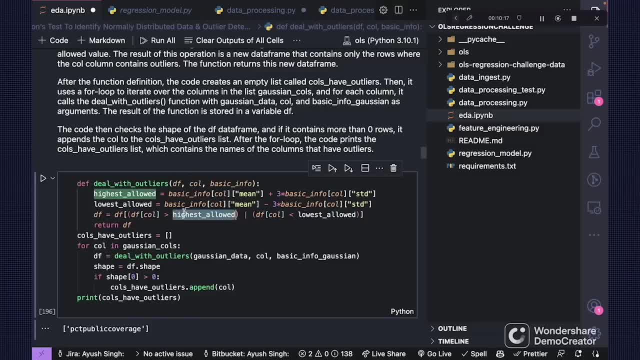 which we where that we select the columns, the rows where the high, where the date, where the values are greater than highest allowed, and select the rows which are smaller than high lowest allowed, and then we return the data frame. okay, now we want to, we want to get the columns from our data set, so we 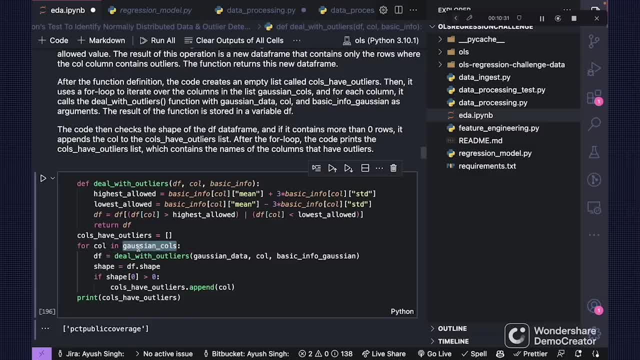 have the gaussian columns. so now you have the gaussian columns where all all our columns which are normally distributed as of now we have the gossip columns which are. there's only one column in that which is normally distributed, but we're going to go forward and talk about to the all the. 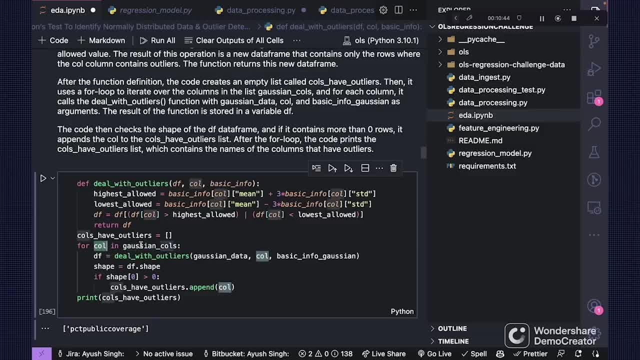 there might be other columns as well when you're working on a project, right, so iterate through every column in the gaussian columns and then you say: deal with outliers. you call that function and then you say: what? what are the? what is the data? data frame we have? 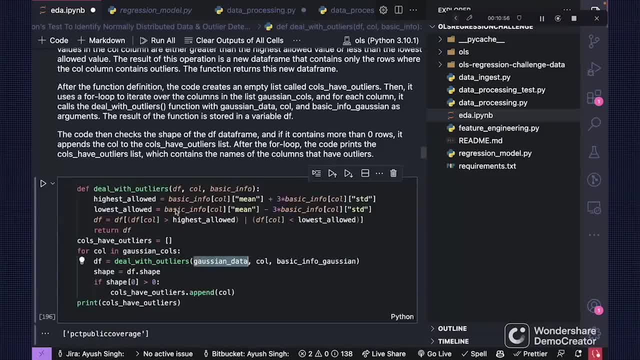 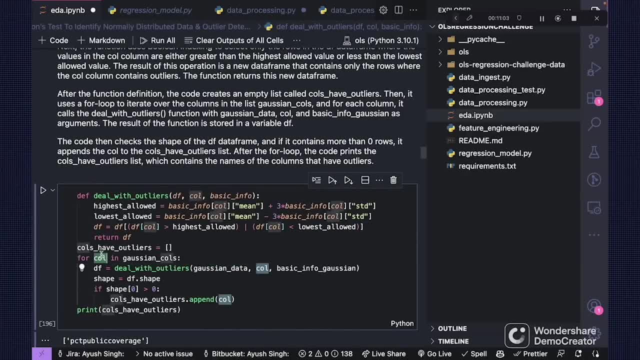 is gaussian data, which you have right now is the gaussian data, where we have only one column, so you have to also convert that to uh, gaussian data, which should be the gaussian data, and in that gaussian data you have these columns, these uh, this, this particular column, because we're iterating the 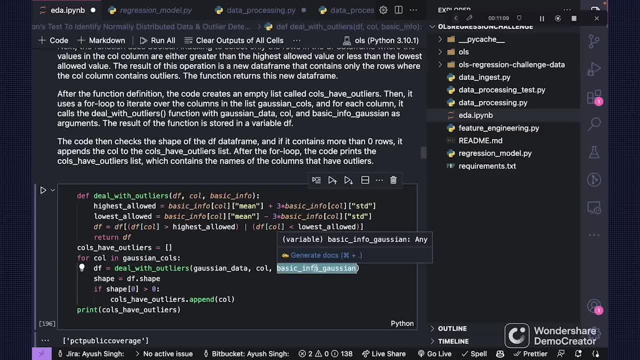 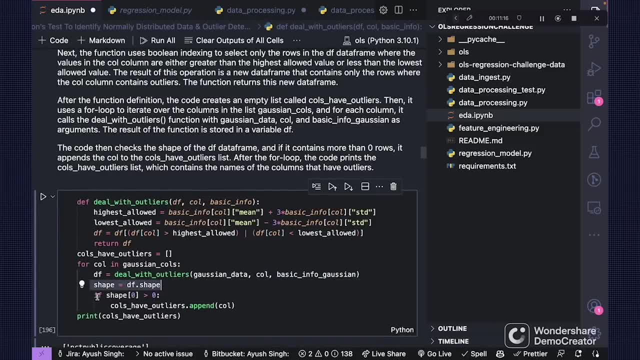 gaussian columns and the basic info which which we wanna give right, the basic info which we have to give as of now. we have already taken out all of these elements from here right now, these three, and when you take out the shape, and if that shape is greater than zero, then we see that. 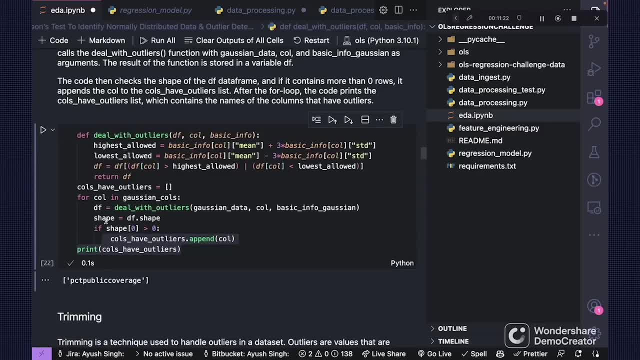 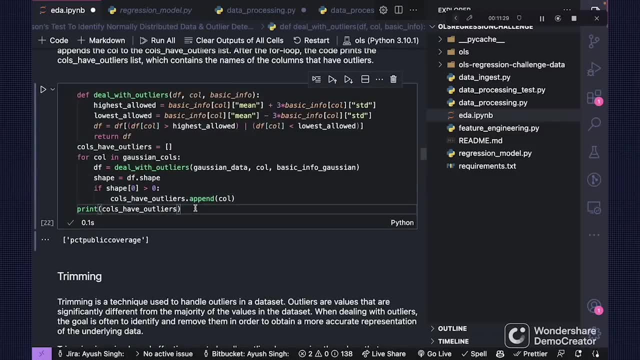 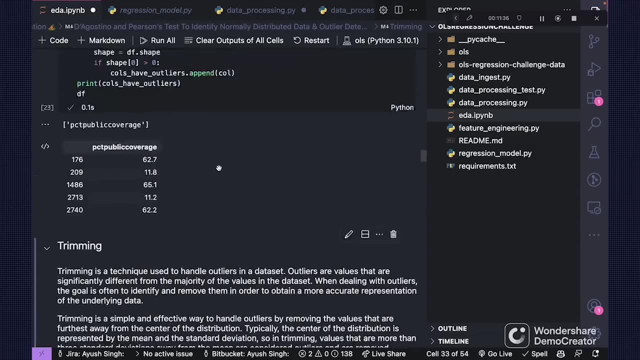 that callers have the, have the outliers. so as of now, the, as we expect, pct public coverage has outliers. okay, so what? so now, if you print out this data frame, now if you print out this data frame, so let's print out the data, let's print out the data frame eventually, so you see that we have the data. 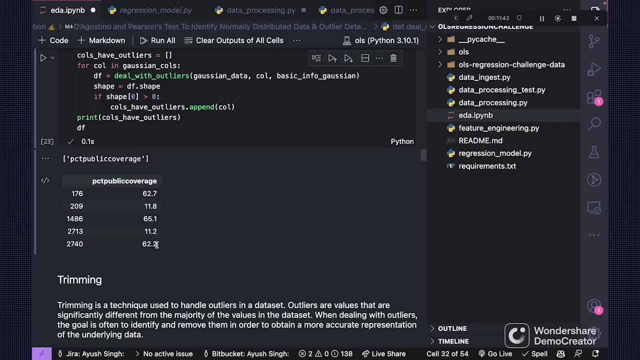 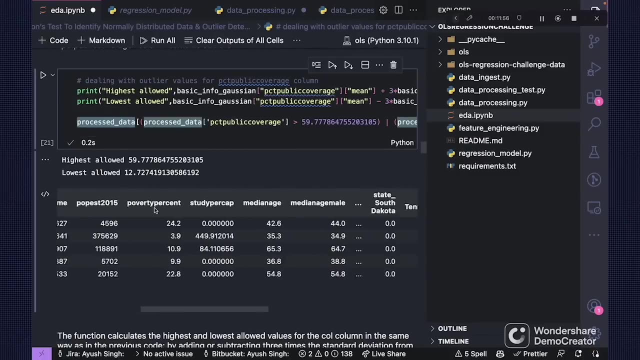 frame. we have the data frame, which is a five rows and five rows column, so you have this particular data frame. okay, in that particular column you have this, this value, which is acting as outliers, which is acting as a outliers, but over here you see, process data is showing all the values, but 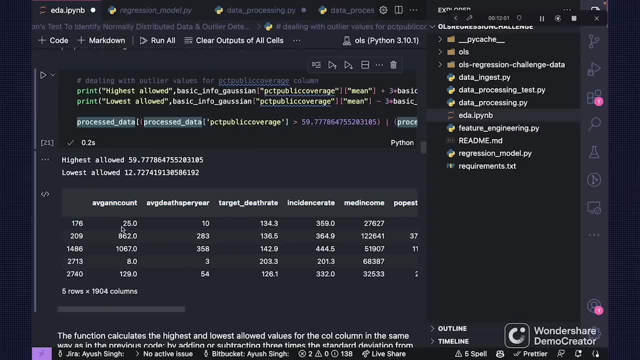 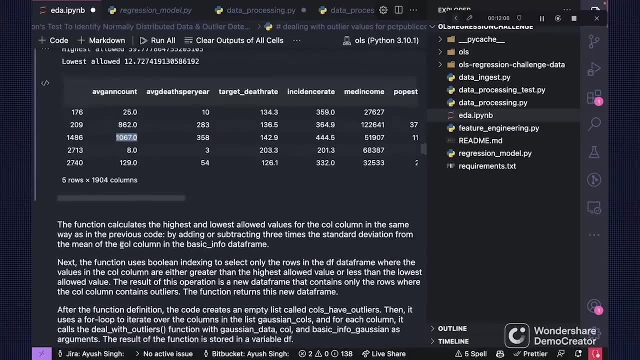 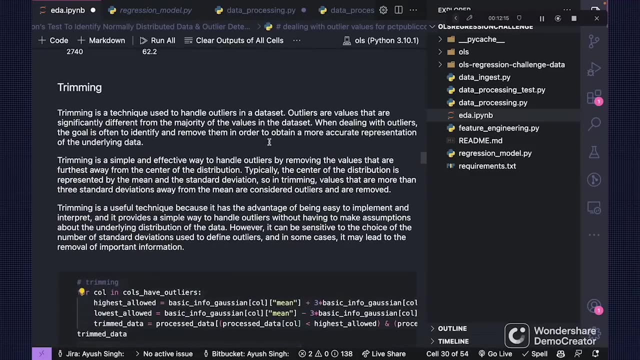 we are interested in only this- put this particular, you know uh columns. so we just remove, we just remove those trimmed, trimmed, those values from our original. so we remove this outlier, this outlier, this outlier, which means removing whole rows. so there are a couple of methods while dealing with outliers. first one is trimming. second word is capping. 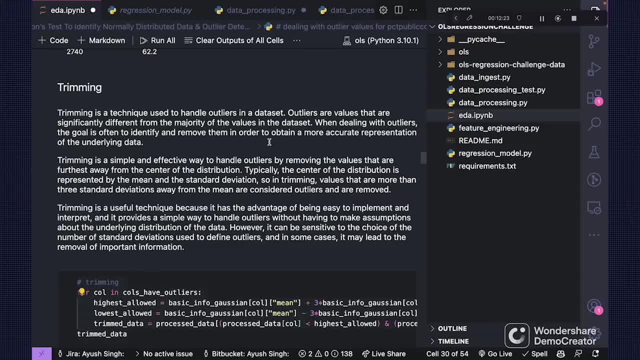 trimming is a technique which is used to handle outliers in a data set, which means that outliers are values that are significantly different from majority of the values in a data set. when dealing with it is it is when dealing with outliers, the goal is to identify or remove them. 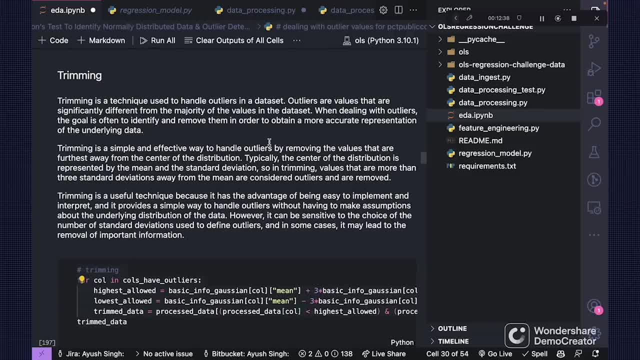 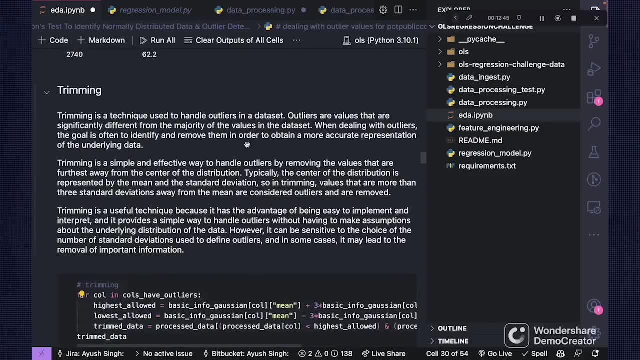 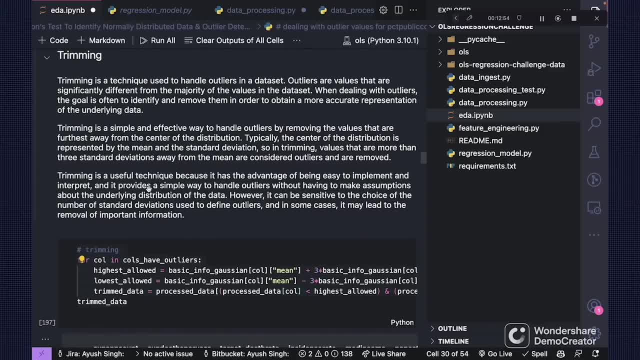 useful if it is useful when it is useful when it uh, when, when, when there's a when we know, uh, it is easy to implement, to be honest, and it and for interpretation of it, it provides a simple way to handle outliers without having to make any sort of assumptions, just about removing, like any missing. 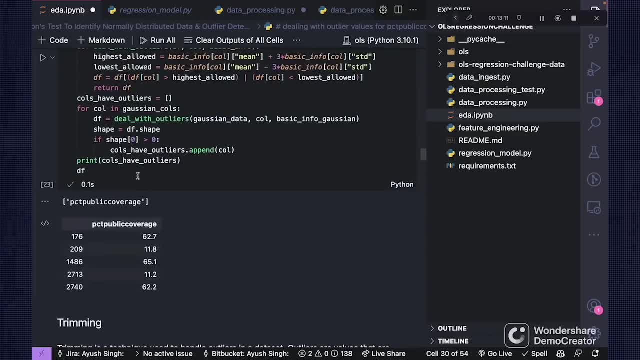 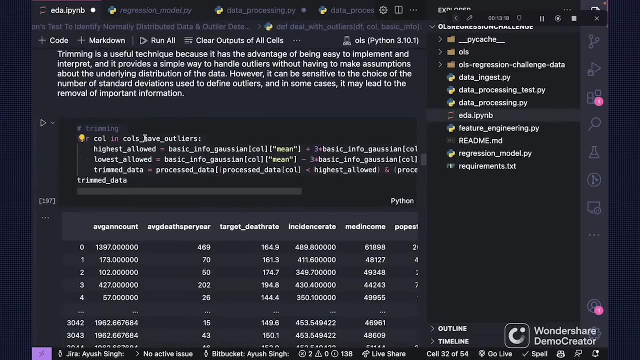 values. so here's what you do: we go to the now we have the now we have the goals that have outliers right, and then we print the date frame where it has the outliers right, where we can see clearly see. then we iterate through all the columns which has outliers, then we just go to highest allowed. 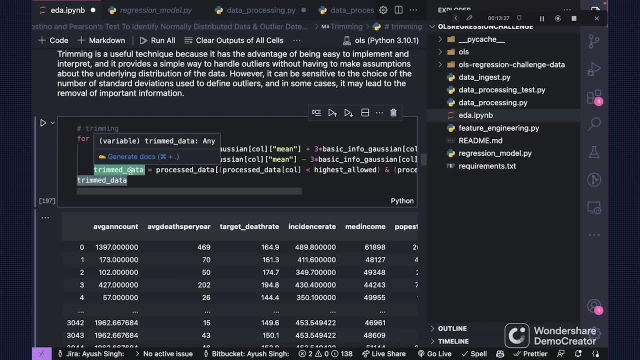 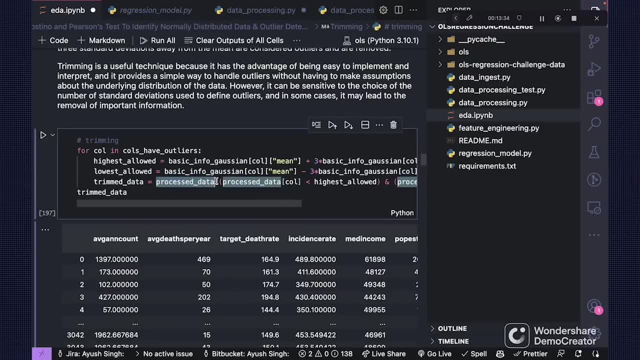 and lowest allowed and when it trimmed data. trimmed data, what does it mean? trimmed data? which means we go to the process data right, and then we say that, and then and, the, and, and then we see that, um, yeah, so over here, over here, we are printing the process data that we tokenized, our 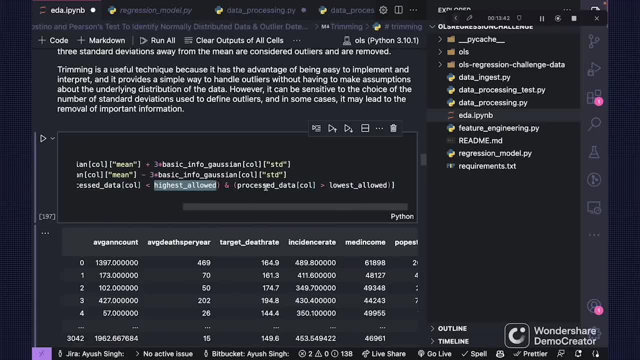 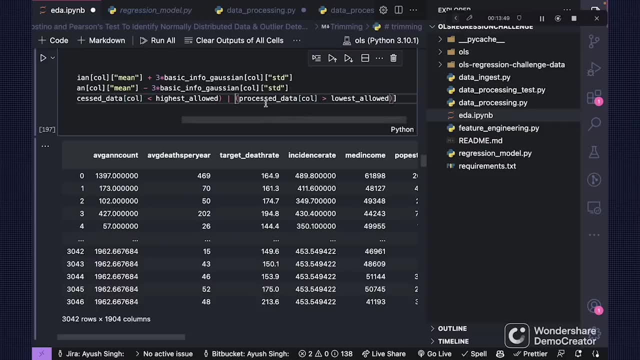 transfer we set using a HOST train and we entonces go into the process screen right, and then we say that, and then, and then we say that oST training. here we say that that particular column is smaller than highest allowed, or i think this should be, or this should be, or, or um, that particular is smaller than lowest allowed, is great, is greater than slow. 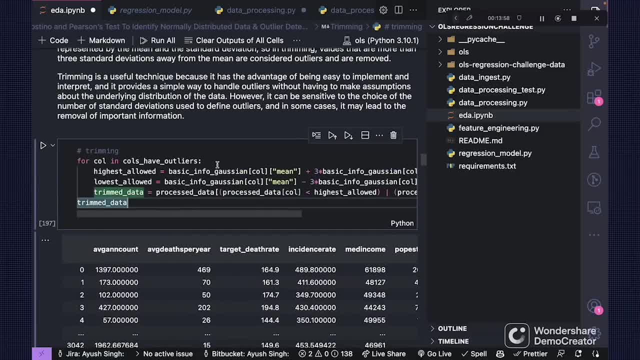 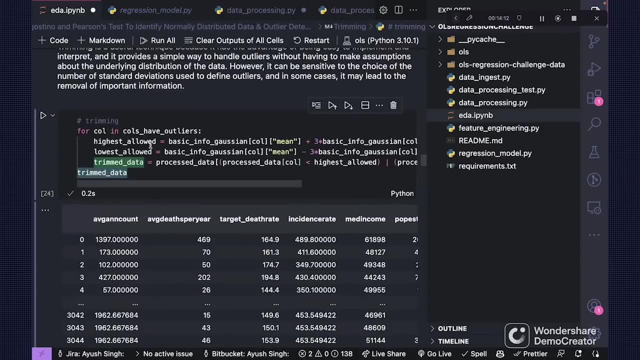 as loud. so if, if that happens, removed, remove the column right, it is a trim data. we're only selecting rows, only selecting rows which satisfies these two conditions which we already seen: which is great, greater than values and, uh, smaller than values, right? so if you see, the process, data. 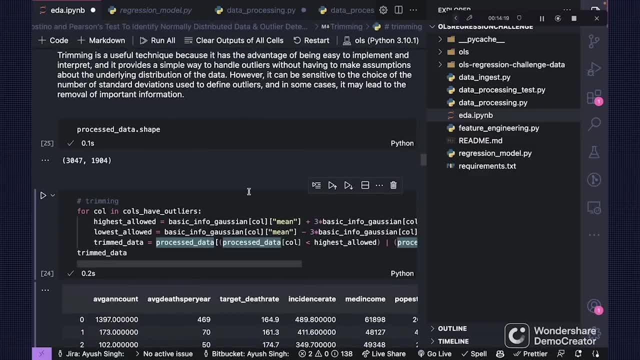 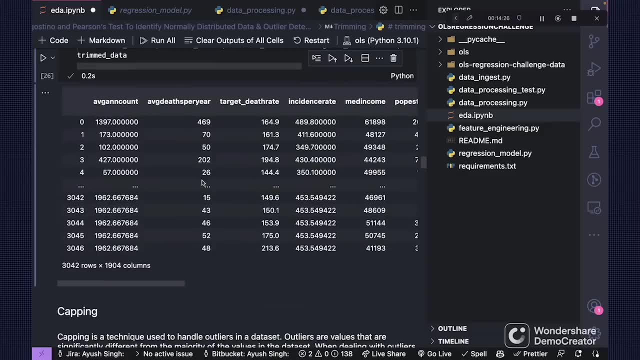 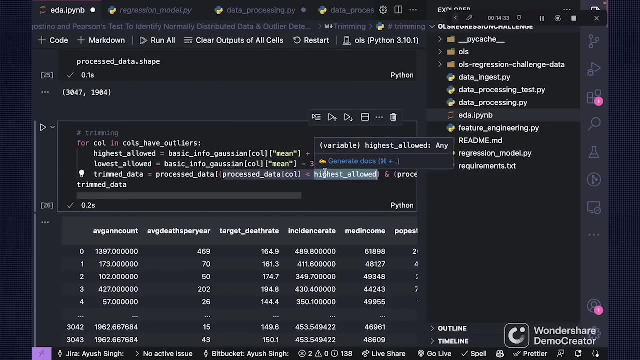 in dot shape, you're 47, so i think we we have to have this, both the conditions right. we have to add this, both of the conditions to further successfully do it very now. it removes all the values which are, you know, uh, satisfies these both condition: it has to satisfy with these, this, this, both. 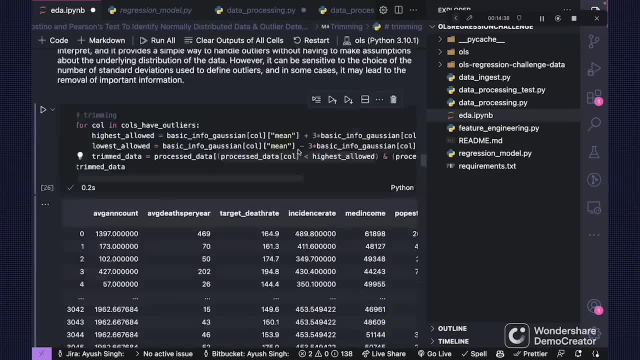 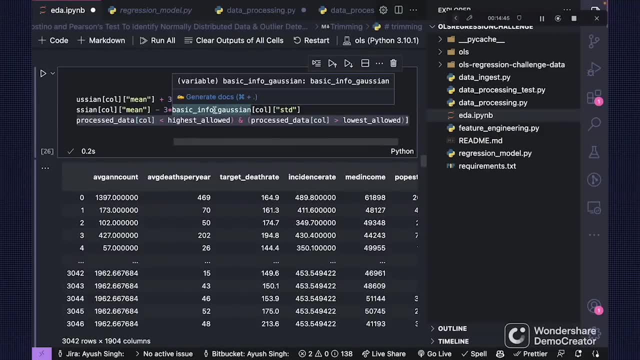 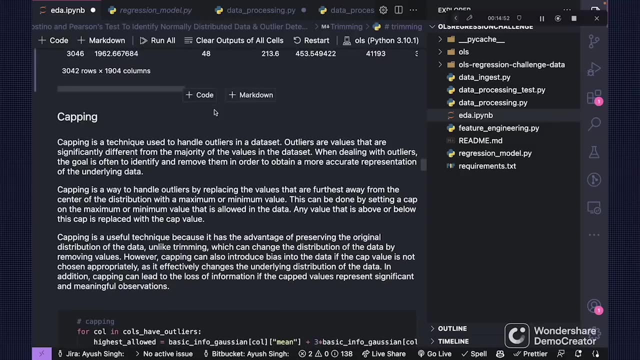 conditions right now. that's trimming. trimming means removing of the outliers by by your data wrangling conditions where we see if that particular value in that particular column is greater than highest allowed for that particular column, we remove that. and then if that particular is less than that lower allowed, then remove that as well. capping, capping is. 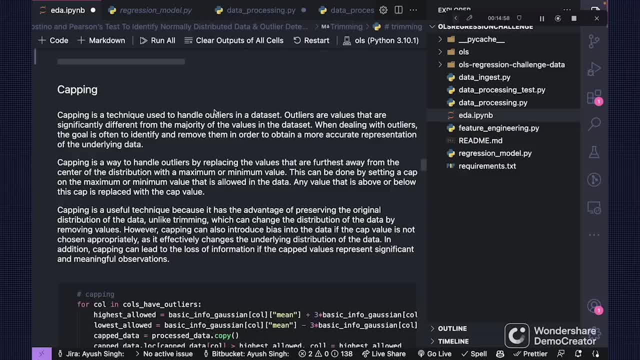 another technique which is used to handle outliers, which means that, uh, which means that to handle outliers, by replacing the values that are farther away with the maximum or minimum value, so we just remove the- you know value- root values of that particular amount with the maximum or minimum. 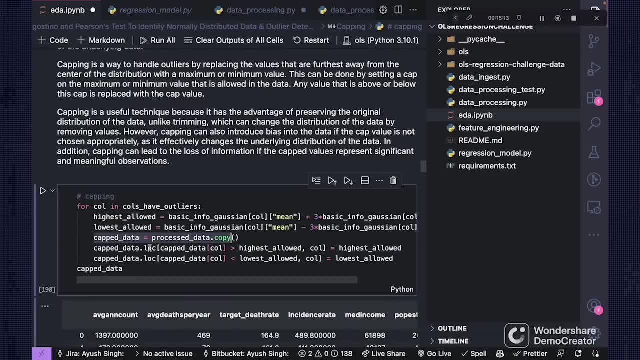 so you can see that highest, and then we create a copy and then we say that in that we lock loc, we go to the values in that particular column, as we saw that column- in this case a public pc to average- then go to this column and then go to the if there's anything which is greater than. 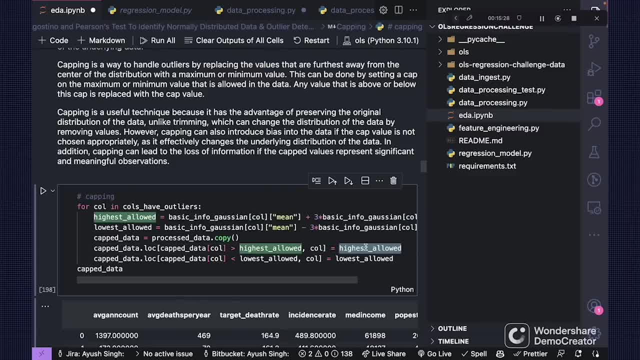 highest allowed, and then we simply go to that column. if Evezy is equal to the highest, that's a maximum, and the same goes for minimum. so we simply have this capped data where we simply re, rim, move our, we simply remove our, you know what our outliers, with a maximum or minimum accordingly. 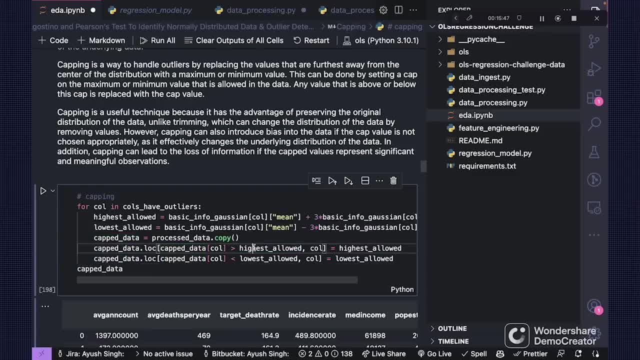 you can see, anything which is greater than highest allowed is going, is going going to be going- going to be replaced with the maximum. anything which is smaller than lowest allowed is going to be replaced with the lowest allowed. now we have the capped. now we have the capped. 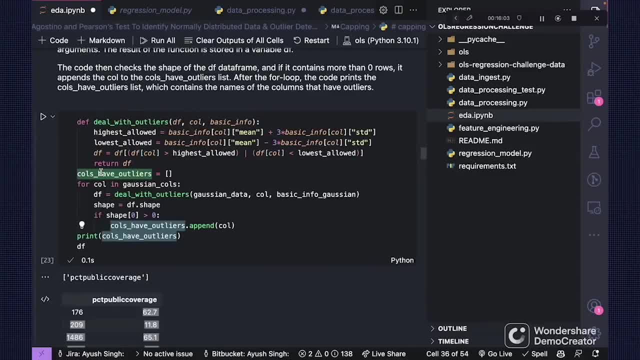 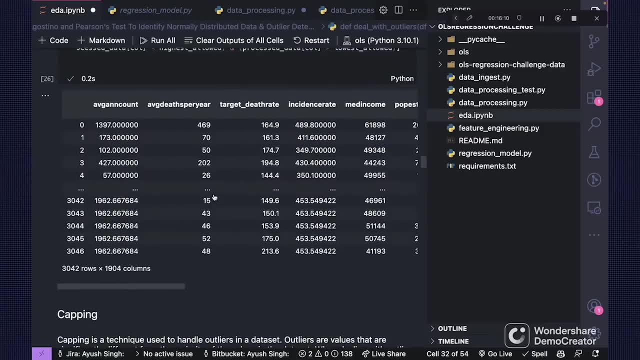 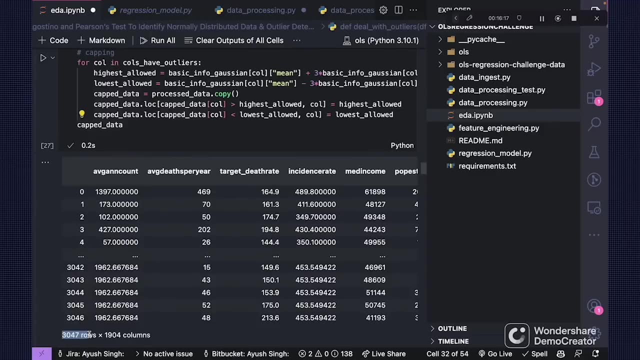 data. now we have the capped data. now you can see that this cap, that now this cap the data will not have any such outliers in this, any such outliers in this, right and always. you can see we do. we are not removing any call and any rows, we just capping it. so this is useful when you don't want to lose. 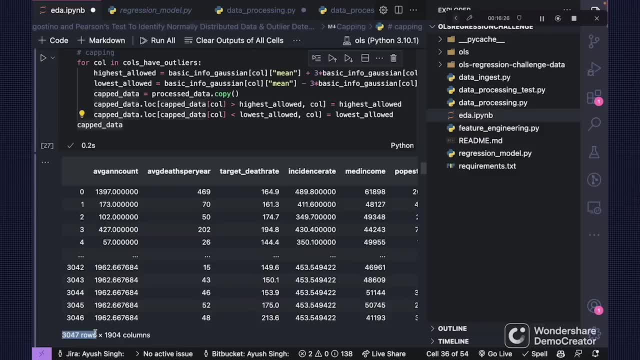 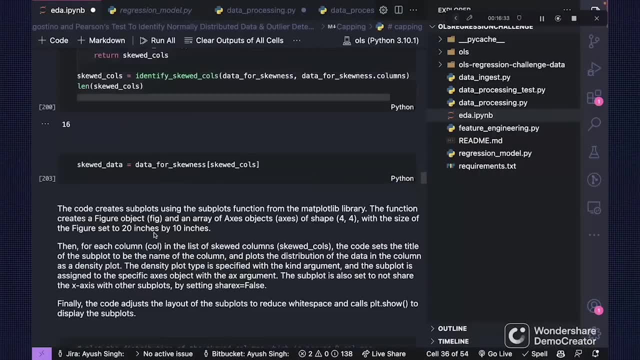 or lose, lose of your information. okay, i hope that really makes sense now. i hope that you want you, you, you. you understood everything which i want to teach about outliers and in the next video, what, what, what you're going to do. i think it's pretty much understandable from now on, but i'll again. 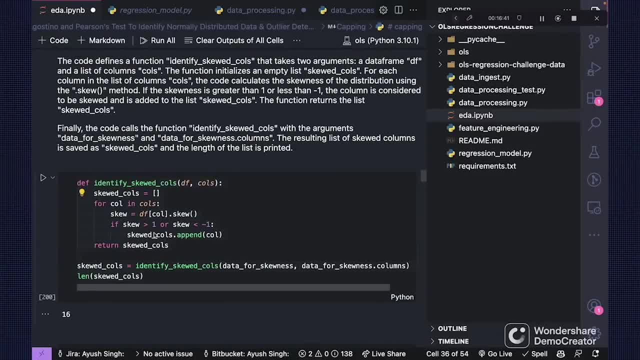 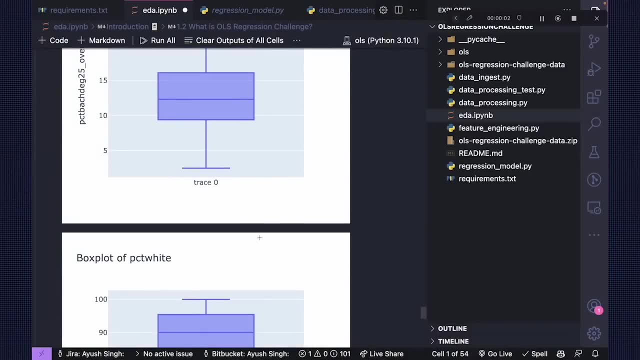 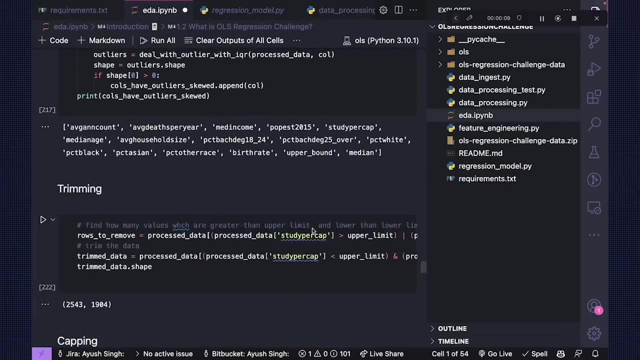 make it for those who didn't understood again. so i'll make another lecture on outlier detection if there is a skewness in your column. so, folks, welcome to the next lecture on um, when, if many, many of you have requested me to work to actually complete this stuff, and that's why i'm just going to going to complete this and 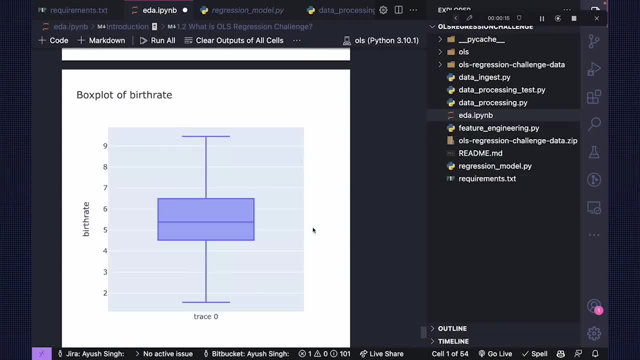 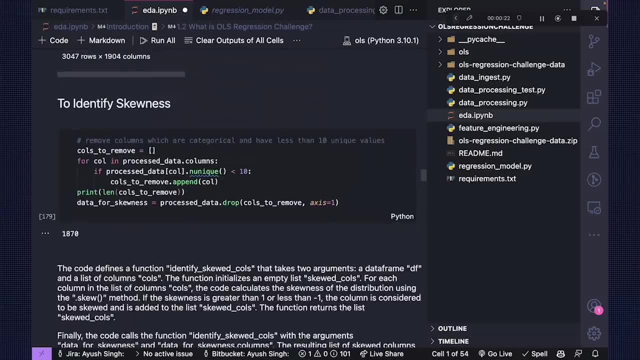 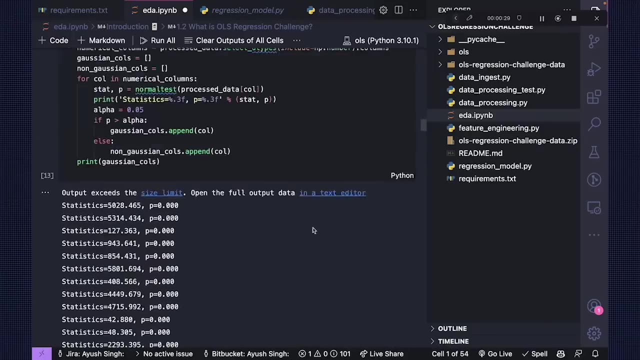 you might have questions around like why the hell? um like on outlier detection, like, uh, first of all, we have used, you know, for we have separated our normally distributed data. so you- so you might be seeing over here- we have separated our normally distributed data, for example, in this, which is which, which we had um outlier detection, i think. 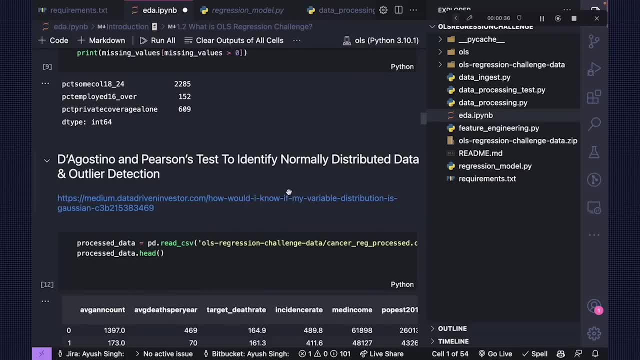 there should be one, yeah, uh, which is outlier, out, outlier detection, using on normally, normally distributed data. so what do you? what we were eventually doing in this um approach is we were trying to uh from our, from our- uh, whole data. we were trying to extract columns, we were 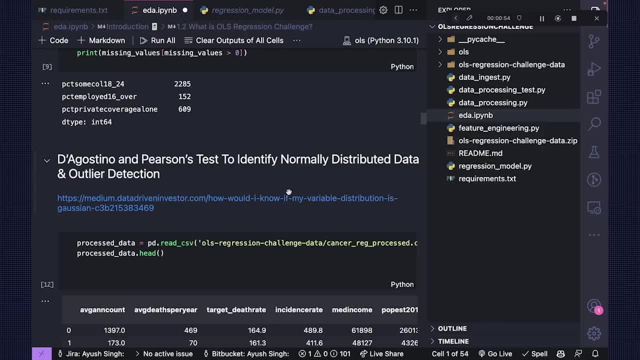 trying to extract columns which are of, uh, which are of which are not normally distributed. okay, so, uh, for example, there are several columns and from that we were trying to extract columns which are normally distributed. um, and if you don't know what normal distribution, please see the lecture. so, 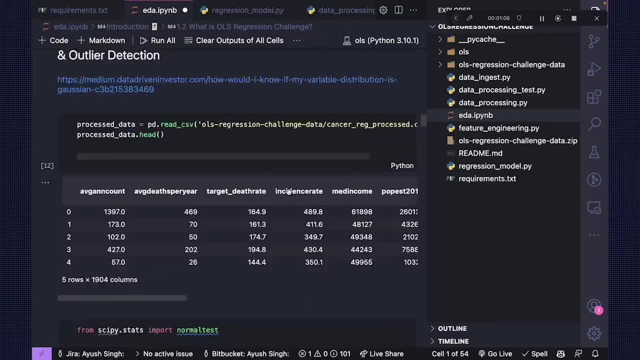 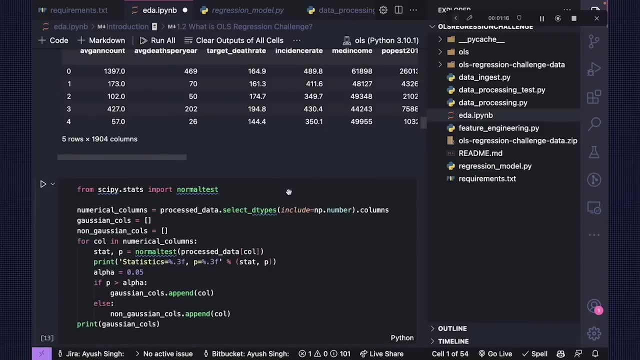 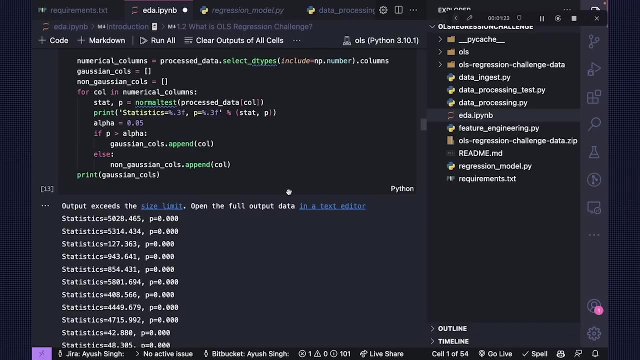 normal distribution, which are prepared in a very nice way. so then we use some tests to to determine, uh, we use some statistical tests to determine whether that is the, whether that variable is normal, distributed or not. and we have used, and then we use, you know, the thing which is p values to, to say to, to identify that particular variable. 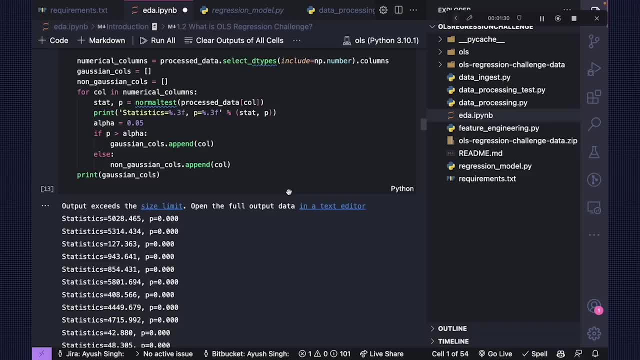 is a normal distributor or not using the certain test. however, you don't need to go in depth about that. how do we identify? that is for more like who wants to go in in depth. but usually in interviews they don't ask like in depth all all of these things. but it's good if you know, if you know. 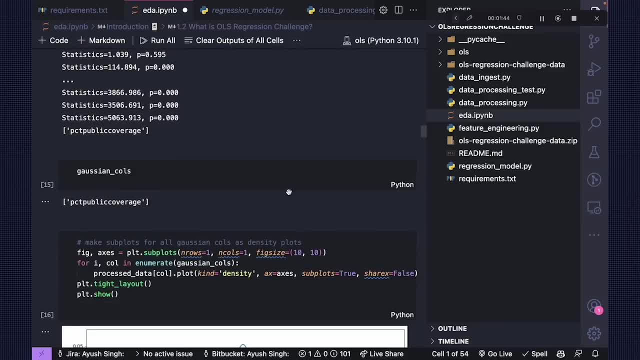 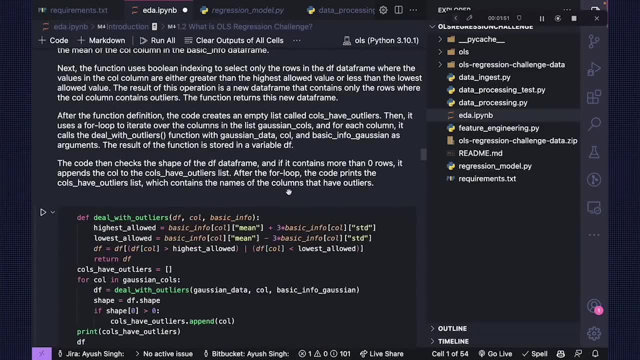 if you know about that, but that's something for statistics majors and all, but not for, uh, i guess, for machine machine learning. so now you're. so only we have, we, only we have analyzed only one columns, the. the reason why we are categorizing it first is for um for them, for, for example, for: 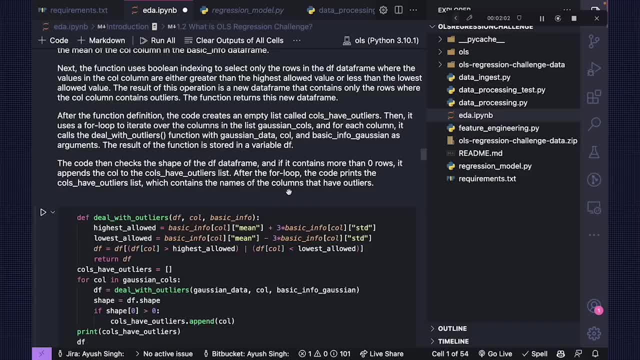 normal, normal distributed. we, we use z score, um for z score, for outlier detection, for normal distributed data. right, but but there are several columns which are not normally distributed as well. unless they are um. like they, they follow other the distribution. so what should what? what should we do? how should we handle? should we go to every individual variables and then identify, uh and 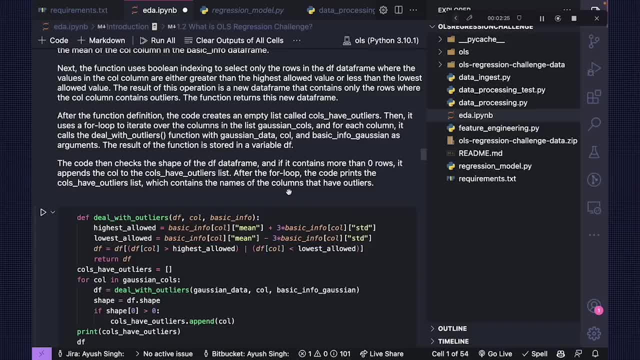 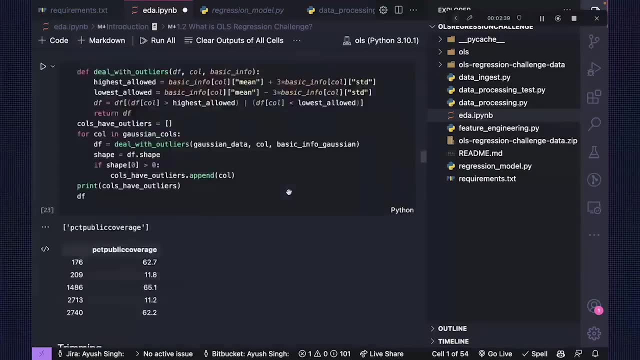 then identify what is there in what is the uh outliers in that particular column, or, or we give, or um, what or what we do. there is something called as iqr, interquartile range, which we use, that for outlier detection, iqr for outlier detection, iqr for outlier detection. so 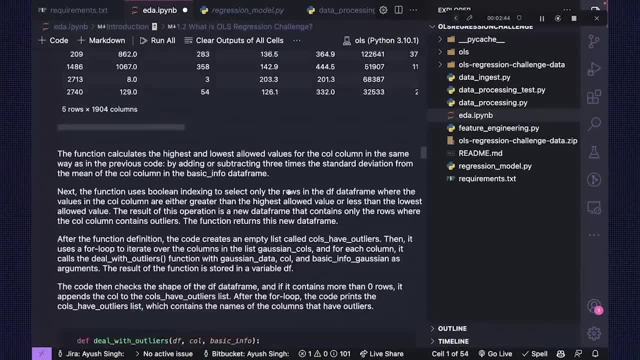 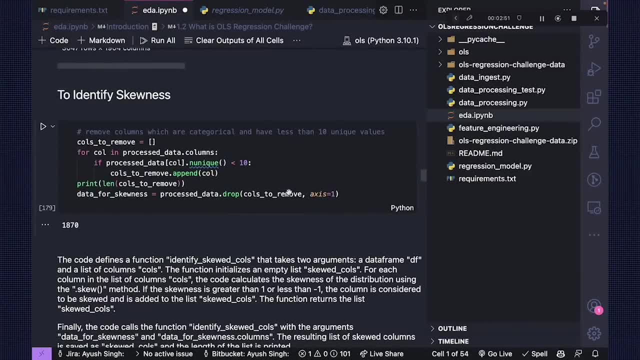 let me just tell you the iqr for outlier detection. yeah, so we use outlier for uh, iqr for outlier detection and then uh. that iqr works on skewed data. skewed means a positively shifted or negative, negatively shifted. we have already talked um. we have. we have already had a talk on this. 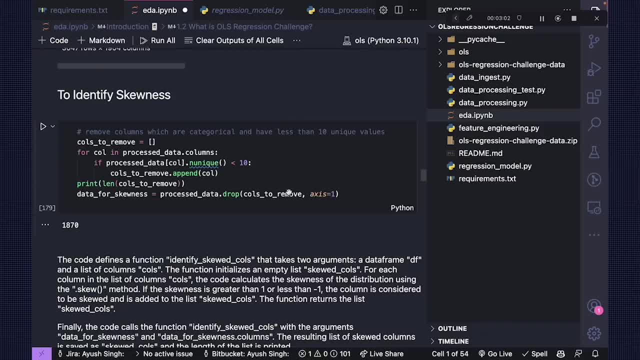 please make sure that you actually um go towards it now. now, coming back to, uh, one of the questions which may arise. wow, like like a student asked me: like: hey, ayush, how can we identify which columns to test with them, whether that column has outlier or not? just, i'll let you know one thing is that this is very, very, you know, a big problem. this is 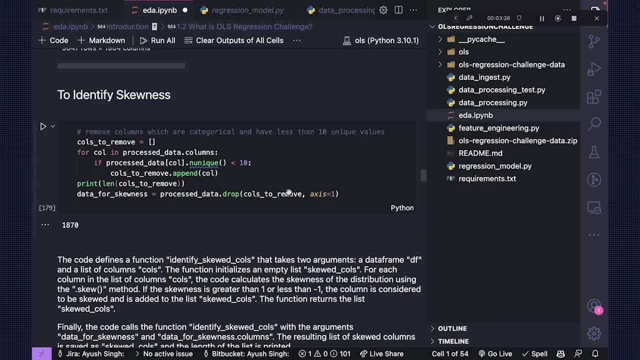 a big problem in um. like you, you can't just go to every variable and then do things according to your own pace. every each one column might follow normal distribution and another column might follow skewed distribution. right, so they have two different distribution and normally, or normally there is z, score works and on a skew there is other. 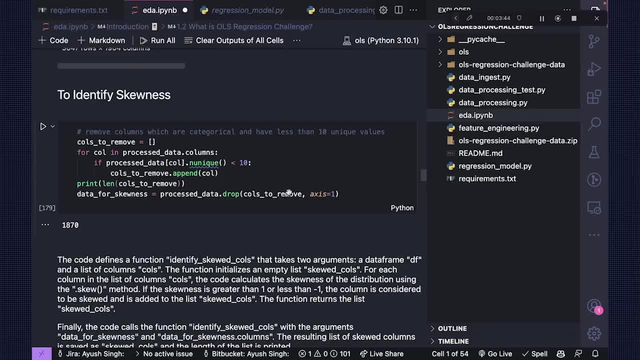 method works right. so that's a defined set of rules which you already have, and, and, and. what we do is simply classify in different, different categories and then we apply the required outlier detection techniques for the same, and mostly our data has a skewed data. so, first of all, what? what we do? uh, you, you might have seen our data has 1900 columns. 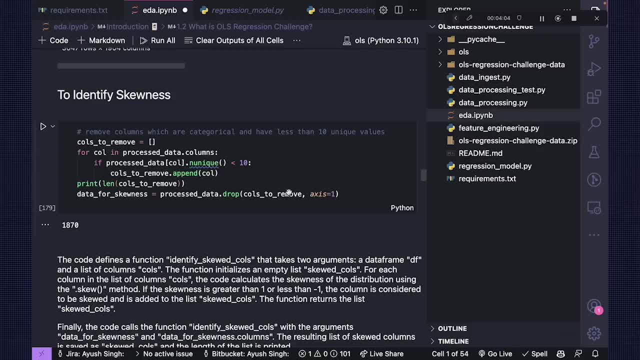 our data has 1900 columns. so what we do? so what we do is we simply say that, um, we take 19. why? why they have 1900 columns? because we have encoded our categorical data. that's why it went from, you know, from small amount to large amount. so, first of all, we identify columns which 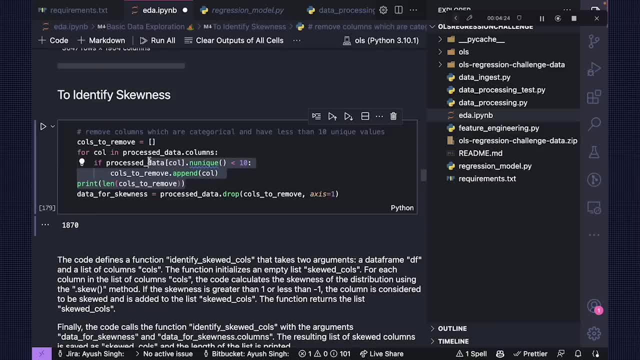 are categorical because they are of course, cute, right, they are of course at one side or another side, so we don't want to touch them because they're categorical. so we separate the categorical values, how what we do we simply say call story move, we simply make a list and then we iterate through. 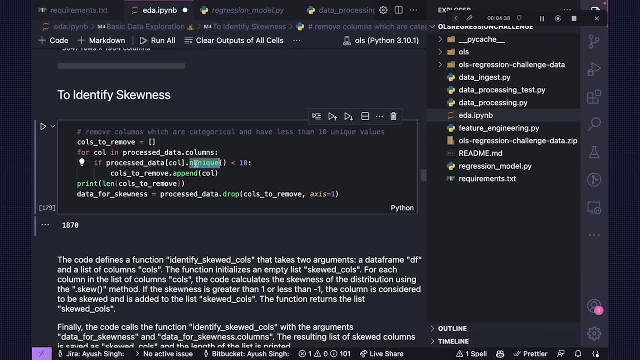 our data columns and then we say: what is the number of between in that particular column? we say if the unique number of values in that, in that column, is less than 10, which means they're categorical. however, there is only two, two unique values if they're categorical. but still, i for a 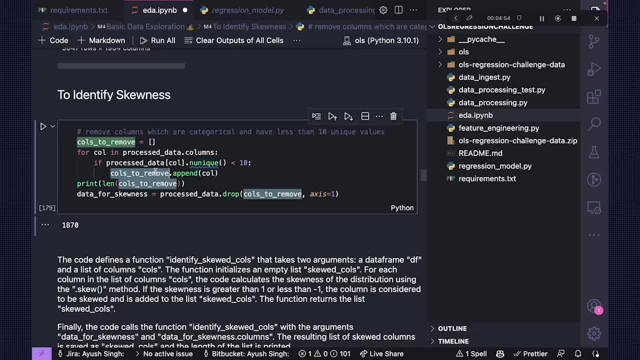 safe journey. i just added 10 and then i added cost to append. now i'm just using that list to drop that. so there is 1870 columns which we are going to going to drop because they're categorical columns. that's a nice strategy. you might have other strategies to remove the categorical. 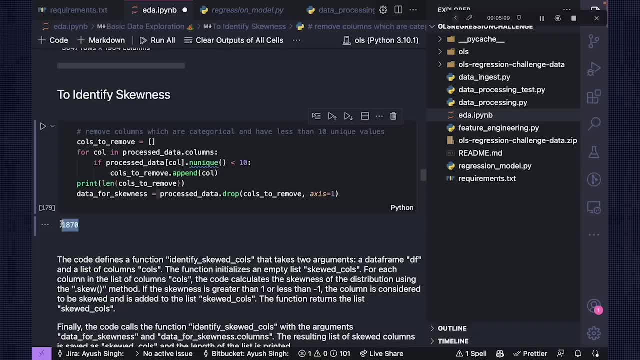 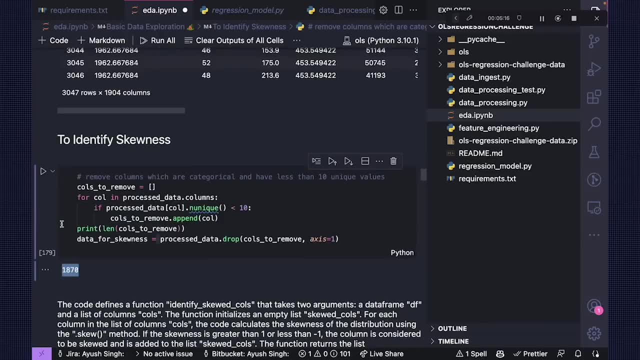 column, because now they are not catech, now they're not string type or object type, they're numerical to numerical types data. but make sure that you don't apply the basic processing like remove one single values of few unique values. don't apply that because you have to know that this is the 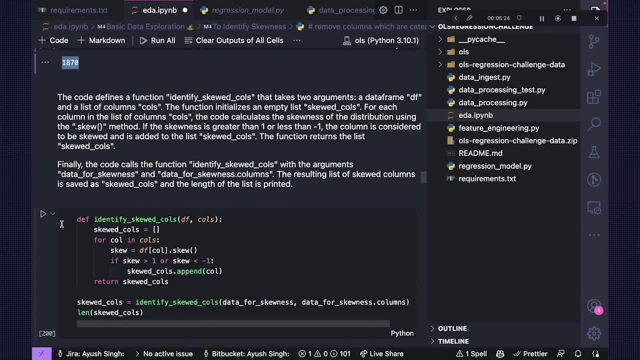 categorical data. right, that's for numeric, not for categorical. now, over here, the code defines, as you can see, that uh, over here else. now what we do. now what we do: we identify the skewed columns. as i said, now we have the normal, normal, normal distributor. now we identify the skewed columns. 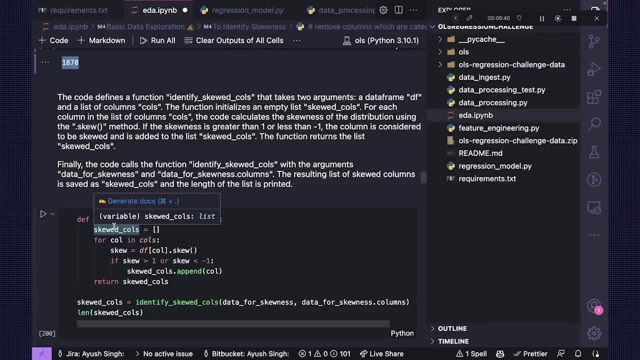 so whenever you try to solve for outlier detection, i i did recommend you do a couple of things. is normal, normal distributed data and skewed data right? so there are different, different distributions, which i might start it right by normal, uniform, etc. i suggest to to take out to. 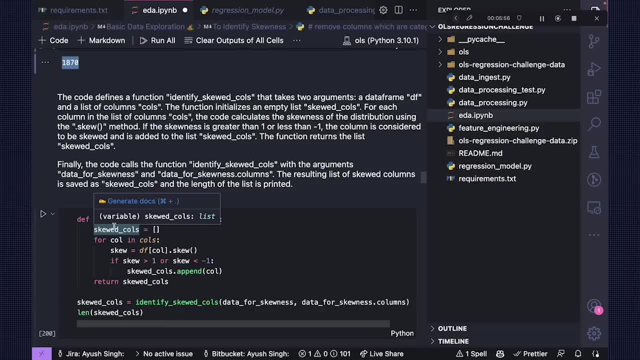 to research on that. okay, this is the distribution. this is distribution of my data. what outlier detection techniques which i can apply to that? so currently i have to use a skewed data. i have to use a skewed data, skewed distribution and skewed you might have it shifted positively, or 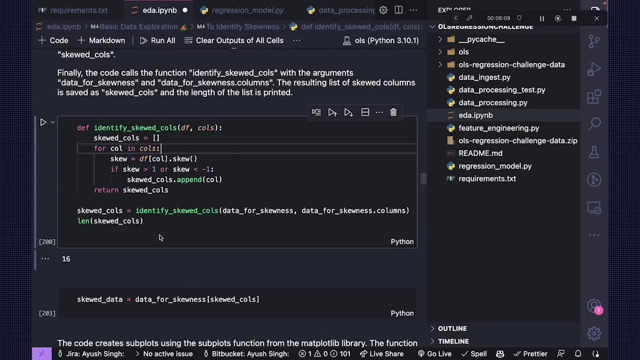 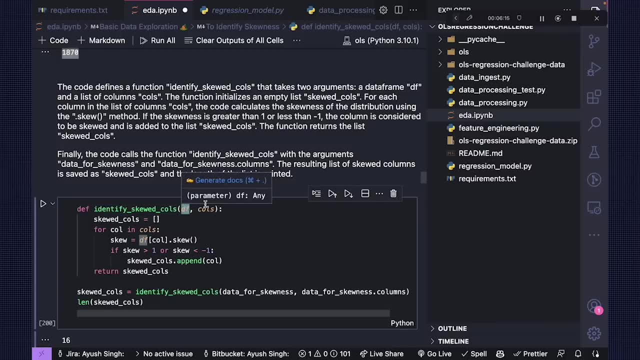 negatively anyway. right so we identify that, that sort of data, and then what we do? we simply say we remove the data and then we combine all these values. right so, for example, over here, what we have over here, we have a function that takes in the process, curve, process, data frame and then the. 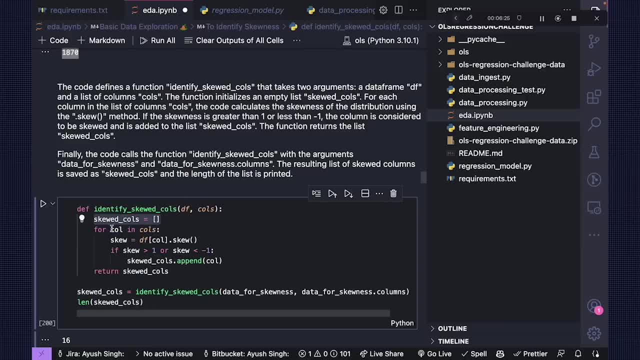 columns. so what does that? columns from columns means the columns in the data, right, so call our columns in there. that's it. we just we maybe we make a list and then we iterate through columns. we take out dots cube using dot skew method. we just take out the, the skewness score, and if that 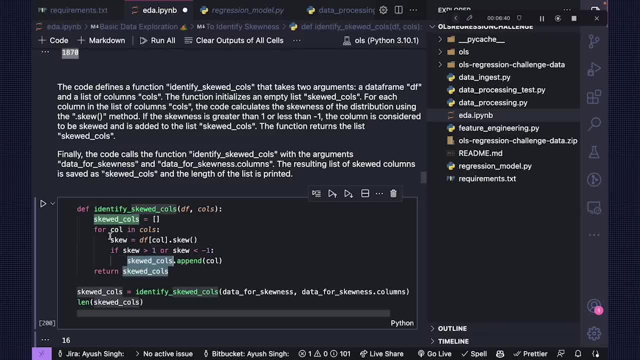 skewness score is greater than one, or if that school score is negative one, then we append that that particular column in that skewed calls and if there's, and if there, and if that does not pass this condition, then we don't depend right um. so you might have questions like how, how exactly? 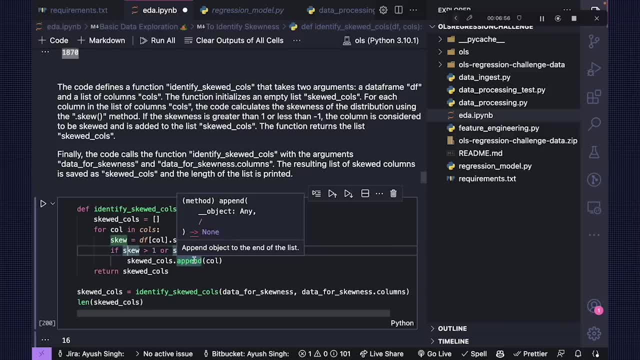 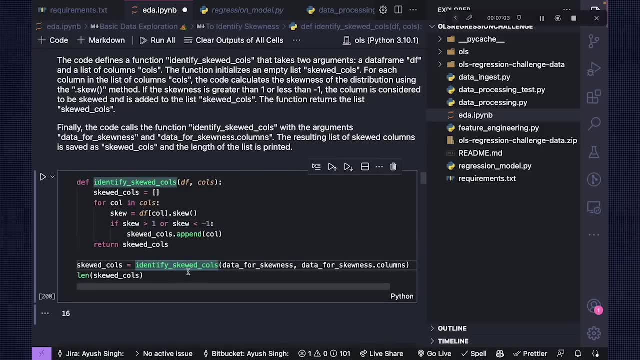 skewness and all, all works. i did recommend to see out the reading materials which have, which we have released for you. please see that that's the best thing which you can do right now, and then you can simply run this one: identify skewed columns, giving the data for skewness and the data for skewness. 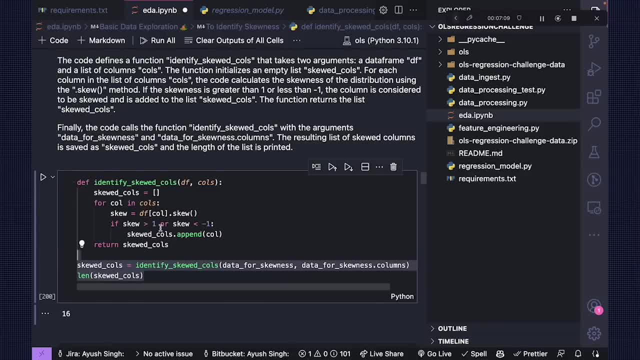 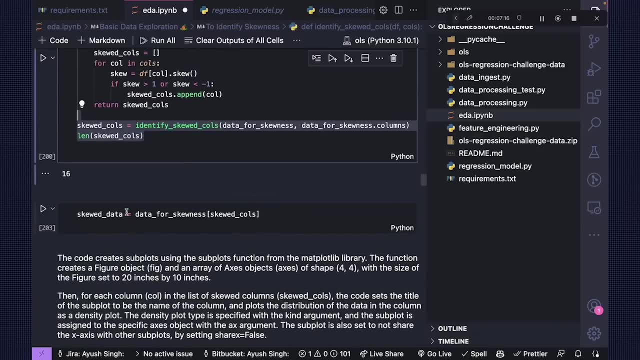 columns and you have total number, 16 columns, 16 columns which are skewed data, right? and then what you do? you simply, uh, you simply make it just like you created the gaussian data. you create the skewed data. and then what you do? you simply create the to see the distribution. so, over here, you see over. 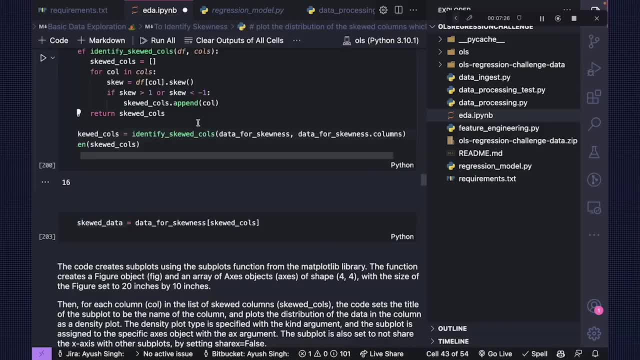 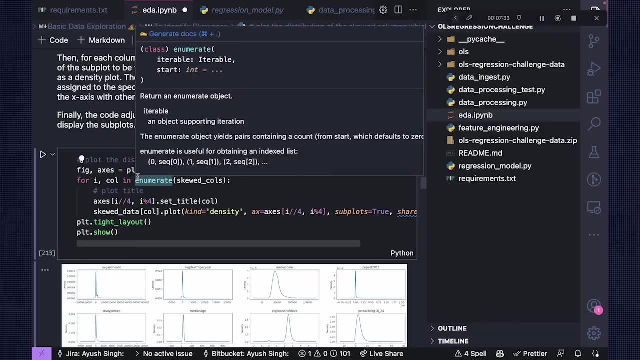 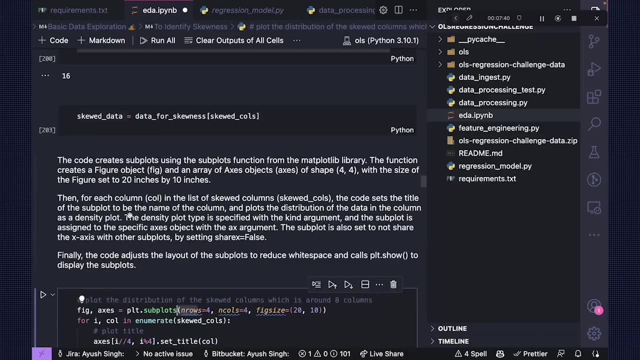 here you sub plotted it where we said we, where we have, i think, four, sixteen and way columns, so you have to sub plot 16, right? so what we do four by four, sixteen, so we can have four by four plots to put the to, to, to plot every 16 variables, which you can see, and I've written the explanation of the code. 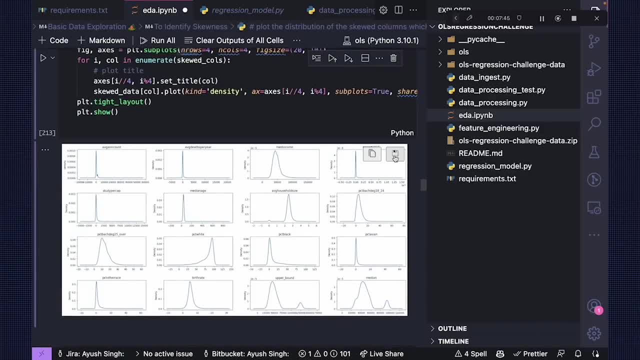 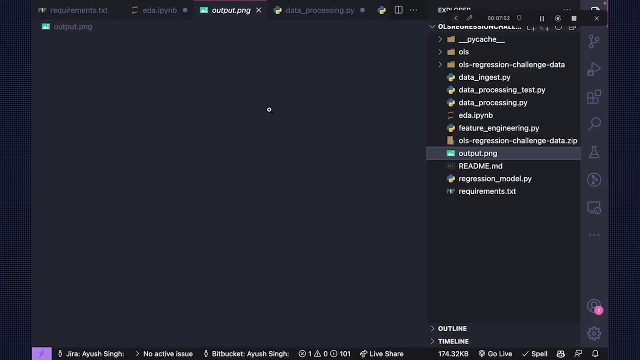 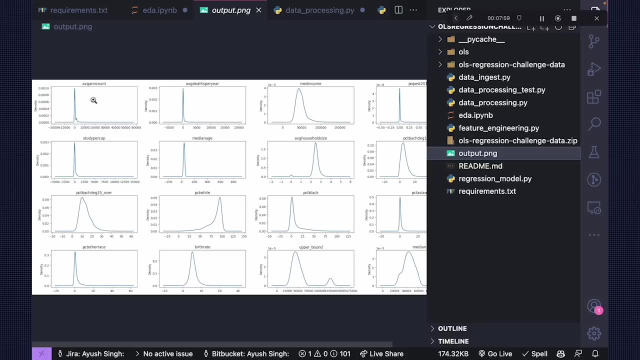 for the same. please see that which you can see. now. if you just, if you just maintain it, let me just say, plot image output, open it please. yeah, so first of all see this. first of all see this: this is the distribution of average n and count. this is the distribution of average that, so you. 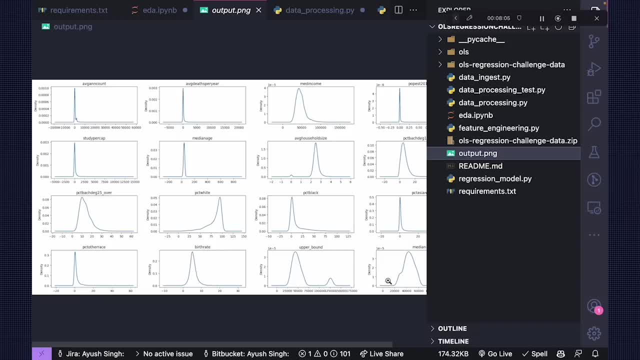 have one, two, three, four, four columns: one, two, three, four, four rows and you have all the 16 variables which you had now. now you can see that they are, they are a distant, they are, you know, they are skewed data which you can see over here, but positively, negatively, and you can see there couldn't. 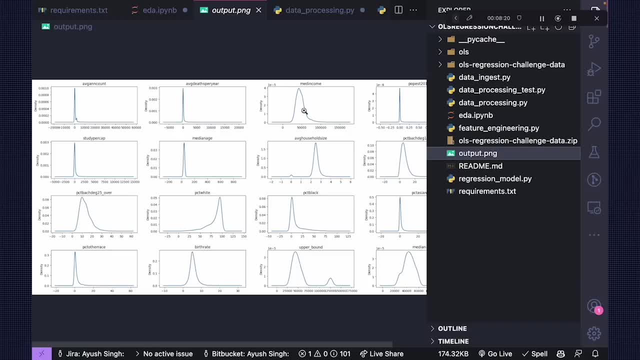 be. this is negatively, this is positively. this is: this is slightly positively, sorry, negatively, I'm sorry. I think I did wrong. this is slightly positively and this is positively so – positively, and you can actually see that we have positive and negative. if it is going from this side, then 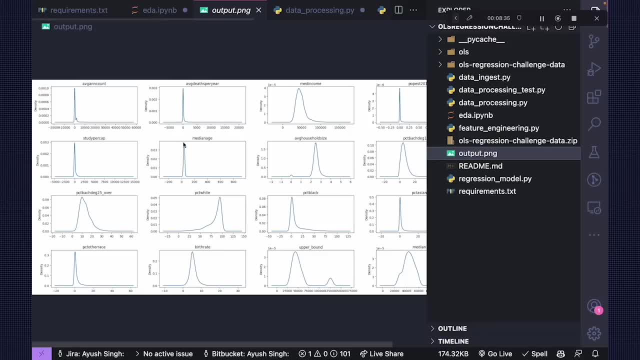 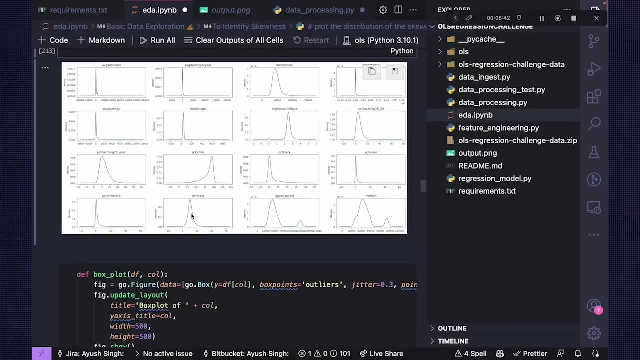 this. if this is going to this side, this is positive. right, so, and then you tight layout so that it adjusts auto automatically, and then I'll show it. now you can see that you're confirmed. okay, these, these, these semicolons just skewed. and then what you do? you simply box plot so that you see that if they did, they do. 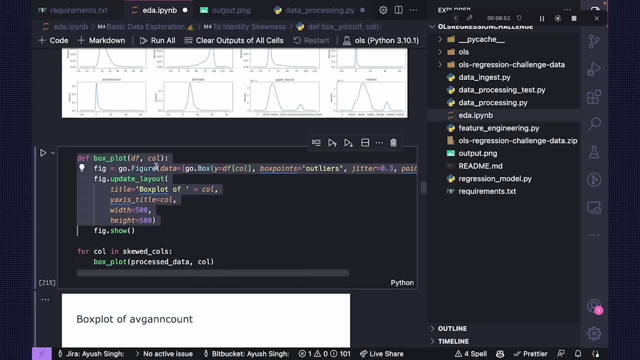 have outliers by using this particular code where you're saying figure video giving the column and the box points outliers, and then your title is box plot: what- what was the number of a column strip to be added? and then you say key go to, and then you apply this function to each and every variable. for that: 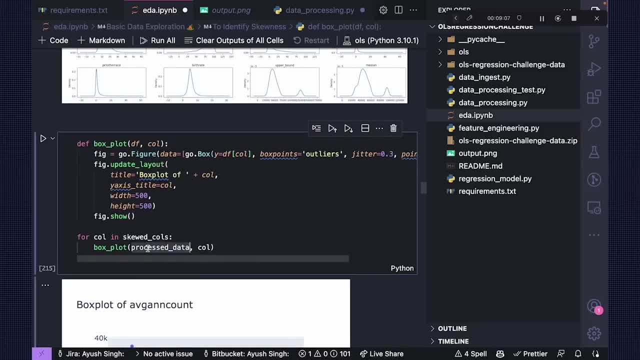 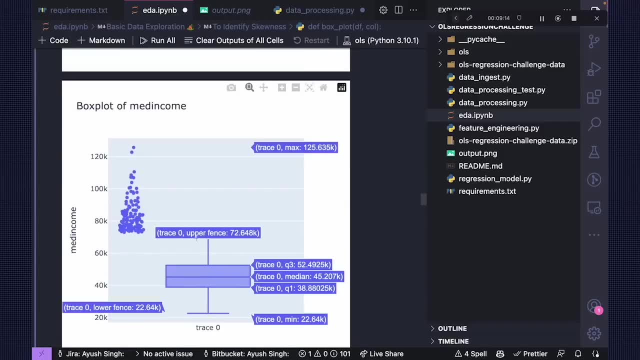 particular data for skin skewed columns, and then a column and then skewed columns, where you have this cute data, and here you can see that, though, OMG, we do have this cute, we do have outliers, so you can see maximum. and then these are the information which are of outside the way, and this is you can see outside the 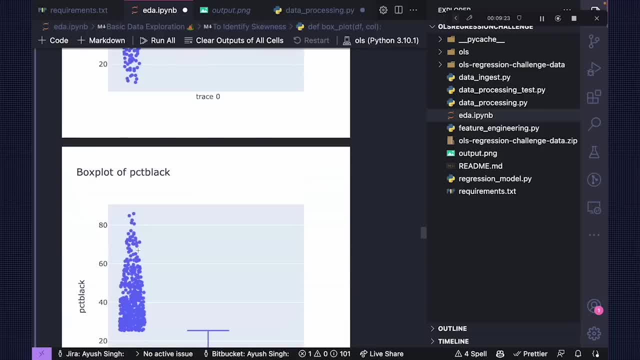 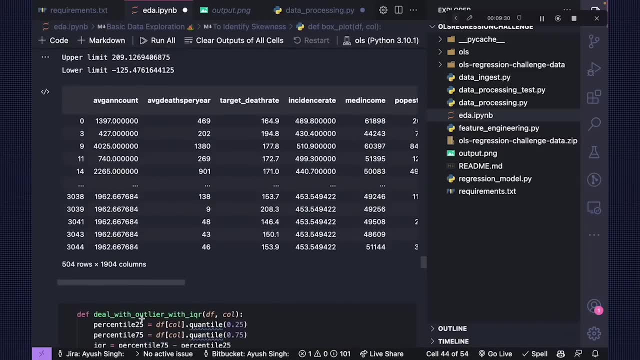 way right, and we have seen the interpretation of the box plots as well. now you can actually see that this is also the outside, the way, these are the variables, etc. so we have this now. how can we deal with this? know what? what we can do? let's take a particular column. 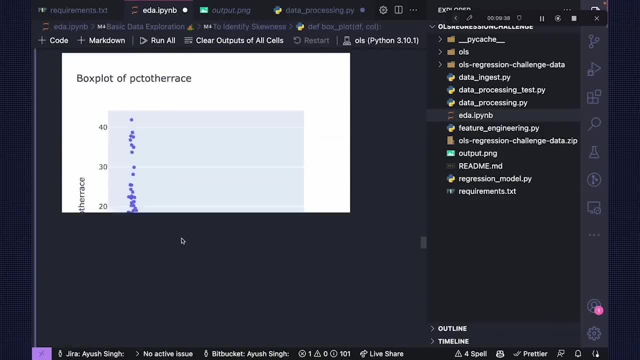 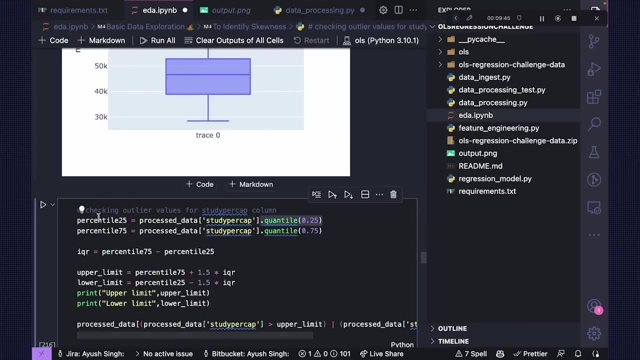 from this. let's take a particular column. I'm going to take this cute column which is, for an example, as of now, study recap, and then we take out the quantile range, 25th percentile, the 25th percentile, and and then we take out 75th percentile. okay, 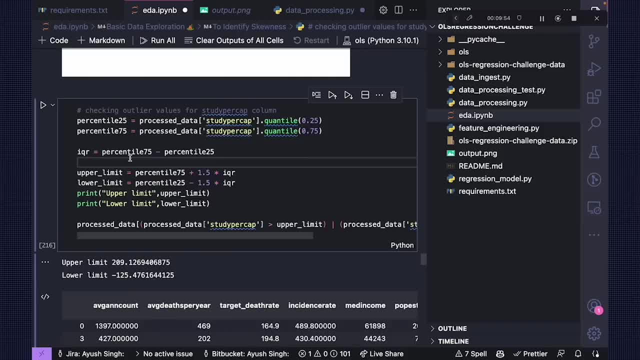 we take a 25th percentile and then we cut, take out so 75th percentile, which is the quarter q1, quartile 1 and quartile 3, and then we take a IQ, are from that okay? and then we have upper limit like: but the maximum value which, which, which, which. 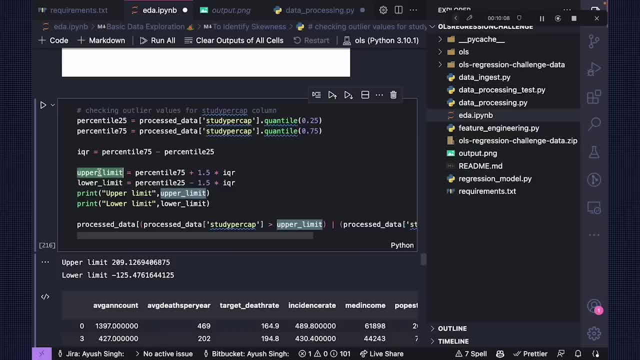 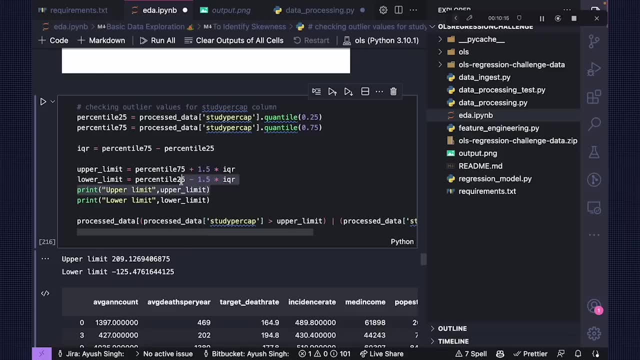 which we should have, and anything goes above this, our outlier and lower limit, which is minimum, and and things. so you can see plus, minus over. here we are multiplying this and it's the strain, strain deviation, or upper limit and lower limit, and then you can simply say the process data, where you have it. there you 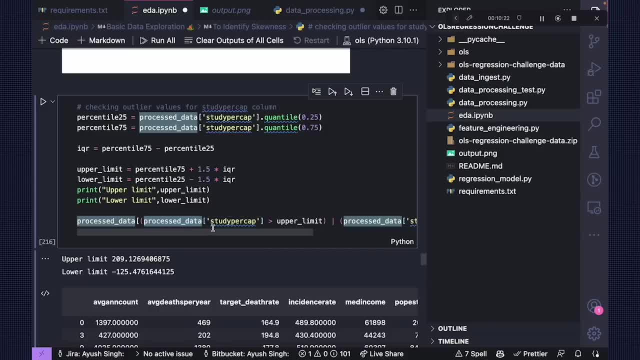 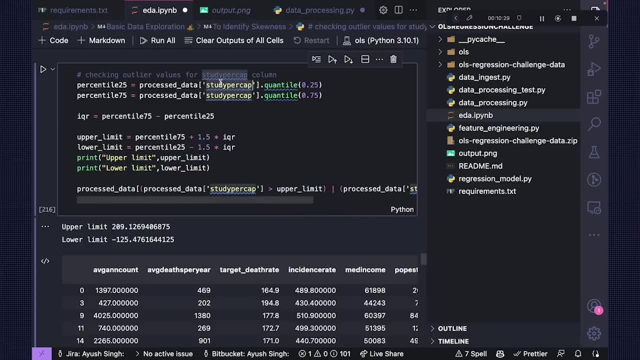 just trim the data out here where you just say: take out the column still which are outlier, which you are seeing our upper limit or there of lower limit. they are below the lower limit. upper limit for this particular column is 209 and lower. limit for upper limit for this particular column is 209 and lower. 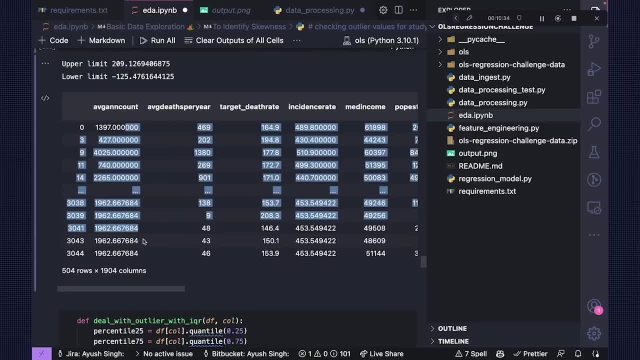 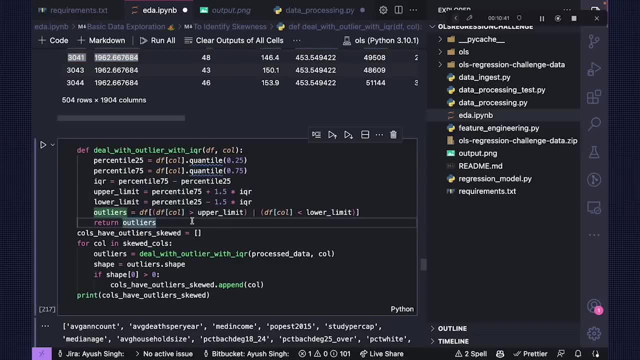 for this is minus one through five, and these are the columns which you 504 rows in that particular column has outliers, and then you simply uh, and then simply apply this, and then you simply apply this column where, where we just had listed this particular, all the code in two of sorts of the 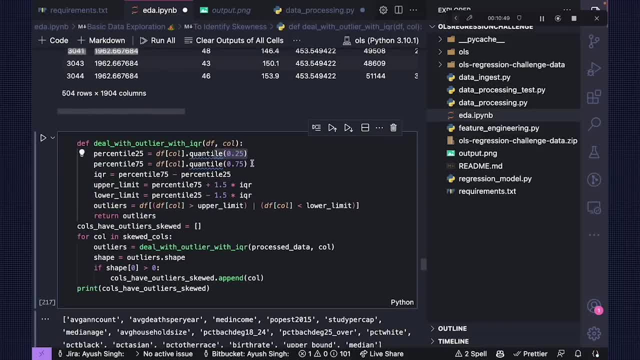 function, a define and column for that particular column is checking the quantiles q1, q3, iqr, and then upper limit, lower limit, and then, and then taking out that and then what you, what you're doing, you're iterating through all columns and then applying this function on that, giving the 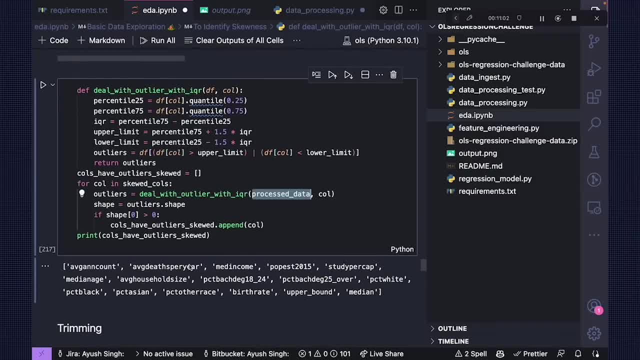 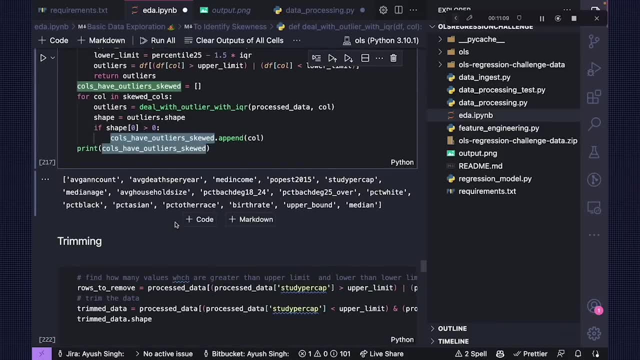 process data and that particular column, and then you simply have the account. then you simply have the columns which has the outliers right now. now you have the columns which has the outliers, so you have 1, 2, 3, 4, 5, 6, 7, 8, 9, 10, 11, 12, 13, 14, 15, 16- all 16 variables have their outliers. so what we, what? 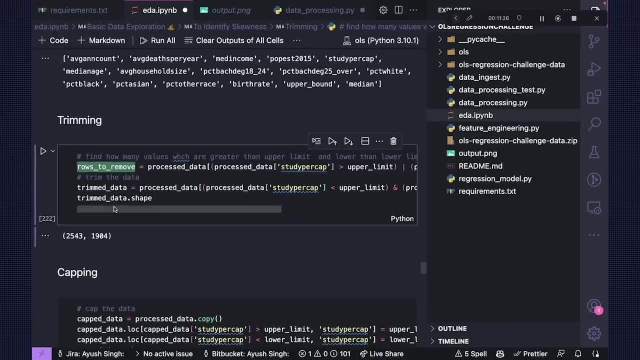 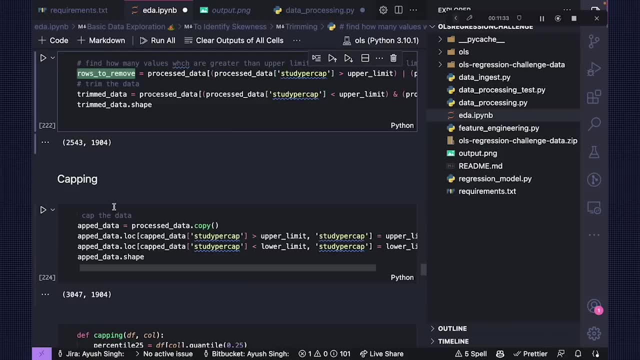 we do. first of all, we take out trimming. there's two approaches. we have to talk trimming and capping. trimming, removing, capping, means um, updating, updating my uh values, like you know what, what, what values, updating my outliers with the maximum on and the minimum right. so if that a maximum, then we if, if, if, if the values. 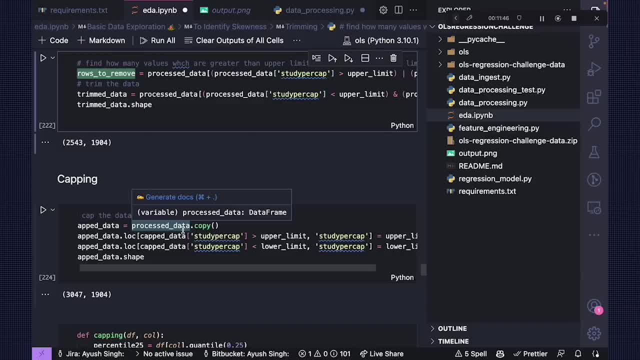 above the maximum, then we update that with maximum. if the values are lower than minimum, then we update that with a minimum. you might be clear if you have seen the previous lecture, otherwise i'm not going to repeat once and once again, right? so, uh, going to this code on trimming. we first of all: 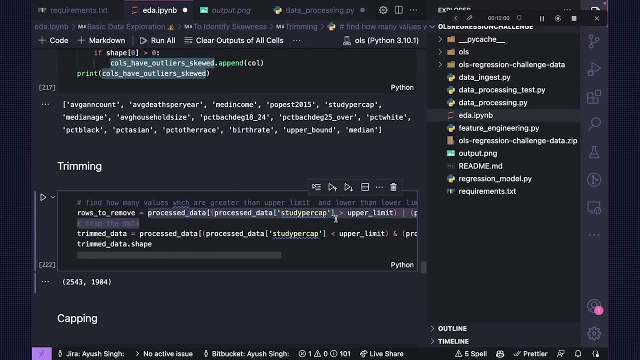 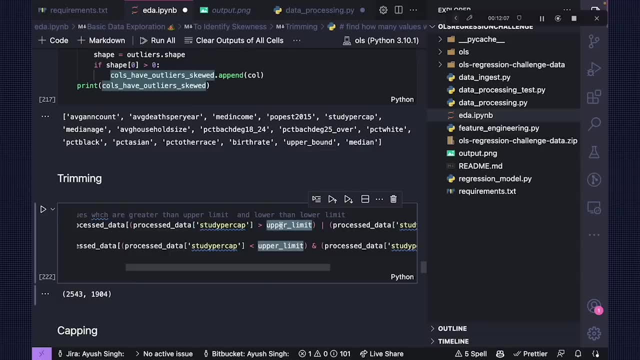 identify what rows to remove. and that's going to be done by this data wrangling or the data extraction, where you're saying, in that particular column, in that particular column, if that is, uh, that if that is greater than lower up upper limit and if that is smaller than lower limit, then these are the rows to remove, and then 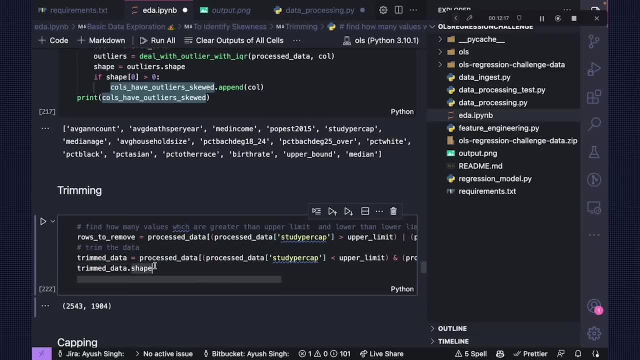 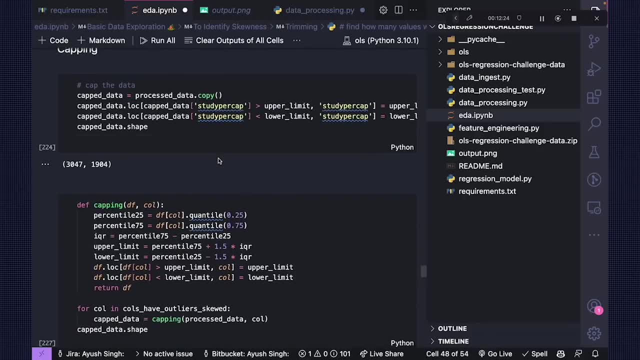 this is a trimmed data where we actually- this is where we actually talk- then trim our whole data and over here we are capping it, here we are capping it out there and and over here what. this is just an example as of now, just to showcase: we'll convert the. 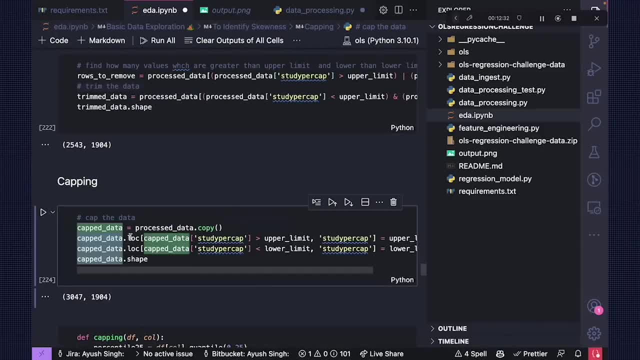 to a function right now and then we simply lock loc to identify the rows. and then we identify the rows where your upper limit, uh, for that particular column, right for that particular column, for that the the upper up, any, any value in that particular column is greater than upper limit. update that. 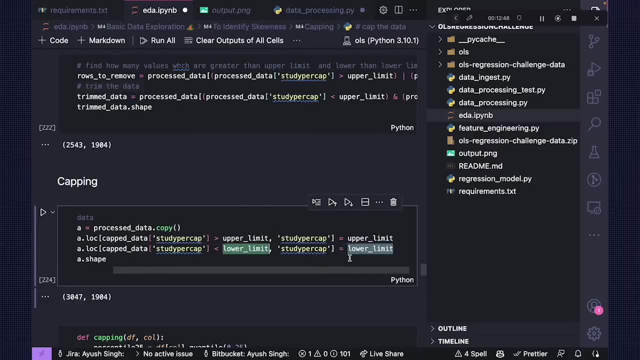 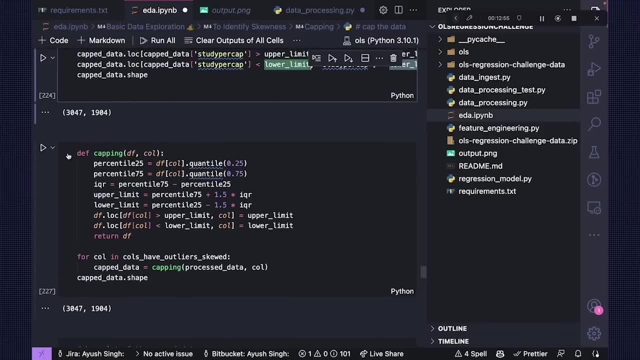 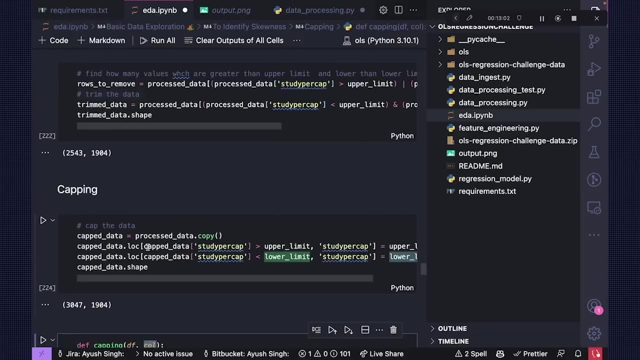 with upper limit and any value below that lower limit. update that with lower limit, which is the minimum value. you see that your data is maintained. the same, but over here your data is trimmed, capping. capping means, um, you see over here again the same thing. you have converted the code to see over here and over here. 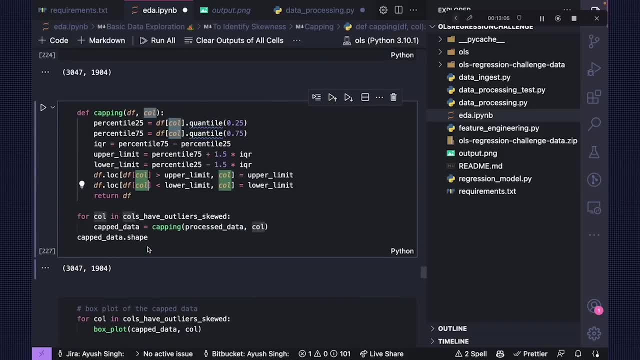 we will. cap will not remove cap. by removing we lose whole chunk, a whole lot of information. that's why we are capping it over here and now you can see we are simply say: go to the particular column, sorry, row in that particular column if that is greater than upper limit. 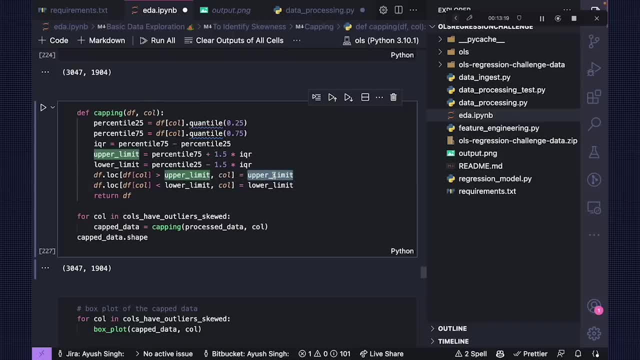 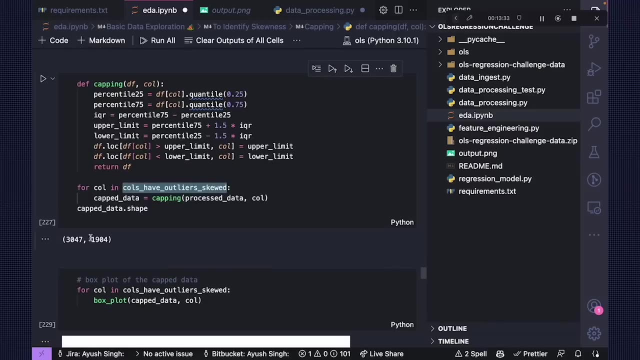 for that particular column, update that with upper limit and if there is more than lower limit, update that with lower limit limit. okay, i hope that that you're getting, and then we apply this capping this on every, every variables. we have outliers, and then we see that we have the data without trimming. 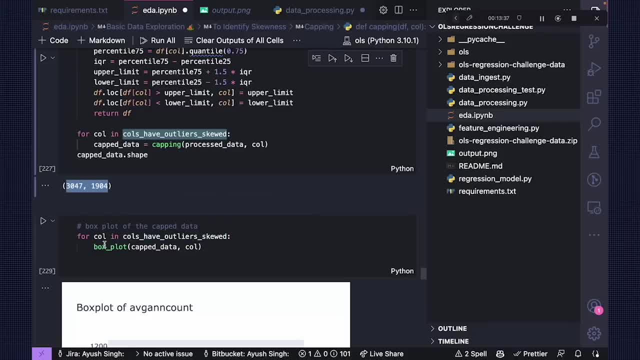 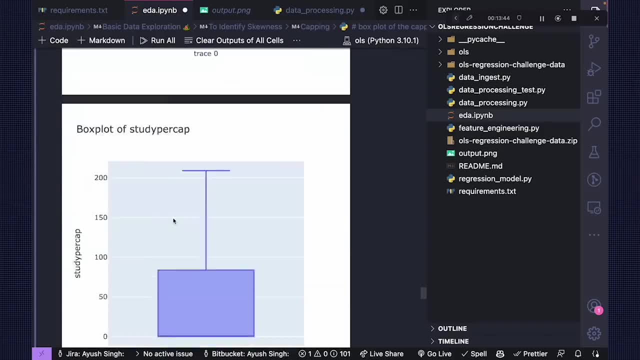 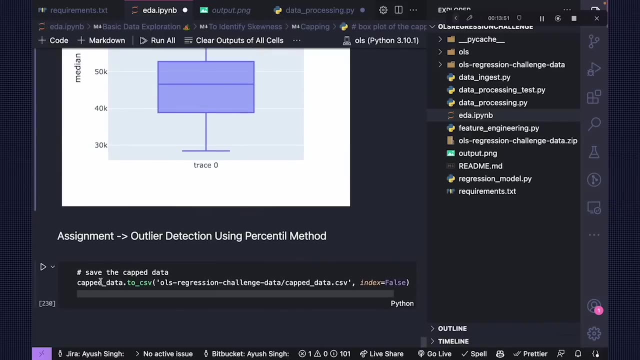 we are just going to cap it. and then you can now box plot on cap data. now your cap data has that. now, if you box plot on that for every columns now you see there there are no outliers, and that's right, you want it, you want the challenge, i hope that you get it. and then we say: now we have, we. 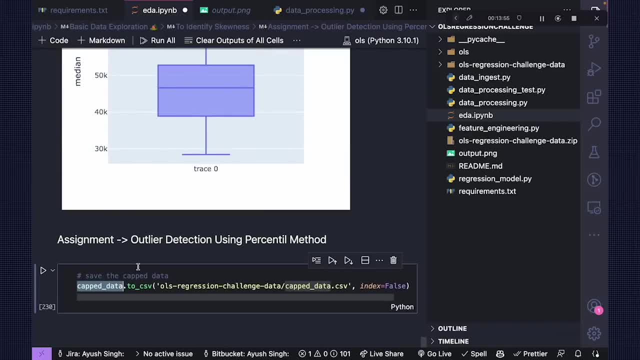 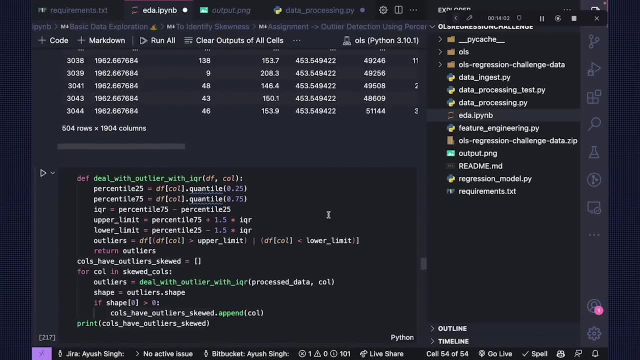 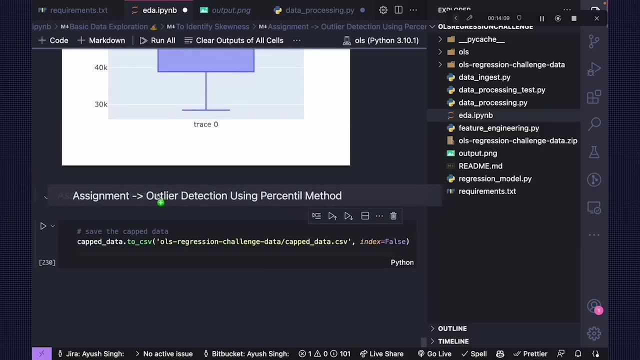 are going to use the cap data only. we are not going to use something, then we save our cap the data into something else. okay, i hope that you. i hope that you go at one point. there is one assignment related to it. there are a lot, lots of things to try out. you can actually try out outline detection using percentile. 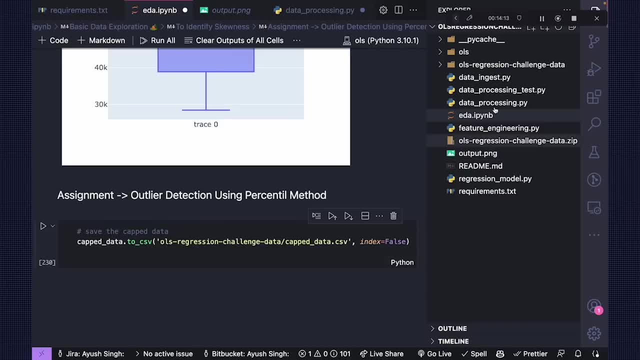 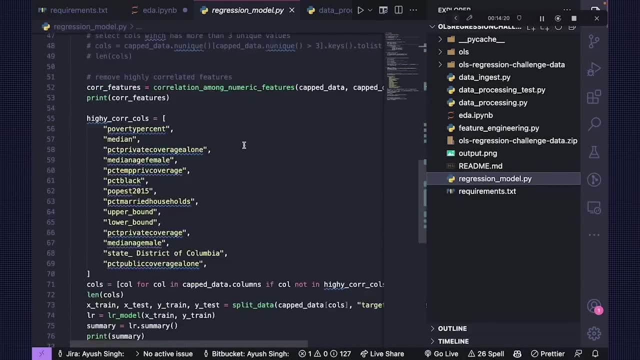 method. that's your thing. now i think we are mostly done with the outline reduction on regression model. on on regression model: uh, let's talk about uh in the, in the next set of videos around a regression model, and then we'll actually talk about that in great detail. let's, let's go in. 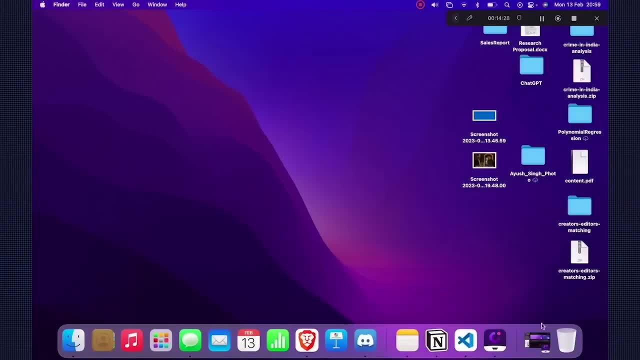 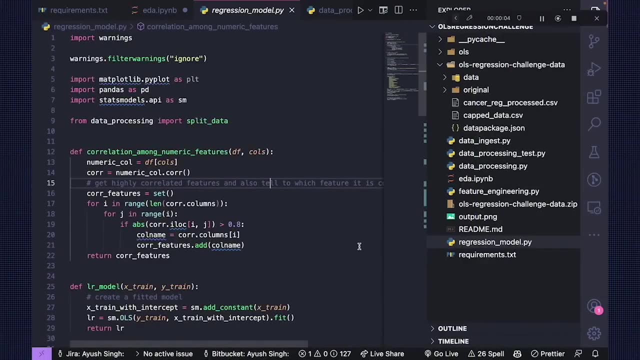 the further video and let's talk about that. okay, cool, uh, so we'll. uh, now we'll come to. now we have done with the data data part, and my whole point from this project is to tell you about data stuff. now we'll just go and quickly review, because 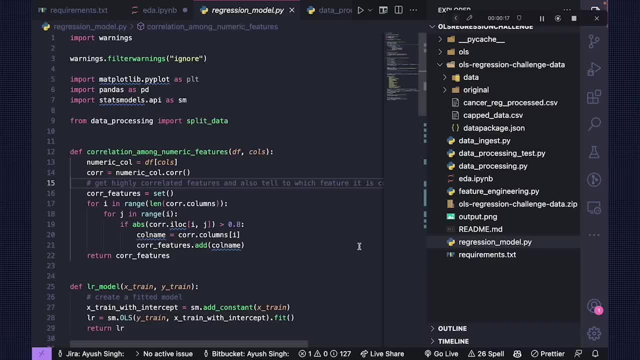 we have already talked a lot on you know how to build regression model and all, and that's not my point on talking in this project. my point was different: to teach you several techniques, feature engineering, collection and all techniques to actually go forward with it now, uh, what? now what we'll do? we'll try to model it very basic, you know, just to let you know you. 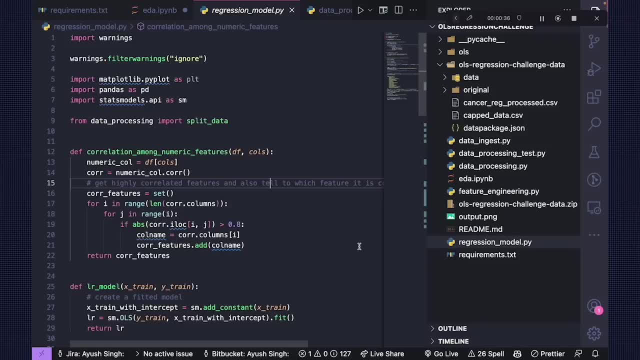 know we have already tried it out, and then now it's now in the assignment you will be given to model it accordingly. so i'm just just going to give you a very small baseline and it's an assignment. you'll actually further update this uh stuff now which which you're seeing, 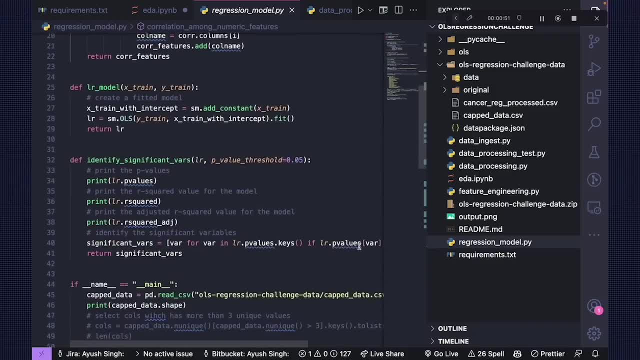 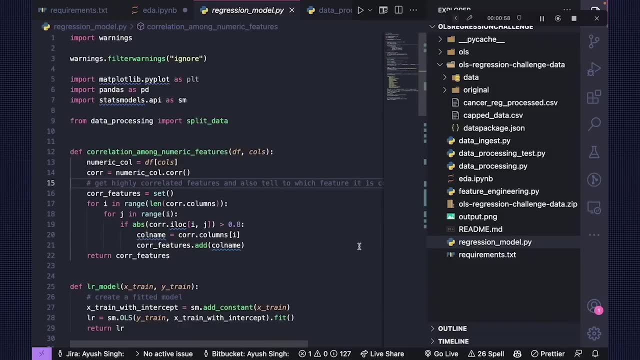 in front of me is: we have the first function, but ignore all, all of that. let's go to the, let's go to over here. so what? what i did? instead of classes or everything, i just created a functions. right, i just created functions so that it is easy for you to understand. but 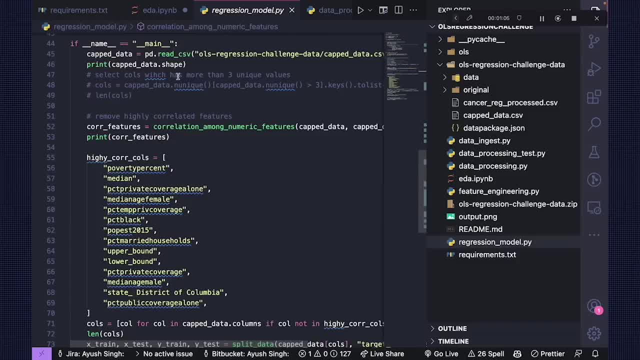 but usually i will suggest you to work with classes. first of all, we are importing our cap data from the cap data which we saved, so you can actually use the df.2 csv and give that particular path. you'll be saving that, your file, and then, if you, 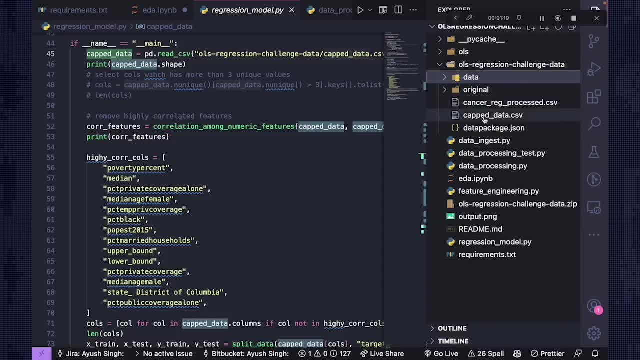 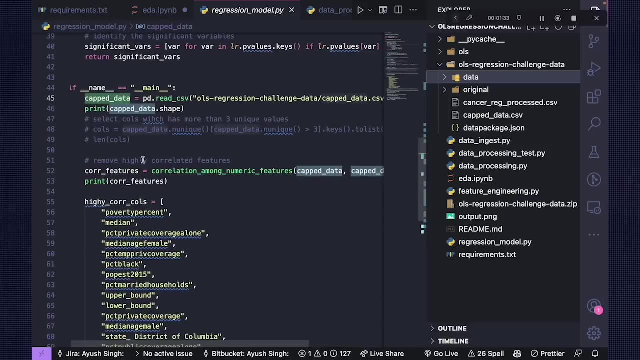 go to the data data folder. you have a cap data over there and cap data is where your, where you have built, dealt with, you know missing values and everything out there, outliers and everything. uh, what you will do is you simply uh, first, is you have this particular thing where you have? 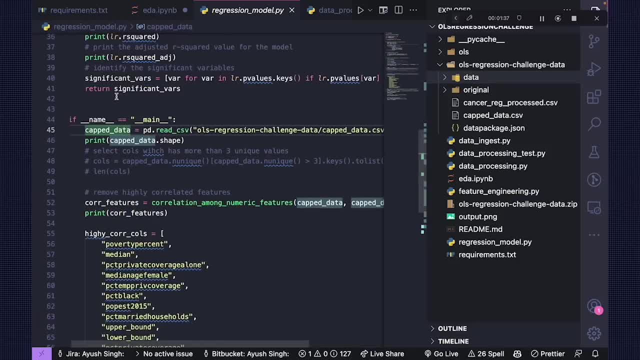 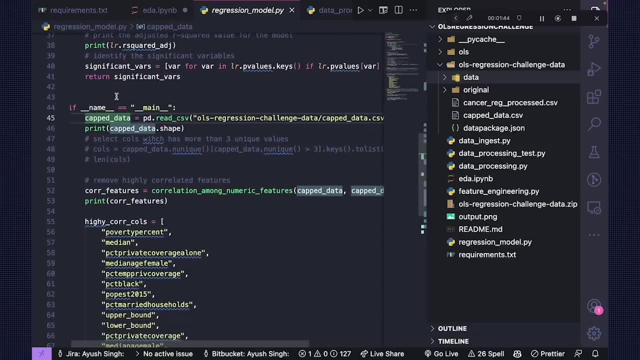 the correlation, first of all, you have the, read it, and then you, and then the second thing which i, which i really like to do, is identify the correlation among numeric features, identify the correlation among numeric features and then, right, right now, it is, it it has, you know, 1900 columns. 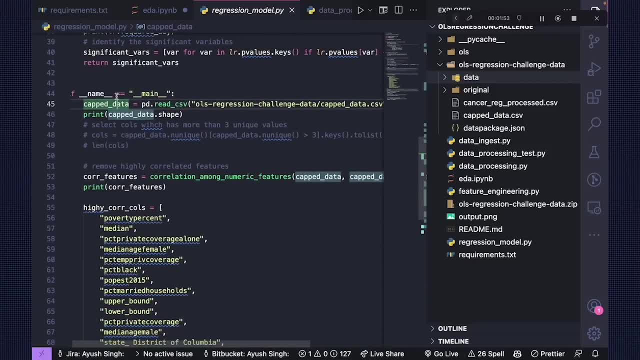 and it will take so much of time. and the reason why i want to identify the numeric correlation, because there is one assumption which you have saw, that the code, they should not be correlated too much. if they're correlated, then they're not providing any sort of information to the output variable. 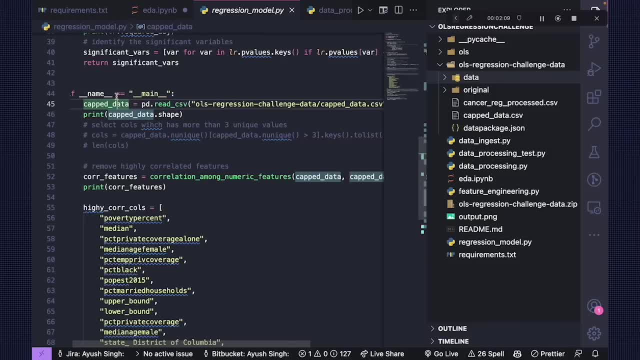 and when i apply my correlation techniques, when i when i apply my correlation techniques and and not have in- not in every process you have to do. you have to do this in exploratory data analysis part, where you're understanding the correlation between variables. this should be done in an eda part. right, i'm doing it right now because i think it's much for me. i think, as 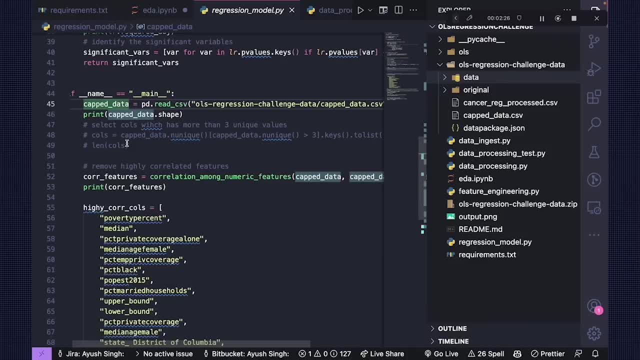 often. i've just added, added over there, just to make sure that we are on a page right, like: why to öz, when we give up co2, when we give up kplT in g for us world data, the things I want five. we are using this, we are using just to know that we we can ignore our highly correlated correlation. 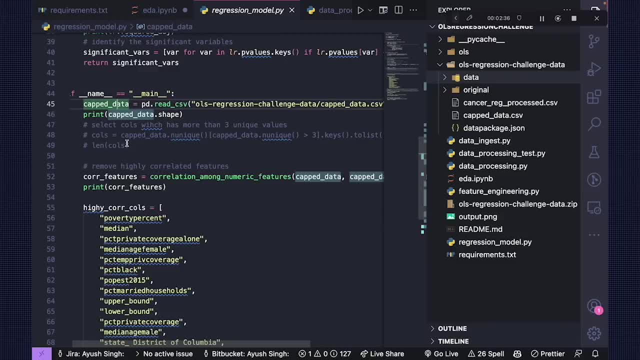 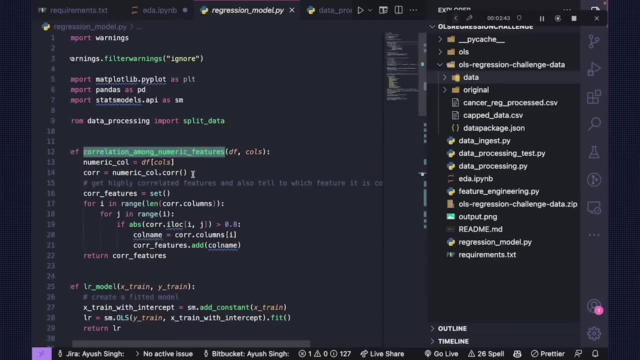 coefficient and then see our result right. so i just added over there for a, for a, for a sake of learning, but this is a part of your eda um. so you have a correlation among numeric features where you're going to the, where you're given the data frame and the columns of the data frame, and then 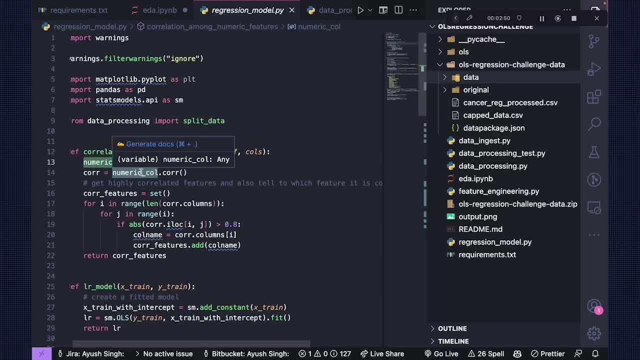 in numeric column. you select all the columns, your numeric, and then, uh to, to be honest, every column is numeric in this right now. and then you take out the correlation it builds a correlation matrix with. we have already talked about correlation. please, we don't want to get it, but i'll tell you. 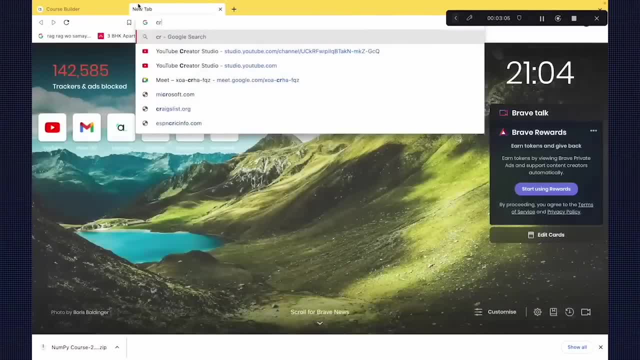 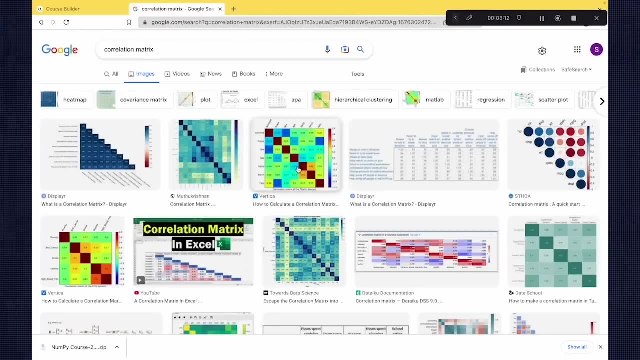 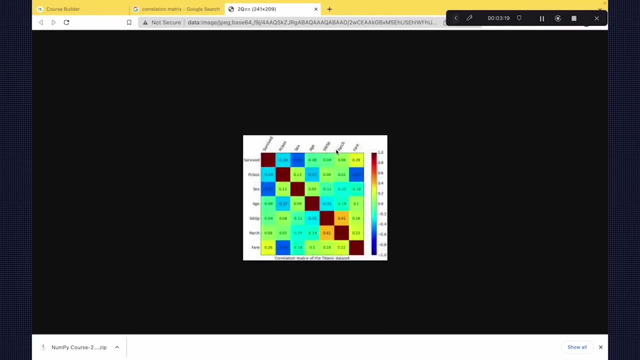 a small uh stuff. so let me, let me just go to correlation matrix and then let's talk about that a bit. so so this is a correlation matrix, so this is a correlation matrix, so i'll just open that in another, another tab. so this is a correlation matrix and in this correlation matrix you have 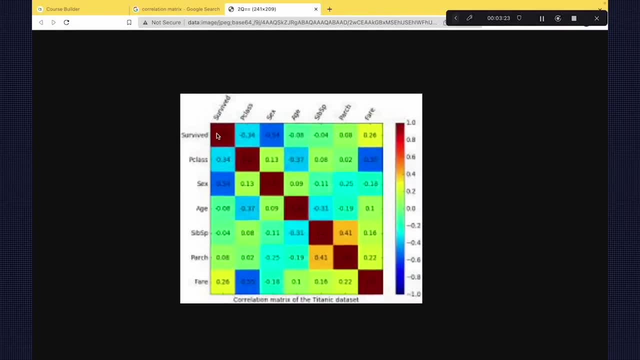 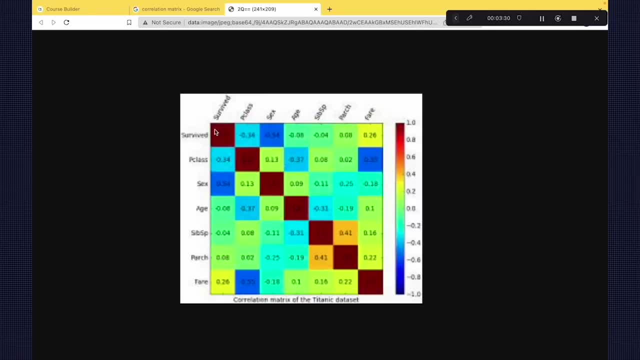 on on over here. on y axis you have the variables. on x axis you also have the variables. they survive. the correlation between the same columns is one. they are highly, highly correlated with each other, but the correlation between surviving p class is negative. the correlation between surviving this variable is this much correlation between surprise. so you have the. 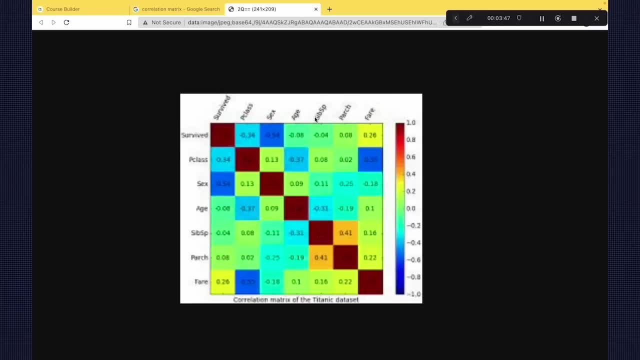 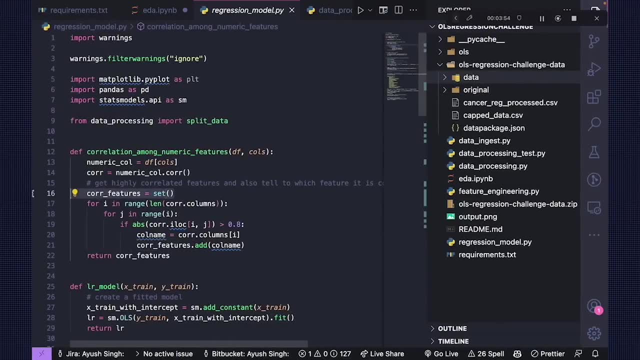 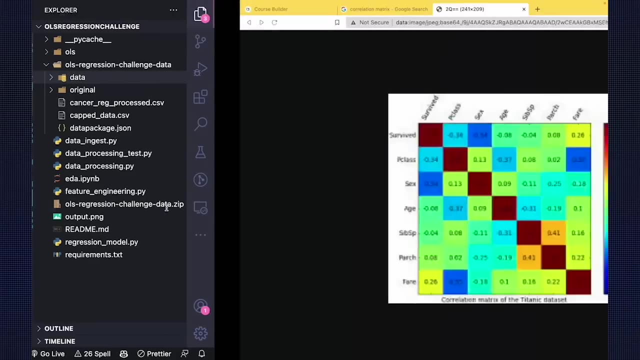 matrix for every, we are taking out the correlation between every variables out there, right? so it goes to, it takes up the correlation, and then it's sick, it, it, it takes it, it has the empty set. and then Then what we are doing, for i in range for that correlation and then we go to j and 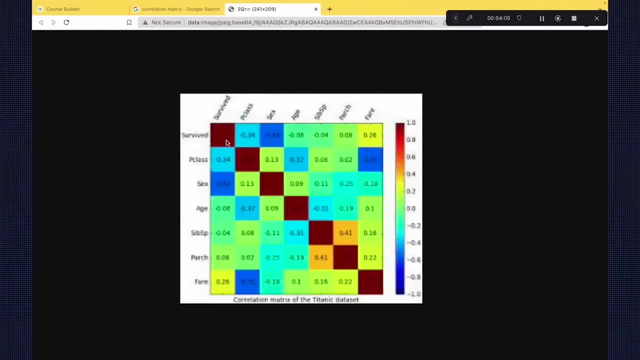 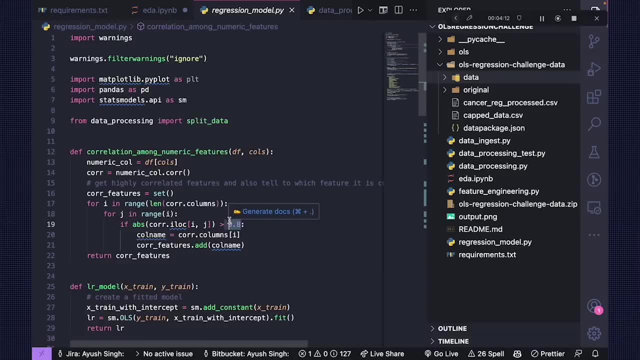 then we are saying: if the correlation of two variables, if the correlation between, for example, survived and p class is greater than 0.8, is 80%, greater than 80%, we simply append that It's highly correlated with each other. 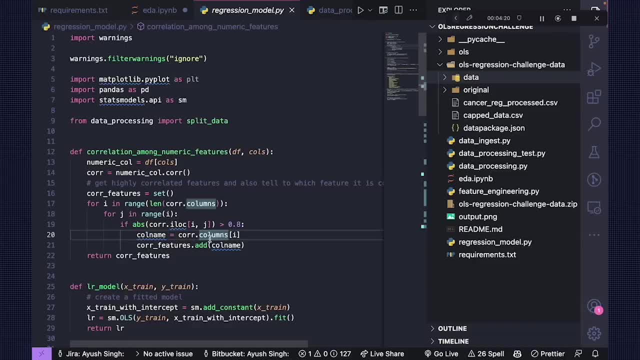 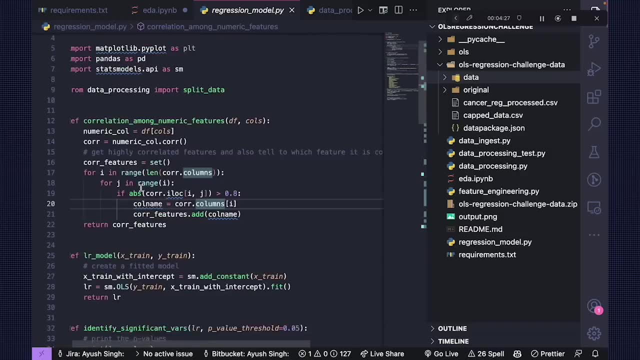 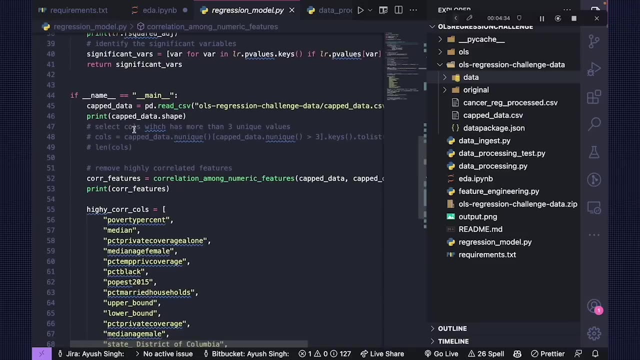 Right, We simply append that. We simply append that column so that we could know that they're highly correlated features. So you're seeing that when I ran that method, when I ran that method by applying this, so basically what you're seeing over here is I had the columns and then over here I had 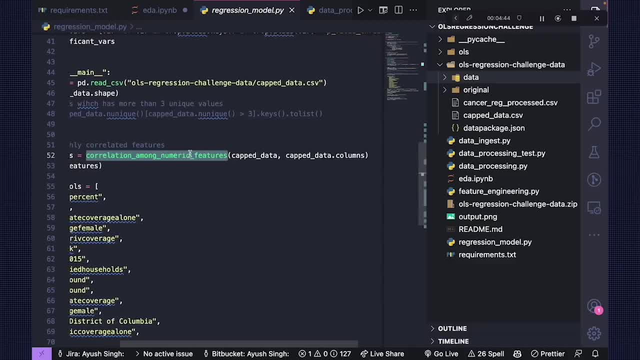 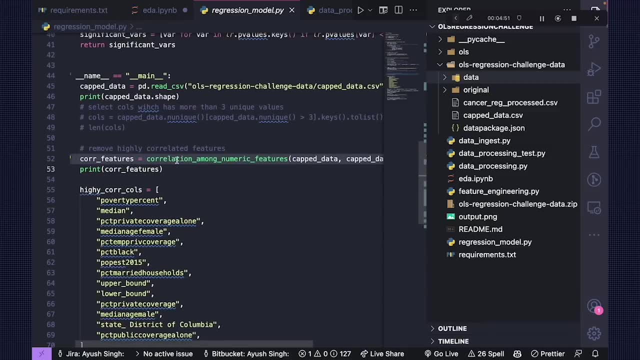 the columns and then over here you can see correlation among numeric features- cap data- and cap data dot columns. So I've just given the cap data and then columns of that cap data And then I was able to take out the correlation features. 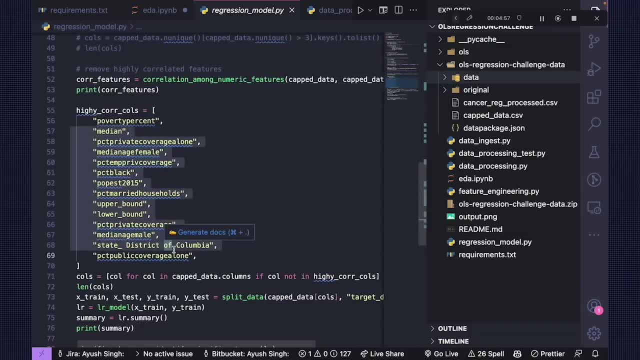 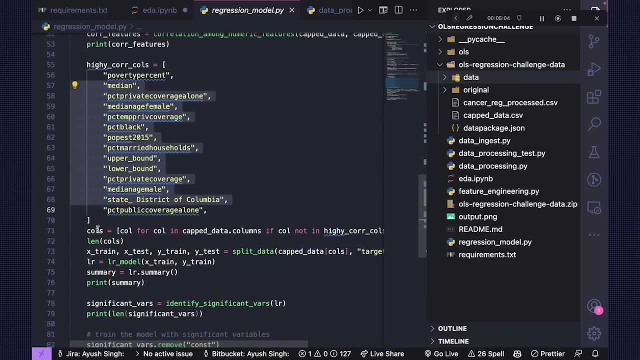 And these were the most highly correlated features among themselves. And now what we can do. we can first of all remove the columns from the data first of all, but I don't really like removing it. So what I'm doing is I'm making a list where I'm telling call for call in cap data dot. 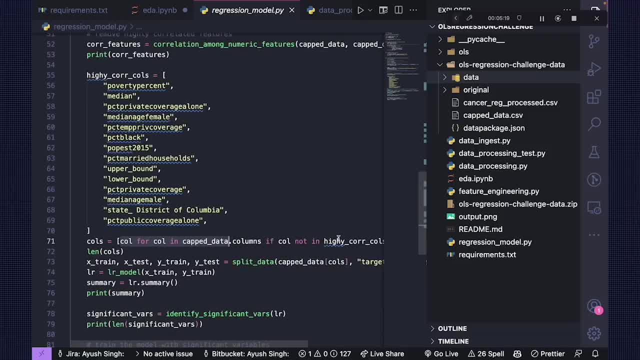 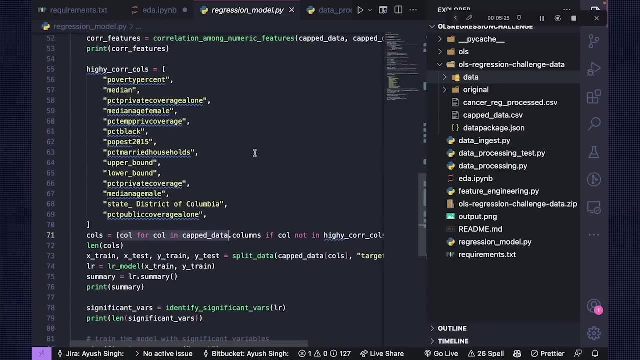 columns if the call is not in highly correlated. So we are just saying: key for every column in your cap data, which is your data, which is for every column. make sure, give me that column names, but also make sure that these are not in these highly correlated if the column is also not in this. 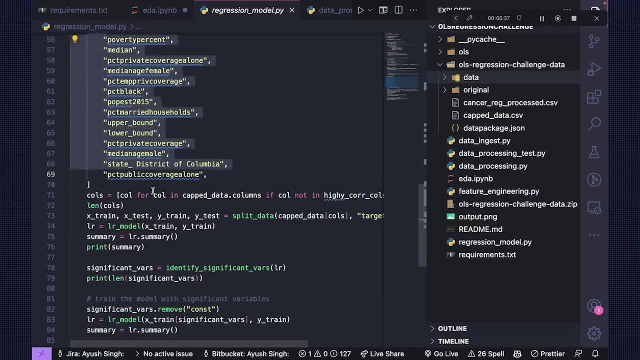 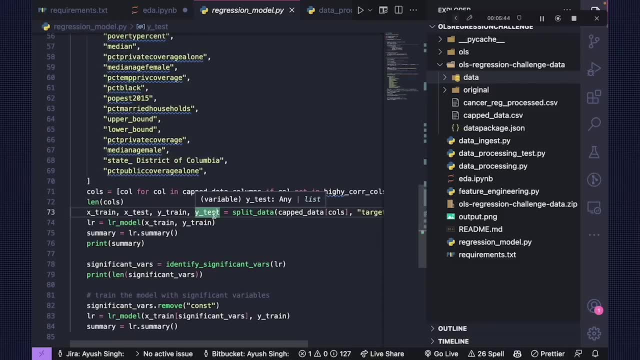 So this is a list comprehension which you might have learned in your Python programming language And, as said, please see the resampling methods for this. I'm not going to explain the single word right now. Please see the resampling method. What we are doing is dividing our data into training and testing. 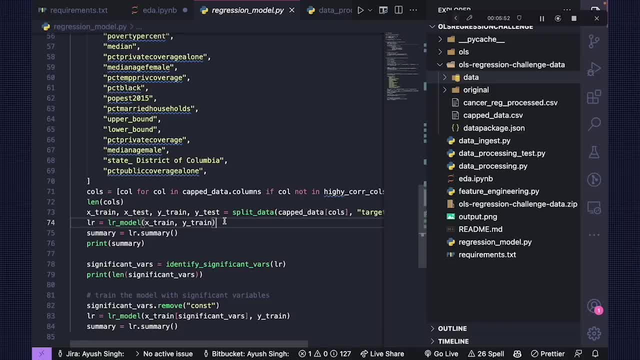 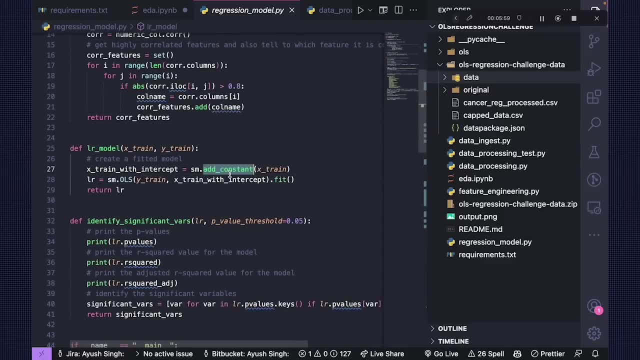 I've already uploaded lectures on resampling. Please go and see that first, before coming to this. Split the data And then we train our model- LR model. I'm not going to go over this. we are adding the constant. Why are we adding the constant? 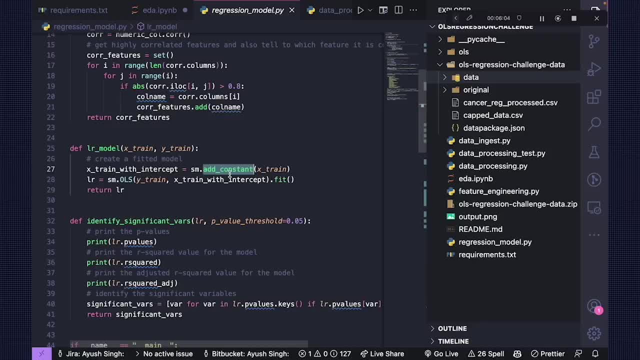 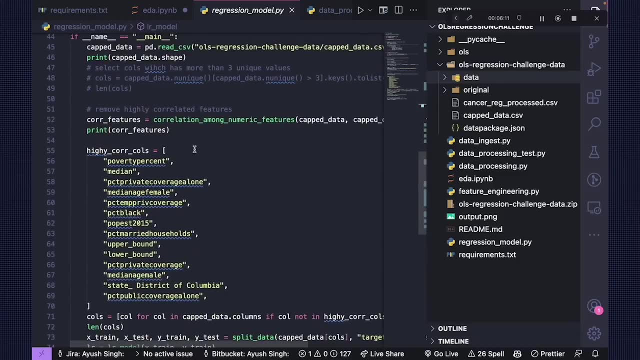 Because we have to multiply with that bias term, that one, you know, x0 is equal to one. So we are adding one to every rows so that whenever b0 multiplies with one, only right, which is the bias term. 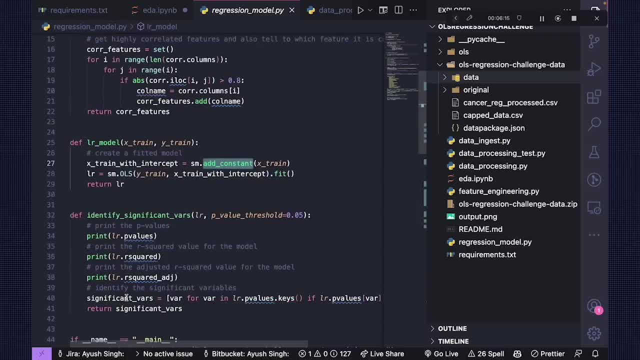 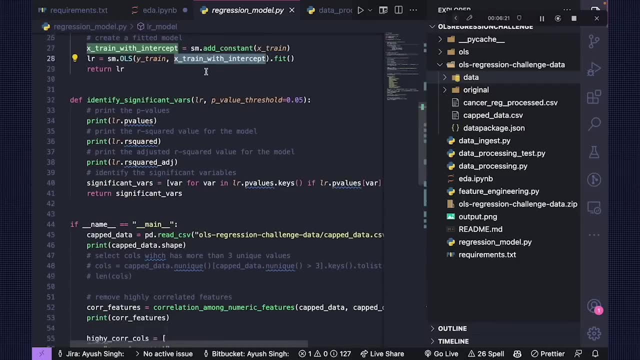 And then we have adding the constant, and then we have LR model. we are training OLS from the stats model API with the y train and x train within intercept, And then we simply take your LR dot summary And then it is printing out the summary. 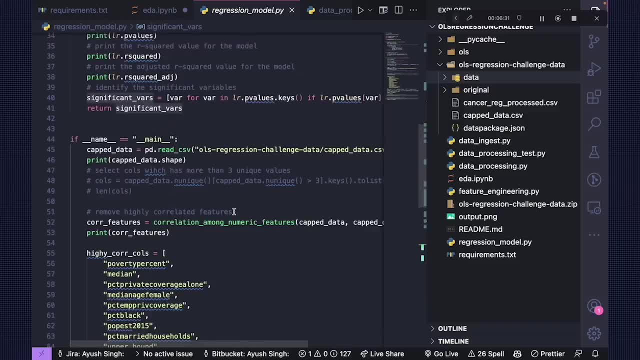 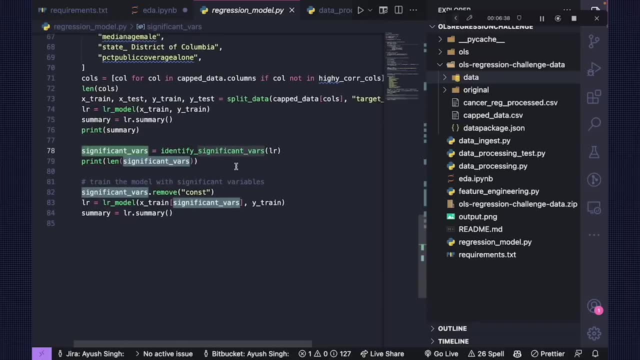 And then you have the same goes for significant variables. So what we are doing, we are identifying the significant variables. So let's talk. let's talk about that, like I'll talk in a bit, but let's run this whatever we have as of now. 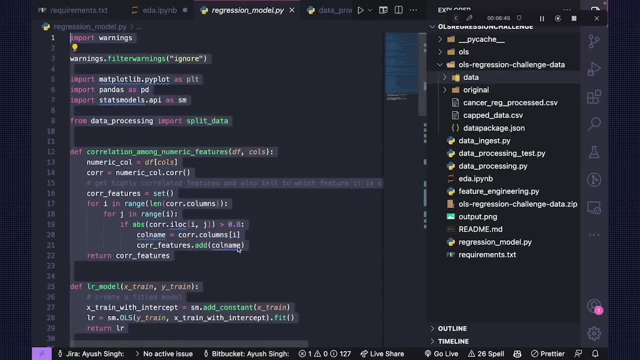 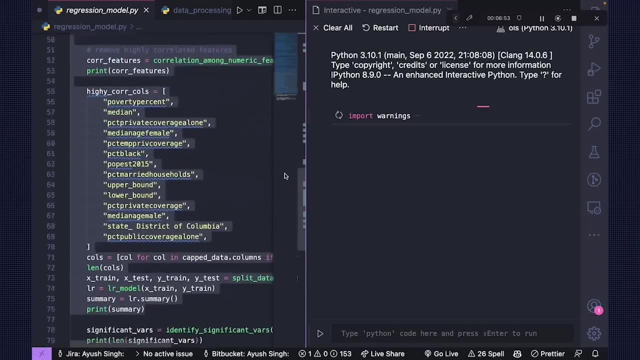 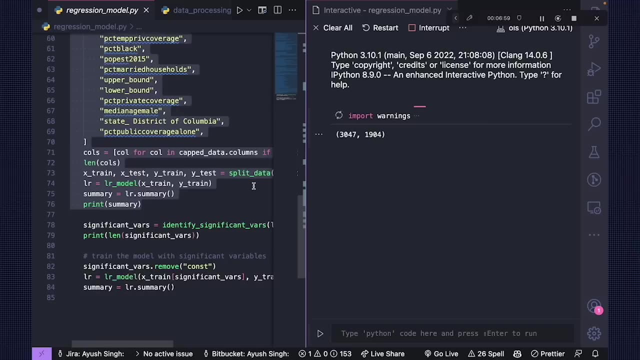 So just to make sure that you're on the right page. So it will take some time to run. we'll just chill. we'll just chill out right now. So it will take some time to run And so we should just stay calm, stay nice to whatever is going to happen right now. 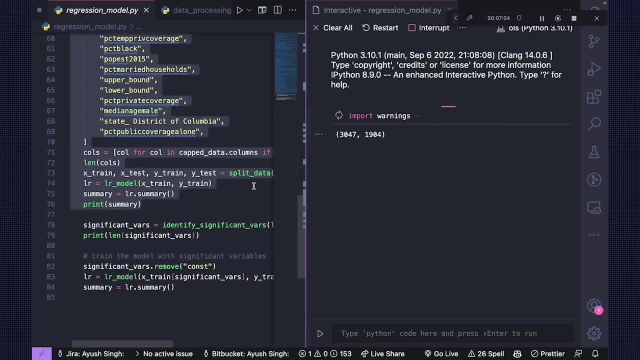 because it will, because the columns are super high And you and you, and first of all, it might be not as much valuable to deal with that categorical but to have those categorical columns. So the correlation between categorical columns. I'll be giving you a very nice article, which 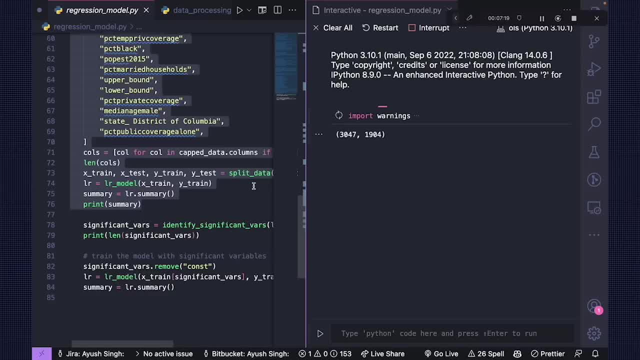 talks about correlation between categorical columns, which tells you whether that with the like, and and and. we'll also worry about key. what are the variables? So let's take a look at that. So let's take a look at that. What are the variables which are significant enough to make our model better? like we cannot? 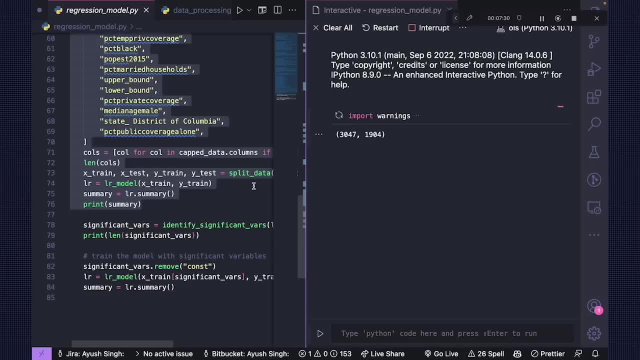 go with these much variables, to be honest, because it will lead to several other problems as well. So, first of all, let's, let's, let's go with this now. you know, if you see over here, it printed out the columns, which is of highly correlated. 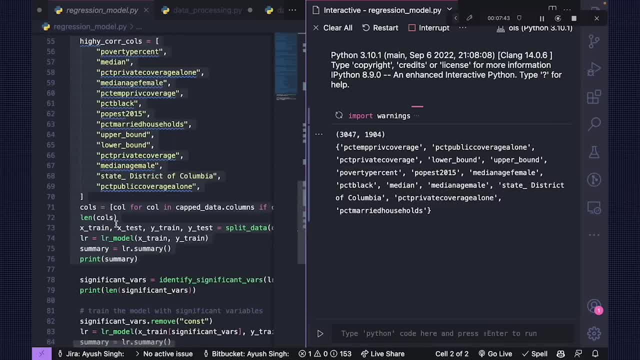 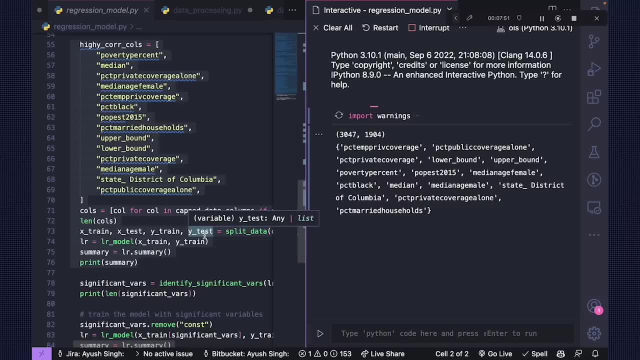 So if you see out here that we print out the highly correlated features, and then now it goes and training of the models, it is training of the linear regression model And it will take extreme vitrine this training out and then it is going to print out the 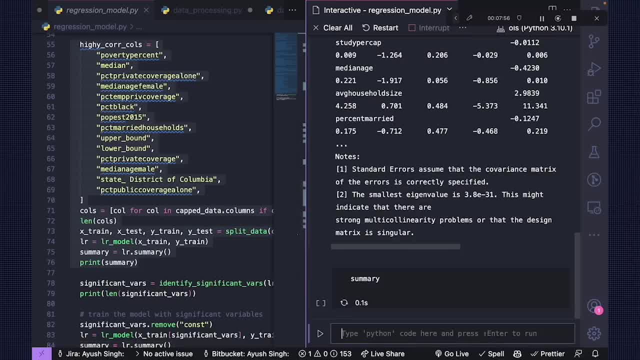 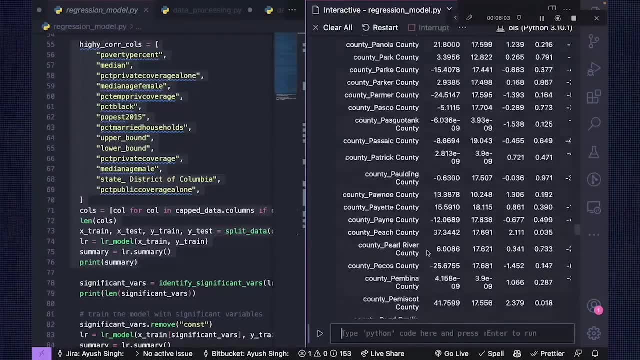 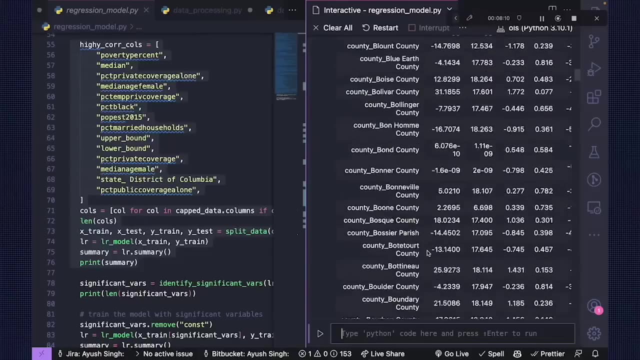 summary. So let's try to take out what exactly summary looks like. Oops, yeah, this is the summary And the summary is too big because you have 1900 columns, bro. you understand your 1900 columns And, to be honest, will end and end the most of the night alone. around 99% are of are. 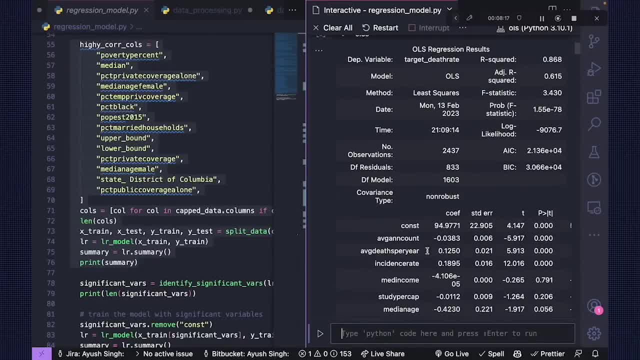 of encoded columns. That's why. that's why, in this case, we, but that's why we, in this case you, have to remove some of them. So, for first of all, see that we have dependent variable, the thing in which you're not going. 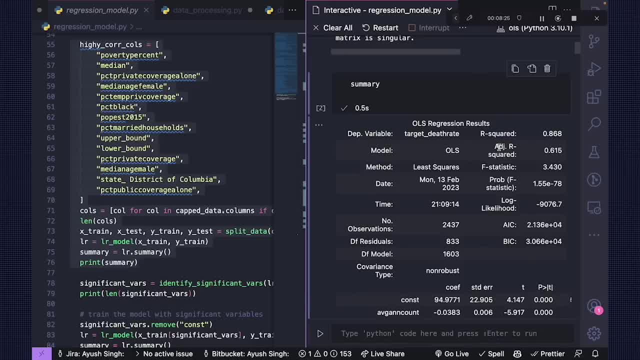 to be able to do that. So let's try to take out what exactly summary looks like. So what we're going to do is we're going to predict our square adjusted, our square F statistic. you know number of observations and residuals. you have model covariance type. 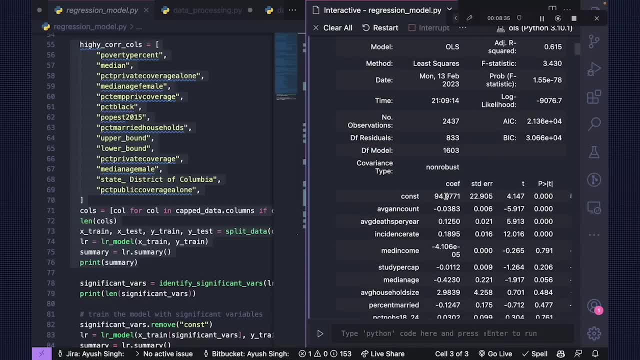 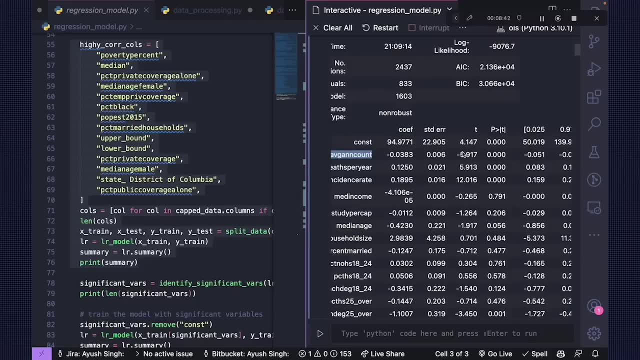 And then for constant, which is the bias term, we have the B, beta zero is 94, the standard deviation, the T and the P value for that average and for every variable. you have this, this much information left. if for every variable you have this much information left and there 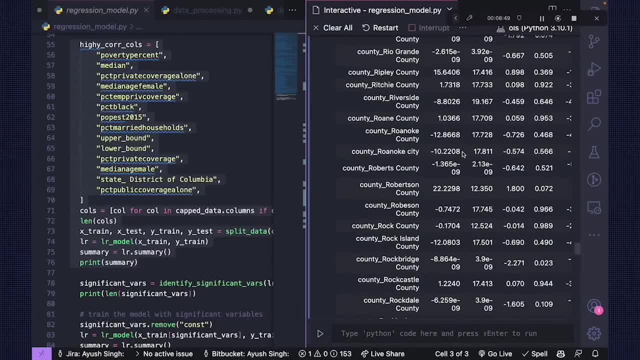 is so much of information and it is not feasible to go to every information. So what I do, I just go through what are the features which are numeric, which are important, which I don't want to go through now. Okay, so what I do is I go through the variables. 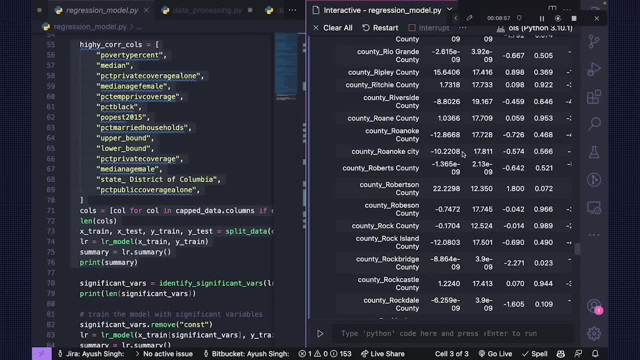 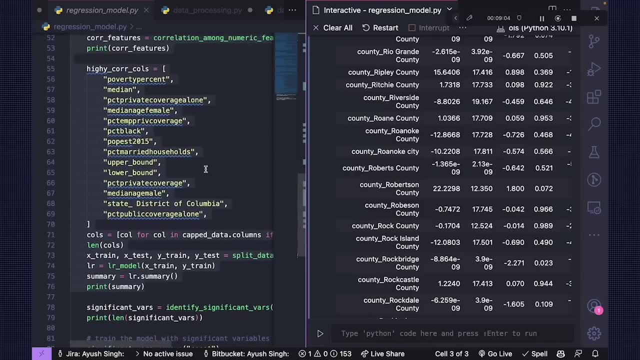 which are not categorical as of now. so what i'm doing, i just could gone through- you can go through- numeric and then talk or talk about some things, but before that, what i can do is talk about things, which is, you know, we can take all the significant variables. we have learned about that. so let's, let's. 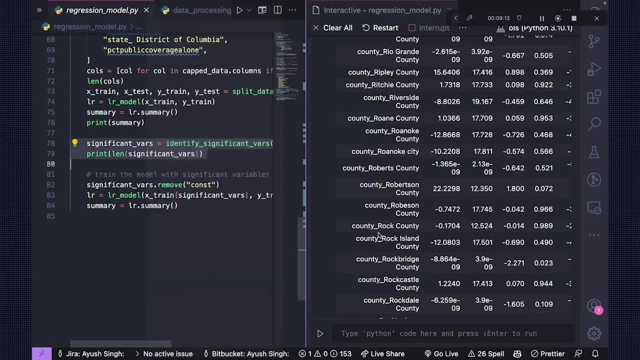 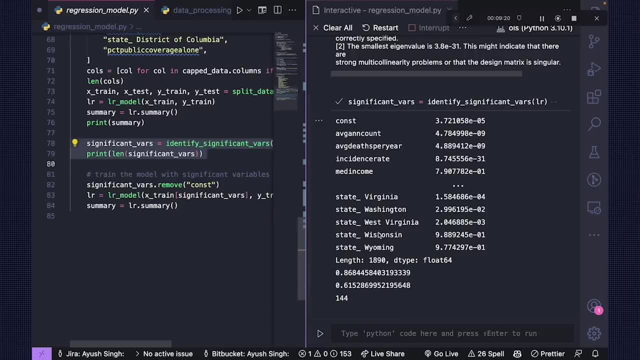 do one thing. well, let's print out the significance variable. so let's print out the variables which are only significant enough. so from 1900 we got to 144 columns, which are significant enough. we have done a lot of tests. we're using p values. you can take out the significance in significance of 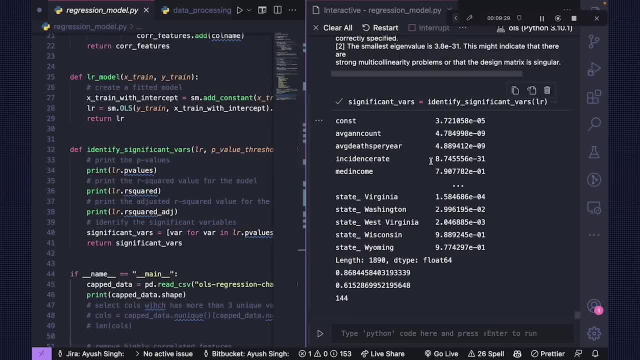 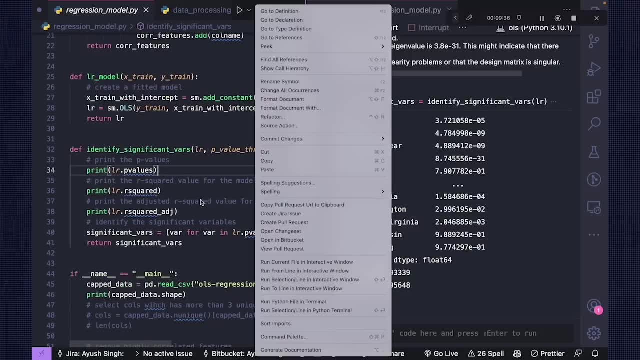 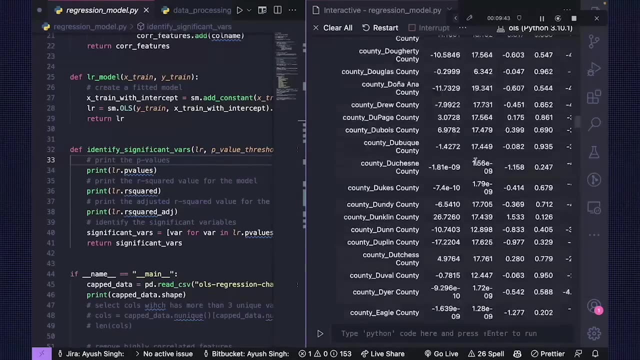 a particular variable. so we, using t, t statistic, using t statistic, we are taking on the significance of each and every variable over here. so we have, we are using lrp values and that p value is this: is this: is this particular thing. t is greater than this particular information. 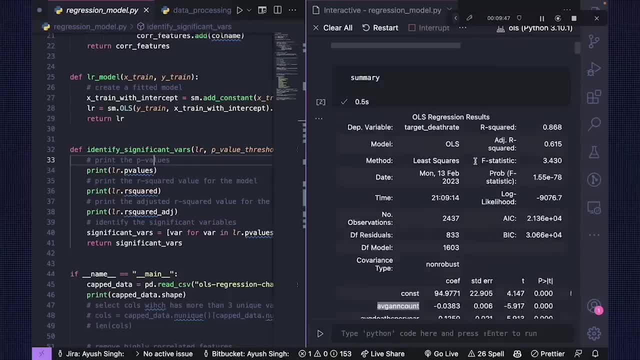 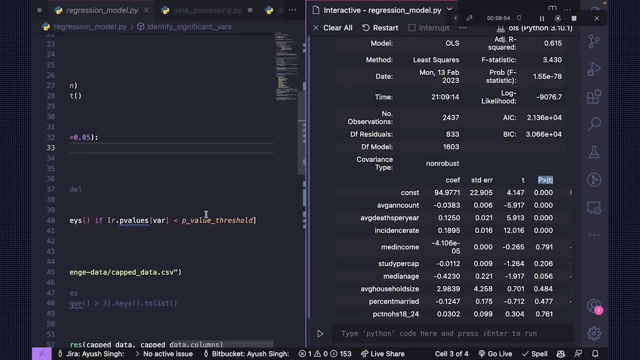 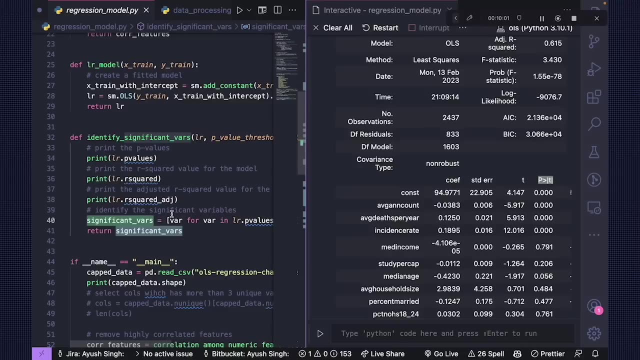 uh, the statistic, we are t test, which which we are using right now, this particular thing which you're seeing right now, p is greater than this particular information, greater than that. so we are using for that, if p value is smaller than p value threshold and threshold is 0.05. okay, i hope that you're getting me that we are taking on the only columns which 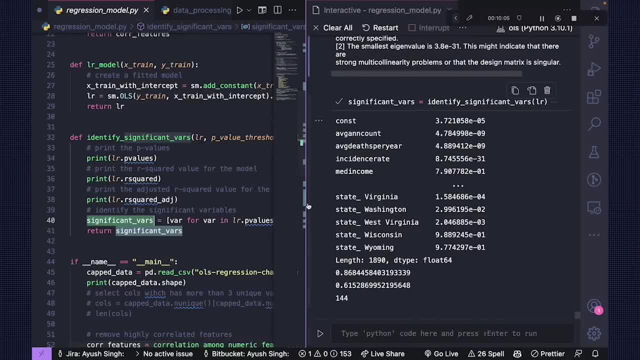 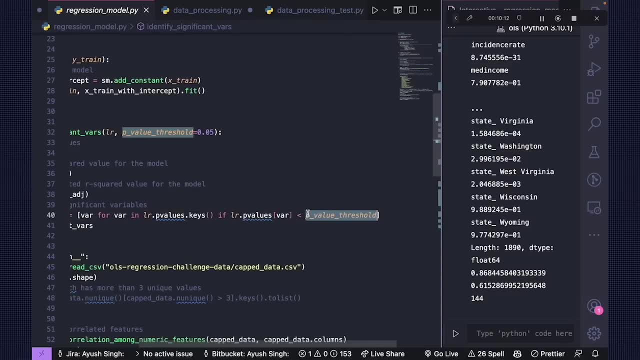 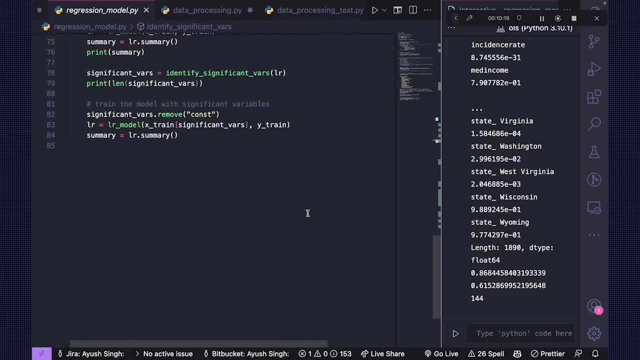 are, which are, which are, which, which are greater than that, so that, uh, sorry, i think, uh, so the the values which are smaller than 0.05, so that we can reject our null hypothesis and say that, okay, these, these variables are important. so we have only 144, 1900 to 144. it reduced the complexity of the model. 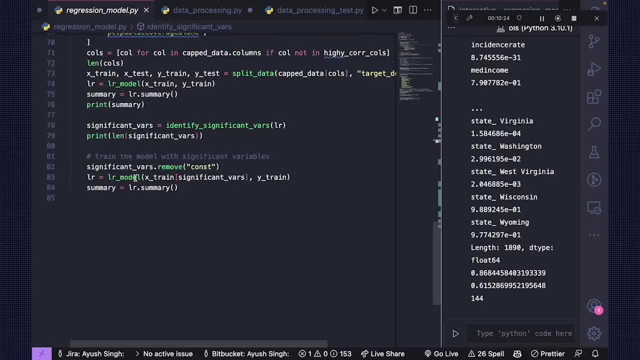 understanding what i'm trying to say now. what you're doing, you're simply training the model, now with significant variables, though the reason why we are removing this, i'll tell you the reason why we are removing this, but first of all, uh, you will get to know. first of all, let's run this, you'll get. 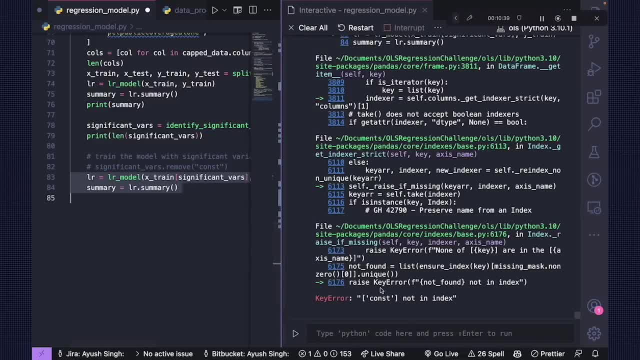 to know you got an error. you got an error, what you got an error in that significant variables. you also have the constant column, or constant means constant, which which has one right. so, whatever what i'm going to do, i'm just going to remove it as of now. 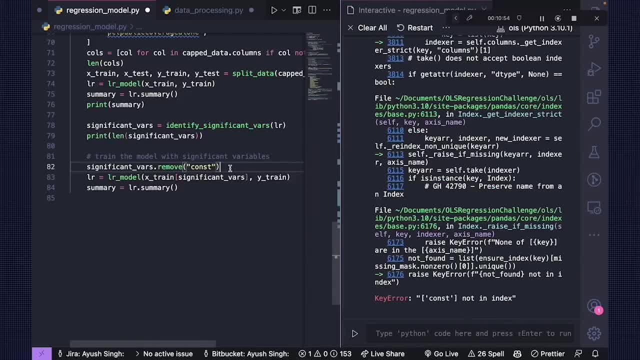 there is actually a lot of fixes right now, but i don't want to uh extend that. you can fix it by your own. so what you can eventually do, you can create, uh, you can create actually x in x train as well. you can create a constant column as well, so that it appears that. so you can actually what? 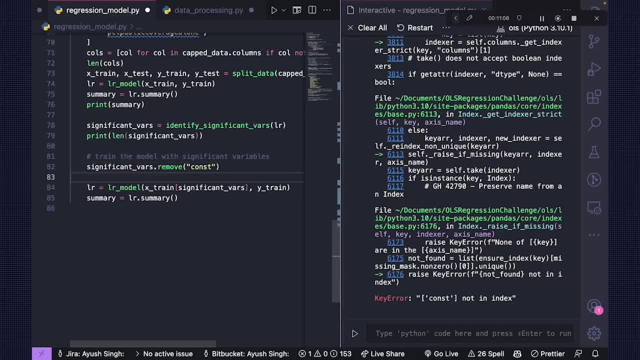 you what you can do. let me do one thing right now. i think that's something which which we, which we can eventually do, uh x train and then just go ahead and then add x train and then constant. i guess what we can eventually do in this, because you can uh. 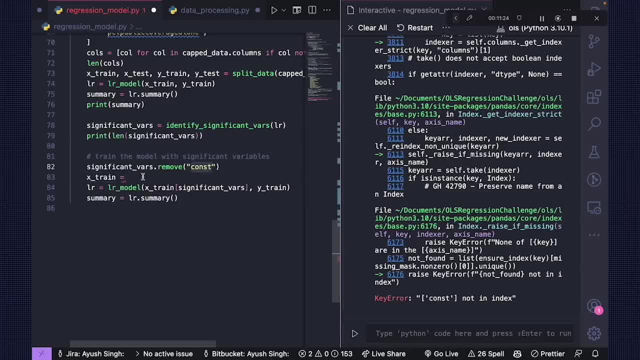 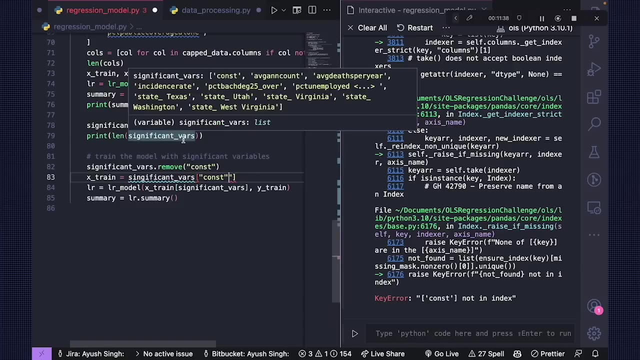 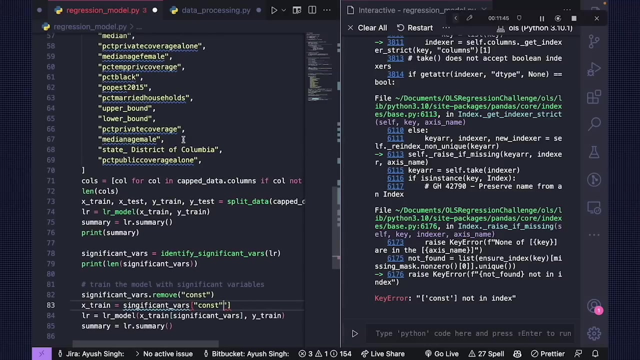 um, add the significant, you know, constant- columns, rather than removing that. so i think, which you can go and then add significant verse and then significant verse, we can add constant. yeah, so you can actually actually do this, but how, however, that significant, actual uh actually should be having your favorite, you know what your that should be having um constant columns, or you can. 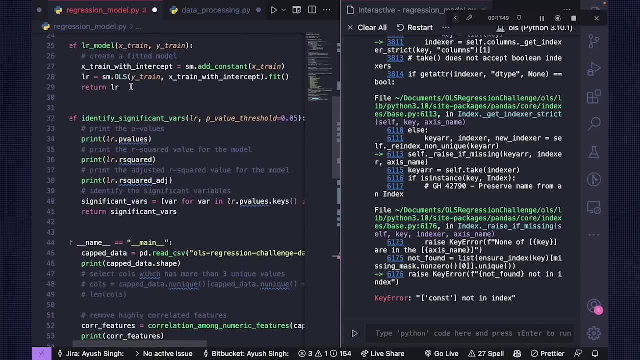 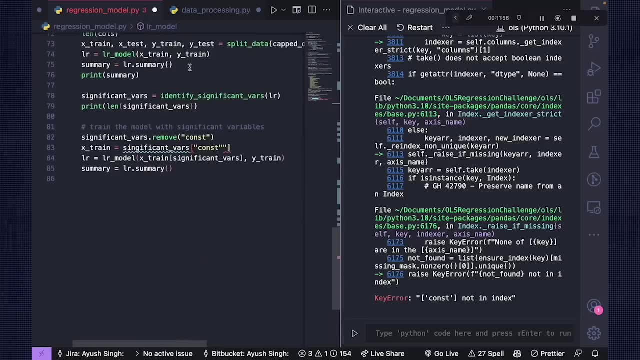 what you can do. you can simply have this sm dot, you know s smadd constant, and then you can simply add that constant as well over there, right? so it is very easy to do, do things. you can actually go to uh, extreme dot, add constant, and then you to the the constant. 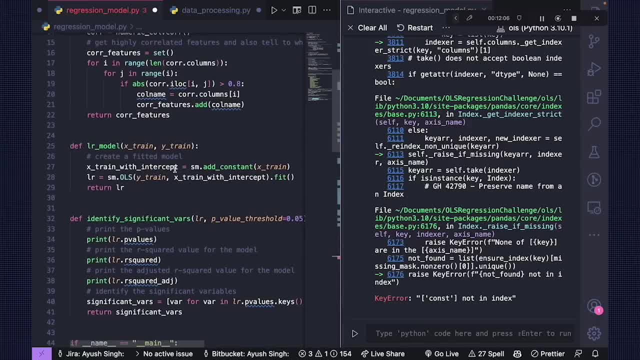 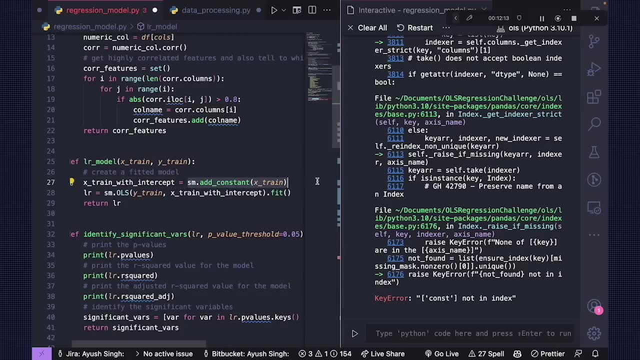 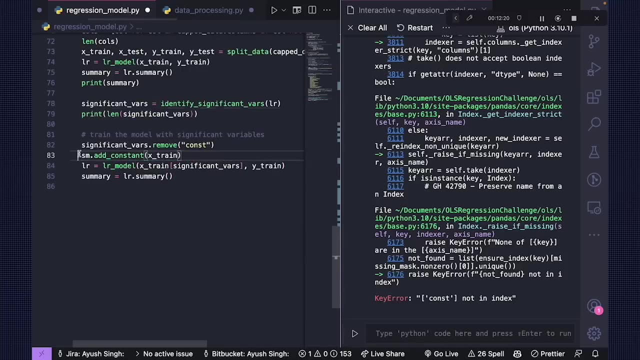 will be also added right. so you can actually go over there and then simply add sm dot, add constant right. sm dot, add cons, because in extremely it it is not added right. so we we can actually go ahead and then add the constant audios as smact, that constant, and then 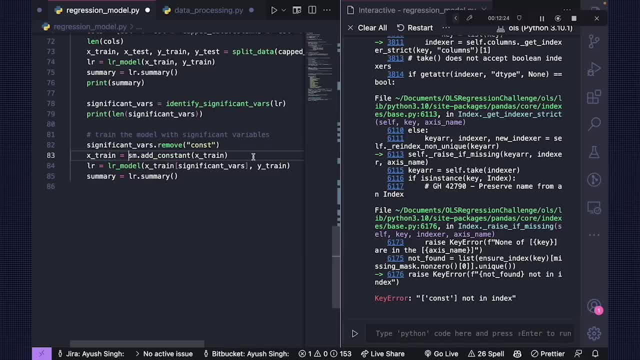 we simply have this x string, so it adds the constant you can actually use for loops and all to also add it. but this is the best way to actually do: do that rather than removing that. so, actually, rather removing that, you can actually add this and then, once you add this, so let's run. 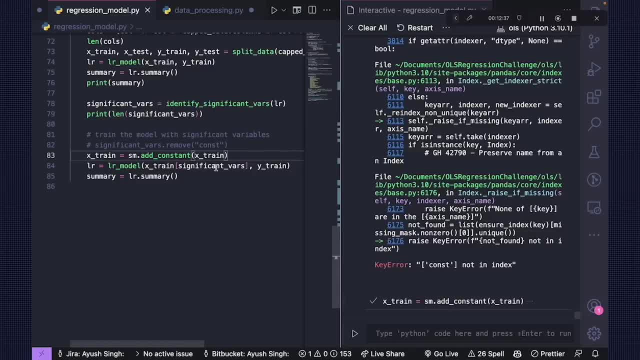 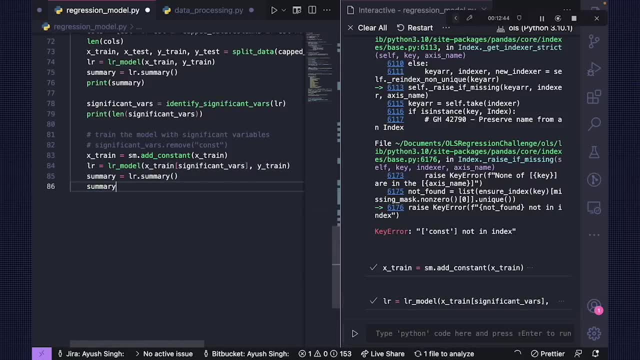 this, so you might be having a nice set of information. so now it it. it is completed. now you run this. now you run this, you should be able to see a very nice set of info. so now let's go and let's print out the summary which you can see. so now, if you run this, now, if you run this, you have. 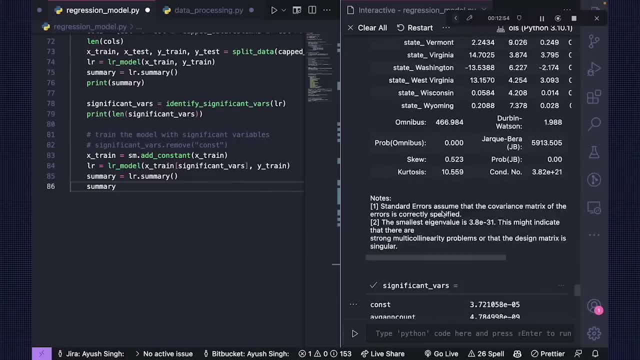 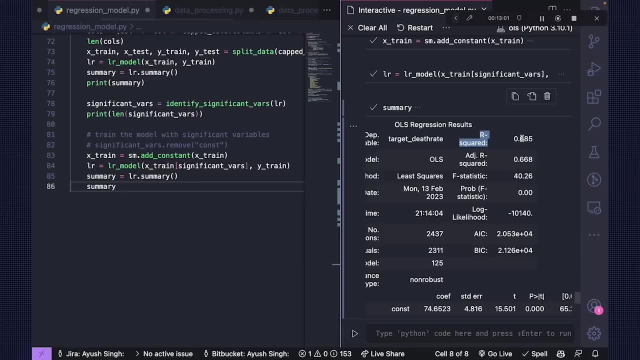 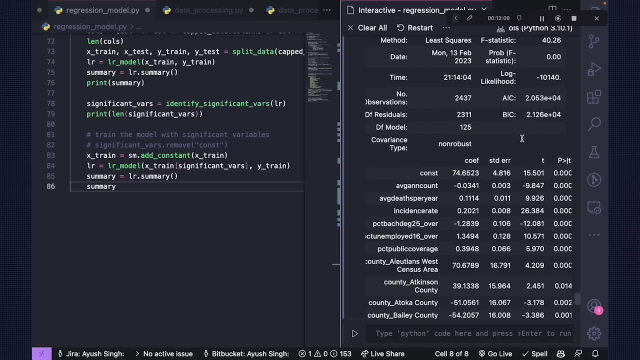 the previous one. you have just only few set of information to go forward to. so, yeah, this is the one. and then you can also see the. the r square is 0.68. however it is, it is decreased, but it is a it. it is a model which we looked for, right, or however. it reduced the complexity of our model. 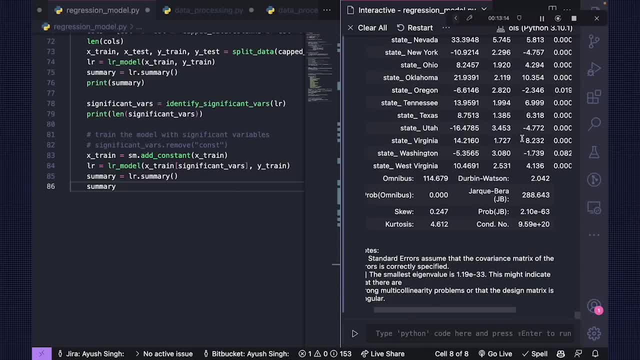 right, our complexity of our model. the more important is not to get the accuracy, but also the robust model, the model which is able to perform in most of the cases very nicely. so this was it for today's video. i hope you enjoyed this video and i hope you enjoyed this project and i hope that. 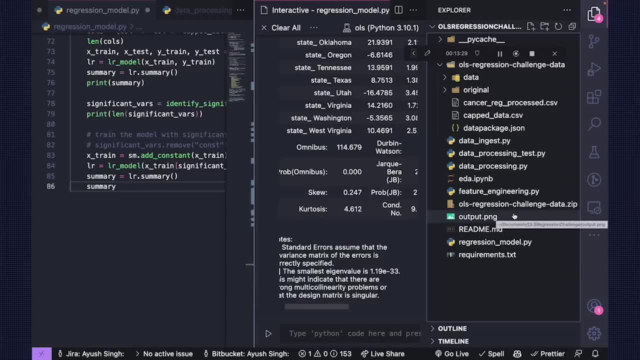 you really like this particular project and um you, now you'll be given assignments for the. for the same, for the rest of the things which you have to do in the project, uh, now you can get started with making your own projects. i have tried to explain each and everything from very scratch. 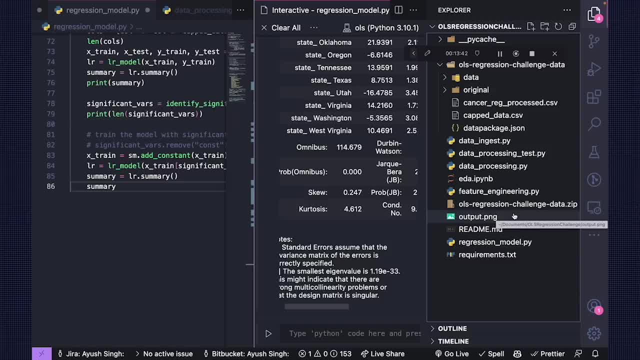 now i suggest to watch resampling methods video regularization videos, which is going to come, so please watch that and thank you for the lectures.